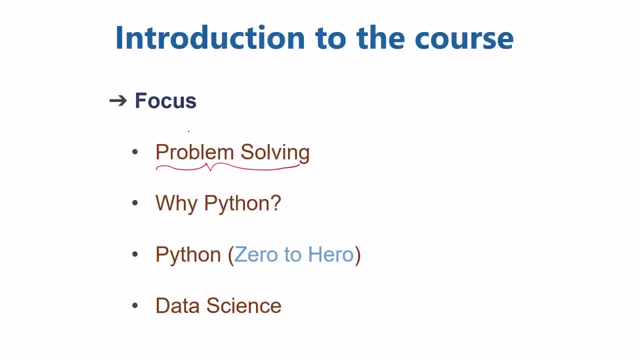 we are not assuming the course taker to have any experience whatsoever about any computer programming language before, Not even the problem solving paradigm that lies in computer science. So we will focus on problem solving for a bit and we will actually start from the very beginning what problem solving is particularly in computer science. The second: 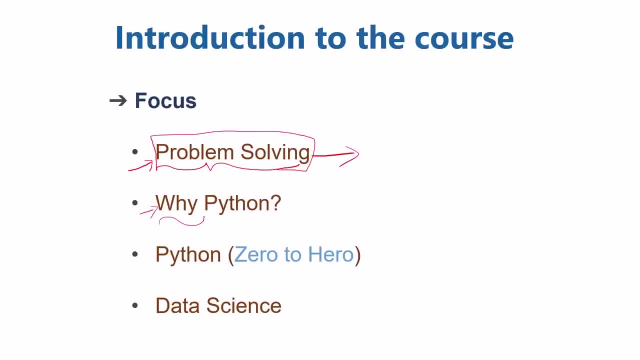 focus of this particular course is mainly telling you why we are choosing Python, Why Python is so important, particularly for data science problems. The third focus and the main core focus is to learn Python, obviously Once we know what are the techniques to solve a problem. 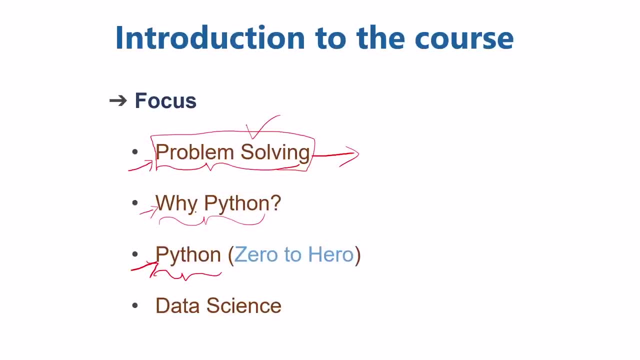 and once we know that Python might be a very good language to go with. then what is Python? How to learn it? Well, the Python is the main core and main focus of this course. Obviously, we will start from the very beginning, very, very beginning, which means we will start from: 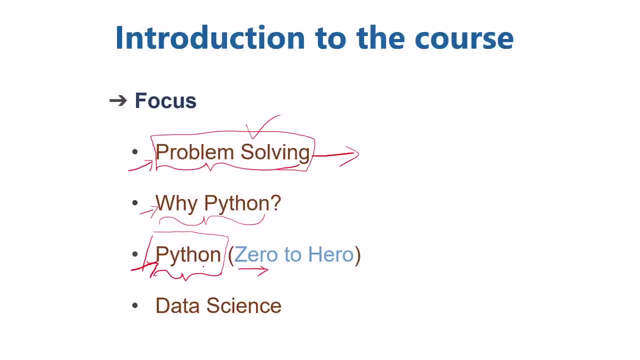 how to install Python, For example. we will start from there And then we will see what are variables. I mean very, very beginning And then, progressively, we will be moving on and on and on to data structures, to complex structures. But that transition from zero to onwards, that transition. 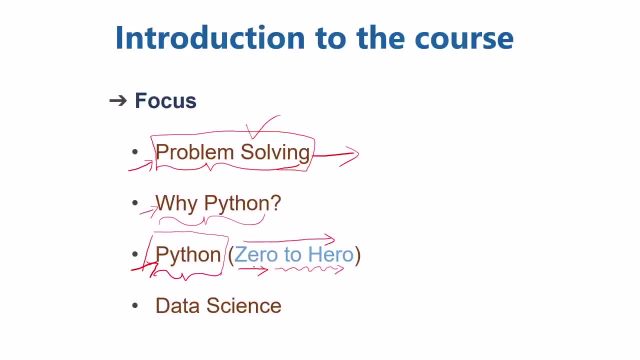 will be very, very smooth. I mean, whatever you know so far in the course you will be able to. that will be helping you to gain more complex structures very, very easily, gaining the understanding of a lot of structures very, very easily. So in this Python we will include all 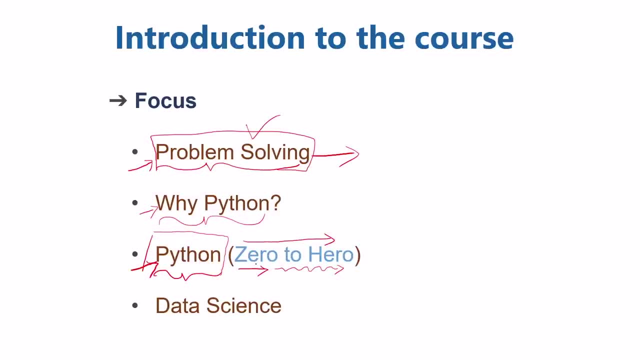 concepts of Python in general. And one more thing After. I mean learning this Python, the way we organize this course. after learning this Python, you will be having understanding of other languages as well. I mean, the contents here are explained in so general way, although with the Python syntax, but the concepts are expressed. 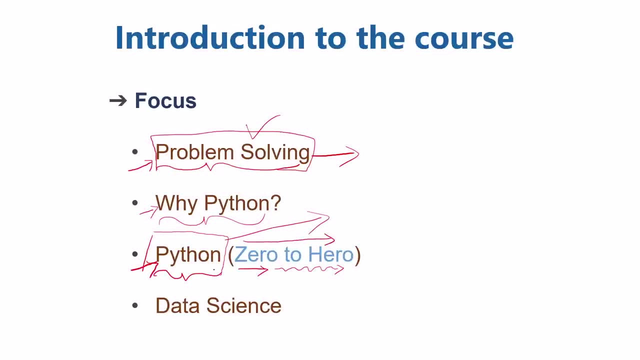 in so general way. the problems that we pick to solve for practice are so generic that you will, after this particular Python course, you will be having understanding of programming languages in general. So data science is one other focus of this course. Actually, the whole course is. 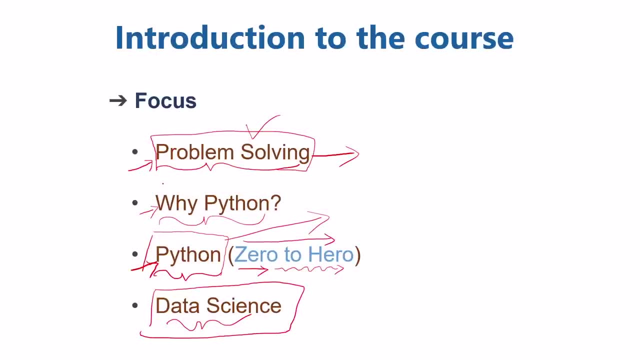 organized in a way that it teaches you about Python, it teaches you problem solving, it teaches you something about overall programming languages and how computer can be used to achieve the solution of different problems, and using Python, of course. And then we will be introducing the data science packages. 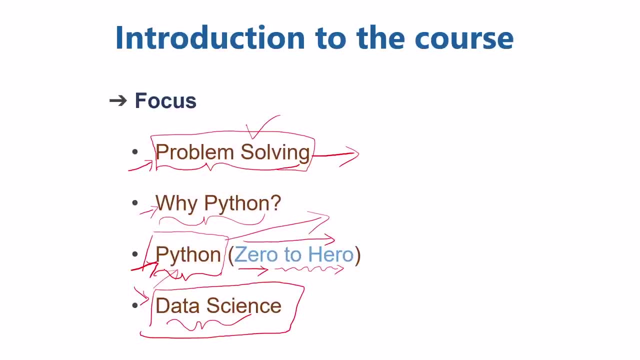 that are available in Python, because they are really really fast, really fundamental, very easy to use and very, very powerful to handle a large amount of data very, very quickly for data understanding, for visualization, for cleaning, processing. 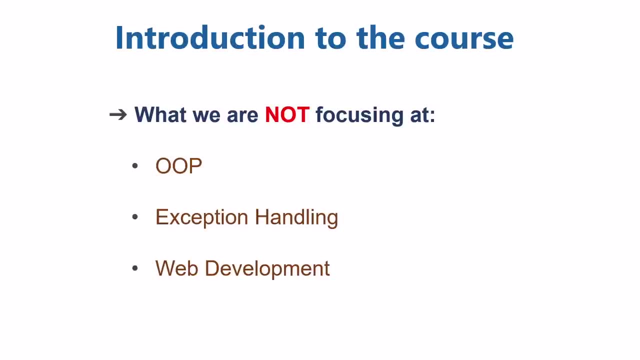 and a lot of stuff, What we are not focusing at, because that's important knowing that. what kind of things are the things that we're not covering? For example, we are not covering OOP, object-oriented programming. We are not covering exception handling. We're not doing. 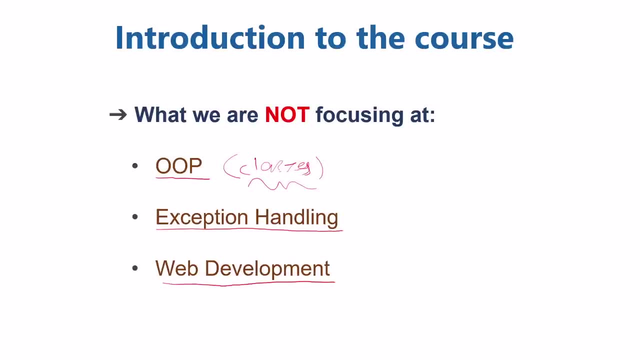 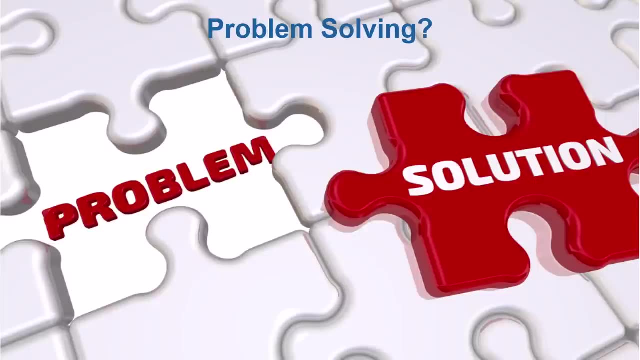 web development or any general kind of tasks that are doable in Python. We are not focusing on those things. Now, do you realize that in Python, for instance, you have these sort of things that are there as an example? You have a question, you have a problem, you end up with a problem and your problem is: 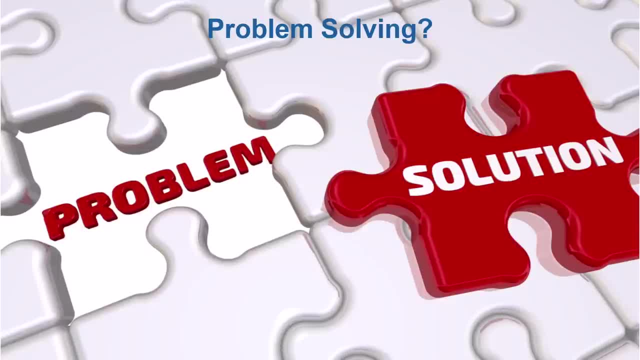 actually solved. It's not a problem that you react to, you don't react to, it's just the problem itself. And in Python, for instance, like you just said, there's a lot of problems and you have two problems. 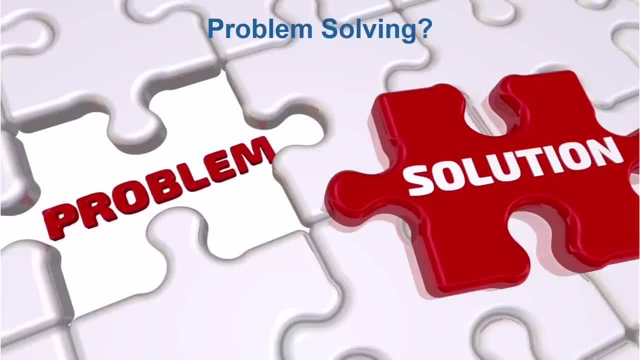 You have a problem before you go into the next level of the service and you have a problem after you go into the next level, and so on. And a problem before you go into the next level and you have a problem before you go the next. 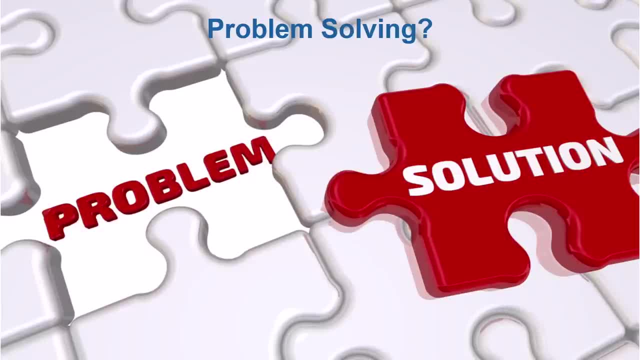 with respect to the sale value, and we have to do it after every eight hours. If the number of instances, if that number is huge, the optimal choice is to automate the solution, if the automation is possible. But how? How to come up with the automated solution? 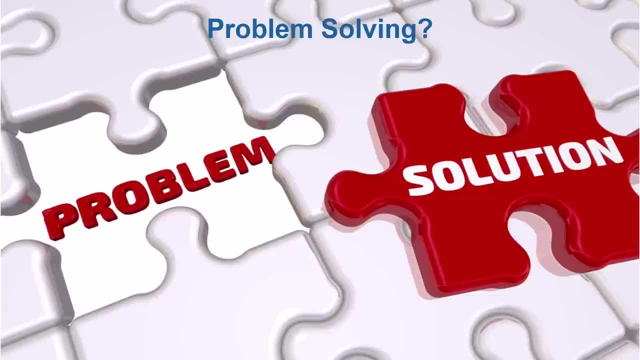 To come up with a general solution that works for every instance of some problem. that is one thing, But to get that solution running on a computer is yet another thing. Problem solving deals with formalizing a general solution that works for every instance And programming languages like Python. 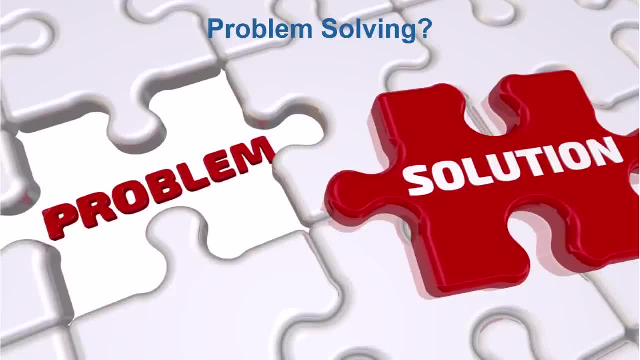 deals with the running of that solution on a computer. Python, as we will see, makes the transition from problem solving to the running solution much easier and quicker, And that's one big plus of Python. A lot of words, I know a lot of words. 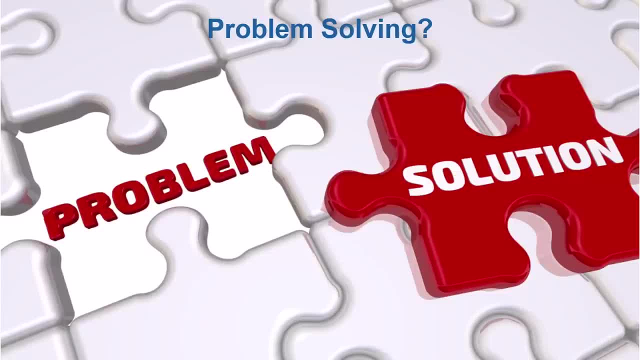 Let me take an example to clarify what I said. Hold on till the end of this video and I will make everything, what I said so far, crystal clear. So let's take an example, Let's dive into it. Let's take an example to see what I just said. 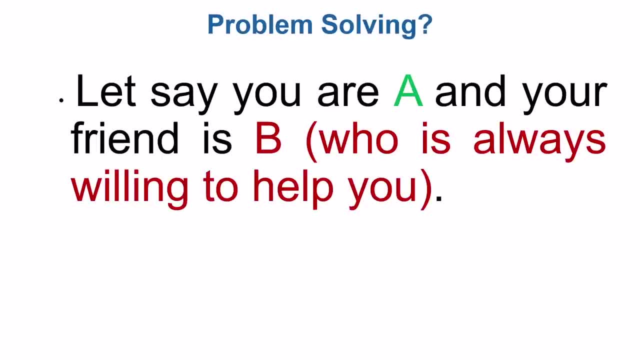 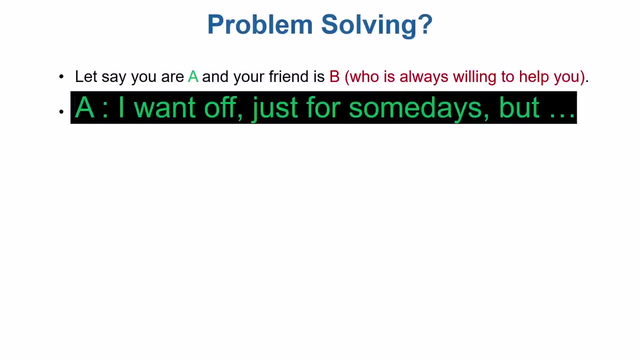 Let's say you are A and your friend is B And your friend B is always willing to help you. Let's say you found such a friend And then A just said I want off just for some days. But B said: but what? 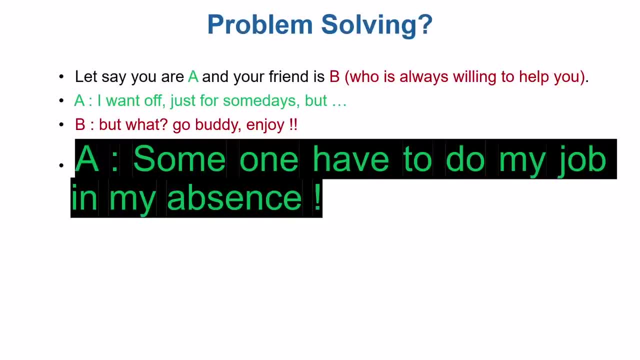 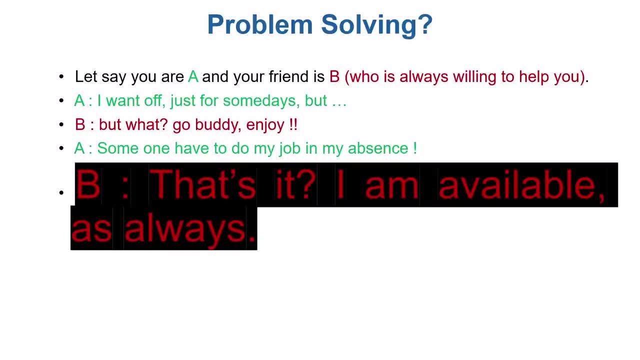 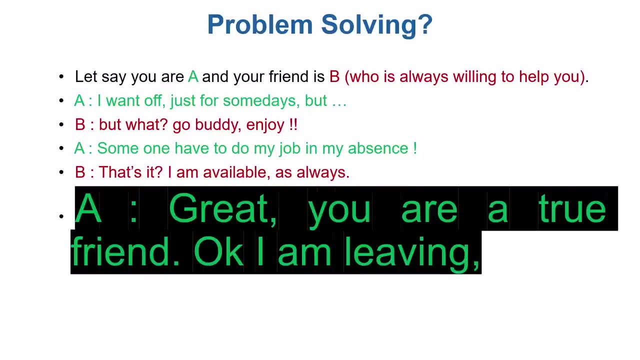 Go buddy, enjoy, Enjoy. A said: someone have to do my job in my absence. And then B said: that's it. Is that your problem? I'm available as always. Go buddy, enjoy. Then A said: great. 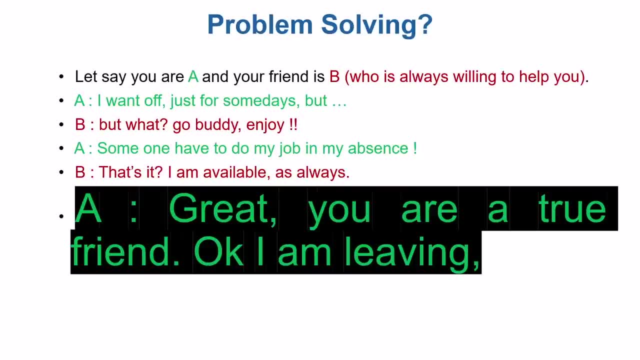 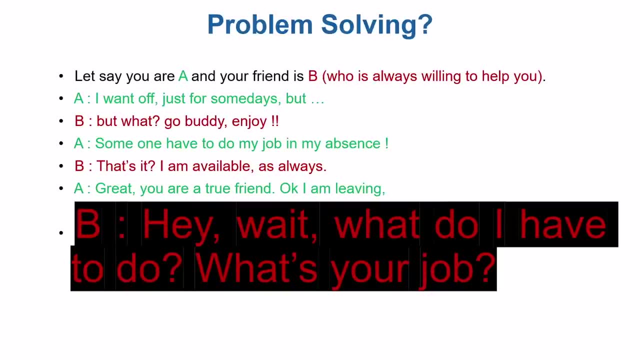 You are a true friend. Okay, I'm leaving. Wow, And B just said: hey, wait, what do I have to do? What's your job? At the end of the day, I'm going to do your job. What's your job? 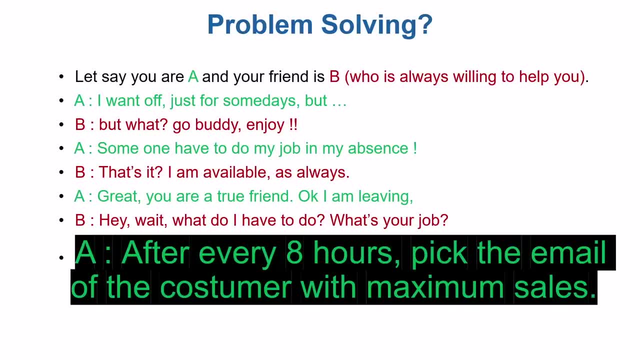 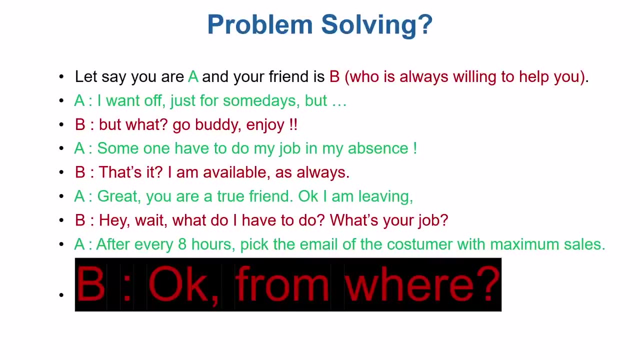 What do you do? And then A said: after every eight hours, pick the email of the customer with the maximum sales. So that's what you have to do. B said: okay, but from where? I mean, I have to pick that email of the customer from where? 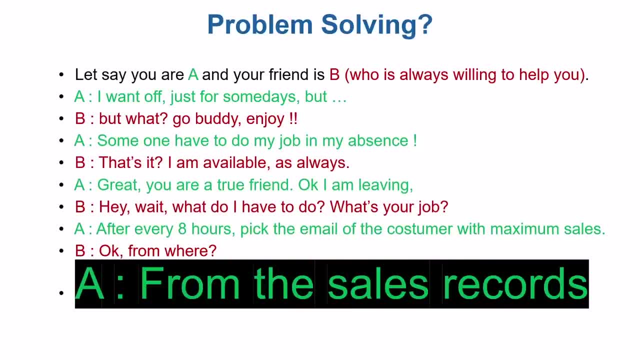 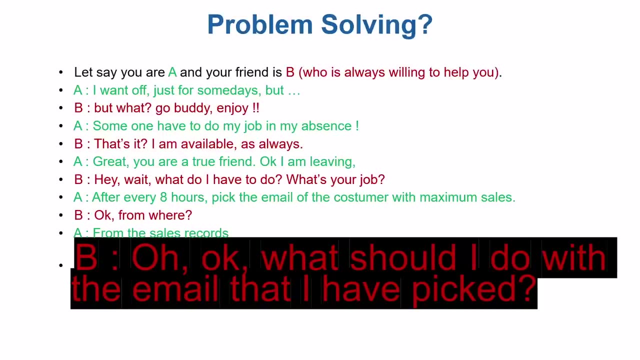 Where are the records? He said: well, there are sales records. I mean, at the job place there are sales records And you have to pick the email of the customer with maximum Sales. B said, oh, okay, but wait, what should I do with the email that I just picked? 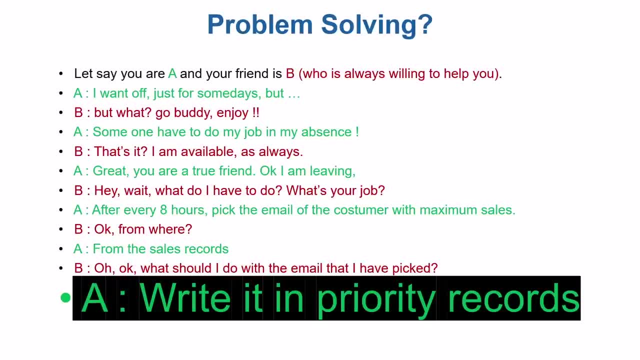 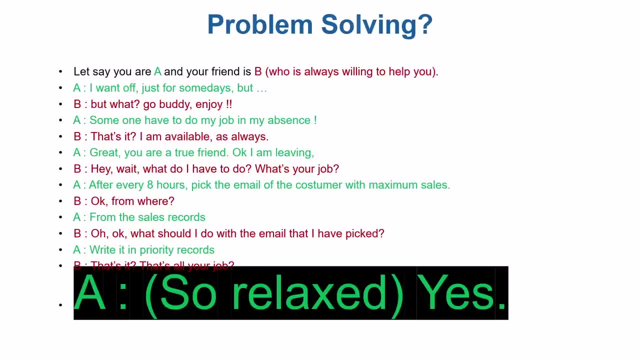 Then A said: oh, there is an other record called Priority Records. Just write that email after eight hours. Just write that email in Priority Records. And then B said that's it, That's all your job. And A said after so relaxed, A said yes, that's my job. 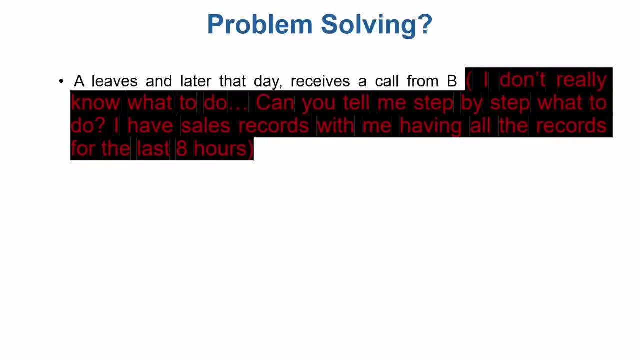 That's all Now. think A leaves and later that day receives a call from B And B said I don't really know what to do. Can you tell me, step by step, what to do? Focus on again. I'm reading this particular sentence again: 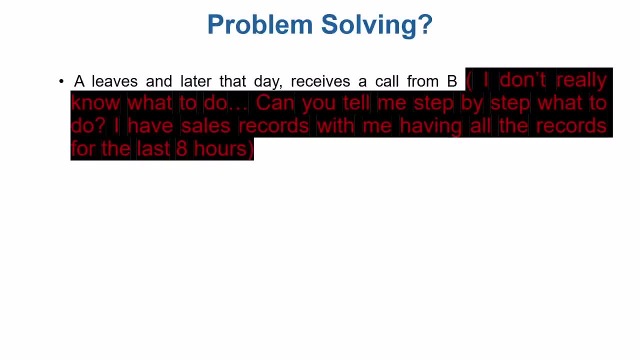 Can you tell me, step by step, what to do? I have sales records with me, having all the records for the last eight hours. What to do? I just messed everything up. I don't know what to do. And then at the call, A just described a procedure to B for his job. 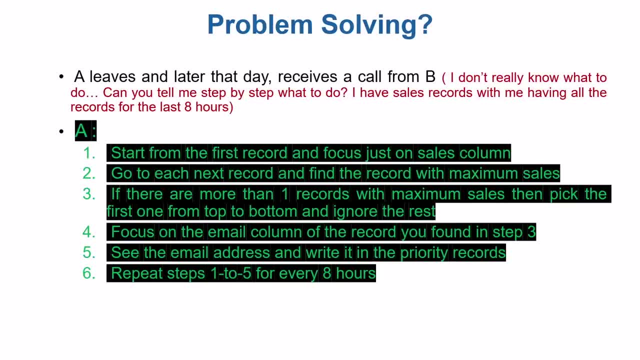 That procedure or a general solution. Let's see the solution. A said number one. start from the first record. There may be several columns of the record: the customer name, the customer phone number, the customer email, the customer products that he buy it and the total sales. 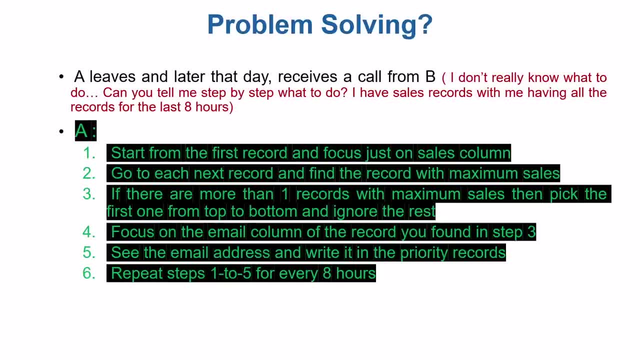 And the point one said A said: start from the first record and focus just on the sales column. Okay, then after that go to each next record one by one, and find the record with the maximum sales, Obviously, once you have. 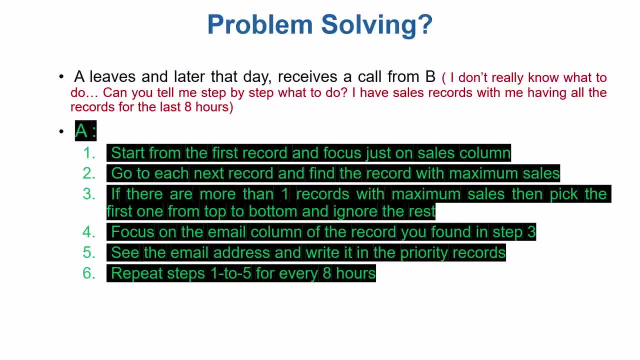 focused on the sales column. you're just comparing sales of different records with each other and will eventually come up with a record that have maximum sales. Number three: If there are more than one records with maximum sales, it is possible that the maximum sale value, let's say, is hundred, whatever the units are. 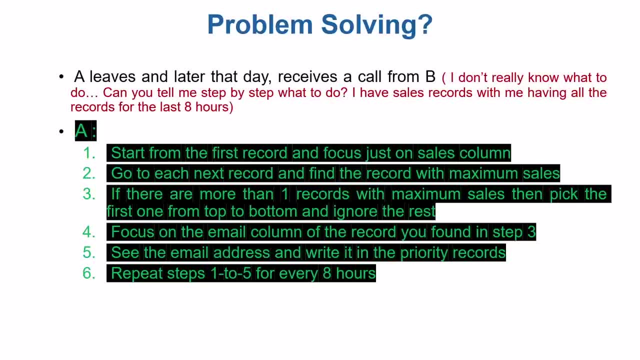 And there may be two or three or maybe five records with the maximum sales hundred, Then which one to pick? A just described here Instead step three, that if there are more than one records with maximum sales, then pick the first one from top to bottom and ignore the rest. 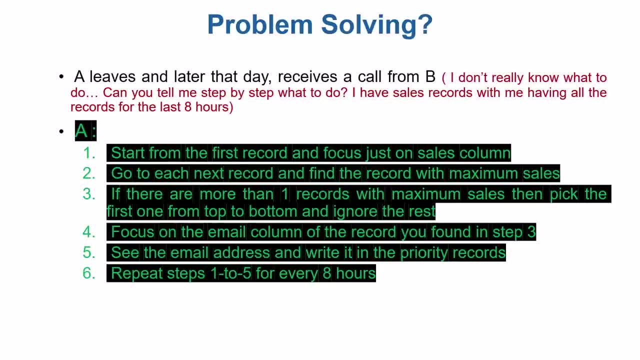 I mean whichever is the so? So let's say you have five records with maximum sale value. Which record appears first from top to down? Just pick that one and ignore the rest. That might be a policy, that might be a tie-breaking policy, but 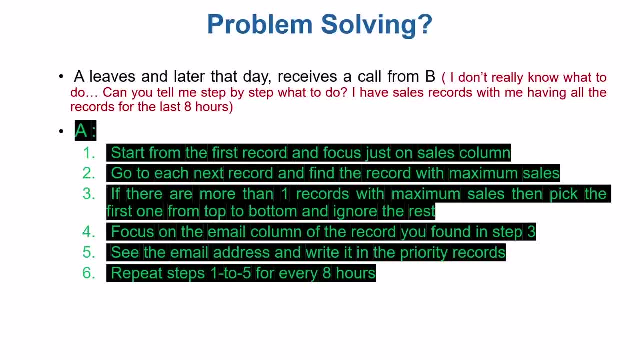 just do that. And then the fourth step is focus on the email column of the record you found in step three. In step three you found a column with maximum sales. Step five: see the email address and write that address in the priority records. 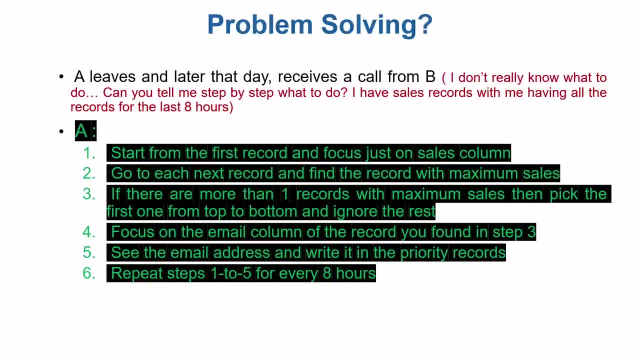 So that's for the eight hours. Then repeat this, see the step six. then repeat this procedure after every eight hours. I mean repeat this procedure. I mean you see the. the solution A is communicating to B in in this. 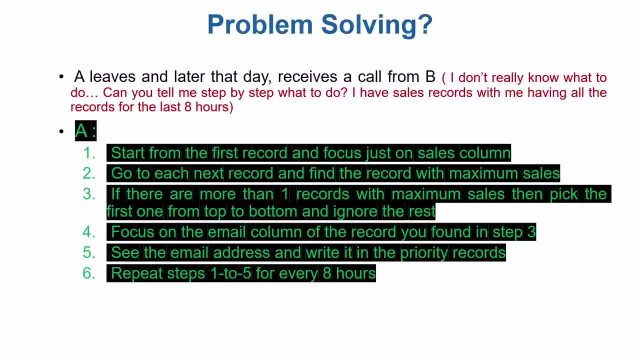 in these kind of steps. It it gives. it gives a precise idea of what to do. Still, there may be some, there may be some questions that B is maybe asking. For example, B may ask how to find out a maximum. 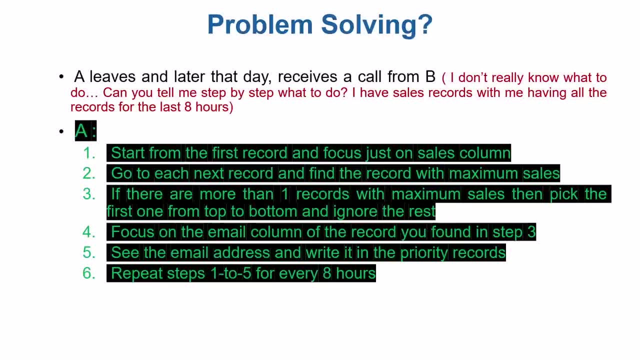 B might be that person who don't know how to find out the maximum. And third, for example, another question B might may ask: is that when, when I'm going to write the email address in the priority records, where should I write? 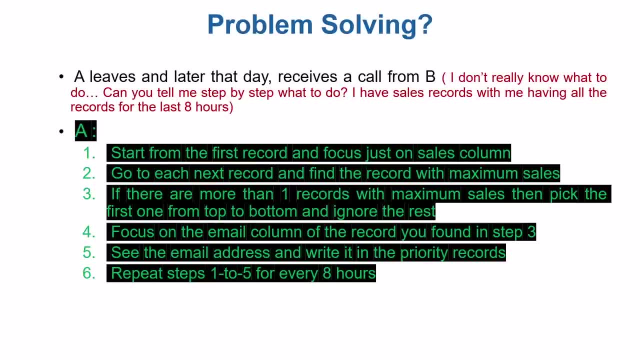 At the very top, or at the end, or, or somewhere or. but at the end of the day, a solution, a step by step solution, is required for communication This kind. if you see the solution, although it has some, it may be explained in. 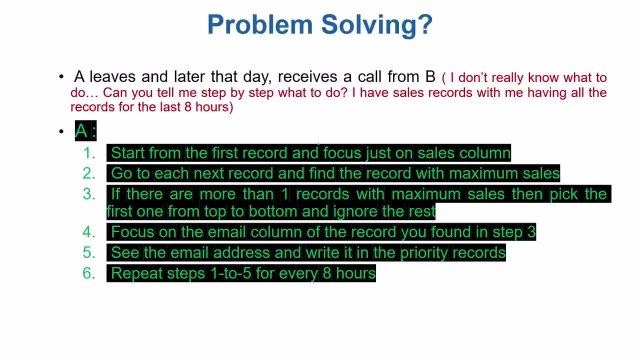 there may be more steps that should be added, But if you see the solution, this step by step solution, this is general solution. This is general solution, much more general solution for every instance. By every instance, I mean after every eight hours. 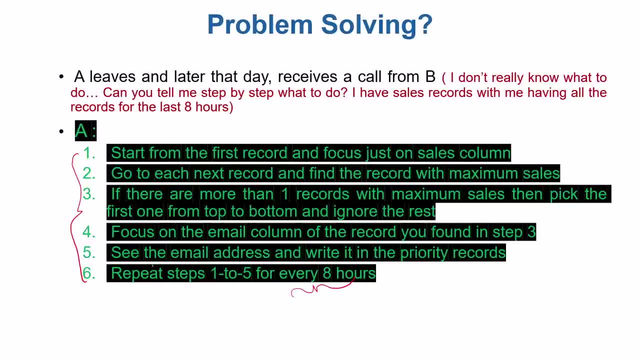 you'll be having some records and you have to do this procedure on the records for that eight hours And then after that, that, after that eight hours- you will be having more records to work on. So after every eight hours you have the same. 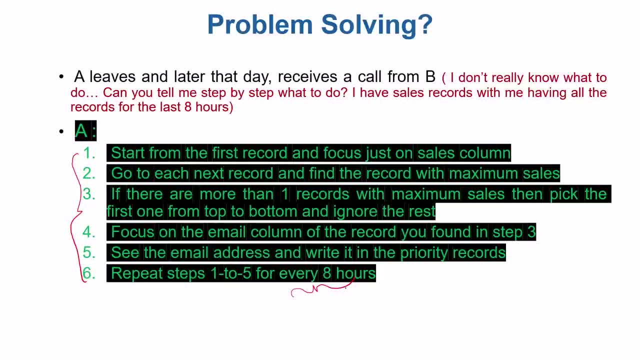 the problem is the same, but the instance is different because the records after eight hours are different. But, but the but. the solution says: whatever the instance you are right right now, whatever the instance is that you're in, just perform these. 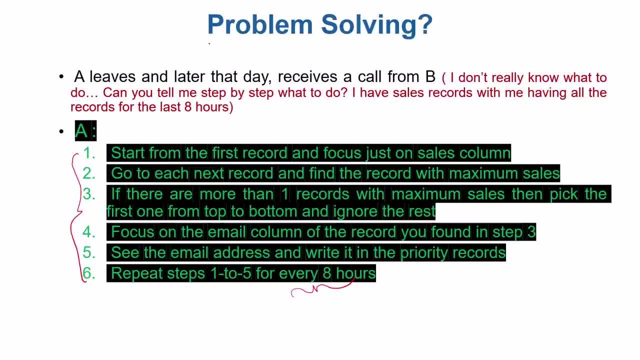 these steps A step by step solution. coming up with a step by step solution is is one module of the one module of the problem solving, And this step by step solution is called algorithm, Algorithm. obviously, this step by step solution is not always required to be communicated in plain English or in natural language. 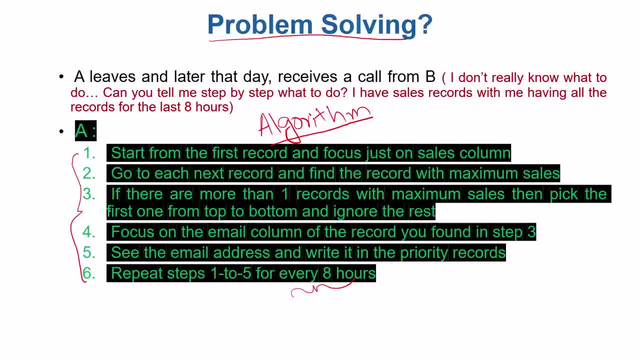 You may come up with shorthands or shortcuts to explain these step by step solution. So the the the more shortcuts, the more precise and unique meaning keywords you use in your step by step solution, the more better communication of your solution takes place. 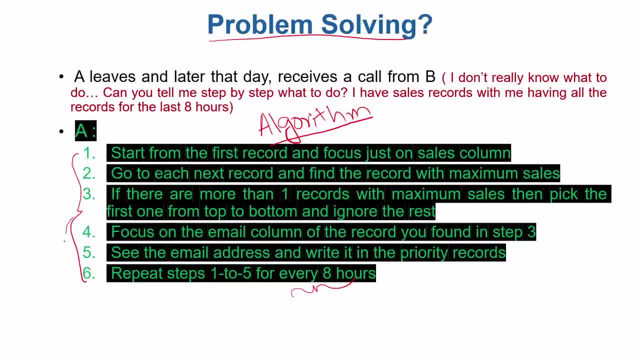 And going from this step by step solution, which is, just in plain English, going from this to a more concise and unique kind of procedure, That that, that kind of one, that one step that will take us from there to there that we will see in the next video, will be called a pseudo code. 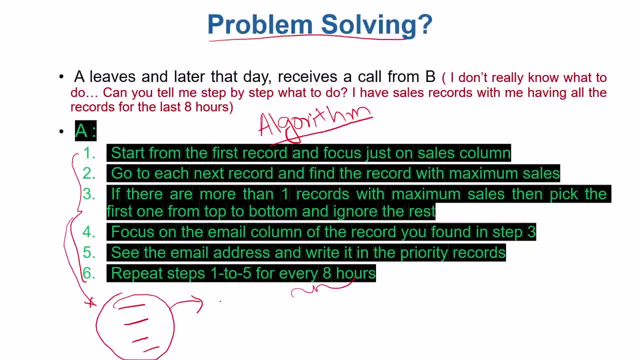 And from that pseudo code there will be a few steps that will take us to the second major problem that the problem languages will solve: to get the solution running on a computer. So just just in this video I I wanted to explain you that solving a problem may not be that hard. 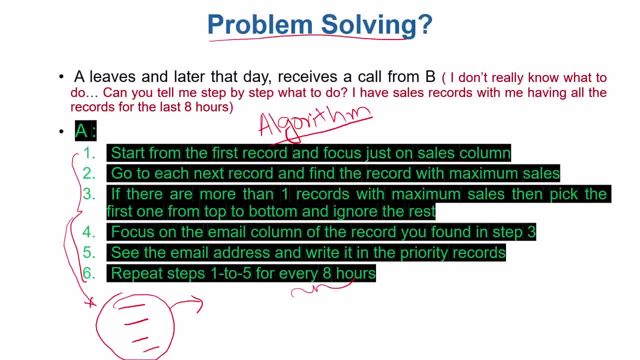 I mean coming up with a coming with. coming up with a solution of a problem may not be that hard, but communicating that solution or or writing that solution in a form of procedure that can solve every instance of that problem, that 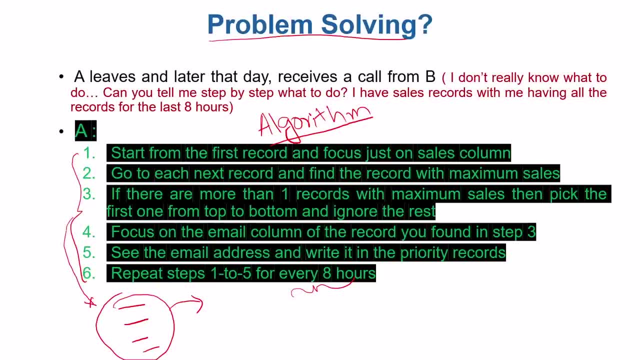 that requires a step by step treatment of the procedure And those those steps. they should be linked in a sequence and they should be unambiguous, And if a particular step requires more elaboration, that step might be broken down to further steps. 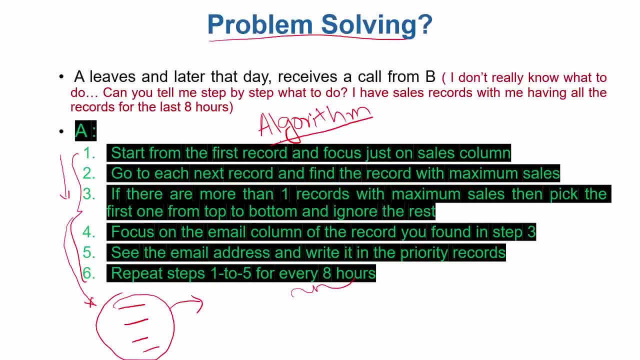 But that step by step solution, at the end of the day, is called algorithm. Now that algorithm might be in English, but we will see in the later video that there are better ways of expressing algorithms, better than English or better than natural languages. So 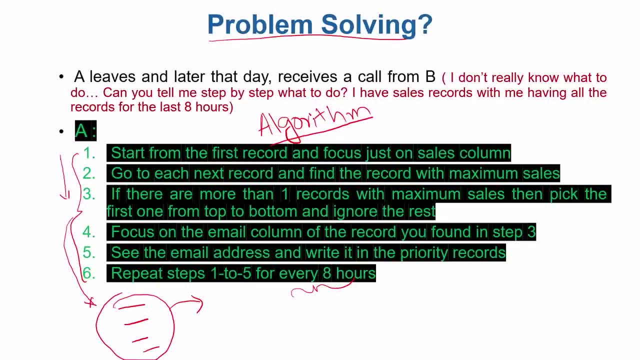 so, if you have another problem, come up with a step by step solution of that, though every instance of that problem should be solved by that step by step solution, which is called algorithm, And in the next video we will see how to actually. 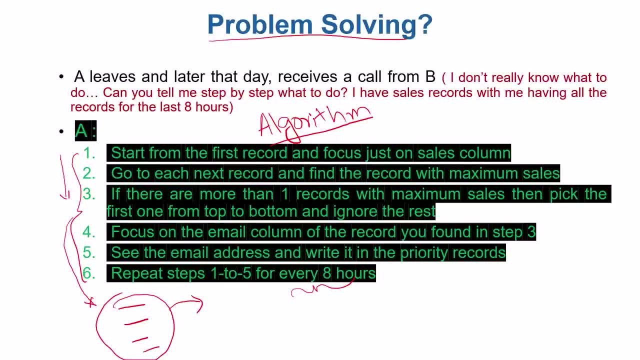 how to actually eliminate the need of having English with us and how to incorporate the uniqueness of understanding of these steps or algorithm using, using the concepts of pseudocode. And after the pseudocodes, we will see it will be very quick to to jump to any programming language and we will see that the Python is very close to what human generally think. 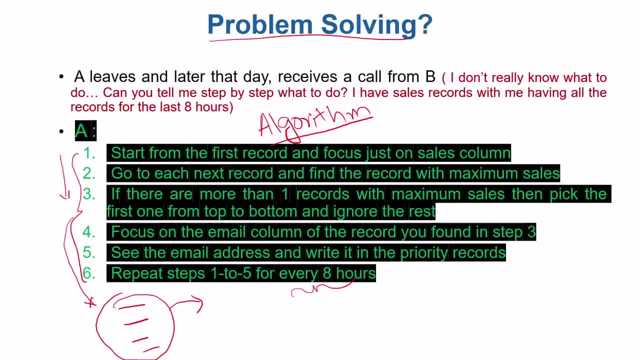 I mean it's very easy. The transition will be very, very easy. So hope to see you in the next video, And I'll be explaining algorithms in, in, in, in a more kind of keyword way, And, and in the same video. 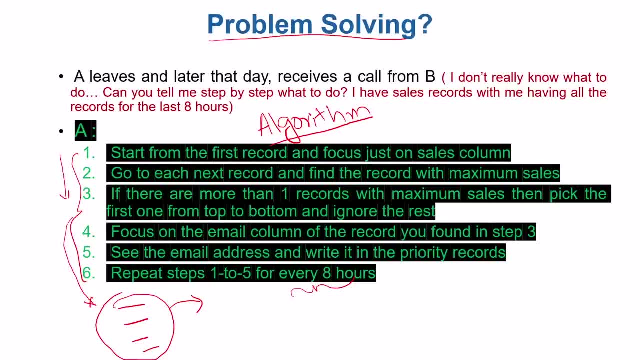 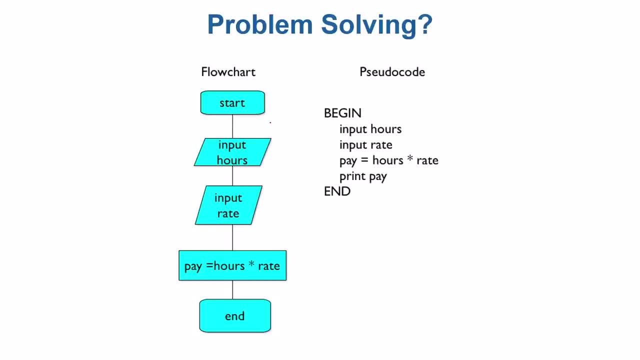 we'll be focusing on pseudocodes, which are basically a pre-step off of the actual code of in any programming language. So hope to see you in the next video. Okay, in in the last video we were talking about the. 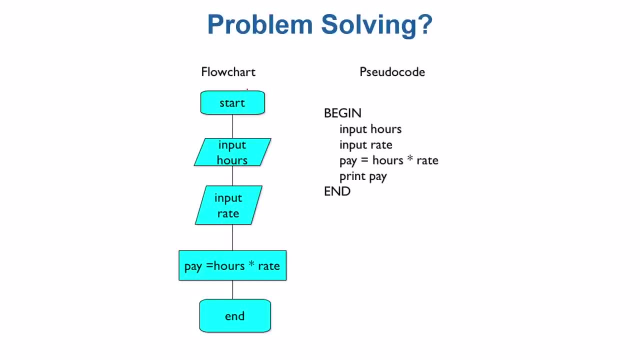 the algorithm, what an algorithm is and how to express that. any, any algorithm. And we saw that algorithm is just a step by step procedure. But but how to express an algorithm may vary. I mean, you need not always to have plain English to. 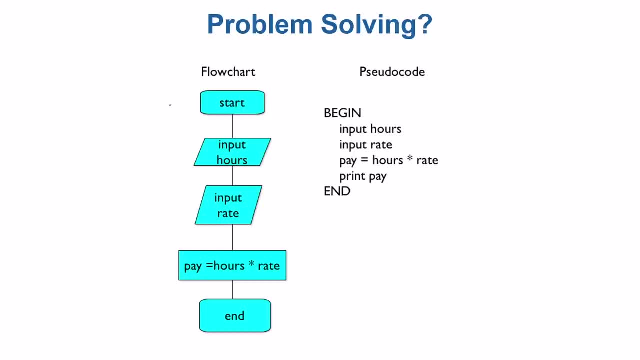 or or any natural language to express algorithm. The reason is that the natural languages are normally so expressive and each and every sentence they may have multiple meanings. So it is. it is a good idea to come up with a structured way to express an algorithm such that each and every statement is completely unambiguous. 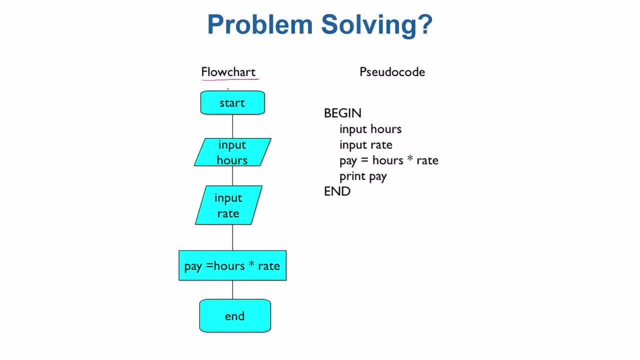 And one such way is is to express algorithms using flowcharts. Flowcharts are are graphical ways of expressing algorithms. Here we are taking the. the problem here we are discussing is is computing pay of different employees of some company And the procedure of. 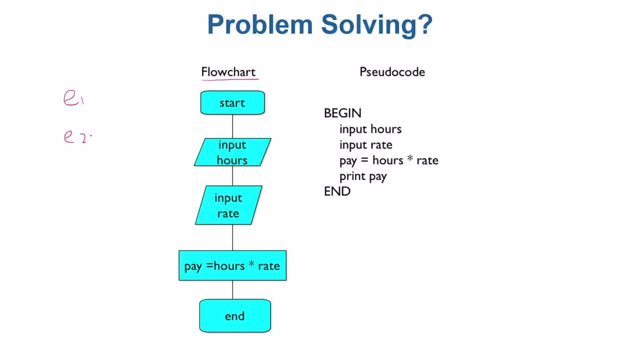 I mean if there are several employees, let's say employee one, employee two, employee three and so on. Let's say there are several employees in a company and having each employee has name, phone number, email and all the credentials. 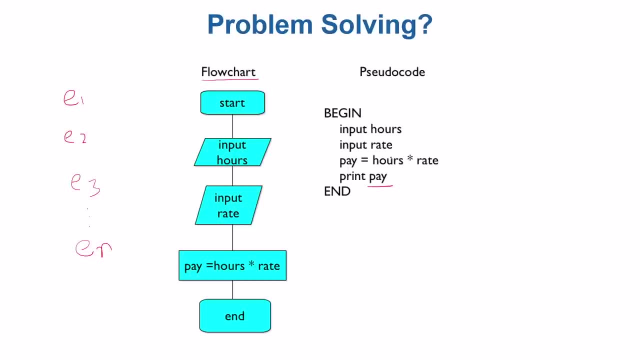 And then let's say the pay is computed on hourly basis and each employee has worked certain hours, for example eight hours, and each employee has an hourly rate. might be, let's say, 100 units. whatever the units are, Employee two might have worked. 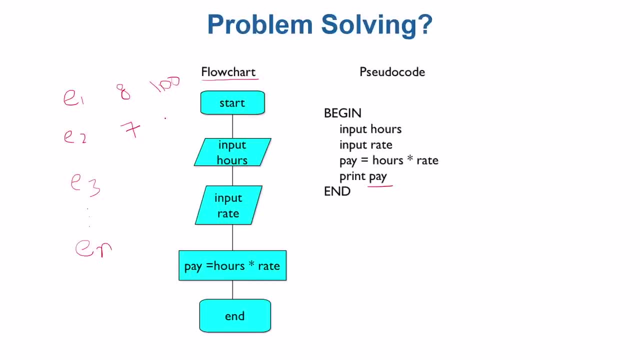 for example, seven hours, but the hourly rate of this employee might be 200 different employees, They might have worked for different number of hours and each employee can have a different hourly rate depending upon the capacity of the employee or the or the job nature the employee is doing, and so on. 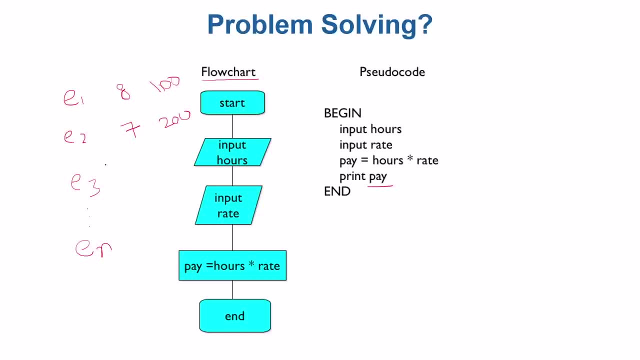 So so. so if we want to compute pay of all employees one by one, the procedure of of computing pay is stays the same, The instances they differ. For employee one, the value of hour is eight. the value of rate is hundred. 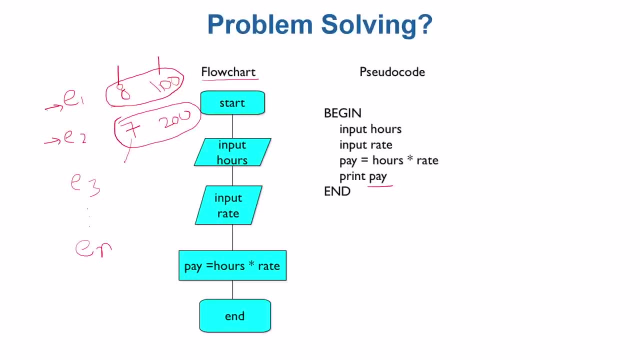 For employee two, the procedure will stay the same: The the values of hour and rate. they will differ. So what should be the procedure? The procedure might be that you take the, take the input of, let's say, employee one or whatever employee you are going to compute salary for. 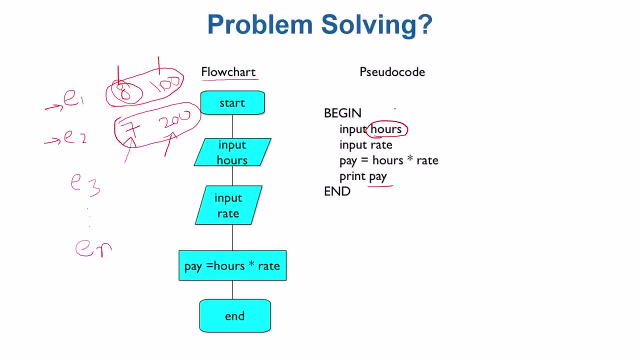 Take the hours hours value in in in a placeholder, call that placeholder. call that placeholder as hours placeholder or a variable. Why this is called a variable? Because for different employees this value will different, will be different. 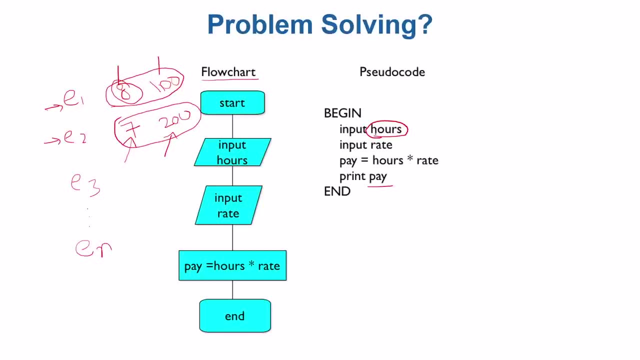 Hours will take value eight for employee one. This, this variable, this placeholder, will take value seven for employee two, and and so on. Similarly, once, whatever employee, whatever employee for which you are going to compute the pay, if you have taken the hours from some records, 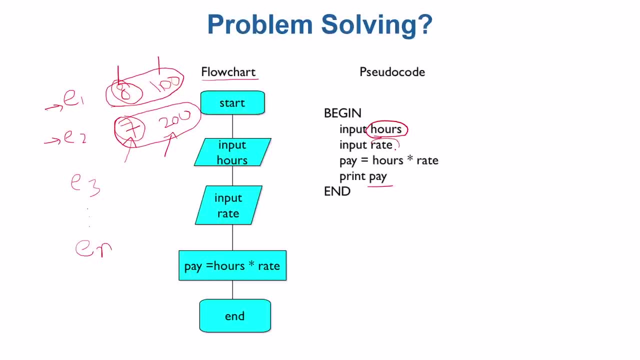 from some working records, then take the rate for the same employee as well. So input this, that's step one. input two, that is step two. The steps, the sequence of these two steps may change. For example, you take the: 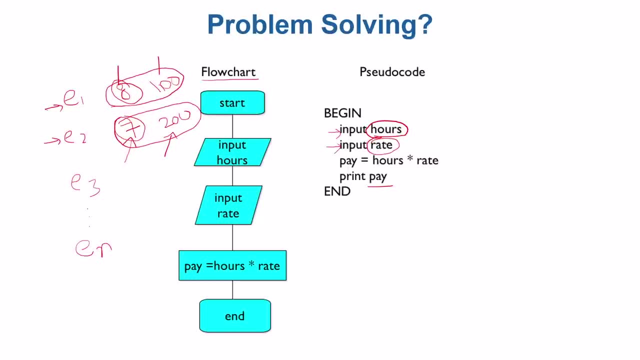 you take the rate value first and the hours value later than that. But either way, that's one way of, that's one way of expressing this, this procedure. And then you compute the pay by this formula: So hours multiplied by rate. 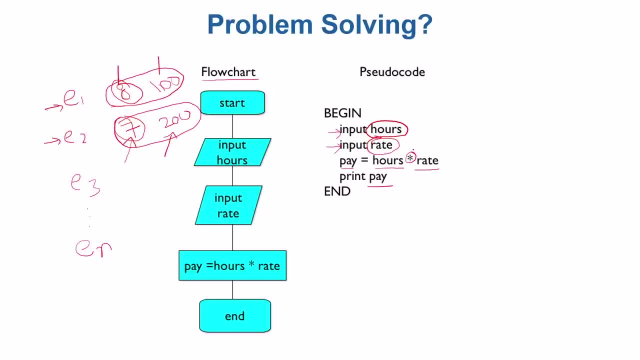 So maybe this is confusing writing a star, Maybe maybe we should write this cross symbol, because that is more common in mathematics, Or maybe this whole line can be replaced by by this particular line, maybe. So pay is equal to multiply Hours and rate. 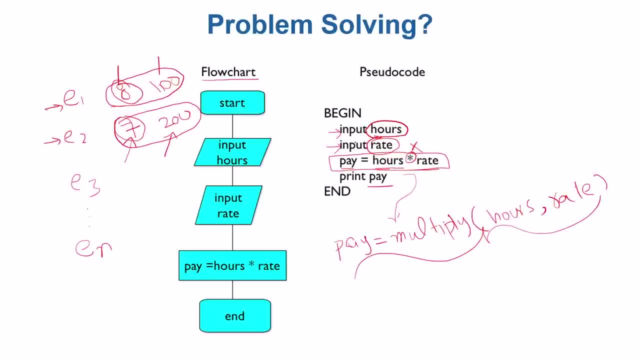 Maybe this is more expressive, but it completely depends. I mean, when you start writing pseudocode or whatever pseudocodes you're writing, what kind of keywords begin, is a keyword and is a keyword, What kind of keywords you are using and stay with those keywords. 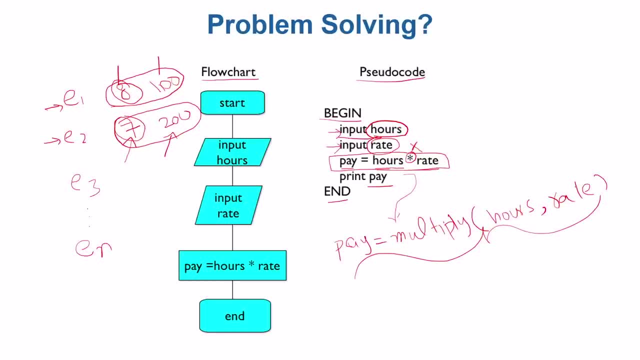 For example, if the keyword input is to use to take to get the values to, to process on, then input should stay everywhere, wherever we want to do such kind of operation, If you, if you're using, for example, the value get rather than input. 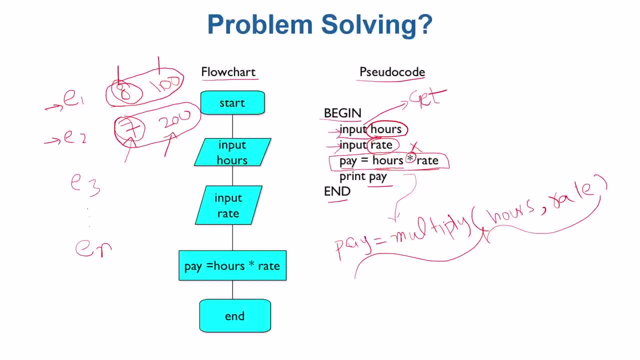 then use get always, but come up with some set of keywords that are expressive as well as concise, and then take the sequence of those statements. Each and every statements should be, should have a unique meaning. It should not be ambiguous, and the sequence should be: 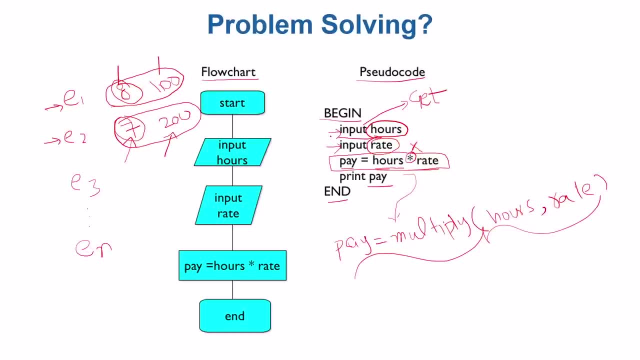 you know the sequence, describe the flow of what is happening, what is going on. So first we take hours, then we take rate, these two values for, for for any kind of employee, and then we will just multiply them And after multiplication, 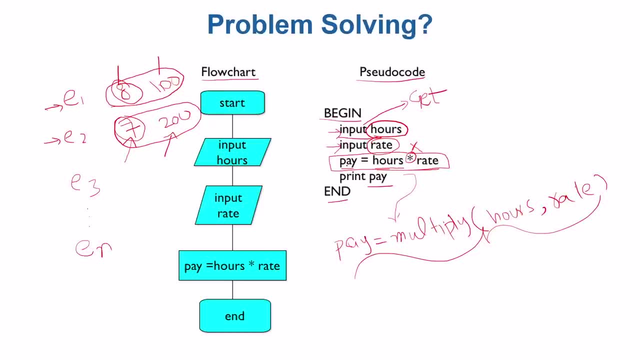 whatever decision we want to make based on this pay, we will do that We may. we may record this value, this pay value, at at some other records register We may. we may print that value on a print slip. We may have emailed this value to some other department. 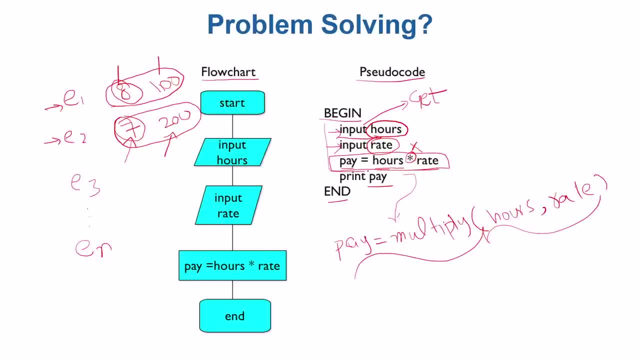 whatever decision we want to make, but the procedure really is still here, Then, based on pay, whatever action we are going to do, that that may differ. Similarly, if, if we go, this is, this is, I mean some kind of structured example of. 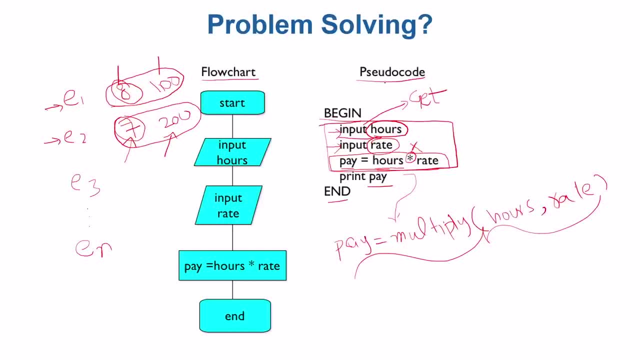 of the of the expressiveness of an algorithm which is called a pseudo code, and what kind of keywords you're going to use. There are no general keywords. I mean some people may use get, some people may use a different kind of keywords for it. 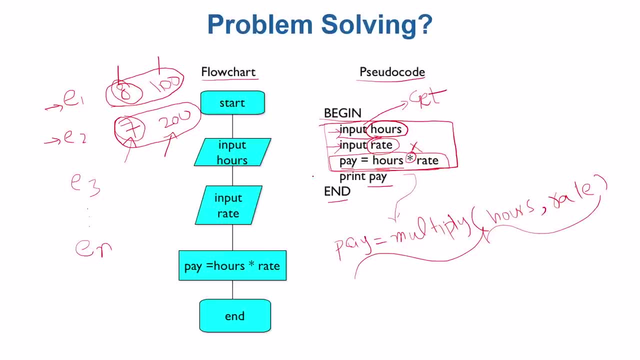 but it is good to come up with a set of keywords to to describe the, describe the solution of the solution of the problem in flow chart, For example, everything, every, every statement here, that is here in in pseudo code, every statement is described as a shape. 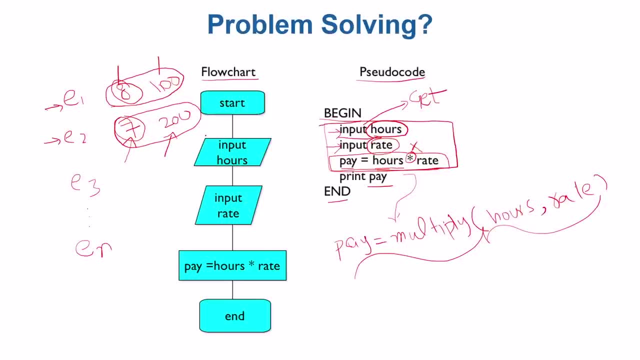 different shapes for different kinds of statements. If you want to take input, then you have to describe that action using a parallelogram. If you're going to do some computation, you have to express that using a rectangle. the start symbol and end symbol. 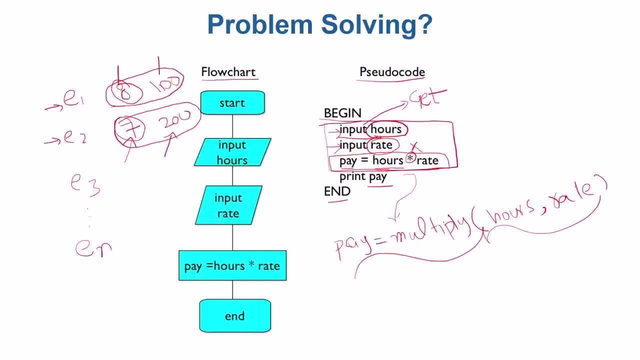 the start and end of any procedure. in flow charts they are described by the, by the ovals, For example, this oval and that oval. Normally the flow chart sequences from top to down, but it is always good to just print the arrows to describe the. 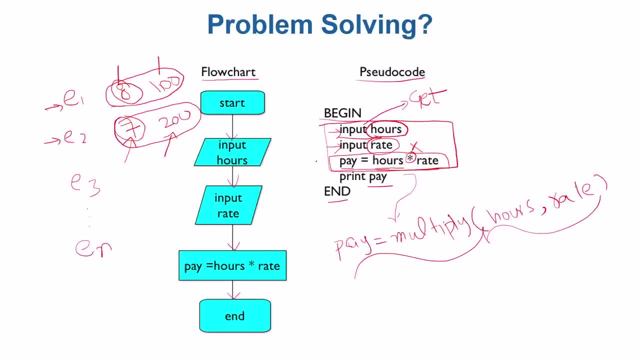 the flow, because in complicated flow charts there are, there are loops, there are if conditions, there are so many things, So it is good always to describe the flow using using arrows. So now the question is: flow chart or pseudo code? because 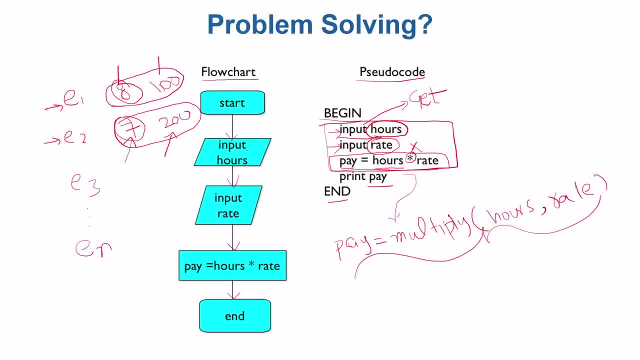 uh, flow chart also looks like a very cool way of writing expressing an algorithm, and pseudo code is also a way of expressing an algorithm. Well, converting flow chart to actual programming code is somewhat tedious- Writing a pseudo code beforehand which is readable. 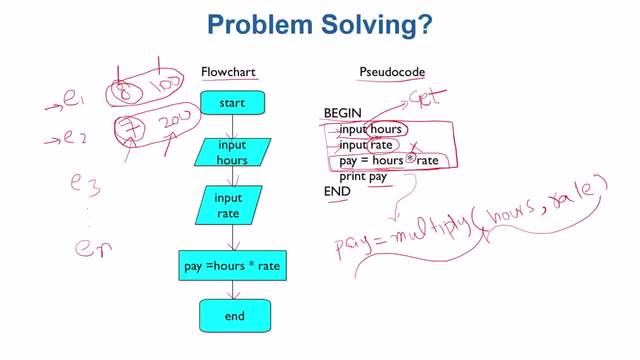 which is precise, concise as well as unambiguous. Then converting that pseudo code to code of any programming language, that is not that hard, That is simple, And writing flow charts for very complicated problems is somewhat tedious, because then it it also requires another transition from flow chart to the actual programming code. 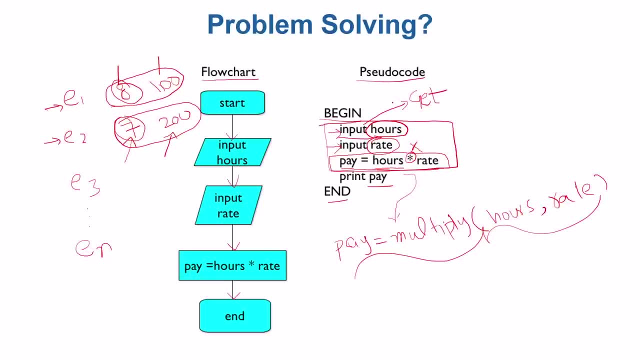 Um, that's why writing pseudo code is more feasible if the goal, eventually, is to convert that pseudo code to some code of programming language. So, um, you can go with flow chart, You can go with pseudo code. Either one is fine. 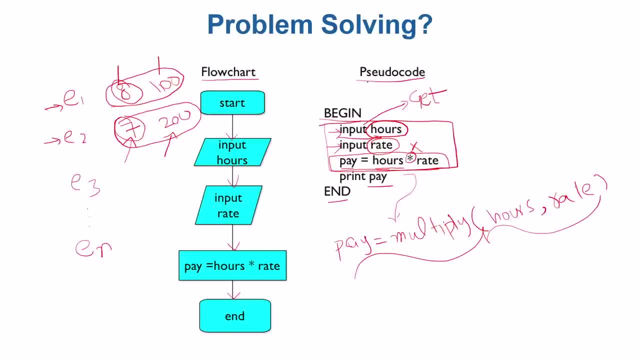 but a more feasible way of expressing Algorithms is a pseudo code, Um. that was just a very simple example. I mean computing, computing salary of an employer, writing a procedure for that. Um, I mean, this is so simple. Nobody make here. 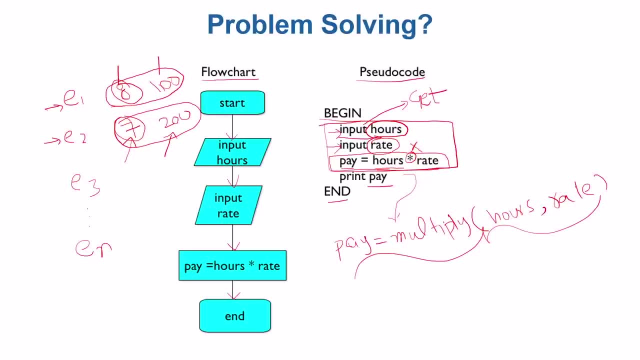 uh writing that kind of uh writing solution of this kind of problem as a, as an algorithm or as a pseudo code, as a flow chart. But the basic idea is is: is is the same, Even if you have a complicated problem. 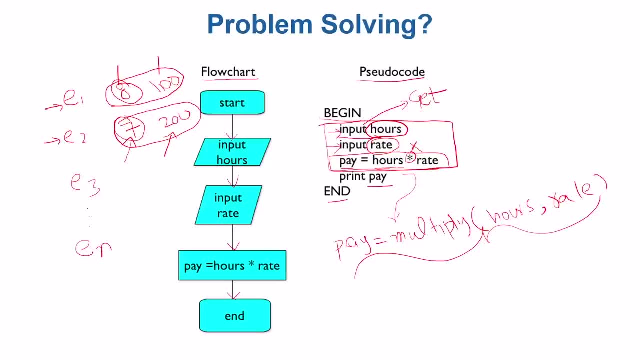 if you, even if you have a problem with maybe many more steps, the, the idea is still the same in the in, in the next video, we, we will, we will see, uh, a procedure, how to. 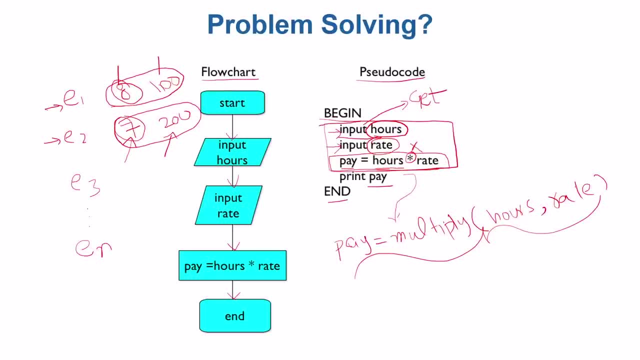 how to make tea, for example. um, that might, that may look, look to you funny. I mean, do we really want? do we really want to know the procedure to make tea? Well, the idea is not to learn how to make tea. 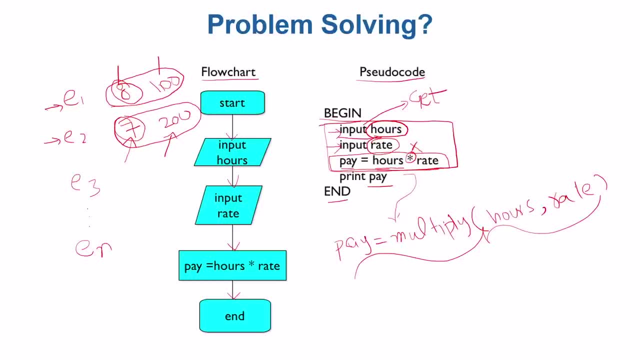 The idea is to learn how to express the solution of this problem. Making tea, That's a problem. The solution of this for how to? how to express solution of that problem as as a pseudo code, And we will see one more example of flow chart as well. 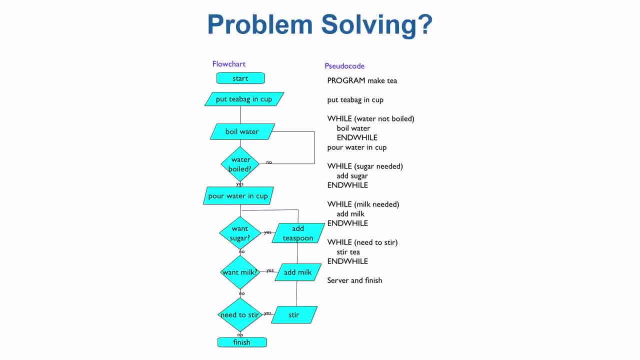 So hope to see you in the next video. Okay, In the last video we saw flow charts and pseudo code. We just took an example of- uh, we took a very simple example: computing salary or pay of employee of a company, given hours and rate. 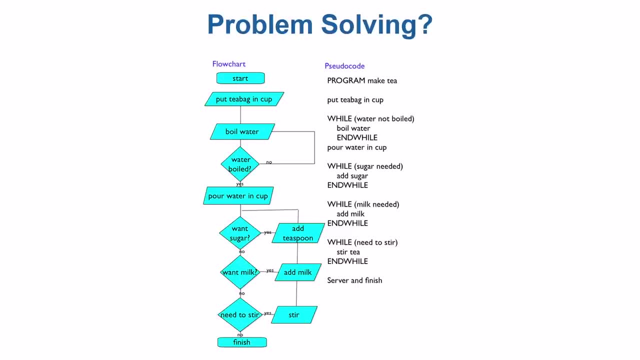 And I also described whether the comparison between flow chart and pseudo code, And I said that pseudo code is closer to the code of some programming language which eventually we need, because eventually we need uh, automation of uh of a solution of a problem. 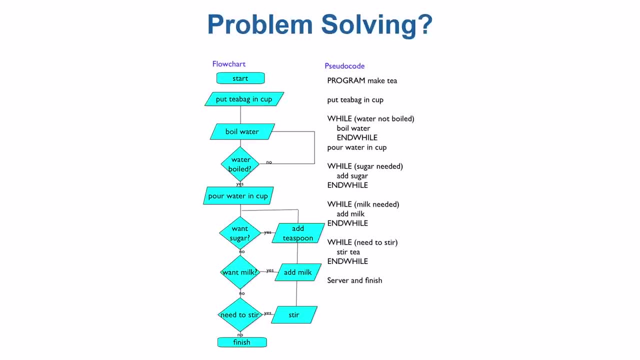 And for that we need a code of the, the, the code for the solution, the general solution in some programming language, So flow chart and pseudo code, and then the code, the code of some programming language like Python. It is somehow. 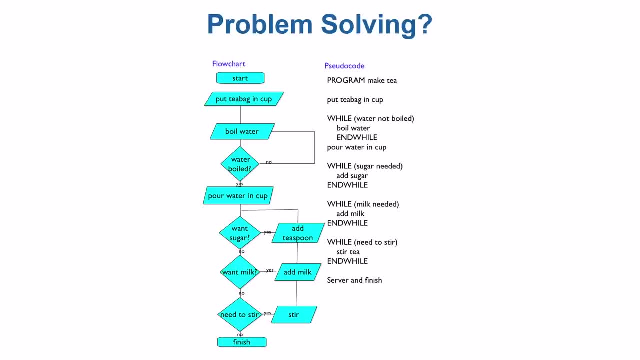 um, and sometimes handy to to break the problem or to device the general solution of any problem, in first step in a flow chart, because that is more expressive, uh, and more generic, more general, maybe in a graphical way, And then, once the proof of concept is clear, 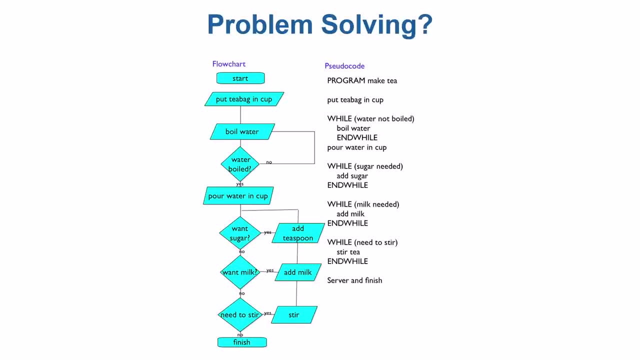 once it is clear that this is indeed a general solution- it has no bugs inside, It has no errors, It will work always- Then we can take another step to convert that flow chart to pseudo code, And then pseudo code can be converted to. 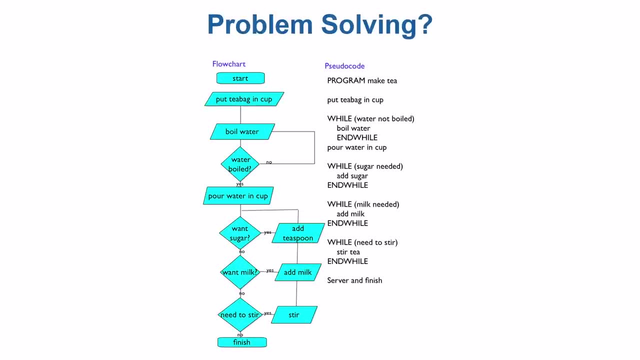 uh, the, the code of any, the code in some programming language. But writing pseudo code um, right away, I mean from the very beginning, without flow charts, is also a common practice. Either way, whichever way suits you, Uh. 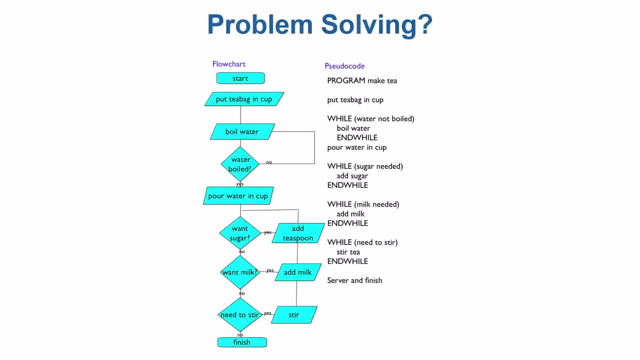 in this particular um video I'm going to talk about uh problem. The problem is: is making tea? Um, you might be thinking what are the different instances of this problem? I mean, making tea is making tea. 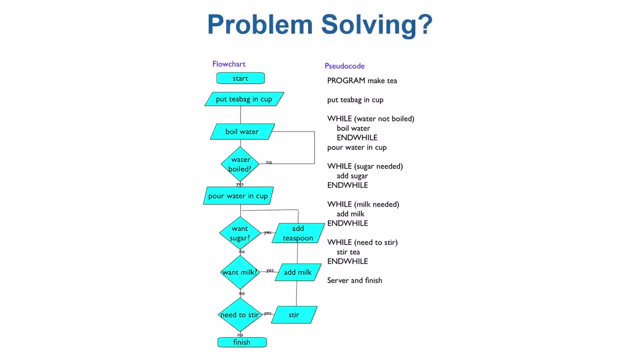 Um, what? what kind of different instances are there? Well, uh, one person may be liking tea with, for example, 1.5,- uh, units of sugar- whatever the units are- And another person may want a tea with 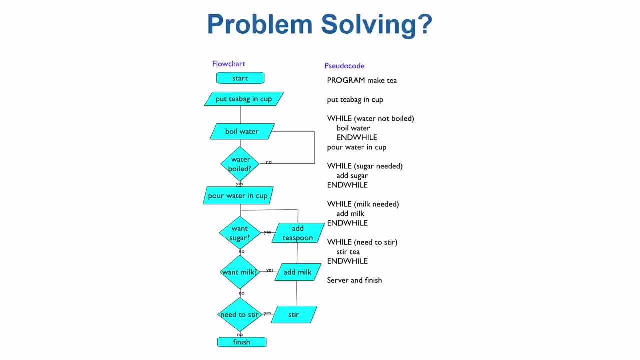 let's say, um, two units of sugar. One person may be, uh, maybe needing a tea with, for example, 0.5 units of milk, and another one maybe a different units of milk, and so on. So the 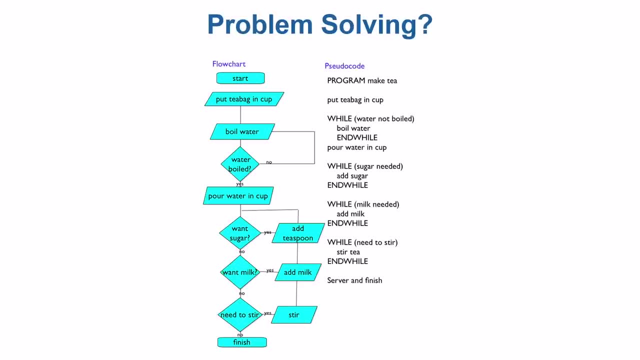 the procedure of making tea should stay the same and the instances, which means the different people want tea in a different kind of combination, that may vary. So let's, let's like, let's see a procedure first in flow chart and then in. 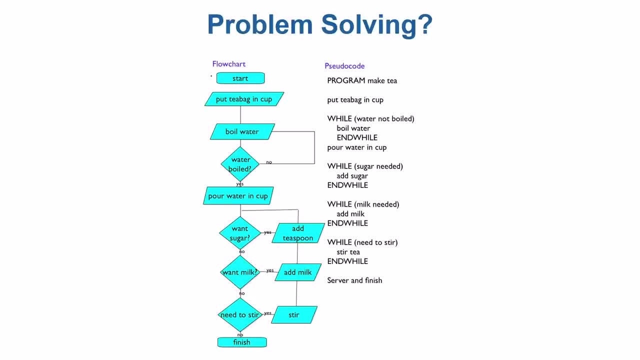 in pseudo code for for making a tea, for making tea. So let's start that. That might look like that might look. you look to you a kind of funny kind of problem, but that's a genuine problem. For example, if you want to make tea, 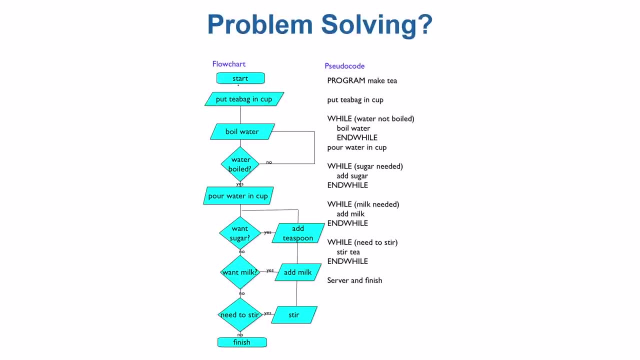 what is algorithm for this? So first we start and then the first step we do is we put tea bag in a cup. That might be a first step. You can argue: should this be a first step? Should that be the second step? 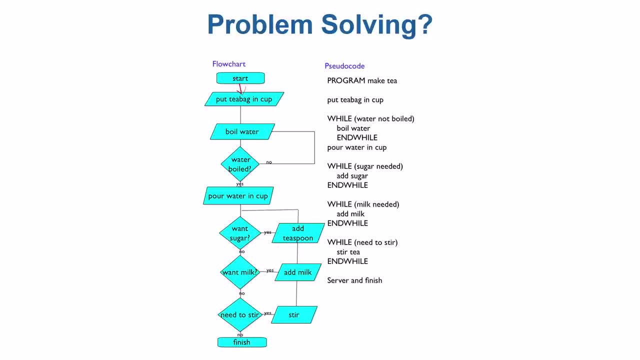 And so on. this the sequence of, by the way, solving one problem. you can have multiple algorithms for that and two different algorithms made just very because of the sequence of statements, even if you have the same statements. So I'm not talking about that. 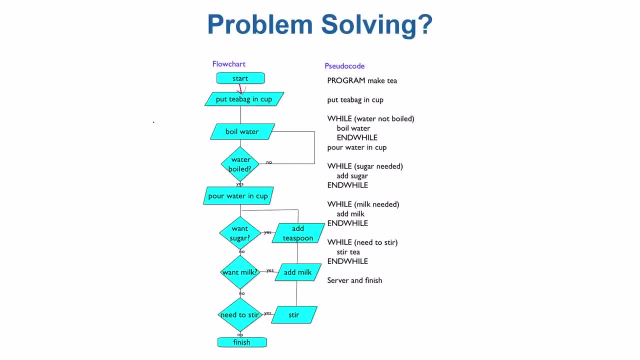 The algorithm or the general solution is unique. You can have multiple different general solutions or procedures. So, for example, putting a tea bag in a cup, that might be first step. or the first step might be the boiled boil, the water and pour the water, and pour the water in the cup and then put the tea bag. 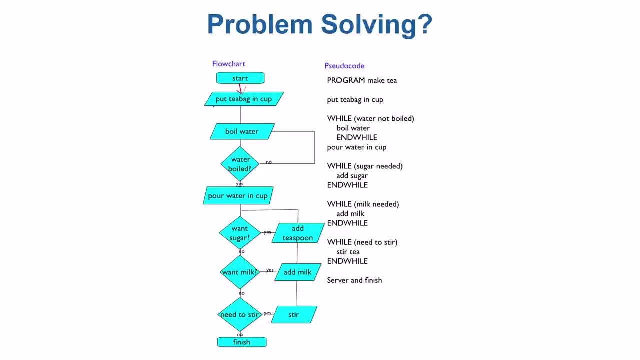 Both are fine. I mean this way or that way. So let's start with putting a tea bag in a cup. So that's an, that's an input. We take a tea bag from somewhere. That's our input. Last time I told you that input is taken as parallelograms. 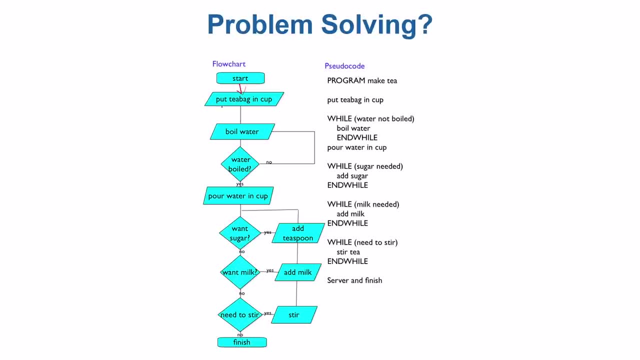 Put a tea bag in a cup and then forget about that cup and boil the water. Somewhere there is a water. I mean take the water from somewhere and boil it and see if after, let's say, five or six or seven time units, 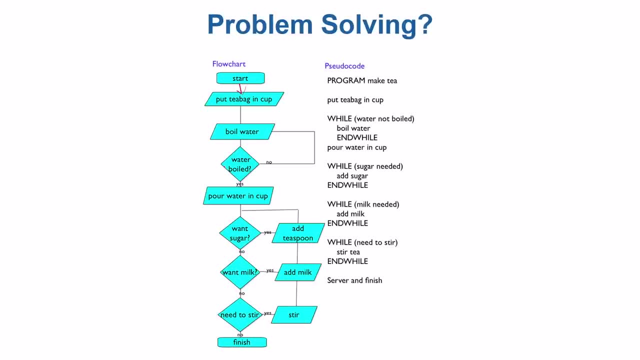 whatever the time units are, see if the water is boiled or not. Assume that there is a test that tells you that the water is boiled or not. So there is a test available to you, So you apply that test and check that the water is boiled or not. 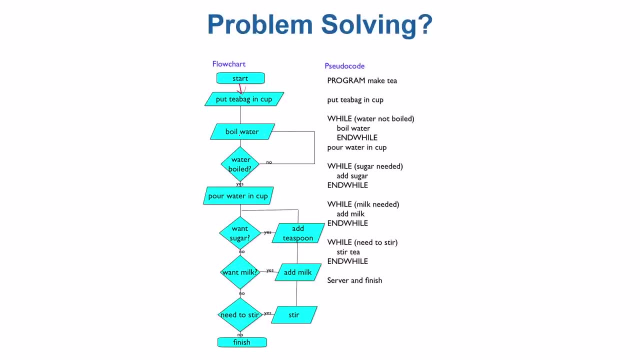 If it is not boil, then keep on boiling. So boil it again And assume there is a procedure of boiling water. In normal case, boiling water is just happened by. I mean keeping the temperature high or putting that thing, putting the pot of water on fire, or something like so. 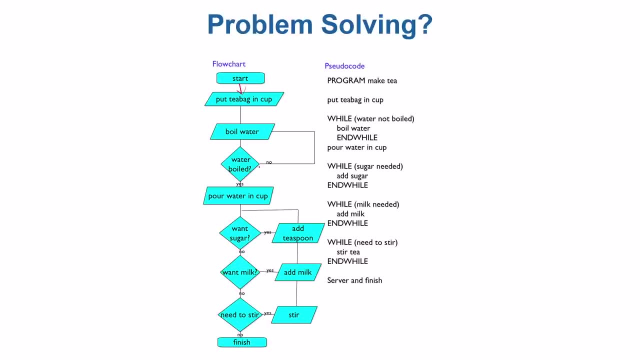 But that that itself is a procedure. So boil the water again and boil the water again. Check if the water is boiled. If no, then boil it again. If boil again, then check. If no, then boil it again. This is called a loop. 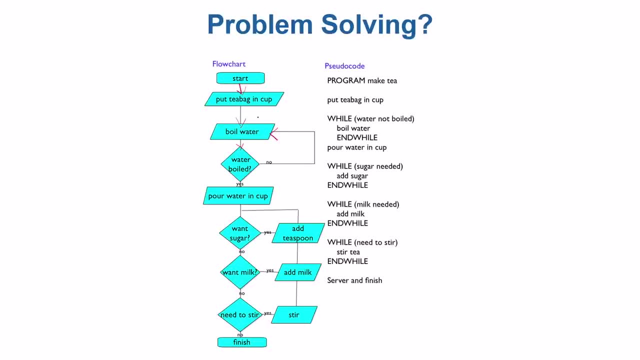 This is called a loop or repetition. You are doing the same kind of stuff again and again until there is a particular condition, that is, that is met. So in this case, the condition is when, while the water is not boiled, keep on doing the same procedure again and again. 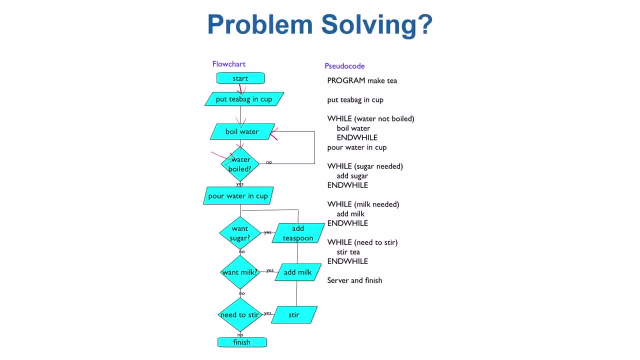 This is called repetition or loop. So you boil the water again, check the condition. If the condition is true, for example, the water boil, Yes, then come out, Then you're, then you can exit this loop and come out Then pour the water. 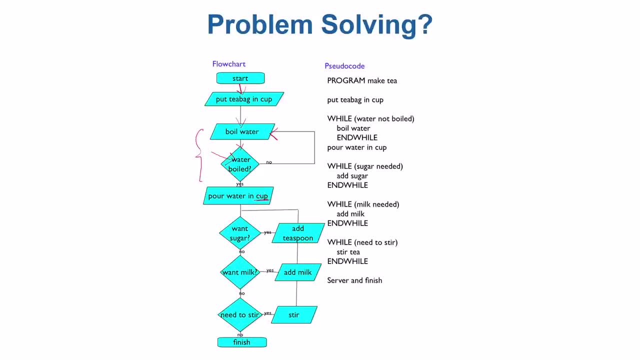 pour the water in in the cup Here. we should here, We should describe that: Is that the same cup or a different cup? Well, the cup here is acting as a placeholder where this tea bag and the water is going in. So we have a cup. 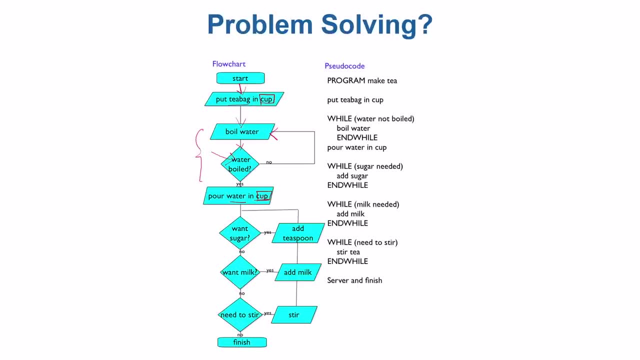 We put tea bag in it, Then we put the boiled water in in it, But before pouring the boiled water in it, we just boiled the water. Okay then, after we have water in a cup and a tea bag in a cup, what should we do next? 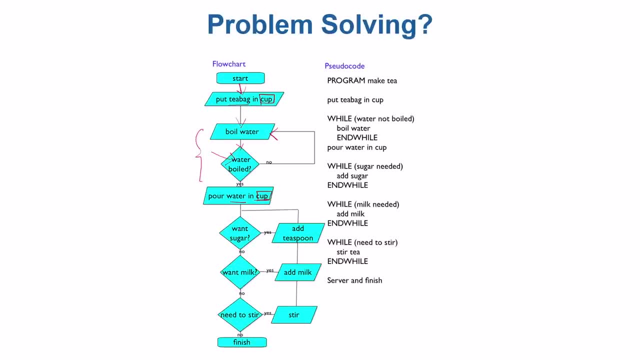 We actually, we actually first test: want sugar or need more sugar? If yes, then then add sugar. So let's apply some arrows. If yes, add some, add sugar and then again ask: do you need, Do you need more sugar? I want sugar now. 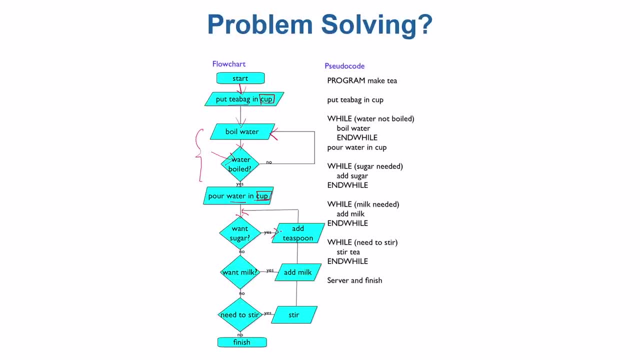 Yes, add sugar, one sugar. Yes, add sugar. That is again a loop, That is a green, a loop while while the while you want sugar, I mean you test that the sugar is okay or not. Here you test that the sugar is okay or not, or whatever sugar you need. 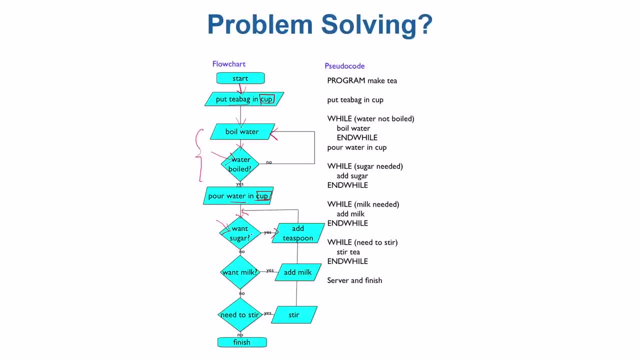 If, is that okay? Not until that condition is not met, You keep on adding the sugar at a teaspoon again, then test at a teaspoon. That is again a loop or repetition. Once the condition is met, one sugar No. then exit this loop and ask: want milk? because some people just take tea without milk. 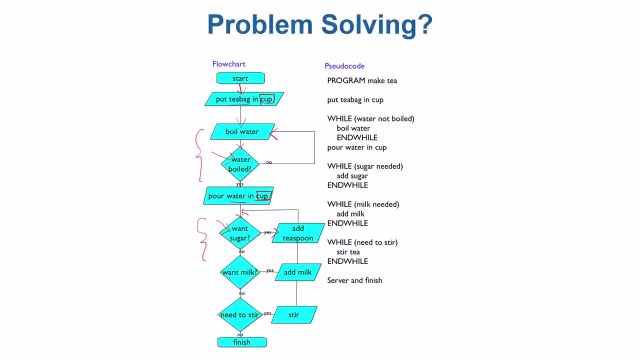 Maybe somebody wants a milk, Maybe somebody don't, so want milk, Yes, So add milk. So that's, that's a mistake. This, this loop, should go there, there, right there, and this line shouldn't be there. That's, that's wrong. 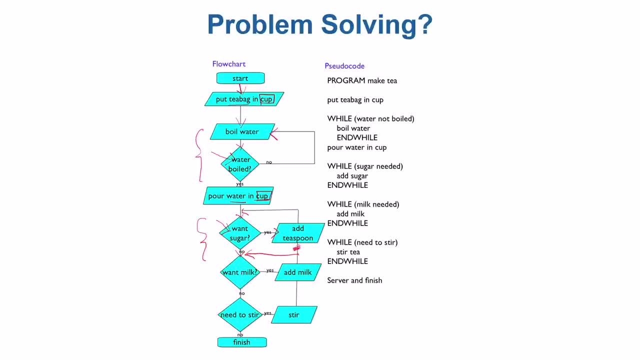 Add milk and then ask: want milk? Yes, Add milk. That's again a loop. Once you exit the loop, then you ask: need to steer? Yes, steer. then ask again: This line again shouldn't be there, So that that's another loop. 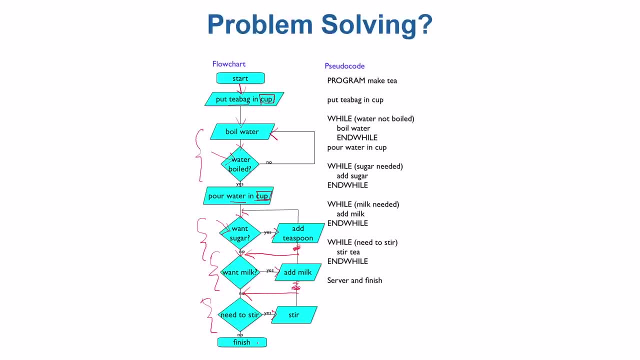 Once you exit this loop, then the tea is ready. You serve that tea. finish. You are done with the procedure. Now let's see the same procedure in. in pseudocode, program is a keyword and that's what program name is. program Make tea put is a keyword. put tea bag in a cup. 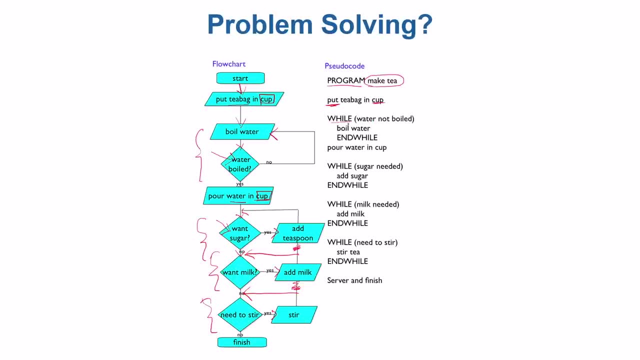 While water not boil. while is a keyword, While this is not, while this condition is not satisfied, Keep on doing this, Whatever written in while and end. while is is the body of this repetition, or called loop. So, while water is not boiled, boil water. 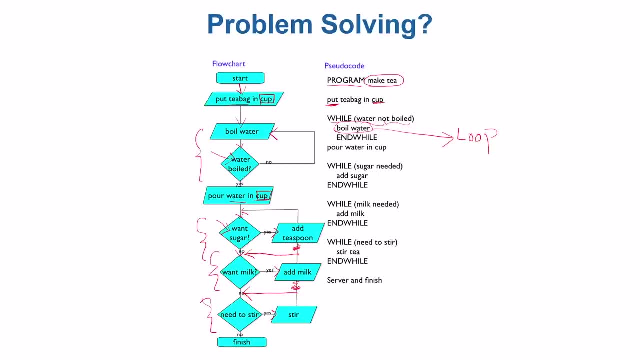 then again check water boiled or not. No, boil again, I mean keep on boiling. So this is repetition. Once the water is boiled, which means this condition is: becomes False water, not boil, becomes false. So water boiled, then you exit this loop. 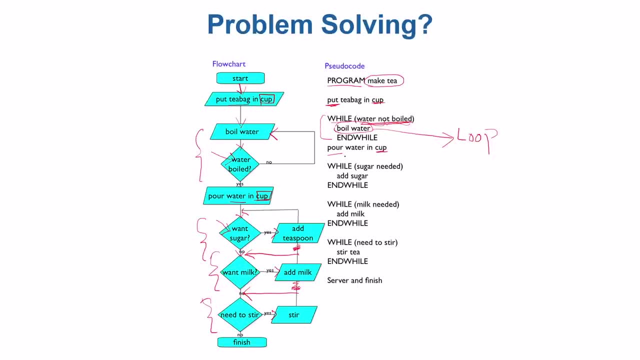 You pour that water in cup- That's again a keyword- you in a cup. and then you ask, okay, need sugar. Yes, add sugar, Need sugar, Yes, add sugar. So you keep on doing this until you don't need sugar anymore. 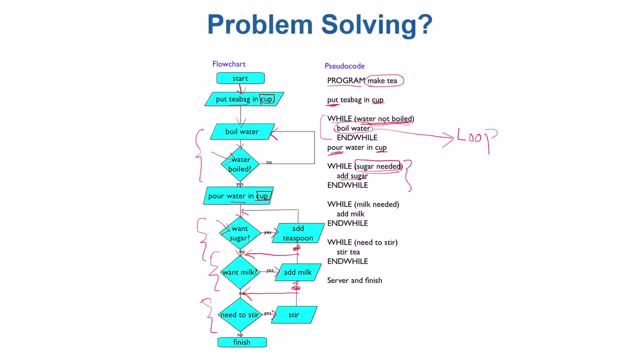 So that's again a loop. So so you might be thinking that why we are writing this add sugar and this boil water to writer to this this why we are really indenting this. That's a style of pseudocode to just display that this is inside this. 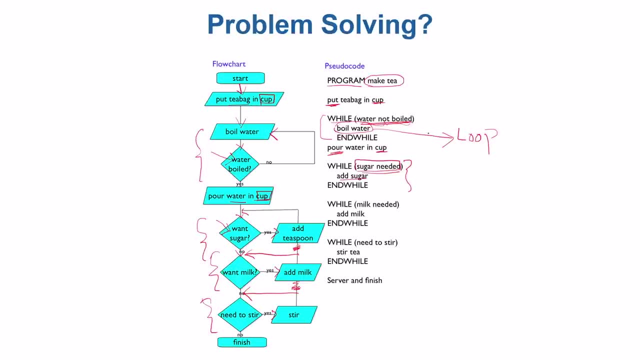 This is this particular statement, or set of statements are called the body of the loop And this end while should be here in this alignment, here in this alignment. So there is a there is a bug in this slide. This should be here, Okay. 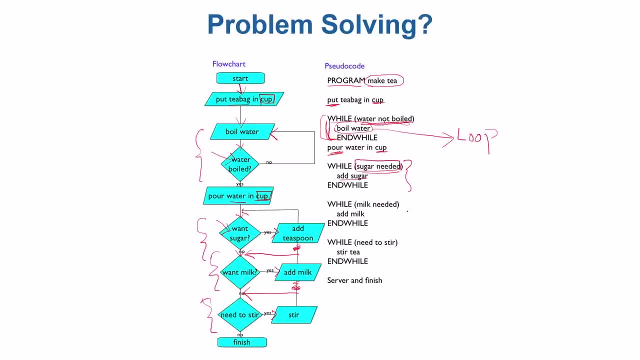 once this condition is false, sugar needed: No. then you can exit this loop and you go here. while milk needed: Yes, add milk. Check again: milk needed: Yes, add milk. milk needed: Yes, add milk. Once this condition becomes false, milk needed. 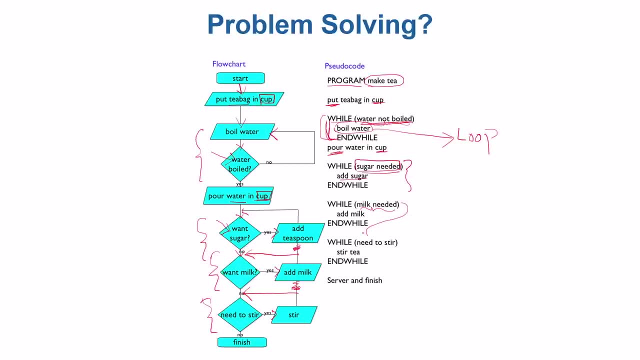 No, then you can exit this loop. You can just go to here while. need a steer. need to steer, steer tea. need to steer- Yes, steer tea. need to steer, Yes, dear tea. Once this condition is false, get out and your tea is ready to, whatever you want to do. 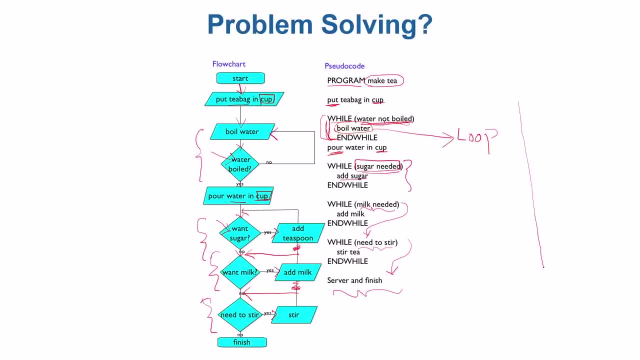 This example was so simple, but it expresses a very powerful tool in in the pseudocode as well as in flow charts, And that tool is sometimes called loop, which is there to repeat a particular procedure, Whatever procedure you want to repeat again and again to until there is a particular condition. 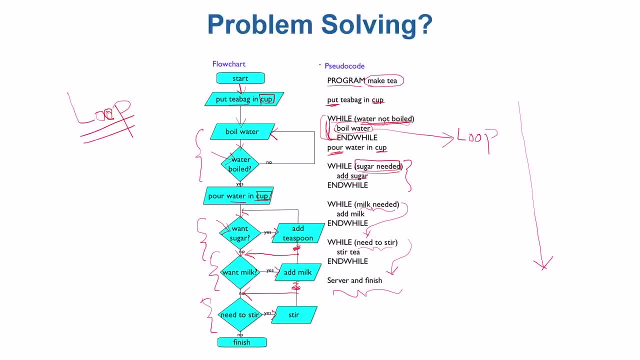 That is met, that is loop, loop is there. So the the the purpose for of this slide is just was just to just to make you, make you convinced and make you comfortable with this pseudocode and and flow chart. We will not be talking about flow charts any further from here on. 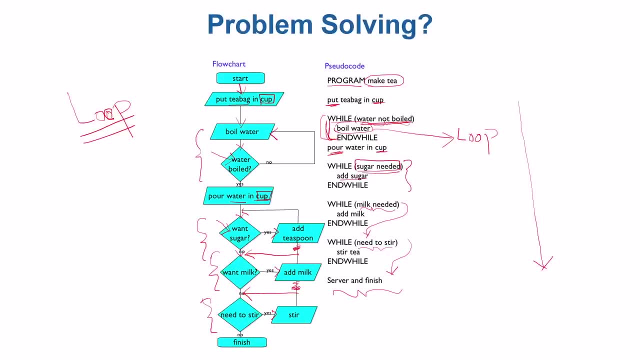 We will be just talking about pseudocode in just one or two more videos and then we will be directly going towards. We will be we will be comfortable enough with pseudocode for solving certain kind of problems that we will then eventually be moving from pseudocode to actual 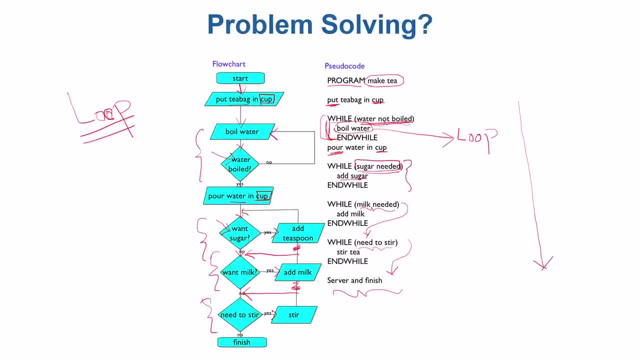 Python code and, and I bet you, I'm going to tell you that the pseudocode in the next video I'm going to explain- that will be very, very easily- will be converted to the actual, exact Python code. So in the next video we are going to actually solve a problem of finding 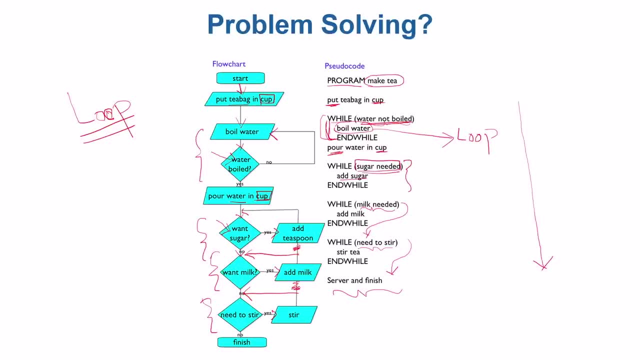 Out minimum value from a list of values, sometimes called the searching problem. We're going to solve it by first using pseudocode and then in a later video we will see how to write the actual Python code for that problem. So hope to see you in the next video. 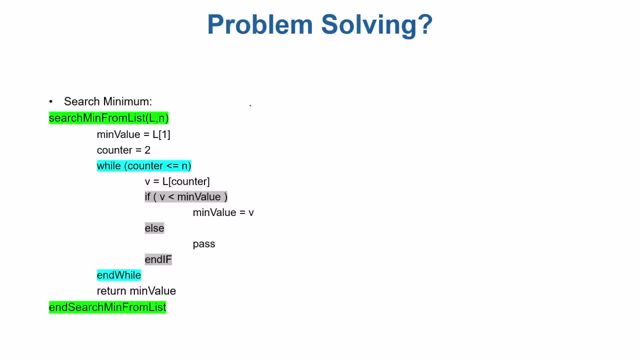 Okay, let's dive into a real problem. Let's say you are given, you are given a list of numbers. Let's say: let's say L Is some list with numbers. Let's say we define list by these, these square brackets. Let's say: the list contains 23.. 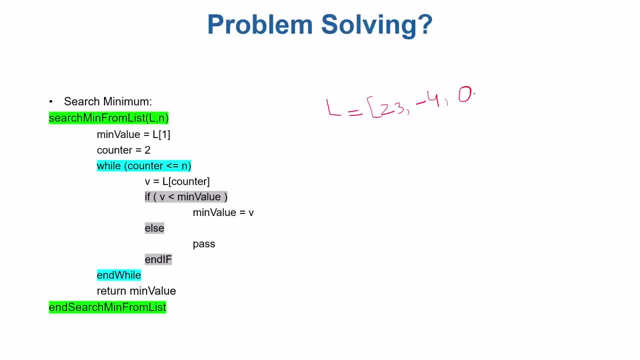 Let's say that's a value minus 4.. That's a value: 0.. That's a value: 73.. That's a value, and maybe maybe minus 10.. That's a value, Maybe 13. That's a value. So let's just take an example that we have one, two, three, four. 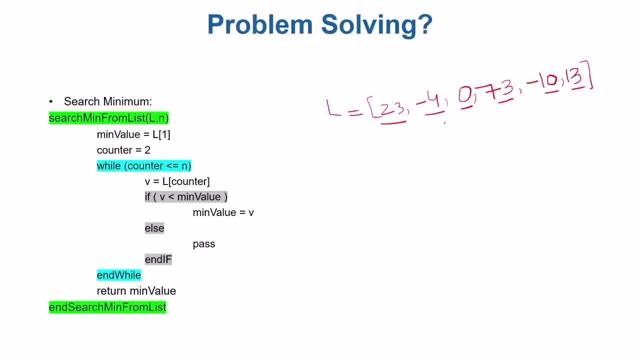 five, six values in a list. So and the list is basically: we took the list here as L and we just describe that. Let's say, the list is declared by or expressed by the square brackets and the elements of the list. They are separated by comma. 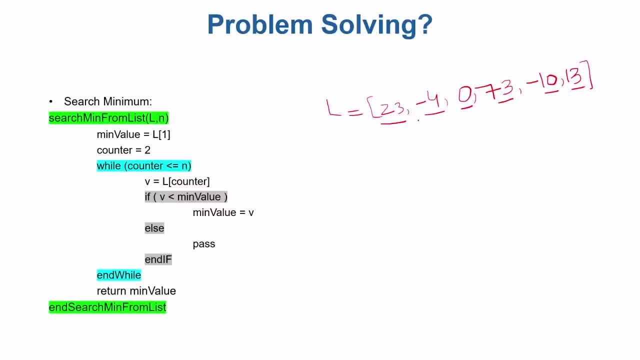 That is just our convention for this kind of problem, for this problem, just for this code and, and- and I'm not talking about Any particular programming language. yet This is just a list of numbers, And let's say we want a procedure that finds out the minimum value of any 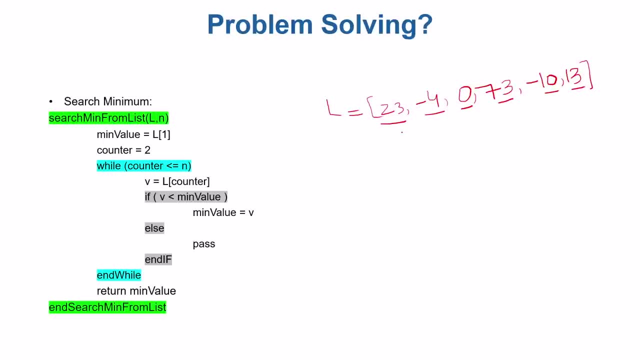 list. Well, first of all, why this problem has multiple instances? Well, we need to come up with a solution that works for any list. For example, if the list is, if the list has these six values, then the procedure should find out the minimum value in this list. 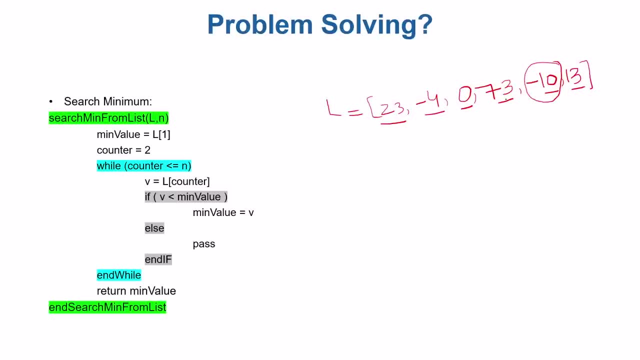 The minimum value in this list, out of all the values, is minus 10.. Because minus 10 is smaller than every other value. 23 is bigger minus 4 is smaller than 23. 0 is bigger than minus 4 because the the value with the negative sign. 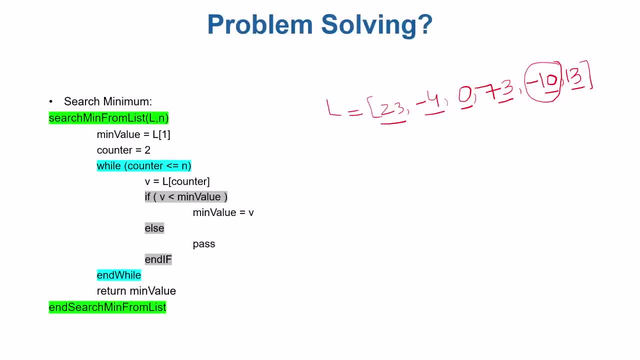 It is smaller with the value of a positive sign. But if you have two values with negative signs, the value with a bigger number in terms of magnitude is, is actually Smaller in negative sense. So if you compare minus 4 and minus 10, minus 10 is smaller in minus in. 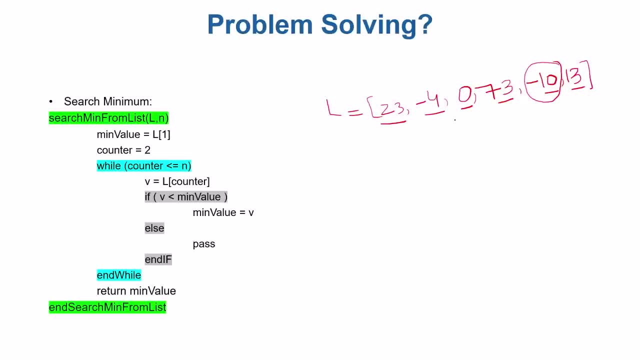 minus domain. in positive domain, the result is different. So I was talking about why this problem has multiple instances, Why you need a general solution for that. That's a list. Just go and find out the minimum. That is minus 10.. 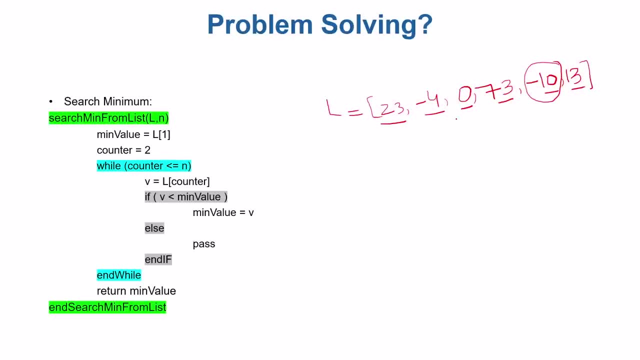 Go home happy. Well, we need a solution that works for another list, another list with different numbers And maybe different number of numbers. Maybe in this list We have six numbers. Another list may have 74 numbers. Another list may have 1 trillion numbers. 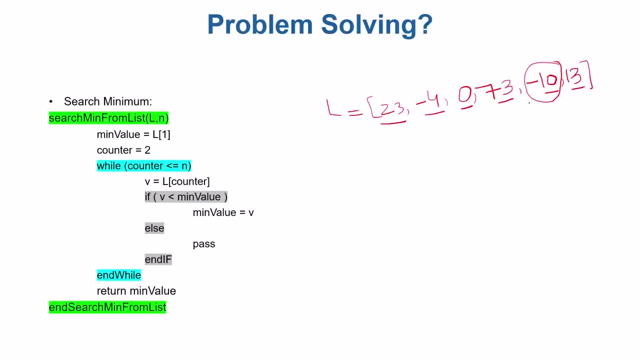 We want to come up with a procedure that always finds out the minimum value in that list. Obviously, the minimum value may repeat. I mean the minimum value may occur more than once in a list. So what is a minimum value, rather than knowing how many times it occur? 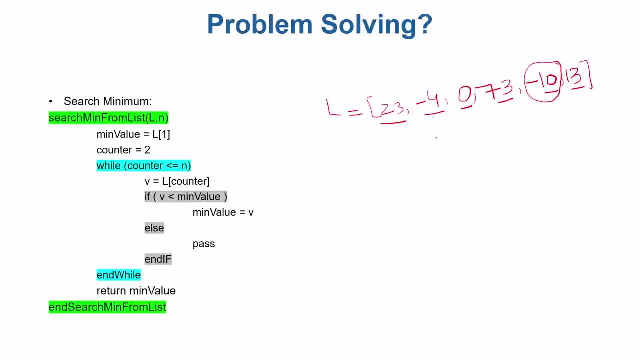 What is the minimum value? That's a problem finding out a minimum value, and we want to find out. We want to come up with a procedure that finds out the minimum value regardless of the list, Whatever the list is. this procedure should actually return or end up. 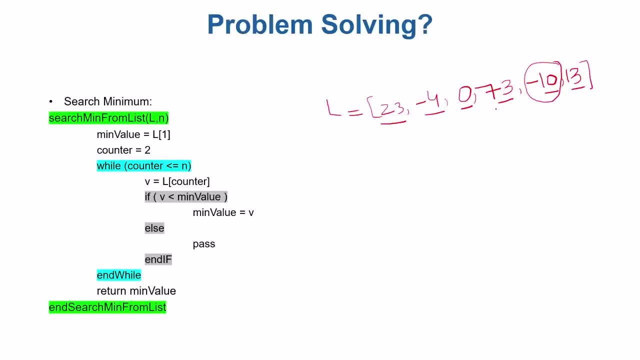 finding out the minimum value. So in this particular case, again, for this particular example, the minimum value is minus 10, and we will take example of this list and we will see how to code a procedure for that. So, but, but before starting this, 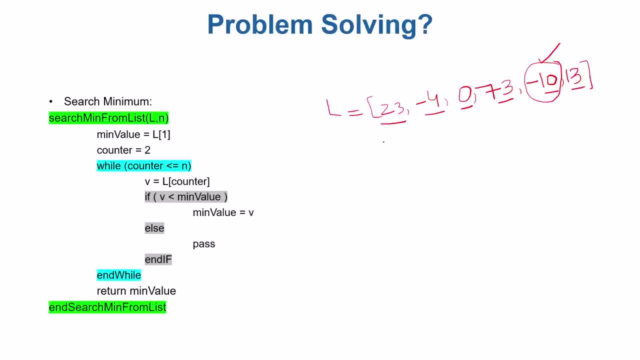 Procedure, what kind of things we really need to to to to write a pseudo code for this kind of problem. We may start by writing that program, Like in the previous video program name as search And then we take input Or input list. then we take input. 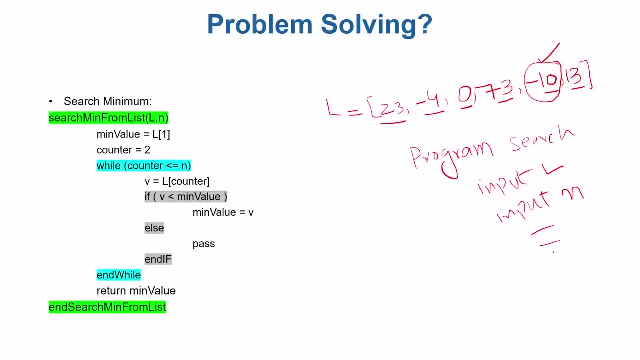 The number of values in the list, the total number of values, and then we move on as as we want to move on. But writing out a procedure in terms of pseudo code, It is always good to to avoid these input statements inside the pseudo code and always supply whatever, whatever needed, always supply the. 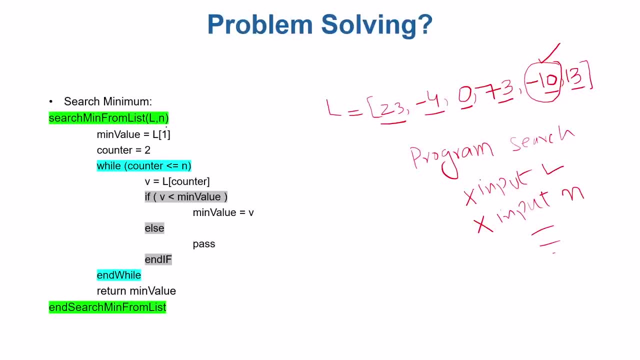 instance from outside and assume that the instance is supplied and then just work on that instance rather than reading the instance, rather than taking the values of instance, A particular instance from inside the code. It is always a good practice to to to supply the instance from outside. 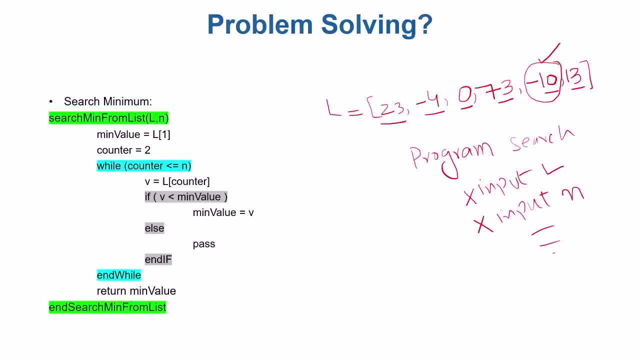 So supply the list from somewhere, and this n is really the size of the list in this particular case. Let's say, if this is the list, then that list will be there, supplied from somewhere. We will see how to supply that and this n value here in this particular case. 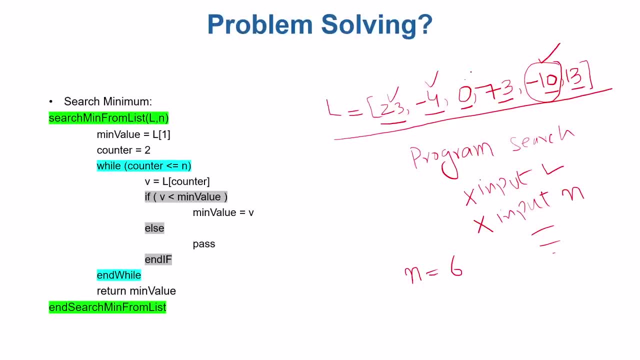 The n value is 6. the total number of values in the list: one, two, three, four, five and six. These are six values. So it is a good practice to, rather than writing program and then this, just write the name of the problem. 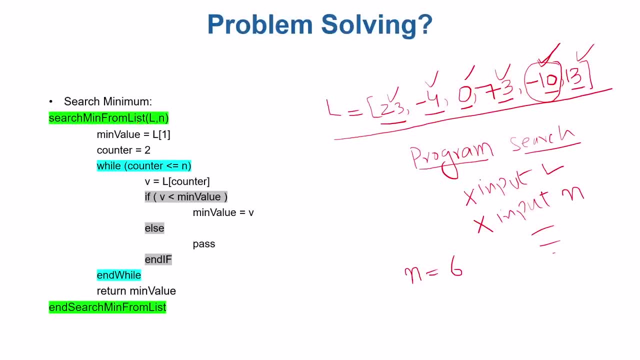 You are going to solve. in this particular case, The name is search minimum from list, and then this particular. we are talking about this list, L, with total number of elements as n. whatever the values inside the L is, we do not know, and and this n may take a different. 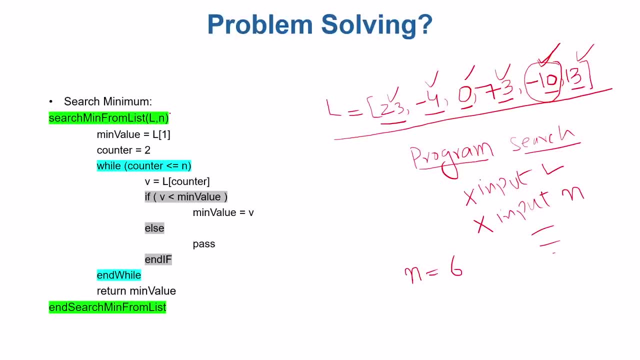 value. this L can be different, This n can be different for different instances, but it is not a good practice to take input from inside here. Then one more convention is that, let's say, list of two represents the second element in the list. in this particular case, L of two is basically L of two is. 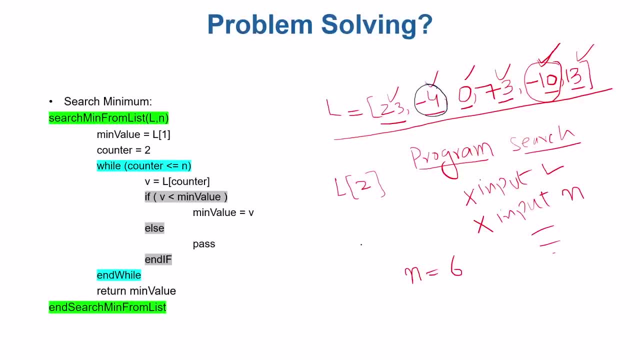 basically the second element in the list, which is minus four L of, Let's say, three is the third element in this list, which is zero, and so on. So let's let's take a convention that whenever we want to access the elements of the lists, but whenever we want to read the elements from the list, we will 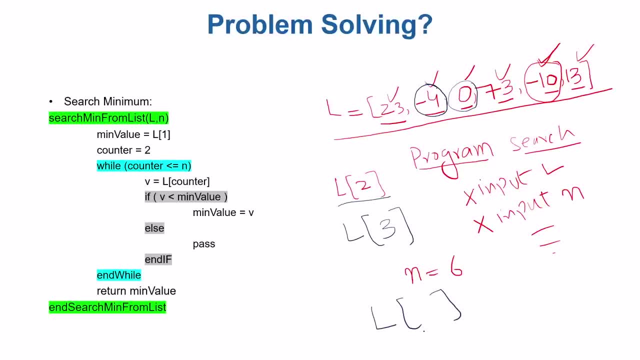 read the element number by giving the element number here. Let's say whatever the, if you write L of I, that means it means the ith element of the list. So first we take a variable. We are assuming here that the list is supplied to us. 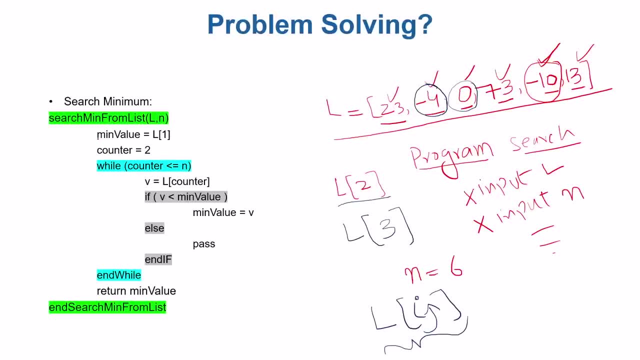 The total number of elements in the list is supplied to us. So we first take the minimum value we which we really want to compute, the minimum value we want to compute, but any list can be supplied in this procedure. So what's the procedure? the minimum value that we can want to compute. 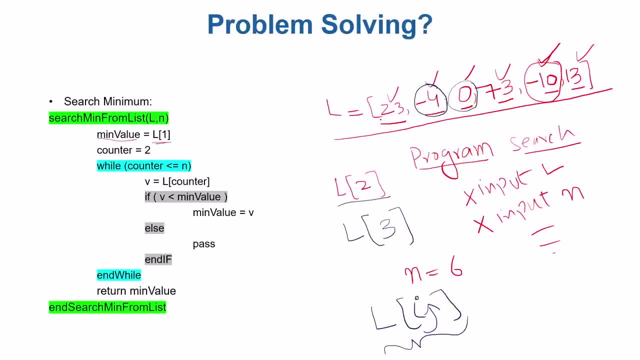 We just consider the very first value of the list. In this case, the very first value is 23.. We consider that is the minimum value. Obviously, that is wrong. This is not minimum value. Minimum value may be somewhere else, or maybe this one may be somewhere else. 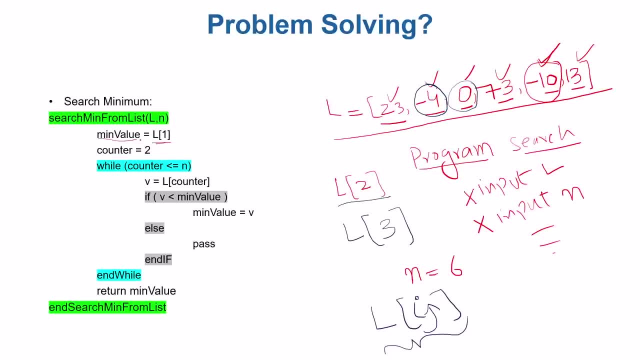 but we are not sure that the first value in the list is the minimum value. But let's, let's just hold on for a moment and move on. Let's say the minimum value is this: here This is called the assignment assignment. This minimum value is this: 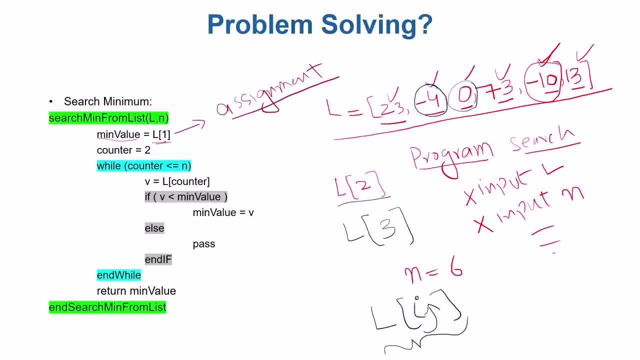 This min value is a placeholder or a variable, and I have assigned this value L1, to it. Now, from here onwards, the min value will be will be having a value which is 23 in this particular case. Okay, so min value is this, which is 23.. 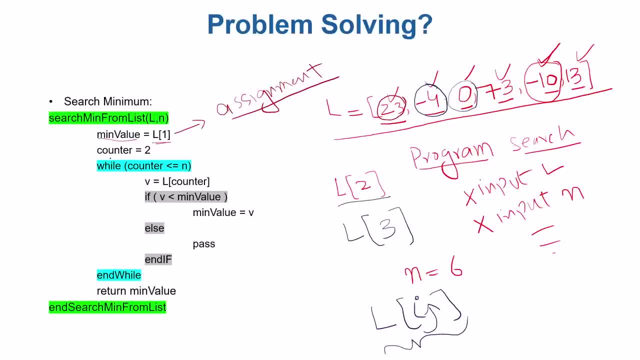 Now let's declare. let's declare another variable, which is called counter. We may need this counter, and let's declare this with To. why we are declaring this with to, it will become clear later on. So now we so so: min value right now for this particular list. 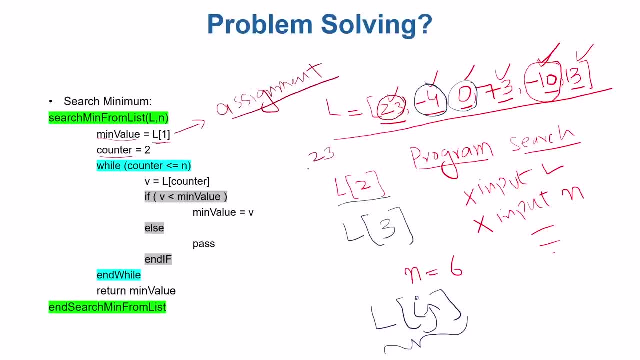 The min value takes the value 23.. So, and counter takes the value to. these are two things for these two variables. Now we apply a loop. while counter is smaller than n, smaller equal to n- Remember the value of n for this particular example is six, and counter here. 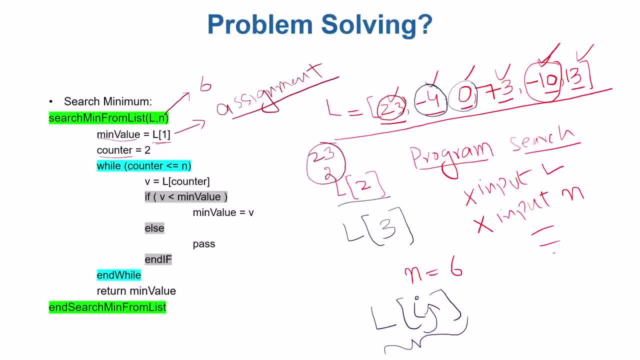 Is to so, because counter has value to, while two is less or equal to six. First check whether this condition is true or false, because if this condition is true, then you will go to the body of the loop. Then this whole box will execute. 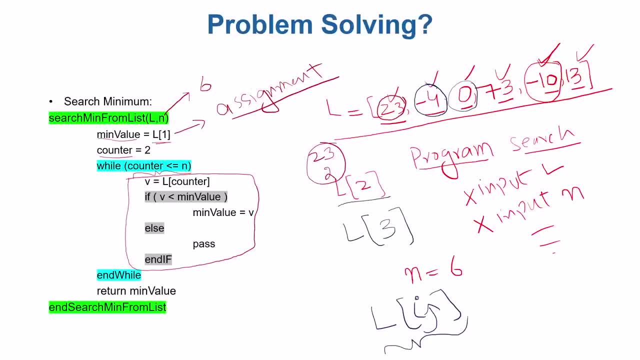 If this condition becomes false, then you will exit the loop and will go out. So now, counter is to the: So two is smaller or equal to six. true, false, That is true. So the condition is true. Two is indeed smaller than or equal to six. 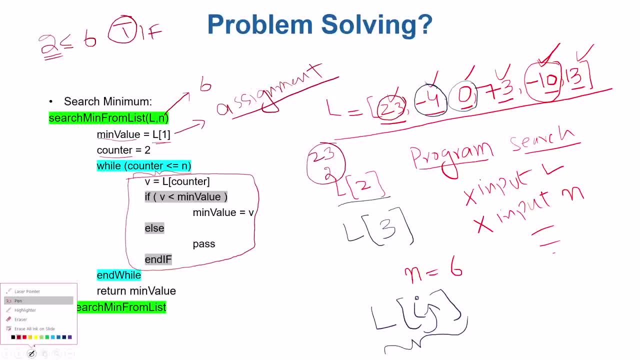 That is true. So we will go inside to the box and see what happens Then. what we will do. we will pick and pick a value from at the index counter. Right now the counter has value to L off. counter means pick the value. 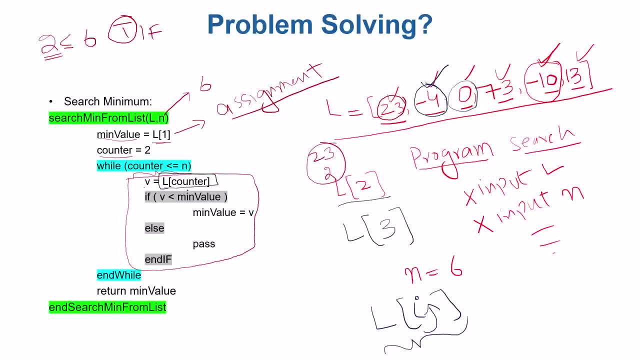 Because the counter has value. to pick the second value, which is minus four, and pick that value minus four from the list. pick that value and copy that value or assign that value to a variable V. That's a new variable We may be needed somewhere. 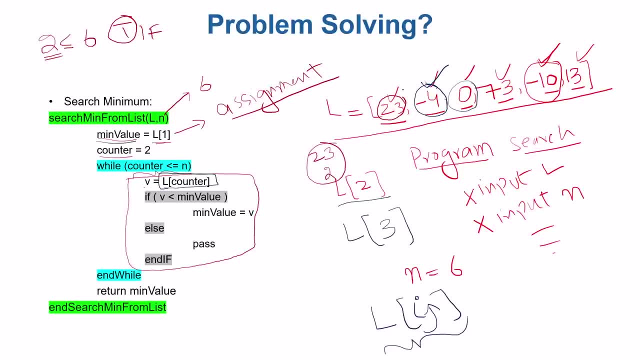 Okay, previously the min value, which is a variable, It was containing the very first value, which is 23.. Now we have picked the second value. The counter value is two. So we have picked the second value from the list, which is minus four. 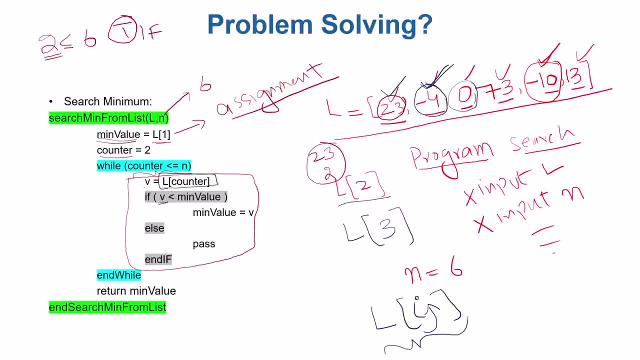 Now we compare: if the value now, which is minus four, is that value smaller than our minimum value So far? the minimum value so far is is 23.. So minus four is smaller than 23.. Yes, the condition is true. 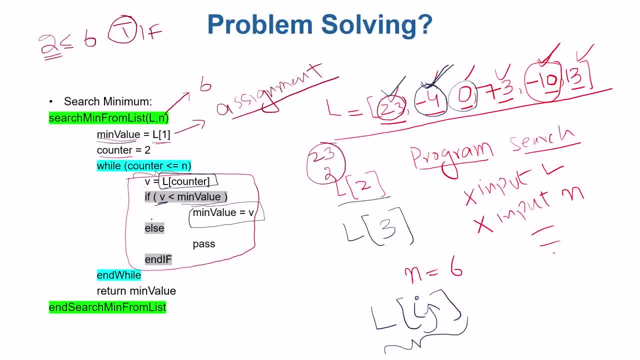 If the condition is true, we will go into this block. Otherwise we will go into this block. So right now the condition is true. So we will go in this block and minimum value will just be replaced by the new value, And the new value right now is minus four. 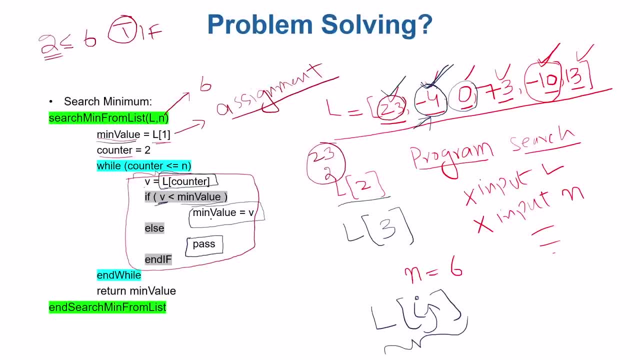 So because a minus four is smaller than 23.. So we are here in this body. The if condition becomes true, you're in this body and the minimum value becomes whatever the value is in V and right. for this example, the value in V is minus four. 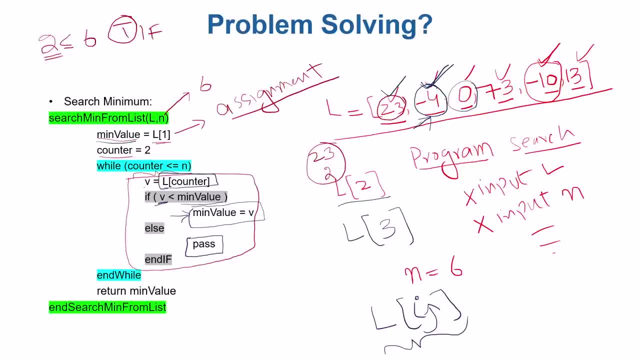 Okay. So if, if, if you go into the if condition, then you're not going into the else part. either You're going to if part or in the else part, one of them. Okay, so then we move back. Oh, there's a bug here. 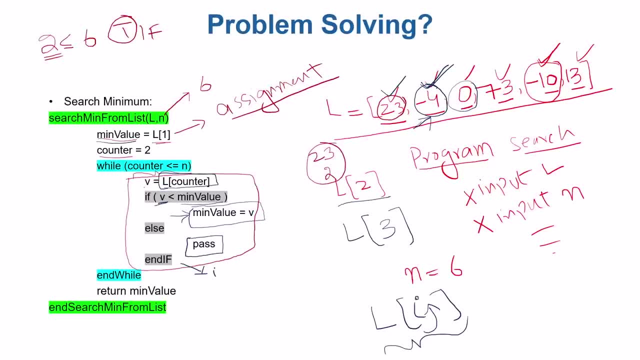 We need to add the counter, We need to increment the counter here. after, after this: before this, there is another statement: increment the counter, Increment counter. That's another statement, Increment counter. So now increment the counter. after this, if part, increment the counter and the counter will become three. 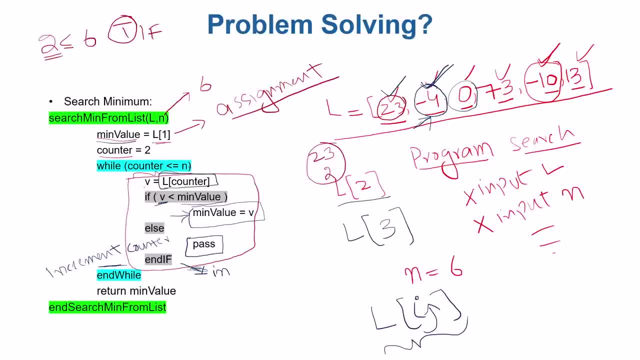 Now we will repeat the procedure and check: three is smaller than six. Yes, we will go inside and we will pick. now The counter value is three, We will go and pick the third entry. and now the third entry will be in V. The V will now contain zero previously. 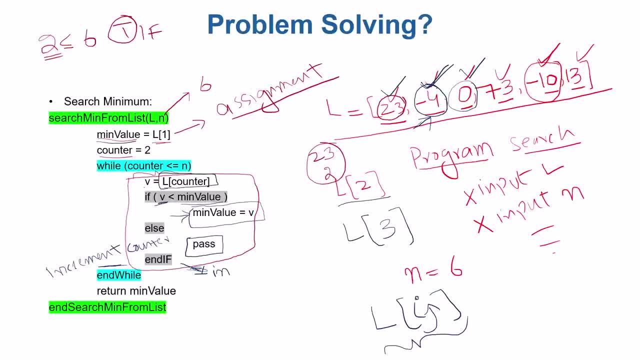 It contained minus four. Now it will contain zero. min Value is containing minus four now. So zero is smaller than minus four. No, if zero is smaller than minus four, then do this, but zero is not smaller than minus four, Then go to the else part. and else part is just saying: just go on, do nothing. 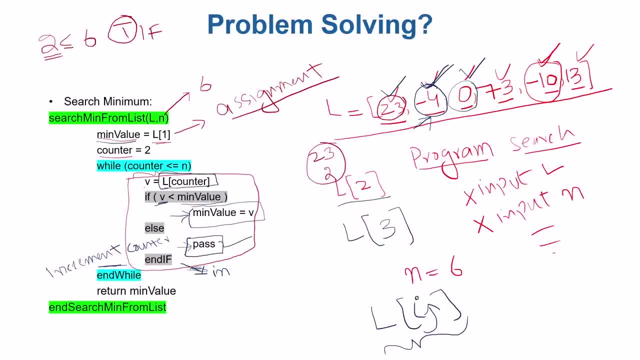 I mean don't do anything. So when you are here, don't do anything, exit. if condition increment the counter again. Now you increment the counter, the counter value will become four and the value at four Is 73. first of all check. four is smaller, equal to six. 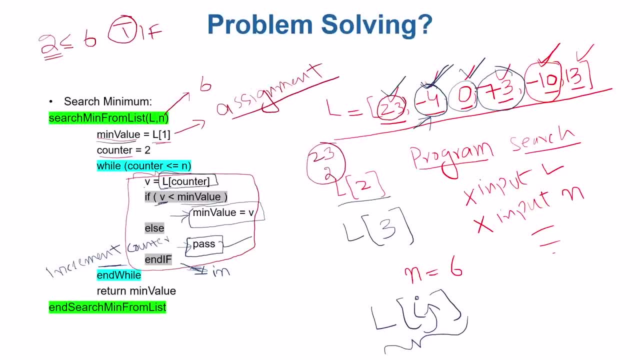 Yes, we will contain the value at index four, which is 73. 73 is smaller than minus four. No, do nothing. increment the counter. check the. if can check the while condition now counter will be five. five is smaller or equal to six. Yes, pick the fifth entry because counter is fifth. 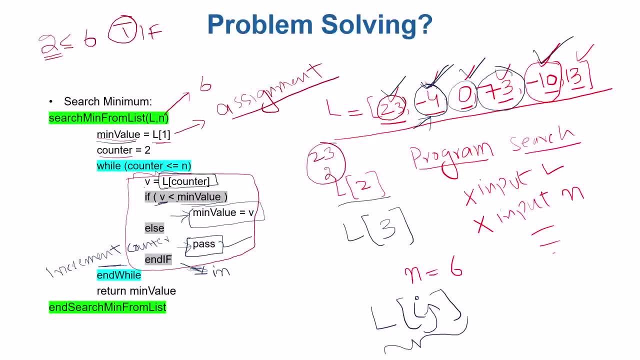 The fifth entry is minus 10. minus 10 is smaller than minus four. Yes, Okay, replace min value with the new value. Now the min value will contain minus 10.. Okay, because if has executed, else will not execute. you exit if condition and then you increment the counter, the counter will become six. 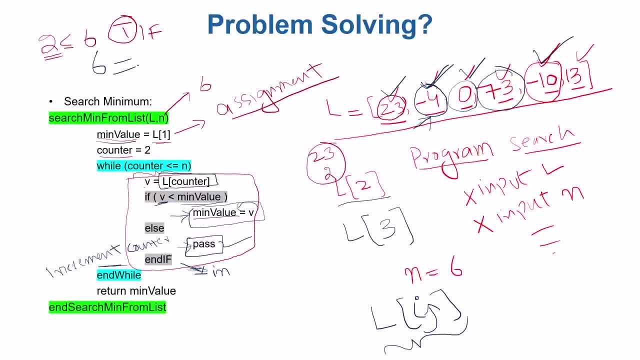 Now, six is smaller, equal to six. Yes, because six is equal to six. Hence the condition is true. Now you go and pick the sixth entry, which is 13.. Check: 13 is smaller than minus 10.. Because min value is containing minus 10 so far. 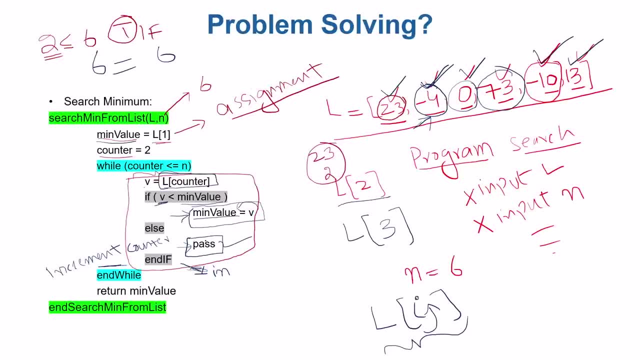 No, that is false. Go to else condition. the two else part just go on to nothing. increment the counter. Now the counter will become seven and you go back and check the condition. Seven is smaller, equal to six- false: exit the loop. Okay, exit the loop. go to this condition. go to this statement. 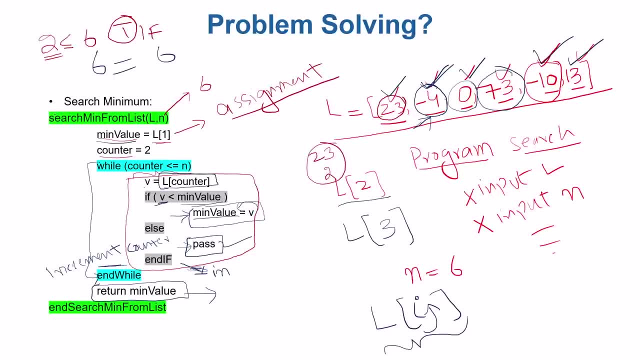 Now, Now you're out of the loop and return the min value and see the min value here is containing the actual min value, which is minus 10.. So that's how we search the minimum. This return is also a keyword, So which means if we, if we, just if we, just if we just use that function. 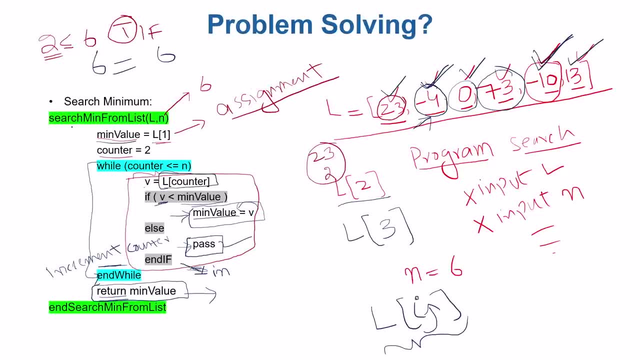 if we, if we just use that pseudo code with, if we just use that sort of code for this different kind of lists with, with its sizes, whatever the list this is. this was just one example. If we change the list, the procedure will work one. 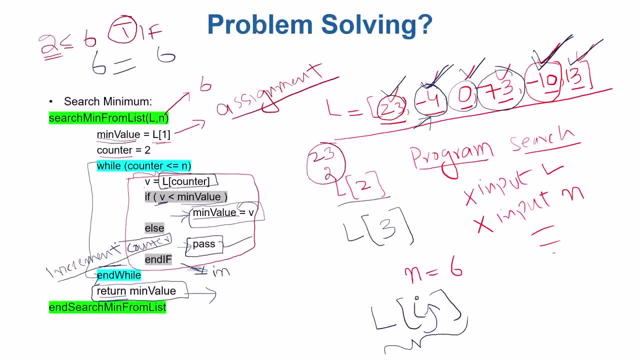 one bug in the in the code was the increment counter statement was not there. It should be there after the this end if and before this end while here. So this: that was a pseudo code of searching minimum. in the next video We are going to use this pseudocode and we will. we will see how to rearrange the values of a list or sort the values of a list such that all the values that are smaller. 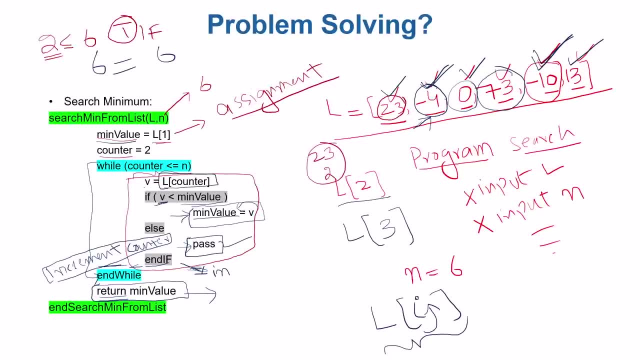 They become earlier than the Bigger values, and the problem is called sorting. So in the, in the next video, we are going to talk about one more problem, Very famous problem, called the sorting problem, And after that problem we will be going towards Python, because after that problem, 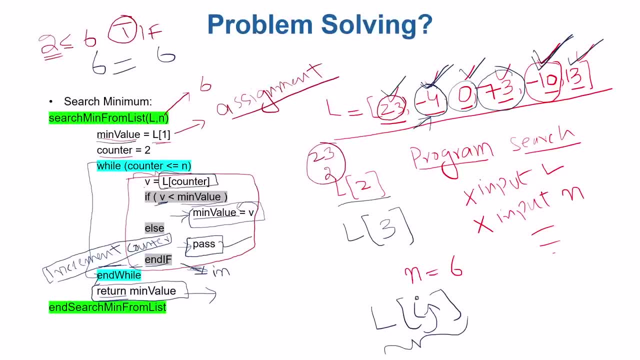 you'll be having a fairly good idea how to solve a problem, how to write a pseudocode for a problem, And the way we are writing the pseudocode is very close to the actual Python code, which will become so clear to you. So hope to see you in the next video. 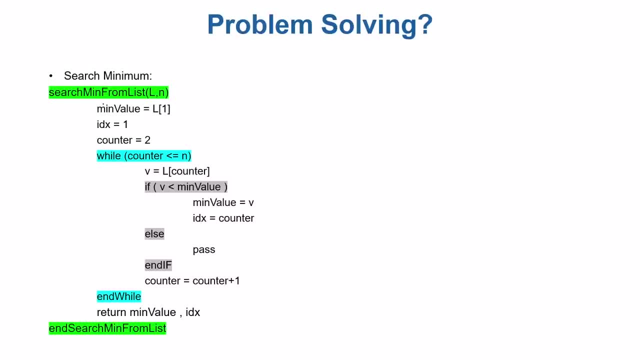 Okay, in the last video we talked about, we talked about this: how to find out the minimum value from a list of values- And we came up with an algorithm with name: search min from list. here We have just made a little modification that, rather than just returning the minimum value, 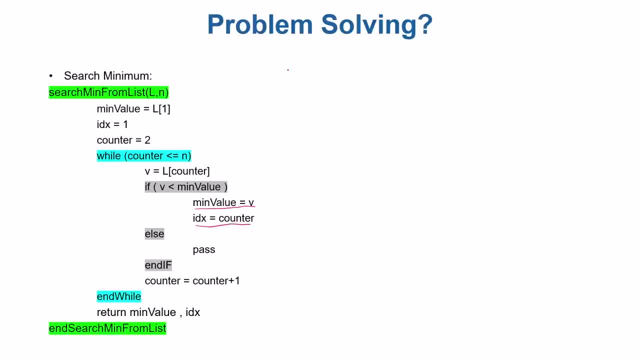 We are also returning the position of the minimum value in the list. So, for example, if the list is one, seven, zero, two, four, let's say in nine, let's say that's our list. There are seven numbers in the list. 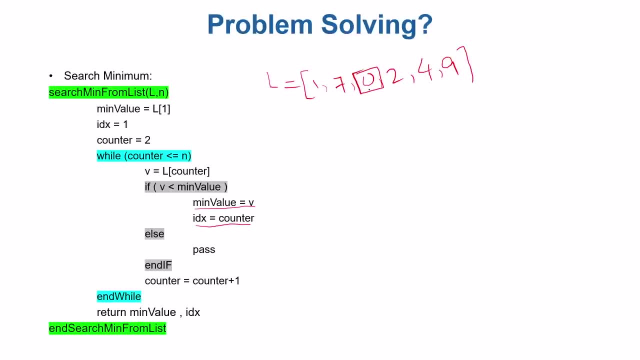 The minimum value is zero, So the value, the minimum value itself is zero, but that appears in position three. So when, when this procedure will end, the min value will contain zero and the IDX, which is the position At which the value, the minimum value, was achieved, that will contain three. 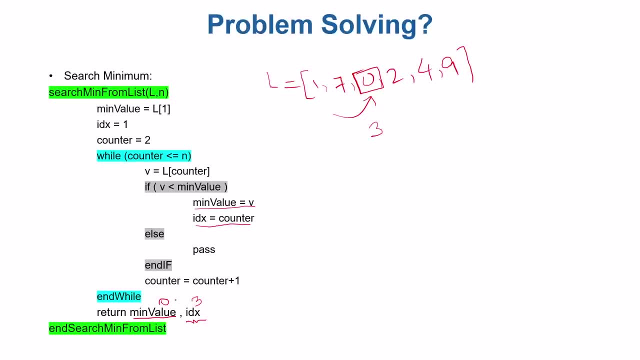 So not only we are, not only we are finding out the minimum value, but also we are finding out the position of the minimum value. This procedure, or a pseudocode, actually describes a very simple, very simple concept. You consider the very first value as a minimum value and the very first position as a position of the minimum value. 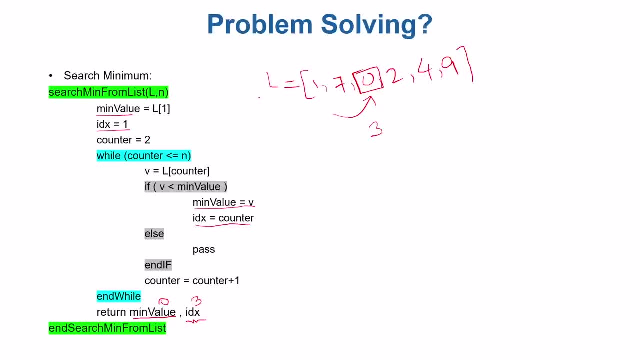 and then traverse the list element by element And and see if you find any value that is smaller than the minimum value So far. if that is found, then replace your minimum value with the new minimum value and update your position number and then keep on moving till the end of the list. 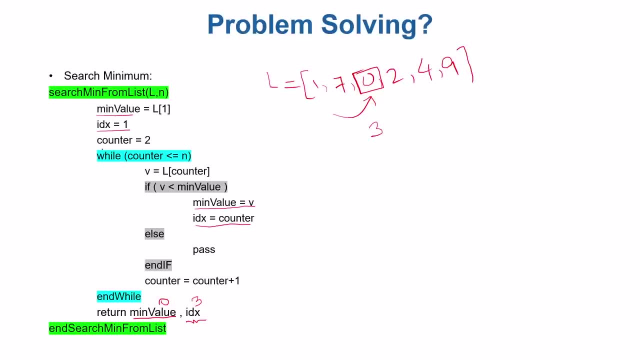 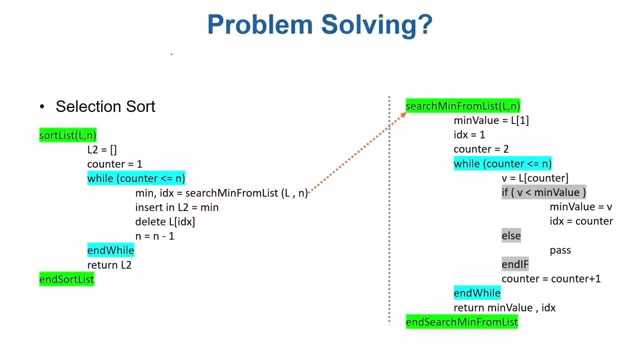 So so that's what that's the concept behind the, behind this algorithm searching minimum from the list and to traverse the list We use this loop while loop. So next we solve a problem called sorting problem, Very, very famous problem in computer science. So the problem really is: let's say we have a list, 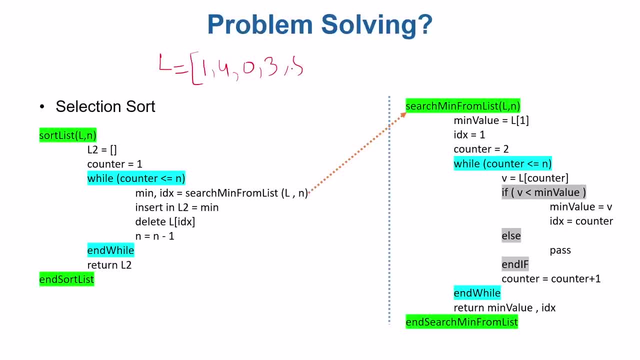 Let's say: one, four, zero, three, five and seven. Let's say: and the sorted order, the ascending sorted order is the order in which the list is presented, So that the minimum value occurs first, then the second minimum, then the third minimum, and so on. 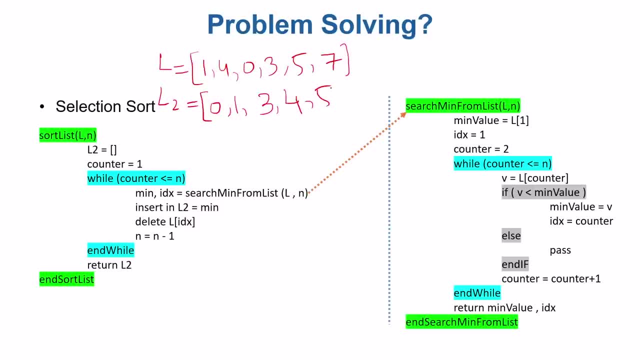 So the sorted order for this particular list will be this. So this is the result. This should be the result of the sorting procedure. So let's see how can we solve this problem. We name this algorithm as sort list, and sort list contains this L in this particular case. 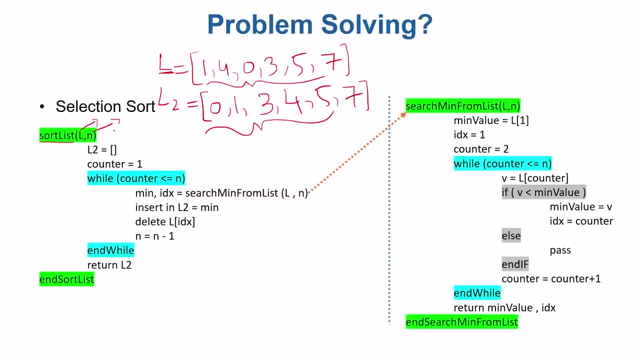 The L is simply this and this N is the size of the list. in this particular case, The size of the list is six. So six And right now L2 is empty. So, although we have to populate L2, but right now it is empty, and counter again: 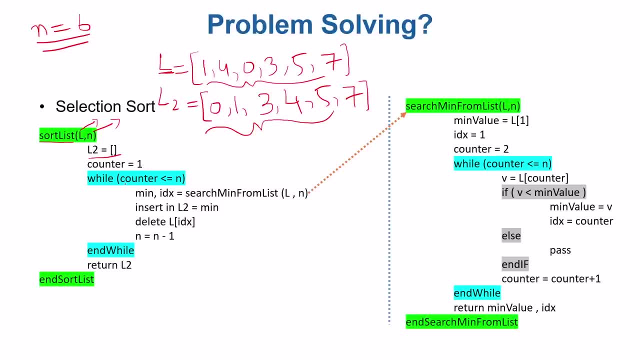 We initialize the counter with one and as as long as the counter is smaller than six, we keep on. we keep on moving inside this, this block, That's the, that's the body of the loop. So what we do is we pass the list and the size of the list. 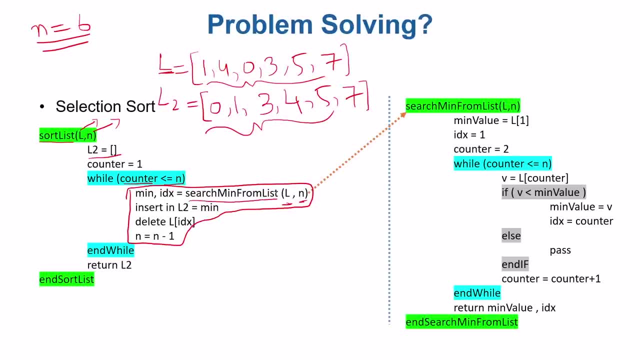 and we use the previous algorithm to find out the minimum from the list. So the minimum from the list will be found as zero and its position will be found as three. So min value will contain zero and IDX will contain three. Then what we do? we pick this minimum value and insert in L2.. 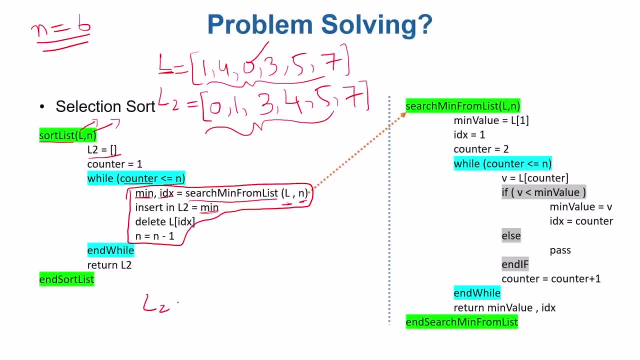 L2 was initially empty, So we insert in L2.. We insert the minimum value, which is zero so far, and then, just in the original list L, we delete The value at the position index. So, for example, the index position is three. 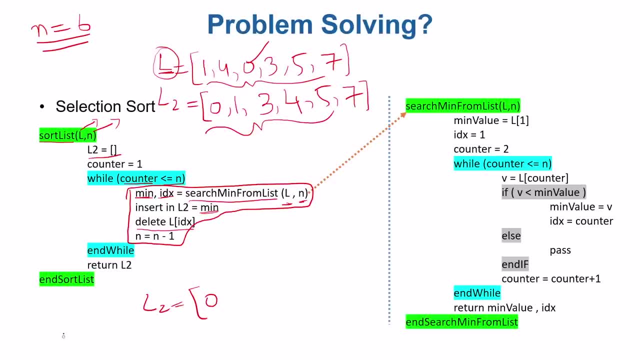 So we delete this particular value. So what we really do is we delete this value. We delete this particular value and the list now becomes with size one, two, three, four and five. So what we do is we decrement the size with with one and then we move on. 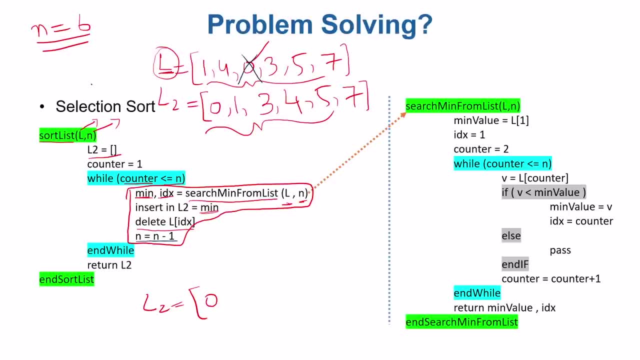 Now the counter is one again the end value, rather than six. Now the end value is five, So one is smaller than five. But the list has no zero now in it because it was deleted. We search the minimum again and we insert the minimum in the list. 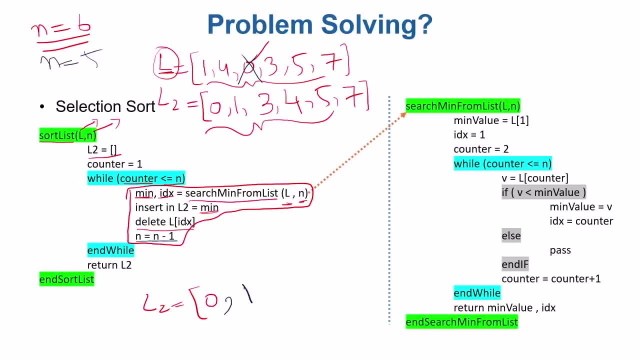 Now the minimum will be one in the new list and we delete that value from the list and we decrement the size. We keep on moving. Eventually, the list L2 will be populated like so, and once and once this value of n becomes negative, which is minus one. 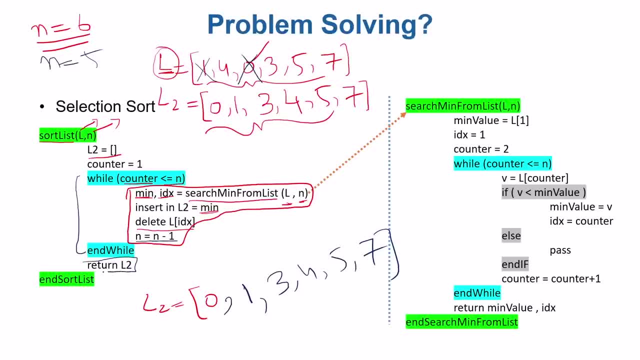 we will exit the loop and we will return The sorted list, but see how this sorting procedure actually uses the algorithm that we, that we defined in in our previous video. I'm not talking about that. This kind of sorting algorithm is the most famous sorting algorithm. 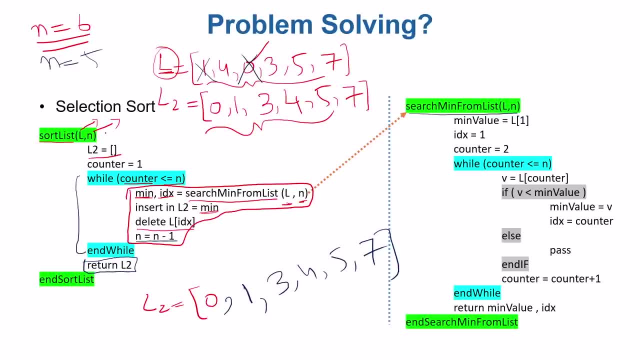 There are efficient algorithms, very great kind of algorithms for sorting, But the idea here is not to actually teach sorting. the idea here to actually come up with a pseudo code for this sorting problem and also to show you how you can use the pseudo code. 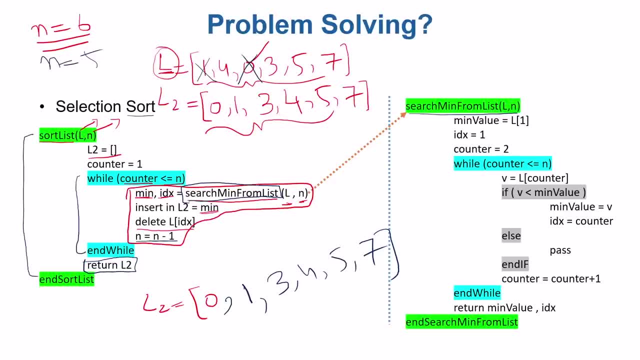 how you can use existing pseudo codes as instructions in other pseudo codes. So that's all about problem solving. If you really understand the selection sort and all that procedure really well, you're actually very good in problem solving, at least the problem solving that we encounter in the logic that we need to solve different kind of problems in computer science. 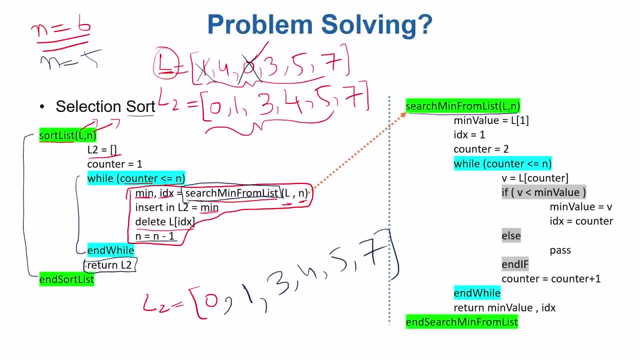 In the next video I'm going to actually convert these pseudo codes to Python codes. What do you need to do to write this sort list procedure in actual Python programming language And how will you change this search minimum from list in actual Python programming language? 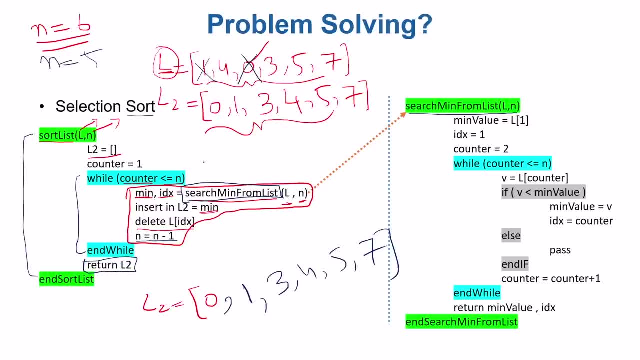 We will see the Python details bit by bit in detail, starting from right zero and ending at the very high details of Python. So in in the next video I will just be showing you how to convert this code, But when we will start learning Python? 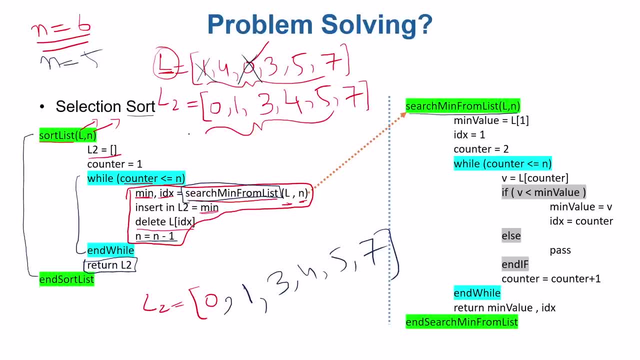 we will start from zero and we will see each and everything of of of Python in in in detail. So don't worry, in the next video, If you see I mean things like lengthy codes in a very beginning, These are just because we have arrived at a pseudo code. 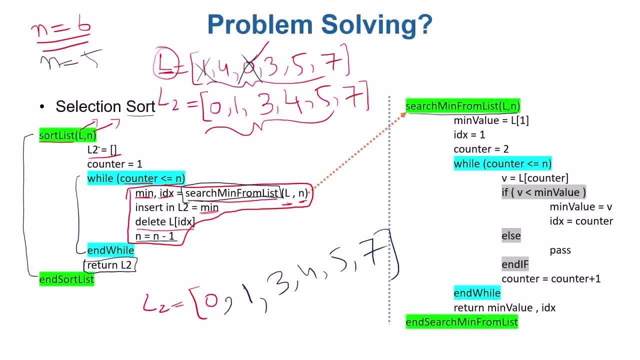 It is very. I'm just want to show you how the pseudo codes, which are very express, how they can be easily converted to Python programming, just to show you the power of and simplicity of Python programming language. So in the next video I'll be converting these pseudo codes to Python code. actual programming code. 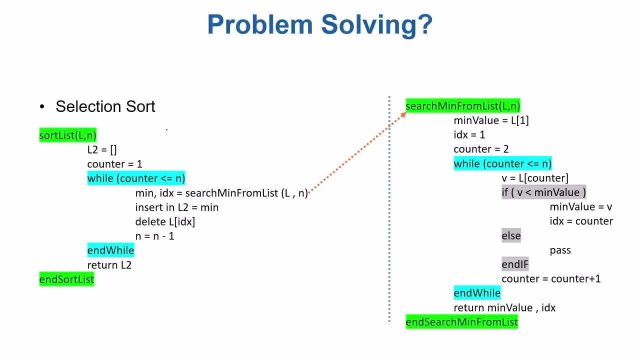 So hope to see you in the in the next video. Okay, in the previous video we just get a flavor of problem solving by using this selection, sort or the sorting procedure. The idea was just to use this procedure To solve this kind of problem and we saw in detail- not in that detail, just just brushed up. 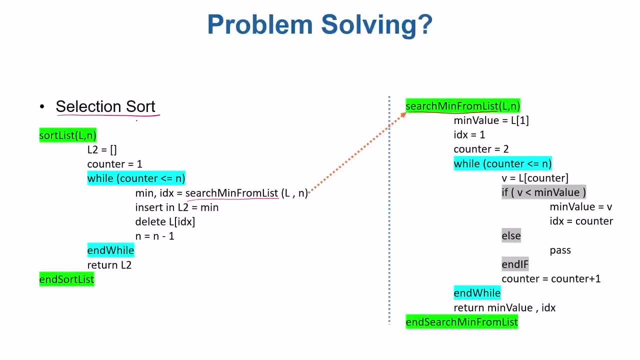 but we saw how to write a pseudo code for solving a problem of sorting which requires actually a list to be sorting in ascending order, For example in this video. I'm going to convert first this code: search minimum from list. You see that code. 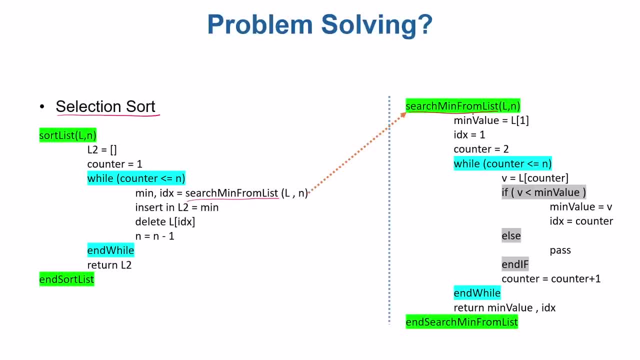 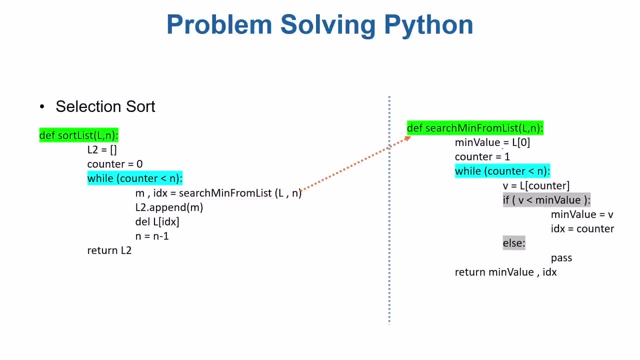 you know that code completely. We're first going to convert that code in Python code and then we will convert this code In Python code. So see step-by-step, what changes are there First of all in Python. that we will see in detail. when you define procedures, different kind of procedures. 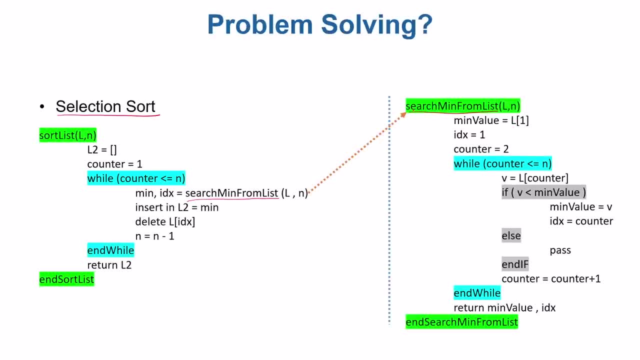 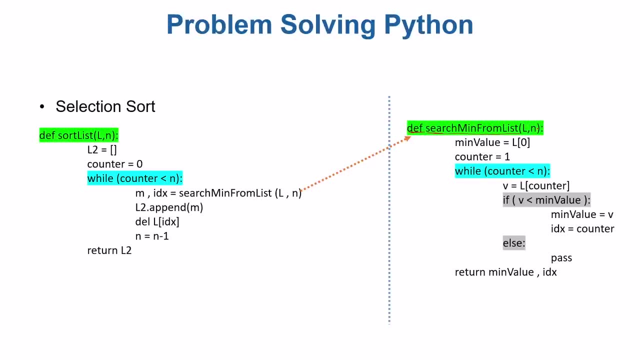 They are called functions in Python, and rather than writing this, we have to write a DEF statement before it, and then whatever name you want to write out, the rest of the thing stays the same, except at the very end We have to write a colon. That's the syntax of Python. 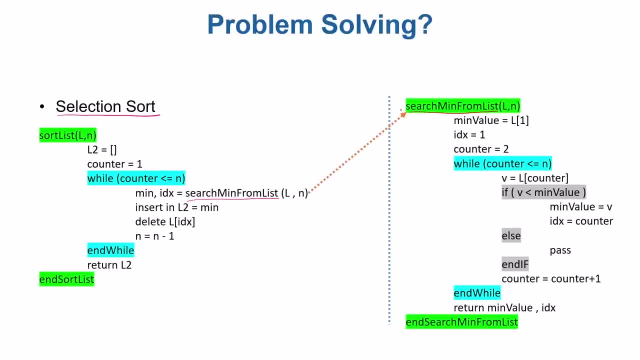 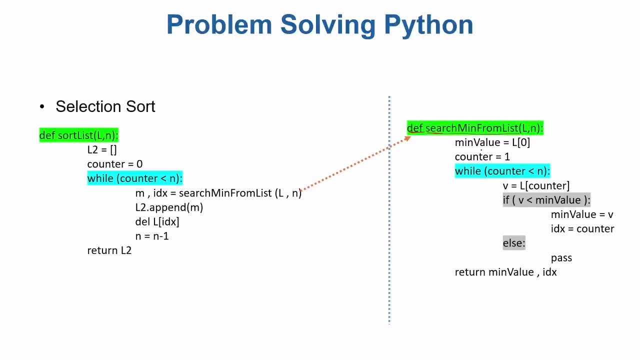 So the changes from here To here is a DEF statement which defines that is used for defining, DEF, for define, And then at the end we write a colon. next thing that we will see in detail, Don't worry if you, if you're, if you just see that why we are messing up with lists. 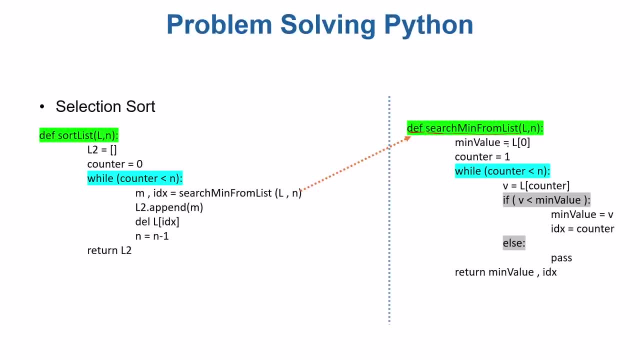 So early. we will see that things in detail. but just to compare the. in pseudo code Normally the lists are indexed, the indexes of the list They start from one. but in Python, the programming language, the first index of the list usually starts from zero. 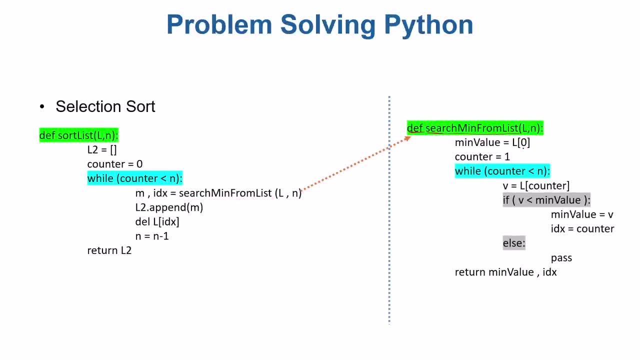 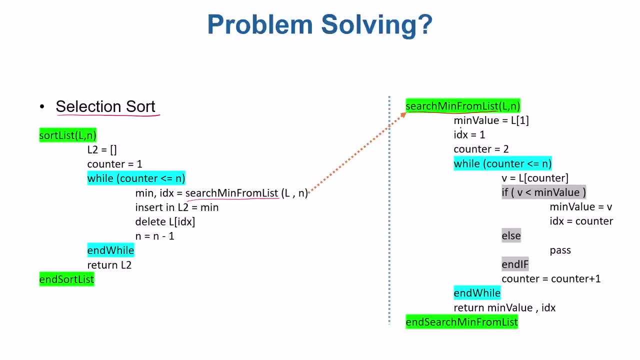 So there, the minimum value was the first value of the list. here The first value is actually the index. in Python is zero. rest of the things are same. You declare the variable as in pseudo code. The same goes exactly in Python. there the because the index was one. 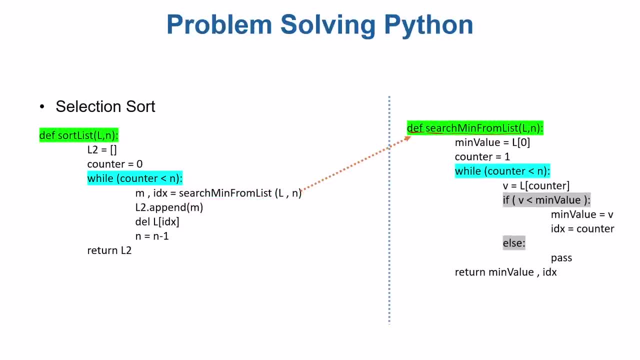 And so the counter was one more than whatever the index was. here The counter is simply One. we need to write here: IDX. IDX equals to zero. that we just missed in the previous. the IDX is one, So here the IDX is zero. That's okay. 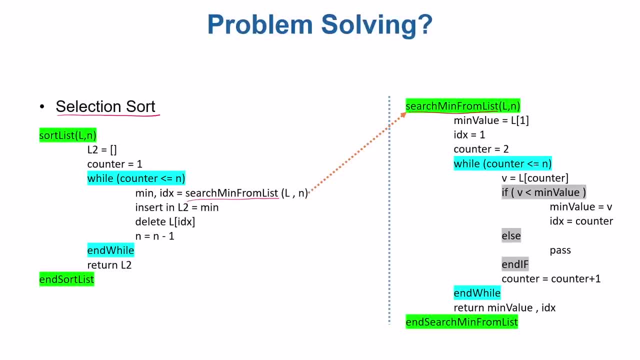 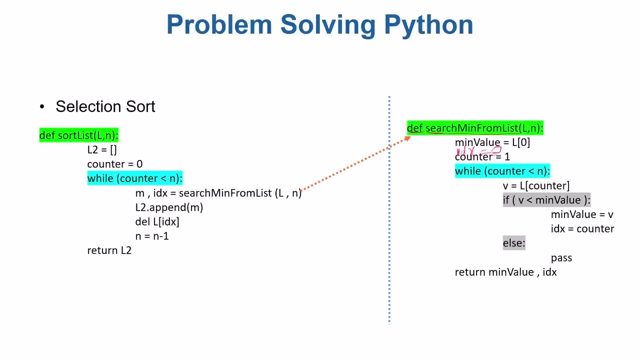 Okay, then next we write: while counter is lesser, equal to n, same thing, while counter is less or equal to n here. So here we just write the, the colon. at the end We might have written This equal sign here. this equal sign We have. we just missed the equal sign. 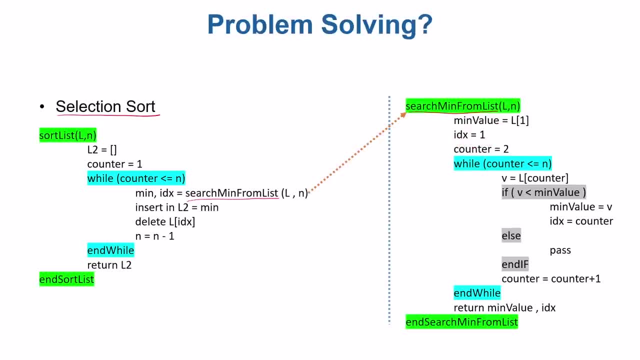 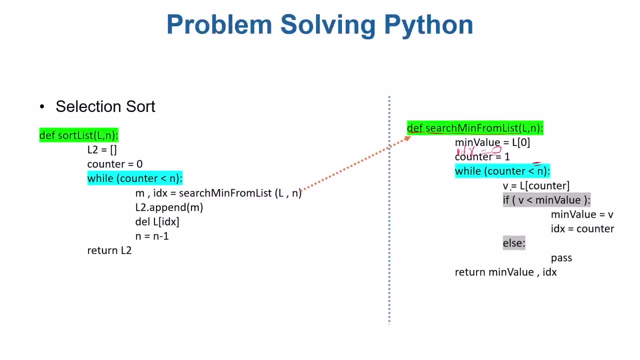 The equal sign is there. So now, but see the see the difference here. The violet goes that way. here We have a colon at the end. rest of the things are exactly the same. Now. V is equal to L counter. V is equal to L counter- the same thing. 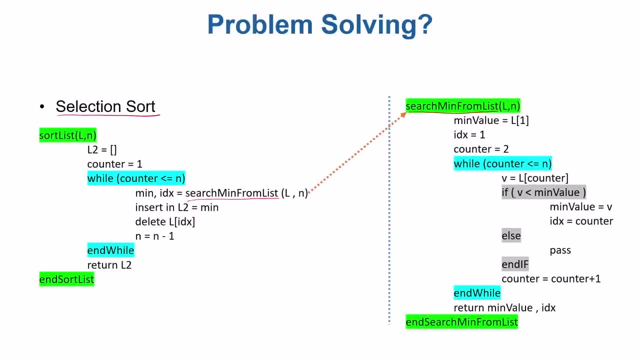 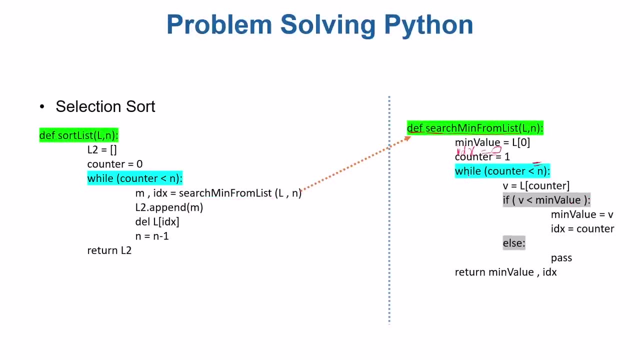 If V is less than the minimum value, the same thing If V is less than the minimum value in the pseudocode python is exactly the same. Just See the colon at the end. We have colon at the end of the while statement. We have colon at the end of the definition. 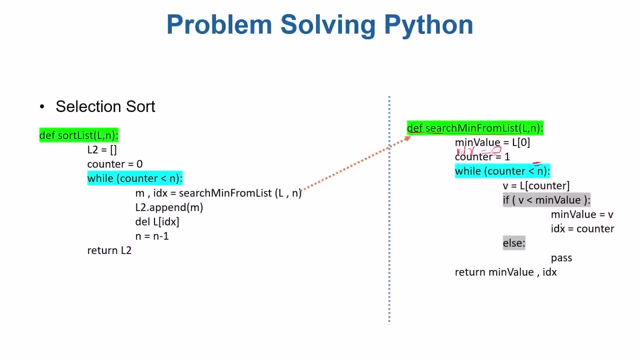 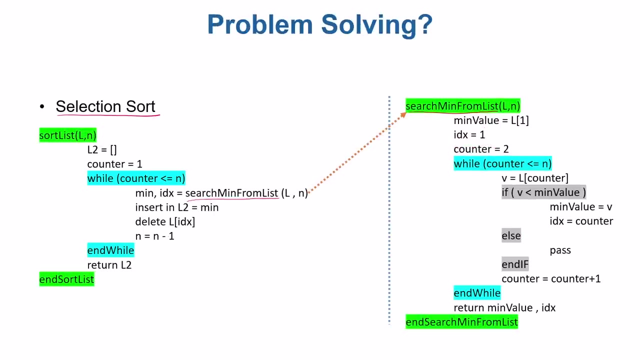 We have colon at the end of the if statement. the other statement in pseudocode in python: exactly same. now in pseudocode We have L statement. in python We have L statement. If you want to write an L statement, we have to write a colon at the end of that. then in python, in pseudocode, 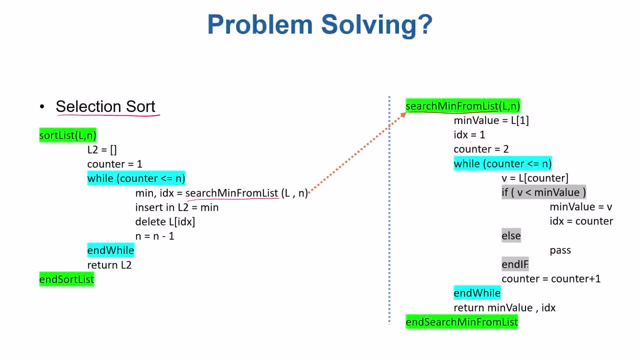 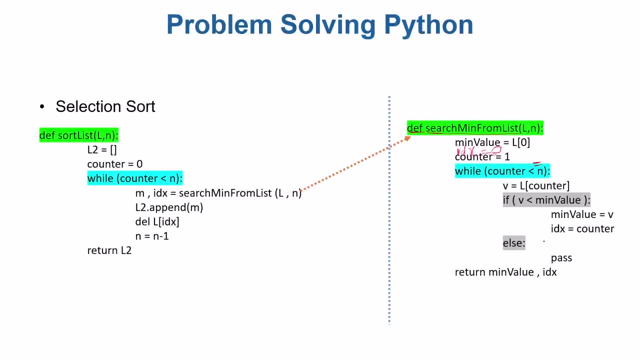 We have a pass statement, python. We have a pass statement. same things in pseudocode. We have end if, just to describe that this F ends in python. Everything is described by the indentation style. So if this indentation goes on, if we, if you're here, 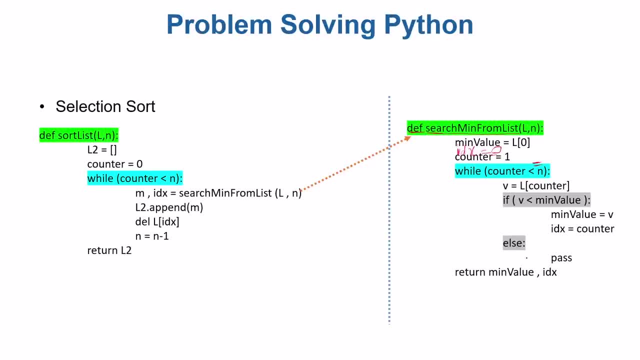 then this if is goes, if this if goes out, so we need not write ends everywhere. Similarly, the vile body has this indentation style: This is all the vile body. whatever that is that is earlier than this is not in the vile body. So, rather than writing the tokens and while and if, the python handles everything using indentation. 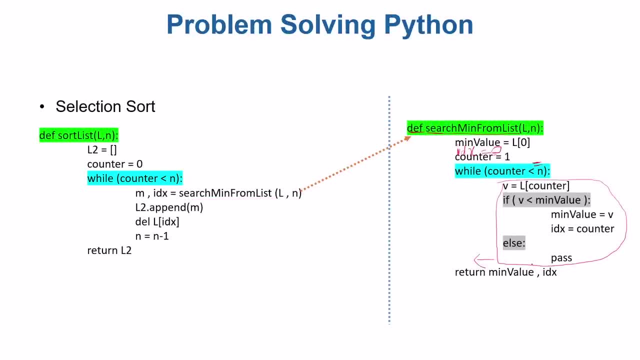 so no need of and if no need of and while: Oh, we haven't tried, We haven't written a counter here, So we have to write a counter plus plus here, So counter, so the same statement. we missed this statement in the python code. 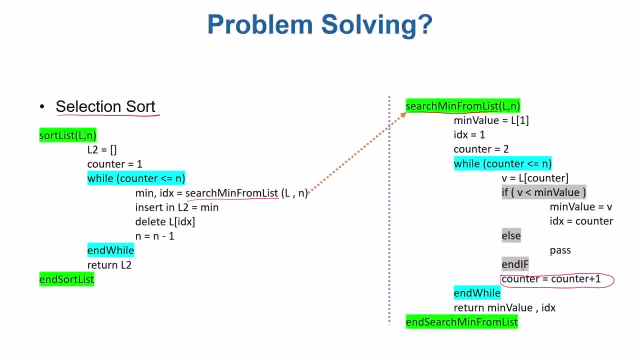 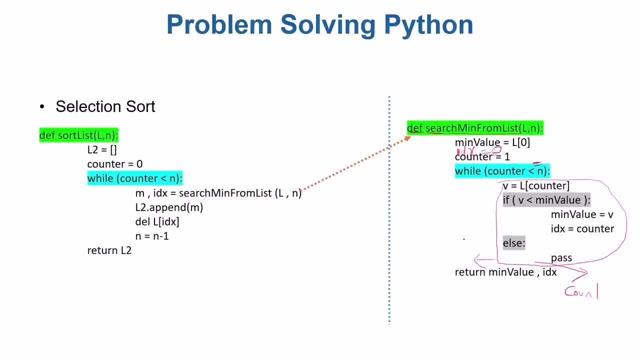 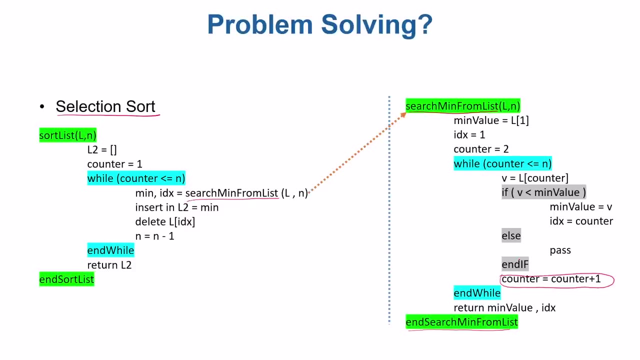 So the same statement, exactly the same statement, goes here. That's it. The rest of the story is same. We do not need an end. So let's go back to the language here. The goal here is to show that the pseudocode is. I mean the way you write the pseudocodes. 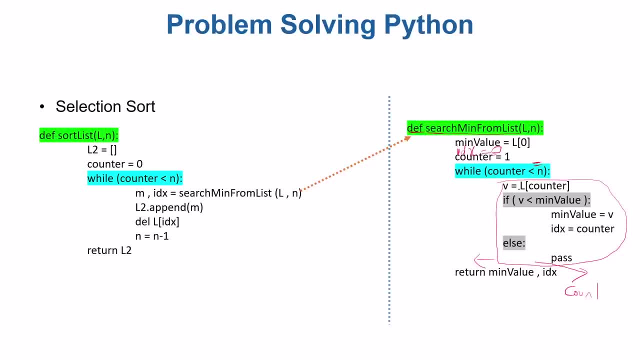 They are. they are highly, they highly resemble with the actual code in python. python is that expressive python is very, very high level language. I mean the way the you, the way you think the problem in the pseudocode, the actual python code, is much similar to it. 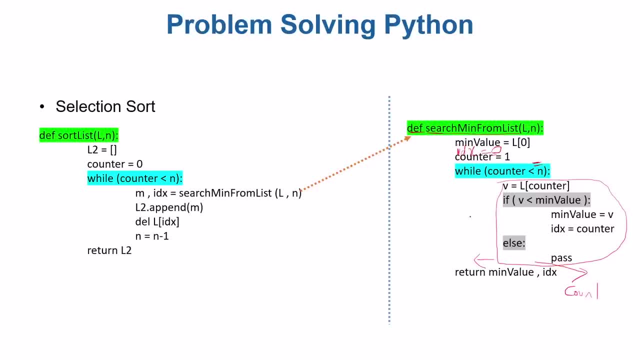 I mean the way the you, the way the code is. the Python is very, very simple. the simplicity of python is really a great property of python and that's one big reason of popularity of of python. Rather, return statement is same and everything is same. 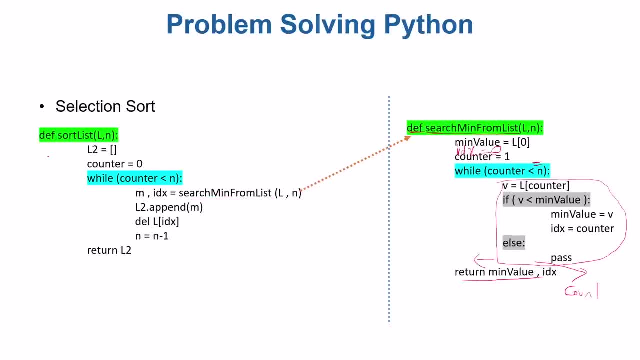 Then we move toward the sorting again. We have sortlist, We have to drive the define, def define, and then we have this colon out there. We have to write the colon there. Then list 2 is defined like empty. It's empty in python as well. 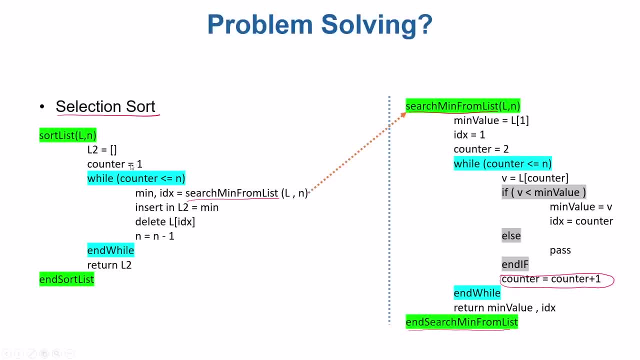 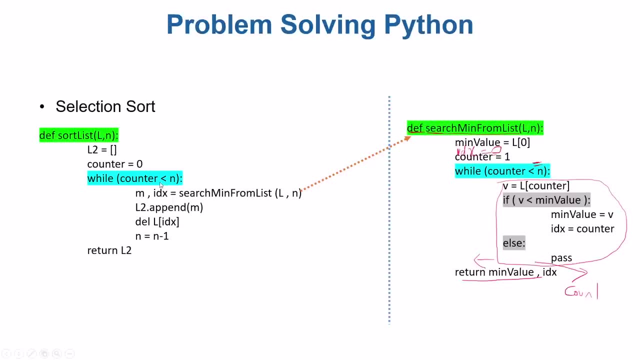 counter starts from 0, because there the list starts from index 1.. In Python the list starts from 0, so we write 0.. While same as this one. here we have this colon: maybe an equal sign. maybe an equal sign should appear here. I guess we are missing an equal sign, But 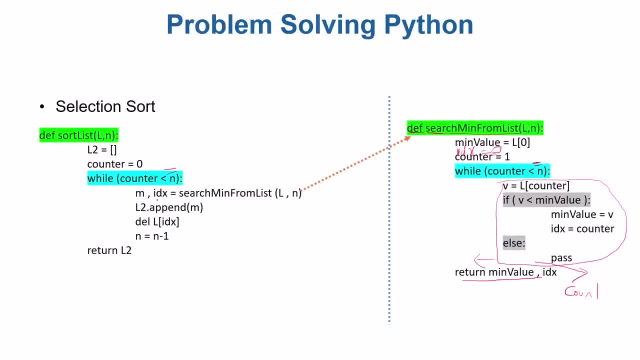 either way, the code is more or less the same. Rest this statement, exactly same as this statement We have insert in L2.. Here we write: append- append function- I'm in Python. Here we write: delete this. In Python, we have a del statement. Rest of the story is exactly. 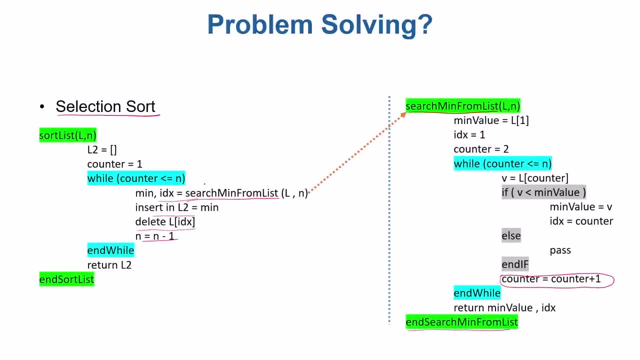 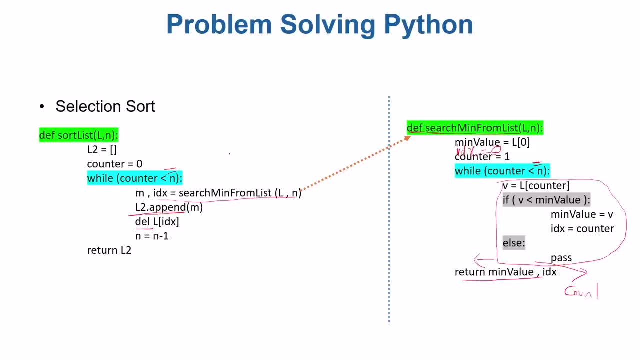 same. So you see, converting pseudocode to Python code is way more easier. This is not a formal introduction to Python. I mean, the goal here in this video, in these kind of session of videos, is just to introduce you with problem solving. But I found this beneficial. 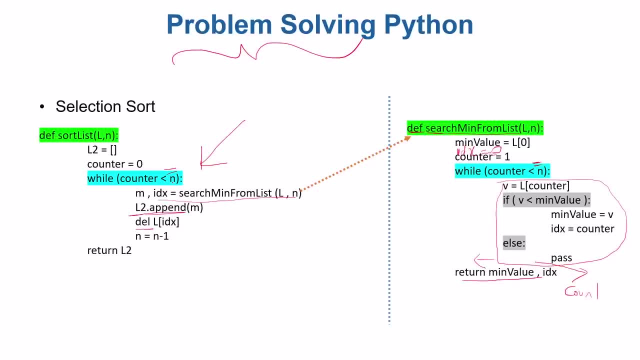 to show you that the pseudocode actually resembles to the actual Python code a lot, Although we will be dealing with variables, lists, while loops, if conditions, all these kind of stuff in a big and huge detail when we, in the upcoming videos, when we will introduce 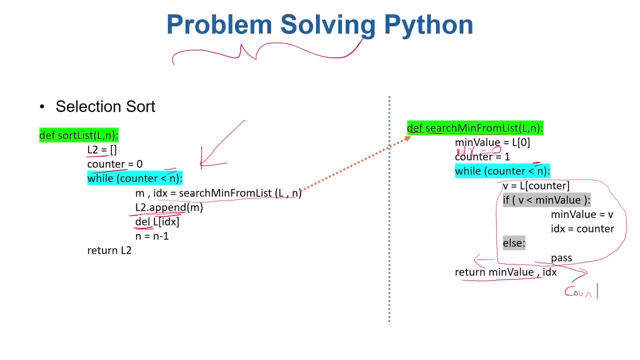 the Python syntax and variables and all that kind of stuff. Actually, you will be mastering each and everything in Python And further. you need not write these lengthy codes to do stuff in Python. I mean the whole that thing is just you write L, dot, sort and 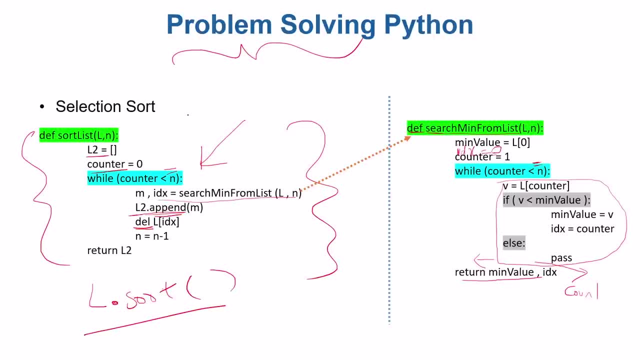 you are done. I mean, you need not write a lot of lines of codes in Python Here. I just showed you that if you have a procedure, you can. If you have a pseudocode, it's going to look like this: It looks like much like the same as Python, which actually tells you. 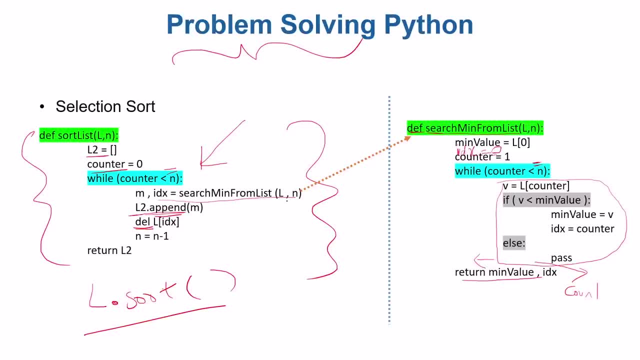 the expressive power of Python and simplicity of Python and how it is closer to what you think. But the actual problem solving in Python does not require so many lines of codes. I mean, there are so many functions, so many powerful procedures for those. you just write one line and a huge amount of work is done for you. 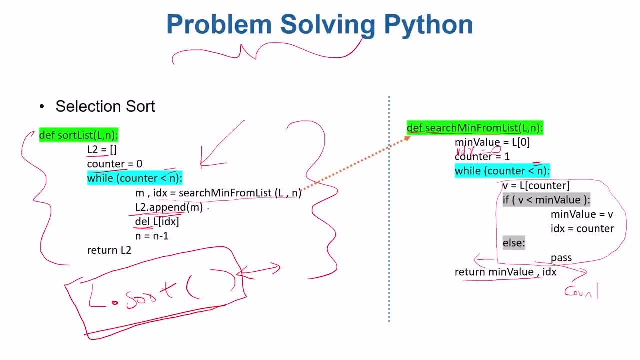 And there are very good one liners for Python. I mean for programming in Python. you need not to write a lot of lines of code to do some stuff. I mean a few lines of code. even a single line of code does a lot for you, And for that you need to know the features. 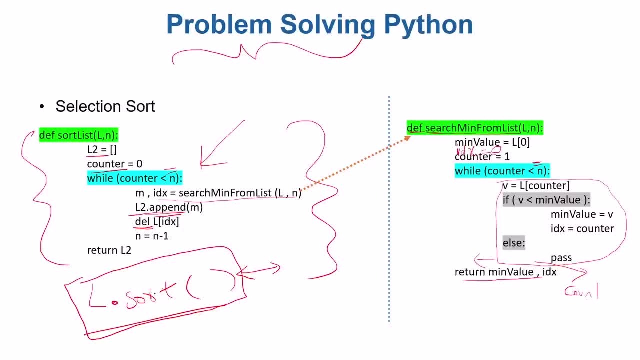 of Python, the feature of the features and the different kinds of syntax and features and libraries and the packages and what is available with Python. I tell you almost each thing is available, Just you need to know what is available Once you know what are. 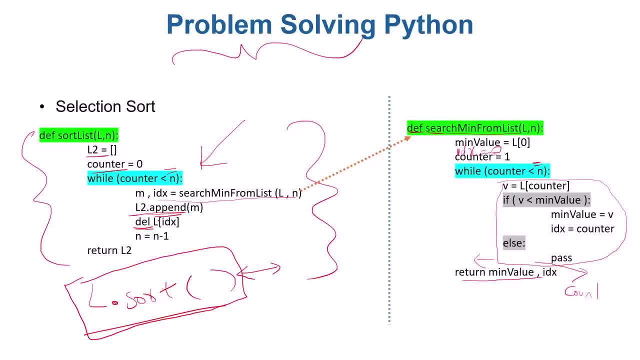 the things that are available. you need not to write lengthy codes, You need not to build a lot of logic on yourself. Things are prepared, They're waiting for you, You just have to figure them out. What are these things to do? What kind of features are there in Python? 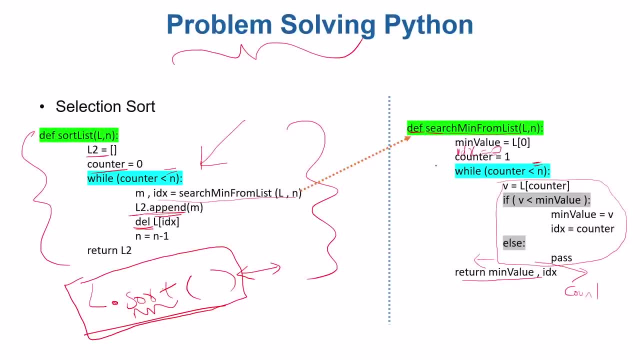 If you know that you are done, So you need not to be writing these kinds of codes and lengthy kinds of codes- although knowing that is, at a high level, A huge advantage- But doing a bigger and bigger and bigger stuff. Python will give you a lot. 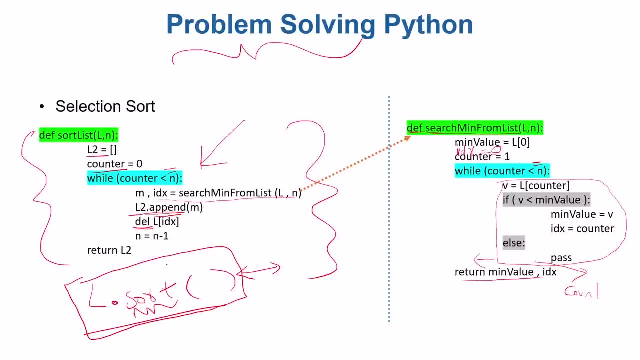 of features, a lot of functionality that you need not to go into and you need not to write a lot of code for it. And that's the second power of Python. One is simplicity. Second, it gives you a lot of features, a lot of functionality, a lot of built-in stuff ready for you. You 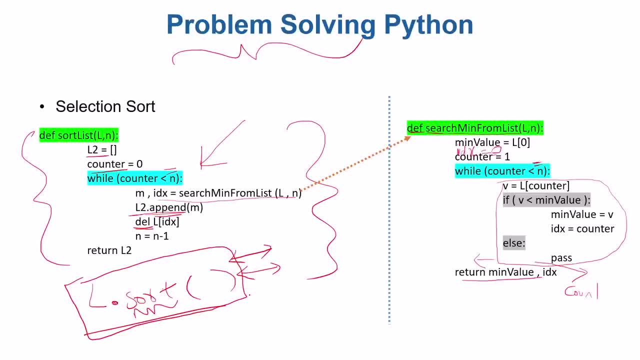 want to do something, it will be probably there. in Python, You need to know where you are, where it is, And for that we have a whole future series on Python: to know Python, each and every step in Python, and to know important packages in Python, Because knowing 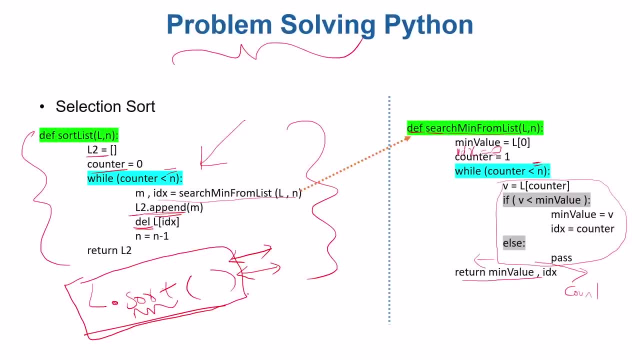 important packages and knowing how to code in Python will save a lot of time for you. So spending some time on learning Python will be saving a lot of your time to solve the actual pure problem- whatever problems you're going to solve- And Python is a real programming. 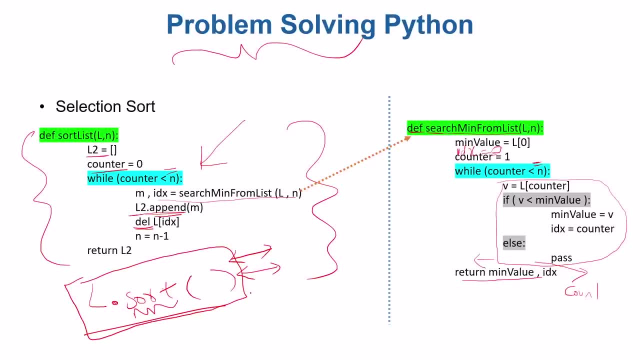 language, Stranding programming language. Knowing this language is almost enough, So hope to see you in the next videos, where we will start Python from exactly zero and we will see each and everything of Python in detail. Hope to see you in the next video. 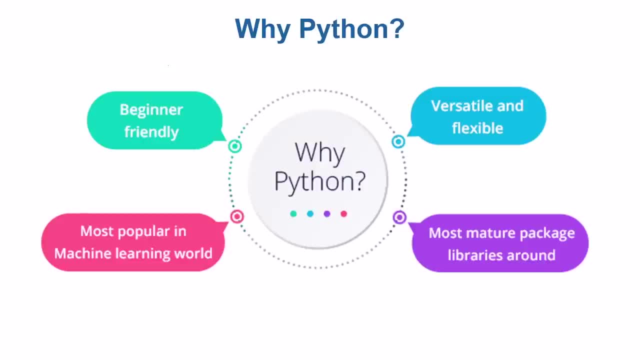 If you're new to data science, you may stuck in choosing the best language for data science, And in this video I'm going to talk about Python, Which is the greatest language so far for data science. To explain the features of Python, let me first go back to a little bit history of Python. 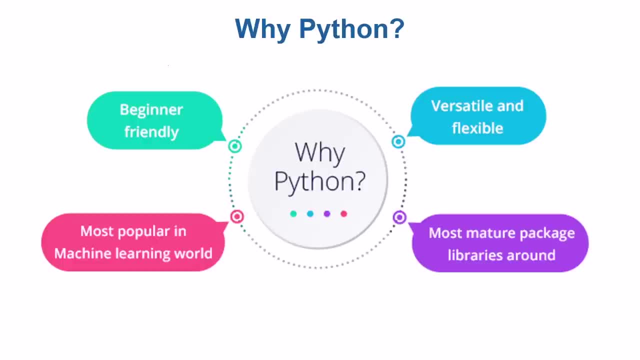 from where it started. It basically starts in 1980s. It was introduced first in 1980s, But with constant improvements and a lot of bug fixes. it was officially launched in 1989, nine years later. 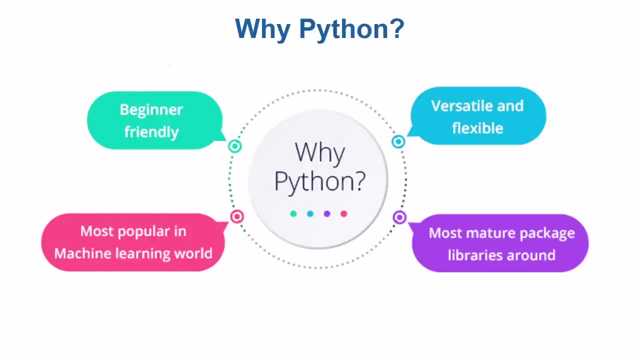 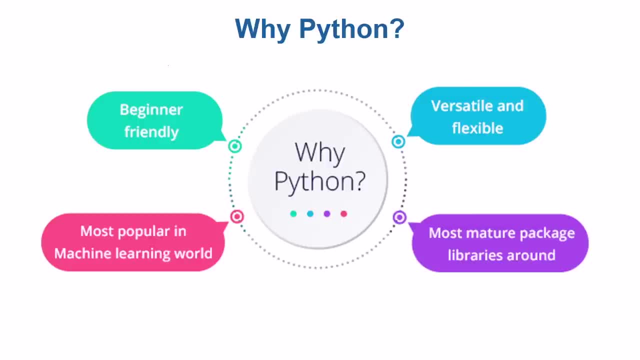 the same task. as compared to other programming languages, It is flexible, portable and can run on any platform easily. It is scalable and can be integrated with other third-party software easily. Python programming is easy to use and has a simple and fast learning curve. New data: 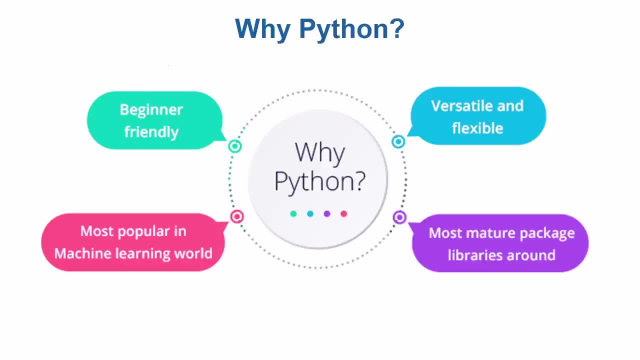 scientists can easily understand Python with its easy-to-use syntax and better readability. So that's what this point is Basically. it's really a beginner-friendly. If you're new to programming, well, Python offers you a very easy environment to go on. It also provides 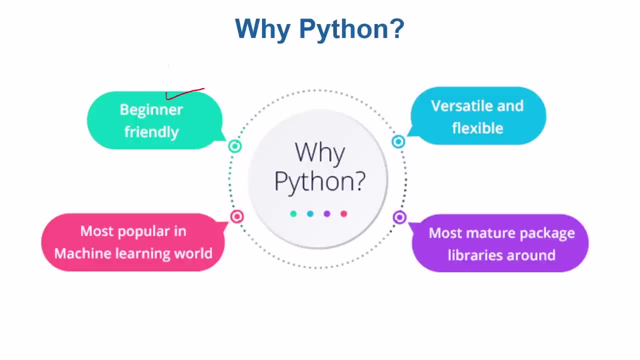 plenty of data processing tools that help in better handling the data. Python is important for data scientists because it provides a vast variety of applications used in data science. It also provides more flexibility in the field of machine learning and deep learning. It has a lot of packages like TensorFlow. 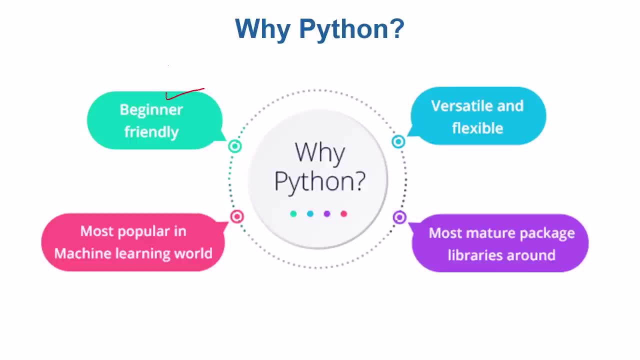 Keras and Theano. that is helping data scientists to develop specifically the trending deep learning algorithms very, very quickly. So basically, the sport of machine learning and deep learning is huge. in Python, Thank you, That's huge, As is the case with many other programming languages, it's the available. 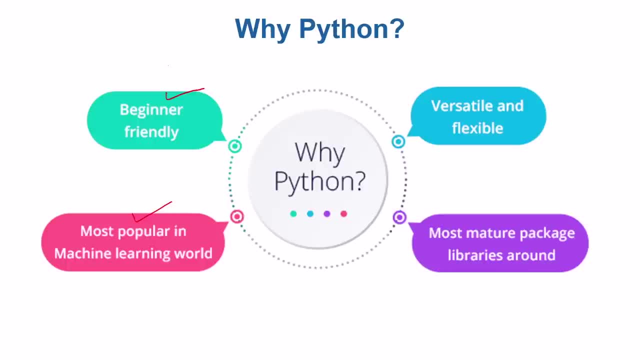 libraries that lead to Python success. Around 72,000 available packages in Python package index, sometimes called PyPy Python, P-Y, Python package index, PyPy. Around 72,000 packages are available and they are growing constantly, So a huge number of packages, mature packages, are available. It is free. 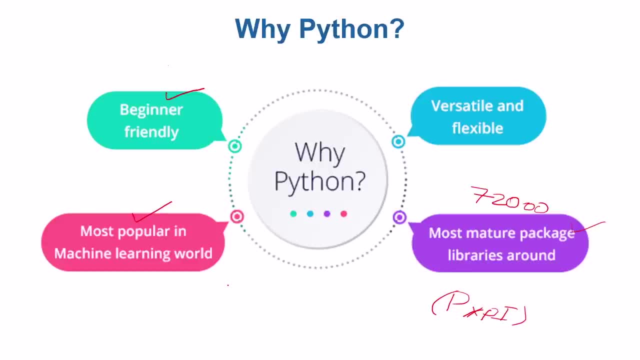 open source and consequently anyone can write a library package to extend its functionality. Data science has become an early beneficiary of these, particularly pandas, high in the open source, and consequently anyone can write a library package to extend its functionality. Data science has become an early beneficiary of these, particularly pandas or the P services. in particular, the Nutrient Phones. What is the benefit of using data science? What is the benefit of using data science as a tool? There are various ways of using them and there is one important aspect, one important aspect that I would like to highlight. If you have done research on the data science program in the past, 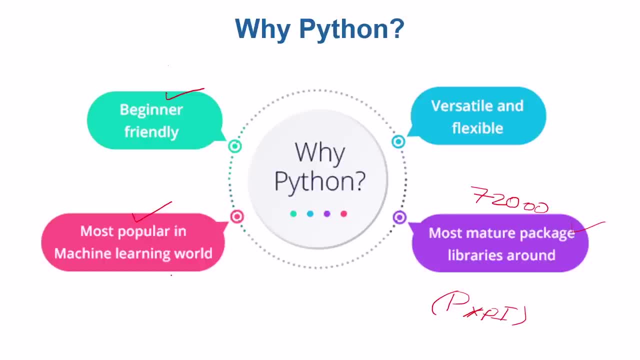 particularly pandas, the big daddy of all of them. the other great thing about python is there are millions of users who are happy to offer advice or suggestions. when you get stuck in something, chances are someone else has been stuck there first. so a lot of community is there? a lot. 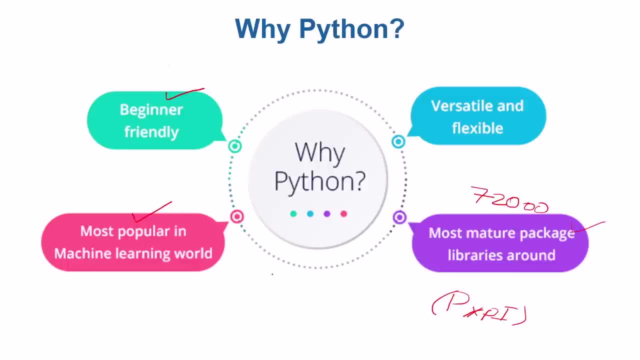 of packages are there. it's open source, it's easy to use, it's easy to learn, it's simple, it's readable, more close to human language. it's high level language. you code less, you do more. i mean you write a very few lines of codes and you achieve a lot of work. um, so i mean i've spoken a lot of. 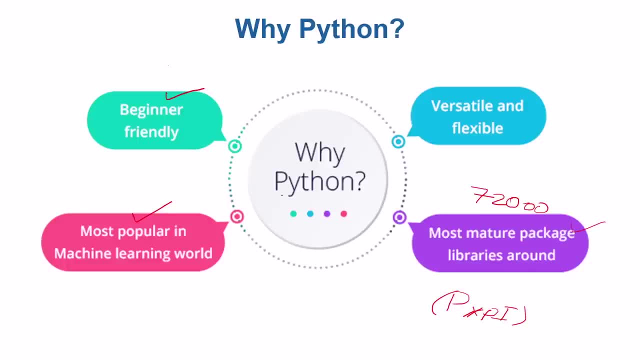 words here, um to to. i mean explain that python really is best suited language for data science. but let me let me introduce you some statistics about python: the popularity of python with respect to um, with respect to its use and with respect to the job opportunities that are there. 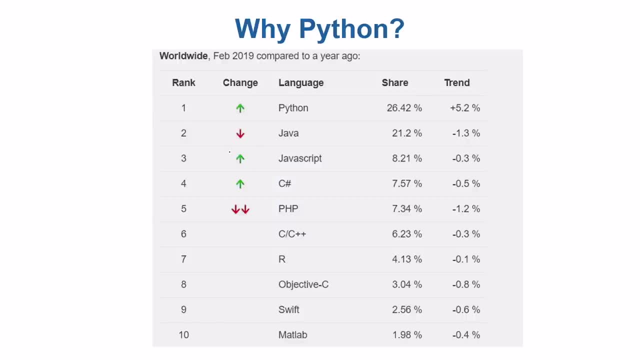 in python. so, for example, if you see this chart in the ranking of top 10 languages, python stays at the top. so that's the latest statistic collected in 2019, february 2019.. um, and out of the out of the total share of the languages, i mean around 26 just goes for python. 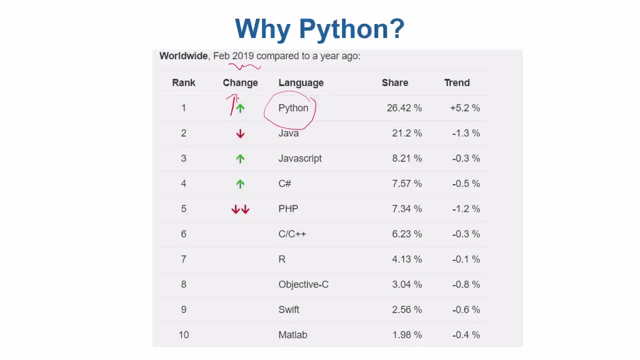 and the trend is moving up, which means people are more interested in python. i mean the trend of using python is getting larger and larger as compared to several other languages like java, javascript, c, sharp, php, c, r, objective c, swift and matlab. i mean many of them are used for. 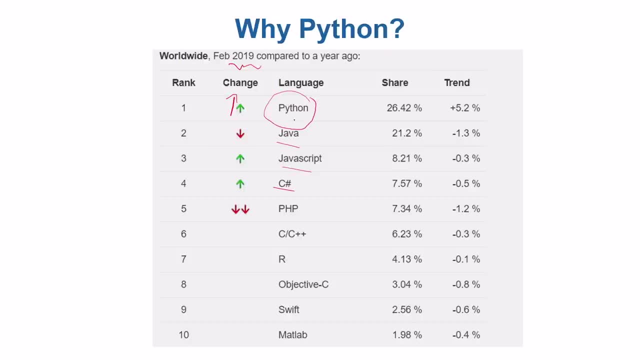 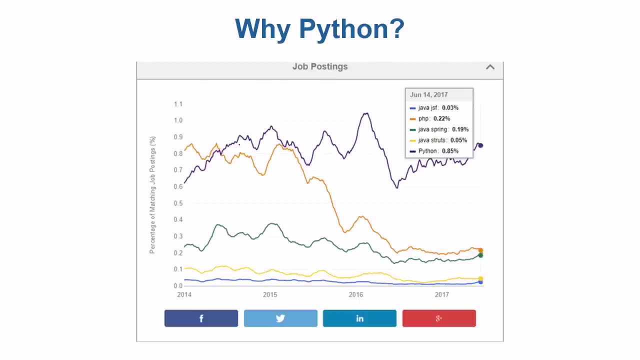 data science, but python stays at the top. i mean this is that popular language, um, and and further if. if you see, for example, the uh job opportunities, uh in in python, so so that says i'm in different companies like facebook, tutor and, and and i'm in google and. 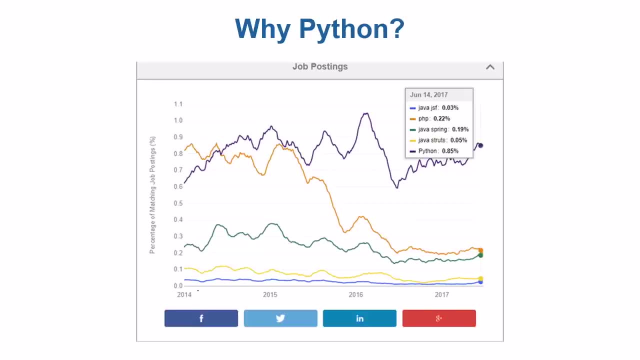 several different companies. um, this, this actually graph shows, uh, from 2014 onwards, that the job opportunities and job postings are in different languages, are at what amount? and you can see the graph of python, although starting a bit low but then stays up and stays up, which means the 80, if you see the numbers, 85 percent of the total jobs. 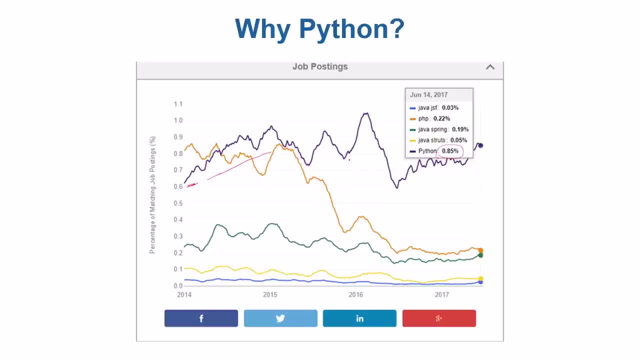 they're just for python and not only i. i mean, python is not just for data science, it's a general purpose programming language. it's open source, it, it can be um, it can be used to perform any kind of task for embedded programming, for, for, for posting, i mean codes or embedding code. 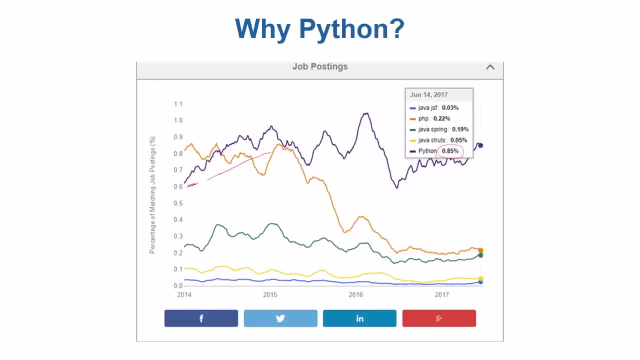 on raspberry pi for web development and whatnot. you can, you can. you can do the desktop development on it. you can use the web development on it, you can use the data science. i mean, i mean, this is general purpose programming language. in other disciplines too, it is performing. 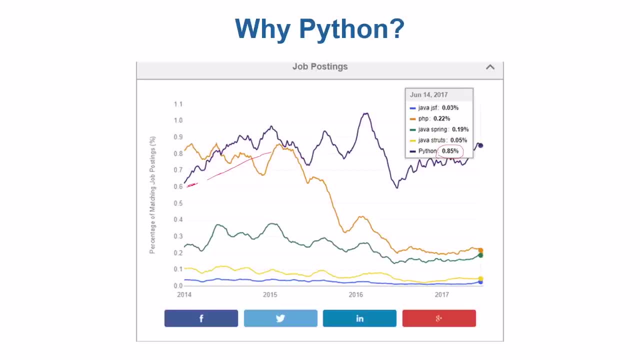 very well, but data science, for data science, it is almost the default language today. um, so, um, i mean, if you're going to learn data science, really, um, we need python. i mean, python really is the choice, the default choice, and we need it and in this particular course, we are going. 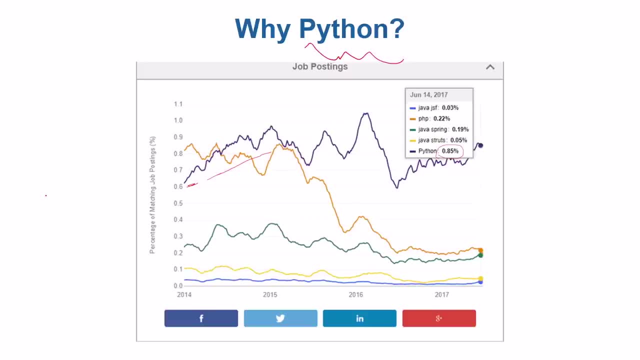 to um. we are going to introduce python to you with all aspects. i mean we will start from the very beginning level and we will gradually move towards um, the very advanced programming in python, including the introduction to the data science packages like pandas and matplotlib for visualizations and numpy for 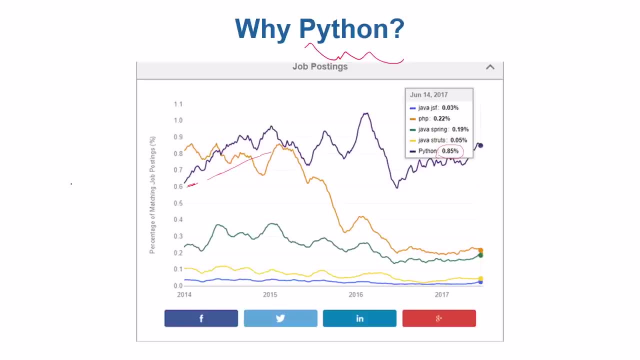 handling numeric data and stuff like so. so, um, in in this particular course, we are really going to teach you python and we are not assuming you have any programming experience before. so, uh, and, and this is one plus of python, i mean, whether you're in java or you're in java, you're going to have 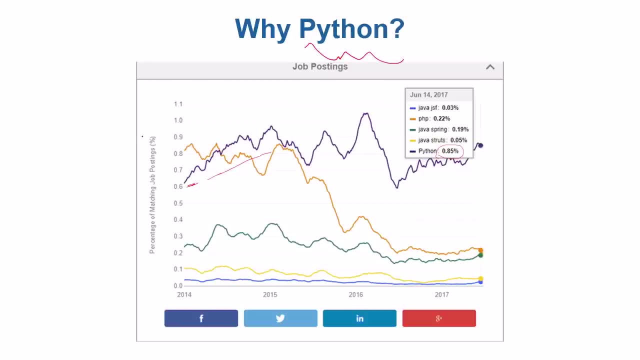 to be an engineer. you're coming from health sciences, you're coming from biology, you're coming from arts, humanities or from wherever. python is something that is very easy to get hands on. so, um, if you're not assuming that you have any programming background, you have any data science. 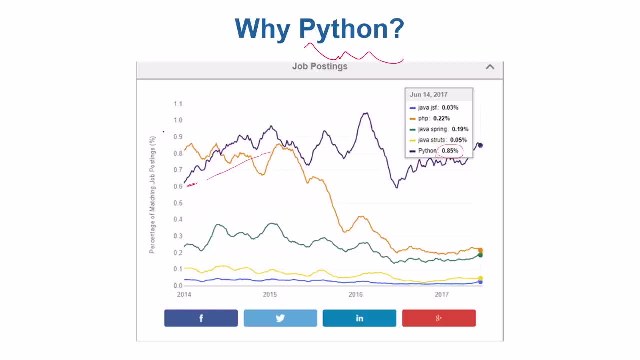 background: nothing. so we will start from the zero and we will gradually move to 200. so, uh, and including the introduction to the data science packages. so, um, python is the best. it is a default if you're going to work in data science. python is the default. 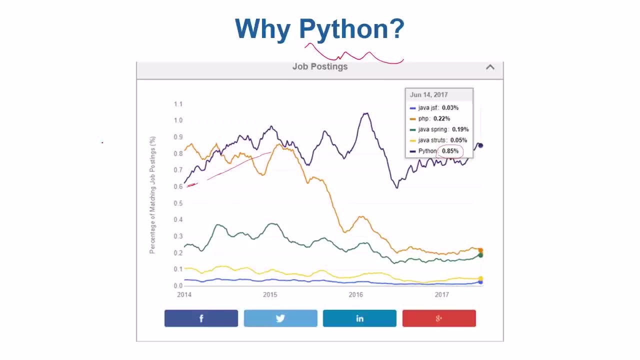 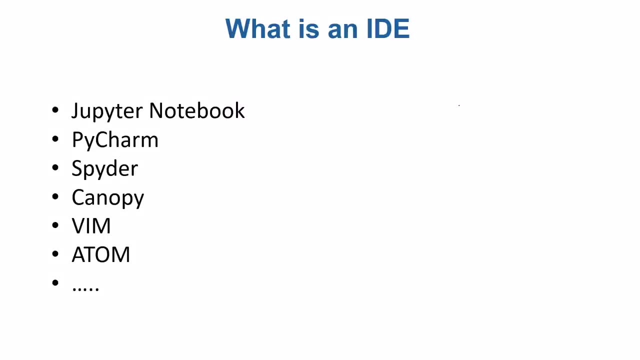 and we are going to. we are going to introduce you python from the very beginning to the very professional, so hope to see you in this course. okay, before actually discussing the best ide for python, and particularly for data science, let's first discuss what an ide is, how an ide works and how an ide is expressed, and what is an ide for the footer or an ide? 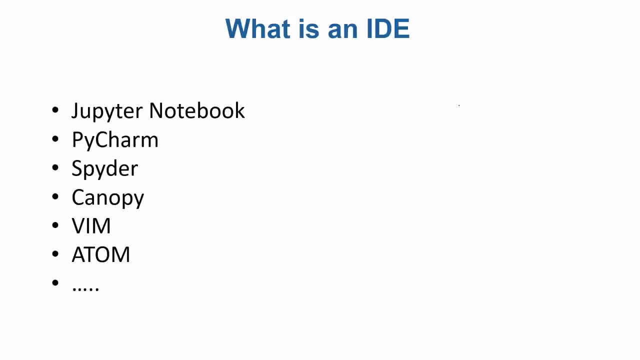 as you start your coding journey. many of you prefer coding in a text editor, maybe like notepad plus plus, where you write the code and then open a terminal window to execute your code. when there is an error detected in your code, you switch back to the text editor. correct? 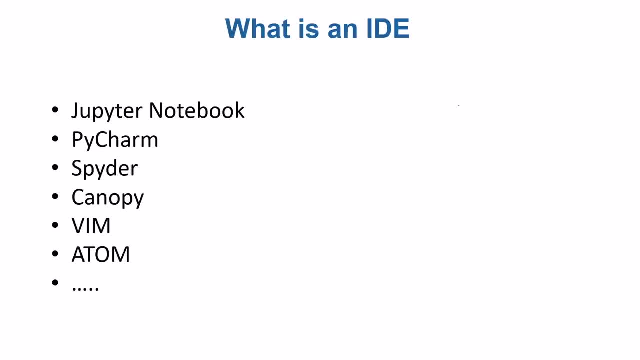 your errors, typos and run the code again in the terminal. everything is fine, typically for large scenarios, which means you also need a testing module. many times you have multiple coding and testing files, and switching between editor and terminal often becomes both confusing and inefficient, so an environment is needed. 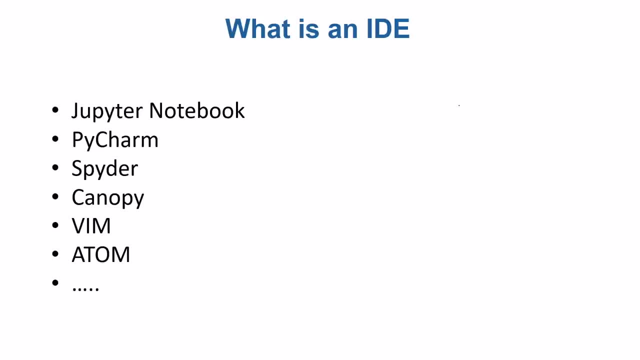 where you can write, you can run and play with your code all at one place. so the one that provides you with the capability of not just coding, not just writing the code, but but also testing your code: running your code, highlighting your syntax bracket, matching Auto completion, debugging your code code. 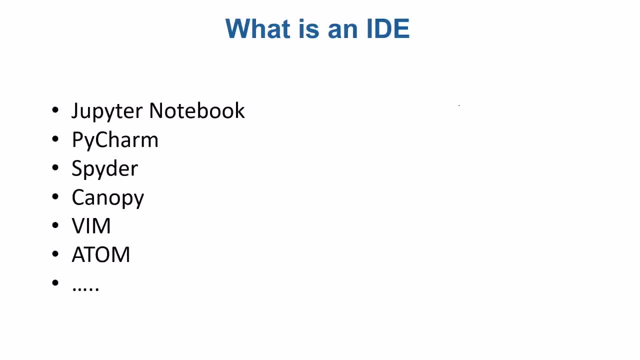 suggestions and and many more features. that is called an ID e or integrated development environment. now there are several I, D e E for different languages. For Python there are several IDEs. For example, Jupyter Notebook is an IDE, PyCharm is an IDE, Spider is an IDE, And Thought Canopy, Vim, Atom and there are a lot. 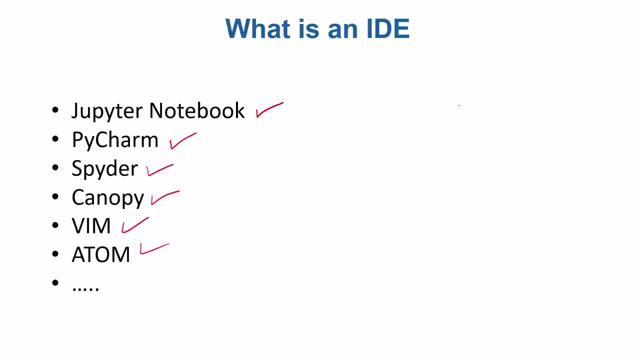 more. There are several of them. Now the question is, for data science in particular, what IDE is the best or what people suggest to be the best? So, before actually showing you the statistics- that which one is the best, before actually showing you the actual numbers, the statistical 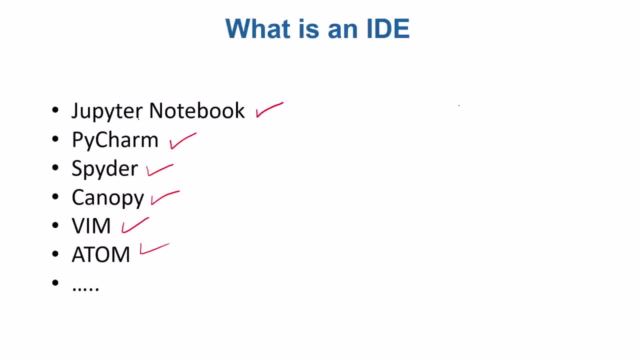 numbers that shows which one is better over the other. let me just go through a few of them, few of IDEs and their features and stuff, And then we will move to statistics and some numbers that will show that which one is better over the other. So let me start with this Jupyter Notebook. 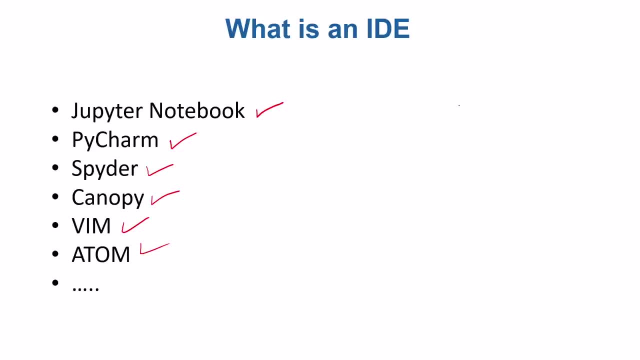 For the past couple of years, Jupyter Notebook has been gaining a lot of popularity in terms of coding and debugging. Notebooks have been redefining the concepts of an IDE and are adding more and more features onto it. Jupiter was introduced in 2014, after its predecessor, IPython, and from that date it is really 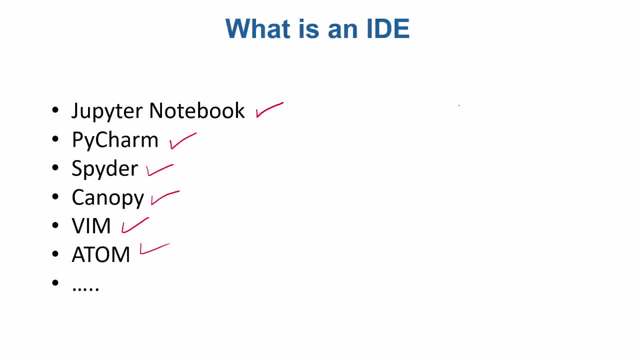 considered to be a bliss in the coding community. Jupiter stands for? I mean. some people say Jupiter stands for Julia Python R, but that acronym does not mean just this. I mean Jupiter Notebook today is supporting more than Julia Python and R and, by the way, this Julia Python, R and R, all these are 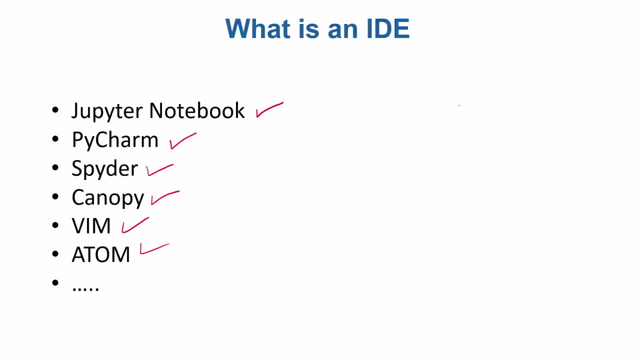 open-source languages and they are best suited for data science. This Jupiter Notebook: it has markdown editor, it allows you to write HTML code, it allows you to indeed give text to your document and it also allows you to allows you to write latex in it. I mean a lot more. 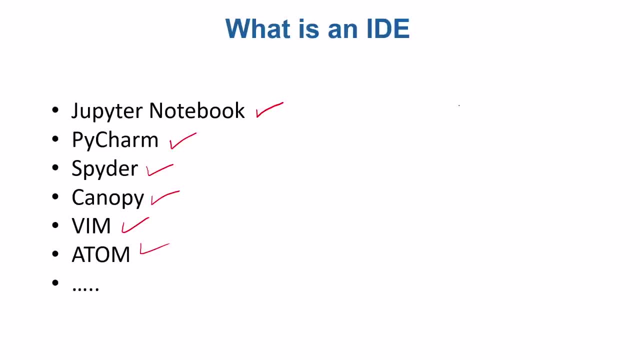 Further this Jupyter Notebook. it's a web application-based server client structure which is easy to use and allows you create, analyze and manipulate documents, And all these documents are in the form of notebooks. Since it's a web interface, it can integrate with many of the existing web libraries. 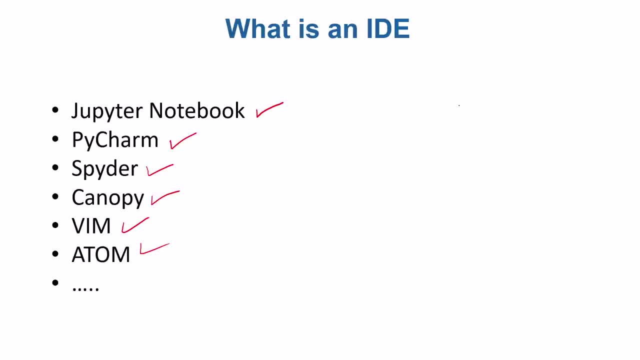 for example for data visualization. Jupyter has so many functionalities. You can write formula using LaTeX, run a Python code and visualization, for example a raw audio signal using matplotlib plotting library- all in the same notebook. Jupyter Notebook is not just an IDE. 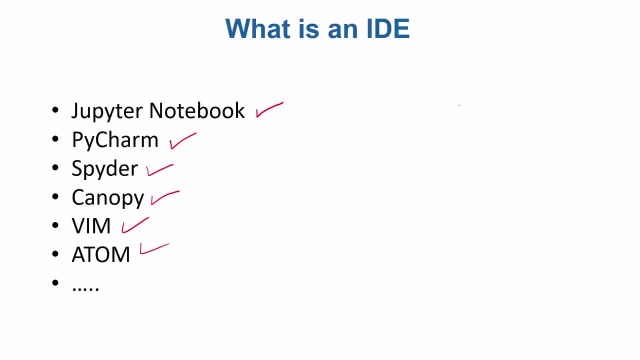 but it's widely used in an educational tool, for presentation and even for writing blogs. You can export your notebook from IPython Notebook format to PDF or to HTML, or even to py, which is the Python file. The user interface of Jupyter makes it a favorite tool. 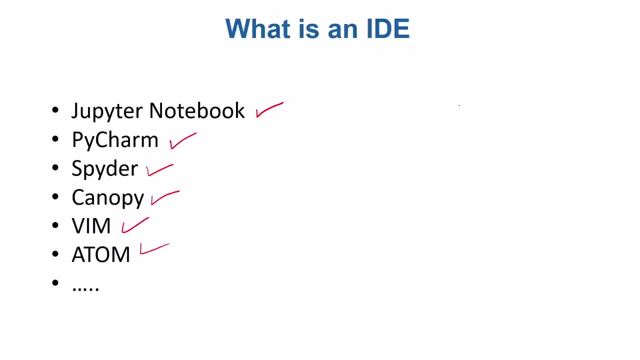 especially amongst the data science community. And one plus of this Jupyter is it's very quick to start. I mean very easy and very quick to start. I mean not much rocket science. to write your first code. You want to write your hello world. 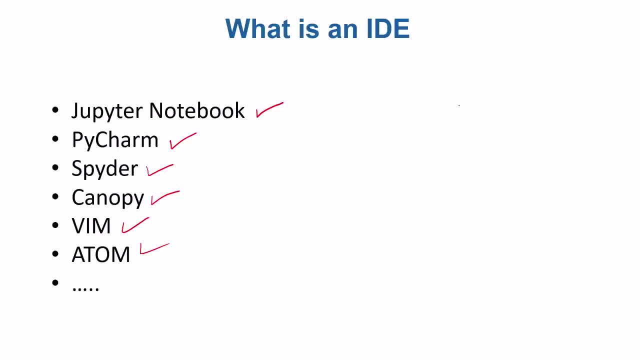 It's very, very quick in Jupyter to go and do that PyCharm. if I discuss PyCharm, however, if I discuss some of its properties, let me just discuss first that the PyCharm is by the company JetBeans. 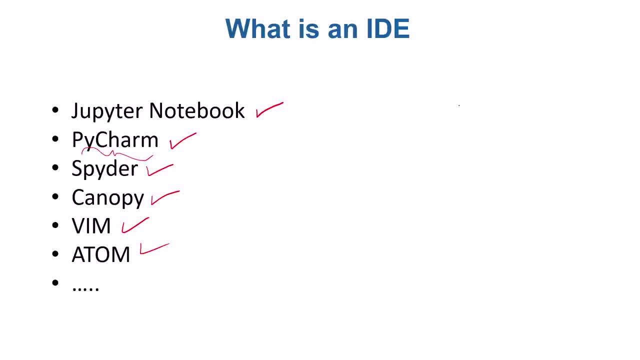 And if you have never used JetBeans, other IDEs like Java IDE, then running your first code successfully can eat up a little bit of your time, Actually, a lot amount of your time maybe, Such as I mean setting up an interpreter, PyCharm. 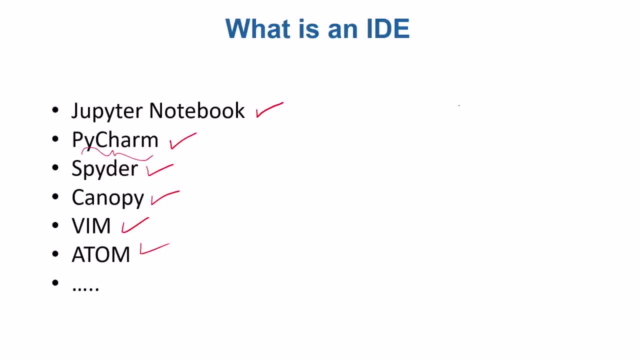 PyCharm, however, is much better for working with multiple scripts, handling vertical files and linking them together, and huge, large scale coding products. The good thing about PyCharm is it supports Anaconda and, as a result, all the packages that fall under Anaconda. 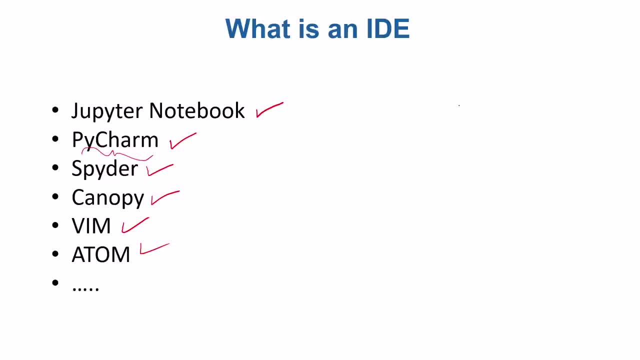 are supported by PyCharm as well And those packages including NumPy, SciPy, Matplotlib and so on. Just like other IDEs, PyCharm has a powerful debugger with a graphical interface. It offers JIT integration. It has secure shell terminal and variant control system. 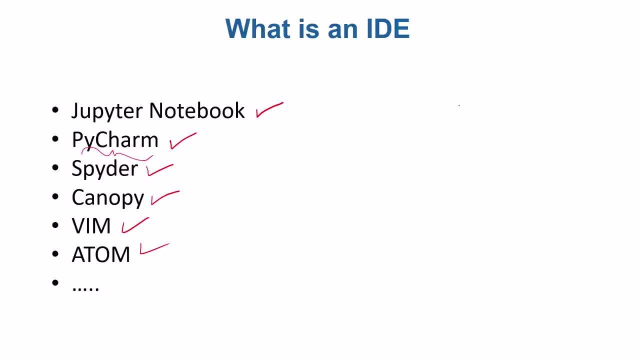 Python IDE is customizable, which allows you to choose between different themes, color schemes and key binding and whatnot. Additionally, PyCharm lets you add plugins for non-Pythonic files, and these plugins take care of indentation highlighting the errors. 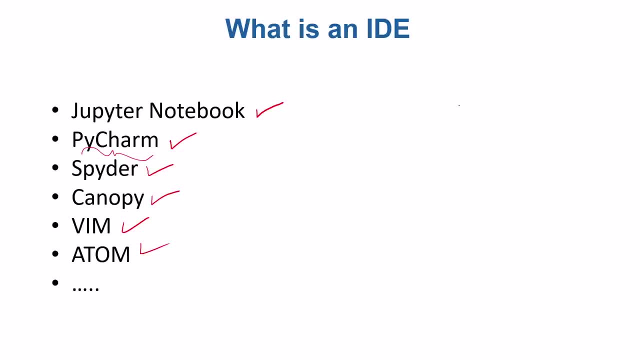 and keywords just on the fly. So PyCharm is also providing, I mean, a huge support for coding Python. But I mean the one bad thing about PyCharm, which is not that bad, but one bad thing is it is memory intensive. 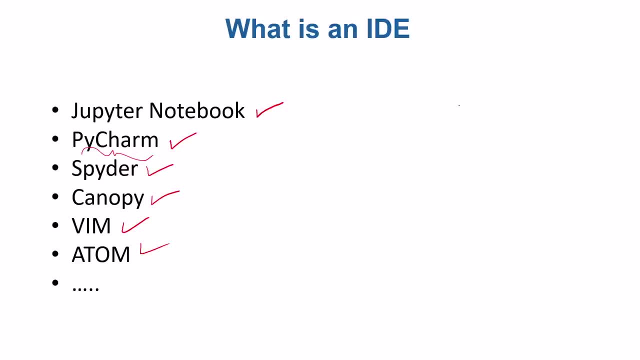 It eats up a lot of memory, It's a heavy thing And secondly, I mean getting started with PyCharm is not that quick. I mean it takes a lot of time to just go with that. Spyder, however, is a lightweight open source IDE. 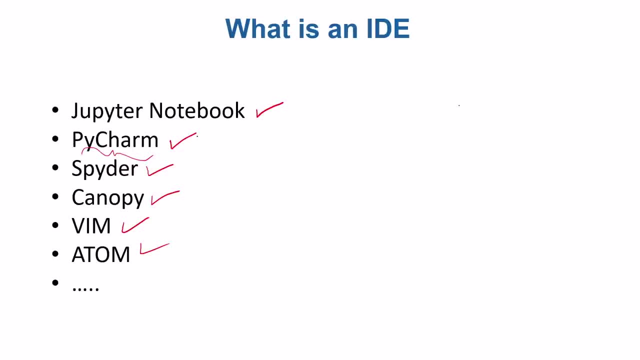 Oh, by the way, this PyCharm is not. I mean, it has professional edition and a community edition and it is not open source completely. Spyder, however, is a lightweight open source IDE that comes pre-installed with Anaconda. 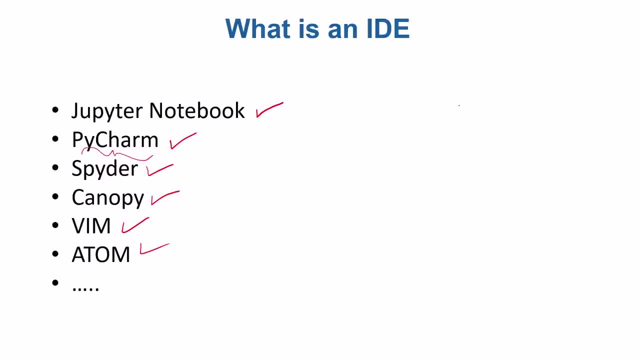 and it was built mainly for data science practitioners and engineers. Its look and feel is much like MATLAB. So if you're a MATLAB programmer, if you've used MATLAB before you switch to Spyder and you get, I mean, much look and feel the same. 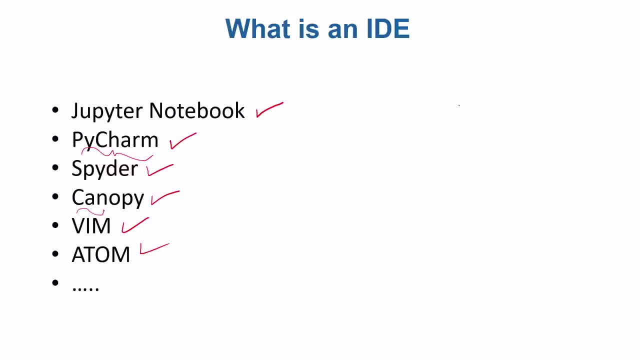 Canopy. by the way, the Anthos Canopy also has roughly the same look and feel as MATLAB. So but Spyder was built for data science community. It is integrated with essential data centric libraries like NumPy, SciPy, Matplotlib, Pandas, IPython and whatnot. 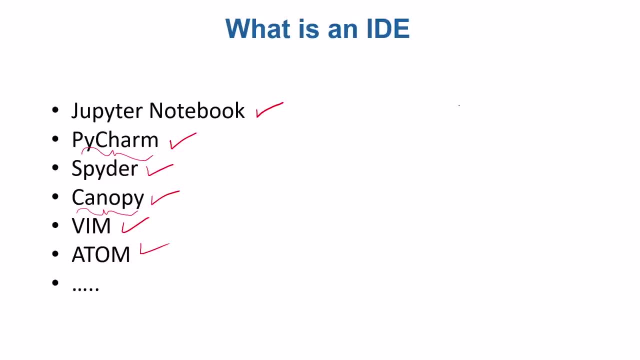 The built-in capabilities can be extended further by plugins and APIs. Spyder contains features like text editor with syntax highlighting, code completion and more. It also has a lot of other features, such as configuration, static code analysis, debugging, variable exploring. 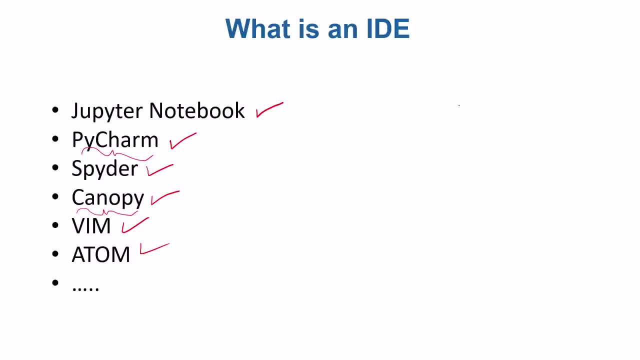 It also has a profiler that recursively determines the runtime and number of calls for every function and methods called in a file. And I mean there's Anthos Canopy, there's a VEM, there's Atom, there are a whole lot of IDEs. 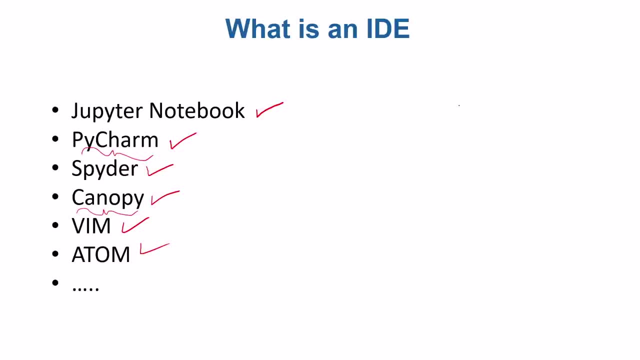 just for Python language. But the question really is: being a data scientist, which one is? which one should you choose? Being a beginner, which one should you choose Even for professionals, if you want to stay in data science? which IDE will you prefer over the other? 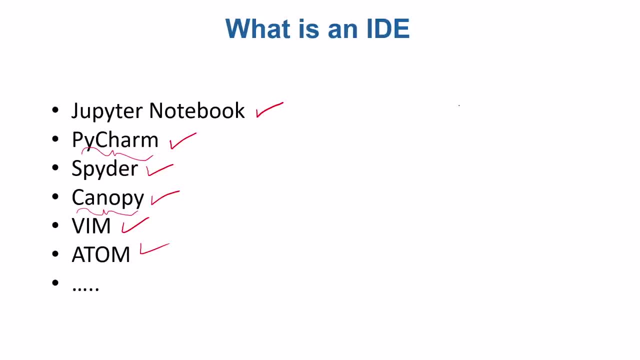 I mean, there are so many of them. I've just described three or four of them. So let's see some stats based on popularity of different IDEs for data science and then decide which one is better over the other. So, for example, this data, this analysis. 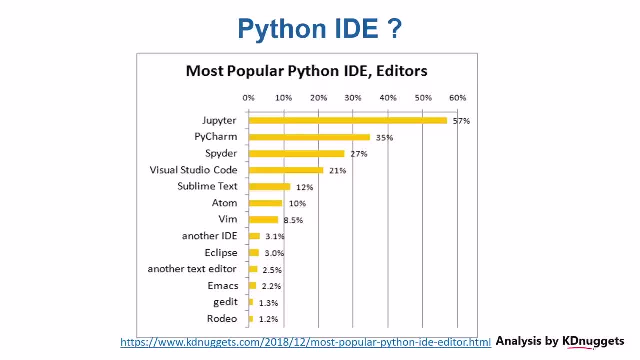 the chart I'm showing here. this analysis was done by KD Nuggets and this is the link for that, And it shows that the most popular Python editors till December 2018.. And you can see that the Jupyter is at the top. 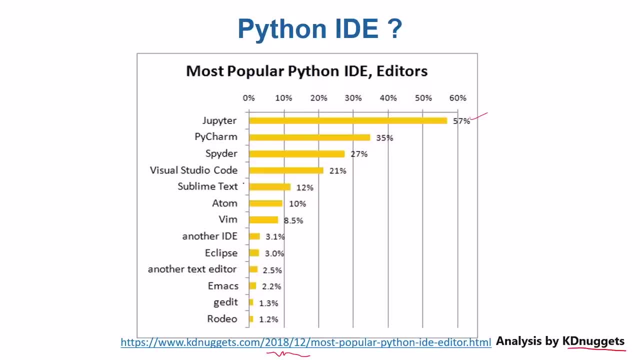 The second is PyCharm, then Spyder, then Visual Studio Code, then Sublime Text, then AtomWim, and there are so many others, But Jupyter is at the top, and this is for. I mean these all are listed with respect to the data science community. 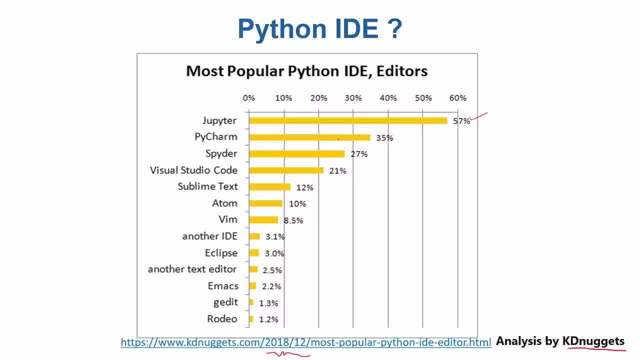 So in the data science community, which Python IDE is best over the other? And Jupyter is at the top. I mean, it is way out, And one reason to this is its simplicity: It's supporting to so many different formats. 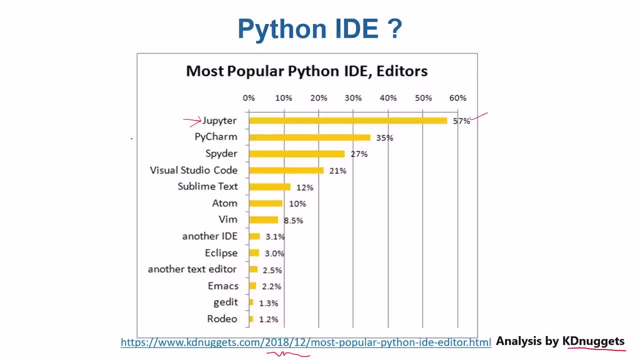 It makes an interactive document. It makes a webpage that is interactive. It makes a web page that is interactive. You can just change the code, You can make another web page, and so on. You can run it on a local system, You can run it online as server-based system and whatnot. 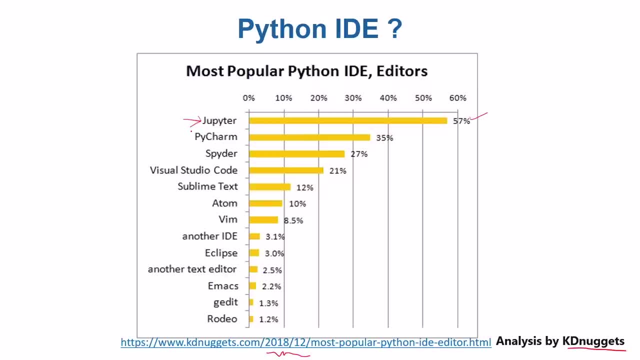 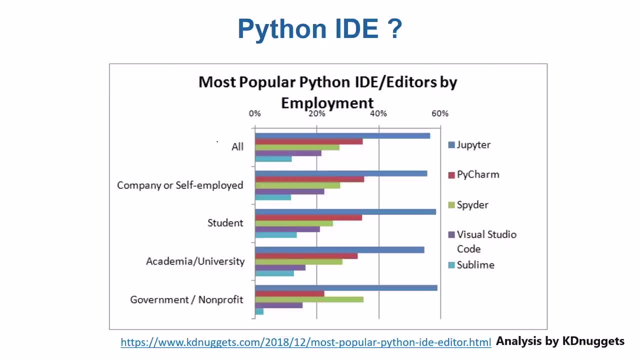 I mean it has so much flexibility and very quick start and easy to use. If you, for example, see the popularity of Python IDEs with respect to the employment, then you can see, overall the Jupyter is winner as compared to PyCharm. 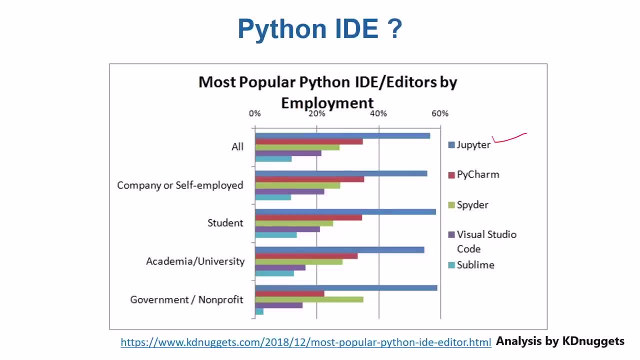 I mean it's not a common spider. We also do a quote in Sublime. If you see company or self-employed, still the Jupyter is way out, it is winner. If you see in a student perspective, Jupyter is a choice. 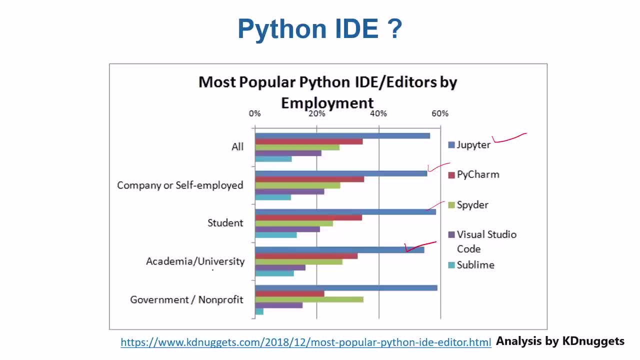 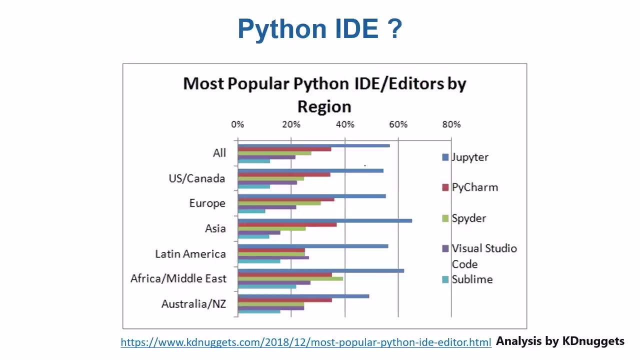 If you go to academia or university, Jupyter is a choice. If you are working with government or nonprofit, Jupyter is a choice. I mean, Jupyter is kind of outlier. It is staying at the top everywhere. Further, if you analyze the popularity of Python IDEs, 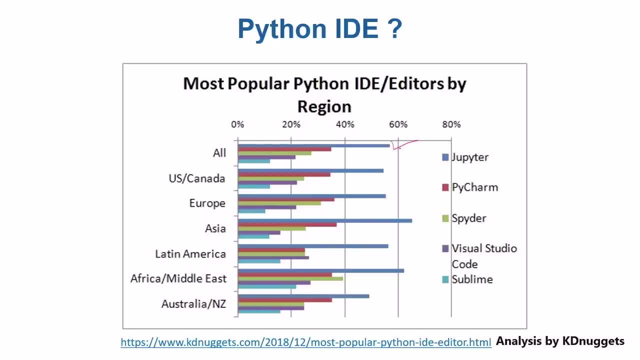 with respect to regions, for example. again, overall, Jupyter is a winner. If you see US or Canada, Jupyter is mostly used. Europe Jupyter is the winner. Asia, Jupyter is a winner. America, Jupyter is a winner. 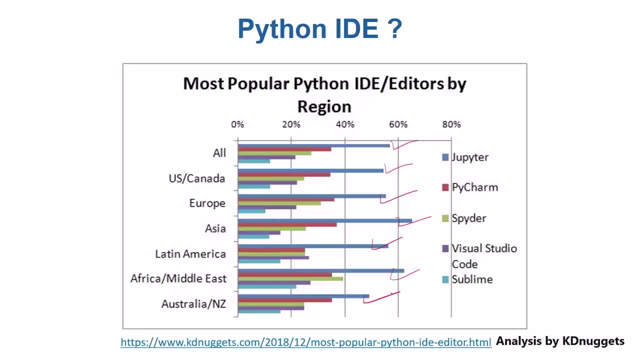 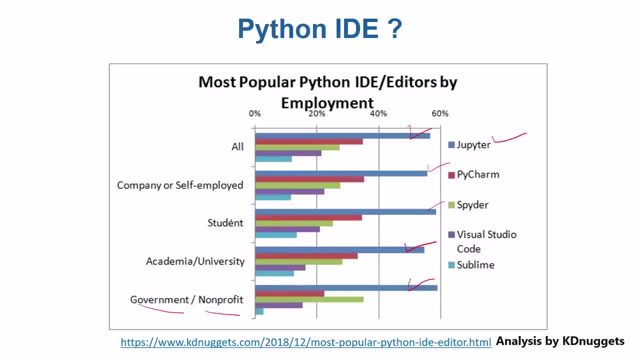 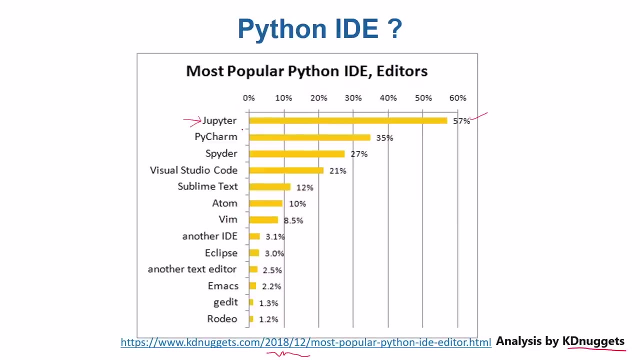 Africa and Middle East. Jupyter, Australia, New Zealand Jupyter. I mean these numbers are suggesting that Jupyter is, I think, one of the worst Hole Dog is at the top, Not just at the top, It's easy. 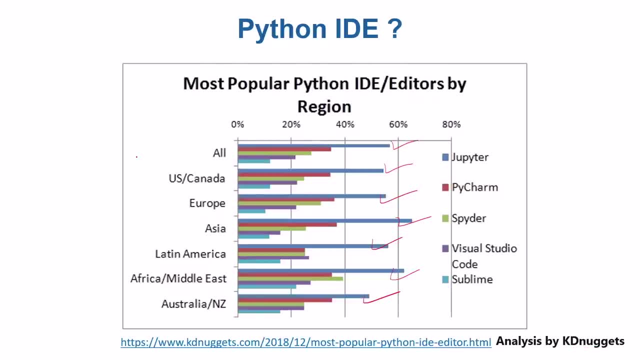 I mean- and maybe that's one reason why Jupyter stands on the top for the data science. So these numbers and these all statistics suggest that we should use Jupyter notebook for Python, and we will be doing that, In fact, for this particular course. 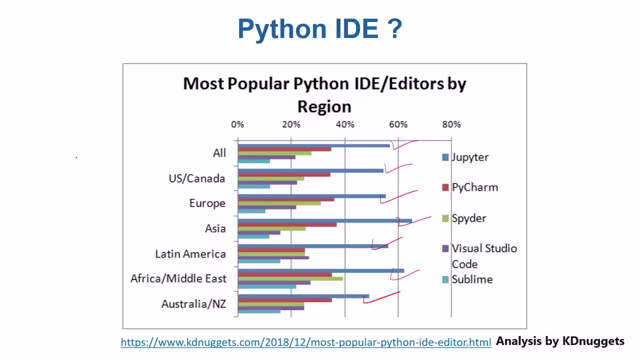 we'll be working on Jupyter for all kind of coding. I'll be just showing you how to install Jupyter environment, how to install basically Python and how to run Jupyter for the first time from it. So hope to see you in the next video. 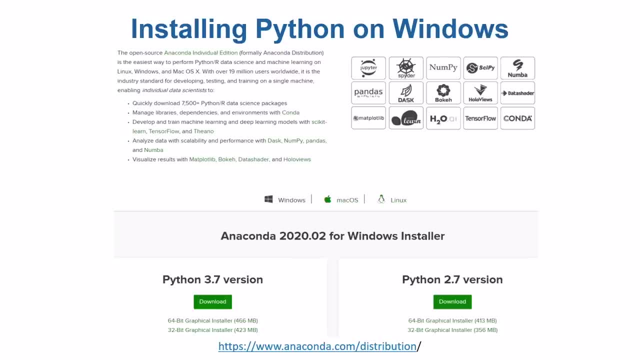 Okay, in this video I will show you how to install Python. There are multiple ways of installing Python. You can go to pythonorg and install Python from there. I would recommend to use Anaconda distribution. It has Python. It has a lot of packages pre-installed. It has 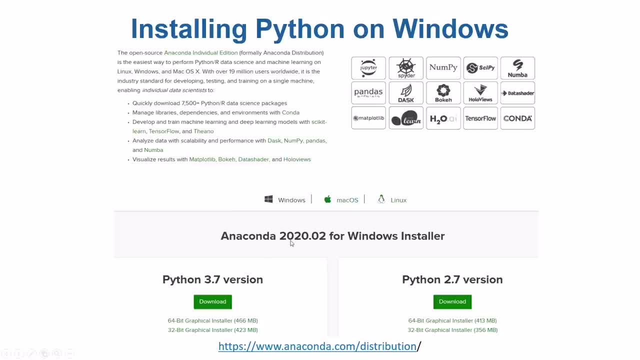 Jupyter notebook as well. So installing through Anaconda is easier as well. So if, for example, if you're working on a Windows system, you should download the executable for Windows. We will be working with Python 3 rather than Python 2.. So you should be installing, you should be downloading. 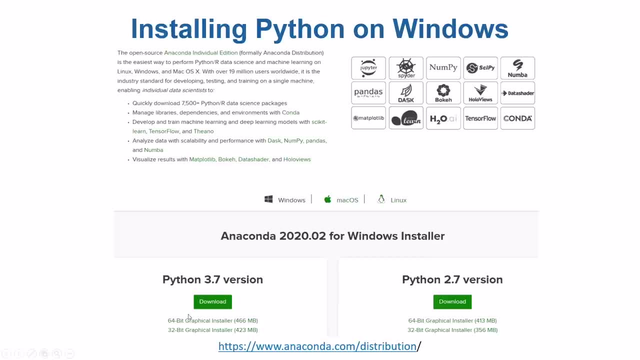 Python 3, point. whatever the latest variant is. Further, if your system is 64-bit, you should be installing 64-bit variant. Otherwise you will be installing 32-bit variant. So let's say you have downloaded the executable file for Windows. Then, after the download, 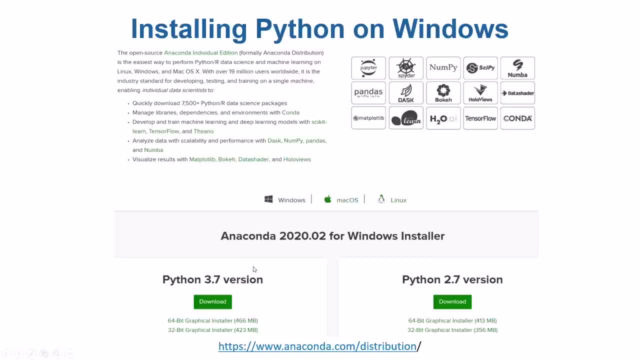 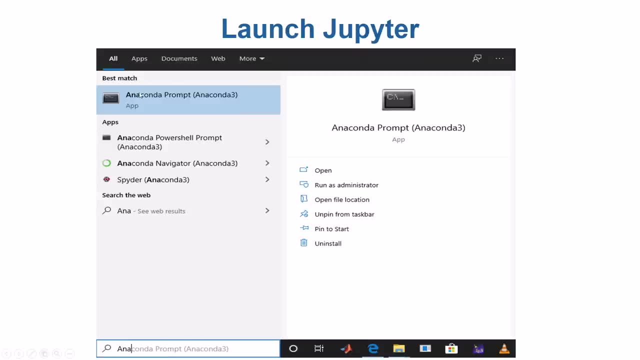 you just run that exe file and follow the steps and you'll be able to install Anaconda. Once the Anaconda is installed, then in the search bar you just type Anaconda prompt and the Anaconda prompt kind of symbol that my mouse is pointing at. this will appear in front of you. 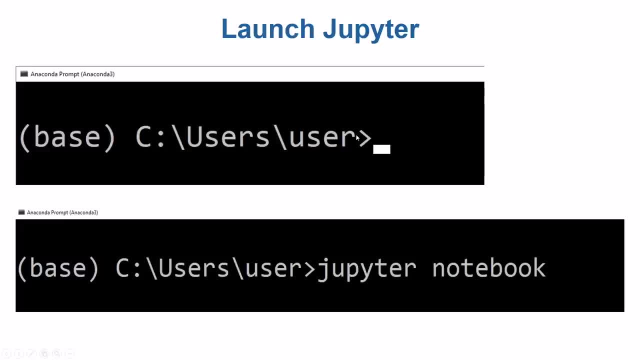 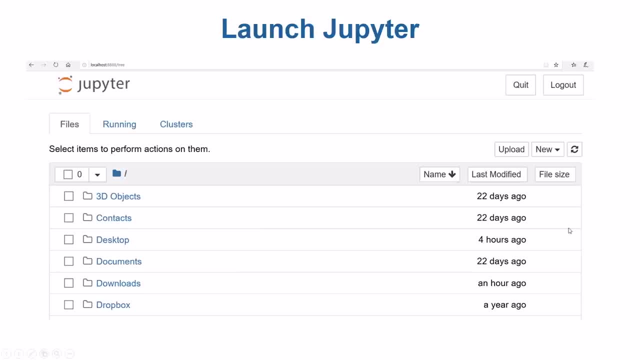 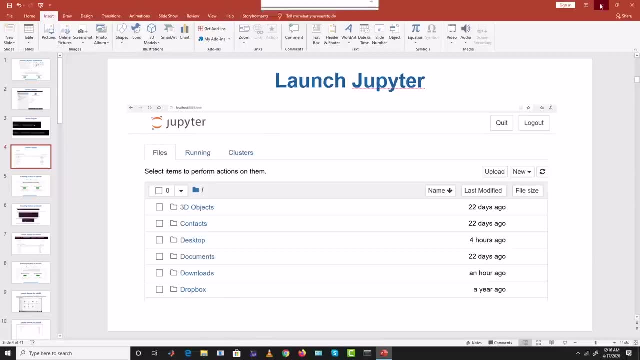 You just run it. You will see a command prompt like so. Then in that just type Jupyter notebook and press enter and you'll be having Jupyter running in front of you. Let me, let me show you that on my, on my system, how to do that. Let's see, For example, this is my search bar. Let me 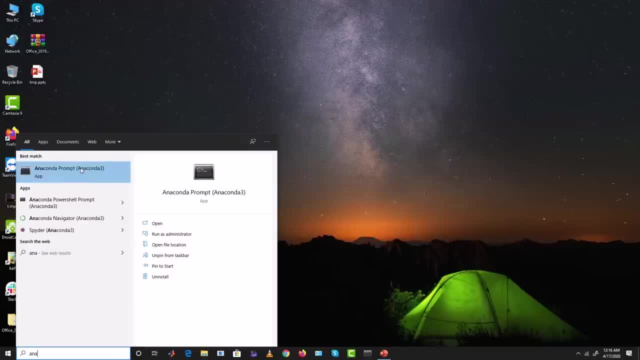 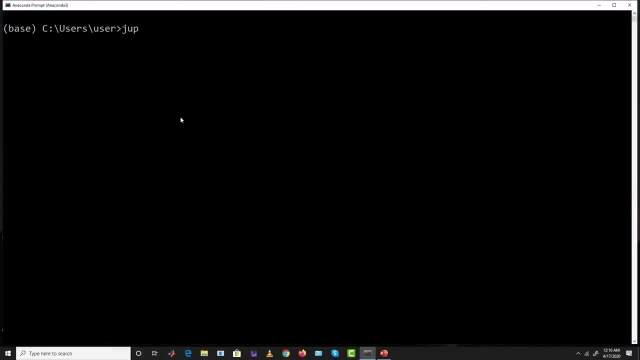 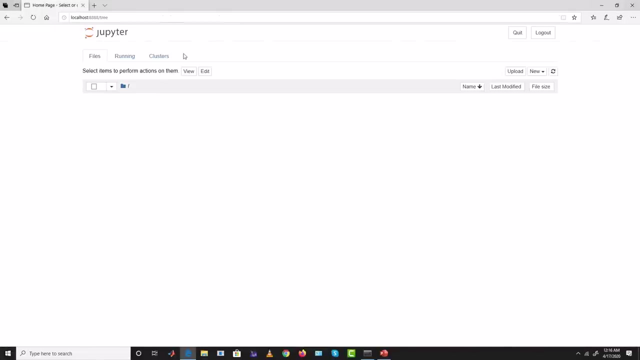 type Anaconda prompt. So this is the Anaconda prompt. So if I click it it runs. Then I just type, for example, Jupiter notebook and then I just press enter For the first time. it will take some seconds to run, So let's wait for it. So yes, it runs and it will show you. 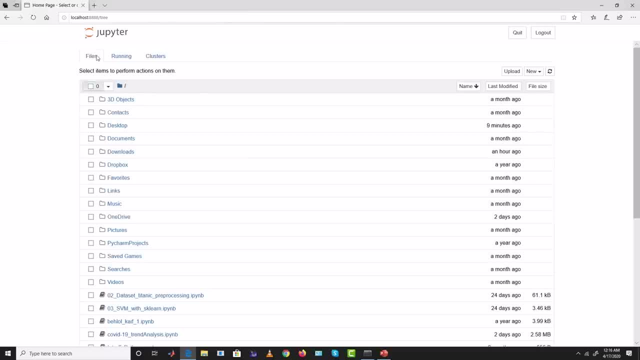 kind of a browser in front of you, And that's what the Jupyter interface is. We will see then how from this Jupyter, how to write the question. Now, if we wait for a while, this Jupyter interface will work. So in this case I will not be able to type the question, I will just type it and then. 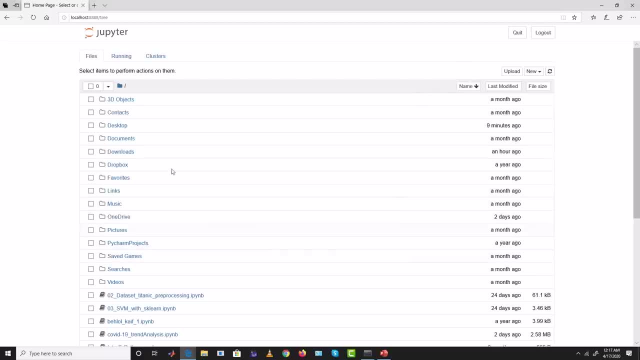 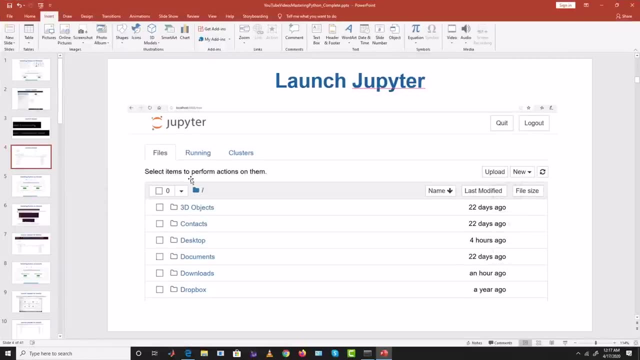 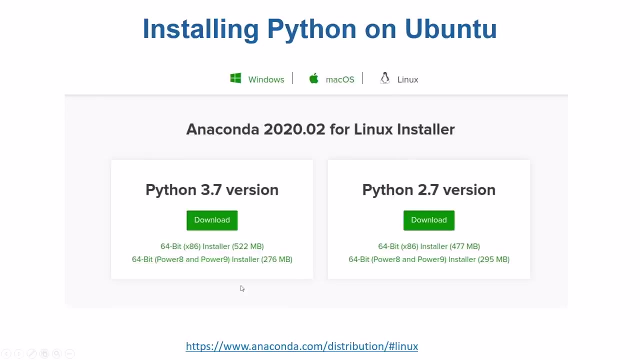 code, how to make the code files and stuff. but that's how, uh, from anaconda installing, after installing anaconda, that's how you will launch the jupiter. um, so this is that easy, no problem? um then, uh, for example, you can install, uh, you can install- python if you're working on linux. 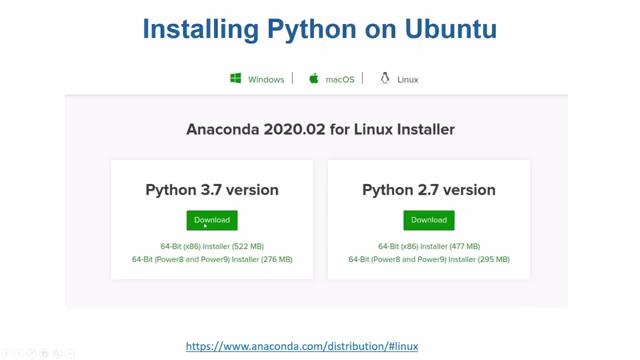 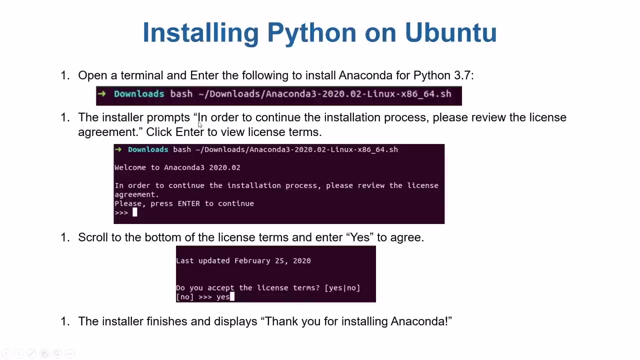 and just download the version for linux and then, uh, then for example, let's say, your, um, your, your file is downloaded in the downloads folder. then run this command, bash, and this dot sh. that's the file name. uh, the installer prompts in order to continue installation process. this i mean. 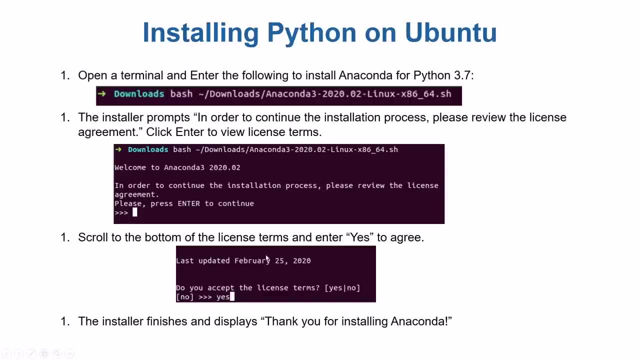 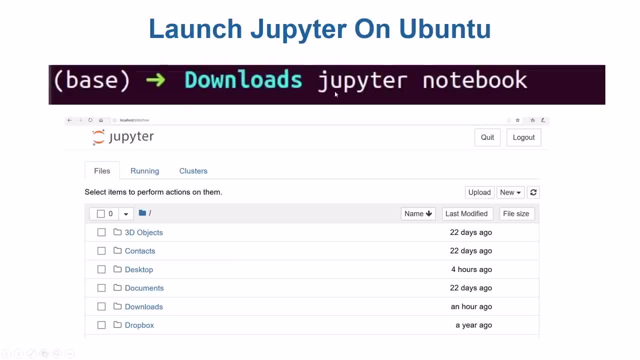 these kind of commands will will appear. press enter to continue, then press yes and the installer will finish with the thanks message. after that you just go to downloads folder and type jupiter notebook and the jupiter notebook uh interface. the browser-based interface will appear in front. 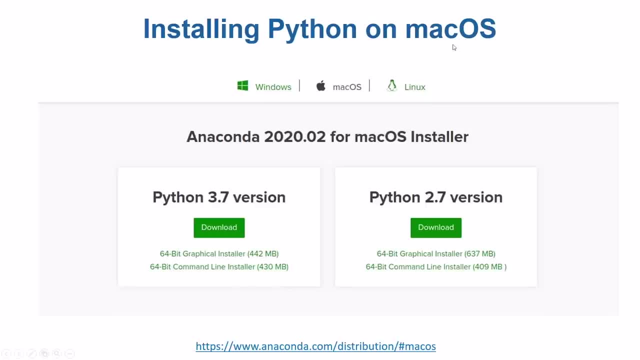 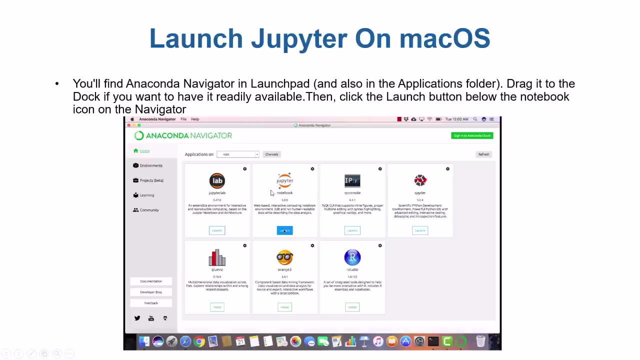 of you. you can have. if you are, if you're working on mac, you can, you can in, you can download the uh anaconda distribution for mac. um then, uh, you'll find an anaconda navigator, the launch pad. you can launch that and then just click there. there's a jupiter icon in front of you. just press the launch button. 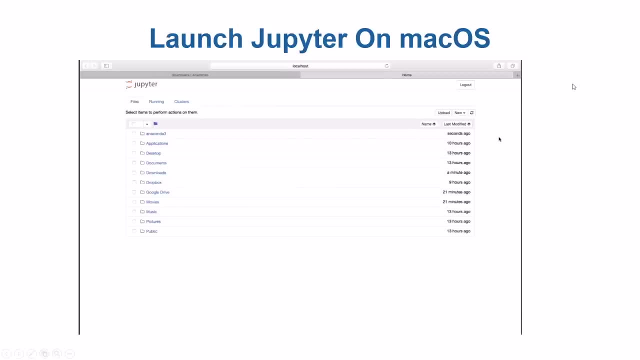 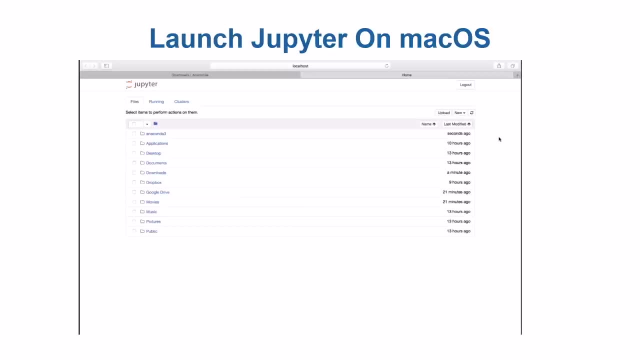 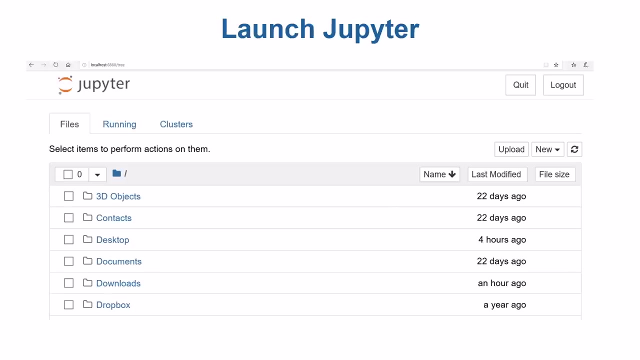 how to install python. uh, if you install python using anaconda, you'll be having jupiter notebook as well. in the next video we will see how to actually uh use that jupiter notebook interface, for example. i work on windows, so i'll be having, uh, this kind of interface, although the interface 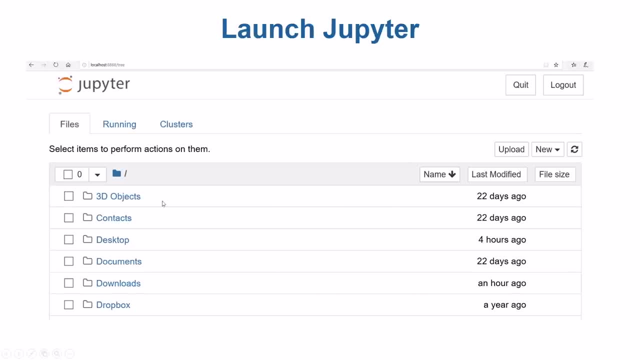 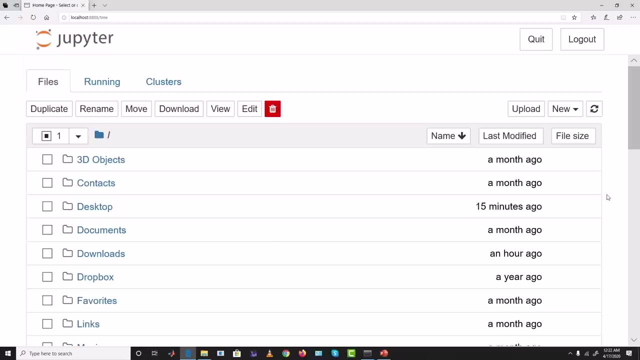 looks like the same because it's a browser-based, web-based uh interface. uh, in the next video i will show you how to get comfortable with jupiter and we will be also writing our first hello world program in python. so hope to see you in the next video. okay, so in this video. 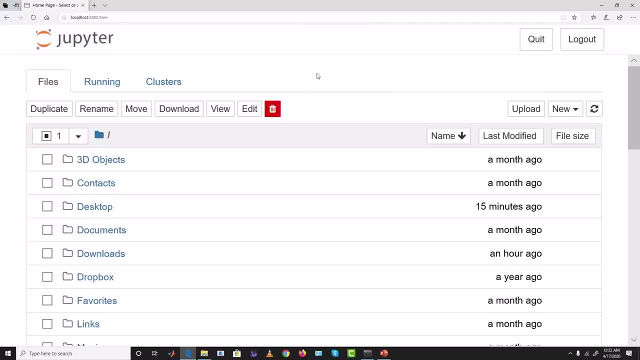 i will show you, uh, how to write the first program in in python, basically the hello world program. before that, uh, in the previous video i show you, i showed you how to launch jupiter notebook. so once you launch jupiter notebook, whether you are working on windows, whether you are working on 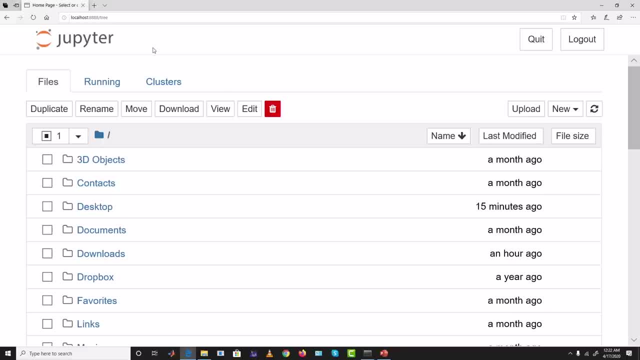 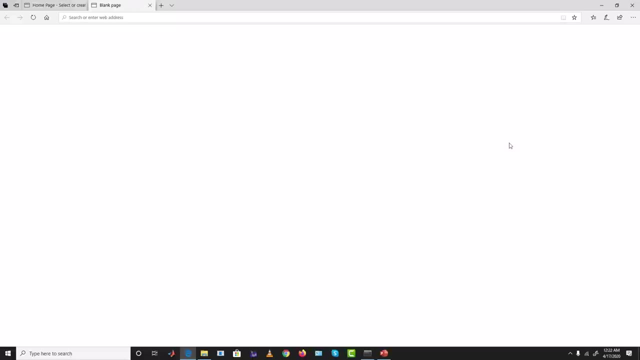 linux or or mac whatever. when you will launch the jupiter notebook, you will see this web-based interface, and here you, in the right corner, you can see the button new. you just click it, you will select python 3 and you will see a beautiful interface in front of you that will allow you to code here there are. 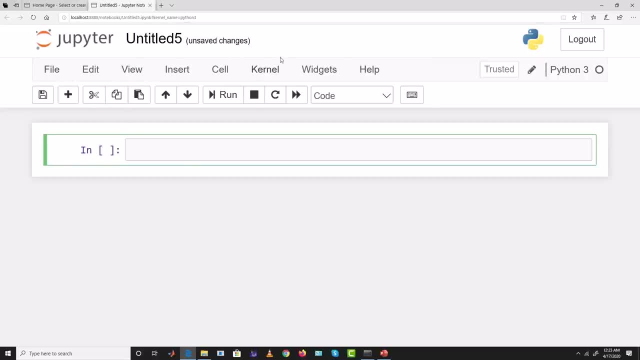 a lot of file edit view. there are a lot of buttons, kernel and a lot of controls here. we will see them as we move on, but this is how you this is. this is what the coding environment is. this is kind of editor as well, as i mean. this is complete ide interface in front of you. so let's see this. 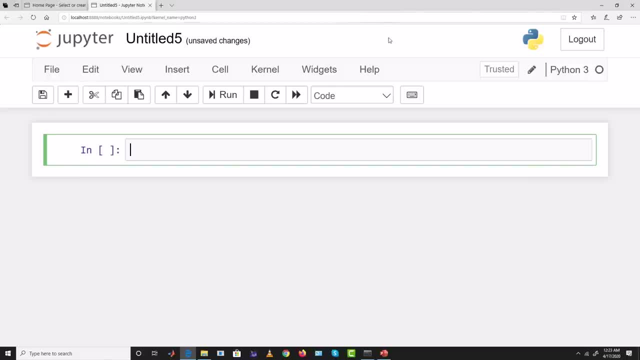 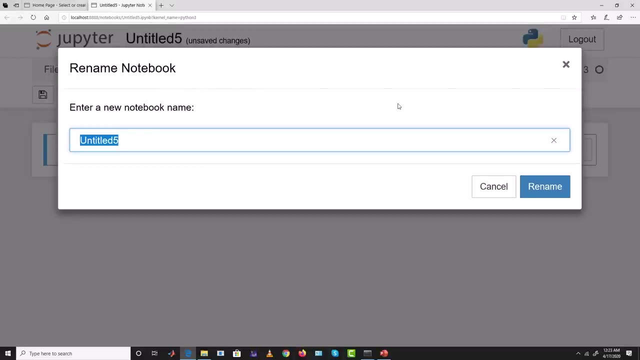 interface a little bit, step by step, at least the the controls that that we need. first of all, you are seeing, uh, where my cursor is moving. that's the file name or the notebook name. you can change the notebook name or you can just write, for example: whatever the name of the? 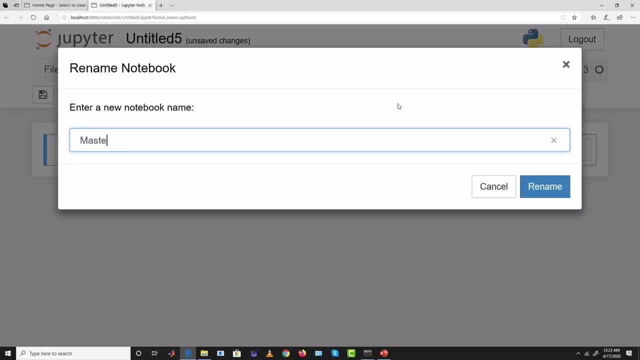 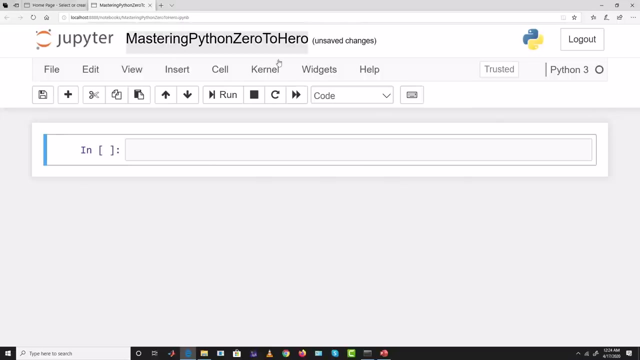 notebook. you want, for example, mastering Python for beginners. okay, so let's say that's your mastering Python. let's say, let's say zero to hero, maybe. so let's say this is your file name. you just create that file and you see this: mastering Python, zero to hero. that file is created with. this file is renamed. 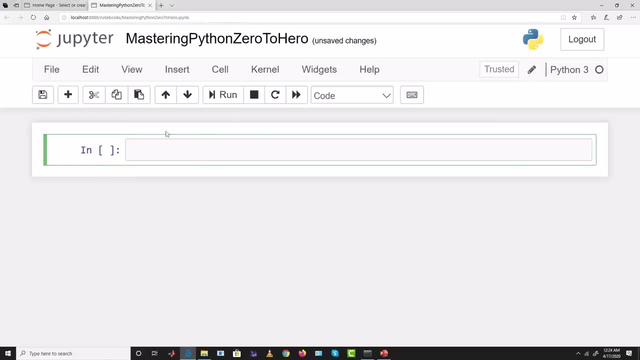 second, this is a cell in which you are going to type your code. the code, I mean the two, the two, the two modes of writing- is one is you can write the Python code. another way is you can write the markdown. the markdown is important in in a way that, if you want, 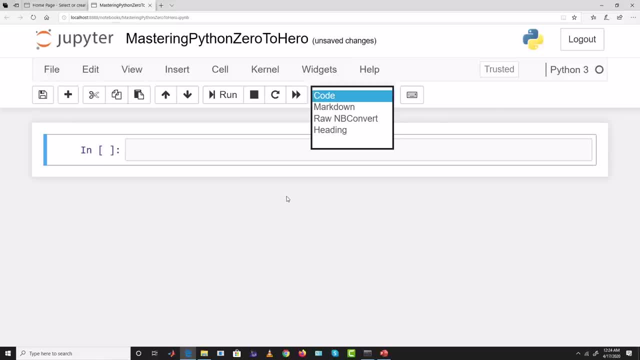 to describe your code. if you want to write other stuff other than Python code, you can use these markdown cells and they will be helping you. for example, if I select this markdown and I I just select this markdown and I type here for example: this is Python tutorial, and then I press shift enter, it will appear as a heading. 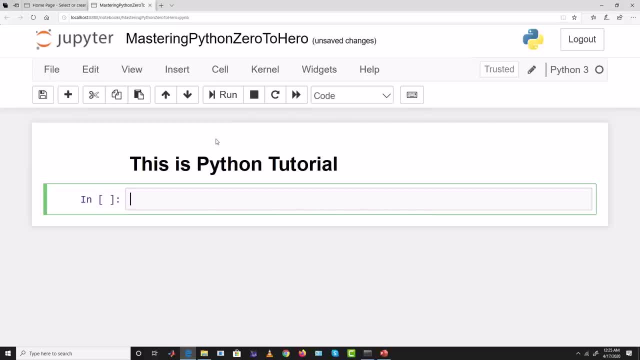 and a new cell will be created down. this is also a cell, but this is a markdown cell. as you can see now in this cell, that's a code cell. you can switch a cell from code to markdown by just pressing an escape key. when you press an escape, 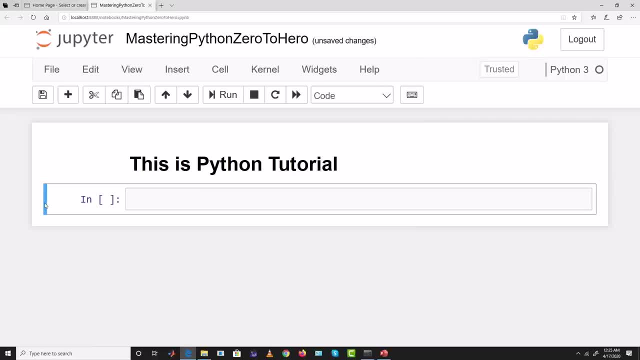 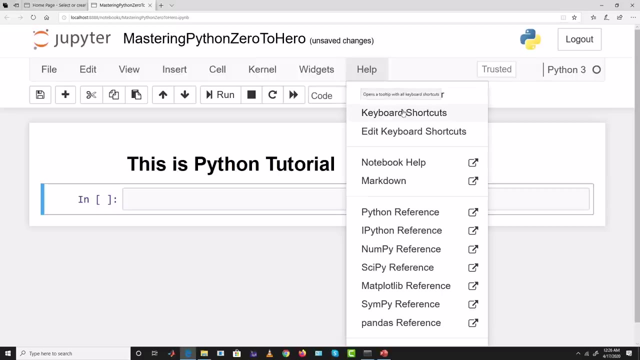 key, you will see the color will change. here you can press escape key. then if you press M it will change to markdown and if you press Y it will change to a code cell. there are several, I mean shortcuts that are available, keyboard shortcuts if you, if you just see, if you go to help and see this keyboard shortcuts there. 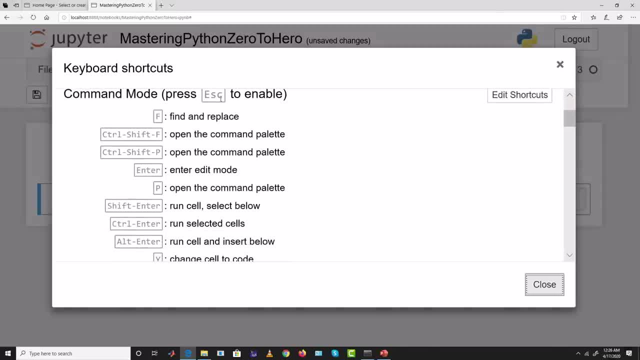 are several shortcuts that will be available in front of you. so, for example, if you press escape and then press F, you can do the find and place operation, and if you press enter, then that will go into edit edit mode, if that's important. if you press shift, enter, the cell will run and the new the, the cursor will go. 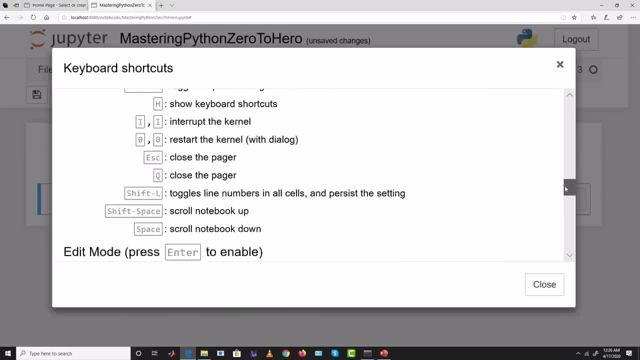 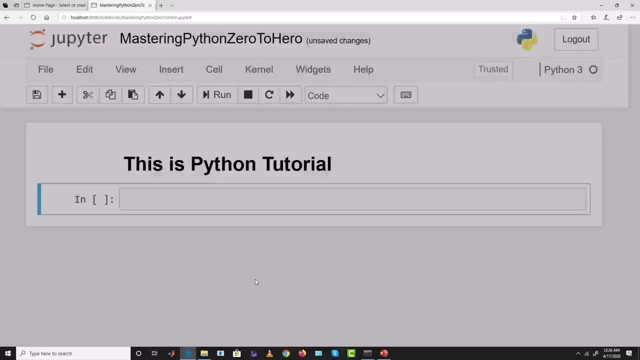 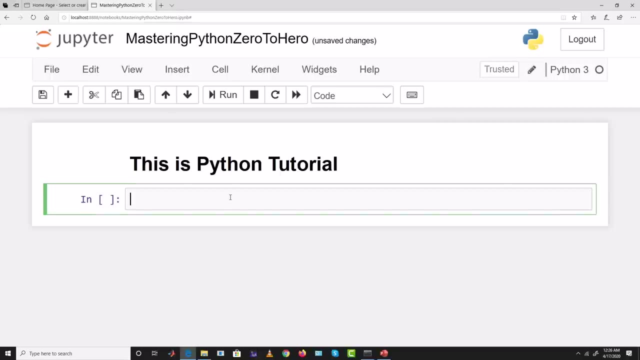 into the new cell and there are of controls. you should be seeing most of them. i mean, getting a good grip on these controls will help you moving in this jupyter notebook very quickly. so, for example, this is a python tutorial. that's a markdown cell. uh, you can also create this, this cell, also as a markdown cell and then 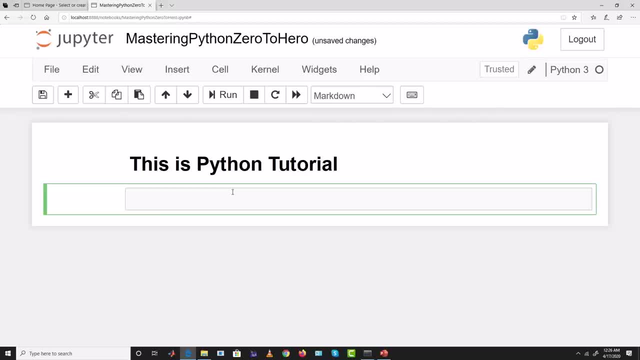 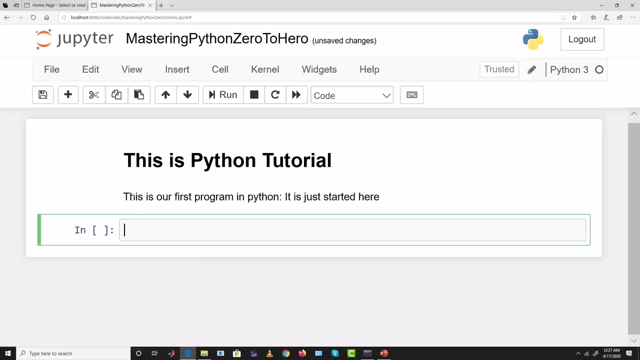 you can type here, for example: um, this is our first program in python it, it, it is just started here, for example, and it just appears like uh, like a description, and again a new cell is graded down and there you're going to have like a description of what we're going to do here. all right, here's a ctrl shift and i i'm going to copy that down here. here's the wizard here for non-granteed for bạn. you like like a description, like uh, like a description, and again a new cell is graded it down and there you 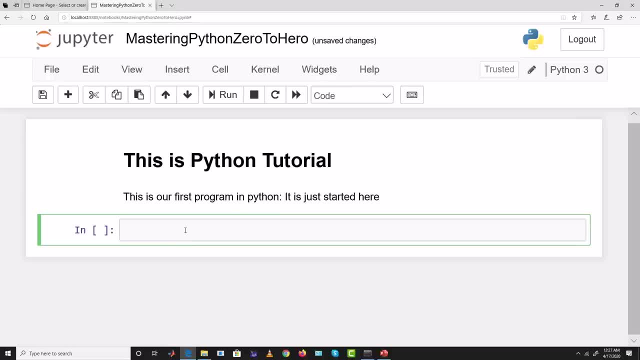 can write your code. so let's write the first python code. hello world. so first of all you will write print. print command will allow you to print anything on the screen: parentheses, double quotes, starts, ends, and in the double quote you write whatever you want to be printed on the screen. 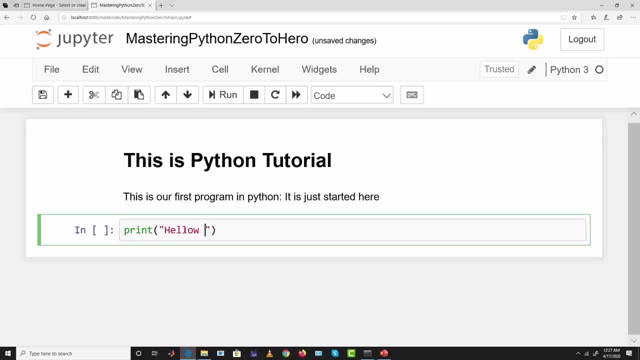 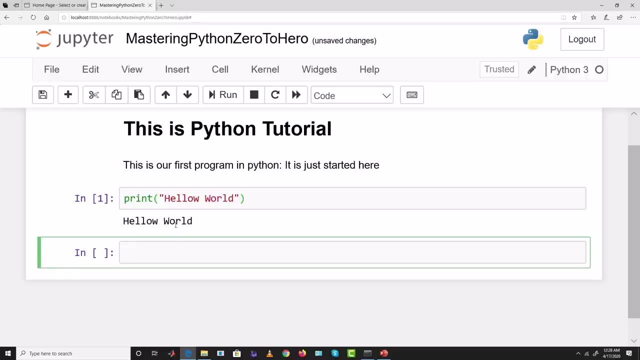 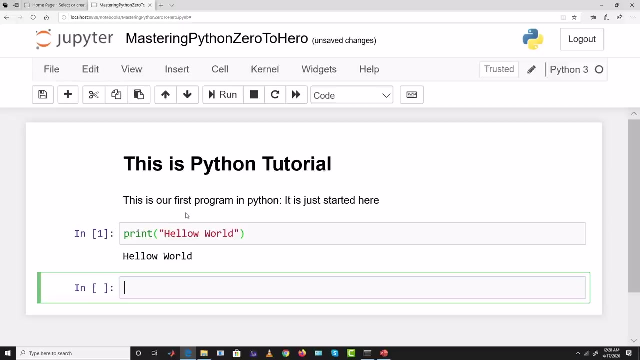 so, for example, hello world. and once you have written that code, just press shift and enter and this code will execute in front of you. so that's hello world, uh, printed in front of you. um, and that's our first program. i mean writing the very first program in jupyter notebook is: is that easy? 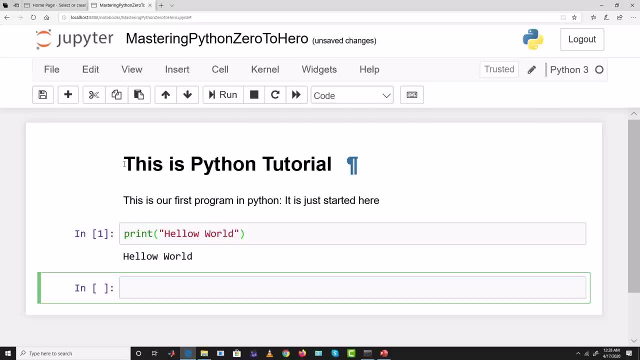 not only that, this jupyter notebook will be created. you can- you can just- i mean- describe anything. you can write the headings, you can write html in it, you can write math using latex and, for example, let me, let me write a latex or math in front of you. just just, let's say you are making a notebook that 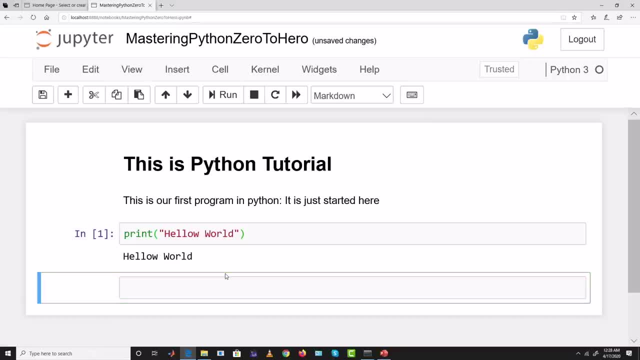 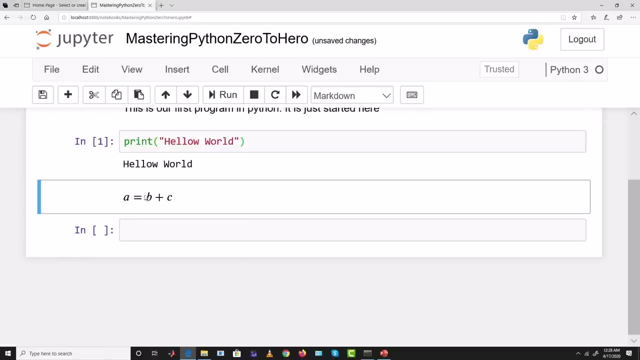 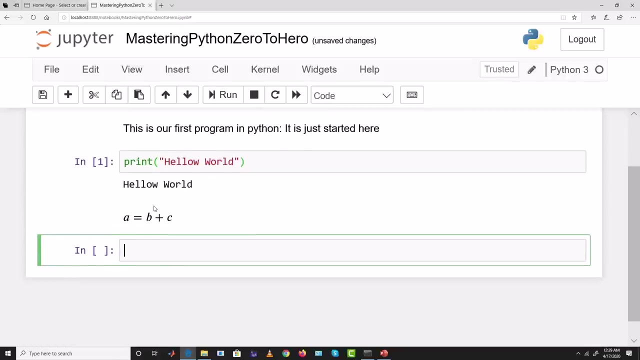 requires some mathematics in it, and it allows you to write mathematics as well. for example, a equals b plus c, shift, enter, and that appears like a mathematical equation. not just this: you can write very complicated equations, um, i mean and, and, and this whole notebook will contain your descriptions. 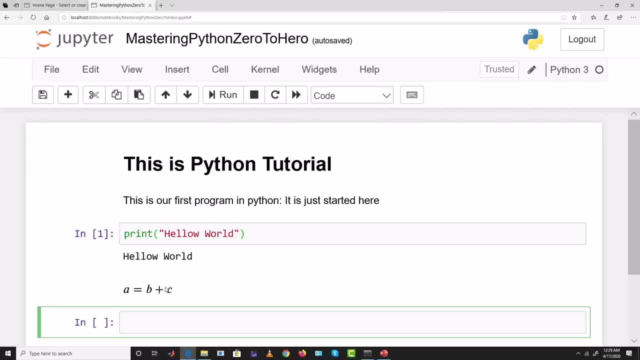 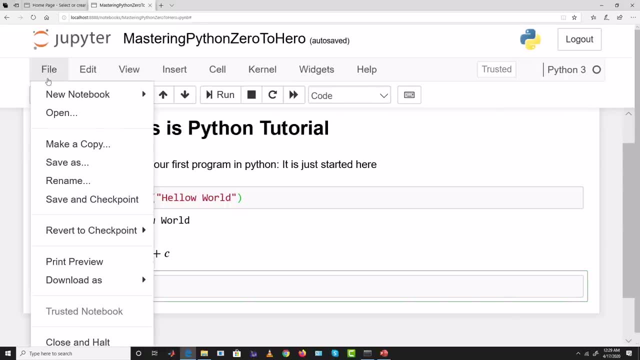 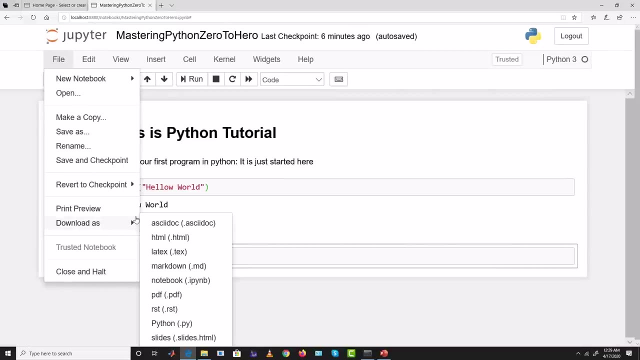 in terms of uh, html's or latex, or descriptions and code and all that mixed up, whatever, and at the end you will, you can, you can just download this, this. you can just download this, uh, this notebook, as if you want a pdf file. pdf file if you want. 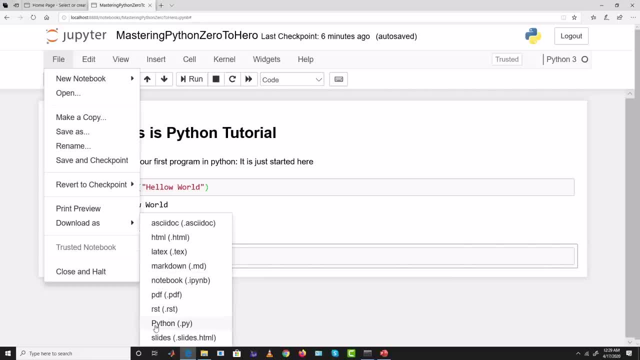 a notebook file, it's a notebook file. if you want a latex, if you want just a python file, if you want slides, for example- i mean you can download the same thing as slides- it will make slides for you. so there are a lot of ways of using this notebook. 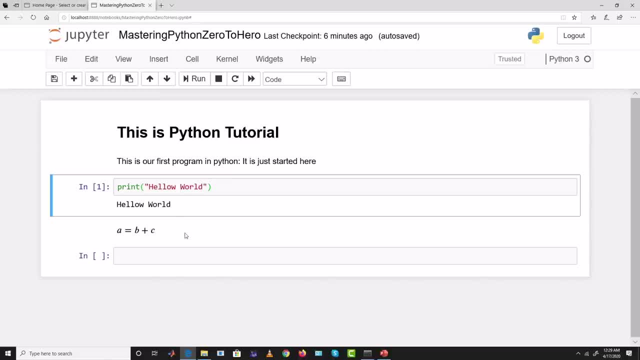 and that's a ready-made document. i mean you end coding, the document is ready for you. um, so this notebook is really really powerful jupyter notebook and coding in it is not just the coding, i mean, it is preparing a document. if you want to prepare a document you want to describe. 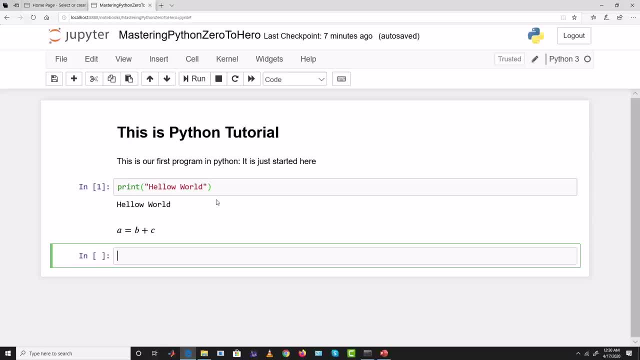 anything you want to add images and at the end of the day it will be an html document for you. it can be shared on web. i mean it's ready, uh, nothing, we we want to further finish it. so that was our hello world program in in python. 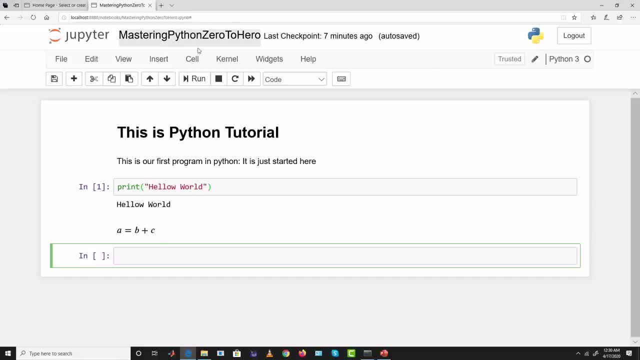 we will continue to build this by mastering Python zero to hero notebook. we will continue coding, in that we will describe the headings, we will write the markdown cells and all that stuff and we will. at the end of this course, you'll be having one notebook with all kind of descriptions and code in it you can use. 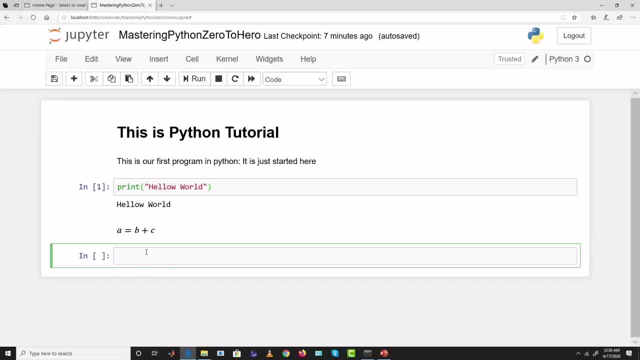 that notebook. afterwards we will be building. well, one notebook, one complete notebook for Python. so that's about it. that's the hello world. in the next video we will see how to. what are, what are the constructs in in Python, what are variables and other stuff? but before that, I also wanted to show that this 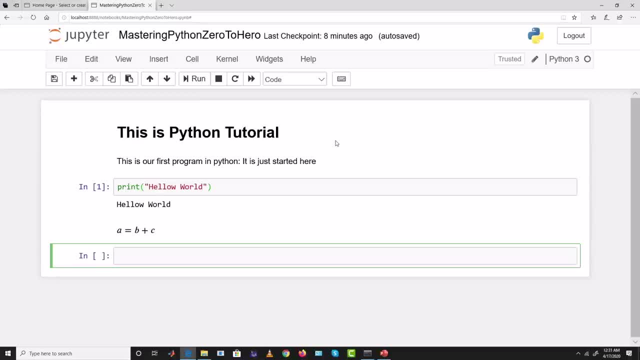 notebook is an enhanced variant or the upgraded variant of IPython shell, and I also want to show you IPython shell as well. so in the next video we will just see the IPython shell and we will see how can we, how can we view Python as just as a calculator by using IPython shell, so hope. 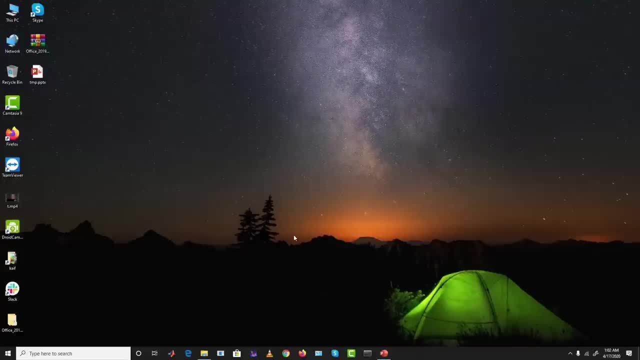 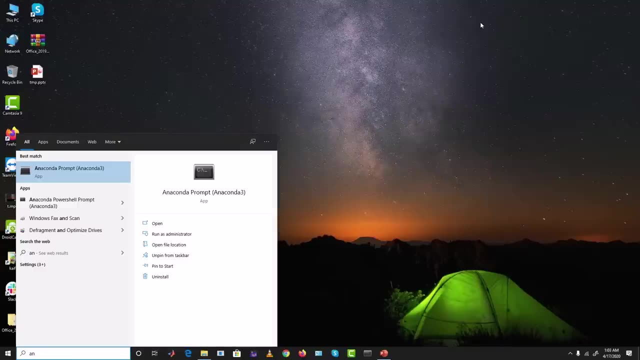 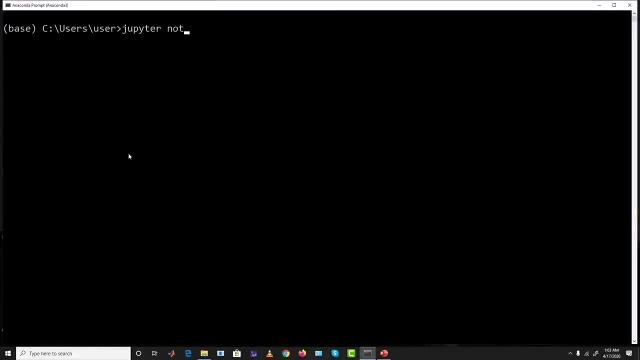 to see you in the next video, okay, so in this particular video I'm going to show you the IPython shell. just open up the Anaconda prompt, as as before. like you want to open a Jupyter notebook, then you just type here Jupyter notebook and you will be. you'll be in the in the notebook words Jupyter. 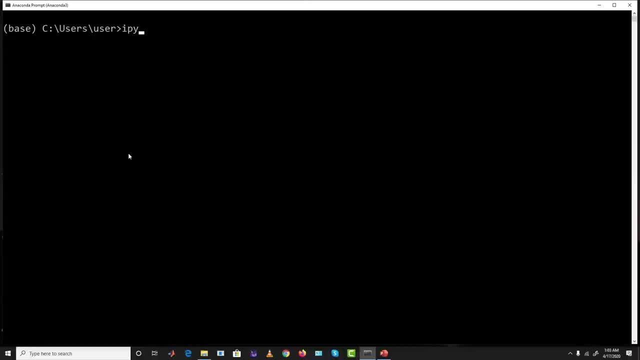 notebook word. but if you just type in ipython and press enter, then a prompt is open for you in a colored way, and this is perfectly fine to write any kind of Python code in here. actually, the Jupyter notebook is more enhanced and more featured, with enough I Python basically for learning how to use it. so now let's. 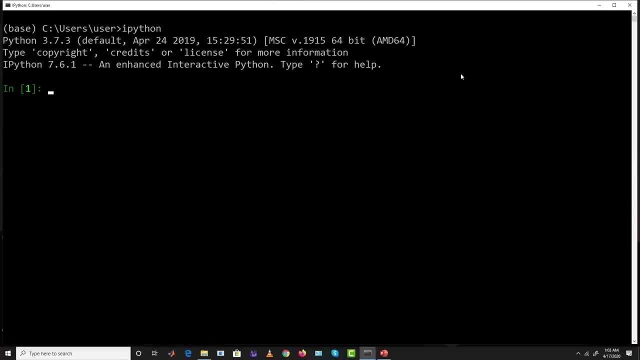 everything that is there in IPython is there in Jupyter notebook as well, but it has more features, more documentation and stuff. so, for example, if I just write a Python code here, hello world, let's say it will work in IPython shell as well, but remember previously, in in Jupyter. 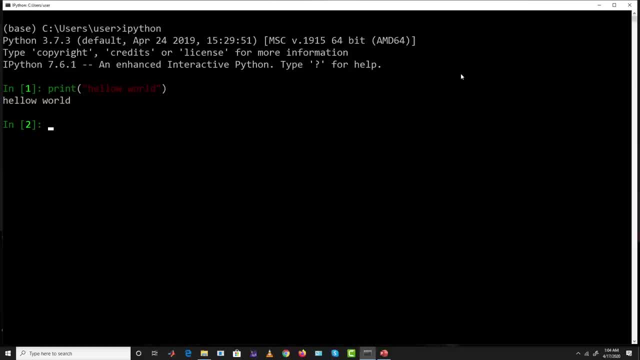 notebook we type shift, enter to run a particular command. here we just press enter and everything will work. if you want to clear the screen here, whatever the whatever we typed here, if you want to clear that, just press ctrl L. if you are on Windows, ctrl L will work on Windows. now IPython is just like you can. 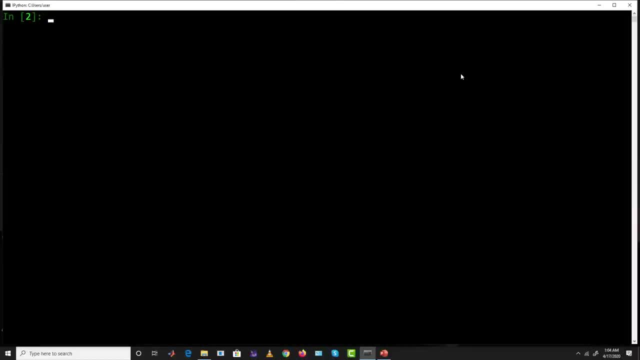 use the Python in in this particular shell just like a calculator. for example, you want 2 plus 3, press enter. that's 5. let's say it's 9 multiplied by 7. the answer is 63. you can write a complicated statement as well for. 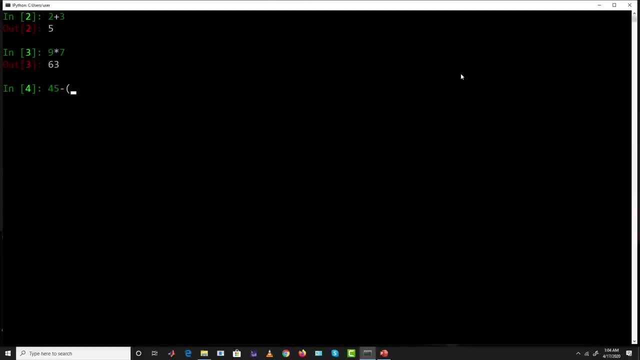 example, 45 minus eight. isotic or multiplication: aesthetic is achieved by multiplication, is achieved by a static symbol: seven. and then you can have this minus ten, divided by two, and then just press enter the answer 16.0. if, for example, by the way, i have just pressed the up arrow key and the last command, 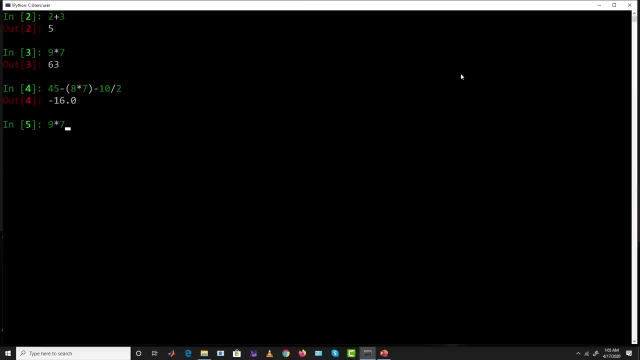 just appears. i have pressed up arrow key again and the second last command appears. i press the up arrow key again and the third last command appears, and now i'm pressing the down arrow keys. so for example, this and you may have, whatever the result is, you may have. 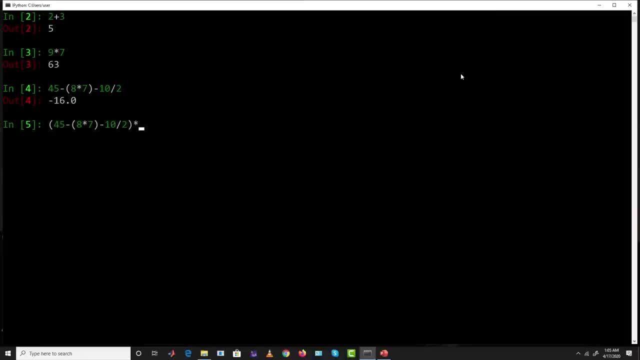 that multiplied by 10 and minus, or or maybe plus plus 15, so the result is minus 145, and so on. so this python, ipython shell, uh, you can write very complicated, or almost. i mean the complete python coding can be written in ipython shell. 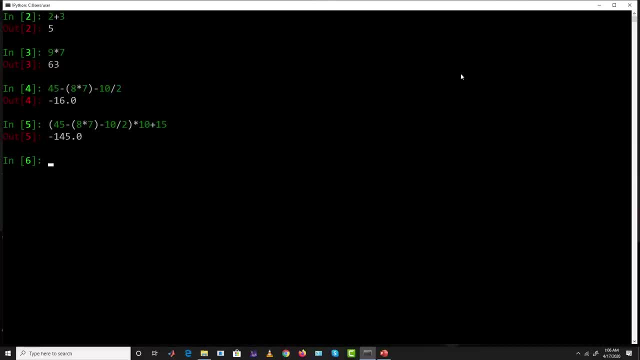 and you can use this to write a very complicated- or almost i mean the complete python. coding can be written in ipython shell and you can use this shell just for a calculator. now let's see, for example, you, you compute this result, let's say 45 minus. 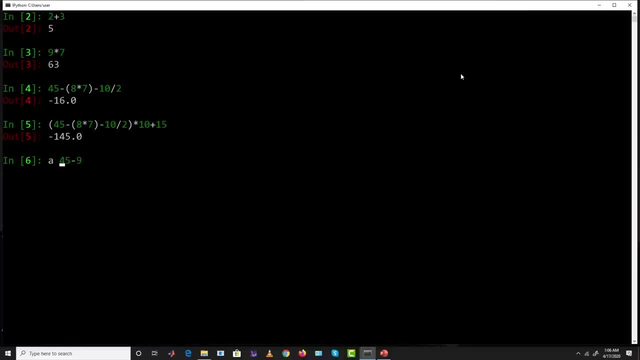 45 minus 9. and let's say you compute this result, whatever the result is, and you save that result in a symbol. let me call that symbol as a variable and here the variable is a. let's say you save that in a. and then you have another variable, let's say b, and three static. 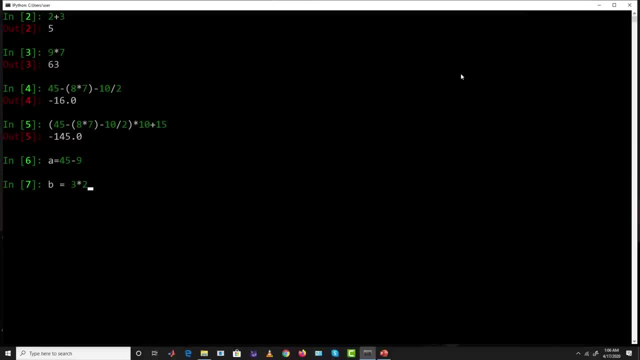 45 or maybe 3, hysteric 2.6, that is saved in b. now you have, you have done this particular calculation, you know that 45 minus 9 is in a, the result is in a. and then you have this particular result that is in b, and now you just want to add the two results together and you want: 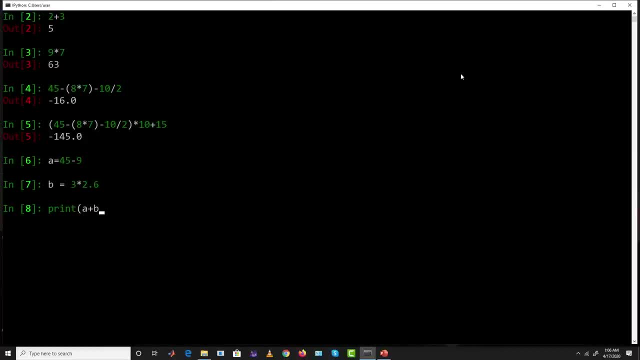 to print the what. what normal calculators does not have Hola and select. the numbers are known as three. so the ctrl v, $$- ladies don't have to use alt values to stay awake. b and it's larger where it's going to matter in the link as much as day. 0e$. it's 100% zero, but i don't. 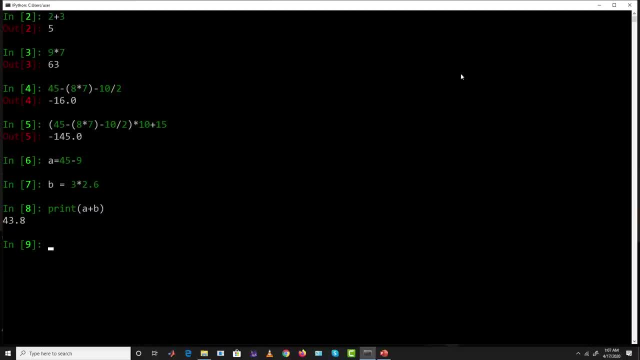 does not have the support of saving the results and reusing them. but here in Python, even if you just want to use the Python just as a calculator, you can declare as many variables as you can and you can save the previous results. you can retrieve the previous results and you can use the previous results save. 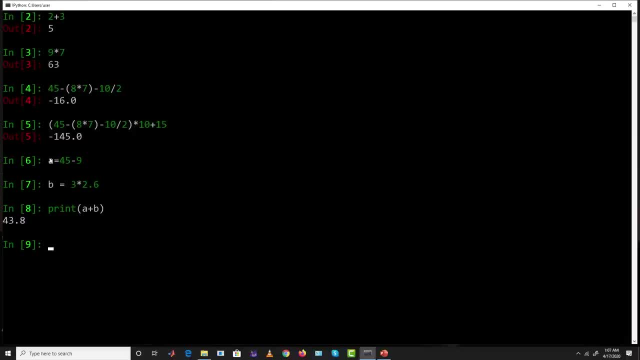 new results and so on, these kind of symbols that are used to save the results and then they can be just used afterwards. these are called variables, and our next video will be on variables. what are these variables? what are their types? what kind of variables the Python supports one way or the other, if you 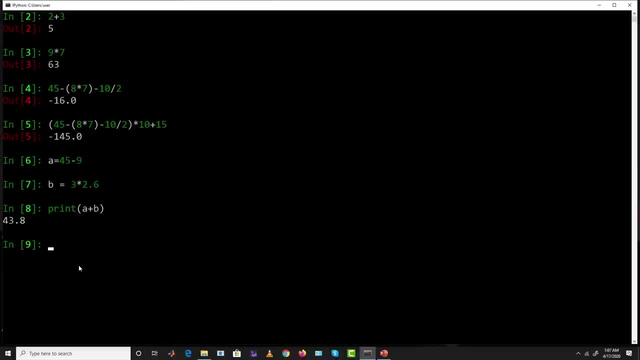 want to go beyond calculators. you need certain results to be saved and retrieved- retrieved afterwards- and the variables are: are the constructs, the variables are the features that that actually do that. so the the calculator is fine. you can use it as a calculator. if you want to use it as a calculator, you can use it as a. 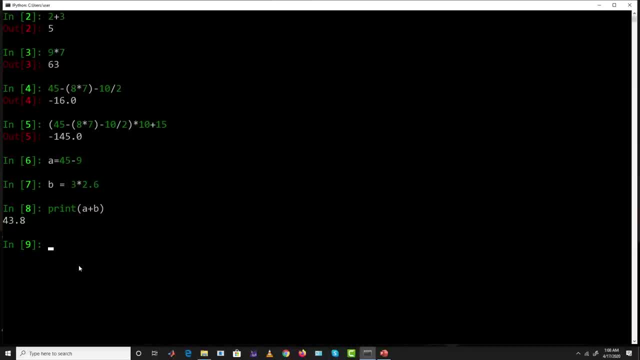 Python shell just as a calculator. but if you want to do interesting programming- complicated programs, I mean, you want to achieve a task that involves much more calculations- one way or the other you have to save certain results in somewhere and then you have to combine the results together, because the longer problems in 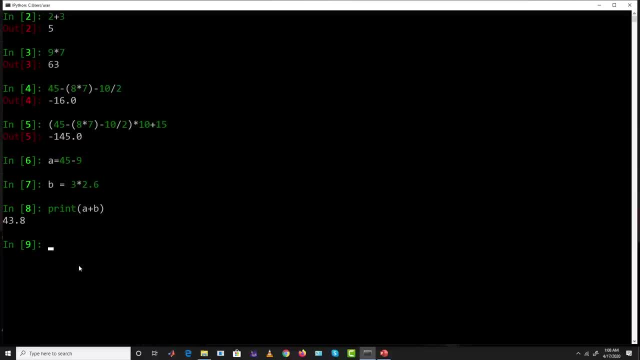 normally are broken up into a smaller piece of problems, and each smaller problem has a result that should be saved somewhere, and afterwards the several results they should be saved somewhere and afterwards the several results they should be combined to achieve the result that we are after. so these variables are: 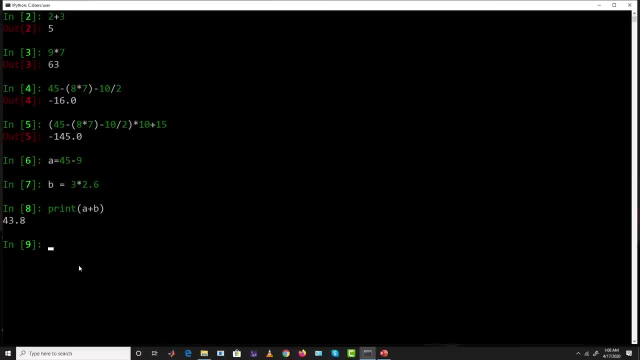 required if you are going to do some interesting or complicated calculations or computations. so you, by the way, before before having these Jupyter notebooks that are just the enhanced variant of this IPython shell. the IPython shell just. people used to write a lot of Python programming just in IPython shell. 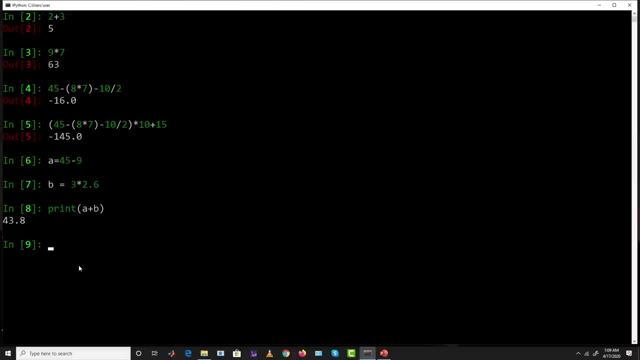 and even even today's several people are writing their code, complete code, in in IPython shell. but the the Jupyter notebook. it is more enhanced for you and more documented more. I mean it has better interfaces and several features that are better than just using IPython. 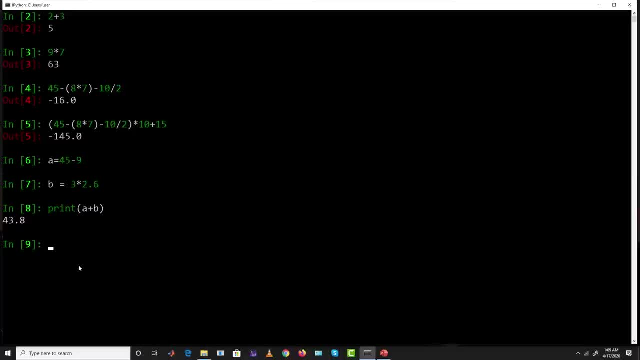 shell. so you have seen this IPython shell. it's very powerful, great. everything is fine with it. but we will be using Jupyter notebooks, which are just the enhanced variants of this IPython, for our upcoming coding. so the purpose of this video was just to, was just to introduce you with IPython shell, and just 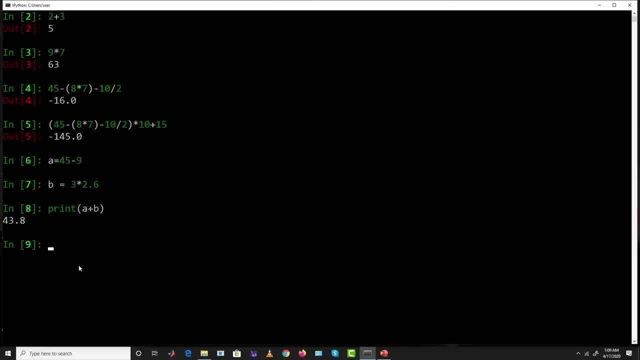 to tell you that you can use Python just as a calculator and even more than that. and in the next video we will be introducing variables in Jupyter notebook and we will see the Python- or Python- is really really much more powerful than just a calculator. so hope to see you in the next video. 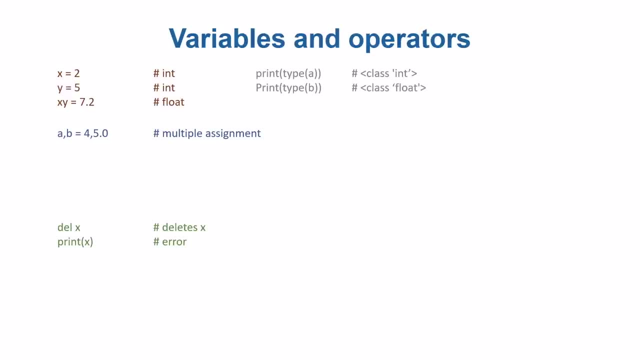 okay, in this video we will talk about variables and operators, the operations that you can perform on on variables. a variable, in a very layman term, is basically a symbol that stores some data that can be used later on. so, for example, this X is a symbol corrector, or a symbol Y is a symbol, XY is a symbol normally, and. 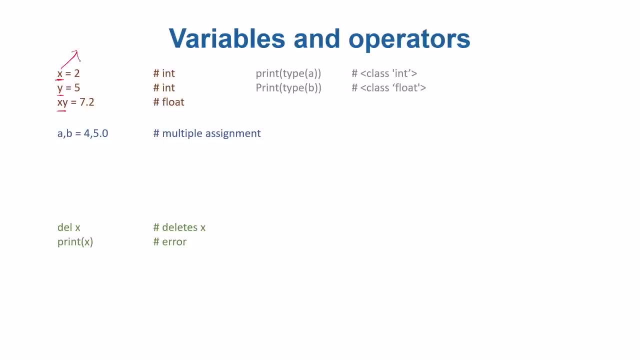 these are called names of the variables. for example, this is a variable name, X, Y is a variable name, Y, XY is a variable name itself. now, these variables, they can store different kind of data. I mean, whenever you want a particular data to be used again and again, it is better to save that data or label that data by a. 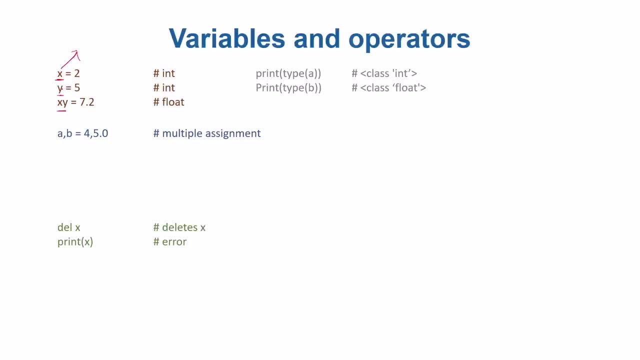 symbol by a descriptive name, so that you can retrieve that name, retrieve that data by using that label or symbol. so, one way or the other, this, this variable, actually is a description of the data that you want to use or store and you want to use later on in your program. different types of data are there for. 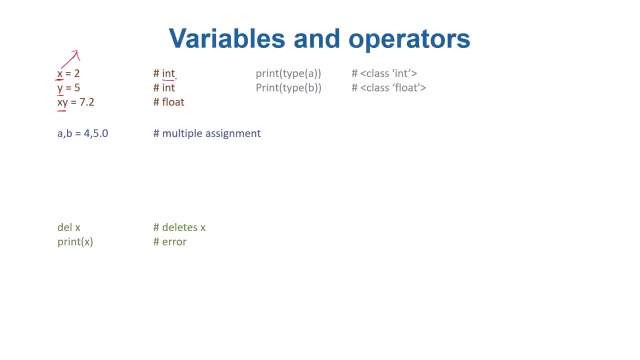 example, the integer type data. for example, if the data you want to store is integer type, it's a number and the number is just the integer number. it does not have a decimal point expansion. that is a type of data and that can be stored in a variable, in that, in that case, the variable type itself will be integer. you. 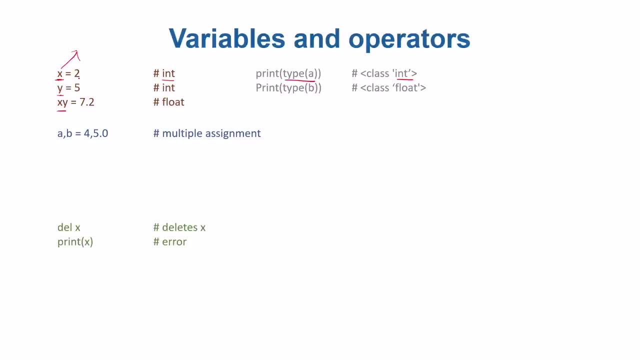 need not to specify the type of variable when you are storing the data to it. the storing data to a variable is sometimes called assigning data to a variable or assignment. for example, if your variable is X and you are assigning a value, let's say 2, then 2 is integer value. it's integer. it does not have a decimal. 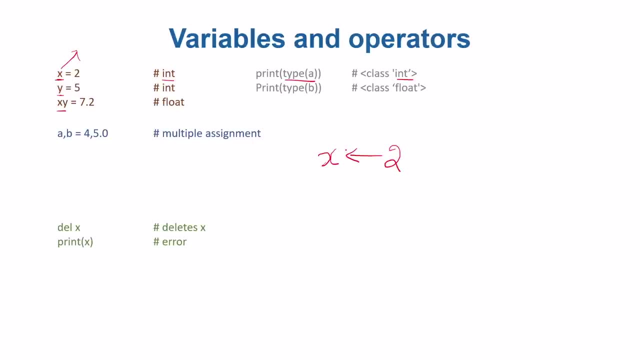 expansion, and when 2 is assigned to X based on the content 2, that 2 basically is an integer type value, automatically this, the type of X, is set to be integer, and that is sometimes called the dynamically typed Python is dynamically typed language or dynamic typing. you need not to specify the type of the. 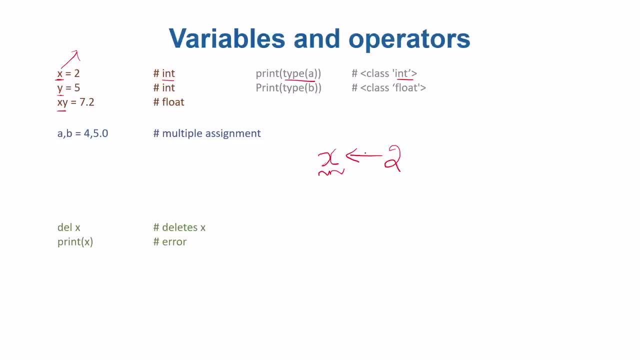 variable, the contents that you are assigning to a variable did. they will define the type of the variable on the fly and the assignment. for example, in here I am storing 2 inside X and next time if I want to print, for example, what is there in X, the, the print value will be 2. now, this kind of symbol is hard to 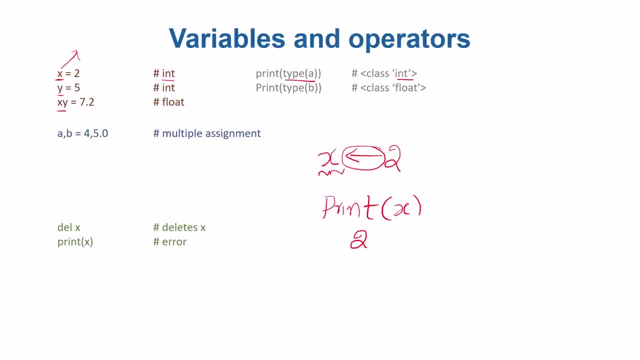 write. there is no keyboard symbol that looks like so. so rather than writing this symbol for a simple type of a variable, you need to define the type of assignment. normally, an equal sign symbol is used for assignment. for example, X is equal to 2. that means 2 is assigned in X. 5 is equal. 5 is equal to 5 means 5 is. 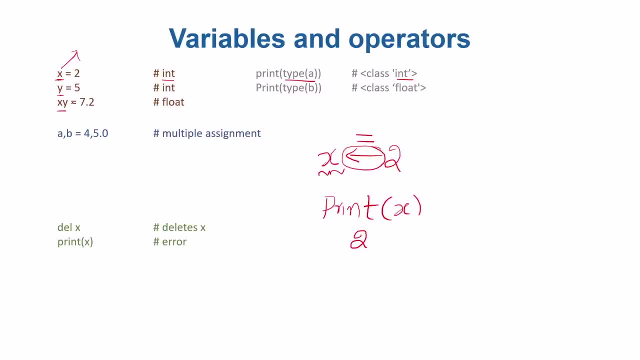 assigned in Y: 7.2 equal X. Y equals 7.2. XY is completely a new variable. it has nothing to do with X or Y and it is handy sometimes to to to suggest the name of the variables that are too descriptive, that are very, very. 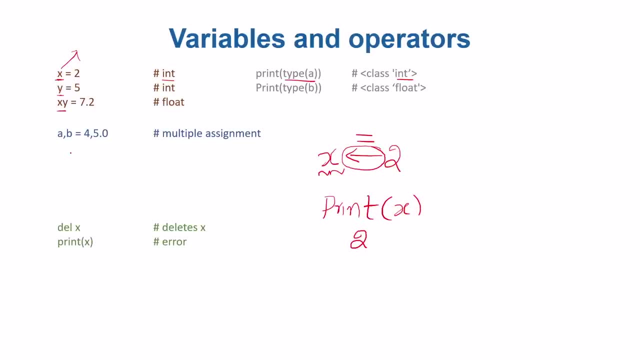 difficult to be used to increase the readability and management of the code, because later on you will- you'll be seeing when you will be working in data science and other stuff. the programs that you will be writing might not be very short programs, they might be lengthy programs. so readability of a 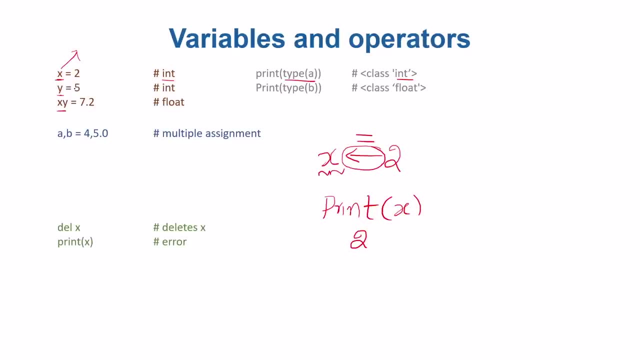 program and management of a program becomes an issue if you, if you, if you do not assign the names of the variables carefully. however, if you write the names in a very descriptive way, by just reading the name of the variable, by just reading the variable symbol or or or the name, it tells a better look and feel of what kind of data inside and what. 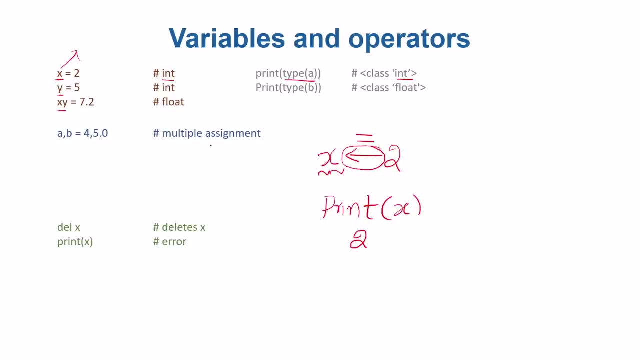 should i do with that? so i was talking about this equal sign. this equal sign is used for assignment here. for example, when 7.2 is assigned to a variable- x- y, automatically the type of x- y- variable is set to be a floating point, floating point number. a float is a data type in in python. 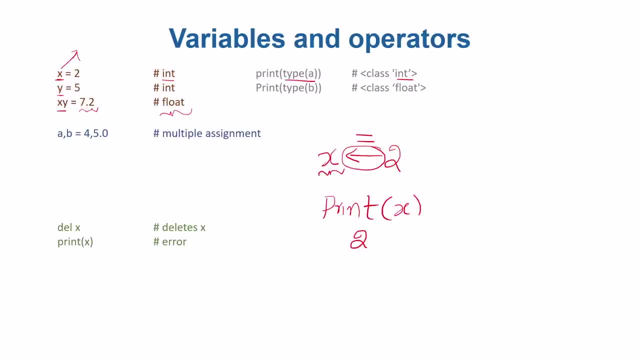 that describes that the particular data is a real value. it may have a decimal expansion as well. uh, not just integer and floats are the only data types in python. there are several others. for example, you can define complex numbers if you, if you want to, you can, for example, 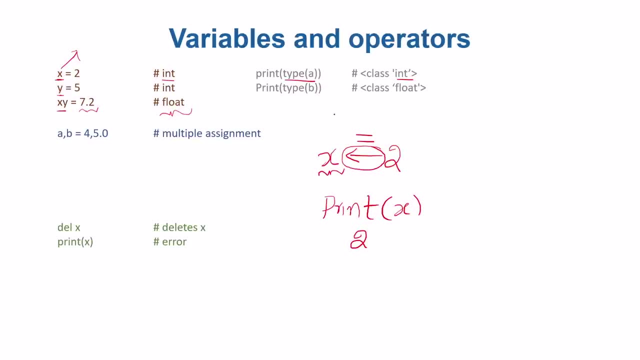 defining a complex number might be, for example, you write the name of C and you write 2 plus 4 J. if you write the symbol J here, it automatically becomes complex and now you can. you can use this. see the way the complex numbers should be treated. similarly, there are other data types. 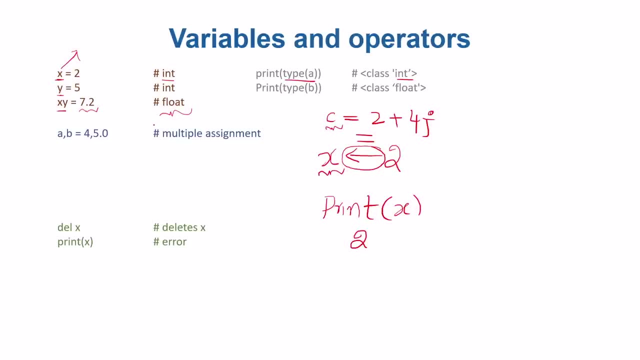 like fractions, decimals, there are. there are further data types, the objects called strings. for example, if you, if you, if you assign, let's say, s equals double quotes, hello, then that s is also a variable and the type of this variable is string. string is just a sequence of a lot of correctors. where H is a character, E is a. 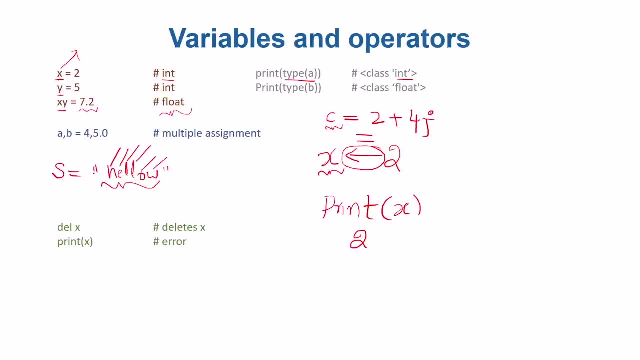 character L is a character. L is a character, always a character. W is a character. and when we will define anything, any sequence will be defined as a variable. and when we will define any sequence of characters inside the double quotes and then end the double quotes here or 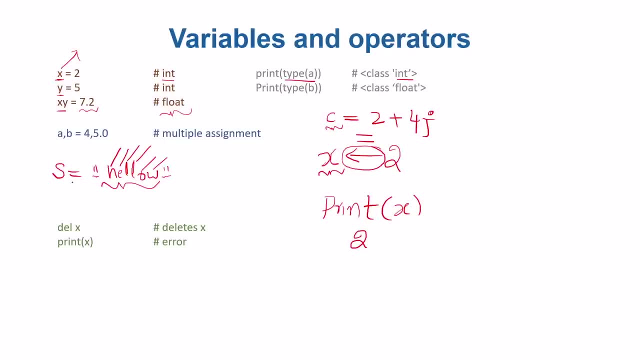 the single quotes. single quotes and double quotes either way. then the type of this s becomes strings and these characters should be treated as it is like. for example, if we have another variable, s2, and we just say 1, 2 in double quotes, now this s2 is no longer 12 as an integer, it is a sequence of. 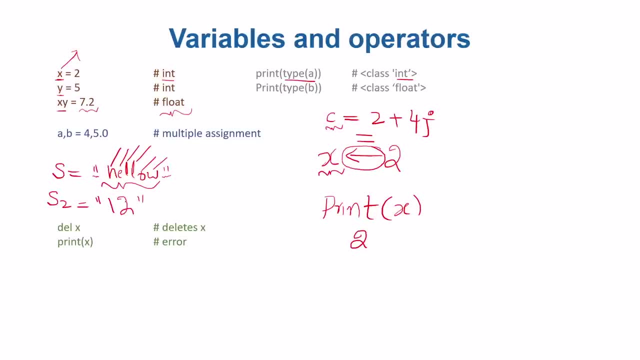 characters. where first character is 1, another character is 2, we will talk about strings as an integer and we will talk about strings as an integer and we will talk about strings in detail in the upcoming videos, but just to give you a look and feel that Python actually supports a lot of data types, a lot of 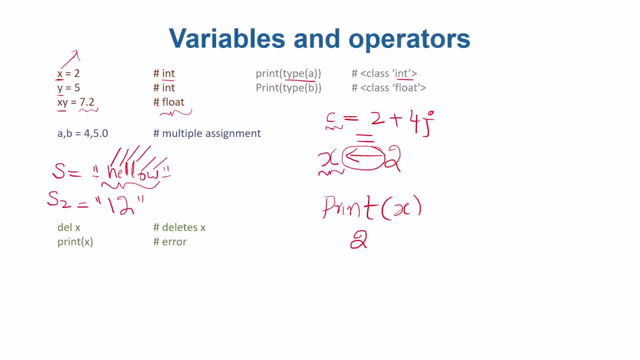 interesting data types, including the most important data type is integer, float and string as well. that we will see in detail further. you can assign. you can assign more than one values to more than one variables in in a single line. that is sometimes called multiple assignment. for example, if you write a 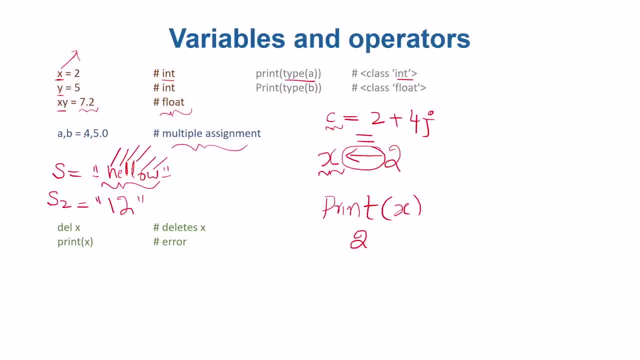 Vietnamese version of A and if there is something that I actually don't see ultimately pointing towards A, for example. so at this point, when we write the real location, they stay in the memory, they occupy a particular space in inside the memory. for example, x is just a label to a memory, the inside the memory there is two located somewhere. similarly, y is also. 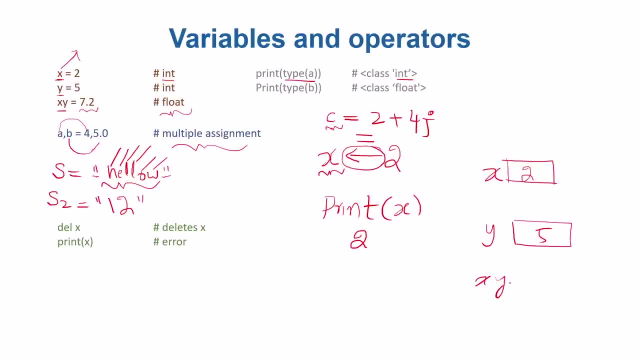 located somewhere in memory and similarly, x, y is also located somewhere in memory and this is the data inside that memory. these will stay in the memory and they occupy the memory. if you, if you decide to no longer use a particular variable in future in in the program, then you can call. 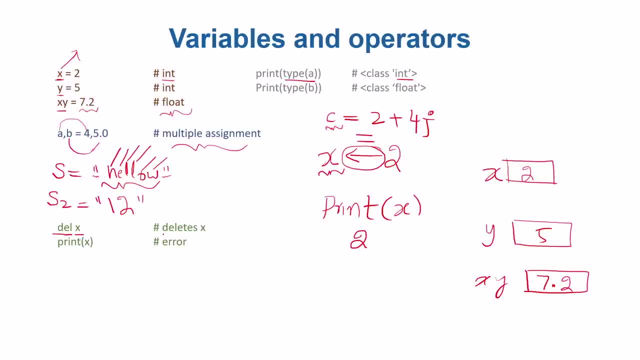 this function del space, whatever the variable name, and it will delete them. it will delete the variable from the memory like it was never there and once the variable is no longer in memory, it is it is not accessible. if you now access the variable again, you will get an error. let's see. 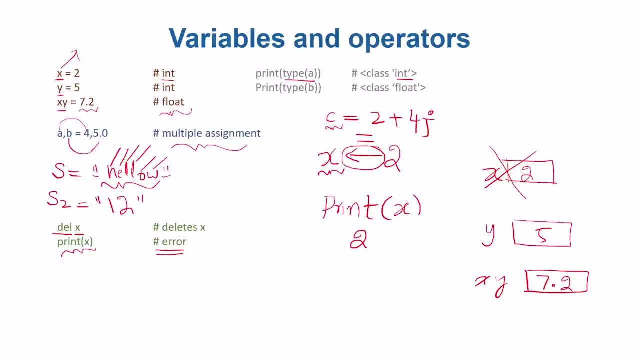 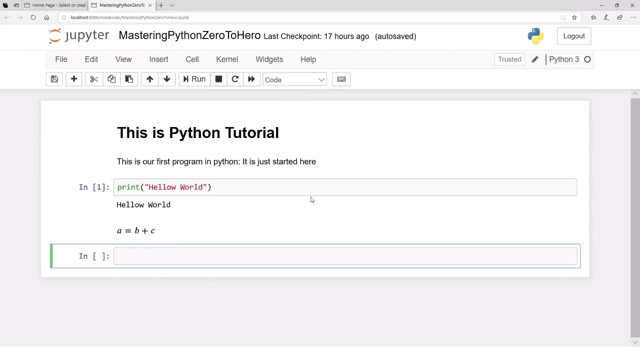 all these concepts. let let's see most of these concepts in Jupyter notebook and let's let's actually define certain variables, use them, print them, do some multiple assignment and see a lot of stuff in in Jupyter notebook. so let's go to Jupyter notebook. so that was our notebook, that we were. 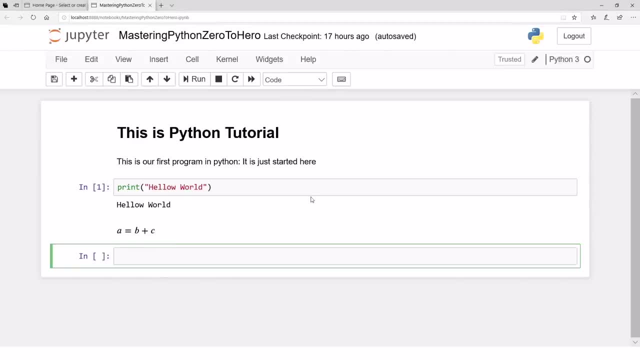 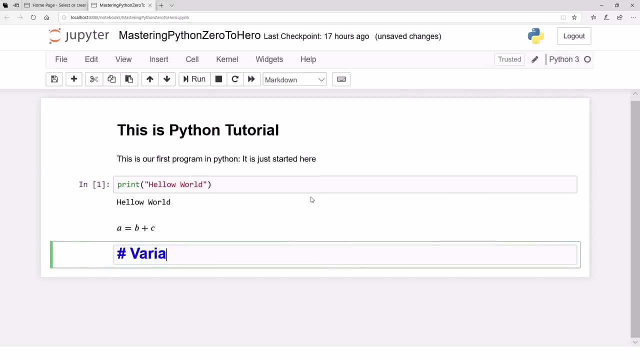 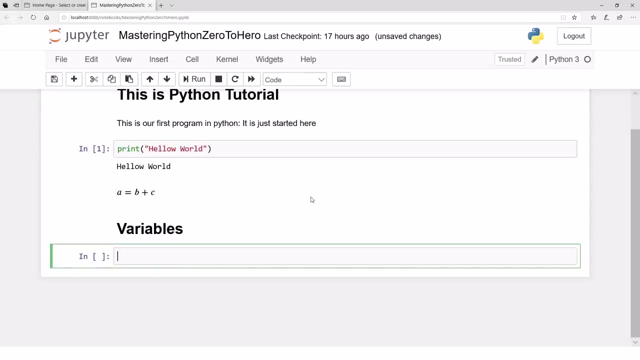 doing that. we were actually working on the last time. so let's say I define a variable X. let's say X is 2, why not? I should describe this as what we are doing here is, let's say, variables. so just to give a heading, that we are now in variables, so variables. notice that. 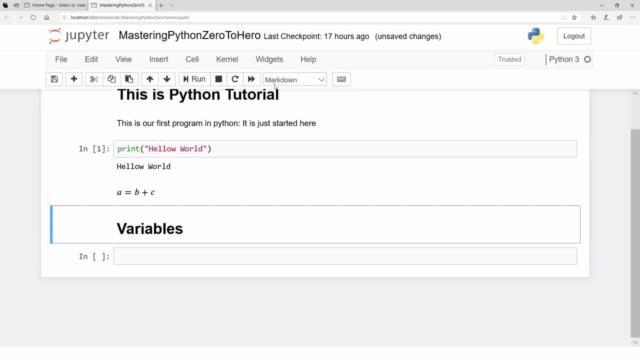 now I'm in a code cell. previously I was in a marked down cell. notice this change in this particular cell. this is marked down in this particular cell. this is code cell. see that code cell. okay, X is equal to, let's say, 3. let's enter this now: X is assigned a value 3 if 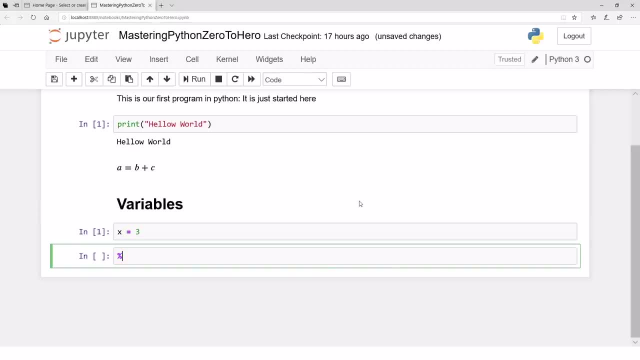 you want to know how many variables right now are there in the memory, we can write this command whose this is a percentage symbol. if you write percentage symbol and then just type a command, WH OS, it will tell you all the variables that are right now, that are there in the memory and right now the 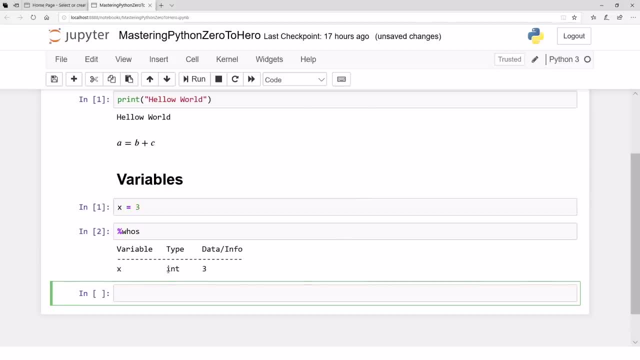 memory has a variable with name X, it's type is integer and the data inside the variable is 3. that's the memory view that you are now seeing. okay, if you want to explicitly check the type of X, you can print type X. so, for example, this function type will will actually finds out the 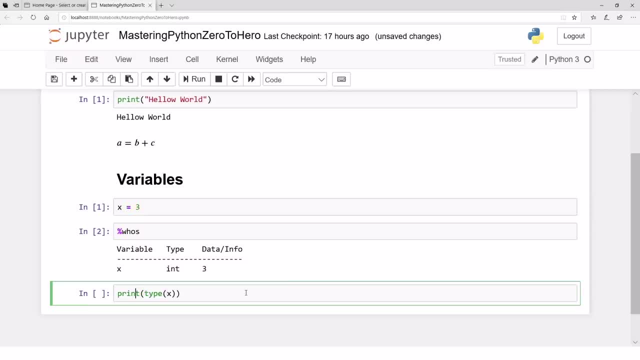 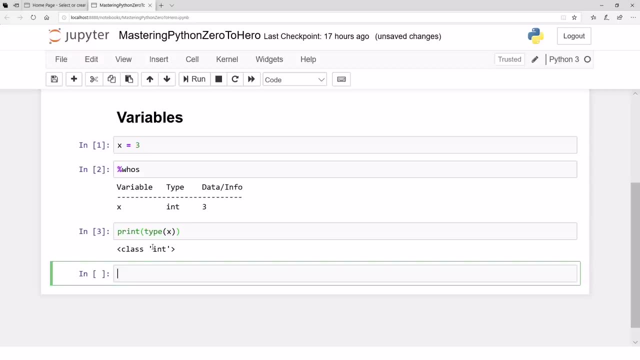 type of every variable you give inside, and then this print function will help you printing that on the notebook. So if you see the type of x, the type is basically its integer type. Now if you, for example, change the value of x as 3 to, let's say, 5.7.. So you have same variable. 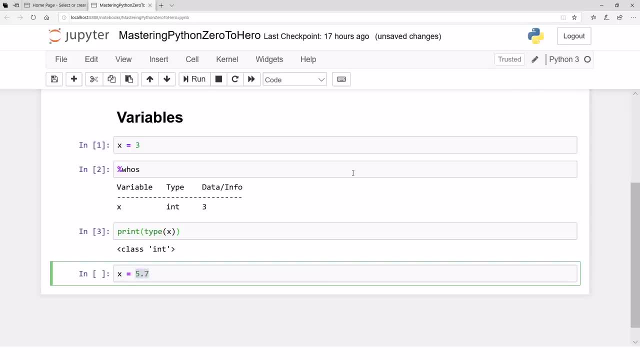 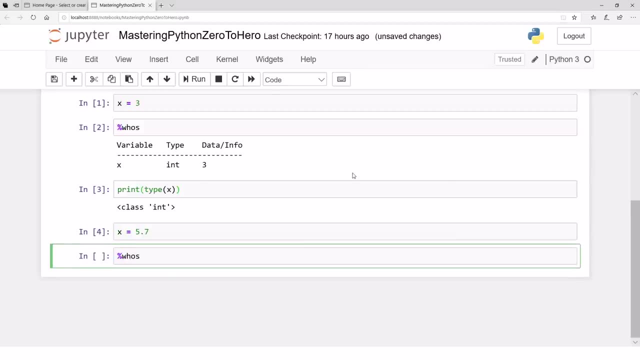 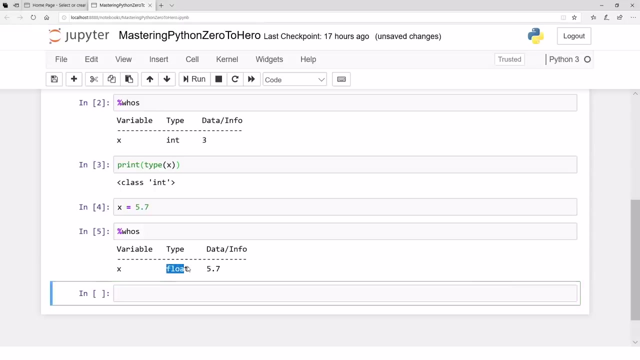 but you just change the value from 3 to 5.7.. So let's see what happens now. So if we call whose again, we have now the variable name is still x, but its type automatically changed to floating point number, because we assign a floating point number to it and this is: 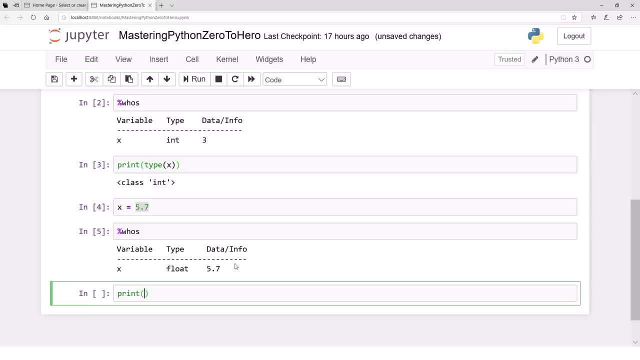 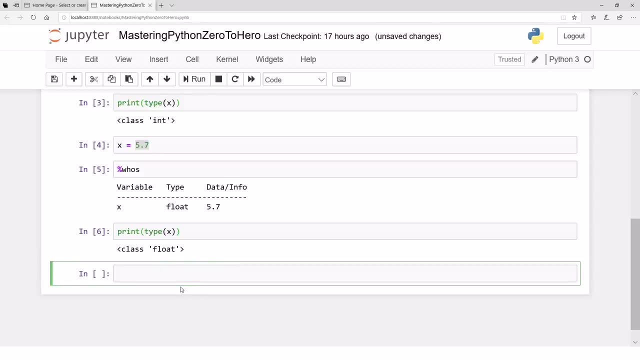 the data. If we want to explicitly check the type of x, let's say 3,, 5,, 6,, 7,, 8,, 9,, 10,, 11,, 12,, 13,, 14,, 15,. 16,, 17,, 18,, 19,, 20,, 21,, 22,, 23,, 24,, 25,, 26,, 27,, 28,, 29,, 30,, 31,, 32,. 33,, 34,, 35,, 36,, 37,, 38,, 39,, 40,, 41,, 42,, 43,, 44,, 45,, 46,, 47,, 47,, 48,. 49,, 50,, 51,, 52,, 52,, 53,, 53,, 54,, 54,, 55,, 56,, 57,, 58,, 59,, 60,, 61,, 62,. 63,, 62,, 63,, 64,, 65,, 66,, 67,, 67,, 68,, 68,, 69,, 69,, 70,, 71,, 72,, 72,, 73,. 74,, 74,, 75,, 76,, 76,, 77,, 78,, 78,, 79,, 79,, 80,, 80,, 80,, 82,, 83,, 84,, 85,. 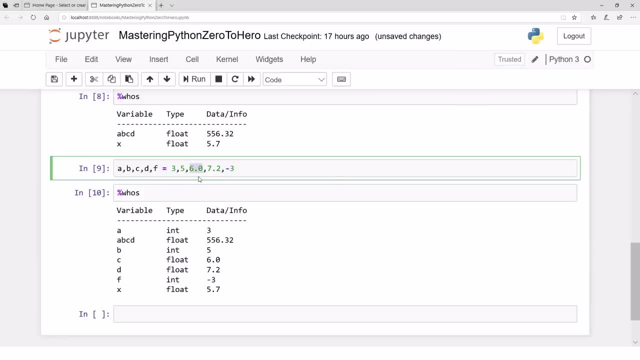 86,, 87,, 88,, 89,, 70,, 70,, 80,, 80,, 100,, 100,, 60,, 140,, 110,, 150,, 120,, 120,, 14 ABCD variable. ABCD, that's one variable that we don't want to use in future and 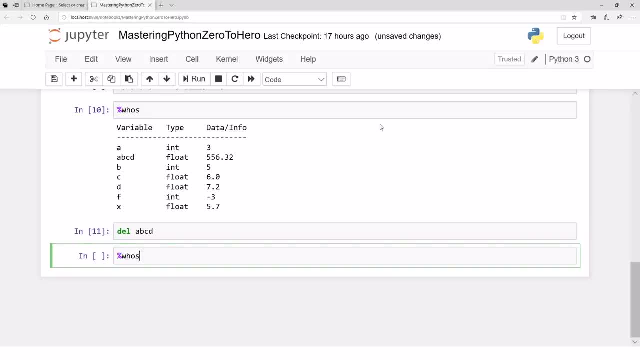 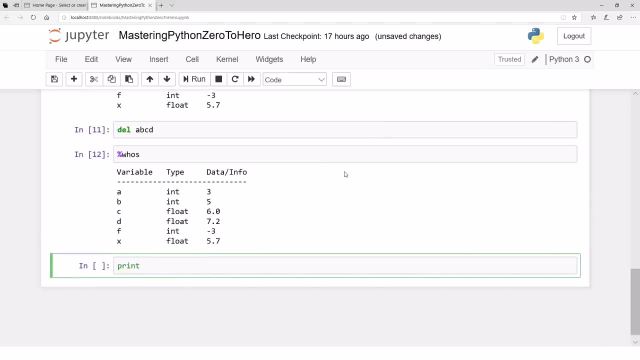 now, if we see again the view of the memory, we don't have this- and if we now want to access this- for example, if you want to print this ABCD- we will get an error. we'll get an error and we should. we should get an error because this: 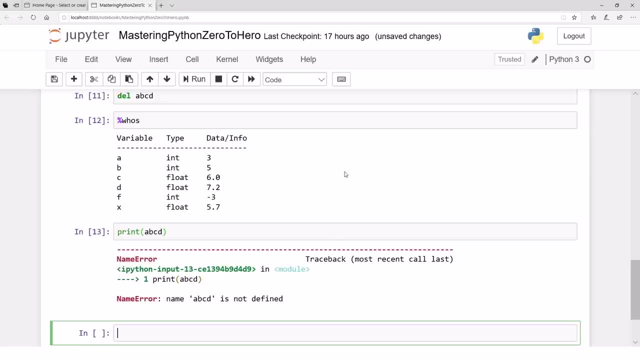 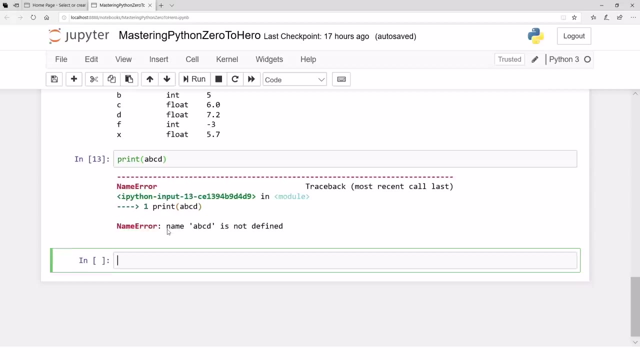 particular variable does not exist in the memory. it points to no data. it has gone. it has gone like it was never. it was never there. so that's about the variables. we just talked about integer and float. there are several other variable types as well, for example- let me just give you an example of an. 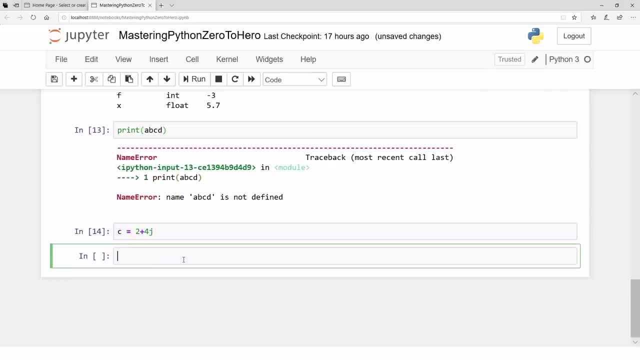 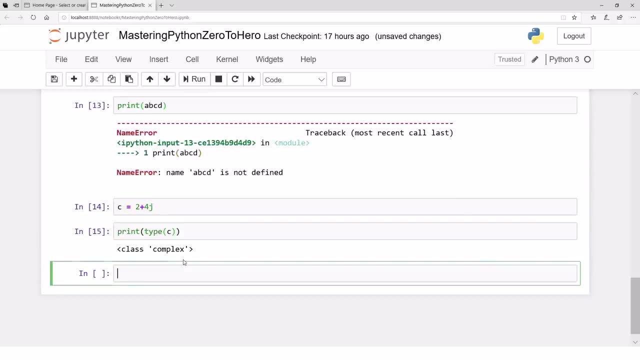 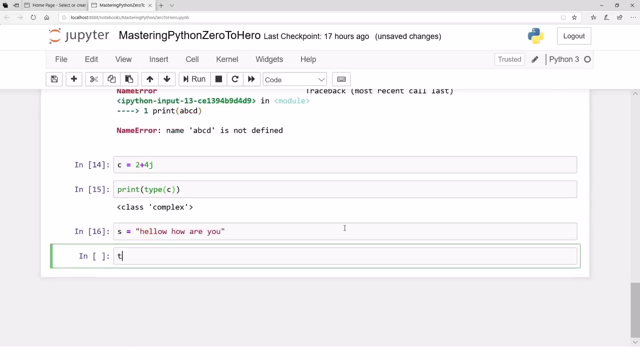 example of a complex number. if you are really interested in that's a complex number, if you print its type, so that the type is complex. similarly, you can have a string variable. let's say: hello, how are you? that's a string variable. if you print type of this, you. 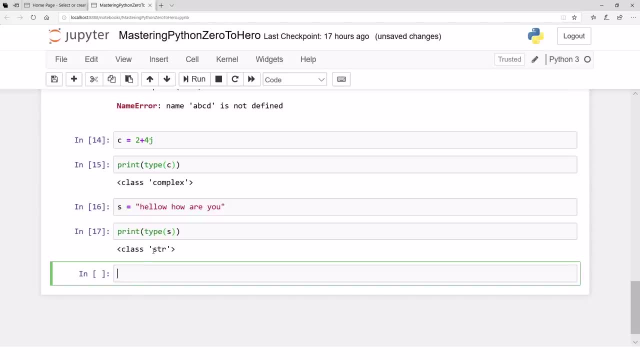 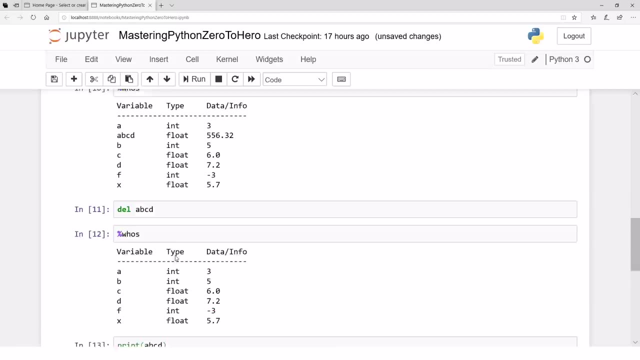 will get a string. we will. we have a whole set of videos just on string data type, because this is very important data type. we will. we will see that in detail, but the purpose here is just to tell you that there are a lot of data types that Python supports and Python is dynamically typed. 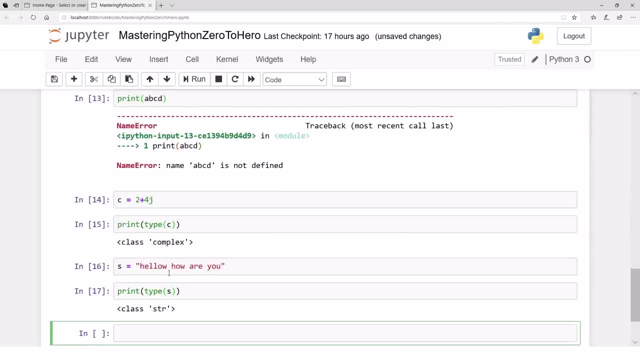 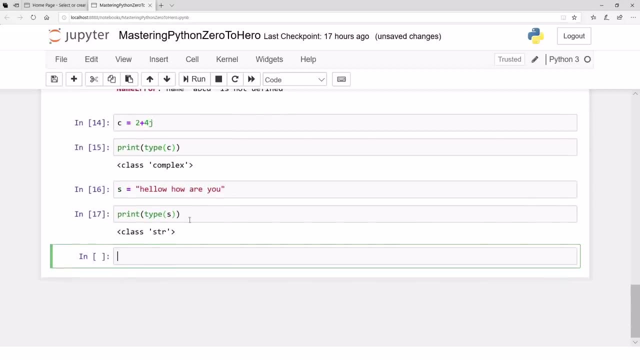 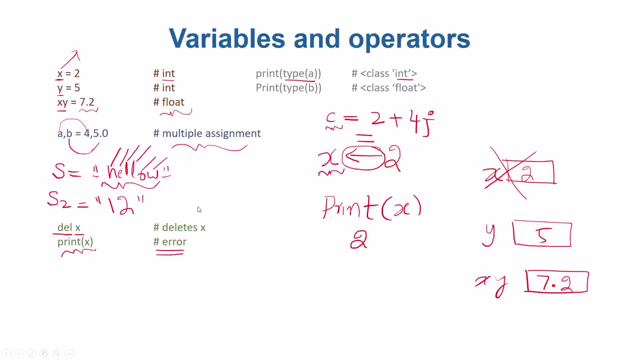 whatever content you are assigning to a variable, the, that content decides the type of the string you need not to specify. so I end this video here. in the next video we will be talking about operators, basically what kind of so? once we have decided one, once we have declared, once we have defined a lot of 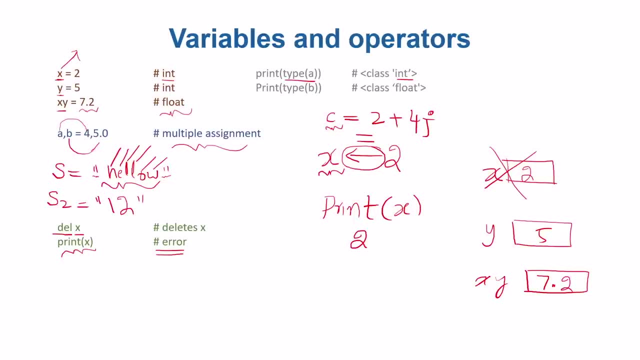 variables what we can do with these variables. can we add two variables together and get the results stored in another variable? can we multiply two variables together? can we have an operation like addition on mix types? for example, one variable is a floating-point number, another variable is integer. 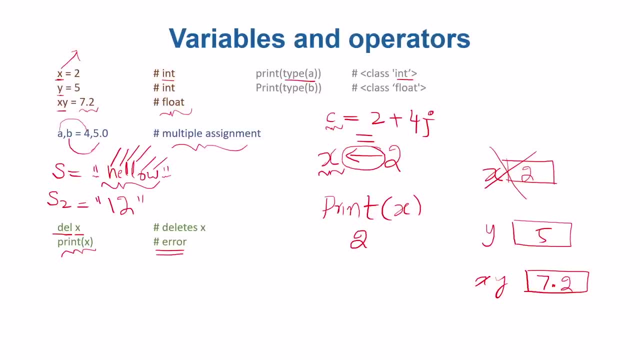 number, integer type. can we mix up those? can we add two different types of variables together and get a result? then what will be the type of the result and so on? so a lot of these discussions on operators, the very basic arithmetic operators, on these variables, particularly the integer and float variables. we will see that in the next video. 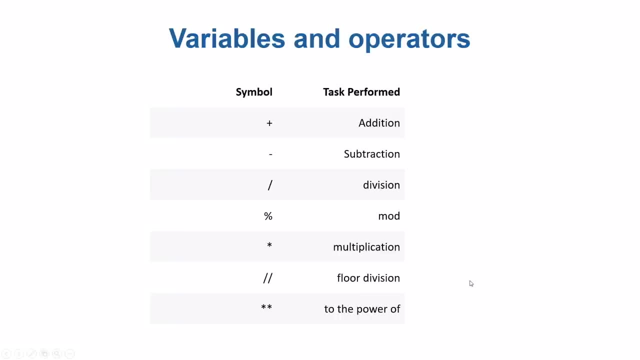 so hope to see you in the next video. so in the last video we saw variables and we particularly saw integer type variable and floating point variable type. we also saw very briefly on Jupyter notebook. we saw complex and string as well. so in this video we are going to talk about 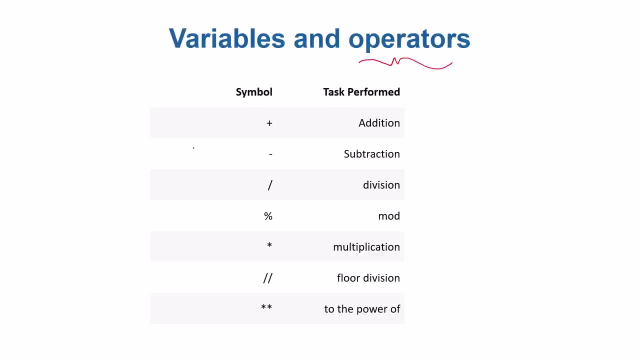 operators, basically the arithmetic operators. obviously, if you are defining variables, you're not defining the them, the variables, just to just to view them. later on, most probably, you'll be storing data to the variables and then you are: you're applying some computation on a set of variables together, computing new results, saving that and doing some stuff. 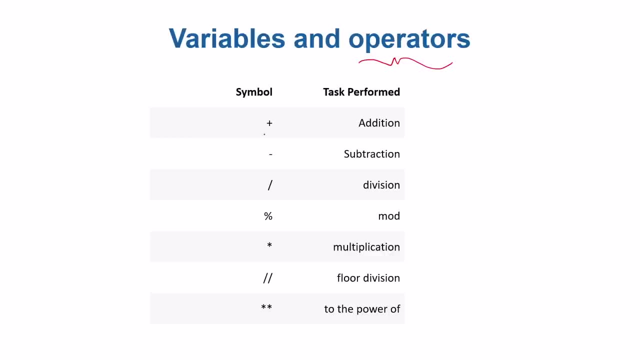 you're applying some computation on a set of variables together, computing new results, saving that and doing some stuff. most probably you will be adding two variables some one way or the other in inside a program. you may have to add two variables. you may have to subtract a variable from the other. you may have. 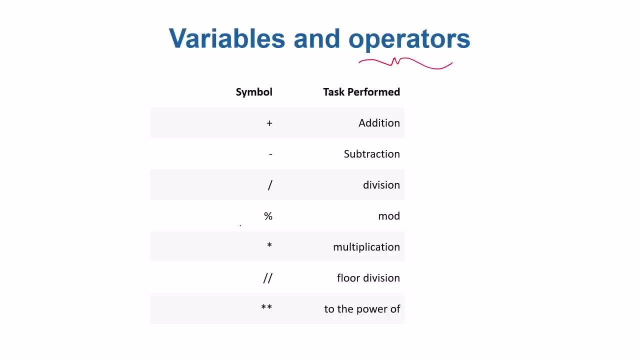 to divide a variable, you may have to compute, for example. these are arithmetic operators. let me let me just this. this plus symbol is used to add two variables. this minus symbol, or subtraction, is used to subtract a variable value from the other variable value. obviously, these all are. 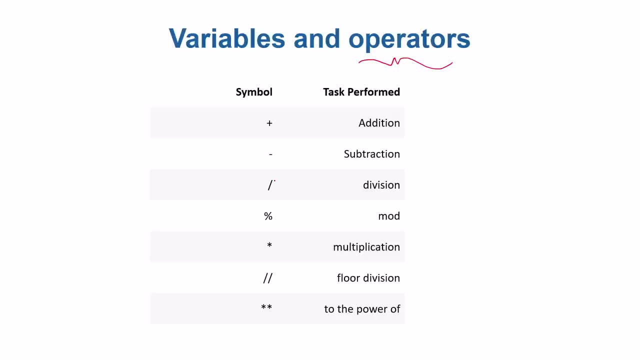 operated on values, not the names, division it like, like the name suggests it's, if you want to divide this, this percentage symbol, when it is applied to two different variables, if X is on left and Y is on right- what it does it? it actually divides X by Y and checks what. 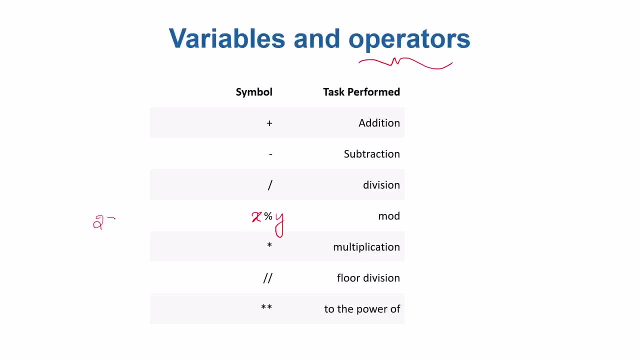 the remainder is, for example, if X is 27 and Y is 5, then what's the remainder? what do you think if we divide the remainder by Y, then what's the remainder? what do you think if we divide 27 by 5? what's the remainder? the remainder will be 2. yes, so the result will be 2 here. so this: 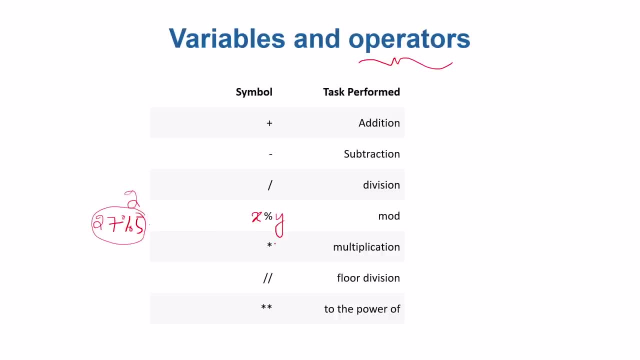 computes the remainder, this multiplication, this star symbol is used as multiplication. like in mathematics, we normally write this cross symbol, but in in Python and in most of programming languages, star symbol is used to achieve multiplication. this double slash is like the division, but it is division. the result flow to the quotient. what I'm saying is the following: for example, if you divide, let's: 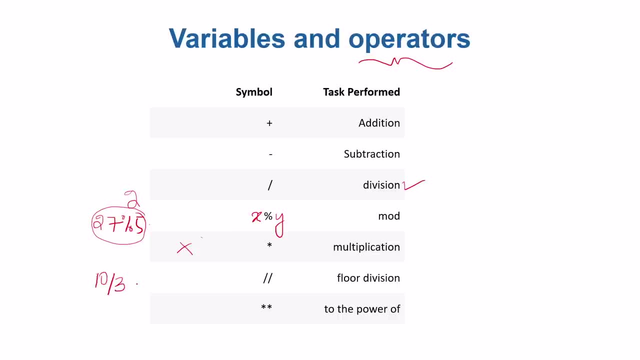 say 10 by 3, the result will be a floating-point number and the result will be 3.33, something like so. but if you want just a quotient, not the remainder, if you want the integer, that's the quotient value 10, you write the double slash 3 and it will return just. 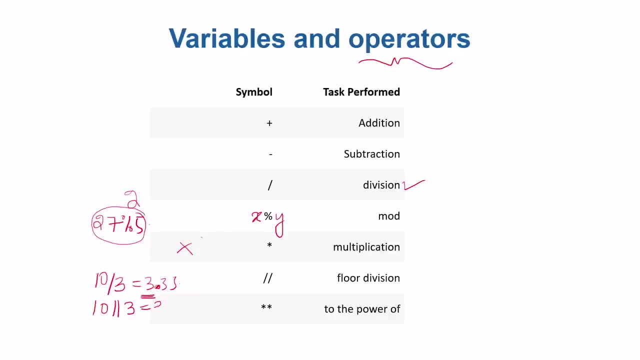 the value, that is that is there before the decimal expansion. so this value will be returned. so this is kind of the integer division or flow division. this double star is used to compute the power. for example, if you want to compute 2, you write a double star, for that means 2 raised to the power, 4. in mathematics we 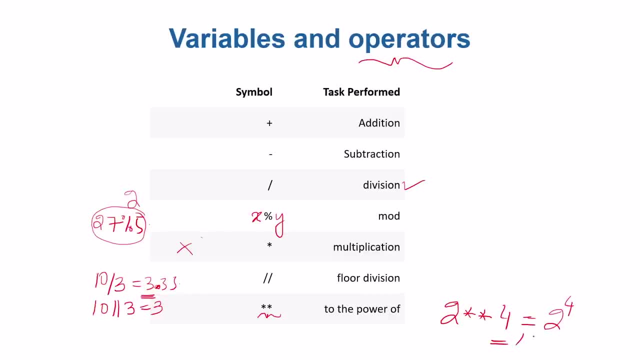 write this as following, and the result will be 16. you can save that result in another way able, or can just print it, or you can write that in a file or whatever. so these are most important operators. one thing that i want to tell you: that these operator are not just for integers. 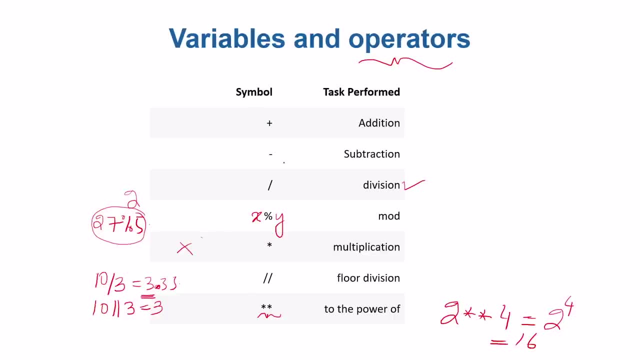 and floating point numbers. the applications of these operators is much broader than these. later we will see the objects or the data types that are collections, and very i mean the data types that are beyond these integers and floats. and still there, this plus, minus division, and all some of these, or all of these, they have their meanings there, even even even this plus is used. 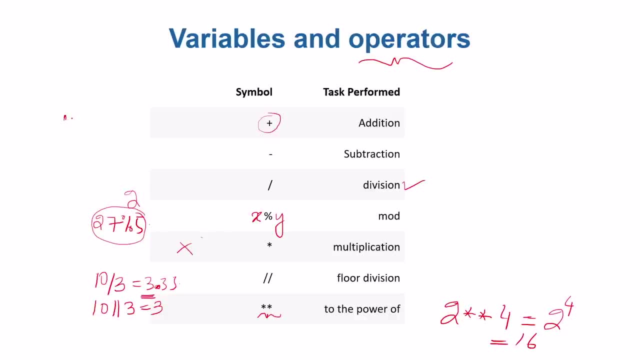 for strings. now think, for example, if you have a string- let's say hello- and you have another string- for example let's say this is string s1- and you have another string, let's say s2, which is y, then python allows you even to add these kind of data types, although some doesn't make any sense. 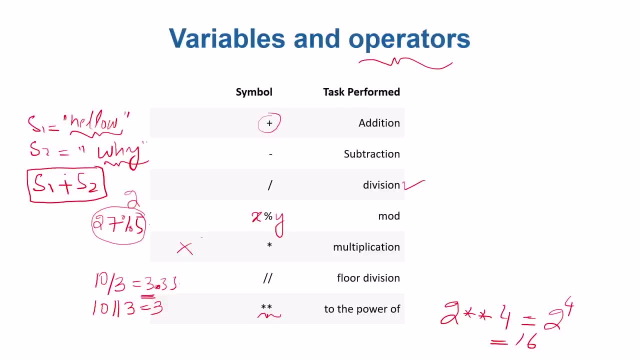 with these kind of string variables. but we will see, for different kind of data types, the the definition of these operators. they actually change or adapt it accordingly. for example, in mathematics we are much more fluent in for with plus, with division, with subtraction, and it makes sense to. 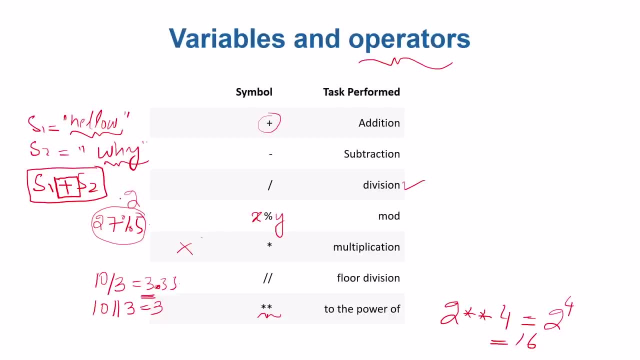 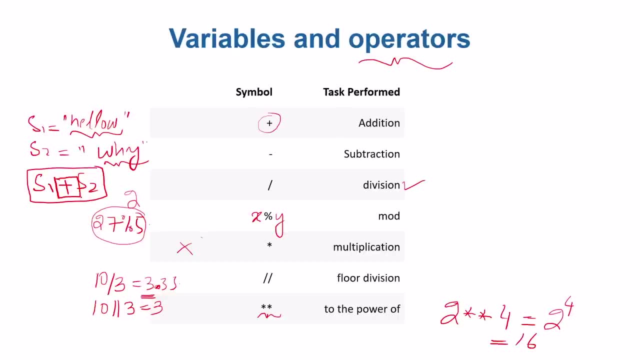 to you. right now these operators may not make that sense to you, but there are definitions there, there are ways to use these variables for the data types that are even, that are even beyond the integer and floating point numbers. we will see all these details as we move on, as we move on to 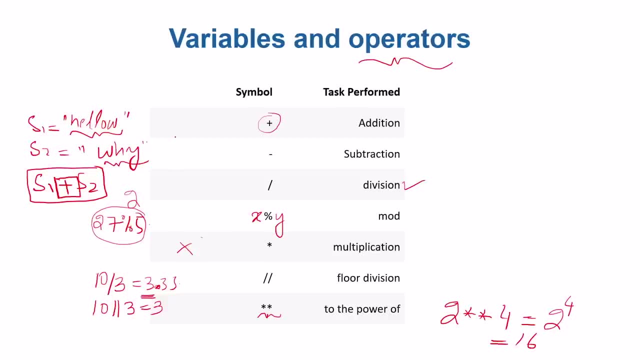 as we move on to the videos and- uh, i mean as in in later on we will see all these things in detail. but just to tell you that these operators are not just limited to integers and floating point numbers or complex numbers. they can be applied to several different. 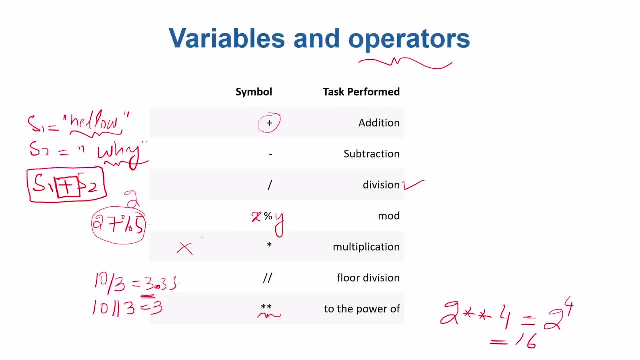 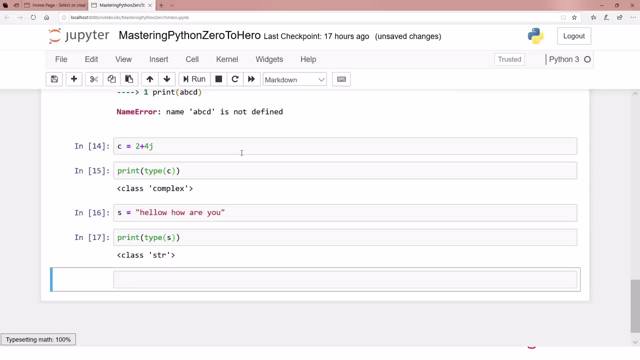 data types. so, um, a lot of words. i guess you are bored. now let's go to jupyter notebook and have fun with these kind of concepts that we are dealing with. so, uh, yeah here. so let's first press escape, then m just to change it to markdown, and then escape one for heading, big heading. 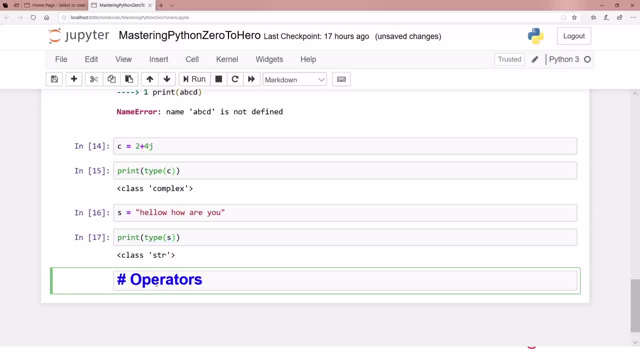 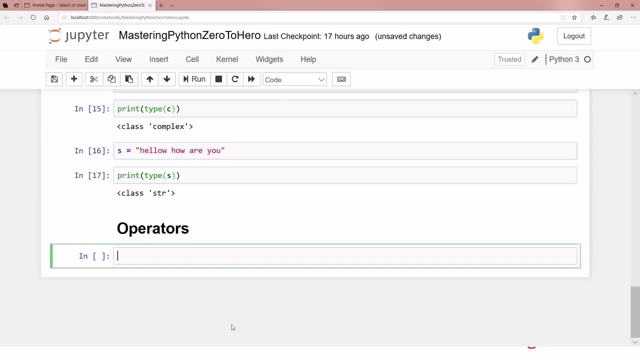 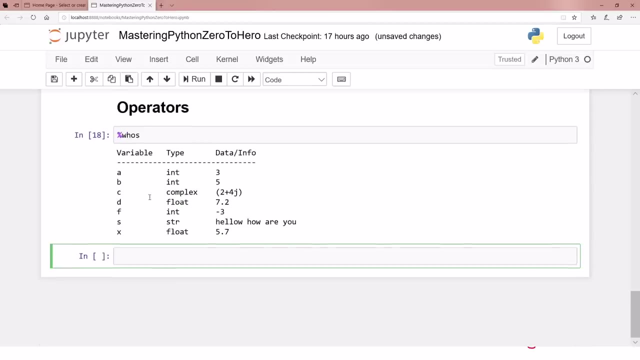 and here i write, let's say, operators, and shift, enter, it runs and automatically then go to code. okay, now let's say i have a variable, so let's say what kind of variables i already have. in the previous video we used that, so we already have these kind of variables with us. 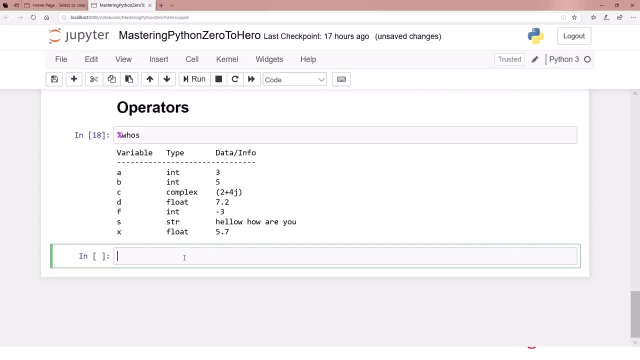 you now what is? let me define a new variable. let's say sum of sum of a- b. that's a new variable. sum underscore a- b, that's a variable name. you can have a better variable name, maybe sum of a and b, that might be a variable name. 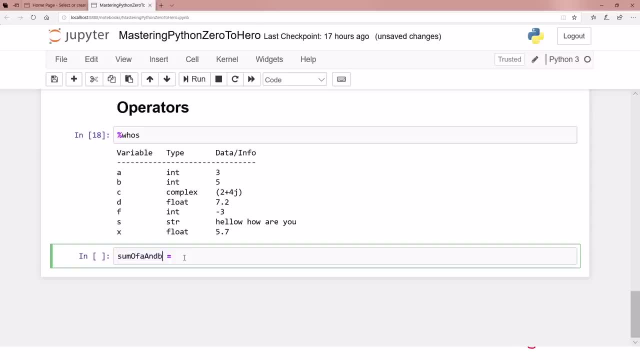 it is good to have the variable names that are descriptive, that describe what data is inside um, because in in programs the programs become manageable, readable and a lot of benefits are there. so sum of a and b, let's say that's a variable name and you add a- b, you just write a plus b. 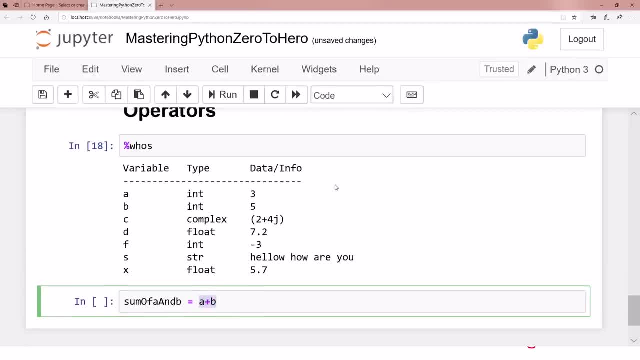 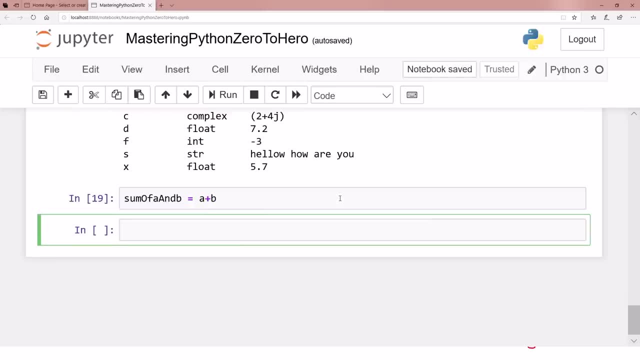 let me make the zoom level a little high so that you can see it clearly. so a plus b, let's say that's there. if you press shift, enter and now you print sum of. by the way, if you have written some off, you need not write everything. 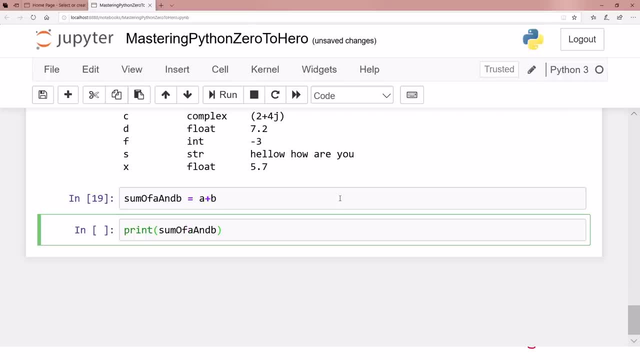 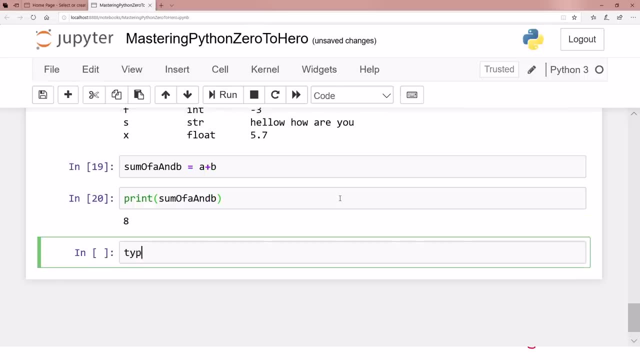 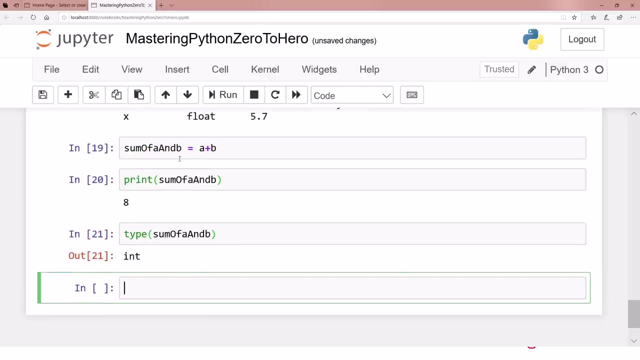 just press tab and it will automatically complete the remaining part of the variable, and press shift, enter and you have eight. if you check the type of this variable- sum of tab or automatically completes tab- that is called tab completion- wow, um, it's integer. the type of this particular variable is integer. that's a new variable and 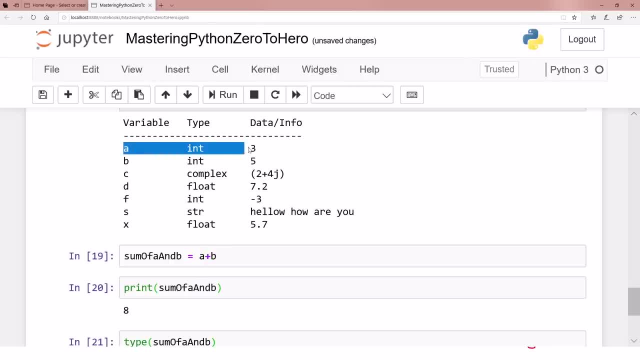 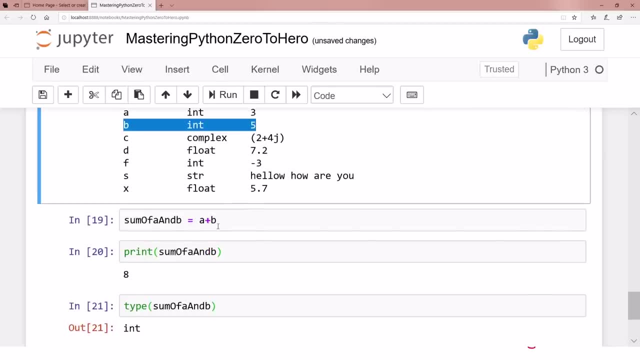 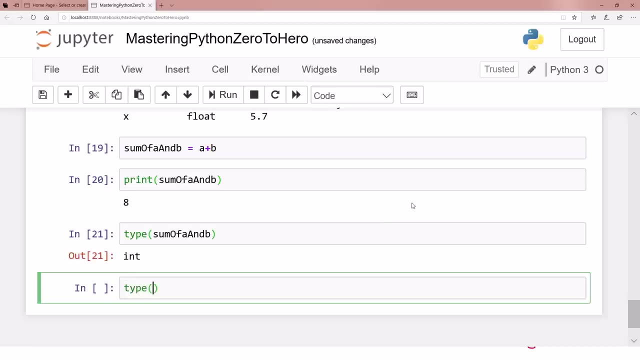 why the type is integer, because a was integer, b was integer and integer plus an integer is an integer. what if we add an integer with a floating point number? what do you think what should be the result? if i just type type a, that's an integer plus. 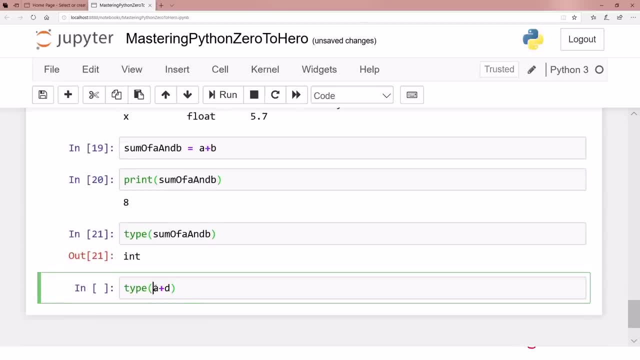 d with some floating point number, so a plus d. the result will be here and type of that result. what will be the type of that result? what do you think? let me pause here, uh, for a few minutes, and oh, no, no, no, not for a few minutes, for a few, maybe seconds, maybe two or three seconds. what will be? 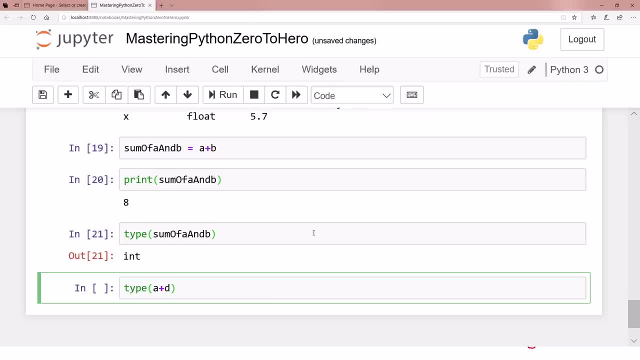 the result. what will be the type of an integer and a float combined? well, um, the types are up, costed by default, because you have a floating point number. the result will be a floating point number. and the reason is: every integer by default is a floating point number. floating point number is a 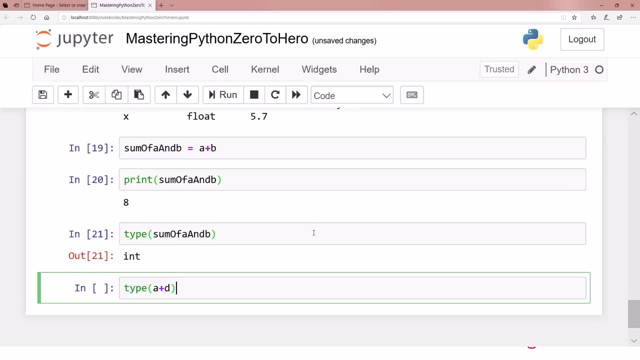 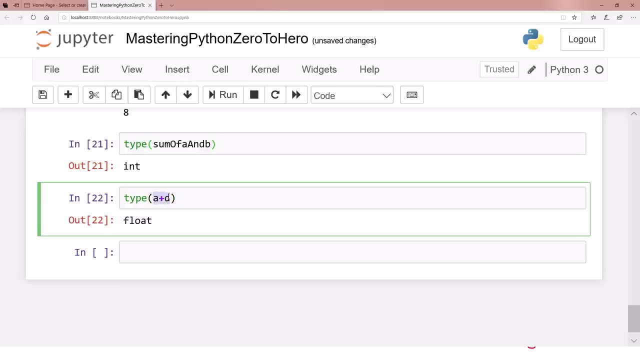 is an upper class or you can say a superset, so a python. in python, by default the types are up costed to super supersets. so here, integer plus a float, the result will be a floating point number. and that's the result you. you might be thinking why we have, why we haven't stored the result in. 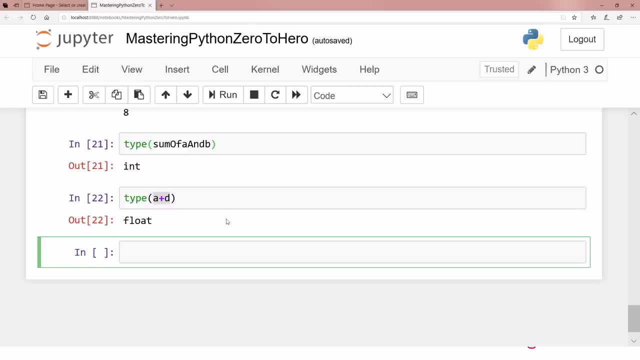 want to store the result in another variable, we can. or if we just compute the result and apply some operation on that, we can do that. for example, we. we could do the following: for example: a plus d, that's whatever the result is raised to the power three, whatever the result is. 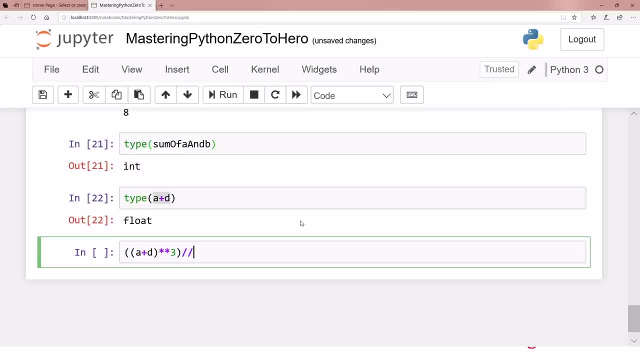 whatever the result is divided by maybe four and we just save that in a new variable. let's say: let's say the new variable is v. let's say we save that value and v and now we print v and we have the result for v. wow, so we can do a lot of stuff with these kind of variables. let me show you a. 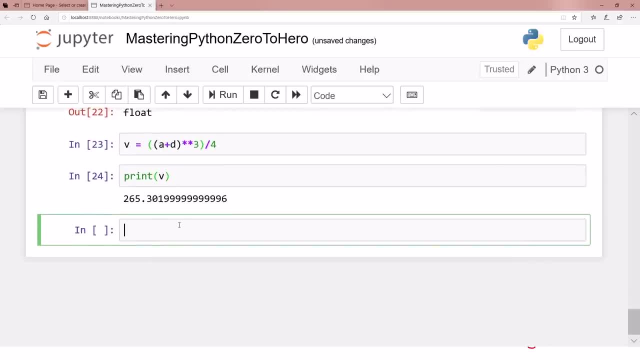 family of variables. let's say we have a family of variables. let's say we have a family of variables. if you don't get the value of your alpha, because if you get itlord, the value of s1, now if you take off s1, you'll see that it is is more relevant than your s12, because it is going. 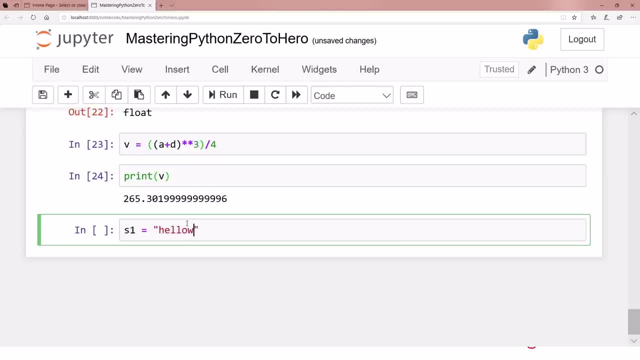 to be rods and if you add s1 properly, the world will be this world. Okey, that's that. you will take hello, Hello, And we have our variable s10, so it will take as s10 in here and it will become a little bit more helpful. you won't worry that if feel I just come back to it. 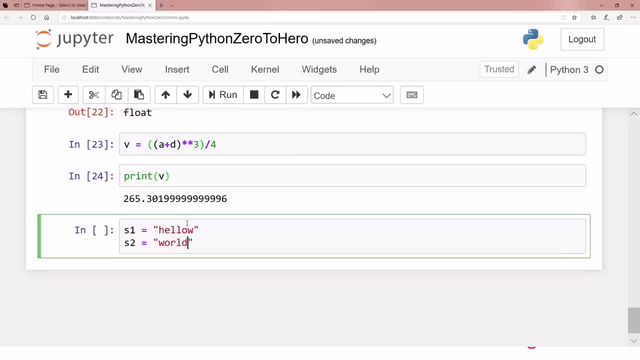 I could do that catastrophically and I'm going back to that right now, But we just want to say hello. and here comes the second one, Sophie, as a little bit hello, let's say hello, hello, And here we'll change the world. And now what's a world? can I say hello and no? 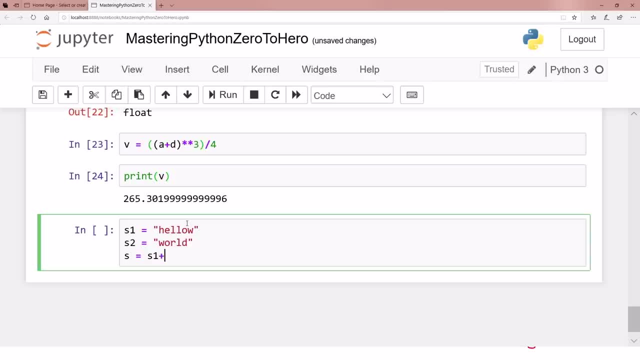 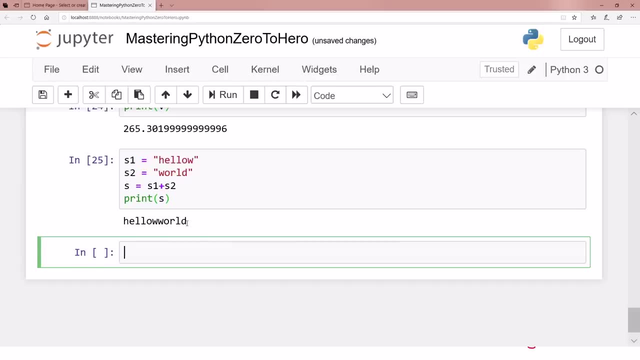 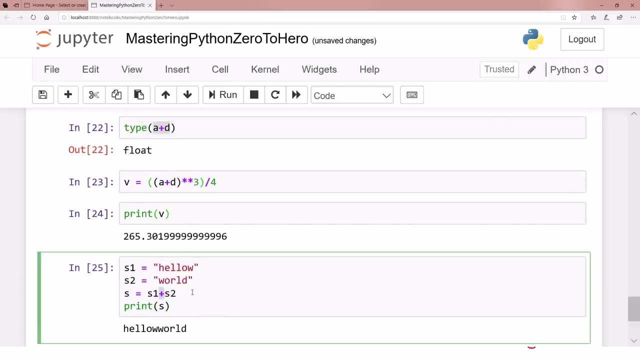 we have another variable, let's say s, which is s1 plus s2. what it will do is it will just concatenate them together. we will see strings a lot later on, but just to tell you this plus is not just for, not just for numbers, it is for other data types, very fancy data types that are there. 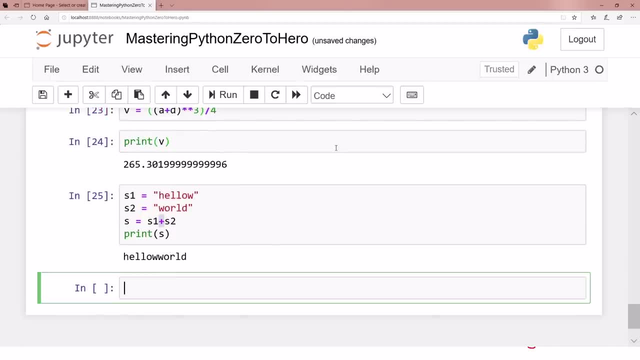 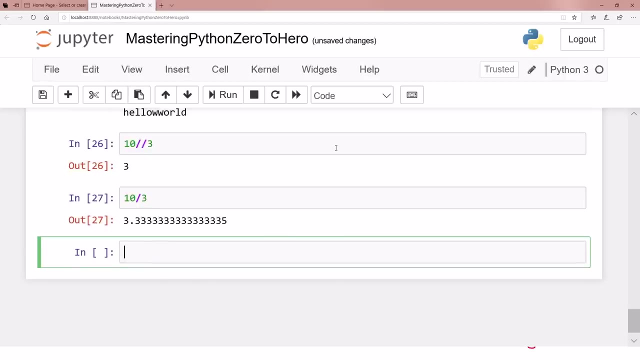 one more thing. let's say we define 10 and we divide it by 3 and we want a quotient. the quotient is 3. however, if we have 10 divided by 3, shift enter. the result actually is 3.33, and so on you. 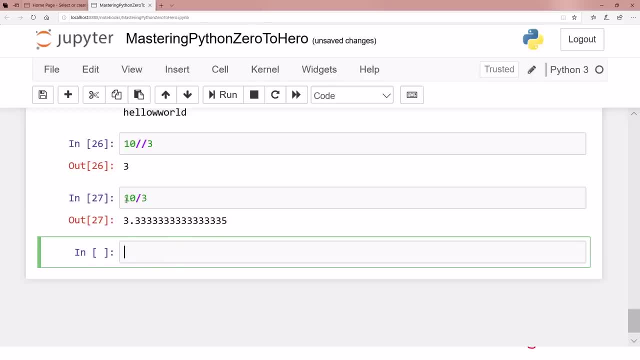 might be wondering. we have not saved that result in a particular variable, so where the result is saved, actually, if you want to save that result, you can do that by just saving the result and you do not. if you do not save the result, if you do not assign the result, for example in this way: 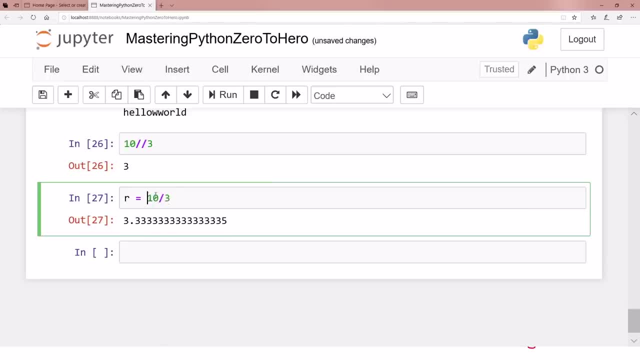 the result will be assigned to a variable R. but if you do not assign, if you do not store the result in a particular variable explicitly, by default, there is a variable in Python which is underscore. underscore contains the last result that you did not store in a particular variable explicitly. so 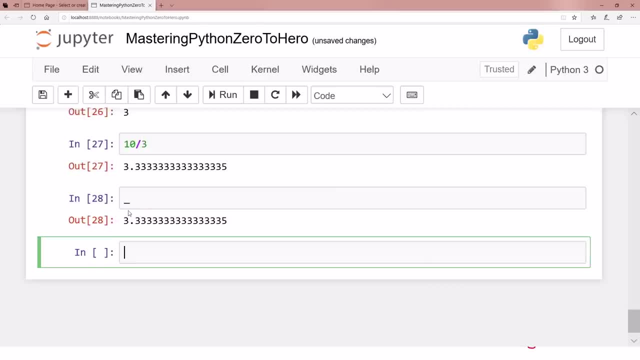 if that underscore is basically one default variable for for the result, if you want, don't try to update this underscore, just just read it. do not assign anything to underscore. for example, if you assign something to underscore, assignment will be done, but then the properties of underscore will no longer be there as they are. 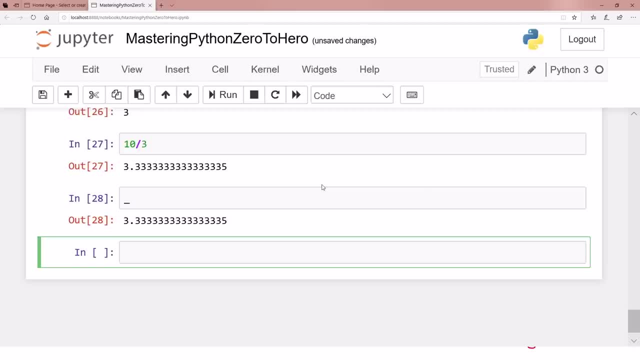 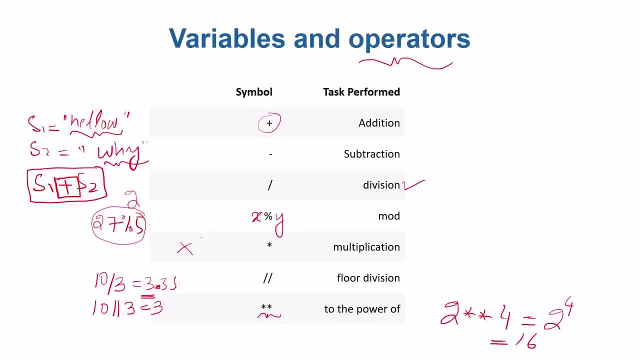 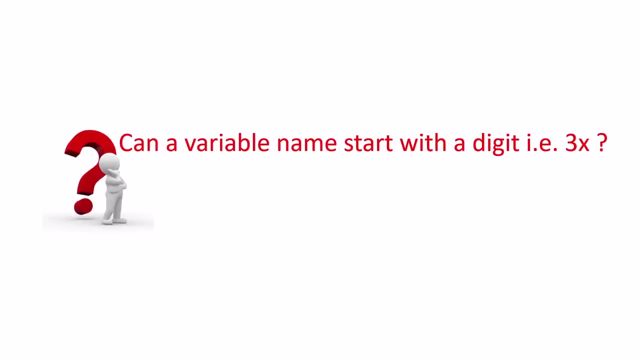 in in Python built-in properties. okay, so that's about it, I guess. so that was the operators. we will see the operators more and more later on, but before ending this video, I leave you with a question. so the question is: we saw the variable names like sum. 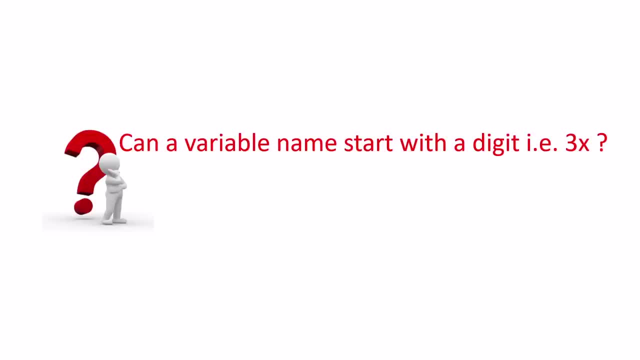 of a and B, X, Y variable name can be, can be lengthy, can be descriptive, can be short anyways. so the question really is: can a variable name start with a digit, for example? is it possible that the variable name really is it starts from? the variable name starts from, for example, a digit is a 3x valid variable name or, for example, at the rate of at the 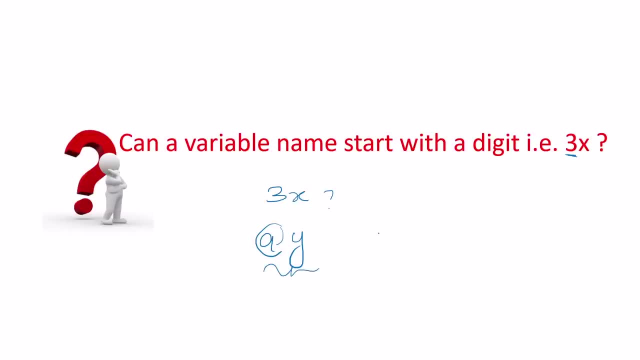 rate of Y. is that a variable name? or for example, this symbol: times 2 times X: is that a variable name? what are the conventions to for variable names? can we, can we write anything? in the left hand side we write, let's say, 3x is equal to 4. that means 3x is now a variable name. is that true in Python, or are 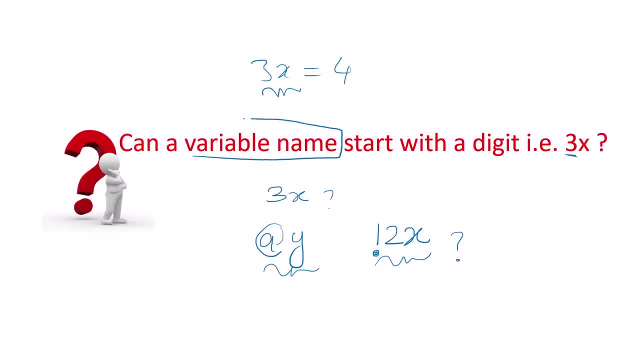 there conventions to define the variable names. so yeah, think about it. I'll see you in the next video with the answer to this, so I hope you will. you'll be having answer for this question. hope to see you in the next video, okay, so in the last video I asked you a question, um, about the naming convention of. 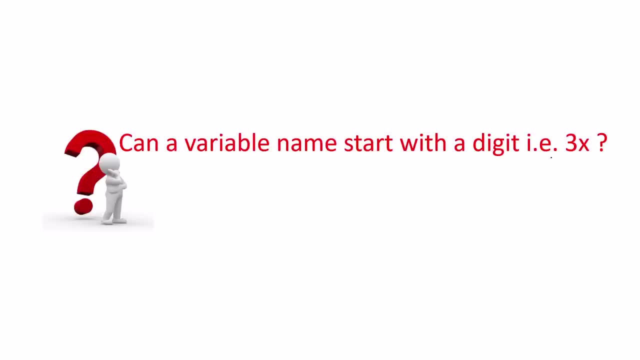 the of variable names, in particular I. I asked you whether 3x is a proper variable name or not in python. so what's your answer? yeah, what do you think? how many of say? how many of you say no, how many of you? you might have tried that, declaring that variable name in Jupyter notebook, and then you 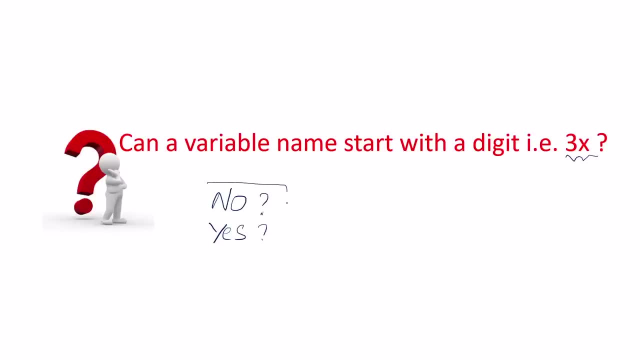 might have got this answer, one of these. well, let me tell you. the answer is no. uh, a variable cannot start with a digit, not with, not with at the rate of not with hash symbol, not with. I mean, there are several other. the special characters are not there, except a few characters. one of those is: 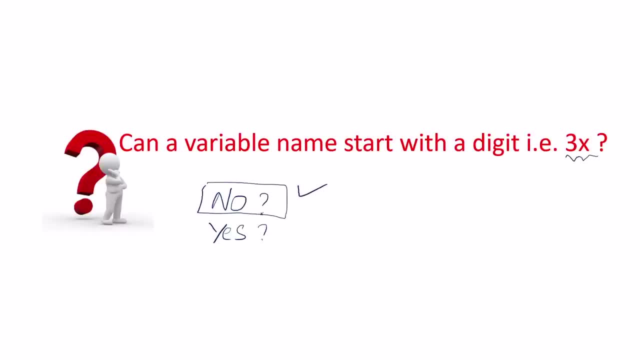 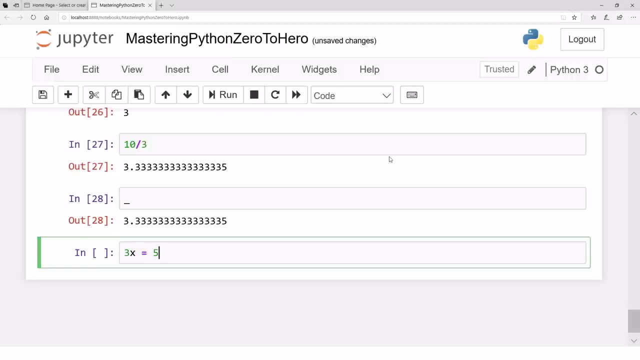 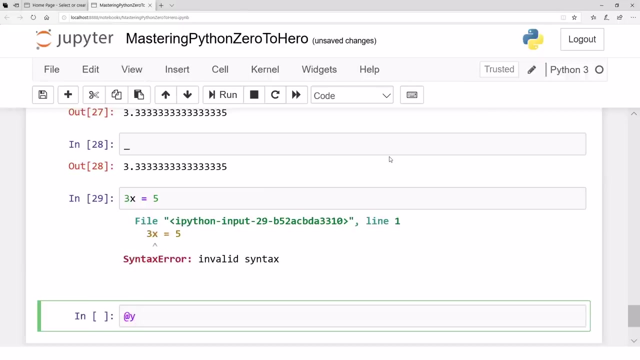 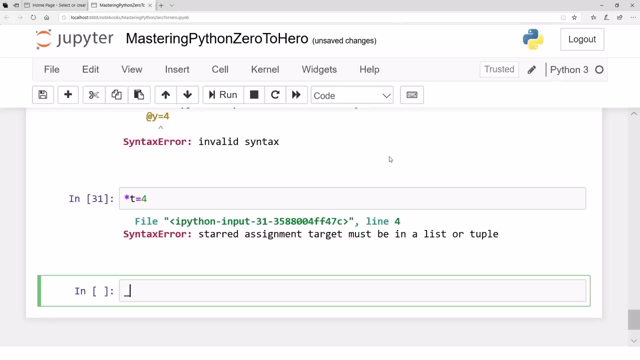 underscore. let's go to. let's go to Jupyter notebook and and check this. so, for example, 3x equals 5- error, invalid syntax. let's say, at the rate, of y equals 4, invalid star. T equals 4- error. well, an exception is underscore. underscore E equals six. that's allowed. 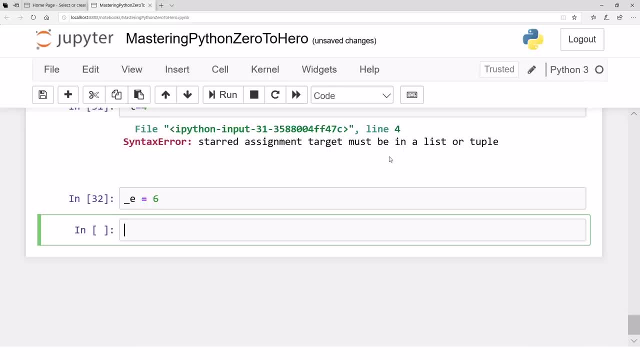 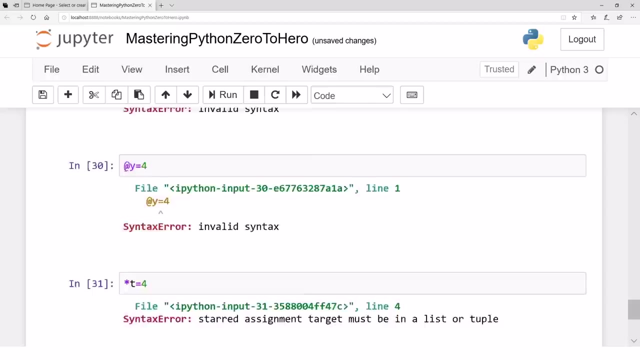 starting a variable name with underscore is allowed. it is different than the underscore that is built in underscore. this is underscore E is different than simply underscore. so it is good to not declare the variable names that start from these, because you will be getting errors further. variable names should be descriptive. they should 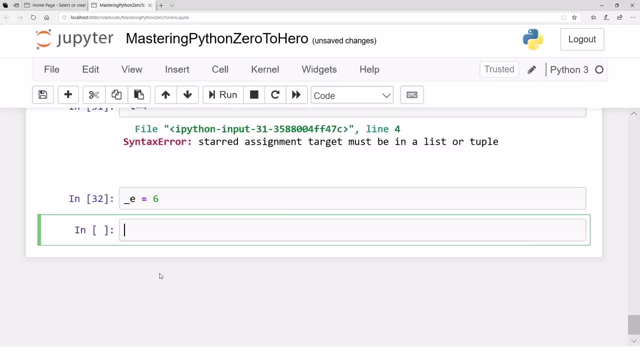 give you a look and feel of the data, what they are containing, and you are free to define variable names as as descriptive as you want. so it is a good practice to to start writing the variable names in a better way. one um one better notation, one better notation of defining these variable. 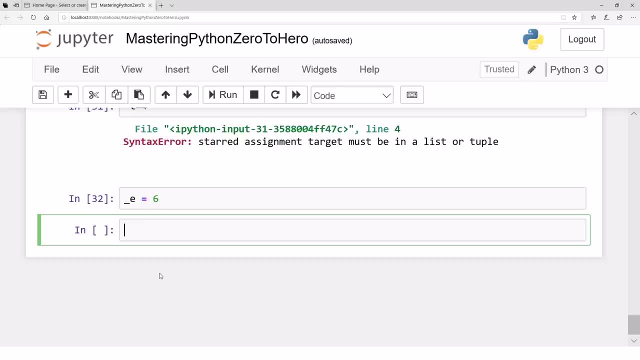 names, even the function names. we will see the functions later on. one way to defining those is to use camel notation. camel notation, camel notation, is you start with the variable name with, for example, lowercase letters. let's say your variable is starting time of the course. let's say that's your variable name. so you write starting. 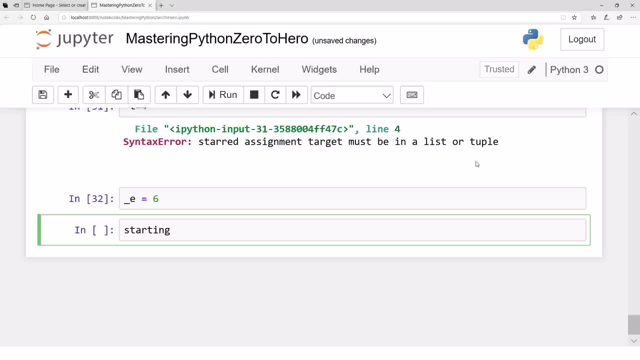 that's one word finishes. then the next word should start from capital t: starting time of the course. let's say so. this kind of notation is called camel notation and very famous, particularly the java developers. they normally follow this and several other developers. but you should come up with a notation. that is one notation. there are other ways of. 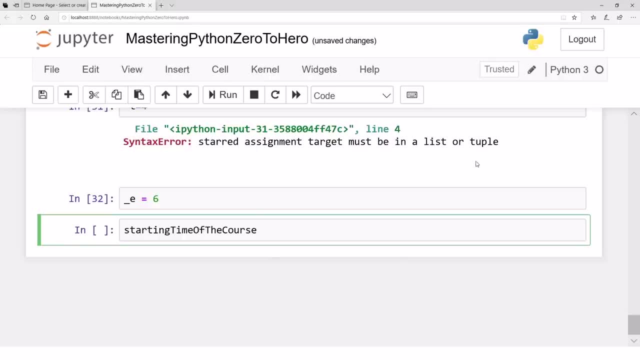 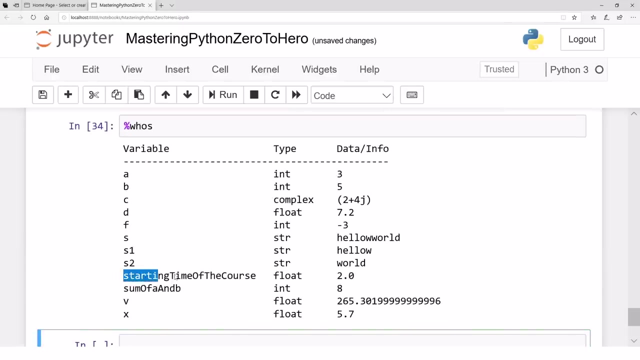 uh, keeping consistently, keeping the consistent strategy of defining variables. there are several other ways. this is one way. so starting time of the course is, let's say, 2.0. let's say so that's a variable name if you, if you now check, that's a variable name. but now, if you see this variable, just just the name suggests. 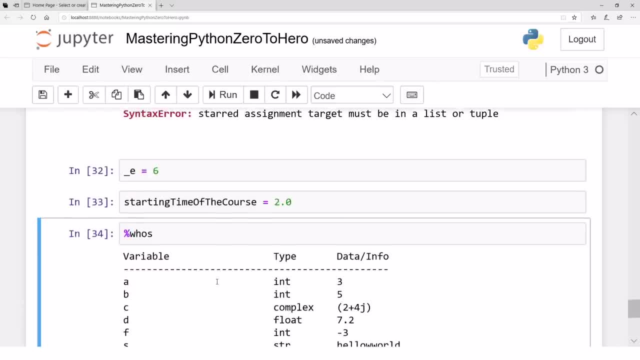 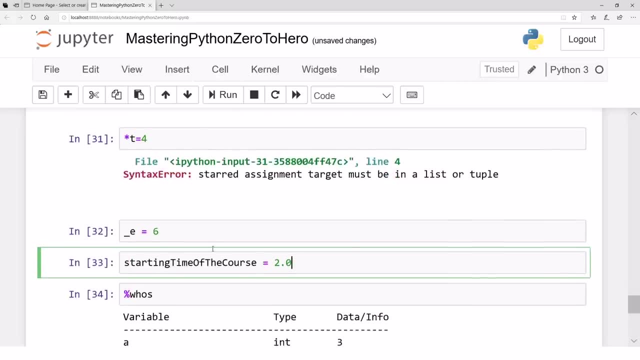 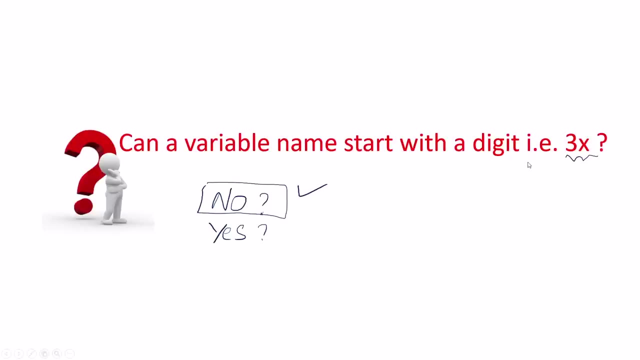 the data inside is doing what. so the names should be descriptive, i mean and, and make that as a habit. so yeah, i guess. uh, we have now answered our question, so let's go ahead and start with the next one. b? um, so in fact, this is a very big problem, um, because we've been talking about this from a lot of. 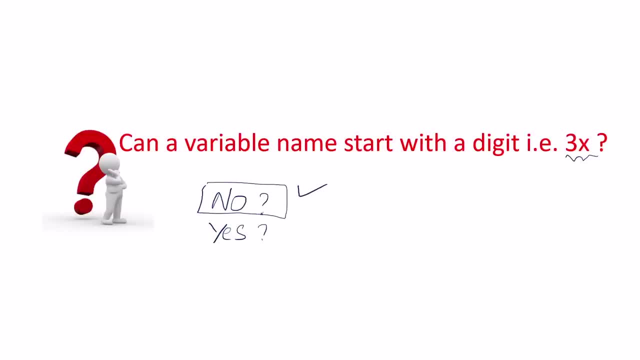 different aspects of the code and we've already done a little interruption and we have two different cases and we have two variables in this query and we have one of which is very easy to understand. but the thing that i'm trying to do here is i'm trying to figure out how to use this question very concretely, that a variable name cannot start with a digit, not with any special character other than underscore. okay, uh, in the next video, um, i'll be introducing comparisons with variables. for example, what if you want to compare whether one variable is smaller than the other or not? what if you want to compare whether the two variables- they are containing values- they are same or not? what if you want to compare whether the two variables- they are same or not? 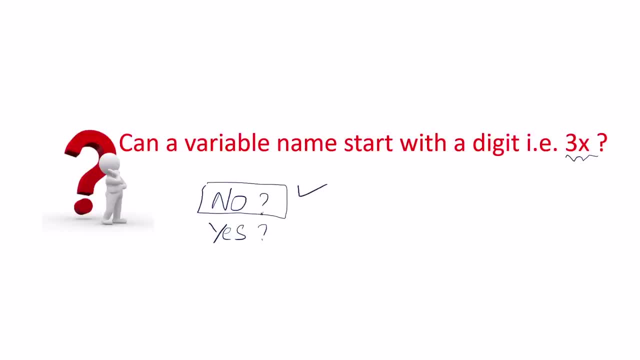 to do comparisons of the of the data that is stored inside the variables and, based on the result of the comparison, you want to do something else. so in the next video we will see a bool data type that is very, very famous and it is used in a lot in decision making, and we will see the 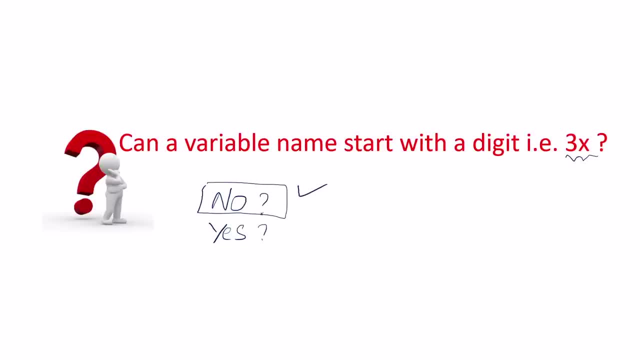 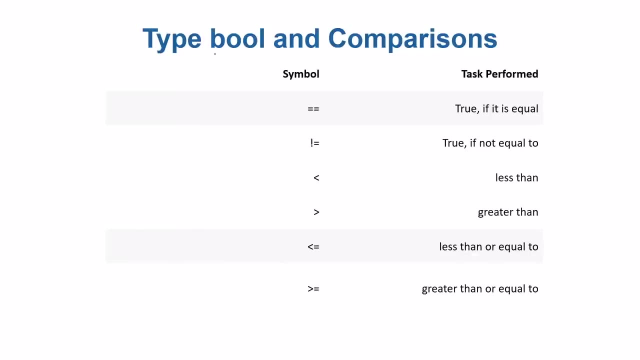 comparison operators, sometimes called the relational operators, in the next video. so hope to see you in the next video. okay, in this video we are going to talk about a data type which is called bool. that's very, very famous data type. actually, it's the most famous data type because 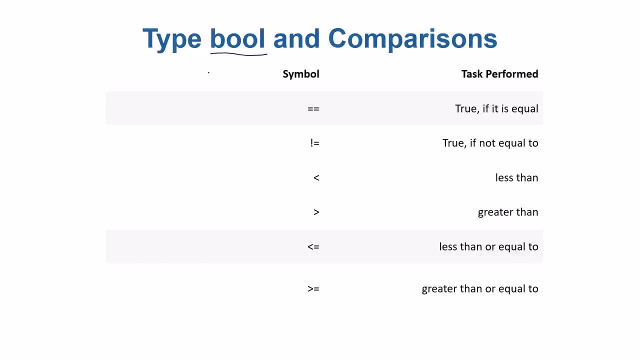 it is used in decision making. all the control flow, most of the control flow, depends on this data type. although it is very, very famous, very much applicable data type, it is very simple: it is a data type with just two states, with just two values. by the way, there are capacities of 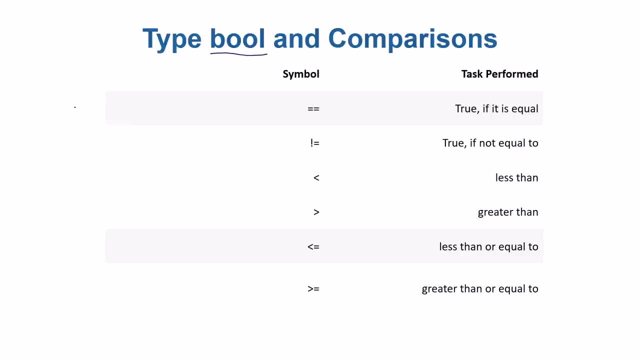 different data types, for example in t, in integer, the different kind of values that you can store are huge. you can store any negative number in it. you can store zero. you can store any positive number. the capacity of floating point number or the number of values that it can save is is even. 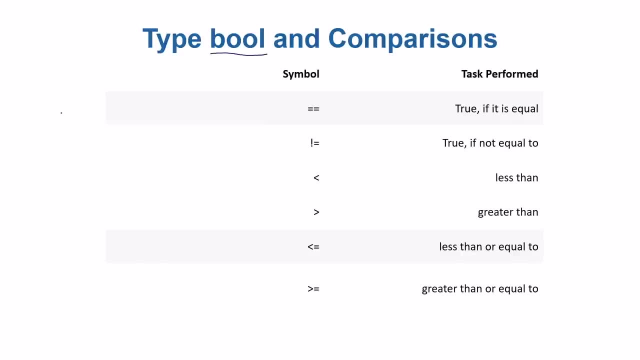 higher than, even higher than integer, and the complex number is even higher than that, and so on. but the bool data type, it has just two states. one state is true. it has just two values: true is a value and false is a value. just these two straights, true or false, in in some programming languages the true is denoted by: 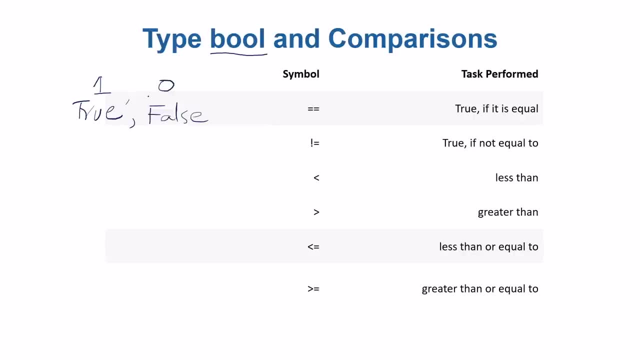 one and the false is denoted by zero. but in python the true is just t r? u e, true that thing, and false is false. that's it. if you, for example, define a variable, let's say any variable name, whatever the name is, let's say b- and you assign true, then its its default data type will become bool. 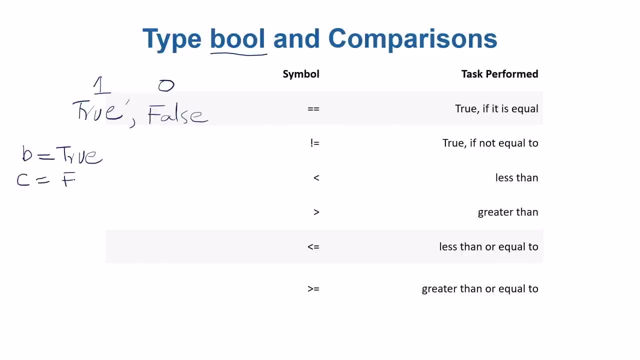 and if you have another variable, let's say c, which is false, then c is also bool. one thing that is important: there are other operations other than arithmetic operators that we saw adding subtraction, division and stuff. there are other operators that we can apply on bool data type, for example. 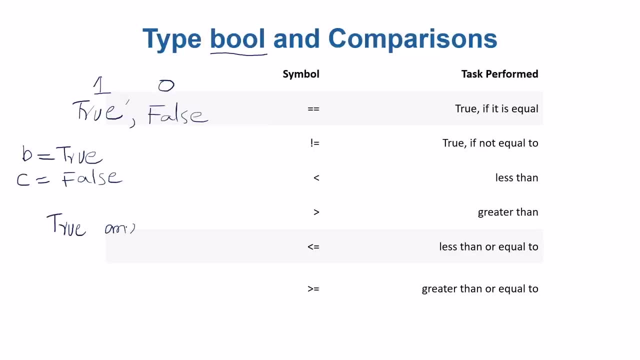 a true and and is a keyword combining true and true. if. if there is a variable, let's say a, if there is a boolean variable a with data true, if there is a boolean variable b with data true, then a and b is also true. so let's say i've used this variable d. 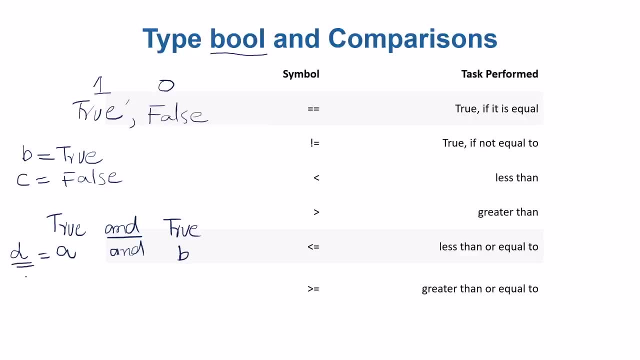 in storing this a and b, the d will also be true. so true and true is always true. further, true and false, this is always false. and this is uh, commutative. for example, true and true is true, true and false is false, false and true is false, false and false is false. so if you apply an operator, 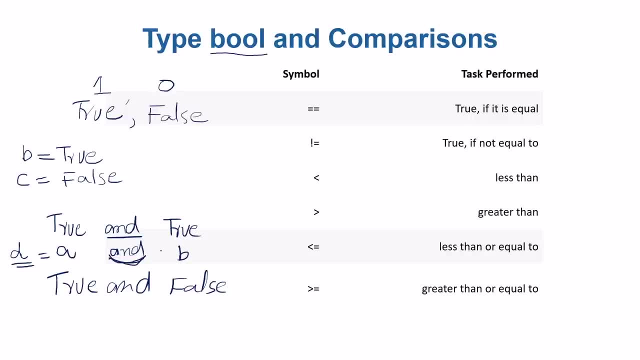 and keyword to combine the two boolean variables together. if both are true, then and will result a true, otherwise and will result false other than this end: there are, there is, there is another uh, there is another uh operator keyword, or so this results false. if both are false, false, false. 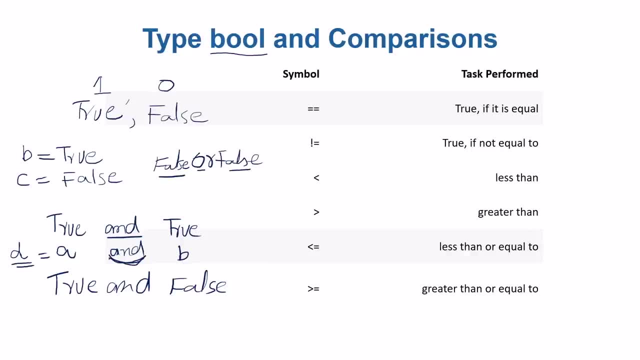 false or false is false. if any one of these is true, then the result is true. remember the difference between and and or and will result false. if any one of the two operands, at least one of the two operands, is false, then the result is false. if both are, or or and will result true if both of the operands are true. otherwise it is false. 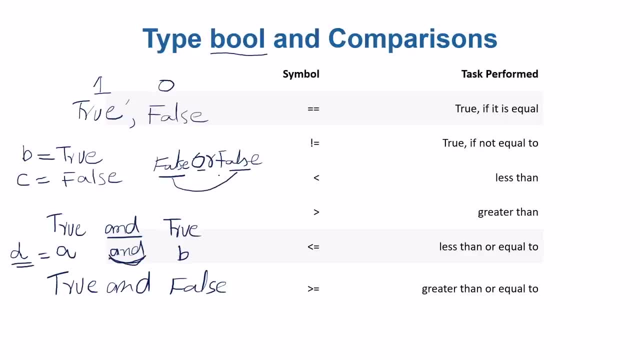 or will result false if both of the operands is false, are false. otherwise it is true. so you now know true and you now know. or there is another operator called not, uh, this is not, so not. for example, returns not true results false and not false. returns true: great, so not is a unary operator. unary means it just takes, it just takes one. 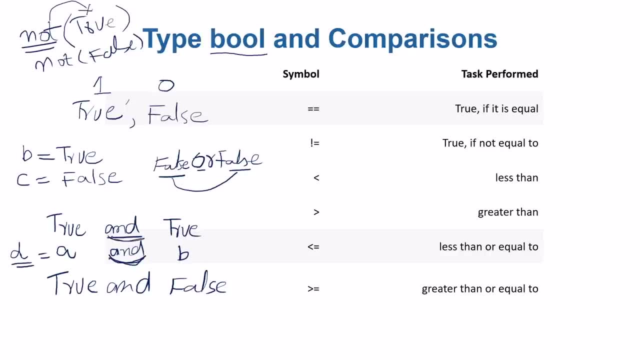 variable and operate on that and is a binary operator, like plus, is a binary operator, it takes two variables to operate on, or is a binary operator, it operate, it takes two operators, it takes two variables to operate on, and so on. so remember, remember these things. one and will return true if both of the variables are true. otherwise the result is false. 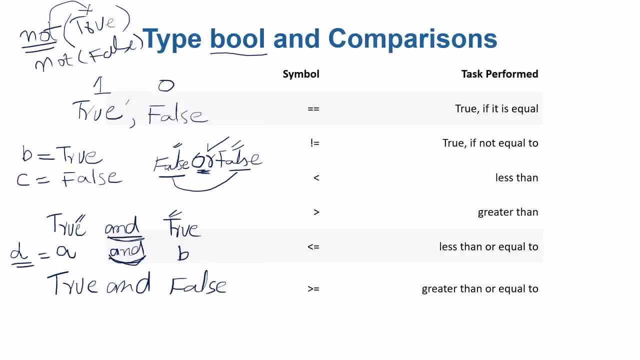 or will result false if both are false. otherwise it will return true and not is not just flips the the state. so not true means false, not false means true. ever so, these are basicallyono that's how you can combine the Boolean variables together. in the next video we will be seeing how to apply these comparison operators and their 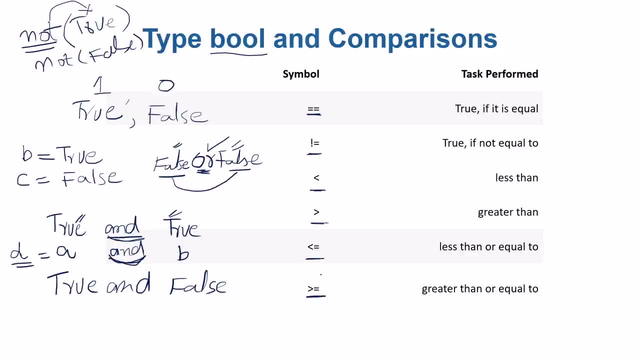 result will be boolean types, and how can we combine the boolean types together to to build a better decision making? so in this particular video, i just- i just introduced the Boolean data type for you with you. in the next video, we will see where the Boolean data type actually appears and how it impacts our programming style or thinking. 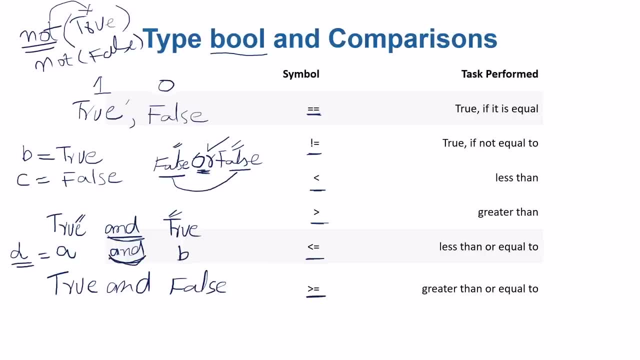 style or coding style. So hope to see you in the next video with comparison operators. that actually produces the Boolean variables. Hope to see you in the next video. Okay, in the last video I discussed Boolean data type and I discussed that- a Boolean variable. 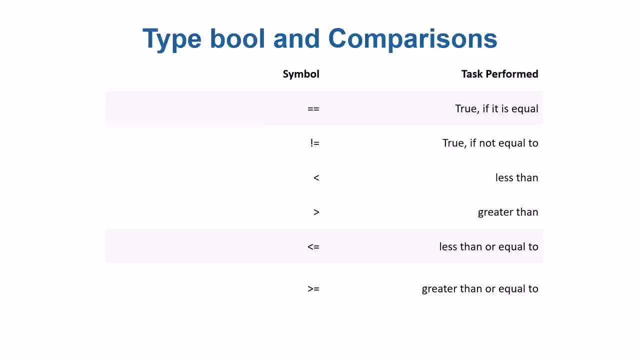 takes either a true or a false and we can combine these Boolean variables together with AND or operators and then we can apply a NOT operator on a particular variable. and we saw that a true AND true returns true and AND otherwise returns false. Similarly, false OR false is false. 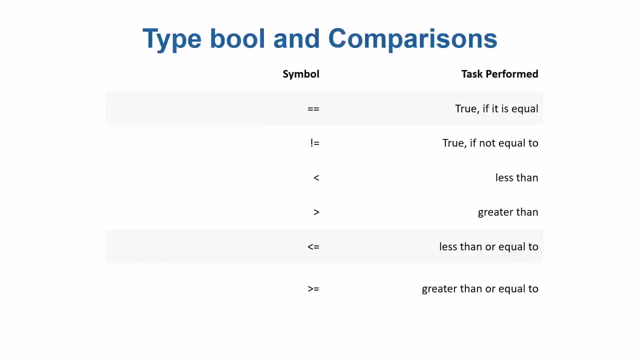 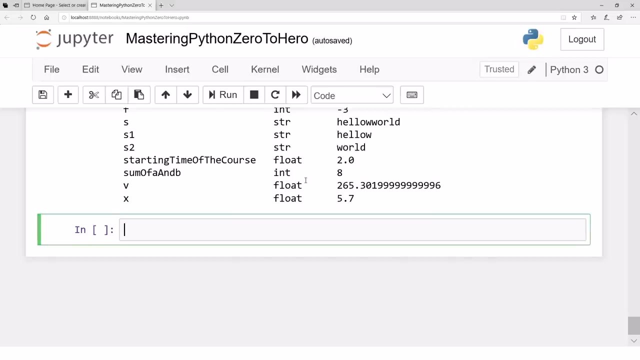 Otherwise, OR always returns a true. Before actually discussing these comparison operators, let's just go to Jupyter and just play with a boolean data type just for a moment. Let us just convert this to a mockdown cell and just write bool. that's a boolean variable. 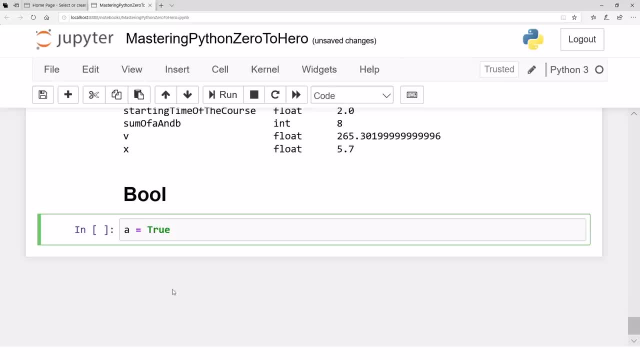 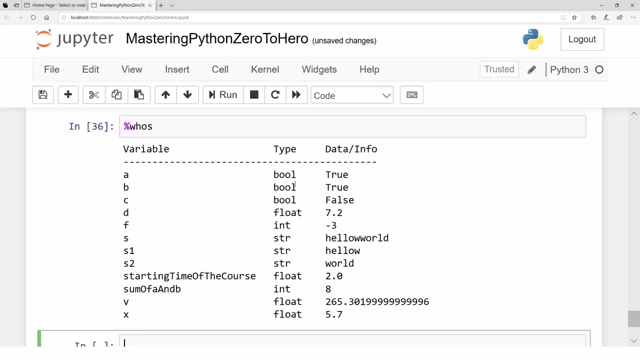 So let's say A is true and B is true and C is false, and okay, so these are our variables. Let's press whose to see what are the states of. So. A is a boolean variable with value true. B is a boolean variable with value true C. 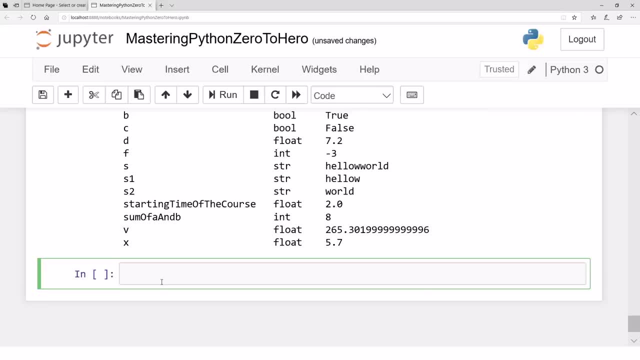 is a boolean variable with value false. So now A is true, B is true, C is false. So let me print A and B. What do you think What will be the result? Let me print A and C. What will be the result? 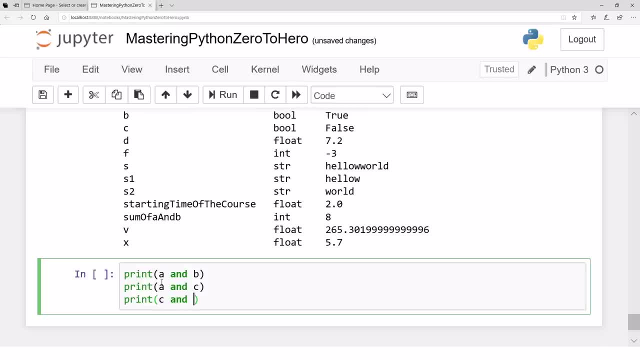 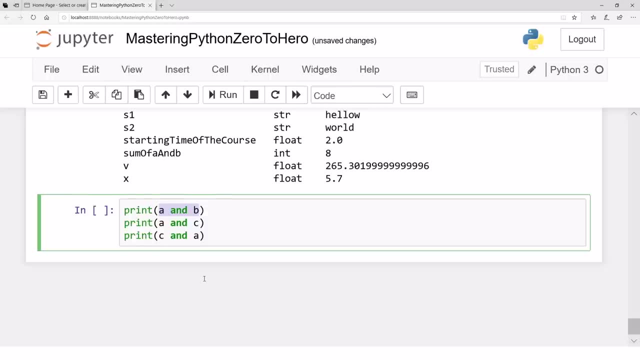 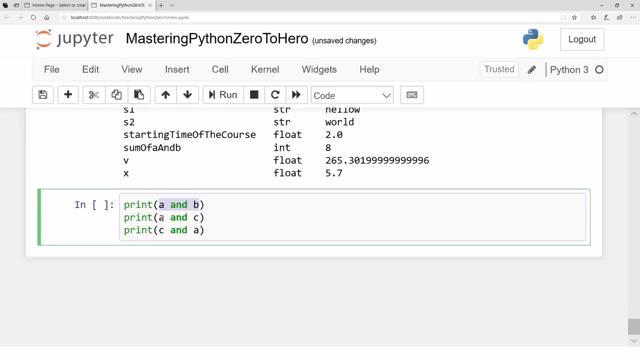 And let me print C and A. So because A and B, both are true, the first result will look like this: So because A is true and C is false, let's pass this. That will be true because C is false, true and true is true the other two statements. 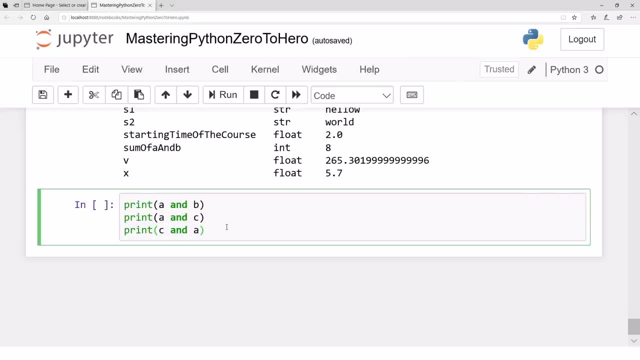 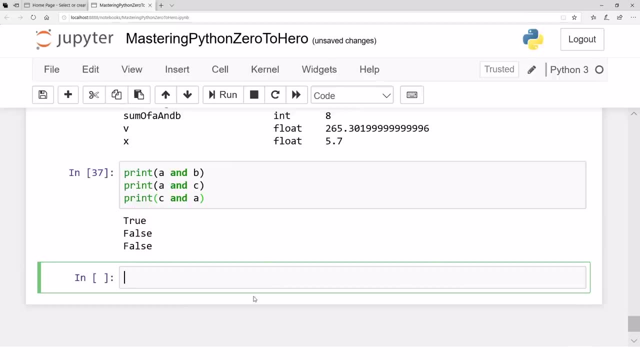 they will result false. So first value will be true, then false, false. So yes, true, false, false. Let's check the or print and, by the way, let's store that. or in another variable, Let's say A is true or C is false. 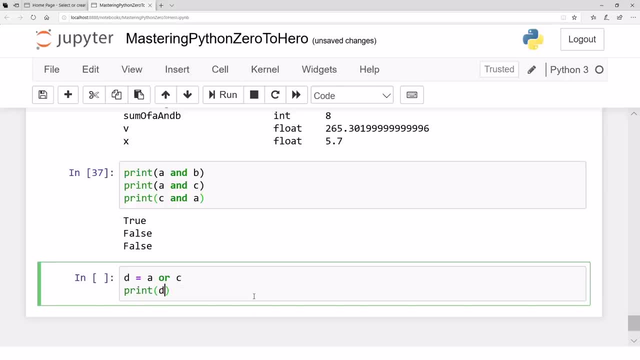 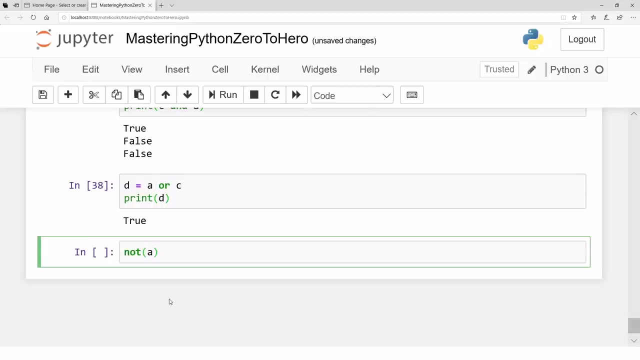 So what do you think will be the result here? because or gives false, when both are false. here a is true, so the value of d will be true. further, not a, because a is true, not a will be false. similarly not b. b is true, so not b will be false, not c. c is true, c is false, so not c will be true, similarly not d. we can save. 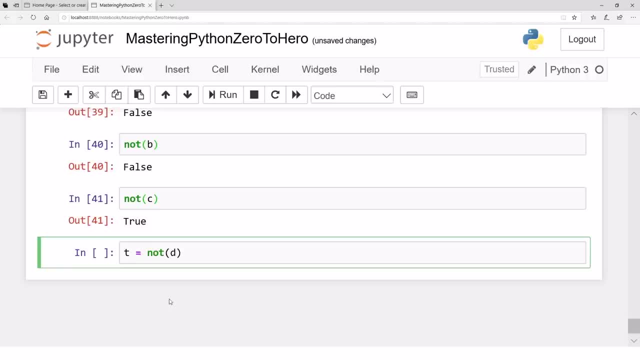 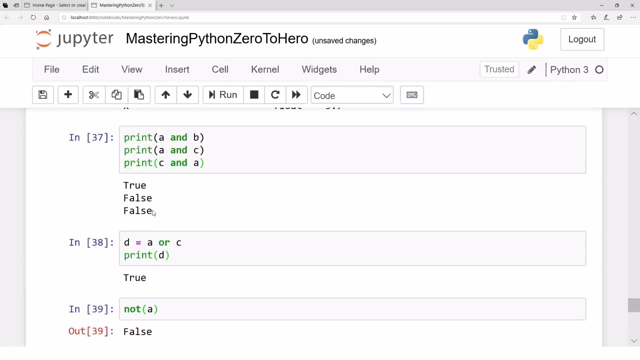 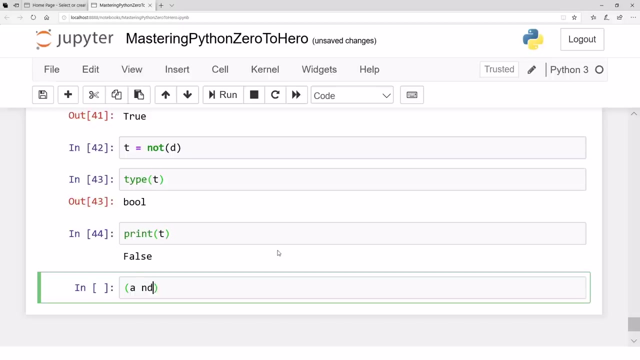 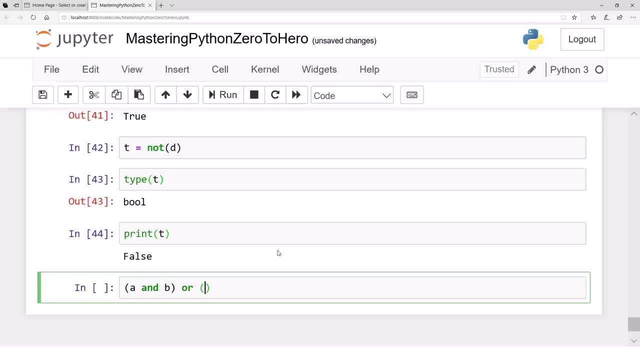 a and b, whatever the result is, or c or d, whatever the result is, and whatever the result is. not of that i i mean we can. we can combine them in a very complicated way. if we want a and b, the result will be some boolean, that boolean. 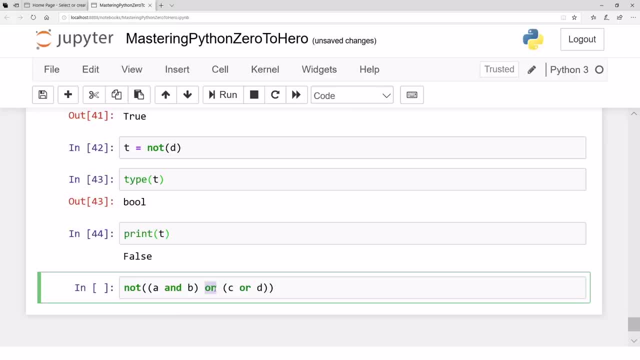 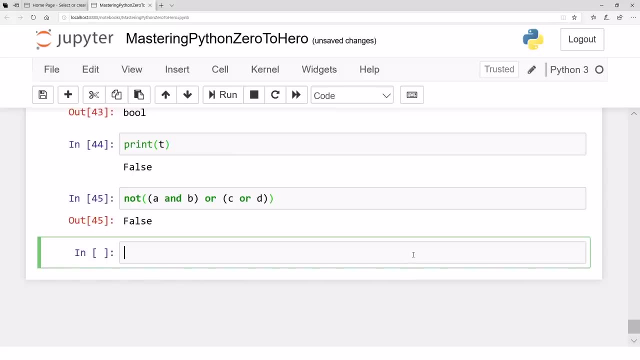 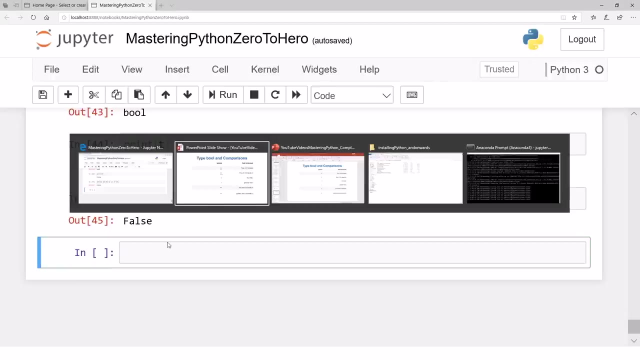 or or two. then at the end we will go to the null. and now, as you can see in the ms here, we can say then: right, so the result is a boolean and that boolean there are. the result eventually will be a boolean and then not of that. so let's check what that is. the result is false. well, why the result is? 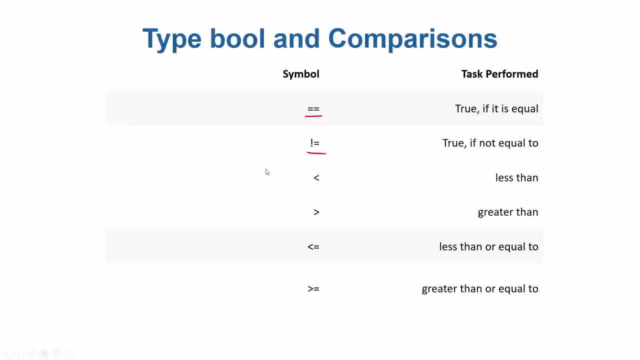 false. um, figure it out why the result is false. let me go to comparison operators. so the comparison operators, let me just compares whether two variables, whether whatever the variables are, whether they are integer floating point, whatever, whether two variables are, are they have same data or not? for example, 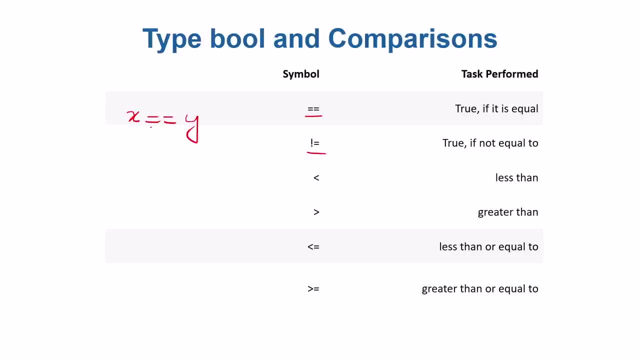 x equals equals to y. that will be true if x and y. they both have same data. so, for example, if x has value 4 and y has value 4, then we are just checking x equal, equal to y or not. the result will be boolean because and x may not be a boolean variable, y may not be a boolean variable. 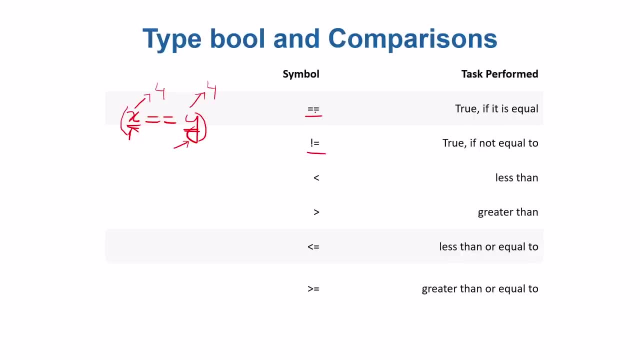 if we want to compare the values of x and y, then we write double equal without a space inside. remember, if we write single equal, that will be an assignment operator. if we write double equal, that means we are checking whether the two values are same or not. similarly, 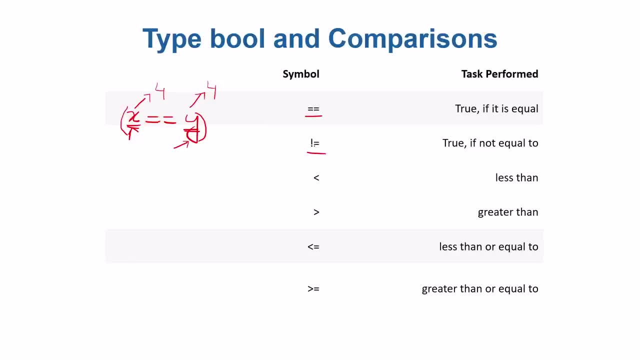 if we write this particular symbol that checks whether two values are not equal or not- for example, x is not equal to y- the result will be true if x and y- they both have different values. otherwise, the result will be false. remember, the result of comparison is always a boolean. it is. 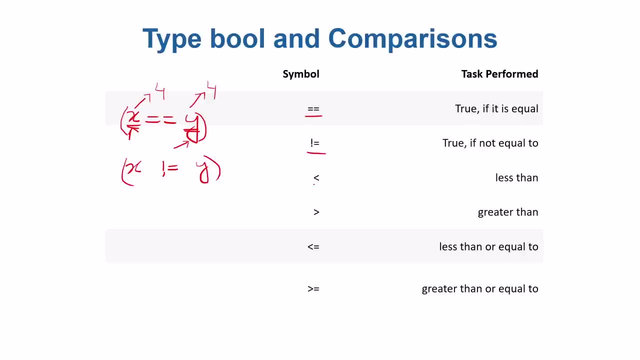 either true or false. okay, next we check whether less than so. for example, if x is less than y, the result will be true. if x indeed has a value that is smaller than y, let's say x is 2 and y is 10. in that case, the result: 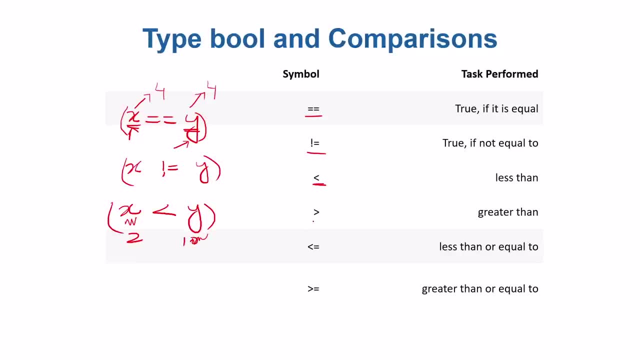 will be a true. otherwise, the result will be false. similarly, we can compare the two variables using greater than we can compare the two variables by uh, less or whether, whether the, whether one variable less or equal to the other. for example, if x is less or equal to y, the result will be true. 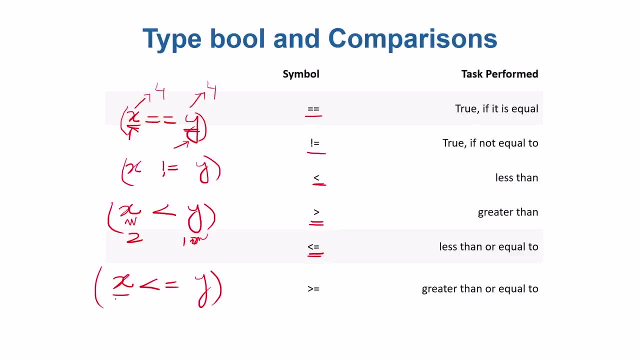 of this comparison, the result will be true if x has a value that is not larger than y, as long as x and y. they are equal or x is smaller than y. in any case, the result will be true, otherwise false. similarly greater than or equal to: okay, so, uh, i end this. 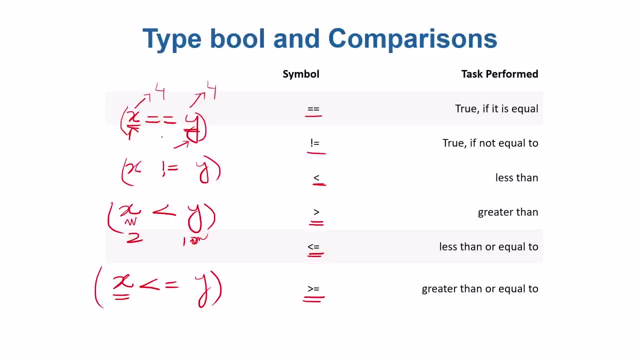 video here. in the next video we will be- uh we will be- moving to jupiter and playing with these operators and seeing the return types of booleans and then combining them together with ands and rs and doing doing uh interesting stuff with that. in this particular video, i just uh talk about, um, the comparison. 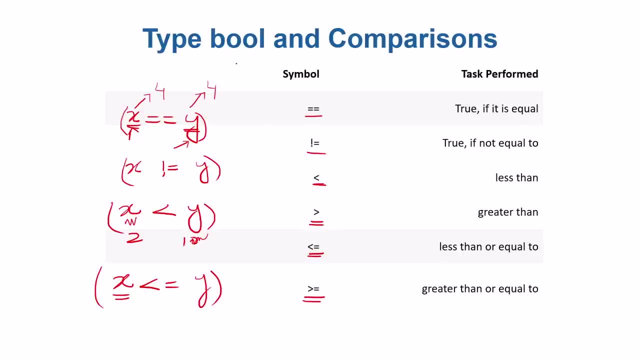 operators, the boolean data type and combining them by and or or not. in the next video we'll be first moving to jupiter. we will see the comparison operators. we will write all these statements in jupiter and just get a good hands-on grip on that, and then we'll be moving onwards. 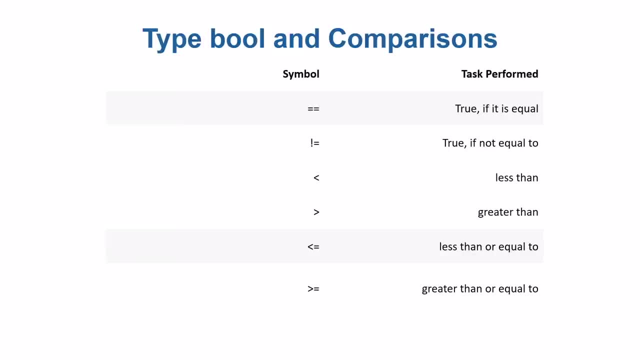 so hope to see you in the next video. so in the last video i talked about comparisons, double equal to- uh, not equal to less than, greater than less than or equal to greater than or equal to. so let's go to jupiter notebook and see how they actually work. so let me just first enter a markdown cell. 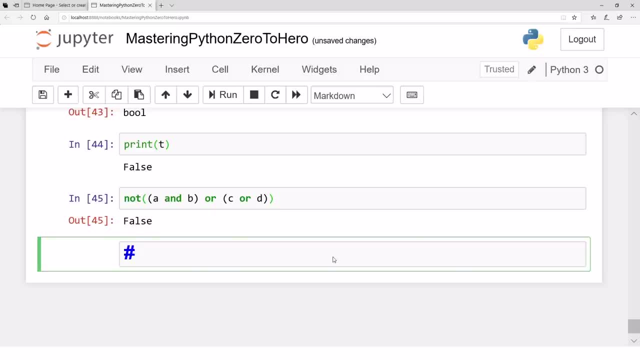 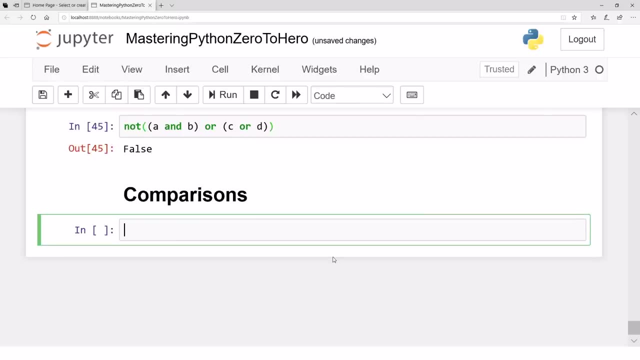 and type that comparisons shift enter comparisons. so we can. we can compare different values by first assigning them to variables and then comparing those variables. or we can, we can compare the values directly. for example, print two is less than three. what do you think? two is less than three? um, the result will be what? 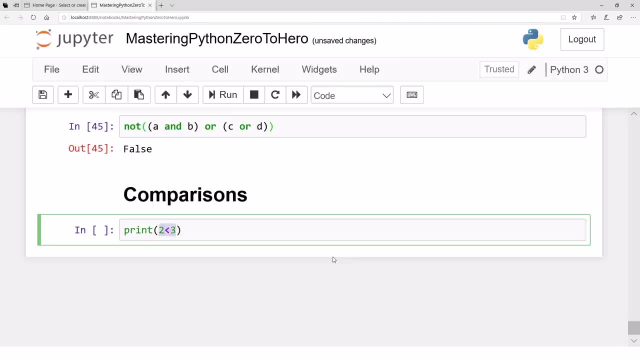 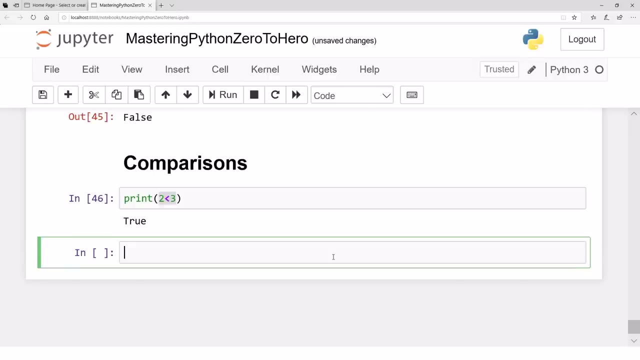 remember, the result of a comparison operator is always boolean. it is either true or false. so in case two is smaller than three, so the result will. because this statement is true, so the result will be true and true will be printed. further, we can store that result in in another variable for. 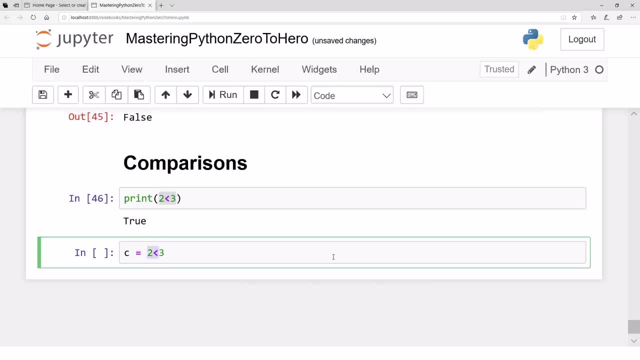 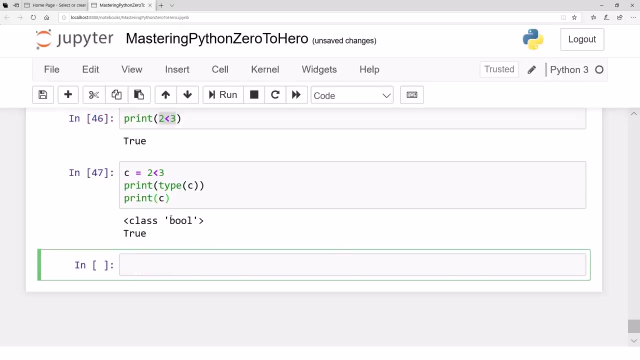 example, two is smaller than three. whatever the result is, the result will be true. the result will be saved in a variable c. if we check the type of c, if we check the type of c, as long as let's print the value of c so you can see the type of c is boolean and c in this particular. 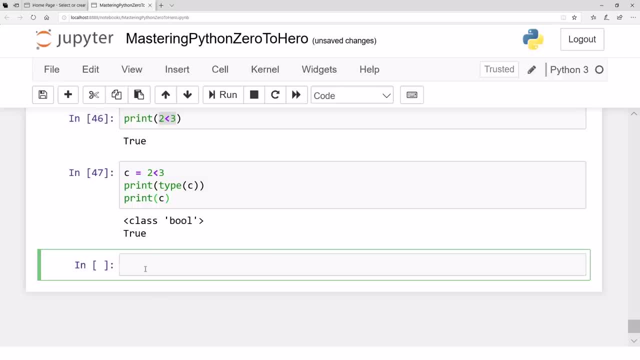 case is true. moreover, for example, let's have three equals to four. is that true or false? what do you think? three equals to four. three double equals to four. that is false. three is not true. so let's print the type of c and then let's check the type of c. 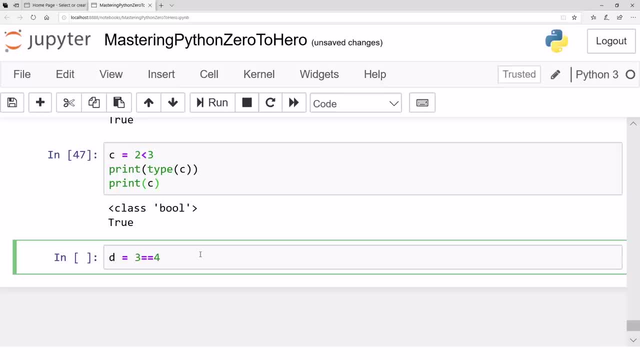 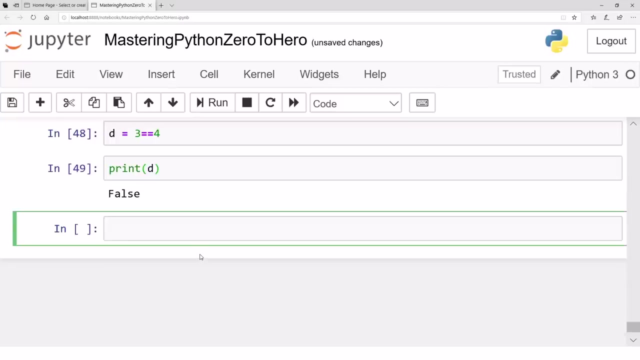 that is not equal to four and let's save this result in d. remember, three double equals to four. that's an operation. the result is false. this equal is an assignment operator that the false value will be assigned to the variable d, and here we can see print d and it is false. similarly, what do you think? 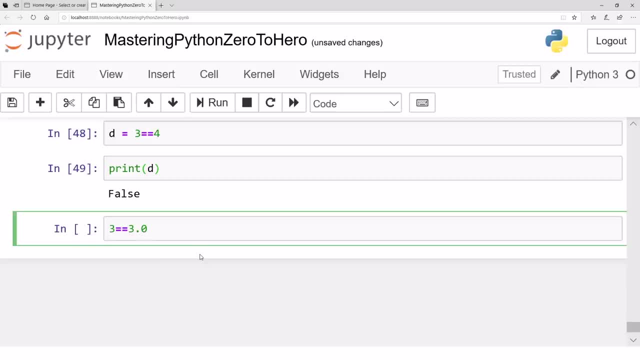 double equal to three point zero. what will be the result? remember, three is integer. three point zero is a floating point number and i'm comparing: three double equals to three point zero. one is integer, another is a floating point number. so what will be the result? let's see. 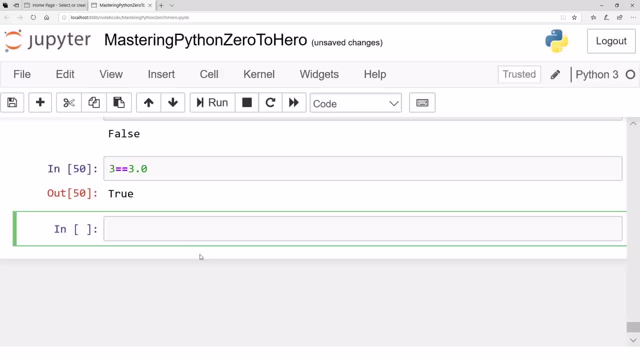 the result is true because they are comparing the values by discarding the decimal, conservative ones, no two, et cetera. um, let's start from the first異: less than 0.4. okay, so here is when we use these variables, though we need to also, 안녕하세요, the final type of d from the correct例计算. 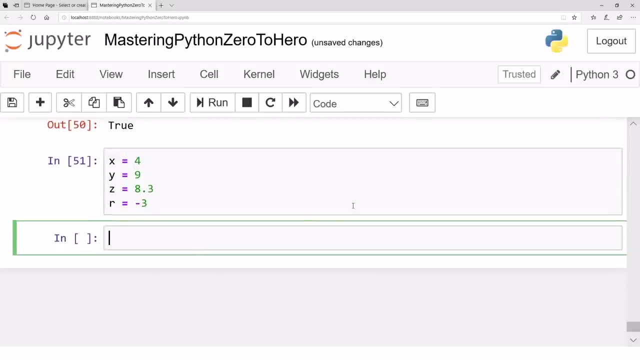 variables. let's say. so what do you think? what will be the result here? X is smaller than Y. what will be the result of that? X is smaller than Y, the result will be true. and Z is smaller than Z is smaller than Y. the result is again true. 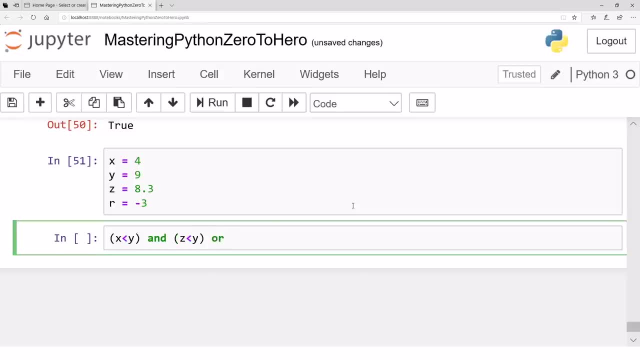 because Z is smaller than Y or R R is. R is equal to, for example, X. so what do you think? what will be the result at the end after this? so let's see first. first, this will be true, this will be again true, and that is false. 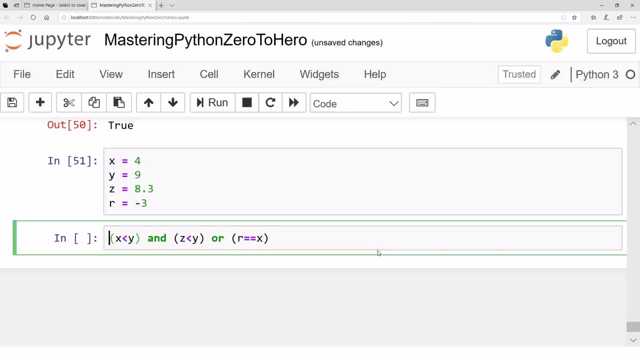 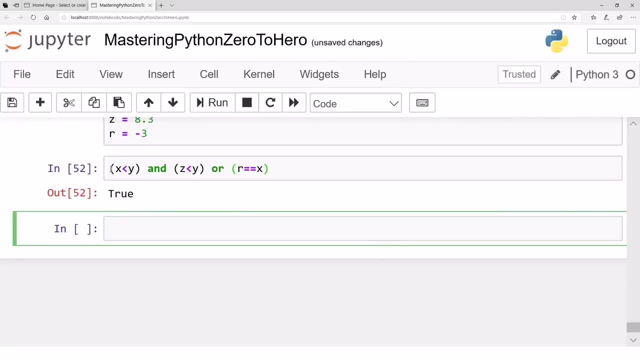 ok, so this true and true will return true and true or anything. the result, final result, is true, so this will return true. but if I just do, if I just switch the order, for example, if I just write this statement which is false, this particular statement corresponds to that statement. now such an error will result. 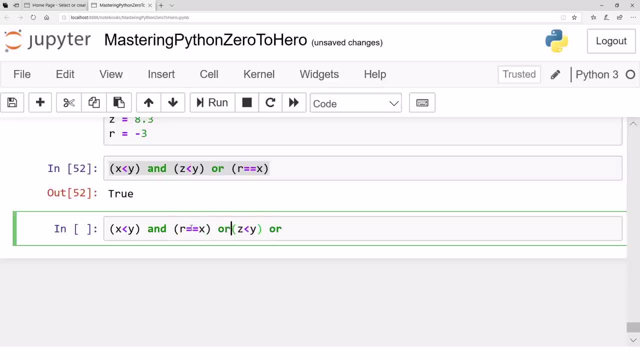 in the result. Now, what does that mean? It means there is no error meaning. there is no error meaning. there is no error here. and then I do this. what will be the result now? now see, X is smaller than Y. it is true. R is equal to X. that is false. so this result will be false eventually. and Z is smaller than Y. that. 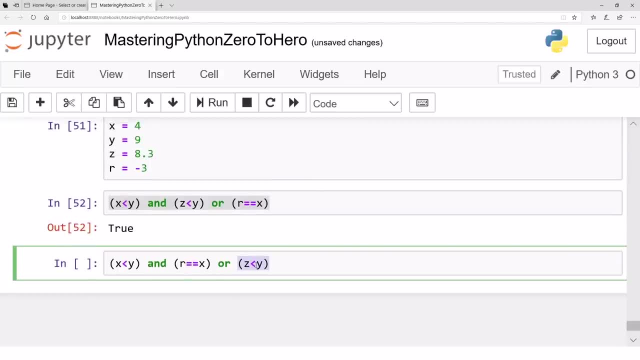 result is: Z is smaller than Y. let me just say Z is larger than Y. let me just check: Z is larger than Y. Z is larger than I. just just to, just to tell you. so this is true, this is false. both and of these are. let me let me switch the. let me switch the this thing: R equals to X. I just want to show. 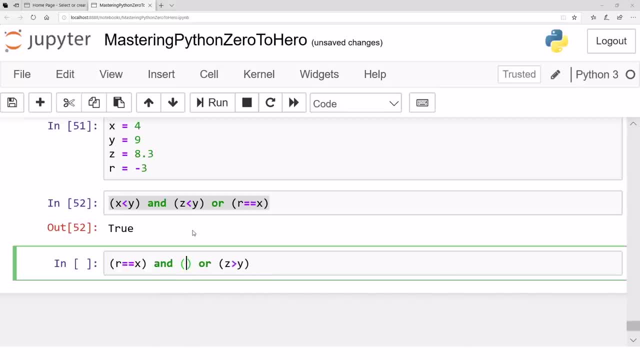 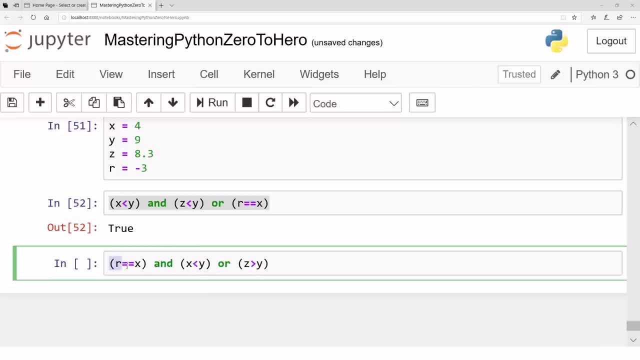 welcome the answer to R. So let's go ahead and we are going to SQL SELECT, the F STEP. now do we even have time until we have rewriting the code star Row, and then you will need to T Elliott's second. but if we do, what are we going to do now? Now, the by right awry is equal to: 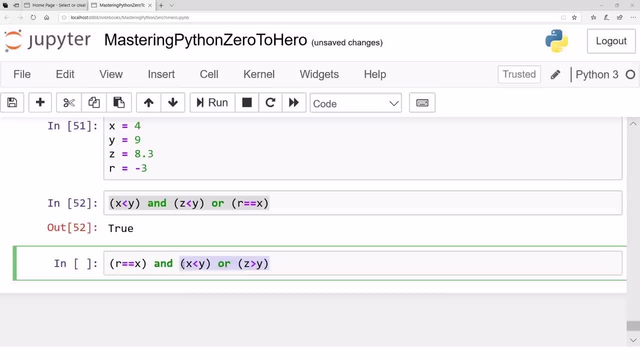 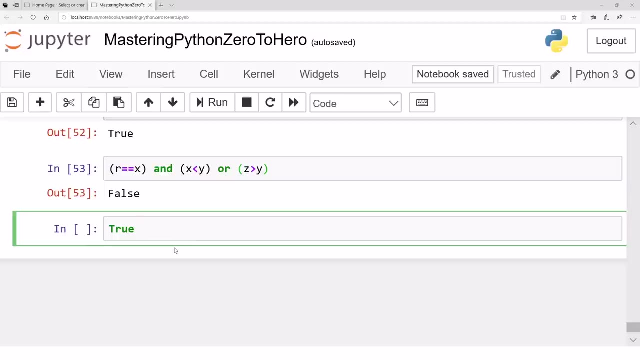 this goes first. if this goes first, I mean, I want to show you whether and and or which one of them will operate first. so in this particular case, the result is false, but it can happen. let me. let me tell you this in more: and true or false, and true or false and true. what do you think? what will? 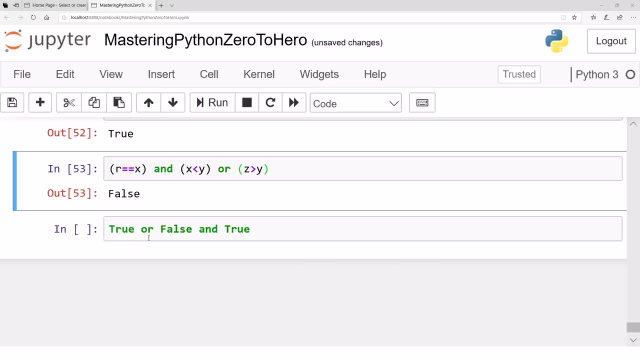 be the result here: true or false, and true. if true or false operate operate first. if true or false operate first, the result will be true, true and true. the result is true if, however- let me let me just write a false here- if or operates first, if or operates first, then false or false is false, and false and true is the result eventually. 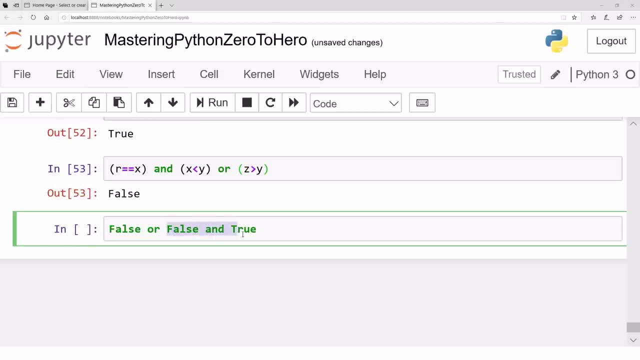 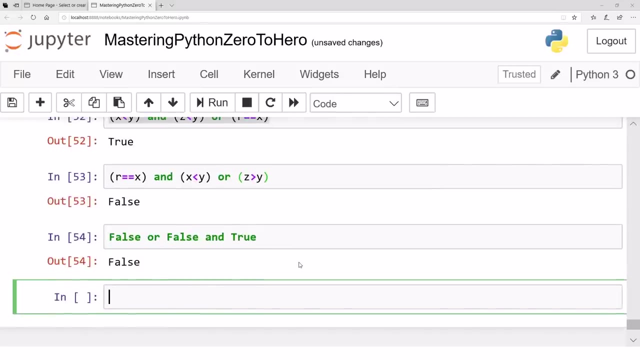 is false and if and operates first, then false and true is false, false or false. the result in both cases is: here is is false. so better way of of representing these kind of sometimes, sometimes they can make confusions. sometimes they can make confusions, for example, if you 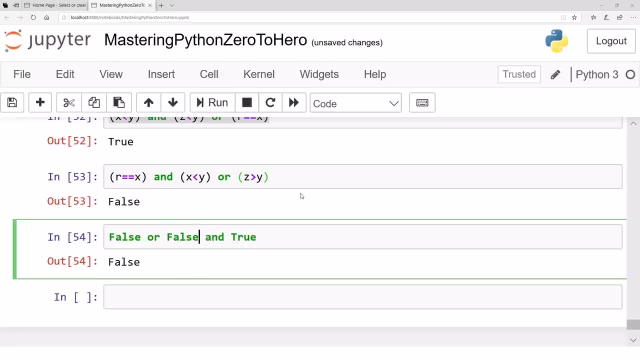 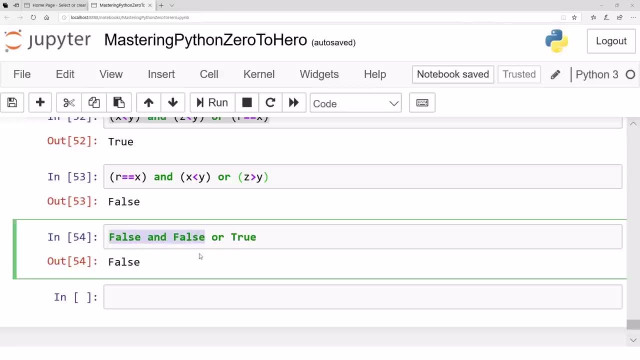 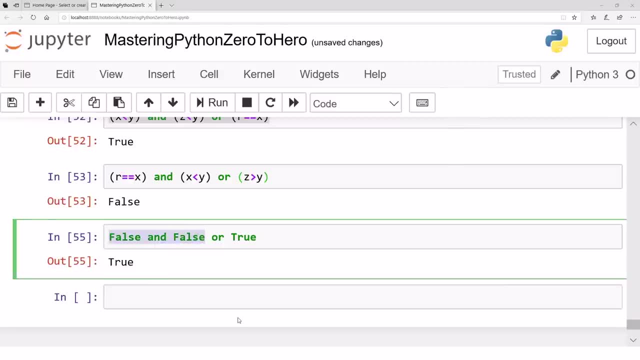 Even if you change this order, for example, even if you pick this thing and apply here, still, the result is: AND will be applied first and OR will be applied after. It is always good rather than to…. one way is to remember the precedence: AND will be applied first, then OR. 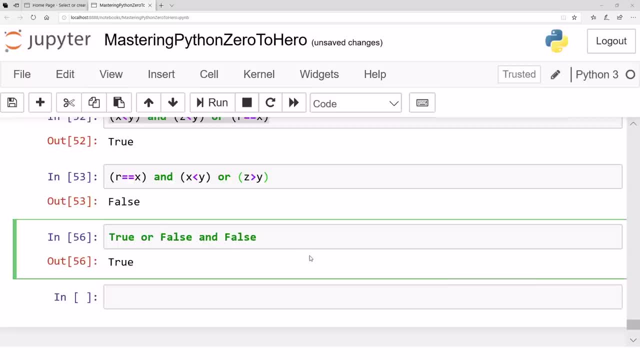 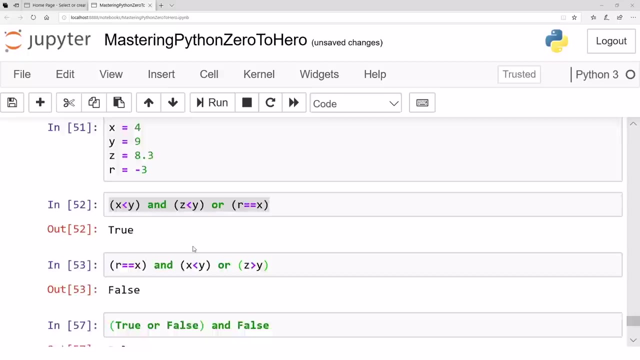 I mean it is good to think about the precedence. Another good thing is to specify the order using parentheses, For example. now we specify this: first, OR will be applied and then for AND will be applied. So it is good for readability to always apply these parentheses- AND and check. 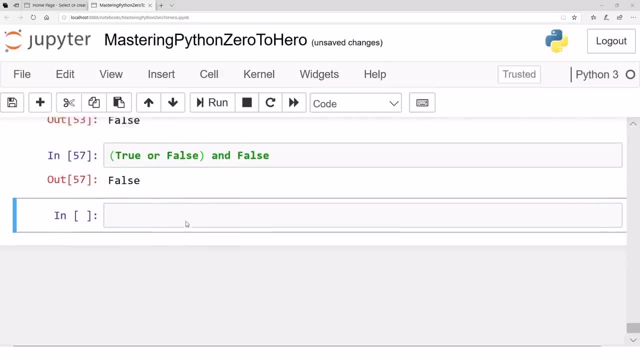 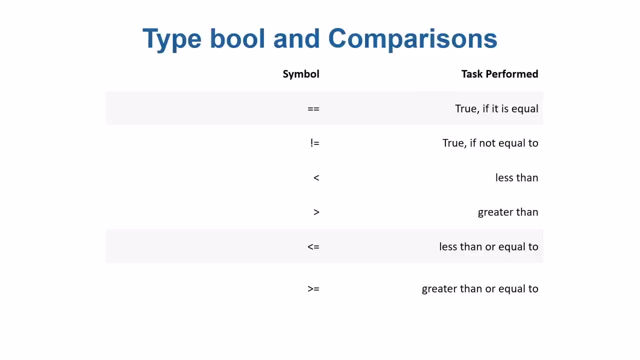 the order in which ANDs and ORs and the combinations will be applied. So in any way, the result of these comparisons will be Booleans Question. what will be the result here? So not 2, not equal to 3 AND true, OR false AND true. 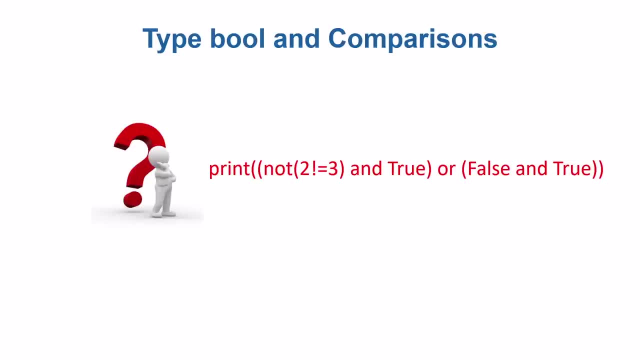 See this slide for a while. Even if you want to pause the video, pause the video, see it and answer. The print will return true OR false. Okay, with this question, I end this video. In this particular video, we just saw the comparisons on Jupyter Notebook. 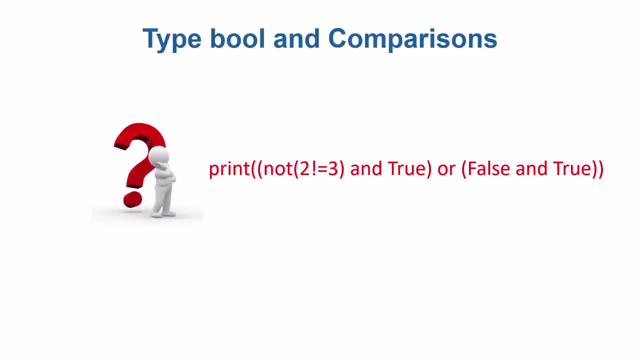 Just see how the comparisons return: true OR false. We combined the different Boolean values using ANDs and ORs, And here is a question for you. Okay, I will see you in the next video with answer of this question. So I left you with a question in the last video, So that was the question, if you remember. 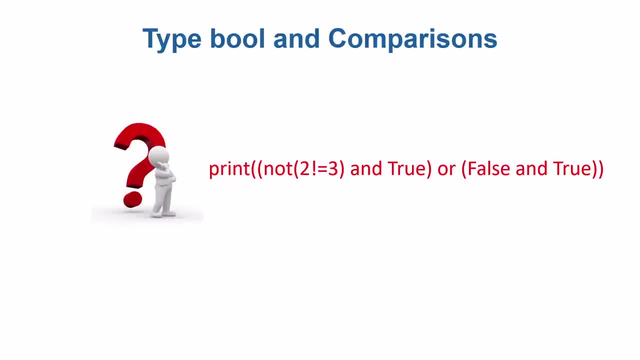 So the question really was: what's the result here? So what's your answer? True OR false? The result either will be true OR false, because these are all comparisons and combination of Boolean values. So let's see step by step. First of all, let's see this: 2 is not equal to 3.. The 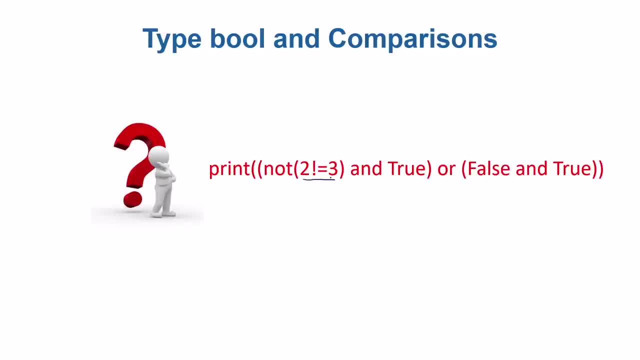 result is: 2 is not equal to 3.. Yes, it is true: 2 is not equal to 3.. That's true. So not true, Not true. The result is false, So this is false, So this whole thing is false. 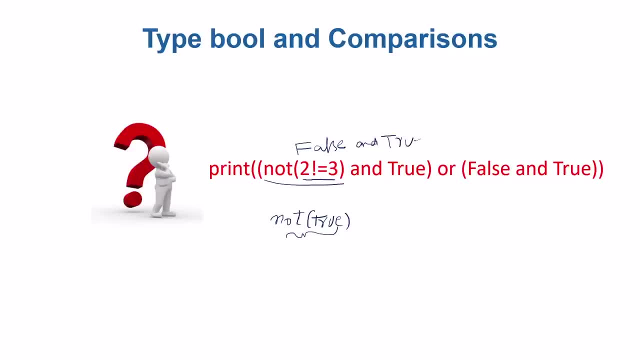 Now false AND true, False AND true. That is false. So this whole thing here till here is false. Now we have OR, OR, And then we have false AND true. Now, false AND true is false. So this whole thing is false. This whole thing is false and OR between. So false OR false. 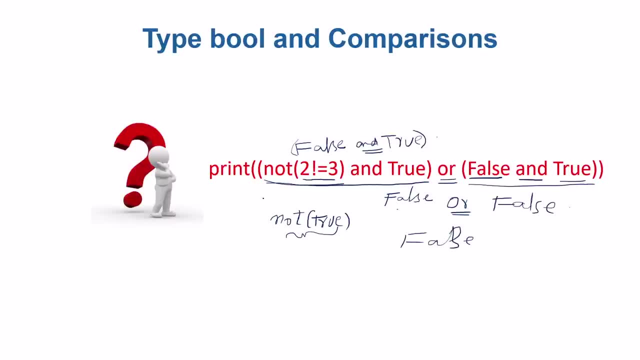 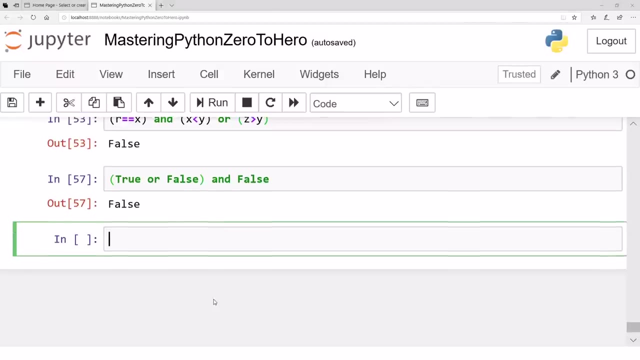 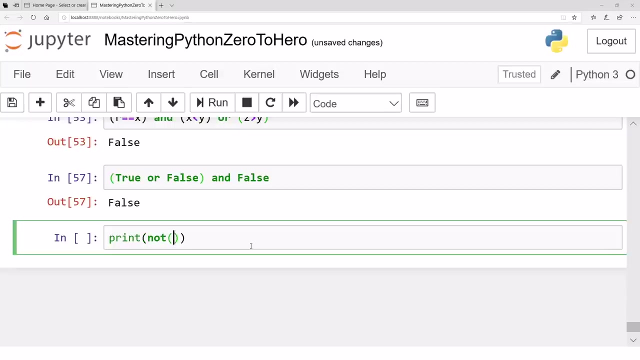 It is false. So the result of this… So the answer to this question is false. Let me just convince you by typing this statement in Jupyter Notebook: so, if you remember, we have print. print not two is not equal to three. and then we were having 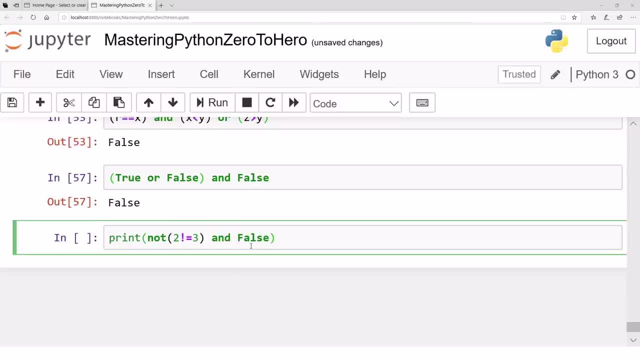 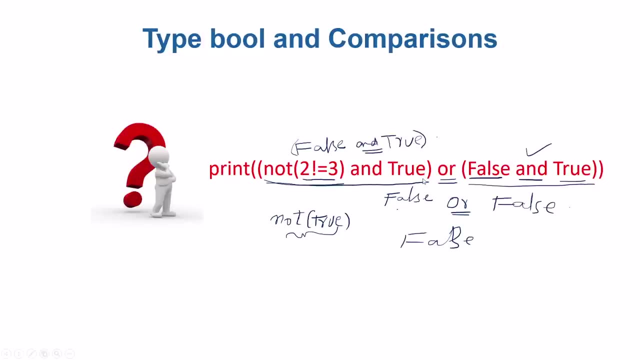 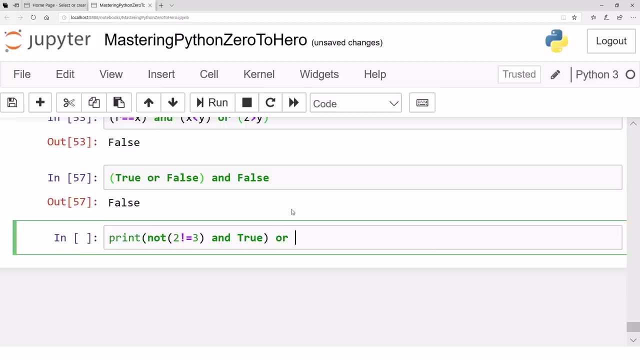 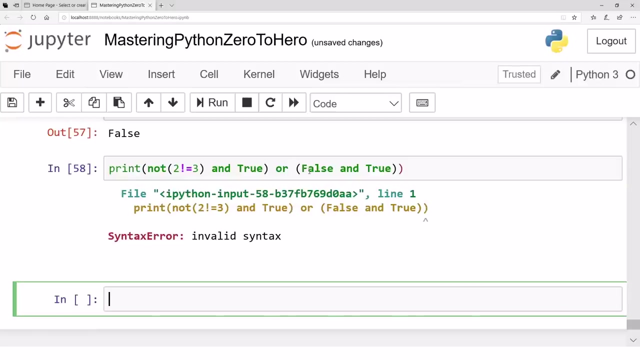 I guess, and false, and yeah, that was a different one. and true, sorry, that was and true, so this was and true. then we were having r and then we were having these, false and true. so the print ends here and the result is: oh, I have some, I have some parenthesis mismatch, so not true and this. 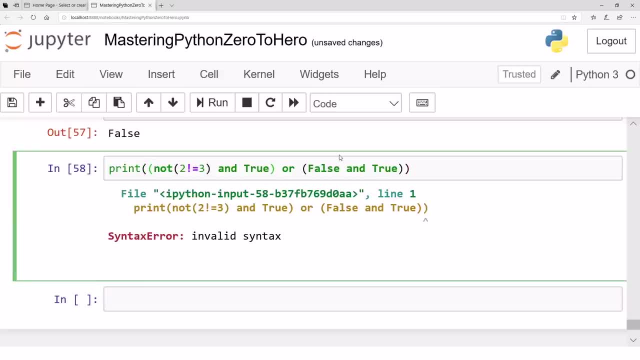 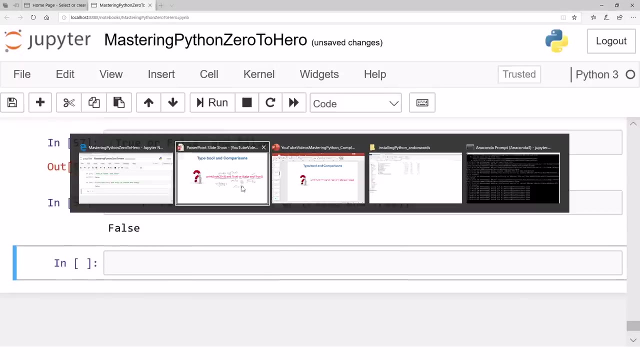 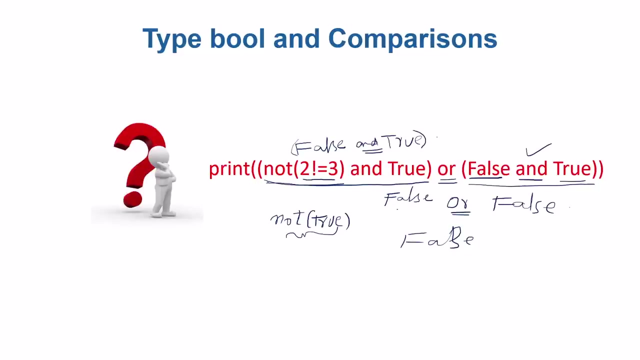 okay, I should have this one. I guess this goes to there and there goes to there, and I guess yes, so the result is false. the result is false, the. the purpose of this question was not just to. the purpose of this question is to appreciate, actually, the the fact how we can combine different boolean values. 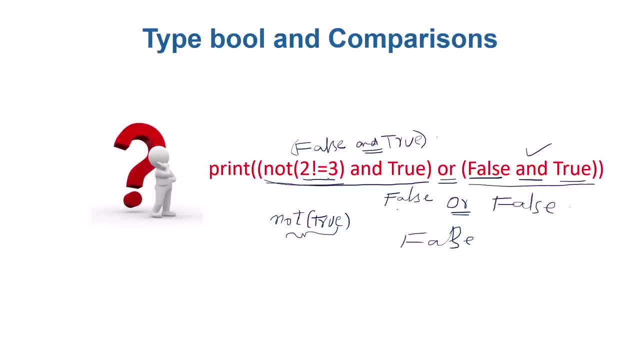 to, to, to achieve the final boolean value, and these kind of combinations will become very, very helpful further in in control flow when we will see the if conditions and the scene making and stuff. so the answer to this question is false. yeah, and I end this video here. in the next video we are going to see some 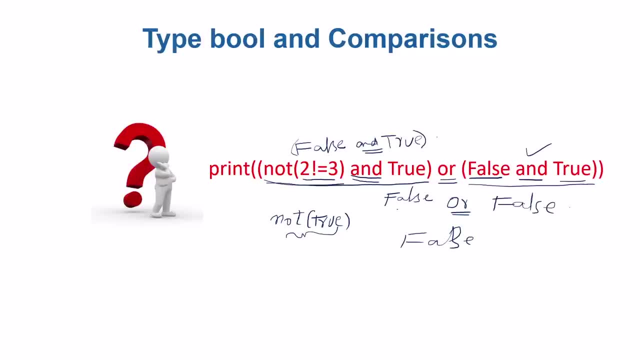 useful functions of Python and after seeing the some, some kind of useful. there are a lot of functions. we will see just a few of them, very useful of them, and after seeing those functions, then we will directly jump to control flow, control flow, basically the if, conditions and stuff, where you will see these comparisons, these 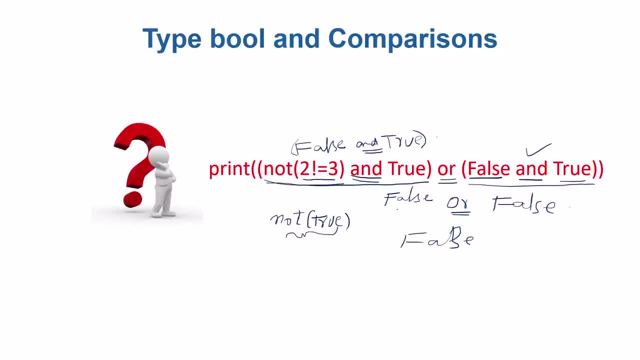 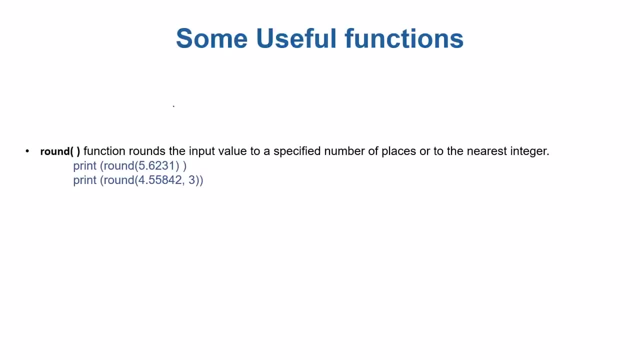 boolean values in a much more applicable sense than than earlier, so hope to see you in the next video. okay, so let's have a very quick tour over some some useful functions in python. obviously there are a lot of functions in python, but i will be covering just a few of them that i 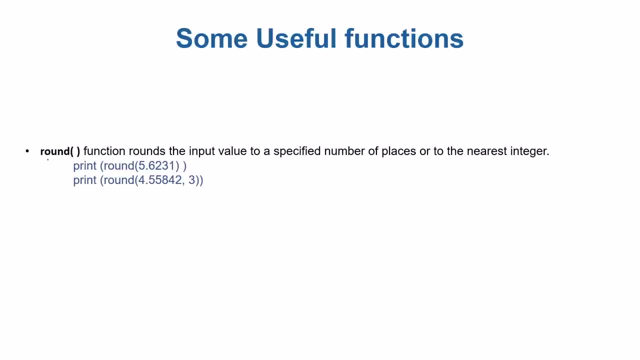 think with the passage of time we will be covering more and more, but let's start. a function, or sometimes particularly a built-in function, is is basically a feature from the language that is supplied for the users to achieve particular tasks, for example, a round function, if you give. 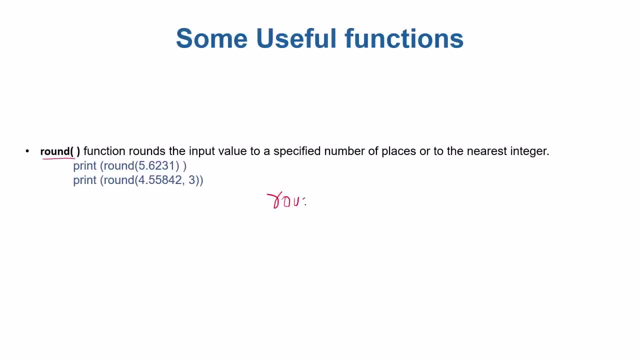 a round, for example, around, let's say, 4.6. this 4.6 is a floating point number and rounding means make it as integer. and what round does is it finds the nearest integer to 4.6. and the nearest integer in this case is 5, because 5 is more closer. 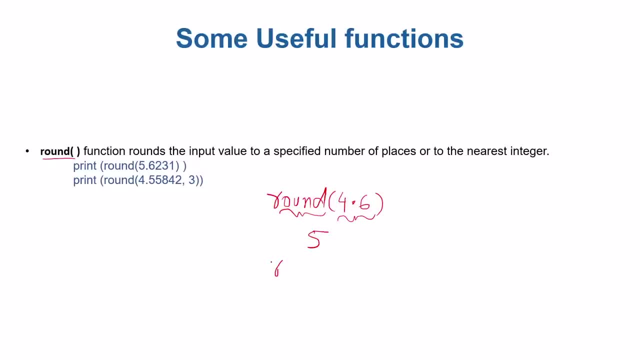 to 4.6 than 4. however, if you call round, for example, on 4 point, let's say 3, then the result will be 4, because 4 is more closer to 4.3 than 5. so that's one you use of round it rounds, basically rounds a floating point number to the nearest integer. another use of: 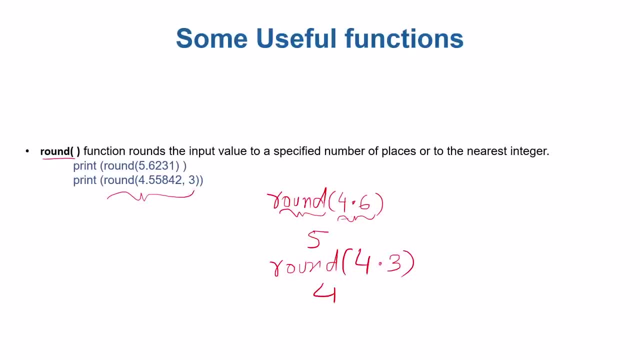 round is if you give another argument, that that is called an argument to the function. for example, when you write print, print, let's say a, this a is called argument to a function, print. similarly, round is a function. 4.6 is an argument. round is a function. 4.3 is an argument. 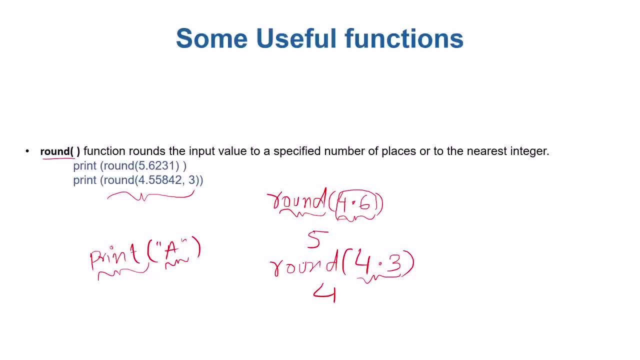 or the Boolean with order. so it's the same thing that they all Earth backwards. but all the early positions型 brings out Subt. Prison should be an operation, asטo, log 2.21t and ok next and the next most definitely a. we will see functions in details and they will be writing our own functions as well. for now, just just peer that, just beer with me. that functions are these kind of features that are available. however, we will be writing our own functions later on. so this particular function accepts two arguments. so round has two different kind of implementation. one is when it accepts only one input argument, it returns the nearest integer to that. if it accepts only one input argument, it returns the nearest integer to that. if it accepts an specialty, then the vieluverte argument returns the nearest integer. 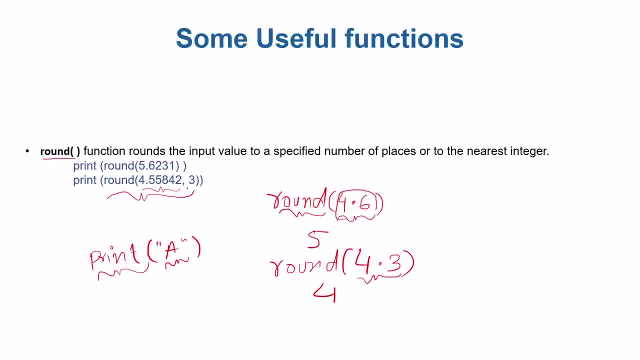 integer to that if it accepts a floating point number as well as another argument like here: we have three. that means after after point, after decimal, go to three places only and then round up, then round, for example, this four point, five, five, and then it will be rounded based on its next value, if the next value is larger. 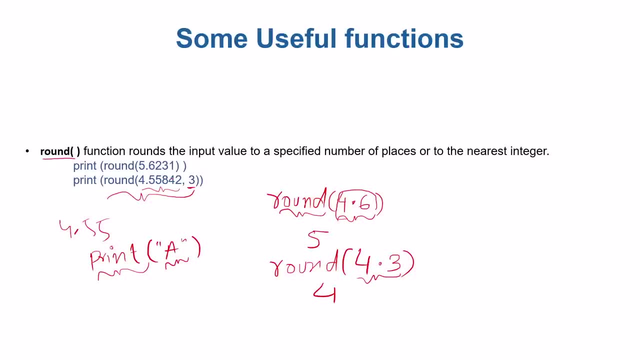 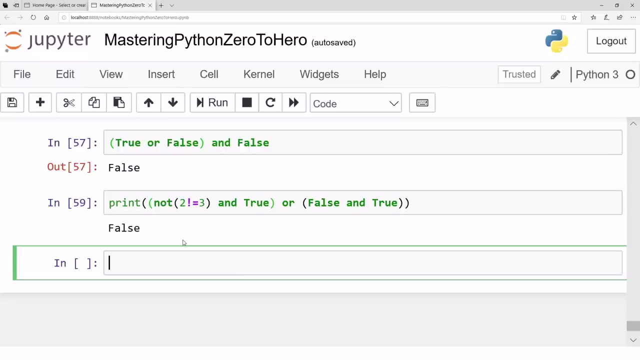 than five, then it will go to nine and stop. if the next value is smaller than five, then it will stay as eight and the result will be three decimal places after this. so let's practice this round function just on a jupiter notebook, very quickly, let's see. so here we are. so let's say print round. let's say four. 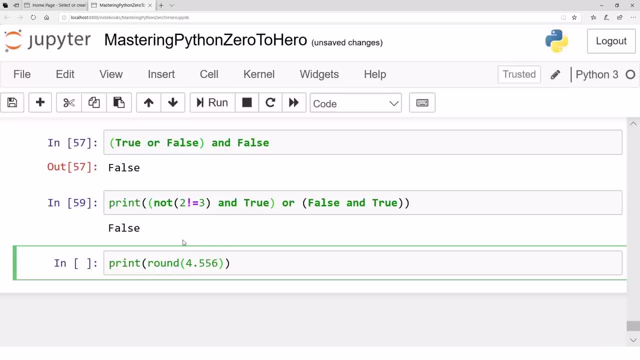 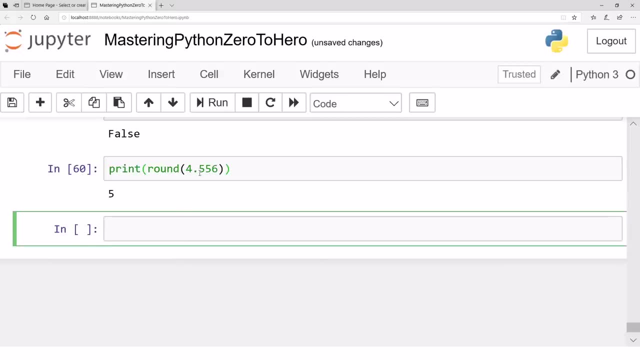 point five, five, six, and in this case, the result will be four point five, and the reason is: four point five, and it's rounded up, it stays to five, and the reason is this: four point five, five, six. it is more closer to five than than four. however, if you, if you just print round, 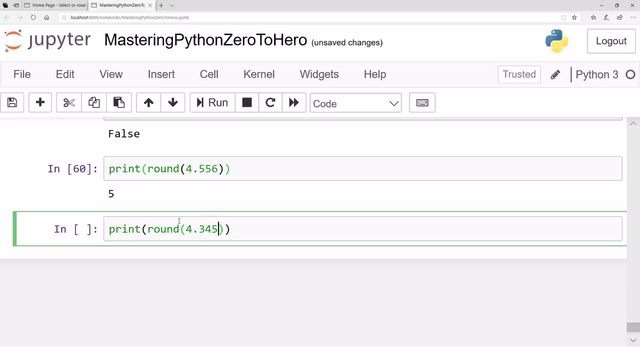 four point. let's say three, four, five, let's say, and the result will be four. the reason is: four point, three, four, five is more closer to four. however, if you call this round function with more than one argument, for example, four point, five, five, six, seven, eight. 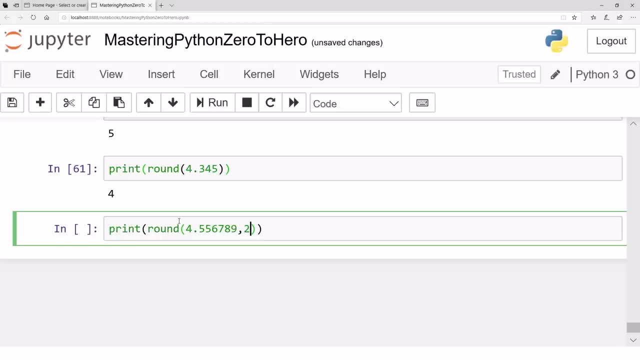 nine, let's say, or with argument, let's do. that means the result should be only two decimal places after the after the decimal point. so in this case the result is four point five, six, and the reason is this: five is rounded based on the next digit, and the next digit is larger than 5. hence it is rounded up so 4.56. if 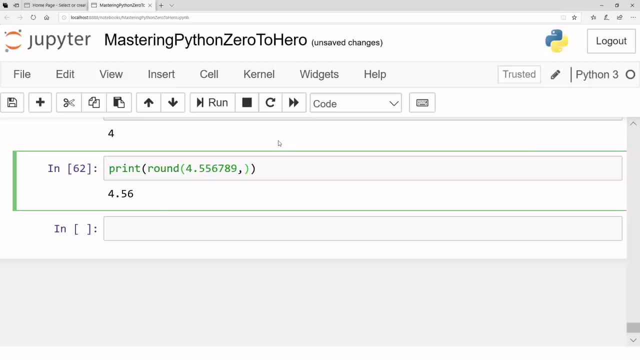 however, I call this function for 3. then what do you think? what will be the result? it will be 4.55 and the 6 will be rounded up based on this 7 and it will become 4.5, 5, 7, yes. however, if, for example, there will be a value at the: 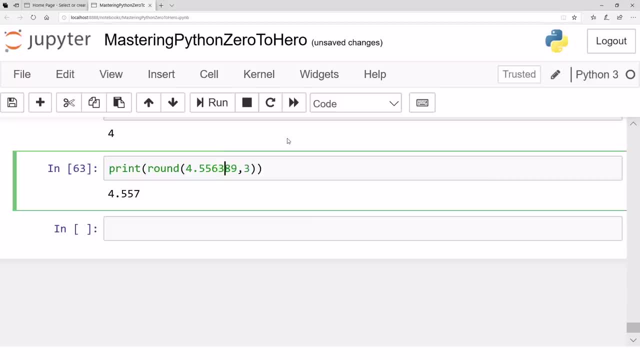 place of 7. if there is a value, let's say 3, then you call this function then 4.556, and then, based on the next value, 3, the 6 will stay as 6 rather than going to 9, and the result will be 4.556. yeah, so that's a, that's the, that's the round. 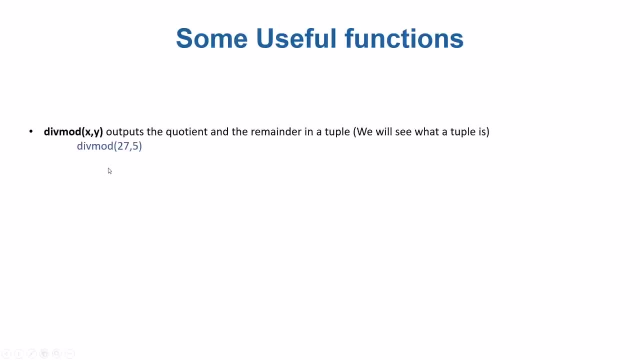 function basically. another function is diff mode. diff mode function basically divides and returns quotient and and remains so. in the next video we will be seeing this diff mode in detail, how it actually works and how, how it is useful. so in this particular video we saw a round. 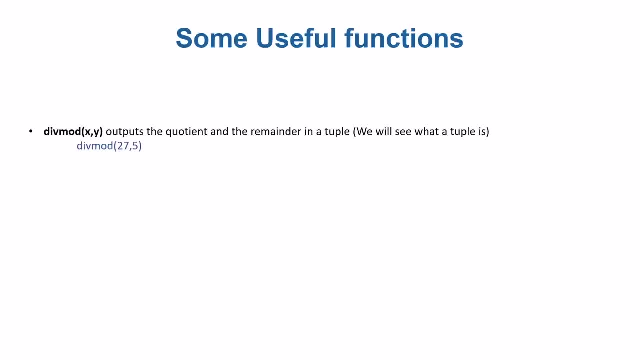 function. in the next video we will see diff mode and there are a couple of more functions that we will see in the upcoming videos, so hope to see you in the next video. so in the last video we saw round function that sometimes accepts one argument and sometimes accept two arguments and behave. 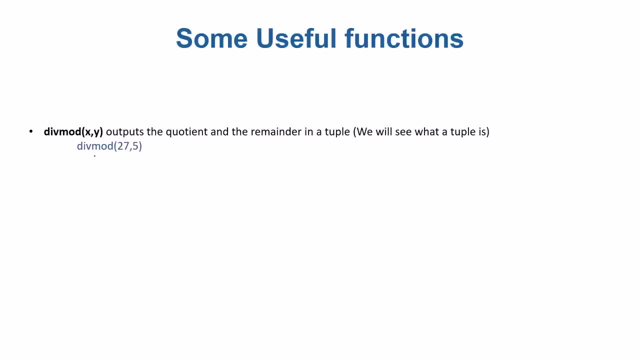 accordingly, in this particular video we are going to see another function, diff mode, and it accepts two arguments, two different arguments, maybe same or different arguments, and it it returns two outputs, two numbers. it returns basically quotient and remainder. for example, in this particular case, the quotient is 5. 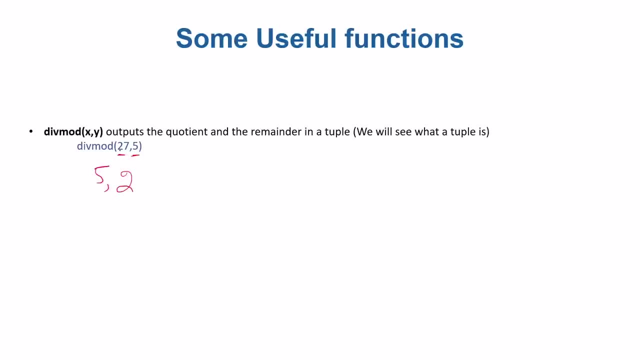 and the remainder is 2, because if 5 is divided by, if 27 is divided by 5, the result is 5, but then the remainder is 2 and the result is returned in a kind of an ordered pair, and and this kind of collection in which we have two or more elements, we call these collection as 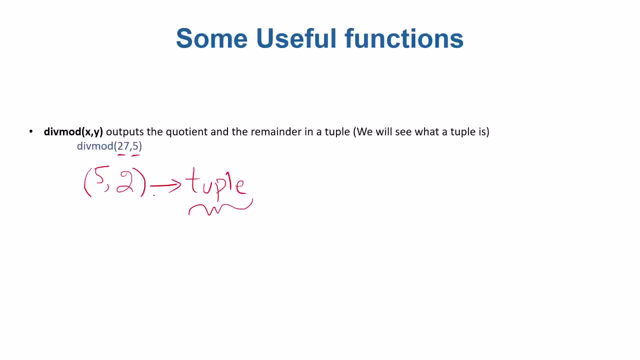 tuple. that we will see in detail when we will see the data structures module of this course. but right now, just bear with me that it returns two numbers, two elements, and the two elements are ordered in an ordered pair, which is a, which is called a tuple. tuple is not just an ordered pair. it can have three more, three, four. 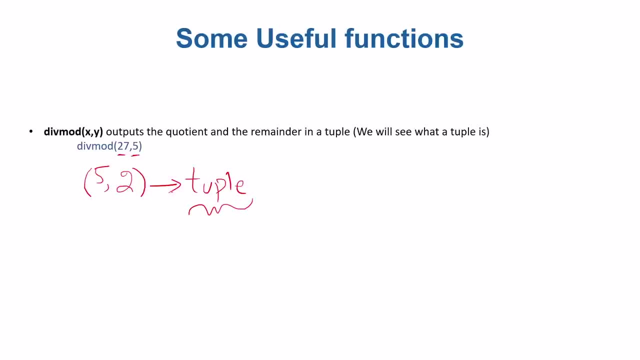 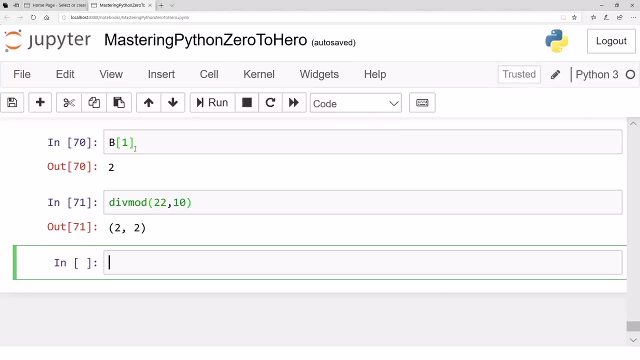 five or seven or maybe several elements, but right now we will. a tuple is just an ordered list which we will see in detail. so let's see the working of this div mode function in in jupyter notebook, let's see. so let's say we have div mode. let's say, for example, we have 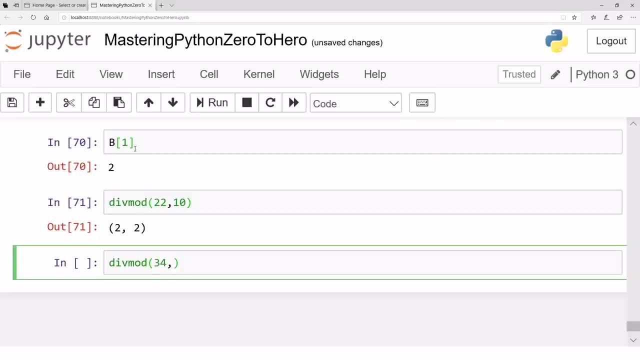 34, and then we have, let's say, 10, or maybe let's say 9. so what do you think? what will be the quotient and what will be the remainder? so 9, 18, 27, so 3, 3 is the quotient and the remainder is. 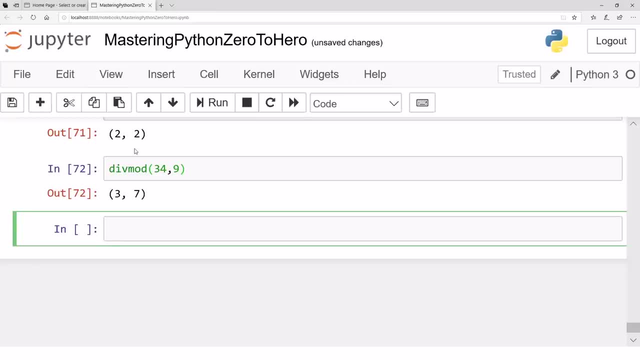 remainder is 7. so 3 is quotient and 7 is the remainder. so and if you save the result, for example, if you save the result in a variable, let's say g- you. so if you see the g, the type of g, if you, if you just type the type of, 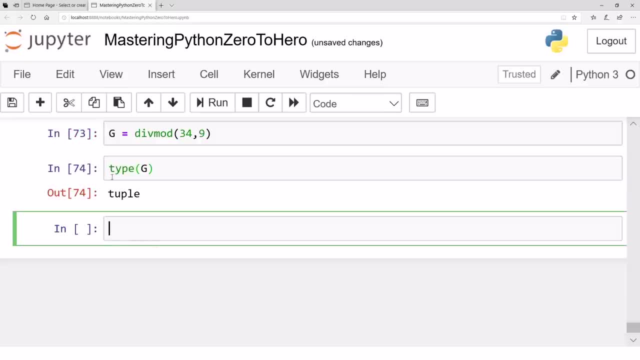 if you just print the type of g, it's a tuple which we will see in details. and if you see the contents of g, if you see the contents of g, the contents of g are three and seven and if you want to access each element independently, then you can access the element. 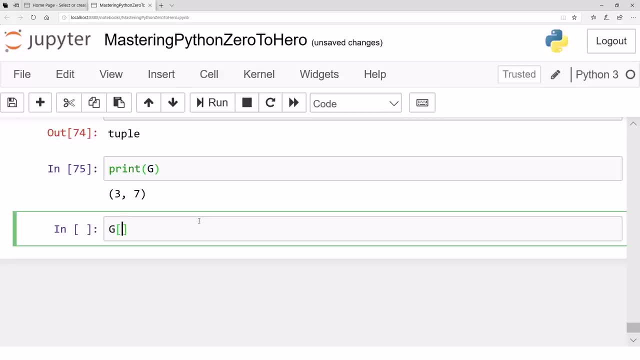 first element, because the if there are multiple elements in in a variable, normally that that kind of variables are called collections. that we will see in detail later on. and these are the indexing, the, the positioning is start by zero rather than one. so g zero means the first element of g, which is three in this case, and 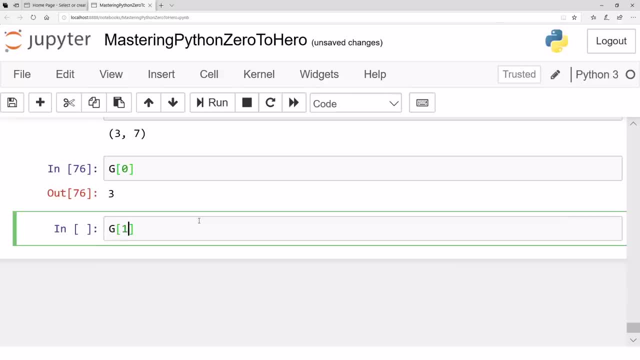 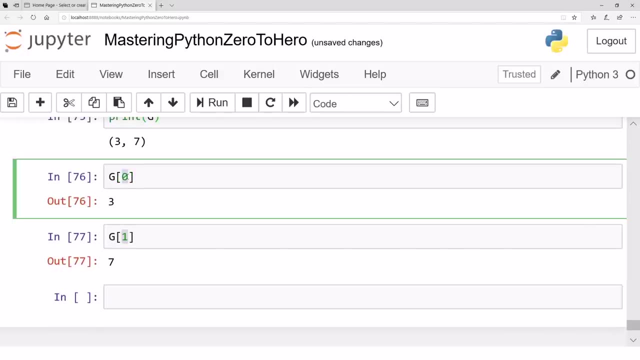 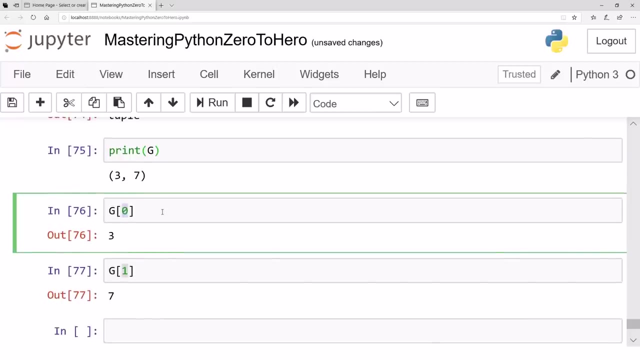 the second element of g is one at at one which is seven. so this is basically this is called the index or position of, of elements or data in in this particular collection. we will see these indexing and and all these kind of collections in detail uh in, uh in the, in the data structures. 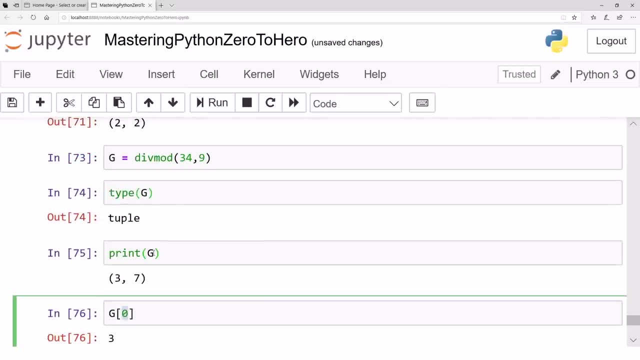 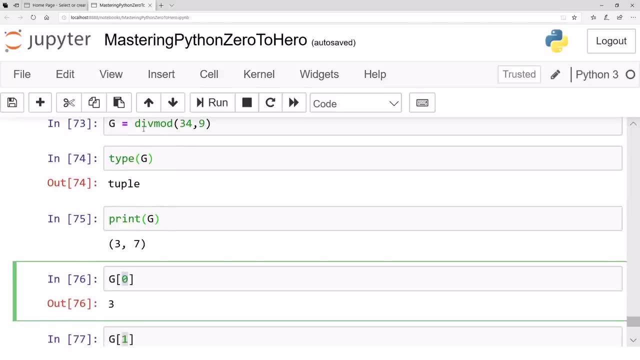 course, when we will see arrays and strings and uh, different kind of structures but and div mode sometimes is uh, is basically uh. sometimes it is helpful, by the way, you can achieve div mode by by another, by another thing. for example, if you want to achieve div mode 34- 9, you can do the same. 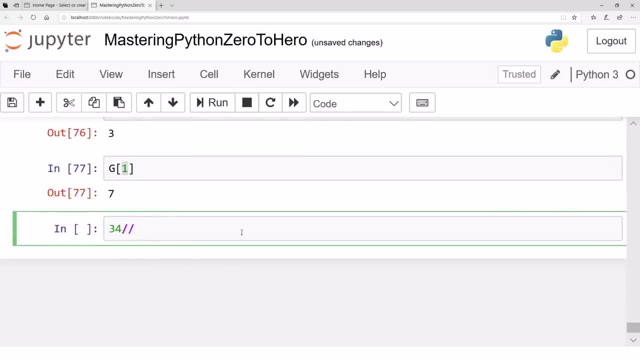 thing by, let's say, 34 divided by- uh, double divided by 9, that will give you quotient and the quotient is 3 and further if you write 34 remainder 9, and that will give you the remainder that you need. so you can call that. 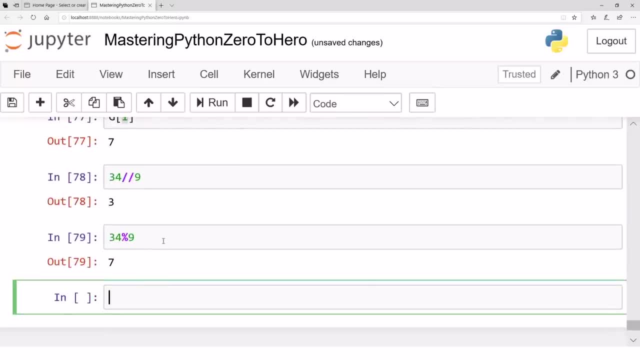 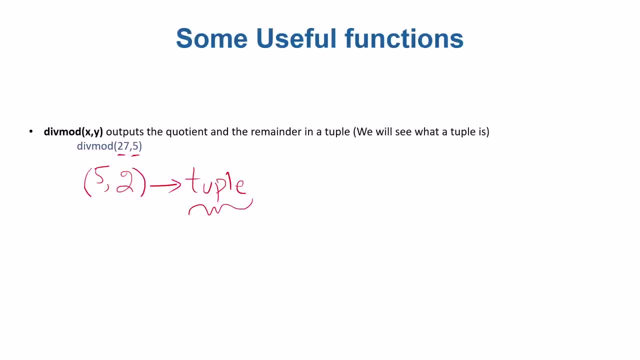 function, div mode, or you can use these two. there are multiple ways of doing the same stuff, okay, so, yes, so i mean, sometimes it is useful when you're coding and knowing this kind of function that returns quotient n and uh count form. uh, remember that there are. there are missinputs that don't belong there, but you 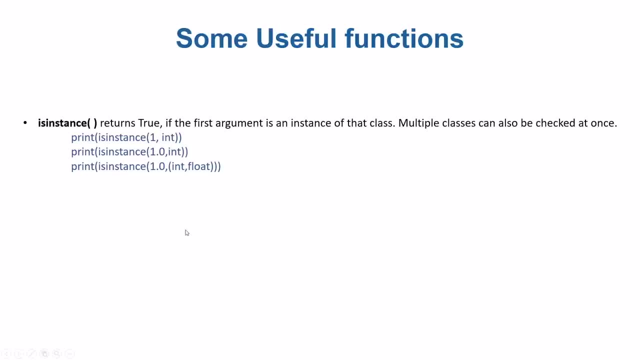 don't have too many. if i who want toberger an white matrix, then you have to enter broad n and so here what? what is this? um? what is this term? enter, and here uh, this mean type is isntave, so it's called a function of uh, of fittings, and it's basically just a function for. 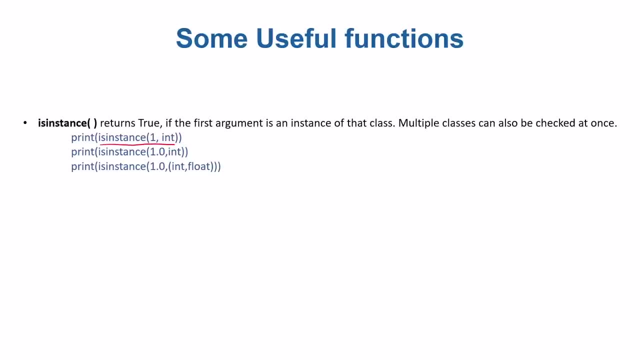 the same type, ofician, as well as its native type, which is function of the équ록, in space liegt, and so this is shows that this is somehow mole. so so you can check that using this function. By the way, you know that one is of type integer. then you may think that why on earth one should be interested in? 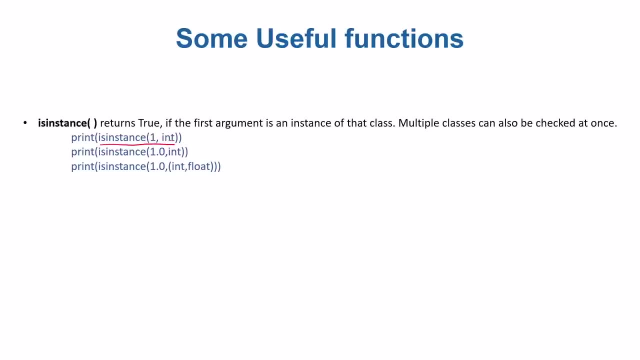 checking the type of one, if somebody know it is integer. Sometimes we have certain variables and certain data is stored in it and we want to check the data inside. it belongs to which kind of type and in. in several cases the value to this variable is not assigned by us. it may be read from some file or maybe. 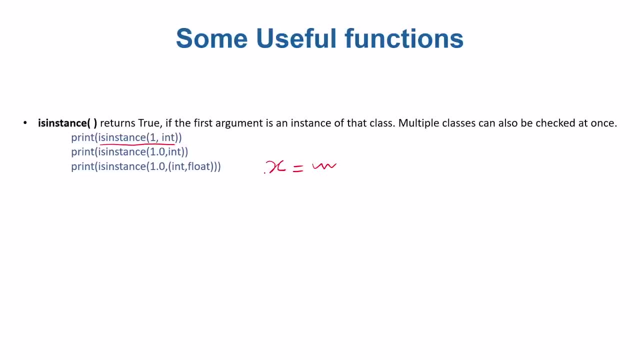 through input. a user gives some number or something like so. So sometimes it becomes important to check the type of a particular way. if we are expecting a particular type of the input and the input is different, then this function might be helpful somewhere. Either way, this is a function available. 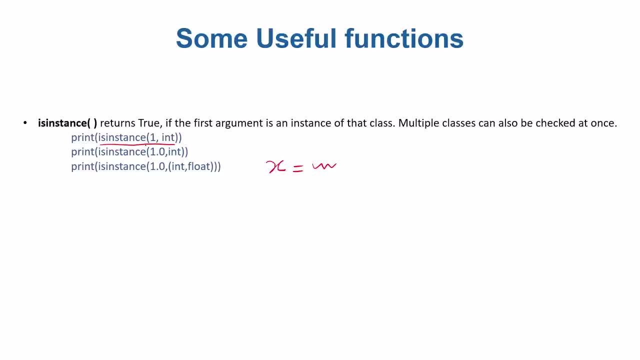 in Python and it checks whether the given value has a particular type of. not So, is instance one int returns true. is instance 1.0 integer that returns false? maybe because this is a floating point number and you can check a particular value belongs to one of the. 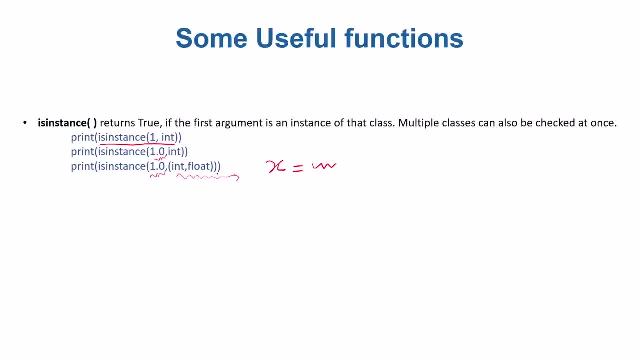 several types or not. you can give several types in in a, in a tuple, and you can check whether it belongs to this this or not. So let's go to Jupyter notebook and see, Actually, how it works. so, by the way, this is the same notebook that we have. 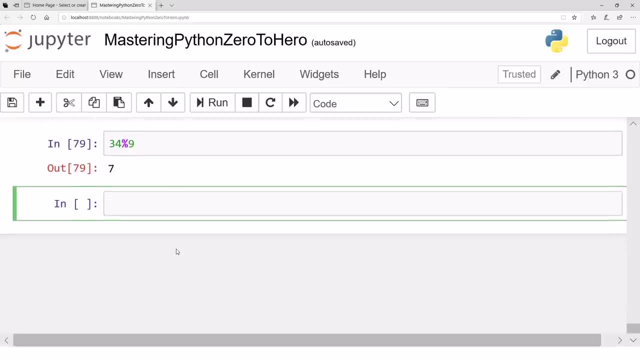 that we are populating. So hold on with me, at the end of the day will be having one notebook complete. So is instance, is instance, let's say three, is that instance of integer? the result is true in this particular case If, for example, we check: 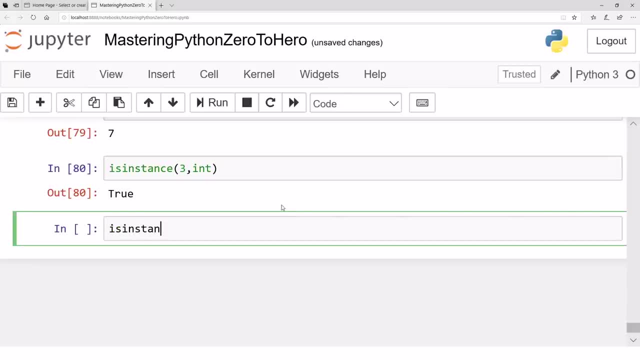 whether is instance three. point four is that and indeed, is there an integer? the answer is no, it is not an integer. If, for example, we check, if this is not an integer, then maybe it is a float. the answer is yes, Or maybe we check that for. 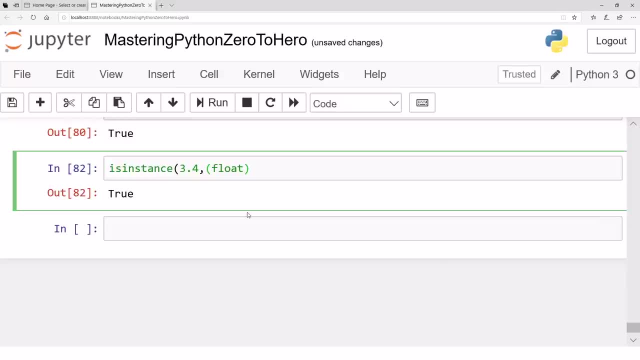 example, if that value is either float or integer, if it is one of these values, this one of those values, if that value is float, then maybe it depends. If, for example, we check, if this is not an integer, then maybe it is a float. the answer is yes. Or maybe we check that, for example, if that value is either float or integer, if it is one of these values, then maybe it is a float. 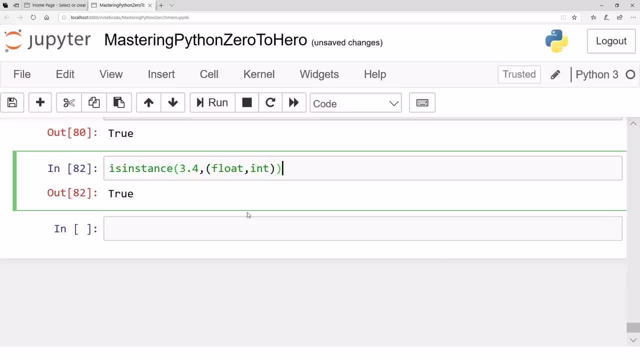 If the delta value is not an integer, if we Shamfari cigarettes it out, it will not get flow. if it is one of these, then I mean check that a particular value, in this particular case 3.4, whether it belongs to one of these types. we can increase these types, for example. so let's say we 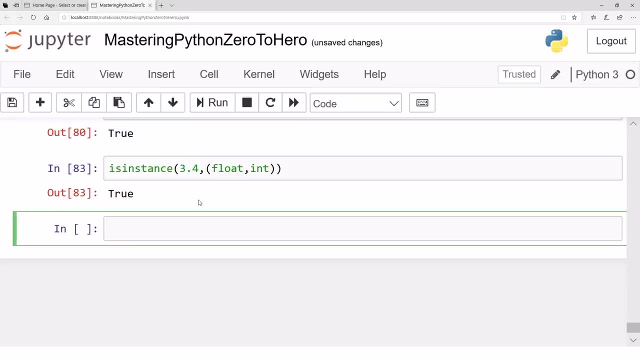 we gave a complex number here, and check is instance. let's say 2 plus 3 J. that's a complex number. and let's say we ask whether it is an integer or float or not. the result is obviously false and the reason is it is neither integer nor float, or even if we give string there, STR, so it 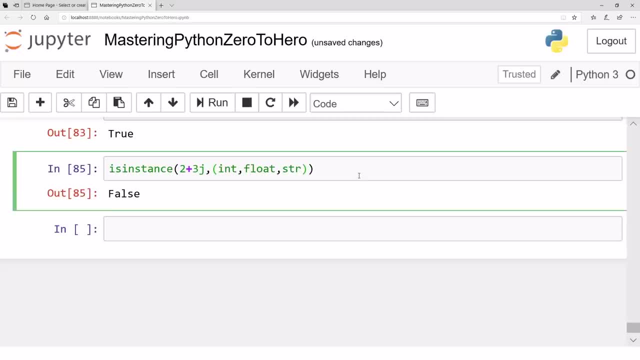 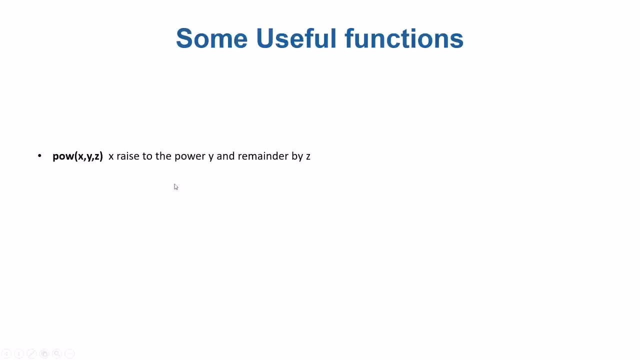 will still say no, it is not not any of these, but maybe there is a complex data type. if we see that, that says yes because it is complex. so sometimes this is instance becomes really useful. next function is power. so power you can. you can compute power, by the way, using using, for example, if you 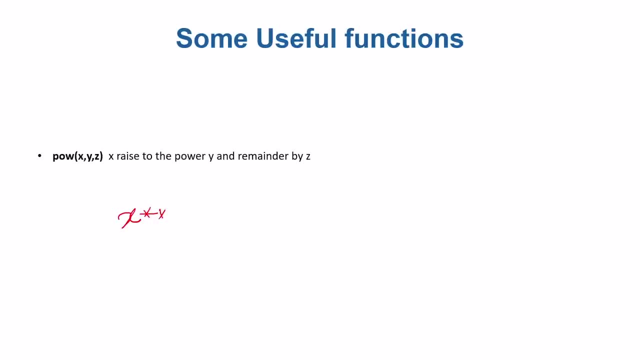 want to compute X raised to the power Y, you can use double star and that computes exactly X raised to the power Y. or, equivalently, you can call the function bow X, comma Y, and that will give you the the same result as this one. but power sometimes take three arguments as well, and in that case it: 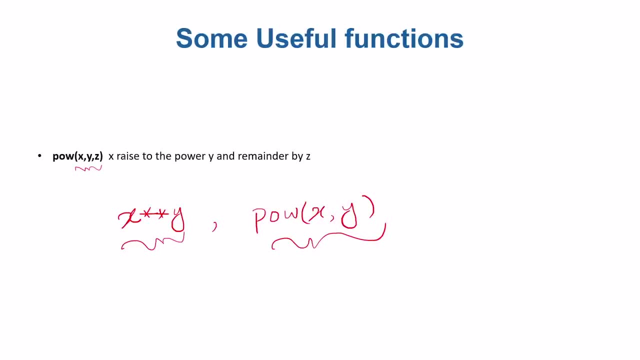 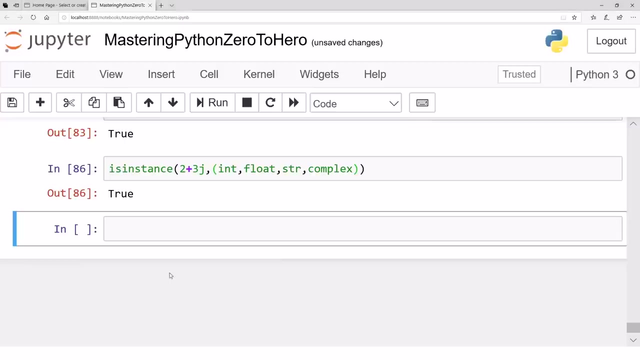 it. it performs the power function in a different behavior. so, for example, if you supply three arguments, what it does it? it raise Y to it, X raised to the power of Y. whatever the result is, then it takes the remainder by Z and gives the result. so let's see the functioning of this power function in Jupiter. 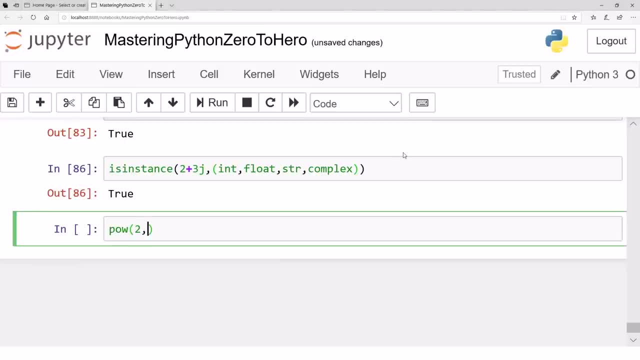 notebook. so let's say power. I want to compute 2 raised to the power 4.. the result is 16.. no problem, 2 raised to the power 4. I can compute the result 16 this way as well, but here is another way. how can we use this? 2 raised to the power 4. whatever the result is, then I want to take the. 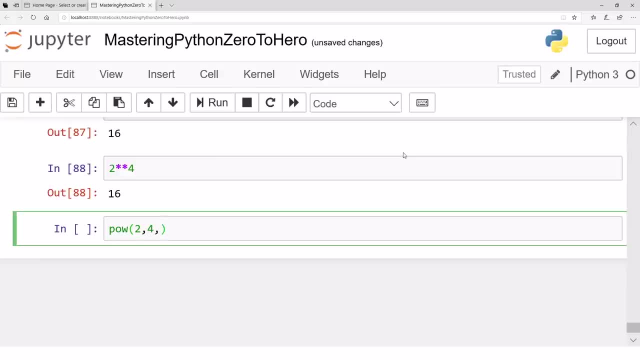 remainder by. let's say, I want to take the remainder by 7.. 2 raised to the power 4 is 16. then if we take the remainder by 7, the result will be 2 and that's the result 2.. so that's how you can use this power. 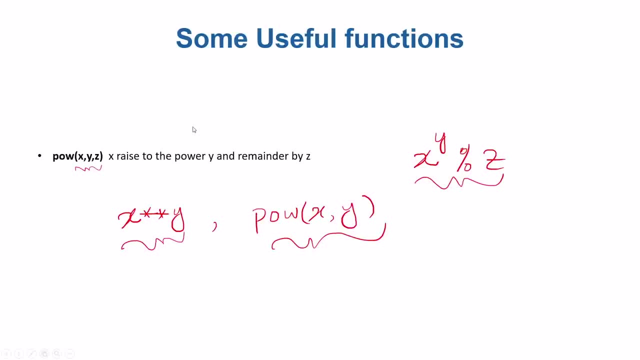 function. I'm just introducing you some built-in functions that are available. there are so many functions that are available. I'm just getting you comfortable with these kind of functions so that in future, if you see another function that you have not seen here, you'll be able to use it and and apply it. so in this, 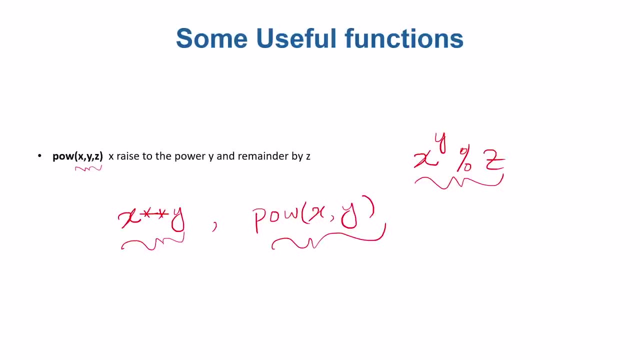 particular video we saw. this is instance function and this power function. in the next video we will see one more function that will allow you to take input from the user. so far, we are supplying values or assigning values to variables directly. what if, on the fly, we want to give the values and those values should be assigned to the variables? so in the 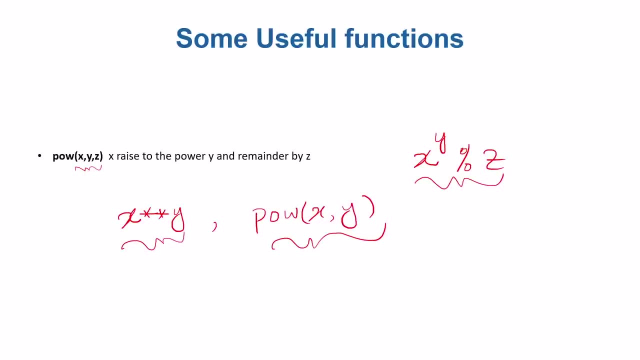 next video we will see the function. we will see a function that will allow you to give input from the keyboard. hope to see you in the next video. so in this video we are going to see a very important function called input. this function is- I mean, this is beneficial for taking input from the keyboard. 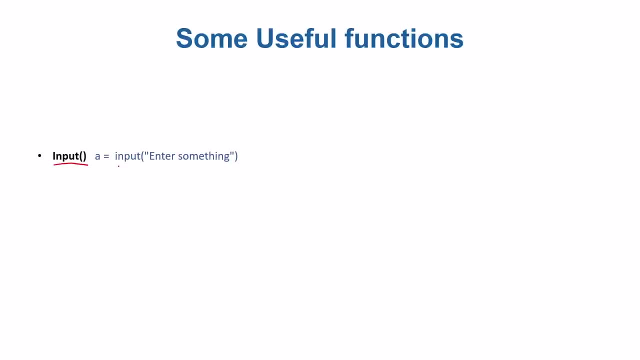 from the user. and the way to call this function is you type input and then you type a message that actually describes the expected entry, that, for example, into something. if you want somebody to, or tell somebody to, just enter, let's say a number, you can write enter number or any. 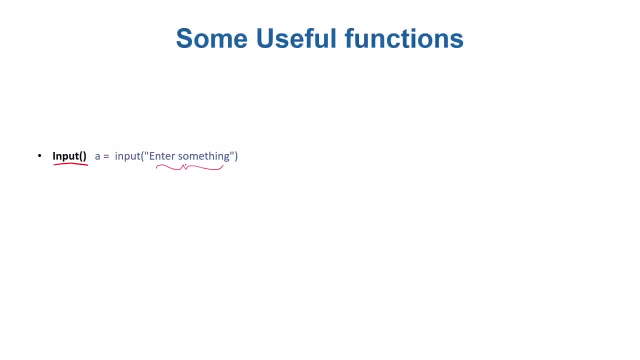 specification to help the user to enter whatever and put the user want to enters properly. and one thing is that no matter what the user will enter, the variable a will be having type string: str. so even if you enter a number, let's say 12 or 34 or whatever, that will be received as a string. 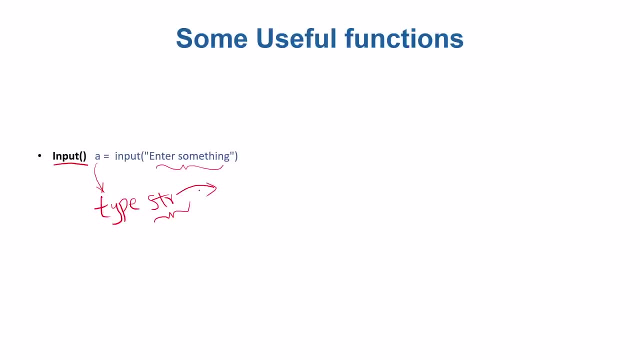 and then there are ways to convert string to number. if that really was a number or so, whatever you receive using input function will be a string. and then there are ways to deal with that string. if that was a number, how to convert that string to a number, and and so on. so, for example, let's see: 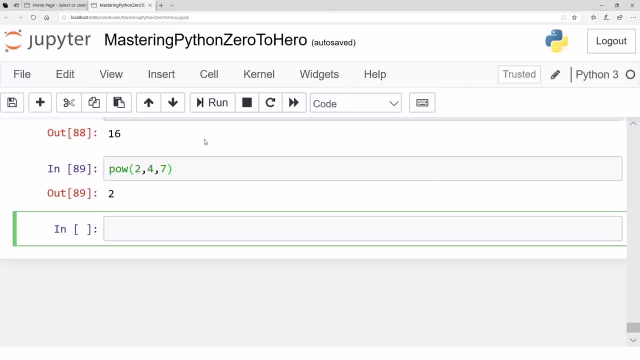 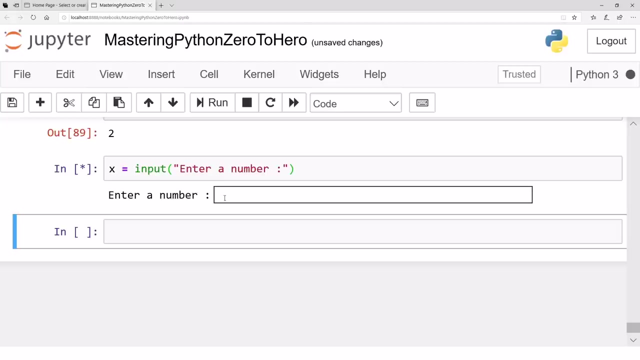 uh, let's see on the Jupiter notebook how it works. so let's see, for example, x is equal to input. enter a number, let's say, and then. then, if I press shift enter, a prompt will appear in front of you that will require you to enter a number. for example, if I enter, let's say, 56, and then I 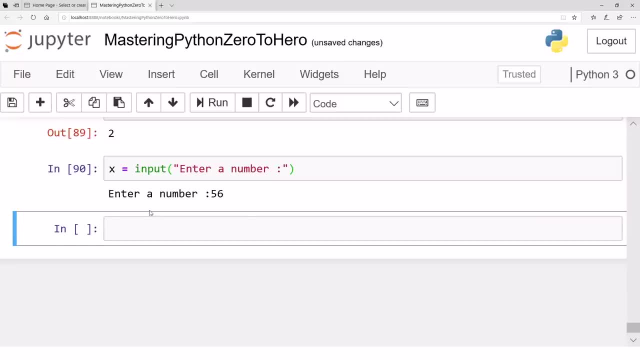 press enter, not shift. enter enter, then x will receive 56.. now you might be thinking this 56 is an integer, so the type of x should be an integer. but this is not the case. the type of x will be a string and the reason is: whatever you enter is received as characters five and six, even. 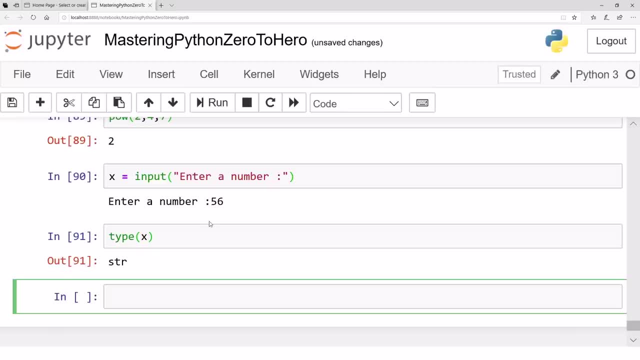 because that would have been received as a sequence of characters. so this is no longer a five as a digit five, six as a digit six. these are some characters. sequence of characters. now, if you want to, I mean, there are ways to convert this- x, for example. maybe you want, let's say y or x as int x. 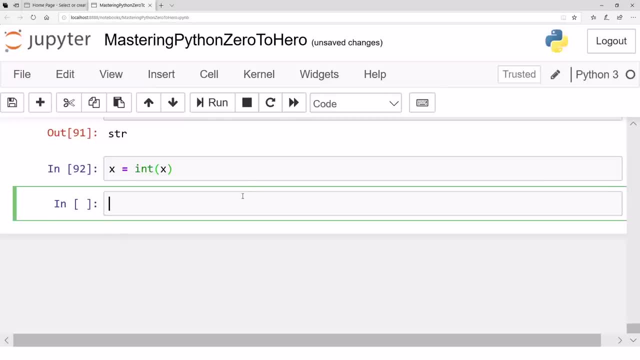 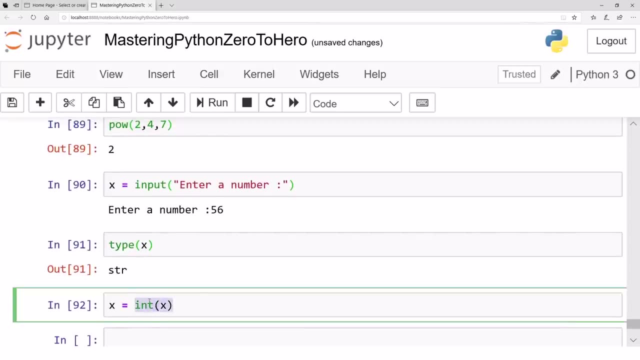 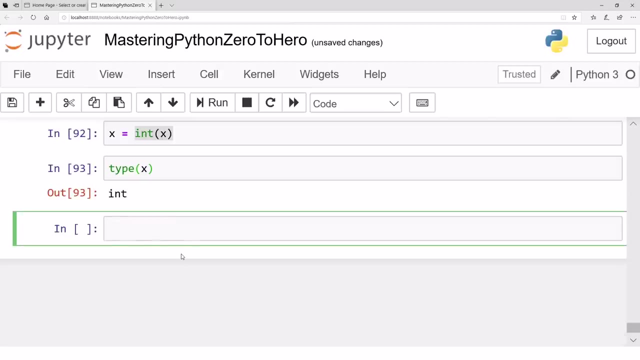 so this means you have now converted this string to integer and then, whatever the result is, you have stored that result in x again. if you now see the type of x, uh, type of x, the result is integer, and you can for example print x minus 34 and the result is: 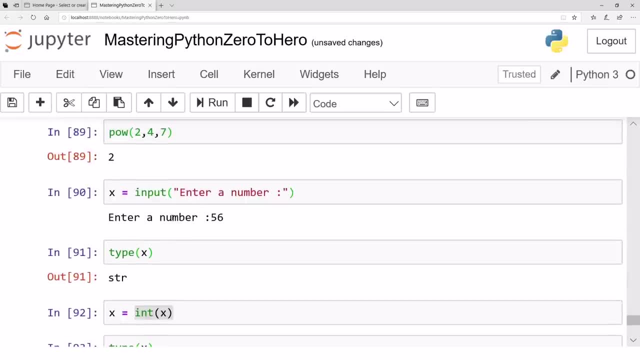 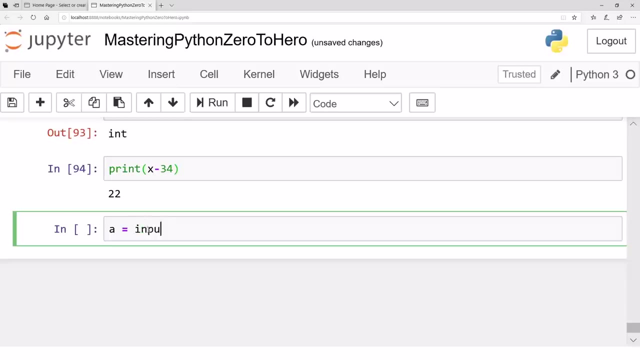 22, because x was, x was 56.. so this input function is- I mean it is, and one way. by the way, if you are expecting an integer or a float value, for example, let's say you are expecting a float value, then it is good to write input. let's say: enter a real number. 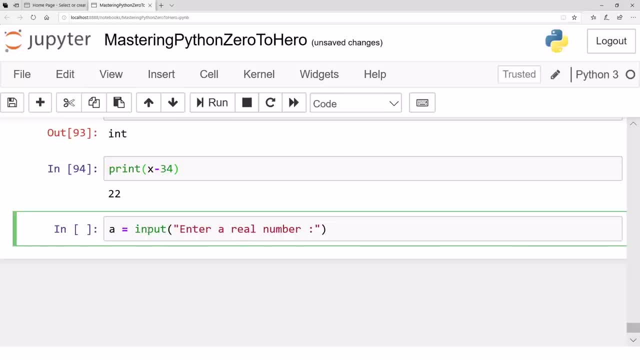 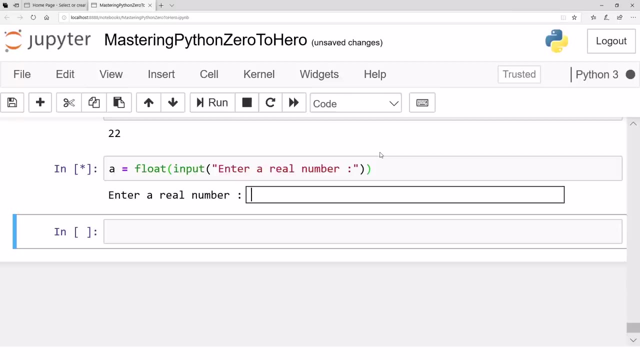 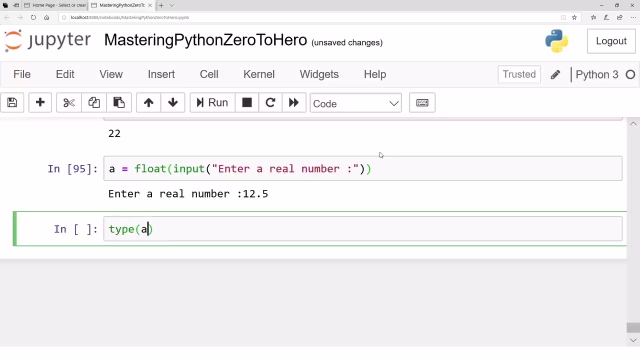 maybe, or, or any message, any message, and then at this particular time, at the time of input, then it is okay to convert that thing to a float and it will become a float. yeah, that's it. so now, for example, you enter 12.5, if you see the type of a, now, type of a will be float, okay, but there are 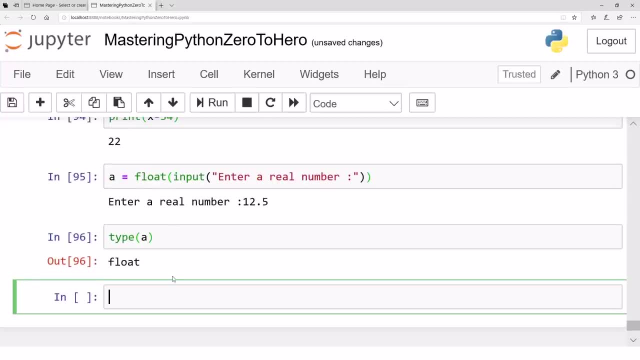 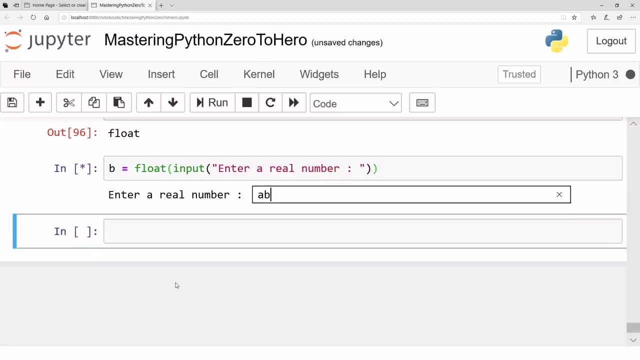 problems. for example, if you are, if you are expecting float, and somebody enters, uh, enters something that is not float, for example, a or let's say b equals float. input, enter a real number, let's say, and then you press shift, enter, and somebody just enters, let's say, abc. so now this: 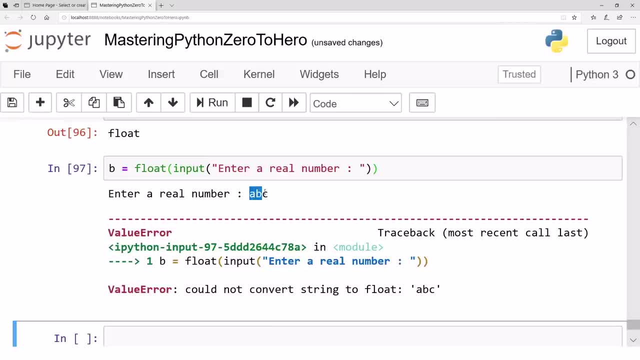 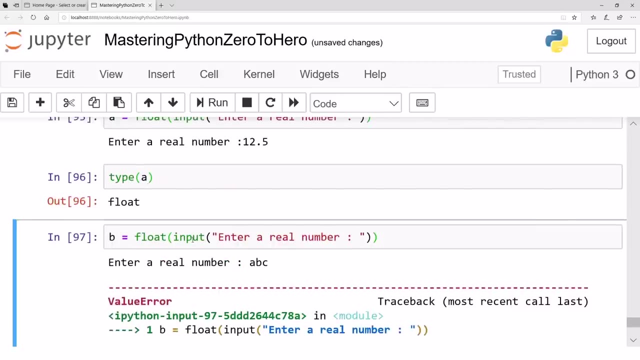 is not a float, abc cannot be converted to a real number no matter what, so you will catch an error. there are ways to avoid these kind of errors and programming program breaks using exception handling, and there are other ways, but be careful. I mean, the user is not. 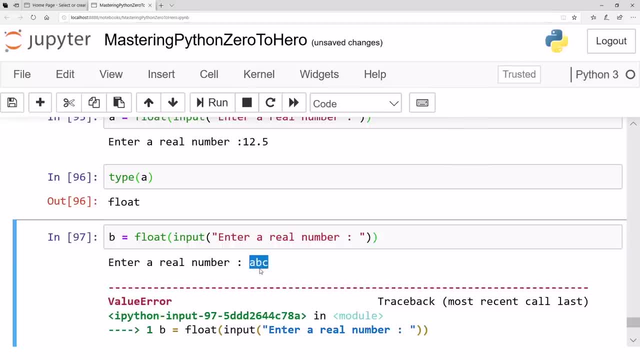 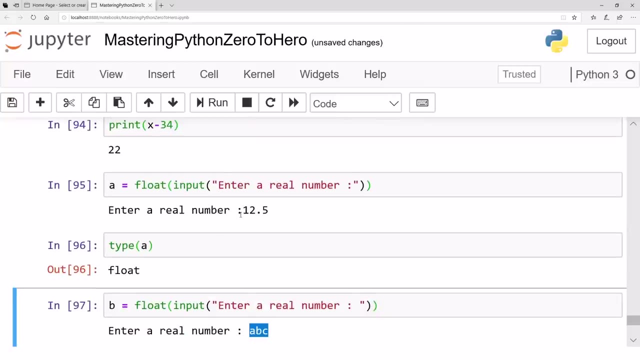 um, I mean the one who is going to enter the, the enter the input. if that that user is not restricted enough, then you can get errors. so i mean this is not the case, that whatever you will enter it will be converted to a float. if it really, if whatever you have entered is really to convert, it is really convertible to a. 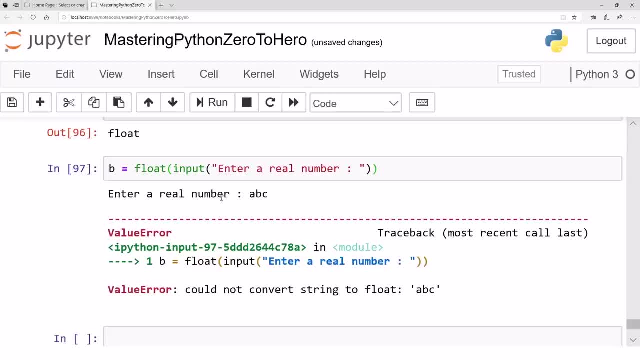 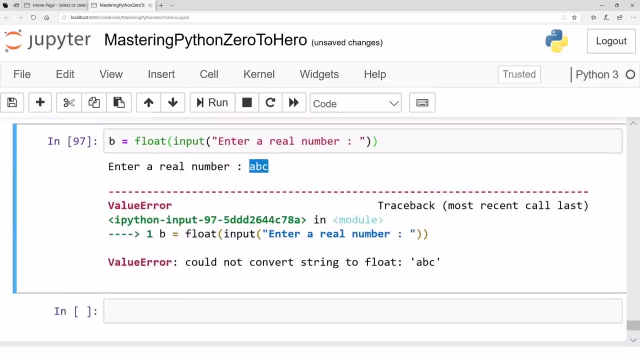 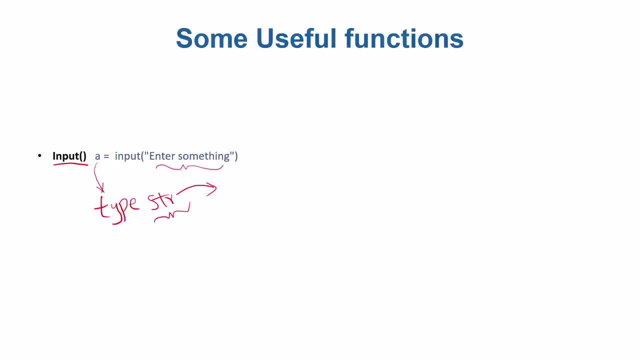 float, then it can be convertible to a float, not otherwise. and at the input time there is no restriction. you cannot restrict the keyboard to enter what or what not, although there are ways, although there are ways to do that. so that's about the input function. so we have seen some of the 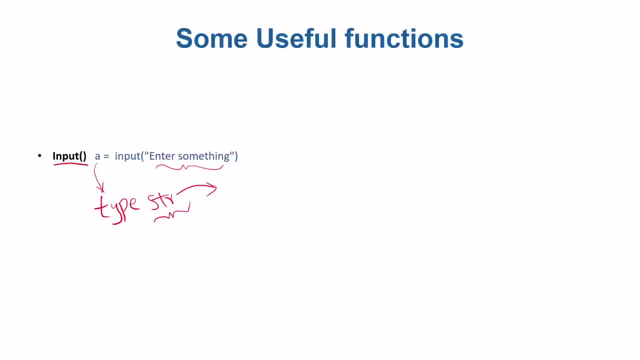 functions. let me just let me just go through quickly. we have seen input. we have seen is in stance. we have seen div mode. we haven't. we have seen power function. we have seen the round function and there are several others. yes, so from now on we will be actually moving towards. 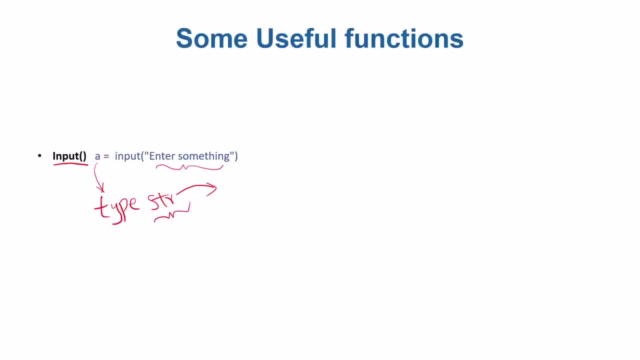 basically decision making based. sometimes we will use these kind of functions. mostly we will be using input function, but sometimes we'll be using maybe other functions like these functions and sometimes we will be doing decision making based on these and and stuff like so one thing that i 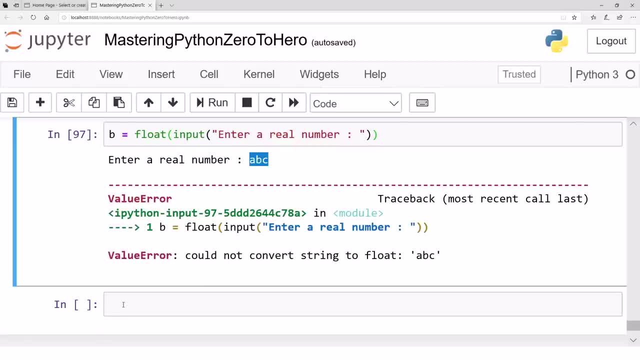 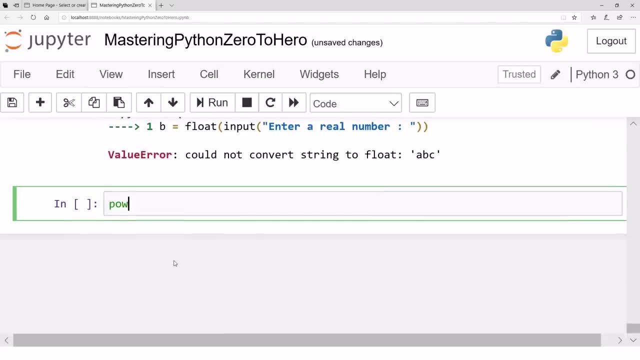 want to tell you is if, for example, you know the function name- function, let's say like power- you know that pow, power is a function, but you do not know how to use that function. one way is to just type a question mark in front of it and then just press shift- enter. 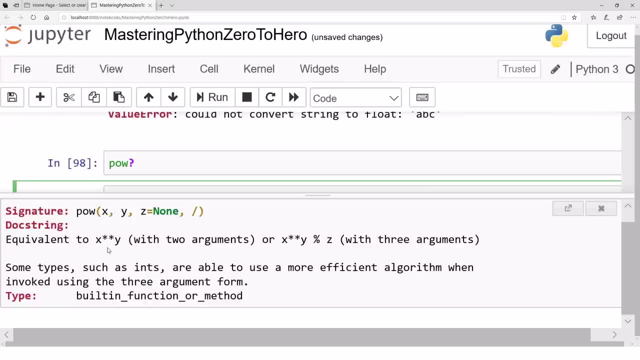 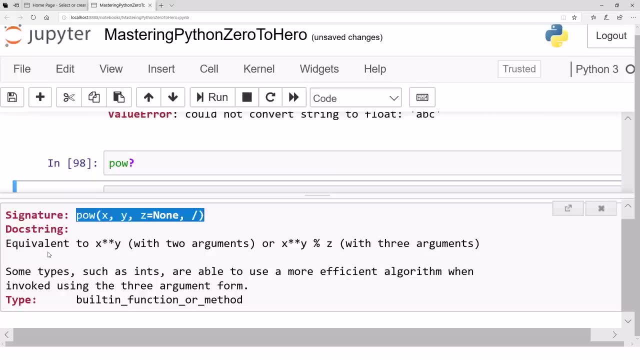 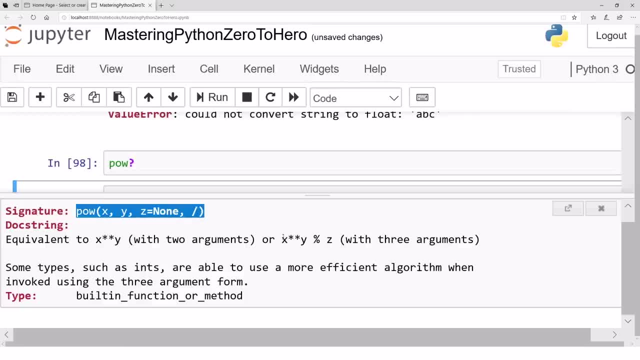 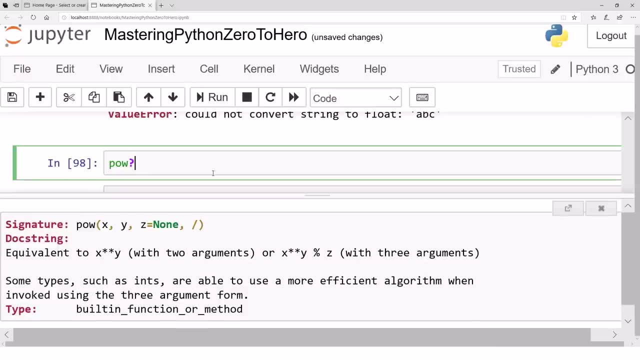 x raised to the power y with no arguments, with two arguments or equivalent to x raised to the power y, remainder with z with three arguments, and so on. if you want to see implementation of this function as well, we will see the functions later on, but if you want to see more about the help, you can type: 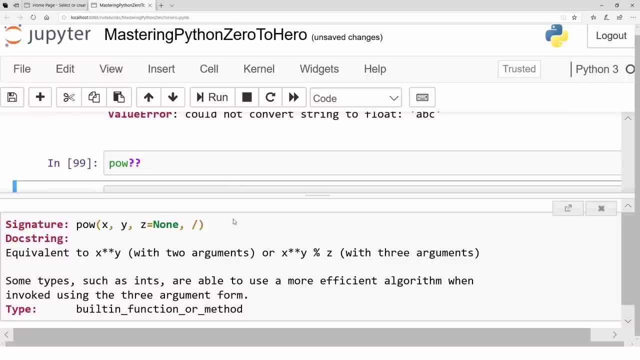 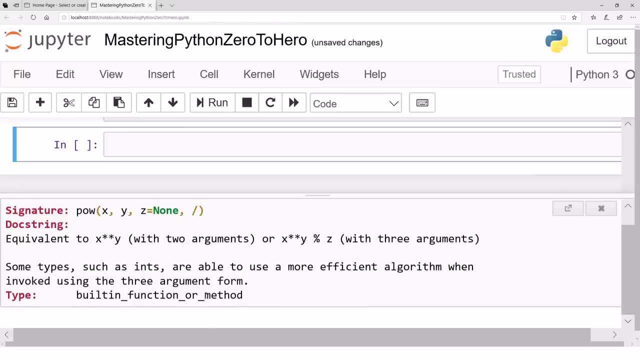 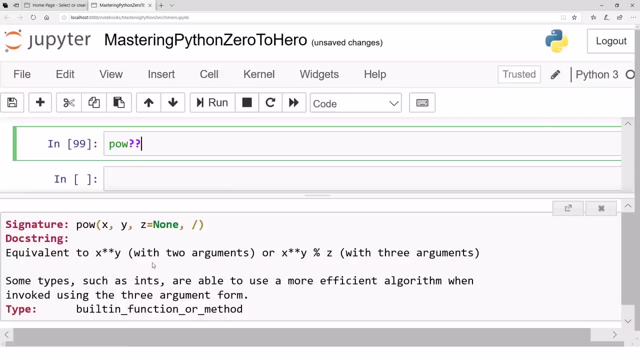 the double semicolon, a double question mark and more things should be open up in front of you. so yeah, in this particular case, the this power function does not have an implementation in python, so the single question mark and double question mark are the same. one more way is to use the help function- help pal, and you will get a lot of information about. 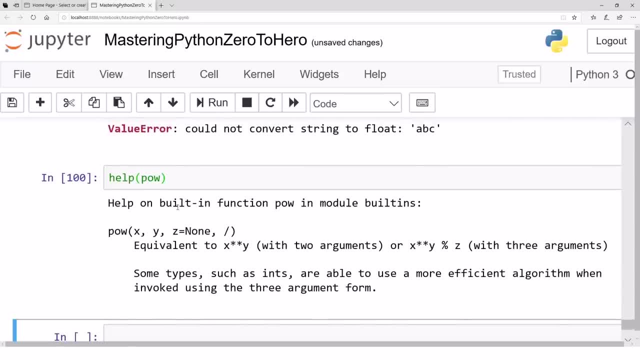 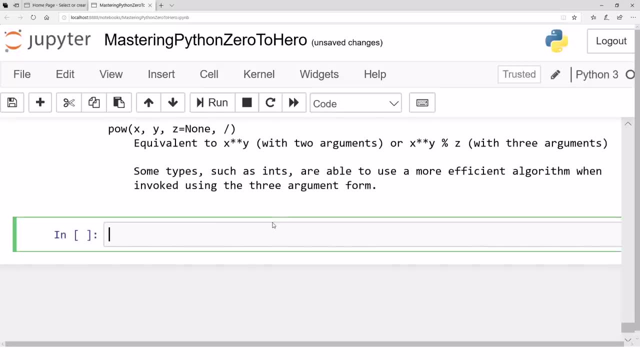 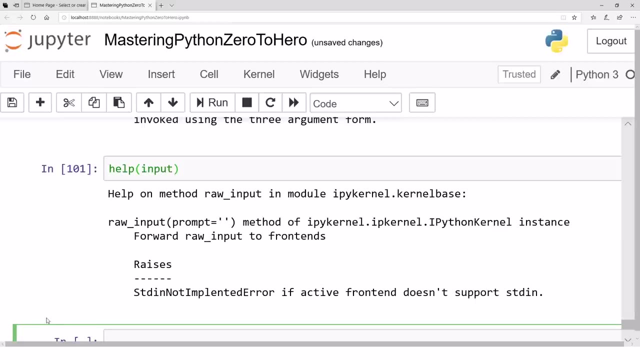 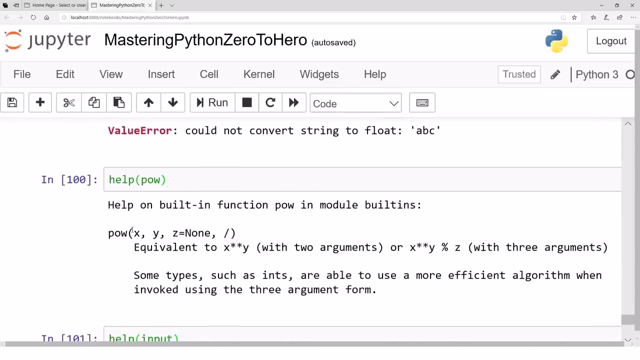 the power, how, for example, help on built-in function power and module built-in. so this is power, this is equivalent to this, some key types and stuff like so. or, for example, you want to know how can i use the input function, for example, so you can write help on input, and this is how this can be used. so sometimes it is okay if, if you know the 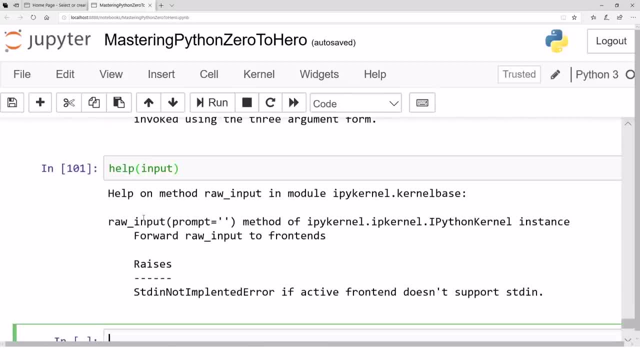 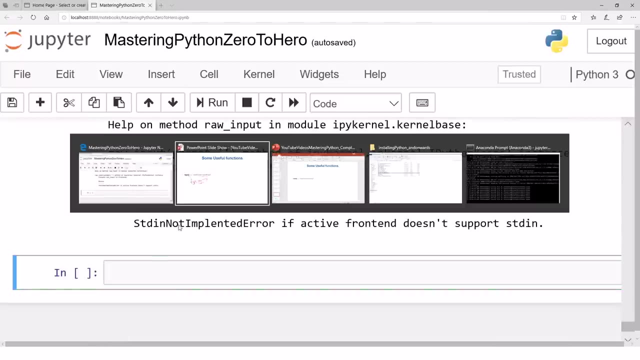 if you know the name of some function and you know how to use it, you can just open up the documentation right here in jupyter notebook by either using a help function, or you can use just a question mark in front of the name and so on. so, um, that's about the functions. um, in the next. 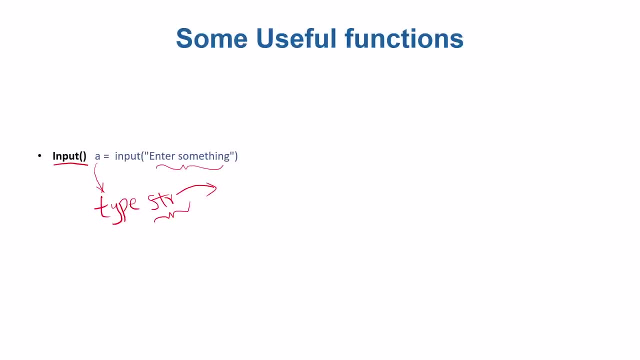 video we will be seeing the power of comparisons and the decision making, or sometimes called the control flow. so the real fun will begin, uh, from the next video, because we will be actually deciding which part of the code should run and which part should not run, based on 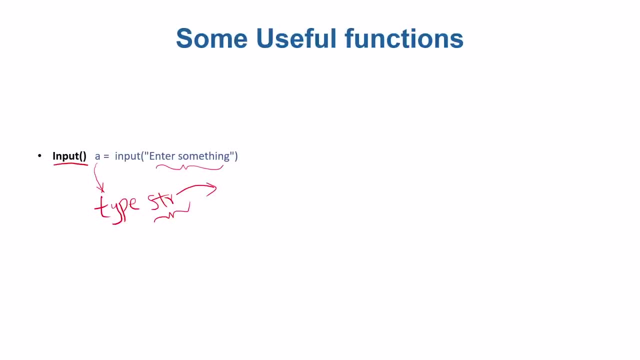 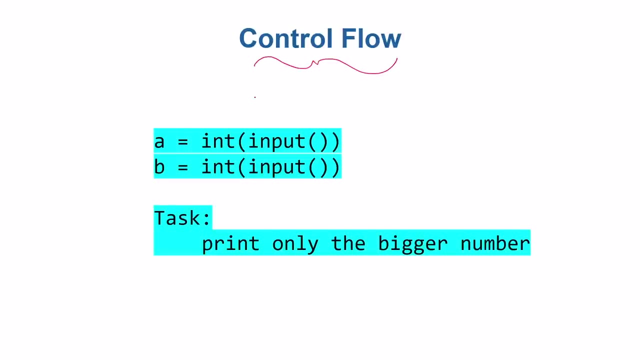 based on certain conditions, so hope to see you in the next video. okay, we are in control flow, the most interesting part of any programming language. well, assume that you have two numbers. you have taken two numbers from the user, a. you've taken that number from the user using input. i have not supplied the input message. 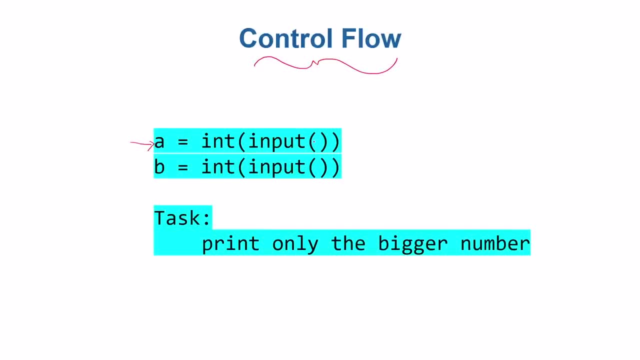 here the message is optional. it's a description. if you supply it to the user, it's not going to supply that, that's okay. if you don't supply even that, that's okay. so a is some number the user will supply when the code will run. b is some number the user will supply when the code will run. 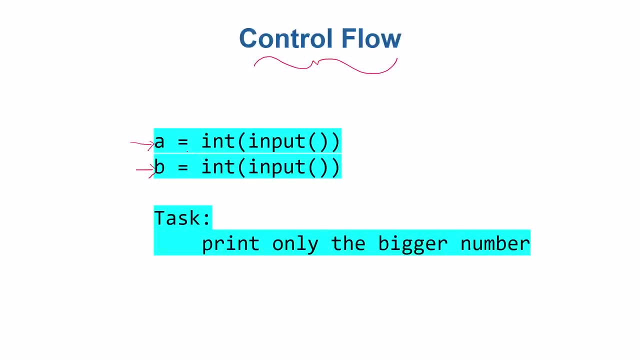 now, once you have a and b in front of you, obviously the user will supply that on the fly. you don't know what the value of a and b are, because when the program will run, only at that time the a will be populated and b will be populated. your task is: whatever the value of a, is that you 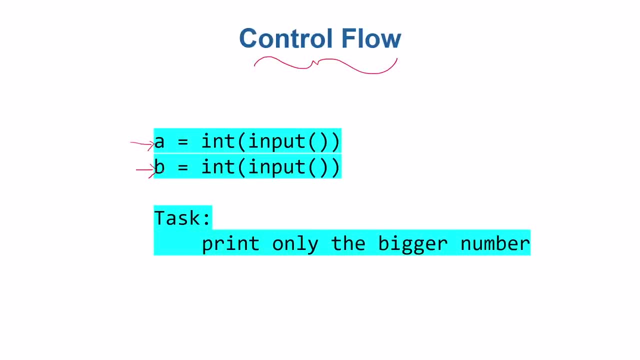 that you don't know. whatever the value of B is that you don't know, the user will supply that those values. your task is to print the value that is bigger than both. so, for example, if a is bigger than B, then print a if B is bigger than. 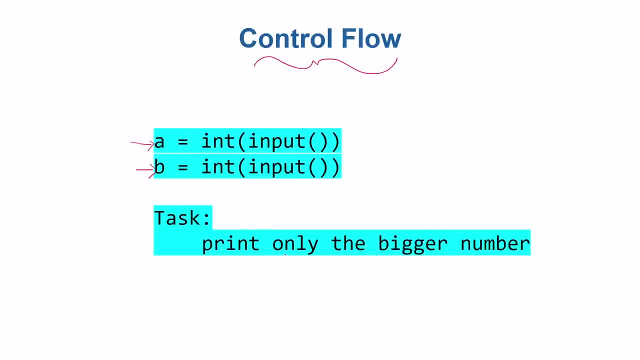 a, then print B. so whatever the bigger value is, print that value. let's say, that's your task. how can you do that? so the question is: how does Python allows us? does Python allow us to do that? for example, if a is bigger than we should print a, if B is bigger than we should print B. remember again and again we are: 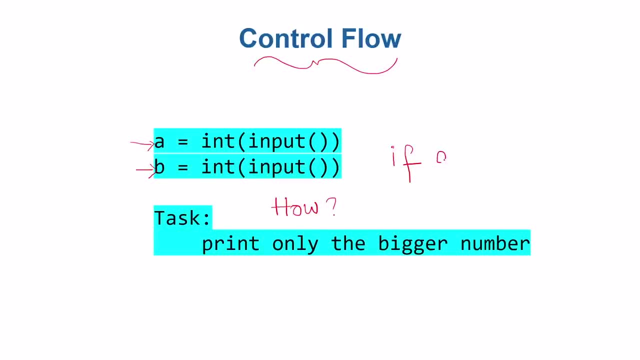 we are talking in terms of if a is bigger. if so, this is this is this is what. if a is larger than B, then this condition will be true. this is like the comparison. so this is true, but then we must have an if condition as well. you. 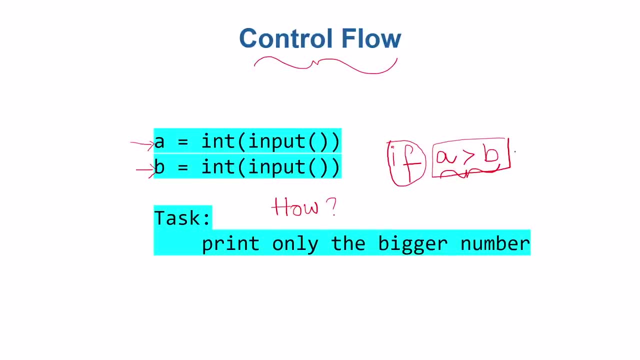 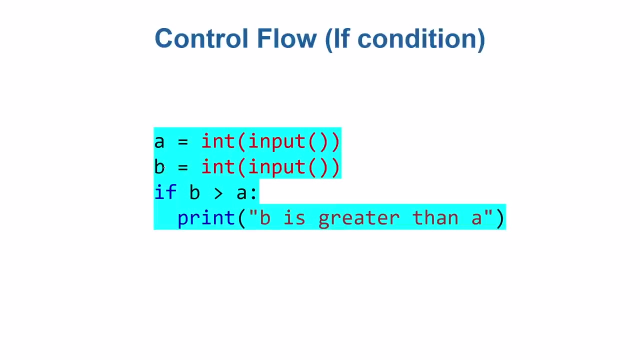 if a is bigger than do what? so if a is bigger than B, then do certain things, otherwise don't do that, those kind of things. so this if condition is really really powerful and is available in all programming languages. in here, for example, let's see if a is an input, B is an input, writing an if condition. that's. 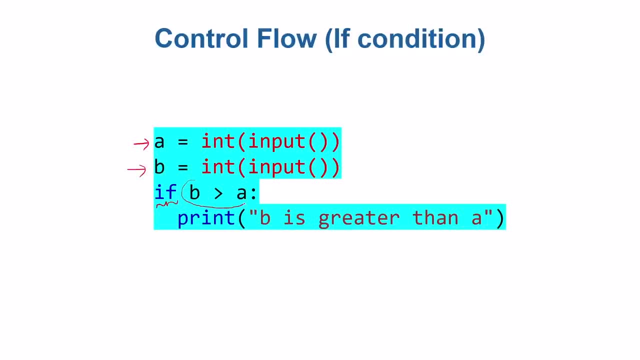 if is a keyword, that's a comparison that we have done earlier as well, and then the syntax required a colon in front of that. so if this condition is true, if this result, if this comparison results true, remember the comparisons: they return a boolean values. if this comparison, if this, whatever the result, 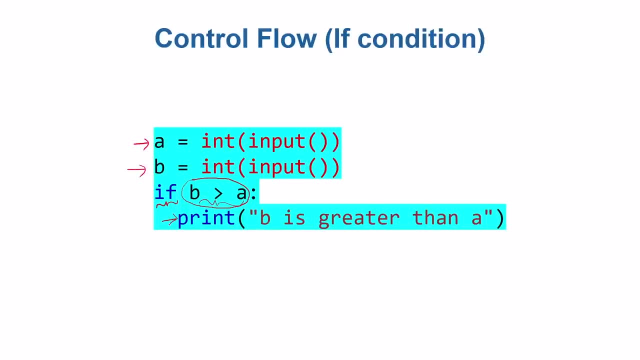 of this operation is: if that is true, then you go into this block and whatever the statement inside is to that, for example, print B is greater than a. now my question is: C: if this bob says progress, deep decrease again if a is greater than A, what statement inside is: do that, for example, print b is greater than a. now my question is: is that? 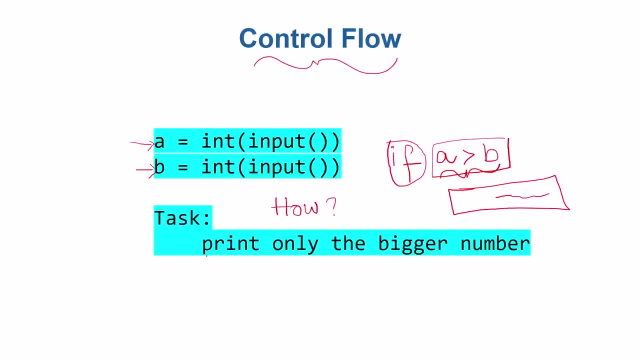 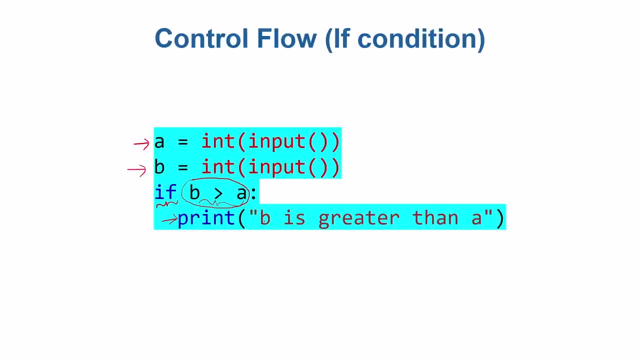 is that done? are we done with the task? the task was to print the bigger number. if b is greater than a, then b will be printed, then or, or we might have printed. for example, we might have printed rather than writing this. we might have, might have printed. let's say, just print b because b is bigger. 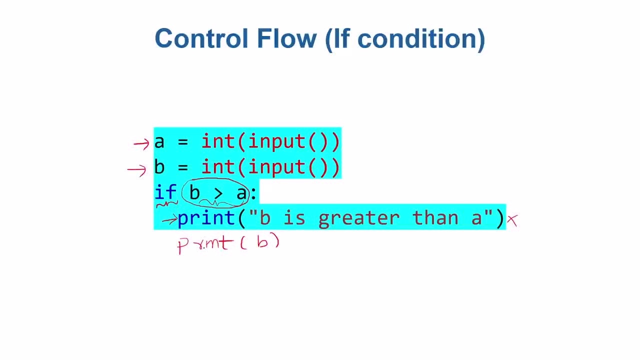 if b is not bigger than a, what will what we will do then? so yeah, if b is bigger than a, then b will be printed. yes, because then you will be inside here. if b is not bigger than a, if this condition is false- we will do what then? so that's a question. so right now i'm just coding this: 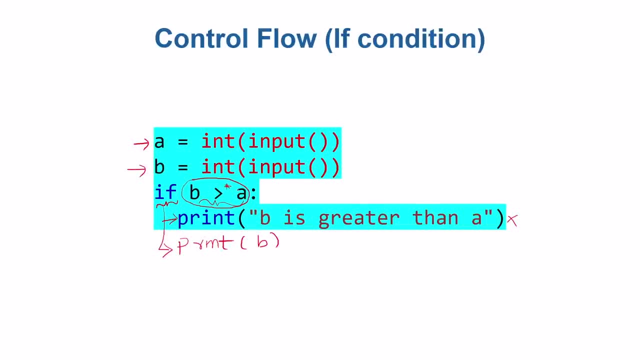 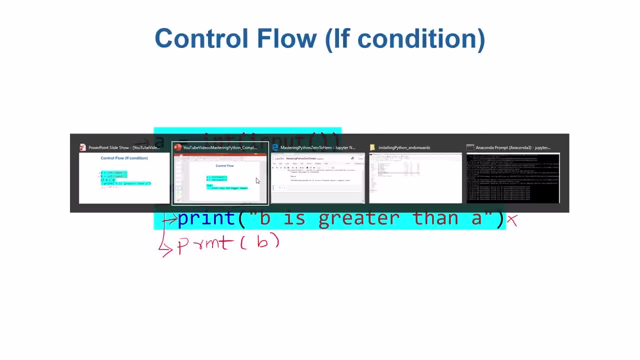 in jupyter notebook and then we will see how can we deal with that. if b is not bigger than a, then we will do what then? so that's a question. so right now i'm just not bigger than a kind of condition, so let's first see the blessings of if condition in jupyter. 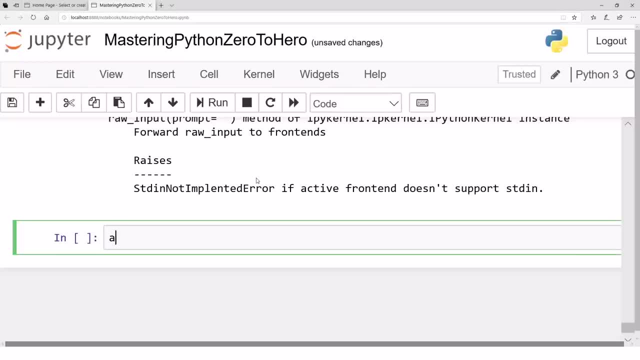 notebook. yeah, so let's say a is an integer, let's say you're expecting an integer input input. let's say: and then you write. if let's say b is again an integer input, maybe, and let's say: if a is greater than b, then print a. that's it, that's your program. remember this indentation? i have not. 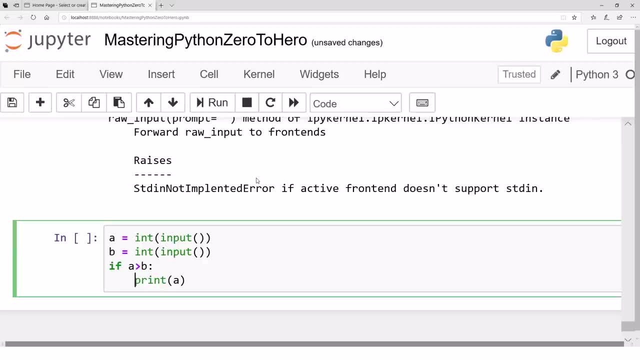 written this print here. this is the indentation that defines the block of a. let's say: if i want to print a, then i want to print. let's say: i am still inside if, condition, condition, and so whatever that starts from this, whatever that starts from, whatever that starts from: 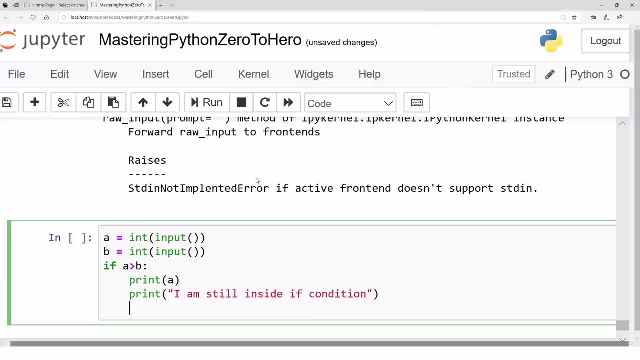 this alignment: if i write something here, let's say, x is equal to five, all that block, all that block is called the body of the if condition if it starts from this alignment. if, however, i type a statement, but i type that statement in that kind of alignment, the alignment like this: 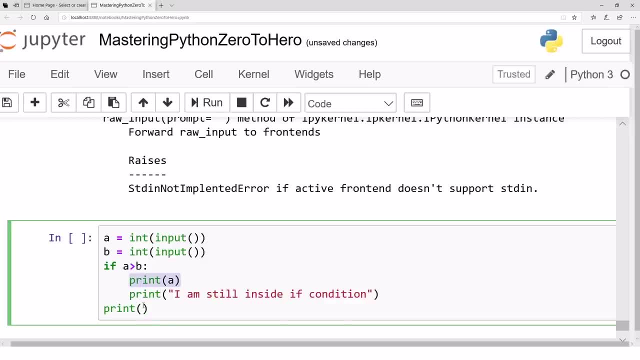 this is no longer inside the if condition. so, for example, here i type: i am outside the if condition, so the purpose of writing these multiple lines is just. if condition does not require to contain only one line of code, it can contain a whole block of code, multiple lines of code. 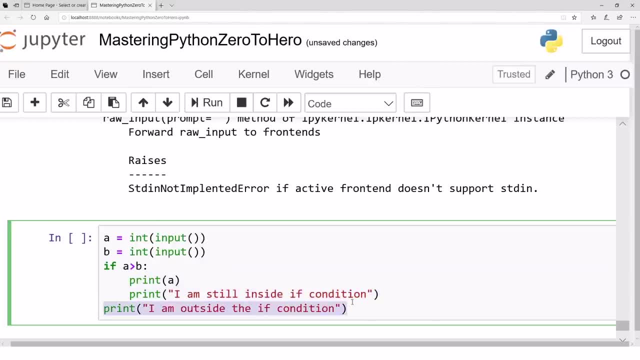 so this is no longer inside the if condition. so now we will take input a, input b, whatever the numbers will be. if the value in a will be larger than b, then this will be printed and this will be printed. once these two are printed, then this has to be printed regardless of the values of a and b. 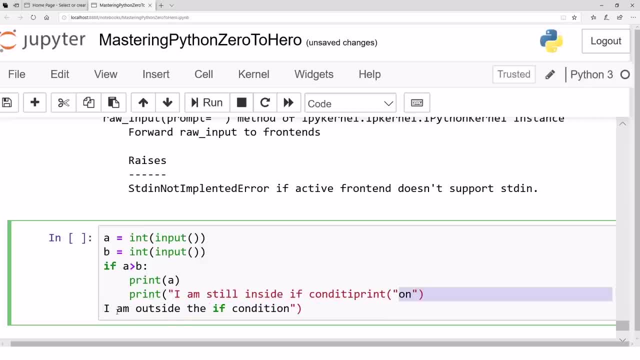 because this does not this last print statement. it does not depend upon. this does not depend upon the values of a and b it has. the if condition has no impact on that. that is just a sequence of statements. the if condition, the statement inside the if, are just these two. for example, if a is not bigger than b, then neither this will. 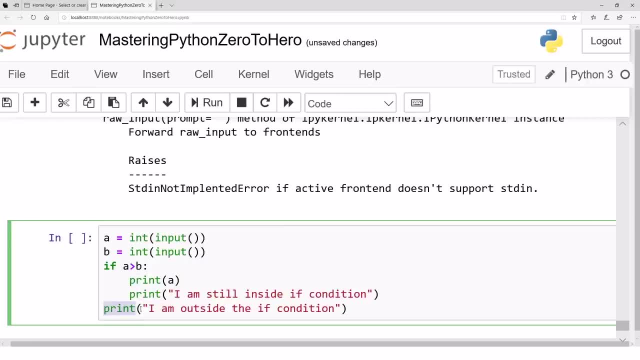 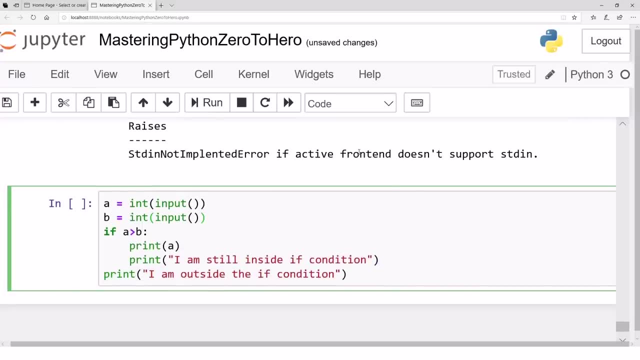 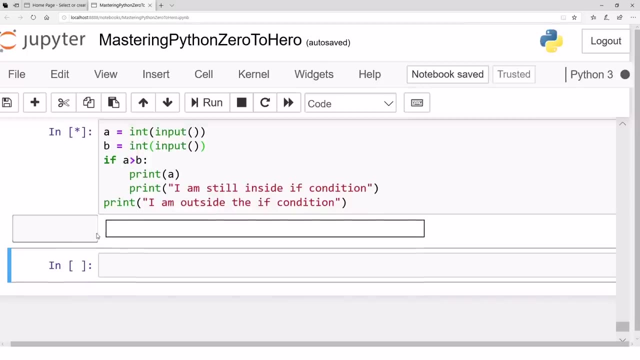 execute, nor this will execute, but this will still execute, because this is. this has nothing to do with if condition. so let's run this code and see how it works. so let's see the value of a, see the power of descriptions. if we could have written a description, then the description could. 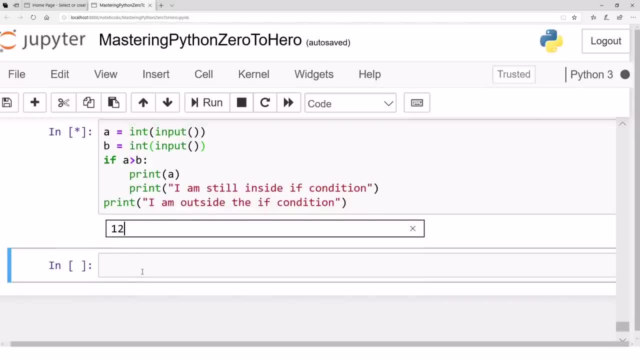 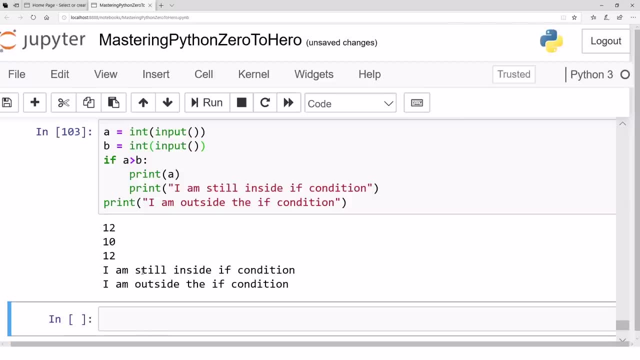 have been, could have appeared here. but let's say: this is the value of a, let's say twelve. the value of b, let's say, let's say 10 in this particular case, because the value of b is 10, the value of a is 12. 12 is bigger than b. if this condition is true, this statement becomes true. 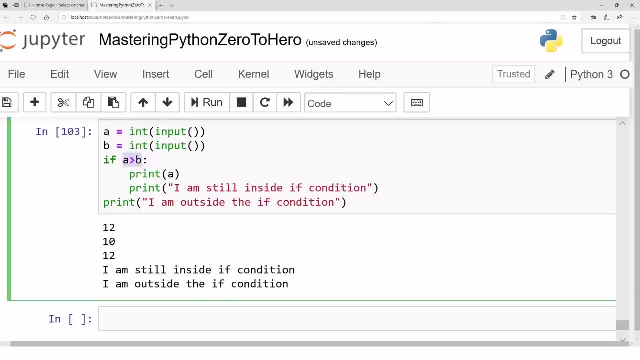 whenever this condition becomes true, you're inside the prints. you are inside the if condition now. this print executes and you, you get 12.. print executes and you get: I am still inside the if condition and this has to execute, no matter what the values of A and B are. So now let me rerun this and give. 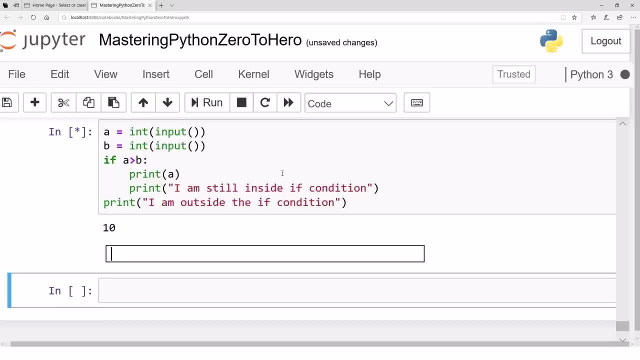 other values of A and B. Let's say the value of A is 10 and the value of B is, let's say, 45. Now this condition becomes false, because 10 is greater than 45. This is not true. this is false. So whenever this condition is, 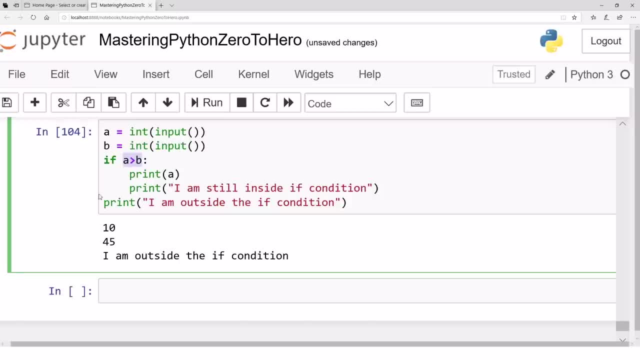 false. you never land inside the if condition and you go out from the if condition. So these are the statements that are inside the if condition. They cannot execute because you never visit them. They can only be executed if the if condition becomes true. So then, once you're out the if condition, that's. 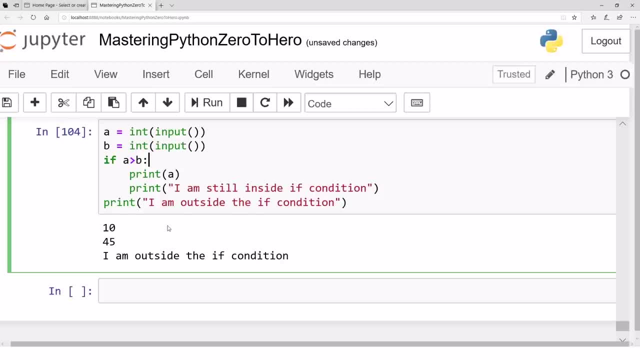 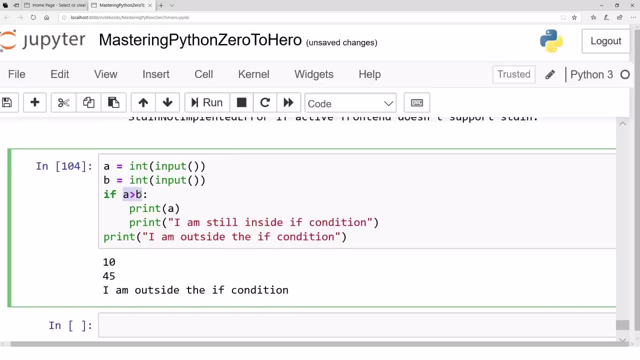 the statement that is going to be executed anyways. So yeah, so that's the flavor of if condition on the CN making. and this is the comparison operator that returns a boolean value. You may have different kind of comparisons here, or combination of comparisons here. no, no problem, depending upon your logic. But 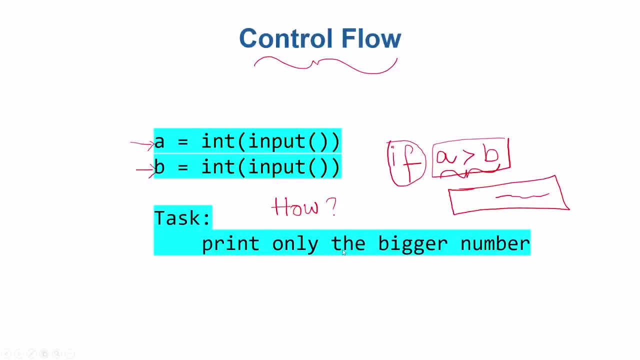 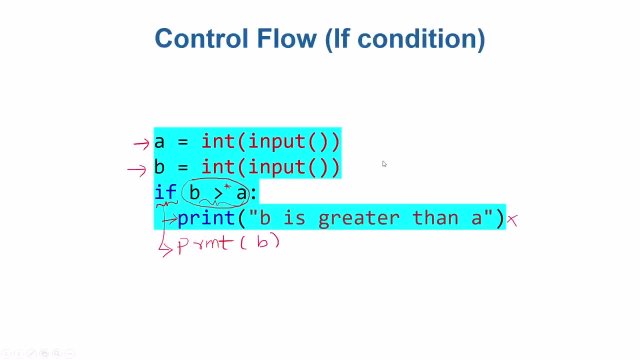 the question is: are we done? We are going to print only the bigger number We have. we have printed the one, that is, if A is bigger, we have printed that. What if? if B is bigger? We have not solved the task yet. This is the task we have not solved. 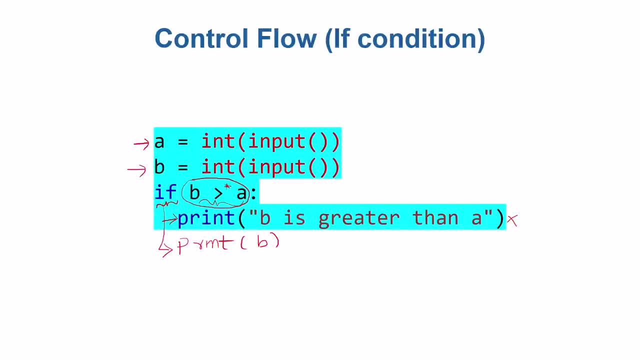 the task yet. So how to do it? Okay? so, yeah, it looks like complicated- How to print only that number that is bigger. So if B is bigger than A, then we will print B. Maybe maybe we should make, maybe we should apply another if condition: If B is bigger than A, then print B, If A is. 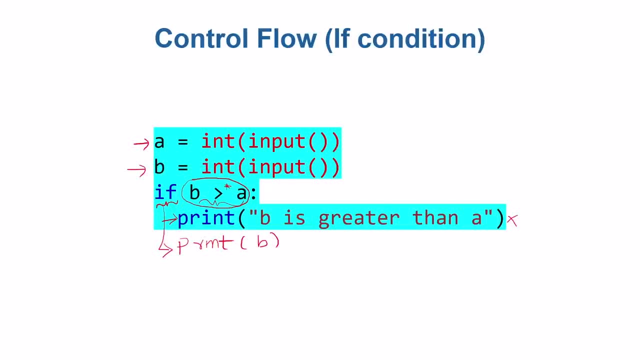 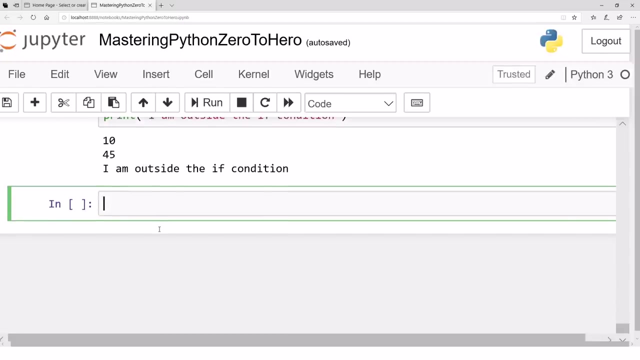 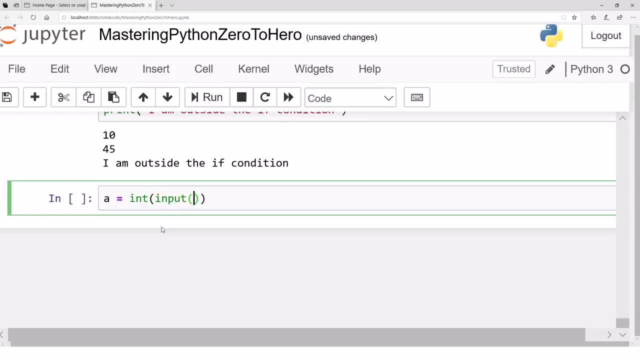 bigger than B, then print A Maybe. yeah, why not So? so, for example, let's go to Jupyter Notebook and and write the following: Let me, let me write a whole new program here: A equals int input. Okay, let's do not have a message- Int input. and then, if 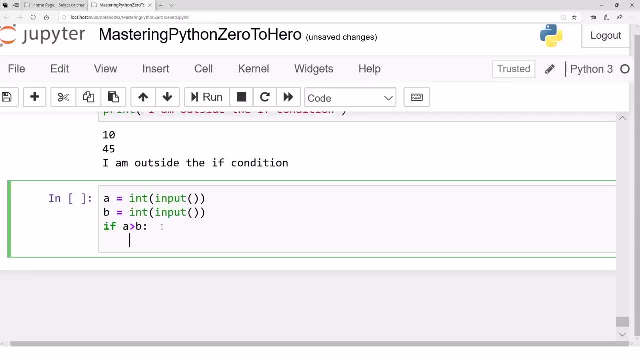 A is bigger than B, then print A, Okay. however, if B is bigger than A, then print B. I guess we are done. If this condition becomes true, then we are here And we know. if this condition becomes true, then this condition cannot become true, Because it can. 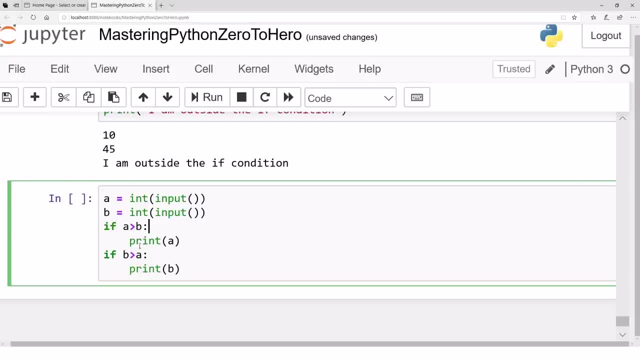 not happen that A is bigger than B as well as B is bigger than A. This cannot happen. So whatever the bigger number will be, that will be executed Further. you can see. I have this if condition and this if condition. they are aligned in a. 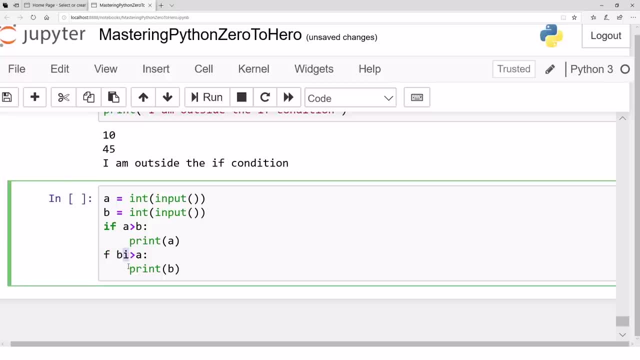 way that this if condition is not this, the second if condition is not inside the body of the first if condition. We will see such a cases, such cases when this is required, but right now I guess we are done. If A is bigger than B, then 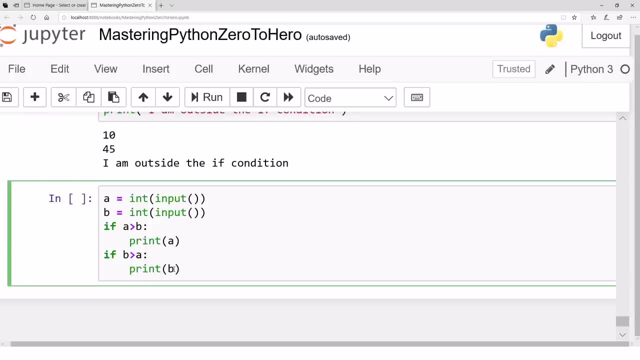 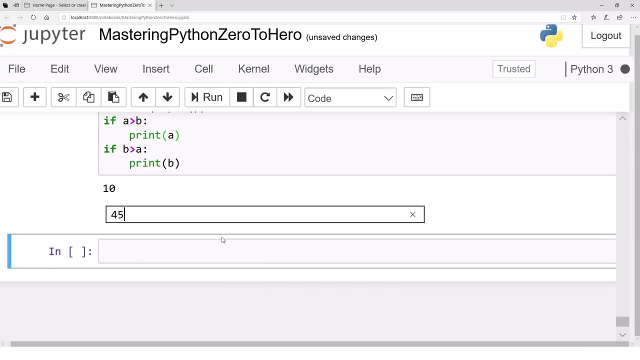 print A. If B is bigger than A, then print B, And only one of these. if conditions will become true, because A is bigger than B, B is bigger than A. These two statements cannot be true at the same time. So let's see. So A is 10, B is 45. So the answer is 45. Wow. 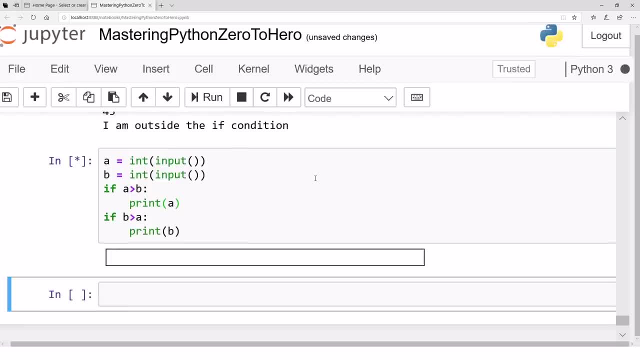 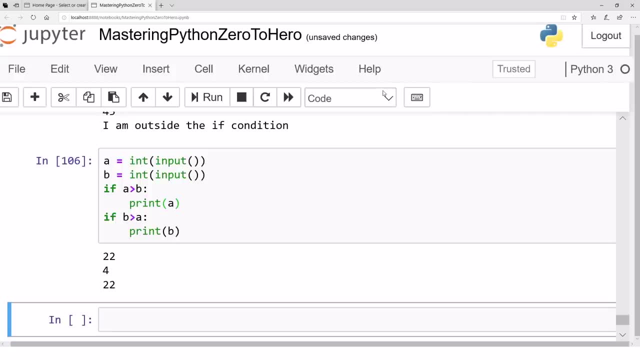 because 45 is bigger. So let's run it again. So A is, let's say, 22, B is, let's say, 4, and the result is 24.. Because 22 is bigger. I guess we are done with the task. We have used this if. 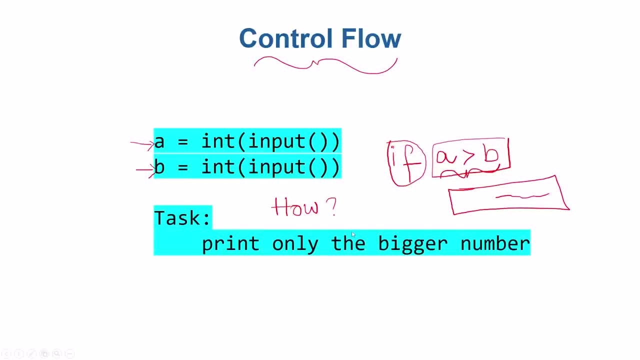 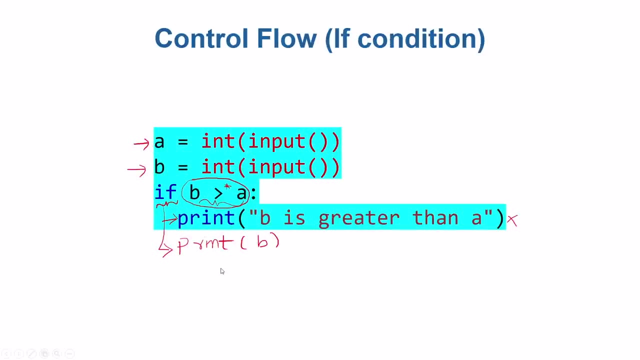 condition twice to achieve the task: to print the number that is bigger and both the numbers we. we took both the numbers from the keyboard. Yeah, I end this video here and in the next video I will tell you more features of this if condition, particularly the else statement, What we have done recently with another. 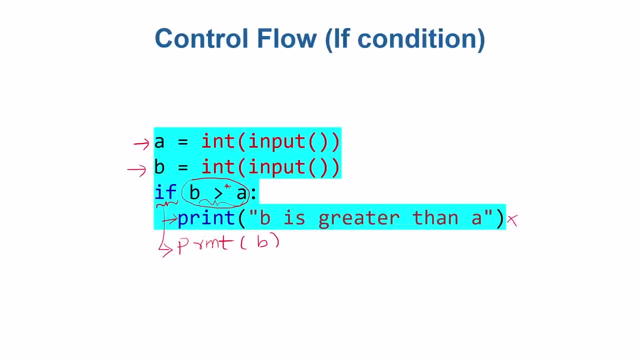 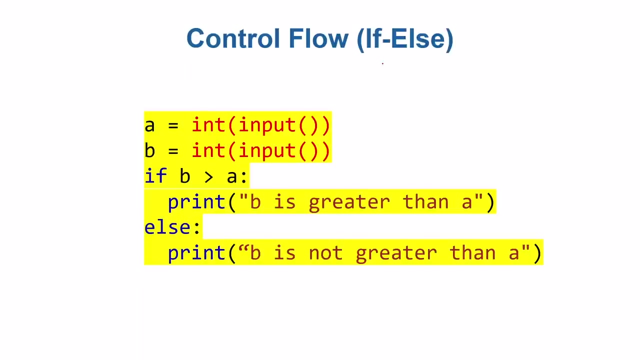 if Could could be achieved through an else statement that is more powerful, more readable. So in the next video I will talk about else statement, which is a part of if. So hope to see you in the next video. OK, In the last video we saw if condition and we actually had an example in which we 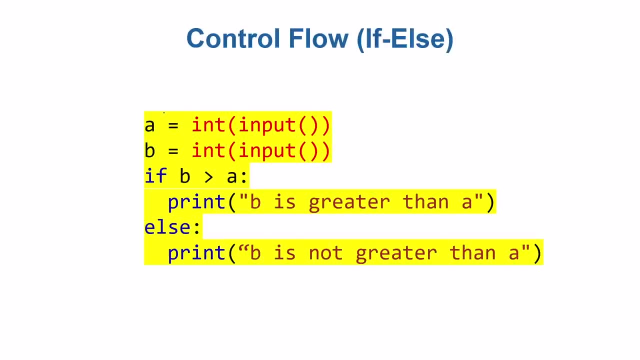 wanted to know what. we wanted to just print the greater number. So we input a number A, We input a number B And if B is greater than A, we printed B is greater than A, Then we applied another if condition to check if A is greater than B, then print A, The else clause or the. 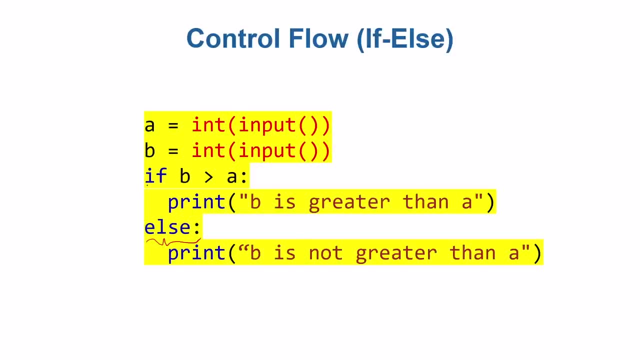 else part of if is, as, as the name suggests, if this condition is true, So if this condition is true, this particular condition is true, Then go there. If this is not true, which means else: if this is true, Then go there, Else go there. So if this is true, then you land here. If this is false, then you land. 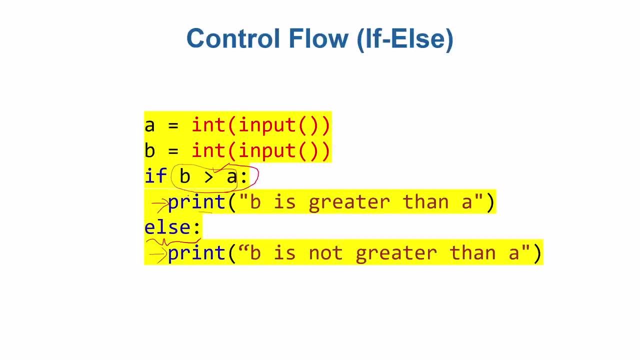 in an else part for sure. And this else is I mean if B is greater than A. if this condition is true, then you print this thing. Otherwise it might be greater than B, or it might be equal to be. either way, you land in a part. 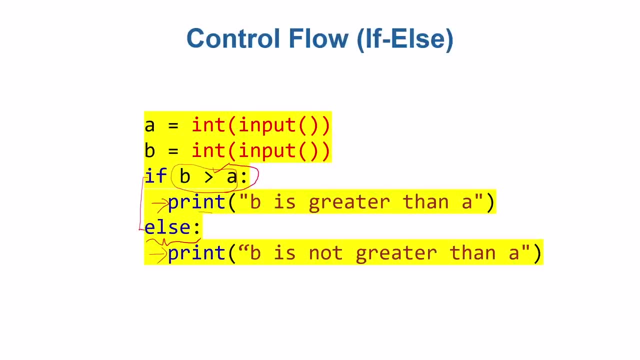 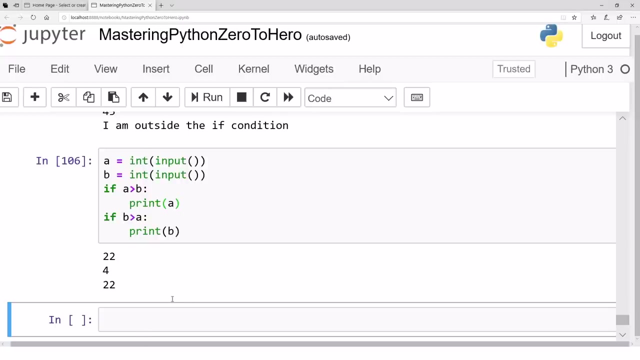 So this and else they both have this alignment. but then the block of else started from this particular alignment. maybe you have more statements here. the alignment of this if block started from here and you may have more statements here. so let's go to your jupiter notebook and see the else running. so let's say a equals int. 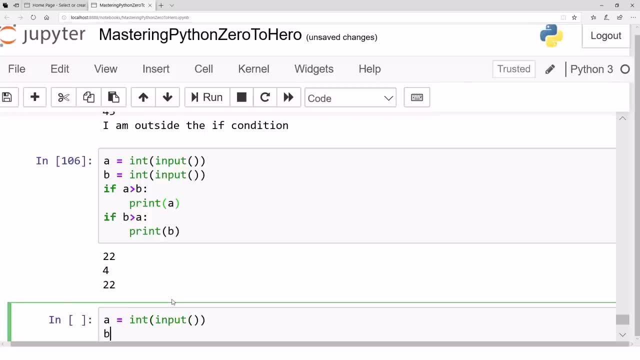 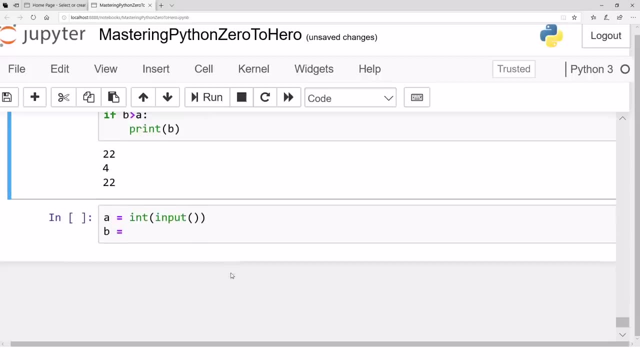 input and B is, B is int, and we say, okay, if a is is greater than b, then print a, else else print, else print b. i'll sprint b now. b will be printed even if it is equal to a or if it is greater than a, either way. 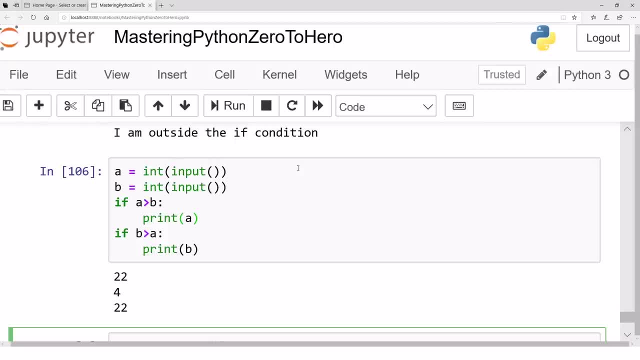 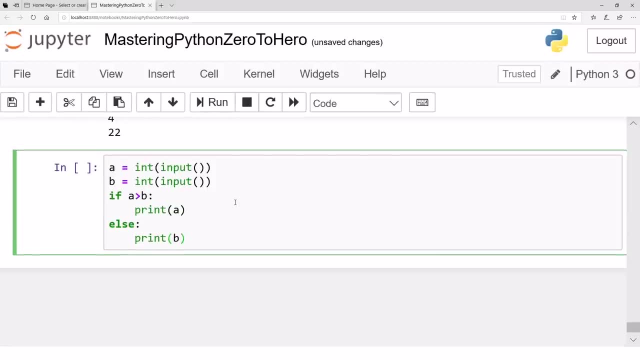 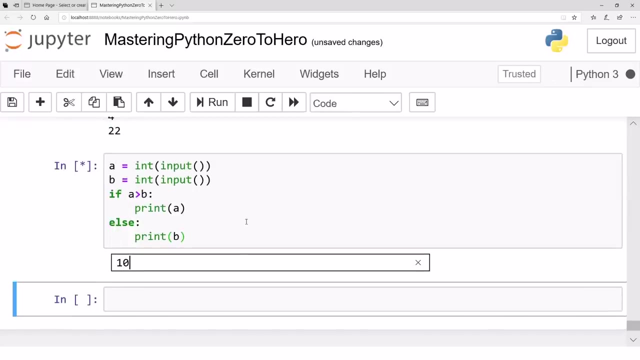 b will be printed. so let's just see, um, let's just run this and see what happens. so shift, enter, so input a number. so a is, let's say, uh, 10 and b is, let's say, 12.. so what do you think? when i will press enter, what will be printed? 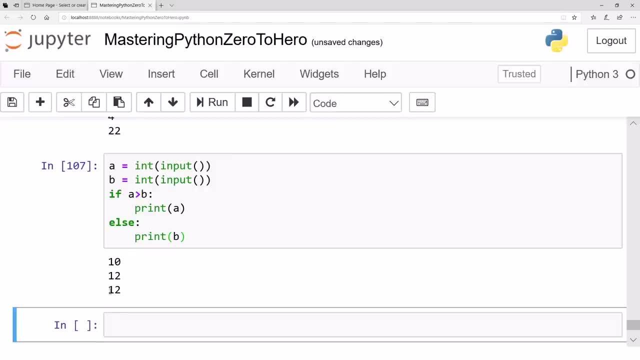 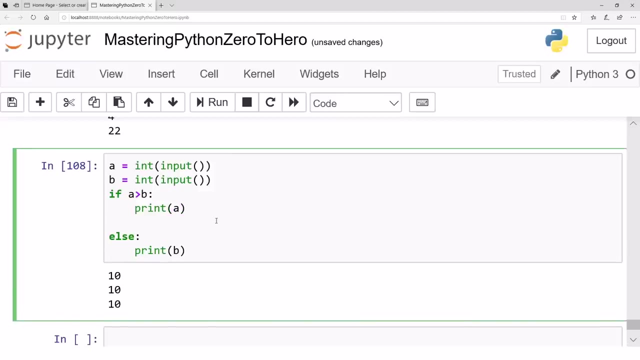 b or a b. yeah, b is printed. that's what b is printed. now, if i run this again and a is 10 and b is 10, still the 10 will be printed. so let's modify, let's, let's just say dot print if part. so that means we landed in if part. otherwise we landed in else part. 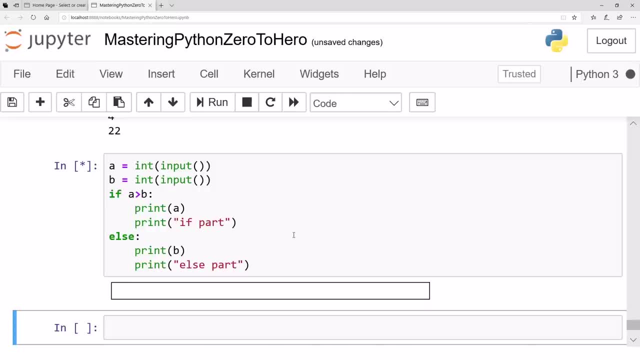 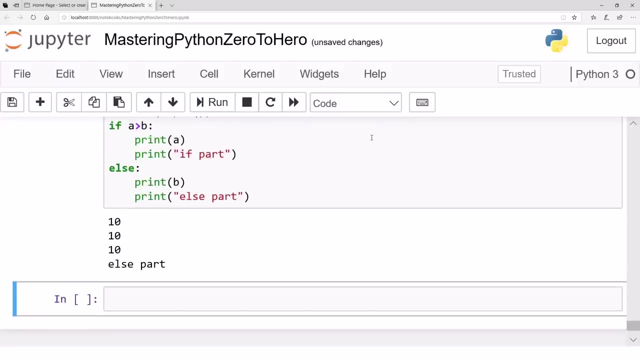 so just to be more elaborative, let's say so 10 and 10, and we landed in else part. and the reason is: if a is greater than b, so 10 is greater than b, 10 is greater than 10. false. so you go to else and 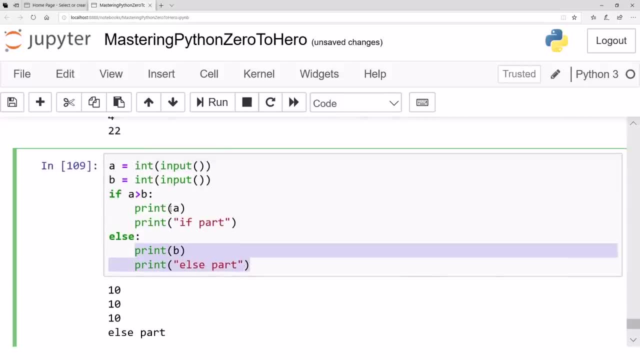 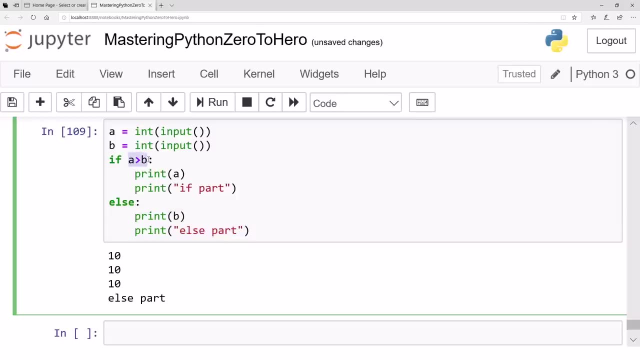 the else block, the whole block just executed. so that's what else is. it's, uh, really very nice to have an else there, whatever this, whatever the, if this is false, whatever that condition is, if that is false, then you land in else. so, um yeah, that's else part, simply. 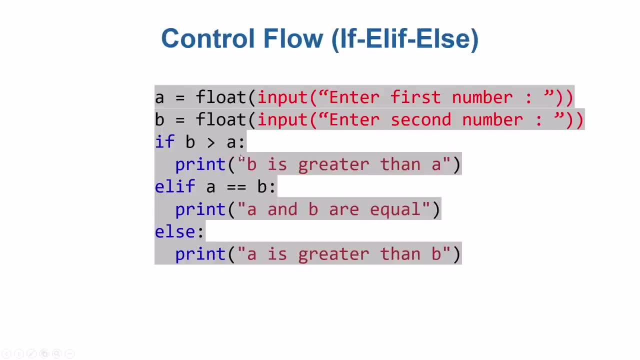 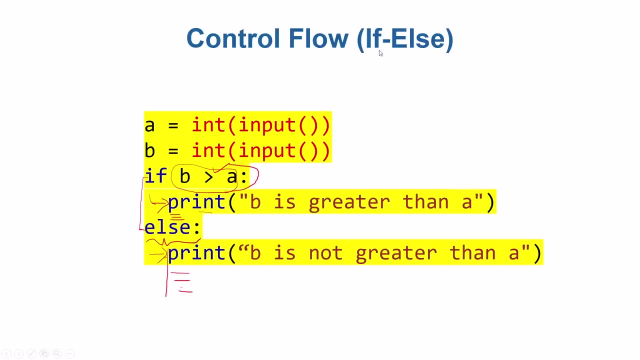 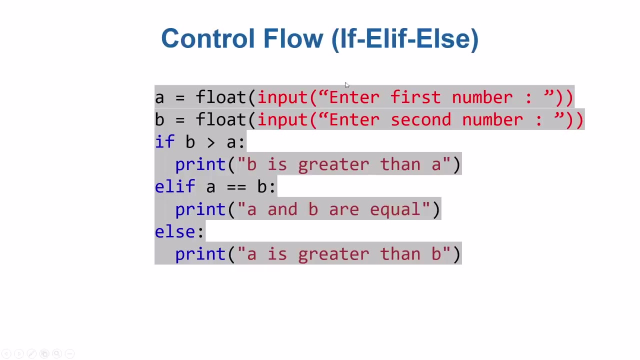 now, um, so first thing we're going to do is, uh, i'm going to withdraw that object and drop the object. now i'm going to say that a sub is a, a sub, j, j, and we'll do just one more reading. i'm just going toMSWRT in order to know if there's buy. 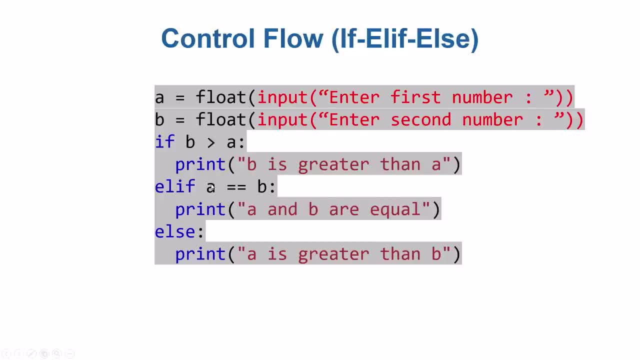 so if there's are for and sell, i'm going to lower it down. so the random upper color in a corner, i'm going to lower them down by one second. so this is the queued box. like i said, if there is a false, then i am printing a current position. it is a tag of x zero, so i am printing a current position. 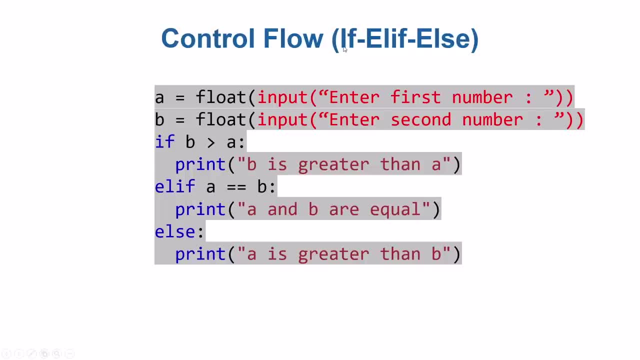 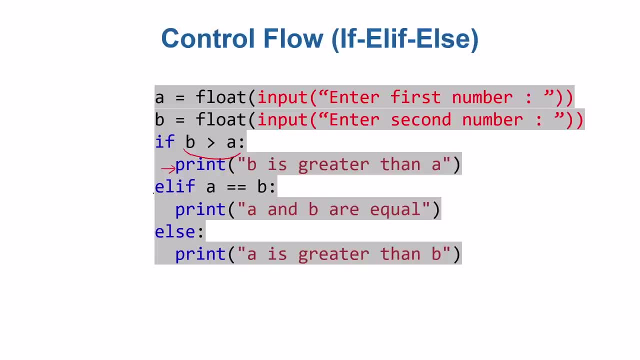 then you land in this part: else, if this l, if is just short form of else, else means b is not greater than a, else you can have another check, else, if a is equal to b, then do what? l? l if we can have one more check, we can have one more check, we can have several checks, and then 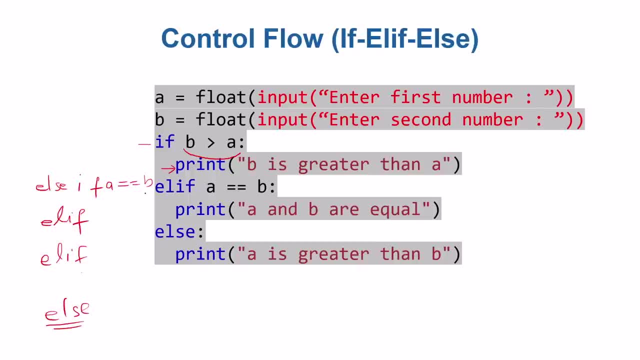 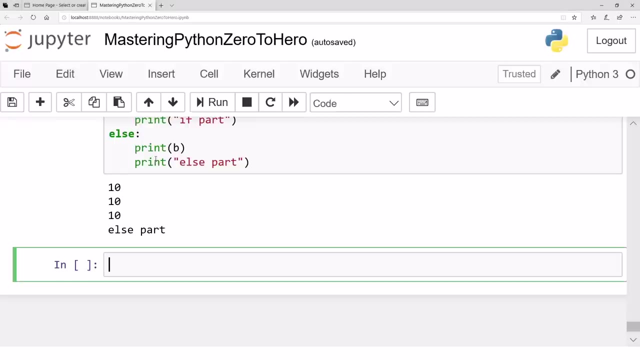 else else will only execute if all if conditions, or else if parts on top their conditions they are false and only then else will be executed. so let's see the else. if running on jupyter notebook, okay, so let's say a is int. so rather than taking inputs, let's say a is one, b is, let's say, five. 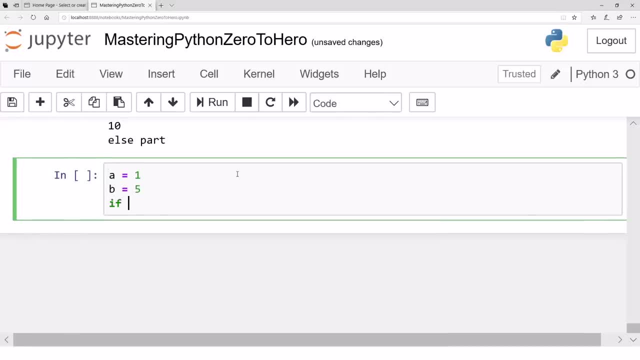 let's say we have taken these inputs: a is one, b is five. if a is, if a is equal to b, then do what rent? and when no, do a fleet function? you have a case if it's if a, if, if a is a less than or less than. 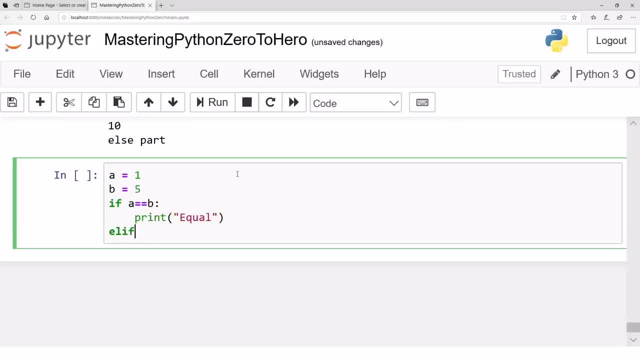 be almost no. for example, b, then is none, and so now the next problem. this is being encountered also. this one is absolutely forthcoming in our paths, you see, just working with a prefix, for we will have to write them. we have to put this in a chil porque. 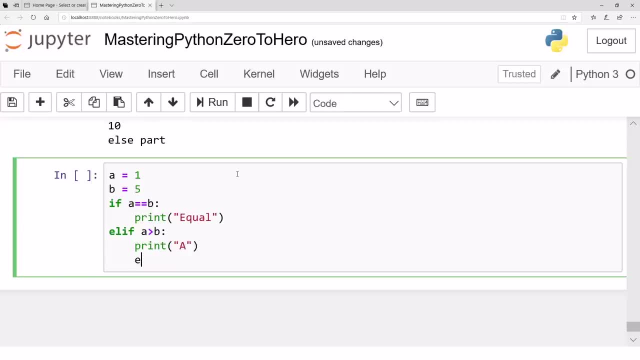 here. first thing we have to do is set. this actually is not for someone tohoo. when this function is working with a parent, we want to use a pegar again and else let's say, you print b, okay, so that's it, and this statement print is not in if condition. 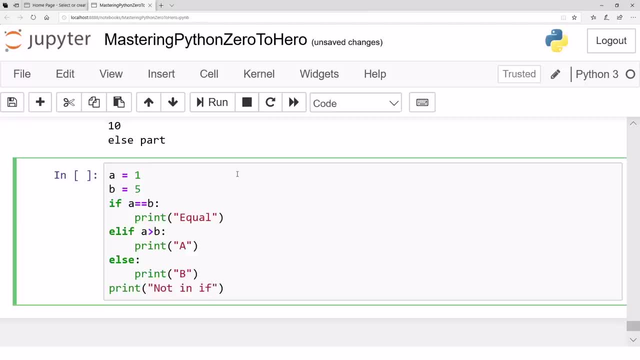 not, not in. if this is outside complete. this is complete if condition with all its else and else if parts, and this is no longer inside. so let's run this. what do you think? what will be the result? if a is 1, b is 5, then else part is going to be run, because a is not equal to b. a is equal to b, that's. 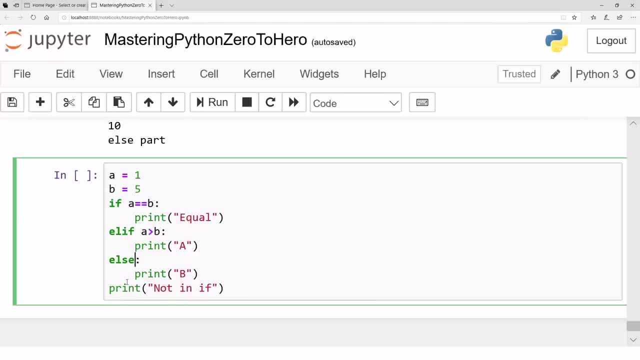 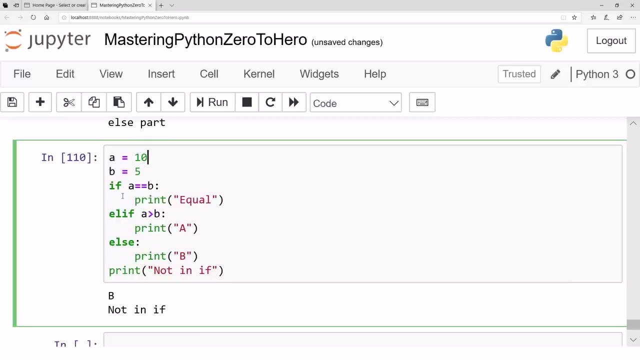 false. a is larger than b. that is also false. so you will land in else part and b will be printed, and then a statement will be printed which is not an f. so yeah, so b is printed and not an f. if b is 10, then what will happen? a equals to b. that is false, so you will not land here. else, if a is larger than 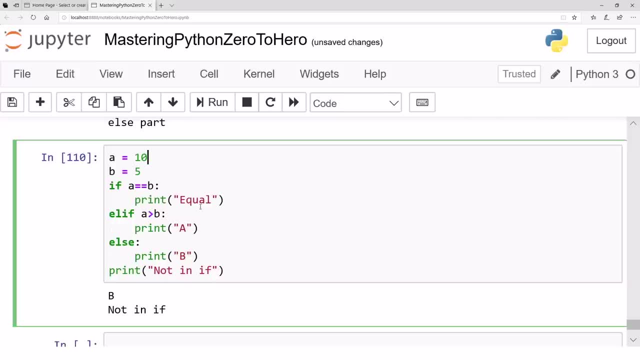 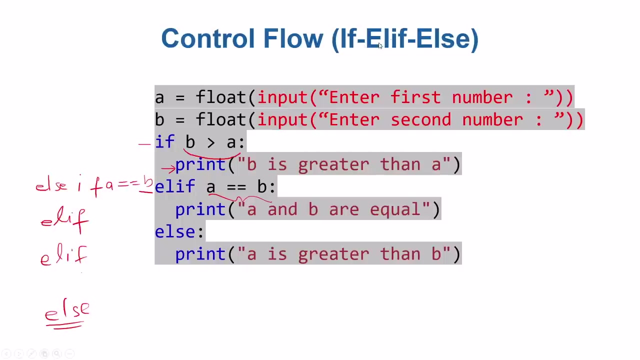 b. true, you will land here, because you land here, else will not execute. so a will be printed and then not enough. if a is 10 and b is also 10, let's say, then you have equal. yeah, so that's else, if, okay, so, um, that's about if else, if, if else, if, or short form is lf, l structure. in the next video we 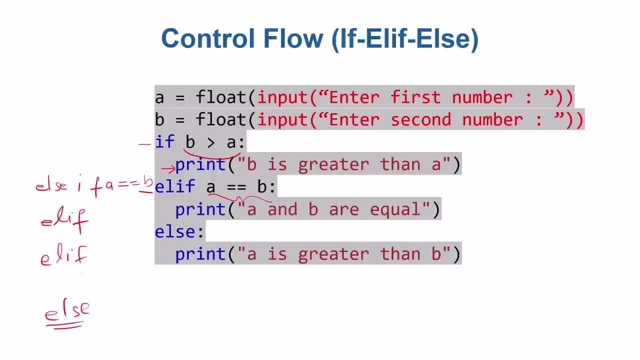 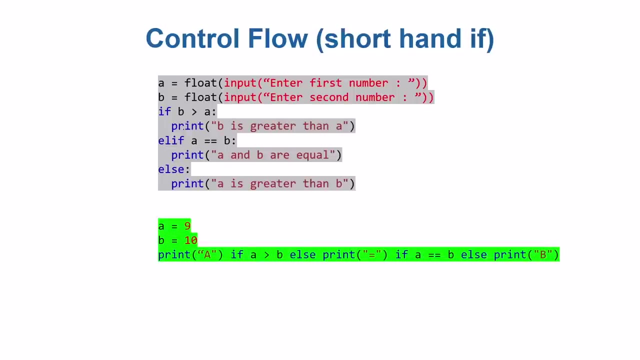 will be talking more about this- if else, if l- structure in a bit more detail, and we will also be giving you a short form of this, this kind of else, if else, if else, if else, of structure. so hope to see you in the next video. okay, one way of writing this: if else, if else, kind of structure. 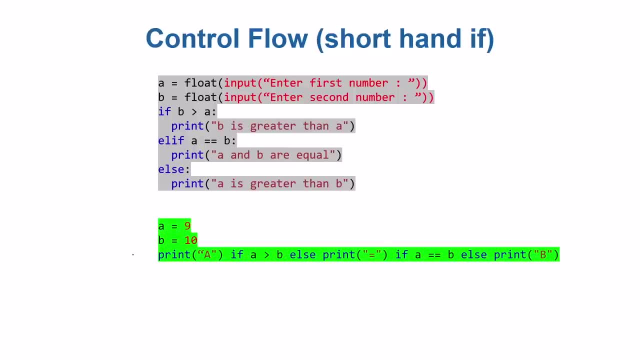 there is a short form as well: uh, which is written down here in a, in this uh green color, for example. this is a kind of a same code that we saw in the last video, but that's the short form. let's say a equals 9 and b equals 10, then print a if a is larger than b. 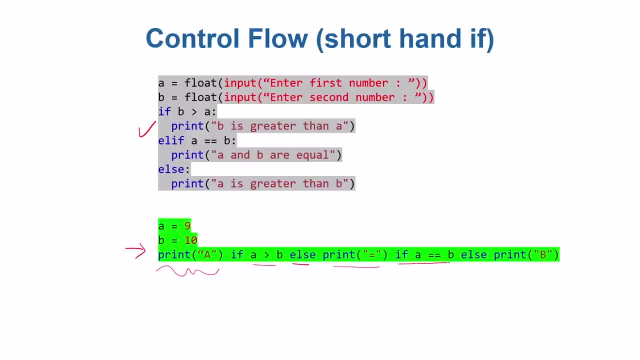 else print this particular thing. if a is equal to b, l sprint that. this is exactly the same kind of structure. for example, print a if a is larger than b. so you just read that if a is larger than b, then print a. else, if a is equal to b, then print equal, else print that. so that is kind of a short form. 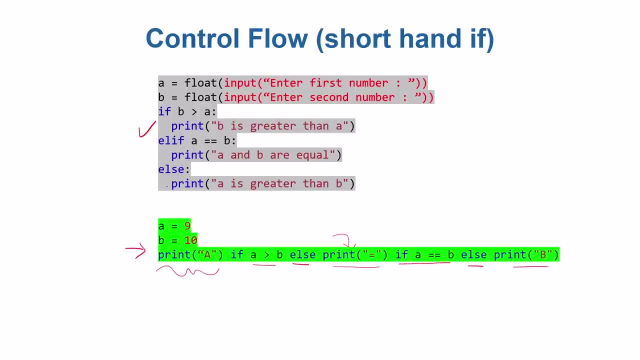 of writing this if lf else kind of structure, but i will, i will recommend to, to to use, i mean, the structure in this particular horizontal form rather than writing that in this particular way, because this kind of structure, that horizontal kind of structure, is much more readable, much more. 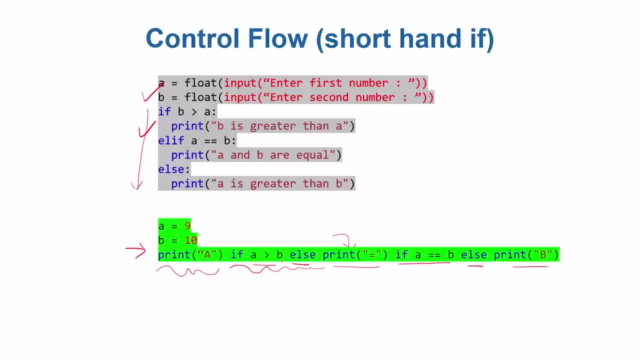 manageable and this might be, this structure might be confusing sometime for for some kind of readers, or yeah, and also, if this structure goes on and on and on which we will see, uh in a, in an example today, uh, writing that writing very deep and lengthy structures in short form is: 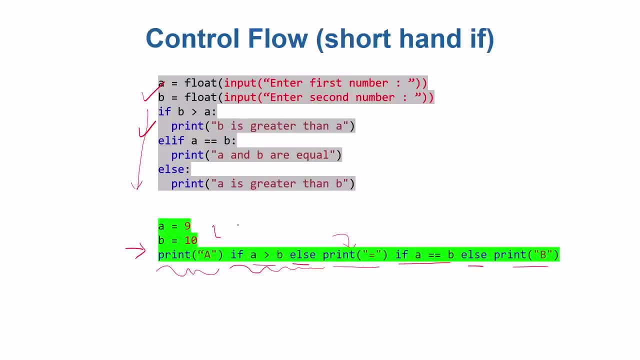 not going to be a very good example of how to write this kind of structure in a short form, very visible. so, although, but but this feature is there, if, if you like to write, if else, if else kind of structure in this way, this is available in python, okay, uh, let's, let's get a good grip on this. 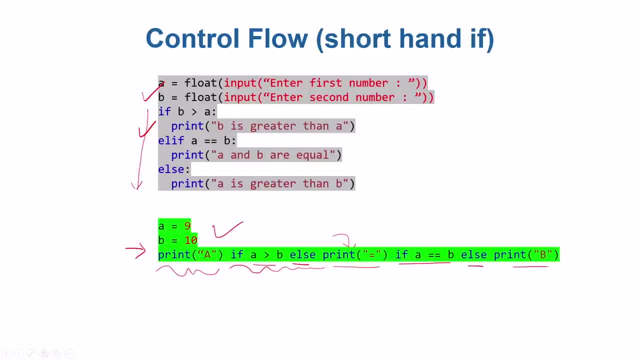 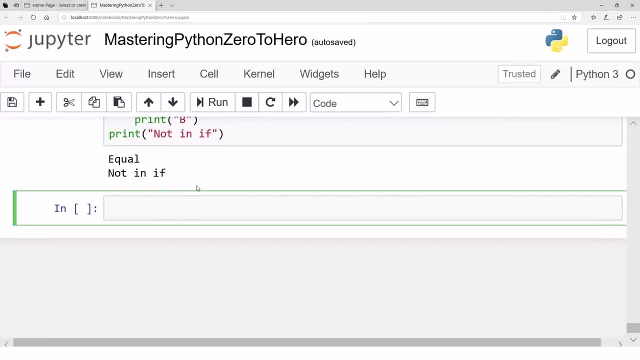 if else, if l structure on jupiter notebook, let's move on to jupiter notebook to see an example. just an example. so let's say the example is: user will input a number. let's say int input. let's say and enter marks. let's say enter marks for a particular subject. 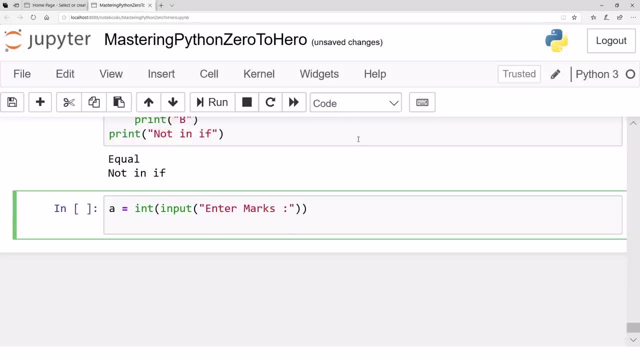 let's say, user will enter some, some marks and our goal is: if the marks are larger than 85, then we will print a grade, if the marks are larger than larger than 80, but smaller than smaller. so if the marks are larger or equal to 85, then we will print a grade. 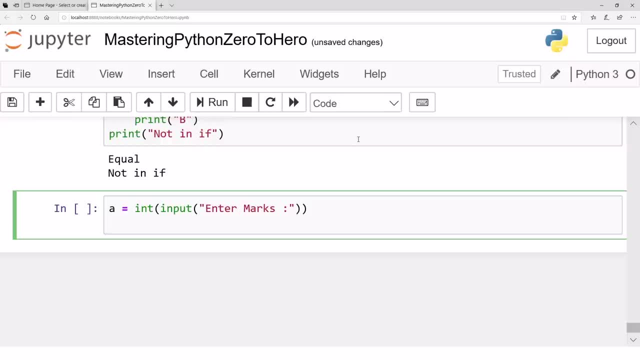 else, if marks are larger or equal to 80 but smaller than 85, then we will print a minus grade. and and if else, if if marks are larger than larger or equal to 75 but smaller than 80, we will paint. we will print, for example, b grade, for example b grade, and and so on. let's print this whole nested structure that 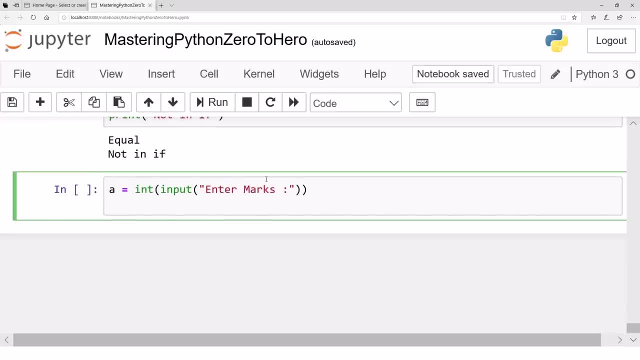 let's let's make this else, if else, if else, if kind of structure a little lengthy, let's let's get comfortable with it. so if a is larger than or equal to 85, to enhance readability it is good to include a spaces, a space after the variable and space. 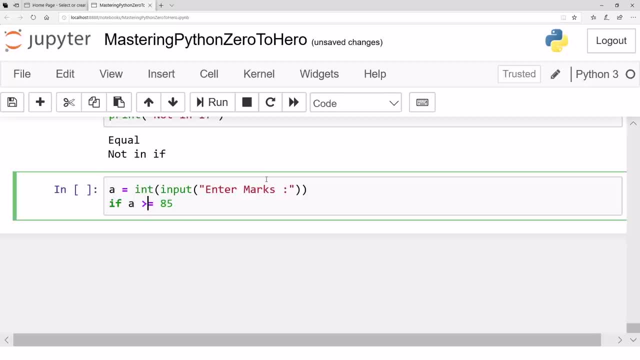 but don't actually write the space inside that, because larger and equal to the combined, without space, is an operator. so if a is larger than 85, then print, let's say, a grade great l if a is a is larger or equal to 80 and a is smaller than 85. so let me, let me write this in a more readable form. else, if a is smaller, 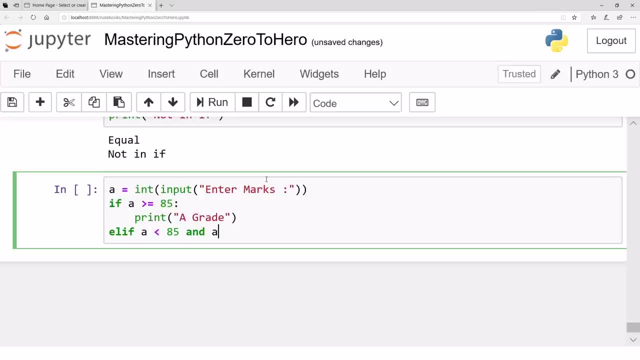 than 85 and a is larger or equal to 80, then we should do what. it is sometimes good to include these kind of uh parentheses. sometimes it is good just to make these things more readable: that this is one block, this is one, this is one boolean, this is one boolean. this is one decen, this is. 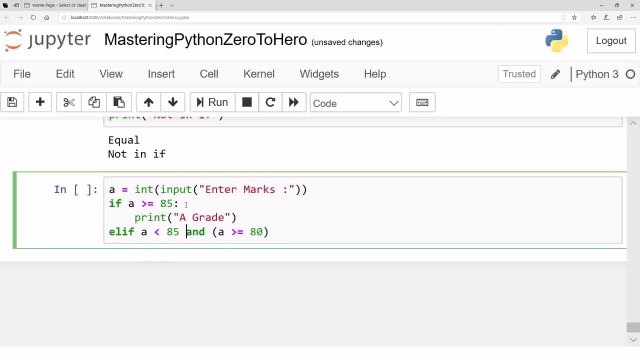 although not writing the parentheses is also okay, but writing the parenthesis makes uh code a little more readable. so, for example, if a is smaller than 85 and a is larger than 80, if that is true, so remember that, make these things more readable. if this Parents guys Eternal quote that you want to know, this changes here a little more readable. so for example, 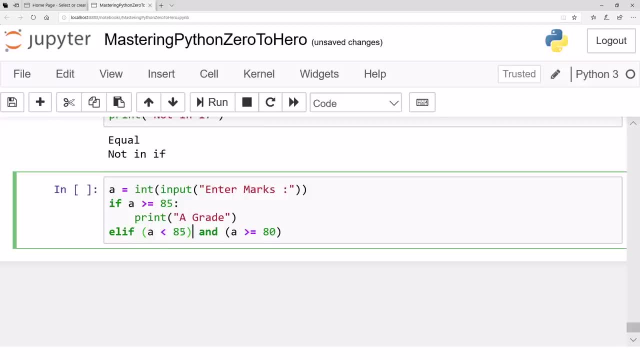 so, for example, if a is smaller than 85 and a is larger than 80, if that is true, so remember, and is true only when the left side is true and right side, both are true, then this whole condition becomes true, and I promised you that I. 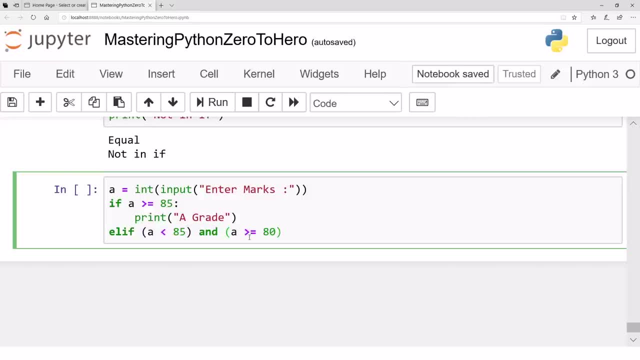 will show you the power of comparisons and actually combining the boolean variables, using ands and ors and stuff like so. so here you are seeing the one. in that case, let's say print, let's say a minus grade, and LF if a is, if a is. 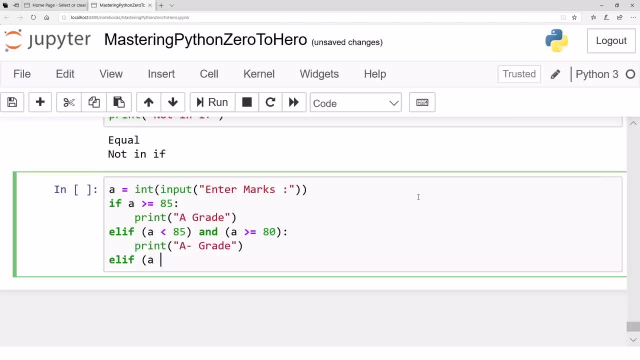 smaller than, if a is smaller than 80 and a is bigger or equal to 75. if that's the case, then what should we do? let me commit the plentiful just to show that, whether writing parentheses or not, writing parentheses is perfectly okay. I just recommend to write parentheses. so. 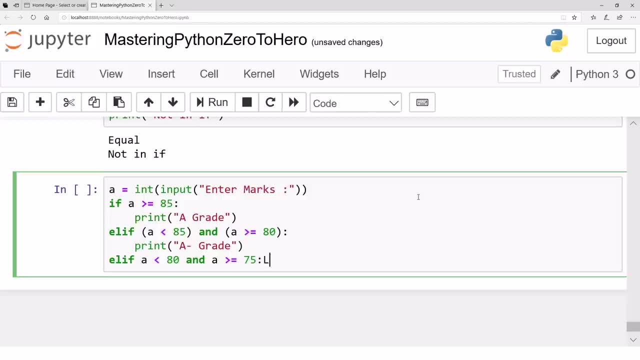 the code becomes much more readable than otherwise. okay, then we have print let's: Let's say B grade and let's say one more LF: if A is smaller than 75 and A is larger or equal to, let's say, 70, then print B minus grade. let's say: 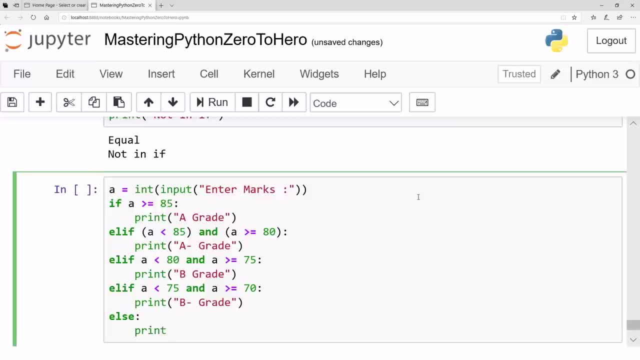 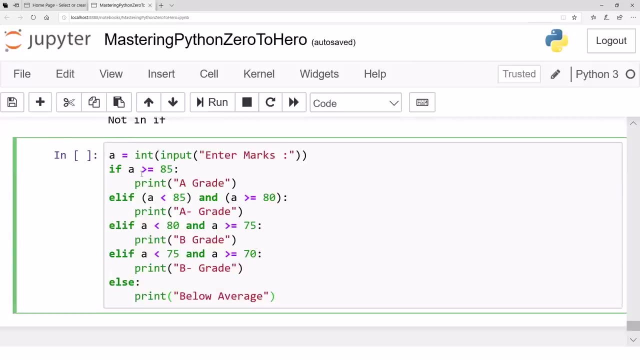 Let's just finish this. Let's else print below 70. Average, for example. Let's say that's our code, So we will enter numbers. If the number is greater than 85, then A grade. If, when this condition becomes true, then this print will execute and we will out of. 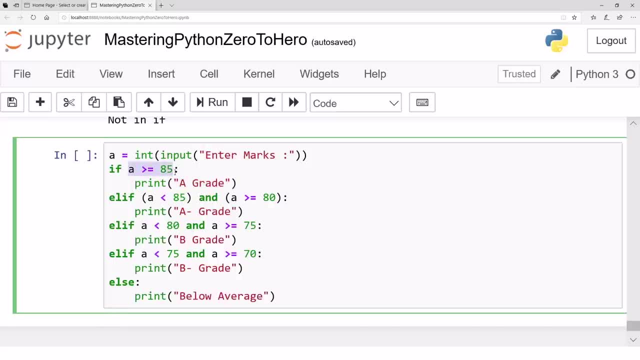 the structure right there. If this condition is false, then this condition will be checked. If this condition becomes true, then this print will execute and we will be out of the structure. If this is false- and this is false- then this will be checked. 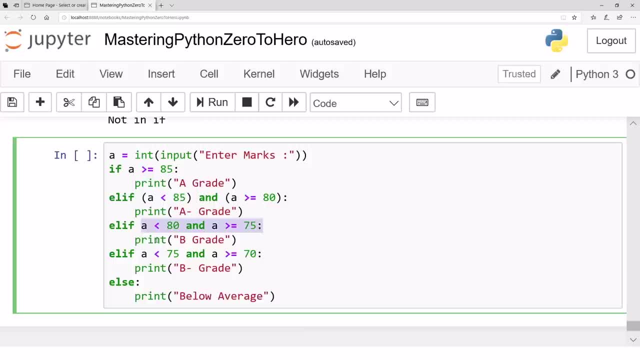 If this is true, then we print B grade and we are out. But if this is false, then this will be checked. And if this is true, then we will print B minus grade and we will be out. If this is also false, then we will dive into else part and we will say: okay, below average. 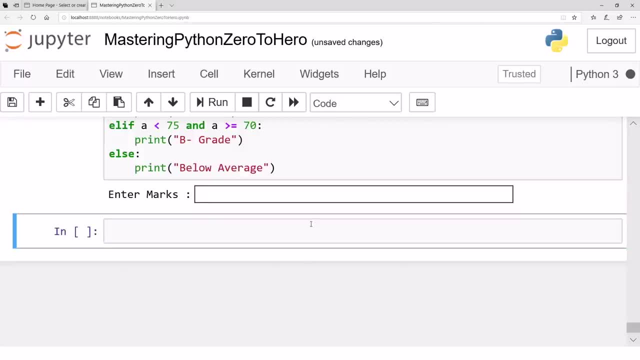 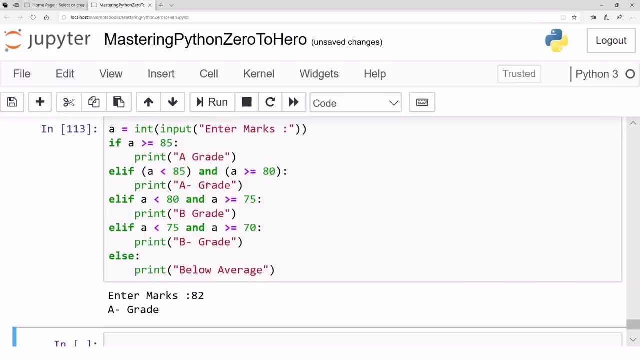 So let's see, for example, Let's say the marks are 82.. 82. So A minus grade. That makes sense. A minus grade Because the marks are smaller than 85 and larger than larger or equal to 80, so A minus. 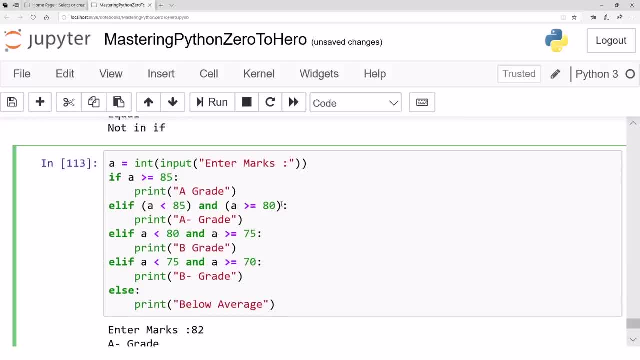 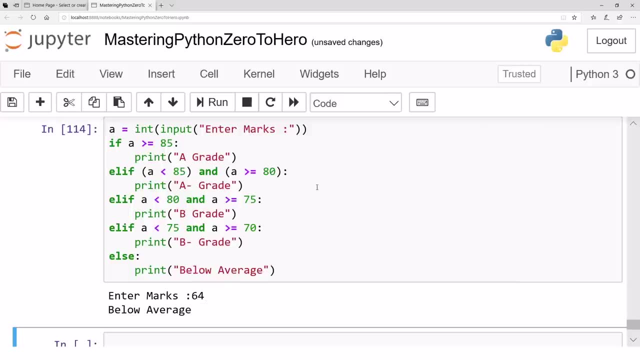 grade. Yeah, Let's run this again. And we have, let's say, marks, let's say 64.. Below average: Okay, Great. So you see this, if elif, elif, elif, else This can go. 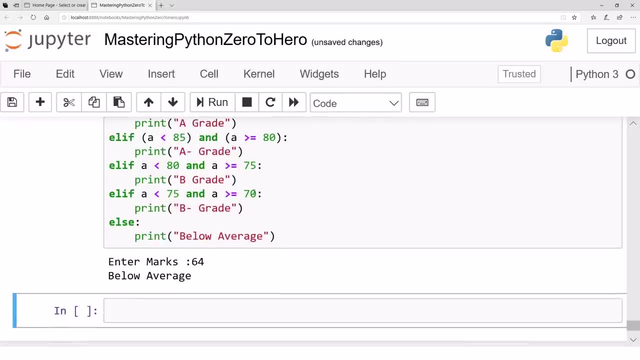 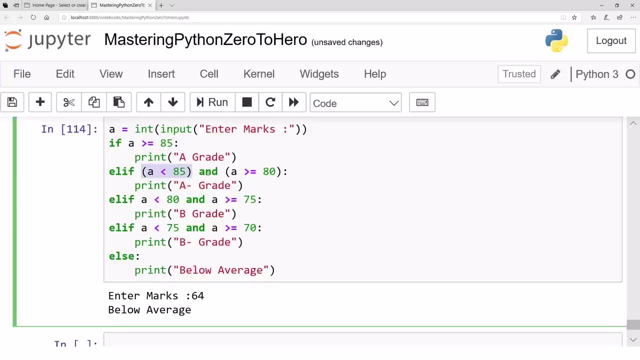 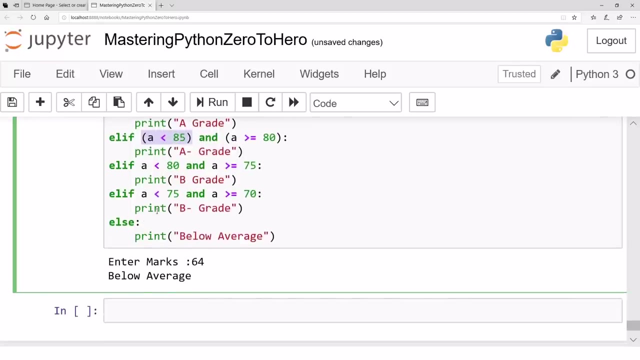 This can go as long as you want, depending upon your logic, So great And further. you can combine several comparisons, several booleans, together with ands and ors and nots, whatever you like to do. Let me give you one more beautiful thing. 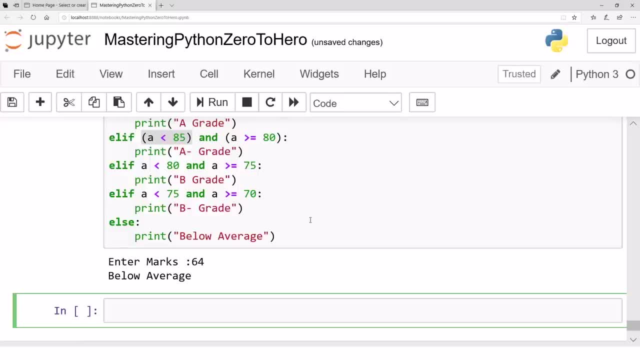 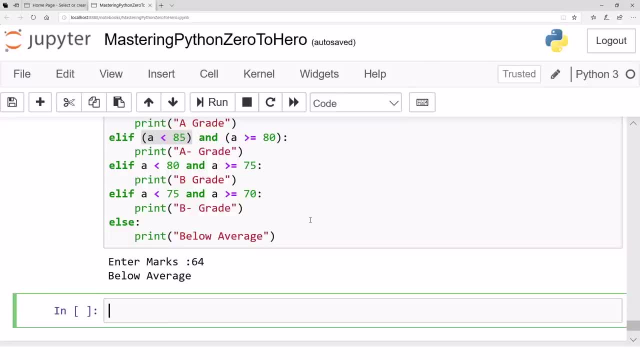 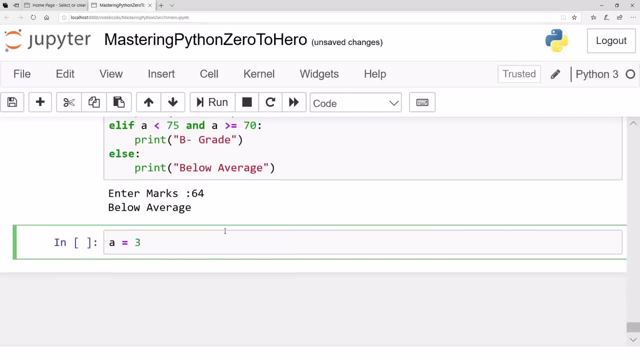 Let's just write elif and else, And then let's just implement else, Completely else. So we're not going to write else explicitly, but we are going to write a program that actually simulates else. So let's see A equals, let's say three. 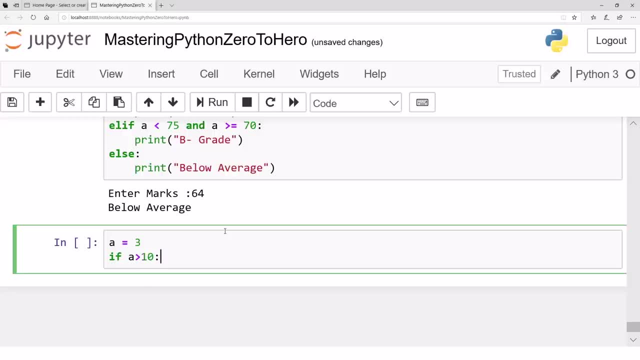 If A is larger than 10, then print, let's say, larger than 10.. Now we are not going to write else, But we are going to achieve the else else, part l. if not a is greater than 10, you see, then print else part. You see that. 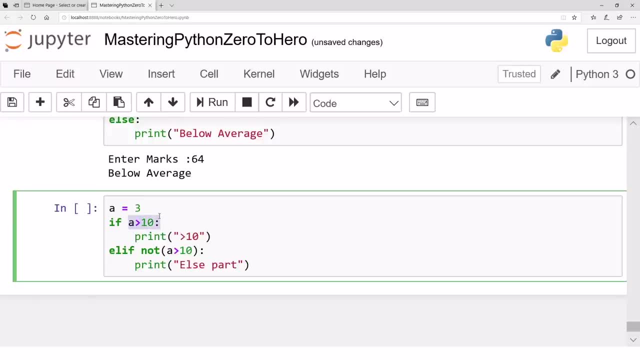 I mean that's beautiful. If this condition is true, then go there. If this condition is false, then not of false is true, then you land here And you need not to write an else part if you want. Just I've implemented. I have implemented else part using l, if So. 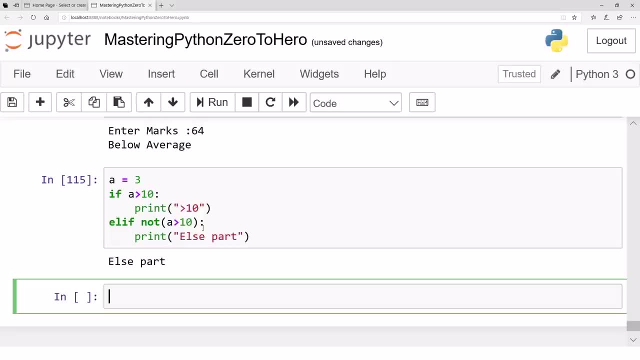 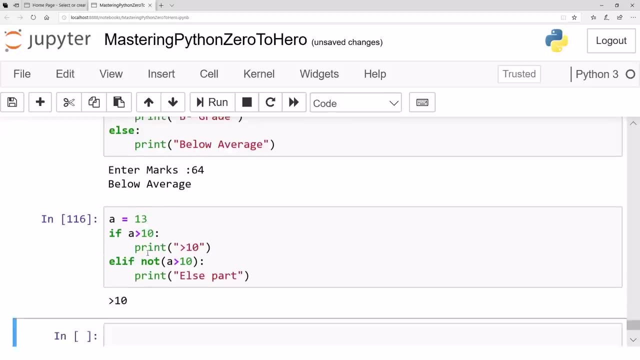 see that. So else part. So we are in else part. If a is, let's say, 13,, then we will print okay, greater than 10.. Oh, just for fun, Just for fun, Okay, Okay, great, So. 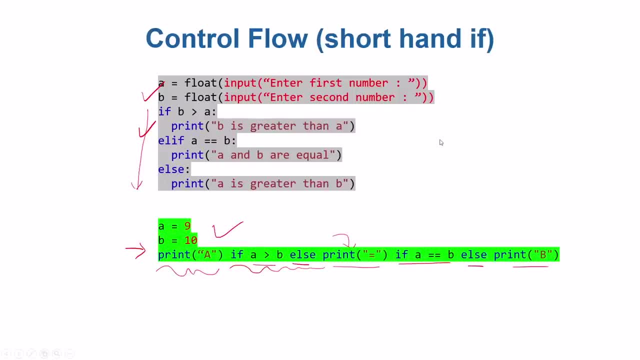 we saw if condition- it's shorthand- and else if structure in a bit more lengthy way. So in the next video we will see if condition inside or in the body of another, if condition, which is called a nested if. So hope to see you in the next video. In the last video, 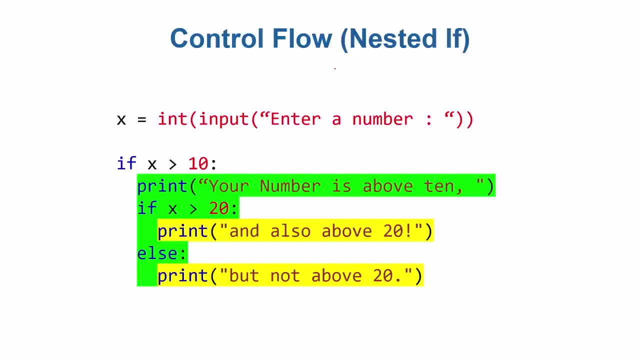 we saw if else if structure. In this particular video we will see nested if, or simply called if, inside the body of another. if So, let's take an example to understand what nested if condition is. Simply, we can understand if condition inside another, if condition. 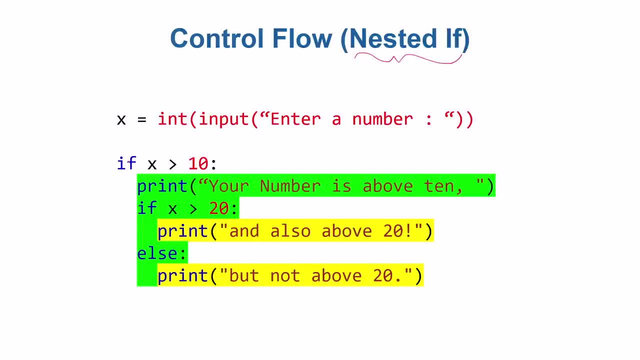 That's all. Rest of the story is the same The way. if works, it works even if it is inside the body of another if or anywhere actually. So let's say we have input a number and then we check if x is larger than 10, then you move inside the if condition. 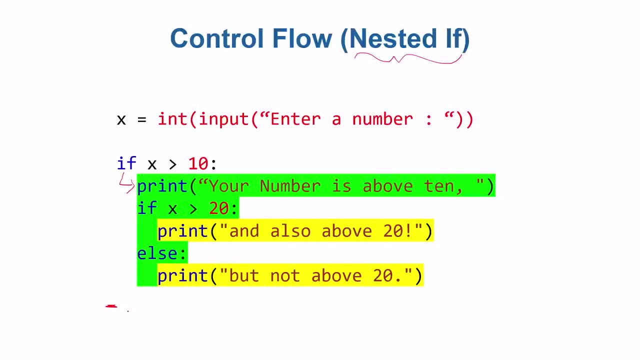 If that is true. If that is false, then you are here. Whatever you write here, it will work from here. But let's say x is greater than 10.. Then you print: your number is greater than 10.. Your number is above 10.. Let's say, you print that Now, after this statement. 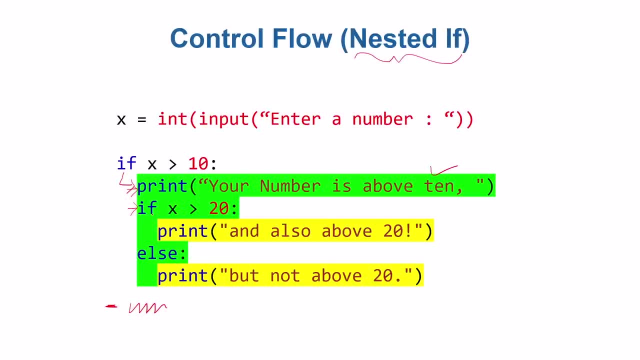 you move to this statement and you just make another check: If x is larger than 20.. Now you see this if condition. This particular statement is inside this particular if condition. If this condition becomes true, only then you dive in, Otherwise you're not. So here you are checking if x. 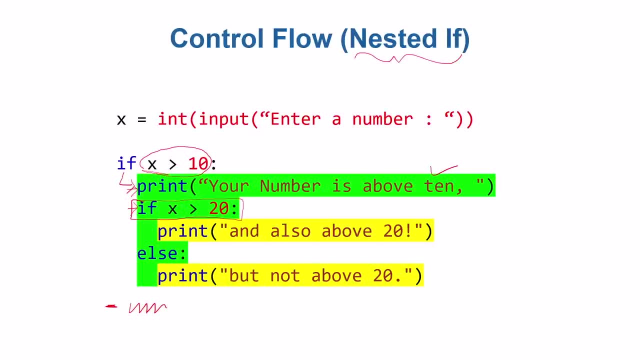 is larger than 10.. Then you move inside, and inside you are making more checks. So, for example, if x is larger than 10, then you print or do some stuff here. Then you apply further, more checks, more granularity, more, whatever your logic is. So let's say here: 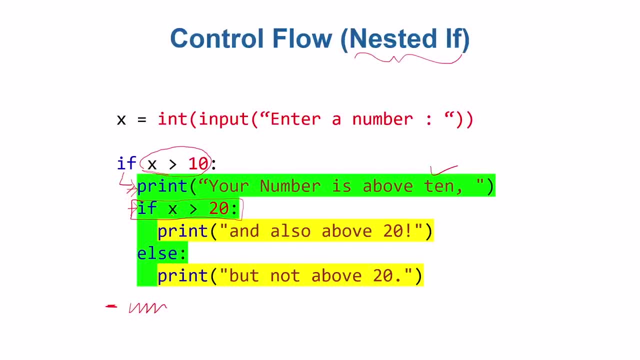 you are checking if x is larger than 20.. than 20 now. if this condition is true, then you move here else. now this else is of this: if if x is not larger than 20, then you move to this else else part and you're here. so 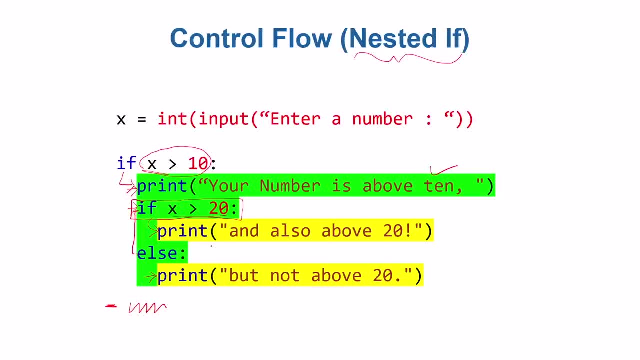 and we can have another if inside this particular if, or an if inside this else part, and so on. so if inside an if is called nested if and we can have, I mean deep structures, for example, if, then something, then if, then something, then if so maybe we can have a very lengthy. 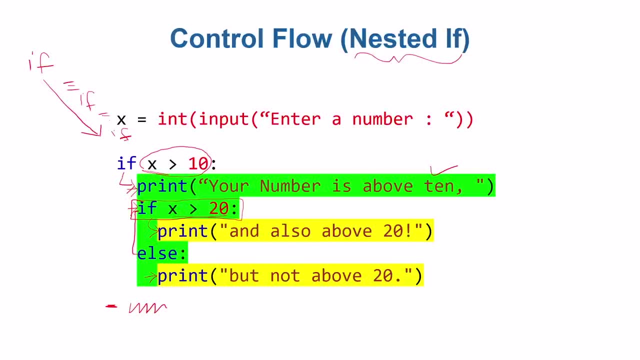 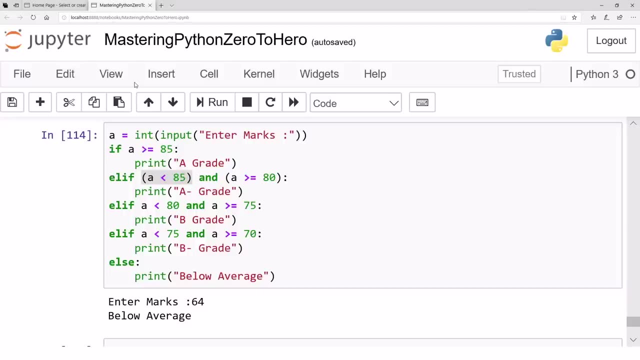 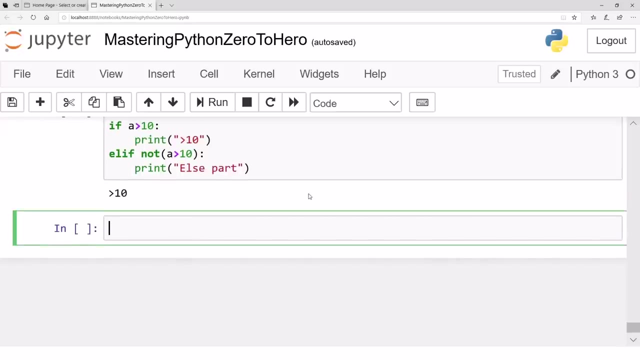 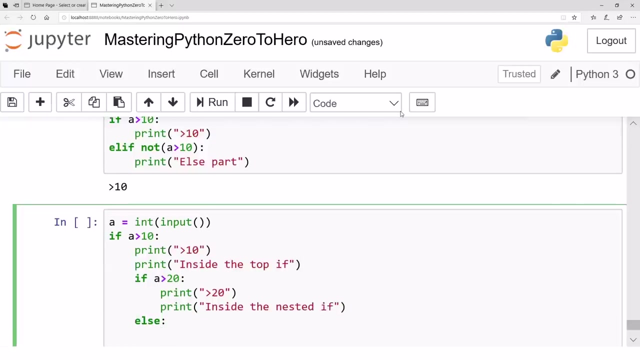 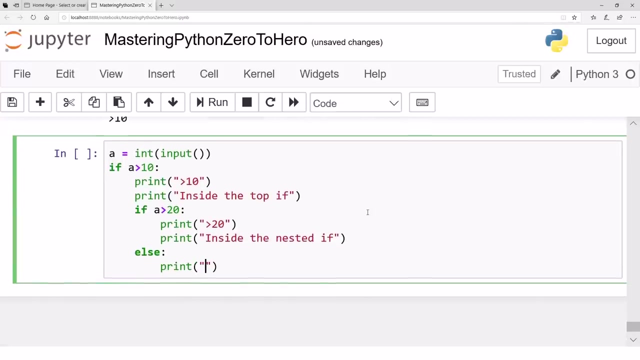 structure if nested, if structure, depending upon the logic. so let's get ourselves comfortable, as always, by writing the code on Jupyter notebook, because that make much more sense when we see things running on on on the notebook. so let's say: a is a is this, is this complete thing, is called the body of this if condition and the body will. 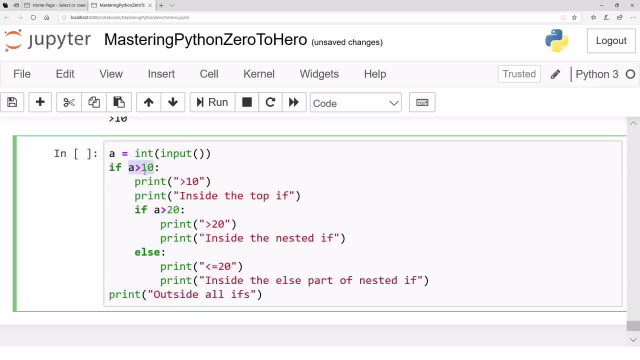 only execute if the condition becomes true, whether that condition is just a single condition or you have a combination of a lot of comparisons and a lot of booleans, whatever. if this condition becomes true, whatever that condition takes form of, then, then, and only then, you dive into. 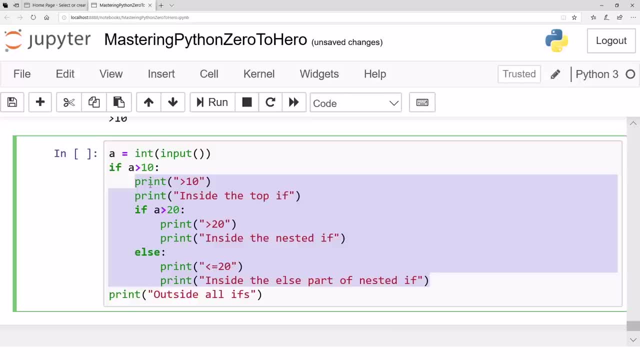 this part, and when you are in this part, then that's a whole new universe, then you are on its own in the new part, in the new part, for example, if this condition becomes true, then you are in this part. that's the body of this particular if condition and that's the body of the else part. see the body of. 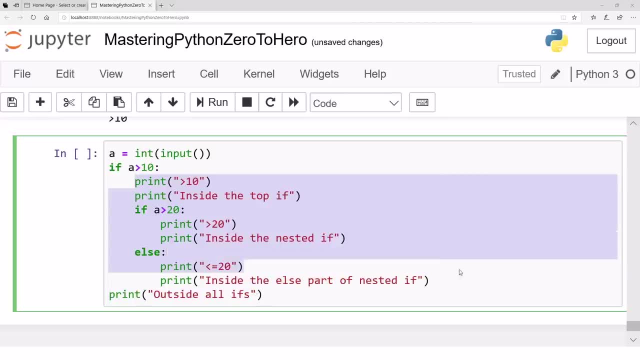 the top if condition has this kind of alignment. all the statements that are in the body of if condition- they start in the same alignment. and all the conditions, all the statements that are in the body of this particular if condition- they have their own alignment, and then what it takes to define them. all super important. 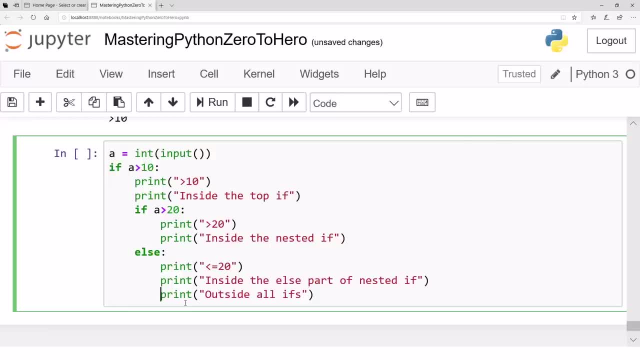 is exactly this. otherwise we are satisfied. we won't much help you when your condition is telling you- in this case it does- you won't much help. but if you делать it like this, then the mentality should always gamers. most of us like: fuck, that is making them just той. 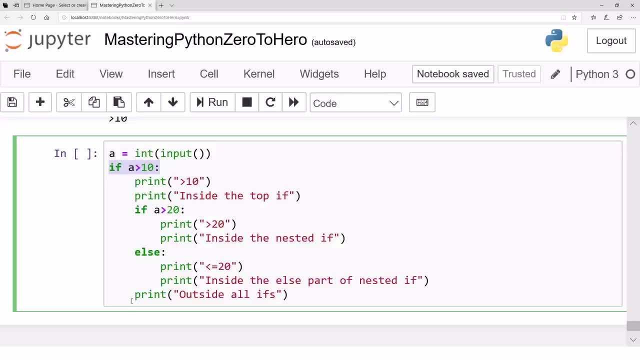 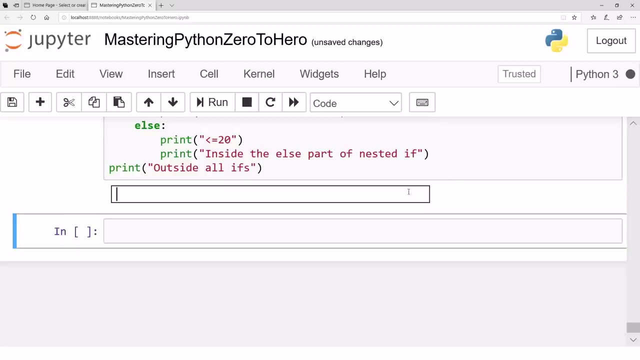 inside this if condition. this is the indentation that is defining the placement of different statements, and if the print starts from here, then it is completely outside of all if conditions. it is like this way. so let's run this code and see what happens. let's say we print. let's say we just write a equals. 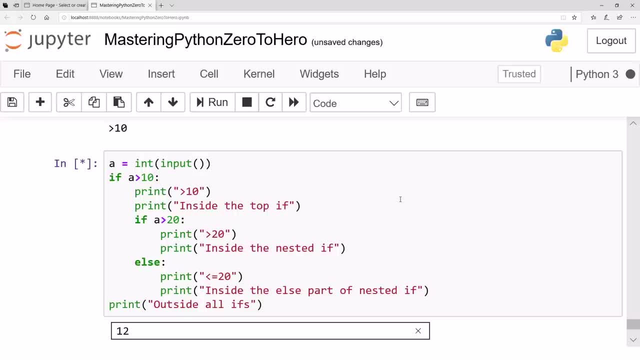 let's say 12. so what do you think what should be printed? if a is 12, then first of all this condition is true, so greater than 10 will be printed inside the top. if that will be printed, then this check will be executed and this condition will. 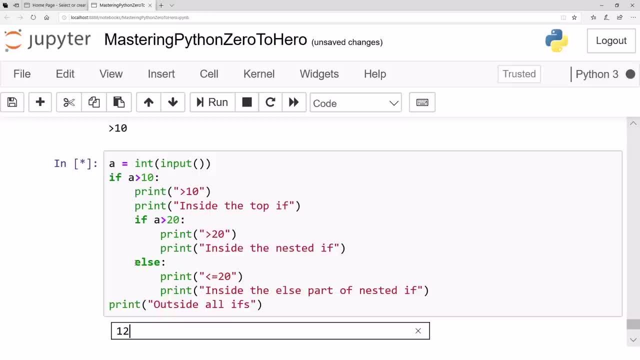 become false because 12 is not larger than 20, then you will go to the else part and less or equal to 20, this number, this string, will be printed and then inside the else part of nested, if that will be printed, and then you will be out. 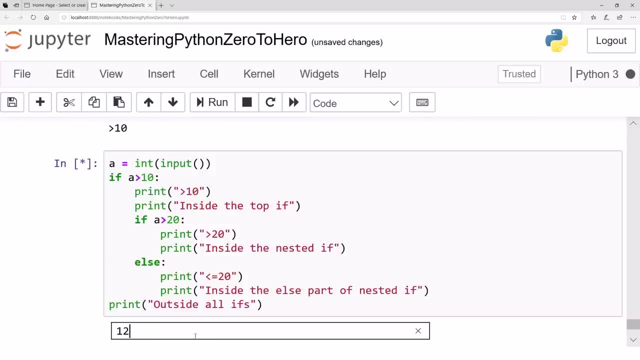 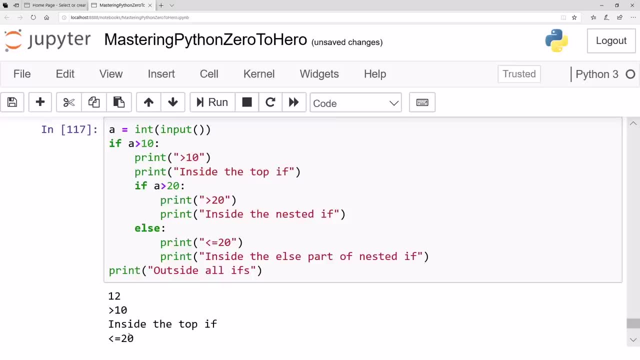 of all if condition, then outside of all ifs, that will be printed. so let's see whether whatever we have said is correct. no, so yes, greater than 10 inside the top. if less or equal to 20 inside the else part of the nested if outside all ifs. yeah, so that's what the nested if is, and 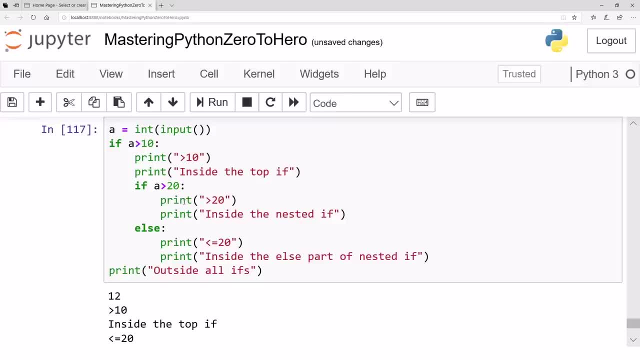 by the way you can have. you can have, for example, more if conditions inside the nested ifs, for example. you can have one more condition here, if a is larger than 30, for example, well then, do what then? print it is larger than 30 as well, and further print. 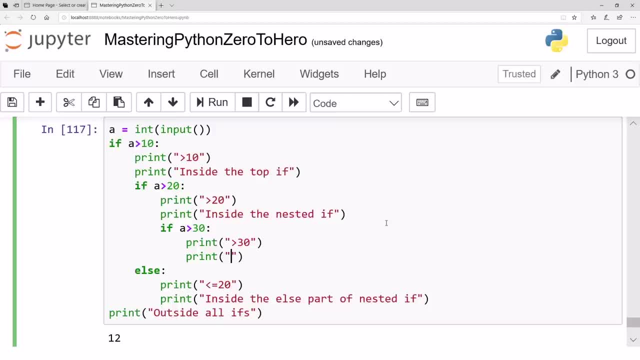 maybe not necessarily that you always write print statements. you can do any interesting stuff inside, inside the nested, if the nested, if fine, and then you can write the else else part of this particular if condition here. if you want to, or, or, or, whatever, I mean you can have as hilarious structure as you want, but that 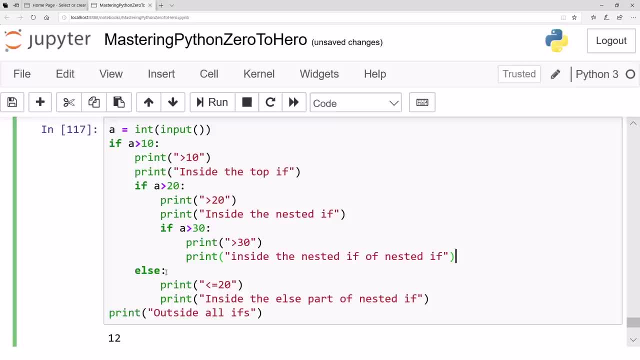 completely depends upon the logic. or you may have an if condition inside that else part. here, for example, you can write an if condition here: if whatever that is also, that is also perfectly fine. so if a is larger than 20, then you print this. if a is larger than 30, then this, for example: and let me write the else. 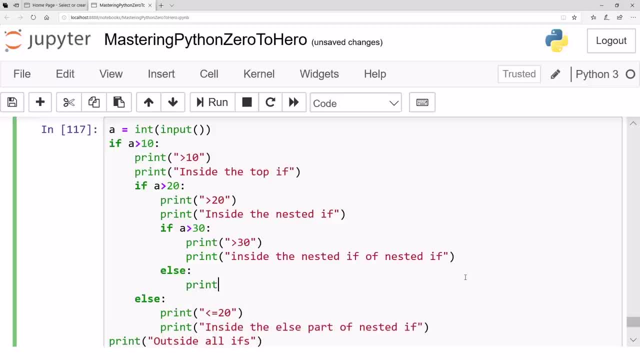 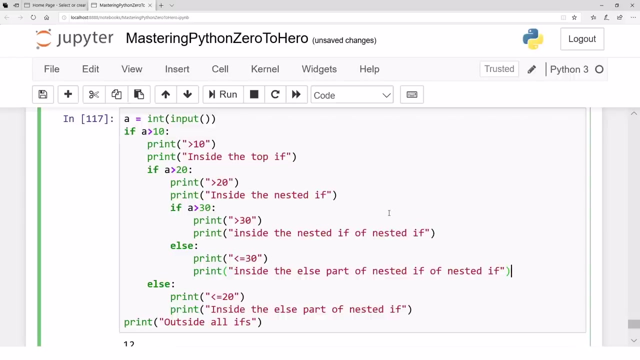 part here else, print less or equal to 30 and we can print inside the nested, inside the else part of nested, if, if of nested, if okay. so, Wow, you see that program. let me, let me just scale it down so that you can see that completely, see that program. I mean, yeah, it makes 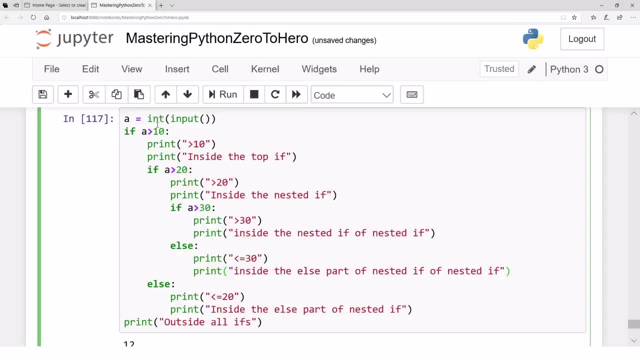 perfectly sense to me. for example, you take an input: if that is larger than 10, then you're here. if it is larger than 20, then you are here. if it is not larger than 20, then you're here. okay, so let's say it is larger than. 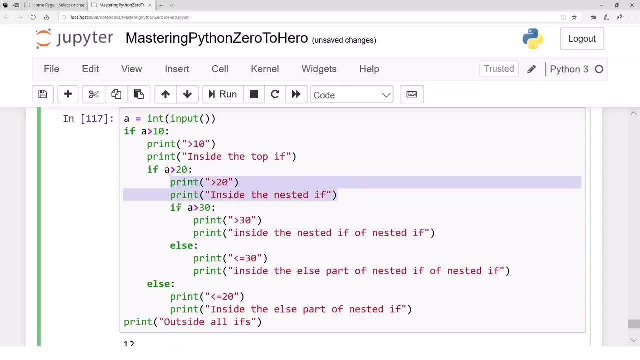 20. if it is larger than 20, then you are here. further, if it is larger than 30, then you are here, otherwise you are here, and once and by the way, if a is not larger than 10, then you are directly here. so let's run this code. let me just. 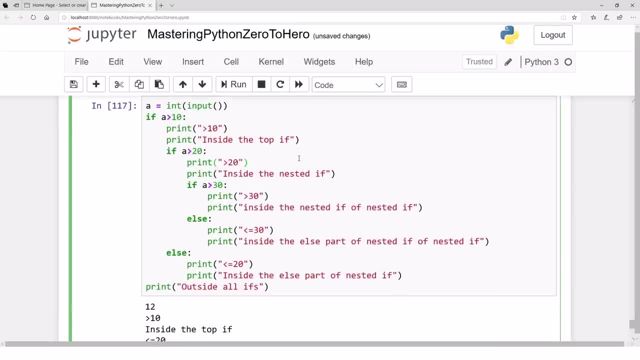 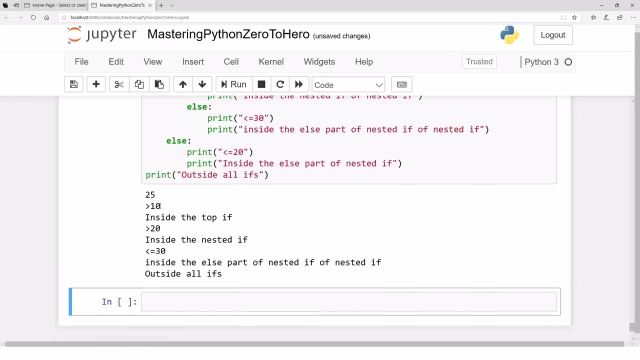 scale it down so that you can see it more. you can see more text. let's say so. let's run this no errors, great. so let's say the number is, let's say, 25. so what do you expect the result? so the number is 25, is greater than 10 inside the top. 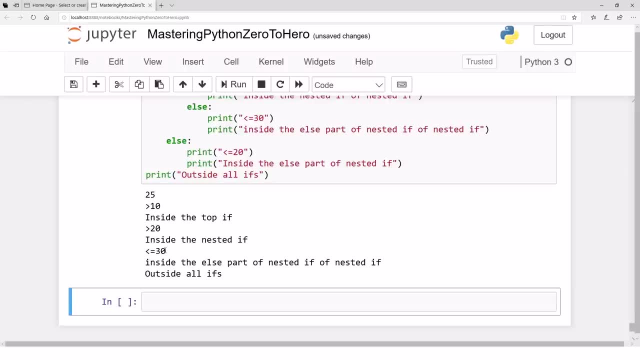 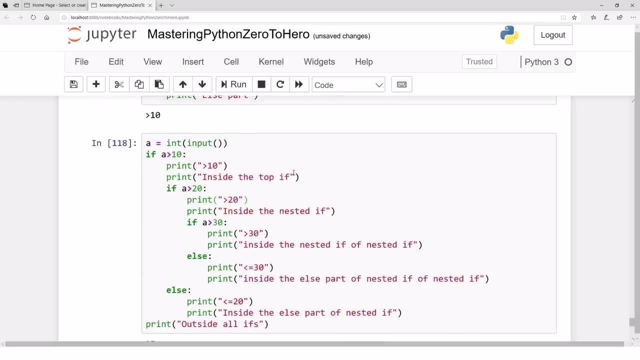 if it is greater than 20, inside the nested if it is smaller than or equal to 30. so inside the else part of nested if, of nested if, and then outside all the hips conditions. great yeah, you enjoyed that, I enjoyed that, great. ok, so that's. 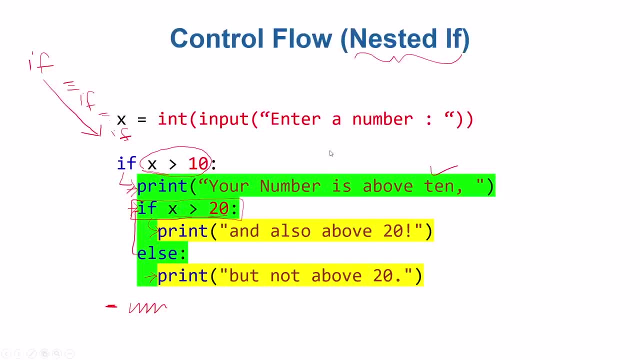 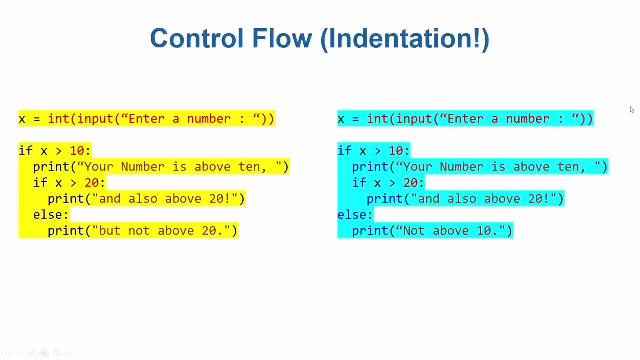 about the nested if. uh, one more thing that i have already uh told you, but just let me tell you the power of indentation. you are here, for example, in this particular if condition, that's the if condition and that's the nested if, and that's the else part of this. if, if you move this else part in in the indentation, or 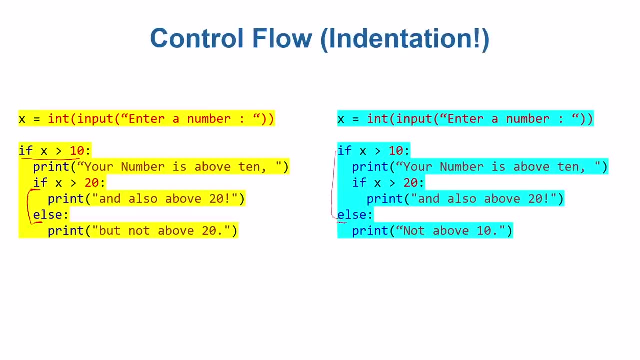 the alignment with this. if, then this is else part of this. if, and this is not the else part of this, if so, remember the power of indentation, the. this is the indentation that defines which part belongs to what, what kind of block or structure in in python, in other languages sometimes, for example, 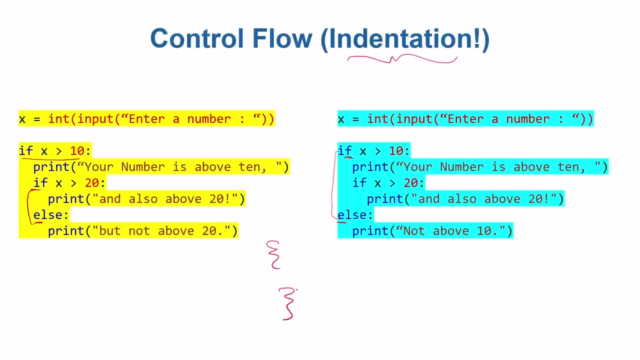 in c plus plus they. they normally use to write these curly brackets to define a block and their indentation doesn't really matter. but in python this is the indentation that actually defines each and everything. so for example, this is a crucial example if this else just moves backwards and, aligned with this, if you get this else with this, if these are two, if 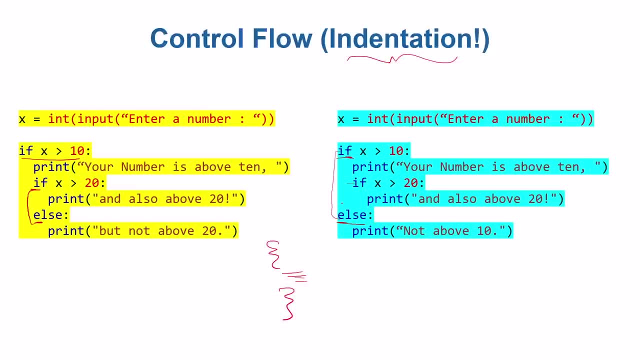 and l structures, this is still nested. if without an else part and if this else move somewhere in between, i mean, if this is not aligned with this, if this is not aligned with this, if you get a syntax error because that is not a proper indentation, so focus on indentation. that is really, really important. um, yeah, so although i have, i've told 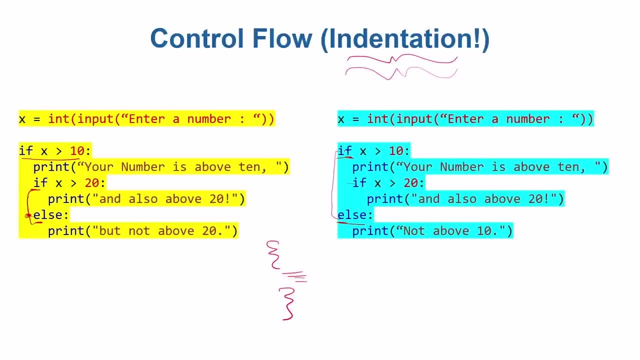 the indentation has already told you, but i just i just found to make a slide over this else part because that's important. sometimes you may get confused whether this else belongs to this, if or that, if. well, the indentation defines this else belong to what? okay, i end this. uh, control flow. 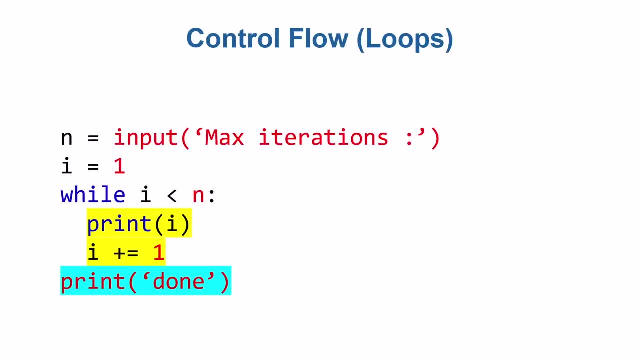 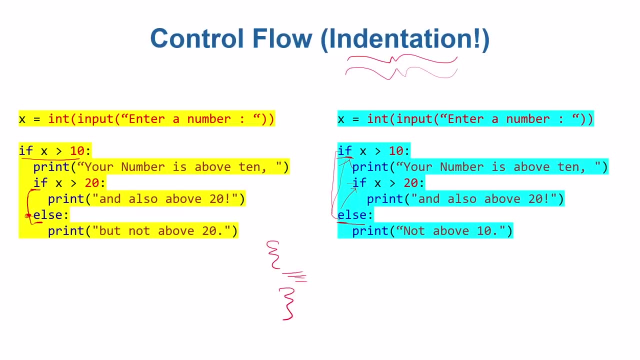 indentation here. so from next video we are jumping toward loops, but before loops, i, i just want to, i just want to write a lengthy program in. if else, if they're combinations, i just want to write a jupiter program for you to um, to get comfortable with. if nested, if um, the, the conditions that are. 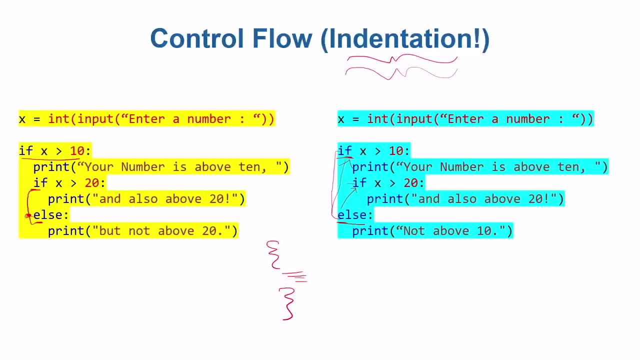 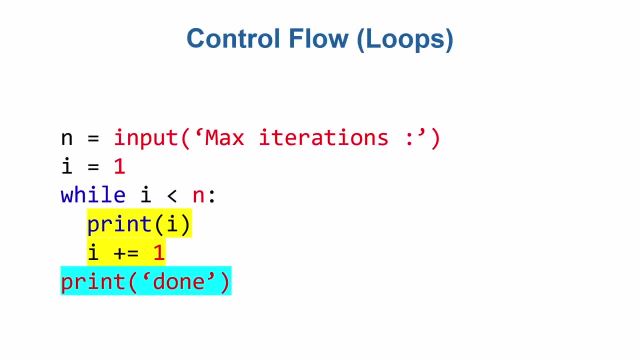 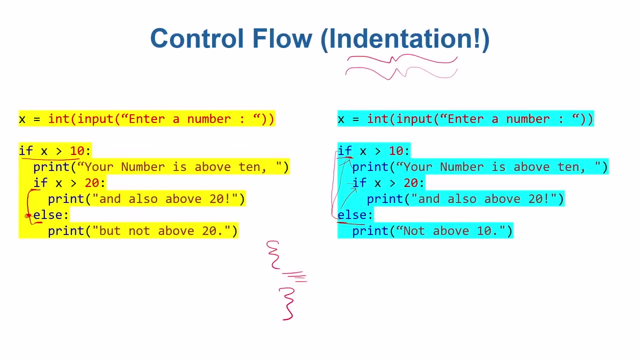 ands and ors and nots or stuff like so. so so in the next video we will be practicing more on jupiter, if conditions, and then, from the next to next video, we will be jumping toward loops, the very, very powerful structure. okay, hope to see you in the next video, okay, so, uh, let's just practice this. 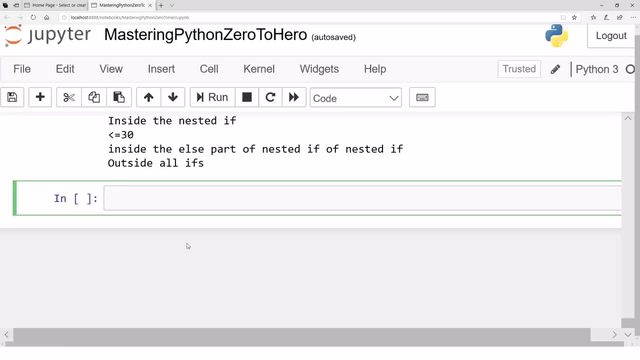 if condition a little bit more uh in this particular video and we are going to achieve a particular task, so let's design some task here. uh, by the way, this is comment comment. comment is a. it starts from a hash symbol and that's a statement that will never be executed. this just. 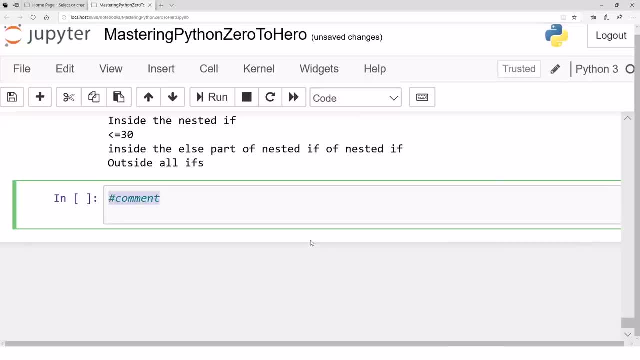 describe your code, for example. so like it, like it. it is not there, but it is there as a text but not as a code file. uh, like hash, uh, sometimes uh represents a comment or description with a single line. if your comment goes on multiple lines, it is good to write a multi-line comment. 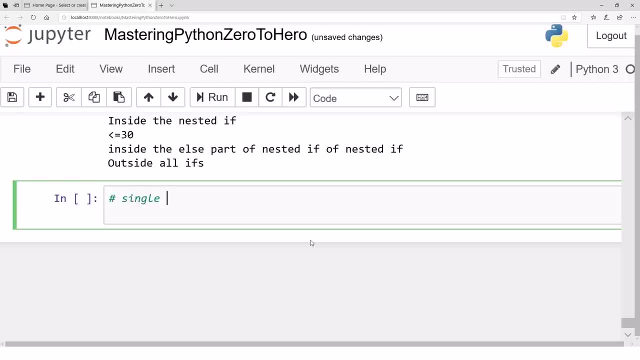 so that's a single line comment. for example, single line comment, the multi-line comments: they start with uh, three quotes and then end with three quotes. so whatever you write inside in these, uh, in this particular block, that's a multi-line comment. so let's describe our problem. 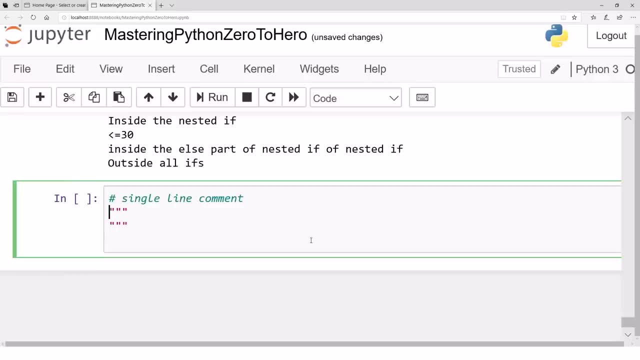 in this multi-line comments, because that's the problem in form of text, and then we will be solving that problem using using the code. so that's just description of the problem. let's say, user will enter a floating point, number, number, let's say 238.915. let's say: okay, your task is. 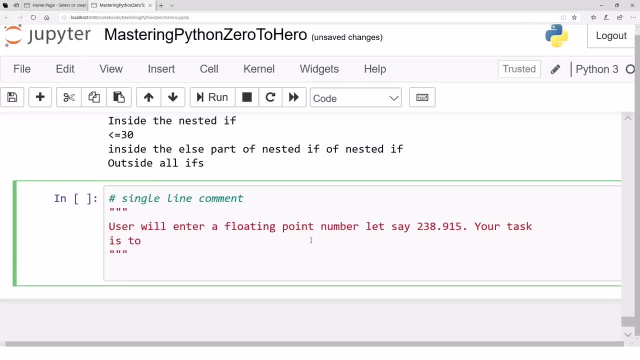 is two. so let's say just, let's just more readable. your task is to find out the integer portion, integer portion before the decimal, before the point, let's say for before the point in this case, in this case, it is set to a figure eight and then 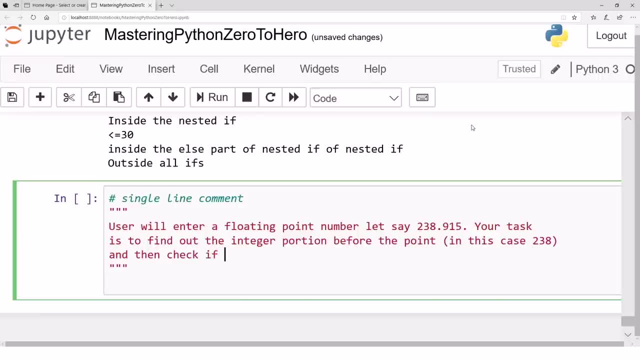 and then check whether if that integer portion is an even number or not. so just print yes or no. so print even if it is even number, otherwise print odd. so that's the, that's the problem statement. that's the problem that we're going to solve. and this is just comment. now we are outside the comment. that's a multi-line comment. 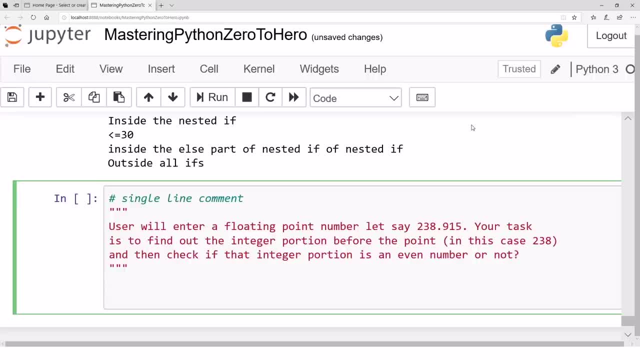 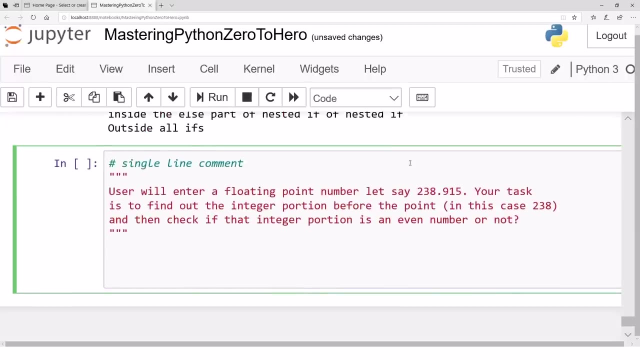 um yeah, so um, how to how to solve that problem? um, yeah, how to solve that problem, so let's start solving this problem. i'm going to spend some time on this program. just to get comfortable with the if conditions, let's say. let's say that number is x is input. let me convert that input. 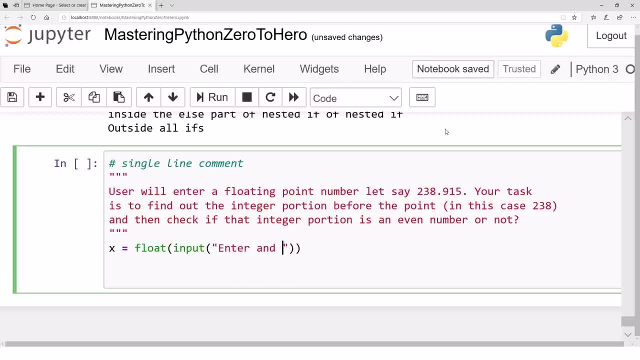 enter a real number. let's say, okay, we are just assuming that the user will enter a real number. uh, it's a real number. real number might be, i mean 238.0, that's a real number, or 238 itself, that's also a real number. 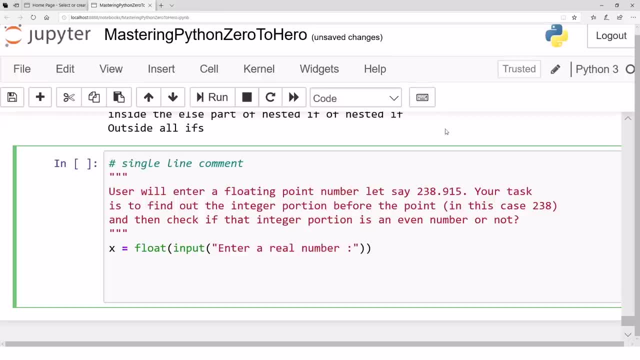 that's okay, but we are not assuming that the user will enter, let's say, some characters like abc or stuff like so just just assuming that, okay. now assume that x contains real number. it may be an integer by default. maybe user just enters 10 and that's it, so it may be already an integer. then we have to check whether that 10. 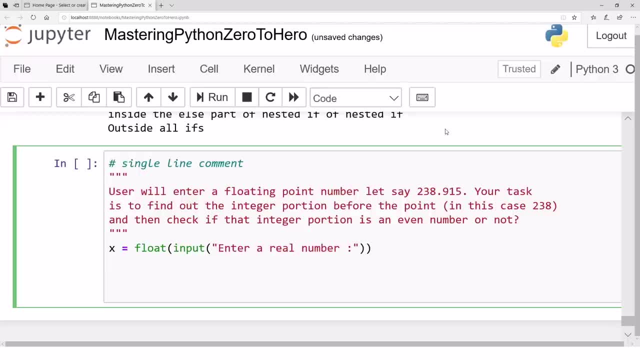 is whether that 10 is even or not. or the user may enter 11.7, or the user may enter minus 34.7, or the user may enter just 0, or user may enter just 0.35. there are a lot of possibilities that. 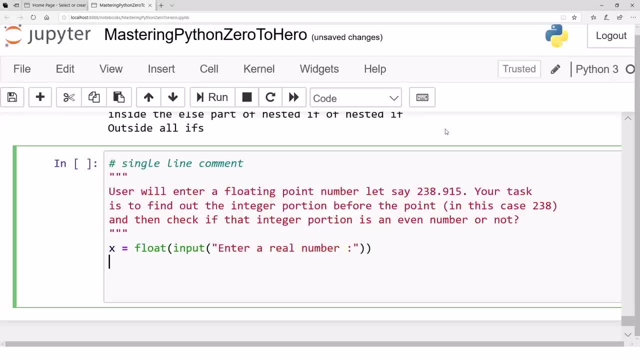 the user come up with this. X can contain any kind of number and we have to check according to. so how can we move? let us just see whether that number, let us just extract the decimal portion, the, the portion before point. let us just extract that. how can we extract that? there are two conditions. first, 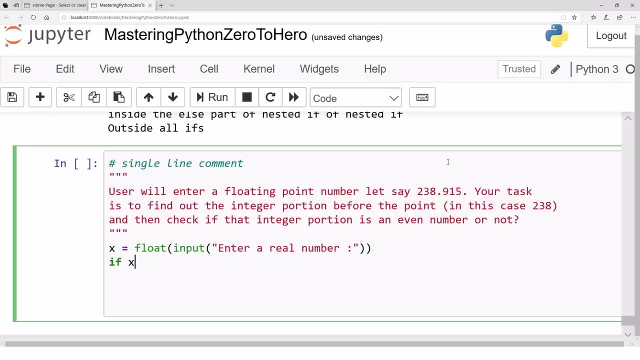 of all, let's see: if X is positive, then do what else, do what? so let's write this structure first: if X is positive, then what we have to do, and if X is negative, then what we have to do. so if X is positive, then what we do, we, we. 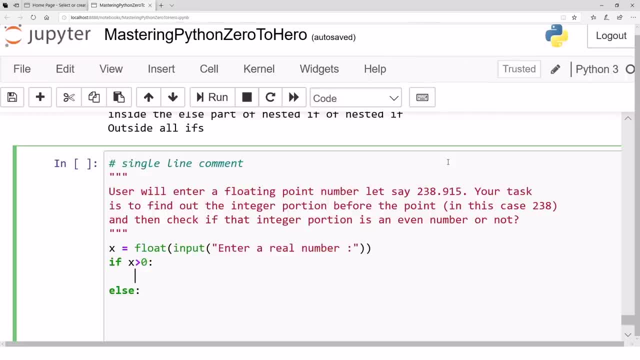 just so, what should we do? I'm just stuck here. how can we extract the, the decimal portion, the portion, without this particular thing? how can we extract that? that's, that's tricky, that's kind of tricky. yeah, so any, any ideas. I guess this the the structure I have. I'm 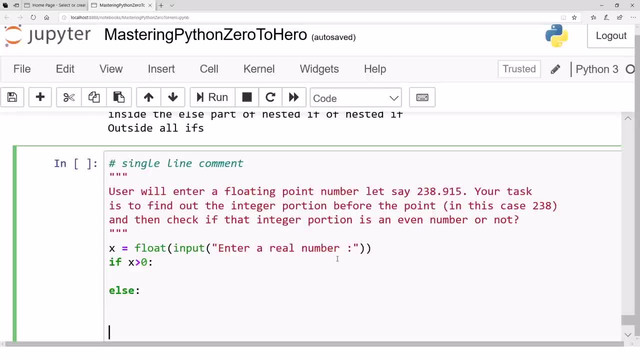 let us just first thing that x is positive, just make our life easier, and then, if X is positive, it's a positive number. how can we extract that correct' X power is a positive should be five and X is either positive or negative. it is either wrong or wrong. 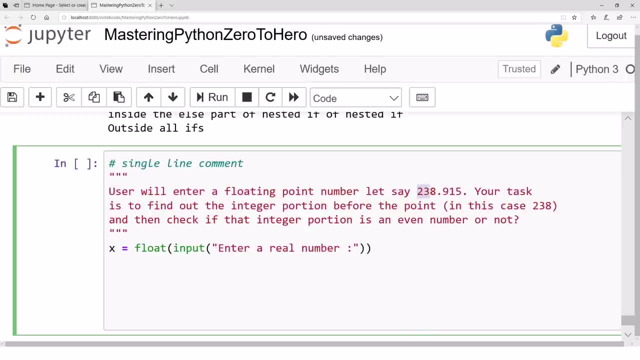 it's a positive number. how can we extract this portion out? just the number that is below, that is, before the decimal point. but what should we do? can we, can we can we apply? apply a round function? will that help, um x? will that help? it helps, yes, but no round function. so let's say y contains the rounded value of 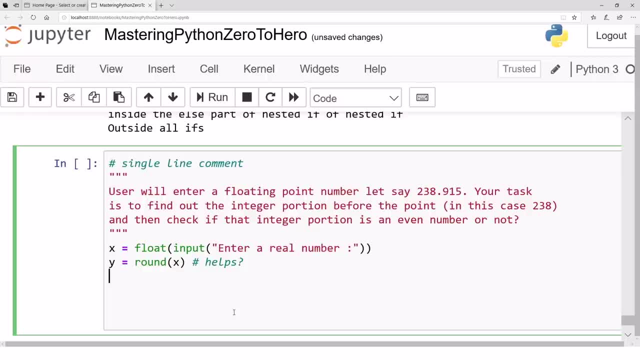 x then. so what then? how can extract? how can we extract the, the, the decimal portion, the, the portion, the integer portion? or maybe there is a function that actually, uh, round downs. let me check whether there is a function float or not. no, floor is not a function, i guess. so let's say: round x. okay, now y contains the rounded value. 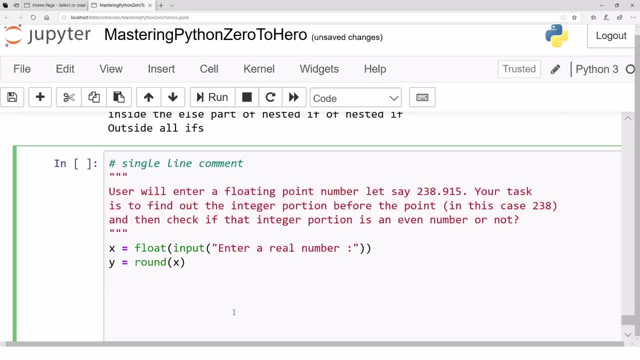 of whatever the x is. we are now assuming that x is positive. okay, then what now if? if y is larger than x, that means we moved up. okay, we moved up, the round goes up. in that case, what we do is we just subtract, uh, uh, so the let me, so we just subtract the integer portion. 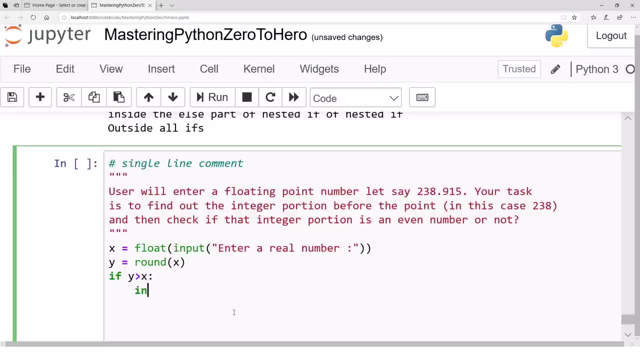 so the uh, let me- integer portion- let's say that's our variable name- then the integer portion is simply y minus one. is that correct? is that correct? if y is larger than x, then integer portion is simply uh, y minus one, for example, for example, just just think about it. 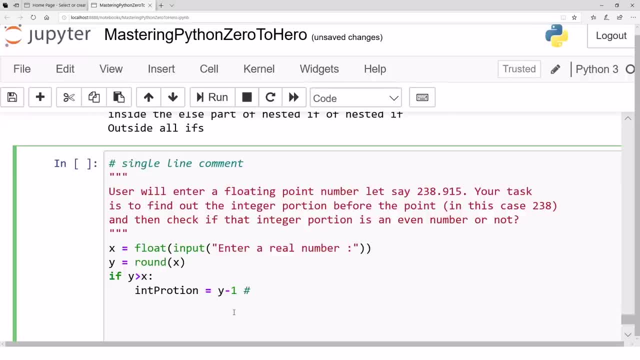 if, uh, when, when? for example, if the value was 29.6 and the rounded value will become 30, so 30 minus 1 will be 29. that is what we are, we are what we are interested in. so yeah, so otherwise, if, for example, else else, if y is not larger than x, then y itself is an integer portion. 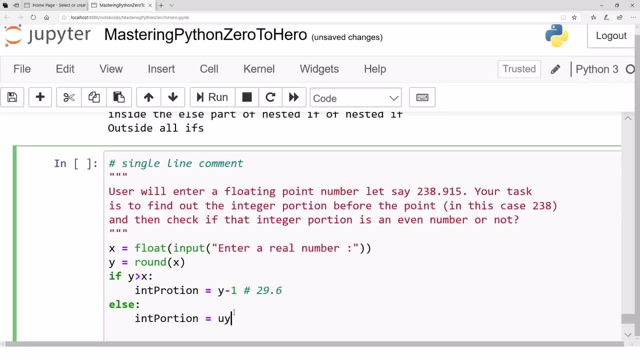 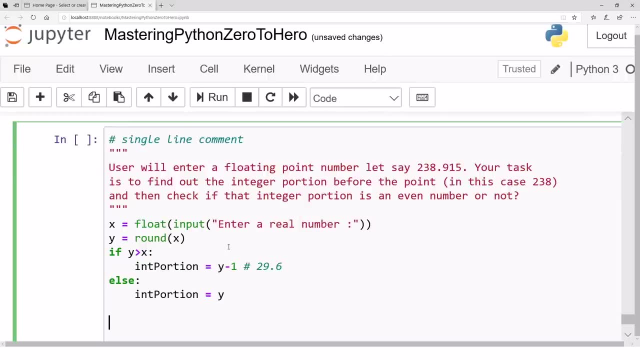 so that means that if we subtract, y itself is an integer portion, we are getting the portion y itself is an integer portion. is that correct? i mean, is that making sense to you that if, for example, if um, if x is larger than, if x is larger than, if the rounded value of x is larger than? 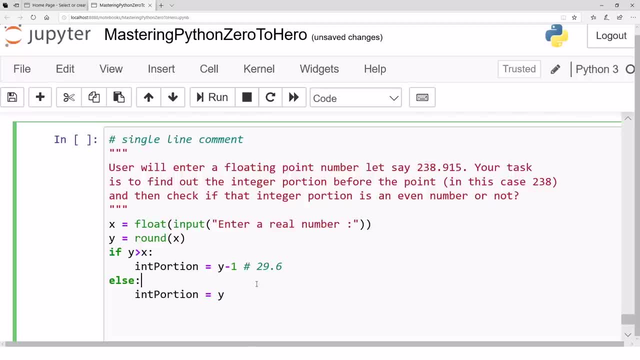 larger than x itself. then we just subtract one and we get the portion. just just, let's just run this, run this code for now, and check whether what, whatever we have done so far, is correct or not. so after that, just print, let's say, the integer portion. 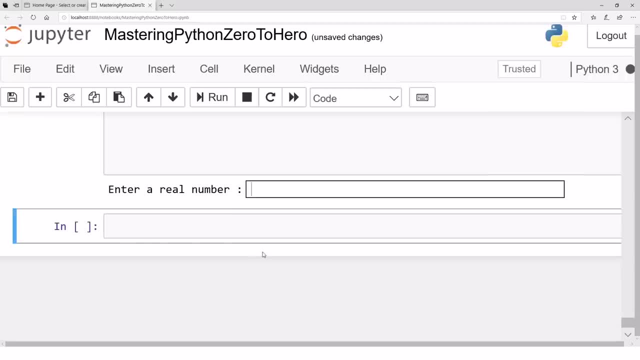 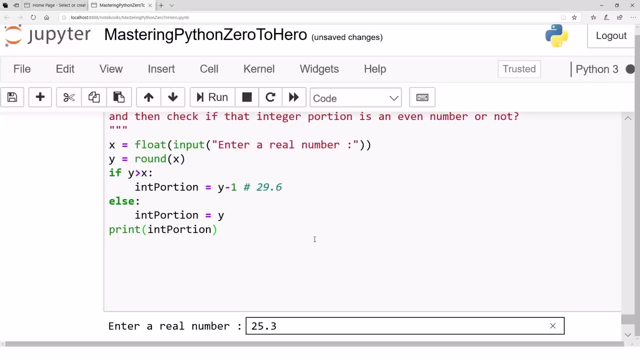 integer portion. let's just print that, okay. so enter a number. let's say the number is uh, let's say 25.3, 25.367. let's say: obviously, the integer portion here is 25. so let's say: let's see, our program returns 25 or not. oh, the result is 25, magically. oh, my god, we found 25. let's run it again. 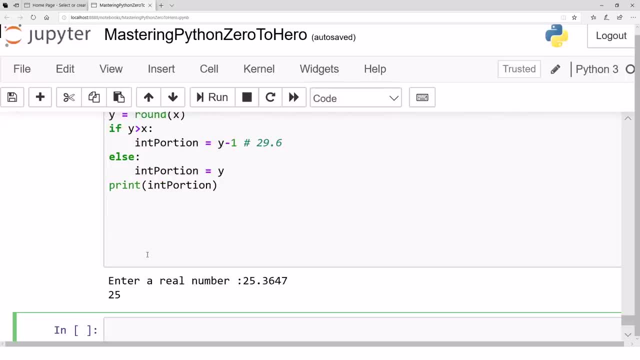 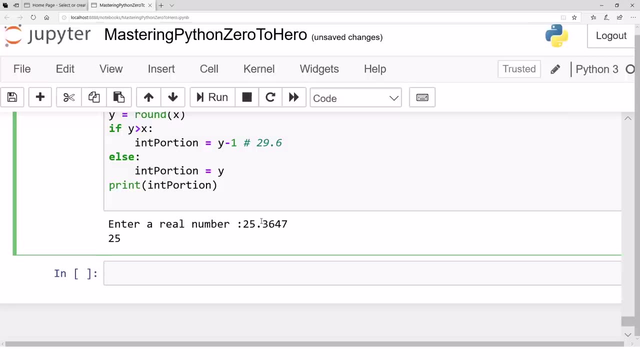 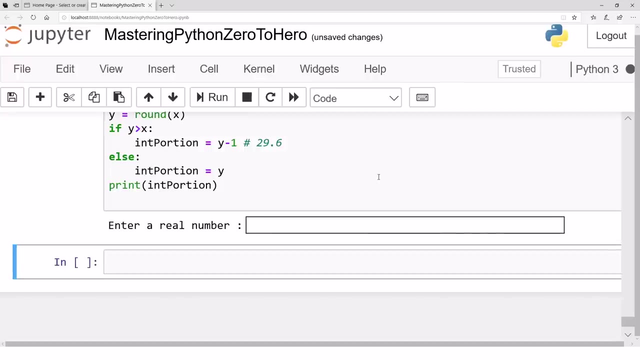 let's run it again, just to see 45.8. okay, let's run this again, and this time let's give it to 45.8. okay, the integer portion is 45, but when we will round we will get 46 and 46 minus 1 we will dive into this particular if. 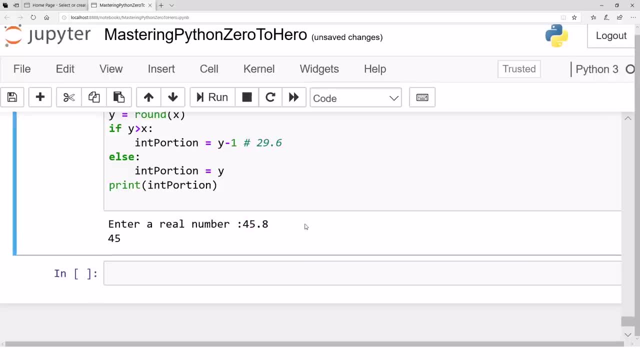 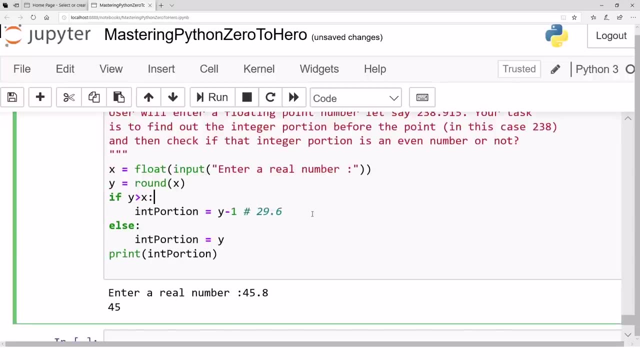 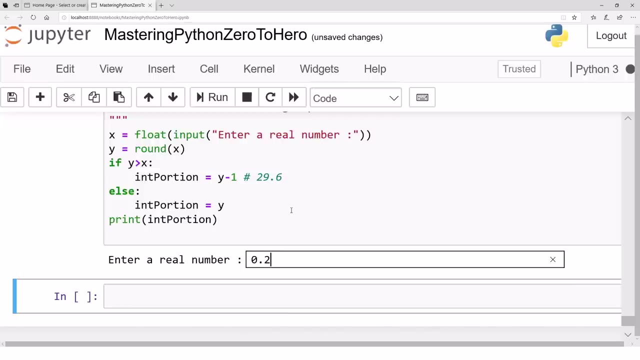 condition. let's see, uh, oh, the result is 45 we are, we are still moving. very well, great, that's, that's okay. now let's run this again. that's great, so okay, um, let's play with it. uh, let's, let's give. uh, let's give 0.2. 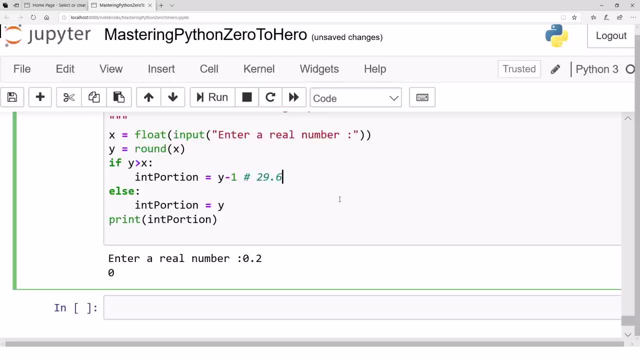 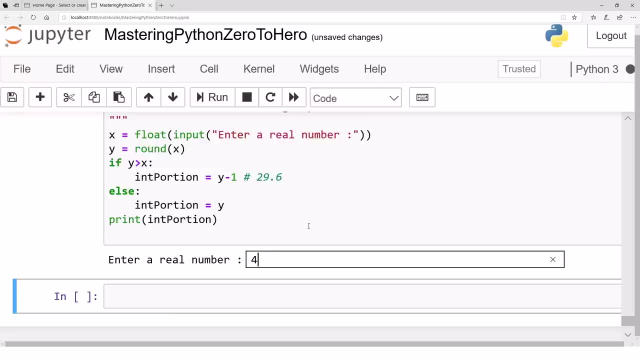 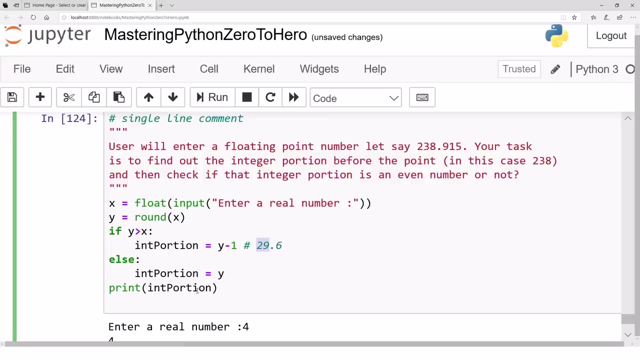 the result should be zero. it is zero, right? um, let's run it again and give it. let's say, let's say four, that's it. the result should be four. now, it is four. great, so we are working very well. we have extracted the integer portion as long as the number was positive. 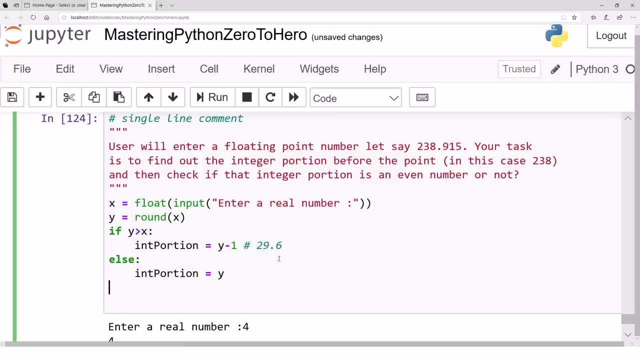 okay, great. what if the number will be negative? let's say that was true. if that was true, so that whole logic works. if x was positive? so if x is positive, then whole this logic just works. okay then else what should we do? if x is positive, then this logic works. 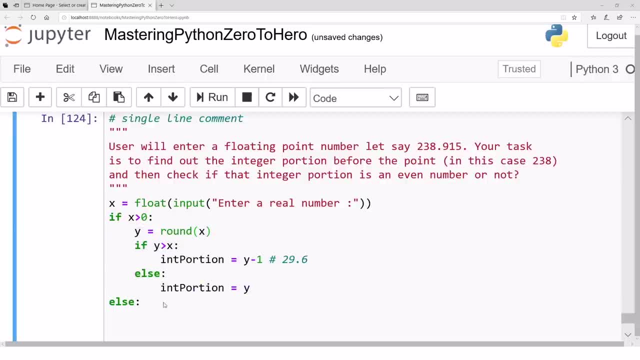 if x is not positive, then what will happen then? how can we find out the integer portion? because first we have to find out the integer portion and then we have to find out whether that integer portion is even or not. finding out whether that integer portion is even or not might be simpler, but 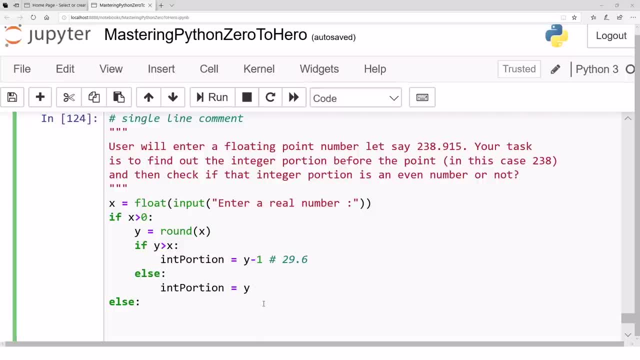 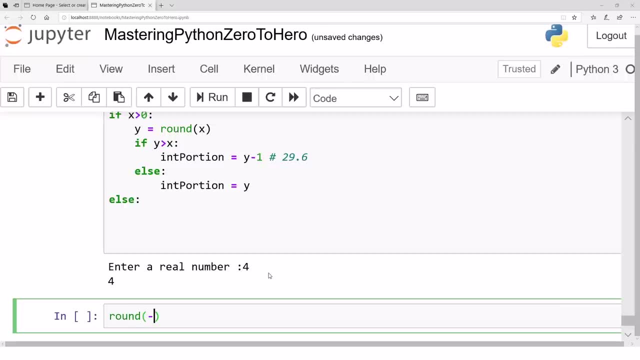 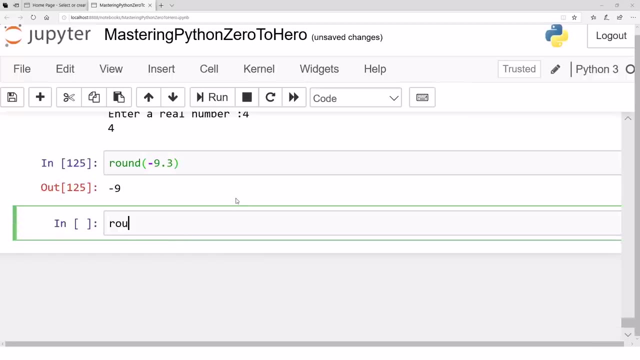 first we have to find out the integer portion. so for example: uh, let's check the behavior of round function on negative numbers. let's say round minus 9.3, so the result is minus 9. okay, if we say okay, round minus 9.6, the result will be: 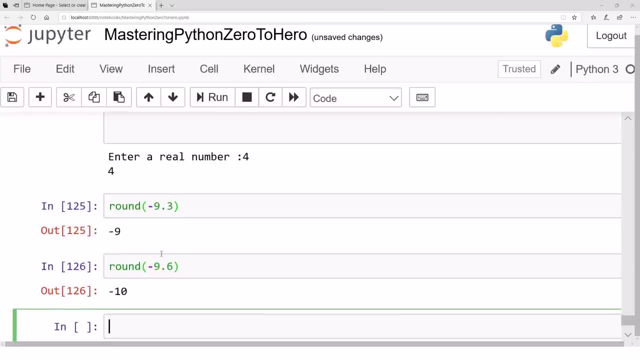 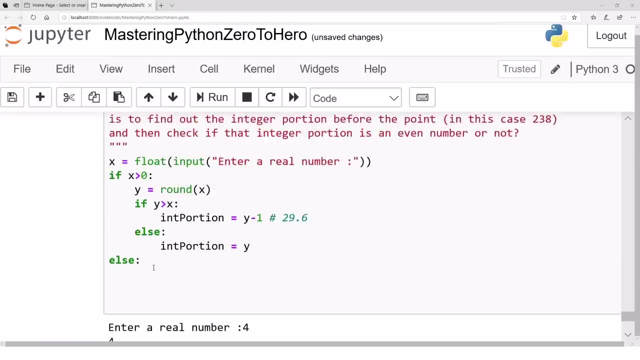 minus 10.. so it looks like the same as working in the positive number. so round function is actually working roughly the same way. it should work in the positive numbers, okay. so what should we do here? any idea? maybe we, maybe we first convert. uh, maybe first convert, by the way, uh, yeah, maybe we first convert the number. let's say y. 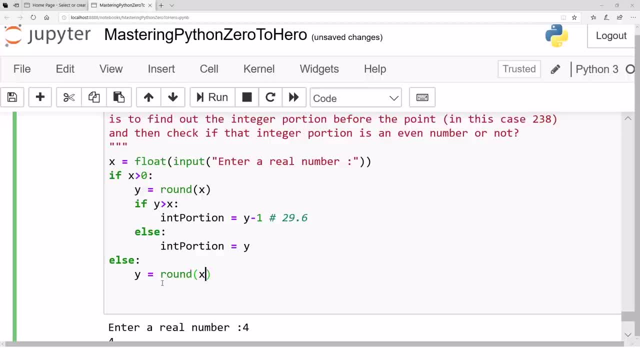 equals around x, again like before. but then what, then what? so maybe this rounding helps the same way, maybe the rounding helps the same way. we should extract this x out from this here, because it is going to work in the else part as well. why to compute it? why to write this redundant code? so y is round x. let's say: 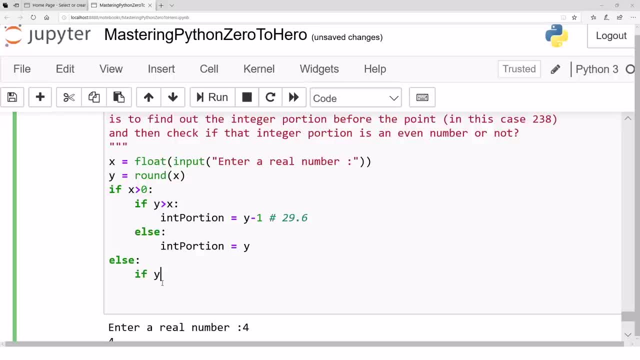 then if y is greater than x, what should we do? if it is negative, y is greater than- then what fit? what will be the portion? it will be the integer portion. will be portion will be what y minus 1 or what y plus 1. yes, you got the answer. 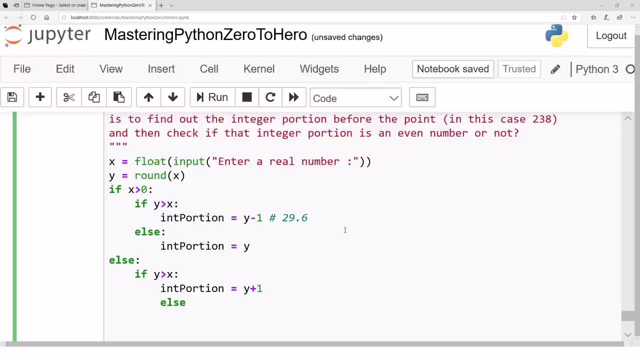 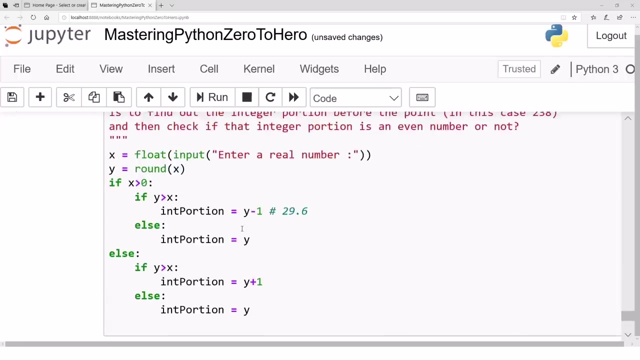 that's why plus 1, great. and else I guess we have integer portion equals Y itself. I guess. yes, I guess that's the. that's the code. that's cool, I guess. let's check, by the way, but I guess that's good. by the way, this else part is: 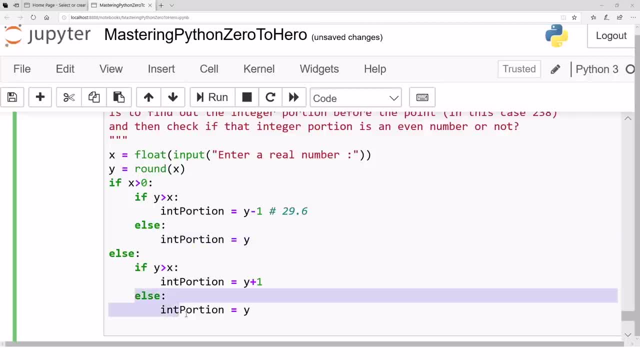 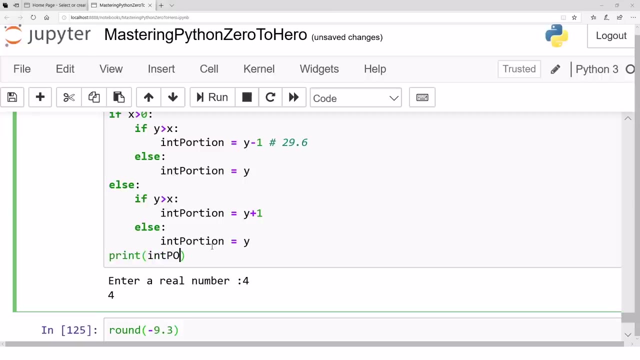 this else part is same in both of these conditions. so maybe, maybe you can combine this code and write a more elegant code, but I guess this will work. let us just print the integer portion, just to check whether we are working well so far or not. so let's enter. let's say twelve, point three. the result is 12. 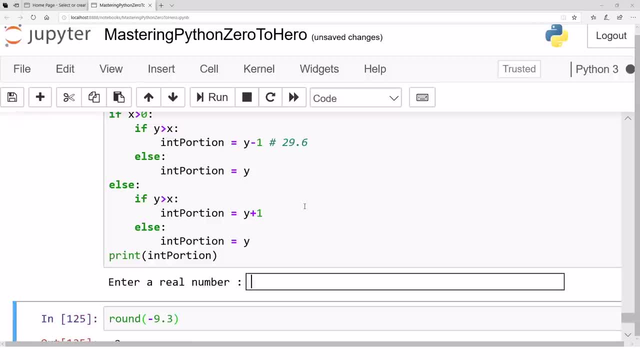 great. so it did not change our previous- I guess our previous- logic. so let's say there is minus nine, point eight. now the integer portion should be minus nine. oh, it is returning ten. why is that? why is that? oh my god, this should be changed. when it is round, it may go that way, or when it. 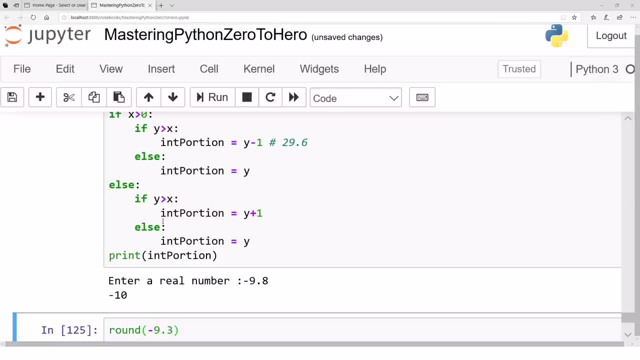 rounds, it actually becomes lesser than ten because when it rounds, it goes up and it becomes less so than in negative world. this condition should flip. yeah, so we are making an error here. let's fix that. okay, let's run this again and see. let's say minus nine point. 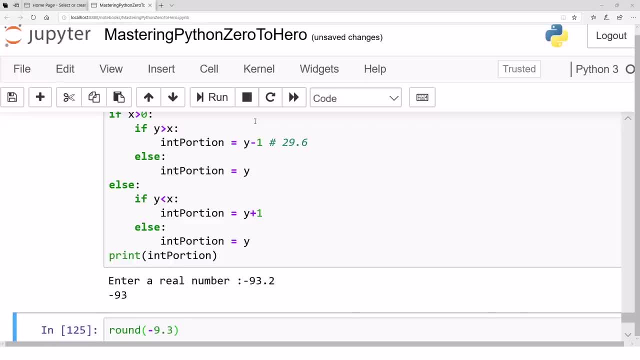 minus nine, t 3.2 minus 93, great. so then we have, let's say, let's run it again- minus eight, point nine minus eight. I guess we are working perfectly fine. once we have an integer portion with us, we just write here at the very end if 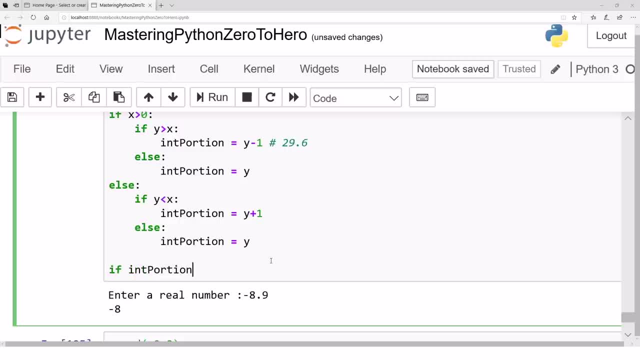 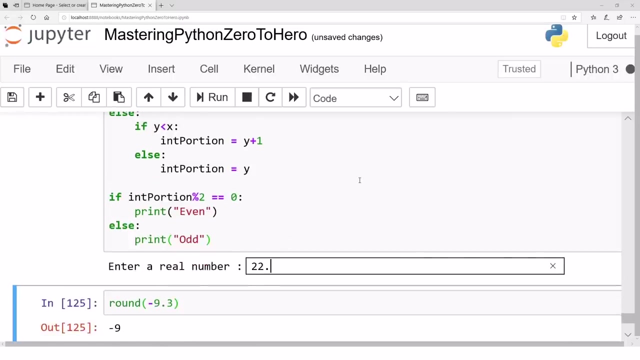 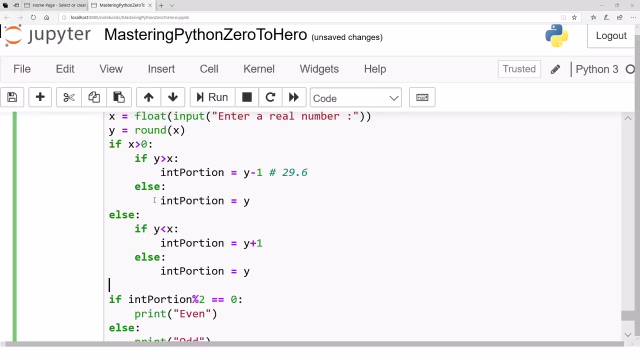 integer portion, integer portion: remainder with two. if that equals two, zero. if that equal to zero, print even, otherwise, else print odd. that's it, that's the whole program. let's see and let's see how is it running? let's say 22.6, it's even. let's say minus 87.3, that's odd rate. so you see the power if, condition and 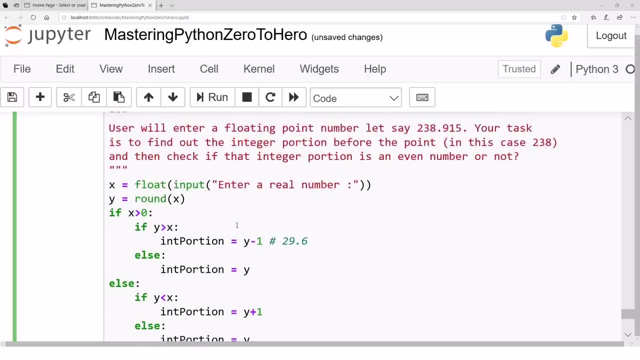 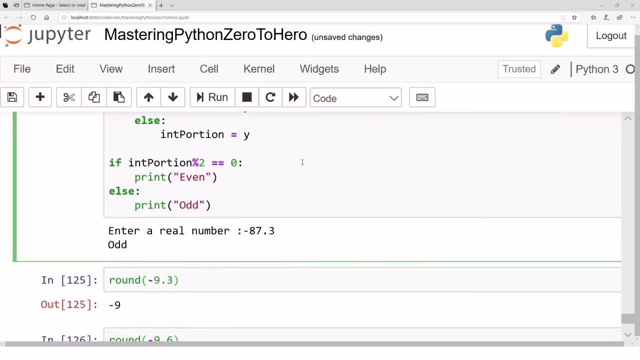 and how can we think in writing these programs and stuff like so? that was a lengthier video, I know, but I guess you get a very good look and feel of of if, conditions and thinking and building a logic and all that stuff. so in the next video we will start loops. so that's a beautiful structure. hope to see you. 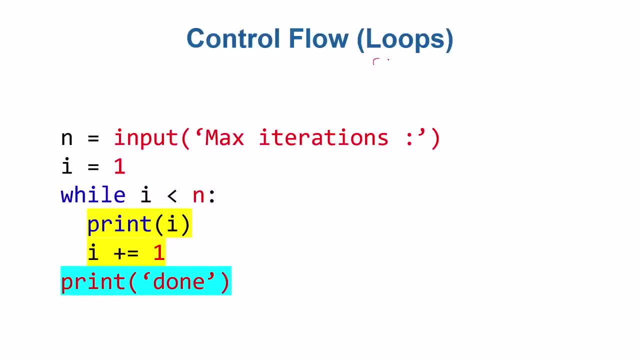 in the next video. the best way to understand loops is to think about in a repetitive structure or repeating structure. let me let me give you an example, and we will. we will dive into this code in a while. the example is: let's say user gives you a number, let's say integer number- and you 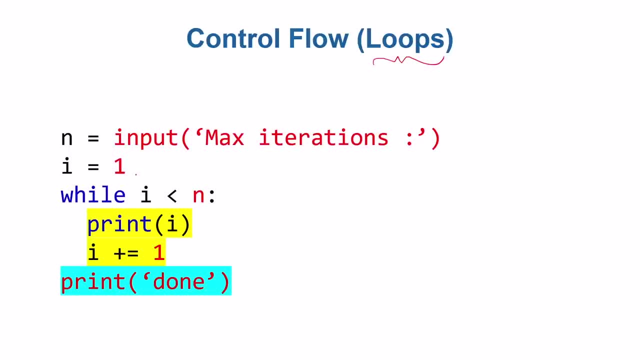 want to print all the numbers. you want to print all the numbers. you want to print all the numbers, all the numbers till that number. let's say you start from one and you keep on moving and printing all the numbers as long as you reach that number. so, for example, if user enters, let's say five, your 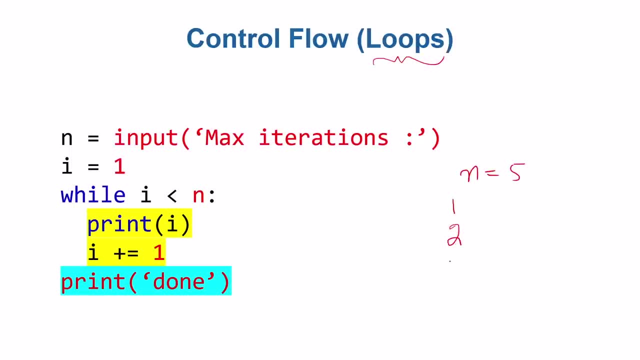 goal is to print one, then print two, then print three, then print four and then stops, then stop just all. or let's say, if user print, if user enter, let's say three, then you print one, you print two and then you stop. this is easy: if user in enters an N, we can just print. we could have written this: 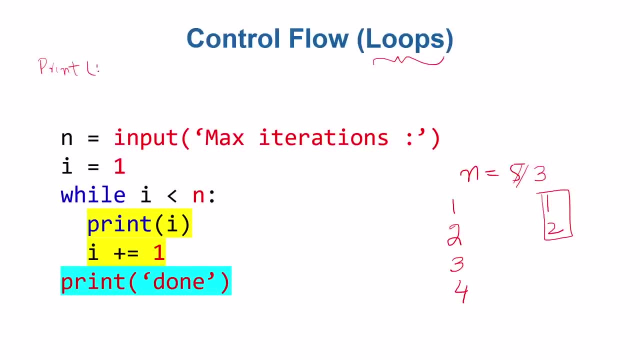 thing: print, print, I. let's initialize a variable I with one, print I, and then I equals to I plus one. or in Python we can write this quickly: as I plus equals to one, that means I. that means in I store I plus one. this is the short form of writing this, and then after that you just 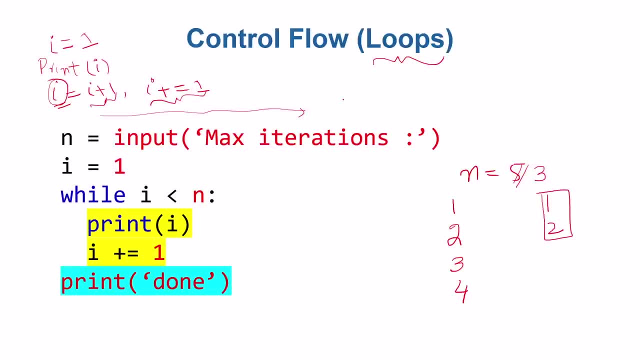 apply an if condition. for example. here you can apply an if condition and say, okay, if i is smaller than n, you keep on printing, and after printing you just increment again this, then check the if condition and keep on moving. well, that is feasible. if n is five or n is three, what if? if n is? let's. 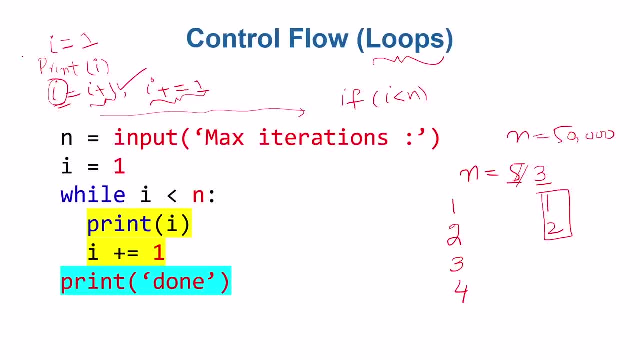 say fifty thousand. you know i mean you're writing all that structure again and again and again. i mean that's a whole lot of code. well, the loops are just a solution of this kind of structure. when you want to perform same kind of task again and again, the loop gives you the facility to do. 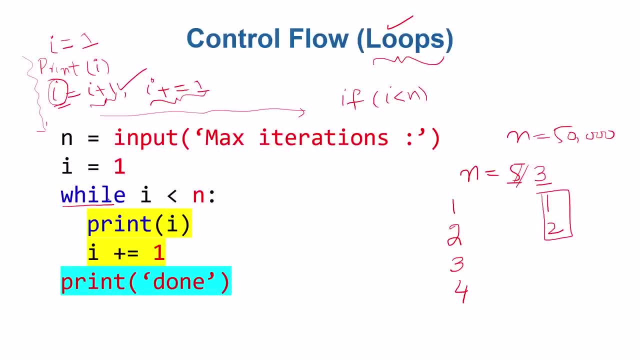 that, for example, let's just consider a while loop. this is again a condition similar like a condition in if condition. like like in if condition, you evaluate this boolean expression, that that's an expression that results a boolean value. while this condition is true, you will stay in this block and after executing whole block once. 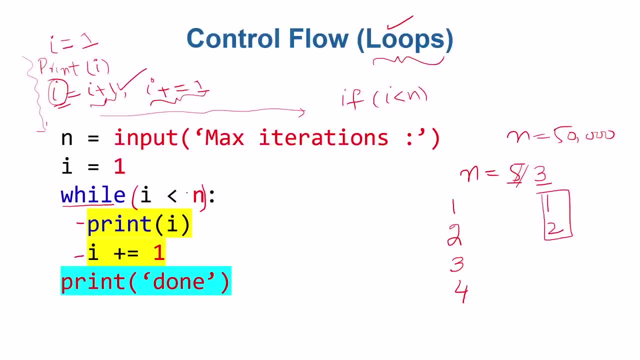 you check this condition again. if this condition is again true, you will dive into this block again. then check the condition. dive into the block. then check the condition. dive into the block. as long as this condition stays true, you stay in the block. you, you move inside the block. 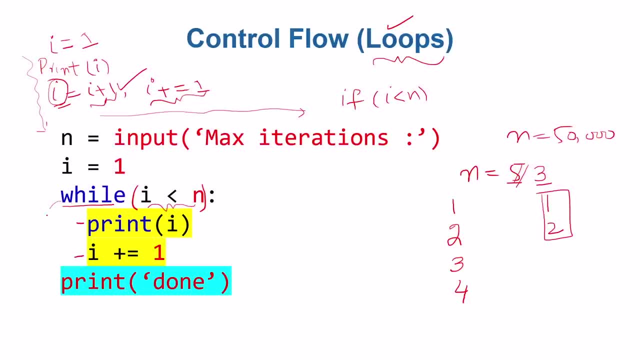 once this condition is false, then you exit this while loop, then the loop terminates and you move on to the further processing. just like in if condition, just like if conditions, if, if the condition becomes false, you exit that if condition and you can move on. moved on. so, in this particular 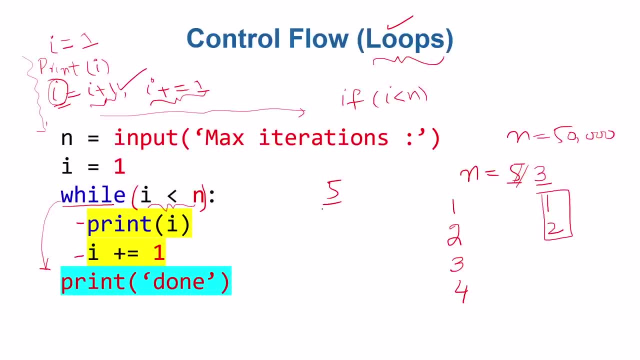 case, for example, if n is 5, let's say: if n is 5, user, give an integer number that is 5, i is equal to 1. now, 1 is smaller than 5. the condition is true. you move inside, you print i the value of i. 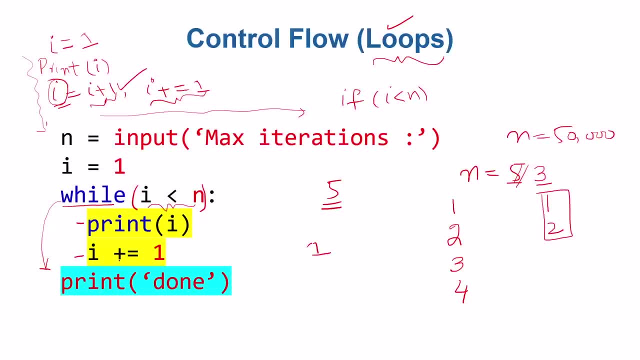 is 1, so that's what you print. you print 1, then you print the value of i, so that's what you print. you change i, you increment i with 1, that means i equals i plus 1, so i becomes 2.. now the body of. 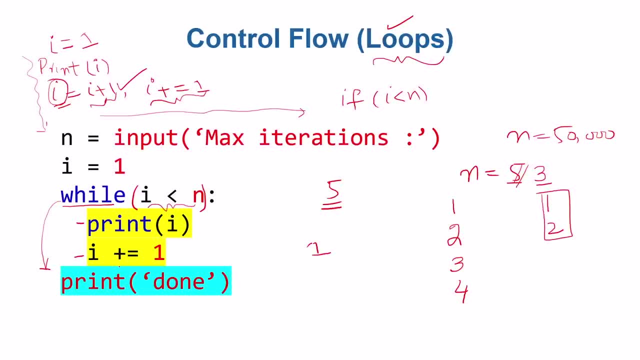 the loop finishes. that's whole body of the loop. the body of the loop can have many, many statements, a whole block of code. once i becomes 2, you move on and you check. okay, 2 is smaller than 5. yes, it is true. you move inside the block again. you print 2, then you update i. the loop body finishes once. 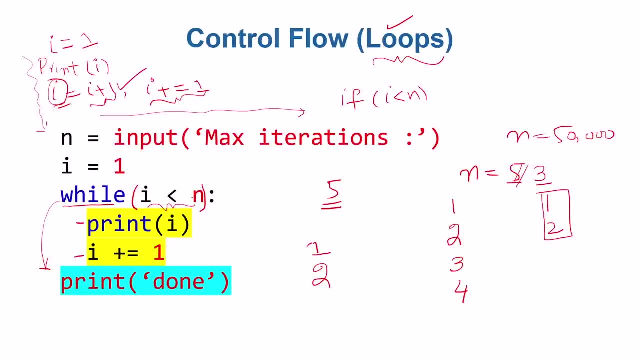 the loop body finishes, you increase it and then now you also just hold the function as true. now you you go and check the condition again whether that condition is still true or not. it is still true. the i is 3, i is 3 is smaller than 5. yes, you move inside, you print 3, you update i, you check the. 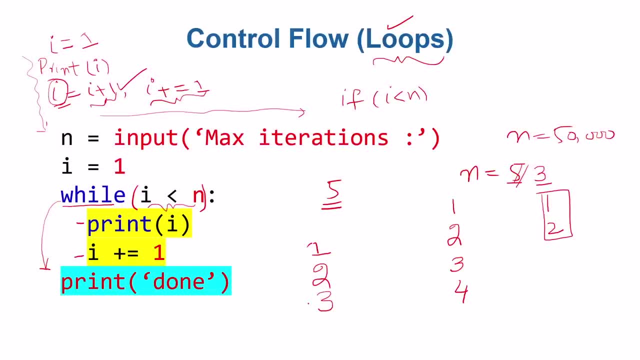 condition 4 is smaller than 5. yes, you move inside, you print 4 and then you update i and then you move on. now, 5 is smaller than 5, false. once the condition is false, you will not dive into the body of the loop, you will exit the loop and you will print done. and that's it done. so this loop. 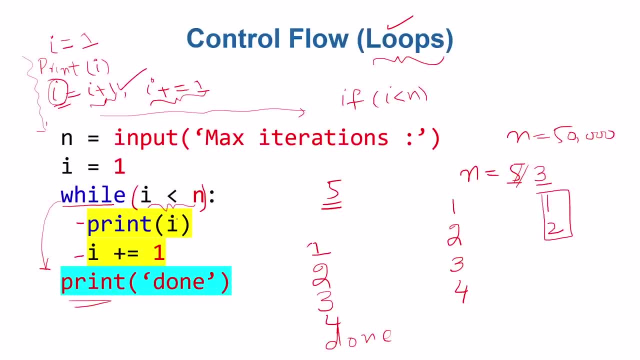 becomes very, very, very handy in, in, in applications that have repetitive structures, and in most of the interesting programs, most of the interesting problems. these are the loops that play a very huge role. so let's go to jupyter just to uh get our hands, uh, get our hands on this. 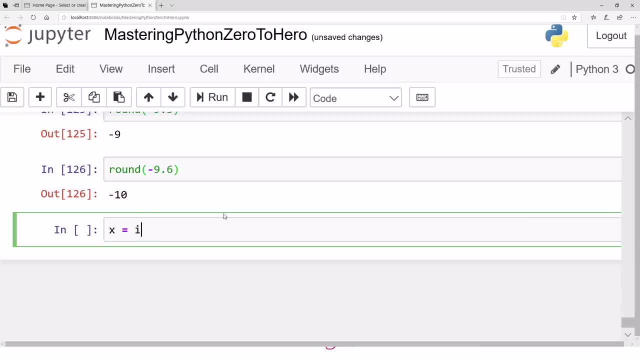 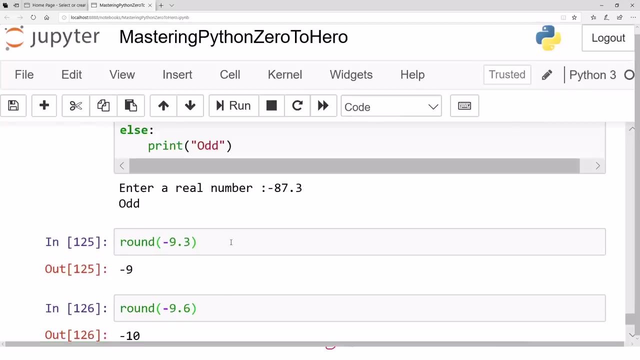 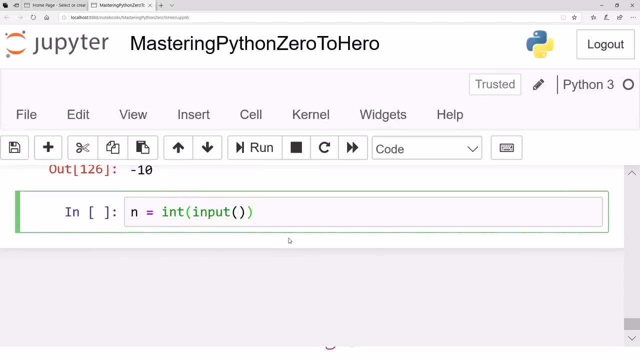 loop. for example, let's say x is uh. again let's say int or n. let's take n. n is int input. let me make this a little bigger, just to let's say that input and input is a number. let's say n. i is your certain. let's say: 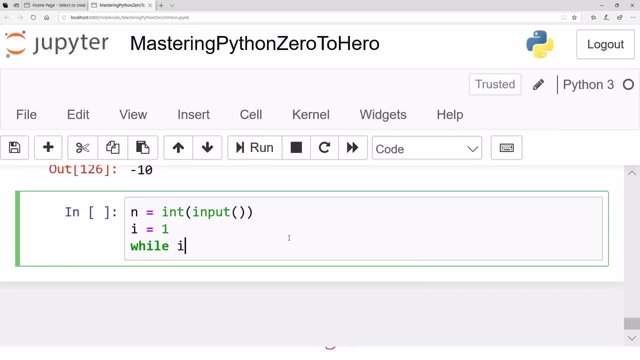 let's say 1, while i is smaller than n. you may have written this, uh parenthesis, just to just to create the readability, just to make the readability, and otherwise. i mean this is also okay, that's perfectly fine if, as long as i is smaller than n, keep doing the following you. what you do is 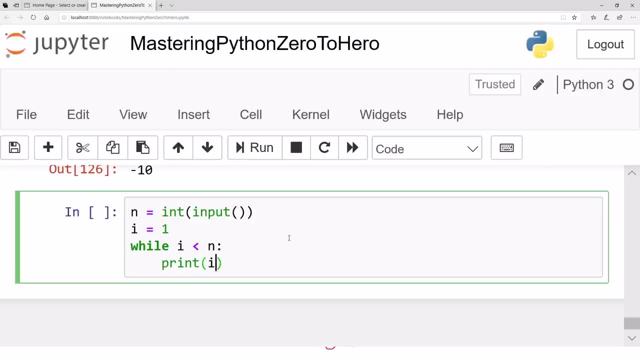 print, for example, the square of. i print the square of. i, that's a square of i, let's say. and then you say: print, for example, this is iteration number, and then you just print: i, that's the iteration number i of the loop, that's the iteration number i. 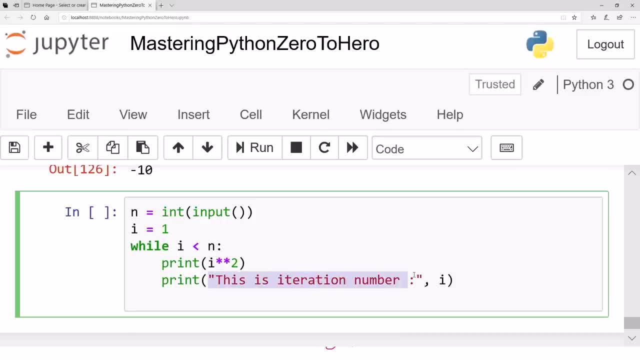 and do. what you do is bring in. this is the real plus part here is when you complete this. so let's say that you'll call this priority function and you're going to be done within this, voir id. you're going to be handle of order variable i plus one andile sum. this is just the string onde and that's a variable. its value will be printed. uh, this print function takes as many arguments as you pass. so you can. you can write a comma here and continue whatever you want to print. that's very flexible function. okay, then what you do? you say, okay, i plus equals to one. by the way, this i plus equals to one is the same as i equals i plus one. 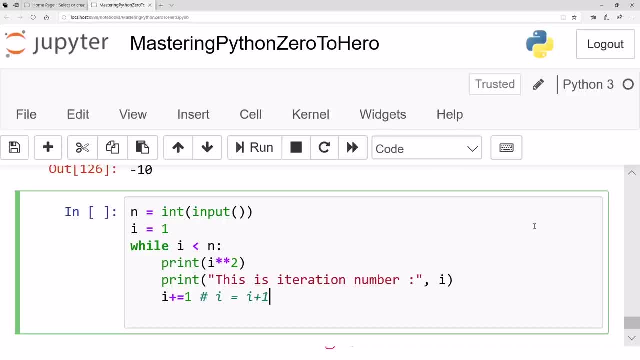 you see, i plus equals one is the same as i equals i plus one. also, I have just commented here just to explain what this is doing. If I just write i equals i plus one, that is also correct in Python, but that's kind. 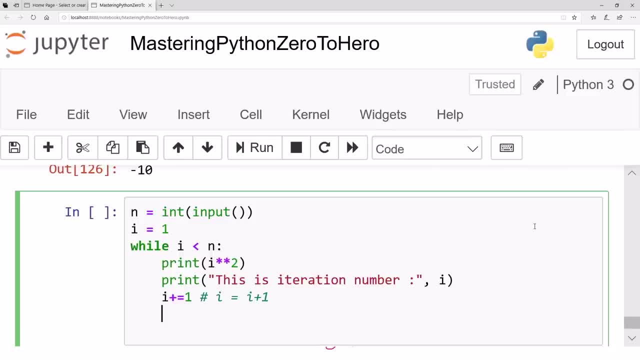 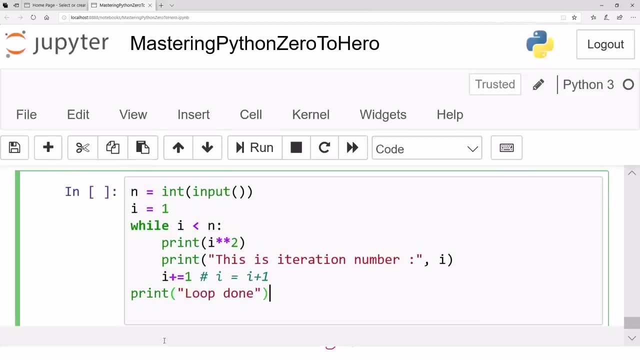 of a shorthand, And that's it. Now again, when I de-indent, I'm outside the loop. This is print loop done for example. So that's the code, for example. So let's run this code. Let's run this code. 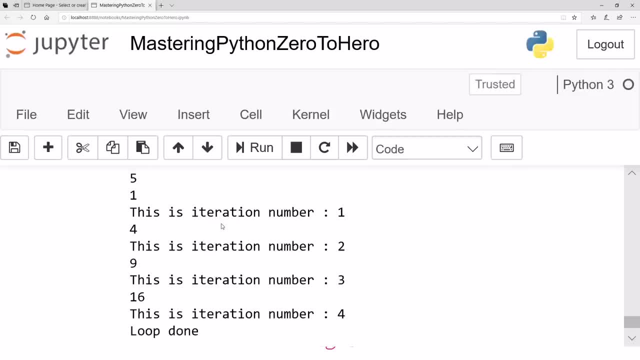 For example, let's say n is equal to five, then we have five, so this is one. this is the iteration number one. then two, square is four. this is the iteration number two. then three, square is nine. the iteration number three. then four, square is sixteen. this is. 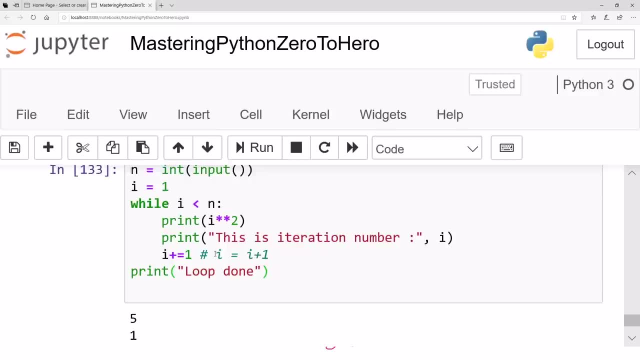 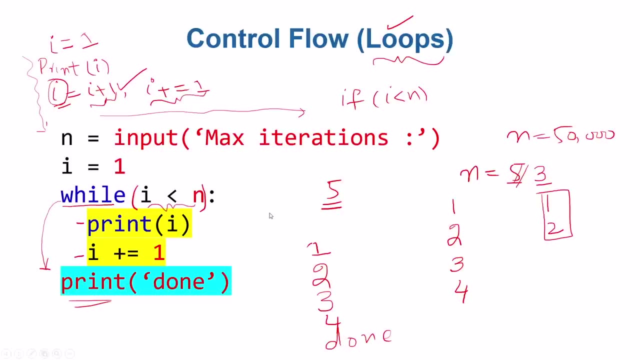 the iteration number four, and then the loop finishes. That's it. That's the first snapshot of the loop. We will continue from here onwards in the next video and I will show you more and more flavors of this loop. So hold on and wait for the next video. 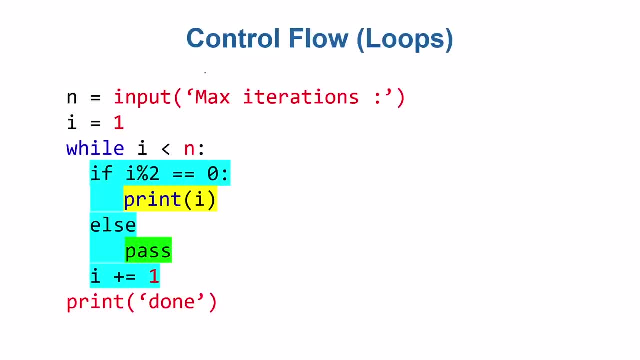 Okay, in the previous video we saw while loop and we saw one program related to while loop just printing a bunch of numbers till a particular number. Well, Well, when you are inside the body of the loop, that's a whole new. you can write whatever. 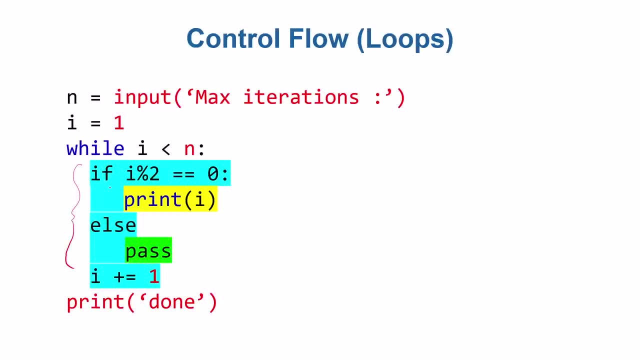 you want to write. For example, you can apply an if condition inside the body and check that at each iteration a particular decision should be made or not. For example, in this particular case I'm going to print i whenever i is an even number. 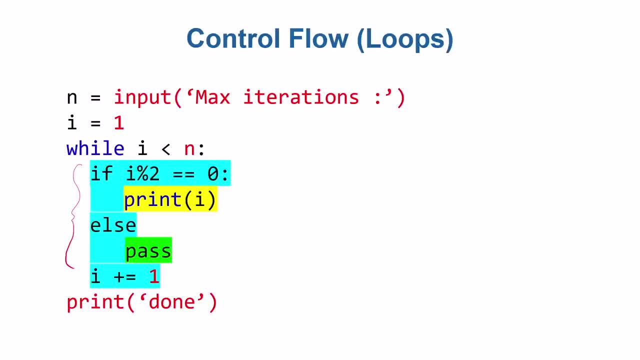 So i is some number. If it is even, then print it Else pass. This pass statement, for example, is just a statement of saying that do nothing. It is just a shortcut of writing do nothing. We could have omitted the whole else part along with this pass, and still the code is: 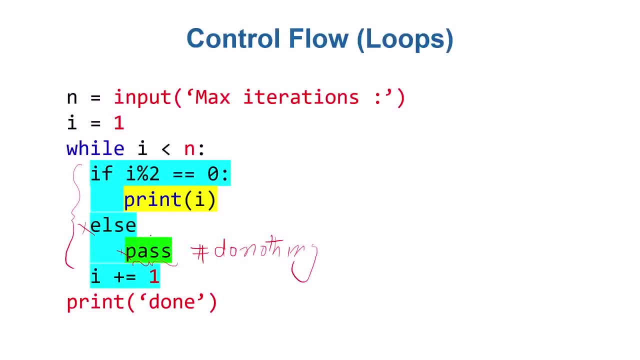 equivalent. but sometimes writing this pass, make the code readable, just So, writing this pass statement just means do nothing and just move on. If we omit else statement and we omit this pass, that's perfectly okay. So, for example, let's try it on this code. 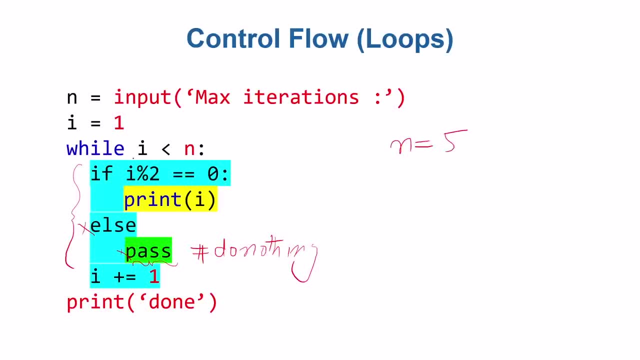 Let's say n is. let's say n is five, i equals one, one is less than five. yes, One is not an even number, So go to else part. Else means pass, which means go on And then increment i. 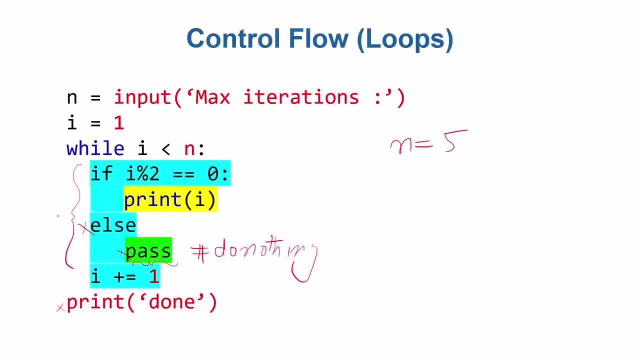 This print statement is outside the loop. This is: this is aligned with this. while This is not an even number, This is not inside the body of the loop, otherwise it should have been indented inside. Now i is incremented, i becomes two. 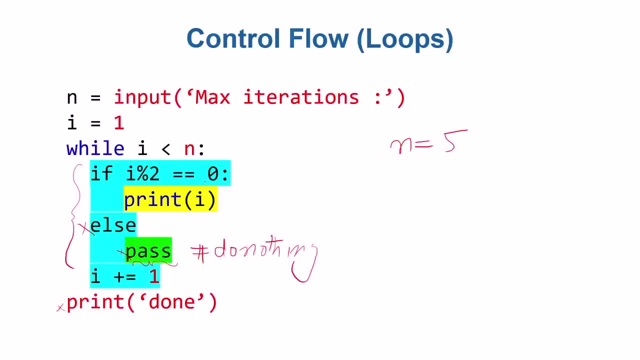 Now move back. Two is smaller than five: yes, Two, remainder two is zero: yes, So print two. So two will be printed Because if executed, else will not execute, and i will increment because i is not inside the if condition. 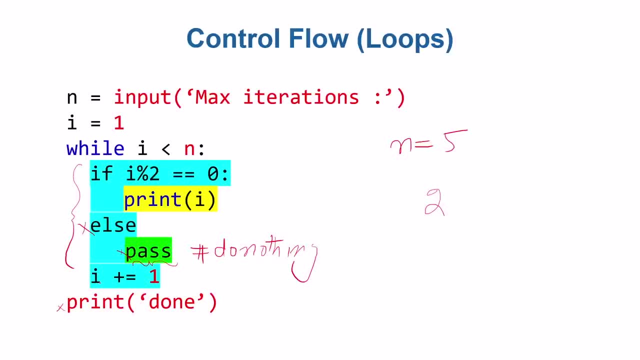 It is inside the body of the loop. So i incremented, i becomes three. you go back. Three is smaller than five: Yes, Three remainder with two is zero, false. So pass i plus one, So i becomes four. Four is smaller than five: yes. 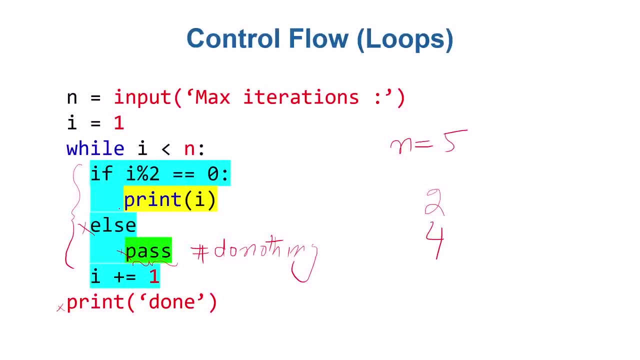 Four. remainder two is zero. yes, So print four, So else will not execute. Now increment i. Once you increment i, you get, for example, i equals five. Now, five is smaller than five, false, So you go out of the loop. 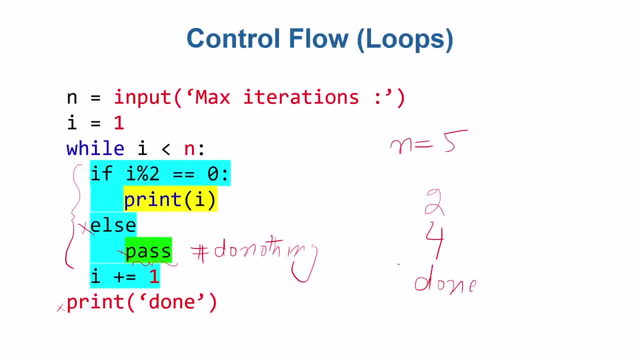 And you print done And that's what this code is. So you can have if condition inside the loop, You can have nested if inside the loop, You can have loop inside the loop, Nested loops. We will see examples of nested loops as well. 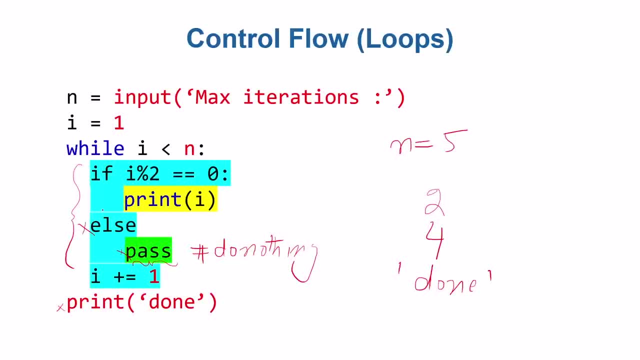 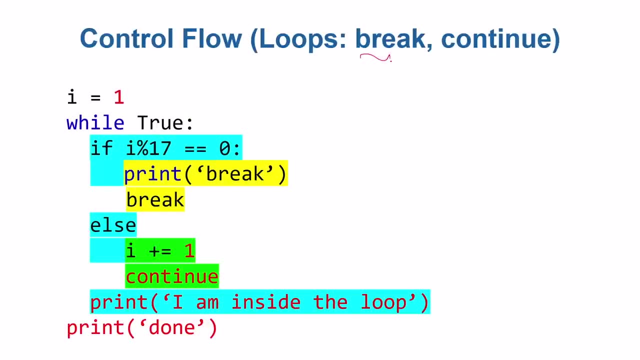 I mean that's all allowed or sometimes really required. Okay, So next, there are two important statements that are there. One is break, One is continue. I want to focus these statements because they have a deep link with loops. A break statement, wherever written inside the body of the loop, tells that exit the 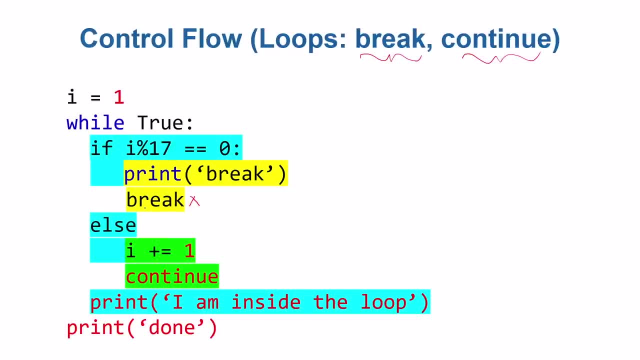 loop immediately, Whenever this break is encountered. whenever this break executes, it exits the loop immediately and brings you outside the body of the loop. That's what it does Break. So, for example, If I becomes divisible by 17 and the remainder becomes zero, you will print a break. 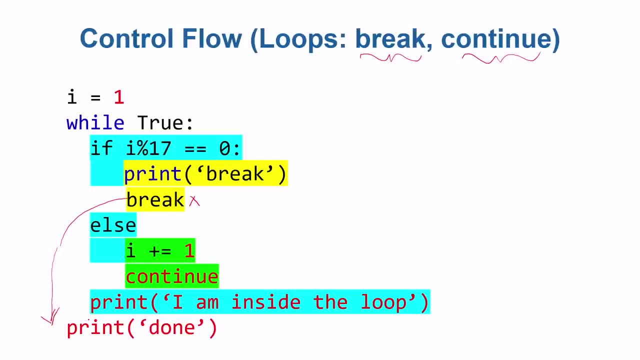 And then, when this break statement will execute, you will exit the loop immediately, regardless of what is the value of I, what are other states, whatever Break exits the loop. Okay, Great, Now the continue, Continue statements. Continue statement wherever encountered. 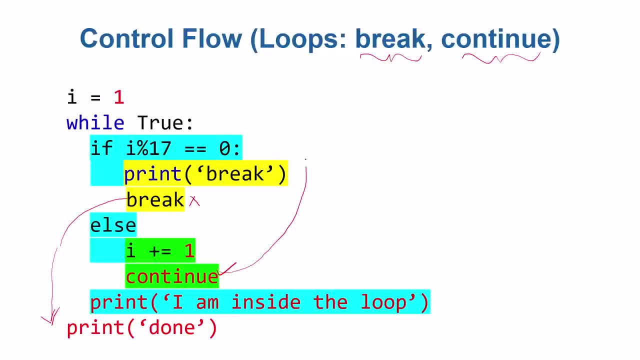 Continue brings The next iteration loaded, regardless of the remaining statements in the loop. For example, when this continue will be executed, no matter how many statements are there onwards that are there in the body of the loop, the loop will not finish its iterations by going. 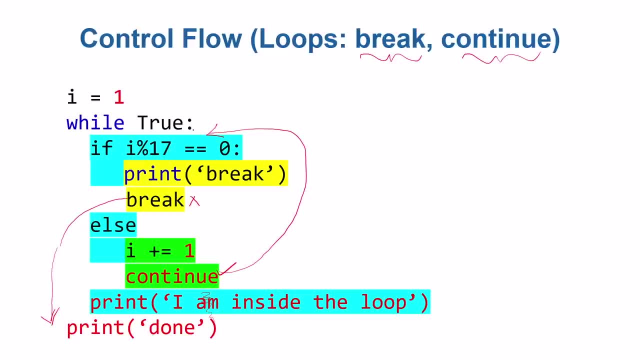 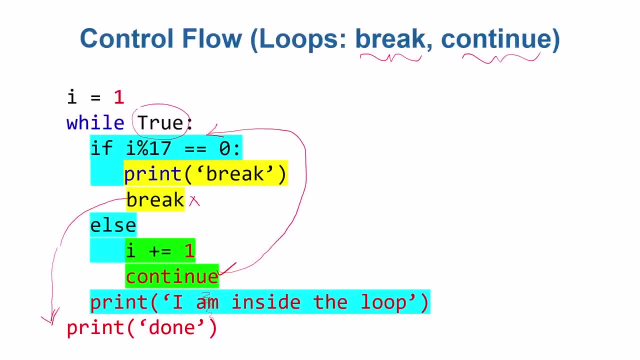 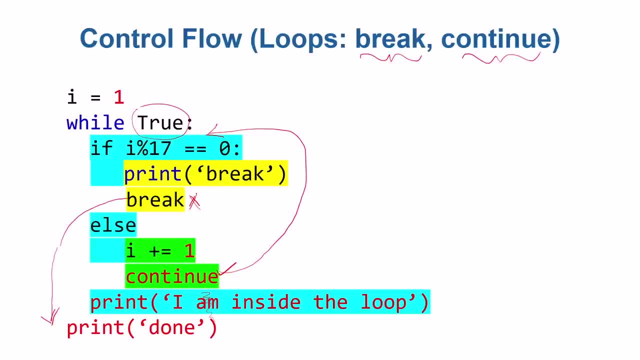 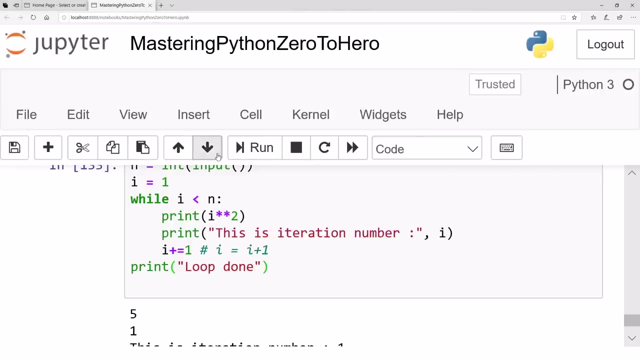 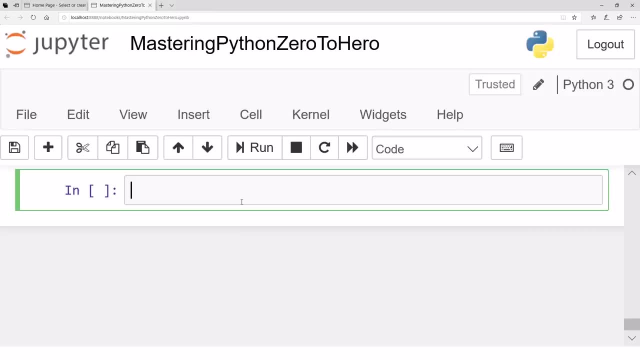 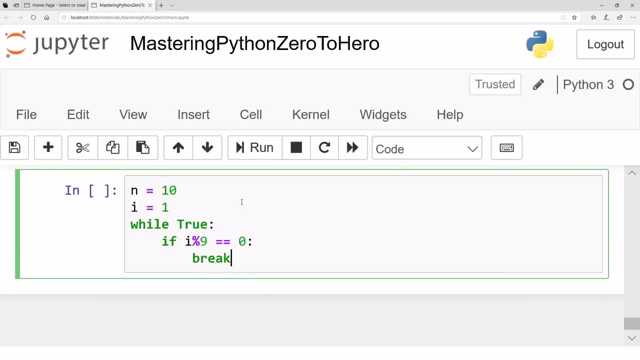 then just break the loop else, else, else. else, what you do is really you increment. else, what you do is: if I is, is, if I is not divisible by 9, then what you do is: I equals I plus 1. that's true. by the way, previously we we have written this: 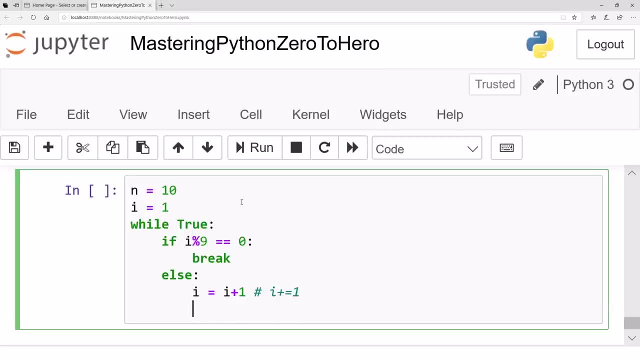 way. so either way is fine, whether you write a short form or this form, so else this. okay, and that's it for this video. That's it. The loop finishes. That's the loop. After the loop, you just write OK, print. The loop is done, Done. So let's see What's the output. The output is done straight away. 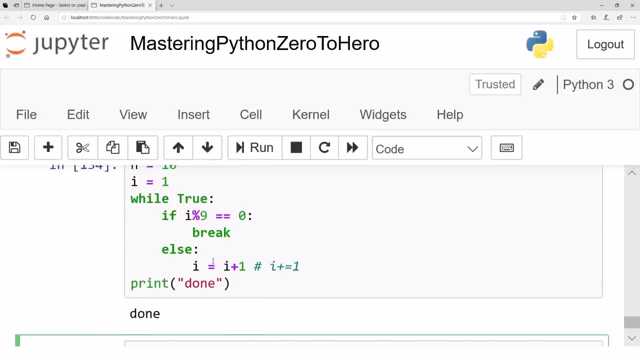 And the reason is why it is. oh, one is not one is divisible by nine. Only then you could have break. While true, why the loop? oh, it does not print anything. We could have printed some statements so that we know that we went inside the loop or not. OK, so inside. 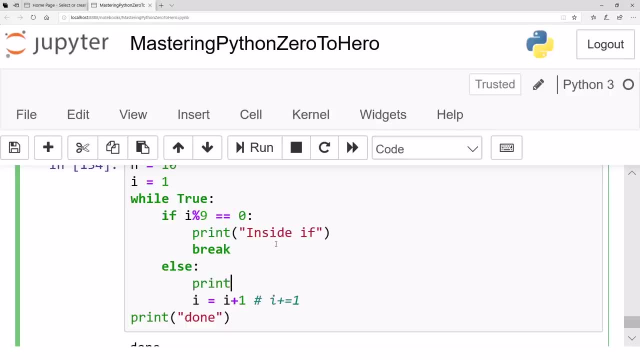 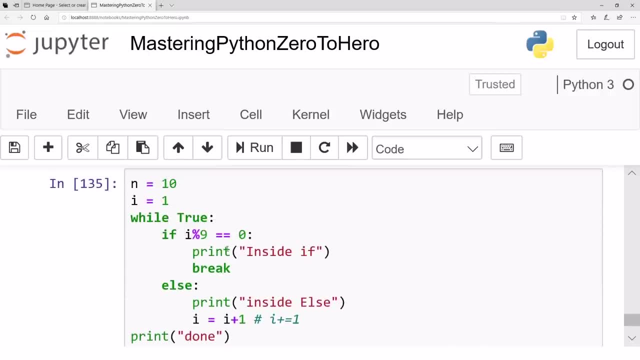 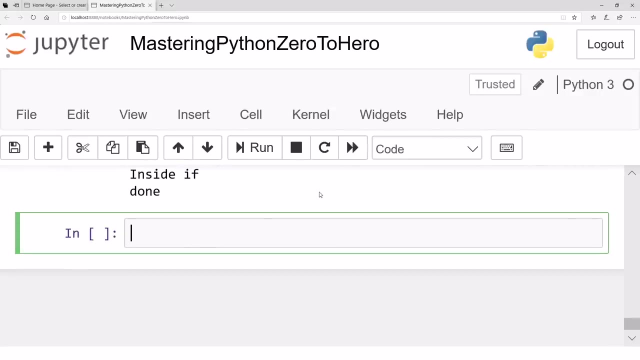 prints done. That's what this break statement does. So let's see an application of continue statement. That's, for example, just copy and paste that code into another cell and see how this continue works. So let's say we have a loop. 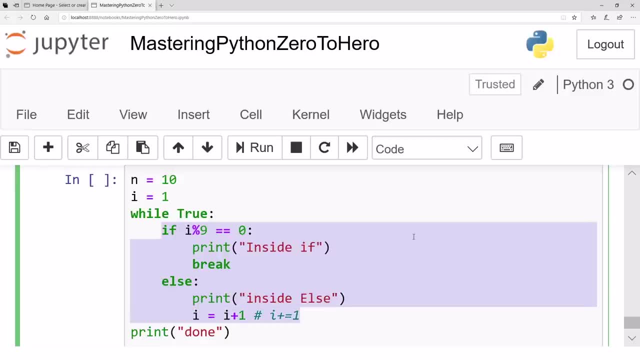 Like so. So what we say is like this: If i is nine is not equal to zero. if this is the case, if i is not divisible by nine, what you do is you take i plus equals to one, and then continue. 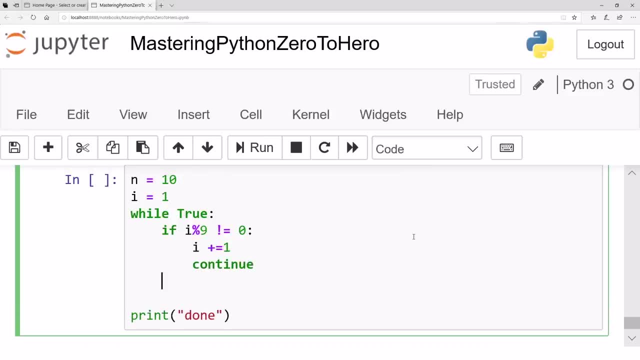 Continue to the next statement And whatever else you write here, for example, print something, print something else, something else whatever that will not be printed And once the continue will be encountered. Whenever this i is, Whenever this i divisible by nine is not true. if i is, then you continue Once this: 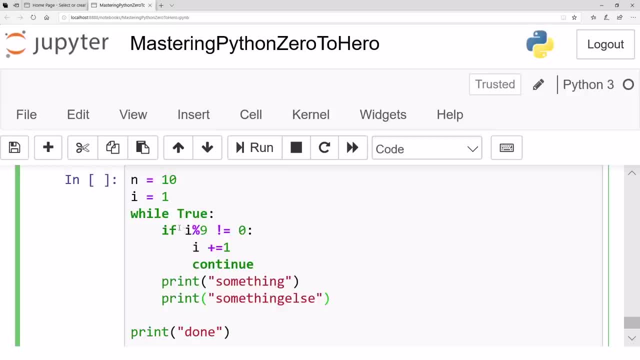 i is divisible by nine, for example, then you will not follow, then you will not dive into this. if condition Only, then these two statements will be printed, because this continue will not allow anything further that should happen. And once these are printed, let's 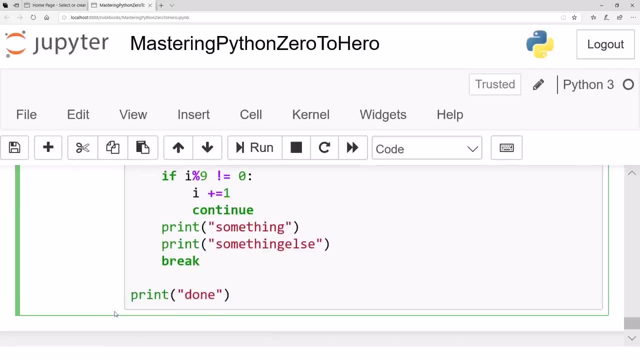 say: we break, We break our loop right there. Let's say So. if, for example, for the very first time, one is not divisible by nine, so i equals two, So continue. these three statements will not be executed. the next loop, the next loop. 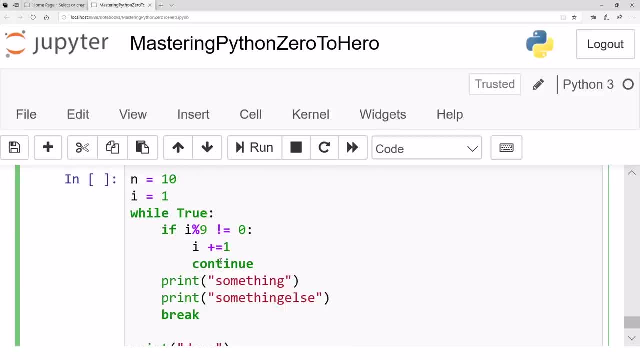 the next loop Once this if condition becomes false, this continue will not operate and then we fingerprint this statement. Then, only then, we will print this statement And only then we will break and we'll exit the loop and print the done. 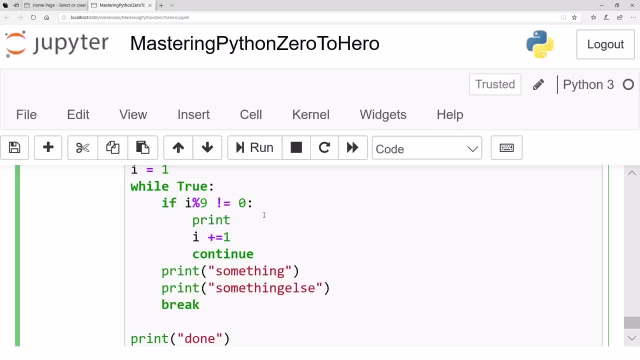 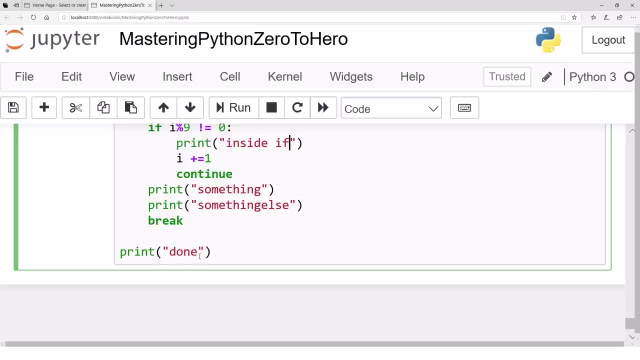 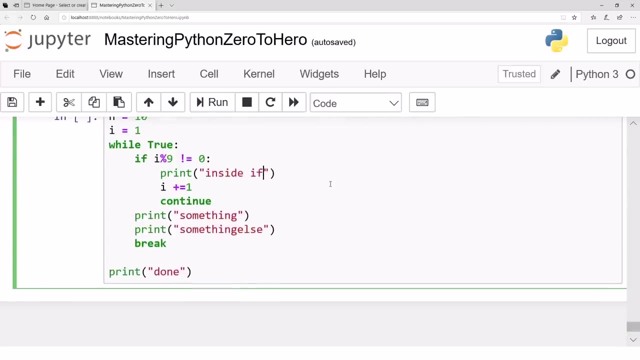 So let's print here, print inside. if so, let's run this code. let's run this code and see what happens. that's the code I should just. yeah, that's a better font. let's run this code. 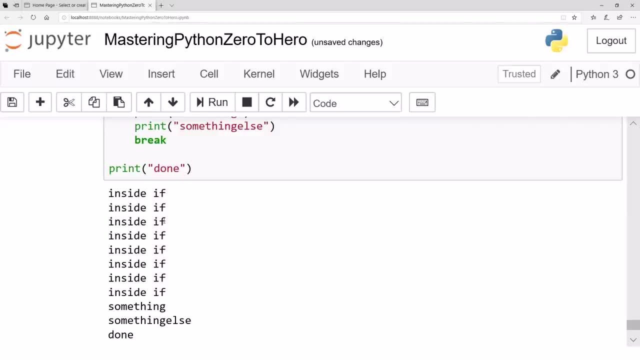 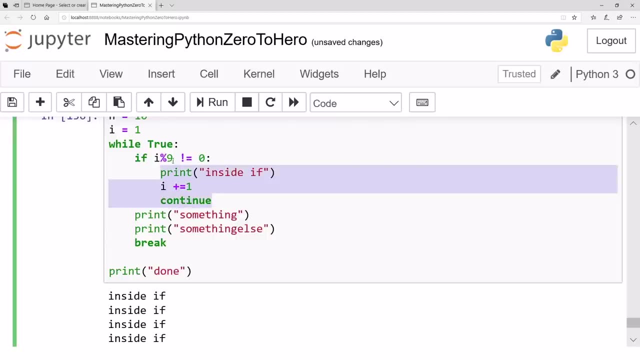 So when the code is run inside if inside, if inside, if you see when you are inside if, when you continue, when this is the body of the if condition, when if condition completes, it should print these two things. but continue is telling the cursor to go back to the next. 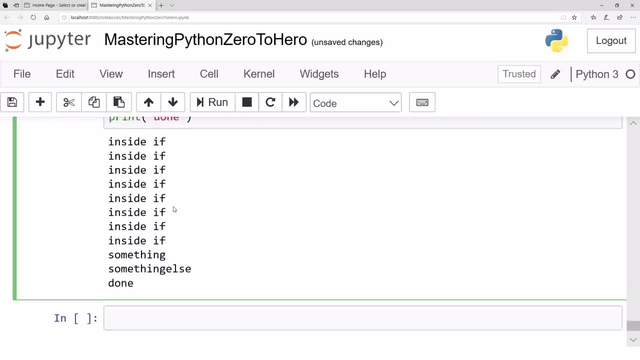 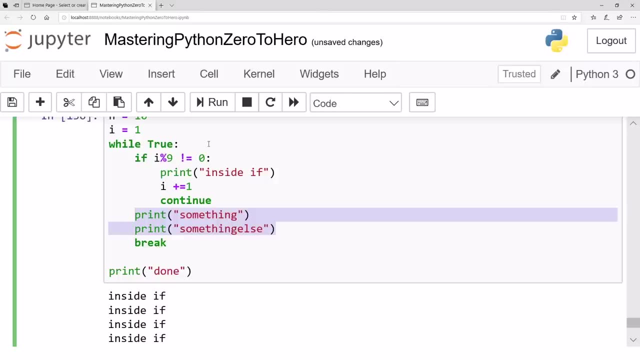 iteration and move on, And once this, if condition becomes false, only then you get this thing printed. this thing printed. if this break was not there, you then again was going to the while loop and you will be running an infinite loop. And then you have done. 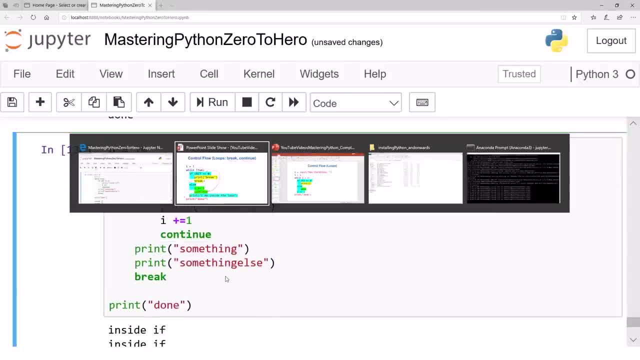 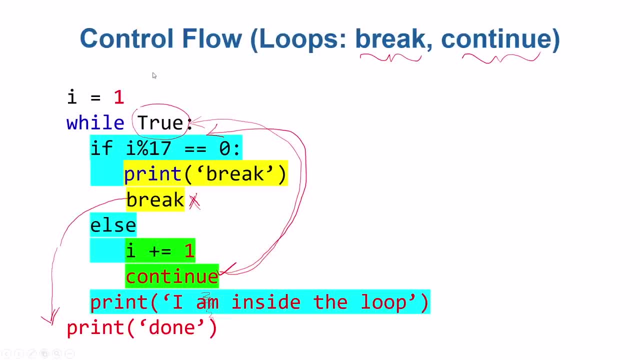 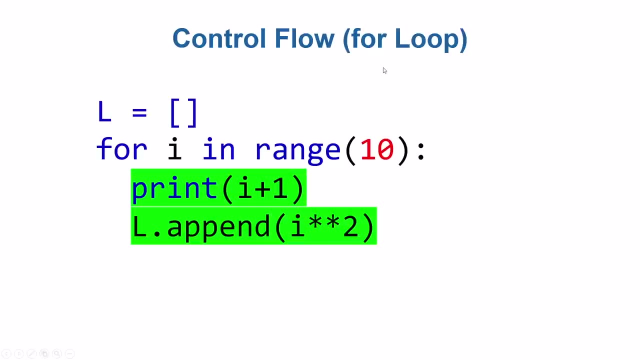 So that's what this continue and break does. So in the very next video we will see another kind of loop. here we saw the while loop. in the next video we will see a for loop- very powerful and very famous kind of loop, for it does almost the same stuff as while loop, while the while loop runs based on a 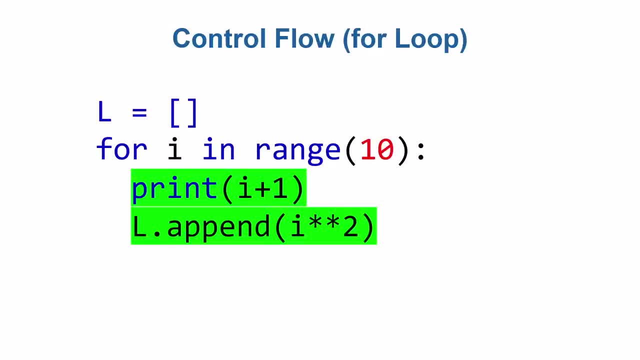 condition the for loop. it runs. It runs based on counter. it's a counter loop that many times it should run, and so on. So we will see the details of for loop and the applications of for loop in the next video. Hope to see you in the next video. 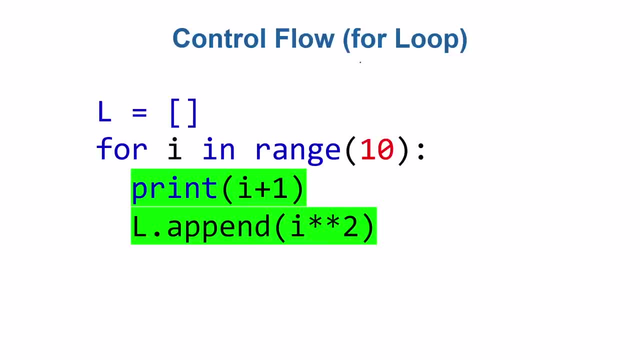 Okay, in this video we are going to discuss for loop, another kind of loop. In the previous video we saw while loop, although most of the stuff, almost all of the stuff, can be achievable through while loop, but sometimes it becomes handy to apply for loop. 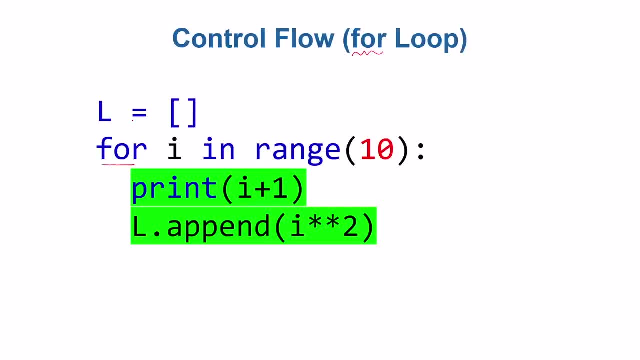 Um, So in this particular example, I am going to populate a list. so, before actually moving towards for loop, let's see very shortly what a list is, Although we are going to. we are going to explore this list in much more detail when. 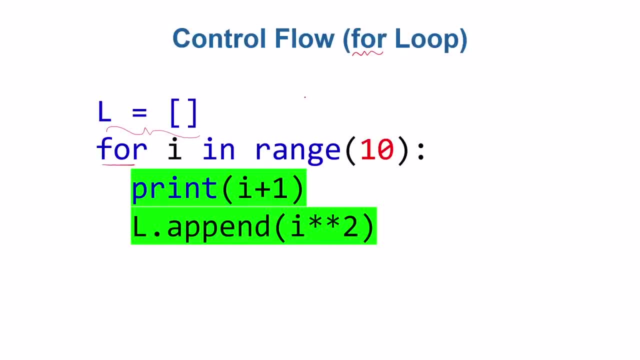 we will discuss the data structures module, but just for the sake of example, a list is a collection of different kind of elements. for example, two, three, four. that's a list of three elements. Okay, Okay, Okay, Okay. 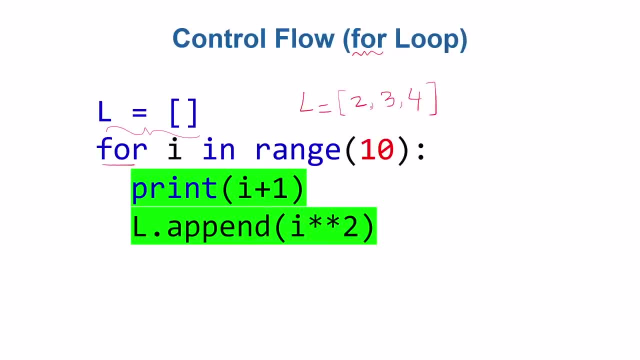 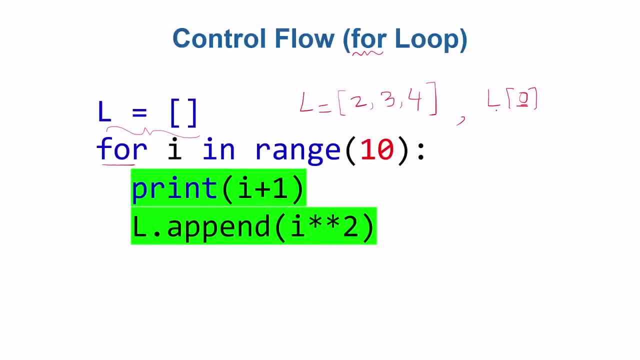 indexing. This is called the index. The index starts from zero, then index one is. so if you print, for example, print L of zero, the result will- the result that will be printed will be two. Similarly, we can append more values. 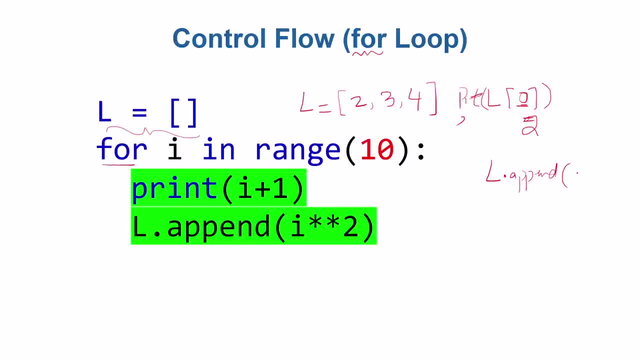 inside a list, append, let's say 53 and the list. after this append operation, the list will be having these values: 2, 3, 4, 53. we can remove, delete, update and do a lot of stuff. we will see lists in detail but just for this example, just think that list is collection of a lot of elements. 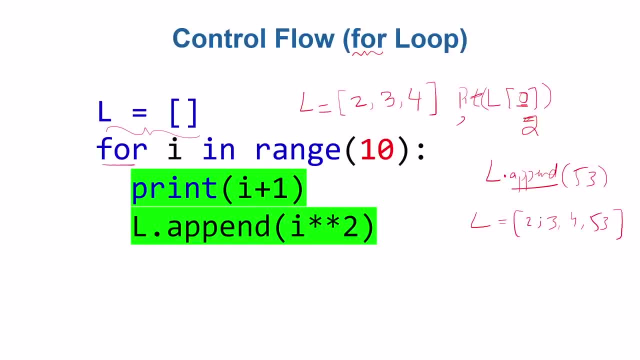 and we can add, insert more elements, we can delete elements, we can change elements and so on. or we can just initialize the list with just an empty list and start inserting elements one by one and expanding that list. okay, now, this is an empty list, for example, and for i, i is just a variable. 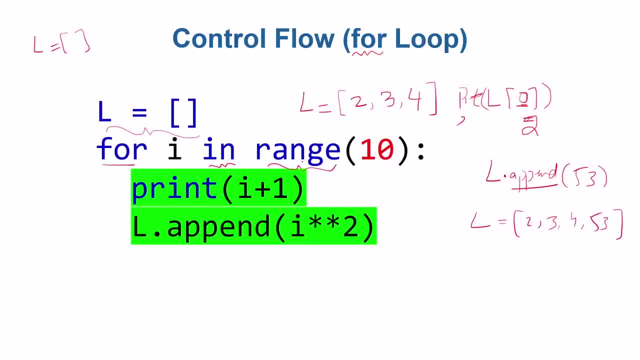 for i in this range is an iterator. range 10 means sequentially give a number one by one, starting from zero. start from zero. give them, give numbers one by one. for example, first time give zero, i will contain zero. second time give one, third time give two and so on. after every iteration the range will give. 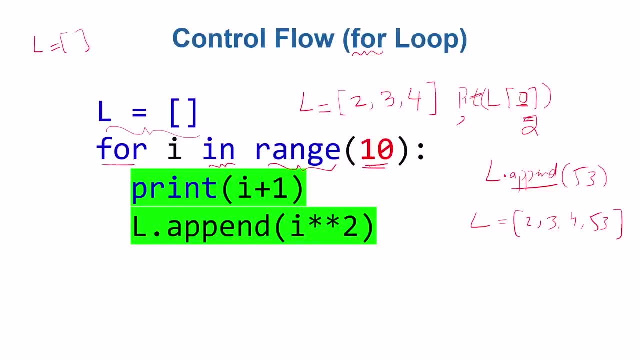 another number. as long as the numbers, they are smaller than 10. so the last number that this range will return will be nine. so whatever this is written inside is not included and it starts from zero. so as long as i is in this range, i is lower than 10. as long as that, you, that's the body. 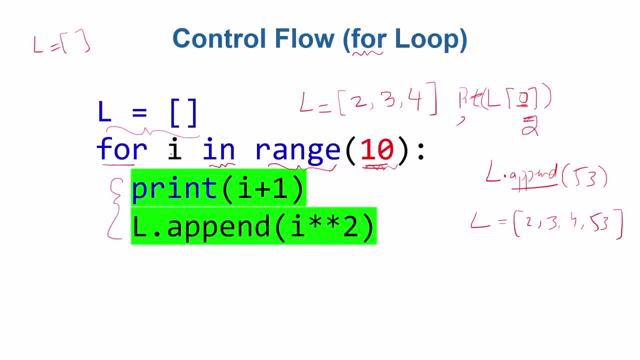 of the loop, just like the body of the while loop. so first time i will be zero and zero is smaller than 10. okay, you print i, i plus one and append the square of that in a list. then next time this range will automatically return the next number into i. 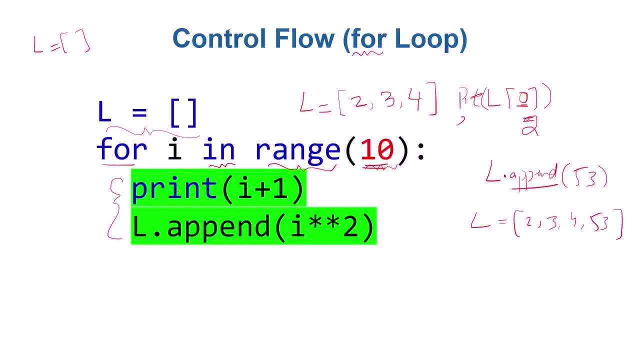 now. next time i will contain a one. next time i will contain two. next time i will contain three, four, five, six, seven, eight and nine, once the value of i becomes nine. that's the last iteration of this range. how many times there is one line- one, three, three, four, six, five- and another line and that 컷? 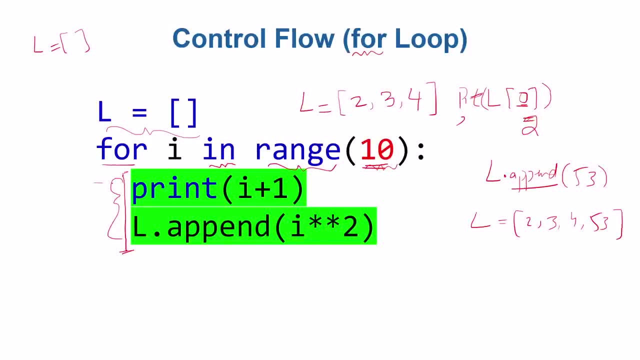 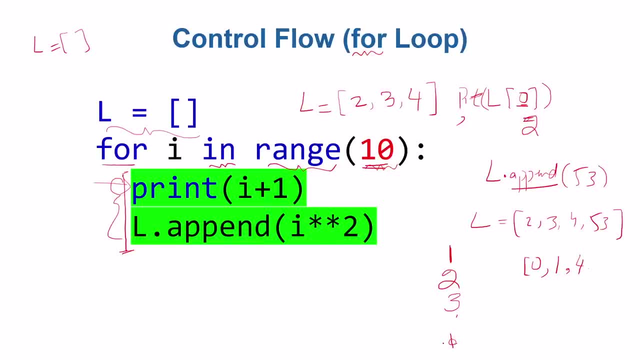 and so on till 10. here, When the I will be nine, we will print 10, and in this list we will be having nine square, which is 81,, I guess, And after that the loop finishes and we will be out of this loop. 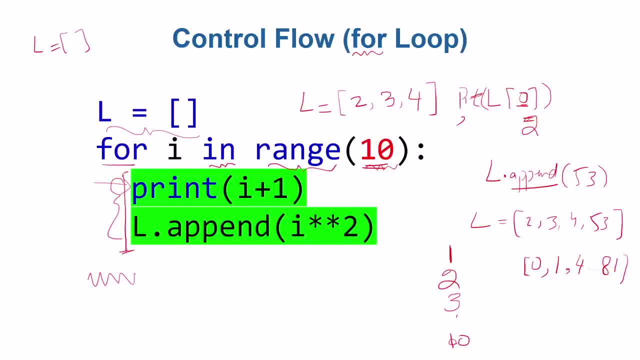 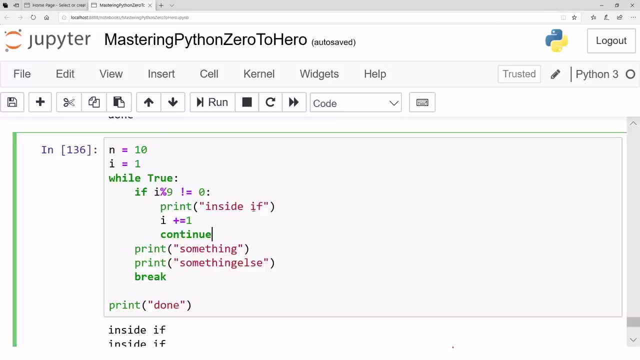 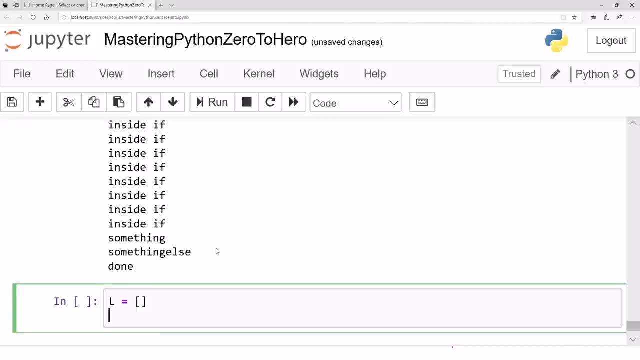 Okay, let's see example of this in Jupyter, just to get more comfortable with the list as well as the for loop. So let's see, Let's say we have an empty list. Let's say an empty list. Just consider a list like this: 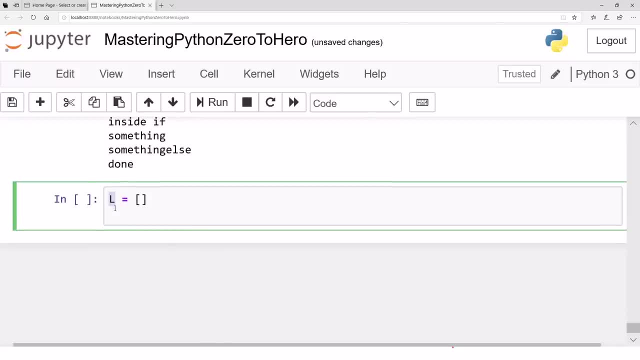 L is just a variable. You can write another variable name. That's a variable name: L. Okay, so for I in range: in is a keyword, range is a function, in is a keyword. I in range, for example, let's say 10.. 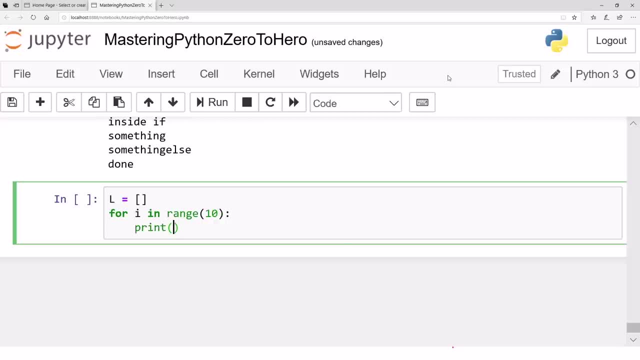 What you do is you print, you print I plus one or whatever you want to do. that's the body of the loop and L dot append. that's the function of the lists. We will see that in detail in the data structure sessions. 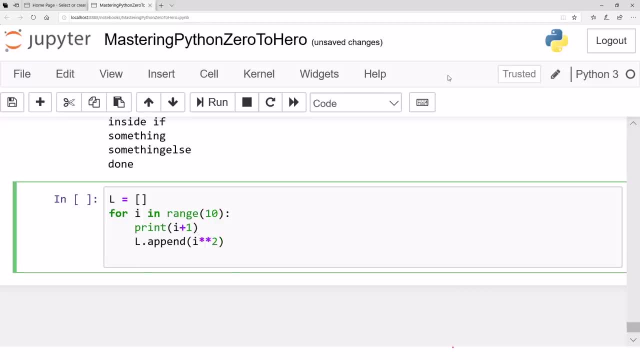 Okay it the loop finishes. when you finish the loop, just print the whole list. so let's say, print the list and you can see the result: 1, 2, 3, 4, 5, 6, 7, 8, 9, 10 and that's. 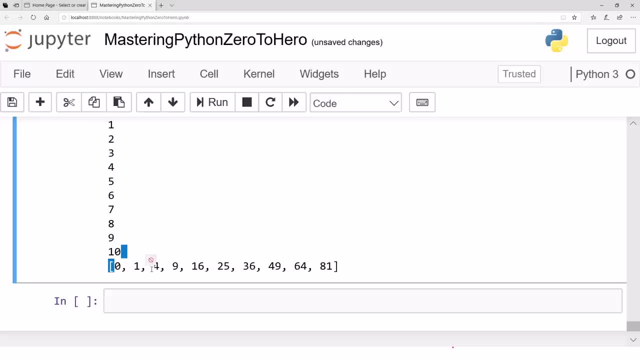 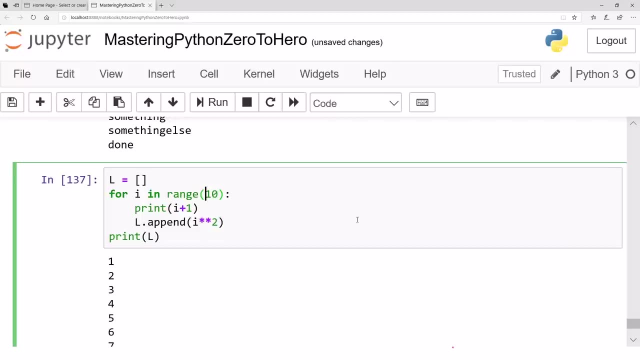 the. these are the values in the list, as, as I mentioned earlier, all these are the values. by the way, this range function actually, if what? if we want I to jump more than just one, for example, we we want I to start from 0, it reaches 10 and. 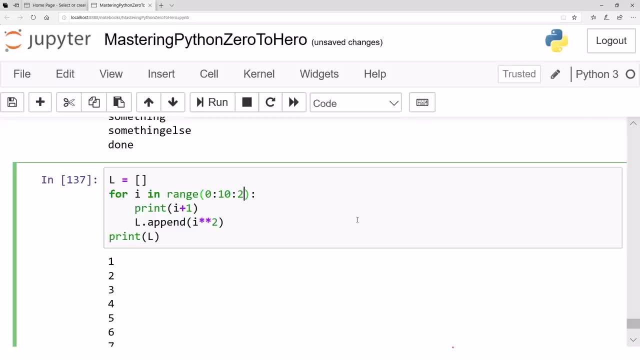 let's say, we want the jumps to be taken as 2 rather than 1 and 1, so the very first time. so that's the start location, that's the end location, which is not included. start location is included and location is not included, and that's the. 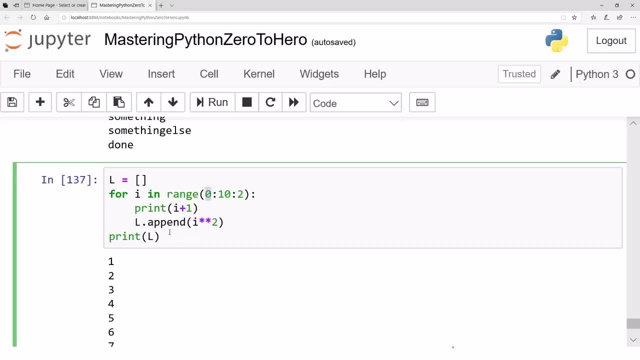 step size. so very first time I will be one. you move inside, then a jump of 2 will be taken. the next time I will be so, So very first time, the i will be zero. Then you move inside, then the jump of two. 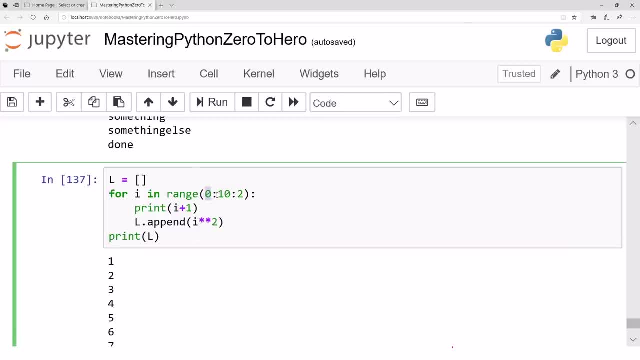 then you move inside, then a jump of two, then you move inside As long as you stay smaller than 10, you will move inside the loop body of the loop. So let's see what now printed. Let's print just i, rather than i plus one. 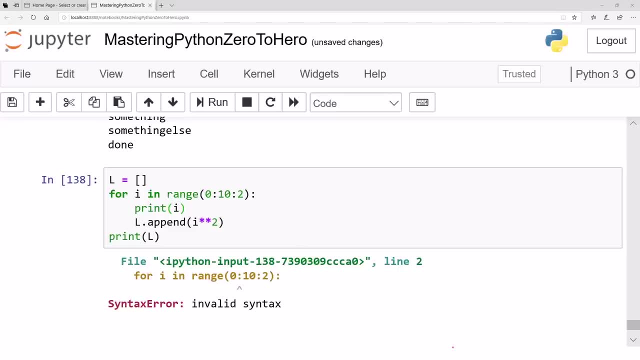 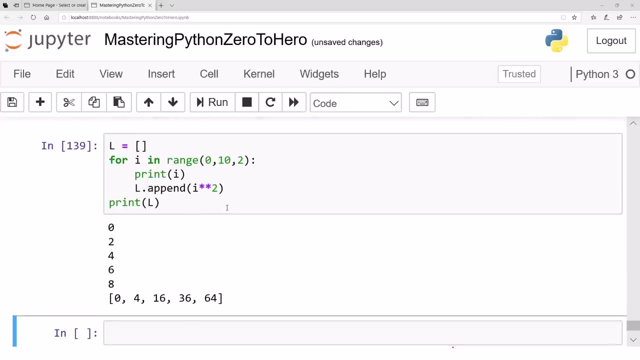 Oh, there's an error. What's the error Zero? oh, the range function does not have colons. It has actually commas. Sorry my mistake. Oh, I was just a MATLAB user once, so MATLAB actually has these colon things. 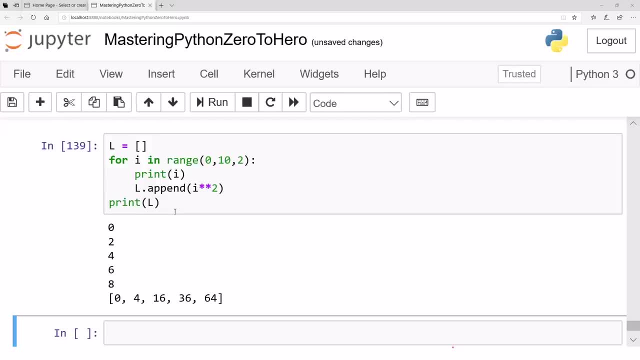 So I was just confusing MATLAB notation with this. Okay, great. So first time i was zero, Next time, a jump of two, i becomes two. Next time a jump of two, i becomes four, Then i becomes six, then i becomes eight. 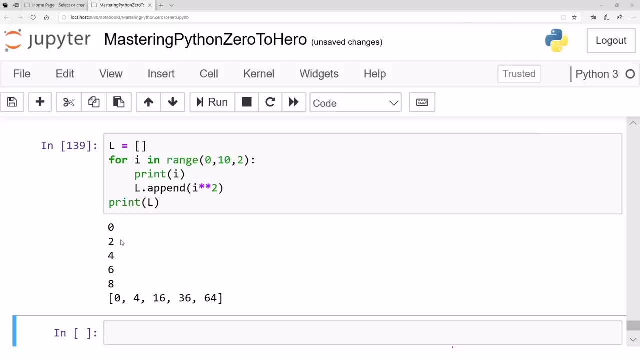 And next time i becomes 10, but 10 is not included, so you're out of the Loop and that's the squares that you got. It is not necessary that you always start from zero. You can start from one and you can take a jump. 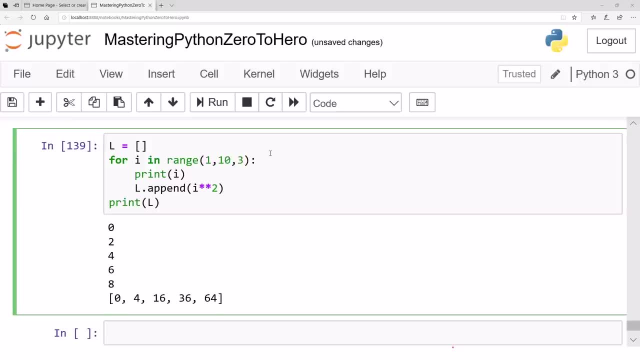 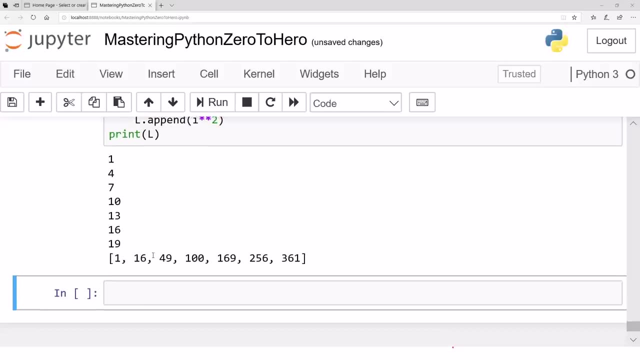 for example, a jump of three, and it's not necessary that you just reach 10.. You can reach, for example, 20. It's up to you, It's completely your choice, And in that case you have this kind of iterations. 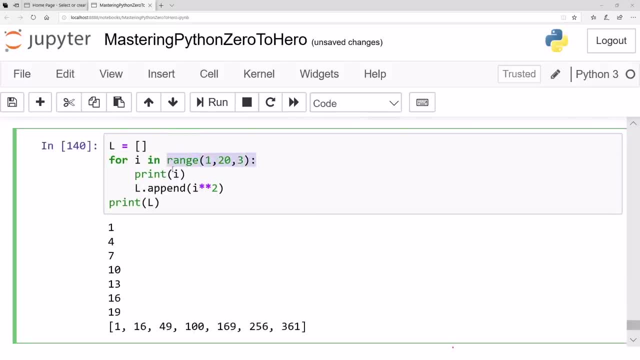 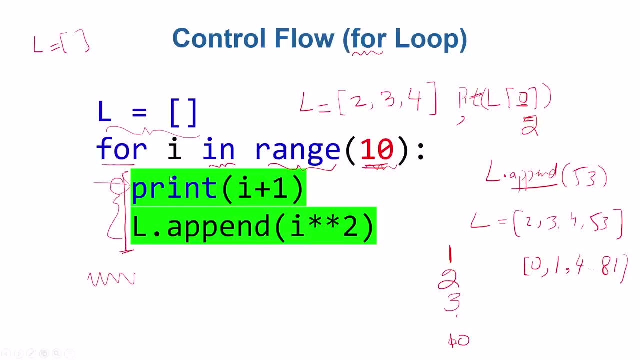 So this range function really is helpful for iterating over over a loop, body or a structure. Okay, great. So that was introduction of for loop and we have iterated here on a list. We just have actually populated a list using for loop. 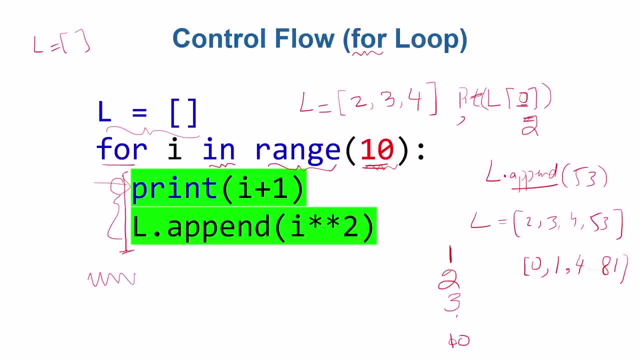 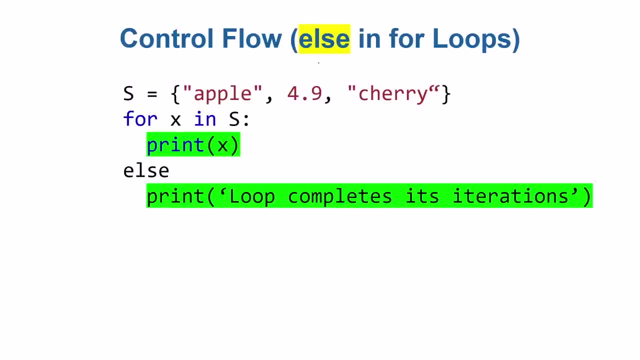 Okay, in the next video we will see more details of this for loop and more fun stuff. Okay, hope to see you in the next video. Last time we saw for loop in the last video and magically this else has something to do. 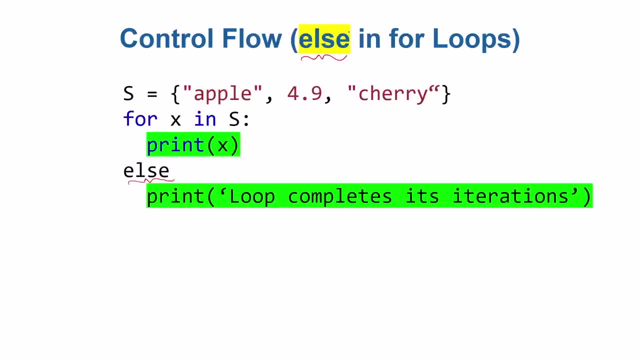 with for loop in Python. Well, this else clause makes sense for if, but in for loop it hardly makes sense. but let me try to make sense of else clause for for loop. There is an else part of for loop as well in Python. 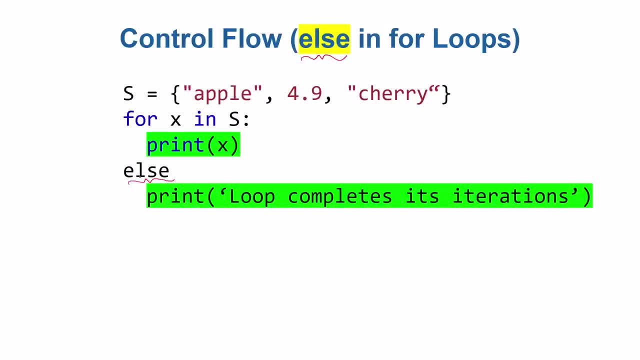 not in other languages. I don't know any other language that has this else part. Maybe there is some, but I don't know. So this else part in Python, particularly in for loop, this else part or else block will only execute if for completes its iterations. 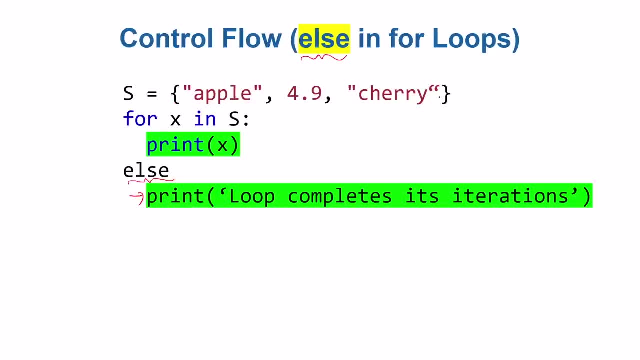 For example, this is a set. A set, like a list, is a collection. List is defined by square brackets. Set is defined by curly brackets. The set is just similar like the set in mathematics. We will see the set, list, tuples, dictionaries and many of these data structures in detail in data. 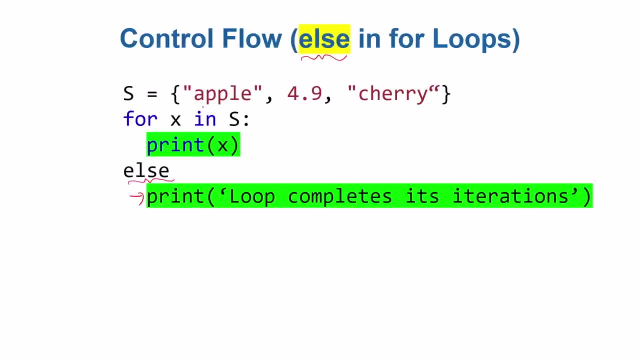 structures portion. but just I have introduced this. just consider: this set has three elements: Apple, 4.9 and cherry. Apple is one object or one data, 4.9 is one data which is a floating-point data, and cherry is one data which is a string. 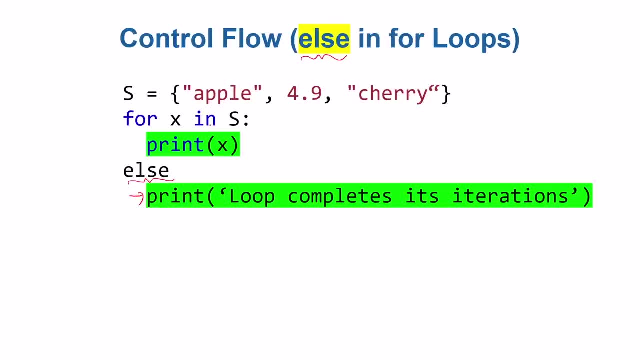 data. okay, so this s has three elements, three different elements. so now for X in this set. as long as X is in the set the very first time, the X will be Apple, so it will print Apple. next time, X will contain a four point nine as long as so. 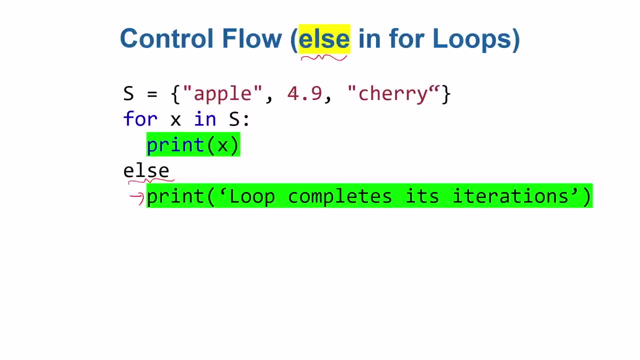 I create over this set. as long as X is inside the set, pick elements one by one and just print them all. okay, we expect that when X is Apple, when the very first time X will be Apple, it will print Apple. next time X will be four point nine it. 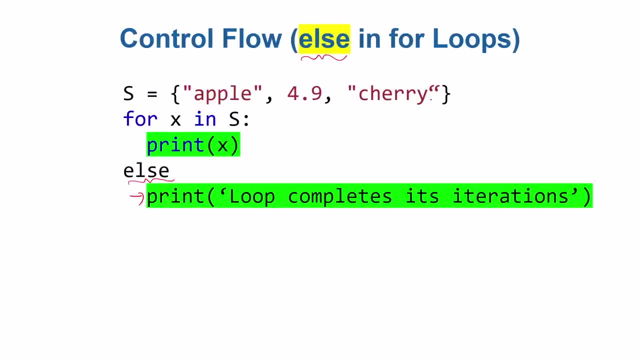 will print four, point nine. next time time x will be cherry, it will print cherry and the loop ends because there is no item in set to iterate over, because the loop finishes its complete iteration. there are expected three iterations and the loop finishes those. now the else part will execute and you will say: okay, loop. 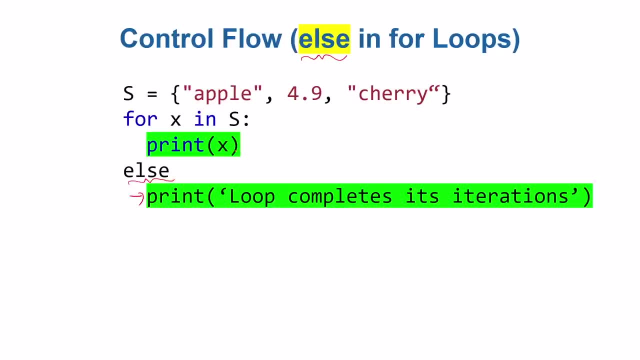 completes its iterations. well, you will be wondering in what case the else will not. else will not execute. if you apply any break statement inside the loop body, which means you forcefully- uh, you forcefully- remove some of the iterations that were going to be executed, but the loop did not completed, did not complete its iterations, then the else part will not run. 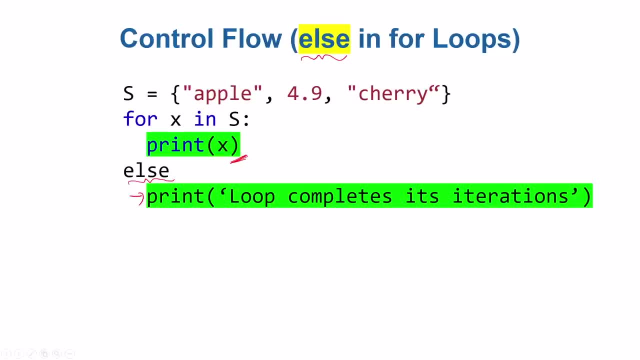 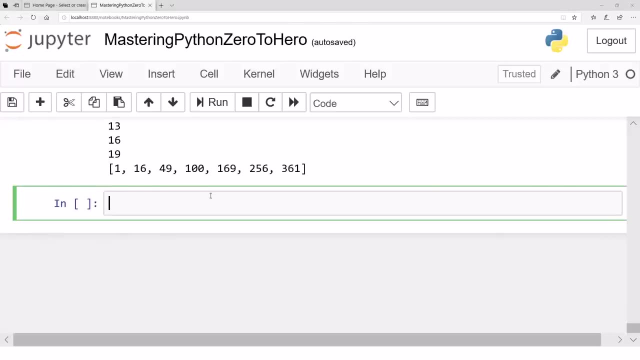 so let's see an example in in in jupiter, to get a good grip on this else. okay, let's define a set s um s is a variable name. you can have any variable name. let's say apple, or let's say 4.9, i guess. and then we was having, let's say: 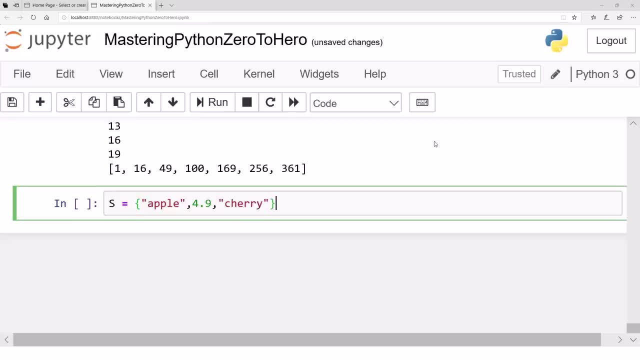 um, cherry, if the, if these spellings are correct, i guess cherry. okay. then for x in s, as long as x is in s, print x okay, fine, else print. when you finish the loop terminates with success or all iterations. it completed all its iterations and this is a statement that is completely outside the loop. 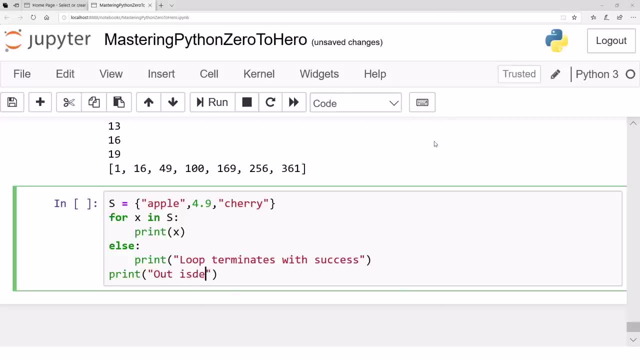 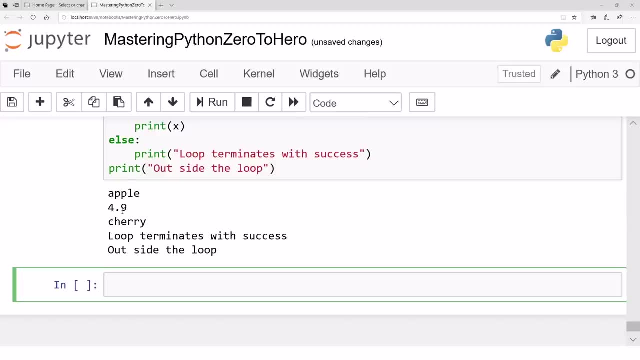 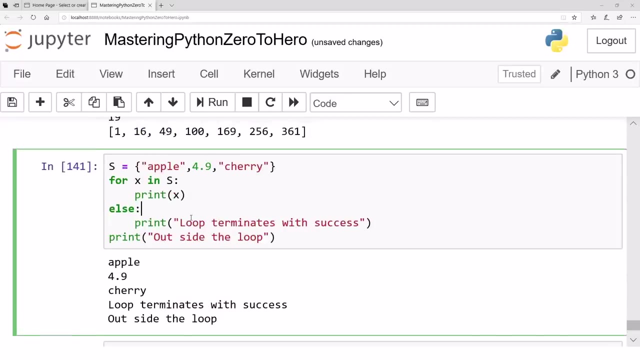 so let's run this so you can see: apple 4.9 cherry loop terminates with success outside the loop. okay, now you might be thinking in what case this uh else will not execute. okay, if, for example, uh, as long as x is in n. if i say okay, let's say i take a counter, and i take a counter, and i take a. 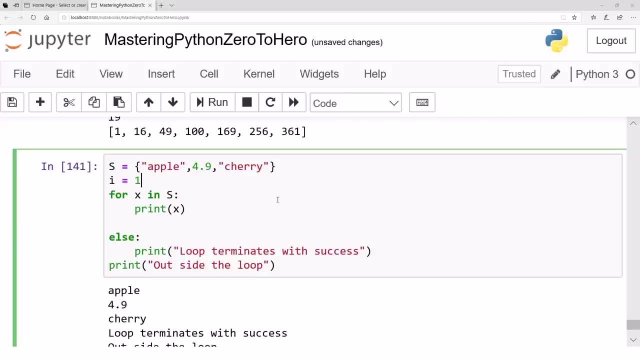 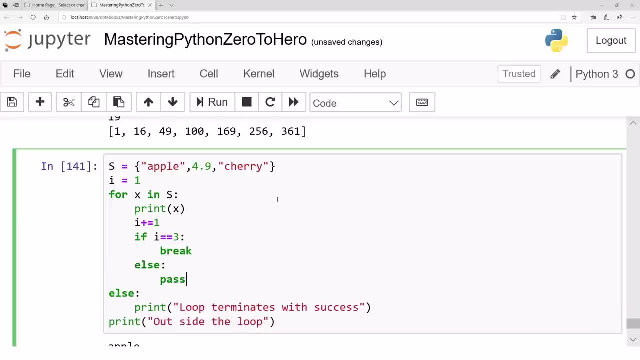 readability, else pass. now this else is else of this four and this else is else of this: if- and this pause statement is just a statement for doing nothing. now what you do. when i is equal to one, you print this: i plus equals, i becomes two. two is equal to three- false. so you pause, you move on. next time x will. 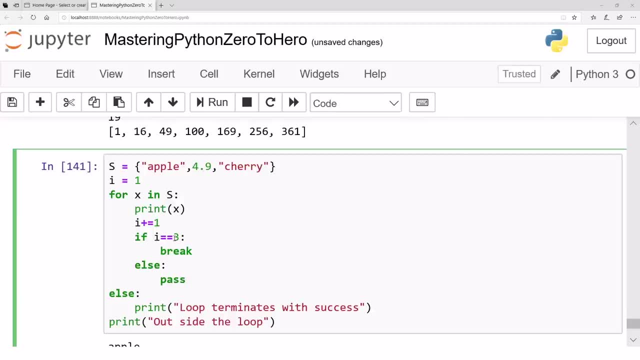 print four, point nine, i will become three, and three is equal to three. that's correct. the break will execute, which means the loop should have one more iteration, but the break just disrupt that one more iteration that should be there, because the loop could not complete its iteration due to. 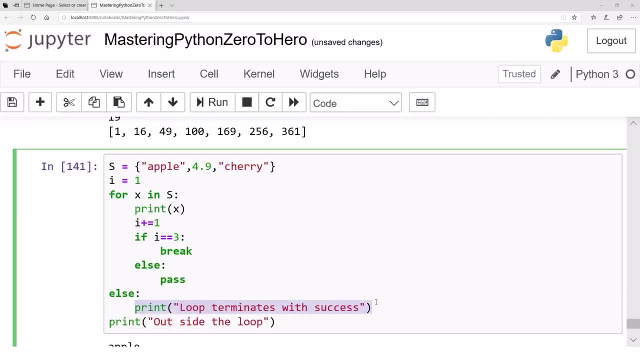 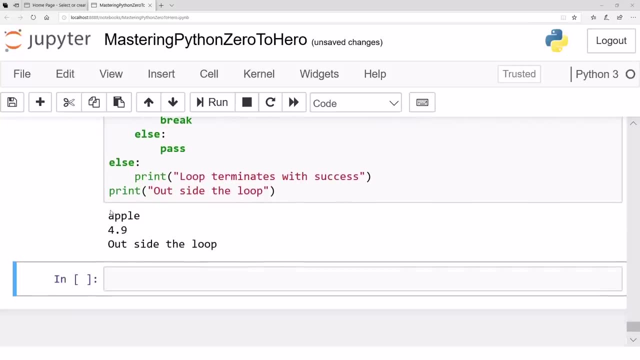 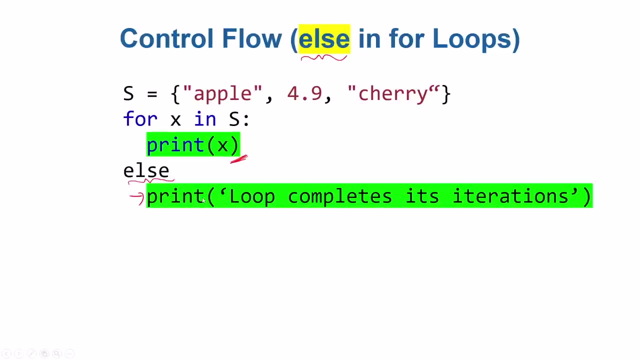 this certain condition. this else part of the loop will not execute and you will go directly outside this loop. so let's run this code and see the result, so you can see this apple 4.9 outside the loop. i would recommend also this: else is there. 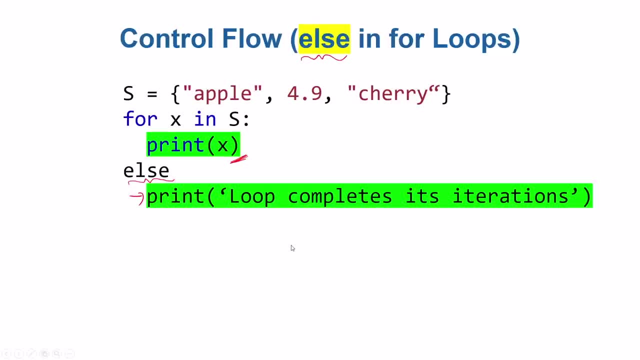 there is a example written here for for loop, but, um, i would recommend to avoid using else. uh, in the beginning, i mean, you may be confusing this else. by the way, there is a. there is a mistake here. this else should be ended with a colon here. okay, so i would recommend to not use else clause for a 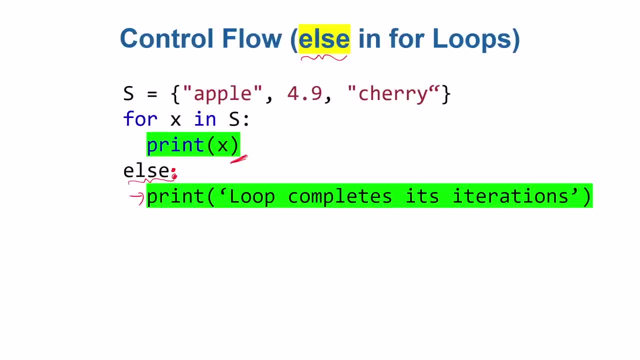 for loop in the beginning until you. you really need it, because you may confuse this else with the, with the else of if condition, and you may think something else and the programmingこれ and the program behave in a different way. so either way, if you want to use 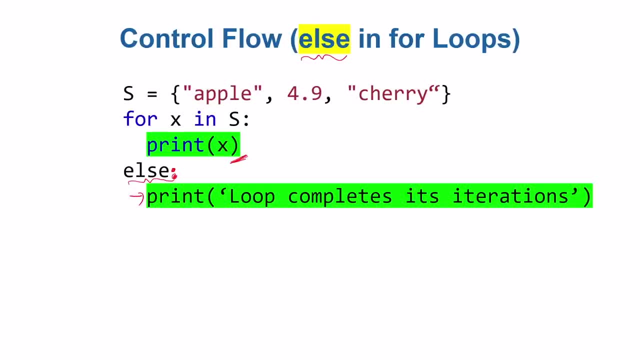 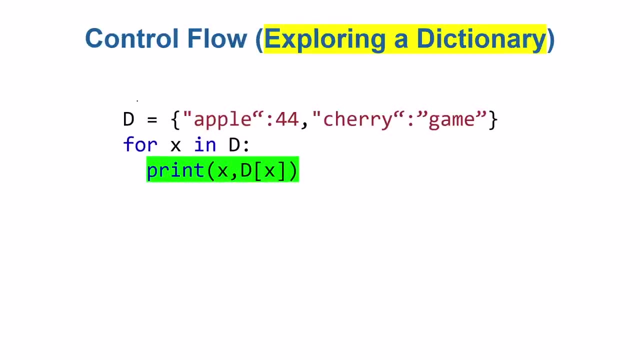 else else for a for loop is there in Python. okay, just one more example of for loop. and here we use dictionary. I'm introducing some data structures here just for fun. we will see these data structures in detail later on. so dictionary. that's a key value period is like set, but one item is consists of two. 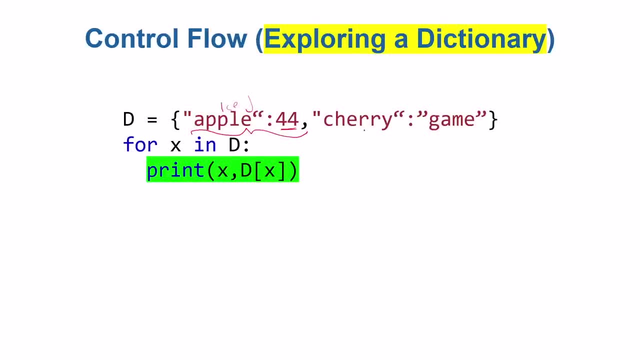 numbers. that's called a key and that is called a value. that's a key and that's a value like a dictionary. we have key and values. so now, as long as X is in X, X represents two key and D is our dictionary and D of X represents to. 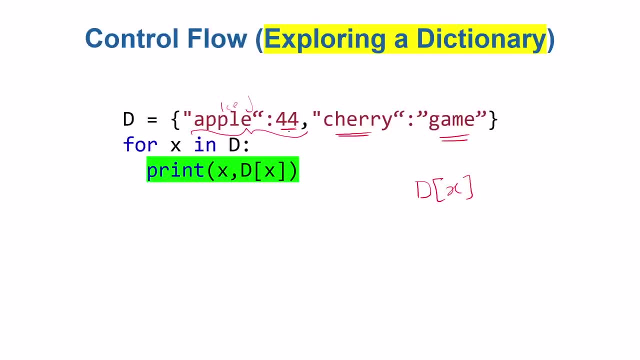 whatever value that X points to, for example, Apple is a key that points to 44. cherry is a key that points to game. for example, if I write D apples, you apple, the result will be 44. similarly, D of cherry, the result will be game. okay, so let's I create over this dictionary using this for loop. all am I showing you? 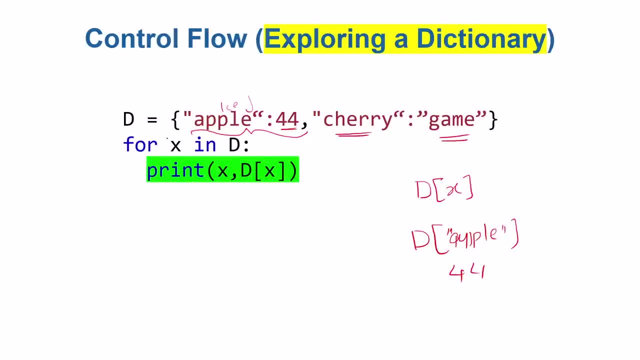 that this for loop is very, very handy of iterating over different data structures and a lot of data and stuff, whereas file loop is more handy in checking the conditions and stuff. although you can do all the stuff using while loop, you can all this stuff using for loop, but one is better. 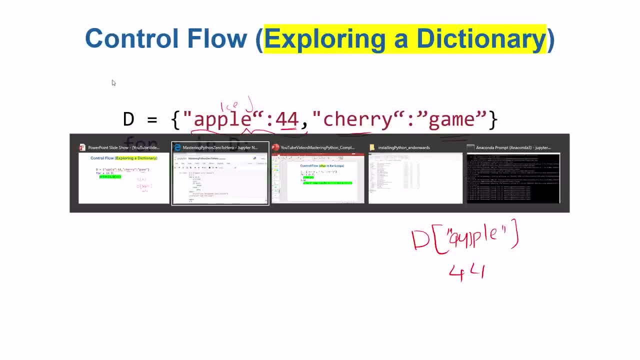 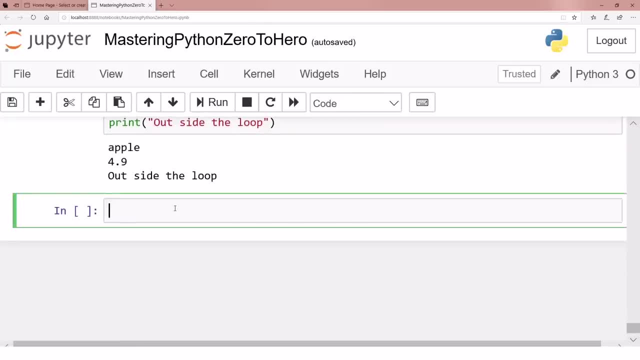 over the other insert in certain situations. so let's, let's, let's just run this for a dictionary. let's say I have a dictionary D. it's defined like a set. let's say: my key is a and my value is 10. let's say my key is B and value is minus. 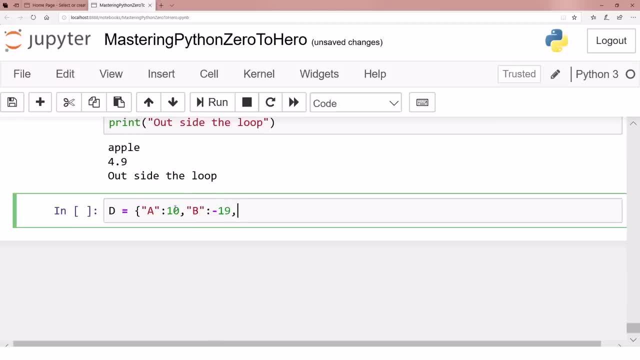 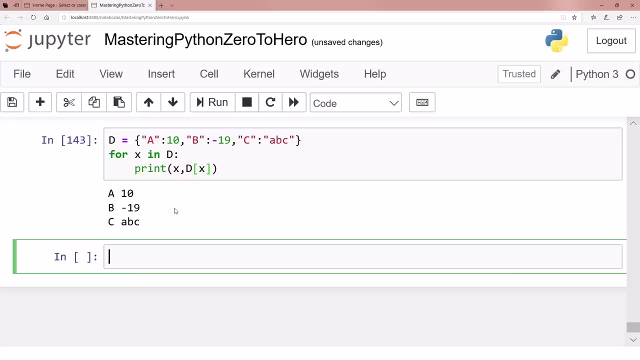 19.5, and that's why it's so hard to find the values of B. and so you can just find. and let's say my key is C and my value is, let's say, ABC. that's it, that's my dictionary. so for X in the print, the key as well as the value of that key. so now, 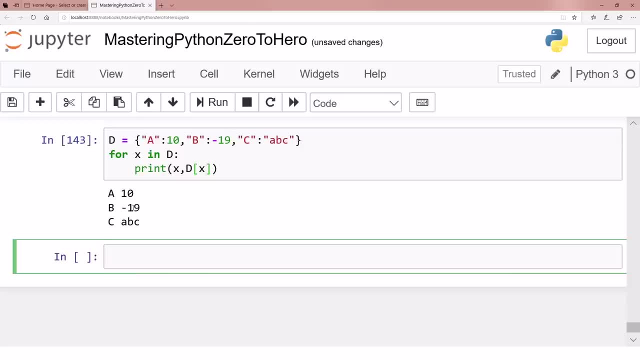 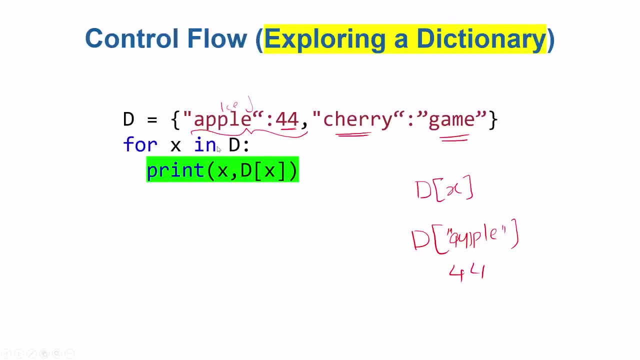 you can see: the key is a, the value is 10, the key is B, the value is minus 19, the key is C, the values ABC. so this for loop is really really handy in iterating over a lot of data structures and stuff, although it has other applications as. 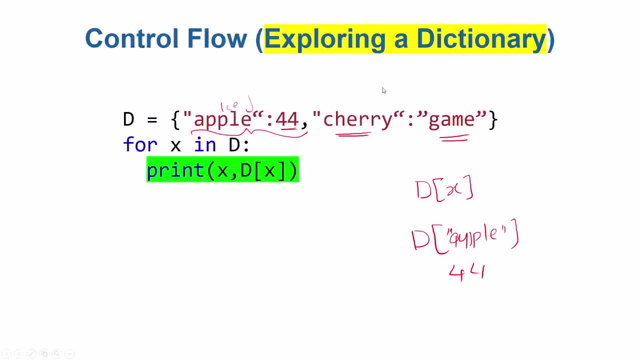 well, but this is handy, okay, great. so that's about loops for loops and while loops. these are two kinds of loops in important. look, these are two important kind of loops in there in Python. in the next video I will you directly go to Jupiter and Jupiter notebook and we will be practicing for 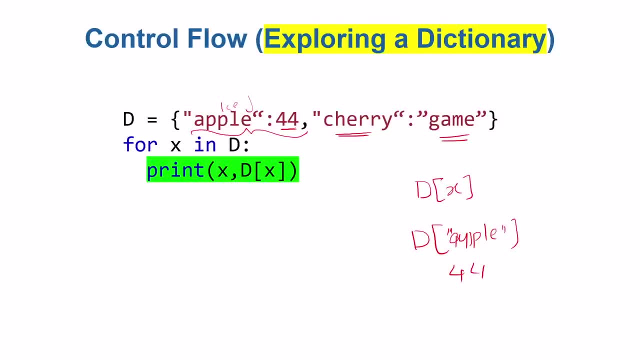 this for loops or while loops. we will be practicing the loops. we will be doing actually examples of nested loops. we will be actually solving a problem, like we did in if conditions. we solved a problem previously, we wrote a code for it. here we will also write a code and we will be get a good grip on the loops. so 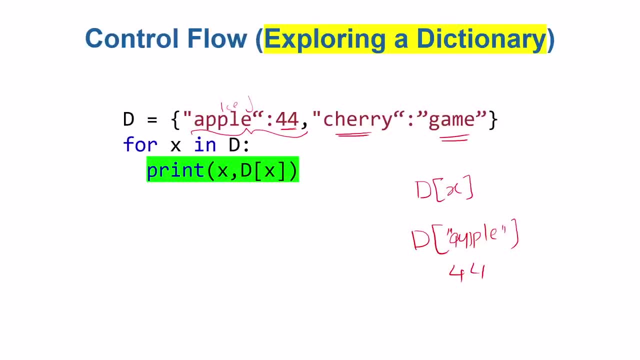 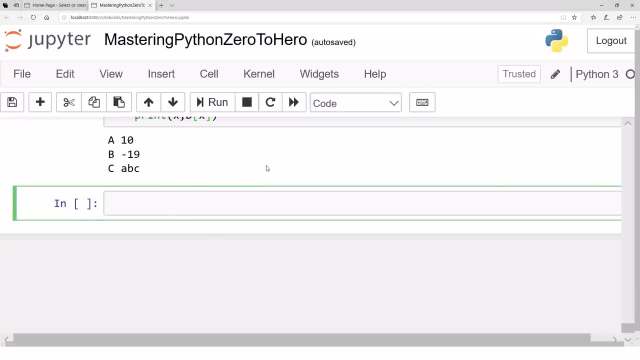 hope to see you in the next video. we will solve a problem in Jupiter notebook directly. okay, hope to see you in the next video. okay, welcome back. in this particular video we are going to practice for loops, or basically loops. so let's have a problem statement first, what problem we are going to solve. let's 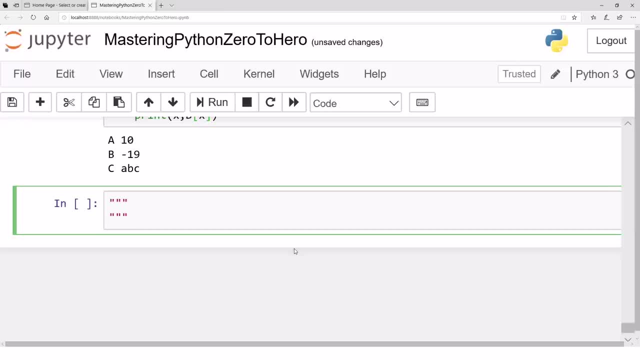 have comments, and the problem we are going to solve is: let's define, given a list of numbers, numbers, for example, ie, let's say 1, 2, 4 minus 5, a, 7, 9, 3, 2, like this. make another list, make another list. 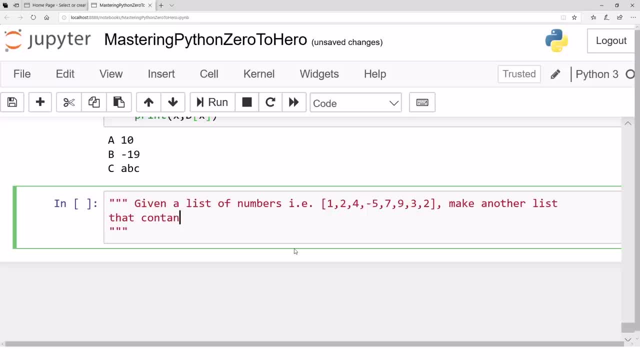 that contains all the items in sorted order from minimum to maximum, ie your result will be another list, like in this particular case. we will be having minus 5, which is smallest, then we will be having one, then we'll be having two, then we'll be having two, then we'll be having 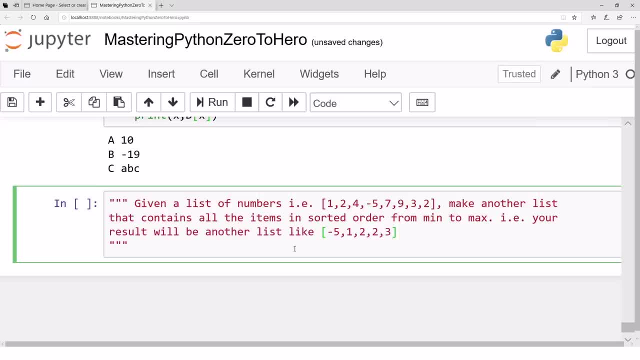 two, then we'll be having three, so all the items, but in minimum to maximum sorted order. then we'll be having, I guess, four, then we'll be having seven and then we'll be having nine. so that's your. that should be your output in another list, so assume this list is available to you, or any list is. 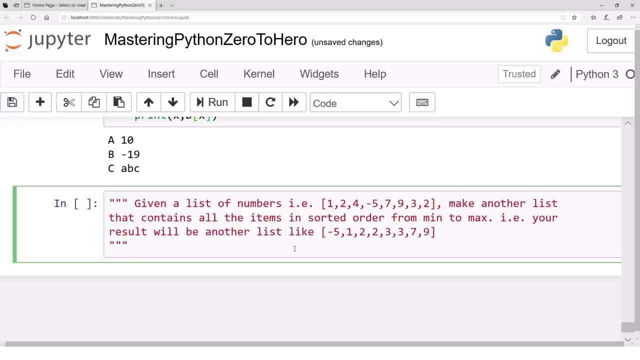 available to you, assume this list is available to you. so how to solve that problem? let's start, okay, let's assume that the list is available. let's say this is the list we are going to sort. let's say this is available, okay, okay. so what should be the logic? what should be the logic? how? 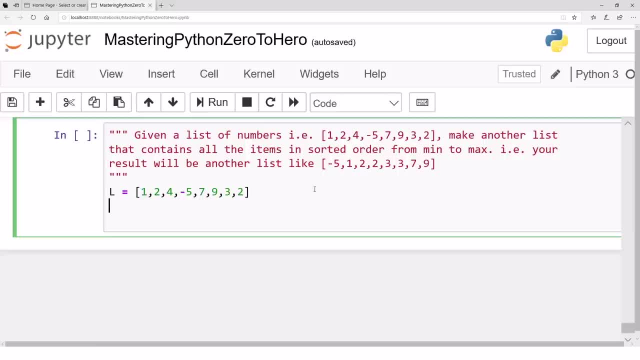 can we solve that problem? this is this is an easy-looking problem, but it is not so easy. let us first write. let us just simplify this problem to just finding out a minimum from the list. let's say we are given a list and we just want to find out minimum number one, minimum from the list. so how can we move? 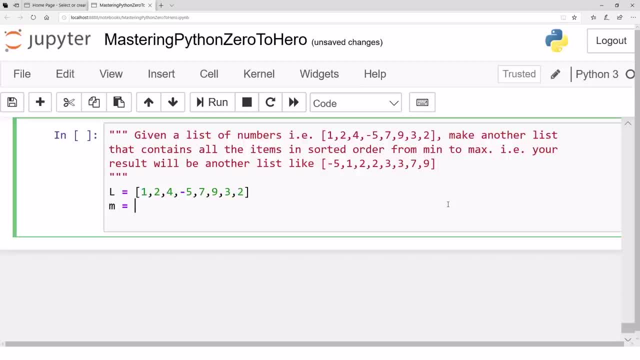 that. so let's say M is some number, so M is the very first value of the list. let's miss our variable. let's say that's the first value and what we do is for I in the, for I in L, as long as I is in L. if I is smaller than M, then if 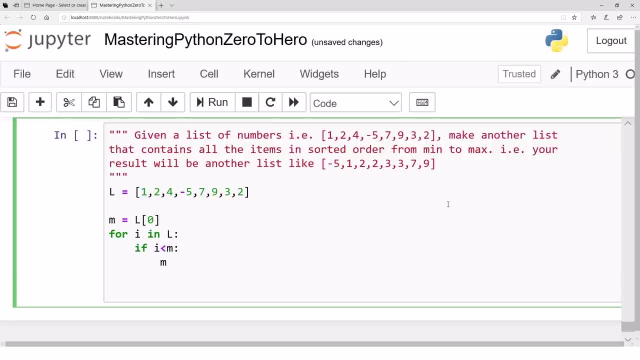 I is smaller than M, then M should contain: I otherwise do nothing. that's it. so at the end, print this M. print this M. at the end. so print the minimum number. that's M, great. so so that's the, that's the basically. so, yeah, that's the that's. 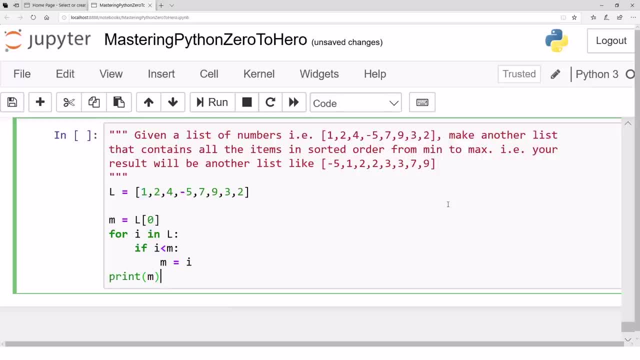 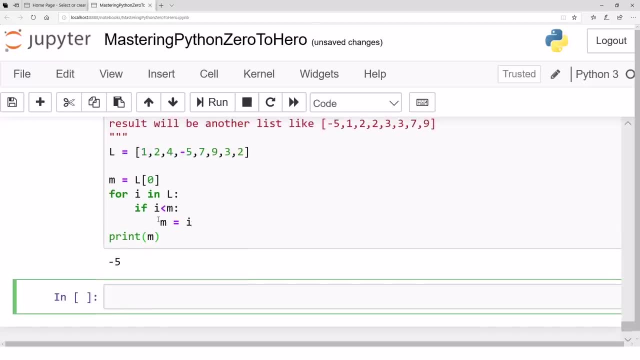 how we will find out just the minimum value. so let's run this code and the minimum is minus 5 available to us. what if we want to store the minimum value as well as the position of that value, for example? we not only want to just find out what is the minimum number. 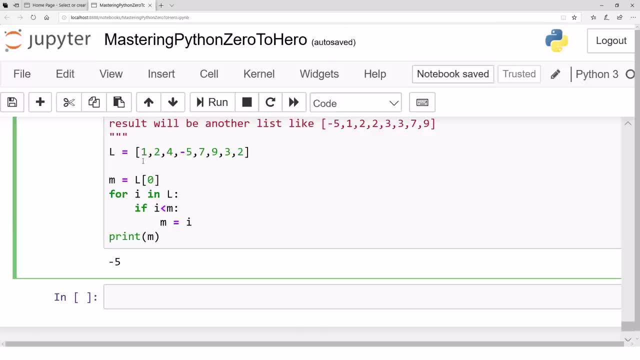 we also want to want to find out at what index- for example here 0, 1, 2 & 3- at the third index we found the minimum. what if we are interested in the index as well? so let's say for the very beginning the index is 0, and then what we do is: 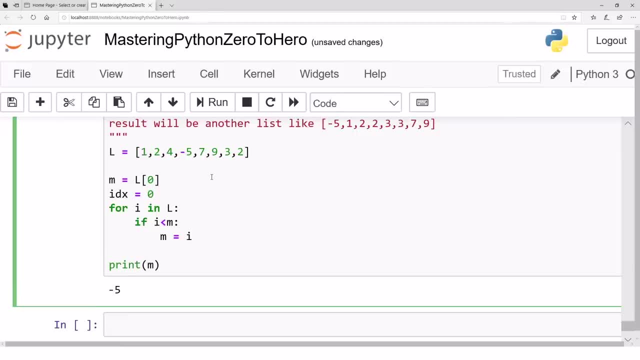 we moved on and we say: okay, we maintain a counter. let's say a counter is C equals, C equals 0, for example, right now, and C just plus equals to 1. that's a counter. and then this ID X is just that C, whatever that C is. so whatever that. 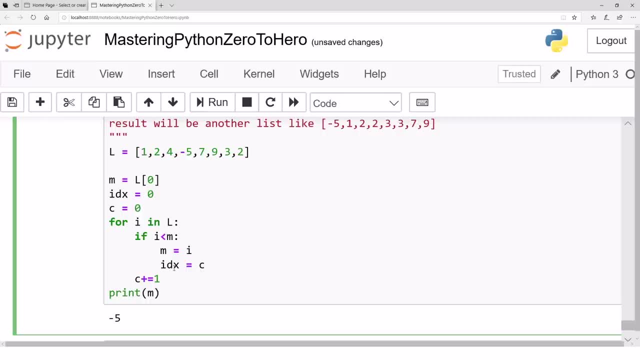 index is when we find this C, that index is also there, so let's print the index as well as the minimum value, so okay. so at the position 3, at index 3, we found the minimum value. okay, now we have written a kind of a code block that helps us finding out the. 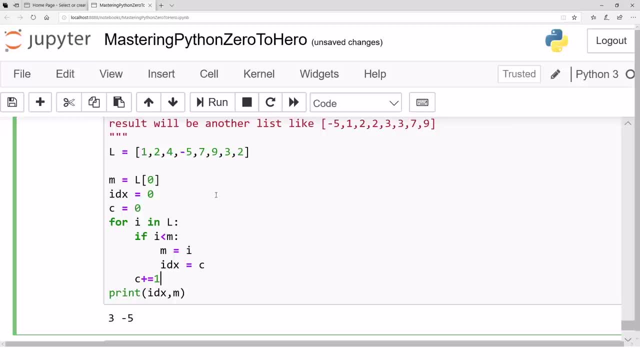 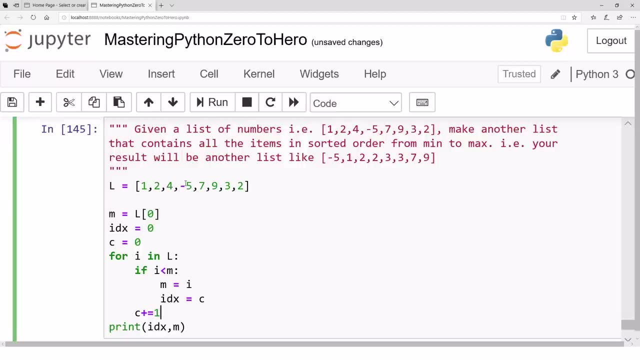 minimum value. how can we actually? how can we actually do? how can we actually? so the basic logic is: you can find the minimum value and you can find the minimum value and swap that value with the very first value- okay, great. and then move the loop. next time, find out the minimum value from the remaining. 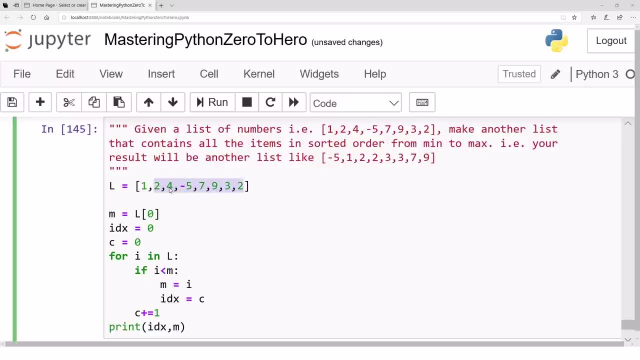 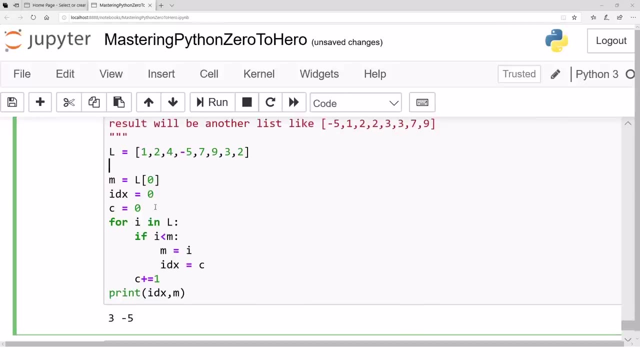 list and swap that minimum value with the second value. next time you find the minimum value as long as the position, and swap that with the third value and so on. so do that stuff and just rearrange the same list using this. but but how can? so that's the logic- find out the minimum value, swap it with the 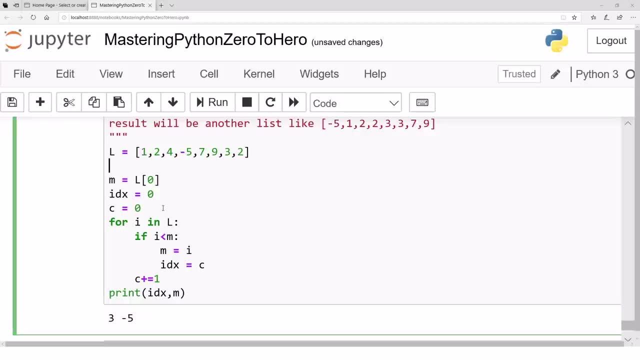 first value and then start from 2 till end. start from this, start from the remaining values, find the minimum, swap it with the first value of the remaining list, then reduce the list step by step and you will be having a sorted order. but how to start with? how to find out like this, how to, how to do that? so any 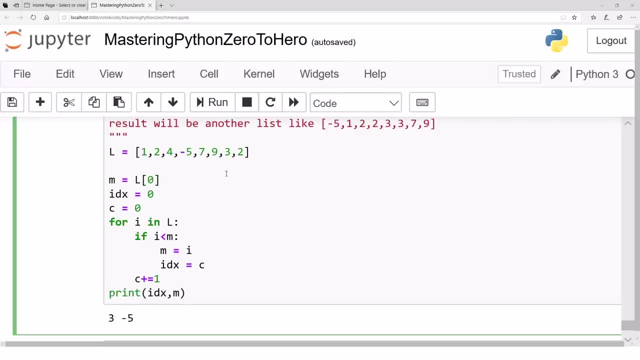 idea. I mean, we are going to subscribe to our YouTube channel and we will see you in the next video. So, for example, in this particular case, if I want to swap the list, what I will do is I will say, okay, swap with zero at the zero. so I will contain a temporary variable. 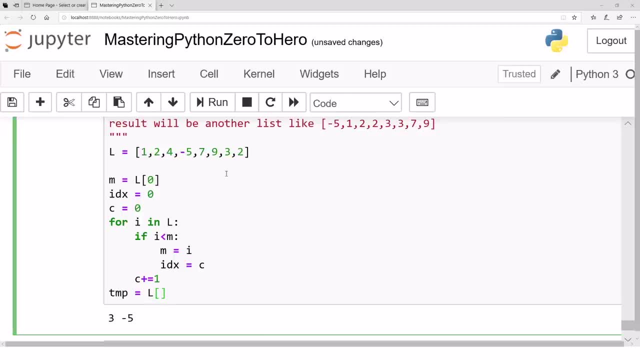 Temporary variable will contain the value of zero, this zero. So what I will do is, at list zero, write the minimum value and the minimum value. so at zero you write the minimum value, but at this particular index, from where we found the, 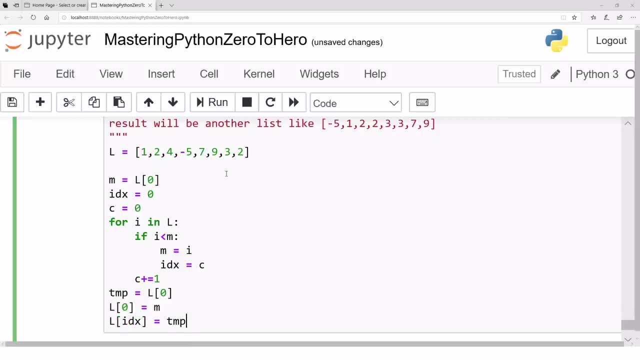 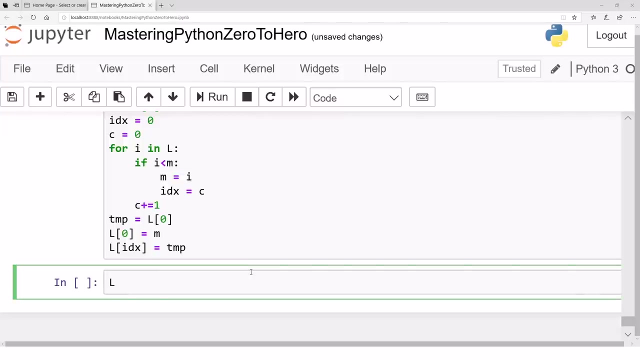 minimum value. just place the value at the very beginning. So after that operation the minimum will be at the first position or the zeroth index, and that value will be so minimum value will be swapped with the very first value. So let's run this code and see what a list looks like after that code. 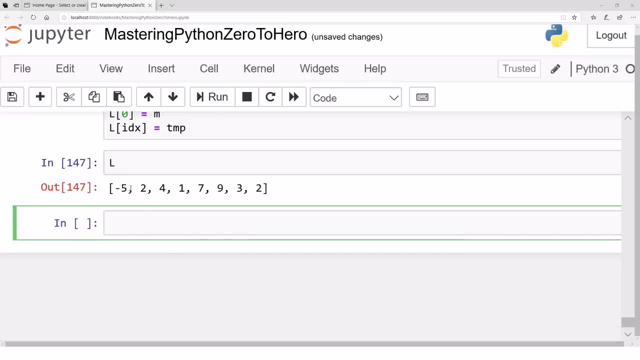 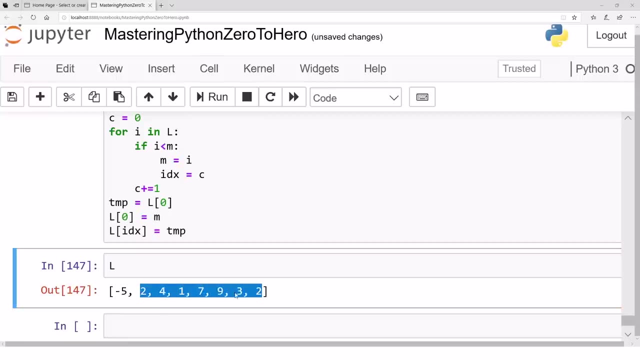 So you see, for example, the minimum value is swapped by the first value, whatever the first value was. But we want to do that progressively for the rest of the list. we want to find out the minimum and swap with the first one for the rest of the list and keep on moving. 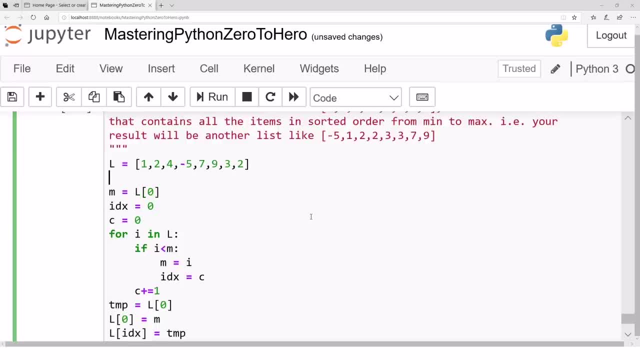 How can we do that? So yeah, that's, that's so. let me define for. so let me first indent that a bit. Let's say control, write bases. that will indent all my code. So for j, in range length of the list. whatever the length of the list, let's say for j is. 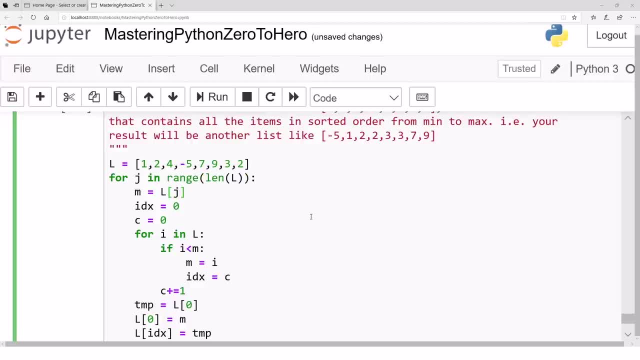 that. So what I do is m is j, The jth value, the index right now is j and the c is also. c is also the counter. c is also starts from j. Okay, great, Now we want i to start with to. now we want this i to start from j and move onwards. yeah, 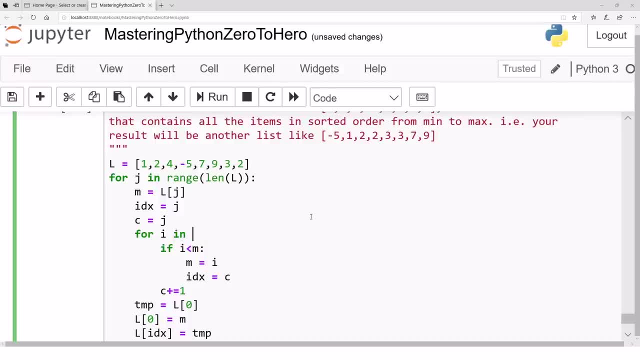 So let's say i, i in range, start from j and go till length of l one by one, Take the step of one. okay, great. So what next? Now? the value will be l of i rather than simply, l of i rather than simply i. 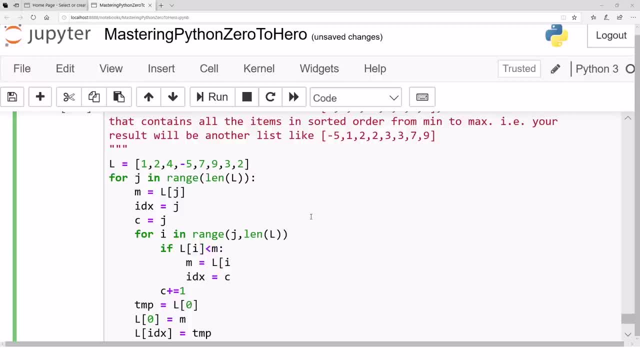 In that case, you do this, Okay, And the index is just c. Okay, great, Keep on, keep on introducing this index again and again. After this loop. what you do is you pick the jth value, you swap the jth value with. 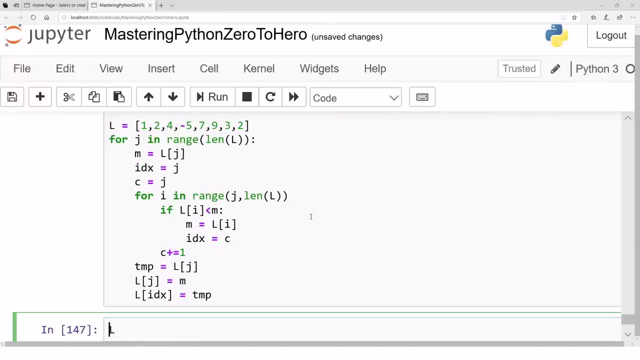 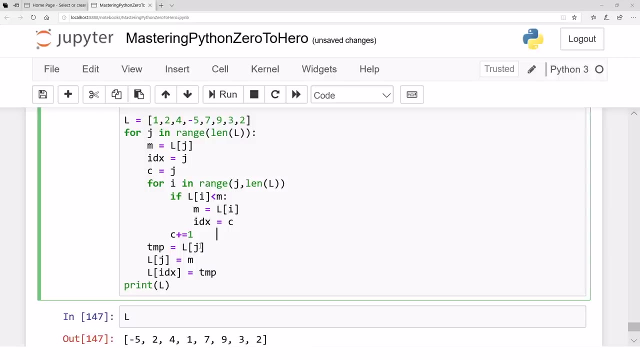 the minimum and you do that and that's it. You keep on moving and after, after the outer loop finishes, if you print your list, you will be having the list sorted order- At least we hope so. So maybe there is a bug in the code. 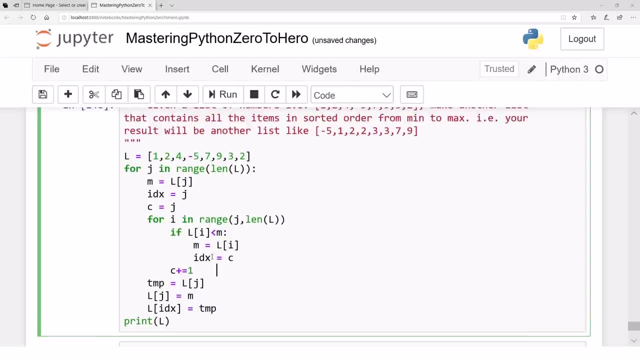 Maybe there is a problem in the code, but we hope this will work. What we are doing progressively. by the way, this is a nested loop, This is a loop inside the loop and that's, and then we have an if condition inside the 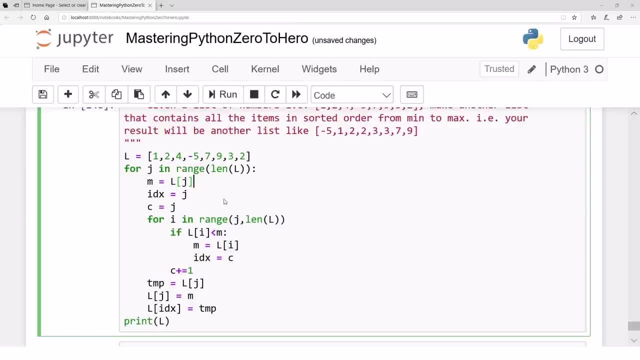 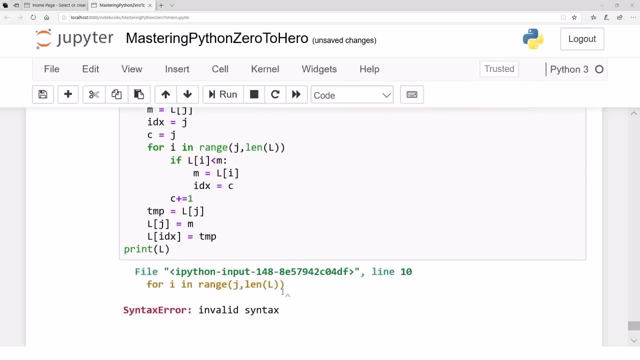 nested loop loop inside the loop. great, Let's see how it how it works. If there is no, oh, there is an error. length of range: oh, we haven't write a column there. Don't forget this colon. 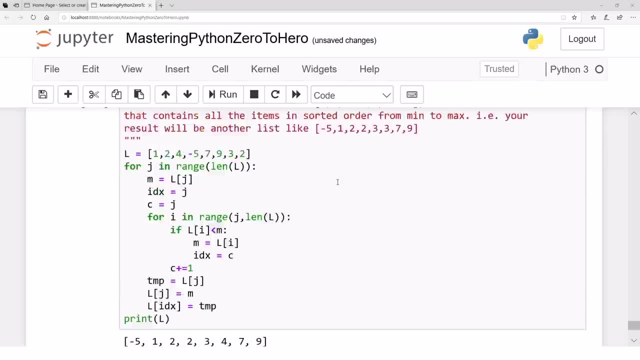 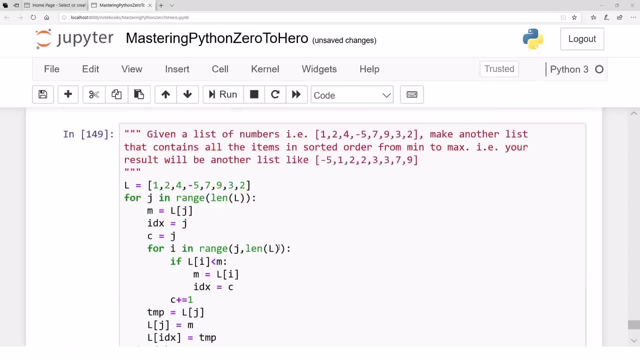 That's a problem. Oh, we have a sorted order. oh my God, we have a result with us. You see the applications of this. oh, one three is missing. where is three? We have two threes. oh, the output we have written here is wrong. there is no two threes. 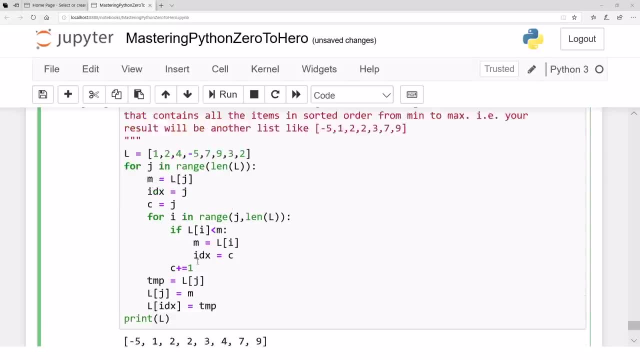 there is only one three. So you have sorted a list. If you remember, we we have written a similar kind of code in the problem solving session very early on Here, where we solved this problem using selection sort, but there we just wrote a pseudo code. 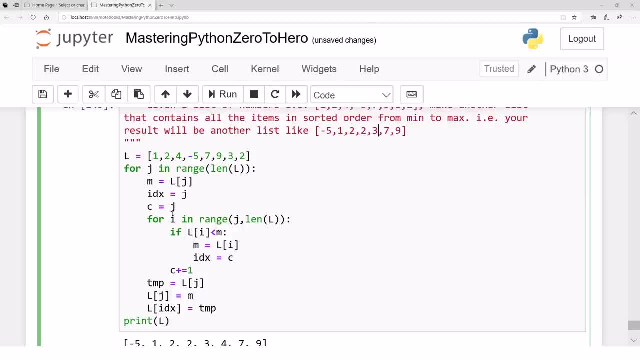 and here we have a code much simpler than actually the Python code. If the problem was just sorting, there are built-in functions to do that, but I'm just telling you how these loops and if, conditions and all that stuff can be used to communicate. 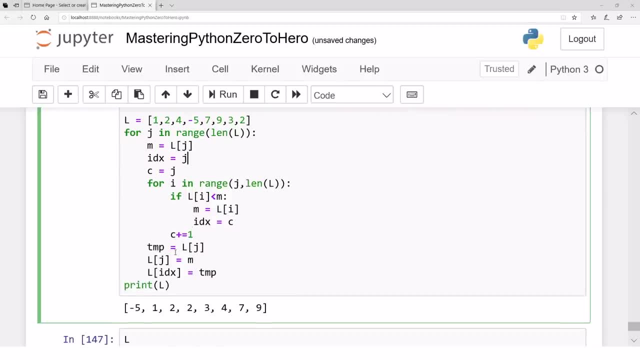 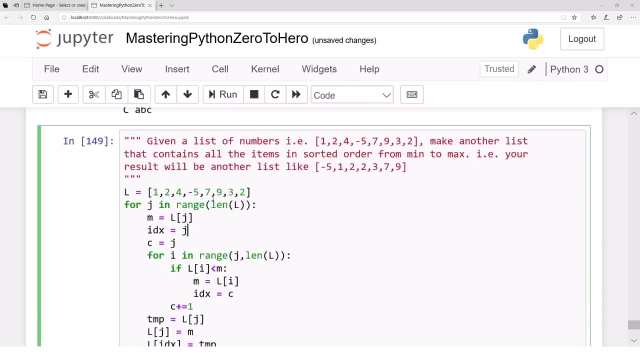 with each other, to match with each other, to to actually perform a problem solving task When given a problem. Although we will see later on in Python most of the problem solving tasks, I mean many more of them. there are built-in functions for those. there are available functions for: 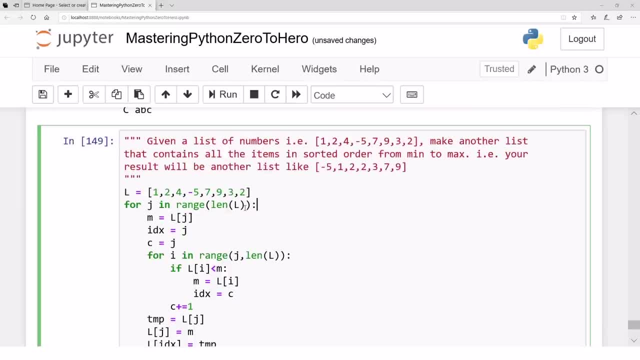 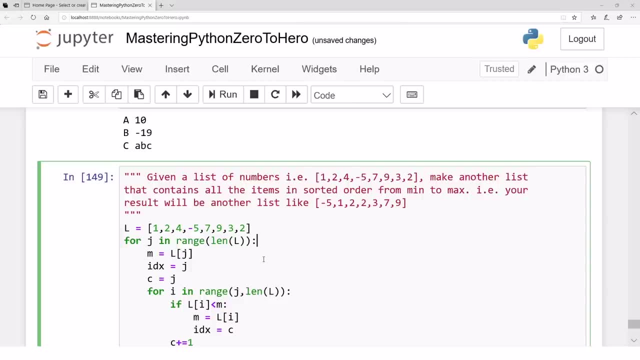 those You need, not to write all that stuff, but to mastering, to. to master any programming language, you have to go through these constructs so that for a new problem or for a very large, complicated kind of problem, eventually you you may need these kind of structures with. 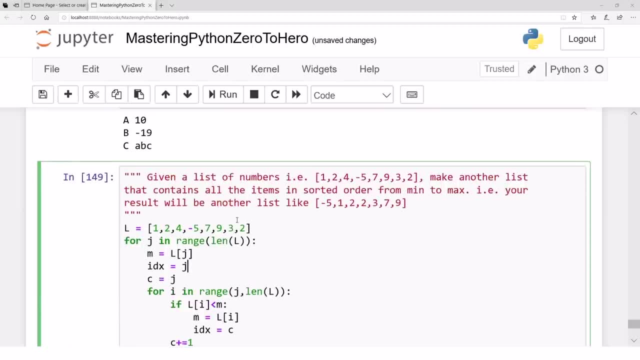 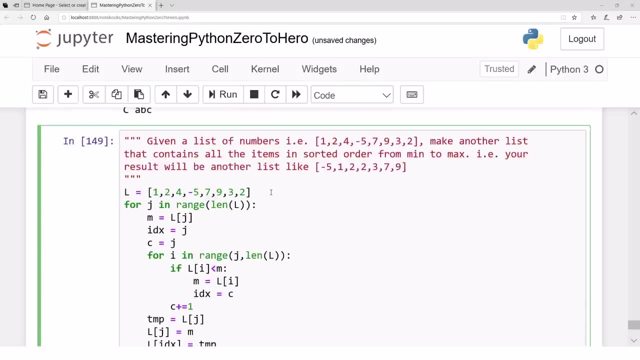 you. So mastering these structures is really essential for problem solving. Okay, Thank you, I appreciate that. I appreciate that. Thank you for giving me this story of problem solving and programming in general. So, okay, that's about the loops and if, conditions and control flow, all of that. 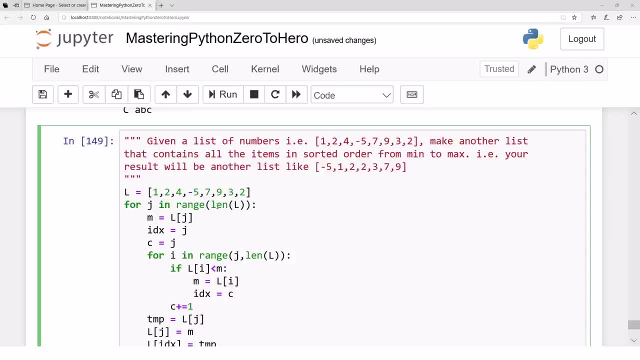 In the next video I will. I will start talking about functions. So you have seen this L E N data function. You have seen this range. that's a, that's a function I rate, or although you have seen around function. 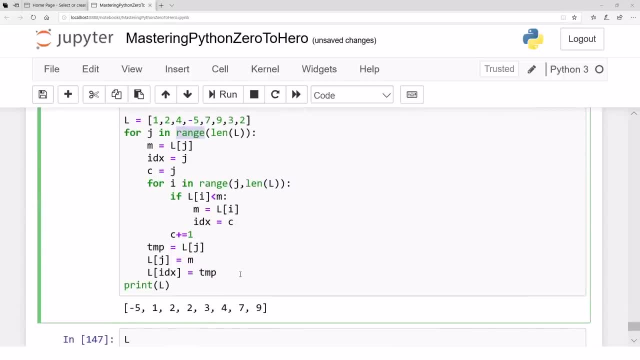 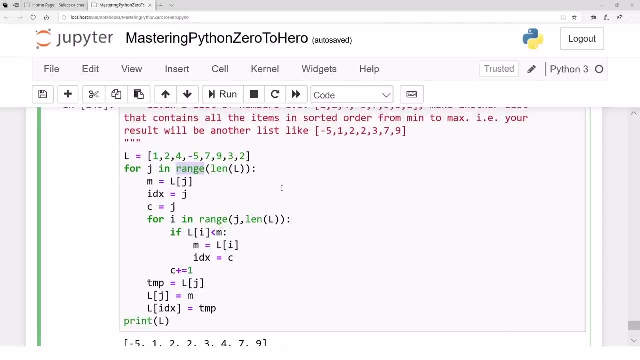 You have seen Diff mode. You have seen Brent function. What if we want to write our own function? how can we do that? From the next video going to show you how can we write our own function- Wow, Isn't that great, That's. 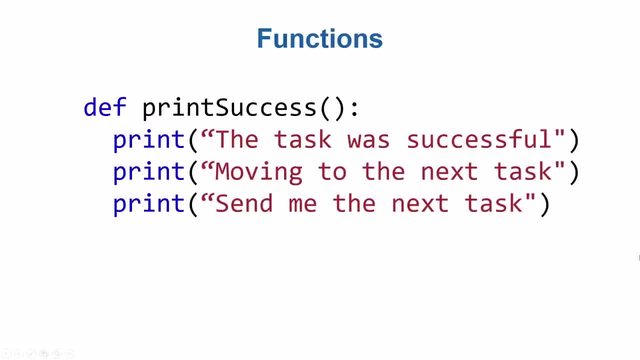 great, So hope to see you in the next video. In this video, I will talk about functions, A very powerful construct in almost every programming language. Python also supports functions. What a function is? let me let me describe the. let me describe the need of the function by a scenario. Let me give you a scenario: The. 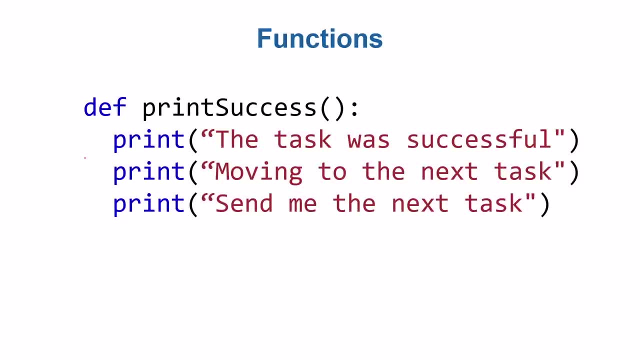 scenario is: let's say you are writing a very lengthy program. The program requires to print particular messages whenever needed. For example, you need to print this particular message, the task, the task was successful. Let's say you need to print this and then you have to print. moving to the next task, maybe to 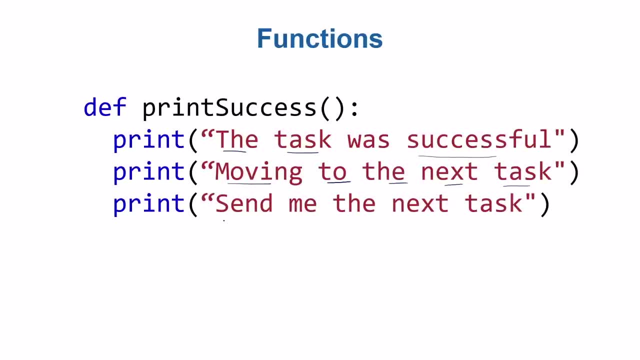 to inform somebody, Maybe to inform your ou client, and then you have to ask: okay, send me the next task, because I'm done with the previous task. let's say you want to print this, or maybe you want to print more or do some more stuff. and let's say 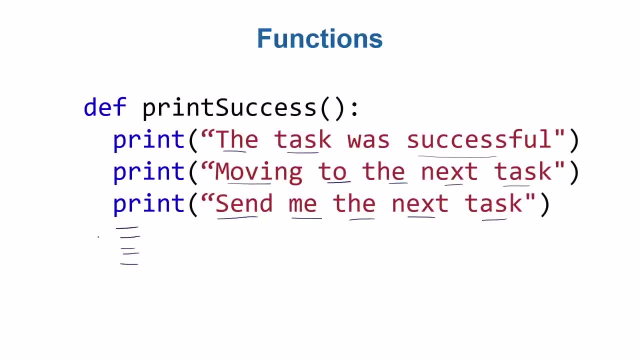 you want to do this again and again, whenever needed, somewhere, whenever you complete a particular task or something, you want to print all these messages, and then somewhere else, whenever a particular event occurs, you need to print all these messages again now. one way to do that is to write just. 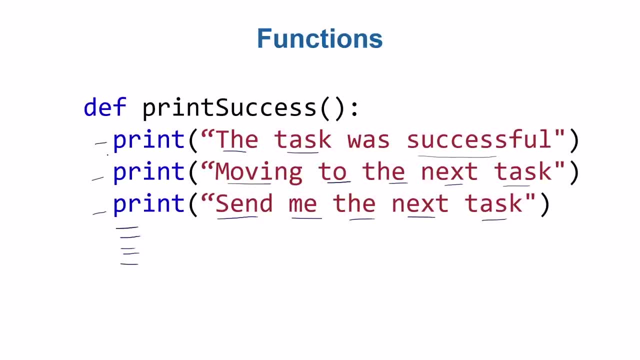 these print statements whenever needed in the program. one way is if you want to perform a task and the task has a lot of coding, maybe, maybe, maybe very small amount of coding or maybe a very large amount or magnitude of the coding. in this case we have just three statements, but 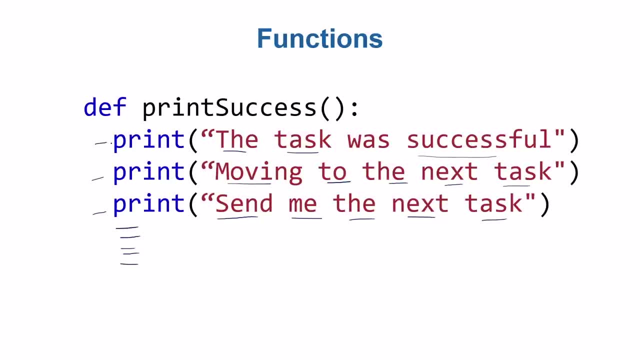 maybe we have a task that we want to perform again and again, and it is really a very lengthy task in terms of the coding. so one way to do that is to just write all the coding coding somewhere and define a function, and that function means the function. 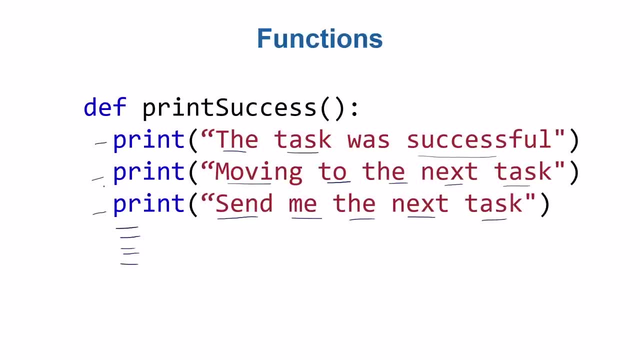 contain all the tasks that you need to perform. whenever you need to perform that particular task, just in your coding, just call this one statement, just this one statement and the whole task that is written under this, under this, maintaining this as a heading that will execute automatically. I mean, however, I 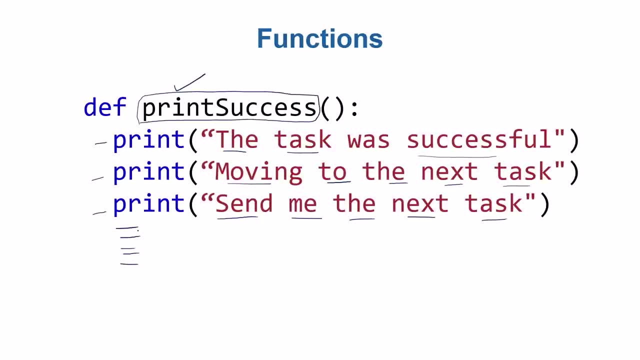 mean that task that is under this heading may be very lengthy, may be short, may be complicated, may be simple one or anything, but the need is we want to perform this task whenever we need and we do not write to code this again and again. we do not write to code, we do not write to, we do not want to write the. 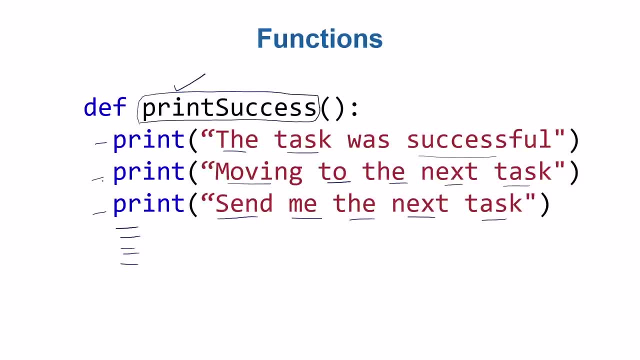 same lines of codes again and again and again and again. in our program you just write this particular lines of code once. define a function just like a task. whenever you need to perform that task, just call the heading or the name of the function and the whole task under that function will execute functions in. 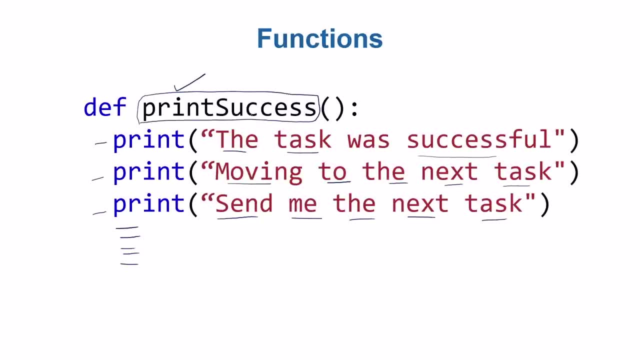 almost all programming languages. they do that, even in mathematics. they do that in: in Python, the syntax of defining function is you. if you want to define a function, you have to first start with D, E, F meaning definition or defining. then you need to write the name of that function. 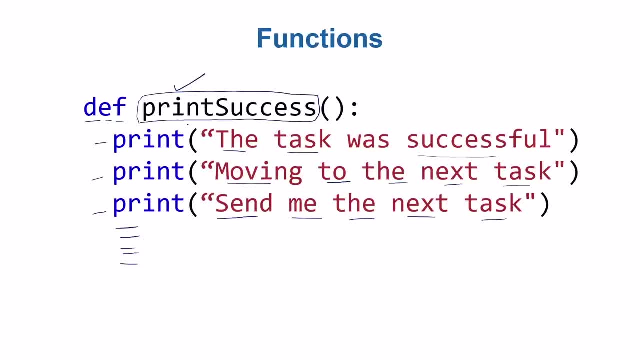 the name of that function. name of function and name of variable has resemblance. I mean the name of function should be descriptive. it should, it should portray what the function actually is doing. so it is good to write, it is good to suggest the names of the functions that are very descriptive to make the 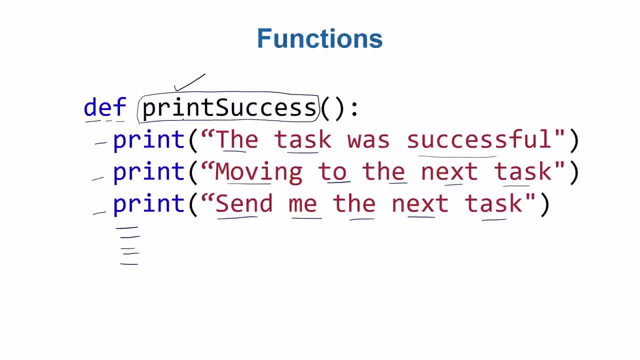 code readable and manageable. so here I have written the function name as print: success. you can write any name. then you start, start parenthesis, then you end parenthesis and then you write a colon, like you have written the colon for if, conditions or for loops or any other constructs, and then you do indent like the body of. 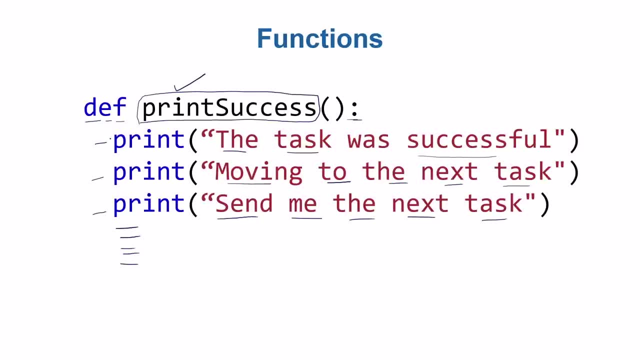 the for loop, like the body of the if condition. this is the body of the function. body of the function is all should all be aligned. then you write all the tasks, all the coding that you need to be performed whenever this function is invoked or called. this body can contain if conditions for. 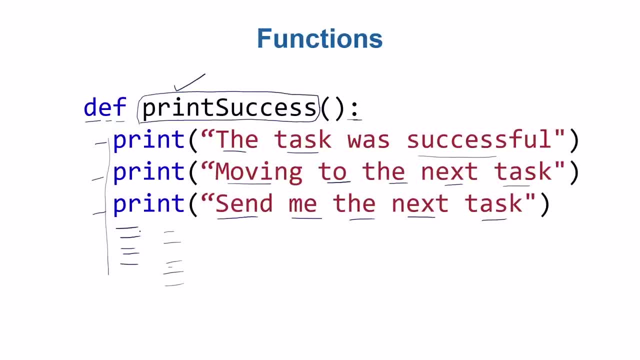 loops inside. I mean, this can have a whole lot of coding inside it, and whenever you will call this function, whenever you will type this command wherever in your coding, the whole task under this will be executed automatically again and again whenever you like. so let's take a look of 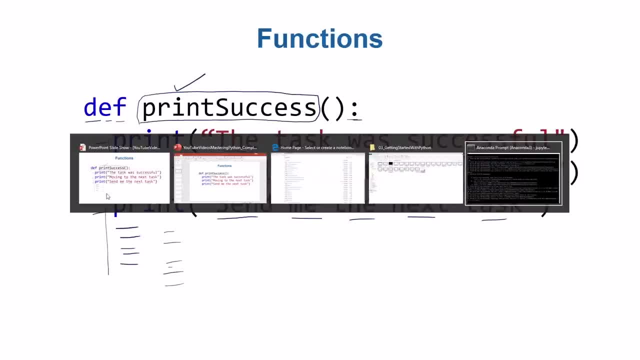 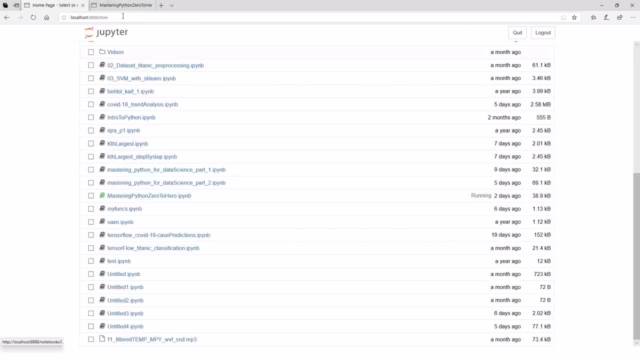 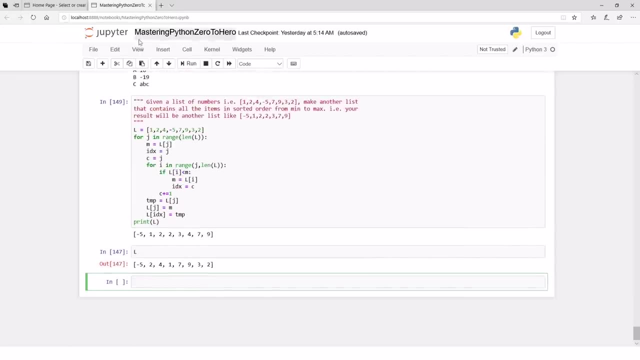 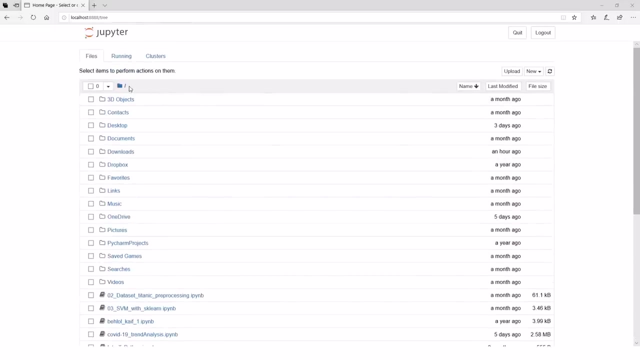 defining our first function in Jupyter notebook. let's just, I guess, yes, so, yeah, so that's our notebook, we were populating that notebook. so, by the way, if you, if you want to know where this notebook is located, if I want to, for example, invoke that notebook again when 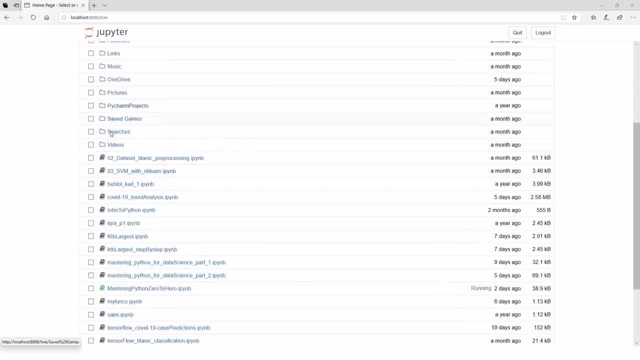 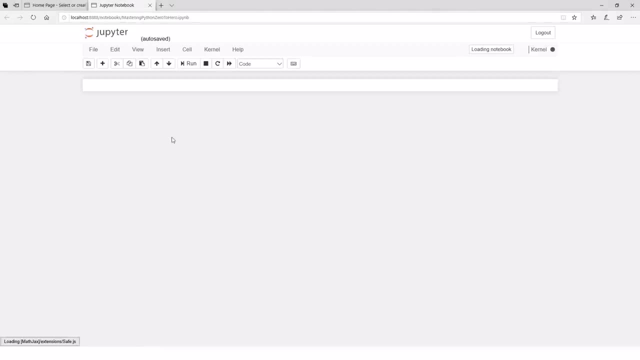 you will run your Jupyter notebook from the anaconda prompt. you'll be having all the files that you are working on and one file is, for example, this: you just click on that and your file- one or more files, whatever you want to open up, that will open up in the Jupyter notebook. so 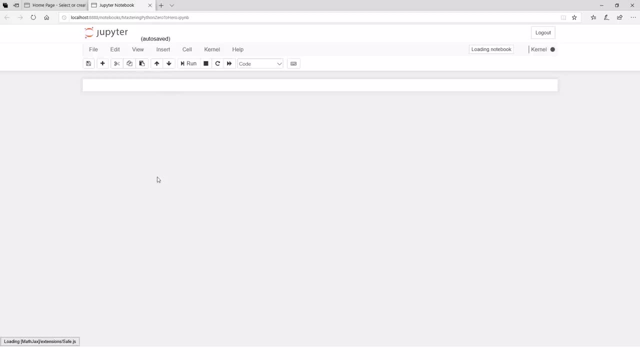 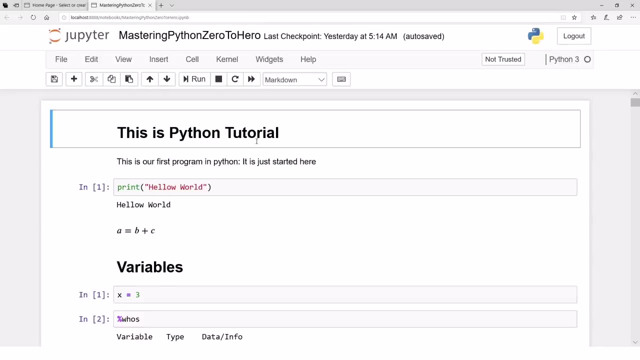 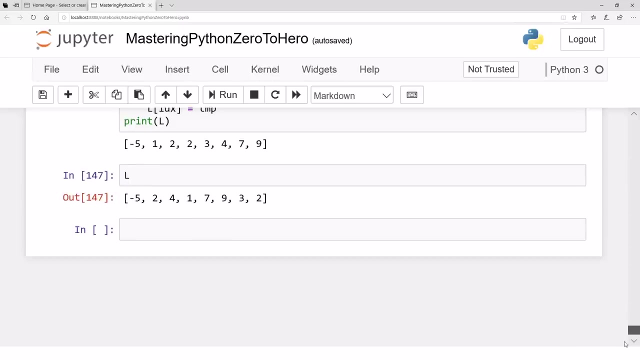 yes, so it is opening up. it's a lengthy file so it may take. may take a second. okay, let me just take a better zoom level just to okay. so we were working on that notebook. let's define our first function. let's say def define. let's say the function name is print success. 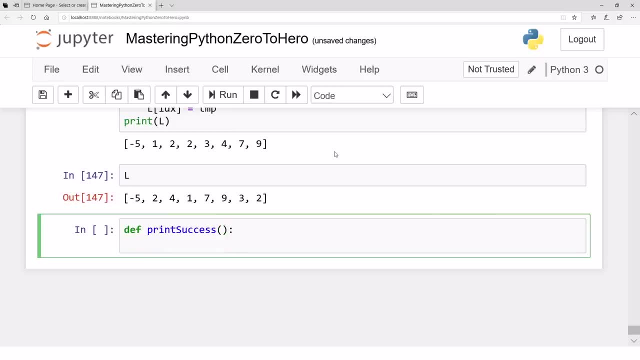 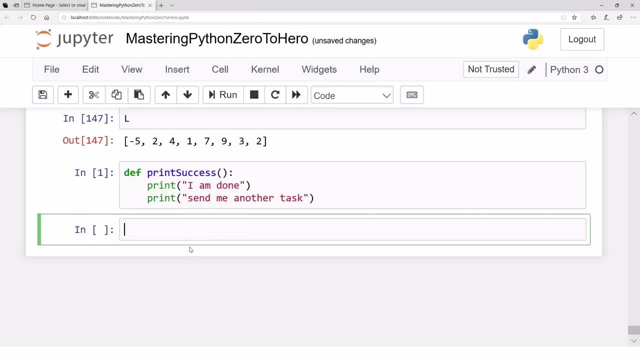 that's a, that's a syntax. then press enter, print. I am done. then print. send me another task. let's say: and that's it. let's say: that's the. that's the body of the function. the body of the function here contains only two statements. okay, then you run this. you run this command, just like shift enter. you run this so that it is, it is. 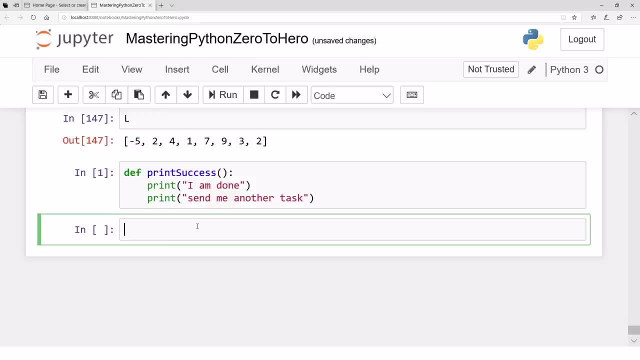 reported in the symbol table. there is a symbol table inside the Python maintaining. Python is maintaining all the variables, all the function information inside. so once you run this cell, then the then this print success function will be registered to Python so that whenever you want to call this function again, it will be available. now if you want to perform this task. 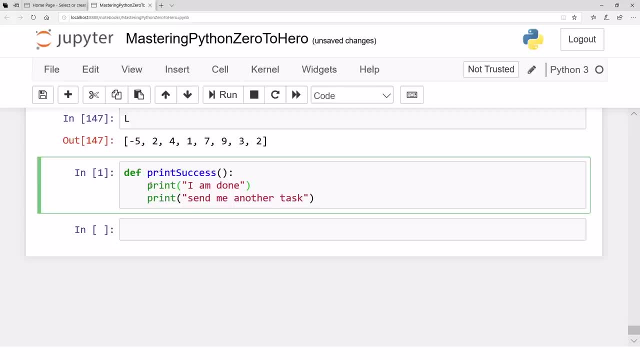 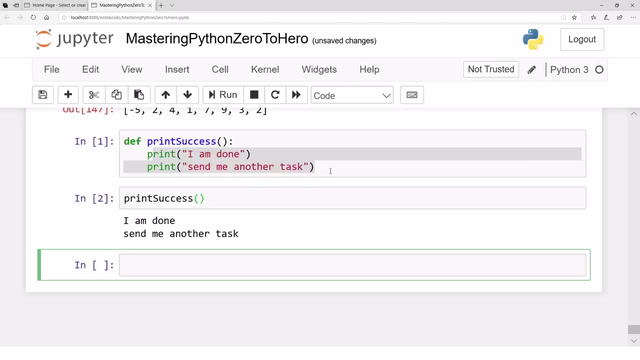 let's say you want to perform. let's say you want to perform this task whenever you want, so you just call this function. this is called calling of the function. whatever I'm doing now, print success and that's it. you press shift, enter and the all the statements that are under this will be executed. 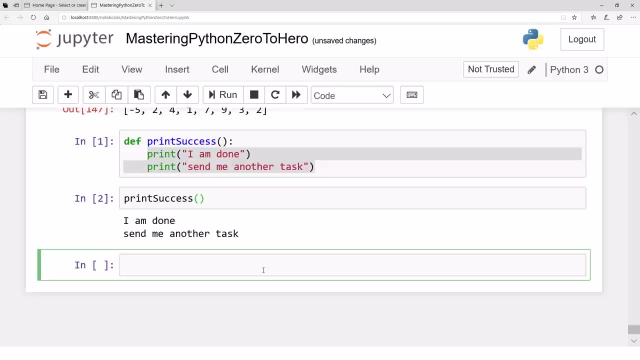 and you do some other stuff. let's say 3 plus 8, that is, that is 11. do some other stuff, and after a while you will be able to do some other stuff. let's say 3 plus 8, that is, that is 11. do some other stuff and after. 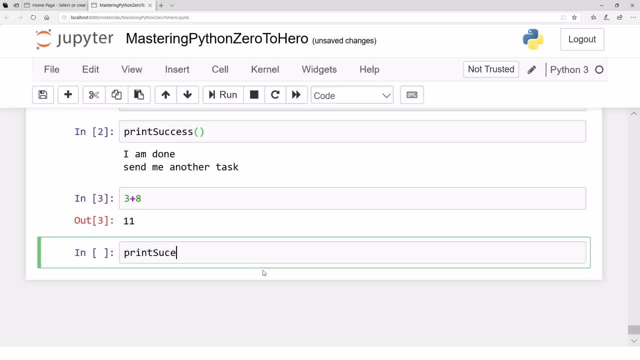 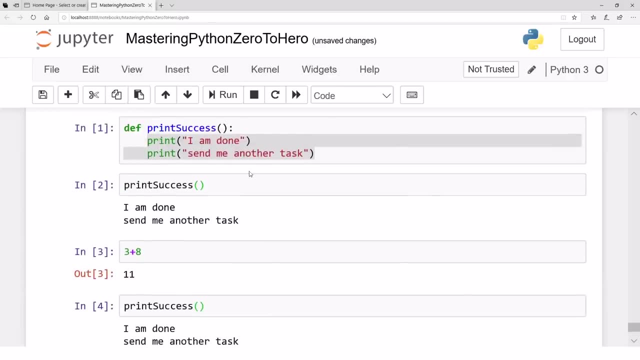 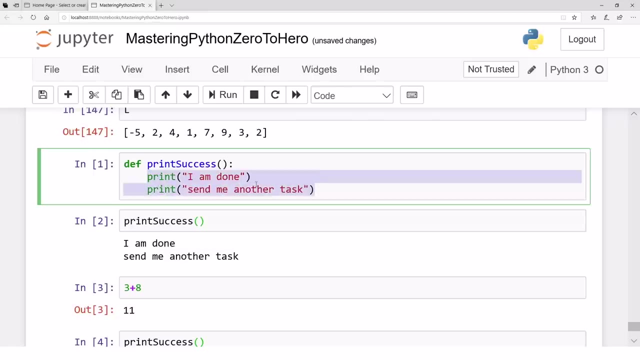 words. if you want to do the same process again, then you call this function again and all the coding inside the function will be executed. it is very, very handy. if a particular task, if you want to perform that task repeatedly, it is good to just write one code for that task in a function. 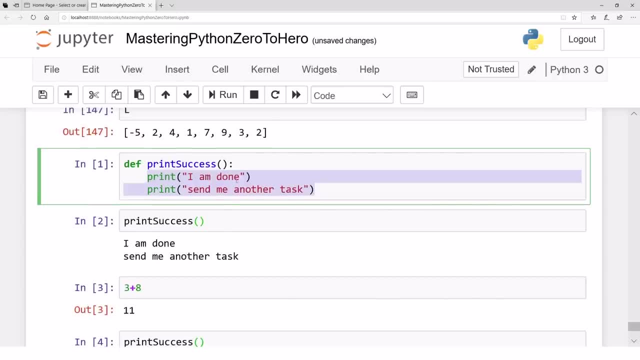 and then just invoke function whenever you need it. it supplies a lot of managing power, a lot of debugging power. if you have an error, for example, inside the function, you just go to the code. you just go to the code of the function itself and fix the error and come back. you need not to you. 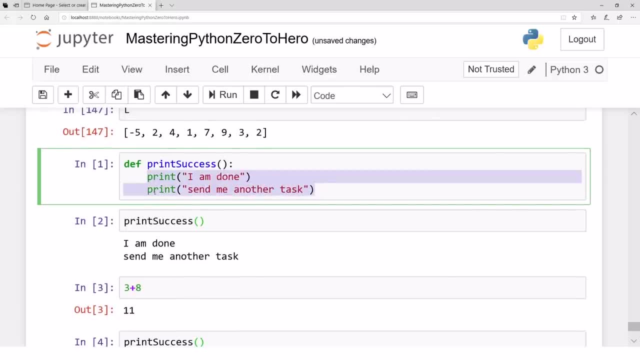 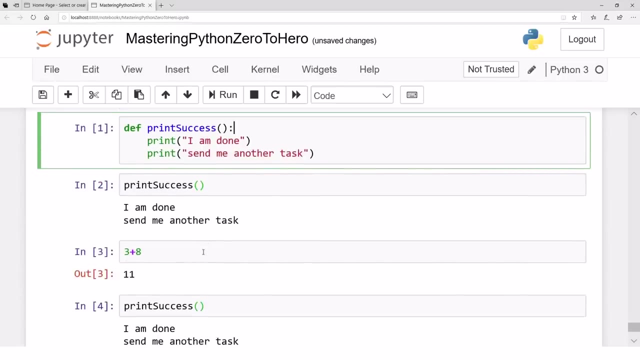 need not to go all over the code. if you have not defined the function and you have called these lines of course everywhere inside your main code, then it will become very difficult to handle and function actually provides a lot, of, a lot of simplicity of managing and readability and a 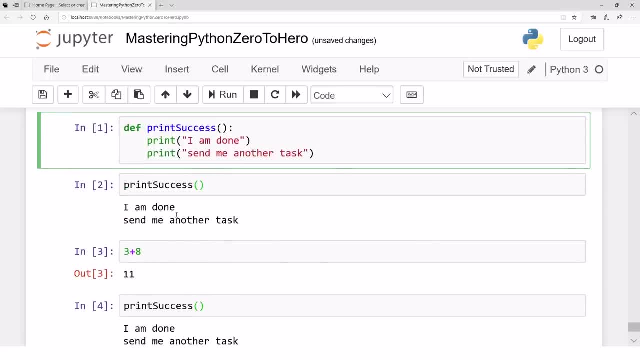 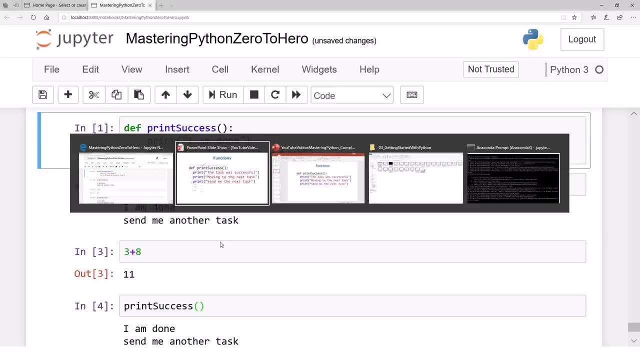 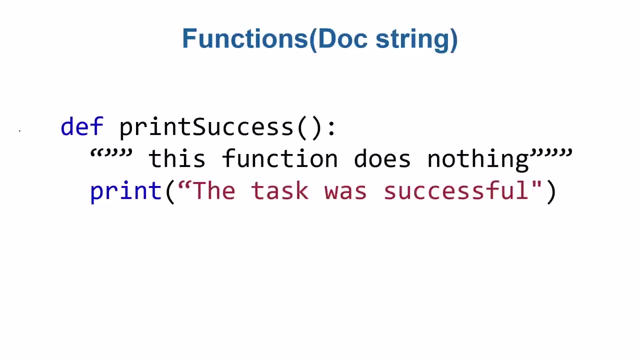 lot and a modular approach in that sense. so that was our first. that was our first function. we will be talking about more. we will talking more about these functions in the next video. so hope to see you in the next video. the function name should be descriptive. that's okay, but it is further. 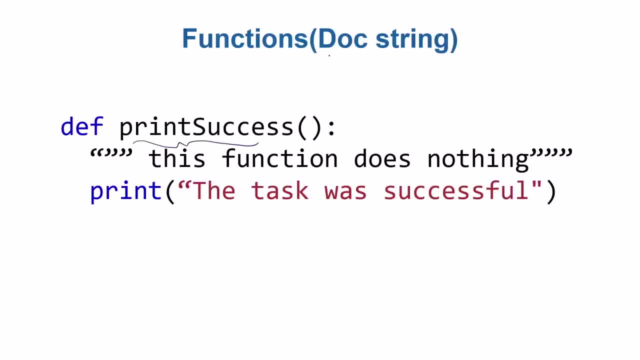 important sometimes to have a documentation of the function, sometimes called the dog string. the dog string allows you to write the description of the function, but that description will never be executed. it will be available whenever you need a help or you need to know what this function does. 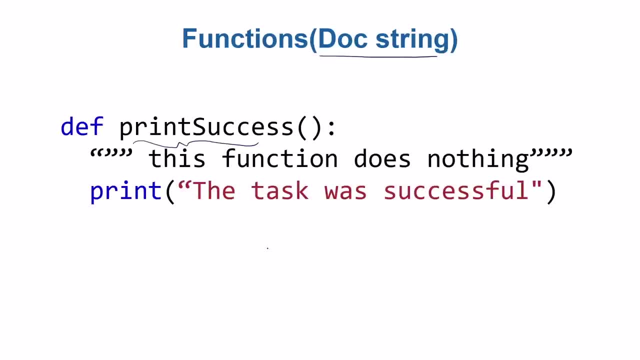 sometimes it happens your function can contain a lot of code. for example, you have a particular function, let's say fun, let's say it can def fun, and it does a lot, of, a lot of complicated stuff inside and it is sometimes required to to to know what this function actually is doing. so 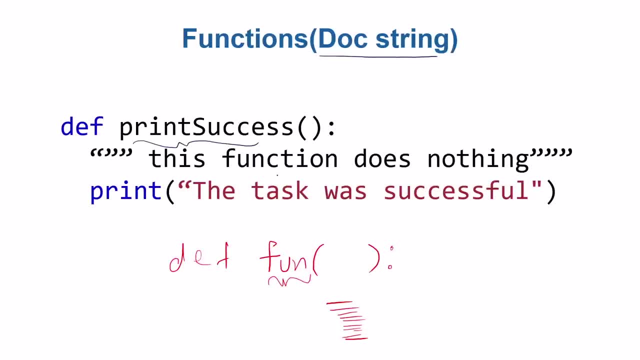 this document string is one way of describing what the function is doing. you might be thinking that if, if you're writing this document string inside the where, the, where the coding of the function should be written, we should open up that the coding file and see what the function is doing. 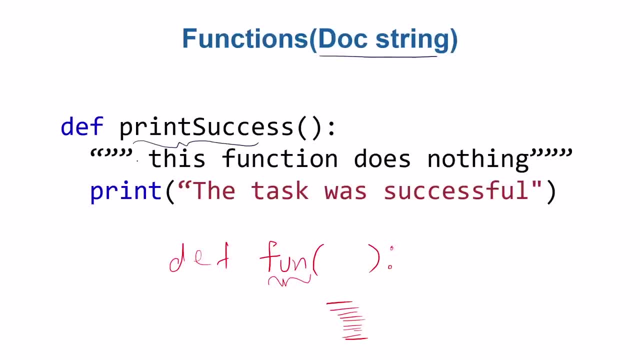 or should we actually open up this function implementation where the function code is written and then we have to read what the function is doing? actually, python gives you another power if you have written the document string inside. that should be a top statement before the first coding statement. whatever description you want as a document string, it will be available without. 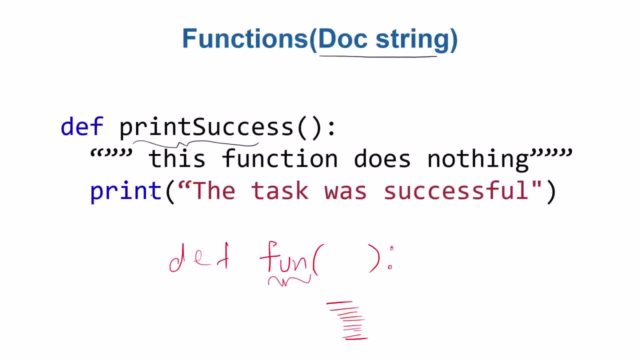 actually opening up with that without actually seeing what inside the fun, without actually opening up the file that contains the implementation of this function. let's see, uh, let's see uh to in jupyter notebook, uh, more completely, whatever i'm saying right now. so, for example, let's: 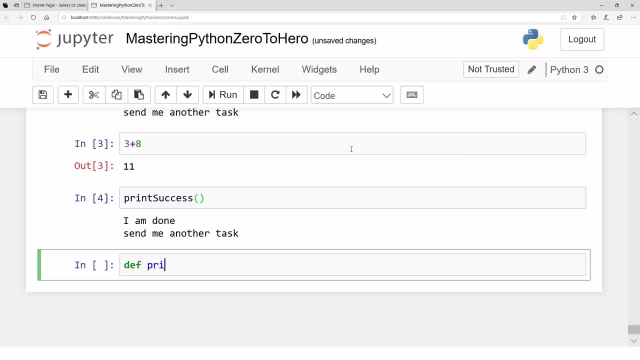 define a function uh. def. print success, um two. let's say the function name. this function is print success two. um. the function name is print success two, although it's not a very descriptive name, but um. the spellings are also not correct, but that's fine. um print success too. here i just define a document string, uh. the document string may contain maybe: 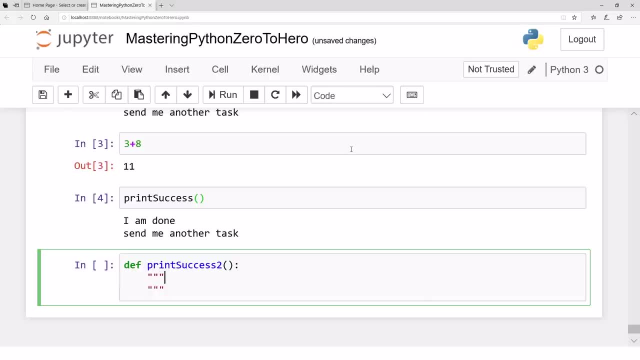 just in one line, or it may be a multi-line. it is like a multi-line comment, or maybe a single line comment, if you want. but uh, it starts with the three quotes and ends with three quotes. let's say i write here. this function is doing nothing except. 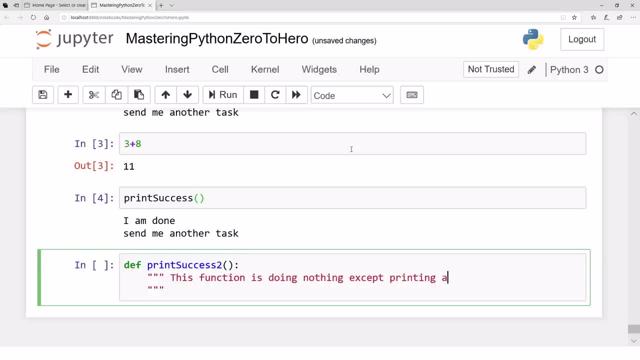 printing a message. printing a message, let's say full stop, and then i further define, let's say, i define more in saying that that message is hello. let's say, let's say, or any description you want for this function. now, this is a document string and it will be available whenever you need it. 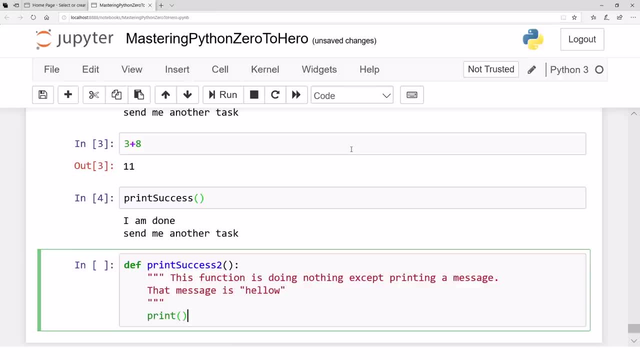 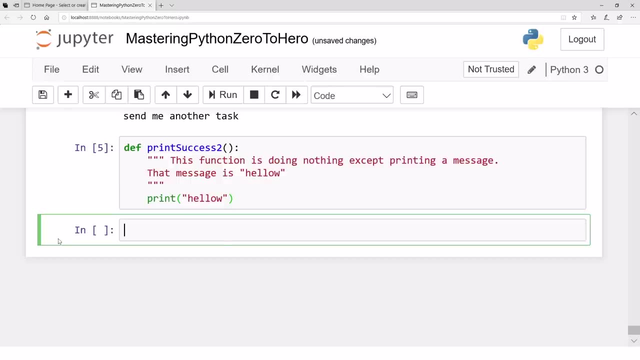 now here the coding starts. let's say you write a coding here and you get hello. let's say: and you run this code. now let's say we are not seeing this function. we are, we are not available with this function, we are not available with the code of this function and we want to know. 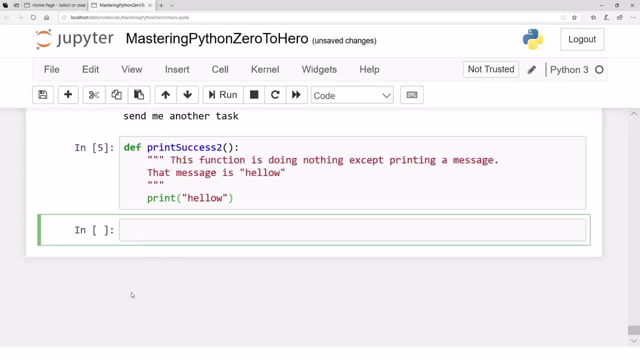 what this function actually does. first of all we can just write. if we write pri and just press tab, the tab will allow us to access all the functions that are available with prefix PRI. so let's say we go to print success, print success, print success. here, print success s should be capital print. 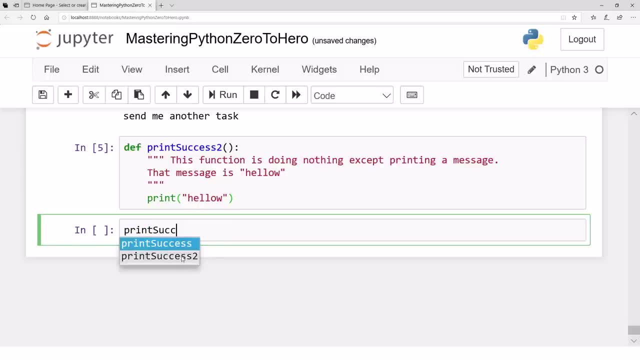 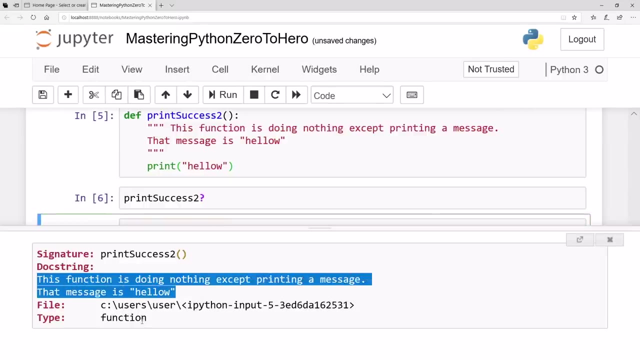 success, let's say so, print success to. let's say: and we write a question mark in front of it and then just press share, enter, it will pull the document string. it will pull the document string, whatever we have written, and we will get to know what actually this, this, is doing, so this document string actually does. 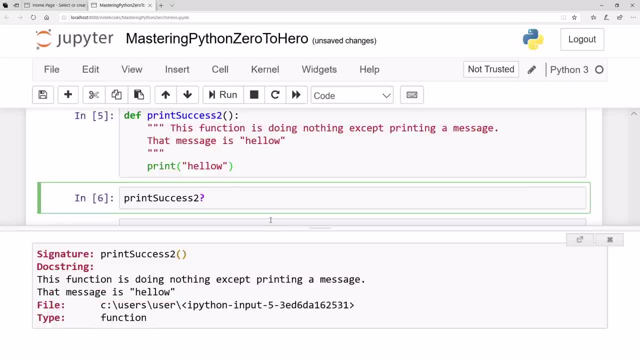 a lot of job further if we- I mean this is this is kind of: whenever we need to know what a function is doing, the document string is one way to just go and check what is what is happening. right now, this function implementation is in front of us. 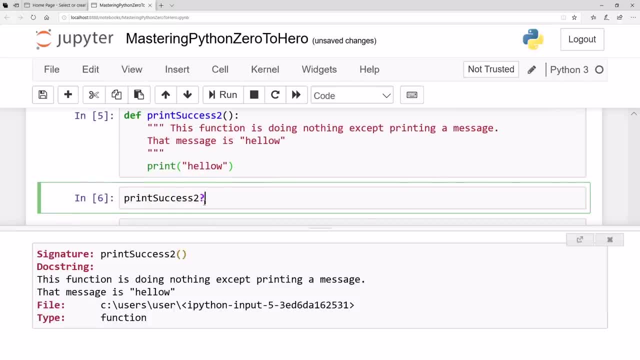 but in several times the function implementation will not be in front of us. several times we will be accessing functions that other people have written in their libraries and we need to know what those functions are doing. so document string is one very, very healthy way of describing our 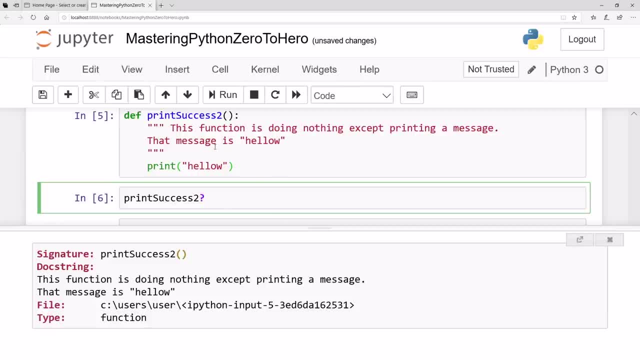 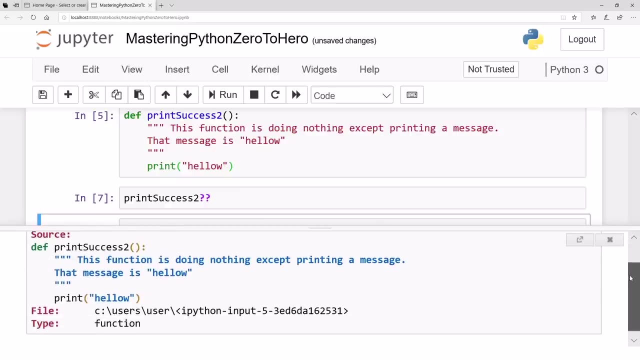 function and I will recommend to make your habit writing document strings every time you write a function. I was telling you that if you write a double question mark, then it will not only pull the document string for you, it will pull the whole implementation as well. so now, if you see you, this is the document string and that's the implementation. so whole implementation. 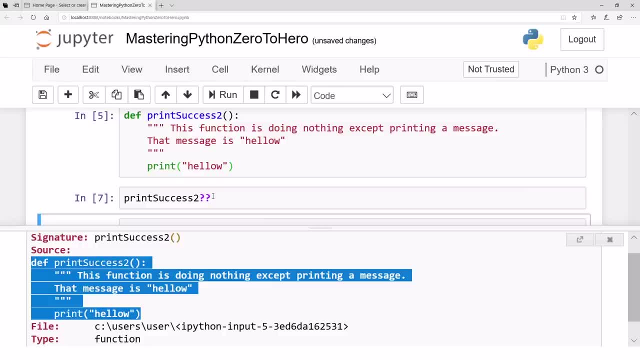 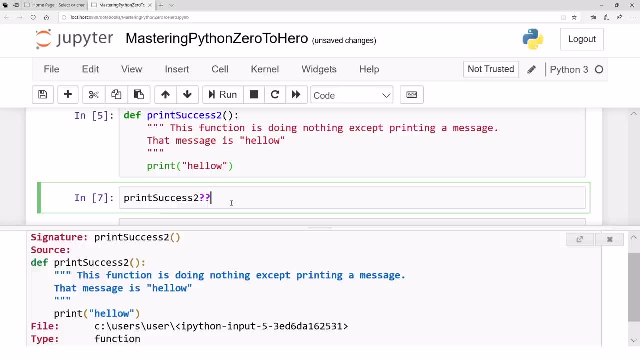 will be available if you want, and this is true for the functions that are that are. that are the functions that are third-party functions, or some other person have written that functions and so on. for example, you know a function length. we have called that function several times, so let's let. 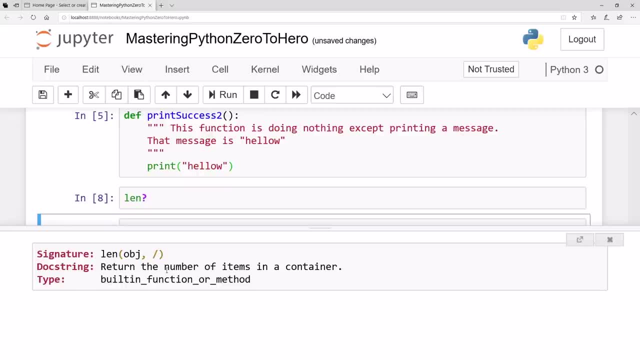 let's, let's see. so. the document string is: return the number of items in our container. that length function is not written by us. somebody have written that function. that's a built-in function, by the way, and we can. this document string tells us, okay, what this function is doing. we don't have. 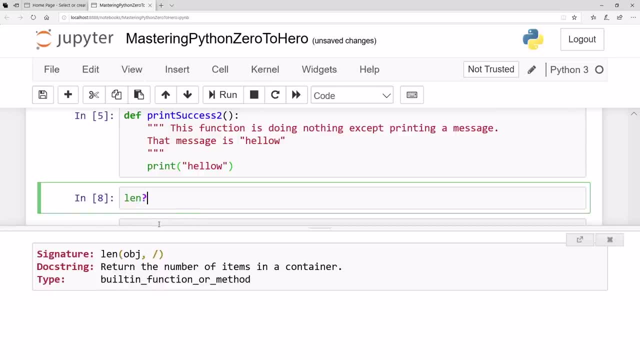 the implementation of that function. obviously somebody have written that function and and if we write double then we should get an implementation, as long as the implementation is not in C++. I haven't told you that a lot, of, a lot of implementation of Python itself has been done in C and some other languages- C mostly. 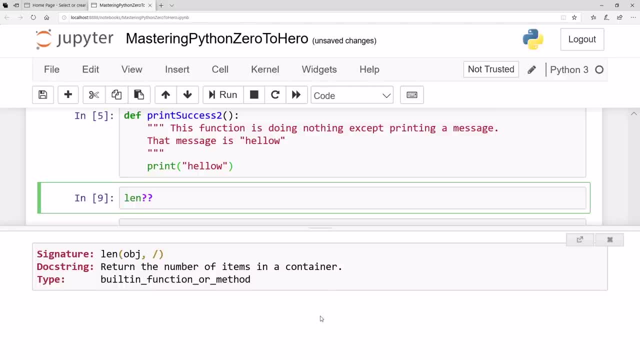 So several built-in functions. because of their speed, they are implemented in C and if you want to get their implementation, they get their code. the code will not be available for most of the functions, So whenever you write a double question mark and the answer is the same as a single question, 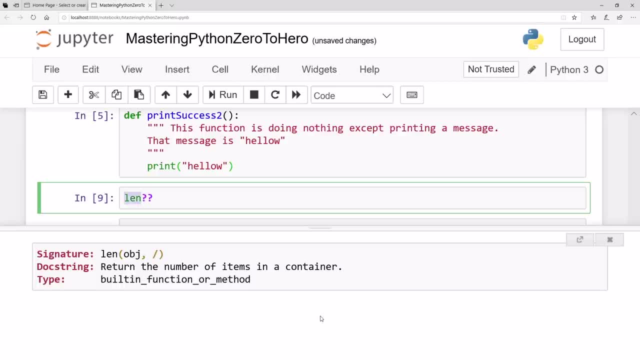 mark. that's an indication that this particular function is not written in plain Python. It is written in some other language and is used in Python. That's another versatility or flexibility of Python. you can engage multiple languages inside. Okay, one more thing. 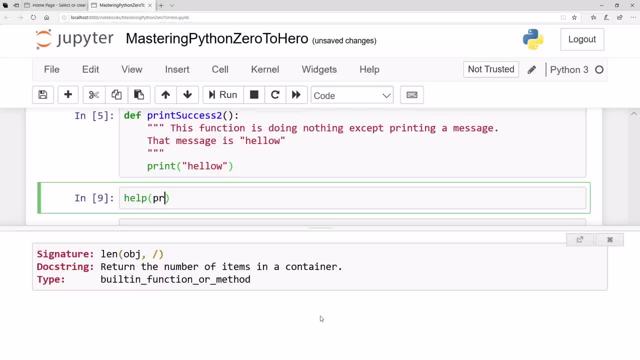 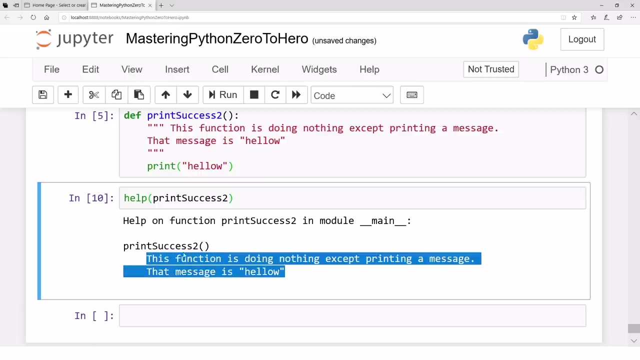 I can write help help command and I can get this print success success2, the help of print success2 by just typing this help command. So this help will tell us. you see, the help is telling us the document string I mean. 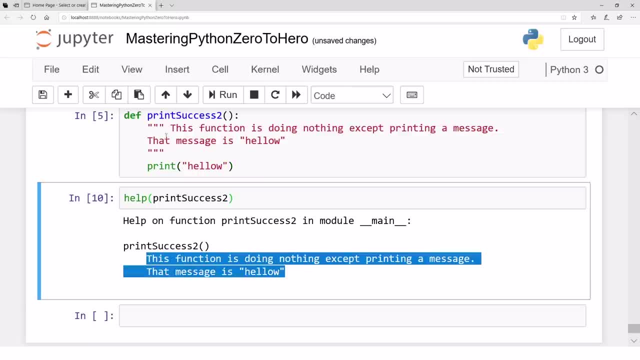 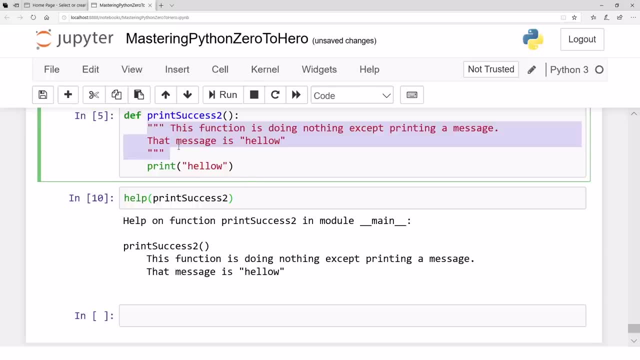 this help on this function, And this is the function we have written. this is the function we have written. This function is doing nothing except whatever description we are giving there, If, at some time, if we are supplying this function to somebody or making a package of, 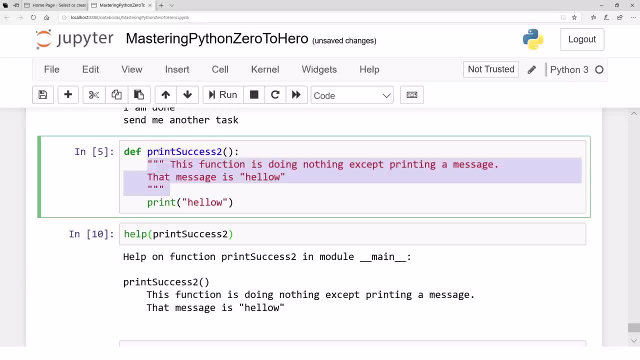 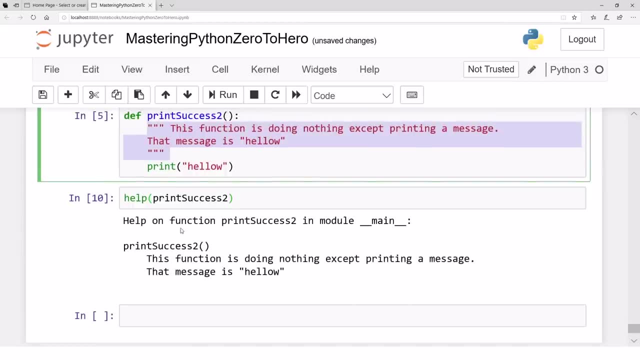 a lot of functions that we are writing. these document strings will help to get to know how to use these functions. By just knowing the function name we can. this document string actually tells us how the what the function is doing- Wow, great. 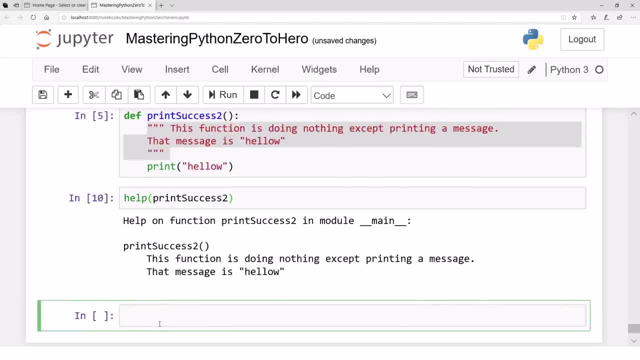 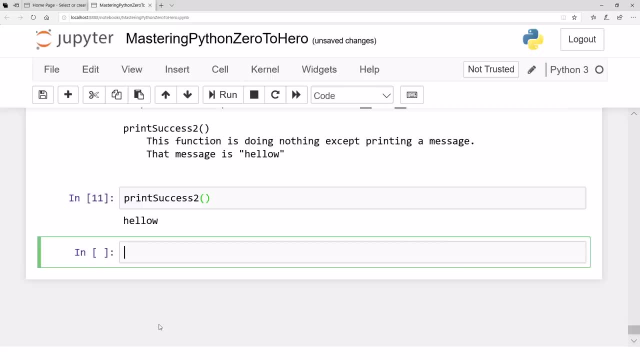 Oh, by the way, we haven't called this function yet. We are just playing with the document string. Let's call the function print. Now we know what the function is doing. Let's print. Let's call this function, And whatever written inside the function will be called C. This is only called. this is. 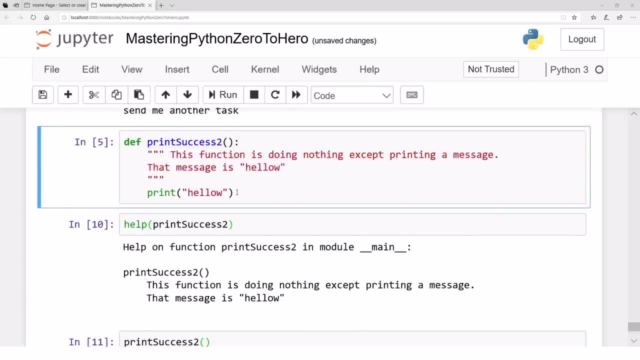 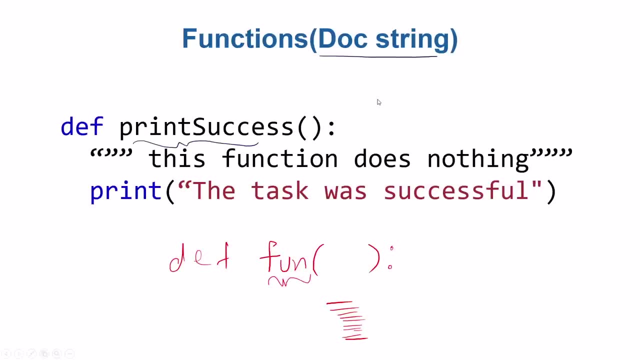 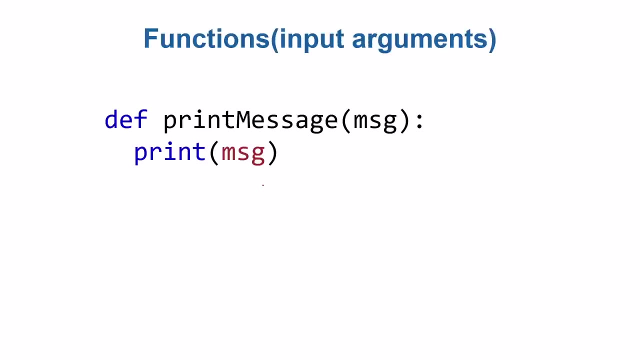 just acting as a comment and it is basically a comment. Okay, Yeah, Okay, Great, Stay with us. There is much more about function that we are going to tell you. Hope to see you in the next video. Okay, In the last video we saw document string. 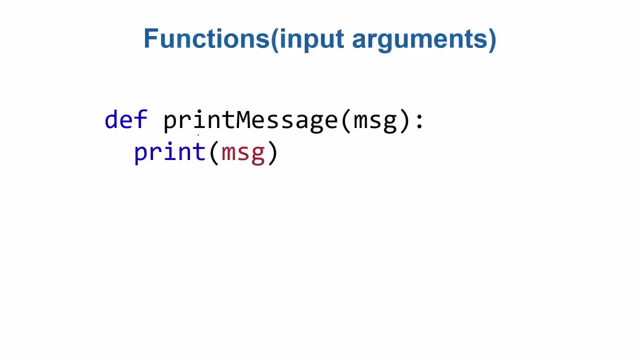 You might be thinking: what is power of this function if it is doing some static task? Well, in this video, I'm going to tell you that the function can, the coding or the behavior of the function can be dynamic, based on based on the arguments, based on some properties. 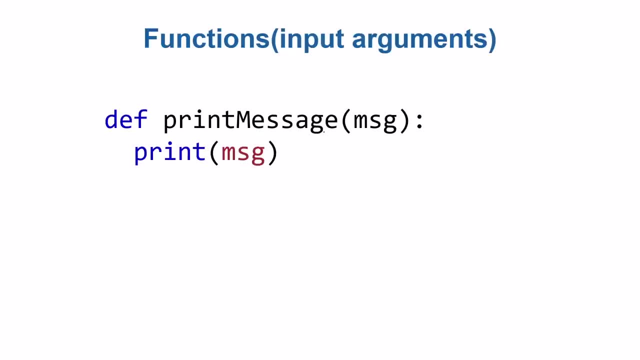 that you will be defining at the call time, For example, the. the function has in in almost all programming languages, the functions. the most interesting functions are the functions that receives an argument And an. an argument is just considered an argument just as a variable and performs its. 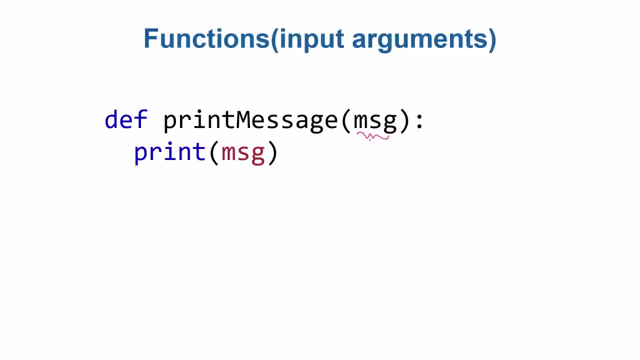 task according to that, to that arguments argument. Just take a single simple example. Let's say, rather than having a function print success, we have a function print message and it it prints whatever message it receives. And at the call time, for example, we call this function like: uh, so print message. 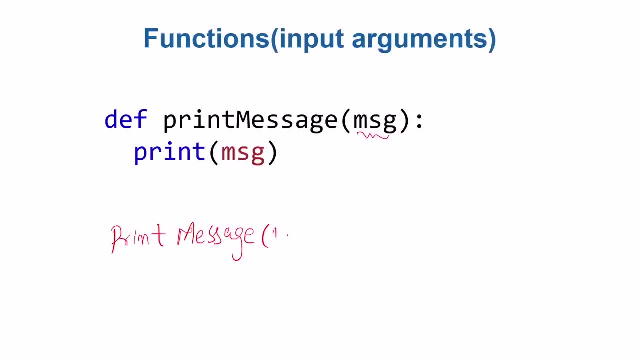 And let's say we call this as um, let's say success, Let's say, now, success will be printed. next time we call the function and we give another argument, Maybe in a string, let's say, uh, 74 errors. let's say: that will be, that will be printed. 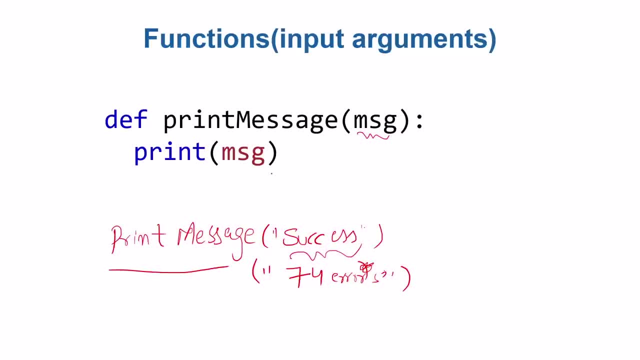 or anything. I mean anything that you supply will be printed. Wow, Isn't that great. I mean one function and, um you, you might be thinking, the plain print function does that? What's the power of this? Well, I'm just telling you the functions. the function does. 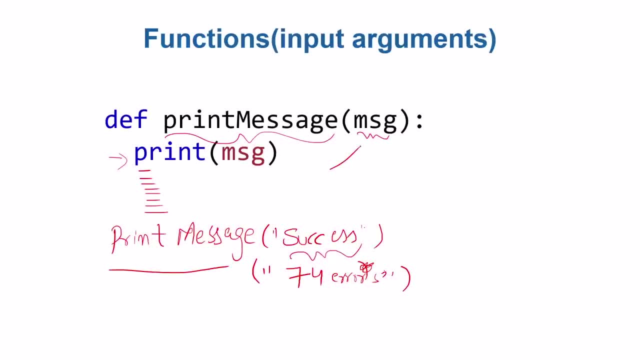 It does not only contain one line, I mean, it can be a whole task depending upon this input argument, and the whole task will perform dynamically based on based on what input argument you are supplying there. Um, you're noticing one, one thing that I that I just forgot. 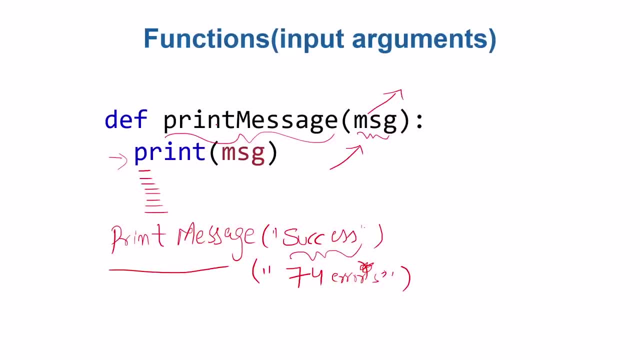 What is that thing? I define this function. Um, I guess everything is fine. I've just. I've just missed something. Oh, document string. I should have written document string, Although document string is not essential. Yeah, You cannot write document string. 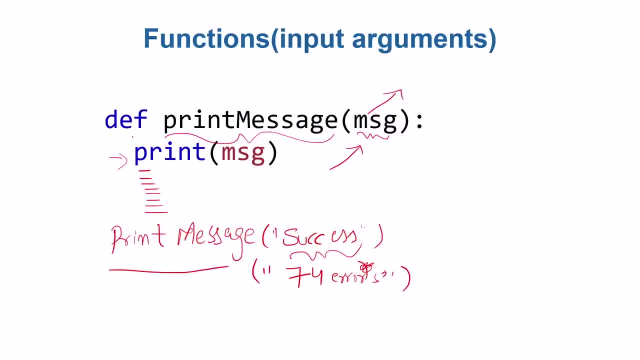 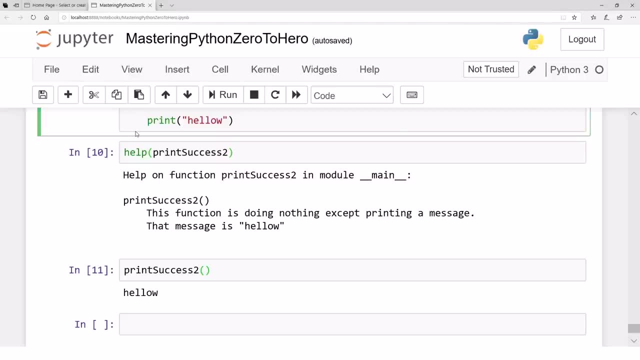 It's perfectly okay. The function will run, but it's a good practice. It's a. it's a good habit to always write a document string. Okay, Let's see the power of input arguments by again going to our good friend, Jupiter notebook. 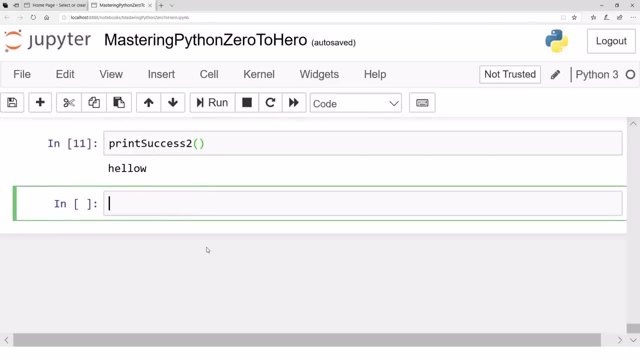 Okay. So let's see, Let's say we define a function, define print print message. let's say: and it receives an argument message, This argument is just a variable. It's just a variable And let's say we say okay, print message or further um. let's say we say um, if is. 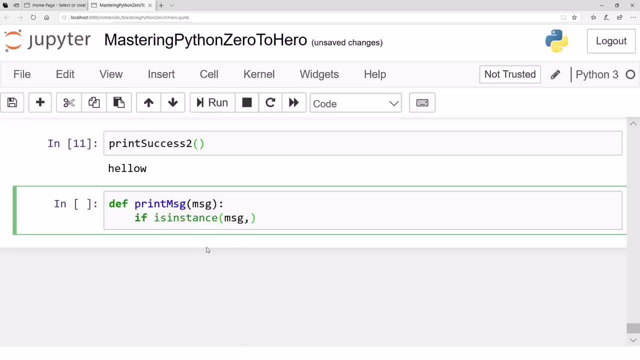 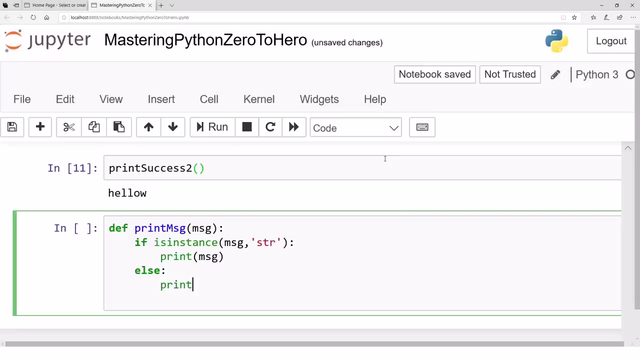 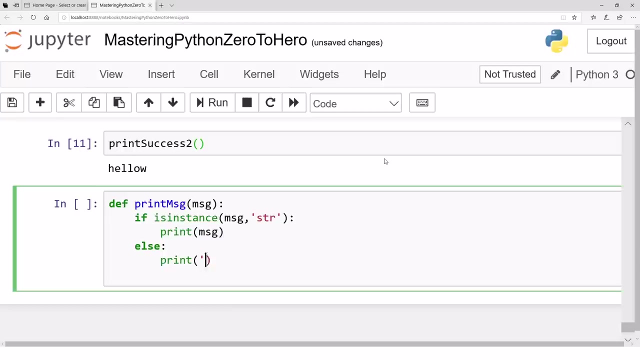 in stance message string. if this is string, then simply, then simply print it. If this is not a string, Then just say: okay, um, print your input. argument is not a string. And then you say: okay, print message. 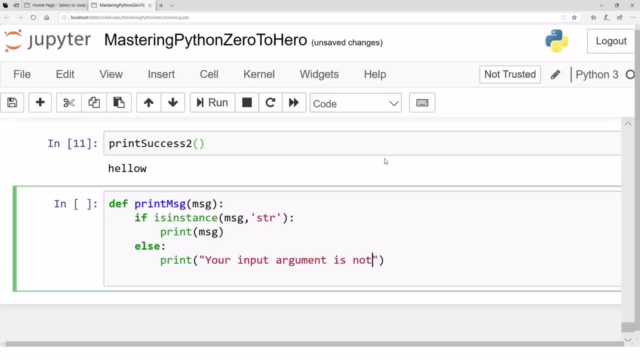 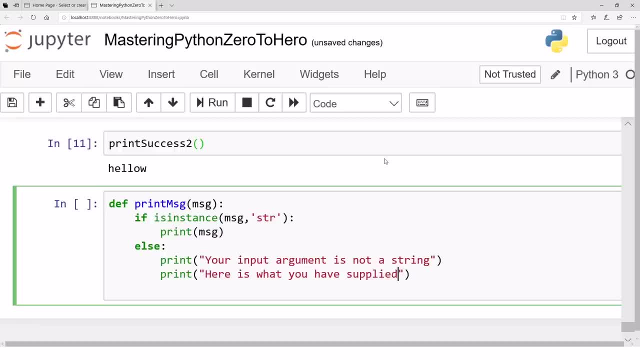 That's it, Okay. Um, so let's say you say here is what you have slide. And then you say, okay, whatever you have slide, just see Okay Message, And that's it. That's it, That's a function. 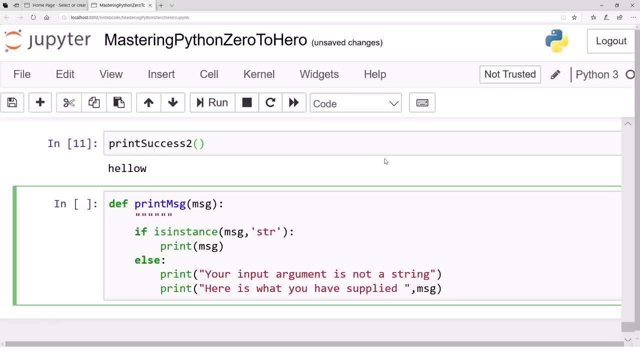 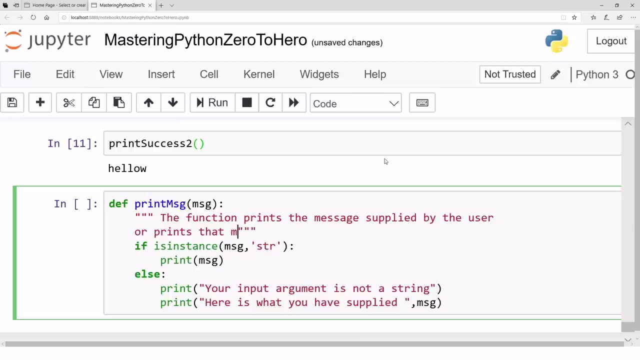 Um, we might have written a document screen for it. Um, the function prints the message Okay, message supplied by the user, or prints that message is not in the form of string. Wow, Don't worry, we have to see the strings in detail. We will see the. 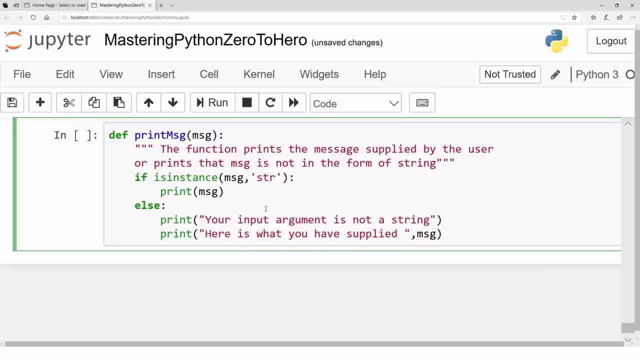 sprint function in detail as well, because the sprint has a lot of lot to do with strings. So just for now, I mean that's our function print message. Let's say, if the message is of string type, this string does not get. this is this should be simply STR. this should not be. that is instance. take like this your: 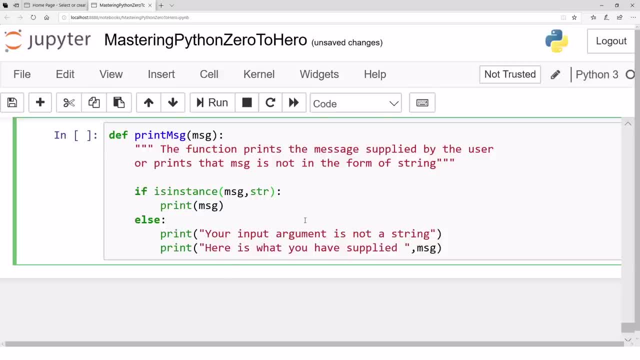 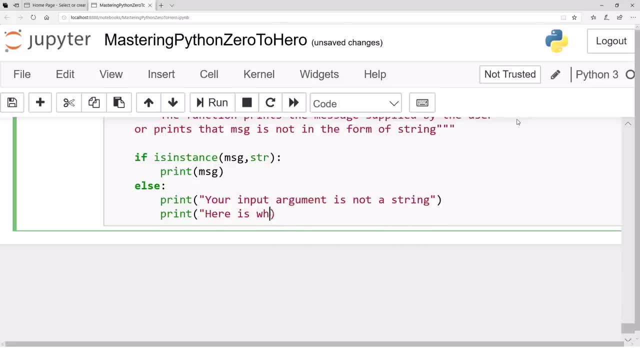 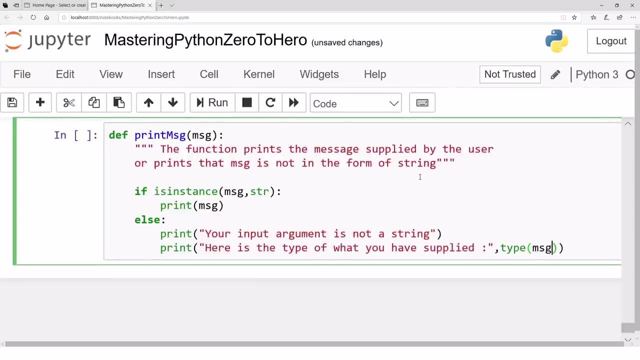 input argument is not a string, here is what you have supplied, here is what you have. so here we can. we can say: here is, here is, here is the type of what you have supplied, and then we can just print the type type: MSG. so the the goal here is to just write a function that prints: 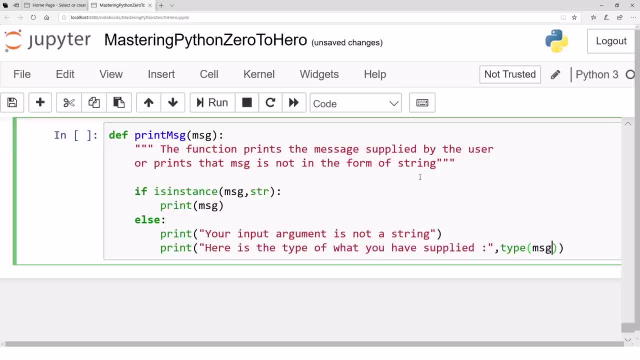 a message, if that message is in plain string form. if it is not a string, then it prints that: okay, you're the. the whatever you have sent is not a string. it is not a proper message in string form. let's say: this print message function receives a string. let's say: that's our logic or something, so let's run this. 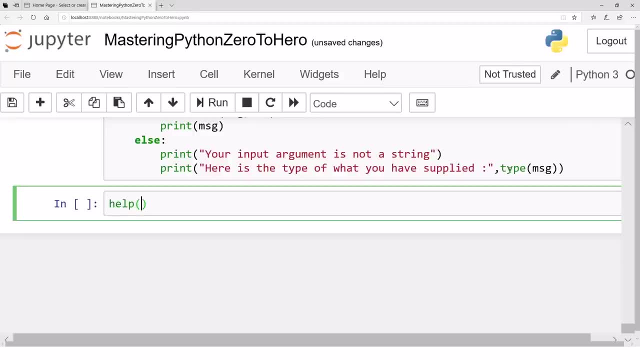 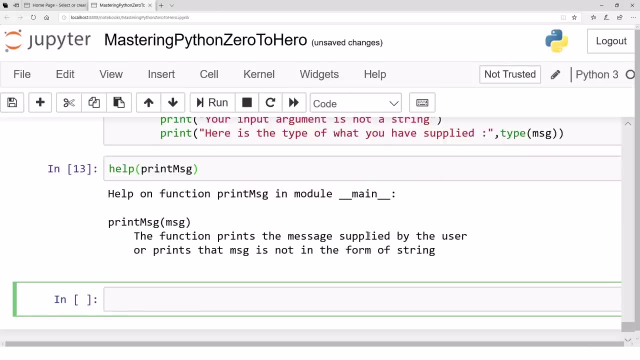 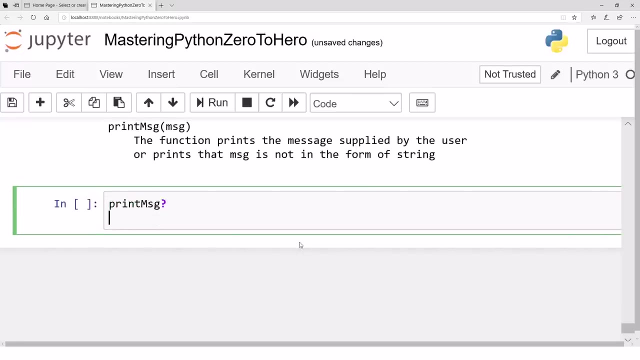 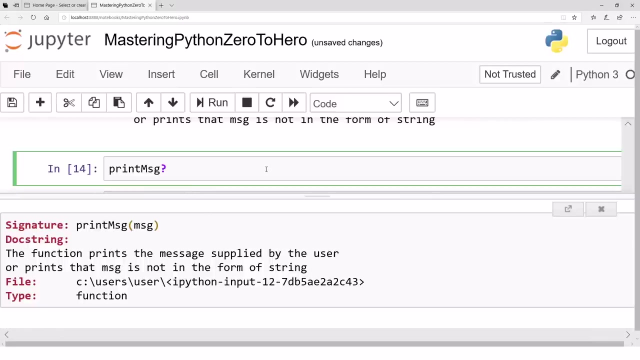 first of all, let's see what it does: help print message. so the function prints the message supplied by the user. we can access the same help by print message: left arrow. Uhh 印 to print message. right arrowого print message. So, in order to open a test Mark, if 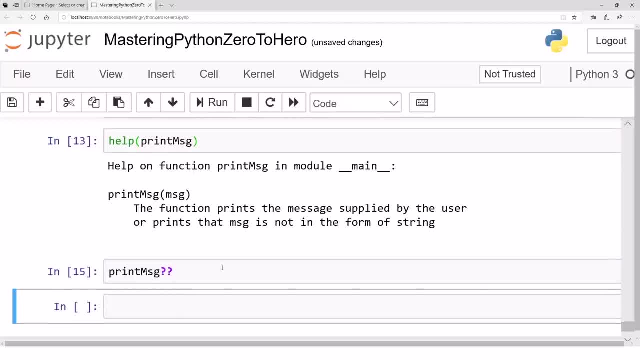 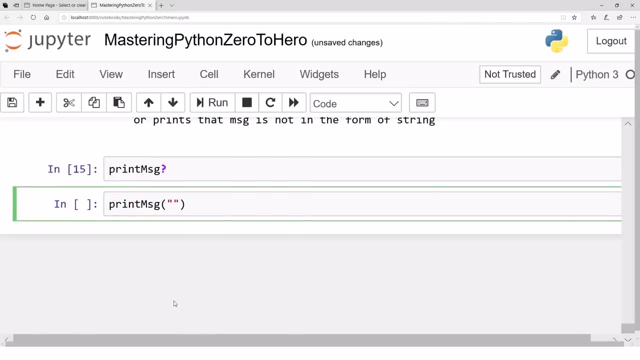 you want, and it gives us the document string. if, however, we want the implementation as well, then we write a double quote and the implementation is also available. Wow, great, Python is really great. Okay, let's call this function message and whatever you want to print, let's say: this is the message. this is the message. let's say: 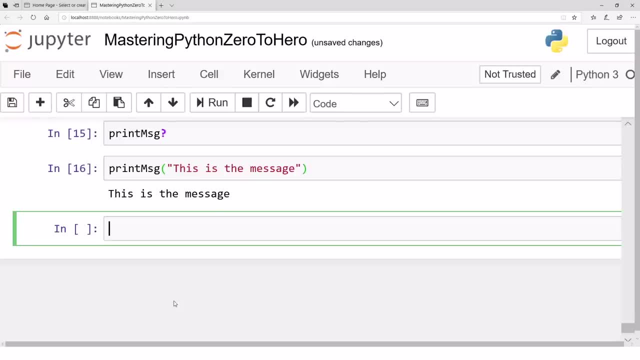 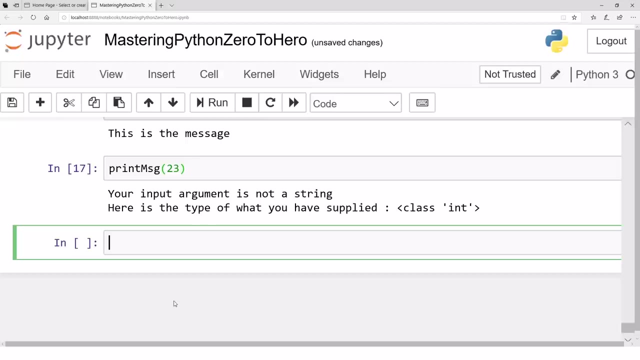 you want to print this and this is the message that's printed. okay, now let's say you call this function again sometime and you supply 23, and it will say: your input argument is not a string. here is the type of what you have supplied. it's an integer type, right, you can? you can have you. 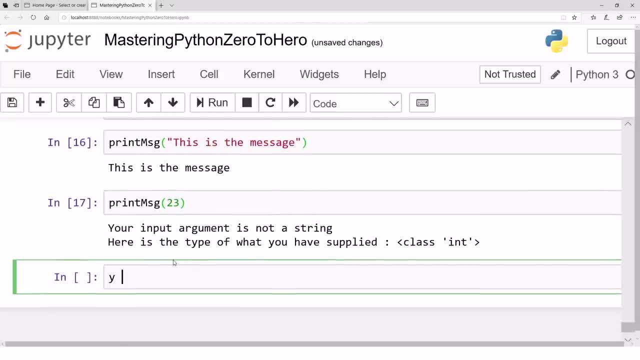 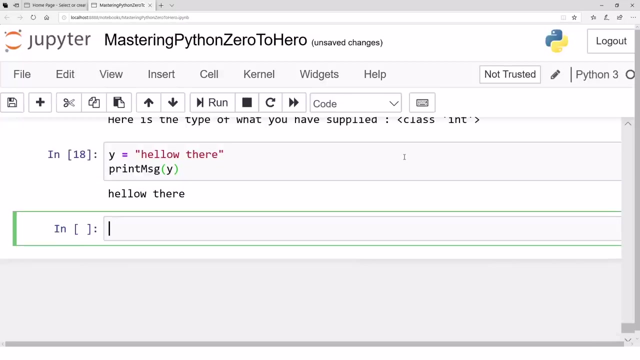 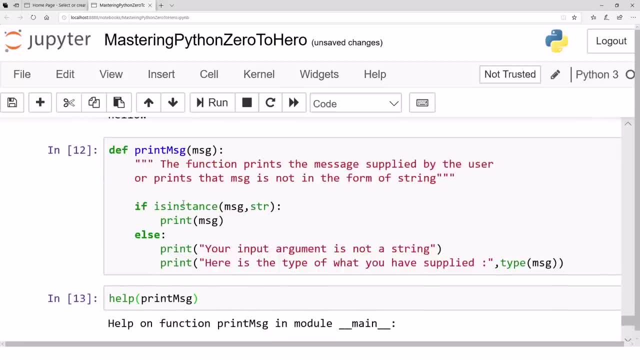 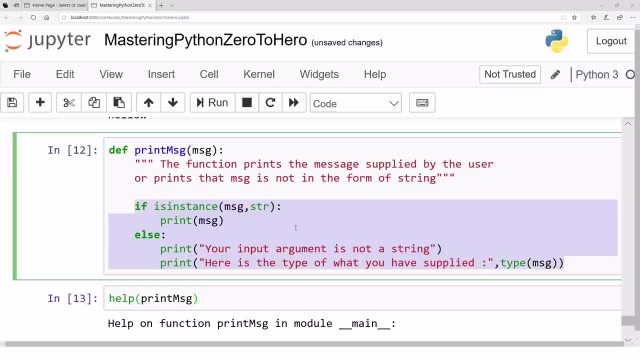 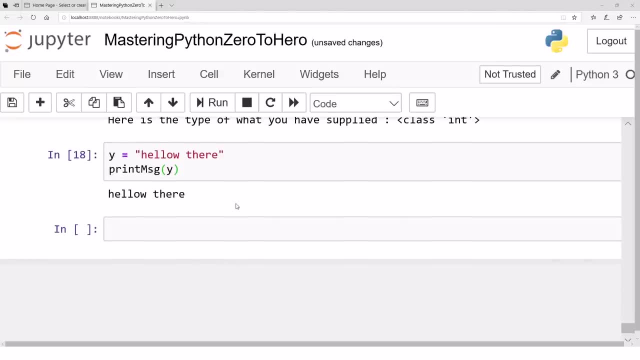 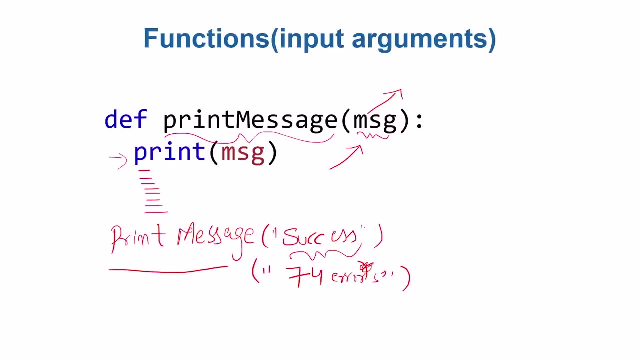 what the task you want to perform, and you need not to write that this again and again. whenever you need this kind of stuff, you just call that function splite arguments and it will behave accordingly. you want great, so you might be thinking that a function only receives one argument. maybe we want to supply more than one arguments, maybe maybe two. 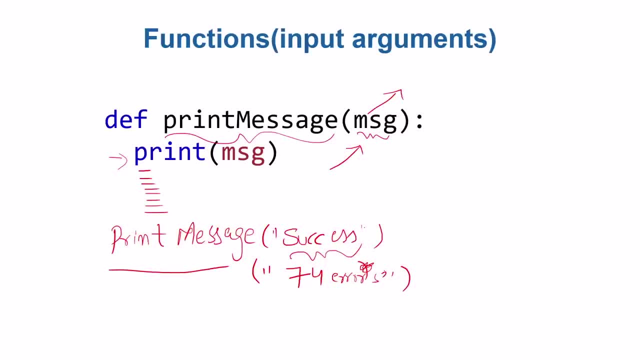 arguments, maybe three, maybe four, maybe five, and maybe we want to supply several arguments and we want to do some task based on the values of those arguments or or those variables. so in the next video I'm going to show you, uh, multiple arguments. okay, hope to see you in the next video. so in the previous video we saw we can define a function and 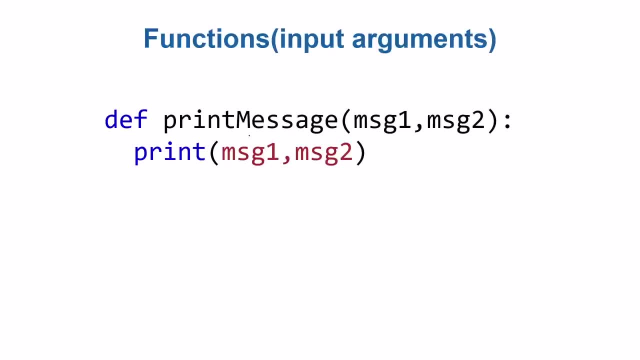 we can supply input argument to it and in this video we are going to see that we can actually send more than one arguments to the function. these arguments are just variables. these are just variables. whatever value we will supply to these arguments dynamically- because python is dynamically typed, dynamically, their type will be defined. 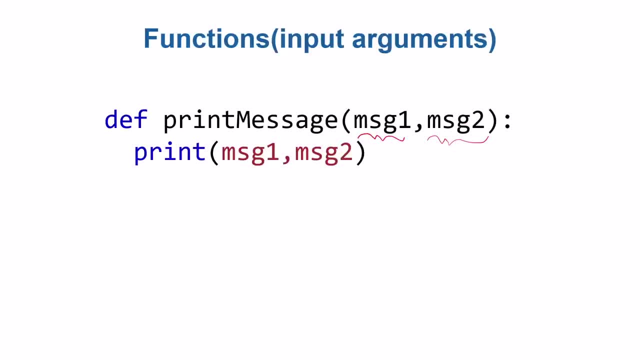 and, for example, here we have supplied just two variables and we just printed them, but based based on uh- supplying more than one input arguments- and based on what logic we are going to perform, we can do anything. we can do anything. so, yes, python allows us to supply multiple input arguments to 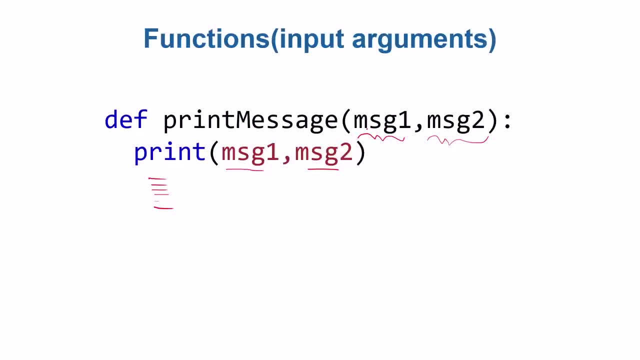 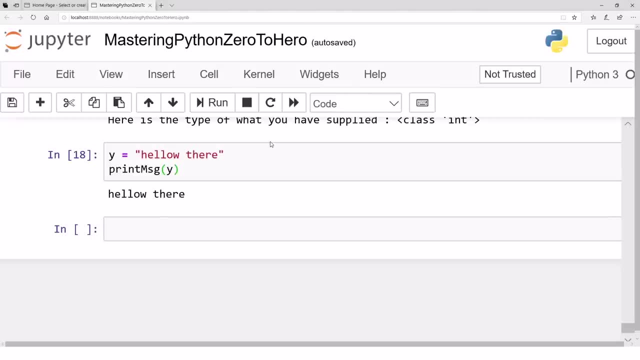 them and, um, and, and, and. we can. we can just perform all the tasks according to whatever logic we are going to do with that. so let's go to our friend Jupiter notebook and see an example of a function with multiple input arguments. let's say the function we. we define a function. let's say: 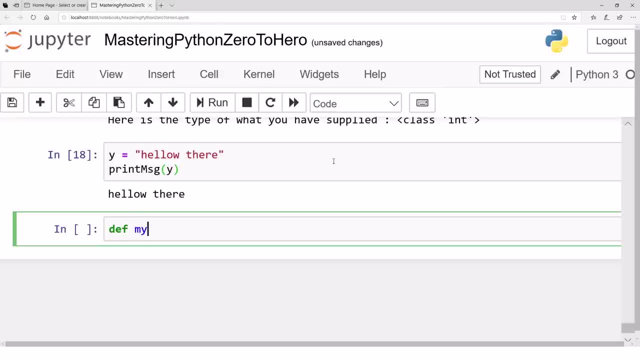 um, my power, let's say my power. let's say: you remember, there is a pow function in in python. that's a built-in function. I'm going to write my own function. let's say it contains a and b? um well, document string, um my. this function computes. 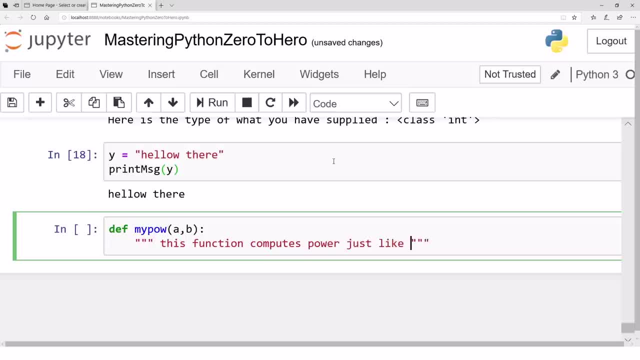 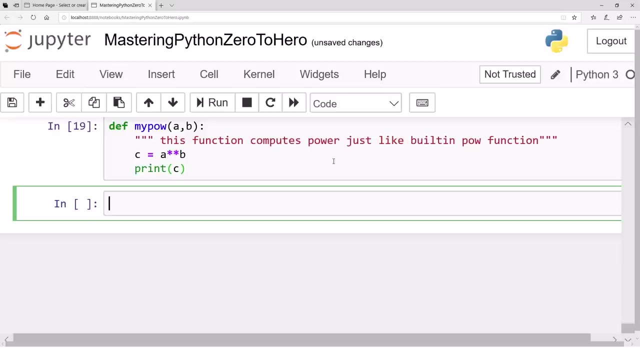 power, just like a built built-in power function. great, that's the document string. okay, uh, now what we want to do is we want to print: um, okay, let's, let's, let's create another variable, C, that is a power B. okay, then we print this C and we are done. let's say that's our goal. so we register that function by just just. 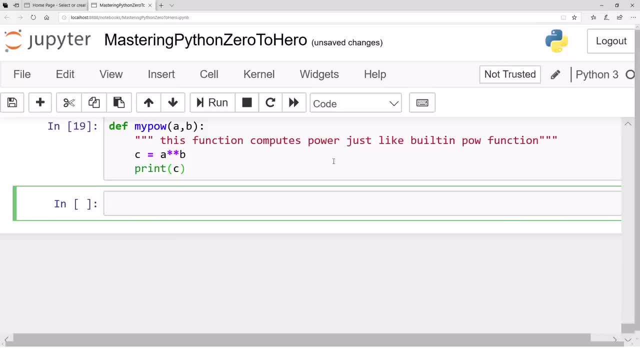 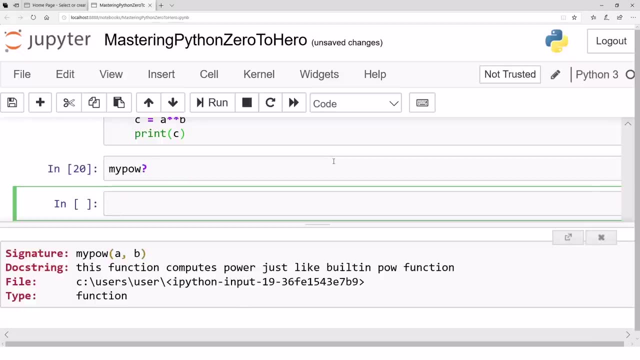 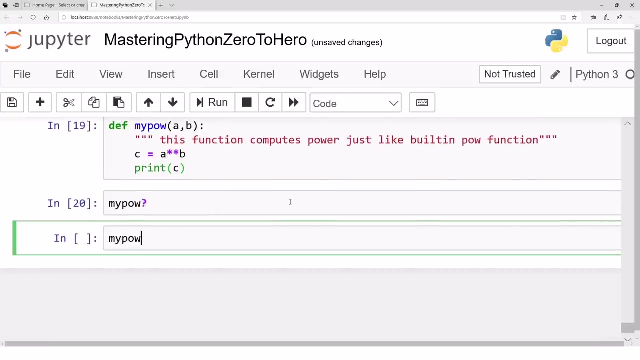 um calling the by just pressing the shift, enter in Jupiter notebook and now we um check what this function does. well, this function computes power, just like built-in power function. okay, just to just to remind you again and again the the importance of document string- I'm writing this again and again- let's run this function, my power. let's say three ways to the. 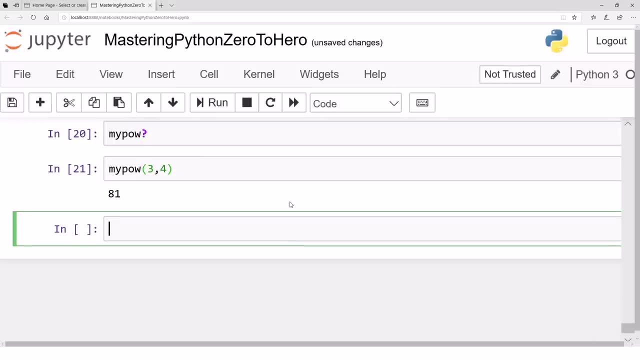 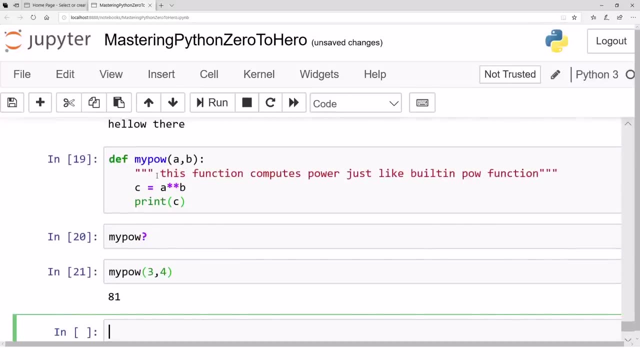 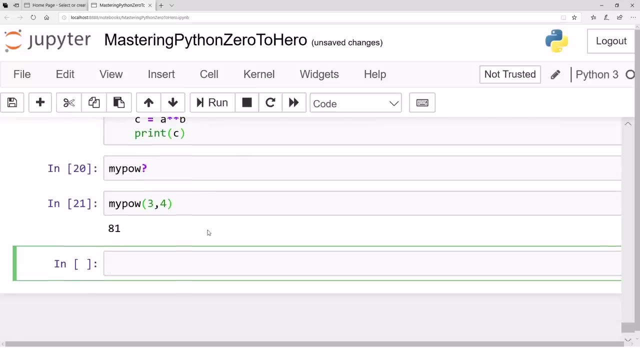 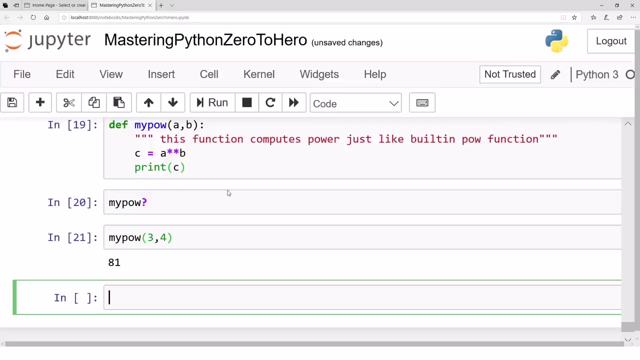 power four. I want this. so the result is 81. oh my God. so whenever, by the way, if you don't have pow function with you, although you have um, you can, you can create your function and whenever you want to use, you can use your function. not a big deal, um, yeah, by the way. um, what if you um? what if you um? what if you let's, you can. 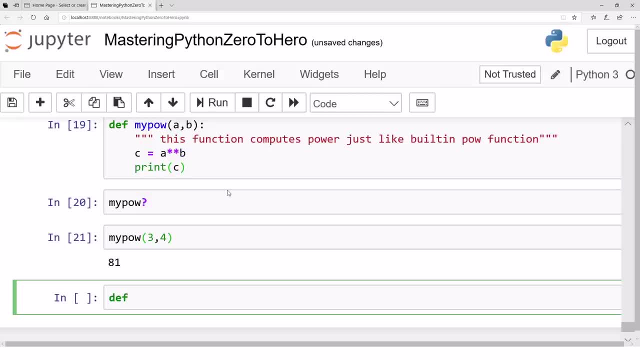 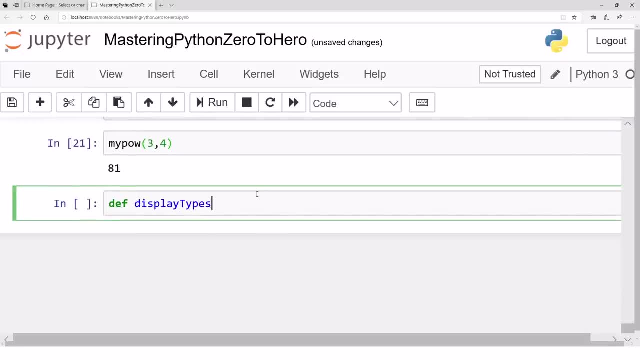 you can define a function with more than two arguments. define, let's say, um display types, let's say that's your function. display types- and all you know is um, are our check arguments. let's say check arcs, let's say that's your function. and A, B, C, D, let's 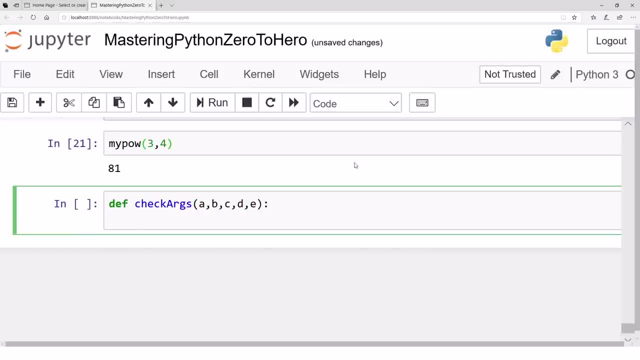 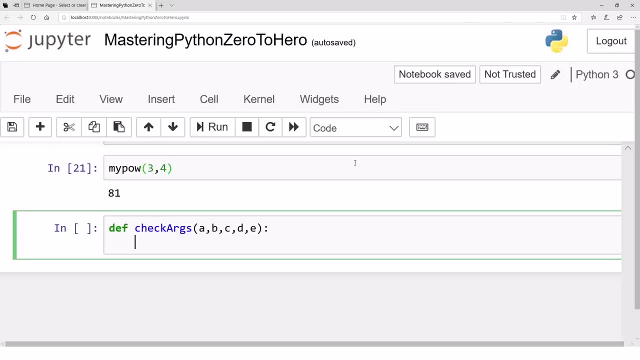 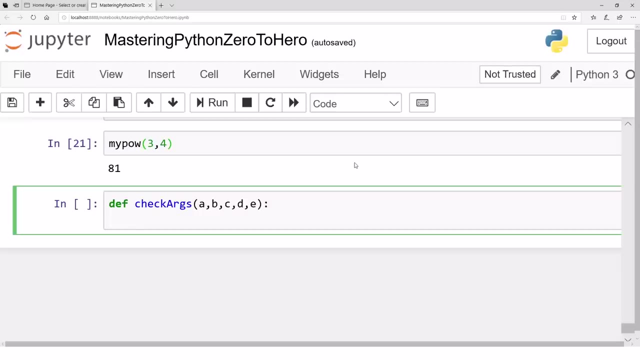 say E, these are the input arguments. and let's say, uh, at some task, you know whether all the five variables that you are working in somewhere, whether all of them are numeric values or not. if they're not numeric values, you're not moving on and you are doing something because you were expert. let's say you: 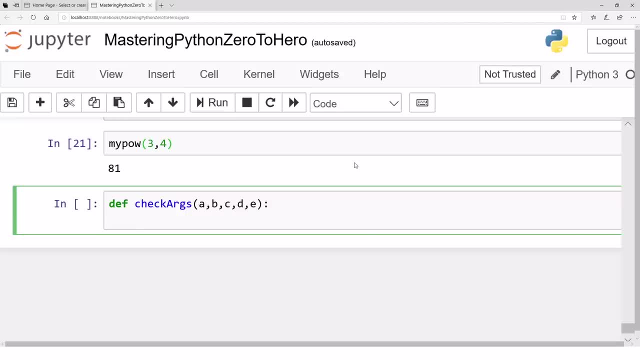 are. let's say, you're taking input from somewhere, reading from a file or whatever, and you need to. you need to check before moving on, whether ABCD and E, whether they are ints or floats. otherwise, if if any of them is not int or float, then you're not processing, then you're not moving on and you are. 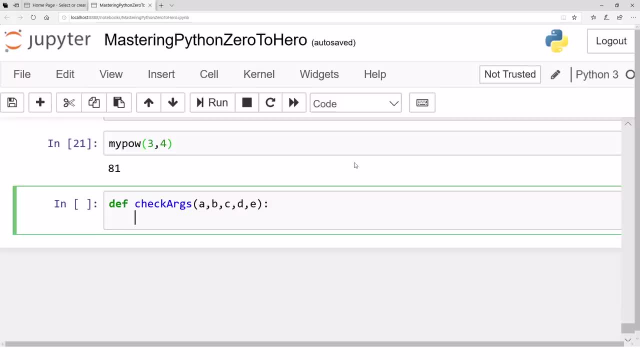 going to check the input arguments again, and so on. these kind of functions are there because whenever you call certain, whenever you want to do processing on data, sometimes it is required to check the type of the data, whether the data is supplied in a way that you were expecting, and so on. so let's have this. 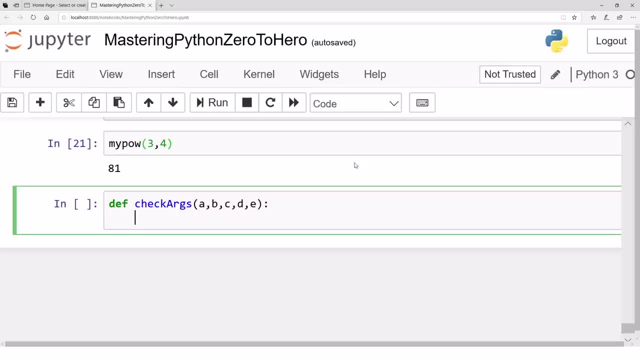 function check orgs writing document string here. I guess I've told you enough to write document string again and again. so let's say: if is instance a, if is instance int, float, if that is true, and let's just have three variables just to just to focus on. if is instance a, then 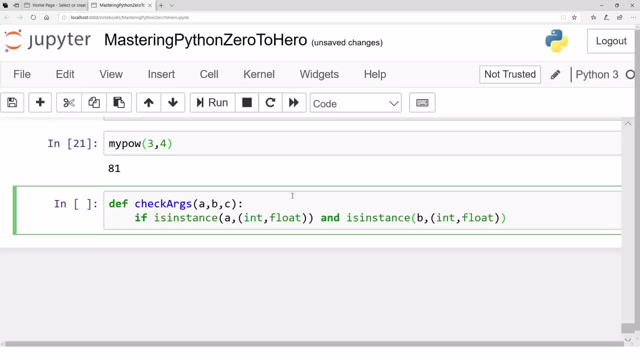 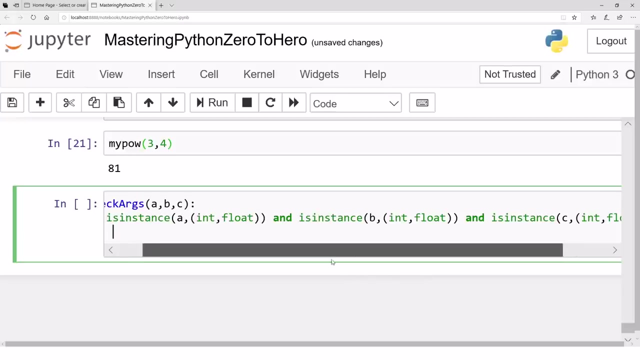 be and is instance C if all of them are, if all of them are, them are, if all of them are integers or floats, then do something. then let's say print a plus B plus C, maybe, or a plus B plus C raised to the power 2, just print. 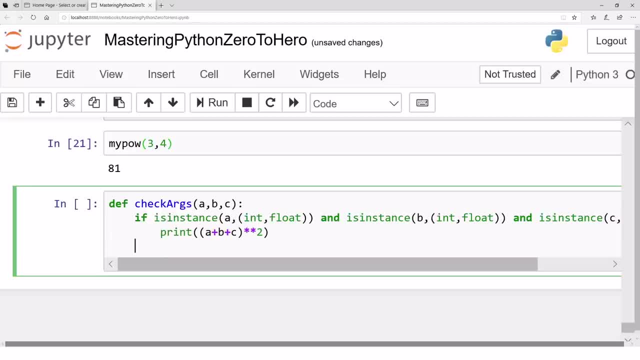 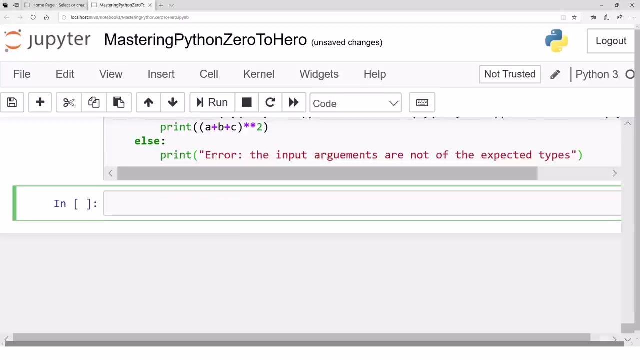 their square. let's say else: or, or, if they are, if they are all integers or floats, then do some interesting task here, some task. otherwise you can say: okay, print error, the input arguments are not of the expected types. fine, you have this function. let's say: let's call this function the function. 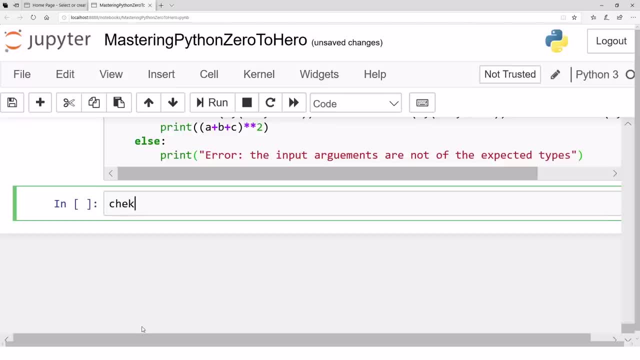 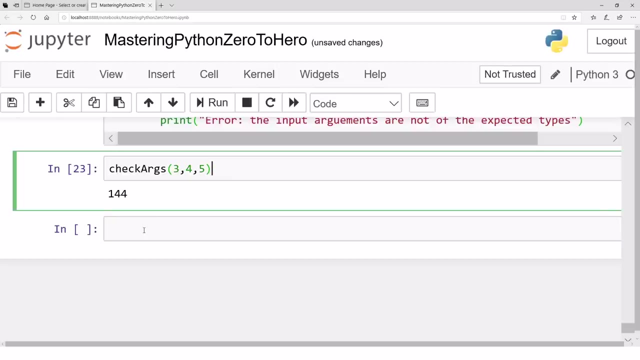 was check args. so let's check args, check args, check args. let's say three, four, five, so now you have all of them are great. let's say you have check args and you call this check args on. let's say three, four, but this five is a string. let's say: 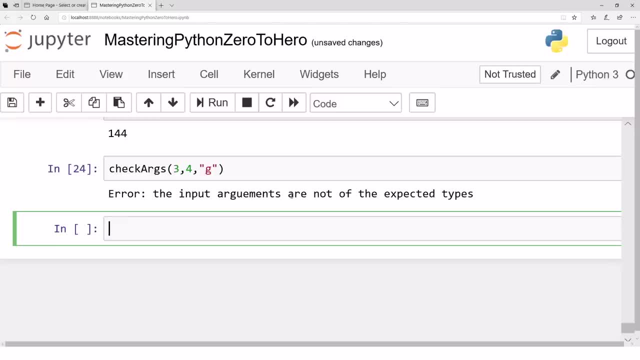 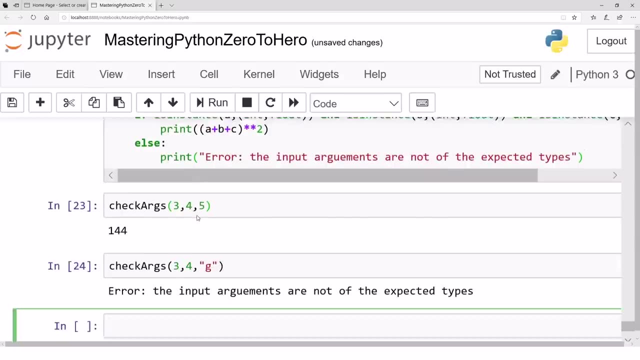 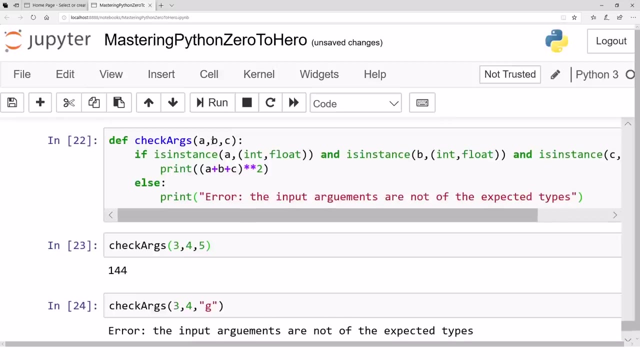 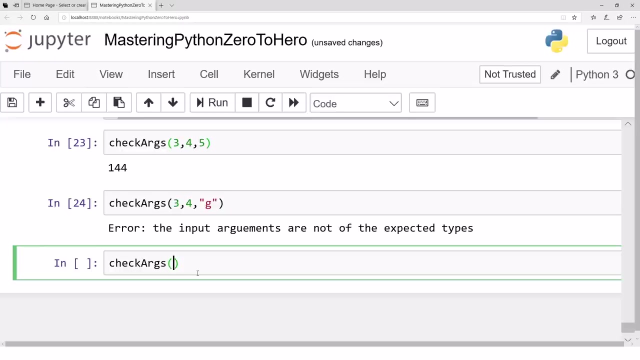 G. now you'll be having an error. the input arguments are not of the expected types: one of them, or more of them, or whatever. yeah, one more thing: the this function is expecting three arguments. if you call this function by less than three or more than three arguments, you'll be getting an error. for example, three, four, although this function is. 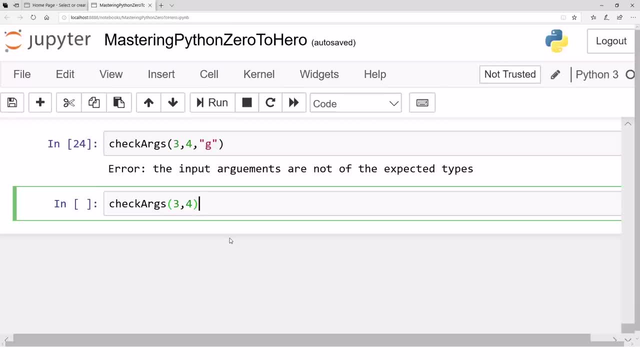 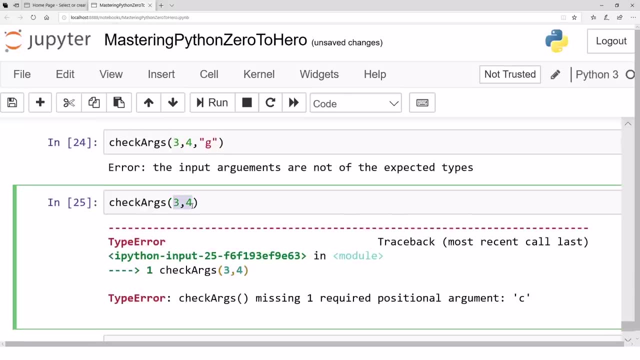 accepting three arguments. you are calling it with just two. you're getting an error because you have not specified all the arguments that the function is requiring, although the the arguments that you have supplied, they are of the type that it is expecting, but you have not supplied this. 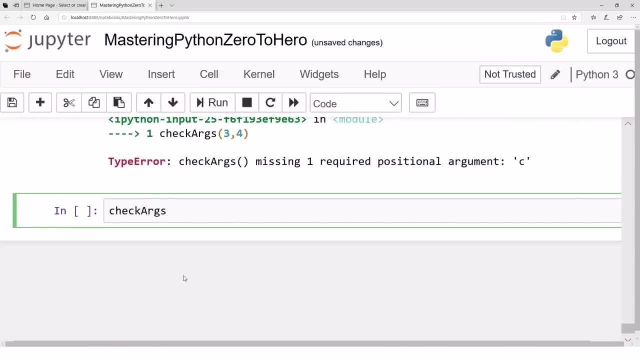 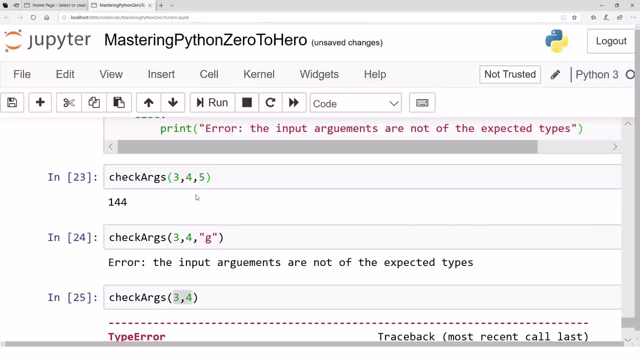 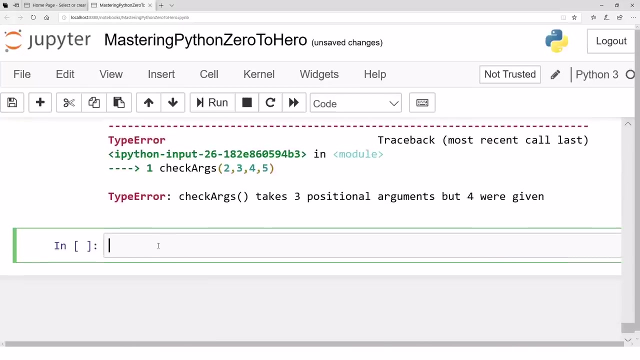 the the number of arguments that the function is expecting. similarly, if you call this function by more than three arguments, although it requires three arguments, you again will get an error because it is expecting three arguments and you have not applied supplied three arguments later on in in later on, we will see how to write a function that accepts variable number of arguments. 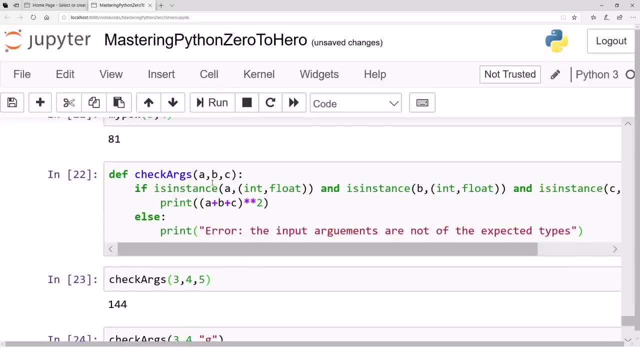 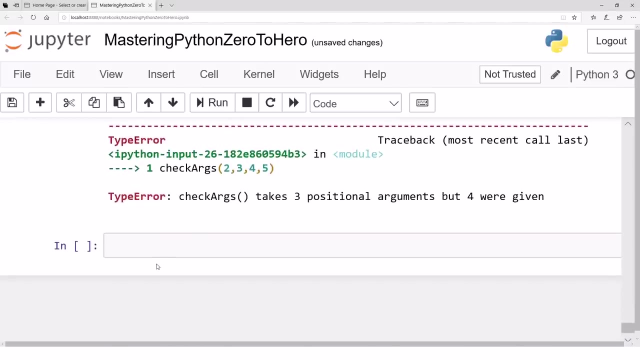 we will see that, but right now, in this particular way, if you write the function and if you define the function in this particular way, you have to define the arguments, the number of, whatever the number of arguments it is expecting. you have to supply exactly as many, otherwise you are getting an error. 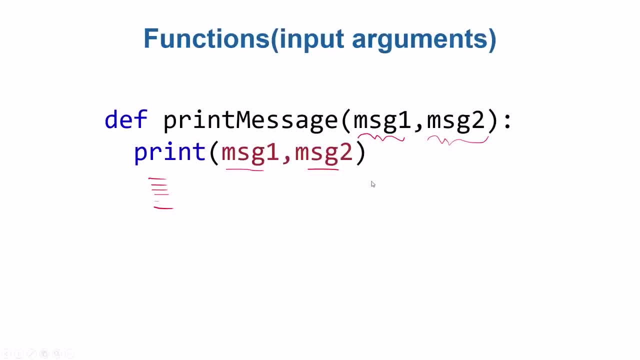 okay, so that's about the multiple arguments. um, okay, what next? well, um, next time in the next video we're going to look at: uh, what is the what's the importance of order of these input arguments? what will happen if i just swap message 2 and message 1? will that? will that change the behavior? 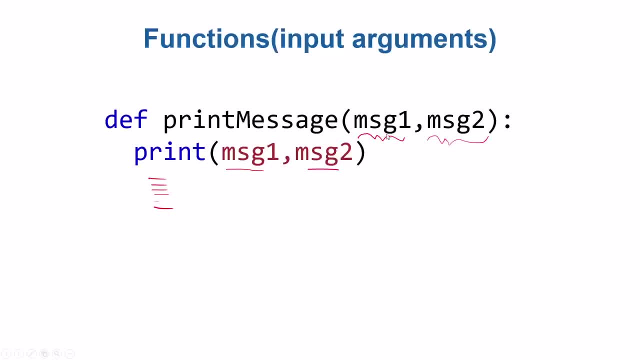 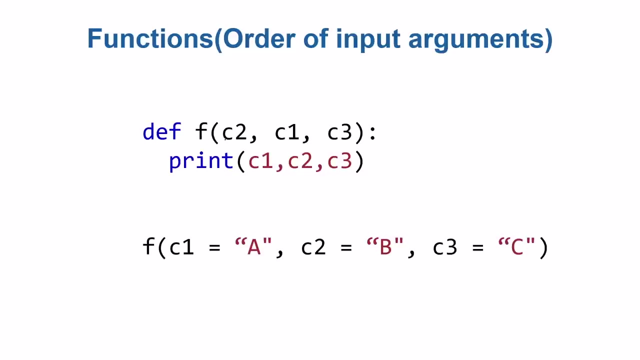 or is there any order? uh, with the first mess, the first variable, the second variable, third variable. is there any ordering inside the input arguments? um, yeah, there is. so let's see in the next video. in the last video we saw how can we pass multiple, how can we define a function with more than one input arguments. 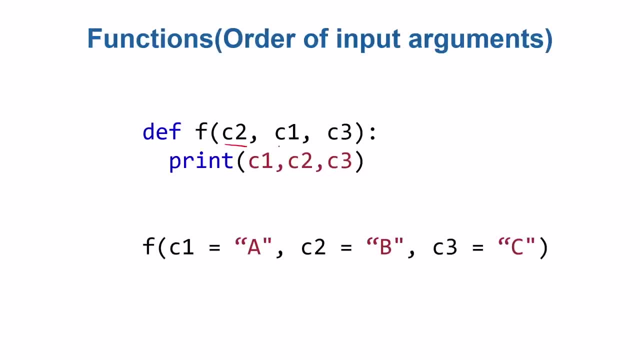 it is important to know that the order of the input argument is really, really important. so, whatever argument at the call time, for example, if you call this particular function, the name of the function is f, that's not a great name. you should have a name that is descriptive. but 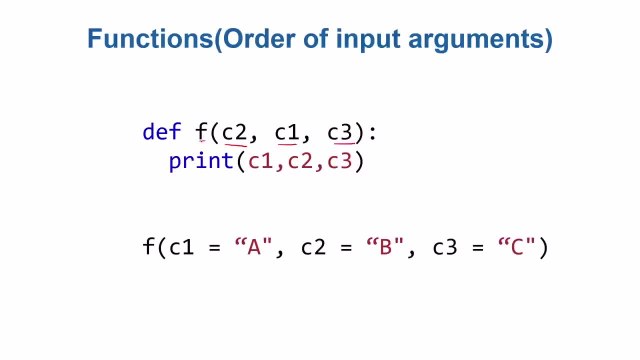 i recommend to write good names. let's say: this is f, that's a function, and the very first variable is f, the second variable is c1, the third variable is c3. now you, let's say, call this function like, like this: let's say, 2, 4 and 9.. what will happen is this 2 will be copied in c2, this 4 will be. 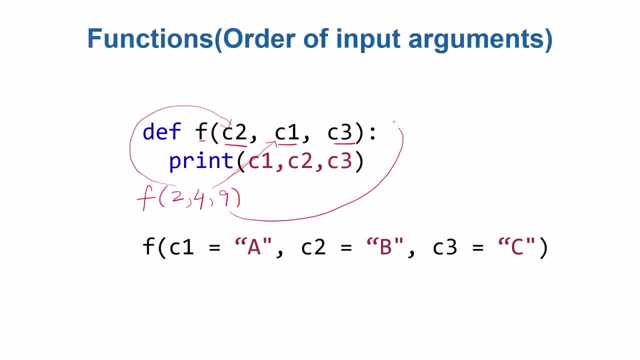 copied in this c1 and this 9 will be copied in this c3. now, c2 has a value 2, c1 has a value 4 and c3 has a value 9.. 9. if you change the symbols or the variables order here, whatever order you have written there, 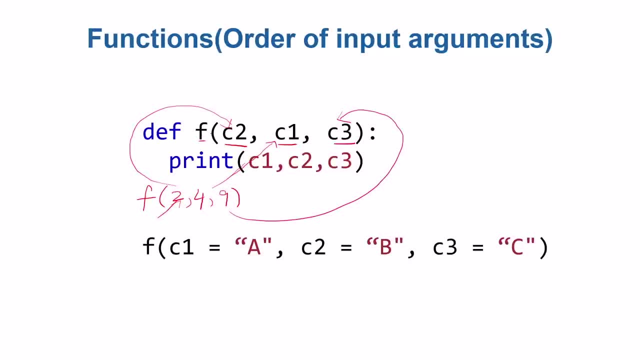 the first value that is passed at the call time will be passed to the first variable, whatever the name of the first variable is. the second value at the call time is copied in the second symbol, whatever the name of the symbol is. so this ordering is really, really important, one way to. 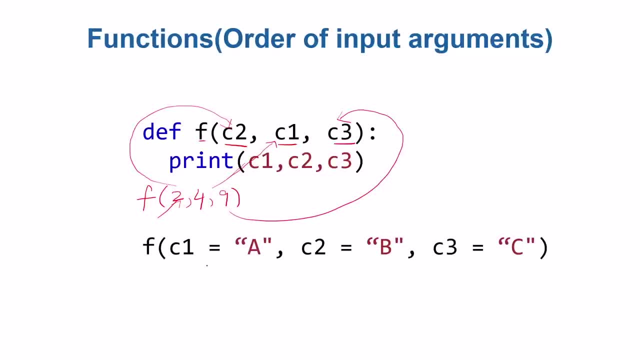 work around, for this is at the call time you actually define the variable names and their values. for example, you call, you call f and you say, okay, c1 has this particular value. but this way you need to know that there is the symbol name in definition is exactly c1. 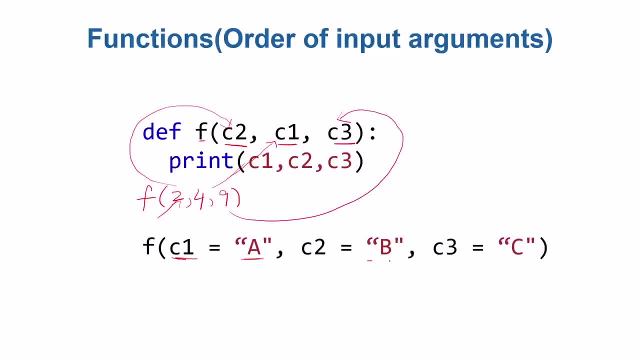 so c1 has this value, c2 has this value, c3 has this value. once you, at the call time, if you have defined your variable names along with their values, then you are order free. now you change whatever. whatever. if, for example, you call this way: c2 is b, c1 is a. now, no matter in what order you have. 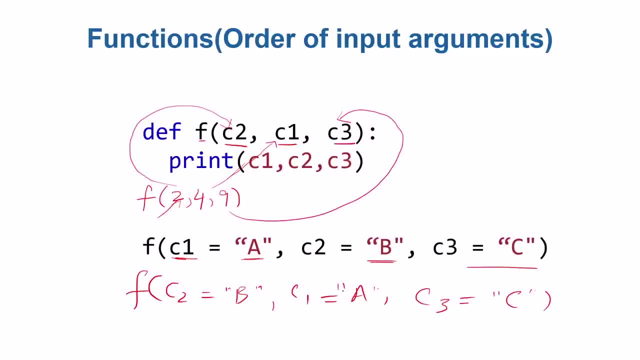 called these: this c1 is going to be copied in c1, this c2 is going to be copied in c2, C2 and this C3 is going to be copied in C3.. For the functions: that has many more arguments. it is good to call the function in this particular way if there is a chance that calling a function 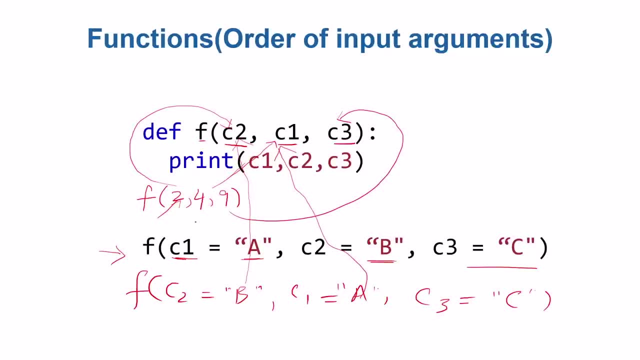 in a different order may become confusing and stuff like. so This actually gives you more grip on this ordering issue. If you are very smart and you say: okay, I will always supply in a particular order, I will always read the document string first and then I. 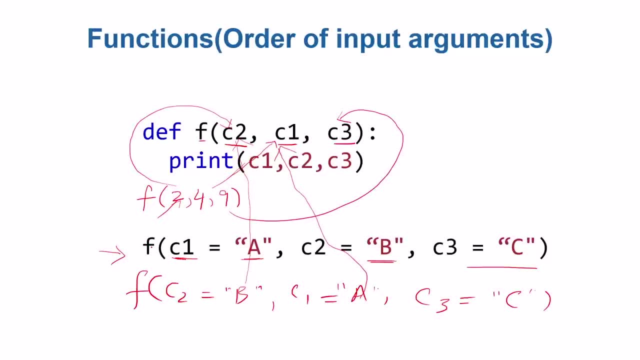 will call that function. that's okay. Otherwise, this is also a feature that is available At the call time. you assign the values of the functions that are there at the definition time and now no matter in what order you are calling that function. C1, a call time. 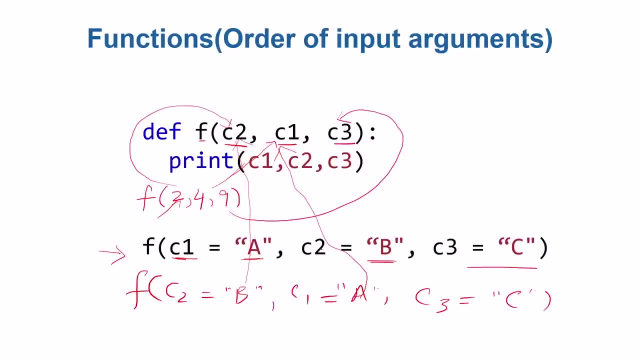 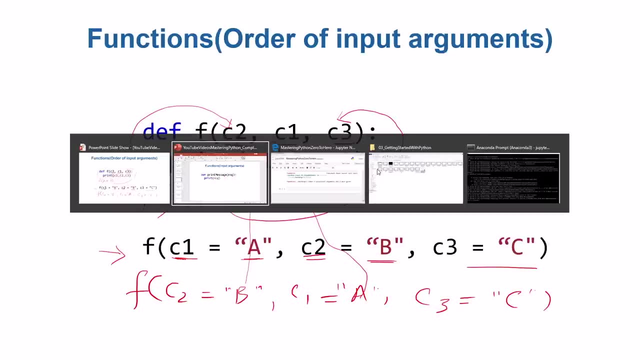 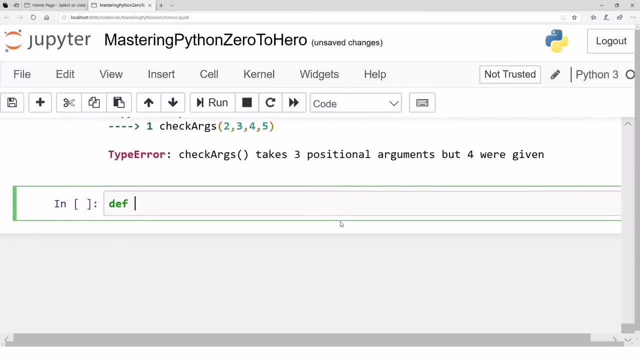 occurs at third position, C2 occurs at first position, the relative values will be copied according to their names. That's a good feature. That's a very good feature. Let's see, for example, a running example of this in Python, in Jupyter Notebook Define, let's say function. 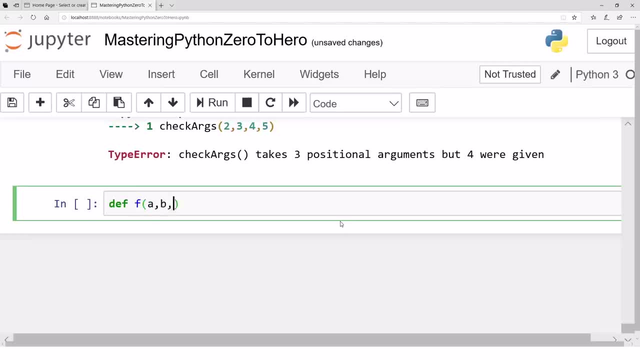 f. Let's say it receives a, b and c. Let's say three values. Let's say it prints. let's say a is, let's say it's print a, a is a, and you say: okay, b is b, and then it prints. 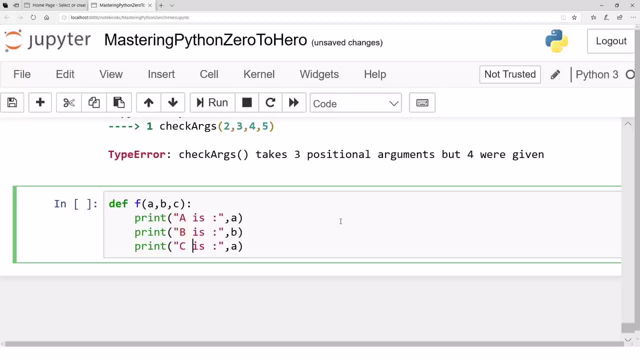 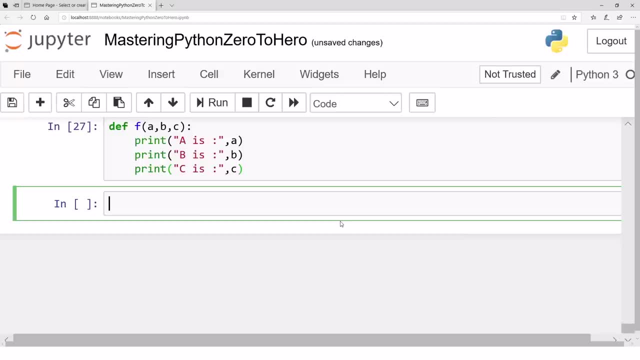 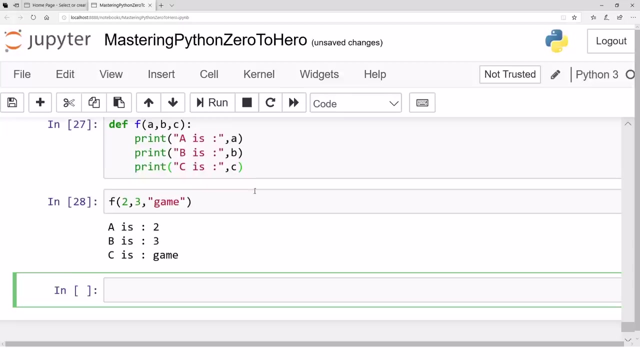 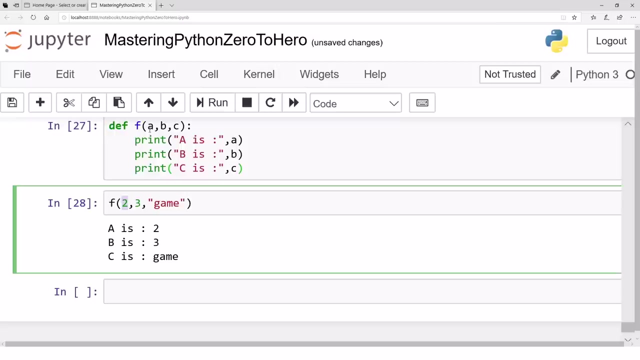 okay, c, c is whatever the value of c is. let's say c. Okay, Now let's call this function f with, let's say two, three and game. We will say, okay, a is two, b is three, c is game. Fine, great, Now this two will be copied in a, no matter. 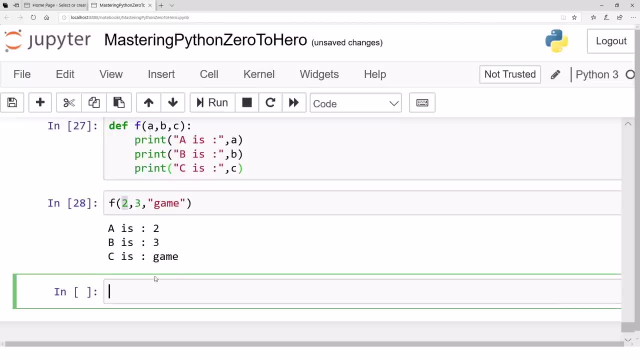 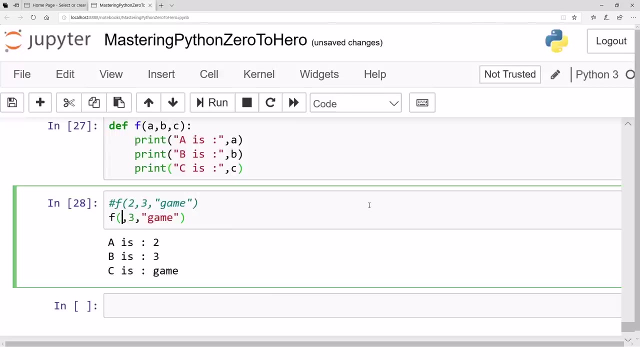 what If we change this calling order? for example, if we change this order, we just move to, we just move to this particular order. we just say: okay, this is three, this is a game, this is two. If we call like: so now, three will be copied in a game will be. 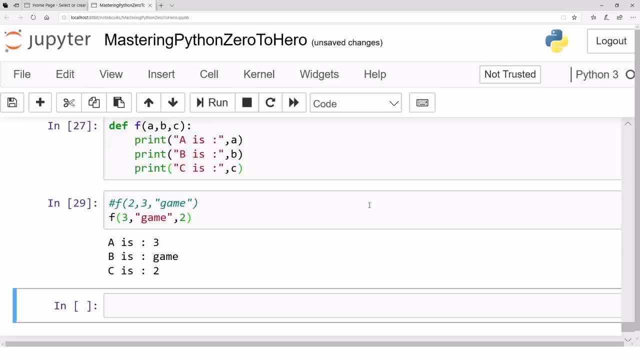 copied in b and two will be copied in c, And that, if that is the behavior you want, then you are good to go. Otherwise is, it is handy to call the function in the following way, to just fix: okay, a is a is two, fine. 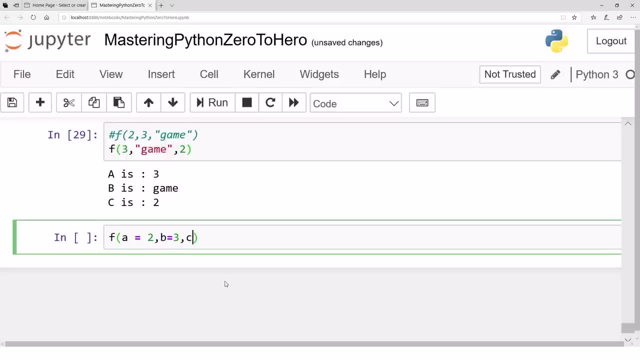 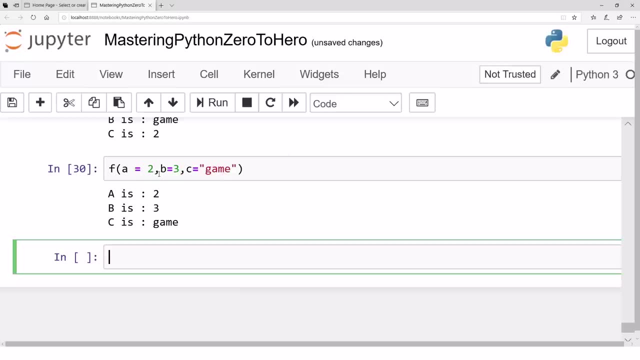 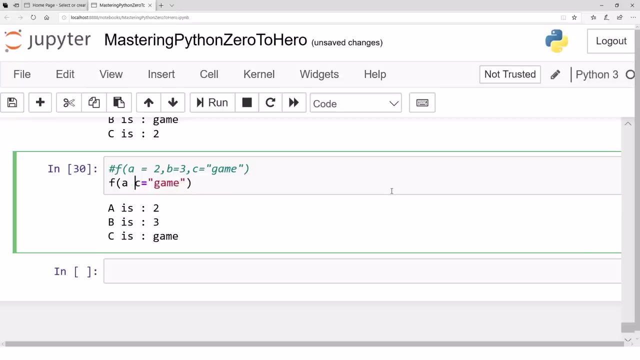 b is three and c is, let's say, game. if you want these numbers now, if you call the function like so, that will happen now. if you change the order, no matter what order of at the calling time you come up with, it will stay the same. for example, you go and say: okay, um, c is at the first position and 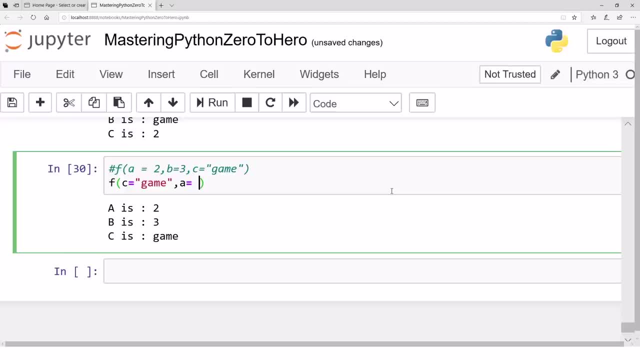 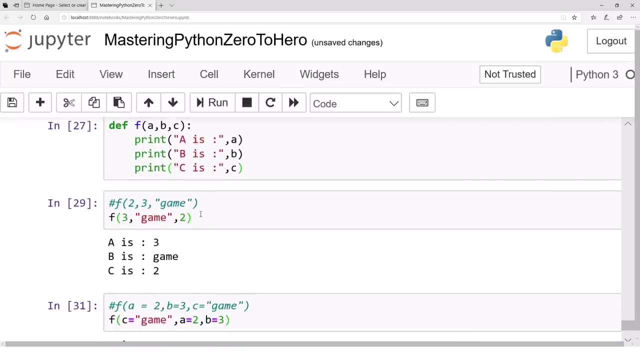 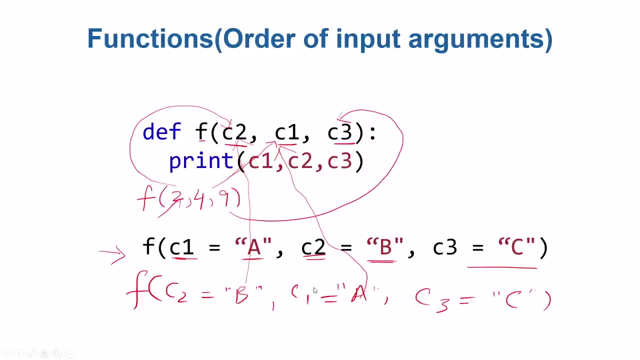 a is at the second position, let's say two, and b is at the third position, three, the output will stay the same, and that's a. that's a beautiful, that's a beautiful thing. so, uh, that's one way of saying um, of handling with the order. If you think, at call time, it is important to define the variable. 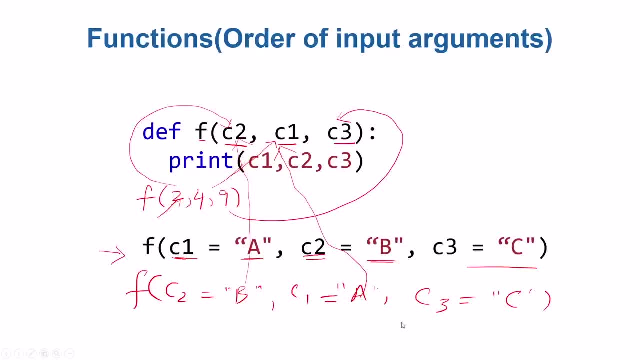 names. but it has one problem: that you need to know exact variable names. If the variable name is C1 there, you need to know it's C1. You need not to. I mean the C1 matches with C, it must match with C1.. C2 must match with C2, and so on. So you need to know these names. 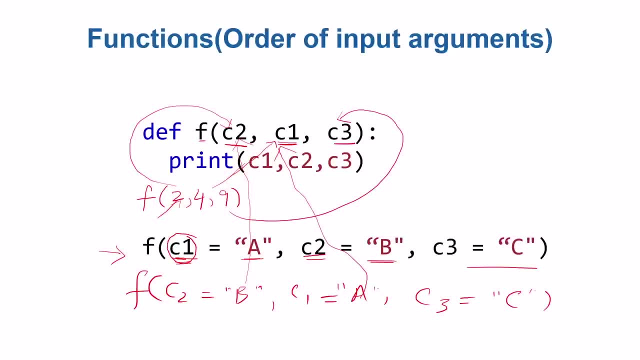 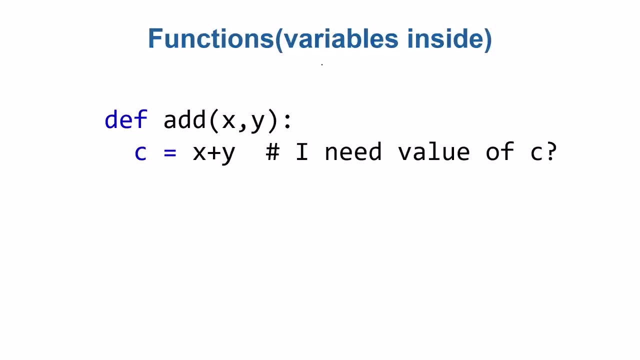 Okay, great. In the upcoming videos, more features of functions are going to be discussed, So stay with us. Hope to see you in the next video. So in the last video we saw the ordering of input arguments in a function And we saw a fix to it. I mean, if there is a chance, 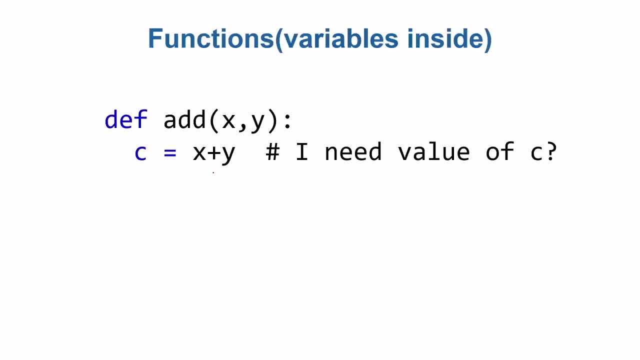 that you may miss a proper order. there is a way to fix. We saw that in the last video. Here we have another thing to discuss: This X variable, X input argument. this is the variable that is defined inside a function, Although the 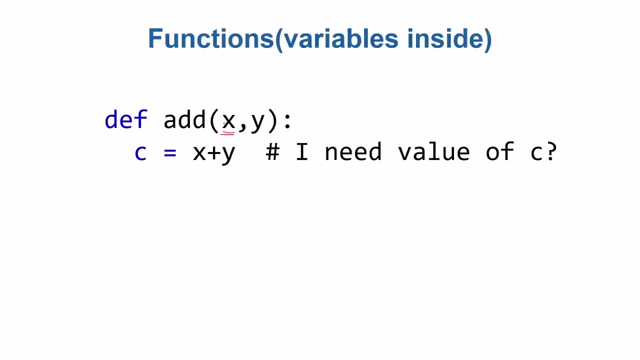 value it receives is copied from somewhere else, but it is defined inside the function. That is also the function variable, or the variable that is in the scope of the function, inside the function, in the body of the function, something like. so Let's say, for example: let's say you compute something, you do some processing on your. 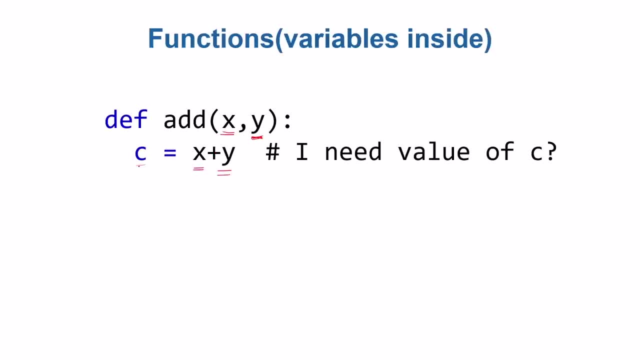 inputs and whatever the result is, you save that result in another variable. And let's say, now you need the value of this variable to do some further process. Let's say what you do is, let's say, at the call time, that's. let's say this is the function. let's say 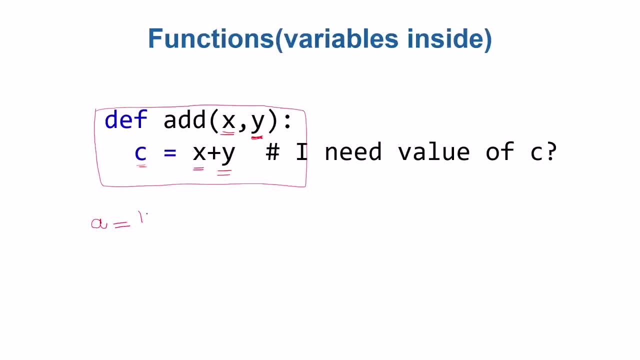 is the complete function. And let's say A is equal to 12 and B is equal to, let's say, 7.. And let's say you call the function add A- B. Now the value of A will be copied in. 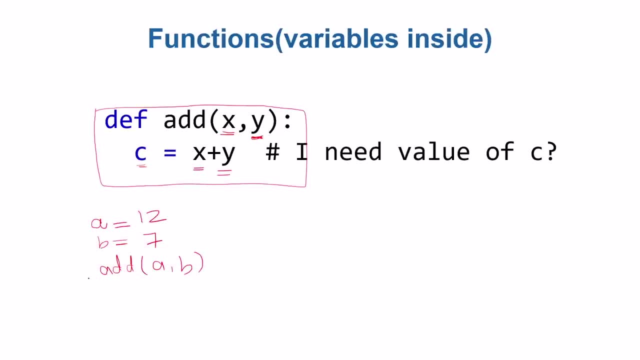 X, the value of B will be copied in Y. okay, And now you need the sum of A and B to be received here in a variable. You want a variable in which the result should be saved. For example, let's say the variable is D. let's say: And then you want to do some more processing on. 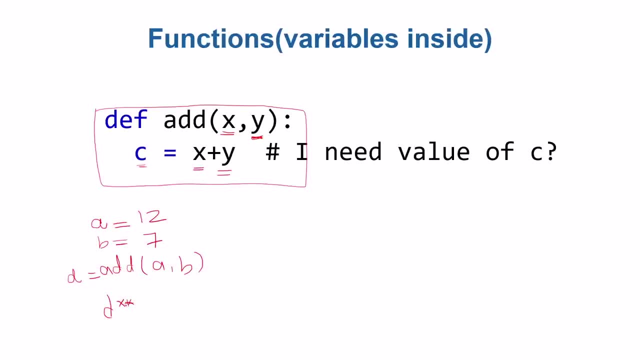 D, Let's say D double-stranded, Let's say D half- scient. You should get D. ofēX is equal to snakes, oh, not really. It's not the height of the very long pair If A horsepower is equal to 5.. 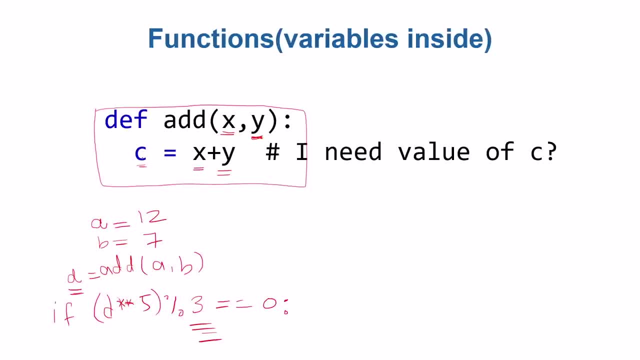 Then you need this variable out. What will happen is this C variable is not accessible outside this function An. the reason is this: C is defined inside the function. When the function body completes it's execution, the C's lost. C is no more available. 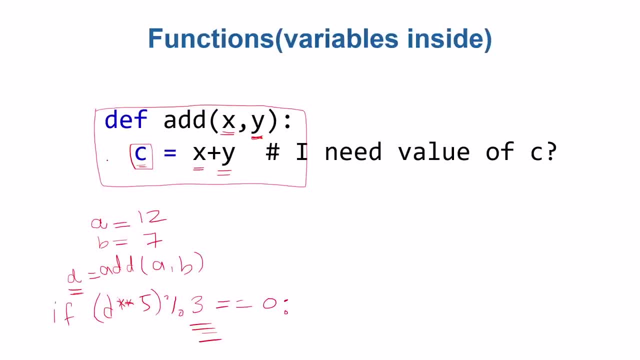 C is defined when the function call has been made. when you are executing this statement, C is defined and a memory location was created in a C, sometimes called the function space in the memory or process space that is created in memory. But once all the body of the function executes all the functions that were inside the variable. 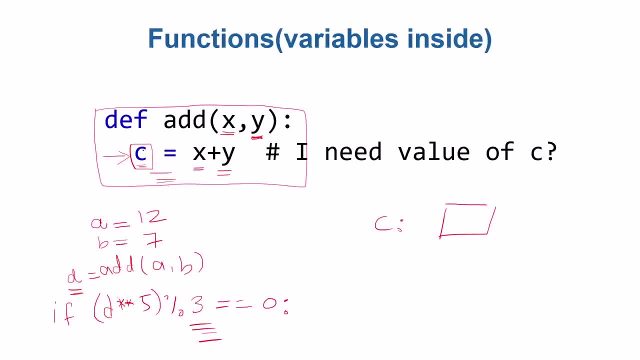 they are lost. How can you receive this value? How can you receive the value inside C outside this function? So that is the question in this slide. how can we do that Further? this particular function can access all the variables that are not defined in. 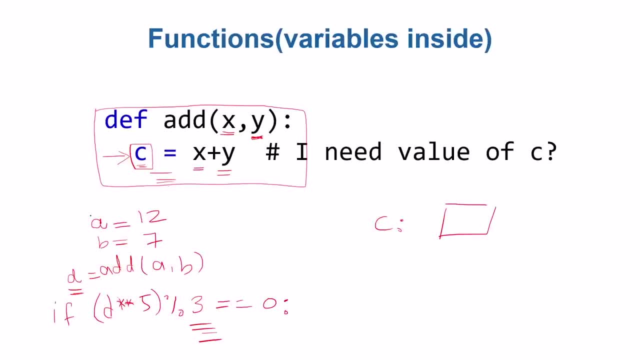 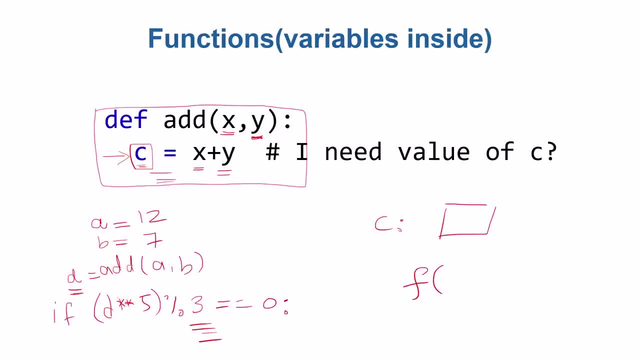 For example, let's say I have a function And the function is, let's say, I have a function F. So if this function is defined like so F, let's say F is your function, And it is defined like DEF, and that's it. 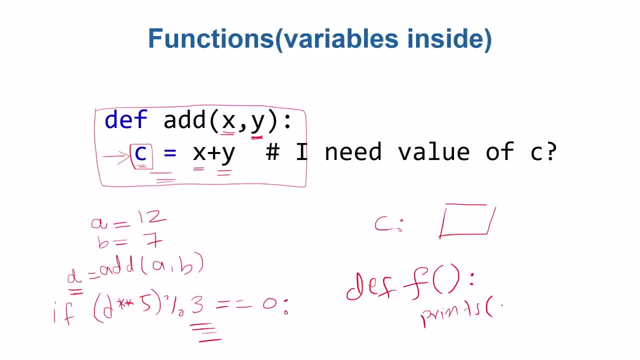 And here it prints: let's say some variable, let's say A. Now this A variable is no longer in F, not even defined in F, But as long as this A variable variable is defined before calling f, for example, that's the cell where we are writing the code, and 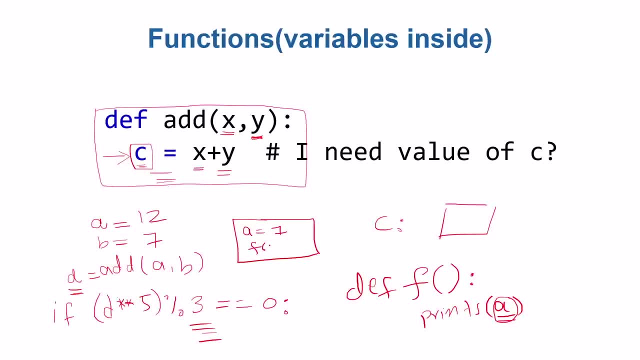 we say, okay, a is equal to seven, and then we just call this f, because a was available before calling f, a will is accessible here. so the functions, the, the variables that are available before the call, they are available inside the functions, but the, the, the variables that are defined inside the. 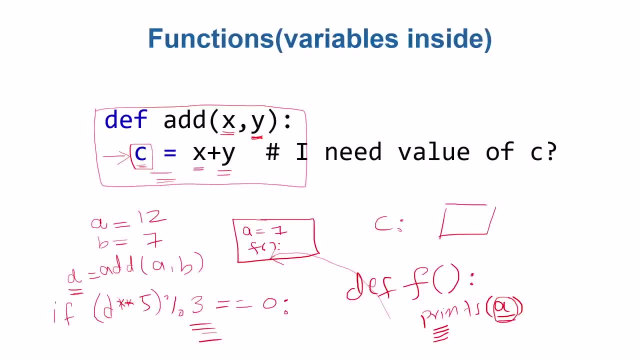 functions. they are not available outside um. that's a problem. further, if we define this a here, a is equal to two. now this a is sometimes called the local variable or the function, the variable that is local to the function. now this a is is is defined inside the function and all the accesses. 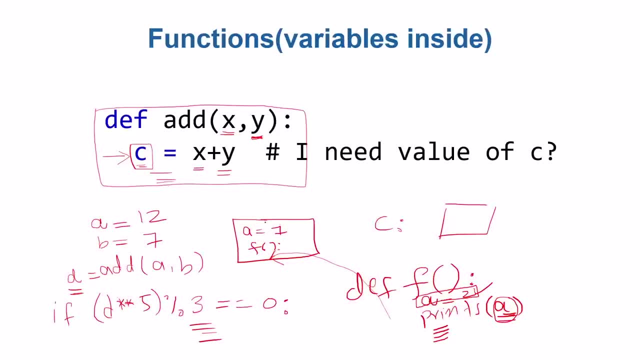 to a will access this value. two rather than the seven. consider: the seven has a separate location in memory and this two has a separate location in memory. both have names, a, but this a will only be referred to when the function is executing. after the. after the execution of the function completes, this is gone from the from the memory. 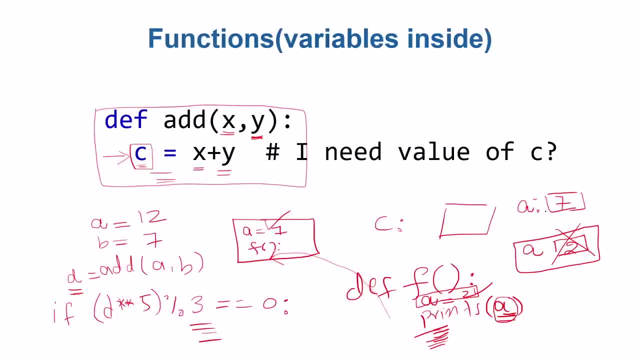 and this will still be available. this seven will still be available. so it is good to know. and and, by the way, if a was not defined here and you still called f, then either you will be getting an error or this a might be a global variable or available. 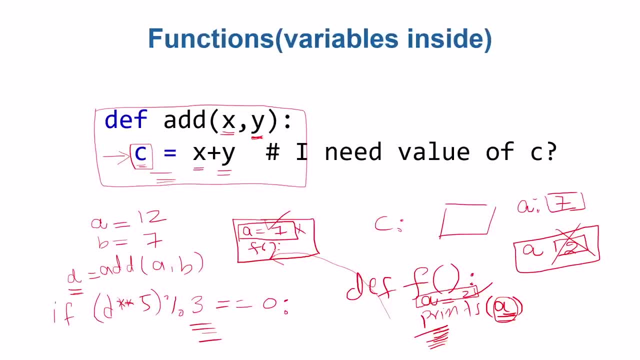 in some package that you have already loaded or stuff like so in that case this a will be accessed if it's a global variable or accessible. so it is good to know the the the scope of the variables inside the function um, because when you're calling them, uh, what functions if this, if x is already defined? 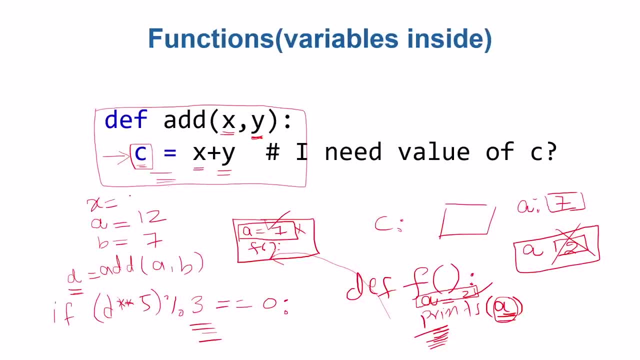 for example, if x is already defined like uh, 34, um, and then this x is 34, as long as this x is not defined here. if x is defined here, then this x is not defined here, then this x is not defined here. this is this x. actually is the local copy and that will be accessed inside the function. 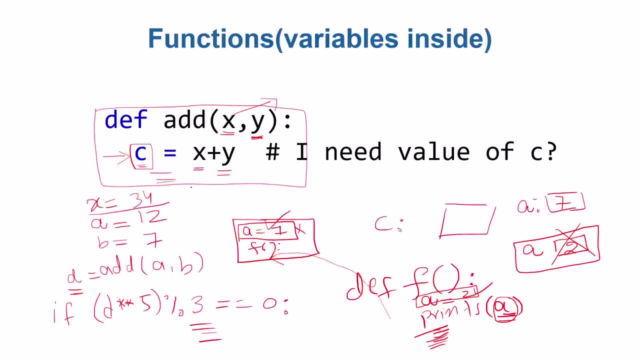 once the function is gone again, x will be 34.. so, uh, it is good to know the local copies, or or the function space itself, the but. but the problem here is how to access this variable, the value of this variable outside the function, because this is completely defined inside. uh, how to access that? 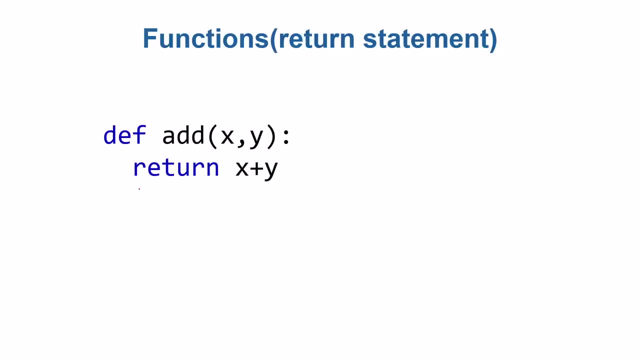 well, um well, there is a fix, and that's what we're going to talk about in the next part of this video. so it is within that, in terms of the way that we're making this, of the feature of the virtual code, we're going to go ahead and ξ explain why c is important. well, c is important, by the way, because 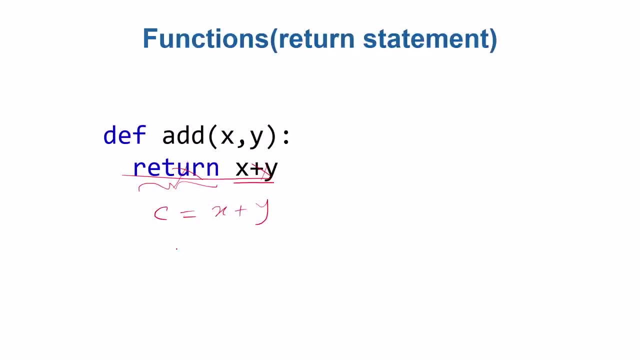 today we're going to call the return variable, and now, just next is the same thing, mas Catalog. it's not going to be inside here that way. it's already used right greater. so, for example, if x is under the leaves of this variable and that's the function inside the component here. besides, 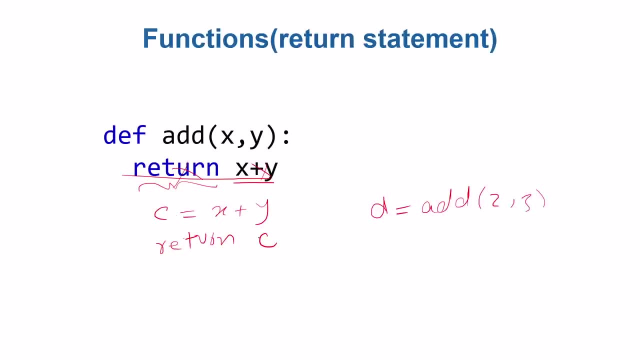 this whole particular function inside the component'd of the interior component- uh, we is five. that value will be returned in d and all the properties of this variables are returned in d. so, just like this, c is copied in d and this is available further, whatever you want to do with. 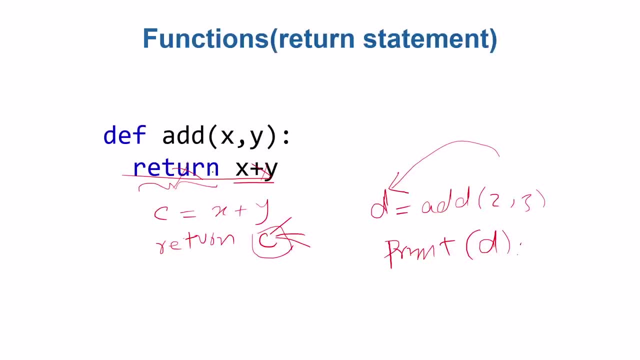 this d, okay, so yeah. so return statement is there. so in the next video we will actually code this in jupyter notebook and see the return statement running, and we will see the scope of the variables and all that in jupyter notebook. so hope to see you in the next video. in the last video we saw 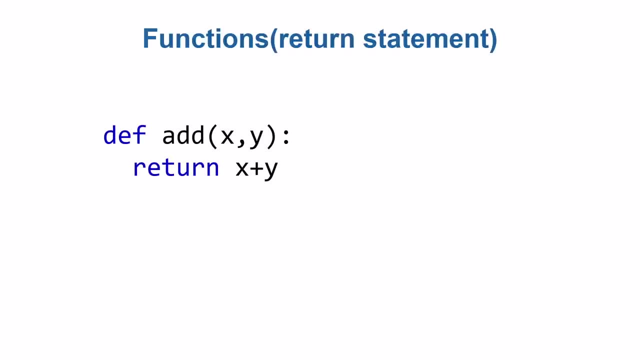 scope of a variable, particularly if a function. if a variable is defined inside a function, is it accessible outside the function, and if a variable is defined outside the function is it accessible inside the function, and vice versa, and so on. so we discussed those kind of things, which is sometimes called school scope of a variable, and further we discussed what 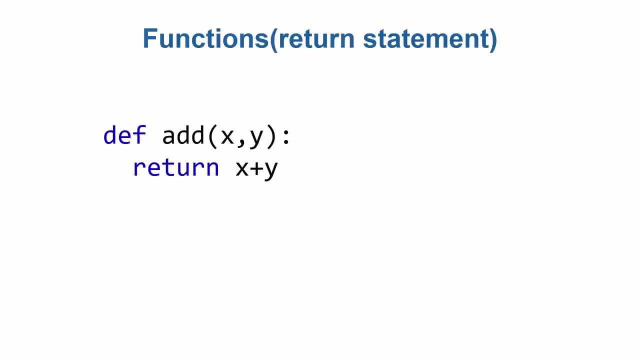 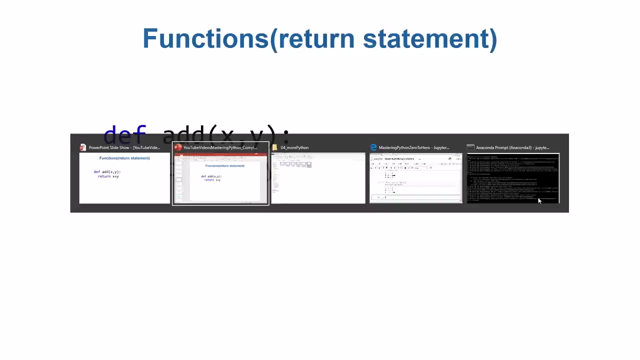 if we want? what if we want a value of the function that is computed, value of some variable or some result that is computed inside a function? what if we want that to be accessed outside, outside the function? so we discussed that in detail in the last video, so let's see all those concepts in a 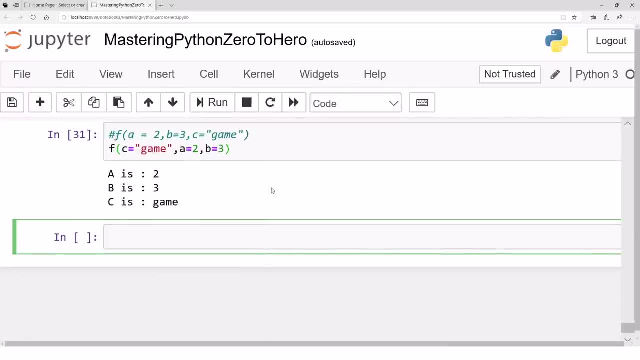 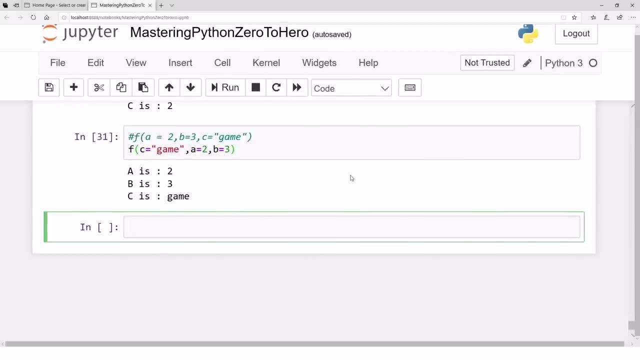 running form in jupyter notebook. so let's see how it works. so first of all, let's define a variable, let's define a function, let's say define, let's say my add, and let's say it receives two arguments. let's say a and b, and and then let's say c is a plus b, let's say that's c or or c value. 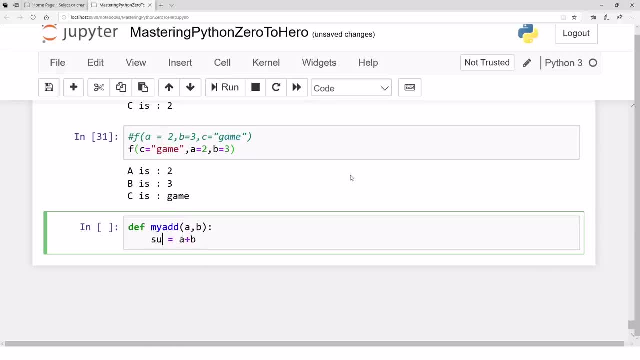 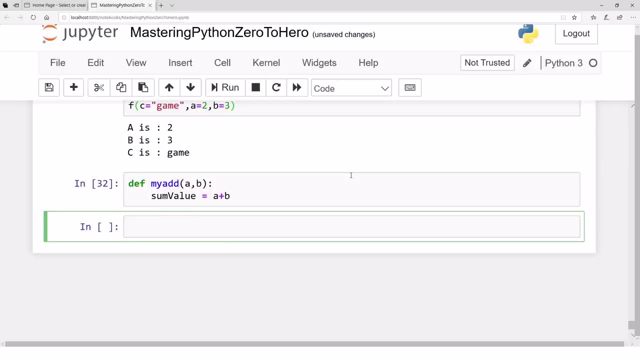 that's a c value or some value, whatever you want to call that value, some value, that's it. let's say we did. we did that. now we want to access that some value from outside the function print some value. by the way, let's first call this function. let's say my add for values. 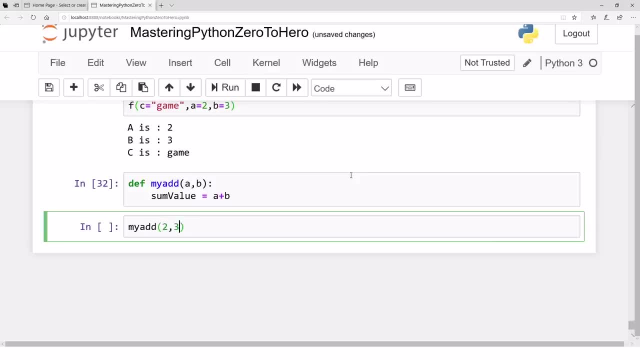 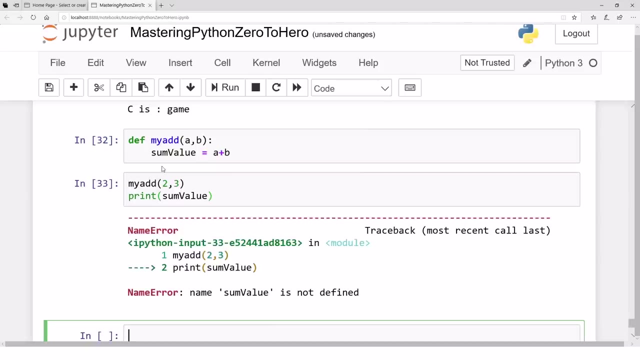 let's say two, three, so two will be copied in a, three will be copied in B. so then let's access, let's try to access this value, some value. it will throw an error and the reason is this variable, some value is not accessible outside this function. what if we want to access? because this is defined inside the 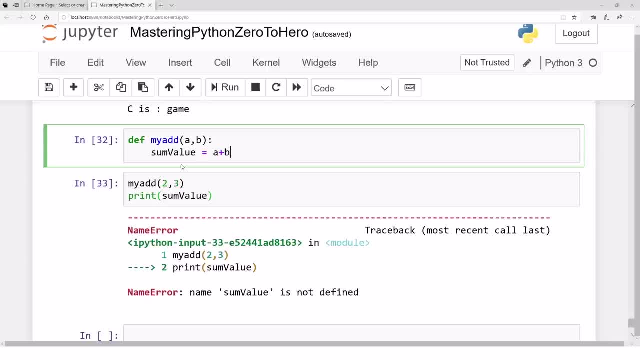 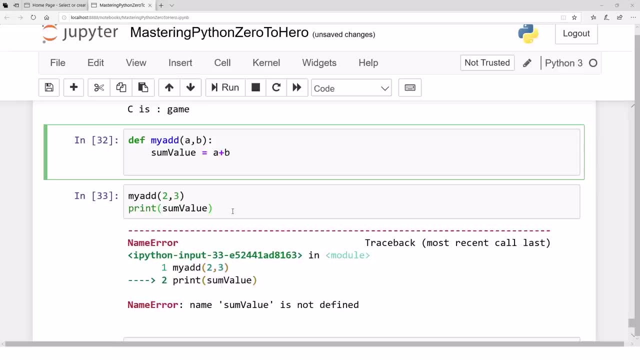 function. what if you want to access this? I mean, what if you want to compute some result and then use that result outside the function? so the way out, as discussed in the last video, is return statement, return value, and now, if we call that again, let me, let me. 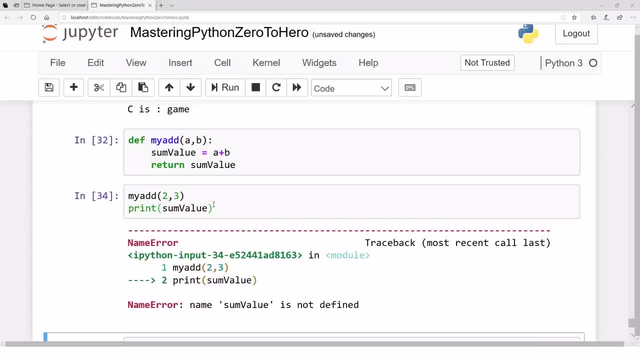 call. if you call that again now, oh, we haven't actually registered. by the way, remember this, that's. that's a common error. I got in that error a lot, of, a lot many times. if you change the implementation of the function, you have to read on that cell. you have to register the updated copy of the 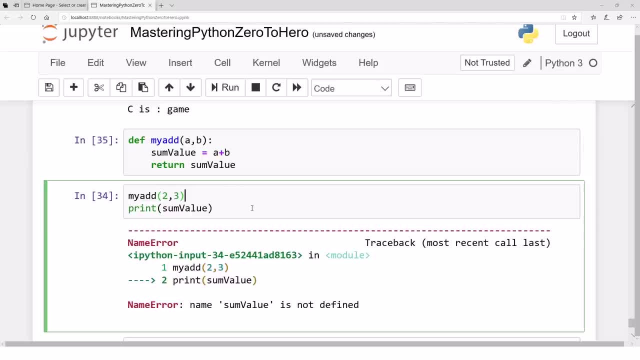 function to the Python, otherwise you will not be able to access the function. let's take a look at that one. so no, oh, this is not how you guys will be getting errors, probably. yeah, oh, what's the problem here? now print some value. we oh this, some value is still not. X still not accessible because some value is not is. 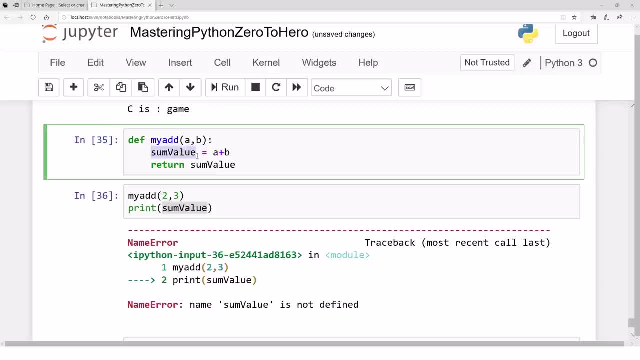 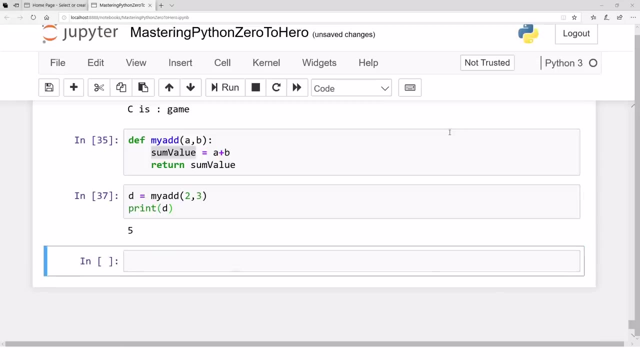 not accessible. it is. it is a variable defined inside the function. it is scope in its. the scope of this variable is just the body of the function. so let's receive this output in a variable d, and then that's where we can find that, given the, Let's just print d, and d is 5, great. 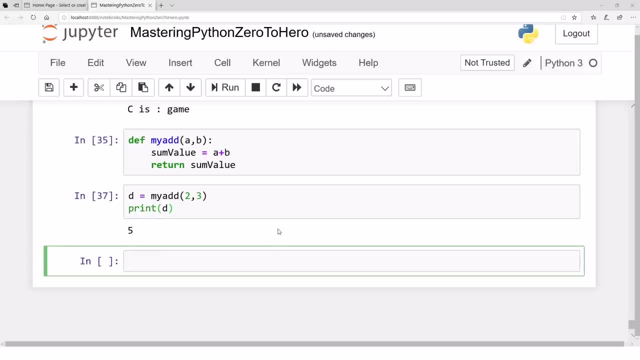 So one more thing. let's say we define a variable here. variable outside the function, that's a variable name, that's a very lengthy name, but let's say that's a name variable outside the function. let's say its value is 3.. 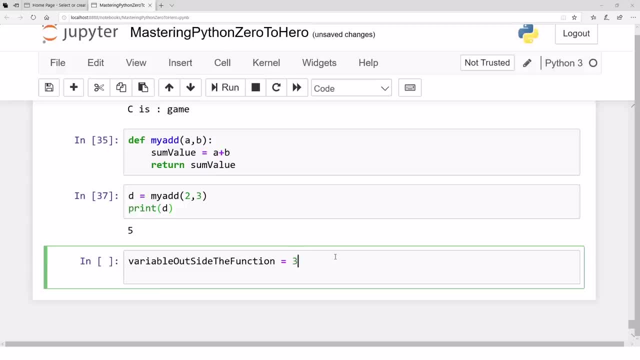 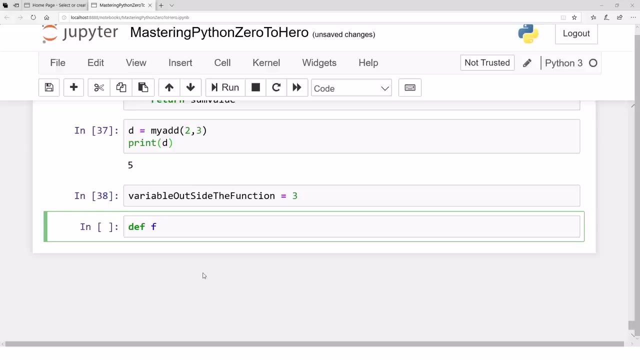 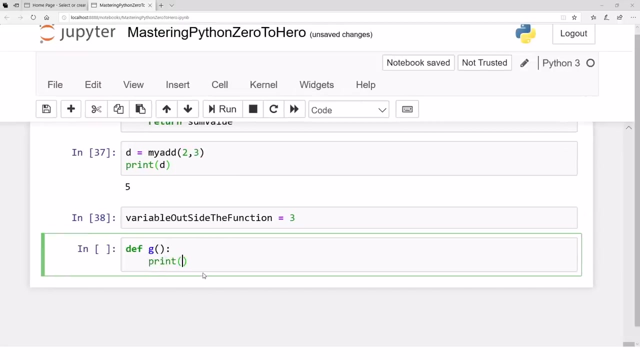 And then then let's define another function somewhere. let's say, let's define another function down somewhere, let's say, define f, maybe g, and it receives nothing, but it prints this let's say: variable outside the function, And that's it. 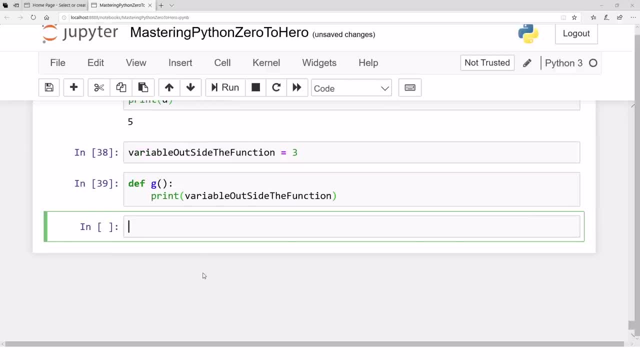 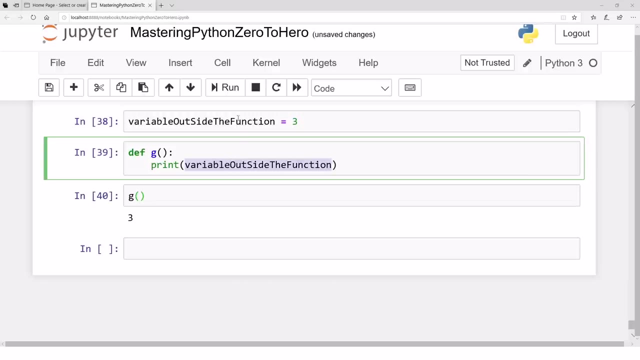 Let's say that's a function. Now, when we call this function, this variable, outside the function, that is accessible inside the function. So so, and if this function and if this variable, it is not defined inside here and 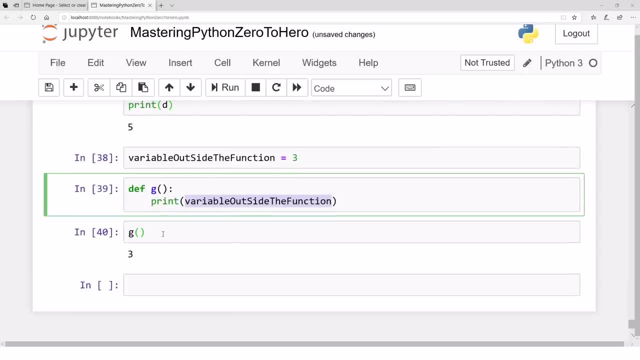 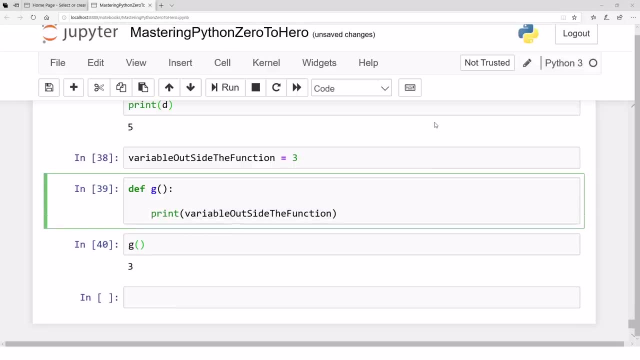 if this is defined somewhere else and it is global or accessible, it will still be accessible. However, if we define a function with the same, the same same name- let's say variable outside the function, let's say 5. Now this function. 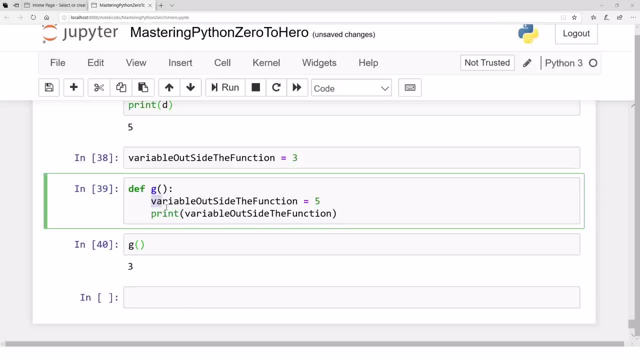 will print 5 because that's the local variable. that's the local variable in the function. Now this will be accessed in this print statement. Let's see Now: the result will be 5, but if you print the variable outside now, the value will be 3 because this variable, this- 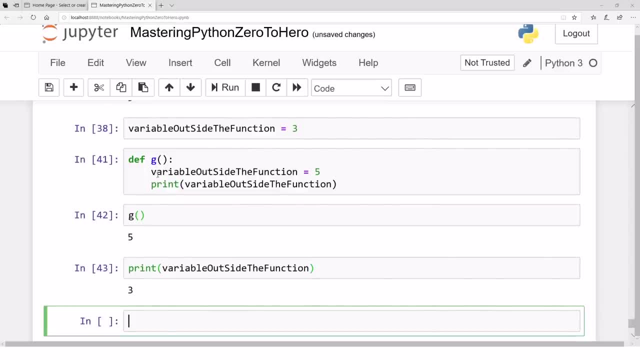 particular variable that was inside the function. it got destroyed when the function finishes And this is available again. So, yeah, so you need to know. by the way, it's a good practice whenever you want to, whenever you want to access a particular variable inside. 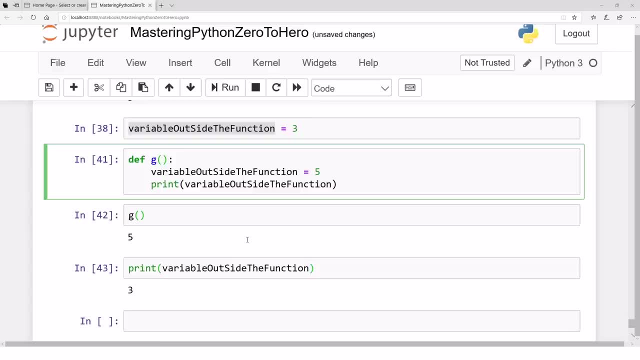 it is a good practice To pass that variable as input argument to minimize the confusions, because this can create a lot of confusions. So it's a good practice- Although the feature is available and sometimes useful as well- but it is always recommended to pass the values as input arguments. that 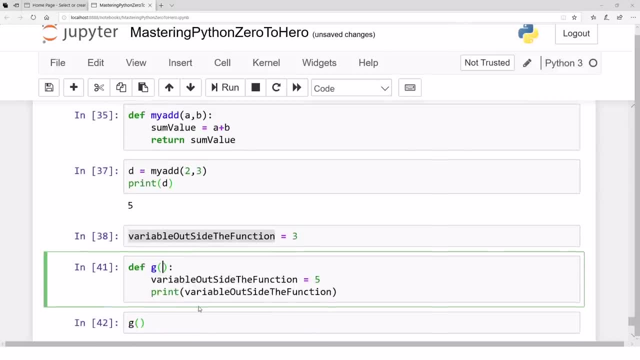 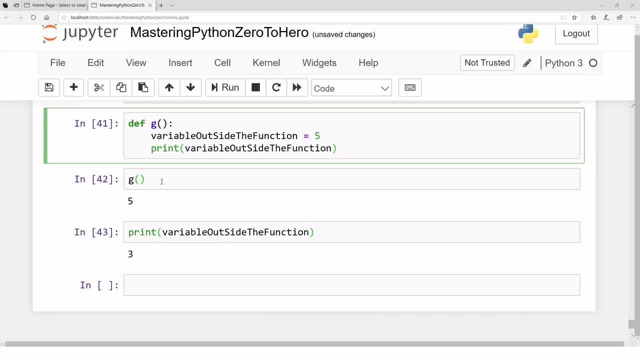 whatever you want to access inside the function. Okay. So one more thing. This function g is returning nothing, For example. it is not returning anything, It is just printing. let's say something, let's say it is not printing anything. Let's say, let's say, this is a comment that said: 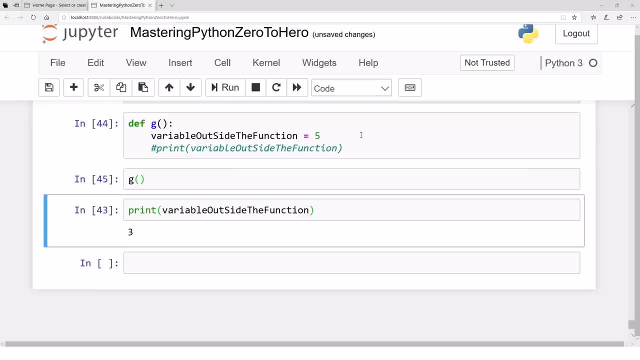 is not printing anything, So this, and then we call this and that's it, So it has no return value. by the way, in Python, even if you, even if any function, even if a function does not return anything, it still returns a value which is called none, which you can see here. 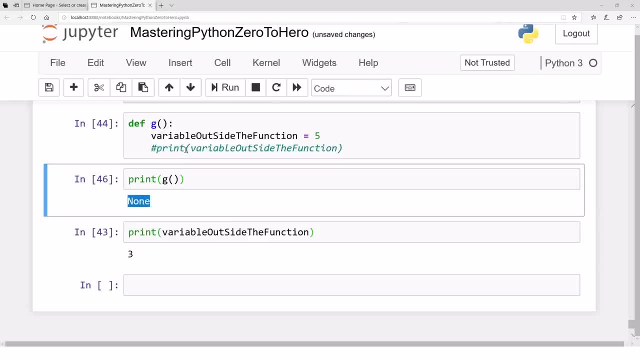 So in Python a function always returns a value. If you write a return statement explicitly, it returns that. If you do not write return statement when the function body finishes, it automatically returns none. Let's see the type of this output. What is the type of this output? 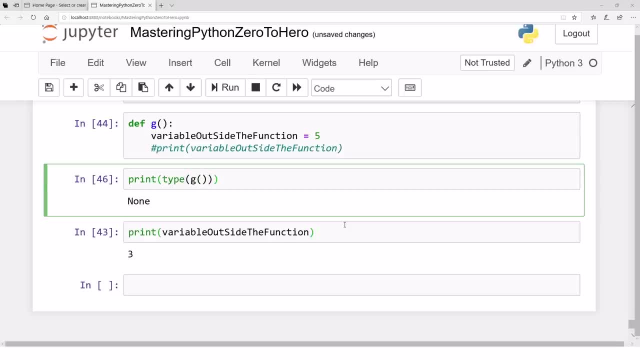 What is the type of this none? What kind of data type is this? Let's see, It's a none type. I mean, that's a type in Python, So it returns a none type output. How fancy, Wow. One more thing. 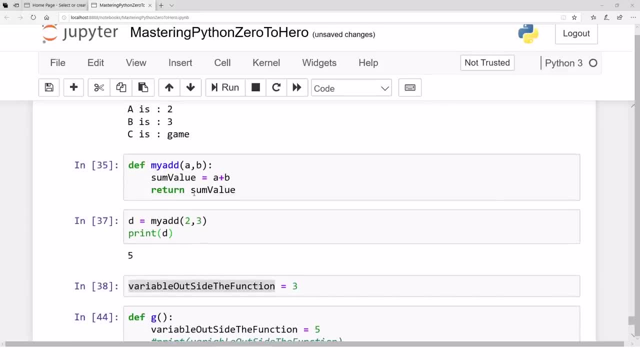 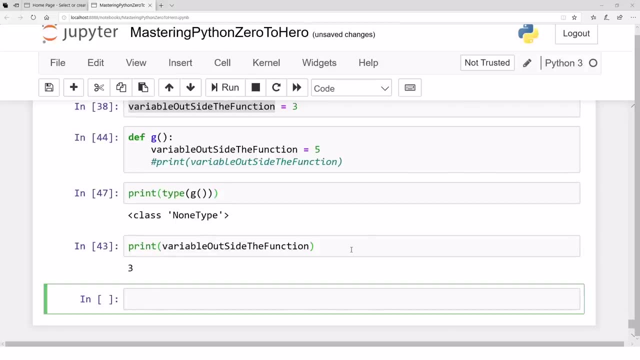 The return statement is not only used to return a particular value. If you, for example, in a particular function- let me write a function here, Let's say def, let's say the function is h and then inside that function you do something, 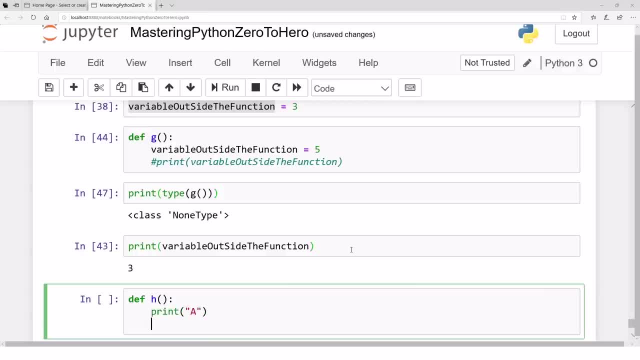 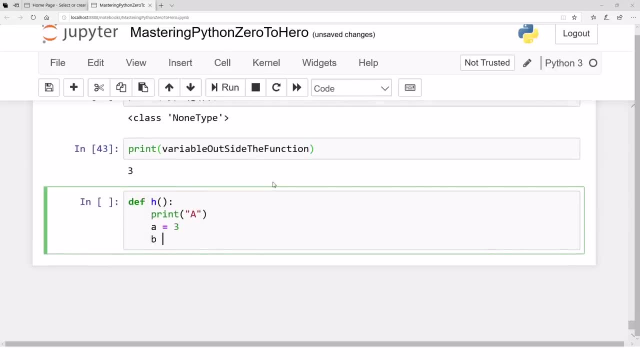 Let's say: print a. let's say: then you define a variable. Let's say a equals two, three. let's say then b equals, let's say five, and then you add those values a and b, and then you do some other stuff. 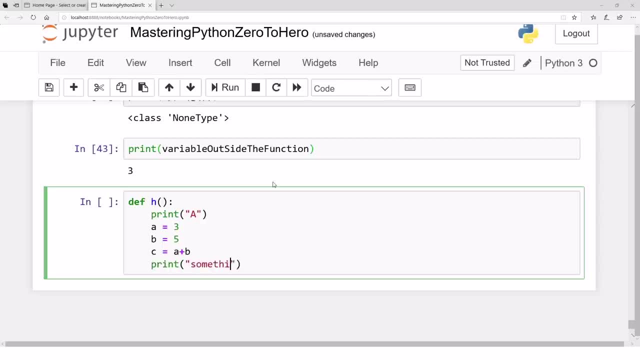 Let's say, print something and then you just write a return statement without any output, or I mean it is not returning anything. You can still. you can still, I mean, continue writing the function body. Let's see The function body more and more. 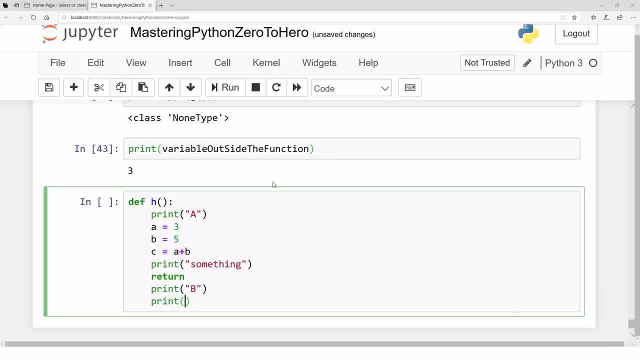 But what happens is whenever the first return will be encountered, the function returns from there. So the effective body of the function is just that: The function returns right from there. If you return a particular value, for example c, you can receive that value outside the 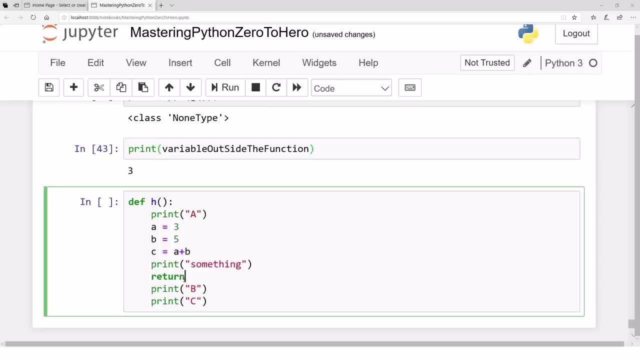 function. If you do not return anything, just type a return statement. That means exit the function right away. It works like the break statement in loop. Remember the break statement. It resembles to the break statement. Return means just exit the function right away. 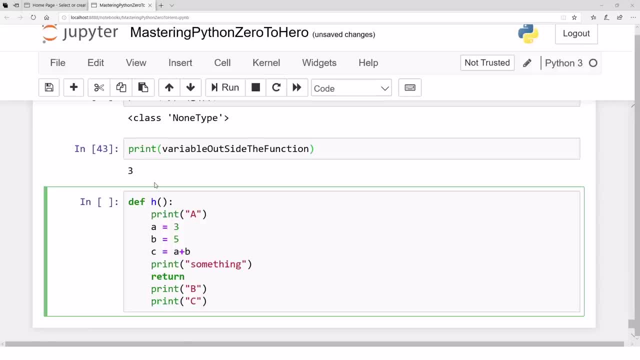 No problem. And, by the way, when return is called, the default return value that is returned is none type if the return is called without an argument here. So, for example, let's run this function, Let's see And let's call that function h. 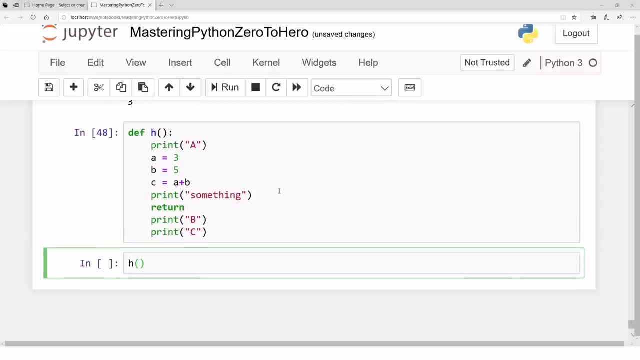 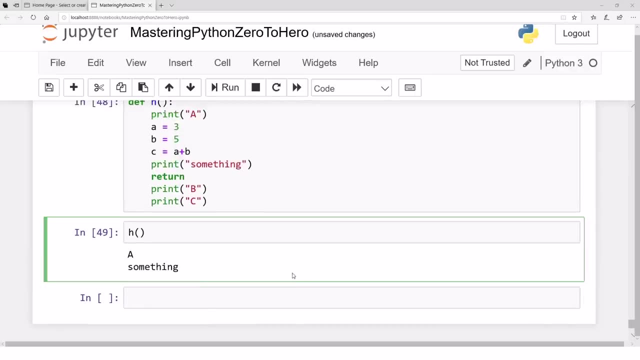 Yeah, So, So, So, So. So it prints A, then it prints something, and then it returns, and it returns. for example, it returns nothing but a none, It returns a none. And if it returns c, for example, then it returns a c value of c which is 8, and this time this: 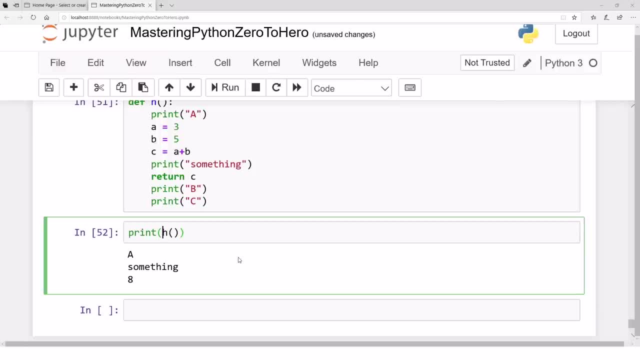 time the return value is no longer none, non-type, It is probably an integer type. Let's see, Yeah, here. So it's integer type, Makes sense. Yeah, So return statement has two purposes. One: you can return a value. Two: you can return: 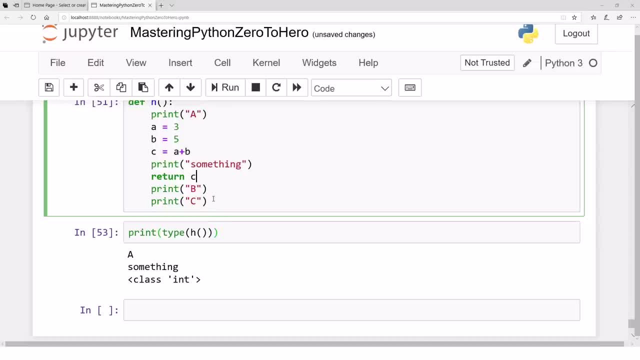 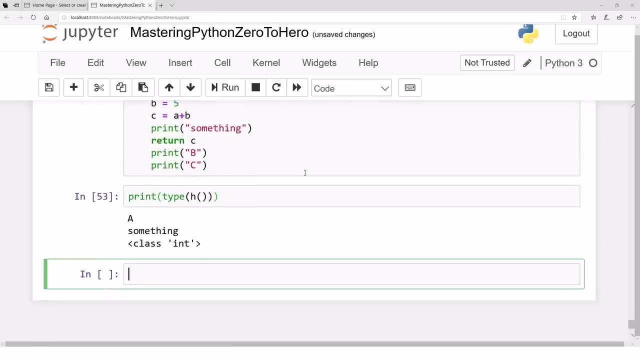 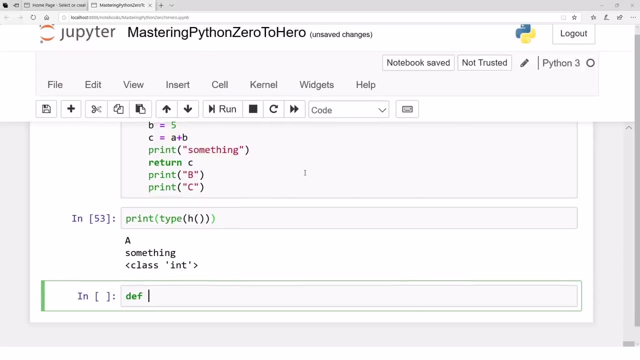 you can just return the control, You can just exit the function, like the break in loops. Just one more thing: Return statement can return multiple values. For example, let's say we have defined a function. Let's say j, Let's say g, g- we already have defined, We can. 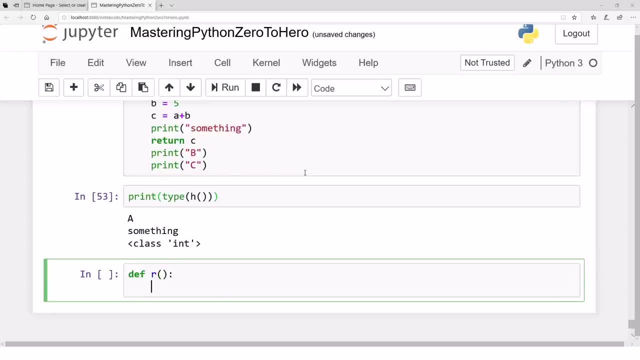 redefine it. But let's say r is our function And we just have a equals 5,, b equals 7, and d equals. let's say something, And then we just return them: a, b and d. So return statement can return multiple values in a sequence. 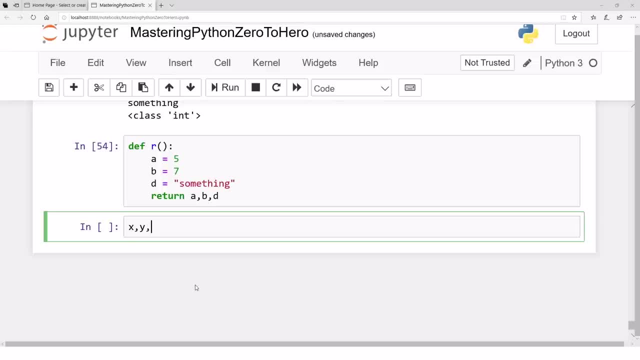 Now, if you receive those values, let's say x, y and z equals r, So a will be copied in. a is the first return value. It will be returned in x. It will be copied in x. b will be copied. 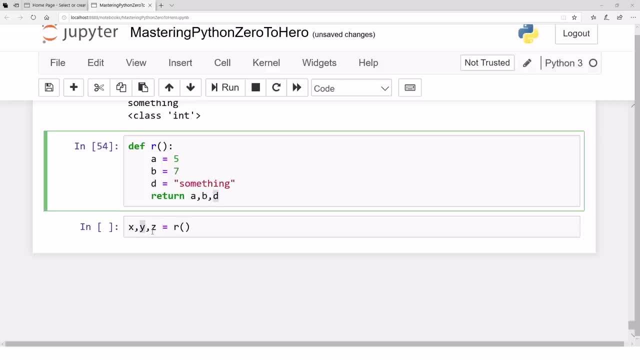 in y And d will be copied in z just as a sequence, as you keep the sequence in the return statement if you change the sequence in the return statement accordingly. so whatever the first value here is the first value here. whatever the second value here is the second value here, and so on. so let's run this and just print. 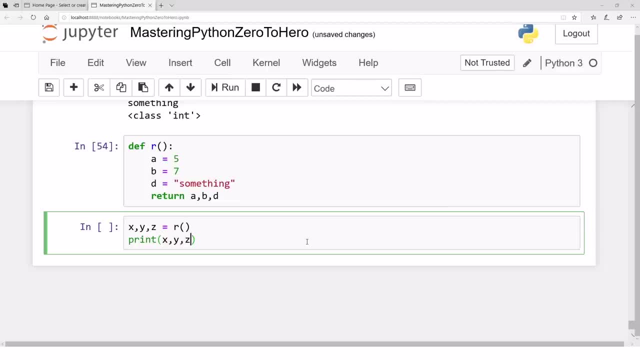 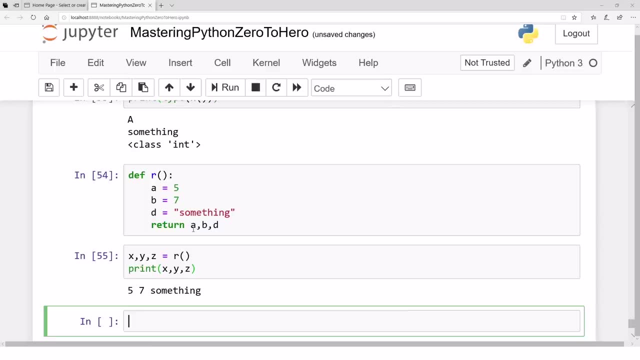 all these things- X, Y and Z, so yeah, five, seven and something. so this return statement is really powerful. I mean, it can return multiple- not all the languages, actually not all the languages. they have feature to return multiple values, but Python does have feature to return more than one values and more. 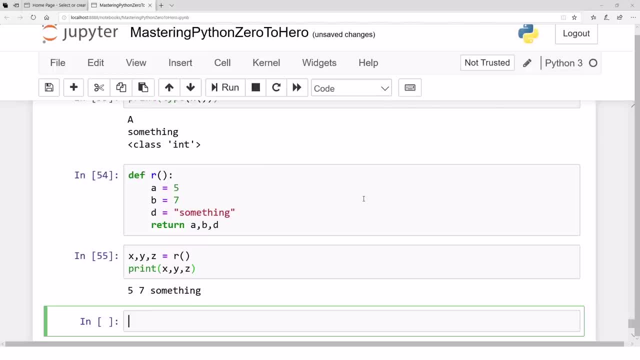 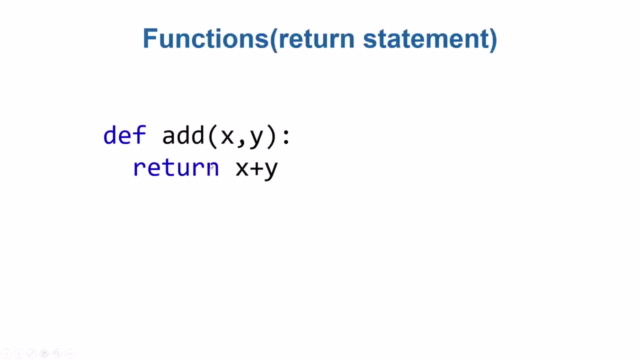 than one. values of any type. a can have different type, B can have different type, D can have different type, and so on. so that's about the, that's about the return statement, as well as the variable scope and whether you can access a variable that is outside the function or inside the function, and so on, and all that kind. 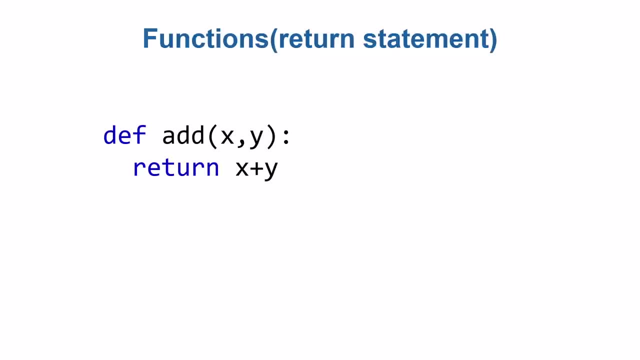 of things. in the next video we'll talk about what if we want to access arbitrary number of input arguments. I mean, we do not know how many arguments will be there inside, but no matter how many arguments a particular user is giving. let's say, if you want to write an add function, just just to give you an example. let's say you want to add write. 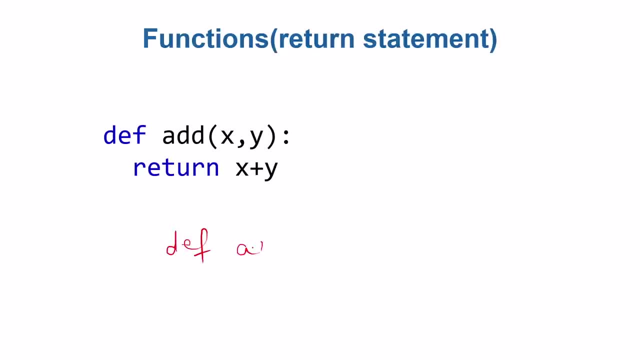 an add function. let's say define, add. let's say add to another function, add to. and let's say it receives an arbitrary number of arguments, D in I don't know how many, and it has some implementation. then anybody who want to call this add to if it. if that person gives two or two arguments, then just. 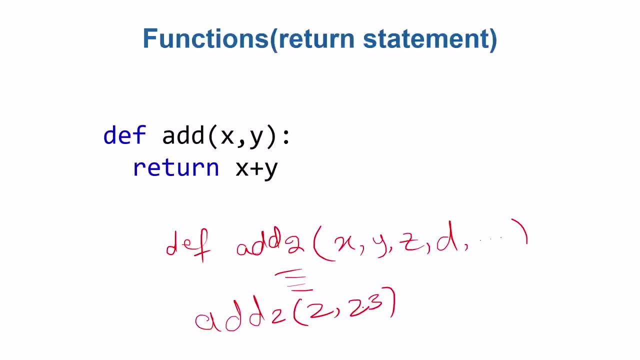 two should be added. if the person gives three arguments, then three should be added. I mean the person can give arbitrary number of arguments. how can we handle that? because, because the color, the, this is the call, this is the call, the color can give five arguments, six arguments, seven arguments and earlier. we saw in the definition the. 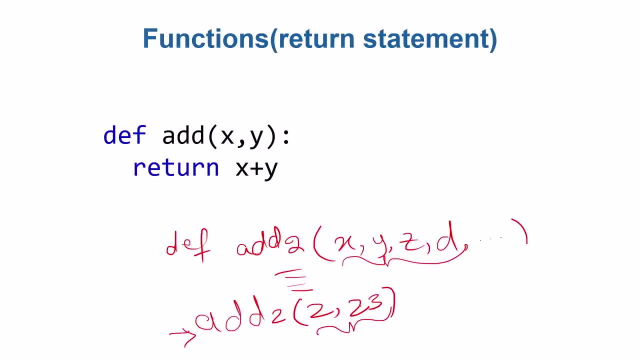 total number of variables. when we specify, we have to pass those many arguments for sure. if a single argument is missing or a single argument is just more than the specified number of variables, we will be getting an error. but how can we handle this situation where we have an arbitrary or 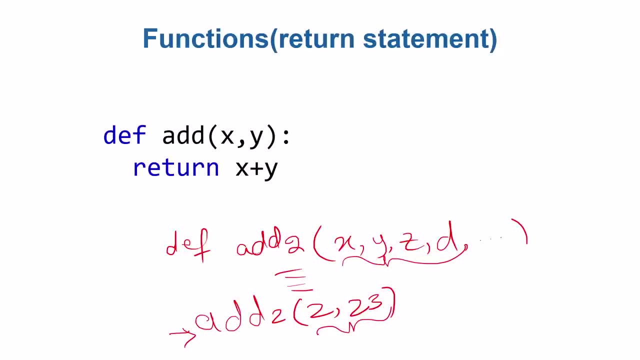 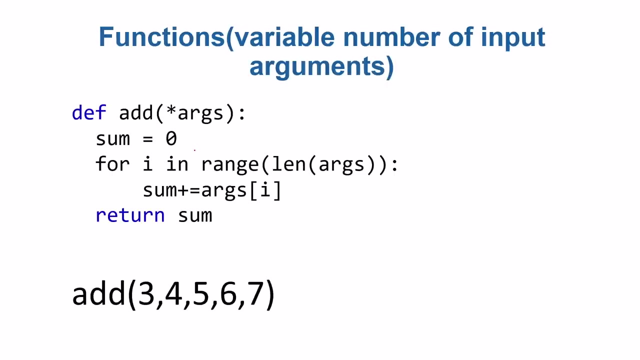 variable number of input arguments. how can we handle that? so, to answer this or to get a, how can we do that? see our next video. it's coming in. the last video we were talking about how can we handle arbitrary number of input arguments, for example? let's let's say we want to write an add. 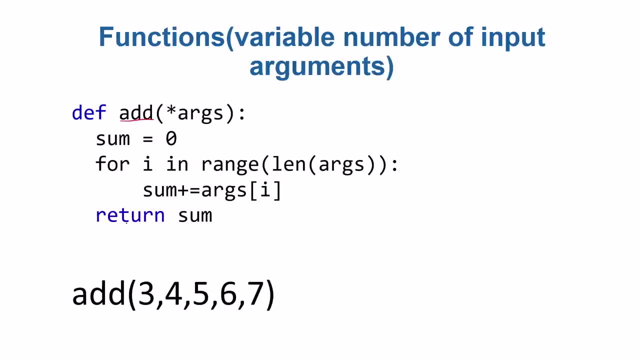 function that should be able to add any number of, let's say, integer or floating point numbers that are passed in. remember last time we discussed in an earlier video that when you are defining a function- the total number of variables that you are defining- you have to pause exactly those many input arguments, otherwise you are getting an. 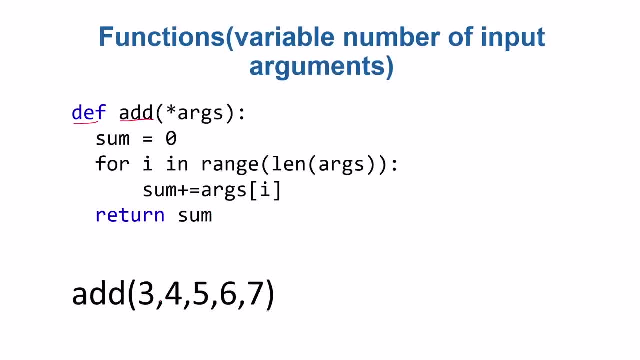 error, but- but this may be required some time- that we want to add a universal kind of add function that has, that has capacity to receive any number of arguments, but no matter how many arguments it receives, it just add them all and return the result. such a function, if available, will be. 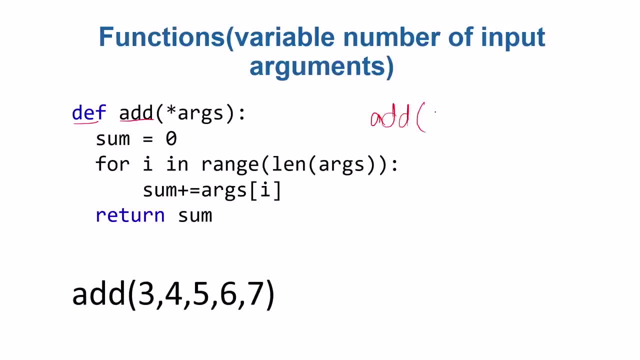 very, very helpful, because sometimes we might be calling that function by just two arguments and sometimes we might be adding, might be calling that function with, let's say, three arguments, and sometimes more arguments or less arguments and so on. how can we have this kind of feature available? 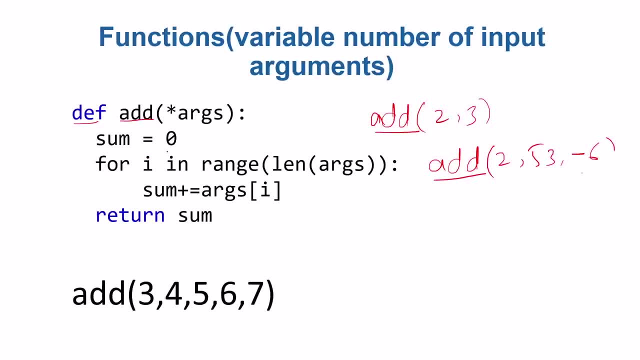 but the implementation is just one-time implementation. well, python, have a very, very easy way of handling this arbitrary or variable number of inputs, and the way you do that is: when you receive, when you are defining a function, you just write a string and you just write a function. 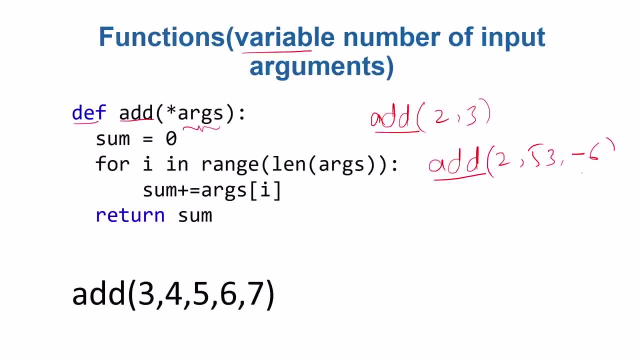 star and then just print, let's say, one variable name, let's say args, uh, and then after that this arts will act like a list and I mean it will be having a lot of properties. args, this args has a property, this, this acts like a list. so all the arguments that you will send in will be received. 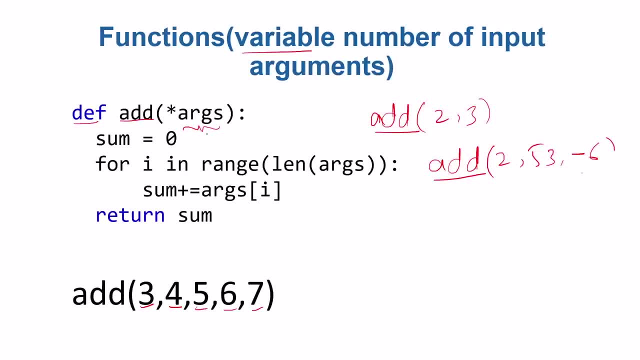 like, like you're receiving those in a in one list and all the elements which are the arguments in the list. they are accessed by different indices. we will see lists in detail later on, but right now just think it is a collection, all the collection. it is received by indices, for example the args, uh, the, the very first. 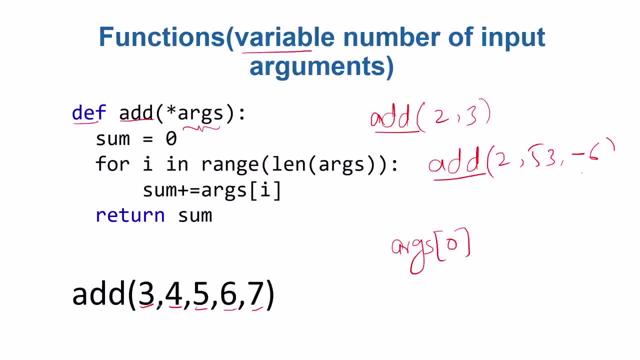 element is indexed by zero. it is at the zeroth location. at the zeroth location, there is a three. at the first location, for example, the location index number one, which is actually the second. look, the four will be copied at this and so on. now, no matter how many arguments you pass a list, it will be of that size and there is a function length. 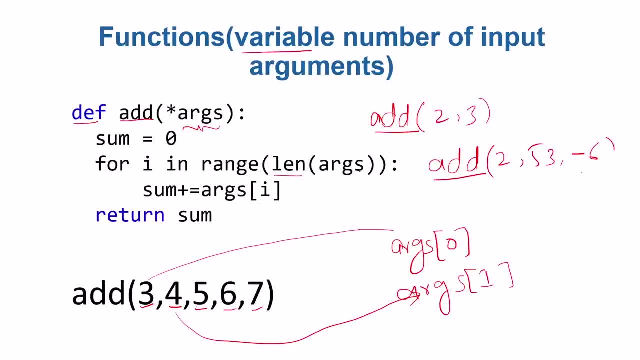 len. that is handy to just check how many arguments are there. now. if you pass two arguments, the args will. the length of the arts will be two. if you have three, if you have passed three arguments, the length of the arts will be three, and so on. no matter how many arguments you pass, this args. 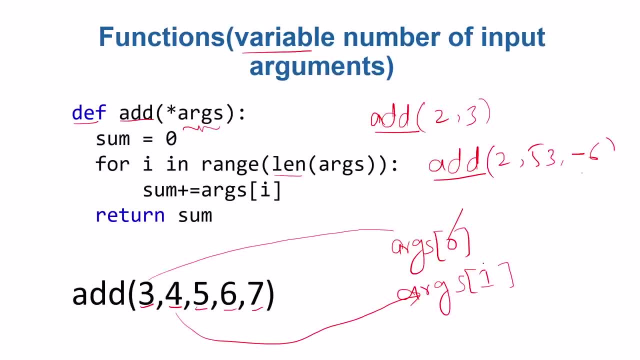 it will receive all them in one by one, and all the elements in that art will be indexed by zero, one, two, starting from zero until the length of the arcs. so see, for example, the uh here, this: so the sum sum equals zero. that's it. let's say we want to add all these for i in range and inside. 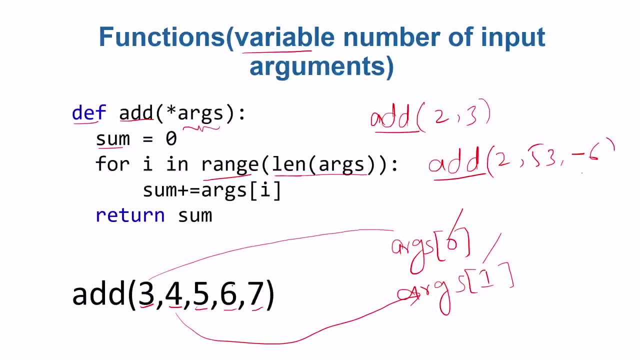 range. we just give the length of arcs. for this example, 1, 2, 3, 4, 5. the length of arg is five. so I will start from zero till till 4, because 5 is not included. so the very first time I will be 0 and. args in subscript 0 are threeung Connect all uh predict 20 flow'll. add those numbers for the range of this example: one, two, three, four, five. the length of arc is five. so I will start from zero till till four, because five is not included. so the very first time I will be zero. and args in subscript zero are 0 and innyt yani vo oggi are at large and there are multiple假utum get fade Эibles and 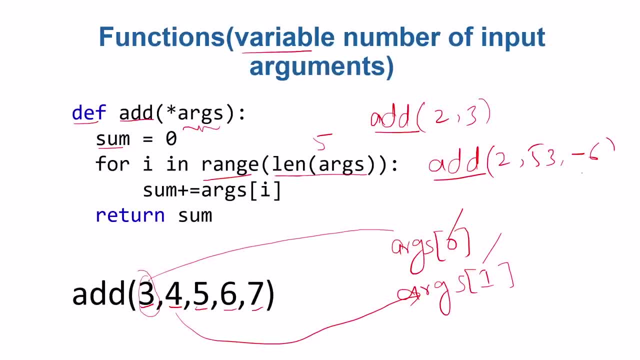 0 is actually the value of the first variable, which is 3.. So 3 is added to 0. Then next time i will be 1, and at the position 1, 4 is located. So 3 plus equals 4,, which means 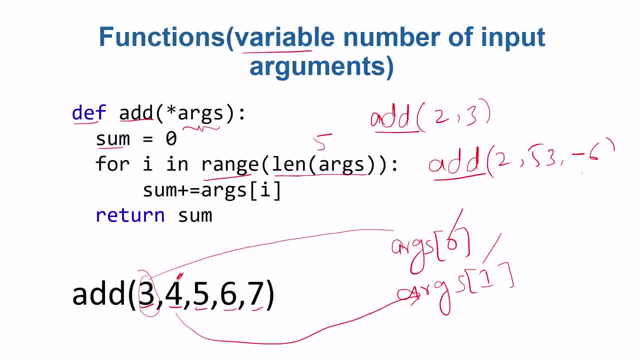 3 equals 3 plus 4, or sum equals whatever the previous value of sum plus 4.. Then next time the value of i will be 4.. You know how this loop works. We discussed the loops in detail And as you move on, you actually explore all these numbers and this variable sum. actually, 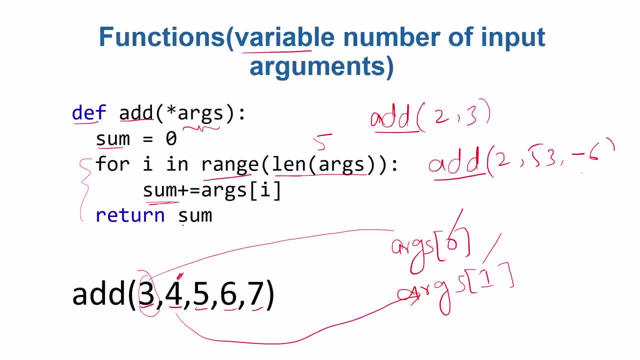 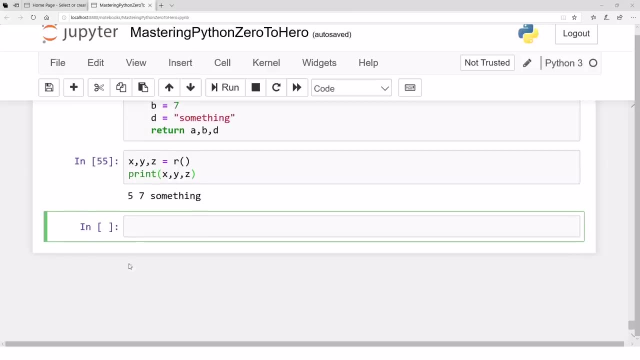 contains the sum of all the variables. Now you can return this sum and this particular function acts like a universal kind of function that receives arbitrary number of arguments. How cool is that? Let's see in Jupyter Notebook to get more convinced how it works. So let's 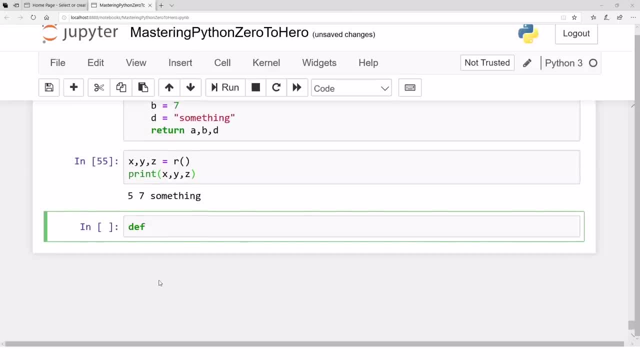 say we have define. Let's say we have any function MyAd. let's say that's a function MyAdPowerful. let's say, Yeah, universal or universal, Universal, MyAdUniversal, And it receives star, whatever the variable name is You can. 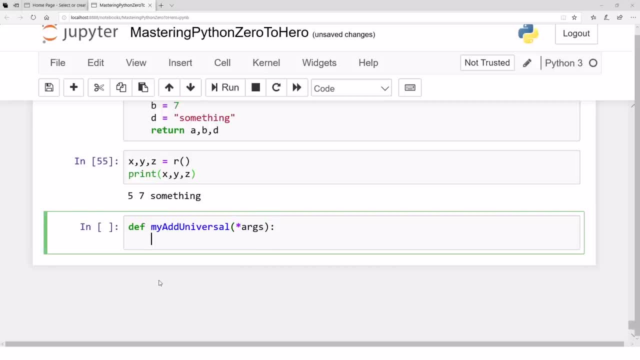 write the name args, or you can write any other variable name. This is just a name of a variable. Okay then let's say we have, let's say we have- s equals 0, which is sum. Then we just apply a loop. I guess you know the loops. We have lengthy discussion on loops. 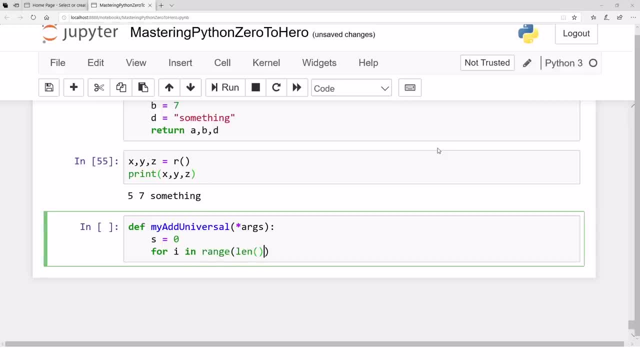 In range length. that's a built-in function: length args. Okay then what should we do? s plus equals args i, which means excess. All the elements one by one, And this is again the same as s, is equal to s plus args i, Either. 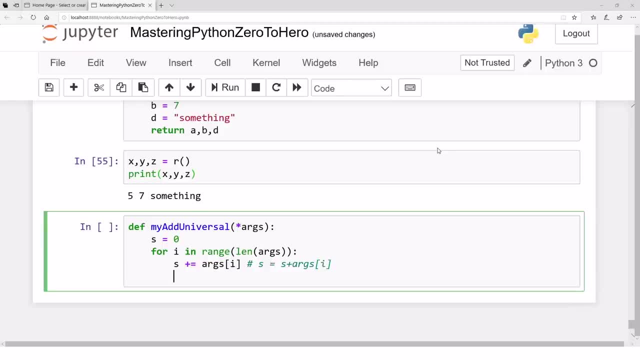 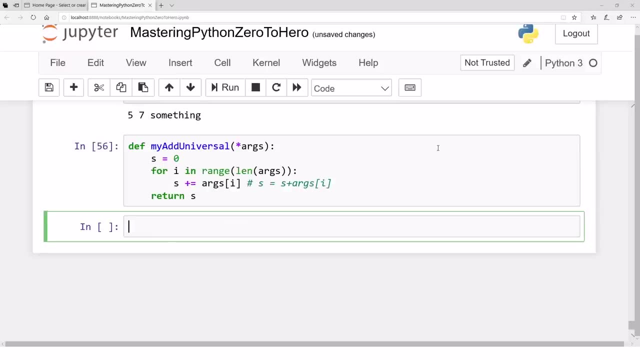 way. you write this way or that way, Both ways are fine. Then, when the loop finishes, s contains the sum. Just return it and you are done. Wow, Now let's call this add function MyAdUniversal. And let's call this function as two, four and five for these. 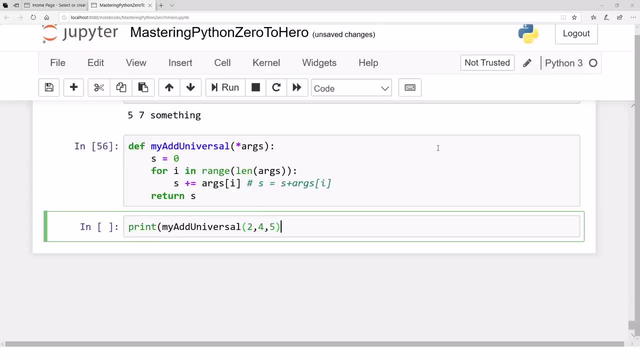 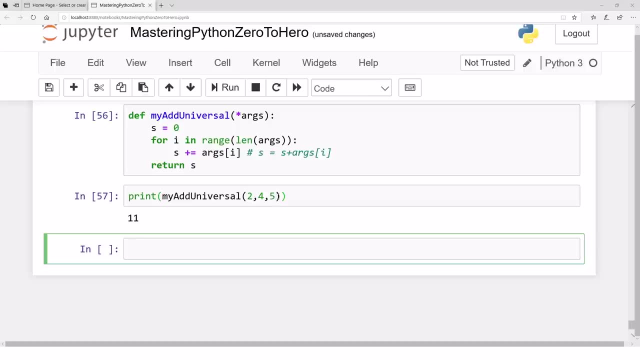 And let's just print the result. Let's just print the result. Okay, the result is 11.. Wow, because two plus four plus five is 11.. Now let's call this function for, let's say for, let's say five arguments. It works. It adds all these five numbers. Wow, That is. 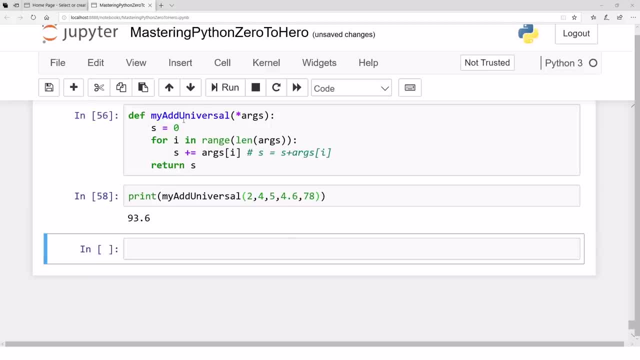 great. I mean, now we can add any. we have one function. We need not to write a function for two arguments and then another function for three arguments, then another function for four arguments, and so on, Depending upon the number of arguments we need not to write. 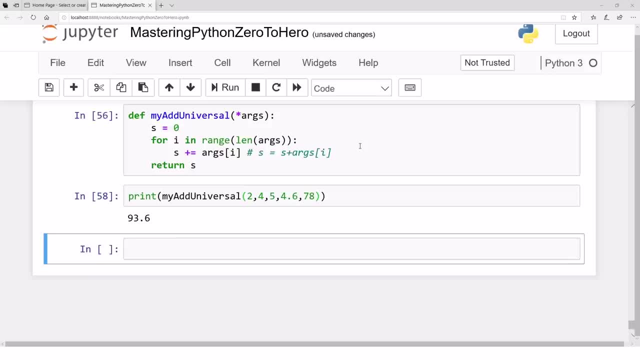 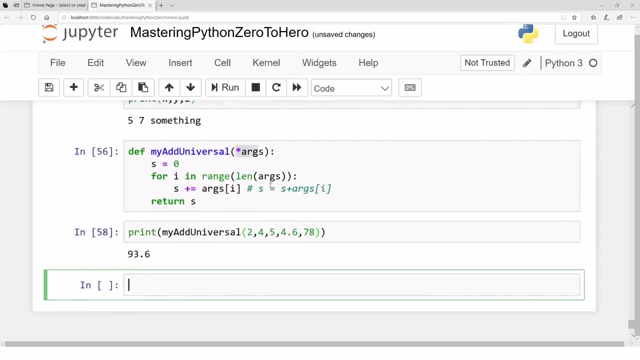 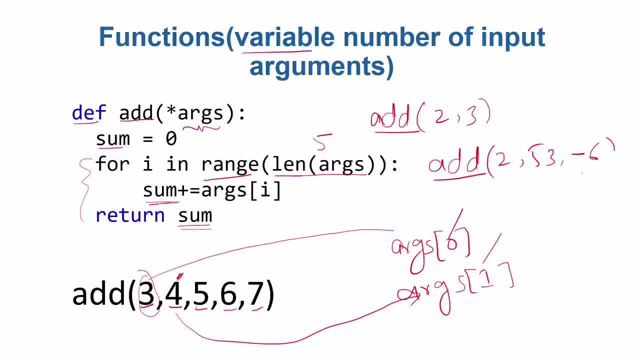 separate functions. We have just one function working in all scenarios. Wow, So yeah, that's doable. I've done in front of you, No problem. Yeah, Python allows this. Yeah, In the next video we are going to see how can we actually handle the same kind. 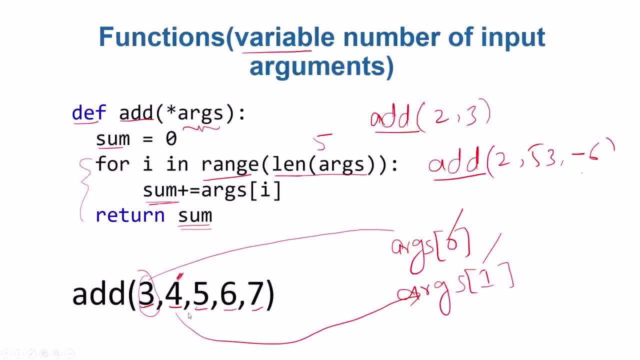 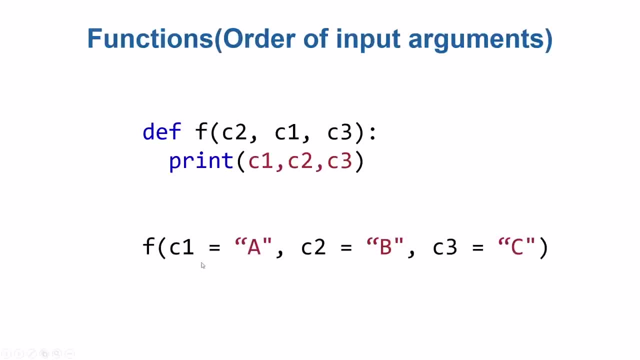 of scenario, but we want to handle the sequence of the input variables in a very controlled way. Remember in some of the previous this: this: yeah, In this order of input arguments: remember that We received three arguments and we passed the three arguments in a very 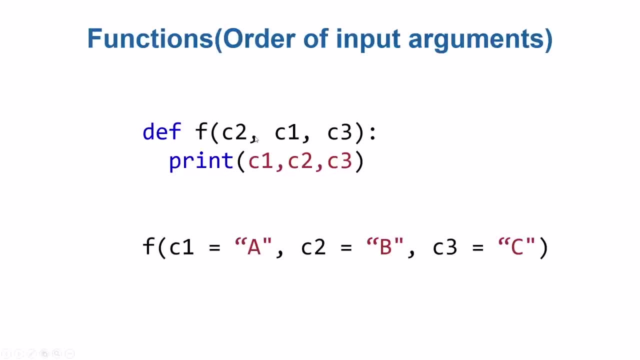 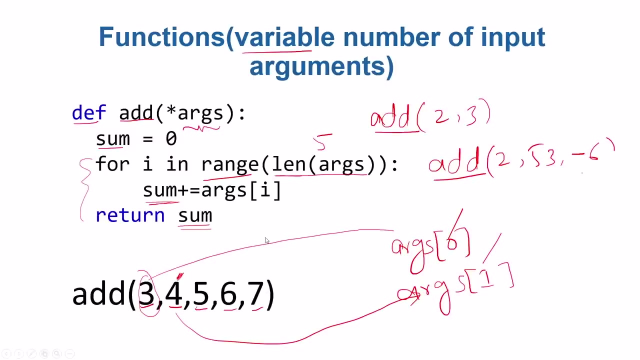 controlled way. And then, whatever these are, we don't care. Whatever the order here, we don't care What if we want to fix the input or we want to become more careful for input argument orderings, but then we also want the arbitrary number of arguments. How can we do that? Yeah, Wait. 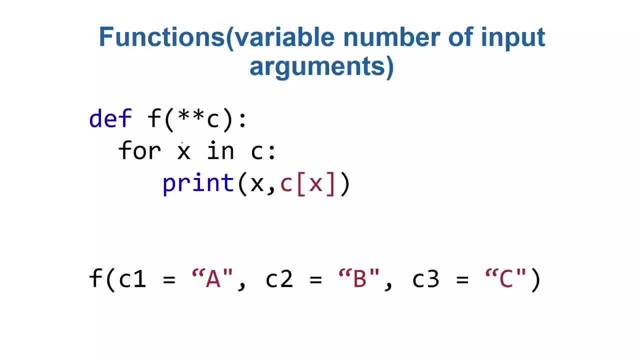 for the next video, and I will show you how can you do that. In the last video I promised you that I will show you how can you achieve the ordering of the input variables, but still theありabulty number of them. Remember, this looks like much familiar to you, That's. 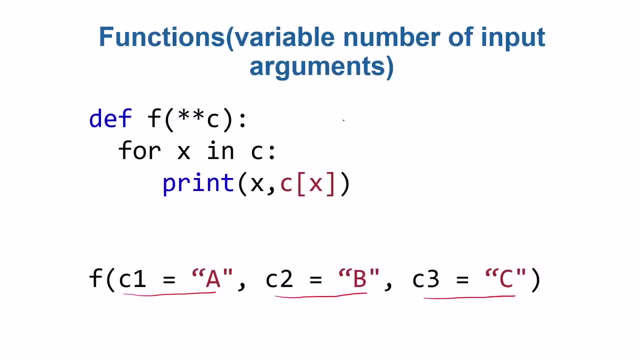 a call that can be made to a function, And remember the function definition in some previous slide was like C1,, C2, and C3 maybe, And then something. What if we want an arbitrary number of arguments to be passed, but we want their control? For example, let's say this: 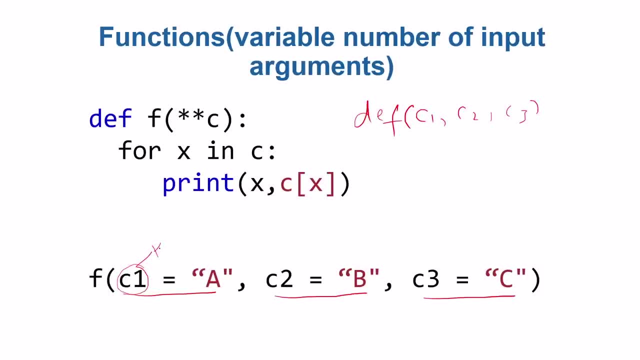 particular variable symbol name that acts as a key, that's a variable name and that's the value. so let me call the variable name as a key and let's: this is the value that is copied in the variable. that's another key, that's a value, that's another key, that's a value, and so on. what if we? 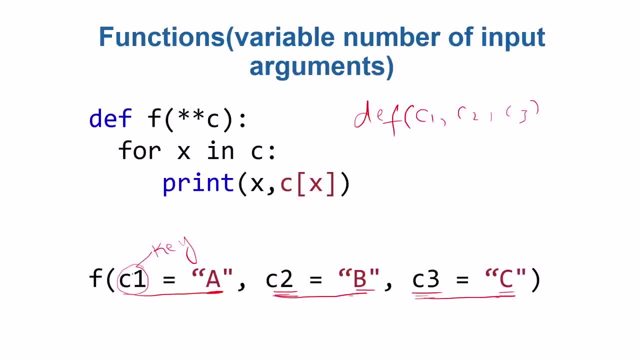 have a lot of key value pairs. what if we have a lot of them and we also want to check which value is of what key? let's say we we want to specify those, but we want to specify an arbitrary number of them. let's say here, for example, there are only three. let's say we want to pass five of them six. 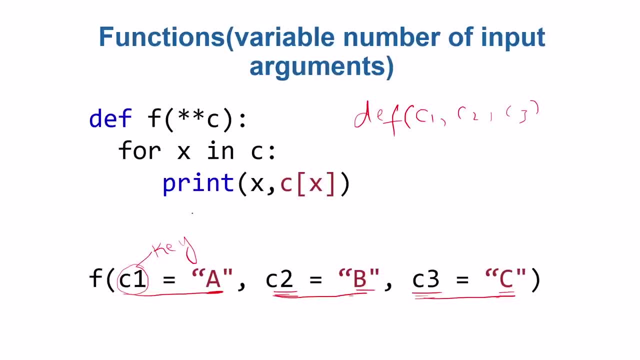 of them, and then we want our function to perform accordingly, no matter how many input arguments it received. yeah, and, and maybe inside the function we may have applied a check- that if the key value is c1, then do this processing, if the key value is c2, then do that kind of processing, and so on. 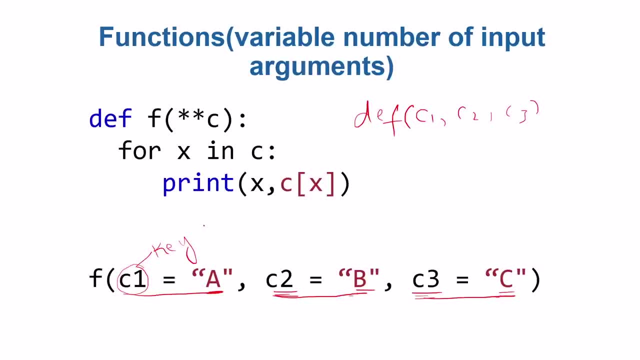 let's say for based on different variable symbol names, we want to process the value differently. how can we achieve that? and still having the need that these number of variables can be can can be in a variable variable length, they can be an arbitrary number of those. so python gives you again a very, very 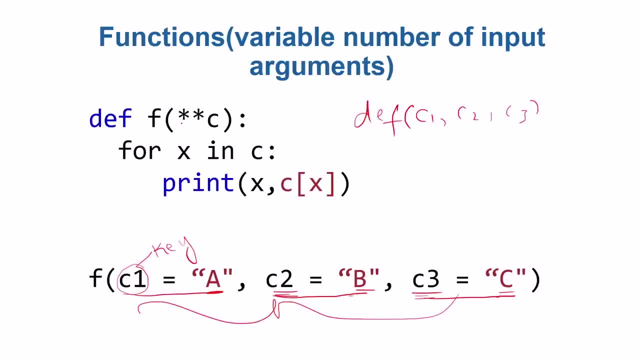 simple way: rather than writing a single star, you write a double star and then you receive in whatever variable name. and now in this double double star means you are receiving a key value pair list. it's a list of key value pairs and you're receiving a key value pair list. 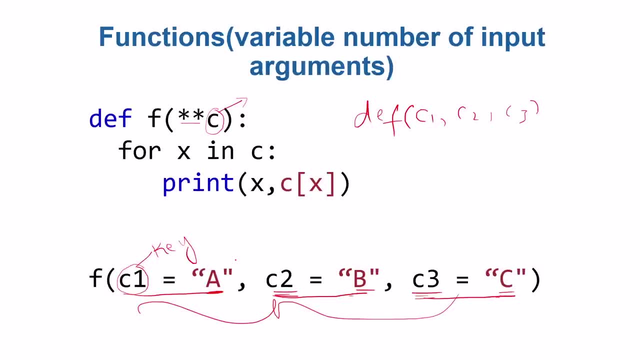 we will see that. that resembles to that resembles to a data structure in python called dictionary. we will see dictionary later on in detail. but right now, just just consider that this input argument, this input variable c, it contains a, it contains a list of key values, pairs, and then you, just, you can just iterate over the c, you can just apply a for loop to check. 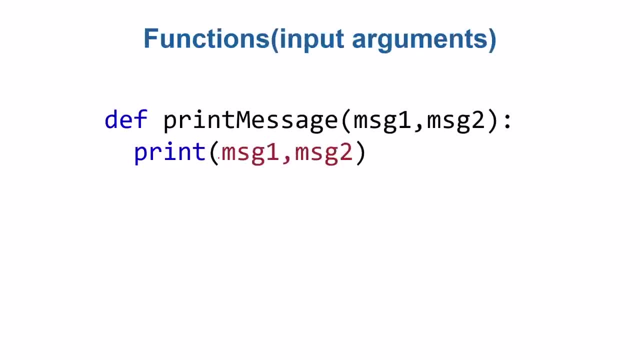 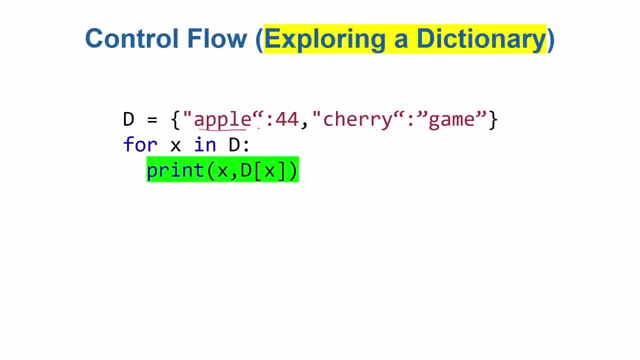 the contents of this. remember, we have actually done that kind of thing in the, in the portion of loops. uh, yeah, here, remember that was a key and that was a value. that was a key, that was a value and we did that thing. we could explore the. we were able to explore the dictionary. 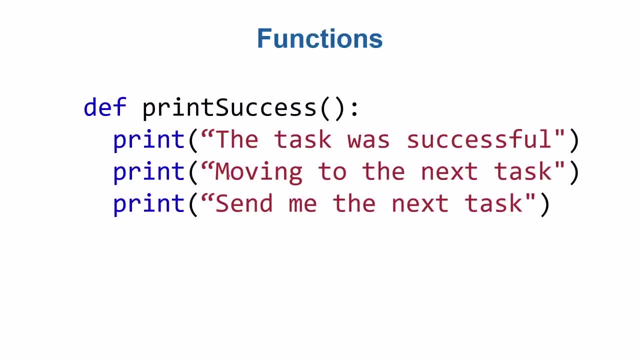 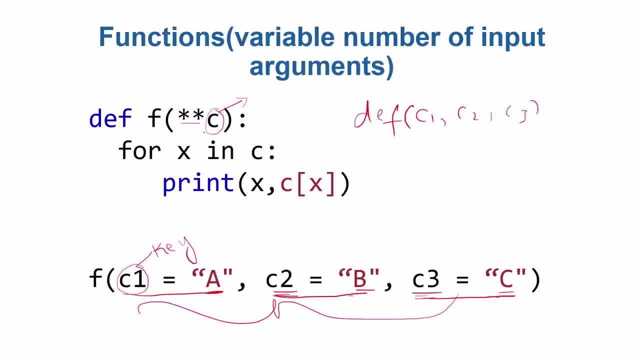 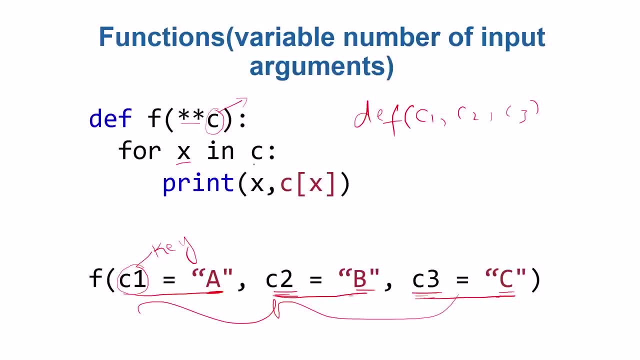 this is value. you can this: x points to the first key, then c of x points to the value based on the, based on the key x, and then x points to the second key, then the second value, and so on. you that that is very simple procedure. you are just printing all the dictionary. but you can, you are printing. 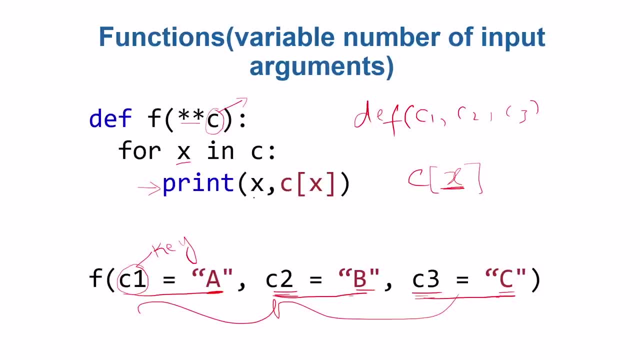 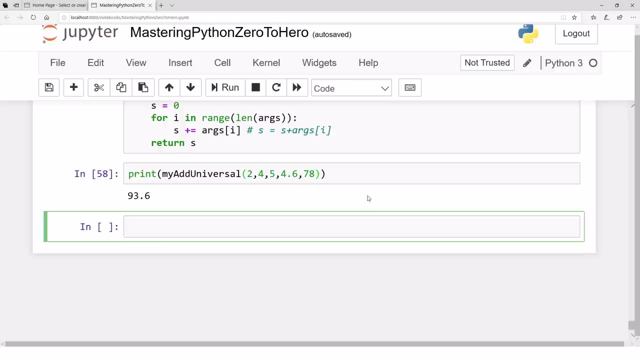 all the variable names and their values. but you can do a very complicated processing if you want to. um, let's go to our friend jupiter notebook to just get convinced that this indeed works. let's see. so let's define a function first. so def, that's the function name, is print, all uh, variable variables and 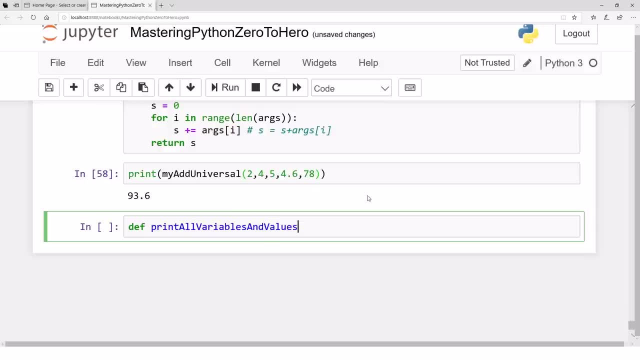 values. so that might be a function name. well, that's lengthy one, but descriptive one. maybe we can make it more descriptive. print all variable variable names and values. wow, that's more descriptive, i guess. so it receives, let's say double star, any variable. let's say the variable name is: 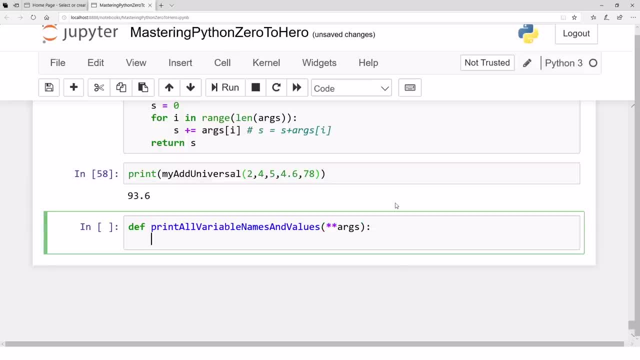 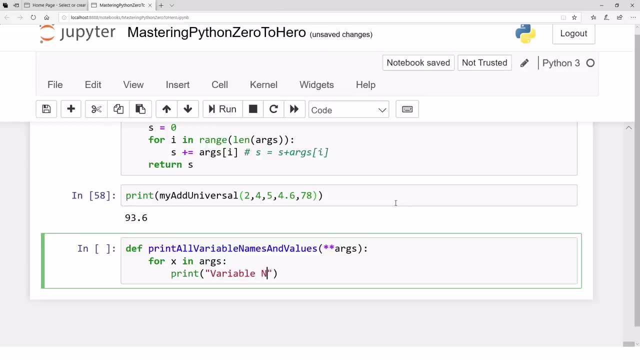 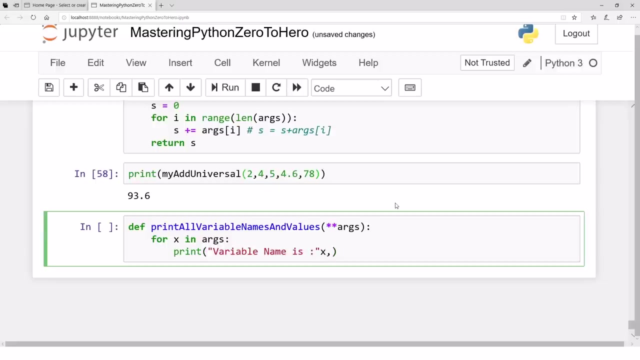 again. let's say args or or anything, whatever you want, then what we do is for x in args, just print it and then the answer is home. we can print table. if we're just doing repeat, we can经 an arrow for x and then say: variable name is num the state and for url we can add a name naming. 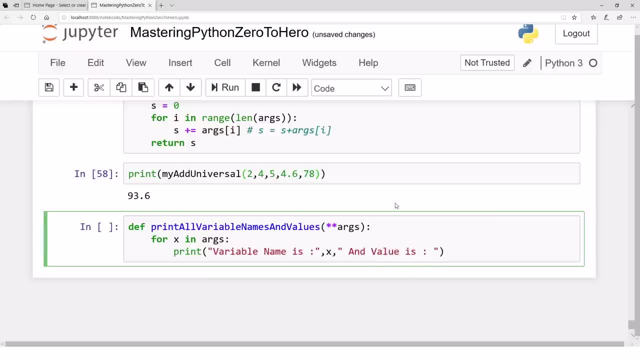 and lol as some of these splitting by saying x, something is missing. okay, OK, northern texan, value is spring-Straight x and then just continue and value is value is argz of x. so this is belongs to x and we are now going. please don't forget that arrow name is num down here, but we wouldn't end with any item after. 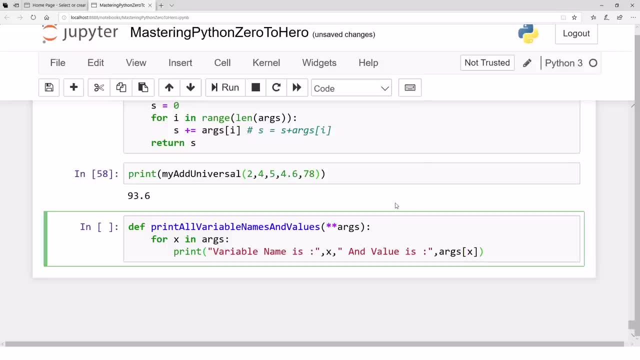 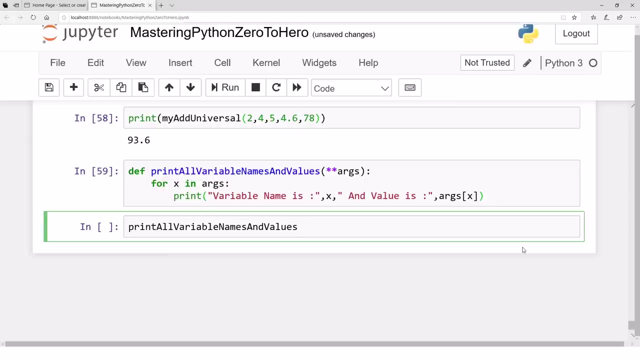 So let's say: you done this. you did this, so the variable name is this and the value is this. Okay, and you want to do this for all the variable and value pairs that you send at the call time. So now let's call this: print all variable names and values and let's call this: let's. 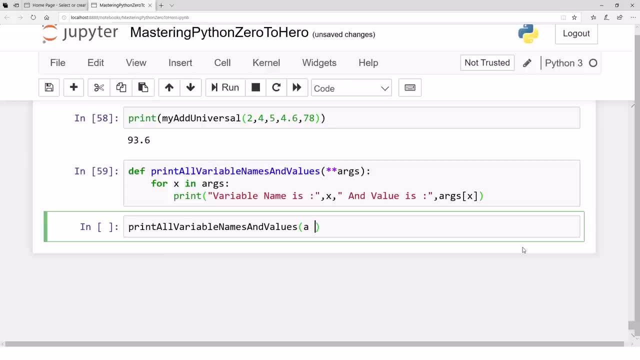 say, the variable first variable name, let's say, is A and its value is 3.. The second variable name is, let's say, B, its value is capital B. Let's say the third variable name is C, its value is CCC. and let's say the fourth variable name, I mean you can define. 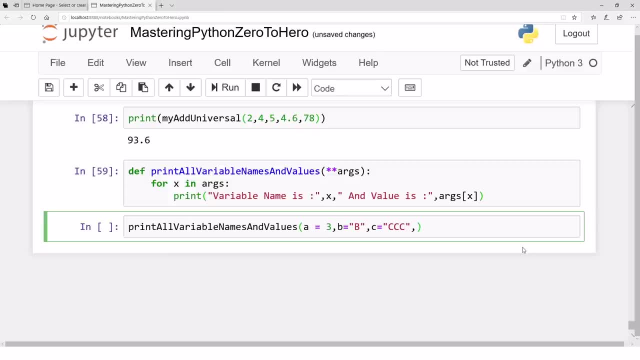 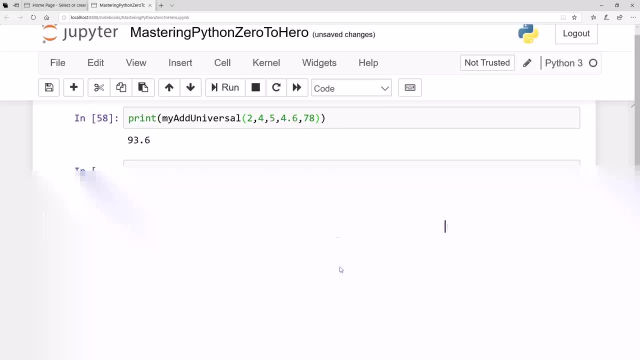 an arbitrary number of arguments here. Wow, that's amazing. Let's say, the fourth variable name is Y, its value is 6.3.. 7, and further notice, you can pass variable and value. all have different types, I mean. 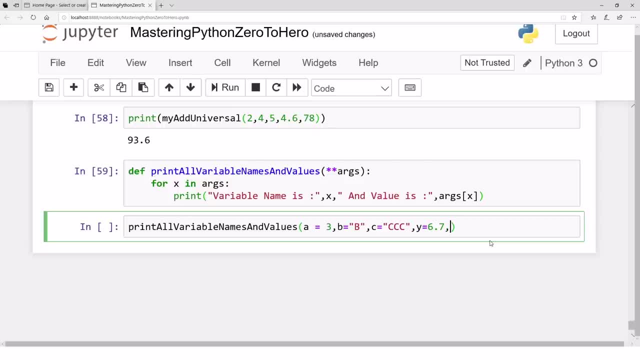 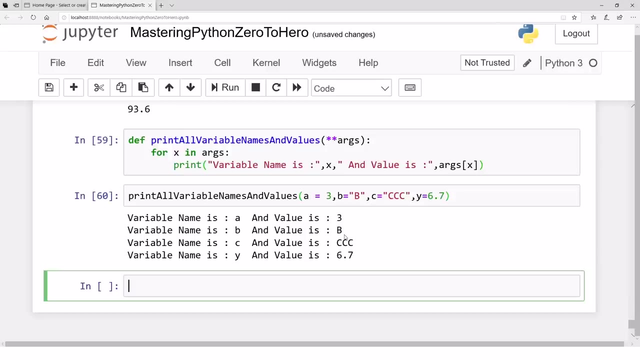 different number of them and much more. yeah, you can do that. So let's call this function by just having four variables and their values. Let's see what we got. So variable name is A and the value is 3.. Variable name is B and the value is B. Variable name is C and the value is CCC. 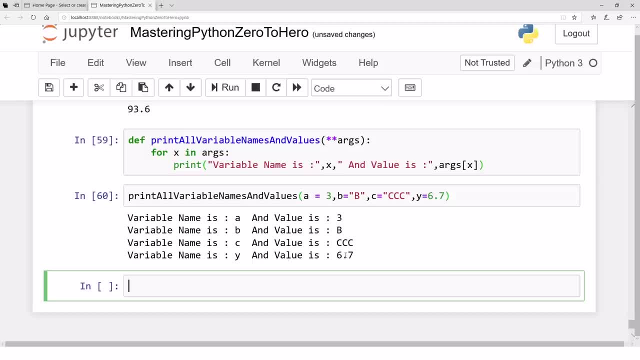 Variable name is A and the value is B. Variable name is C and the value is CCC. Variable name is Y and the value is 6.7.. You can give an arbitrary lengthy list here if you want, and Python just allows you to do that, and it allows you to do that in a very, very simple way. 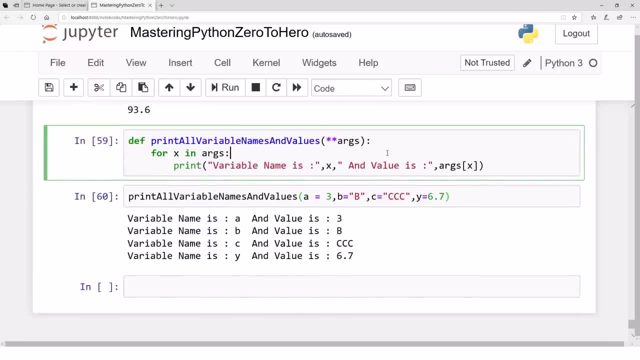 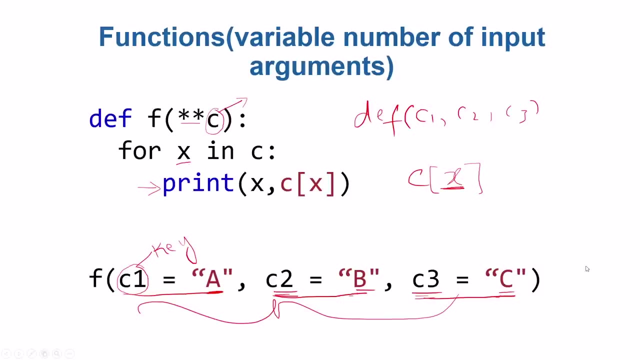 That's amazing. That's amazing. I mean, that's what a high level language, or really a powerful language, should have a feature. So Python does have this feature. I'm really amazed, I'm really astonished. I really astonished Python. By the way, I'm not saying the other languages don't have this. 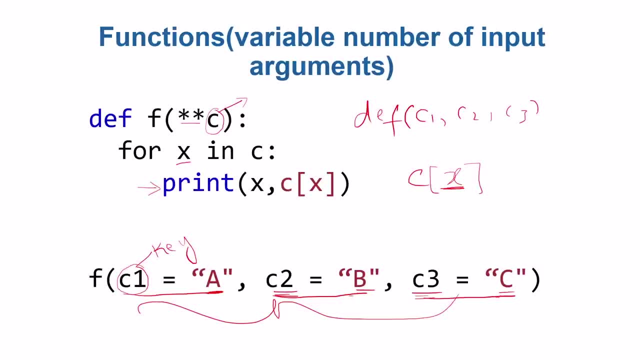 Several languages actually support this kind of feature, but Python supports it in a very easy way. It's very easy to do that. I mean, it's not a rocket science, Yeah, Okay, So now we have handled an arbitrary number of arguments. even with ordering is really. 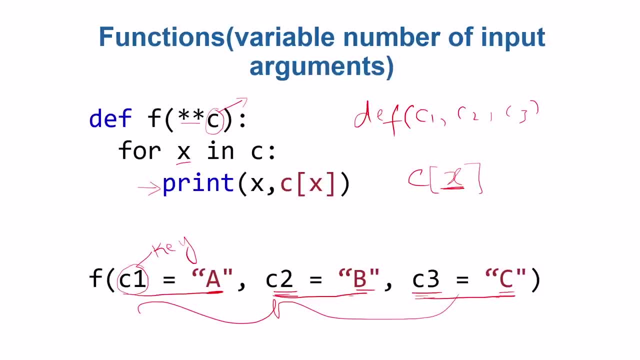 controlled. We have one or two more videos on functions, Just one, Just to explain a bit more. Then we will practice on Jupyter Notebook. We will practice, We will play with these functions a lot and we will be calling one function inside the. 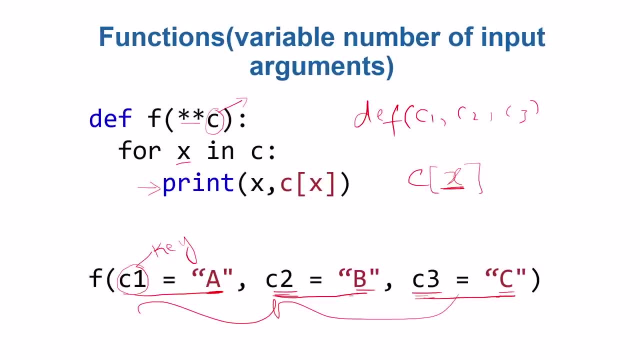 other function and so on. We will be having one better program, just program on Jupyter Notebook, just to get comfortable with these functions. But before that let's have one or two more things to discuss about the functions. Yeah, Let's see. 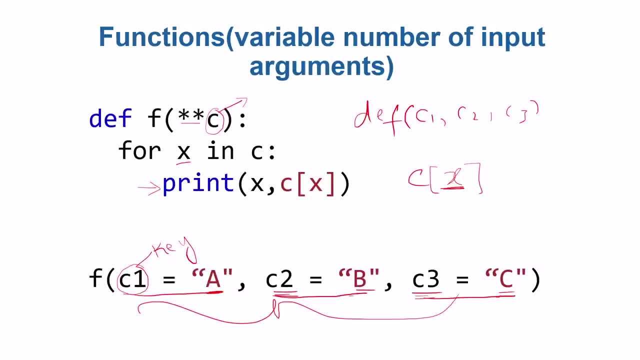 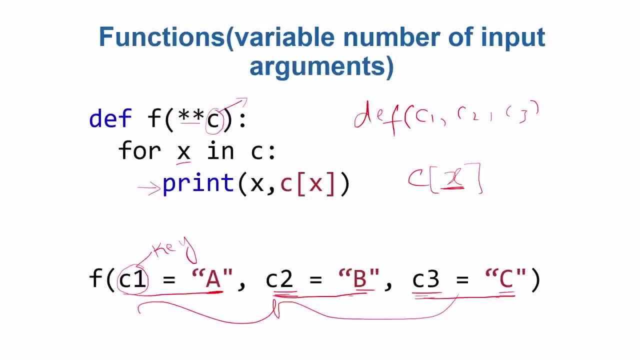 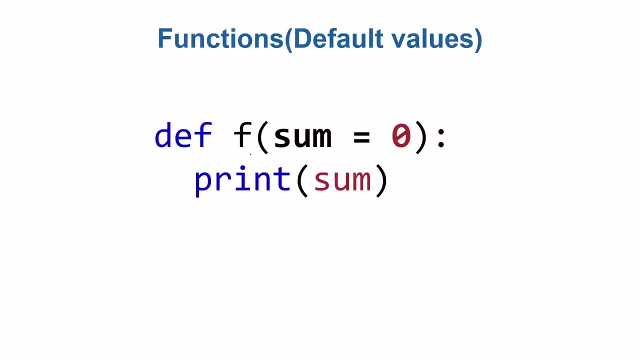 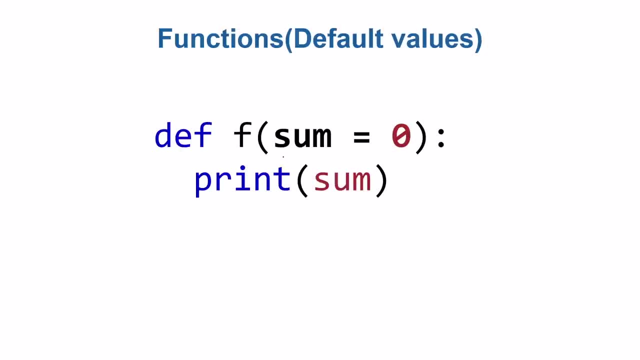 Okay, I really want to talk about these default values for a function as well, because that's important and mostly needed. The default value is a value of the input variable that you assign while you are defining a function, and if the value is, For example, if you call this f with, let's say, the input value three, then three will. 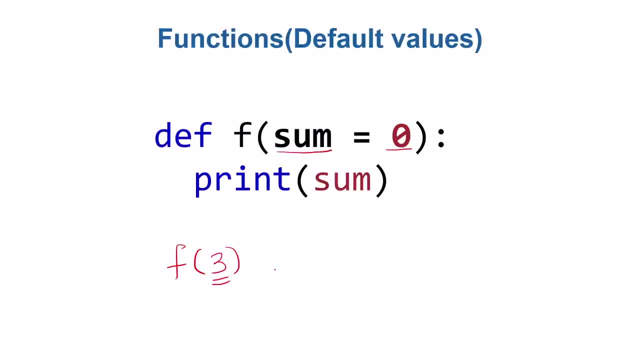 be copied in. the sum print will be three, but if you call this function without the input, then this value acts as as if you have passed this. so this is the default value. if you do not supply the value, this is the value that is going to operate and, by the way, you can have multiple variables with default values. some. 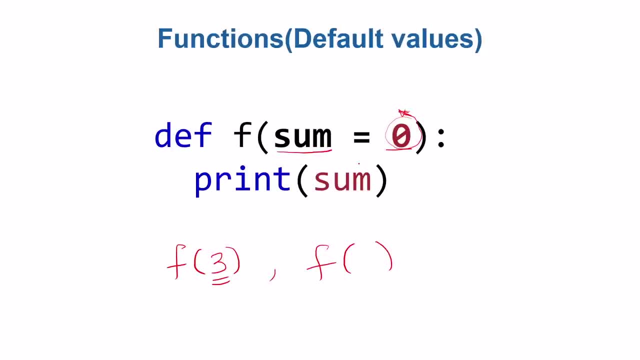 variables with default values defined, some variables with default variables, default values not defined, and so on. so you can have this one. care must be taken here that the default value when you actually define the function and you compile this function, actually you, you run the cell shift, enter in jupyter notebook at that very time this variable is assigned this value at that. 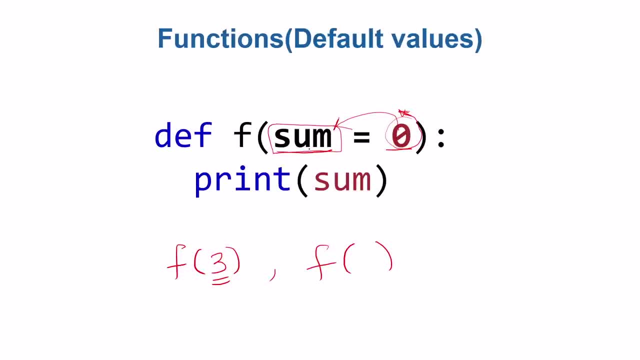 particular time. it is not assigned at the call time, so sum equals to zero is already there when you actually press shift enter for a cell that contains this code. now, later on, if you pass a value, that value will be overwritten on sum. if you don't pass the value, the zero will go on. it looks like very easy, but one care that i. 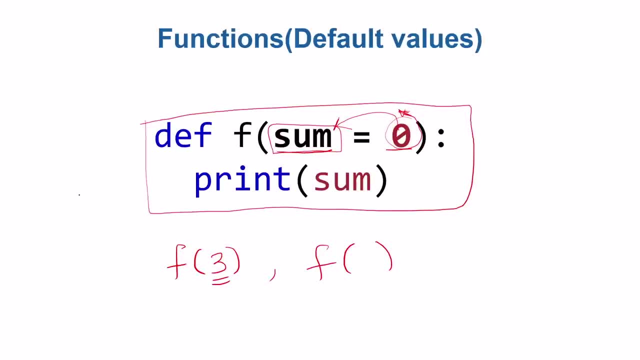 want to mention here that i haven't mentioned earlier. in python there are certain variables that are uh, that are referenced rather than copied. i will discuss the referencing in the copying in in detail in data structures, but let me just tell you one one, one example. let's say: 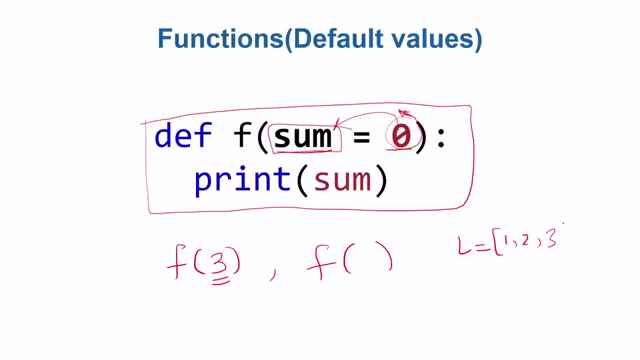 you defined a list- let's say one, two and three- and then what you do? you copy the list into another variable, let's say l2. what will happen is in the memory, this list in a particular way. this is not the exact view of the memory i'm just showing you. 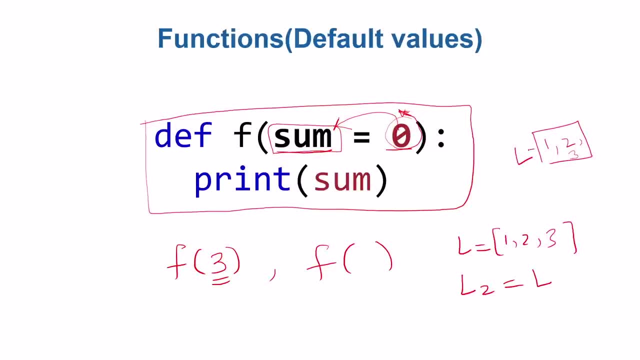 let's say this is the particular memory layout for which this l is pointing to. this. l is labeled for that, l2 is also labeled for that, which means actually in memory. this is not the copy of the structure that is made. i mean, this is not like in variables, for example, if a is equal. 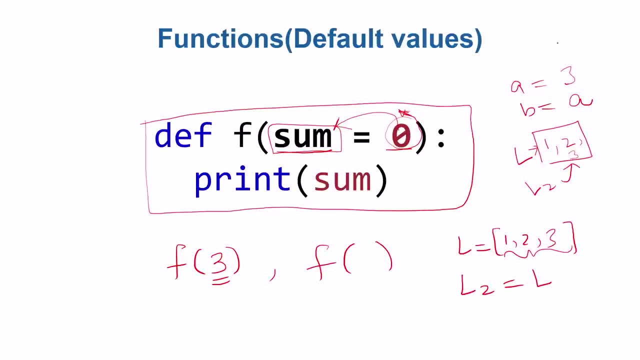 to three and b is equal to a. a will be, a will be a position in memory and b will be a separate position in memory. that is what a view of the memory in ordinary variables are. but there are certain variables in memory just for memory efficient and code efficiency and time people. 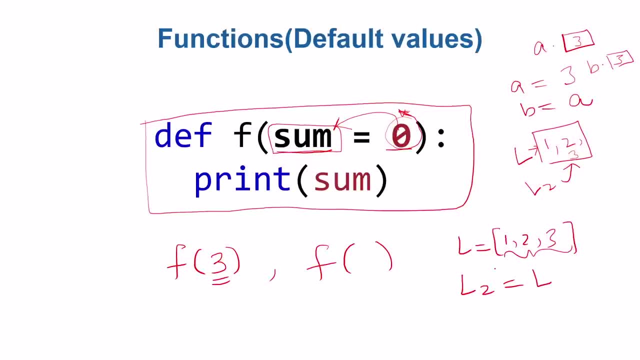 have. people have designed these data structures in a way that when you copy them, when you just assign a variable to another variable, the memory view doesn't change, the just it's. it's another name for the same, for the same, uh, for the same memory location. so what happens is if you change any value in, let's say l2, let's say l2 at the very, at the. 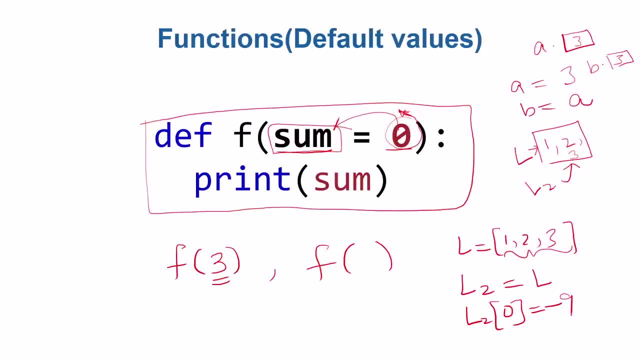 zeroth at the zeroth index. let's say you change that by minus nine, the, because it is the same view in memory that changes minus nine. and now if you print the elements of l rather than l2, you will get the changed value, you will see the change value and that happens. 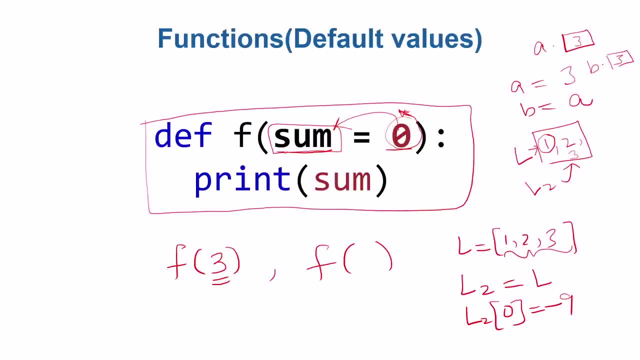 now why that is important in terms of these default values here for the function. the reason is, if you are accepting a list, let's say, uh, the default is a list and you're accepting a list and you are also defining some default value for the list, if that's your definition. 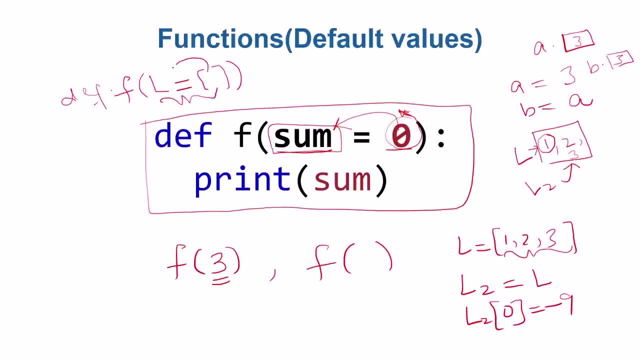 let's say then, this list, this default value, is assigned at the at the very first, at the very first time, and this l is really a local variable inside, inside the, inside the memory now, when, once this cell is run, not the call time at the, at the, at the, so so what? 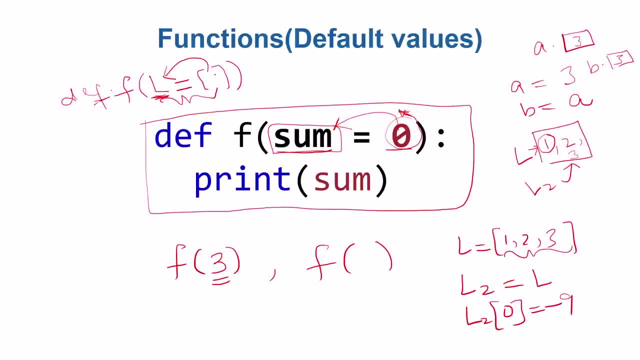 call the compile time. when the cell is run, this l is assigned this, and that just happens once. now if you call this list with some other list- let's say l2, let's say two, three and four- then if you call this l2, l2 will go there, it will be copied in l and everything is fine. but don't then uh expect. 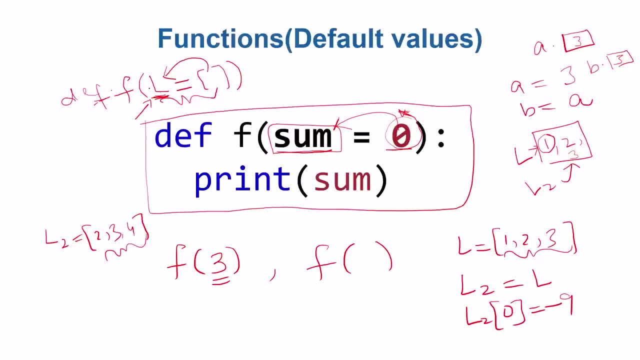 this the contents of l2 to stay same as stay in l, because l is this: default values. they are assigned just once and they stay as it is every time you call the function. they don't change. um, they are not assigned at the call time, they are assigned at the compile time and they stay fixed so that. 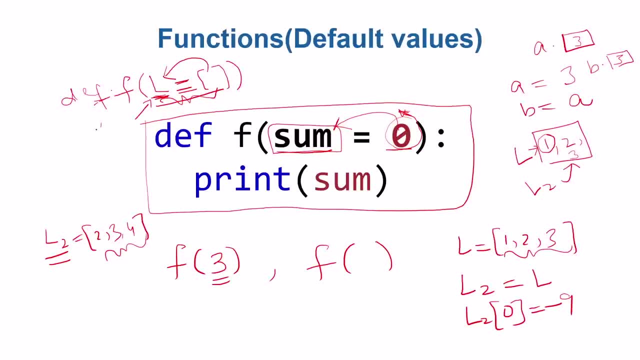 care must be taken. i will show you that example, that particular example in jupyter notebook, shortly. this: this might be confusing right now because we have not defined, we have not seen lists in detail, but, um, i just want to make this point, i just want to mention this because that's important. 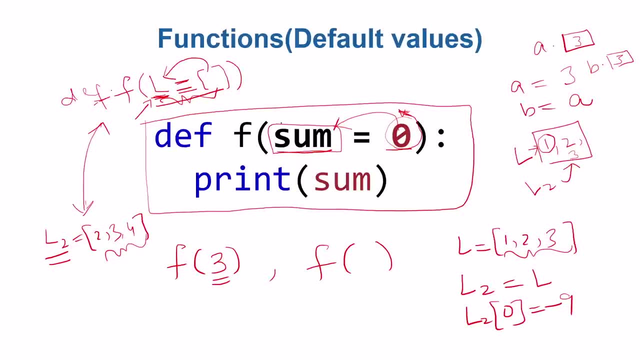 difference with ordinary variables. that i mean default value is just. i mean just like, like a value, and if you don't supply a value, the default value just works. but with the variable- that are reference type variables- you may expect something else and the python function behaves maybe. 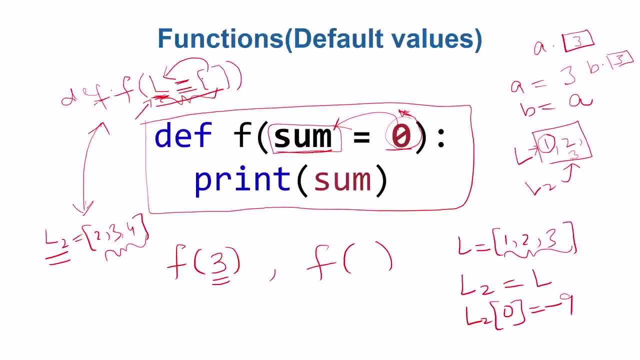 differently and that's because these default values, they are assigned at compile time. they are not or compile time actually, this is not a compiled language. i should not use the word compiled- compiled again and again. just think, when we define this function and we run the cell at: 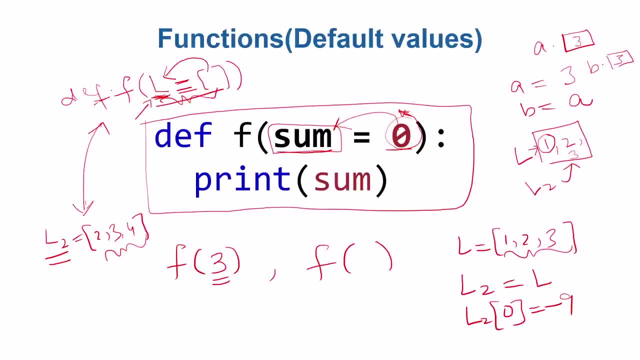 that particular time the default value is assigned. and the default value never changes. it stays fixed. um, yeah, so, and i will show you that example. why don't we move to jupyter notebook and see that example? yeah so. or or why don't we do that in the next video? what do you think? 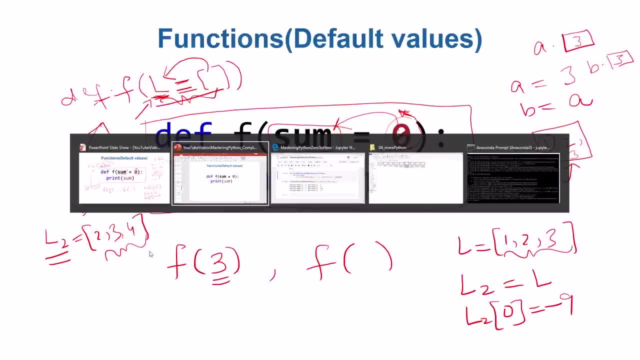 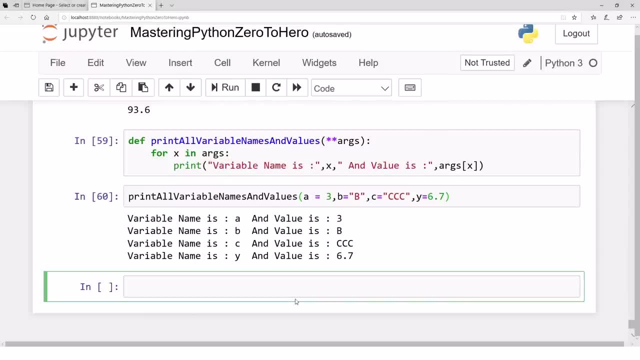 this video. okay, same with you. okay, let's go to jupyter mode notebook and see the default values. for example, let's see uh. let's say we have uh, define a function. let's say uh, gg, and the default value s is equal to four. let's say that's a default value and we want to print. let's say s. 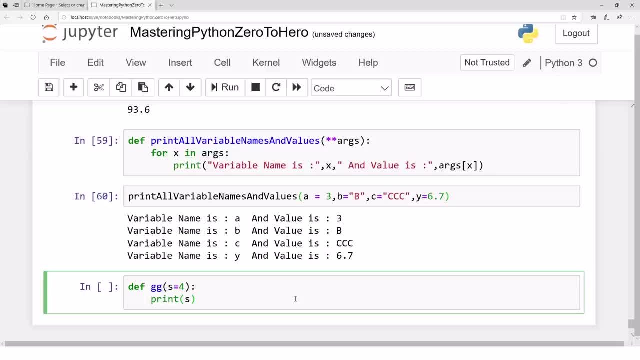 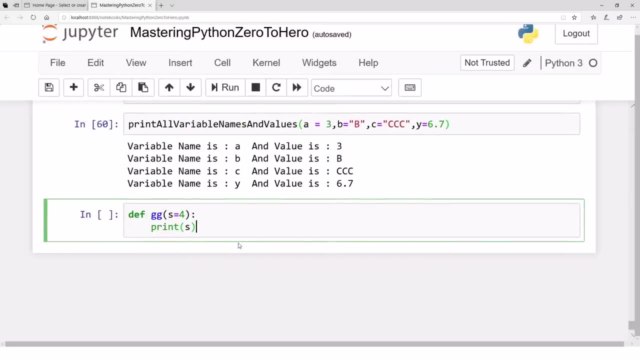 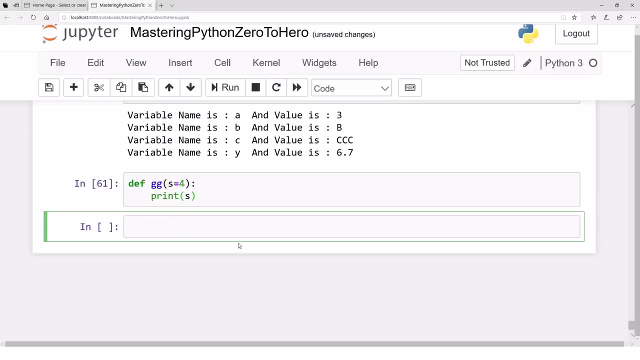 if available, uh, from the call time. if not available, then four will be printed now. we print now, right now. we are going to print now. we are going to press shift enter at that time. s is assigned to 4.. s has no value. 4 it. 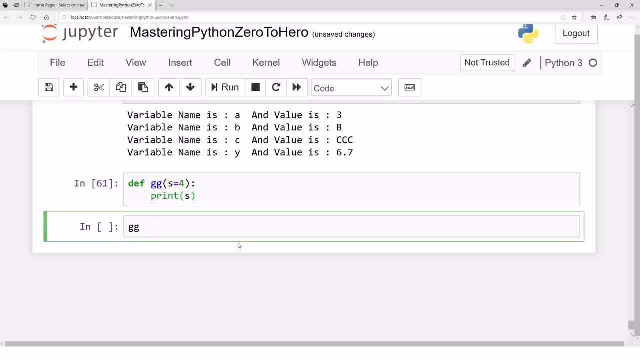 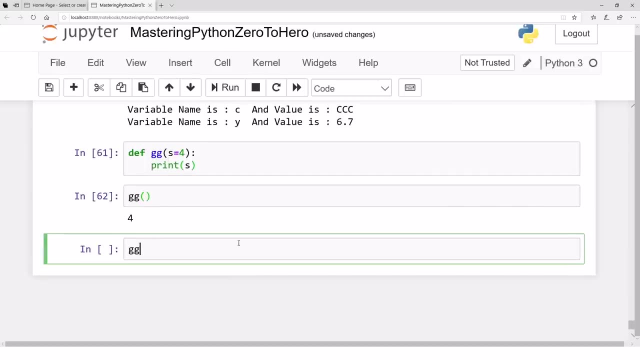 is assigned there. now we call gg, that's it. and we call gg without input arguments: now the 4 will be printed. if we call this gg with some input argument, let's say 56, now the 56 be printed, no problem, everything is fine. let's see about the lists, for example. let's say the list is: 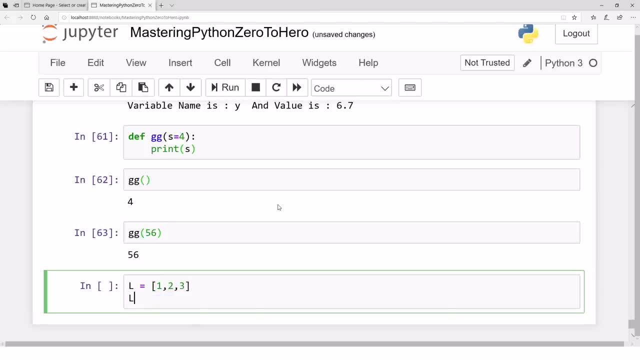 let's say one, two, three, that's a list. and then l2 is simply. let's say l2 is l, then what we do is we change the contents of l2. let's say, we change the very first value in l2 and we place that value as 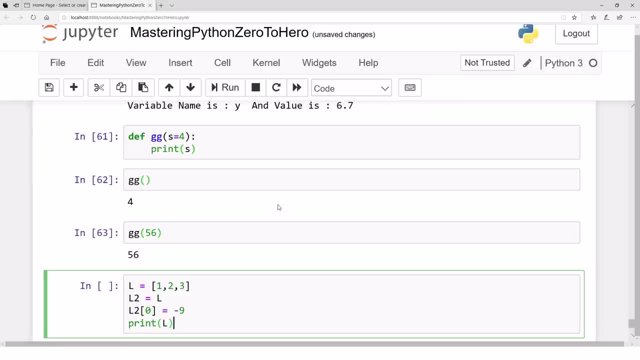 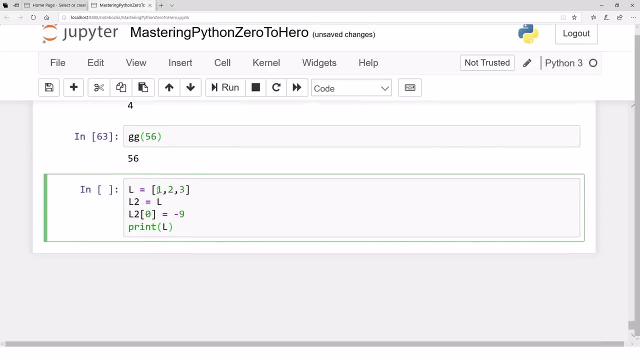 minus 9 and then we print l. now you might be expecting that l is a different thing, l2 is a different thing because l and l2, they both are pointing to the same memory. uh, this, the content through l2 actually changes the memory view and l also changes and that gives the result. 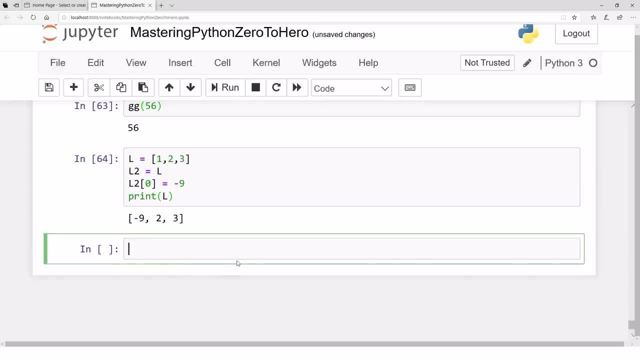 minus 9 in l. well, the behavior that i want to show you is different in the default values. when we, when we talk about, for example, let's say, we define a function, ff and it accepts a list and the default value is empty list or the default. 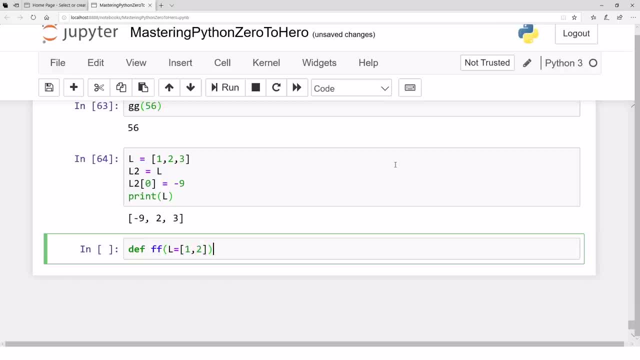 value is, let's say, 1, 2. that's the default value. let's say: if, if, if no list is passed, the default list is 1, 2.. now, in this particular scenario, if we just print, so for example, for i in list print i. let's say: 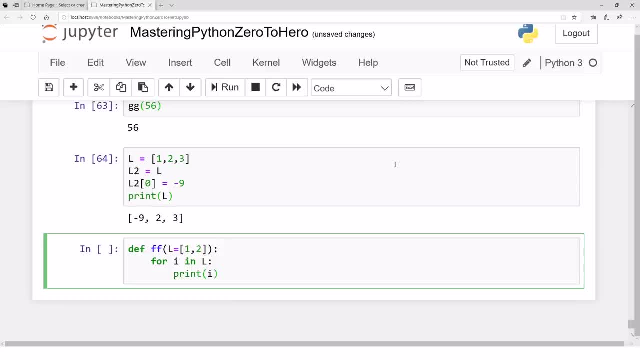 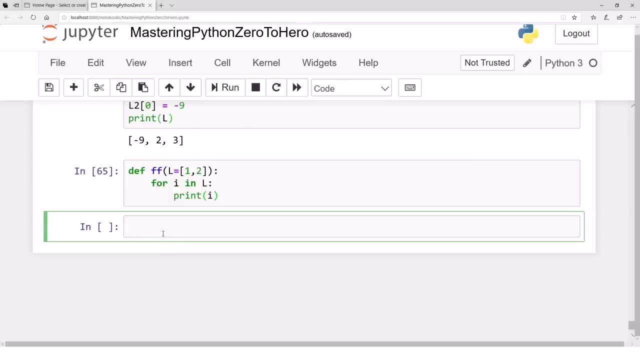 we just print all the list and that's it. now we will press shift, enter and at this time this l is assigned this value and that's a default value that never, that is not going to change. now let's say we have an l2. that is simply, let's say 2, 3 and 4, or let's say 12, 3 and 4, and what we do is: 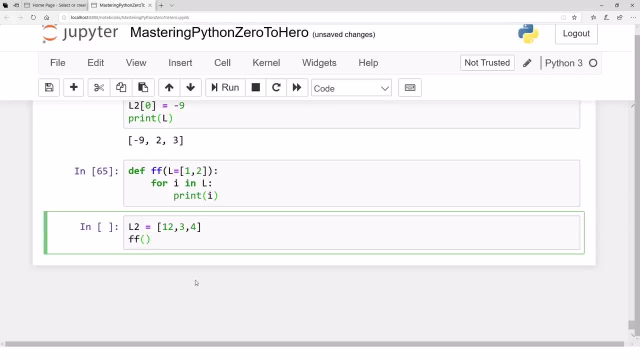 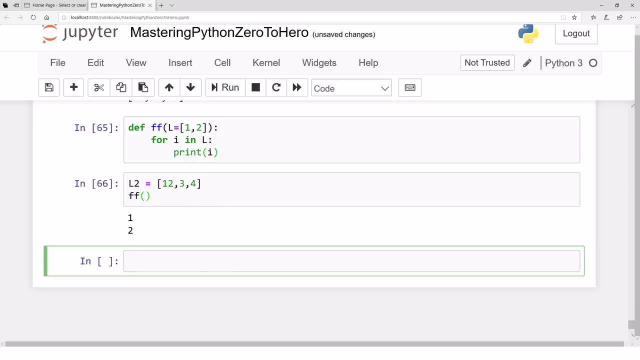 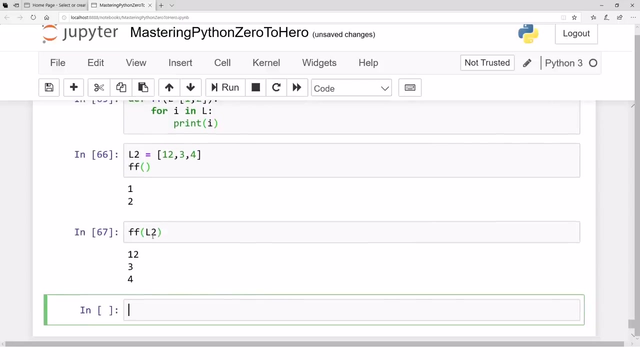 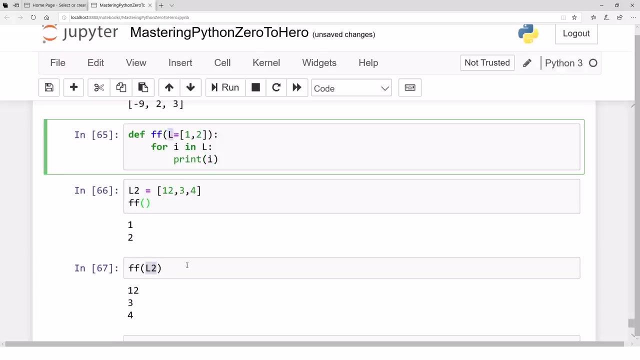 we call ff and we just press shift enter. now, um, oh, why not? oh, oh, we call ff without anything. so the default list is printed. if we call this ff with uh, l2, the l2 will be printed. now the notice that this l2 actually is copied in this l because we supplied it. so l and l2. you may tend to think that. 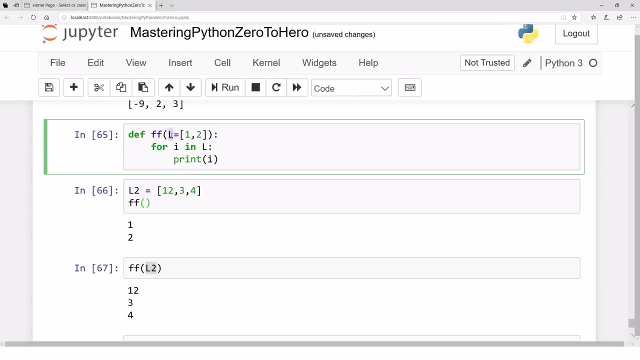 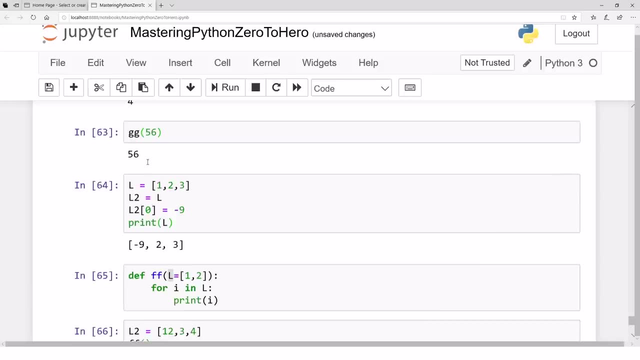 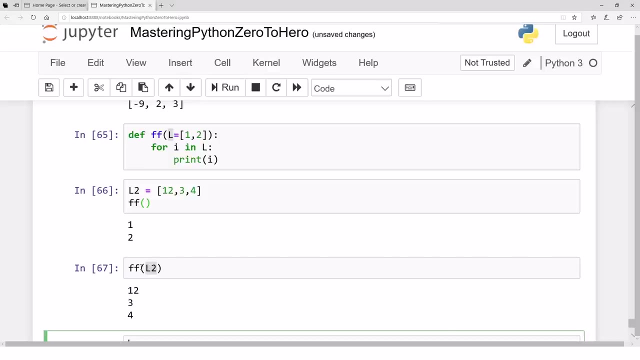 l is the same in this case, but l is now also pointing to l2. i mean, l has also the same contents as l2. so if next time, because because of the behavior of these lists, because they are by reference, next time you may, you might be thinking that because l2 is past there, so l2, l is. 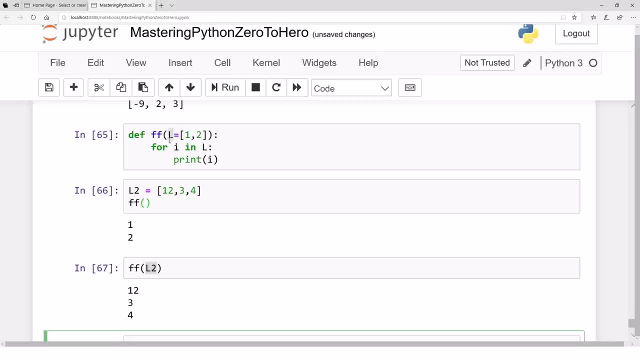 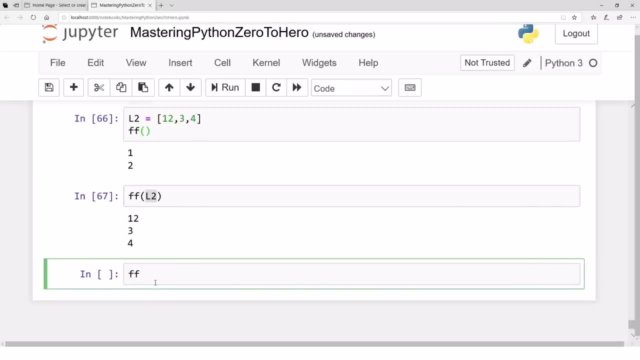 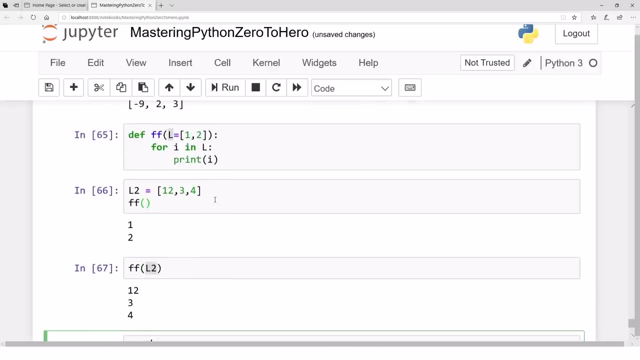 also l. l2 is copied in l in a memory view layout, so l has also l2. and next time if we call this function without input arguments, then l might be pointing out to l2 value. so 12, 3 and 4 might be printed. but that is not going to happen. the default values they. 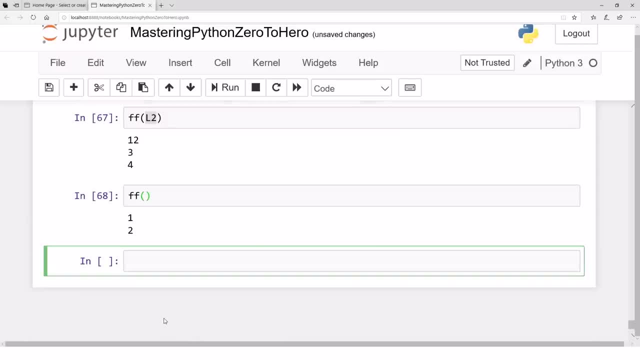 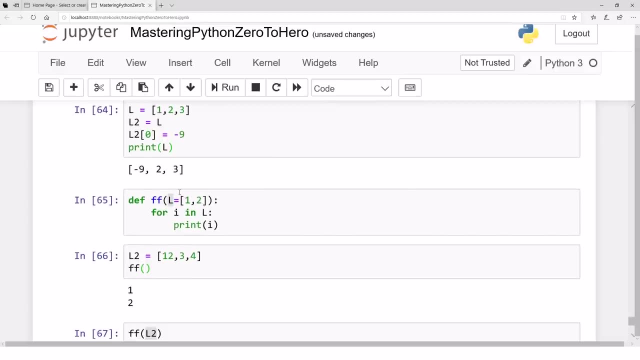 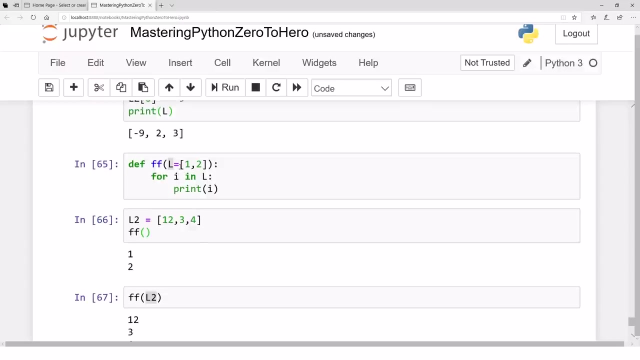 never change. so again you will be getting one, two. so the behavior of these reference type variables, that is different ordinarily. but when you do that in in the default value structure, that that that might work in a different way, and the reason is you. you must know that these default values, they 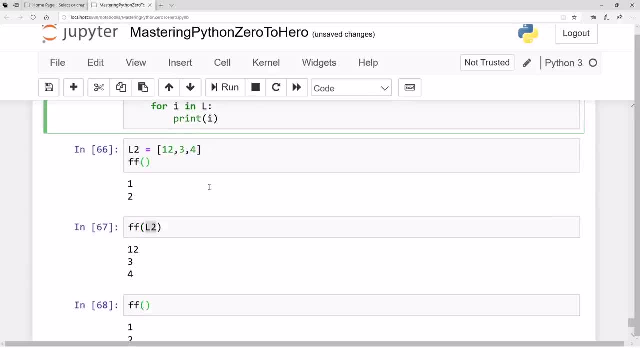 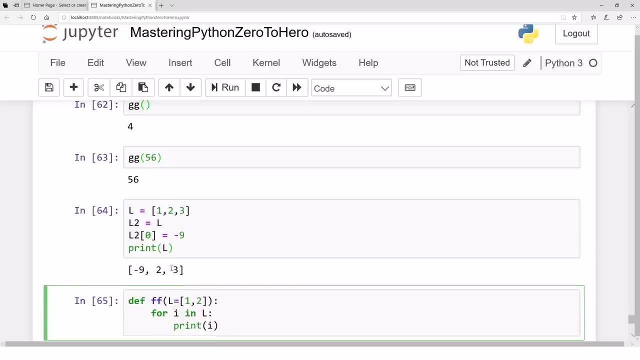 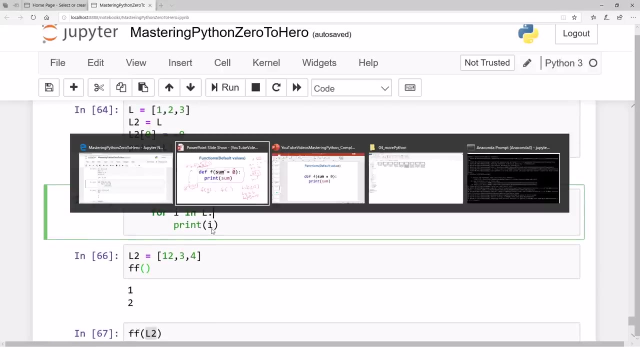 are assigned at at the time when the function is created, not at the function when the function is called, and they are not going to change whatsoever. so so that was about the default value. by the way, the default value was a simple concept. I guess I have made it too complicated by telling you lists. 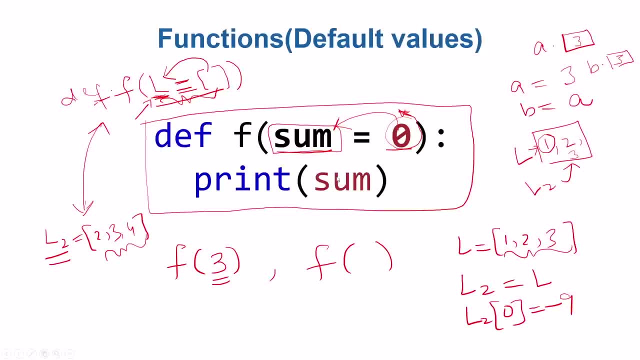 and default values and creation of the variables at what time and at the call time. I made this complicated. I guess I shouldn't have told you the list values and all that stuff, but but that's true. I mean, whatever I have told you is true. maybe I have told you in a very complicated way, but it's true. yeah, okay, one more video on the. 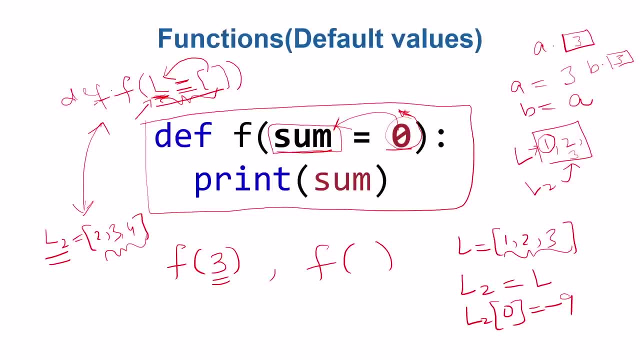 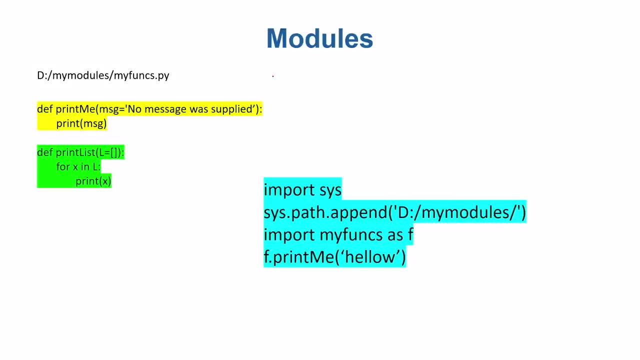 functions and then we will be practicing functions in detail on on Jupyter notebook. so just be your one more video with me. hope to see you in the next video. okay, this is probably the last video on on the functions. yeah, we will be having one more video, but but that will be like coding and practicing. 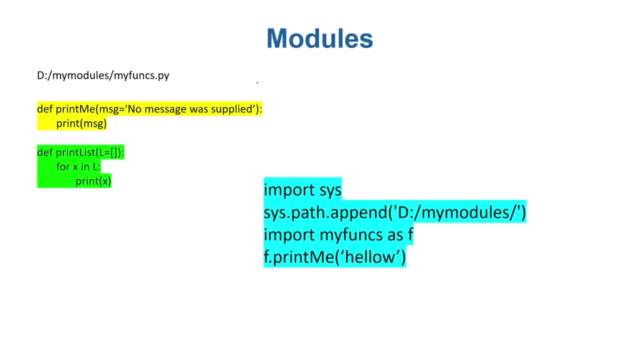 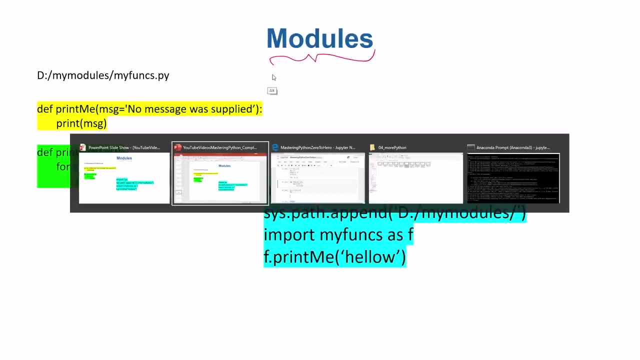 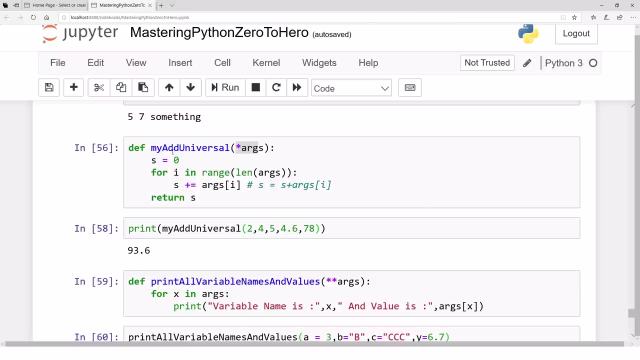 all the concepts that we've learned about the functions, not not something, not not new theoretical concepts. yeah so let me ask you a question to to actually make you understand about this slide. let me go to the Jupyter and ask you about a few questions. let's say you have. let's say, let's say you have this particular function and you let's say my ad. 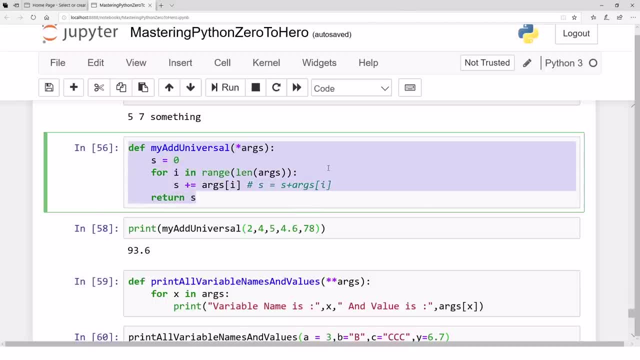 my ad universal. let's say we have written that function, maybe a, two or three, three videos before. let's say you have this function. you have written this function and you are very, very excited. wow, what kind of masterpiece you have generated. it can add an arbitrary number of values passed in it. Wow. but this particular function is written inside this. 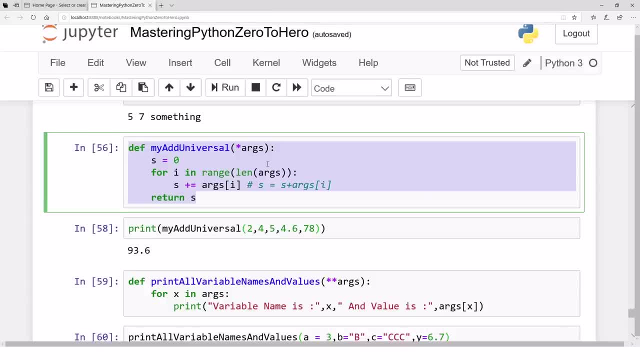 particular file which is mastering Python zero to hero. later on, let's say two or three months later, you are writing some code for some, some project, or you were doing something somewhere and you are writing code and there you just needed, you just needed. you just needed a code for adding a lot. 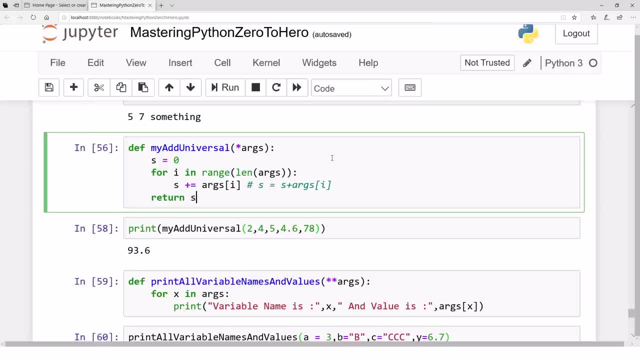 of a lot of values together and then you just remember, oh, I have written some function somewhere. how can you use that function? one way is to just go back to that file mastering Python zero to hero, and just copy this function, this particular, this code, and paste in. 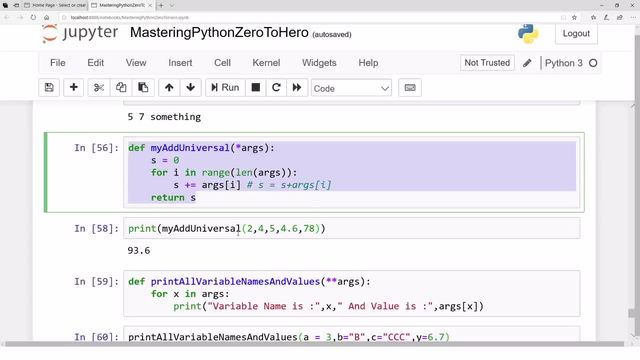 the new file, run that, register that and then call that happy. what if you want to use, let's say, a hundred different functions? let's say you've written a lot of functions in a lot of different files and now you want to use all of them and and let's say this is a repetitive kind of 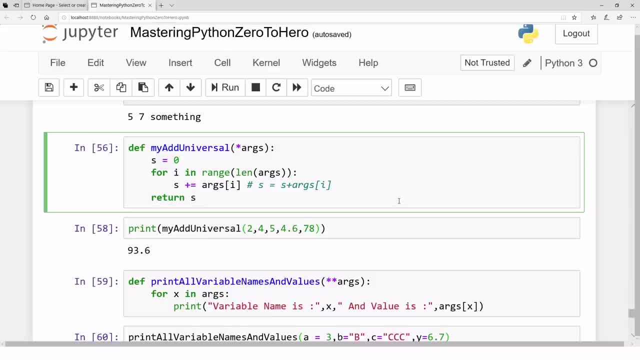 demand several times. you notice that this usually happens, that this particular kind of function you require almost every, almost in every project, let's say a set of maybe 50 or 60 functions that are that are required always. one way to do that, as I told you, is to just copy paste those functions in. 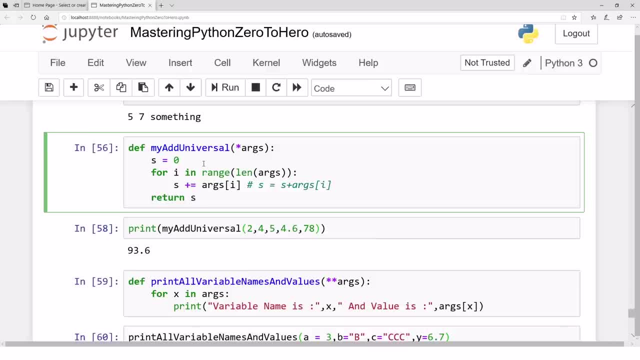 every file, run them. and do that another way is to just just- I mean, make a module, a file of containing just those functions and, whenever any of those functions is required, just import that module into your coding file, which is one line of code, and then access all the functions. 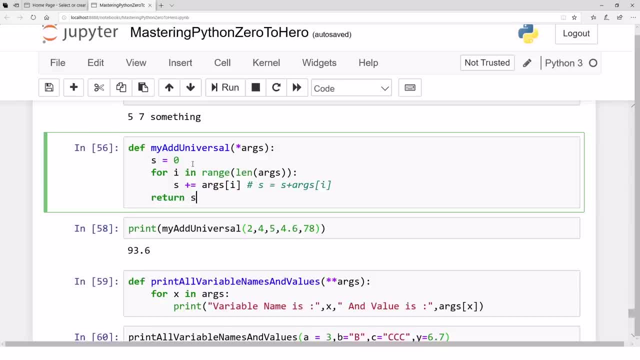 as if they were. they were they were actually available in in the code file that you are working on. so that's about the. that's about making modules of of. so so module is basically a Python file that contains functions that you want to use in several different coding projects or the functions that you don't want to. 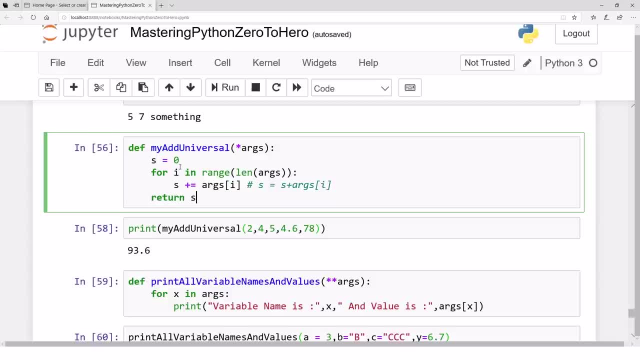 write in your the functions having the implementation that you don't want to write in your current coding file, so you can have several of those functions stayed somewhere else in a different directory. there's residing there. whenever you want to use any of them, you just import the whole module and 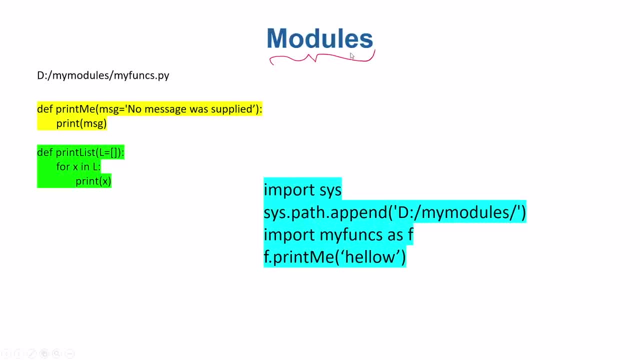 use the functions. so so module is just a Python file that that can contain a code for you that whenever you want to use, you can use it. normally it contains functions, maybe more than one function and several functions. normally it contains functions that you repetitively use and that you have written once in. 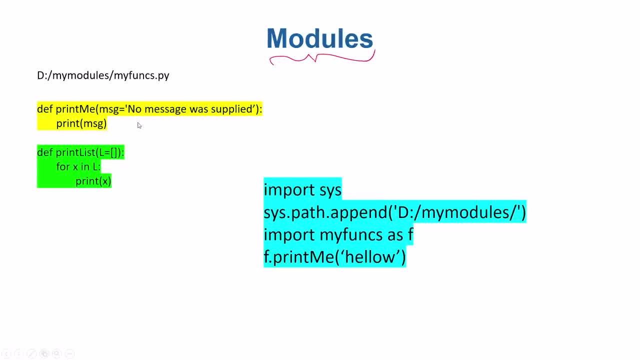 very careful way, and then now you want to use it again and again in several different ways. you need not to write the function definition in every coding file you need. you just make one coding file, or that that is the most important for you. that is called a. 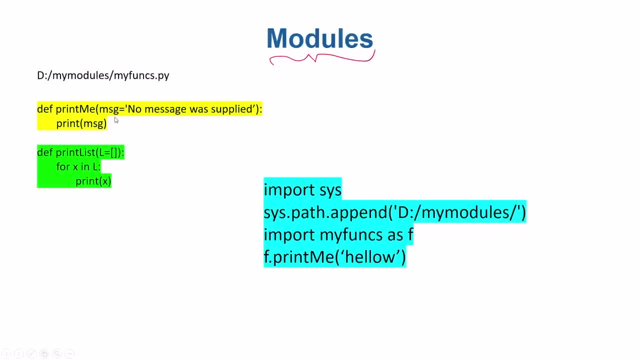 module. wherever you want to use any of those functions that are there in that module, you can call it, you can use it. so that's about the modules we are going to make. I'm going to show you one example of making module and how to use that. but 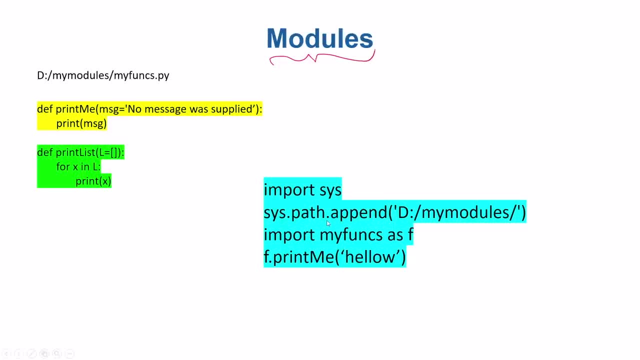 but to use the module we need to actually specify the path where the module actually resides, using this sys module so, and then we have to do some this import kind of commands and then I mean there is some work that we need to do to actually get this module running in our code, so in the 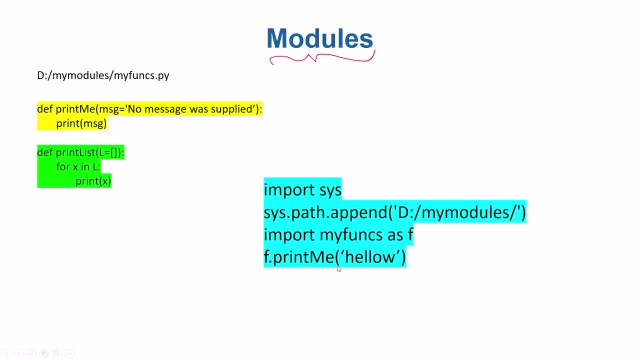 next video, I'm going to tell you what that extra work. very little amount of work. what that extra work? you have to do so here, for example, myfunxpy, that's my Python file and it contains these two functions and let's say, I want to use 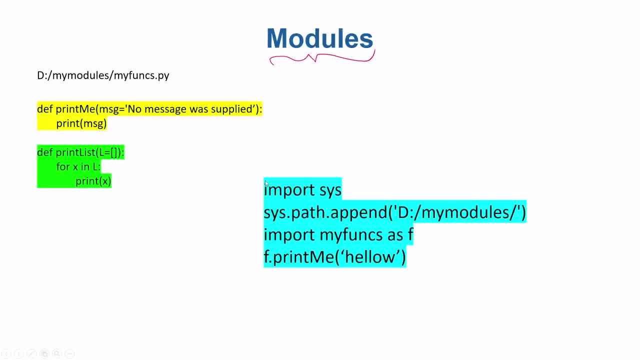 one of these or both of these functions in some other file and that file contains this particular code. so in the next video I will show you how to how to actually make and use the modules. yeah, so hope to see you in the next video. okay, in the last video I told you about modules. module is just a Python file. 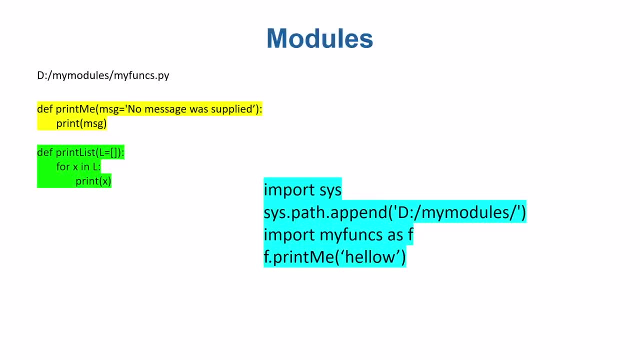 that can contain a code that can be used anywhere if you want normally that module, normally the modules, they contain a lot of functions but they can contain variables and other values and and so on. so think about file my func, start by that: contain this, these two functions, and think about a different file maybe. 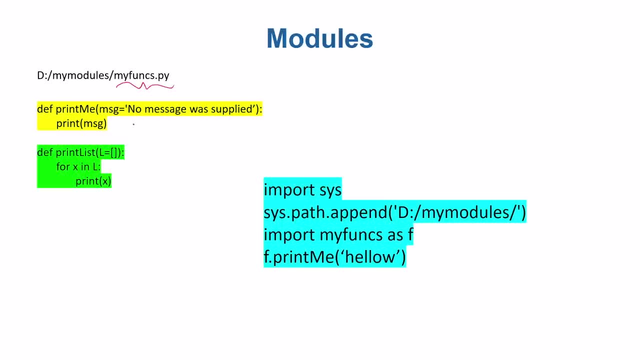 Jupiter. maybe you're working in a Jupiter notebook and now you want to use these two functions, so you first have to import another module called the system module sis. you have to. you have to make this path available. there are a lot of built-in modules that are already there in the path, all the already there in the search path. when 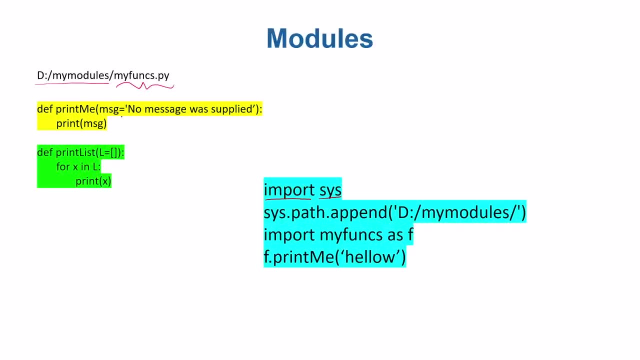 you want to call a function, it is written in some module that is already in the search path. if you are making your modules, you have to either either copy those those modules into the module and then you have to import the modules into the modules that are built-in, or, if you want to maintain them separately, 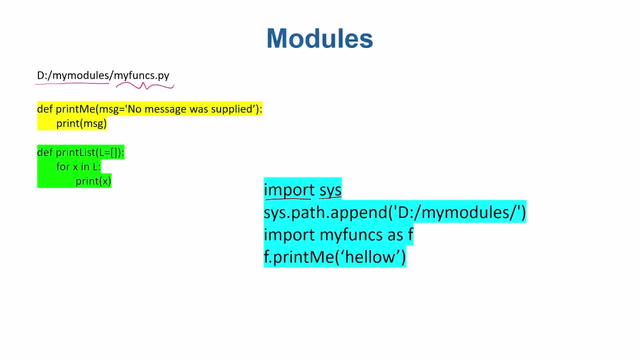 somewhere else, then you have to add the part of these in the search path as well, and the way to actually insert this path is sis, dot, path, dot, append, and then you actually write the top of the directory where this module file, one or more files, are located. once this is added to the path, now you can write the: 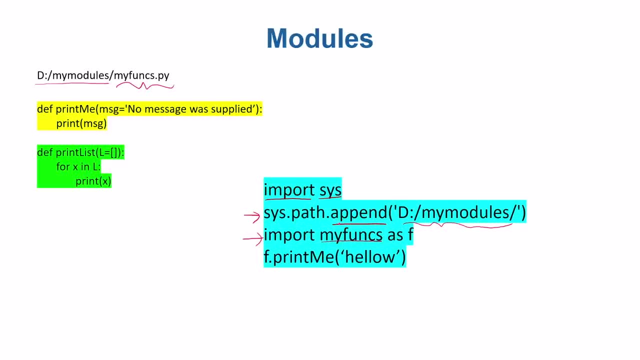 import and you can import your file as it is, or you can import your file with some other name if you want. You can rename that on the fly, if you want. Once this is imported, now you can use all the functions, like the built-in functions. 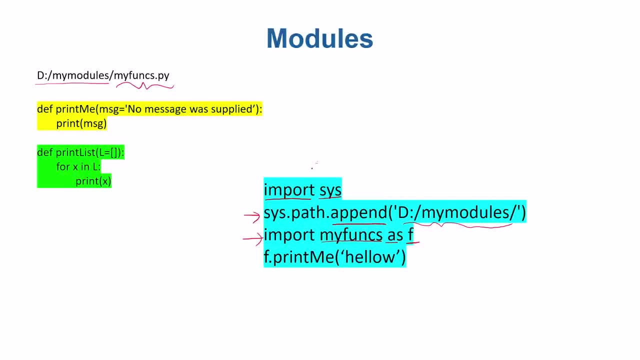 The implementation of these functions are not there in your coding file. You are just using those and you can now import this module into some other file and use there and so on For very large kind of projects. it is good to make modules. Actually it is better to make packages, which is actually the directory structures that 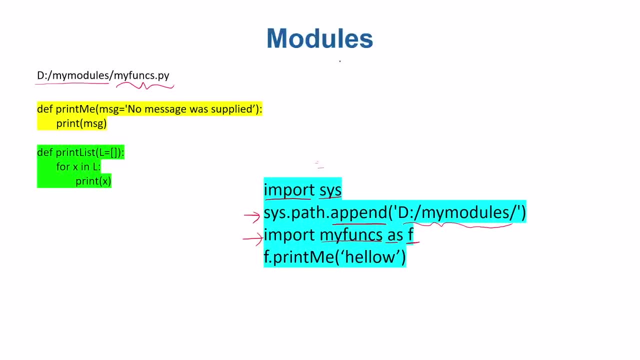 contain modules, But modules, at least, are really good for maintaining a large amount of codes, or actually the functions that you want to use again and again. So let's make a module, Why not? So let's make a module. Let's say: 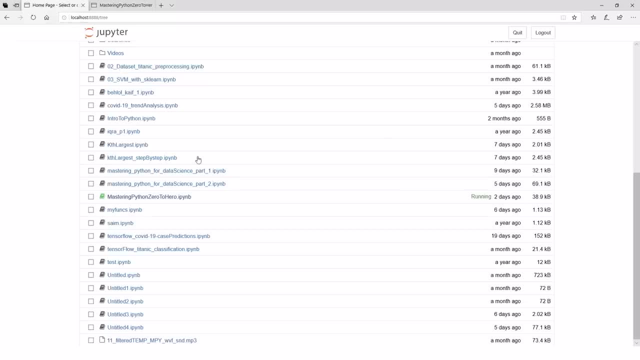 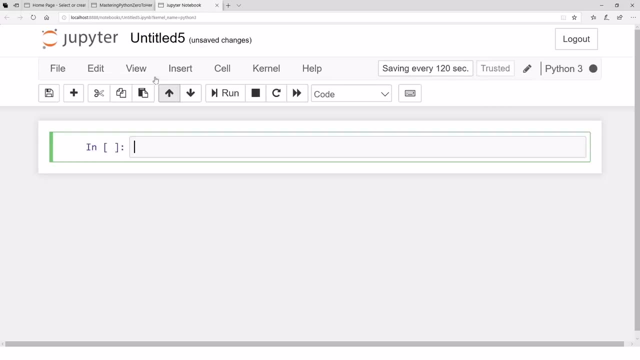 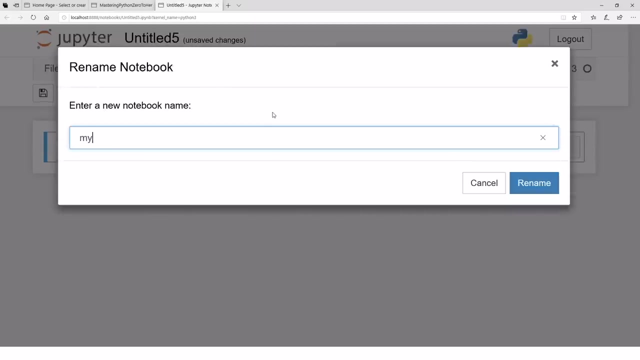 Let's create a Jupyter Notebook. Let's create another file. Let's create another file, Let's say new Python 3, and let's name this file as my. Let's name this file as my universal. Let's use underscores My universal functions. 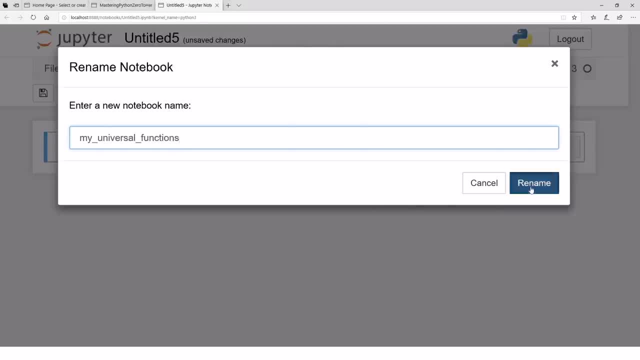 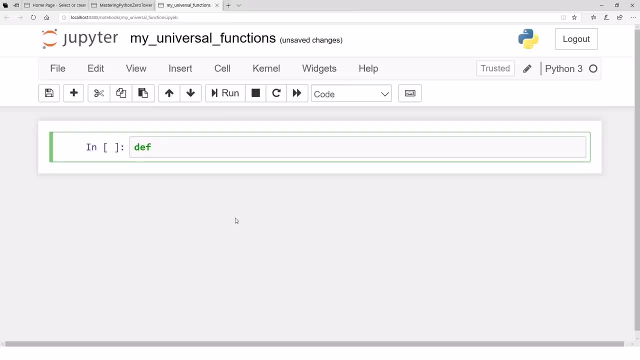 Okay, Let's say that's a file name. Let's create another notebook. Right now it's just a notebook. Let's define some functions. Let's say we want to define one function as check all args. Let's say that's the function. 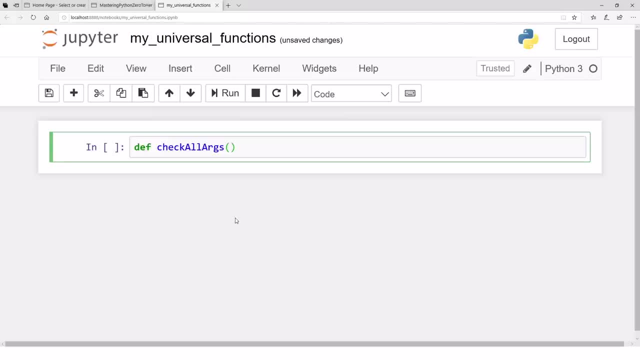 It receives. let's say, Let's say it receives a dictionary-like input And then it checks the type. Let's say: check, Check type of all args. And let's say: Let's say you write a function, check if not numeric. 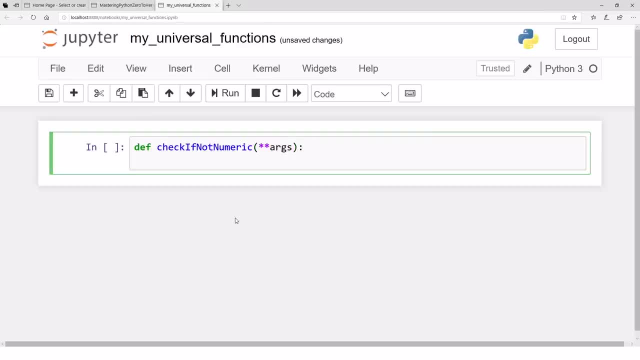 Let's say. Let's say you want to write a function that just accepts a lot of arguments and you want to check whether any one of them, If any one of them, is not numeric. you want to return, let's say, a flag. 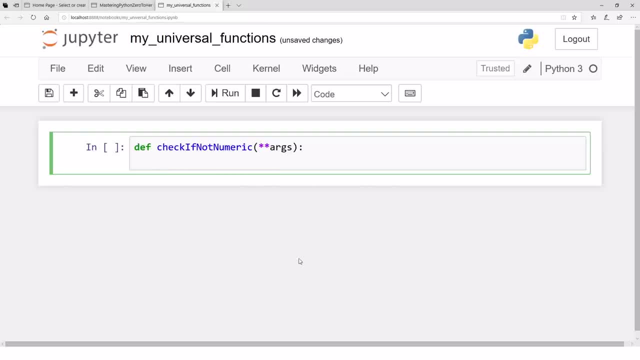 Otherwise you want to return a true, let's say So. for example, you may need this function in several places. Let's say, in your code you're expecting numerical inputs, And if the input is, And let's say there are a lot of variables that you are working on and if any one of 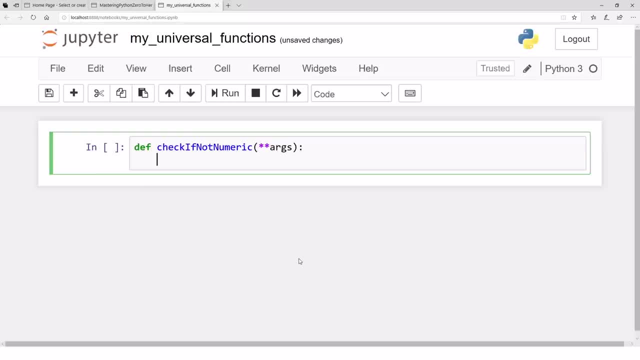 them is not numeric. you might want to check all the You check all the variables and their values. One way of doing that is just to create a list and that's it. I mean that's, And you may have several of those. 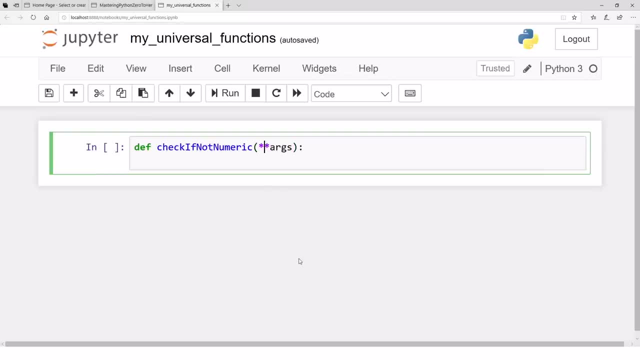 I mean you can check all of them, Maybe here, Maybe here. we do not need the dictionary kind of argument, So maybe we just are happy with just one. So let's say for. So the output, Let's say output is. 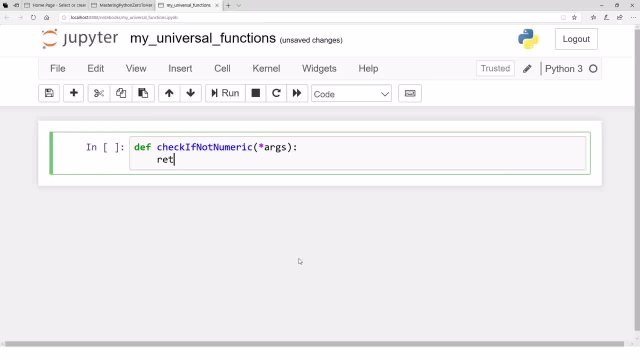 Is, let's say r, or the return value, rect value. Let's say that is already true And we will say okay for x in args. Let's say for x in args, If x, If is instance X is. 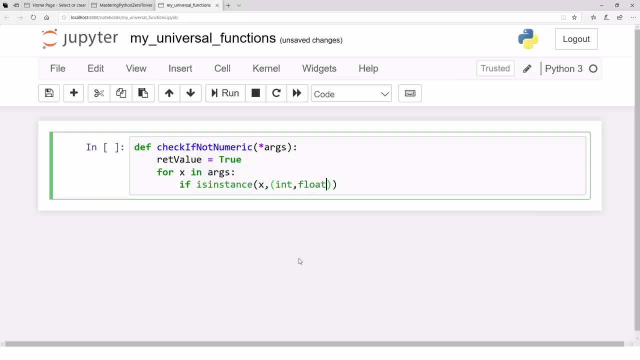 In Float. If that is true, then we are happy, But if that is not true, if that is not true, then there is a trouble. Then we say: okay, if this is not true for any value, then we just return false. 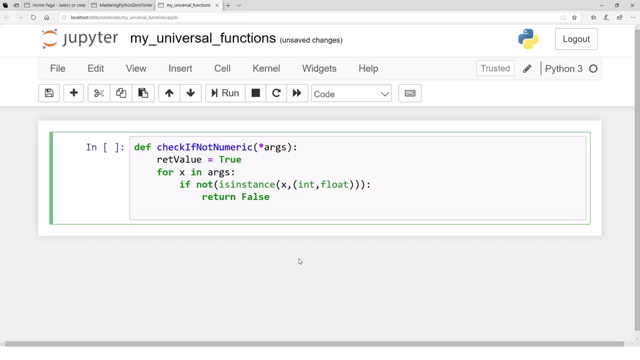 Okay, We just return false. I mean we need not to break anything, We just return false. Return means return whatever. Otherwise, If we Finish this loop, If the loop finishes successfully, there is no return statement. that is called already. 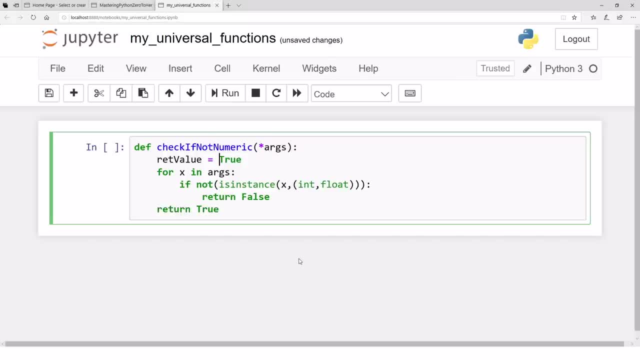 then we return maybe true. So we need- We do not need actually this variable. let's say So this function will return true if all the variables are either int or float. If any of them is not of this type, this function returns false. 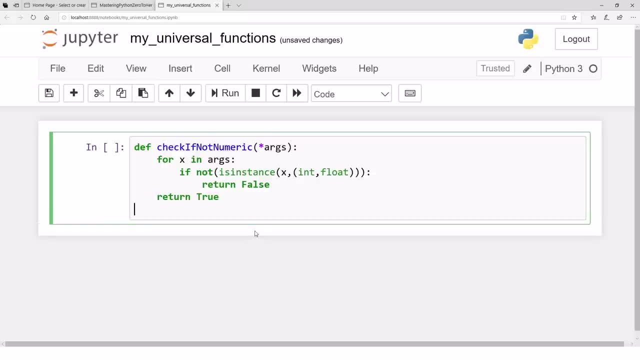 Wow, We can have another, We can have another function. maybe We can write. We can write several functions in the same cell or in different cells. either way, Define, let's say, another function, universal, or add all values. 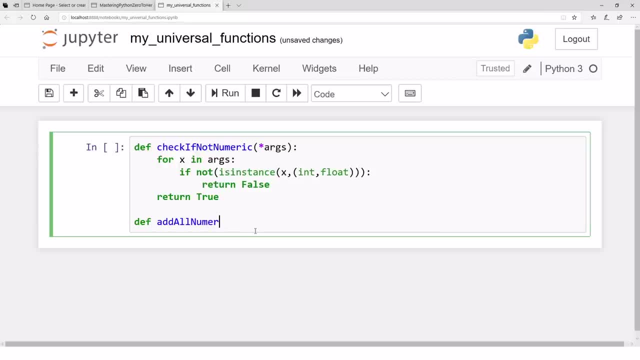 Let's say: add all, Let's say numerics, Add all numerics. And it also contains, let's say, args, And the goal of this function is just to add all the values in return, The sum. So let's say s, equals zero for x in. 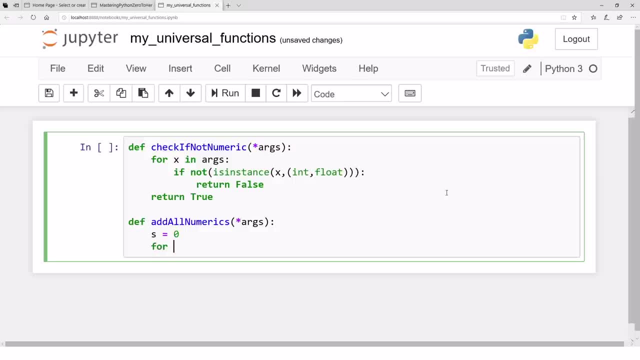 For x in args, S plus equals to x, And that's it. Then return s. Let's say these are two functions And maybe one more, The name of this Or some, Some variable. Let's say You, I mean these are two functions. 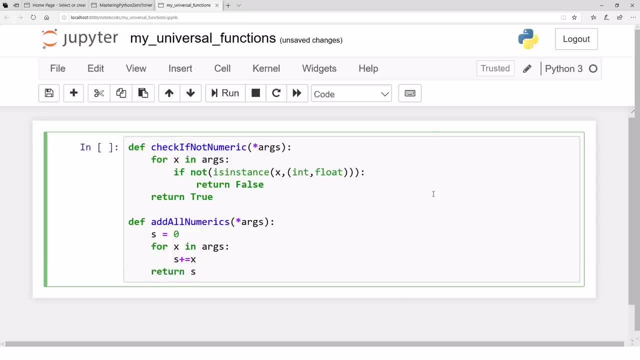 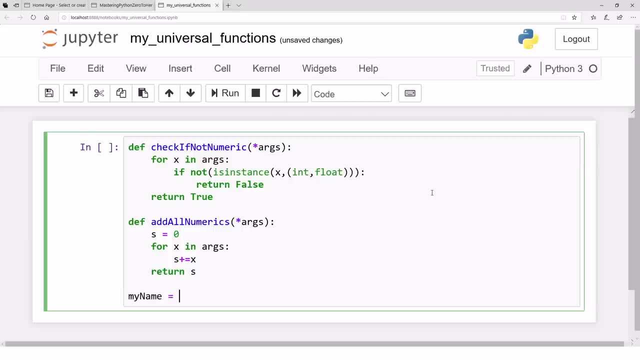 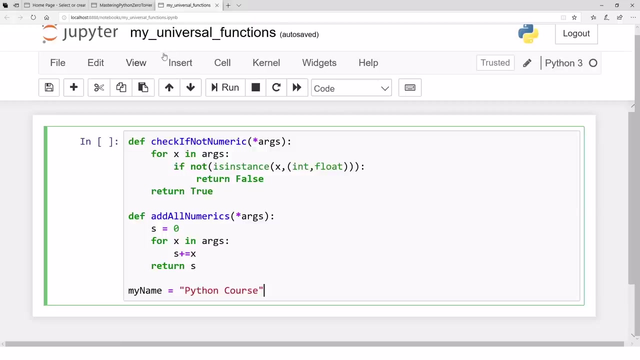 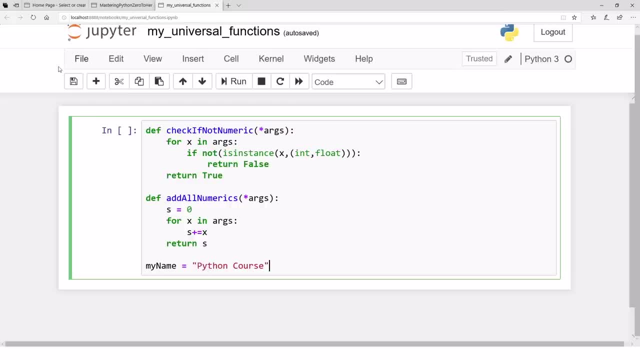 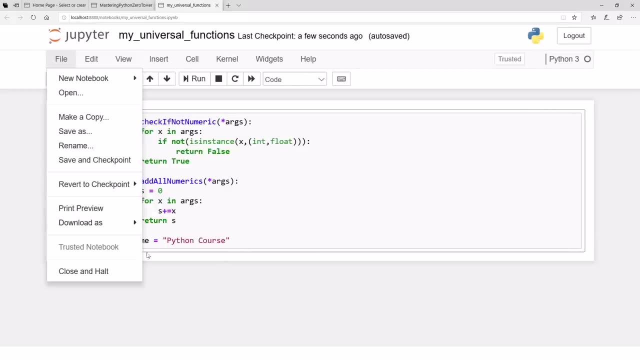 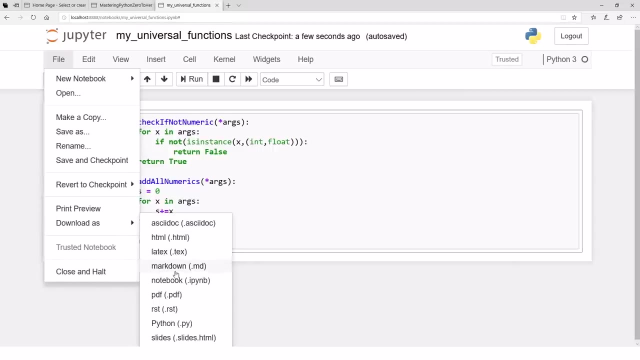 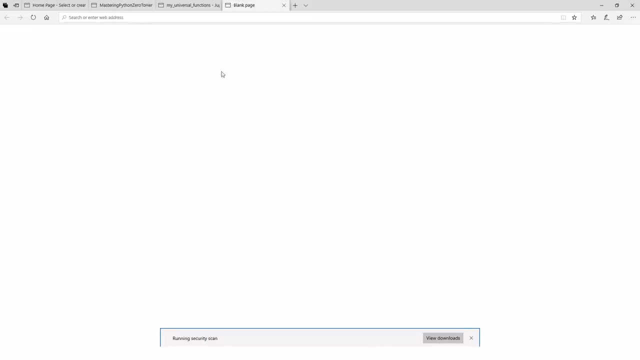 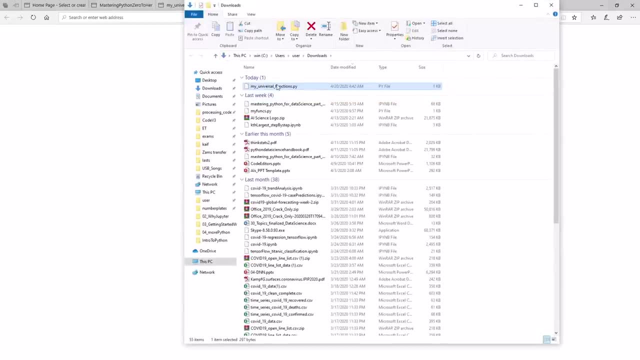 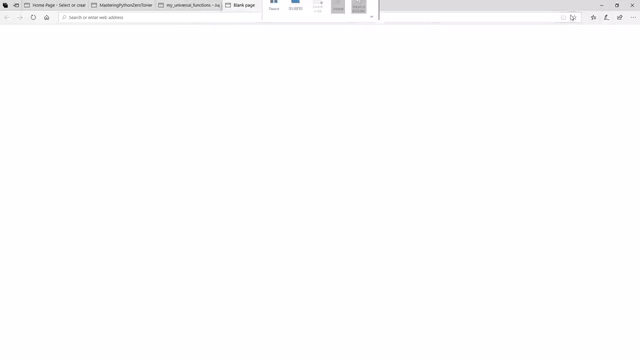 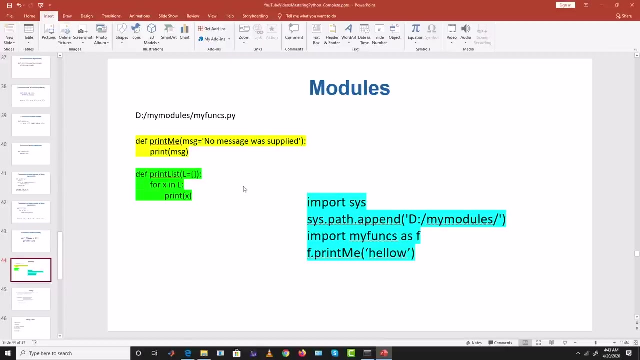 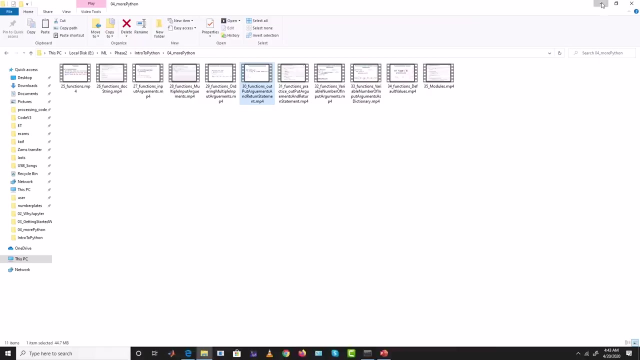 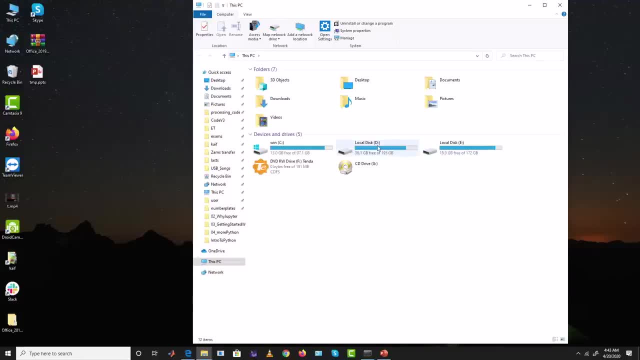 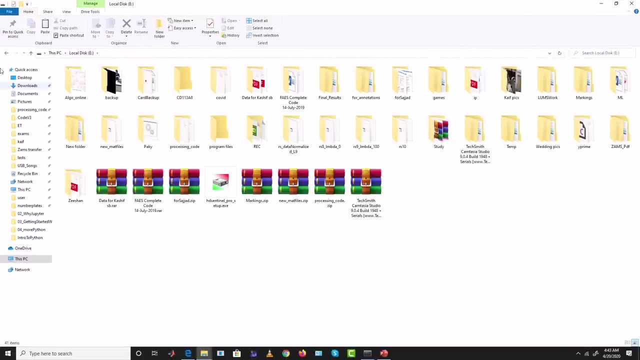 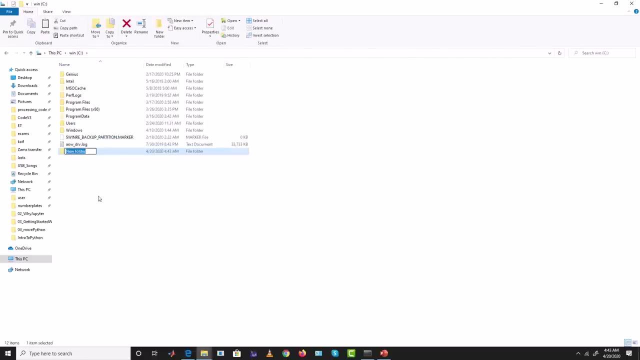 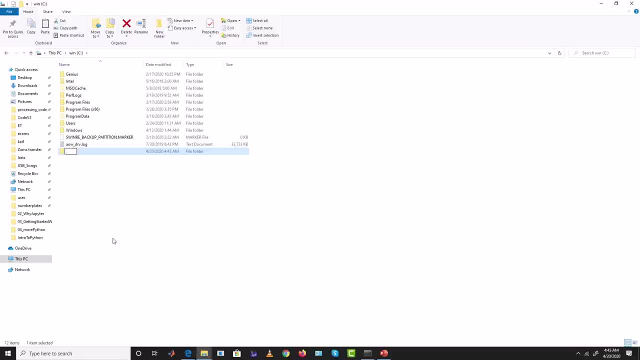 So, So, So, So, So, So, So, Whatever name I mean, let's call it as ABC, for example, ABC, whatever, And you just make that and just copy that Python file here: myuniversalfunctionspy. 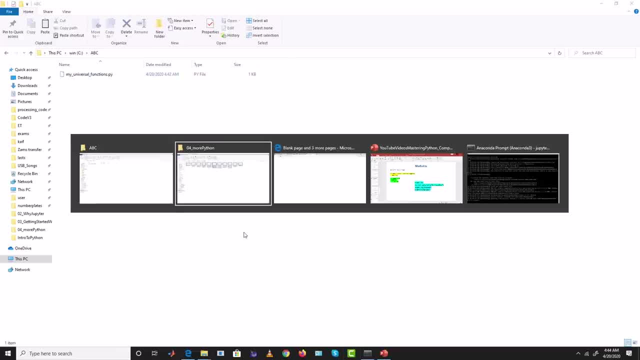 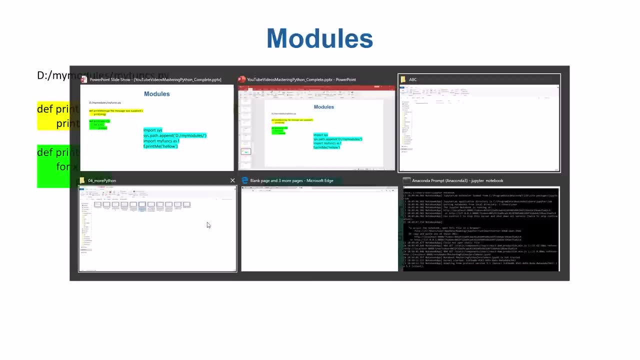 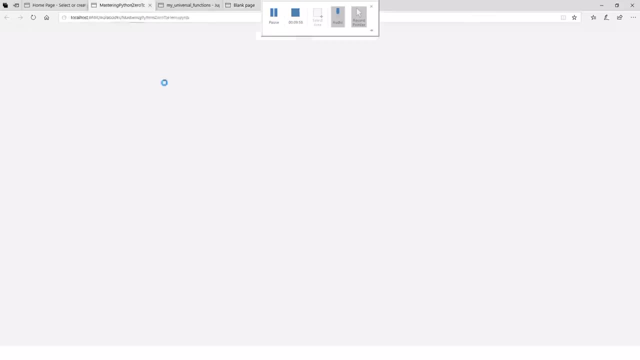 Now, if you go back, if you go back to your where? here is the Jupyter, here is the Jupyter. Now you go back to your code. This is your file. Go back to your code. Let's say this file is no longer here. 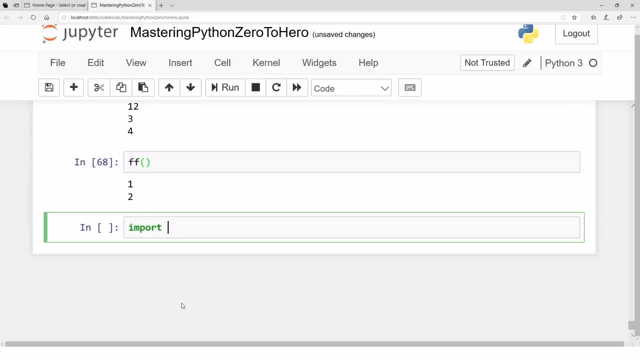 And what you do is you import sys, That's a system module. Then syspathappend Write the path here where the module is located. So the module right now is located at ABC. This is the path of the module. Once done, you can import. 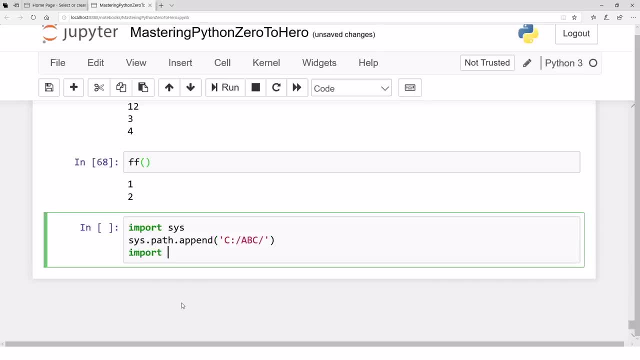 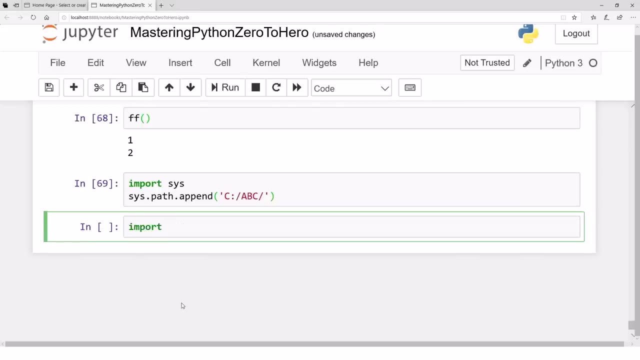 What was the name of the module? You need to know that That was my, my what. So I just, I just don't remember the name. Let's import my universal functions how it appears. Actually, when I, when I have added this path, then this import command, and after the tab completion, just fetches that file. 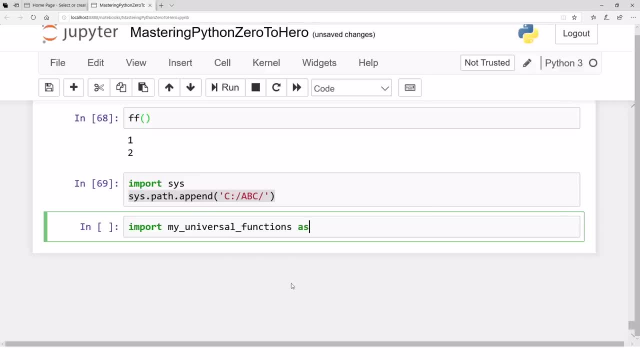 So that that that name might be very lengthy. so you can rename that as, let's say, my apps or or whatever Name you want. So you import that. Once you have imported that, now you can use the functions if you want. 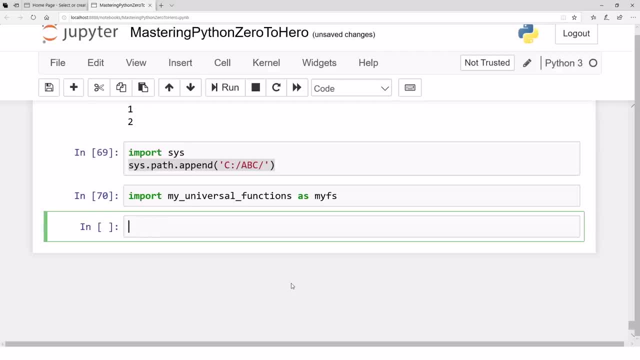 For example, you can check the uh implementation of my apps dot. if you see dot add numerics, you want to check the implementation of that uh here. This, remember: this file is no longer in this particular file. This is located somewhere else. 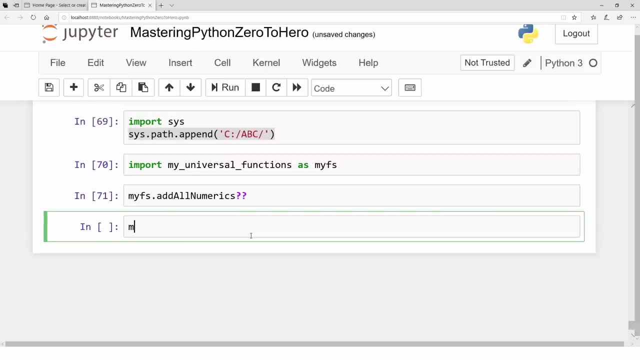 Um, and you can call this function like, uh, like the built-in functions, my apps dot add All numerics um, and you can have, for example, uh, let's say accepts the input arguments. let's say two, three, four, let's say six and um, that's it. 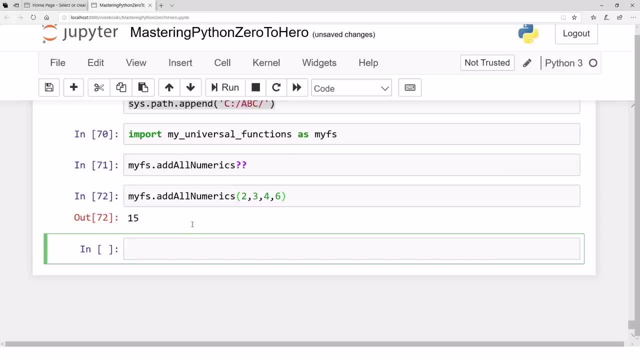 That's the, that's the return value. Uh, you can. you can save the return value in some other way, but let's just see, And then later on you can print this C? uh or do some stuff with this, uh. 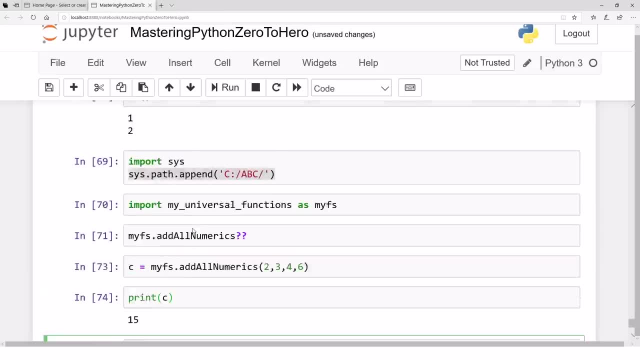 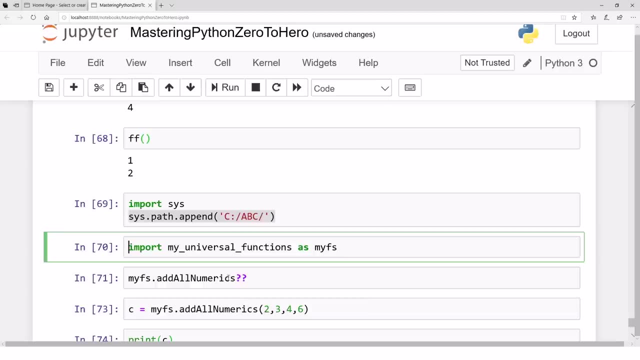 So C? that's one thing. Another way of importing the same thing is: let's say you don't want to use all the functions, You just need this. add all numerics. Let's say that's, that's the only function that you want to use again and again. 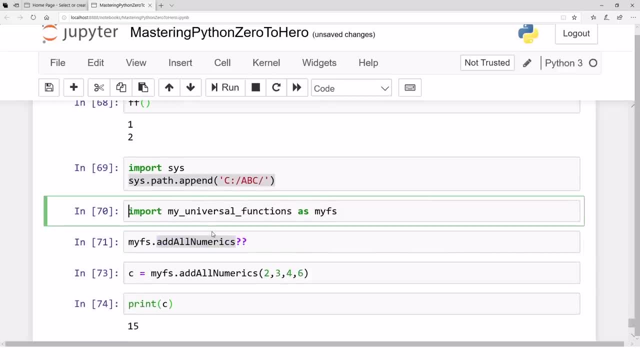 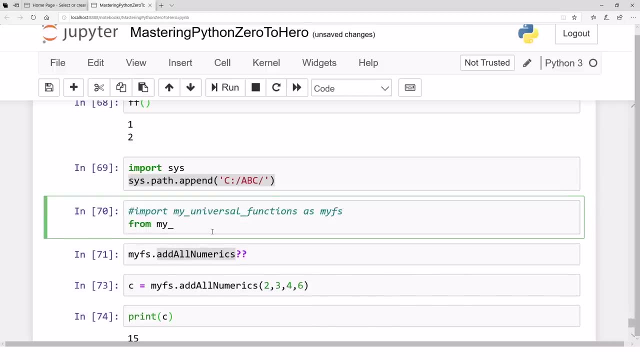 So you need not the other functions. Let's say, for this particular file you do not need the other functions. Then what you can do is you can just say, okay, from my universal functions, import, Uh, add all numerics and you can really rename this function as something and you can call that function the same way. 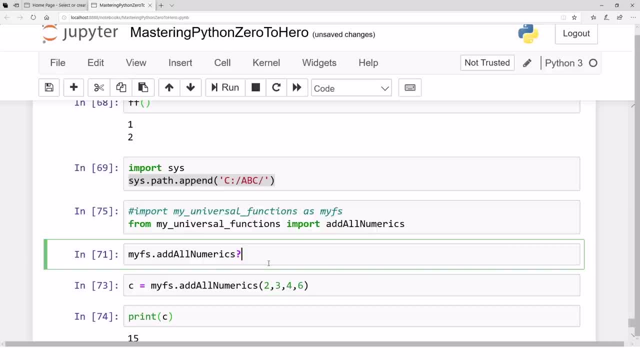 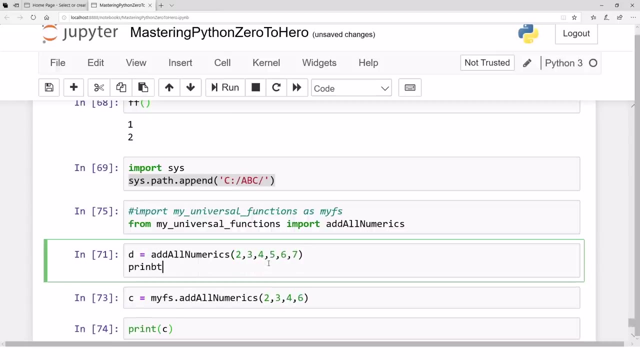 So you do that Now you need not to write any dot kind of thing, You just call: add all numerics because it is imported now, and you say, okay, two, three, four, five, six, seven, and you save that in- let's say D, and then you print D if you want or do whatever. 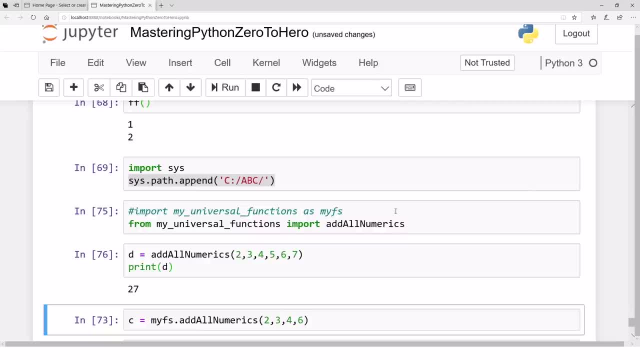 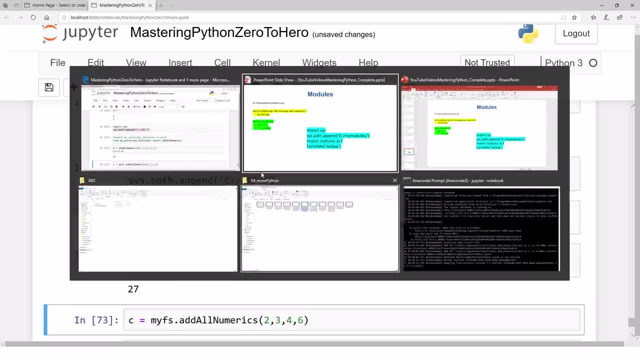 Okay With that. that's it. or you can import several- I mean multiple- functions, or you can import all of them. um other than modules, there are, uh, I mean for complex codes. I mean this is not one module that is there. 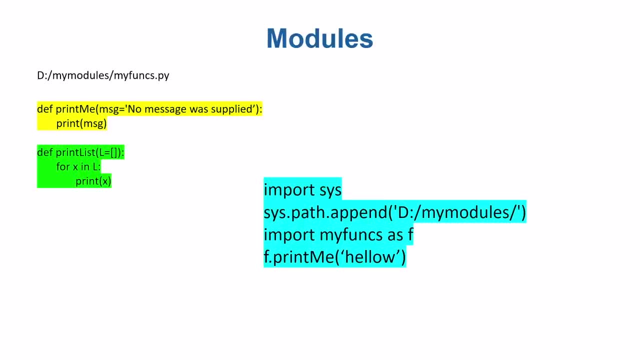 I mean, there are several modules, uh, and the several modules may be arranged in in a directory structure where the directory and the subdirectory and the subdirectory and so on. So the modules that are arranged in directory structure, although they are excellent, 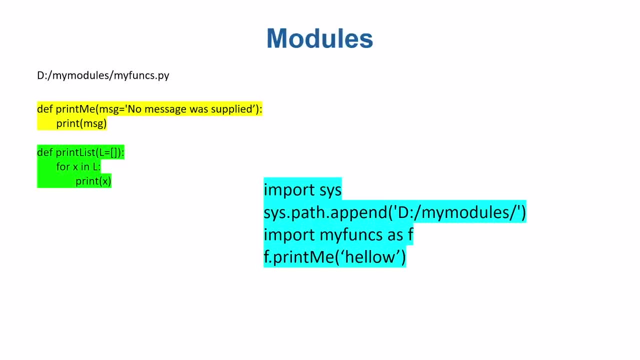 They are accessed much like the same way. uh, that directory structure is sometimes called package and these are basically the packages that are that are most useful. and uh, we will be seeing some data science packages. uh, like NumPy is a data science package, um then, uh, we will be seeing Pandas- uh, that's a data science package. we will be seeing, uh, Matplotlib- that's a data science package for plotting, and uh, visualizations and stuff. 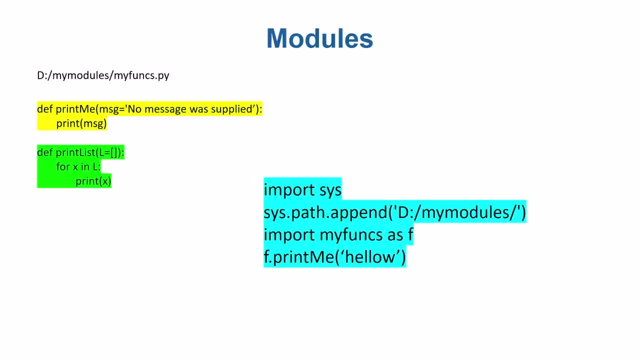 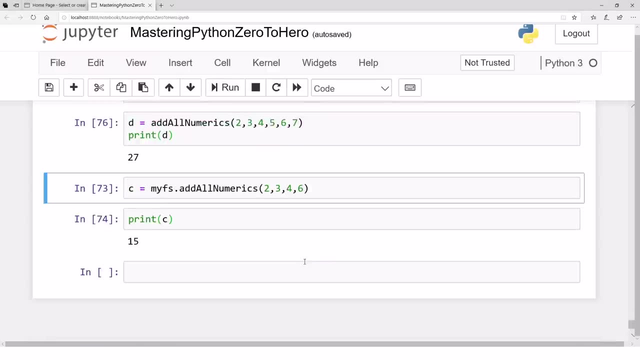 So package is just the module, So the modules that are arranged in directory structures, um, so now you know what module is and uh, the oh we. we missed to. we actually missed to. uh import the name. uh, to see the name. we, we have saved a name there as well. 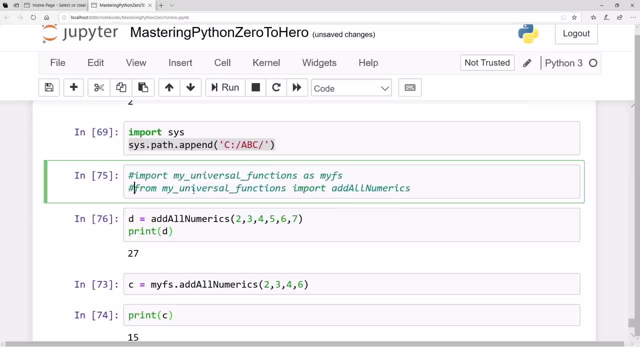 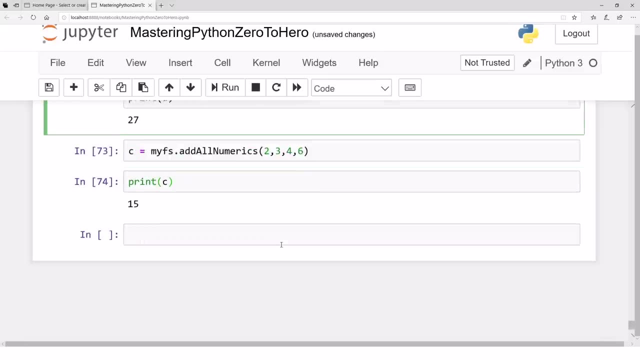 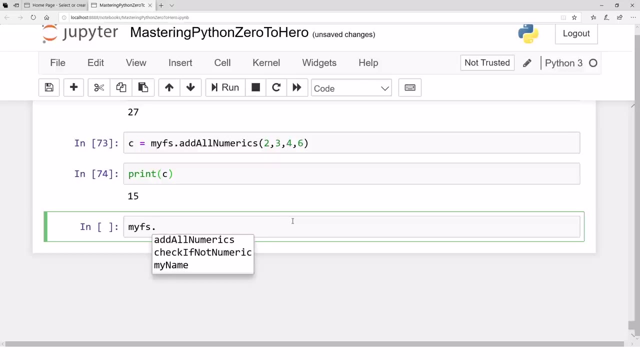 So let's go back, and let's go back and do that and see how how many things are available. Uh, let's go to some other cell, an empty cell. So myfsdata: I have completion, My name is available. 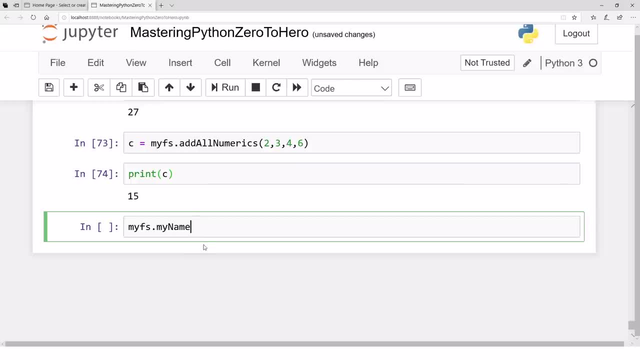 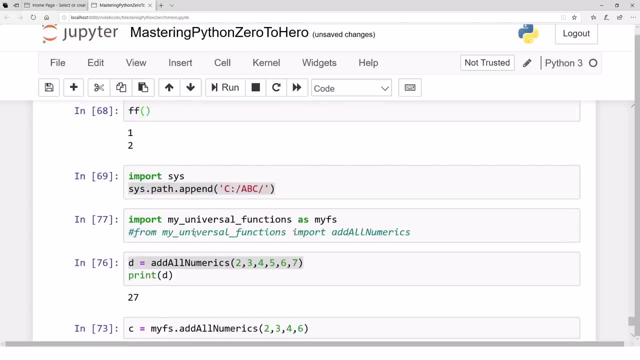 Uh, remember that was a variable. Yeah, that's available. So the name is Python course. So this module file does not require to only contain functions. It can contain any information, any data that you want to use in other files, other coding. 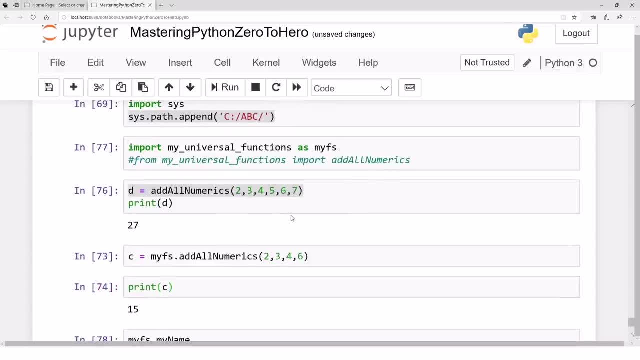 and stuff and so on. So, um, yeah, that's about modules In the. in the next video we will practice about these functions a little bit. Um, We will be seeing how to call a function inside another function, how to make a lot of functions. 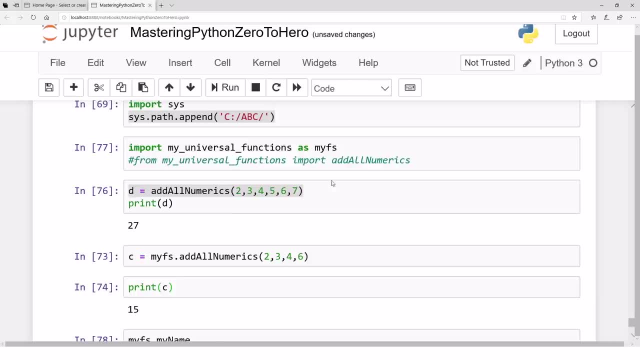 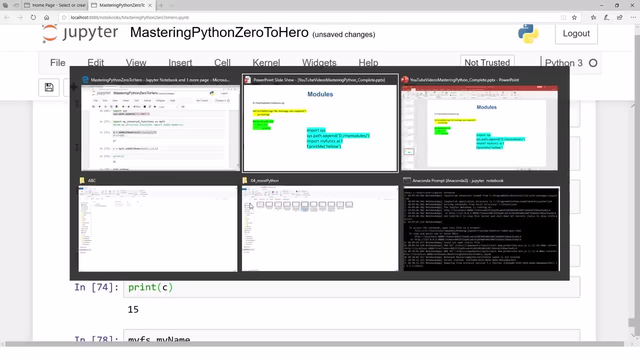 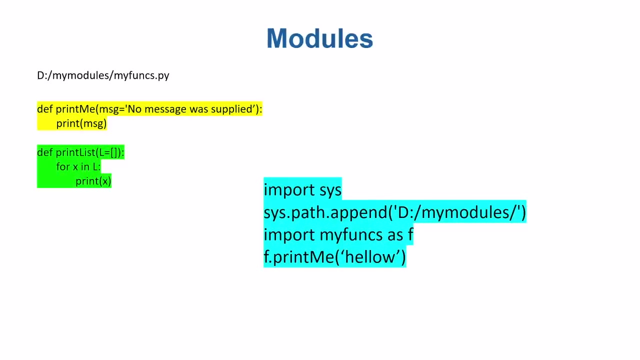 that are calling each other and so on. So we will be practicing more um on uh about these functions, not theoretically, just in Jupyter Notebook, just to get a better look and feel of um of functions more. And after that practice we will be then jumping towards data structures, starting from strings. 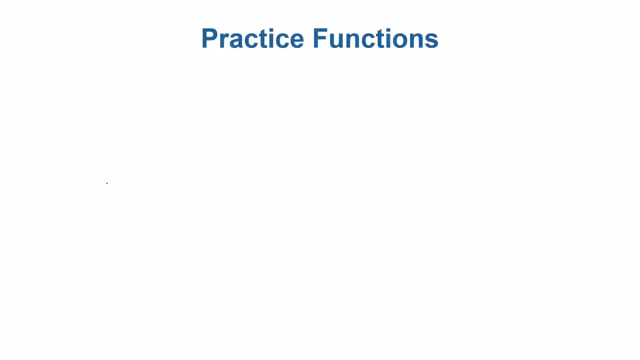 So hope to see you in the next video. Okay, Uh. So let's just practice some, uh, some, some. I mean let's let's get a good grip on functions and multiple functions and handling those, And the best way to do that is to solve actually a problem. 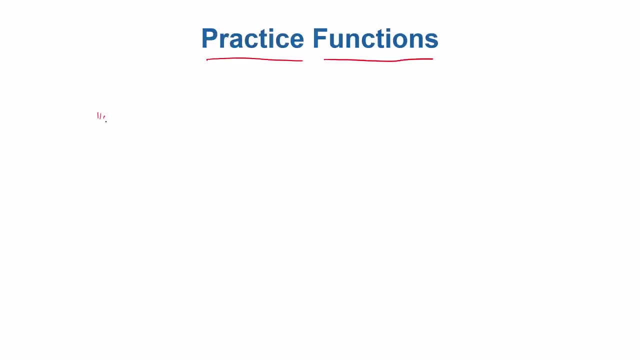 Remember, we solved a problem when we uh, when we uh, when we are done, when we were done with if conditions. then we solved another problem when we were done with loops. just to get a good grip on loops. Uh, let's solve a problem. 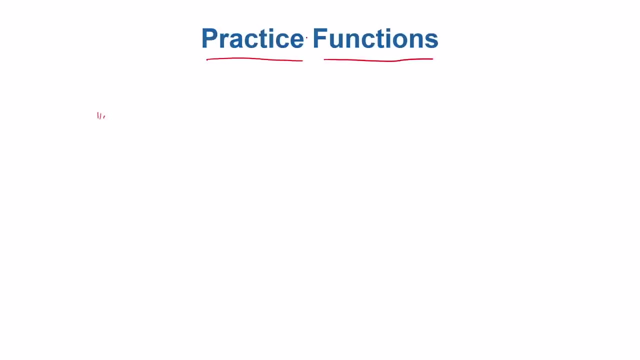 Uh, uh, let's just solve a problem using using Jupyter Notebook, Using using the functions, just to get a good idea of functions. Um, what kind of problems should we solve here? Um, should we solve an older problem? 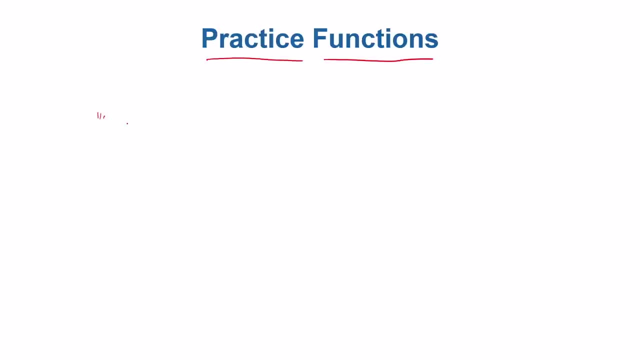 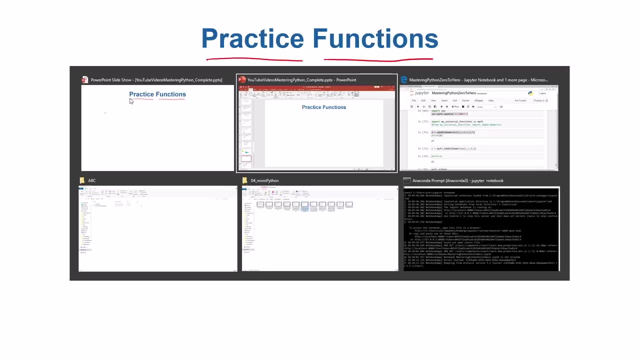 Uh, last time we solved a problem using loops that were sorting a list. Why, why don't we? why don't we solve the same problem? uh, but in a different way. So let's go to Jupyter and see um. see our file: Jupyter file. 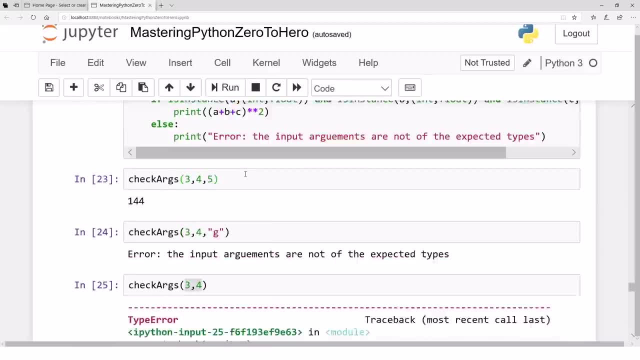 We have actually solved a function somewhere using loops. So let's go to Jupyter and see, um, see our file, Jupyter file. We have actually solved a function somewhere using loops. Okay, Let's just let. let me just find that out. 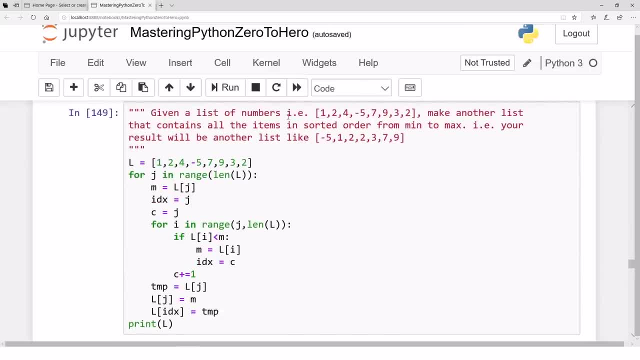 Oh yeah, they're here, So here. So, given a list of numbers that's this, Make another list, or maybe the same list that contains all the items in the sorted order from minimum to maximum. your result will be another list like this: 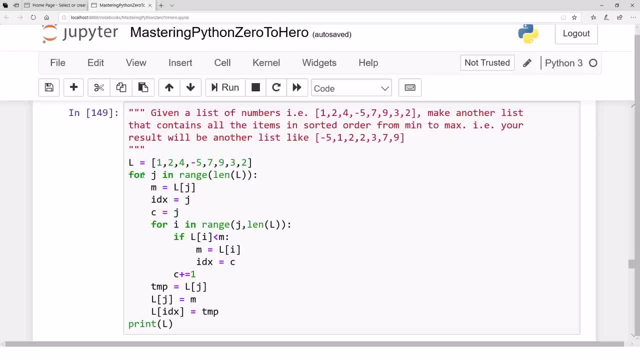 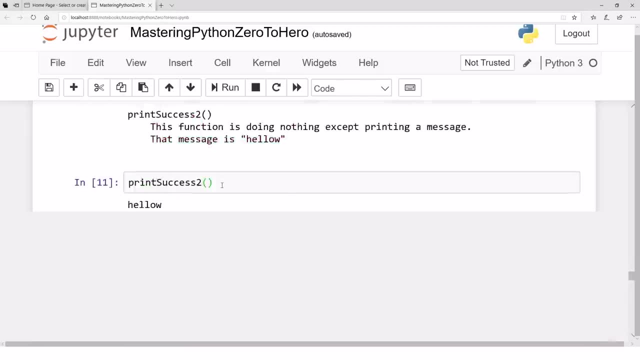 And we solved that using loops. Um, okay, Let's solve the same problem. um, exactly the same problems. Let's solve the same problem using a different way, Using a different, uh, using using functions just to get a grip on functions. 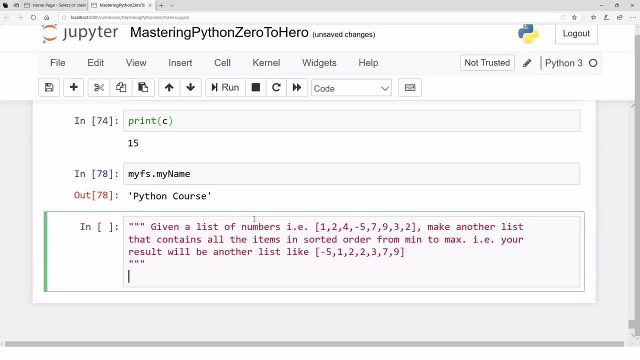 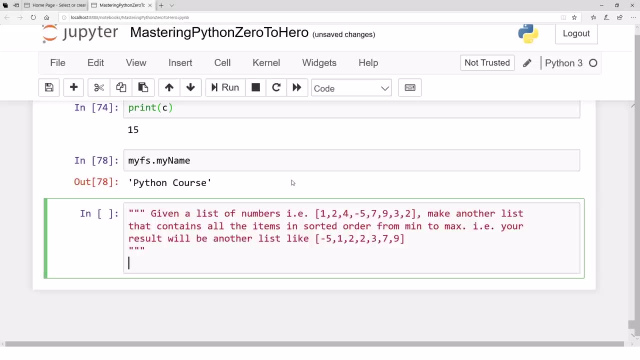 So let's say: that's our problem, we want to solve, So that's the problem again, and we want to solve that. So how can we solve that? Um, to solve that, let's first define a function. uh, let's just uh, make a function, um, um. 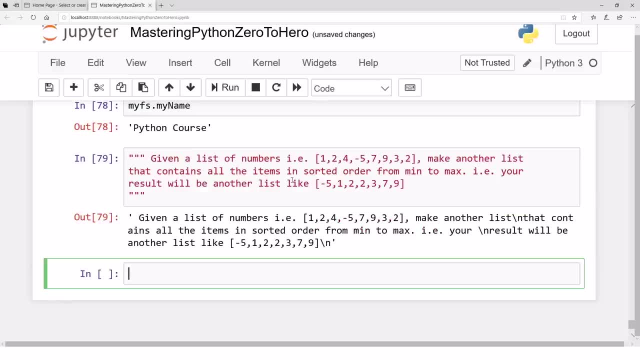 let's just make a function that um, um. let's just make a function. let's say, define, find minimum, And the function accepts a list and returns the minimum value in the list, Not only the minimum value of the list, but also the position of that minimum value. 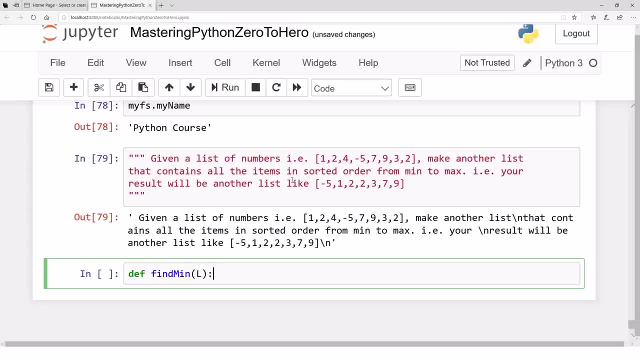 So find minimum as well as find, uh, so minimum as well as the position of the minimum in the list. So how can we, how can we solve that problem? Uh, that that's. that's one standalone function. No matter what list you pass in, it will find the minimum. 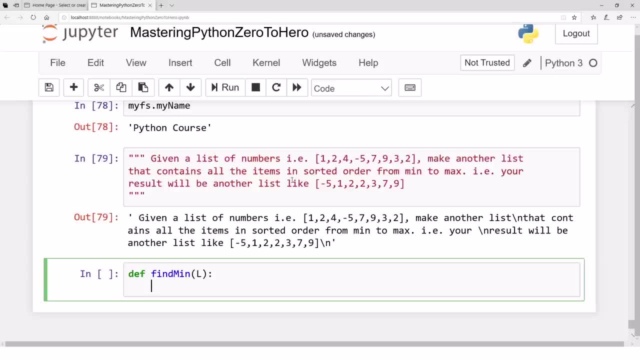 Okay, So let's uh, the minimum is defined for the items of the list. For example, the list items are, let's say, all numerics. Um, okay, How can we? how can we do that? Let's say: minimum value is the list zero. 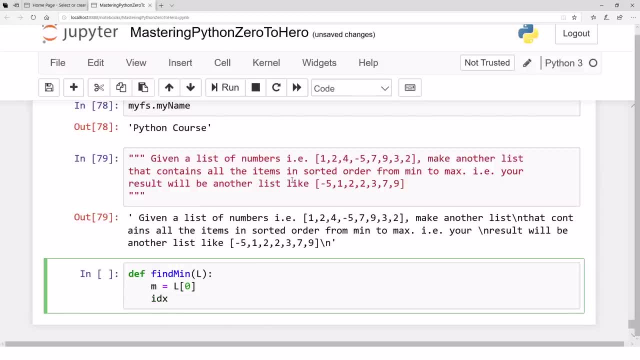 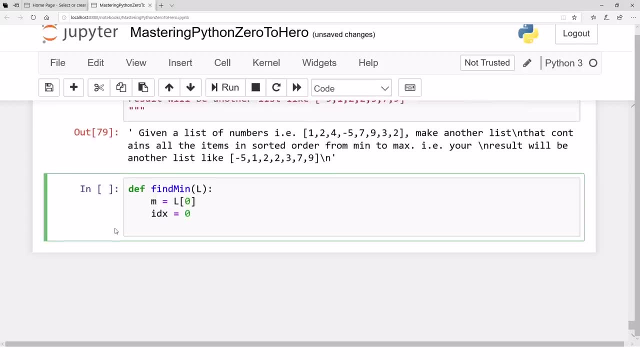 That's, let's say, the minimum value, And right now the index at the minimum value is, let's say, um is zero. Okay, Uh, like we did in the loops. like it is, it is kind of the same code, but uh, let. 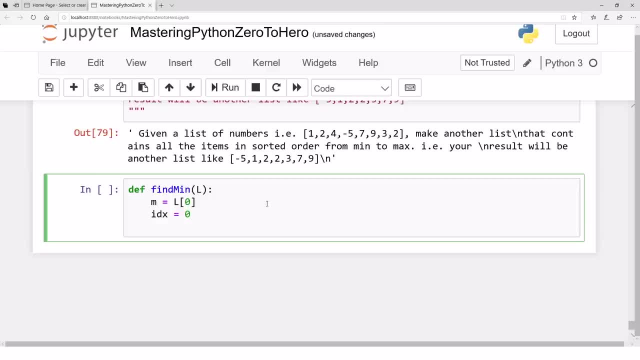 let's try to function for it. Okay, So that's a function, Find min. So, uh, how can we, how can we proceed? What should we write here? Uh, let's see a counter. Let's say: um, uh, counter is. let's say: or I maybe let's say the counter right now. 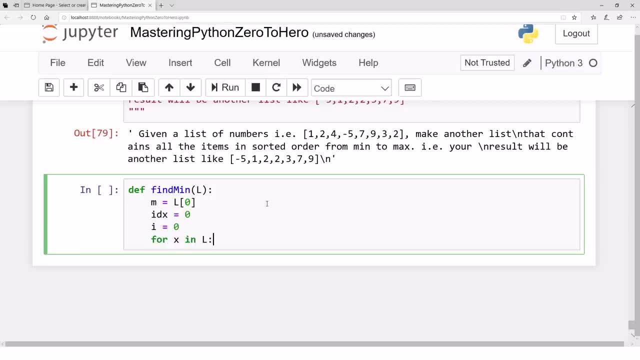 is zero for X in L If X is smaller than our minimum value. if that's true, then the minimum value Indeed is X, and the index where we found that is: I Okay, great, Else do nothing, I mean, else just go away- and I plus equals one. 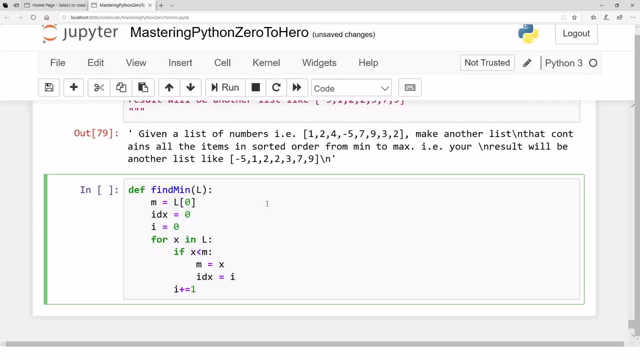 So move on. So I is just the position. So I is moving on and on and on as you follow the list. and M contains the minimum value and ID X variable contains the position of the minimum value. So that's the function. So for for readability, we might be adding an else clause, just to write boss, and that. 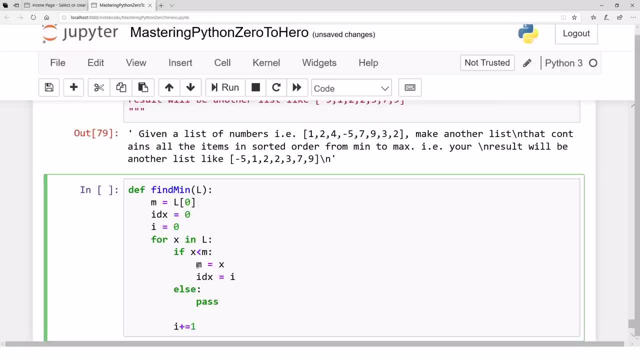 means the if condition finishes. I mean: do if this condition holds true, do that stuff, Otherwise do nothing. Uh, that's just because of readability. If you want, even if you don't write the else clause and pause statement, even then everything. 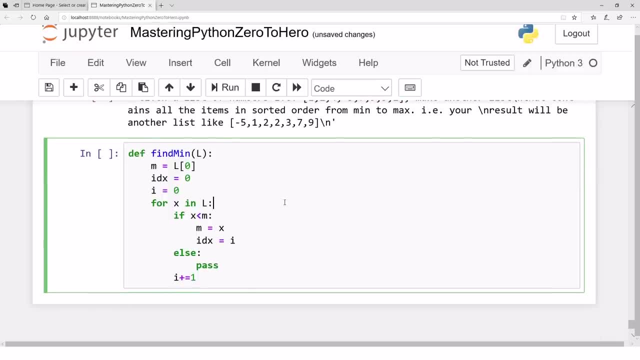 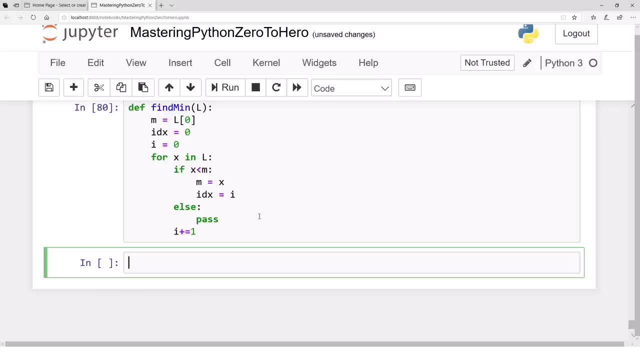 is fine. So let's call this function, just to test whether this function is working properly or not. So let's just find: um, Oh, Okay, We haven't returned anything. Uh, we need. we need the minimum value as well as the index. 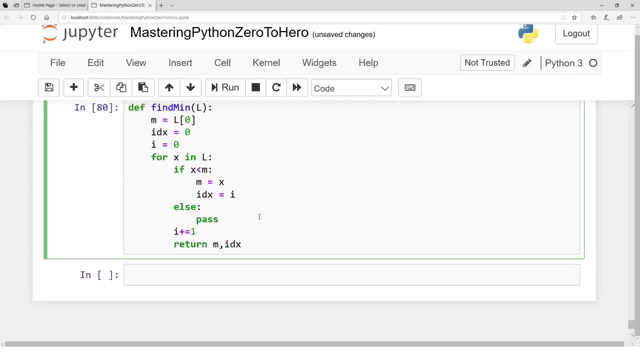 So return minimum value as well as the position. So return that. Okay, Oh, but we we are returning that inside the loop that becomes in the body of the loop. Oh, no, no, no, no, no, That's bad, because even in the first iteration the return will be called. 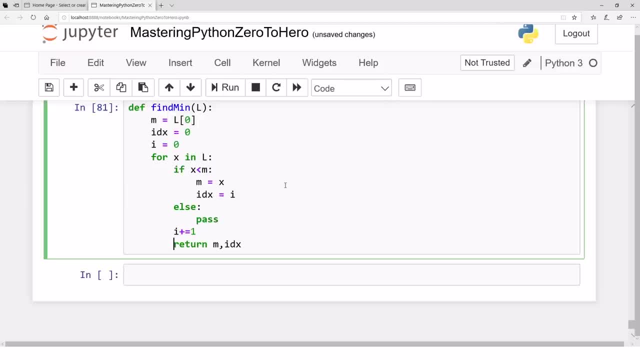 And even in the first iteration, the function will finish indentation. Remember indentation. Now, that's better. Now this is no longer inside the body of the loop. Great, That was a bug, We fixed it. Great, Okay. So let's go find. let's receive a b. 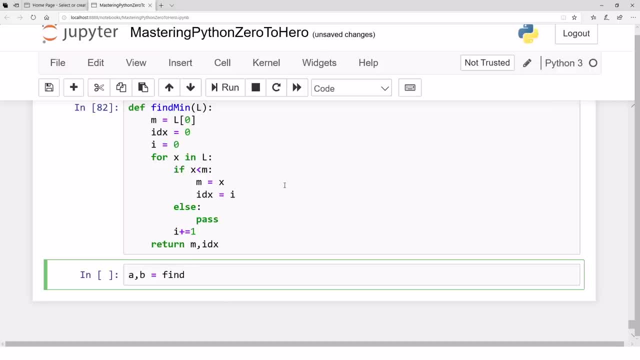 So a will contain the minimum value and b will contain the index of the minimum value. So find min, for example, and the list, let's, let's give it the list: 1, 3, 4,. uh, 2, 3,. 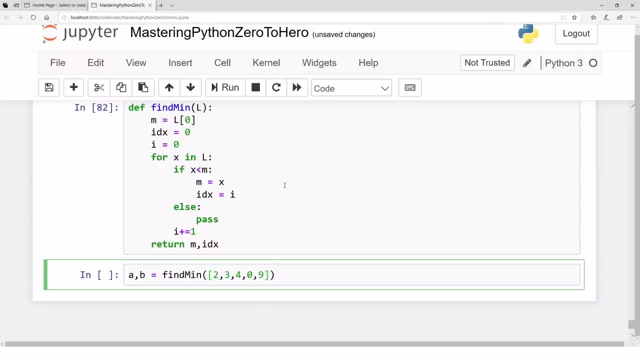 4, um 0, 9.. Let's see: Uh, now the minimum value is 0 and that minimum value appears at 0,, 1,, 2,, 3.. That's the third index. So b should be 3,, a should be 0.. 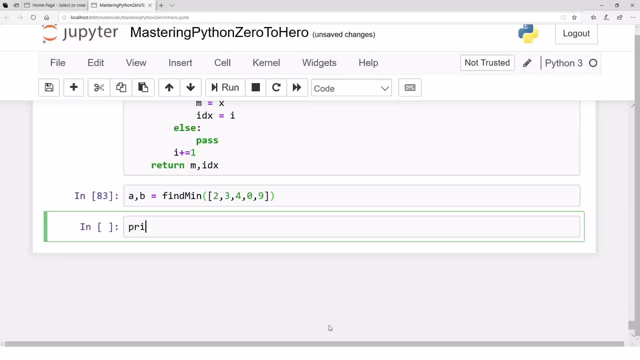 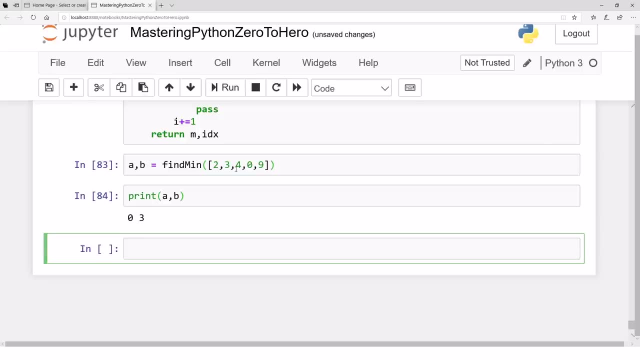 So let's see what's the value, what's the result. So print ab. So a is 0,, yes, and the position of minimum is 3.. I guess it is working fine. Great, So that's one function. Uh, find minimum. 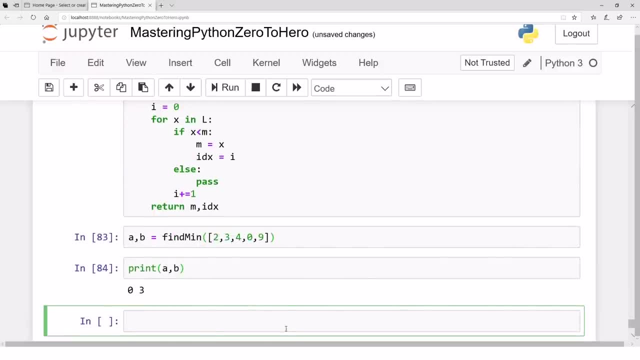 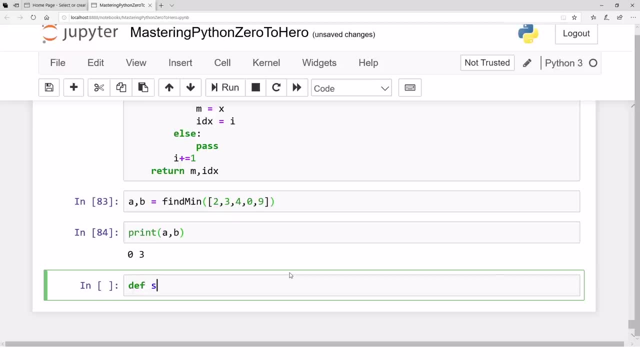 Let's find another. let let's write another function: uh swap. So define. define another function, Let's say swap values. And what we do, is it it? it actually uh accepts two indices: index 1.. 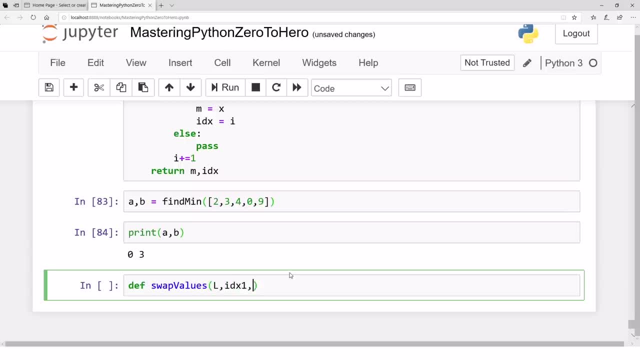 It actually accepts a list, then two indices: index 1 and index 2.. And what it does is it actually swaps the values. So index 1 values should go to index 2 position and index 2 values should go to index 1 position. 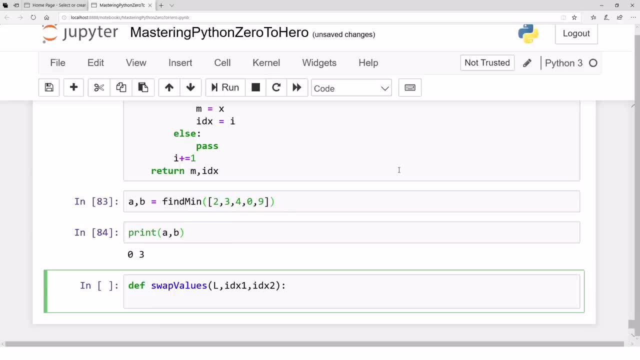 in the same list And then it returns the list. Okay, great, So it it so. so that's a. that's a good example. It re: it accepts a list- uh type variable. It accepts uh index type variable, which are integers. 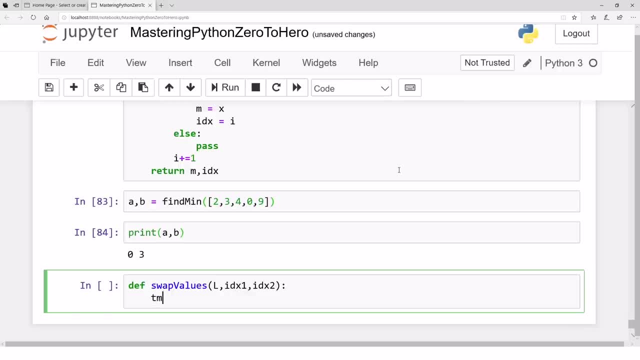 Great. So let's contain. let's define a variable temp that contains l. Okay, So id x, index 1, just store it in a temporary variable. Then, uh at this particular index, index 1, just copy this value. 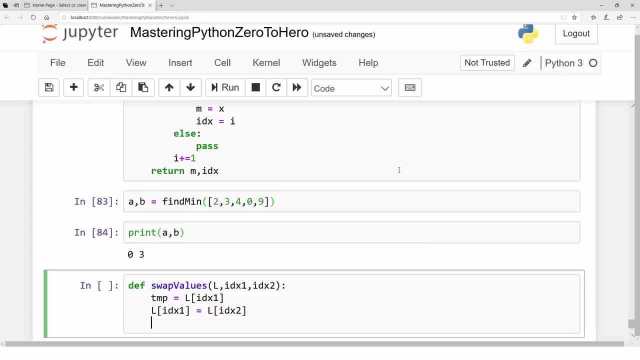 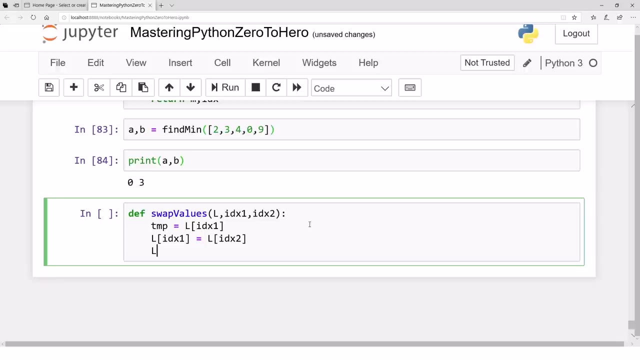 Don't worry, we'll see lists in detail later on. Now list now at index 1, the value of index 2 is copied, But uh, it is not overwritten because we already have saved the value somewhere before that copying appears. So l at idx2 is simply temp and now return the list. So that's how you. 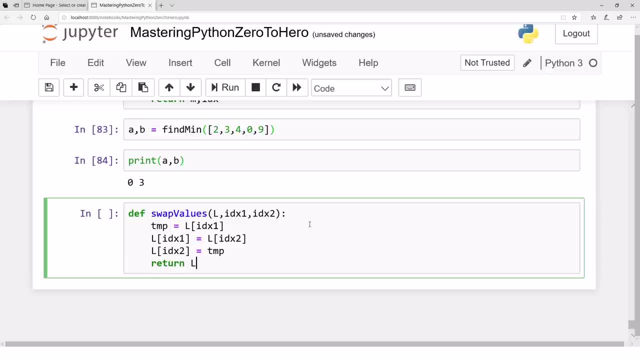 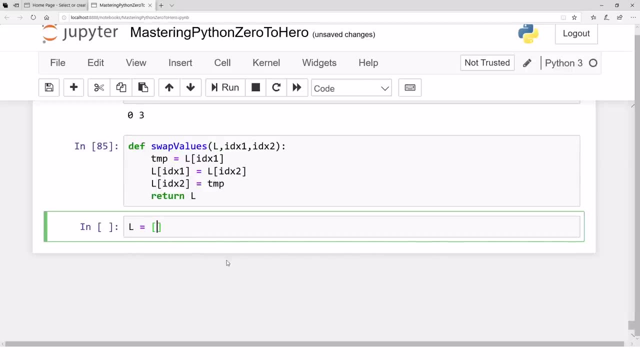 can swap the two values if you want, Great. So let's just check it whether the two values are swapped or not. So let's say list is 2, 3,, 6 and 7.. Let's say that's list, and let's 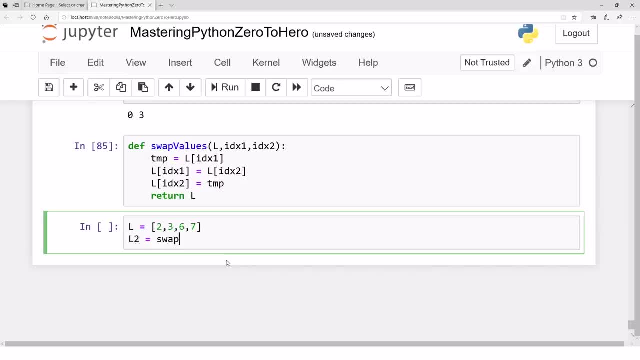 say we want l2.. That is swap values. and let's say we pass the list and we want the values to be swapped at position 1 and position 3.. At position 1, the value is 3 because the position starts from 0, and at the 3rd position the value is 7.. So we want these to swap. 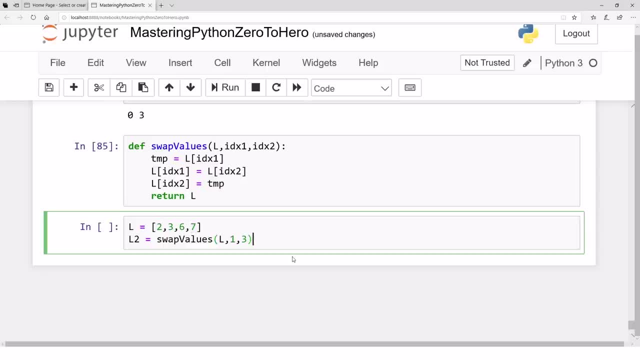 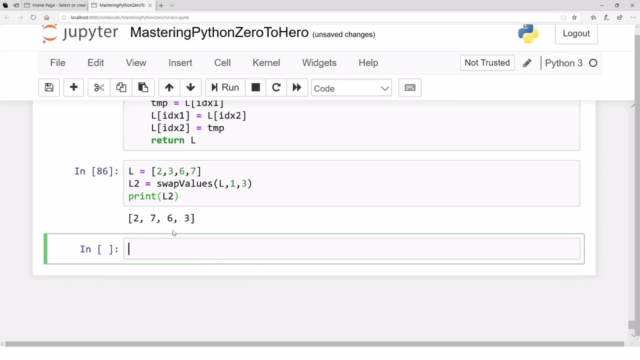 So the result will be 2,, 7,, 6 and 3.. Let's see what's the result. So let's print l2 and, yeah, it works great. what else? what else do we need? uh, so we have find minimum function. we. 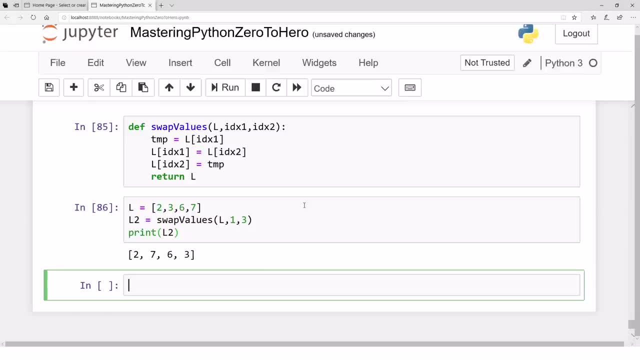 have swap values function. what else? so, um, yeah, what should we do now? let's write the main function, sorting. let's write that function and we will call. we will use these kind of functions inside that function. we will call these functions. so let's define um sort list. let's say that's our 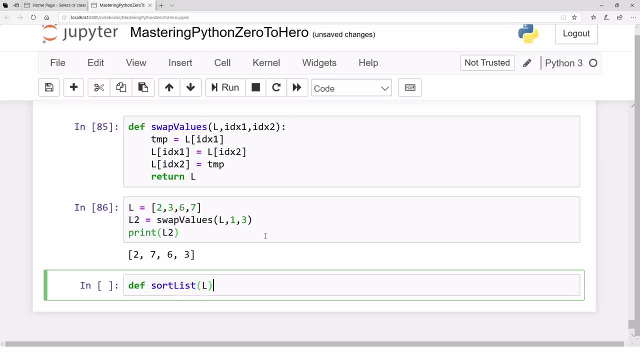 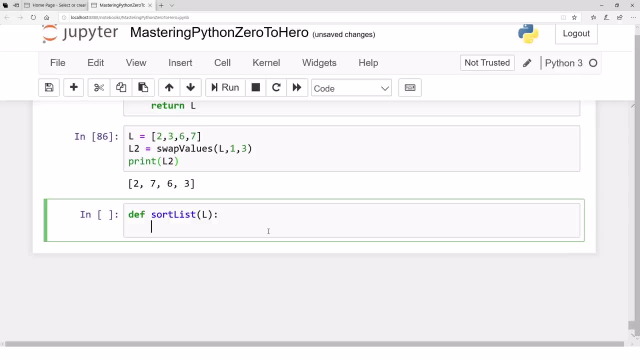 function. it accepts a list and it returns a sorted list. okay, what should we do? what do you think? what should we do for the very first time? well, first of all, we should check whether all these list it contains the list contains all the numeric values or not. let's 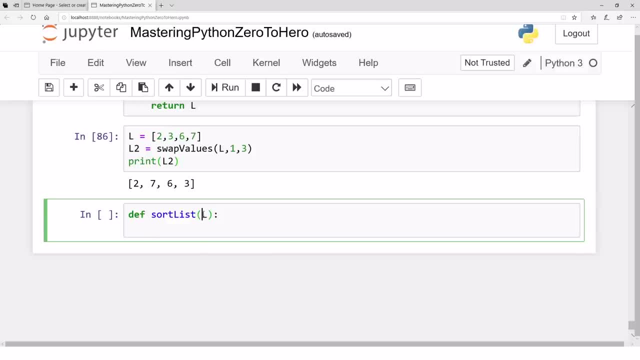 say, we are just doing this for numeric values, so we should first check that all the arguments are are of numeric type or not. for that we should write a function that should do that. oh, remember, that function is all written in in a module. remember that module. we made that module ourselves. 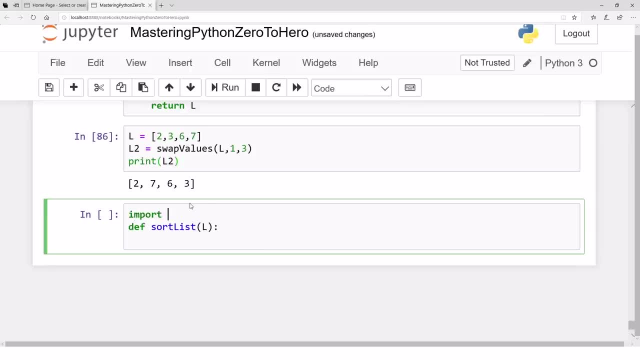 so we can import that module. if we want import, um, my, remember that my universal functions and we just need that function, just need that function. wow, just from from my universal functions: import what import? uh, check if numerics, check if not numeric, as so you can write that function name something else. but 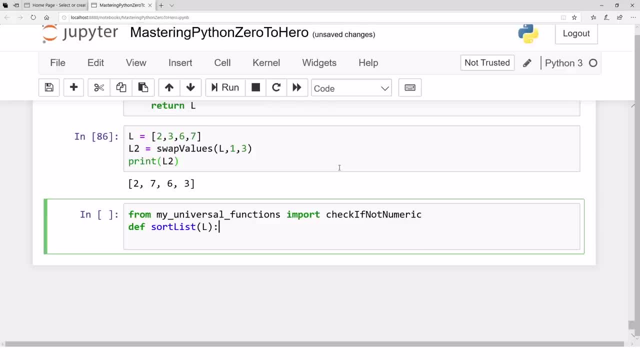 just this. so you import that function now you may be able to use that function. so after that you can use that function if check, if not, numeric list. remember that function returns true if all the values are numeric. otherwise it returns false. so if it is true, then move on. if it is not true, if it is not true, what should you do? if it is not? 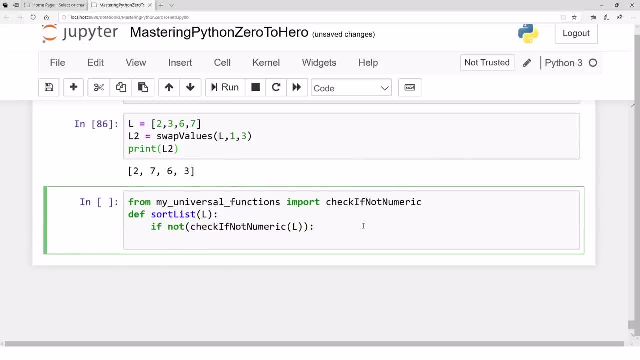 true. if it is not true, then Then you might be printing an error- error list does not contain numeric values, maybe that- and then you just return, return. that's it. I mean return, Don't need to write anything in return. fine, great. 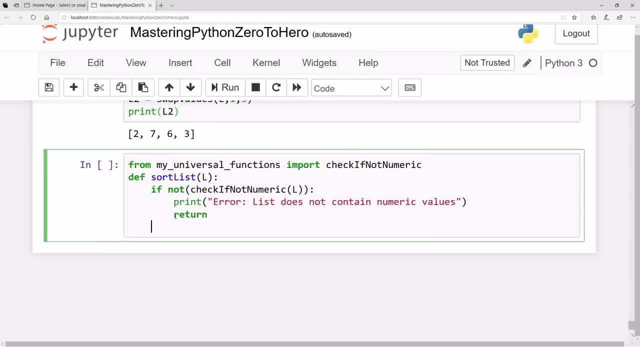 So else we need not to write else, because this return will take care of that, but for readability it is good to write else. If all are numeric, then what should we do? Okay, what should we do if all are numeric? 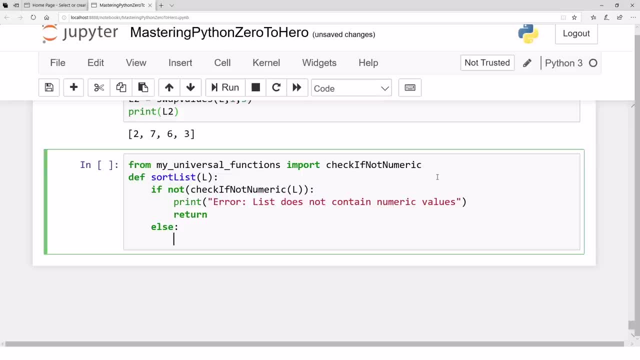 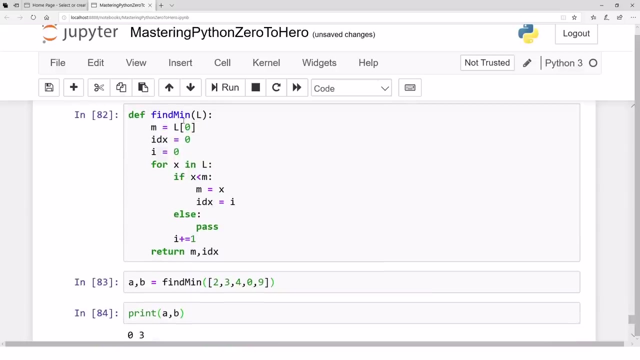 What we do is: we will be doing what We will be finding minimum, we'll be finding out the minimum and then we will be swapping the minimum from. what should we do? We have already a function- find minimum- that we can call just right away. we have a function. 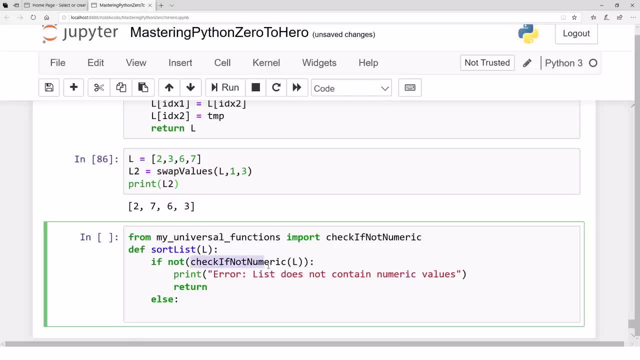 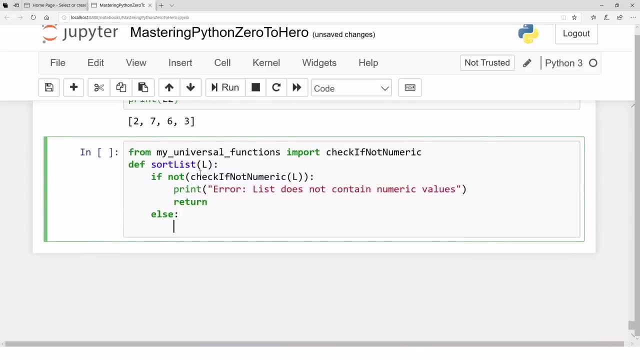 swap values that we can call right away. we already have used this function. how can we combine all these functions? how can we use all these functions just to achieve the problem sorting? We want to sort a list. how can we do that? 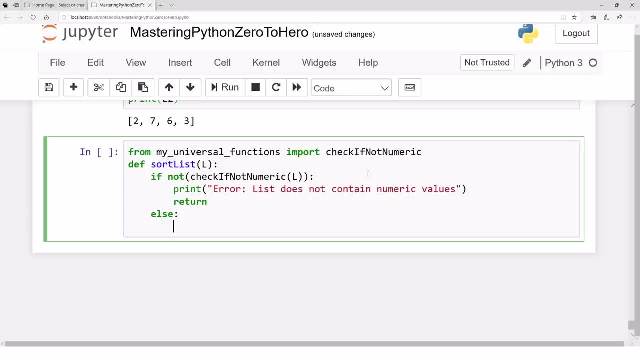 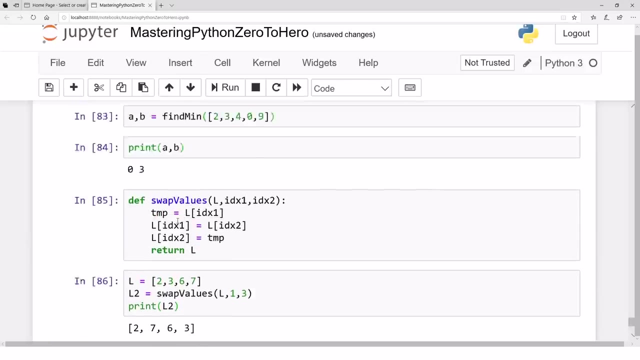 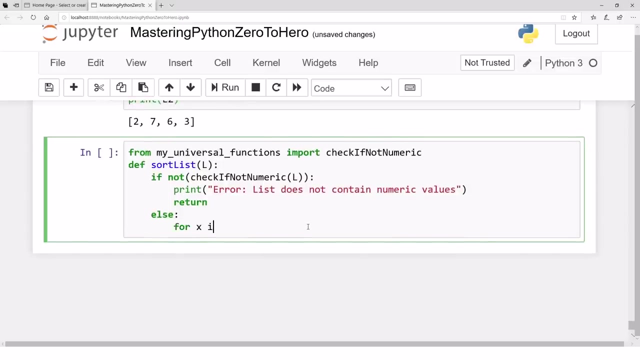 Okay, Yeah, that's, that's it looks like. yeah, it looks like a different thing, maybe, maybe. so let's just write out: let's just for x in the list. let's start thinking here for every element that is in list. 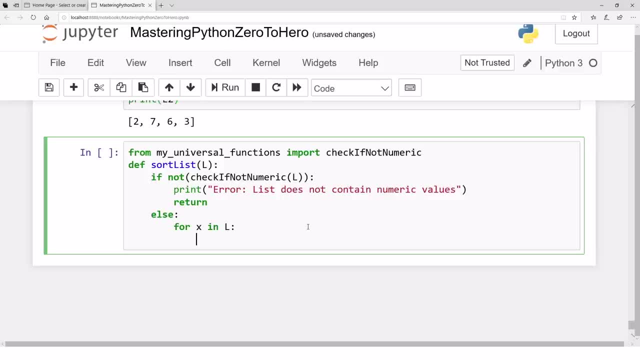 For x in the list. what should we do? We should- we should find out the minimum and swap the minimum with x, or so we should find out the minimum as well as the index of the minimum and should swap it with with. 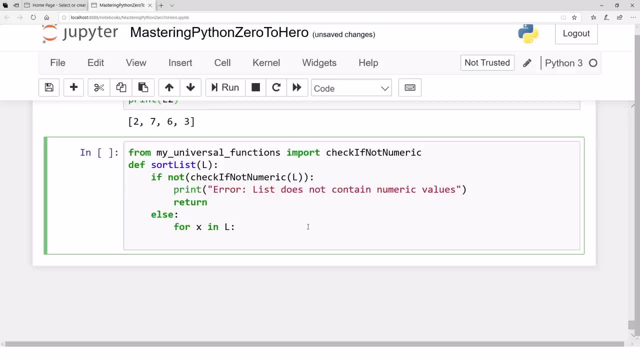 the value x and everything will become great. yeah, I guess, yes, okay, so what? what we are going to do is We are going to maintain a counter. right now, the counter is zero, which is just the index. 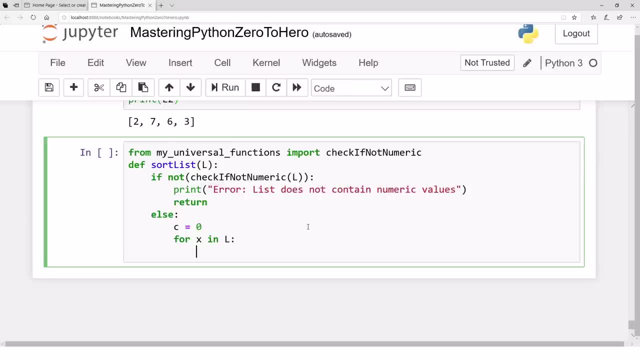 What we are going to do is we are going to find out the minimum minimum and the index where the minimum lies, so by find minimum in the list, so it will return us the minimum as well as the index where the minimum lies. and then what we do is we will say: okay, 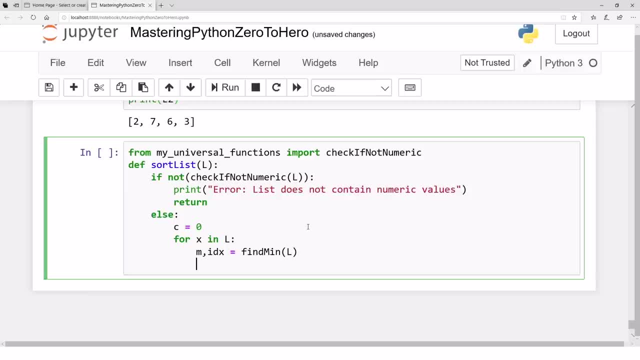 um. Okay, what we want to do is um, um. l is actually um, l is um. swap swap values with index c. swap values in the list with index c. so index c should be swapped with idx. yeah. 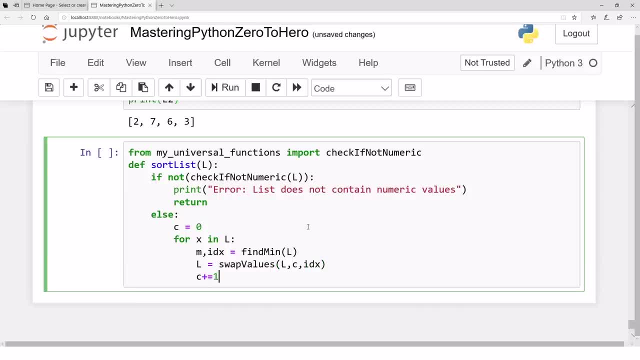 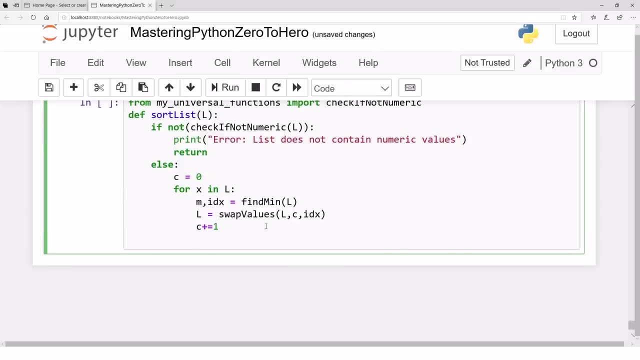 Okay, And c plus equals one. will that work? um, will that work? So after this, will the, will the whole list be sorted? So let's return a list. l, is that true? I mean, we are finding out the minimum value. 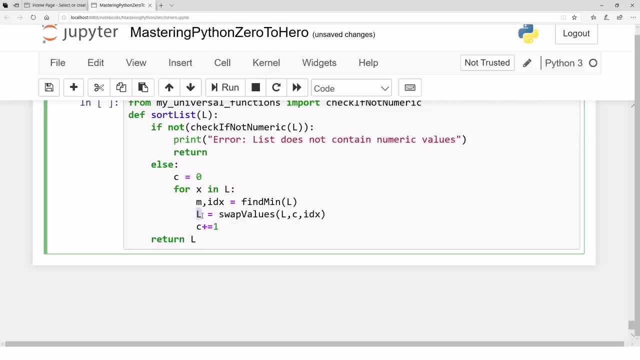 one by one. the only catch is the list is updated here and uh oh, there is a problem. okay, When we are finding out the, when we are finding out the minimum, we are finding out the minimum from the list and every time the same minimum will be returned. that's a big problem. 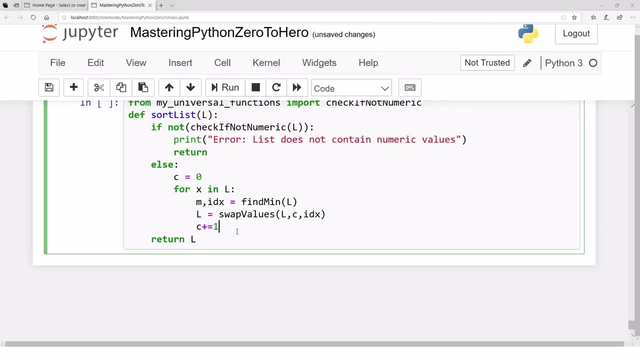 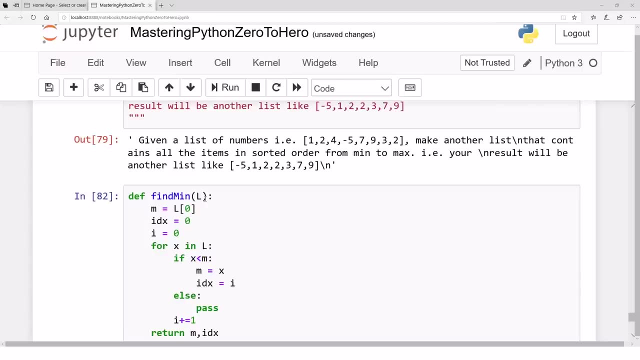 So looks like this: find minimum function is not doing our job. uh, what we need to do really is we. we should go uh to find minimum function and give it that. start your, uh, start your, find minimum. We should right click, right click, right click. uh, start your find minimum from a. 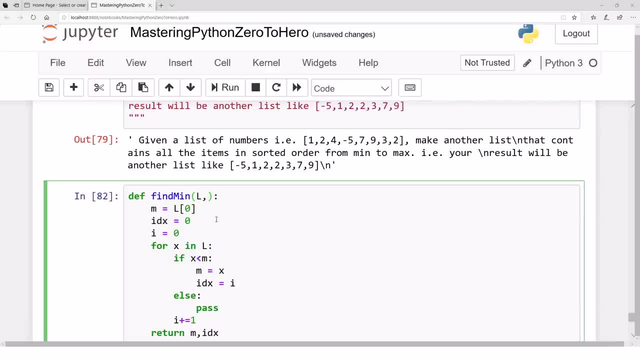 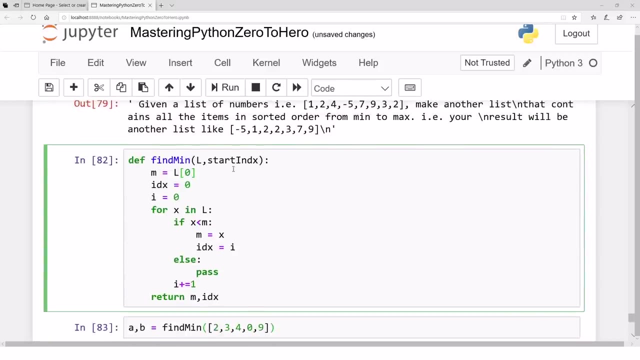 particular from a particular index. So so don't don't search the whole list to find the minimum start, uh, finding out the minimum from the following index, for example. so let's give a start index And maybe an end index, but let's give a start index. 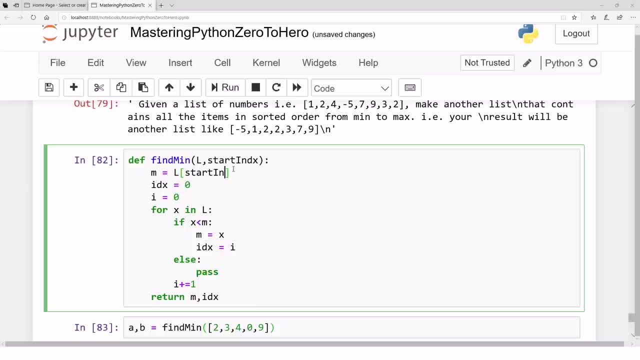 So start searching the minimum from right from there. How can we change all the code right now? Oh, that's a bad thing. startIndex. let's say this: The index right now is startIndex, and i is also start. we may use a range function here. That might be much more feasible to us, So let's use 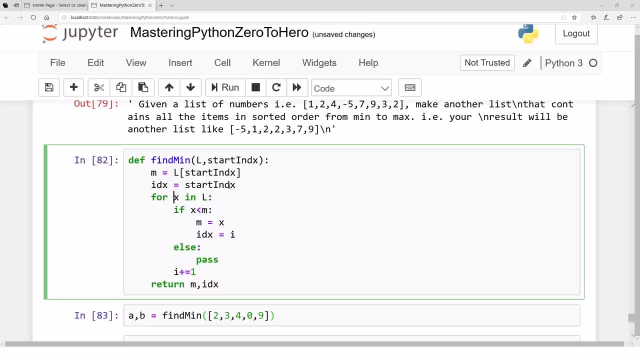 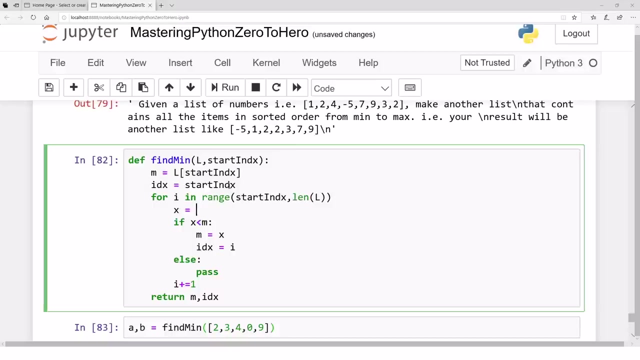 a range function Rather than this. let's change the coding a whole lot. That's a bad thing. we need to change the code For i in range, starting from startIndex, ending at length of the list and doing a step of one. Now x really is, x is really list at the index. 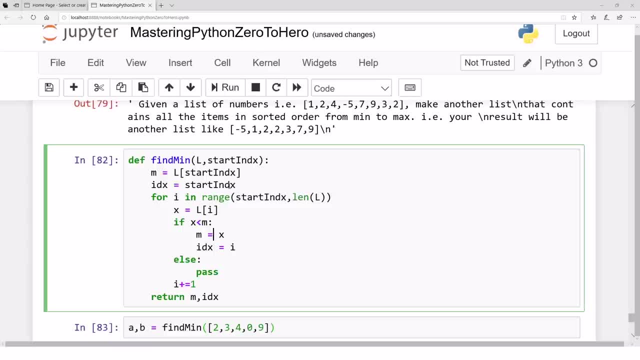 i. Okay, if x is smaller than m, then this is that, and index is i, Otherwise this. we need not to do this because this is happening automatically and rest of the story is same. I guess, yes, that will work out, Okay, great, Oh, there is a problem. Oh, we just missed. 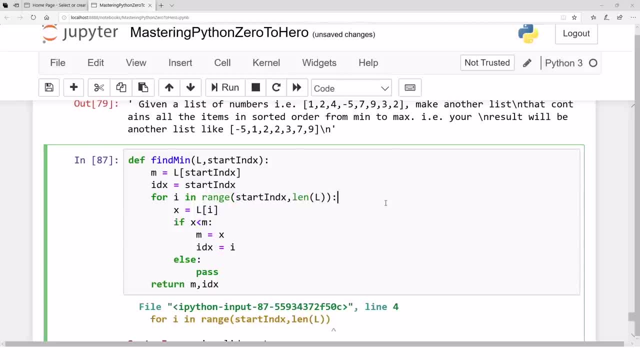 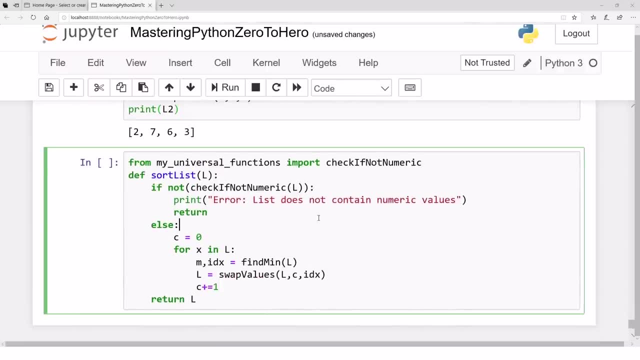 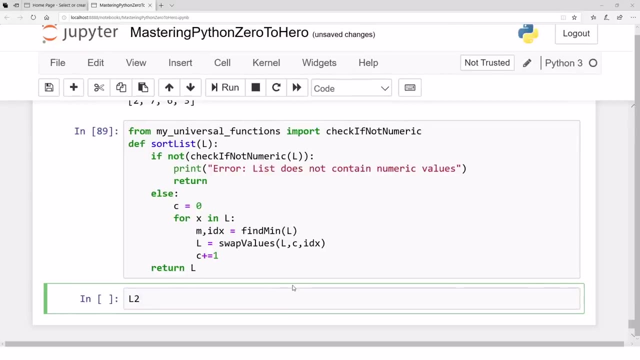 this colon here. Great, We fix it. Okay now swap value is there. Maybe this works, maybe it doesn't, Maybe there is a bug, Let's see. Let's just call this function. So let's call this function. l2 is sort list and let's pass the list as two, one, five, three minus eight seventeen. 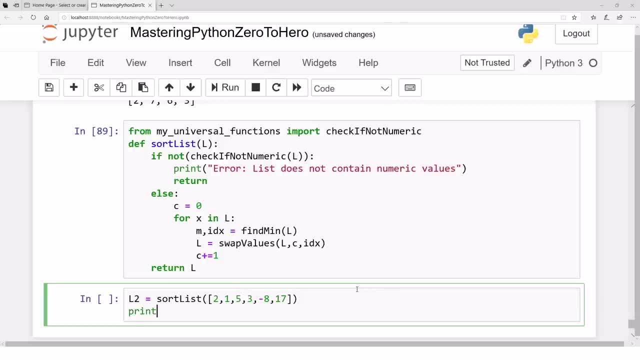 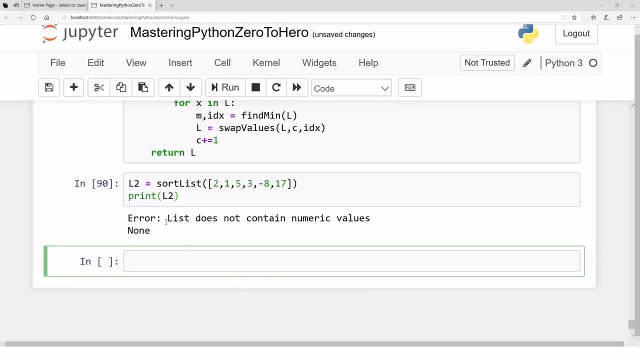 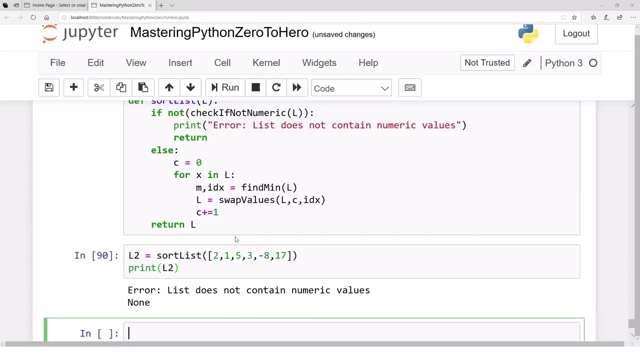 Let's say, Let's pass this list and see what it returns. If it returns, fine we might be. otherwise we will see where is the bug. if there is a bug, Oh, list does not contain numeric values- Why not? List does not contain numeric values. Why is that? 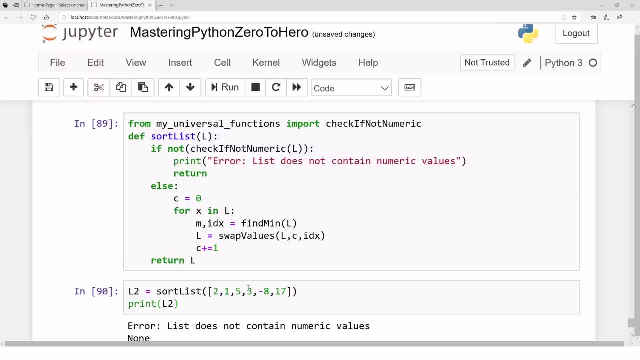 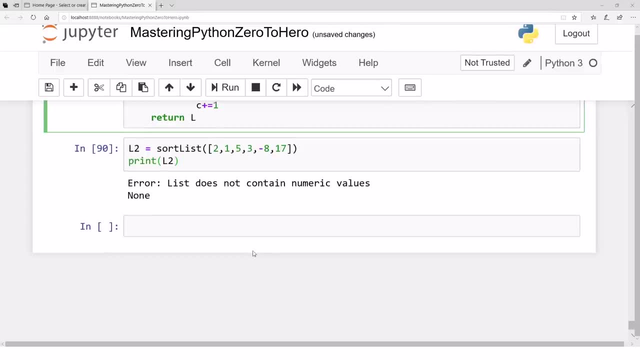 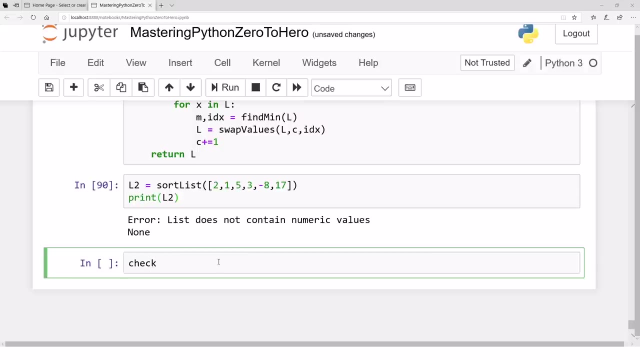 happening List actually contains all the numeric values. Where is the problem? Check if not numeric, Let's see the implementation of check if not numeric, Let's see that. Check if not numeric, Let's see the implementation. And where is the bug? Because all these are numeric. So check if not numeric. X in. 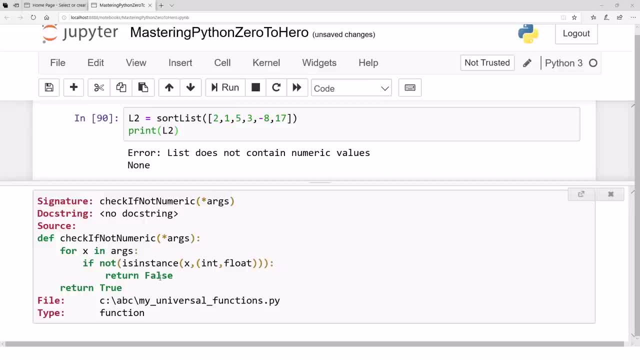 args. If not is instance, then return false. So if everything is int or float, so if X is int or float, then return. otherwise return true. So it returns true if all are. if all are numerics, So it returns true. if all are numerics. So not true means false And it. 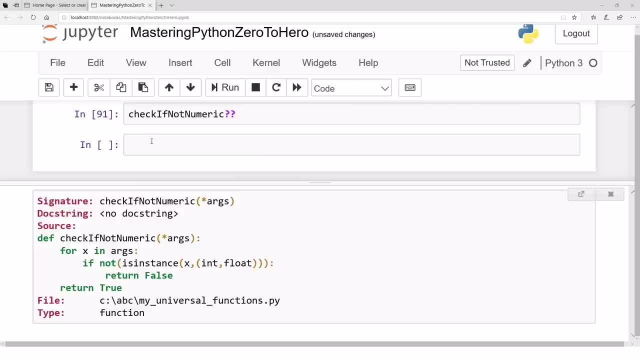 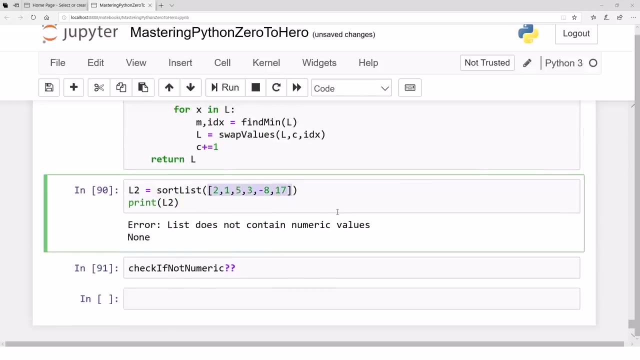 should. why? why it is why it is returning false. So that is just was. let us just see why it is returning false. That's a that's a bad news. Something is happening wrong. Let us just see how this is. 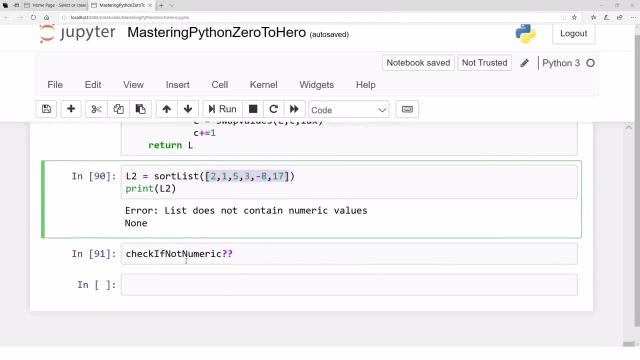 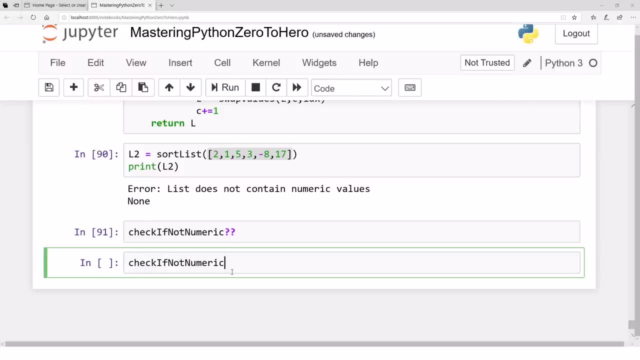 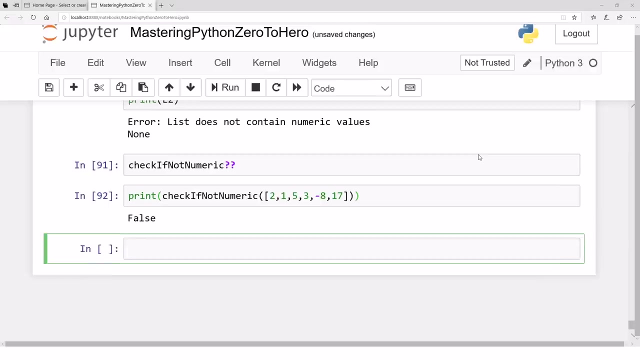 working. So let us just check, check if not numeric, And let's pass the list, this list, And let's see what is returned. Let's just print the return thing. Print: It is either true or false, So it returns a false. 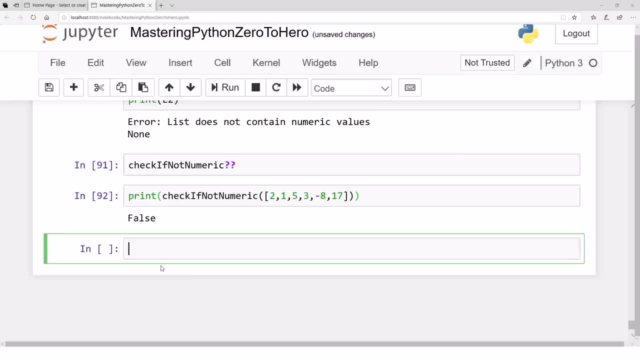 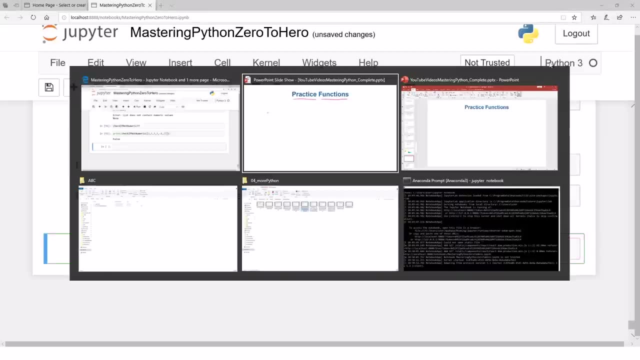 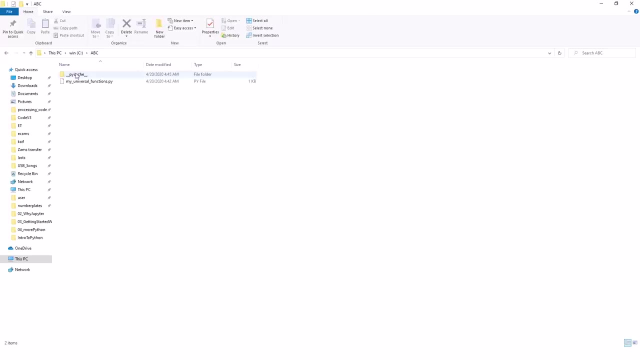 Why it is you're turning a false. It is a bad thing. Why is it returning a false? Let's go to the file. Let's go to the file here. maybe a notepad, why not? or maybe some other fancy editor. 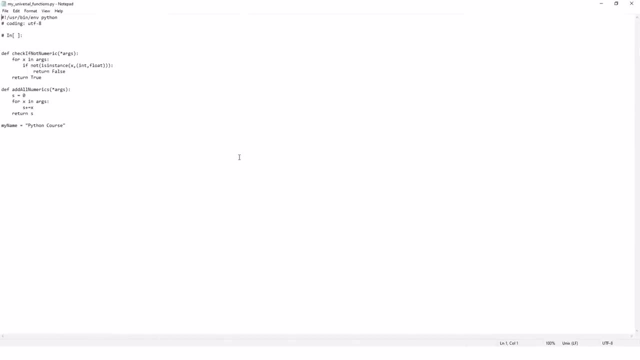 Let's open this up and see what is happening. Format font: let's have a bigger font and see what is happening. Font of 20.. Bugs are bad. they're really bad For x in args, if not is instance, so first of all is instance. 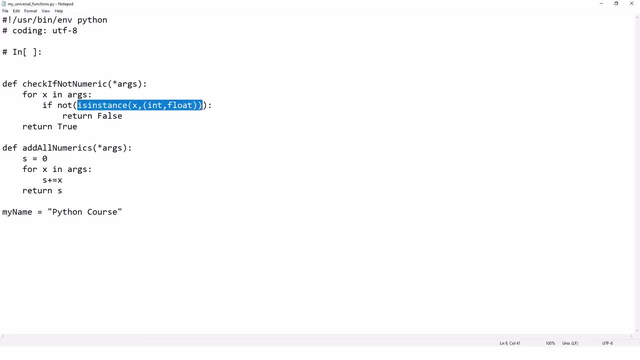 this: it will return true always. If not true, which means false, then we'll move on and the loop will be running, if anywhere you where it is finding out, where it is finding out. basically, So this this is working really fine, Let's. 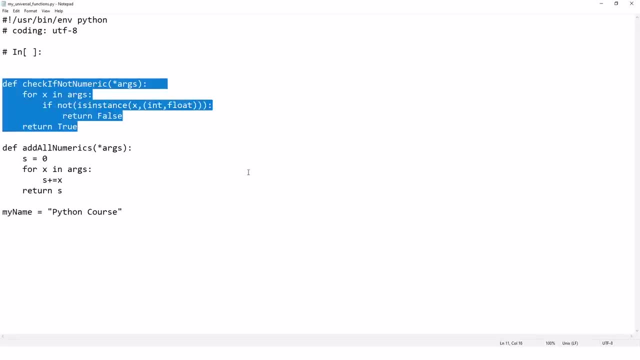 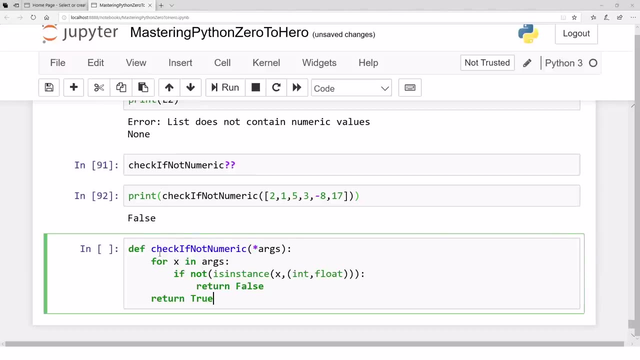 let's let's write this function somewhere inside our notebook and see what is. let's say, rather than this: let's write this function like check numeric two, check numeric two, check, if not numeric two, and let's call that function and see what happens. check numeric two. 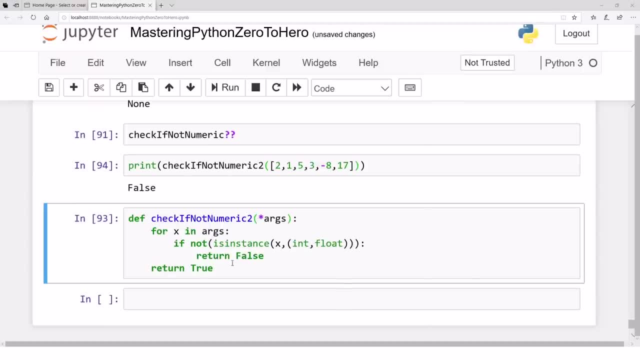 It is returning false again. Why is it returning false? That's amazing. Where is the false? So two is integer. yes, One is integer, yes. So true, true, true, true. All these are true. Oh, minus eight might be a problem. 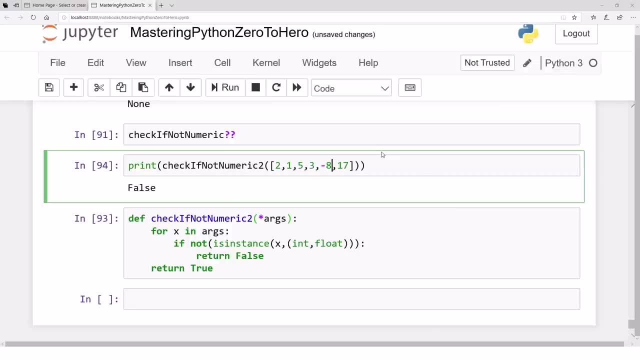 Minus eight might be a problem. Let's see, Maybe I don't know Well. well, there is, it is still false. I mean, I'm stuck here, Guys. I'm stuck here, I don't know what to do. 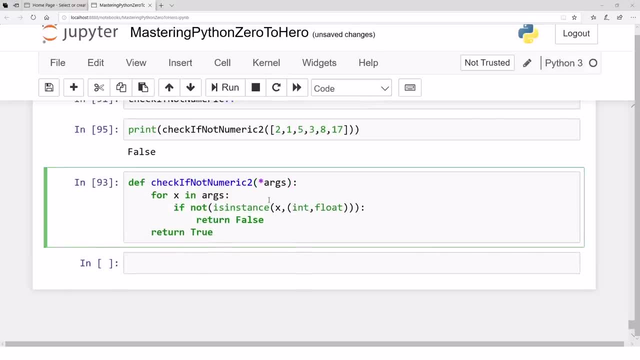 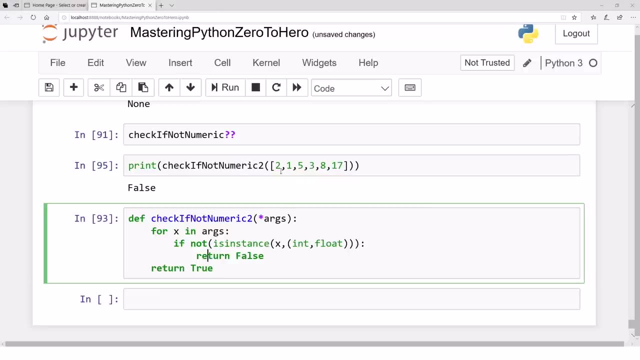 I don't know what to do. I have to debug this function. I have to go inside that function and see what is happening. So what? we really args. Oh my God, the big trouble, the big trouble. Yeah, I found the error. We are passing a list and that list is dead. 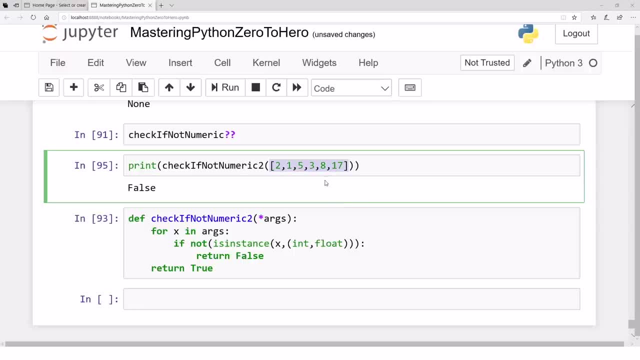 It's just one argument. That is not a lot of arguments. We have to pass all these arguments in in a different way. I mean, if you want to, you're getting, you're getting the bug. The bug is we are passing one variable, not a lot of them. 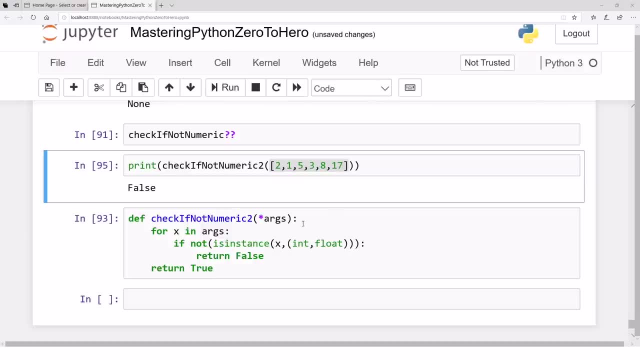 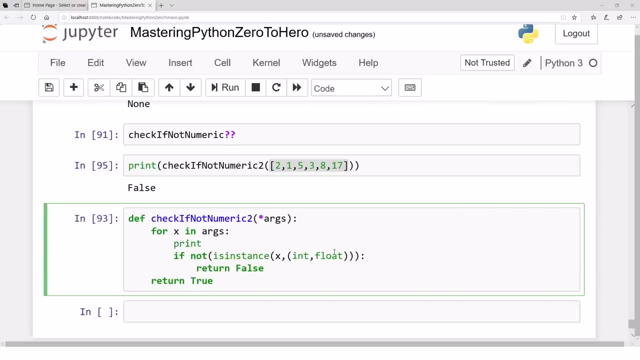 2,, 1,, 5,, 3,, 8, 17.. These are not all different variables. For example, if we just go inside and print X, for just first X, it is the all, it is all the. 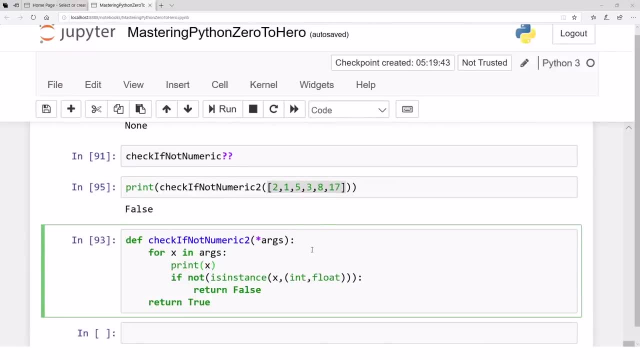 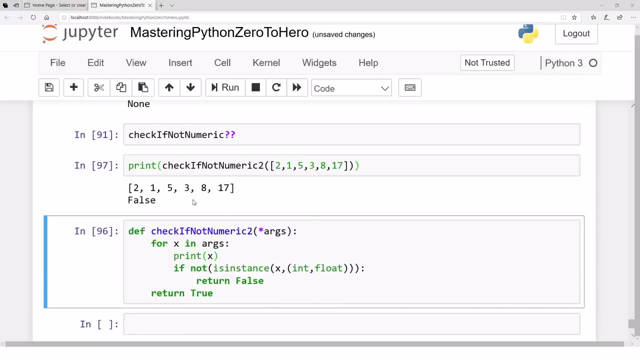 it is all the list. It is all the list. It is not the variables, one by one. Let's see: Yeah, I found the bug, Found the bug, Great, Yeah, see, it is not. it is not a lot of, it is not a lot of variables. 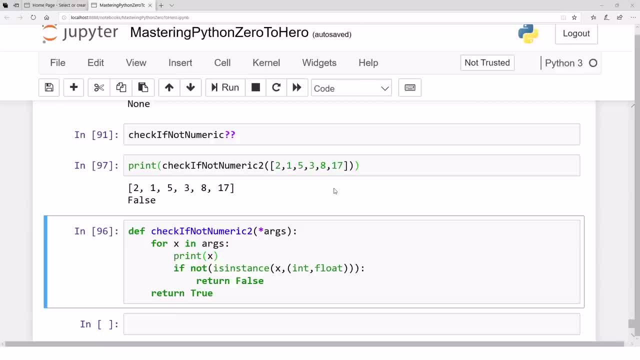 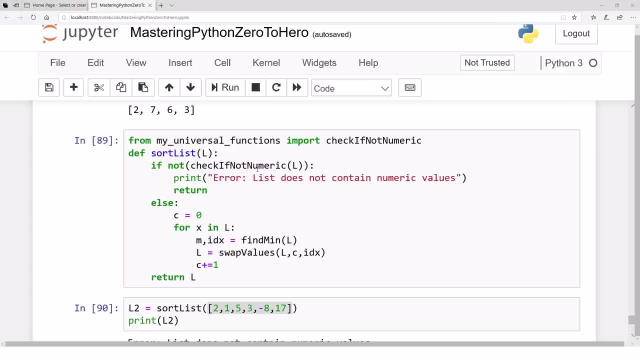 It is not a lot of arguments, It is just one argument that is in the form of list variable. That's the trouble. What should we do? Should we go inside and add another function: Check if not numeric for lists rather than variable number of arguments? 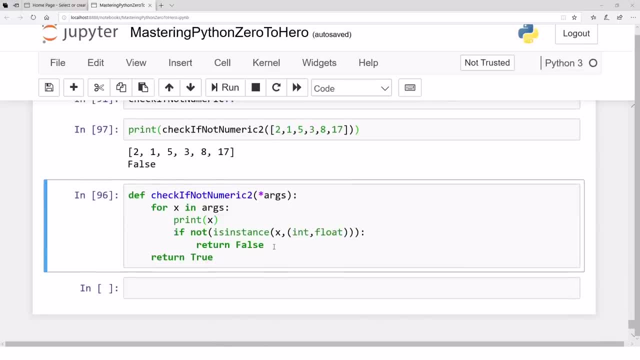 What should we do? Let's write another function that check for the list. Let's write here a checkNumeric2.. It contains a list, for example, just accepts list L or maybe L or whatever X, or just simply you can call the or L list and it goes through all the list and does. 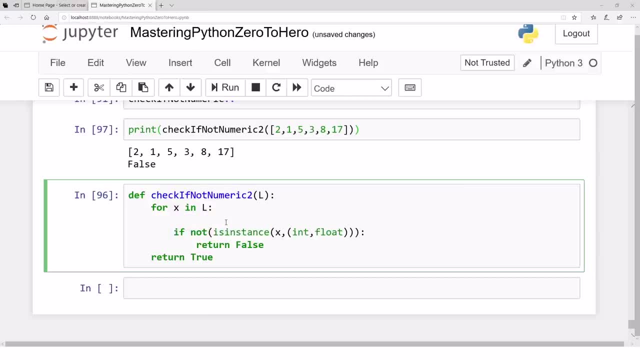 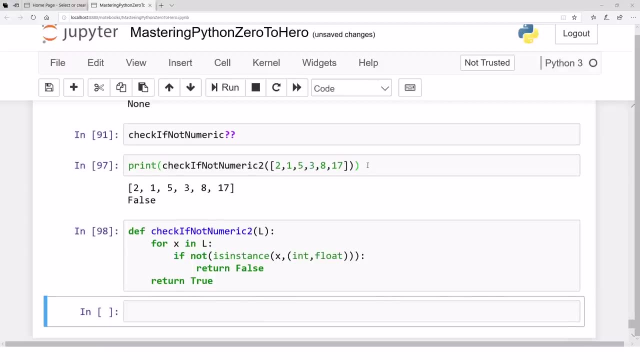 does the same job as previous. So now, now this will work. So the function that was there in our module is no longer working and it will not work. Yeah, So we are not going to use the function that is in the module. 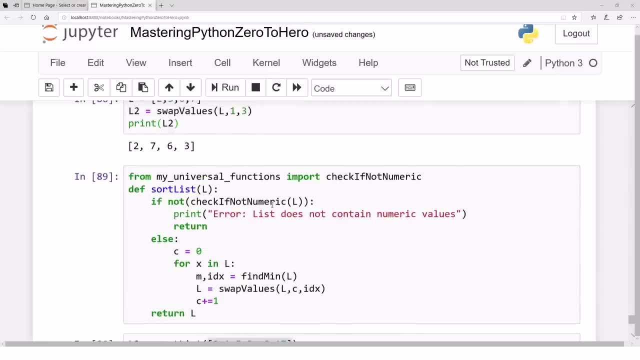 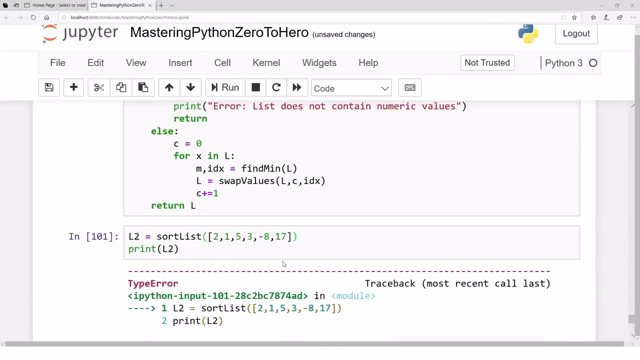 We are going to write another function that will help us here, And we have written that, And here we go, We just change that function in that And we just register that again And let's see what happens now. Oh, there is another error. 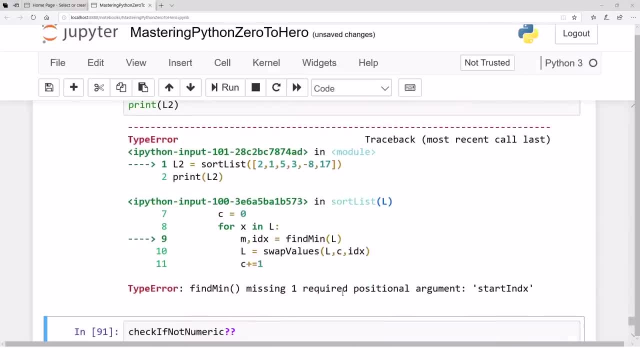 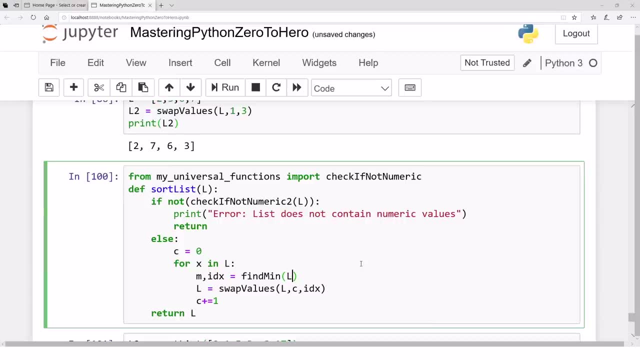 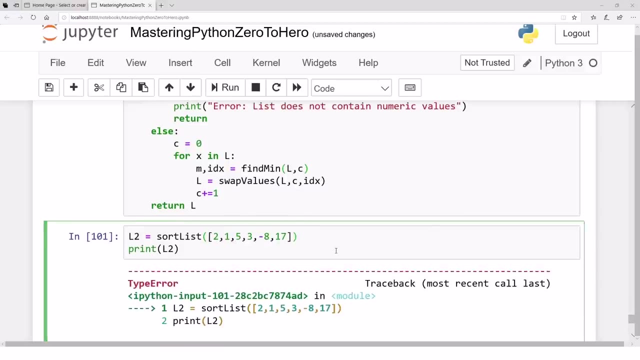 Which error? FindMin missing one? Oh, we did not find this. FindMin is missing the starting index. So the starting index is C. Great, Great, That's a problem, That's a huge problem. List is sorted, Oh my God. 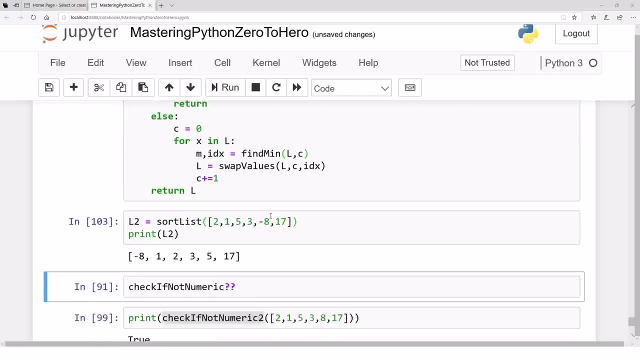 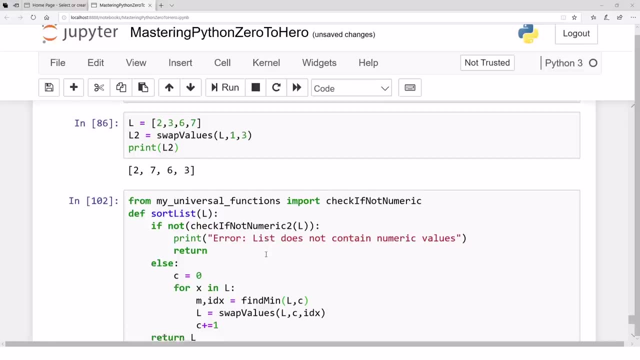 List finally is sorted. Oh, huge, huge, huge. So you see, you can call the functions inside other functions. You can call the functions from modules. if they are no longer working or no longer beneficial for you, You can write new functions. 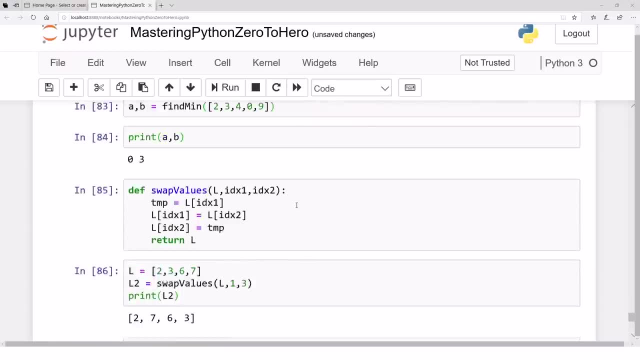 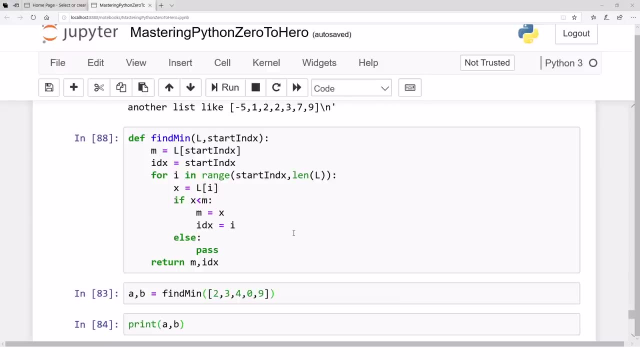 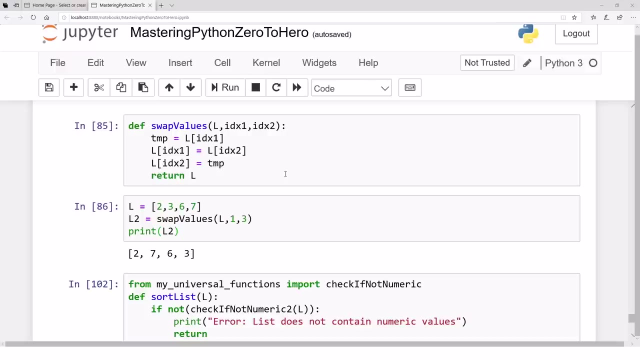 You can call them, You can yeah, all that stuff. I guess that lengthy video taught you a lot of lessons how to code. actually- And this actually happens when you are doing tasks that are really big- You have to define different functions. 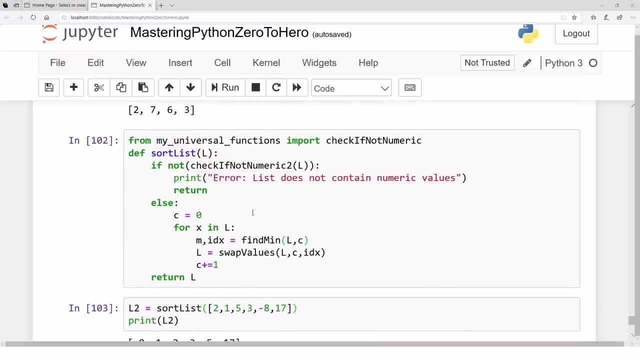 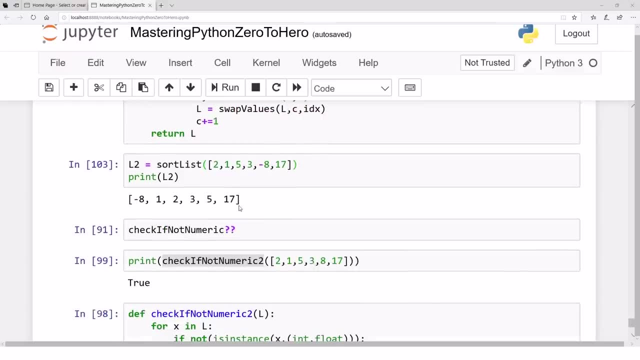 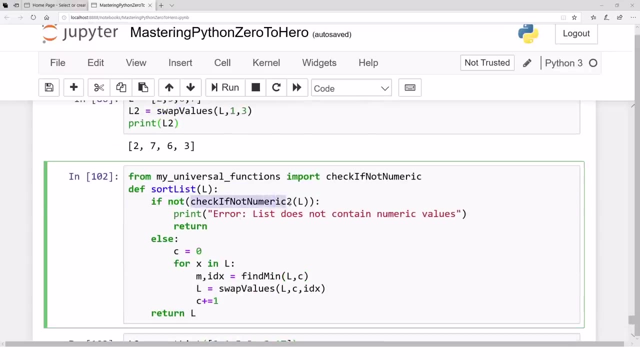 You need to define different functions for modular approach and focus on each function as a separate entity And that makes much simplicity in managing the code and bug fixing and all that stuff. You see, I fixed the bug by just noticing that, by just focusing on this function. 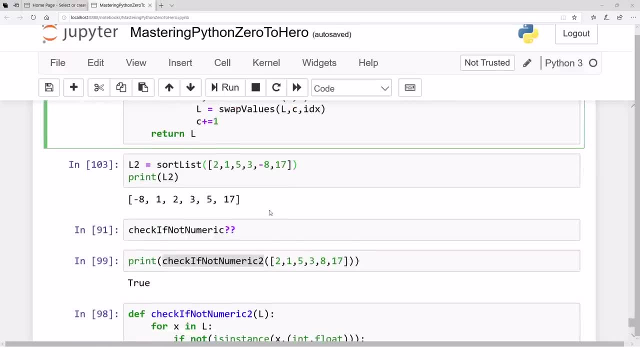 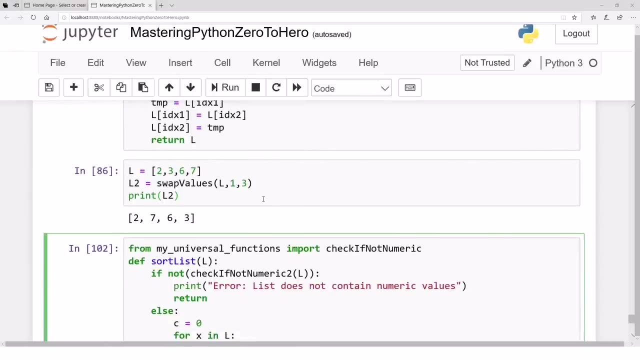 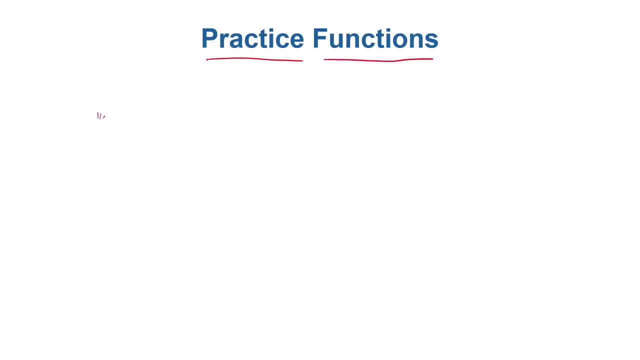 I have not taught anything else. Just focus on that function, Go and see the implementation, Fix that Everything else stays the same. Yeah, So too lengthy. Yeah, Let's stop here. Okay, Now you have done a lot of practice about functions, loops and a lot of stuff. 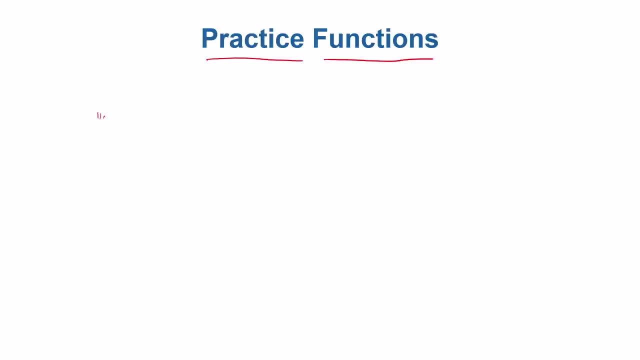 That was all the basic programming in Python In the next video. from the next video, you will see the real power- much more real power, of Python, where you need not write a lot of loops and a lot of code And still you will be able to achieve a lot of stuff. 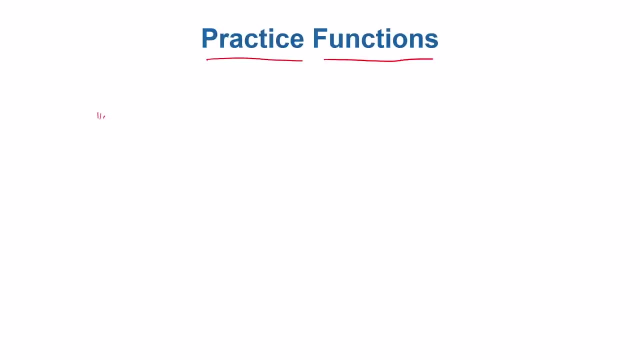 And for that we need to go through the data structures that are available in Python. So from the very next video we will start seeing strings. That's the data structure. We will see list in detail. We will see set in detail. 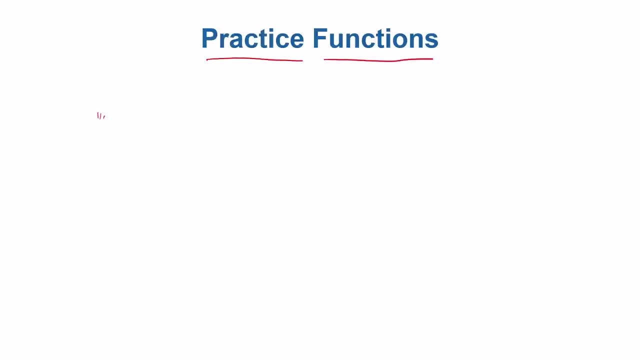 We will see dictionary in detail, We will see tuples in detail, And after going through all these data structures and getting a good grip for the data structures, then finally we will move to the packages that are available for data science, Particularly NumPy, Pandas, Matplotlib. 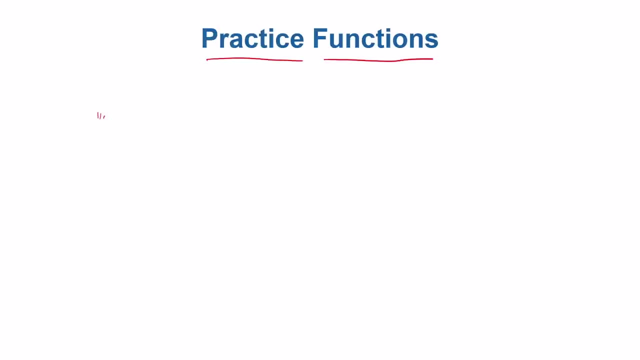 And we will see. maybe I include one or two videos for scikit-learn as well. So hope to see you for the whole new phase in Python, the data structures. So hope to see you in the next video. Okay, Let's dive into the long-awaited strings. 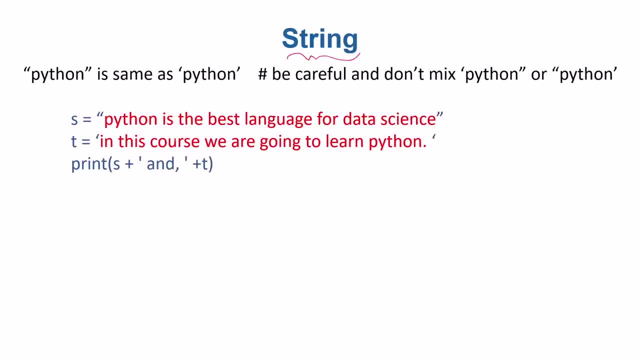 String is basically just a sequence of characters And it's a data type. It's kind of a data type in Python. It's much more powerful. The reason of I mean making this a whole new data type in almost every language is the reason is that almost all the data, all the text that appears in sequence of characters, 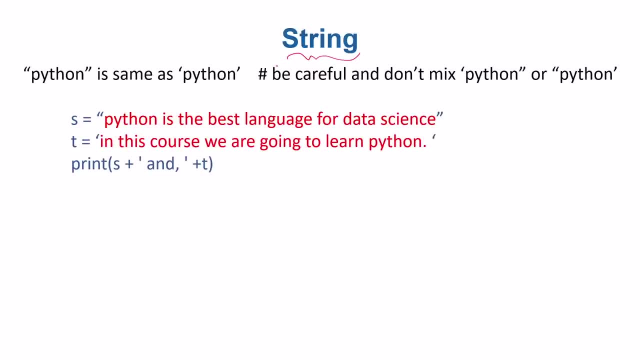 So making that sequence of characters, the whole text, as one kind of data type and writing special kind of functions to run it. And that's what string is. In Python, for example, you can declare a string, variable s or any variable name by just double quotes. 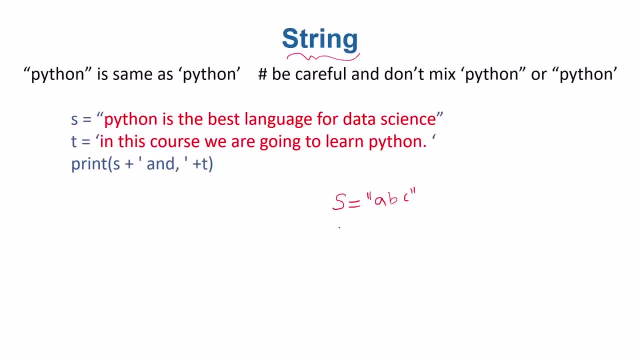 Let's say a, b, c or equivalently by single quotes. Either way is fine: D, e, f. So either way is fine. You can declare using double quotes or single quotes, Either way is fine. One thing is: be careful. 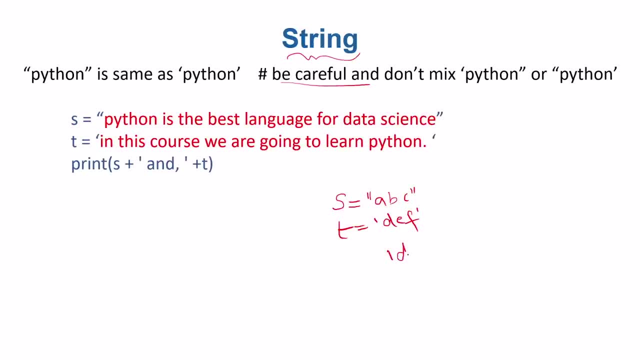 Don't mix. I mean don't start by single quote and think that now I will end with double quote and that will be fine. So don't mix them together. If you're using single quotes, use single quotes. If you're using double quotes, use double quotes. 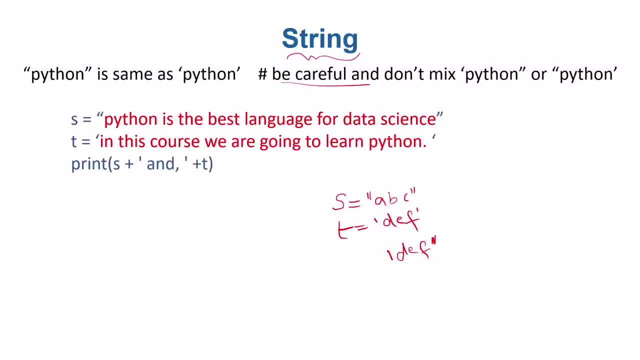 Don't mix them together. That might be much more confusing later on. So let's say this: s is a string, Python is the best language for data science. Let's say: t is another string. that is defined by single quotes. In this course we are going to learn Python. 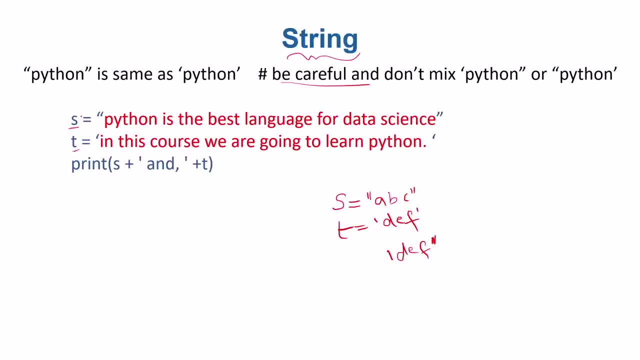 Then you can print s in a different way. Let's say, you can call a print s, You can call a print to t. By the way, you can add two string variables, s and t, and the result is a new variable, That's a v. 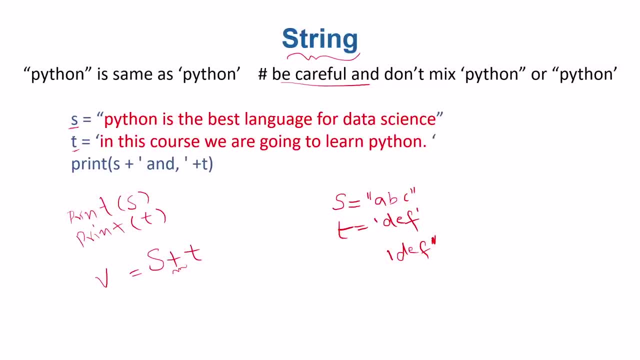 How the plus symbol works in strings is: plus in strings means just to concatenate them together. so first you just copy this string, the whole string, and then you just concatenate the other string with it and the the result is a new string. now that's a new variable. you can use that variable. 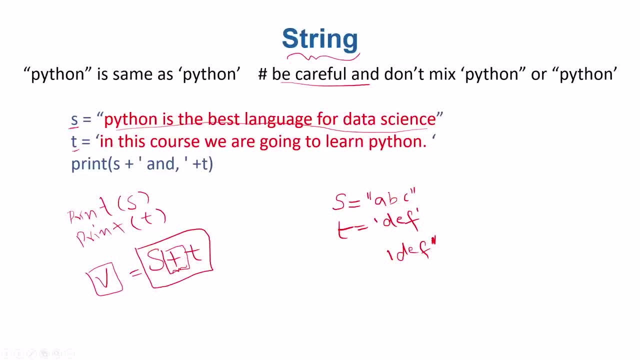 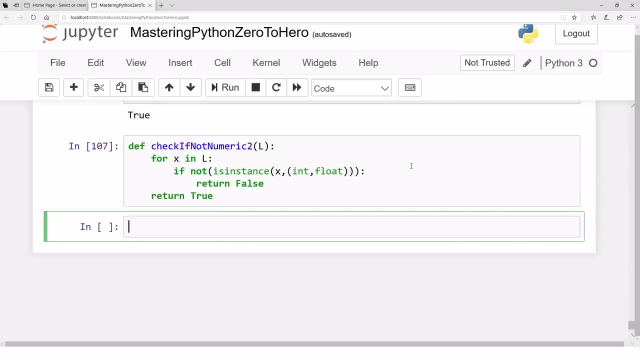 and do a lot of stuff with it. so let's go to python and see actually the prints in in the, the strings in in the running form. so let's say s is a string. let's say python is a good language. let's say: and let's have another string, t, that is using single quotes, it's good for. 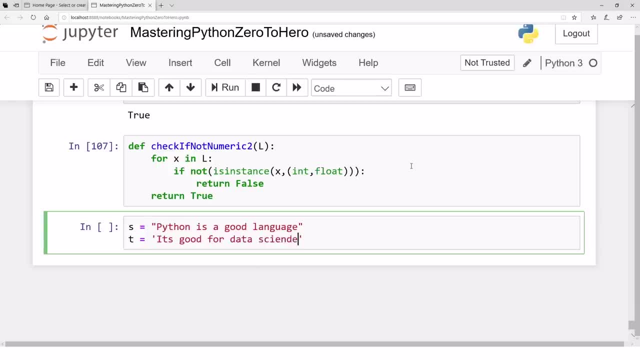 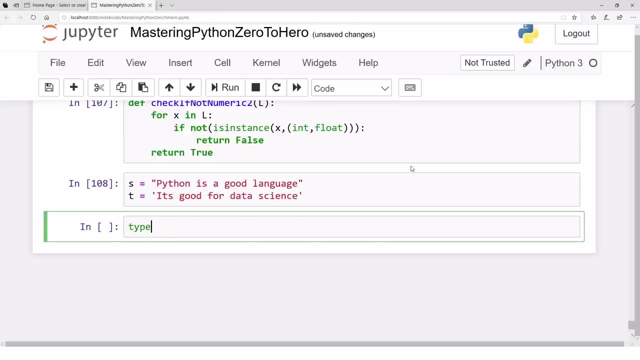 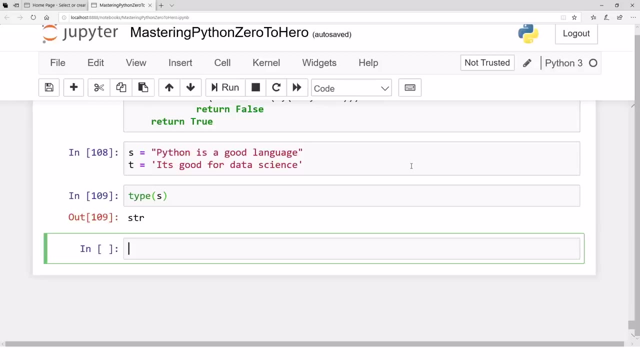 data science: s, c, i, n, c. okay, it's good for data science. let's run these two and see the type of s. what's the type of s? the type is str, string, str. that's what the type is, and if you just print s, that will be printed. python is a good language, remember. so far we are using this print. 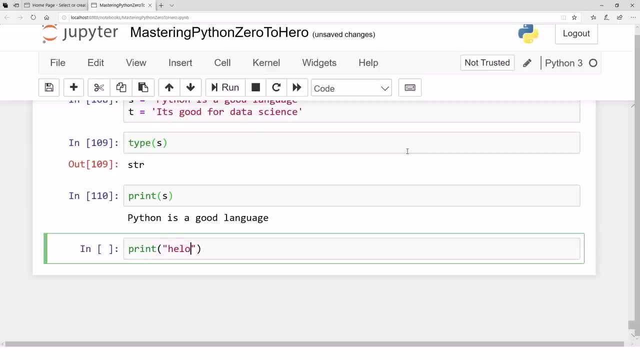 and always we use this kind of hello or something like that. that's basically is a string, because, uh, by the way, this print function- actually it takes an arbitrary number of arguments- we can print hello, then we can print anything in another type, then we can print another hello. let's say hello to, hello to. that's a multi, multi variable argument function. 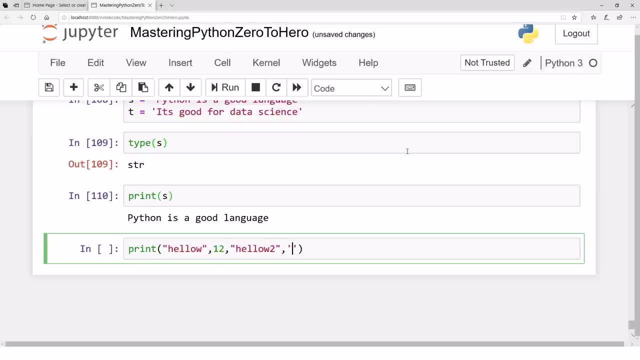 print, then we can have another string, maybe who are you, and then maybe a floating point number: 5.9. so we have used these kind of uh, we have used these kind of uh, i mean stuff a lot. um, we have used print function and we, we, we were using these double quotes again and again, but, but these are actually. 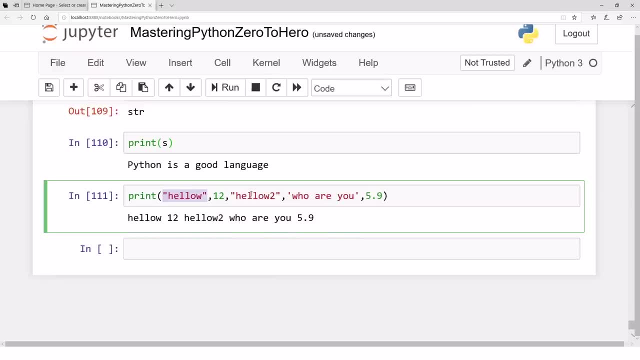 strings. um, that we will be, that we were using later there. uh, so the sprint function actually accepts strings and all these kind of normally the whenever you use print, normally you are using, normally you're going to actually display some text and maybe you're writing that text into some file and so on. 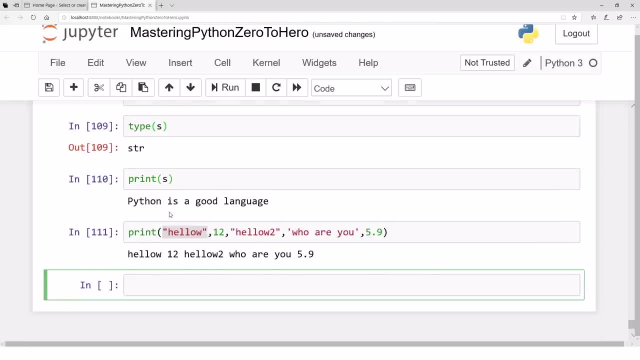 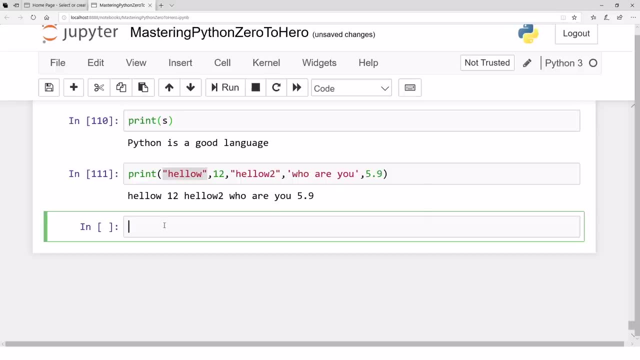 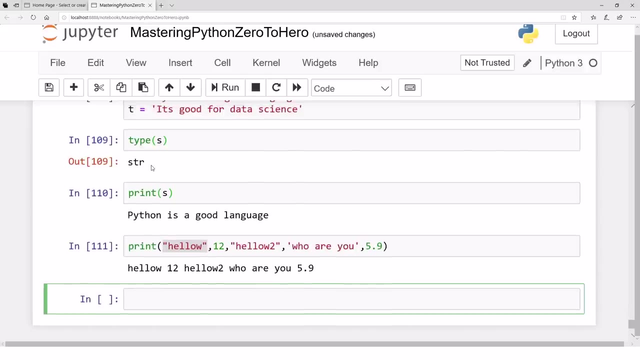 so this string is highly, highly useful. most of the data is available in the text form, in the string form, and we want to process the data. we want to find the anomalies in data, we want to fix them again. we want to stay in the text. so it is good to have a data type that actually have a lot of 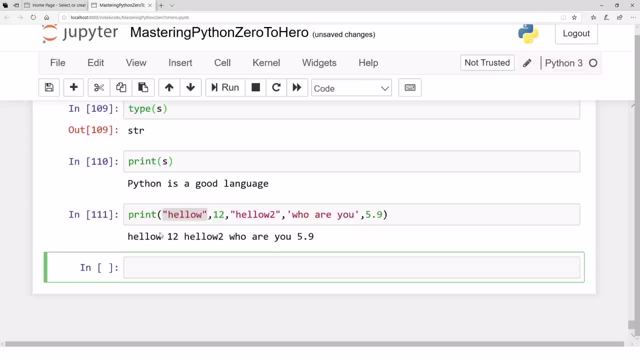 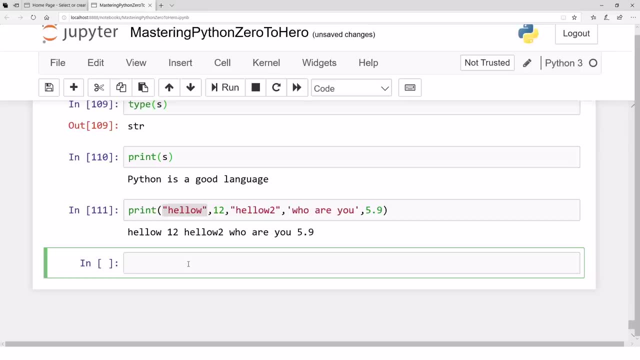 functionality that handles all that stuff. so, um, let's see, for example, another uh, um, another uh. let's see how can we concatenate the, the two strings, for example s and t. let's say we have v, that is s plus t, that's concatenated v, and let's print v. 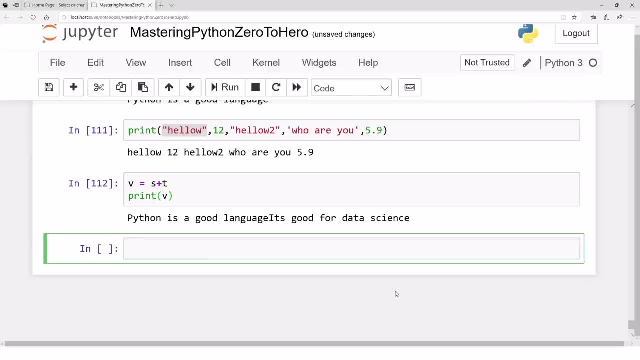 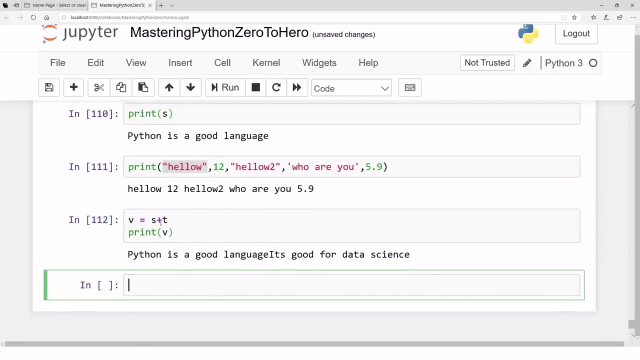 and v is concatenated. wow, python is a good language. it's good for data science. well, it is concatenated. but, um, there is no space between two, because wherever the first string ends, the second string starts right from there. what if we concatenate three strings: uh s plus another string that just contains a space? 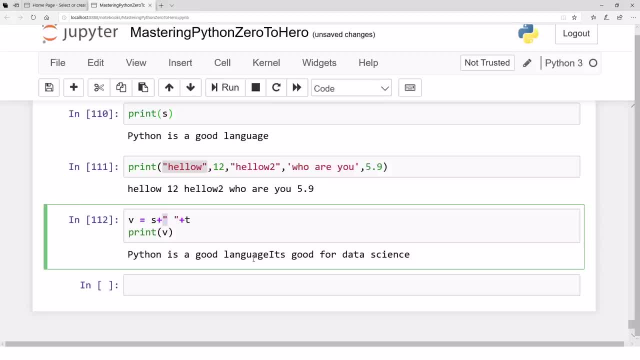 character, then the string. by the way, whatever that is there in double quotes or single quotes, whatever one character, two track character, all these things are are called strings. so now we are concatenating three strings together: s a space, one space string that contains just a space character, then t, and let's see what happens now. 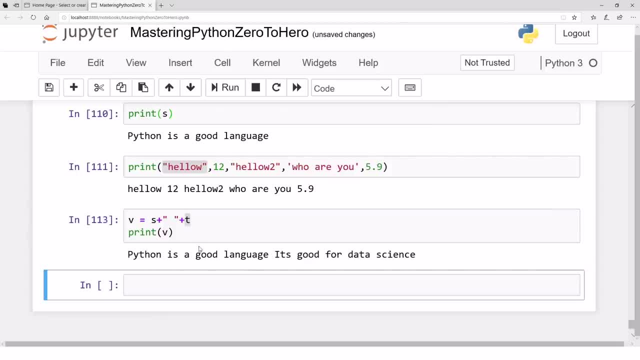 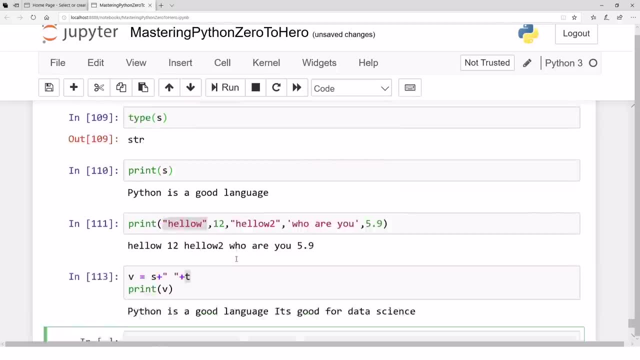 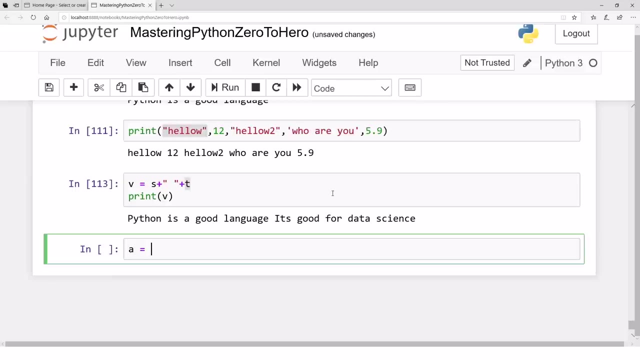 so python is a good language space, it's good for data science and so on. um, wow, so, um, yeah, so that's basically the introduction of string. what if we want, for example, uh, to concatenate? what if we want? we have a variable a which is 12, and let's say, uh, we have a variable b. 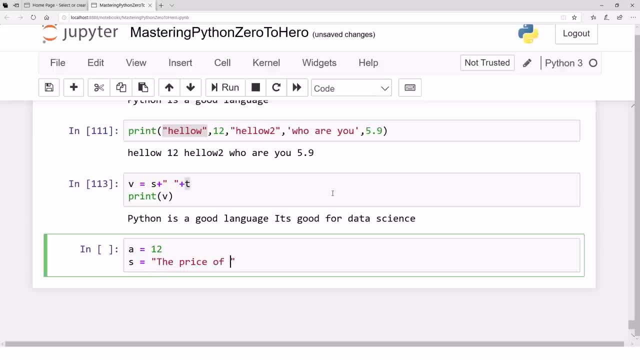 uh, the price of this book. let's say the price of this book and a is 12.. so let's say this is our price. now, price is in integer form, s is in book form. let's say we want to make another string v that contains the following kind of thing: the price of this book. 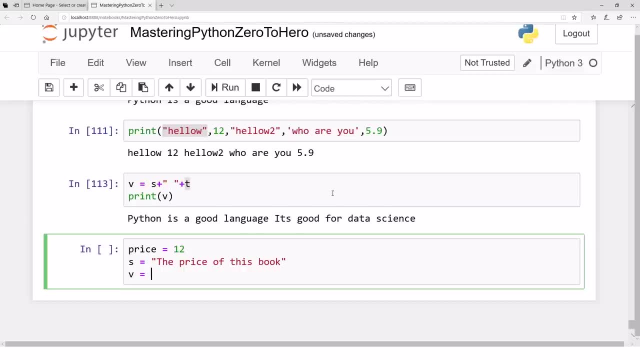 is, and then whatever the price price is, that should be there. so what? how can we do that? so let's say s plus maybe, maybe another string, is then maybe a space, so that after that the price appears. now, if we write plus and write price, price is no longer a string, it is an integer. 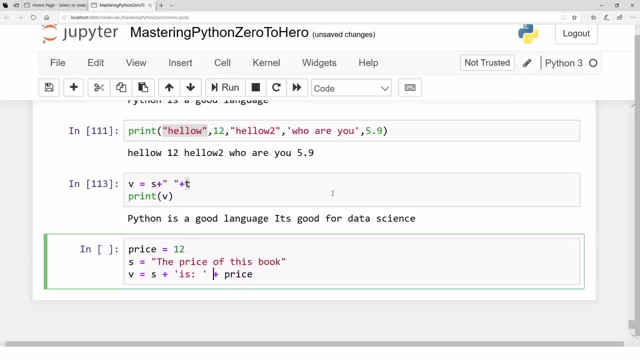 and an integer cannot be concatenated with the string in a straightforward way like plus. how can we, how can we make a message like that? the the price of this book is whatever the value of the price is. one way to do that is to convert the variable price, to convert the type of the variable of price. 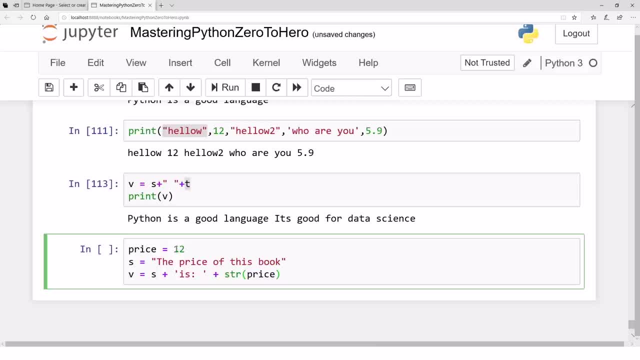 from integer to string. that means whatever the value- in this case 12 is written, that becomes a string of characters- one and two- and now it can be concatenated with with the rest of the string and we will contain the message that we want. so, for example, if we now see what is v: 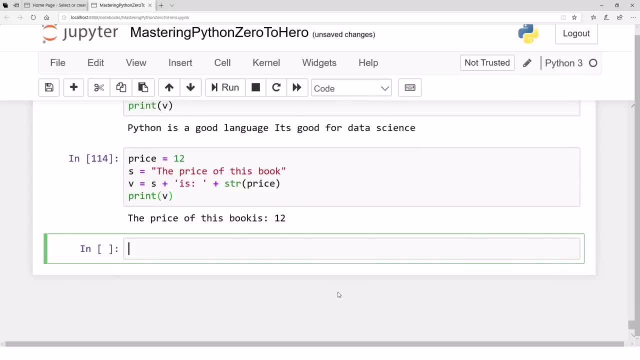 that is the price of this book is. this book is 12.. oh, we don't have a space before is so let's, let's type a space there. space is also a corrector, can be handled in string. wow, so that's how we can convert different types to string. we can have a flow type. we can convert that to string. 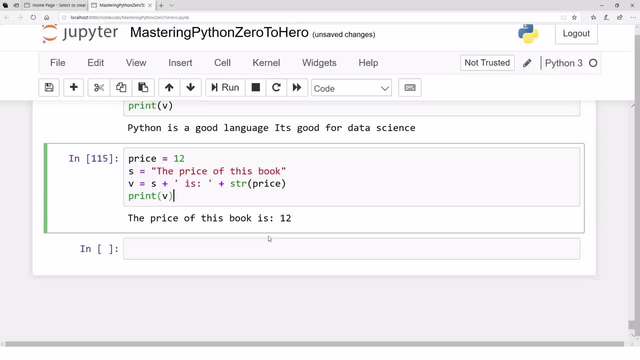 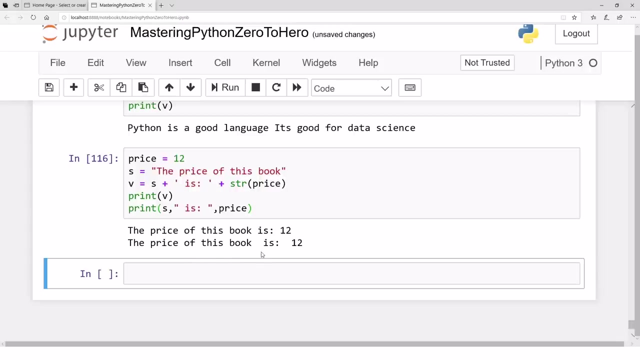 and so on. another way of doing the same or achieving the same kind of stuff is to write print. the price of this book is- i mean we can use the power of the variable number of arguments- of then price. that's exactly the same thing. the price of this book is 12. the price of this book. 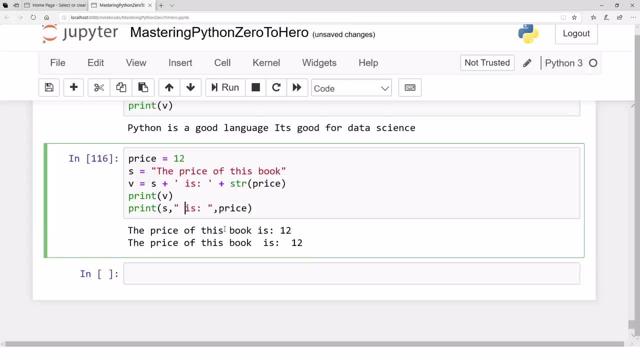 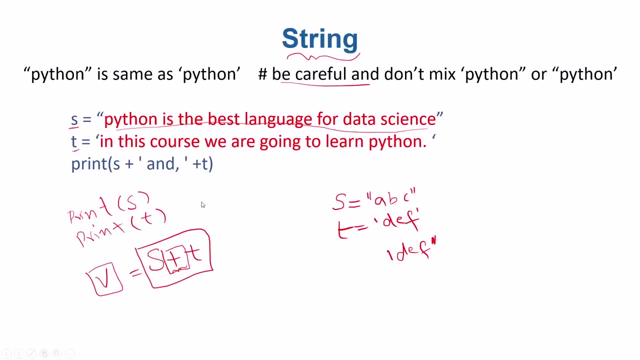 however, consider one thing: the print function automatically adds the space for different kind of arguments. you can see that here. yeah, you need not to specify a specific space. the space is automatically added if it is. if it is considered to be a different argument in the print function. okay, great. so, um, that's the introduction of a string. uh, we are going to. 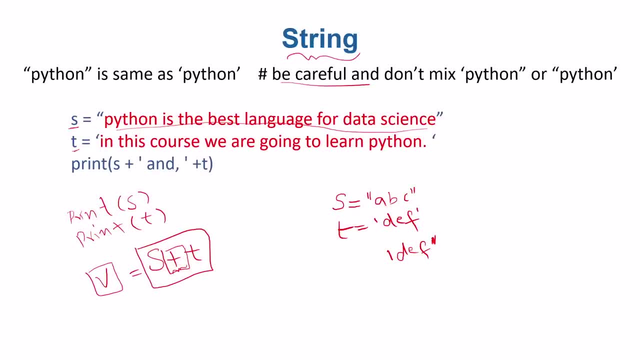 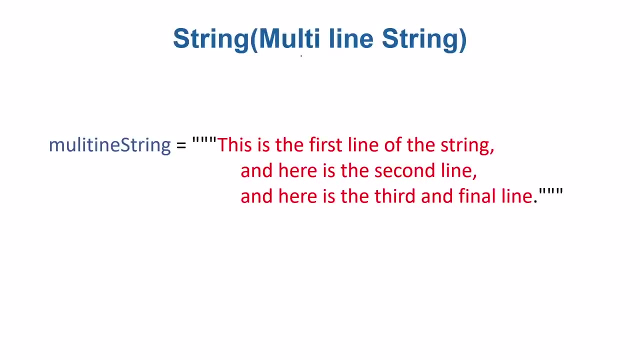 explore string in much more detail. uh, in in the upcoming videos. so stay with us. we are going to see string in much more detail. okay, hope to see you in the next video. a string might be very lengthy or may span. I mean very lengthy and may span more than one lines. or maybe the formatting is in a way that 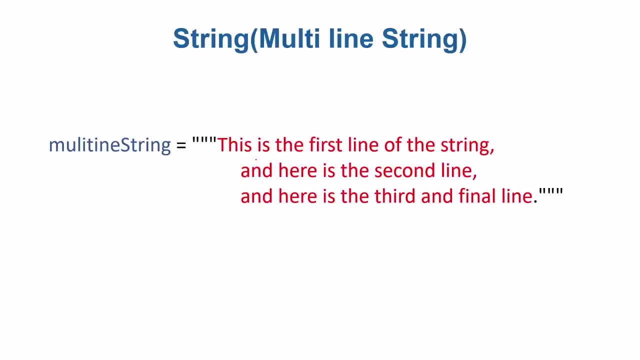 you want to. even if it, even if it is not very lengthy, you still want the different chunks of the same string to be appear in different lines. so there is a way to declare multi-line string, again using either three single quotes or three double quotes, and then three double quotes, or 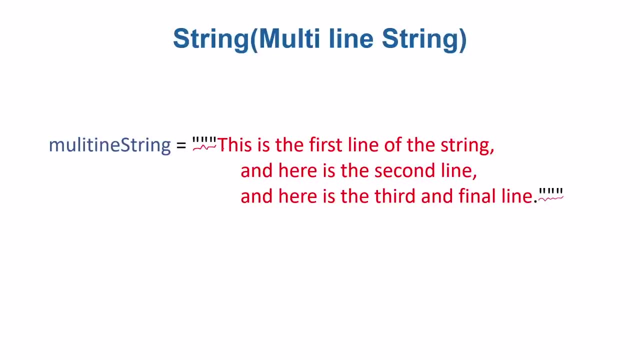 single quotes. whatever convention you follow, then you write all the string in, no matter how many lines you want, and that one variable actually contains a multi-line string. if you now print, for example, if you call the print function on this multi-line, that that's, by the way, a variable. 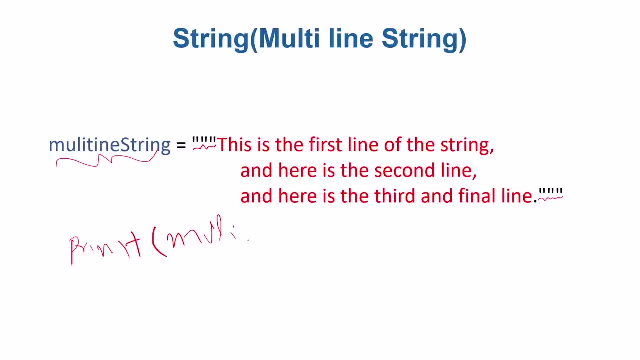 name multi-line string that contains this data: multi-line, multi, multi T line that the spelling or spellings are wrong here. I just written multi-line anyways, if you, if you call that print function, this will, the print will display this string as it is like it is there. so let's see the and and, by the way, the same multi-line string, kind of. 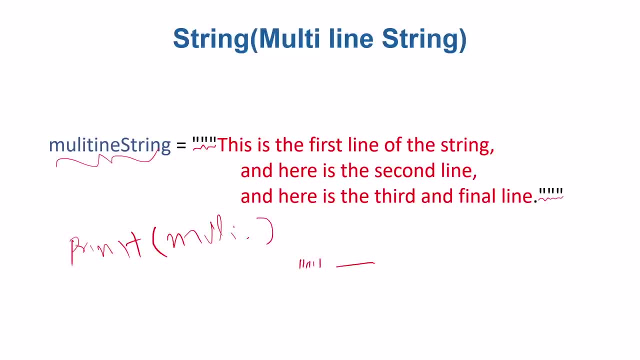 fashion. remember that that is used for comments as well. if you have comments that span on multiple lines, you can use this. so this multi-line string really is- if it is not saved in a variable and used as it is somewhere in the code, then that that's a multi-line comment. 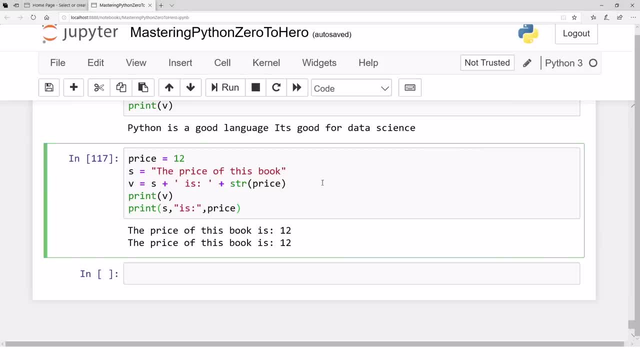 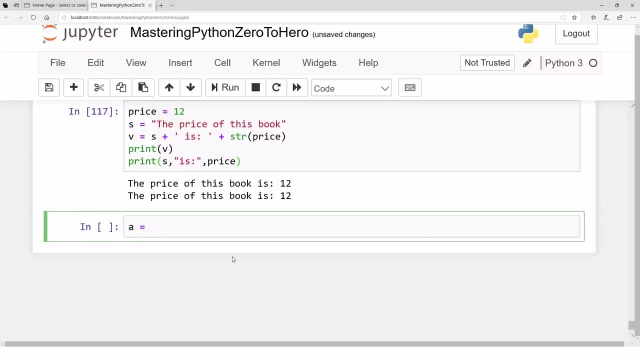 correct, so that Jesus practice the multi-line strange and interpret or notebook, see, so that they have a variable a that is multi-line strange. and let's see, the spring is this inside, and we have this is knowing too. and then we have this is last line and this line is three. that's it. okay, great, that's a multi-line screen. let's see how can 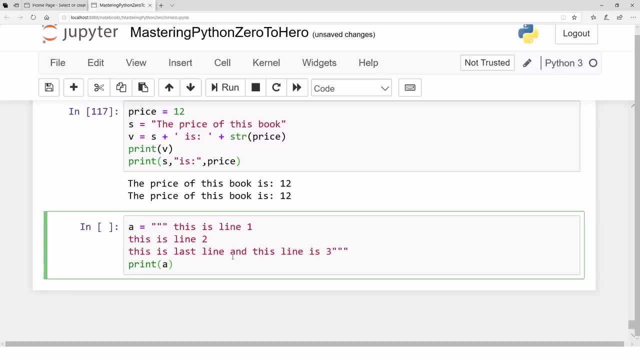 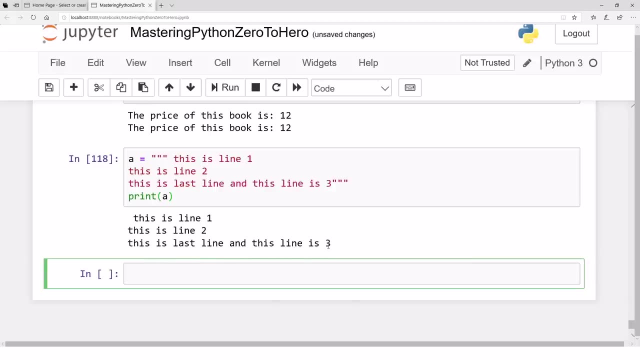 if we print a, what happens? so this is line one, this is line two, this is last line and this line is three. why this the first? this is shifted one character, right? oh, there is a space here. let's remove that space if not required and run this again. Wow, because face is a character that will. 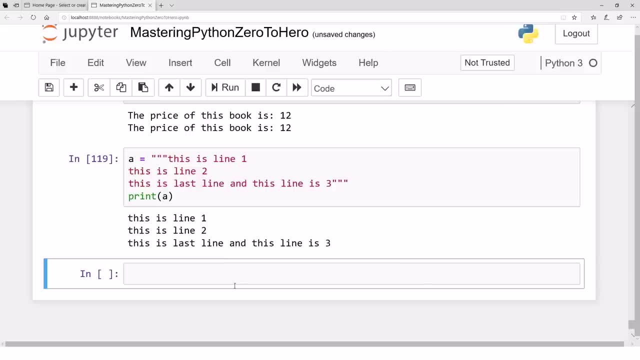 be printed. if you want. okay, what? if you really want the really want the following kind of stuff, you have, let's say, print. so what you really do is you want to print the following way: the following options are available, and the options are: let's say tab, tab, tab. let's say hyphen a and that does. 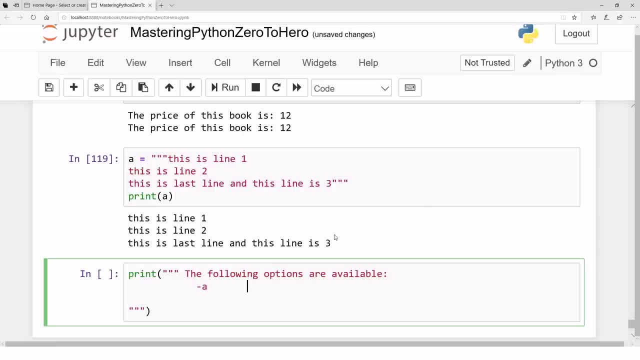 hyphen a, that does nothing. and then we have, let's say, hyphen b and there also also does nothing. let's say, you want our message to be printed in in such a way. what will happen? let's see. ok, the following options are available: hyphen a does nothing. 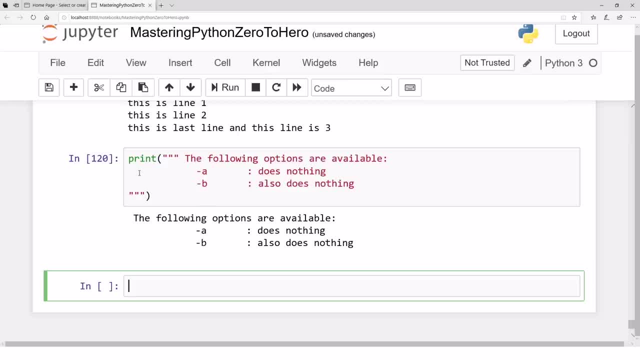 hyphen be. i mean, all this is a string, multi-line string, these characters that you think they are not there. these are spaces and they are. i mean, the spaces are printed here. the spaces are printed here. you're seeing, nothing is printed. these are the spaces that are printed there. 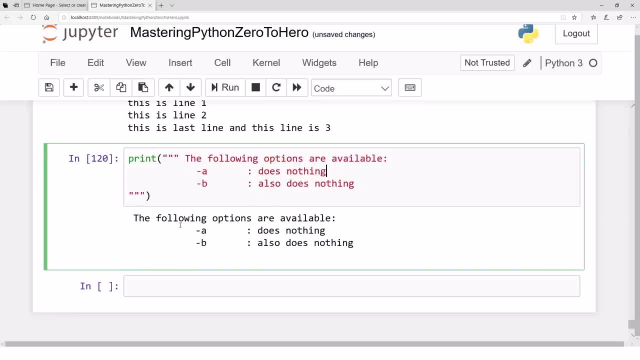 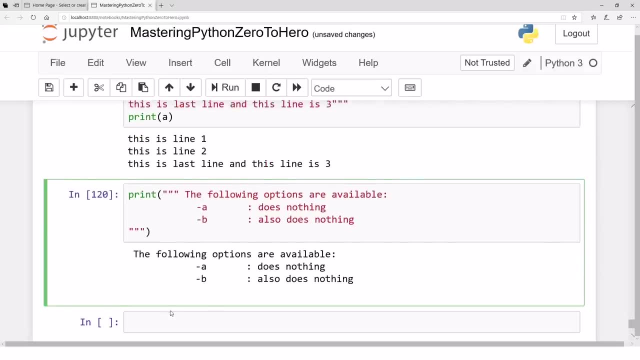 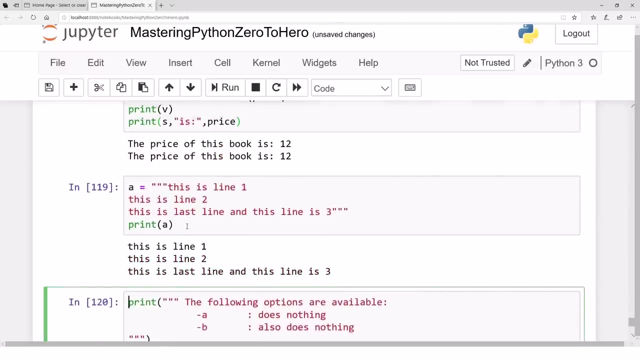 so sometimes, this multi-line string, it helps to format our message in a way that we like, so that's helpful, helpful in most of the cases. further, if you write this multi-line, by the way, if you write this multi-line comment in the start and end of any code script, that means the. if you write this, 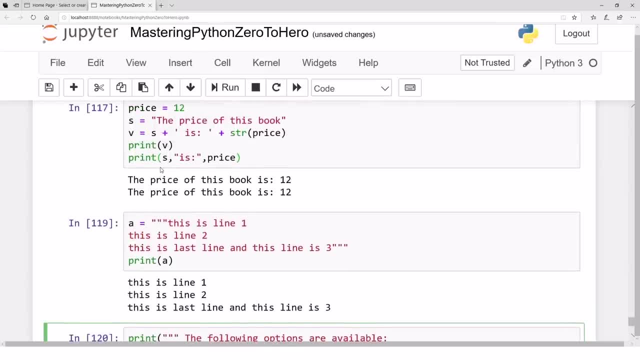 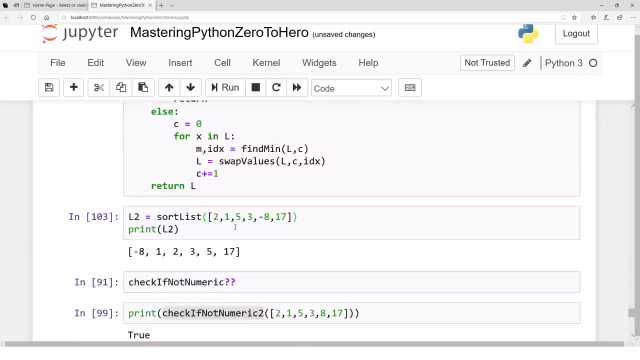 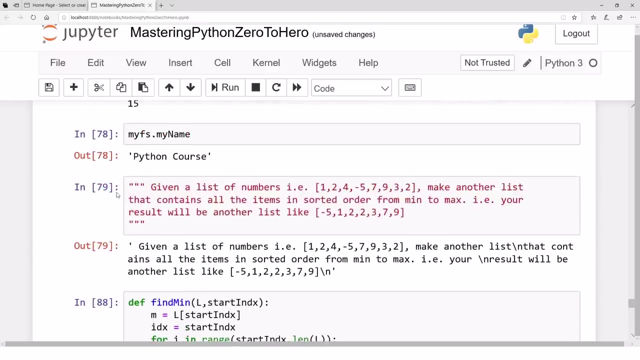 multi-line way of defining the strings at the start and end of any code script. that code script is commented. that we have seen several times earlier as well. so, for example, in problem solving, remember that we define all: oh yeah, so that's the comment, that's a comment. 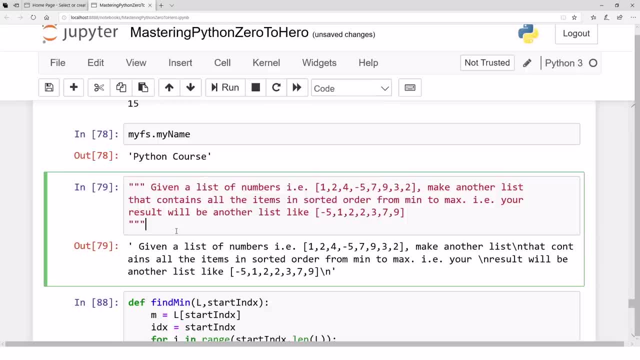 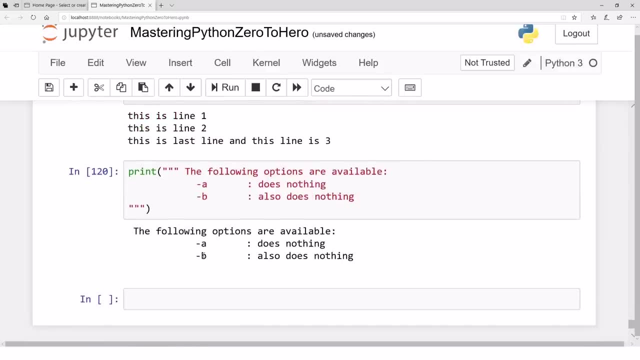 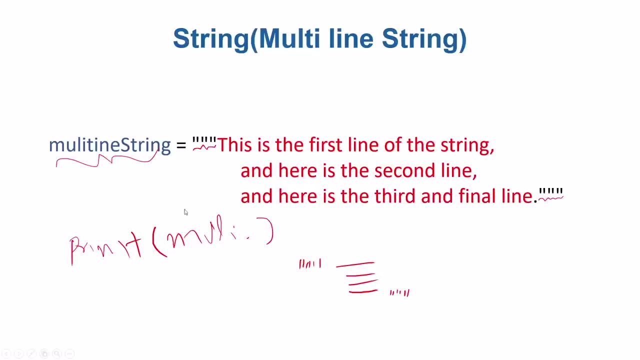 you, even if some code is written inside that will not be executed, right? okay, so that's about the multi-line string. in the next video we will see because- because the string really is- is basically a collection of all these characters- what if you want to access a particular character, for example? 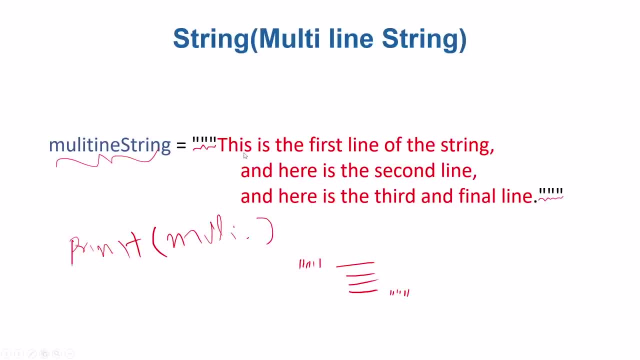 this is the first character. is t here? the second character is h, the third character is i, the fourth character is s, the fifth character is space and all that. what if you want to access you particular characters inside the string, because the string contains a lot of characters. 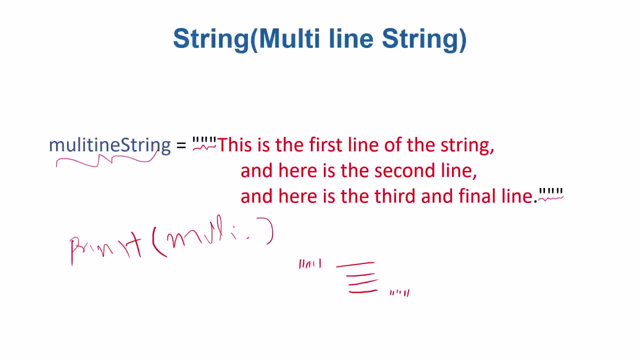 what if we want to play with some of the characters inside the string? how can we access different characters? for example, if i want to access a seventh character of the string, how can we do that? so let's see in the next video how can we index different characters inside a string. hope. 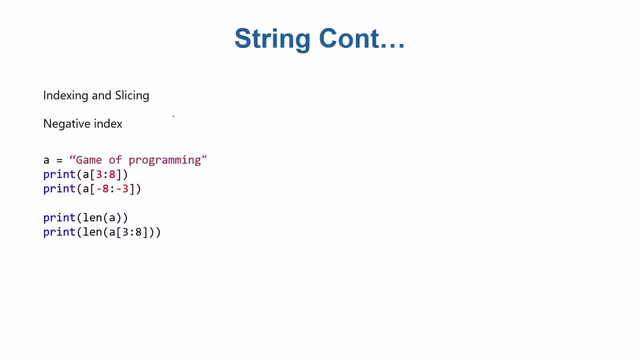 to see you in the next video. okay, in this video we are going to actually access different characters inside the string sometimes called indexing. uh, the term slicing is basically more relevant to arrays. lists are, uh, actually the, the mutable structures, but we will see. uh, um, i'm, i'm just comparing, because you you may listen this term slicing again and again, but 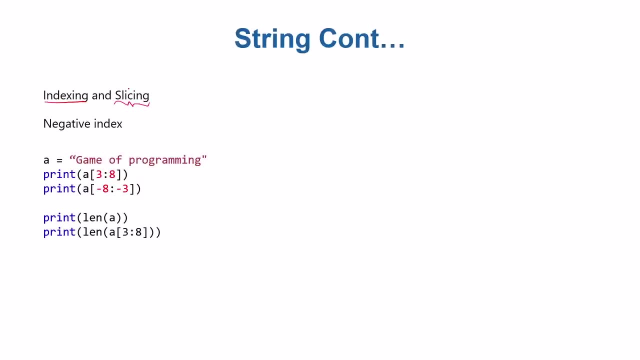 really it is indexing, but we will see that indexing or slicing- sometimes these two terms are used interchangeably. we will see the examples of slicing in detail in lists and and in more detail in numpy arrays. but here you just think that indexing and slicing are the same things. index. so, for example, I 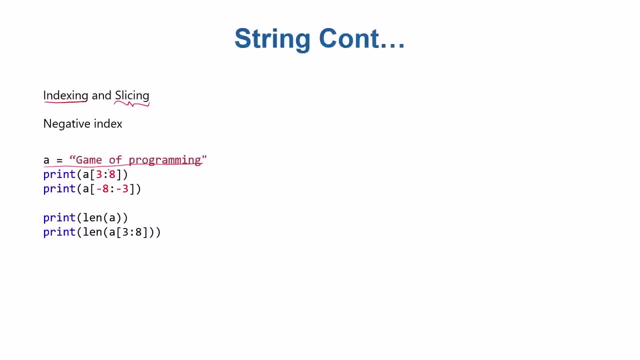 have this a. let's say this is a array a and I want to access its fourth element here. the fourth corrector element is e. by the way, this a is a variable. if I want to access the very first corrector, the, the indexing the number, the. 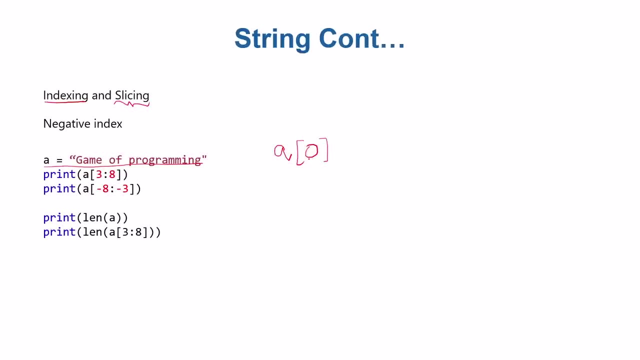 positioning starts from the integer 0. that's the first corrector. so if I want to print out of it, that will print G. if I access. for example, if I write the index 3, what do we mean? that means the fourth element. the fourth element is e. 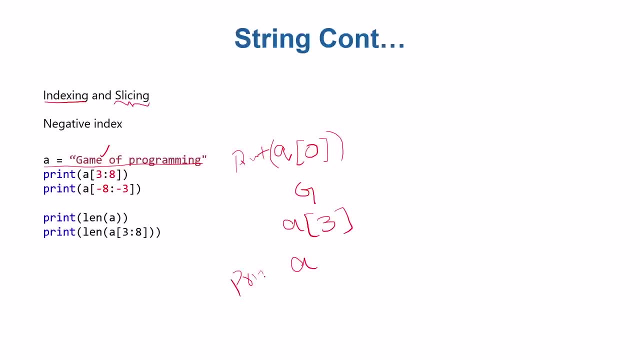 what? what will be printed? what will be printed? if I access the fourth element of the index 3, index 4, if I access this thing, a space will be printed and you will be seeing nothing, because when a space is printed, actually nothing colorful is printed there and you might be thinking: oh, nothing is printed. nothing, nothing have. 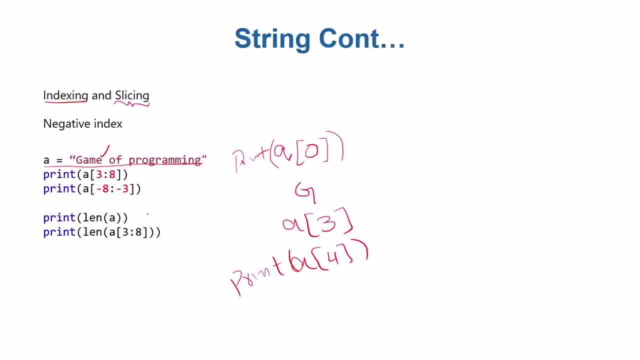 been accessed. actually, a space corrector have been accessed. so, yeah, a more we can we can, we can actually access. we can actually access a substring inside a string as well. for example, we want to access, for example, a substring starting from index 3 and all the way up to index 8, but does not. 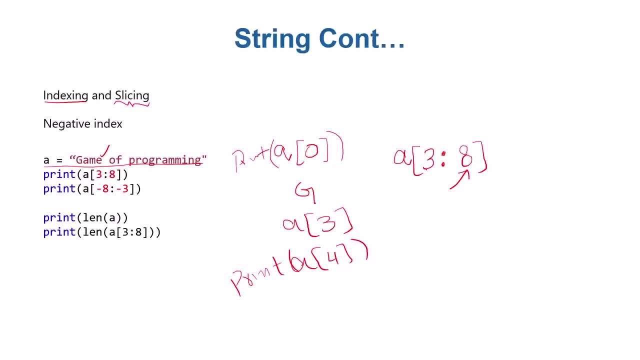 include the index 8, so it will include the corrector at index 3, which is e, corrector at index 4, which is space. let me write space in this way: corrector at index 5, which is o. corrector at index 6, next vector, which is F, then a space. 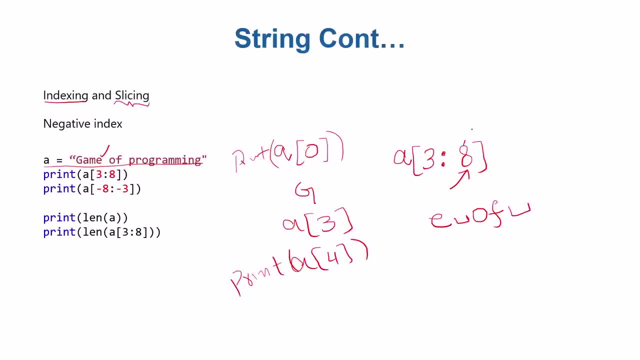 which is 7, and then the corrector at index 6, which is a space, which is 7, and then the corrector at 8, and so so this is not included, to be accessed. this is included. this is inside. this is included. this is not included. so we can access a. 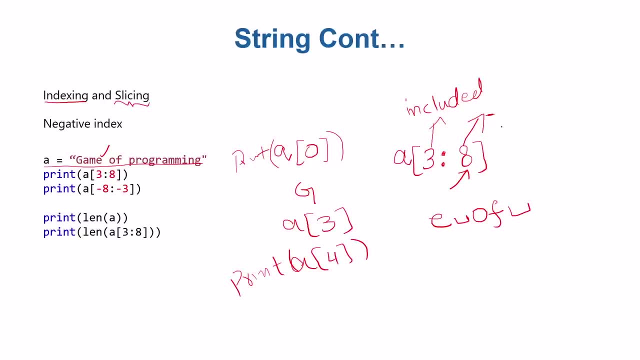 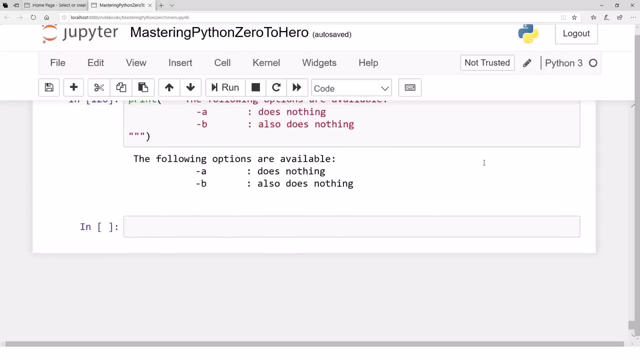 substring. so, starting from 3, ending at 8, let's see, let's see an example, and we'll come back to this slide again after, after a few minutes. so let's say we have a string s, let's say you and who are you. let's say so, let's say that's a string okay, and what we? 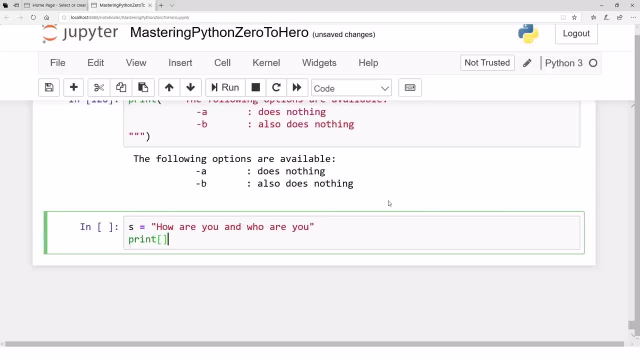 really want is. we want to access, for example, the. we want to access the element. to access the elements, you have to write the square brackets. that's a standard notation in Python. whenever you have a collection and you want to access different elements, that collection might be a string that. 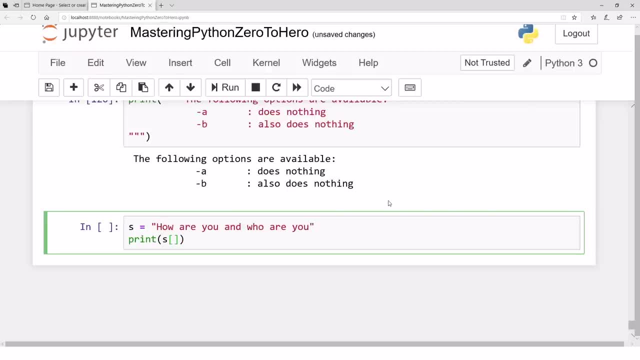 collection. later on we will receive might be a list, maybe a tuple dictionary, maybe a set, maybe an umpire, maybe a pandas structure. I mean anything that. that is a collection. normally it is accessed by if it has different elements and we want to index them. the indexing notation is: 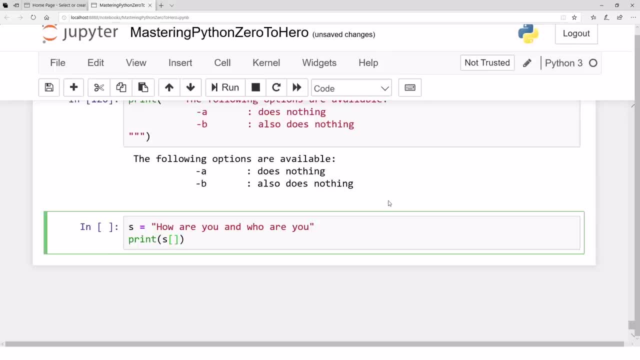 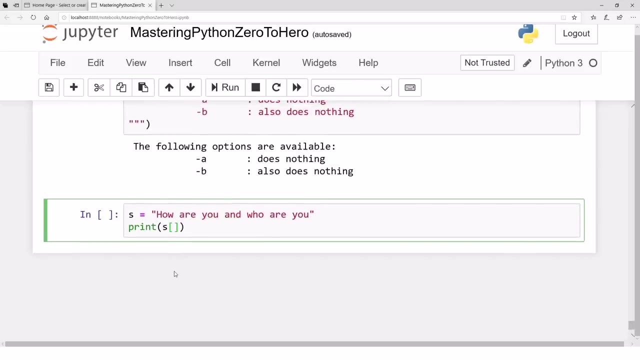 square brackets and indexing always starts from 0 rather than 1 in in Python, there are some languages in which the indexing starts from 1, for example MATLAB, the indexing starts from 1, but in Python and in several other languages there's a string that starts from 0 and the indexing starts from 0, which has some 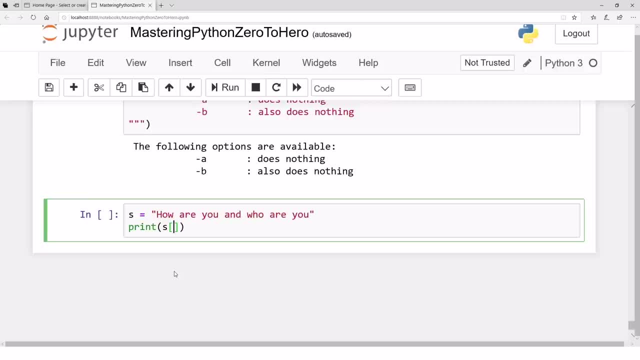 benefits over starting with 1. it has some benefits, so starting with 0 is okay, it's okay. so let's say we want to access element add index 5. the element add index 5 is actually the sixth element in the string starting from 0. so first, 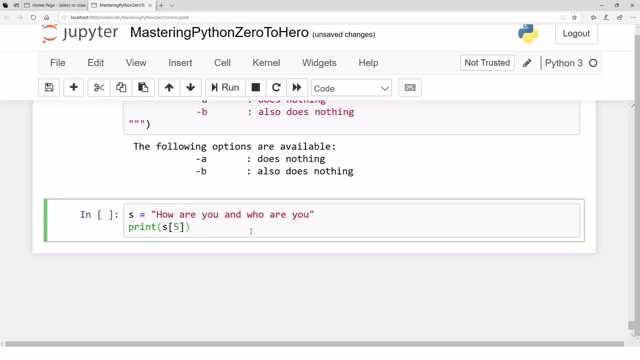 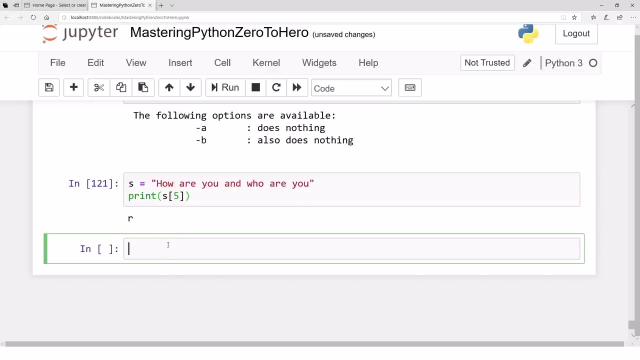 second, third, fourth, fifth, sixth, so R will be printed. so let's see, let's check the, let's check the type of this return value, let's check the type of this, this one element, which is R. what is the type of it? so, type of different elements in a string, different characters in a string, what are the? 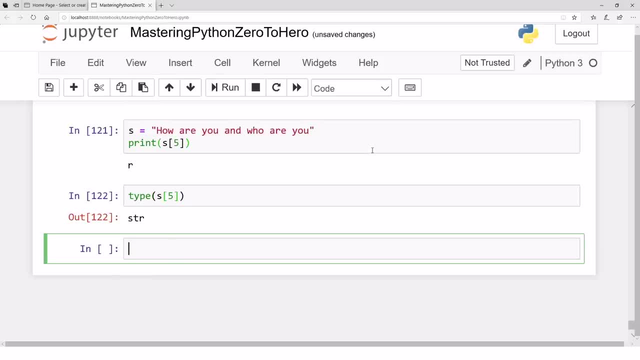 types. so what is the type of it? so the type is also string, so each and every character is also of string type. in some other languages that the type might be a correct character is another type, but in, in, in Python, each and every one character is also a string. more than one characters is also string, as long as they are. 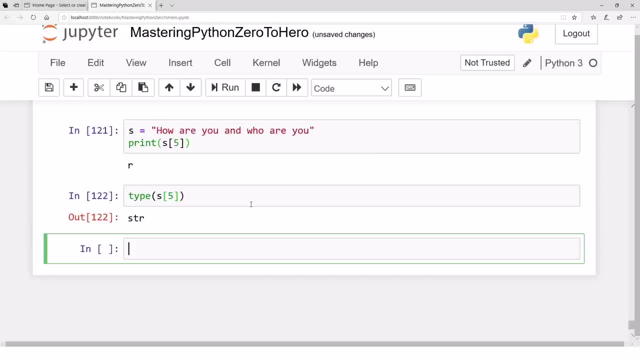 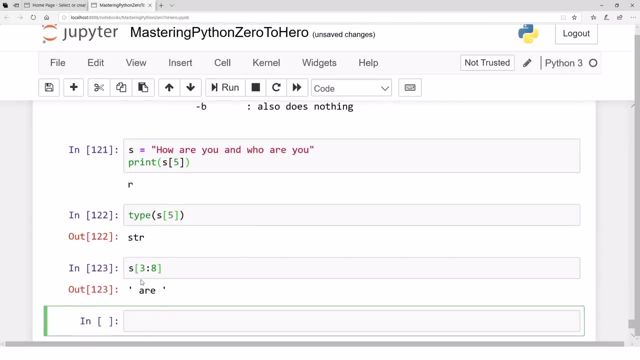 accessed from a string. okay, let's access, for example, the element number three, two element number, let's say eight, so the result is R. so element number three, oh, not three, actually starting from three, which means the fourth character, which is space, and then E or E, and then 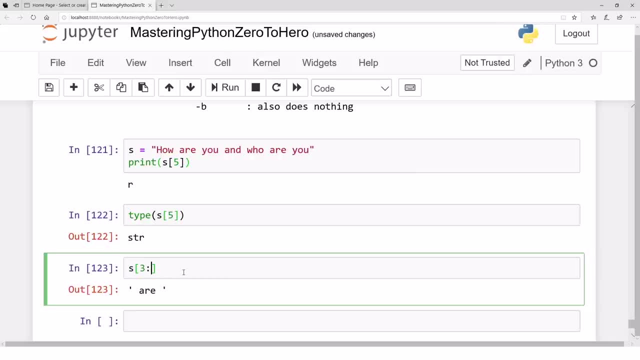 space, and then then we finish. if you, for example, move to from three to nine, let's say, and the, the value will be ry. or we may move to from, for example, we may start from the very beginning. so, for example, index zero, we may end at the index 10, but not including the 10.. 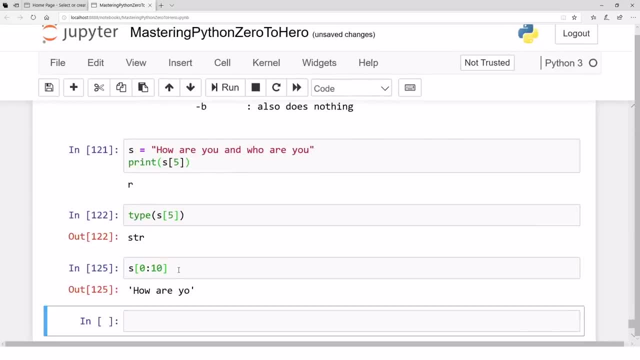 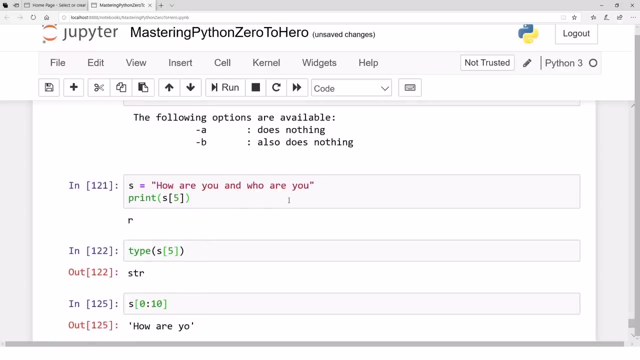 so the result is: how are you? and then I mean, why, oh, and not the you included, because that's index number 10 and index number 10, the last index is not included. great, uh, we can have negative indices in strings as well. so a negative index is just, uh, just the indexing from the right side, not from. 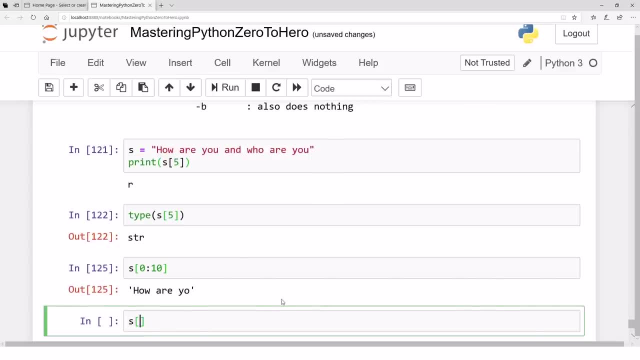 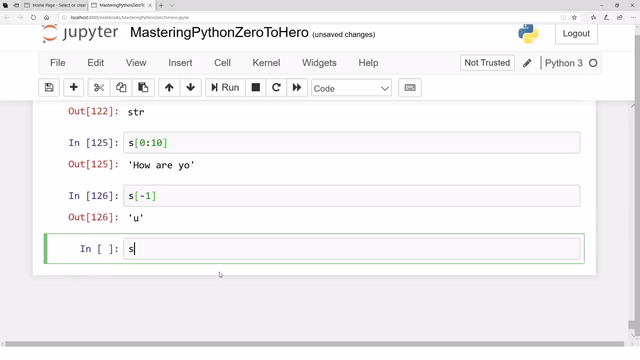 the left side, for example, a negative index, uh, so minus one points to the last corrector, for example. similarly minus two points to the second last corrector, and so on. so minus one, let's say it will access you. and similarly we have uh minus three, and that will access Y, or we may have start. 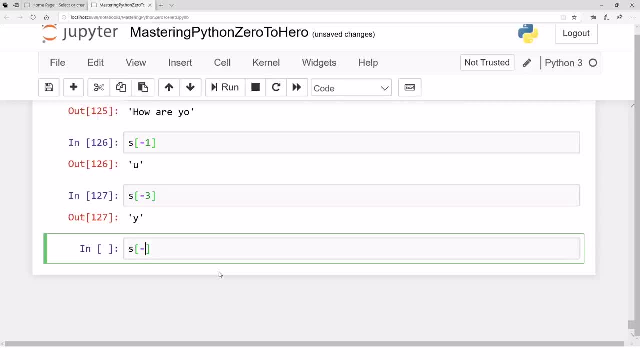 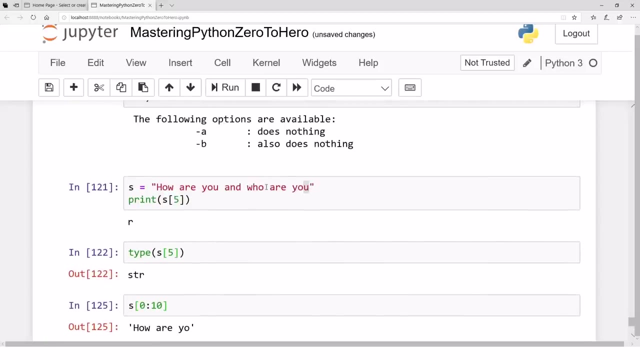 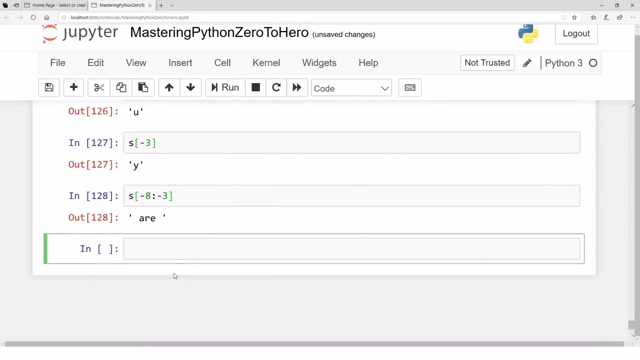 from let's say minus um. start from let's say minus uh, eight and go till minus three. that means go back to go back to minus eight index and then move to minus three index. okay, and minus three in this case. let's see what. what's the result are? what is that? why are? oh, this? 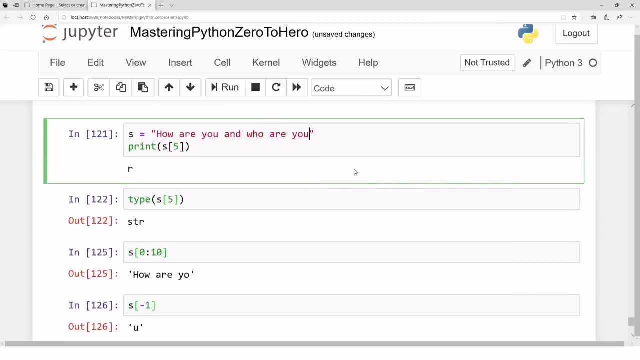 are. I guess this are. let's check it out. uh, so this is this you. this is minus one minus two, minus three, that's index number three. so three is not included, minus three is not included, so it has to stop here. okay, that's uh, minus four minus five, minus six, minus seven and minus eight. oh great, so that should. 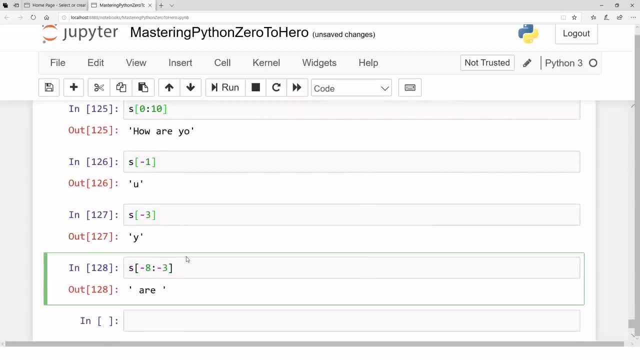 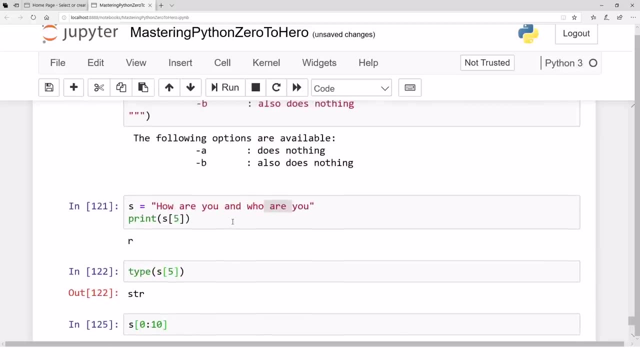 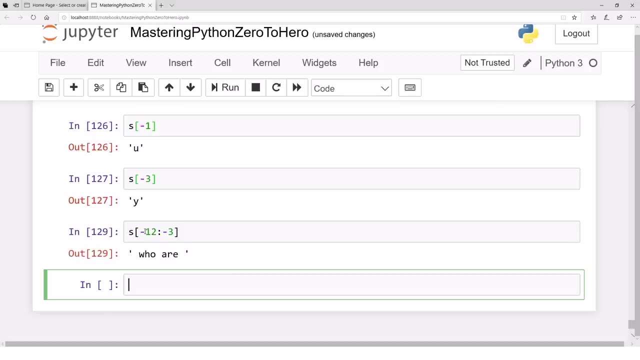 be printed. it has printed. so let's say, we have, rather than minus eight, we start from minus 12 and we reach to minus three. so who are? okay, great, so we have negative indices as well. um, and, by the way, this kind of fetching, this kind of substring. 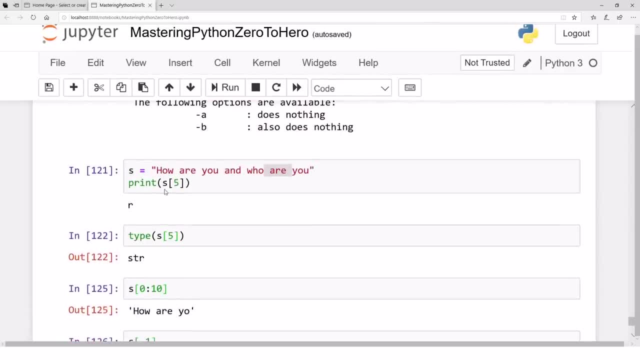 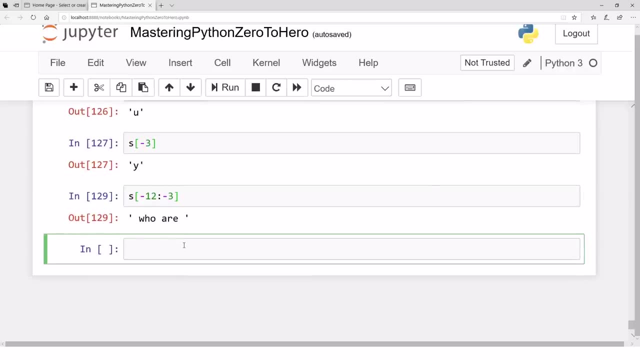 is sometimes called uh slicing. I mean, we are just fetching the slicing, although the term slicing is much more popular in in in mutable data structures. uh, what? what is a mutable data structure? what is a immutable data structure? well, um, yeah, I should tell you right now you. 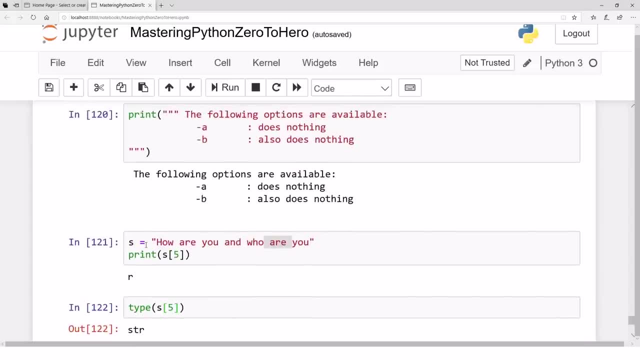 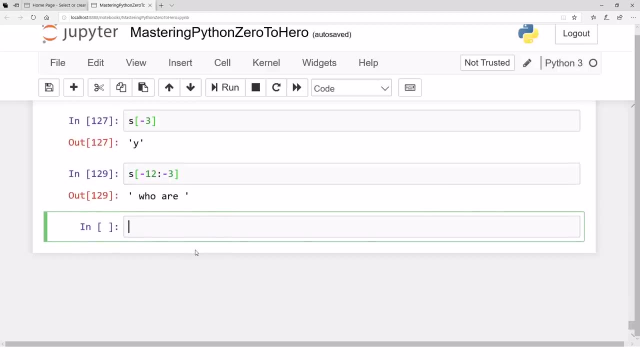 can change. you cannot change um any corrector in the string. um that might. that might look like a bad news for you, but once the string is created, the elements in the strings are not changeable. so for example, let's say, at position number one you want to place a corrector. let's say E, that's. 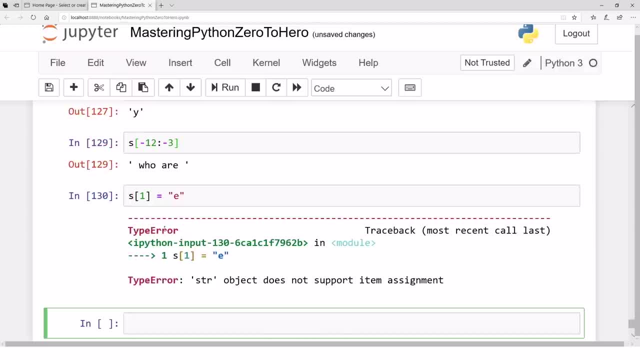 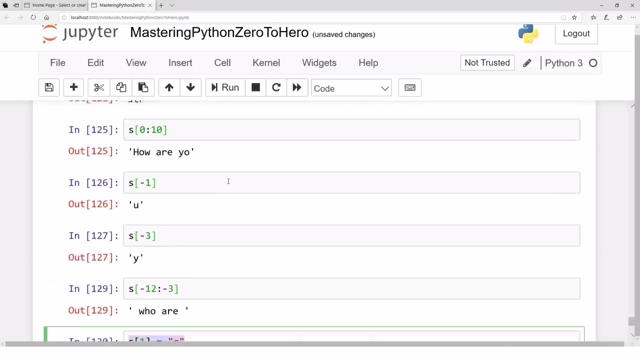 not possible, and the reason is: the string is a data structure, the string is a variable type, a data type that is immutable. immutable or unchangeable once created, you cannot change its contents. they stay fixed. you cannot change them, you cannot alter them, you you cannot delete. 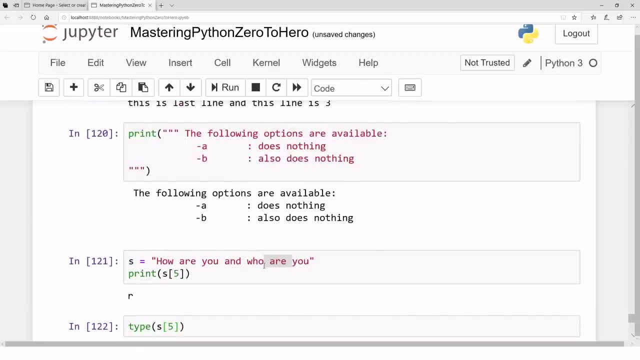 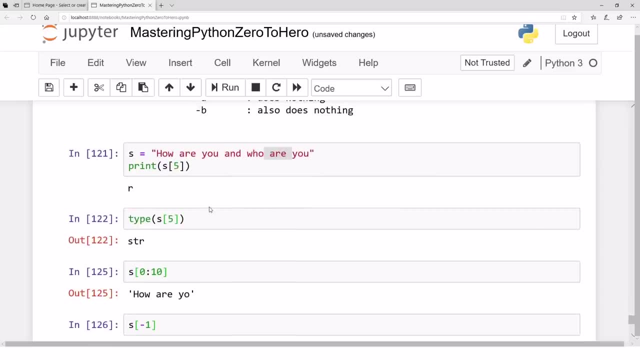 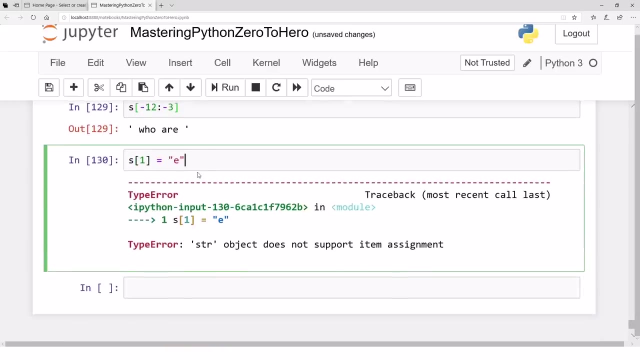 certain contents from it. I mean, once created, it stays as it is. you can copy this into another string, you can copy and paste. but you can get a substring and copy into another variable, for example, but the contents of S cannot be changed. so all the kind of data types in Python that are 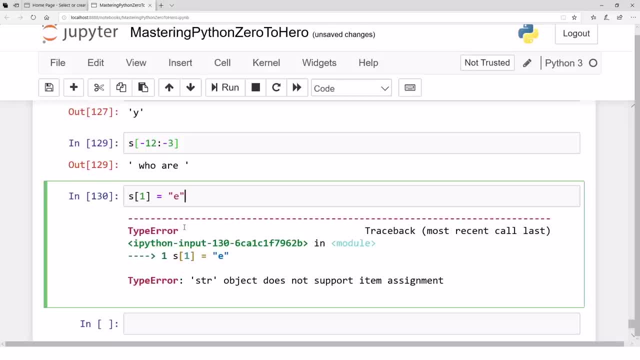 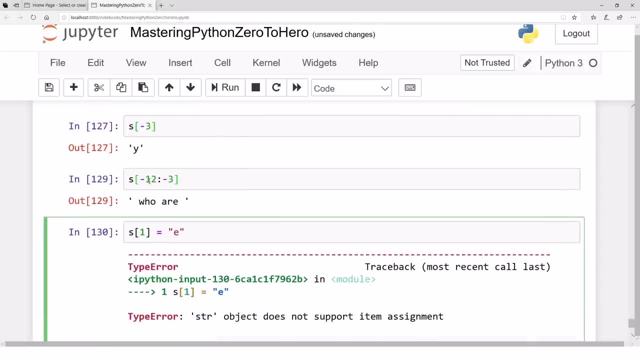 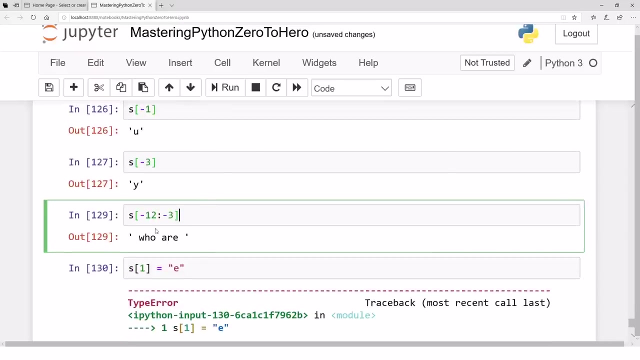 unchangeable. the contents are not changeable, um, so so the the the term slicing makes much more uh, I mean sense or it. it is more popular in the data structures that are mutable, um, that are mutable, although you can use term slicing, indexing, both interchangeably, but it refers to roughly, it refers to uh, fetching a substructure or substring. 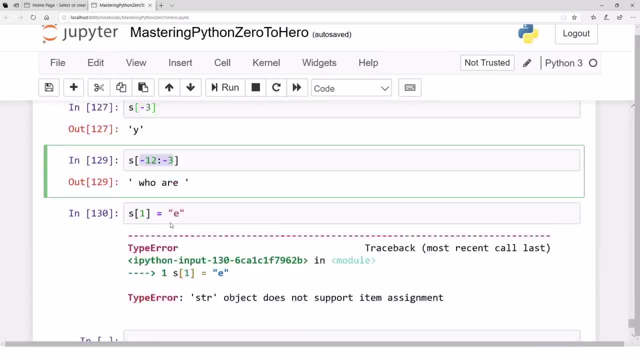 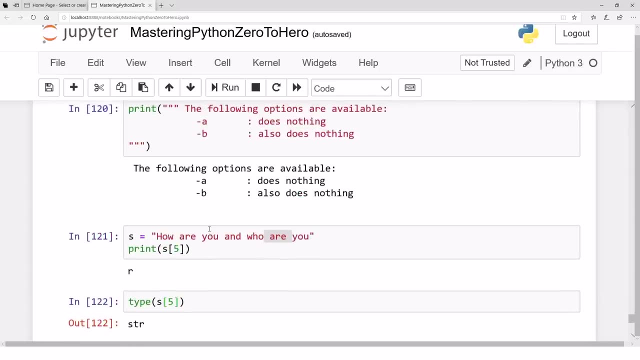 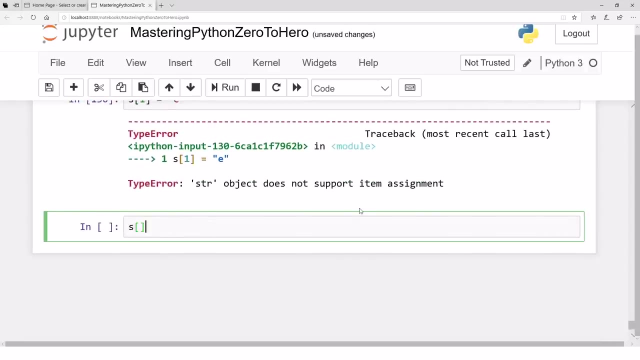 in this case in the list, it will be a sub list or so on. so that's what slicing is. yeah, um, great. why don't we do some more fun with the string? yeah, let me show you more fun with the string, more indexing. let's say, you start at index zero, you go to index. 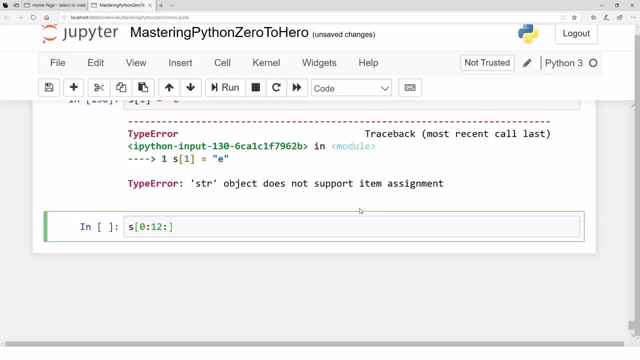 12, but not including 12.. and then you jump. you take a jump of two rather than one. what will it do is it will fetch all the correctors starting from index zero all the way to index 12, but not including 12.. but it will take a jump of two rather than taking a. 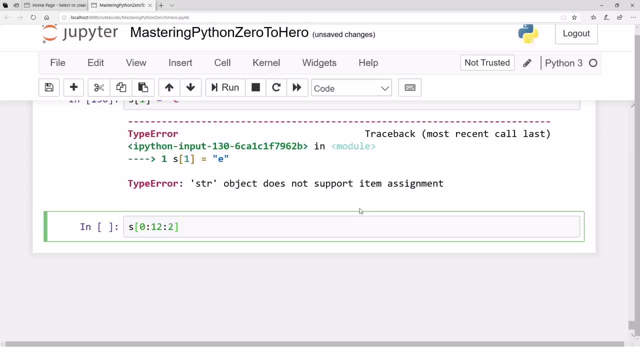 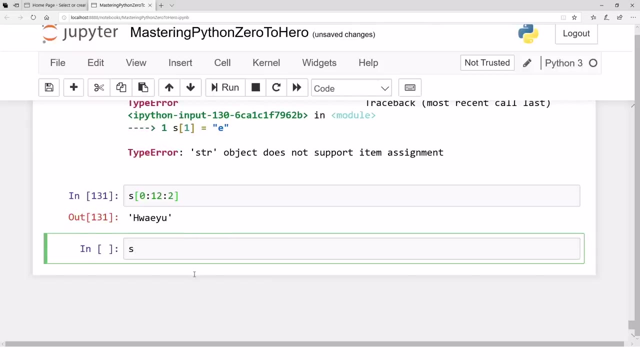 jump of two. so first character, then take a jump of two, then pick a character, then take a jump of two and then pick a character, so it will actually pick every other character starting from zero. so let's see that. so, for example, if you remember the string, that's the string, so it starts from H. fine, then it. 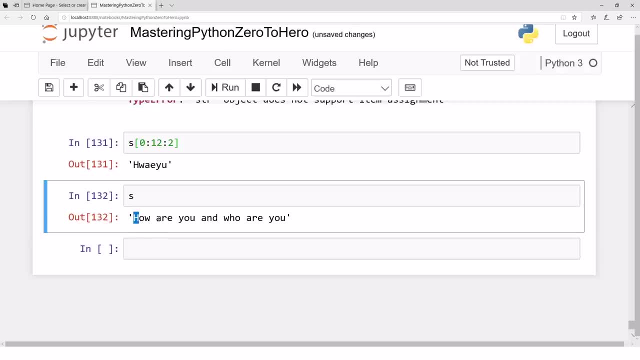 skips O and go to W, then it skips space and go to A, then it skips R and go to E, then it skips space and go to U, and then it skips O and go to U, and then the 12th achieved and we stop there. wow, so the the general. 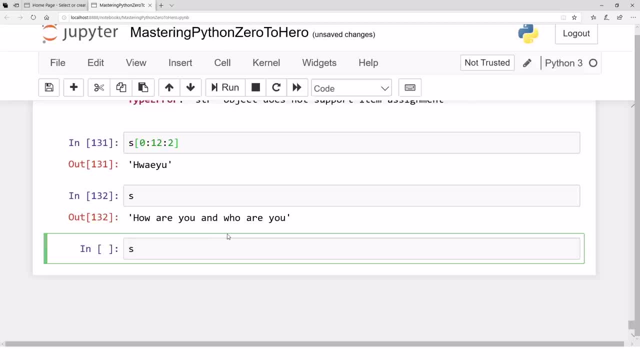 way of slicing or indexing. the general way is you have a start index, start, then you have end index and then you have a step size. if you do not mention the step size, the step size by default is one that we were doing already. if you do not mention the end, the default end is the till, the 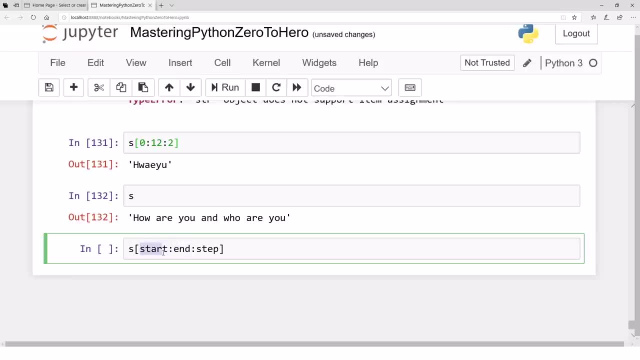 end the total list size. if you do not mention the start, the default start is zero, for example. let me make that a comment and just practice a few. for example, let's start from zero. we do not mention the start. let's start from zero and go to 12.. if you do not mention the starting index, that 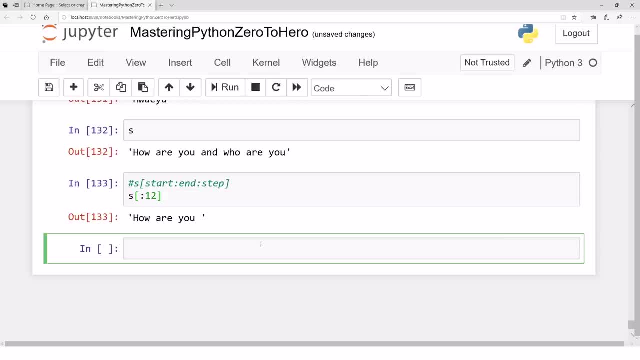 starts from the very beginning: zero, go to the 12th. okay, great, if we do not mention. for example, we start from three and we do not mention the end. that means go till the end, starting from index three, including the last character. okay, if we do not mention the step. for example, if you start from one, go to 12, and we do. 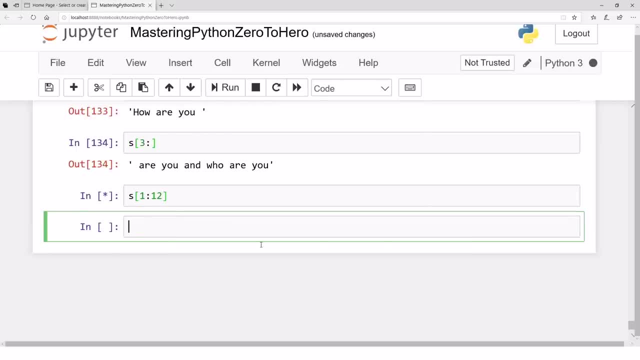 not mention the step. the default step is one. okay, there's one way of reversing the string. I mean very beautiful way. I mean you do not, you do not start the mention and you do not mention the start, you do not mention the end, and then just take a. 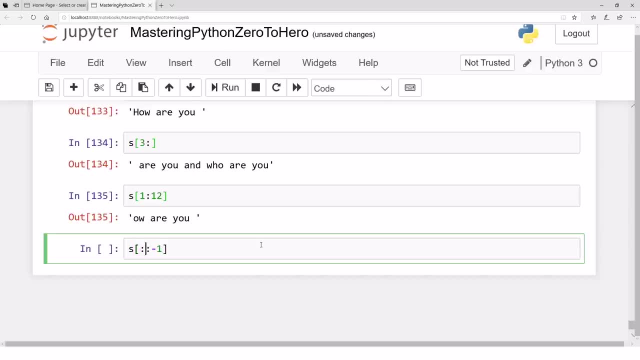 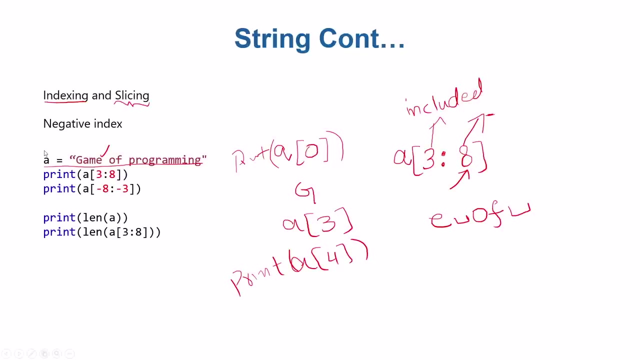 step of minus one. in this particular way, the star and end index they are. they are just swept and you get the string reversed way. wow, so that's the reverse string. isn't that fancy? yes, it is okay. a lot about indexing. you can find out the length of any string by using len function. you can find out the length. 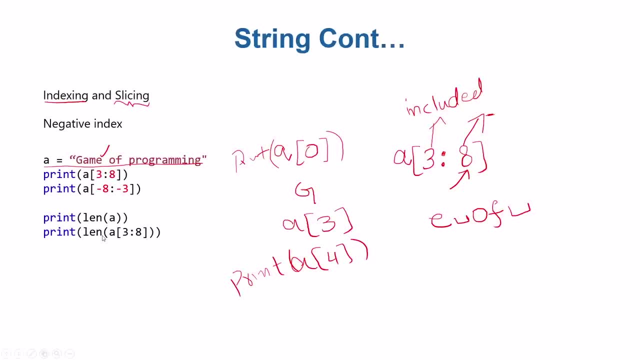 of any substring if you want to. if you have a substring using, again, a length function, alien, that's okay. okay, now we have seen how to access substrings and how we cannot change the elements of a string because it is immutable, but we can access them. we can access them, we can. 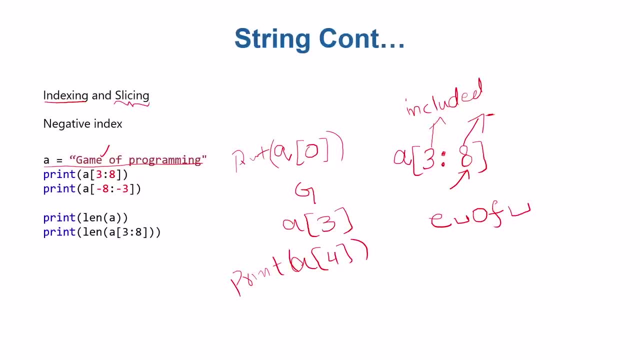 just display them, we can analyze them, and so on. in the next video we will see, uh, some functions that are supplied for string processing, what we can do with strings, and I mean, how can we manipulate the those strings? although we cannot manipulate the contents of a string, but we may copy a string, we may get a string, manipulate it and save it to another. 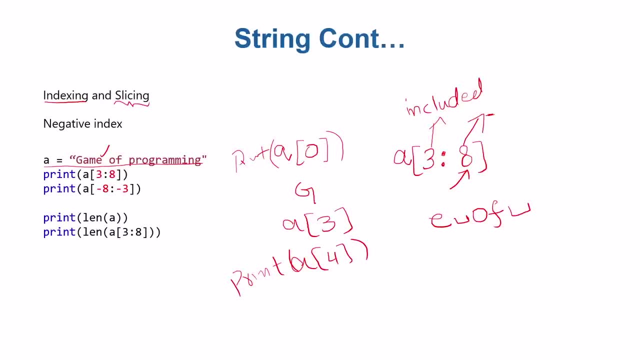 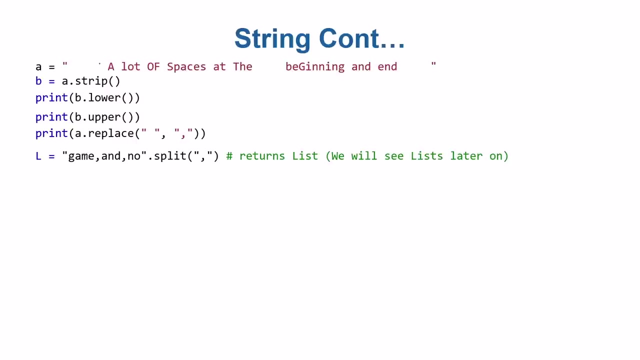 variable and how, what kind of functions that are available in string in string data structure, string data type. so let's see that in the next video. hope to see you in the next video. okay, let's see different functions that are available to play with the strings in in this string data structure. 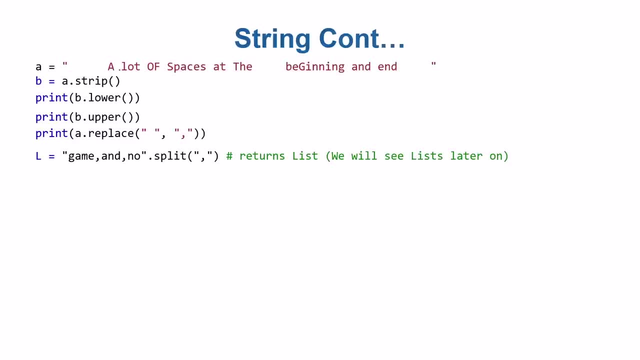 let's say you have the string a, a lot of spaces. these are a lot of spaces at the beginning and these are a lot of spaces at the end. there are some spaces in the middle as well. so there is one function called strip, all the functions of the string. they are called by taking a dot, a dot. 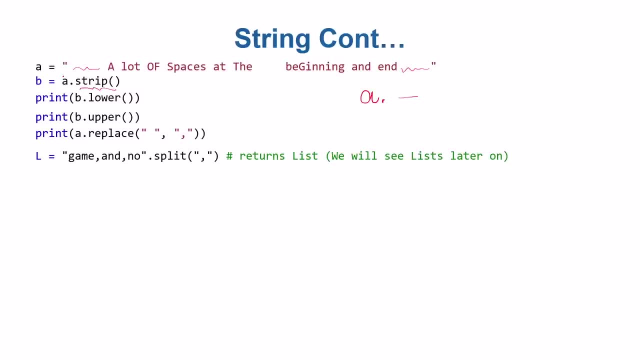 you, you, you can loosely call them functions, but, um, those kind of functions that are related to some data structure and called with dot, they are sometimes called methods. uh, the. the term method is more related to object-oriented programming. actually, string is a class, so all these are. 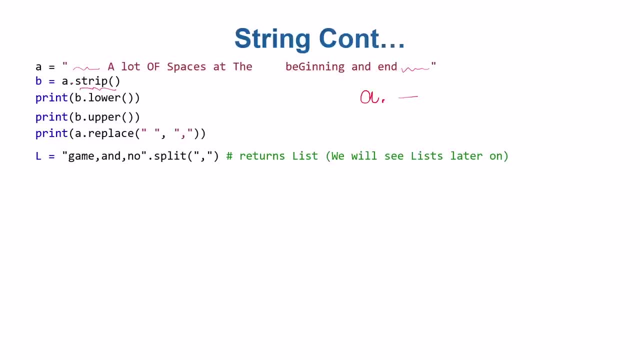 the methods. but even without knowing that, it's perfectly okay. you can call it method or function. that's perfectly okay. you can. I mean it's okay. it's okay without knowing what a class is, without knowing what an object-oriented programming is? this a dot, some function that operates on this? a? 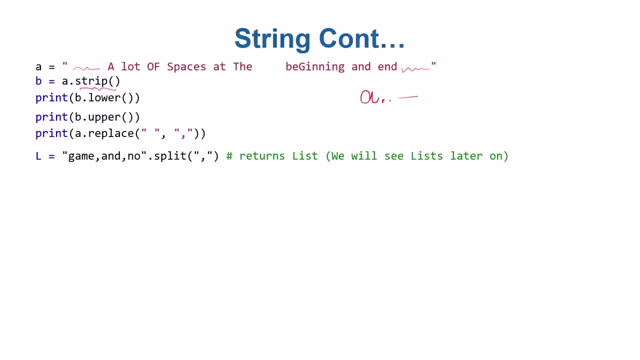 um, one difference with method and function is when you call a function with a dot and you call some function, let's say a dot strip, then inside the definition of the function, this a object or the, a variable is available, like, like, you have passed that variable as an input argument, that's. 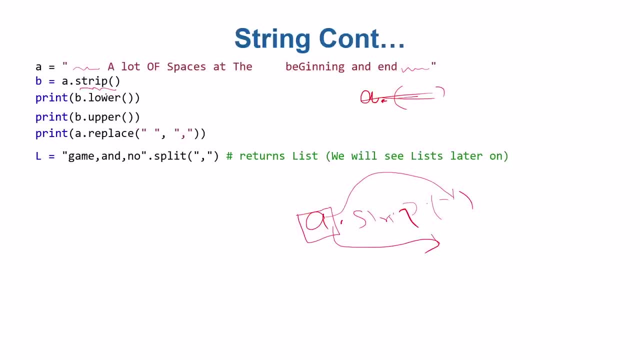 all you need to know, uh, about the difference of method and function. the rest of the story, um, is perfectly okay, even if you don't know, that's, that's fine. okay, a dot strip. it operates on a, which means the a is passed in this function as just as input argument, or it is available there inside the function implementation. 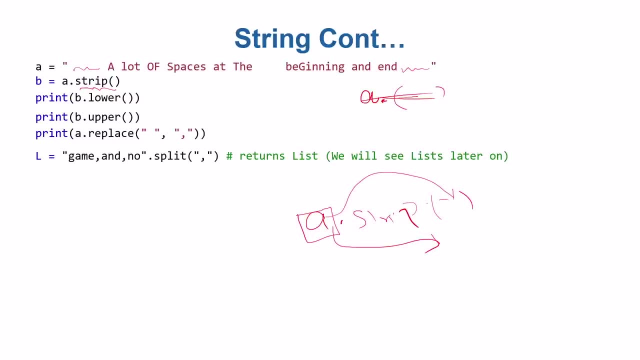 and then the strip function. what it does is it removes all the spaces that are in the beginning and removes all the spaces that are at the end and returns another string that has that has no spaces at the beginning and no spaces at the end, and the new string is: 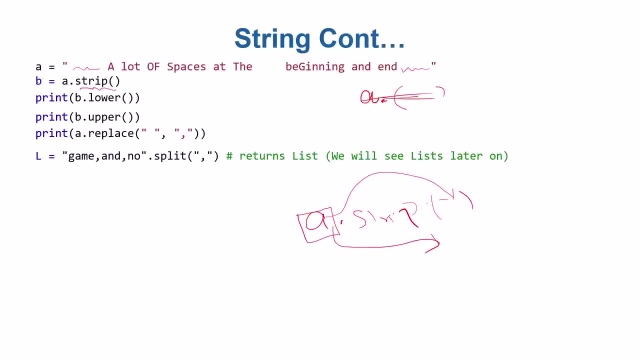 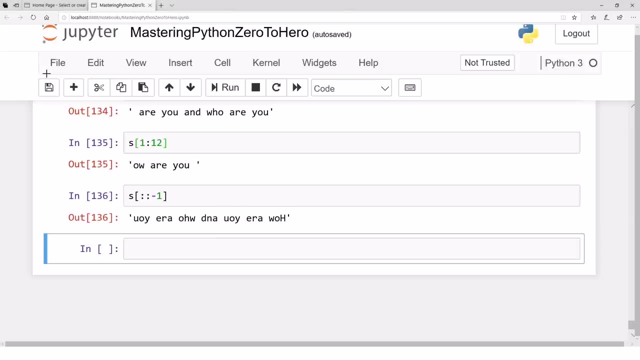 copied or created in a variable B. let's say: whatever that variable, we can, we can have another name of that variable. so let's see, uh, let's see the running form of this strip function in our friend Jupiter notebook. so let's say a is a string variable. let's say a lot of spaces: a, b, c, d, e, f, a. 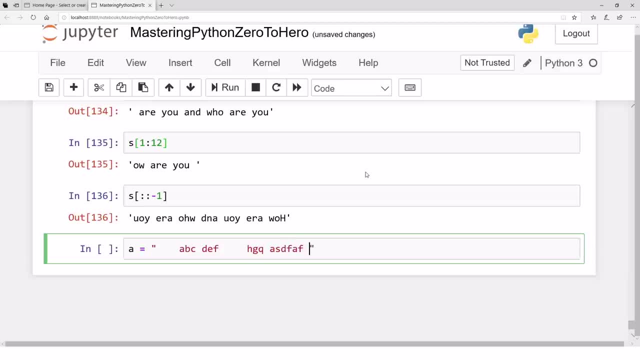 spaces, then h, g, q and whatever, and then a lot of spaces. let's say this is a, and then we have b. let's say a dot strip, okay, and that's print b. so b is, uh, actually everything without spaces, without the starting spaces and without the ending spaces. it does not hurt the spaces. 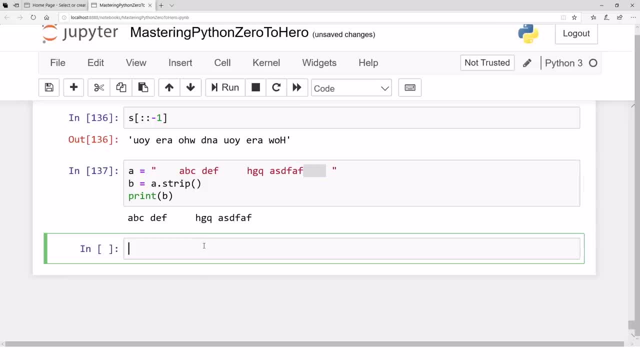 inside. so that's a strip function, sometimes processing the data. when we, when we read the data from a file, it may have a lot of spaces at the beginning, at the end, maybe due to formatting issues or something like so- and it is. this function is available if we want to remove. 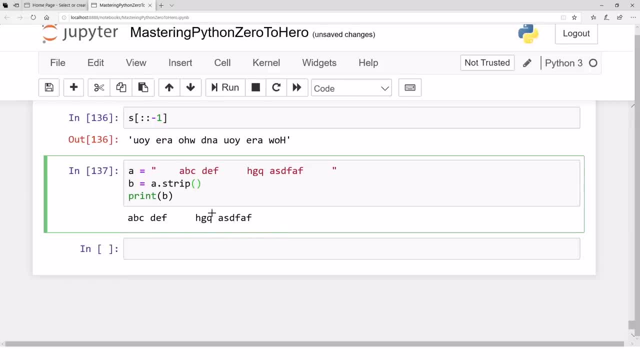 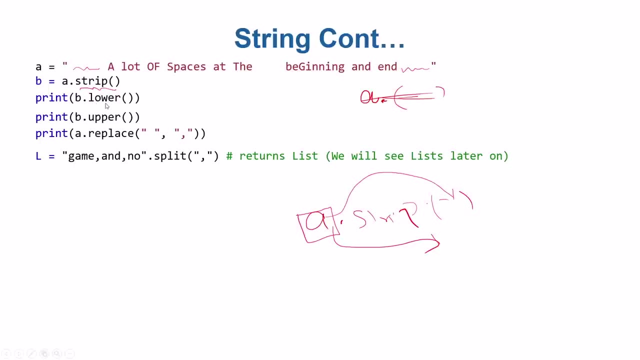 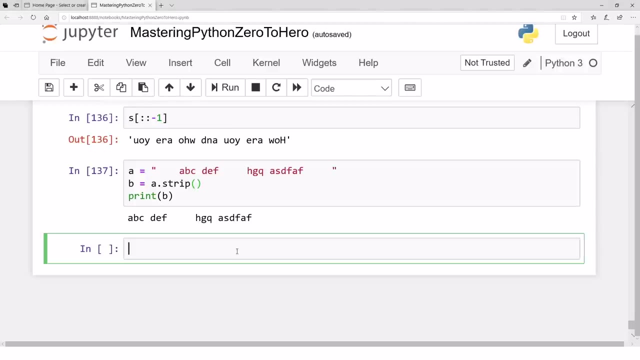 those spaces from beginning or from the end. let's see more functions. another function is lower, like the name suggests it. actually, it actually converts all the string to lower case. for example, let's say we have a string. let's say a, b. let's say we have a string a. 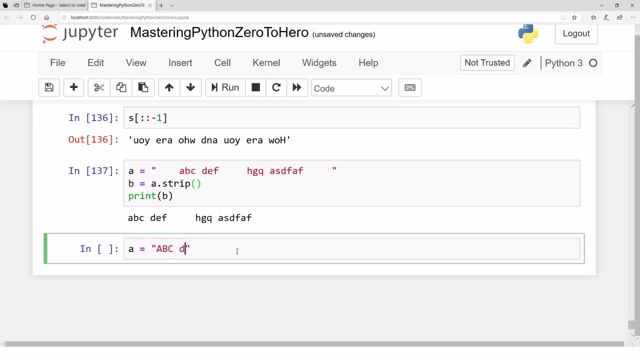 equals a, b, c, d, e, f, g and some correctors, some other correctors and q, f. let's say that's a string. and now what we do is b equals a dot lower. what it does is it converts all the string to lower case for the correctors that are already in lower case. it doesn't hurt it for the correctors. 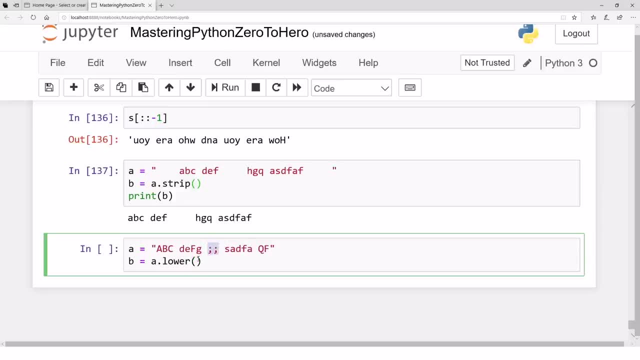 that has nothing to do with lower or upper case. it doesn't hurt that. all the characters that are not in the lower case and can be converted to lower case, those are converted to lower case and this is available, yeah, great. so similarly, we have another function called upper, for example. 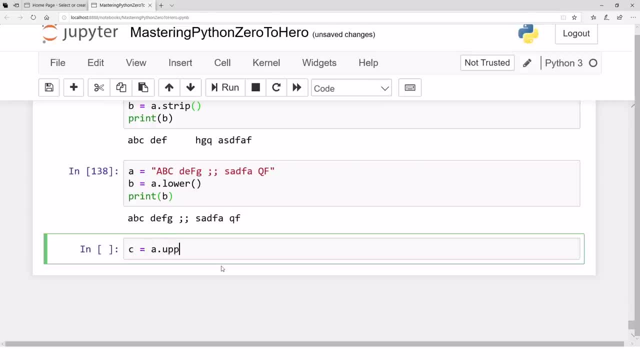 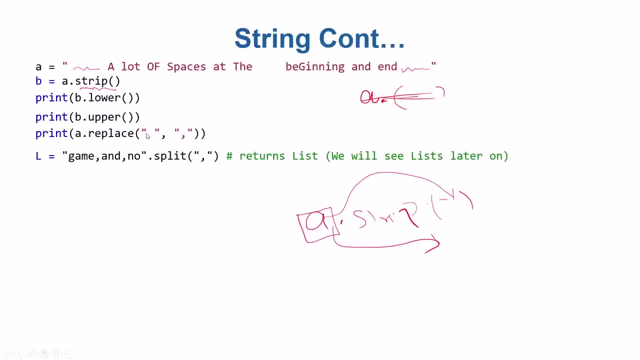 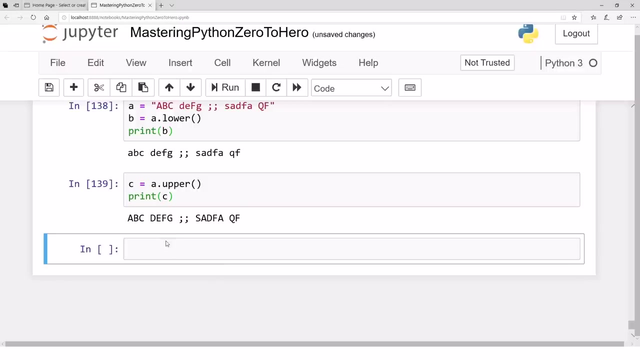 c is equal to a dot upper that, like the name suggests, it converts all the characters to upper case. wow, let's see more functions. oh, there is a function: replace the replace function. what it does is it takes a substring and replaces that substring with another substring. okay, let's see it. for example, let's say: we have, we want to, we have. 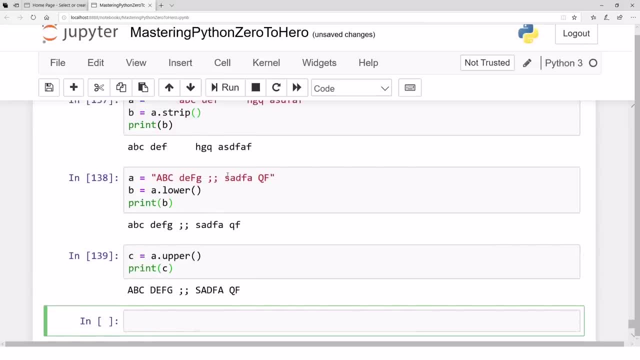 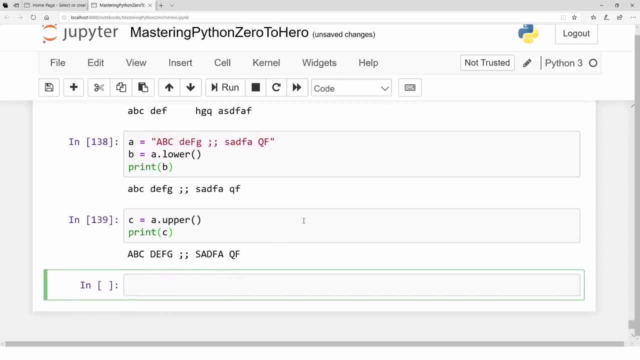 the same a. let's say the a is: uh, this thing. let's say that's a, and what we want to do is we want to replace the semicolons. let's say with, uh, with, with the semicolon. we want to replace the semicolons. 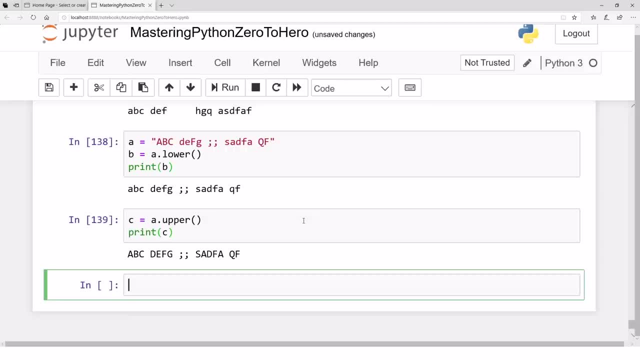 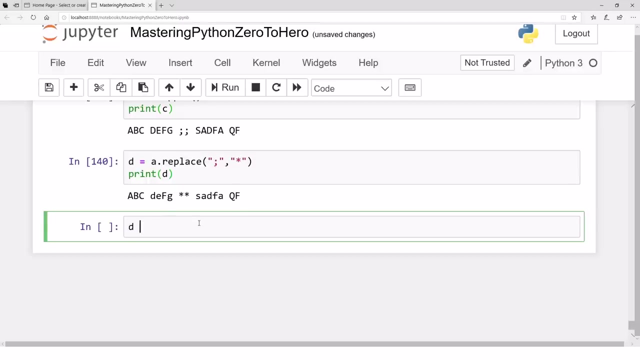 with hysterics. so what we can do is we can say, okay, d equals a dot, replace um, replace the semicolon with uh, with, let's say, hysteric, or yeah. so let's see what d is. so each semicolon is replaced by a static. by the way, if you, if you want to replace, for example, a, 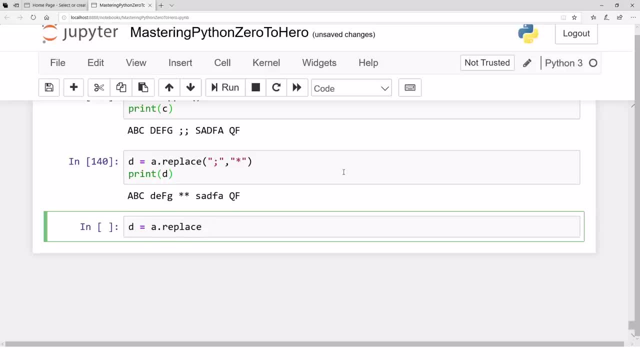 a dot replace. if you want to replace one, is there one semicolon, one semicolon with a string. for example, the string is star, star and and hat hat person person. that semicolon will be replaced by this, with this string, and the other semicolon will also be. 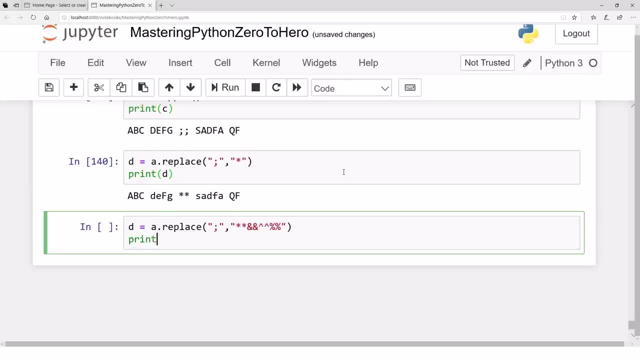 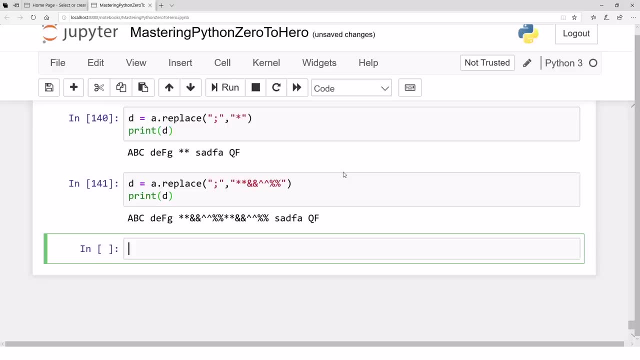 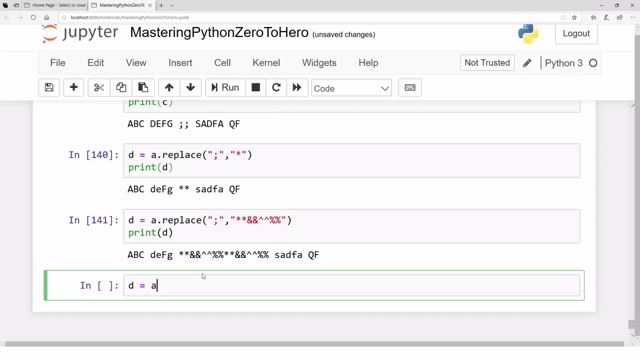 replaced by the string and the result will be as expected. each semicolon will be replaced by the string and that's the result, what it is. further, if you want, for example, um, if you want, for example, let's say, d equals a dot, replace, if you want, this particular substring. 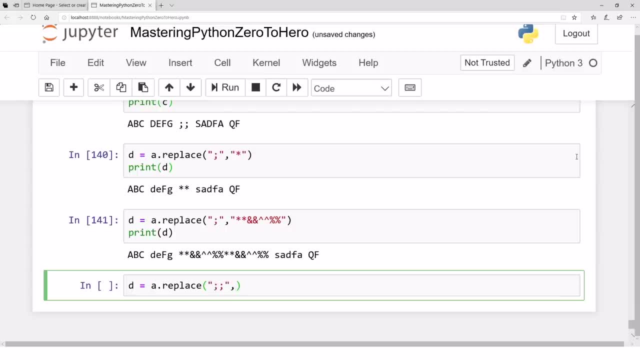 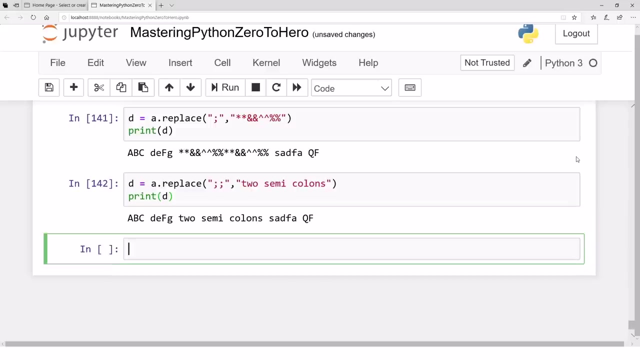 that contains the two semicolons. if you want the two semicolons to be replaced by another substring, let's say two semicolons, that's it, and that is also possible. I mean you, you replace one substring with another one. yeah, great, there is one more function called split. um, that what it does. 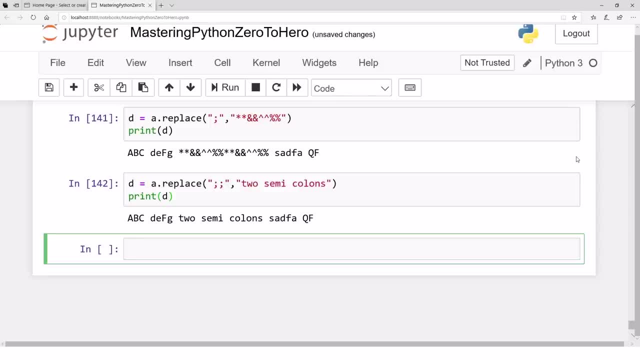 what? what the split does is uh, um, for example, you have a string, for example um. let's say a equals a string. let's say a, b, c, then you have this colon, then you have d, e, f, then you have semicolon, then you have h, g, y, this then. 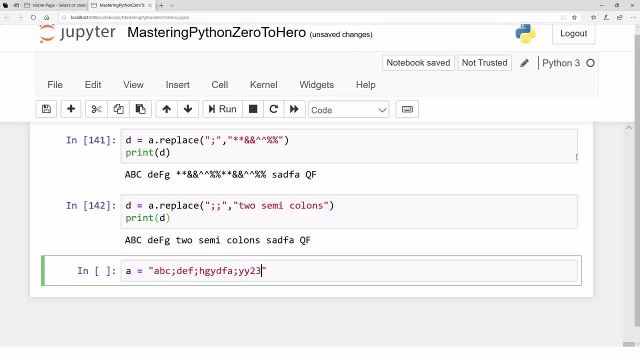 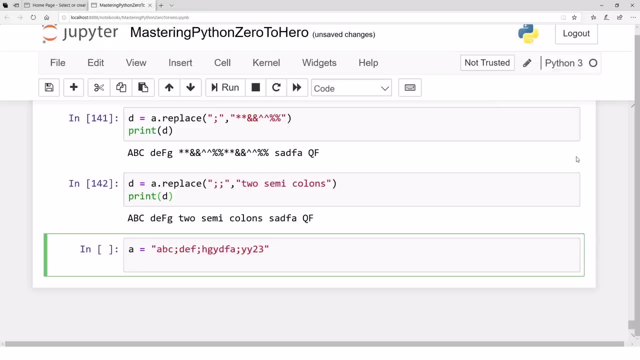 semicolon. then you have y, y, 3, 2, 2, 3, and that's it. that's your string. uh, let's say you read that string from some CSV file and this appears: and now what you want? you want all these uh values to be separated out, that are that? that? 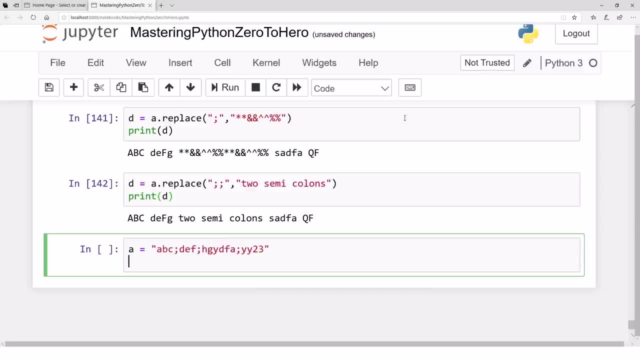 are separated by the semicolon. maybe these are different values. ABC is a different value, then it is separated by a semicolon. semicolon may be an indication or token that the next value started, and and so on. let's say you want to separate them. let's say you want to just split them, all of them. 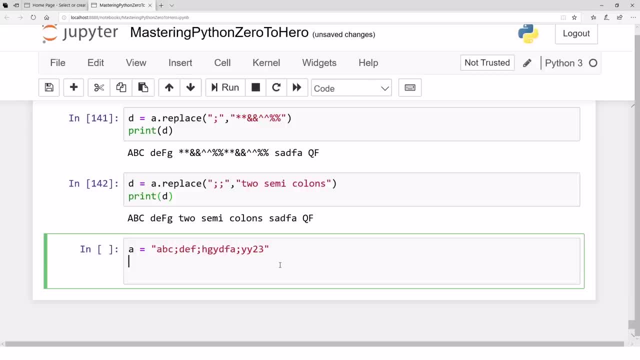 with a particular splitter and here, let's say, the splitter is semicolon. so what you can do is you can have a list and a dot split and in the split you can specify the corrector that, uh, that is used for splitting after and before we split that and remember the split. 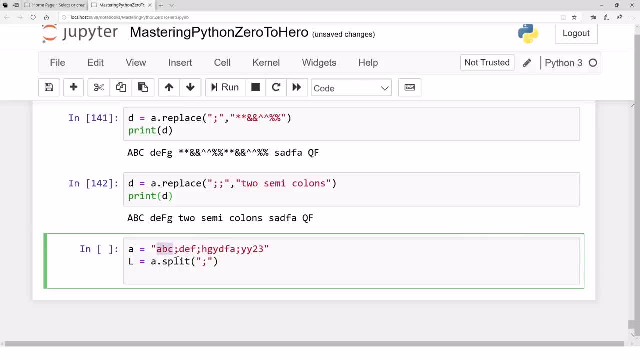 function actually returns a list of strings, where this is the first element of the list, this is the second element of the list, this is the third element of the list, this is the fourth element of the list, and so on, because once you will split, uh, you will be having different elements. 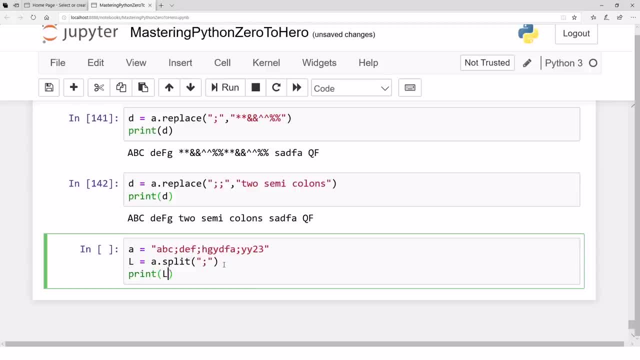 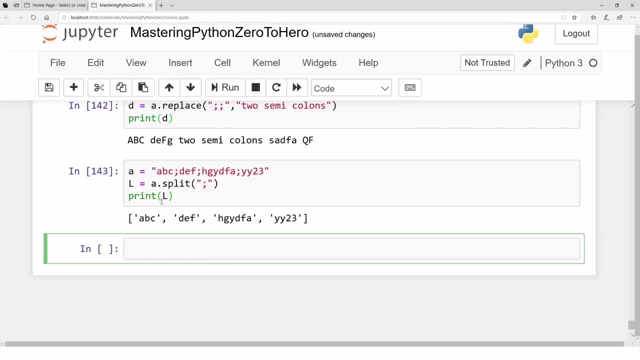 that are splitted out. so if you print, for example, L, you will be having a list of different strings, ABC and all that. oh, don't worry about this single code. the single code and double code is the same thing. now we can access, for example, the third element, or or maybe the second element, by index. 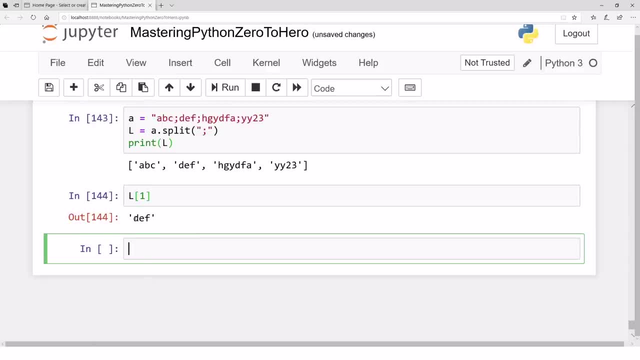 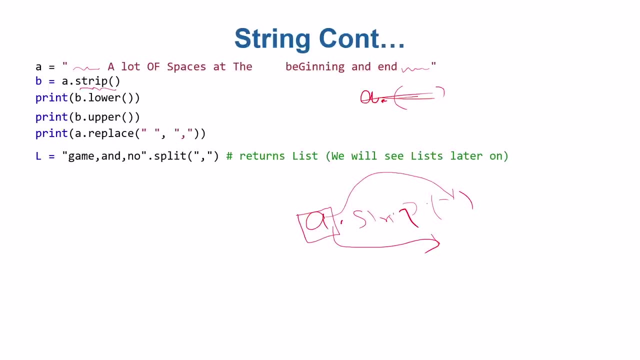 one. and the second element here is def and we can work more on that. okay, um, is that it? I mean, are there any available strip function, lower upper, replace and split function, or is that it? that's all the string is about. uh, maybe there are more functions. uh, how many functions are there in? 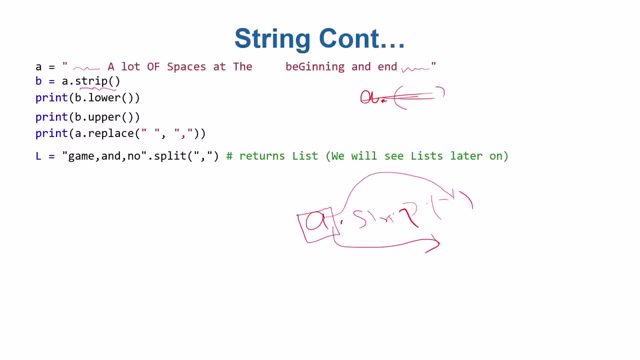 string. how can we use them? what are the? what are the total number of functions? where is the list? where is the documentation? should should we follow some book? should we go to some tutorial and find all the string functions and see how to use them? well, if you want. 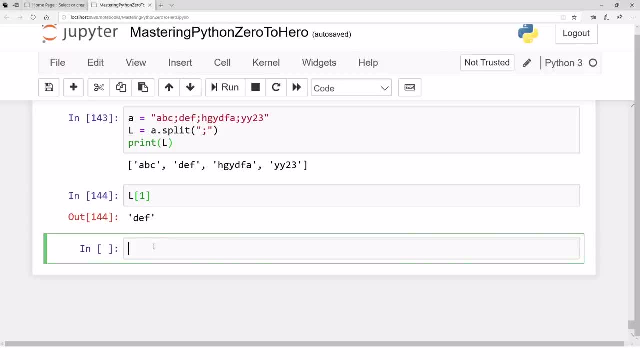 to do that. you can do that. but there is another smart way. let's say, a is a string that you know. you write a dot and then a press tab and all the things that the that are there in in string, they will, they will appear in front of you. I mean several things. you can go to this. you can go. 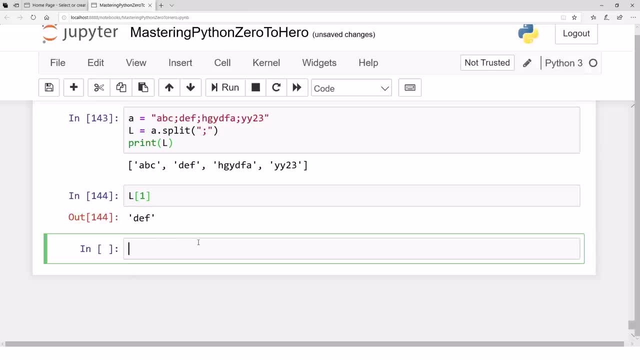 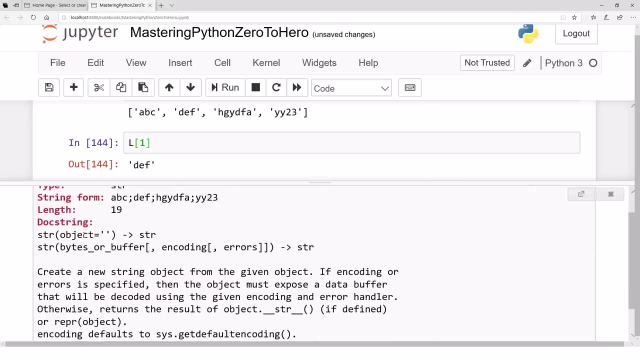 to that, you can go to that and so on. so just you can check the documentation of a, for example, if you, if you press a, then what it does, let's see it's a string object and all that stuff. fine, it's string. so further what we can do: 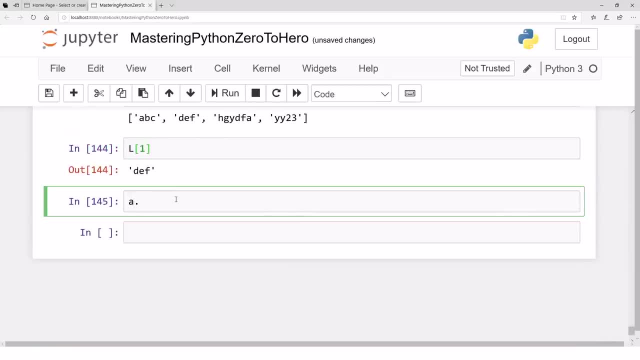 so let's say a dot, we press a and then we press tab. is there anything that starts from a? no. is there anything that starts from B? no. is there anything that starts from C? yes, capitalize, case, fold, Center, count. these are the functions that are available that starts from C. okay, let's focus on capitalize. okay, what is that thing? how? 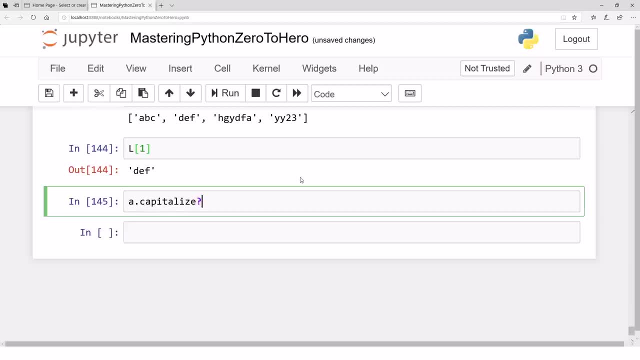 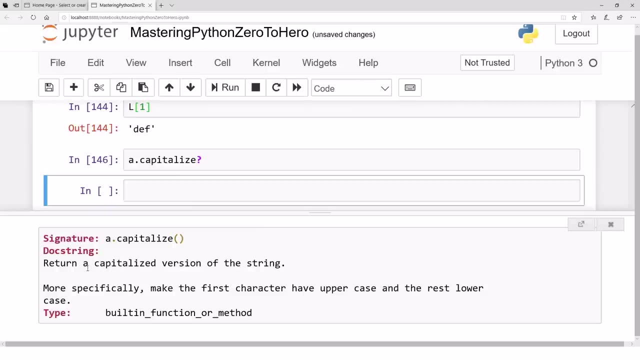 to use it. let's press colon, uh, question mark and see what this is and what it does. okay, so here is the documentation. here is a dog. string returns a capitalized variant of the string. capitalized variant of the string. is that the same as upper? maybe, so let's see. now we know what it is. 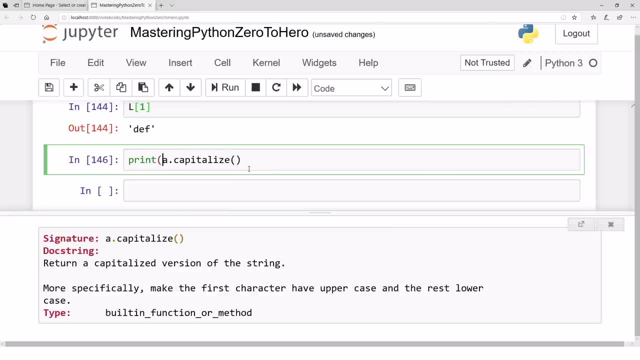 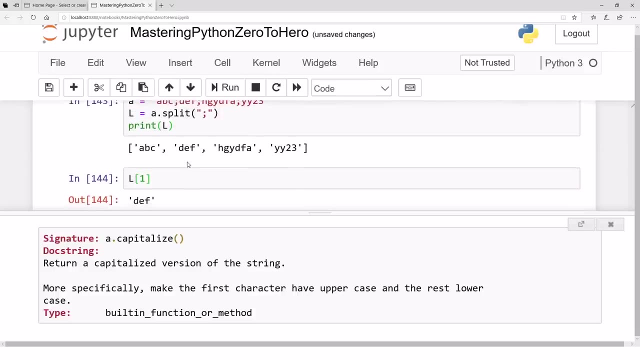 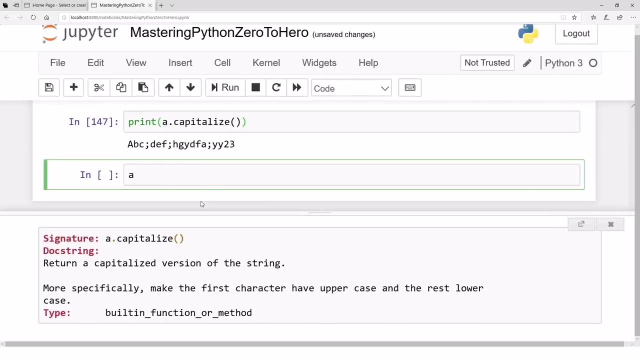 does. let's just check it out. print a capitalized and see what's the result. oh, it's kept. oh, no, it does not capitalize the whole string, does it? uh, the the the string a was. it does not capitalize the whole string. um, what? what is a? let's see what is a. a is the following string: 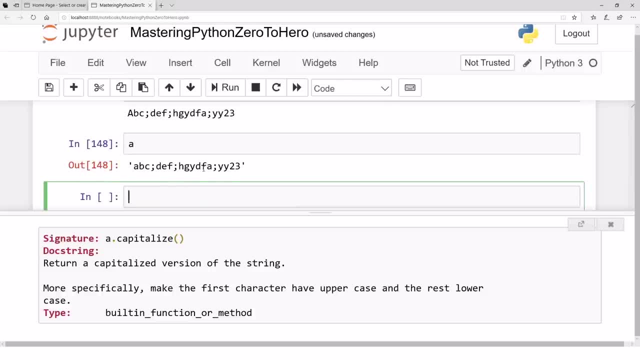 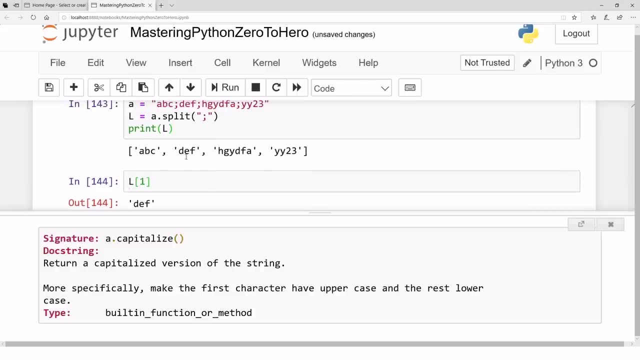 a is the following string, so it does not capitalize the whole string. oh, the difference between the capitalize maybe and the upper is that the capitalize when it encounters- uh, when it encounters no, no, no, capitalize just capitalizes the first character. let me, let me read the doc. 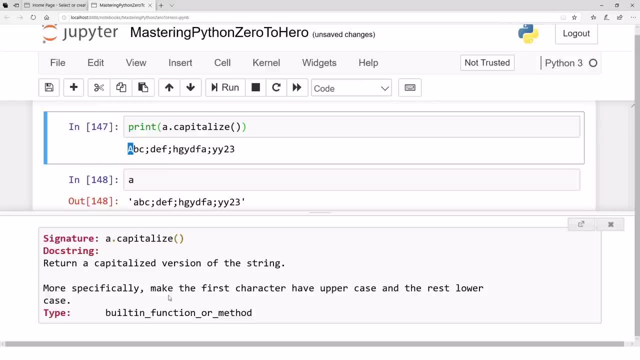 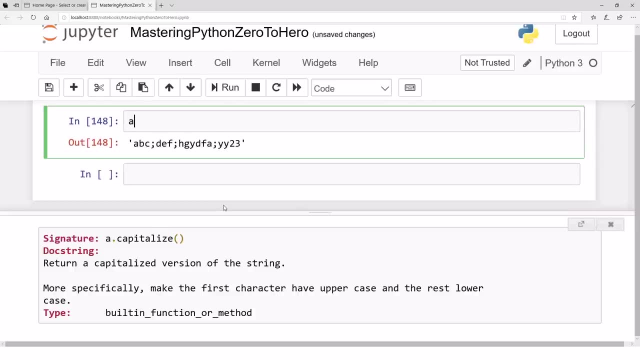 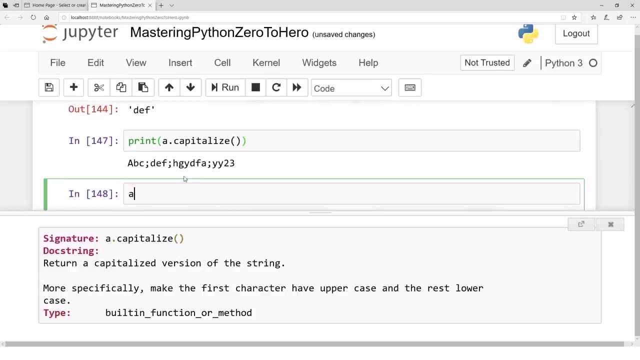 string again returns a capitalized variant of the string. more specifically, make the first character have upper and lower strings so it does not capitalize the whole string. oh, the difference between the first character and the rest lower case. okay, that means if we have a string that has a mix of values, the capitalize will do the following: it will convert the first character. 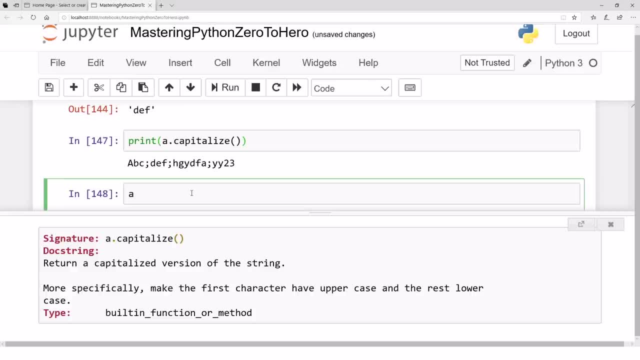 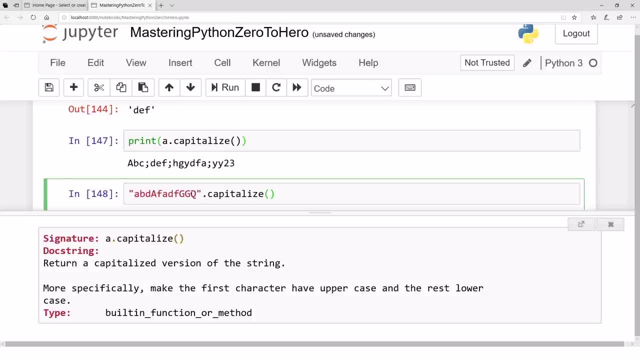 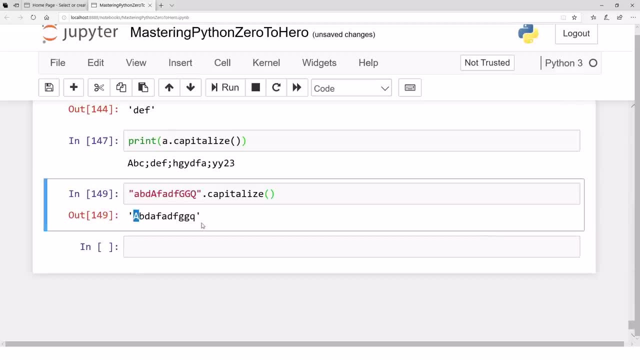 let's say so. what that does is it actually capitalizes the first character and all the rest of the characters there as it is- and there are other functions as well- a dot, um a dot, let's say, count what it does a dot count what it does a dot count. what is that thing? let's check it out. or maybe we can check that out using help. 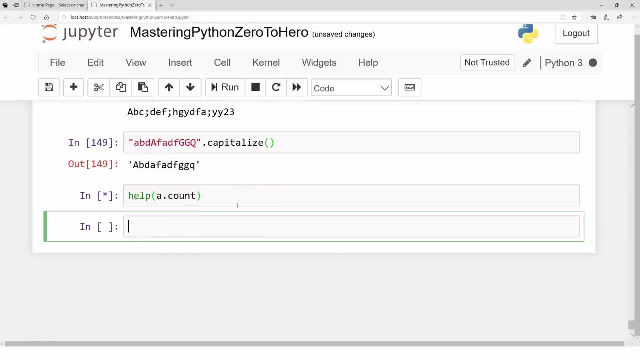 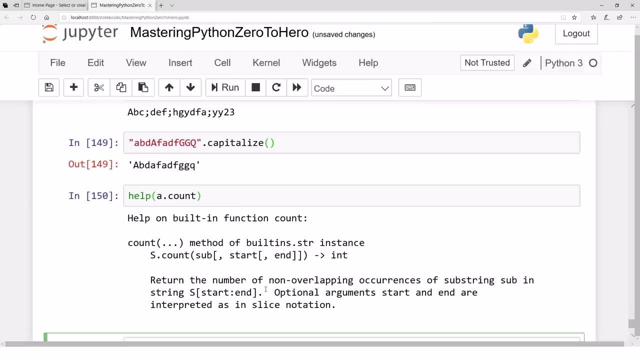 what is a dot count? so let's see what is a dot count. it's a built-in function. account method is an instance of, and it returns a number of non-overlapping occurrences of a substring. uh, sub in. oh, my god, if you, i mean, that's what it. what? what is written there um non-overlapping occurrences of a substring? great. 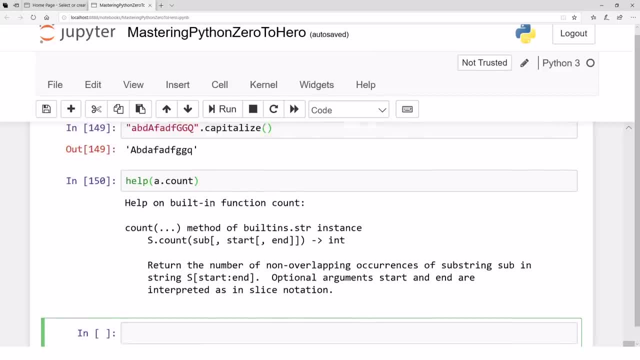 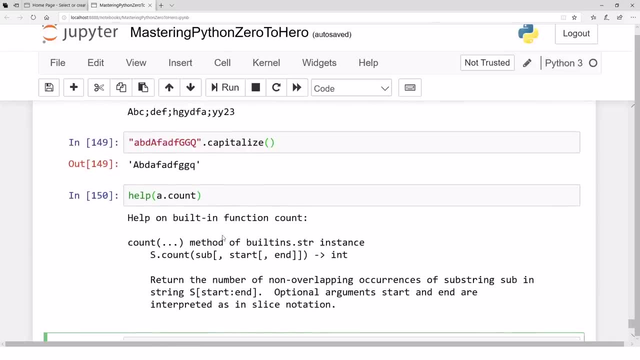 oh, my god. so, um, basically there are. there are a whole load of functions, uh, of strings that are available. there are several hues of the string. there are several ways of molding and playing with the strings. some of the functions are available, some you can make your own. 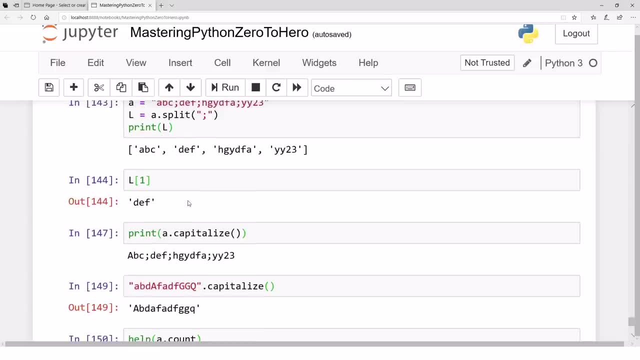 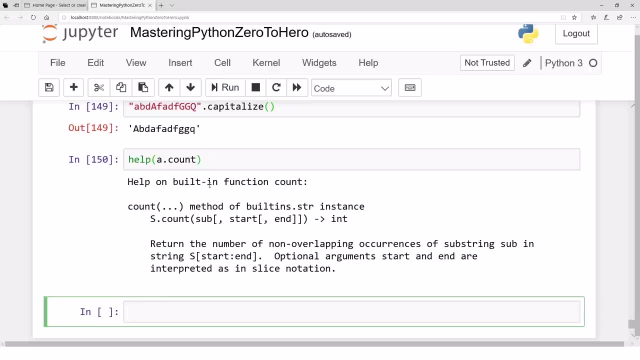 you can make your own modules on top of that to customize your uh, to customize according to your requirements. a lot of these are available and you should know how to use them. and first thing, if you want to do something with string or with any data type in python, first check whether some method is. 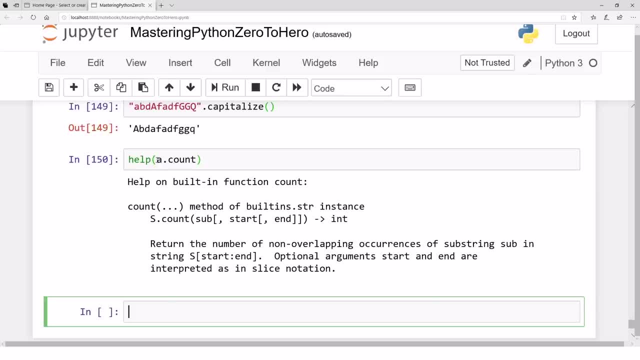 available or not, and one way to go that is just right away from here. another way is to go to internet and see- i want to do this in python with strings- whether there is a function available or not. the good chances are there will be a built-in function that is available, and in that case i will encourage to use that. 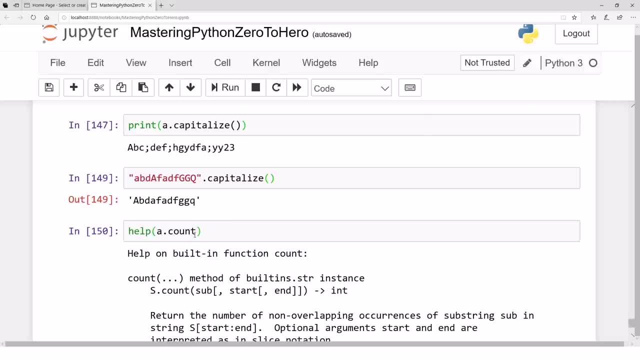 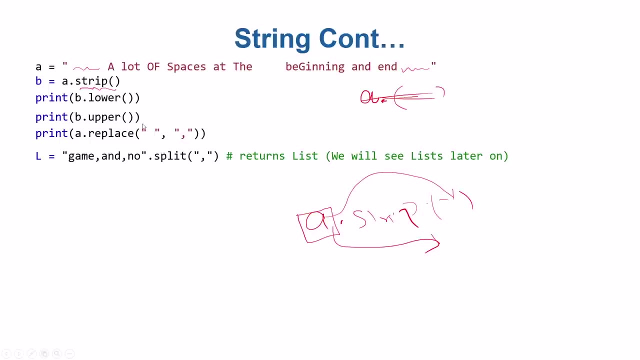 function rather than to write your own one, because using the built-in function or the method that is tied up there will be much more faster, probably, than the function you'll be writing at your end, even if you're too smart in algorithms. so, uh, yeah, so that's about the string methods. there are so many other methods that are available. 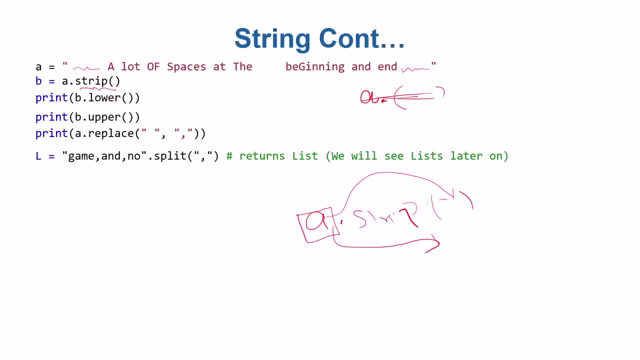 in the next video we will see some more, some more manipulation and processing and and some more working with strings, and then we will move to other data structures. okay, hope to see you in the next video. in the last video we saw some methods of string, and these are just a few of 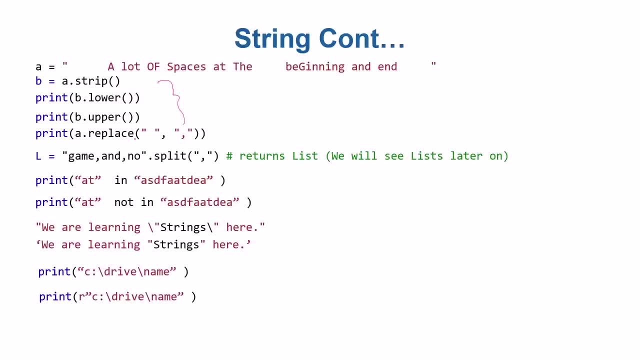 them, a lot of them- and we will see you in the next video, bye, bye- are available. we just we just discussed some of them. um, in this video, we are going to talk more about strings, uh, in a particular way. for example, what if you want to find out whether a particular 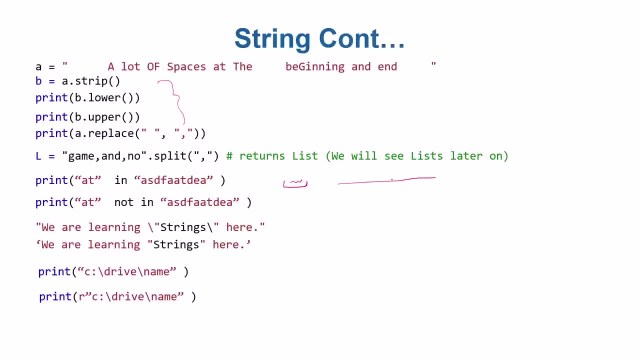 substring is there in a string or not. let's say you have a string and you want to know whether a particular substring is there inside a string or not. well, you can easily find out that using an n keyword and similarly not in means the reverse of that. 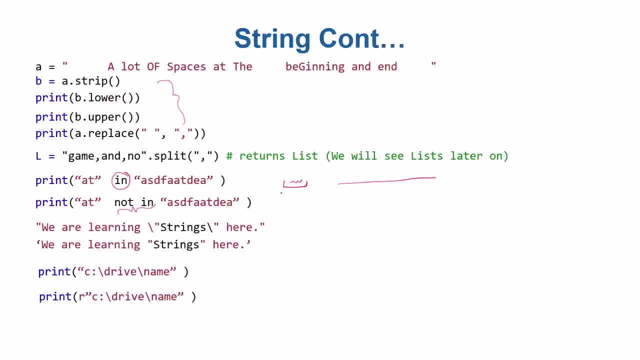 the complement of that or not of that. and in keyword always will return either true or boolean or false. if it is inside the string, it will return true. if it is not inside, it will return false. so let's check this. the implementation of that in in the in jupyter notebook. so let's see. 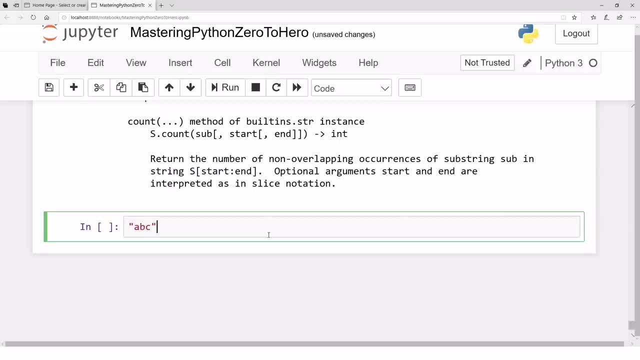 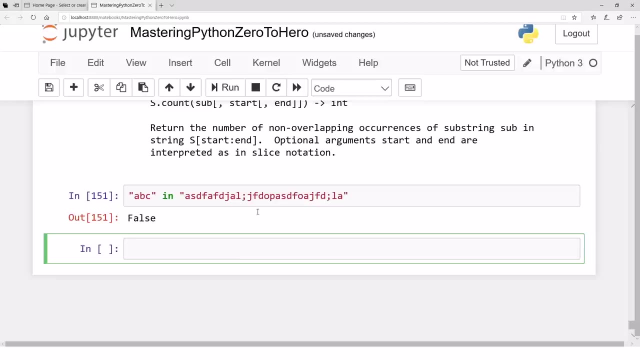 so let's say we have a string, abc, abc- and we want to check whether this string is there in particular string or not. So the return value is false because ABC as a stop string is no longer there. A is there, for example, here, AB is here, but ABC is no. 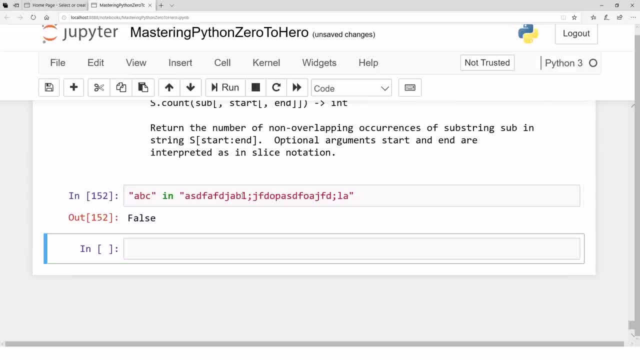 longer there. Yeah, so if we, for example, have an ABC somewhere, at least once, then the result will be true. In the last video, or maybe in the very first video for strings, I showed you that you can use plus with strings. Can you compare two strings using less than or equal to? I mean how? 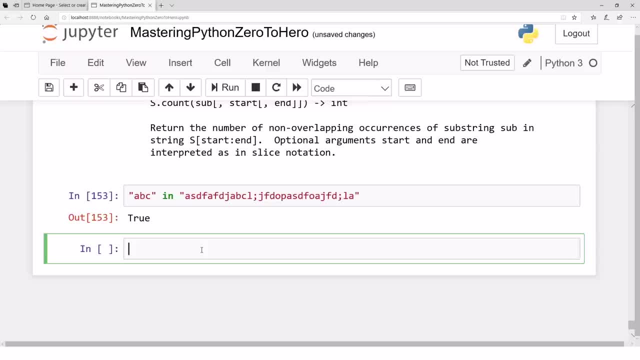 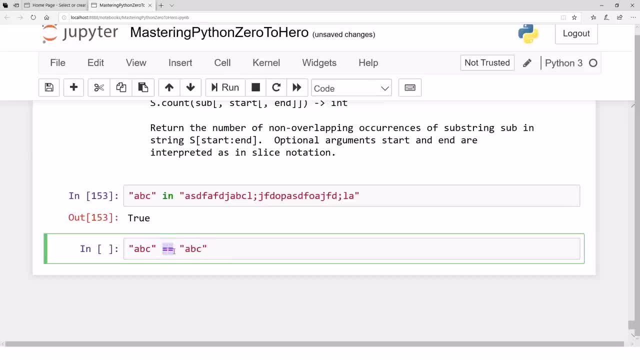 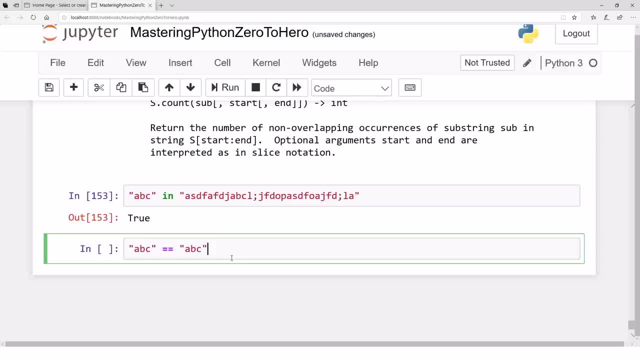 for comparing two strings. Well, the answer is yes. What will be the meaning of less than A string is less than the other? Is that true? For example, ABC is less than, let's say, DEF. Is that true? If it is true, 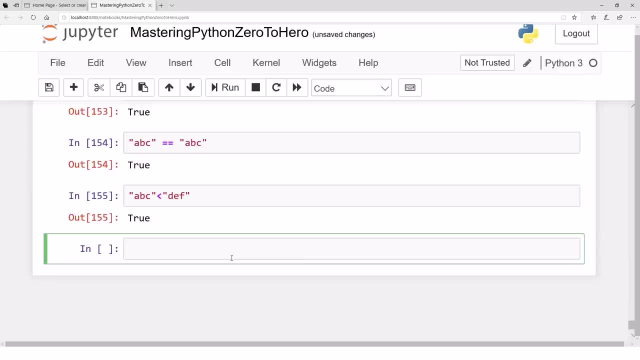 for example. what does it really mean? How can we define one string? is I mean this string is lesser than the other string? Maybe this, maybe this operator is working based on the length of the strings, but if, even if that, then this length is the same as this length and, to be more precise, we can change that. 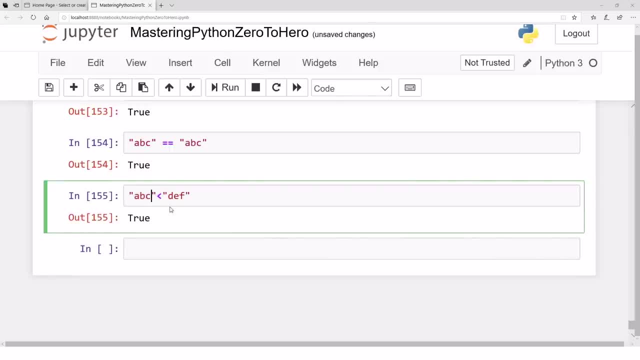 length, for example, by just saying okay, ABC, DEF, GH, I, and I guess this string will be still smaller than the right string. So how this comparison is working. Well, I guess the comparison is working based on the based on the alphabetic order, and you know the alphabetic order: A becomes: 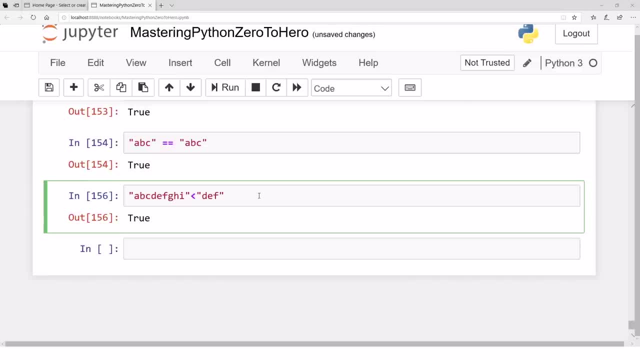 first and B, then C and all the alphabetic order that is there in English dictionaries. That's how the strings are working here, and the alphabetic orders for all the special characters will also be defined in Python, For example. that's a special character, for example, Maybe this string: Is this string smaller? 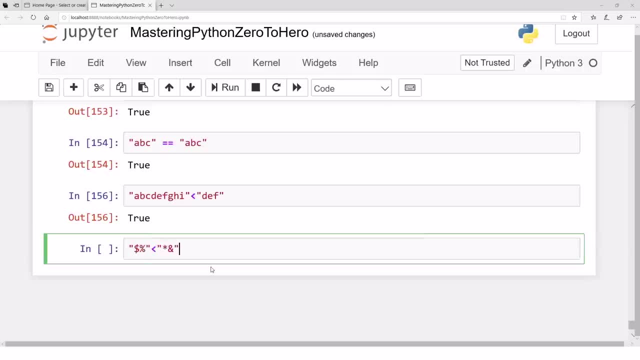 than the following string: Yeah, Return true or false. Because there is particular ordering in Python that is defined for these characters: that this becomes first and this, like, A becomes first and B, B becomes first and C and so on. So whatever the alphabetic order is based, 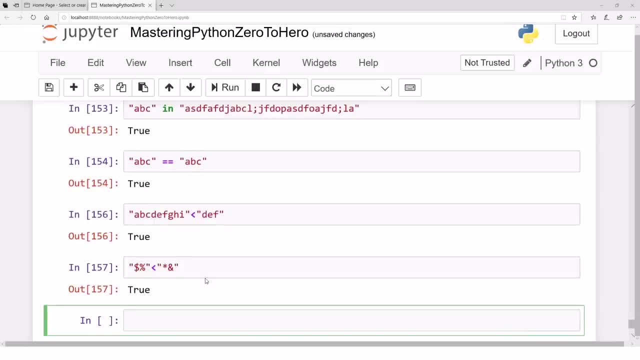 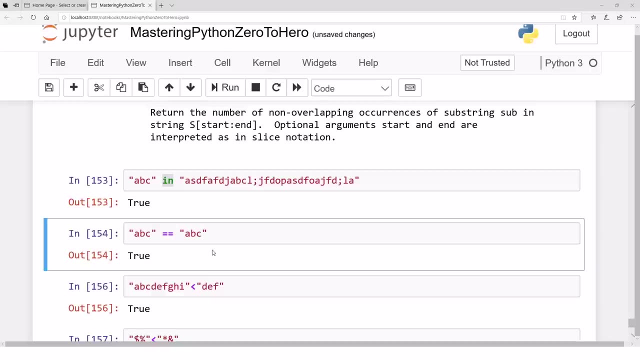 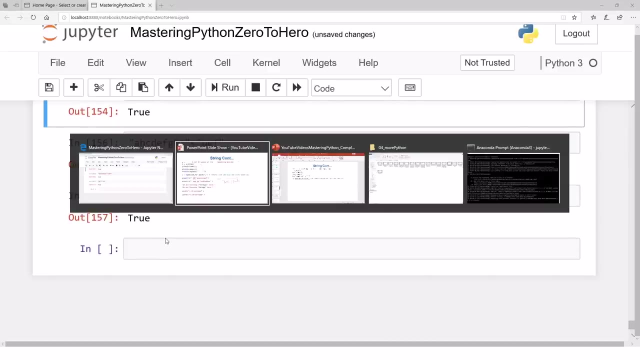 on that order. you can compare the two strings, no problem. So these are also available. and the third thing is in function that is also available, to check whether a particular string is inside a substring, is inside or not to in another string. One more thing that I want to talk about in that. 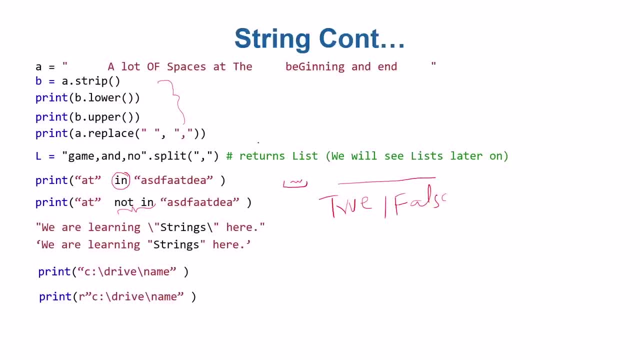 for example, what if your goal is to print the following. let's say: let's say you want to print the following: we are learning. and let's say you want to print the string in double quotes. We are learning string here. Let's say: you want to print this, You want this. 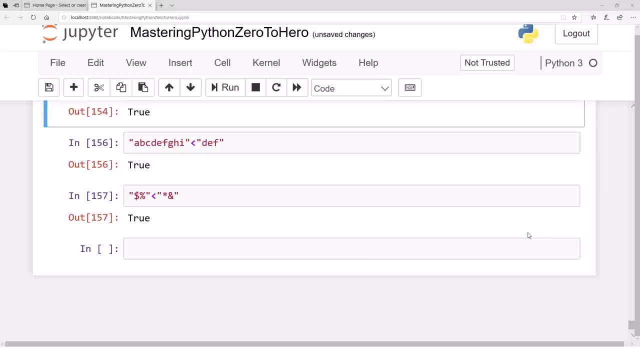 string to appear in double quote. How can you do that in Python? Well, it looks like same. What's the difficulty? Let's, let's call the print function and then- just right, here we are learning. then write the double quote: here string and here That's. 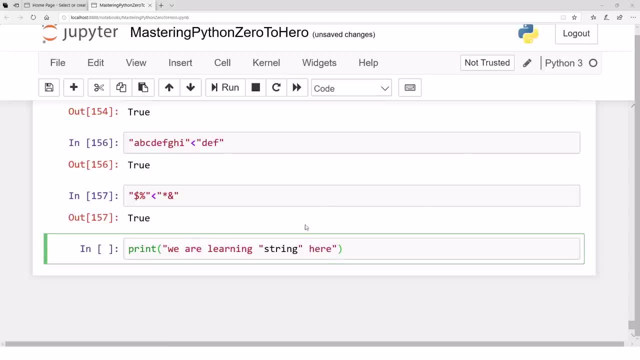 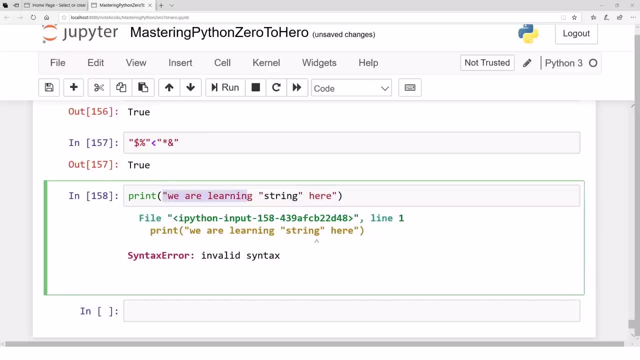 it. But there is a problem. The reason is. the reason is, when we call this, when we write this double quote, actually the string ends here, Exactly The string ends here, And when we write this single quote and this double quote, that another string starts here and this is no longer a string. 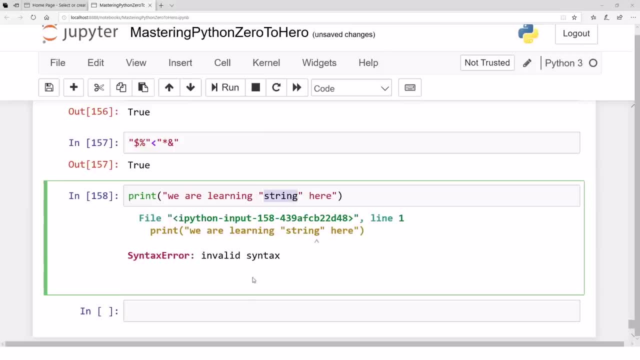 I mean what? it has no data type inside. Well, how can we then insert these double codes inside? Well, there are several ways. One way is to use escape sequence, and escape sequence is just like you use a slash and then whatever you use is considered as a corrector inside. 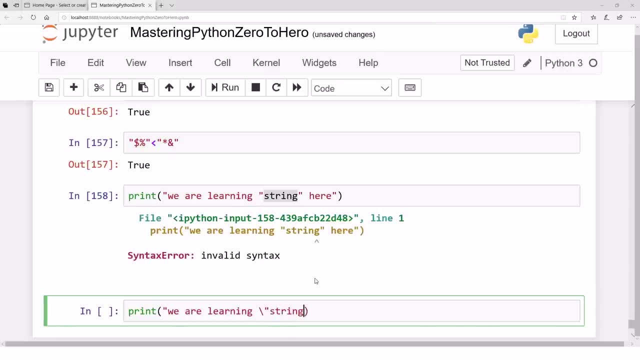 the string that you're using. And now, if you want another double code, you use a corrector, which is the backslash or maybe a forward slash, and if you use that, that means that means whatever that is coming in front of it should be used as it is rather than rather. 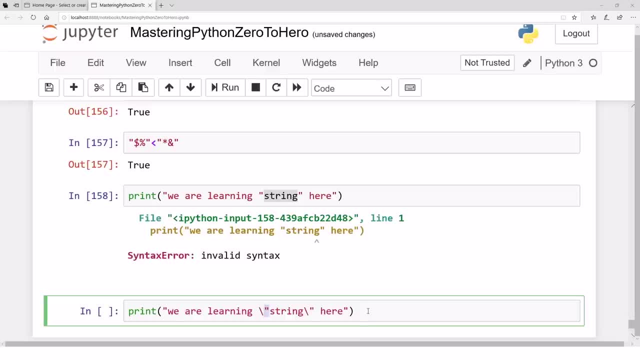 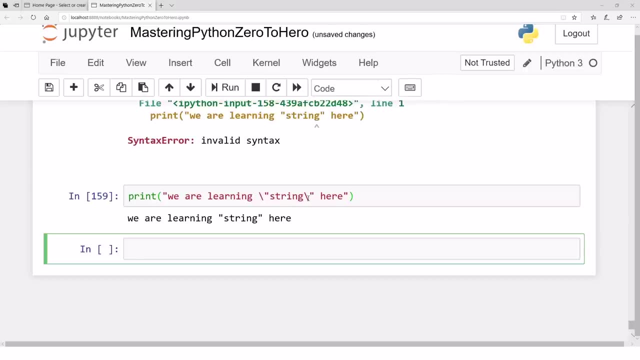 than considering that that's a special string defining symbol. Now, in this particular case, you'll be having your double codes available and the backslash will be just out. it's just defining that. don't touch this double code. it has nothing to do with defining a string. 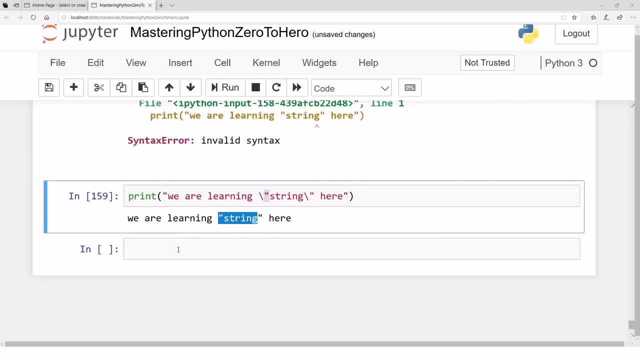 it is just a string, It's just because I want to highlight this word. Another more. another, more easy way is to use the single quotes. for example, we are learning and use the double quotes as a corrector. inside that, Now the single quote, wherever it starts and ends, they define. 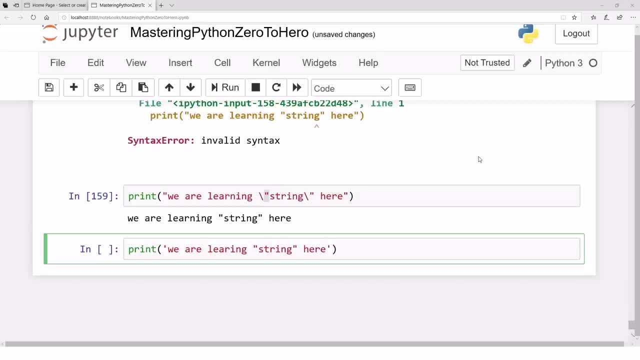 the string. everything else is a corrector. We do not need an escape corrector where we want, Okay, great. And there are a lot of escape correctors. for example, I'm going to use the double quotes. for example we have. we are backslash n, that means go to. 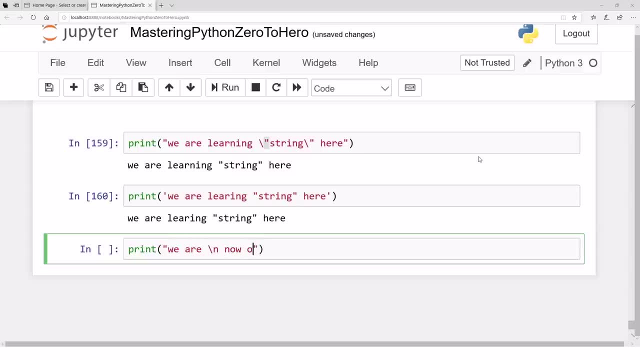 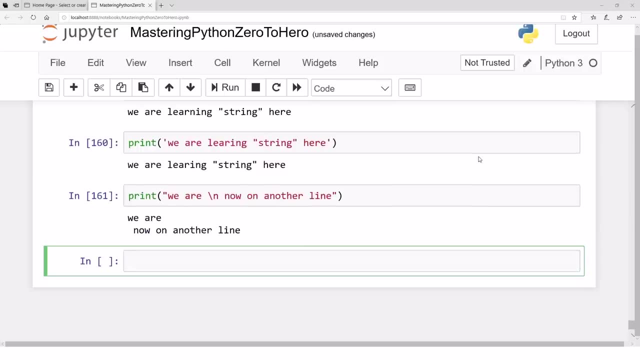 new line. we are now on an other line, So this backslash n actually puts everything that comes after to a new line. that's an escape corrector. Similarly, we have an escape corrector backslash t that actually inserts a tab whenever we want. so we are then a. 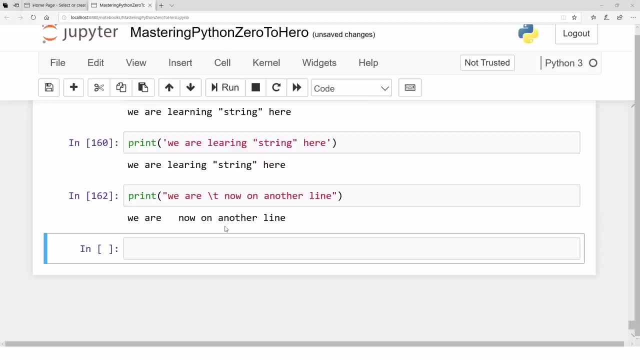 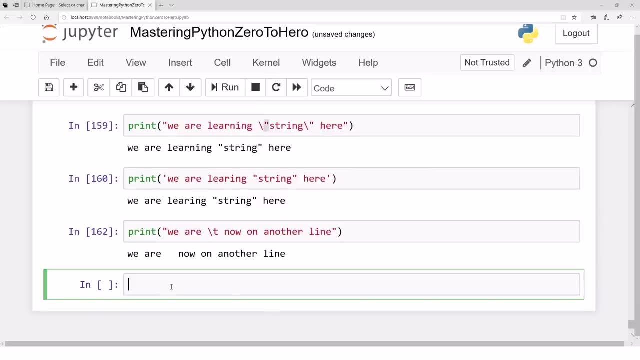 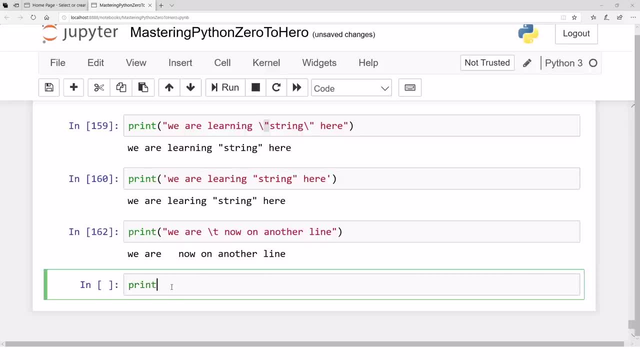 those. One more thing that is important. for example, let's say you want to print. let's say you want to print some address on the drive. let's say c backslash, backslash forward drive. let's say you want to do that and your goal was to just print that path. what will happen is: 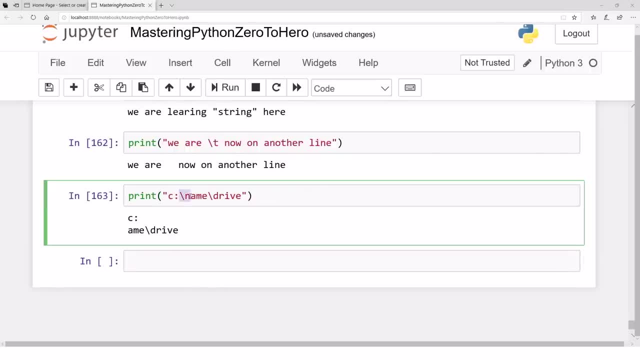 this. backslash n will be treated as a new line escape sequence and backslash n will tell: okay, go to the next line and treat the rest of the things. but because backslash d is not any escape sequence, it is not listed inside, it is treated as it is and that way this slash is also treated. 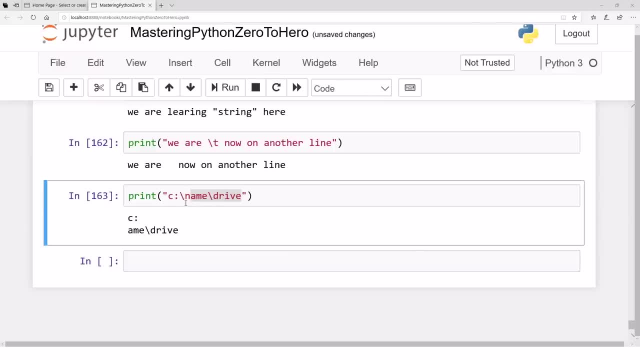 as a character, but here because if this slash followed by this n, that's a combination that is already there for a new line that is treated in a different way. if you want this to be used as it is and you don't want these, you don't want this behavior, you just want that all this should be. 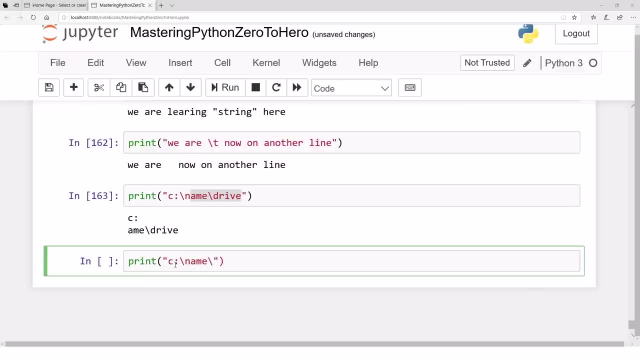 treated in a very literal or raw sense, then you should just apply an r there and that's it, and r will tell: okay, that's a, that's a raw string. everything inside just treat that as a raw string. there is no escape sequence inside: great. so um, and there is much more about string. 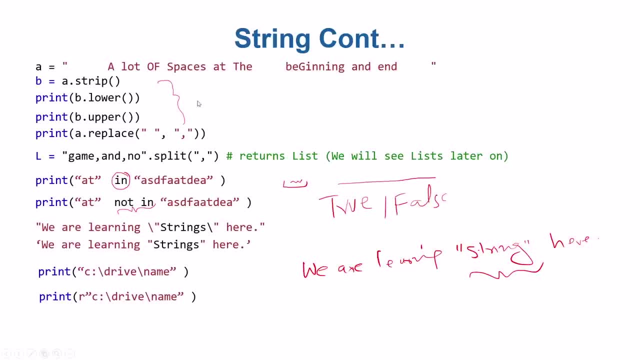 we can talk, but that that was the most important that i, that i told you, at least to me. uh, we can explore this more. actually, you should now explore this more. what are other functions of string? how can we play with strings in another way, and stuff and so on. 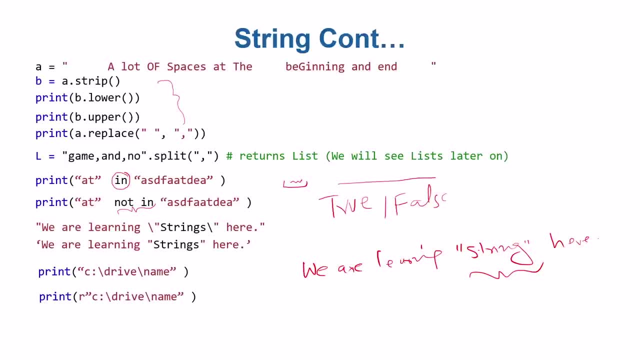 if i talk about strings, i can just- i mean, i can give a whole course on strings as well, but here i just give you a snapshot of strings. if you need more about strings, i mean you should be searching on internet or seeing documentations and seeing, basically, uh, what you want according. 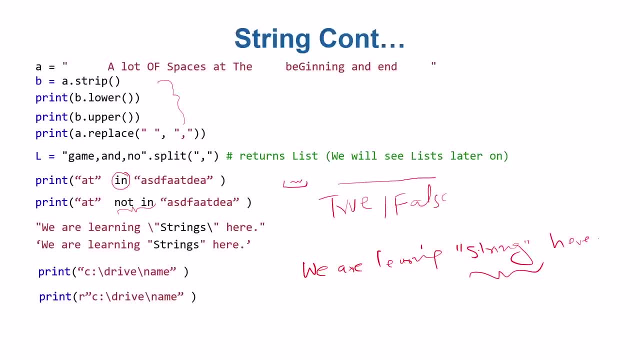 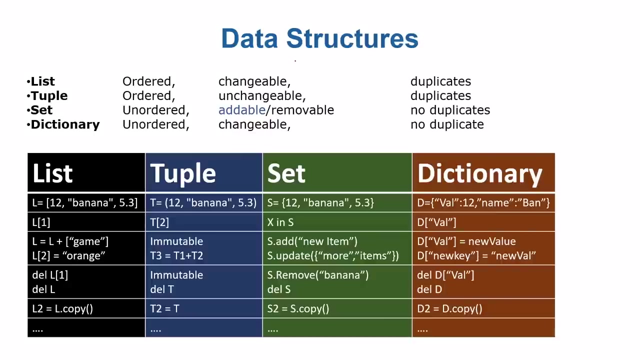 to your requirements. search the functions: uh, probably they will be available. okay, um, in the next video we are going towards list, tuples, uh, sets and dictionaries, some other data structures that we were talking about earlier. we will be going to explore them in more detail from the next video. hope to see you in the next video. a data structure, informally or in a very naive 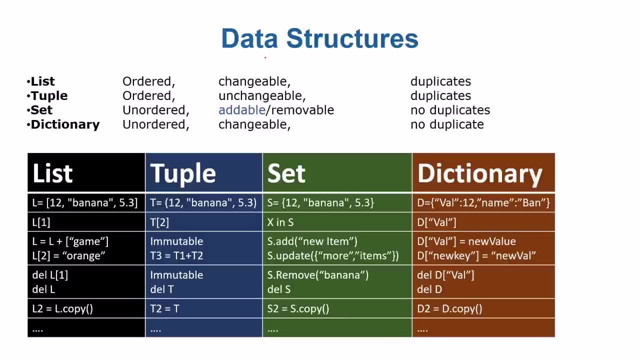 sense is basically collection of a lot of basic data types that contains data. one structure contain a lot of data and we can define sometimes several methods and several specialized kind of functions are customized and defined just because of that uh data structure to perform efficiently uh different kind of- i mean for different 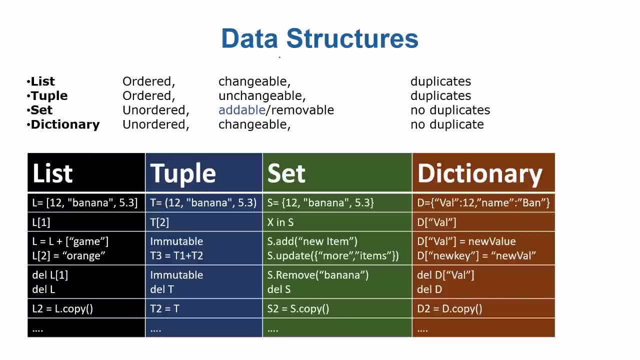 kind of tasks. we may have to define or we may have to choose different kind of data structures. the basic data structures that are available in python is a list, tuple set and dictionary. these are the basic data structures that are available. we can create our own data structures if we want to. but most of the problems, almost all of 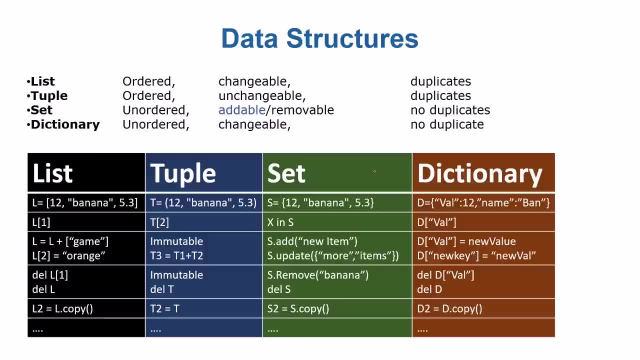 the problems. mostly they are solved by these four basic data structures, although a lot of these are not that efficient. uh, there are efficient uh ways for uh customized kind of problems. uh, we will see that efficiency when we will deal with the package numpy that is. uh, that is faster than all of these. 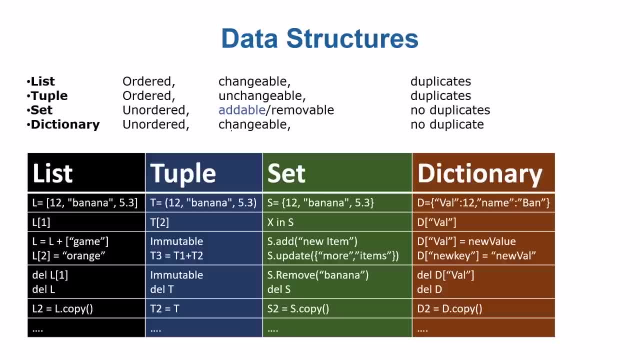 uh, but, but we will see what kind of constraints are there to make it faster anyways. uh, data set in a very loose term is collection. it is collection of a lot of values, a lot of data inside and all these data structures, list, tuple set and dictionary, they, they are. 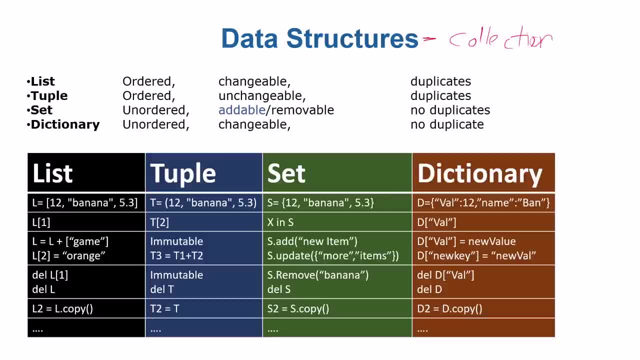 collection of data of heterogeneous types, which means one value can be integer, another element- let me call an element- another element or item. another item or element can be of string type. another element can be of, let's say, floating point number. another element is a whole list itself another element. 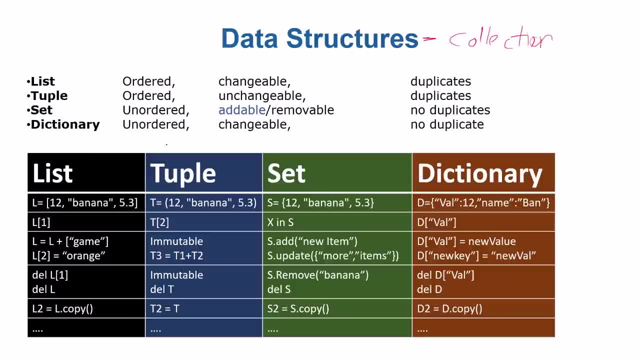 is a tuple and so on, so different elements can be of different types, and that makes this heterogeneity, that makes these four data structures much more applicable and much more abstract, and they can be applied to almost all the problems. so let's see one by one and let's compare. 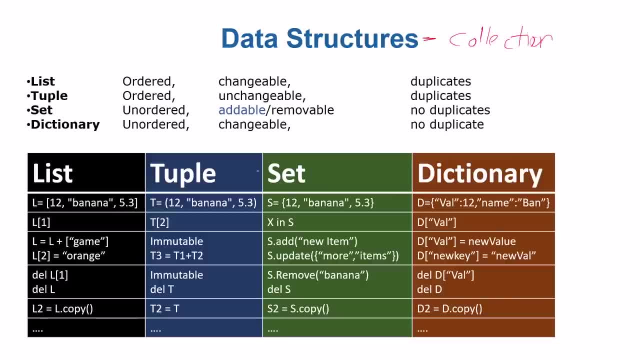 them together, because the best way to understand four of these is just to compare them. which can do as compared to the rest? so let's, let's compare them and learn how. how can we use those in detail? so list first is list. list is ordered. ordered here means it is indexable, which means uh, there is a. 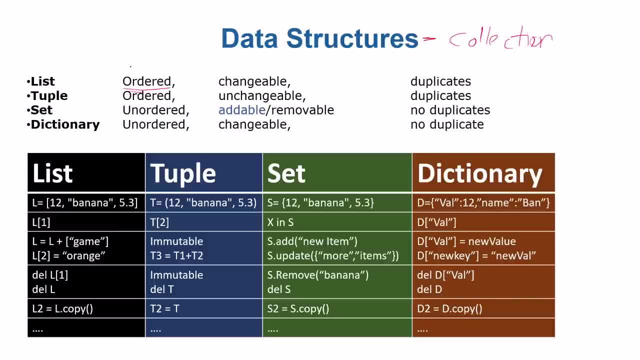 part. the element number one is at position one element. there is an ordering of elements. first element, second, third, 25th element. there is an ordering of element with respect to their position. so that's what we mean by ordered. uh, changeable, or sometimes called more reasonable term or more usable term, is mutable. mutable needed. 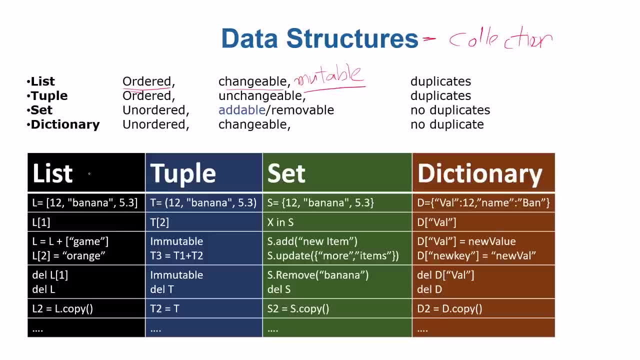 like this one and the lks, which means that the list where the element is put next. then, as we ոx gli Lin els: one element, one element, click on he or I who is within goal. one element: the location, return category and for function, wego and change its elements. example: you. 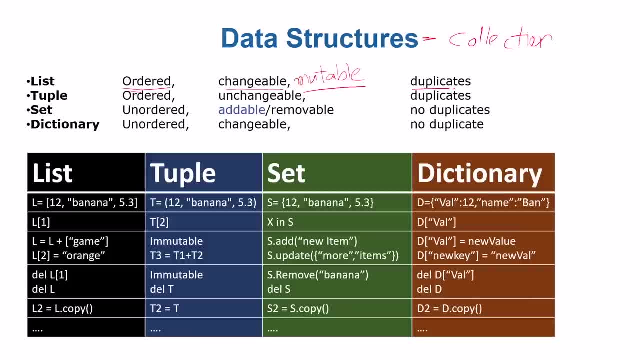 can change the third element with another element and that's perfectly fine. you can change it that. what we mean by a changeable, or more popularly called as mutable duplicates, means the At the position number 3, you can have the same item and position number 5, you can. 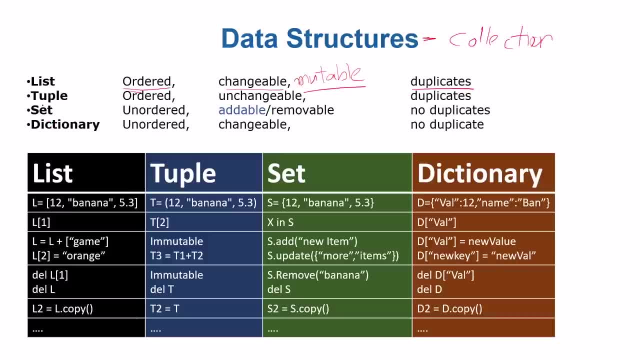 have the same item, so the duplicates are allowed. Tuple, however, although ordered, there is an ordering of elements. there are indices of different elements. this is immutable Once tuple is created like strings. once the tuple is created, you cannot change different. 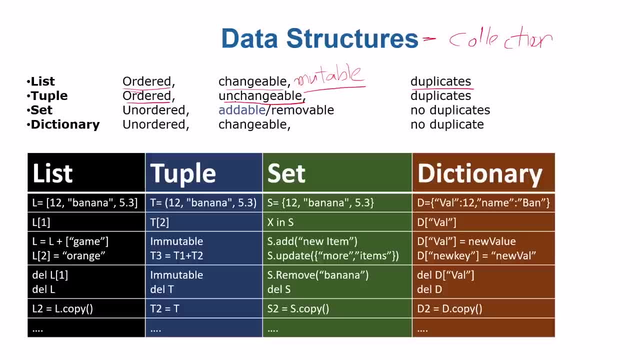 elements in the tuple. You have to create a new tuple if you want to, but you cannot change the items in the tuple and the duplicates are allowed again. Set, on the other hand, is unordered, which means there is no indexing, there is no positioning. 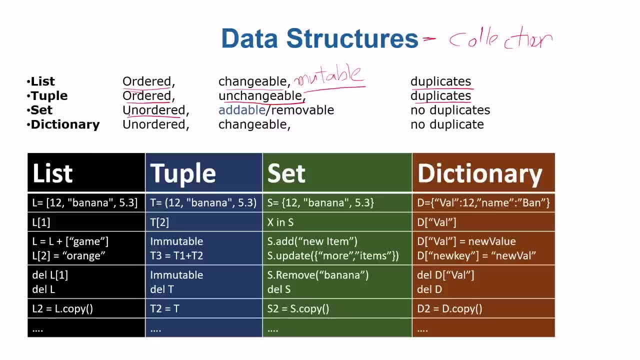 there is no first element, there is no third element, there is no fifth element. That's a collection without actually indexing. Because you cannot access a particular element with index. you cannot change it. but what you can do is you can insert more elements and you can remove existing elements, if you. 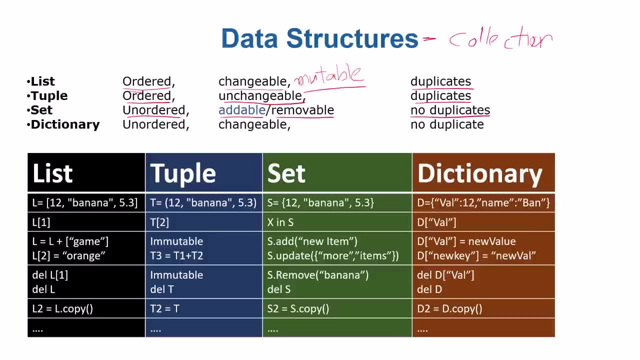 want to. Again, the set, like in mathematics sets, does not contain any duplicates, so one item appears just once. We will see the examples. Dictionary is a very, very, very powerful data structure. Again, it is dictionary is just like a set. it's a set. it is unordered, again changeable. 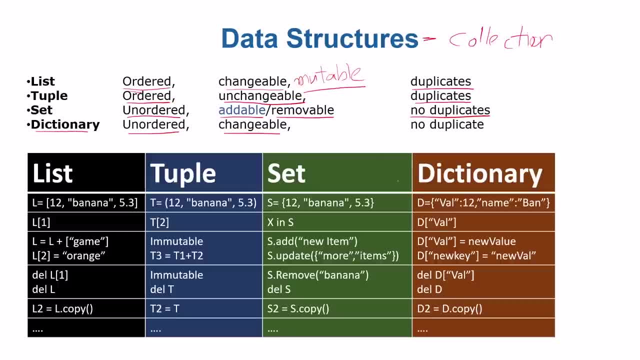 you can change the items and the dictionary and it does not have duplicates because it's basically a set. It is just like a set. The power of dictionary is each item consists of a pair and one value in the pair is called. 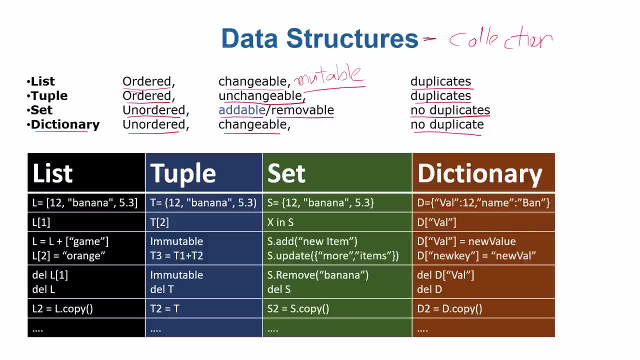 key and another is called a value. For example, val is key for 12, name is key for ban, and so on. So we have seen this dictionary before in loops and stuff in just a very loose way, but that's really a very, very powerful data structure. 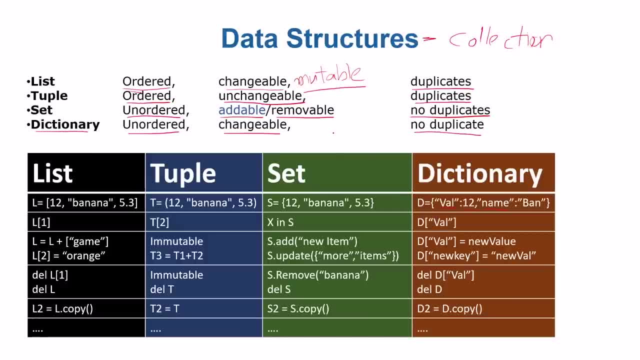 And later on we will see in pandas basically all the data is basically managed just like a dictionary. If you have a good knowledge of dictionary you'll be having a very good grip very quickly on a big data science library or big data science package which is called pandas. because 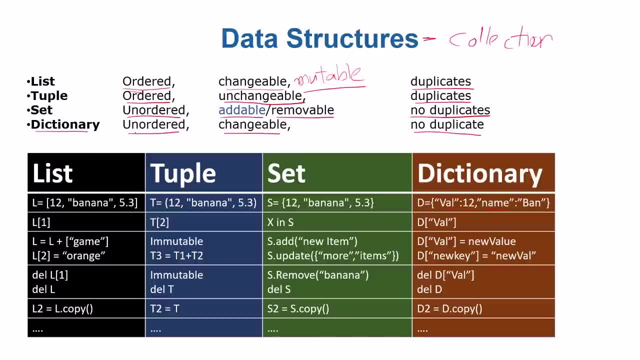 each and everything in pandas is handled just like you're handling a dictionary, So it's a really powerful data structure to know about. So yeah, So list is mutable. dictionary is mutable. set is mutable in a sense that you can insert. 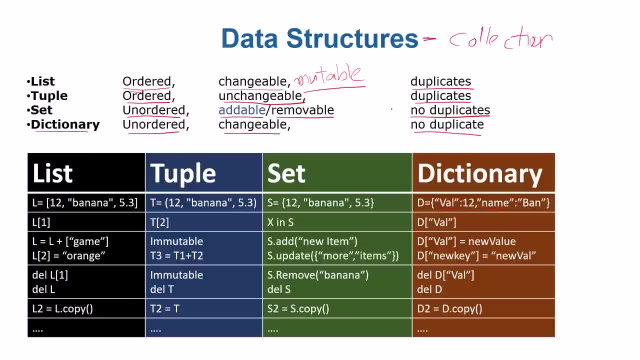 and remove elements. tuple is not mutable, And that's the comparison. theoretically, what is there? All these types. each and every of them is a collection of different values and the values can have different types. That's the abstract power of all these data structures. 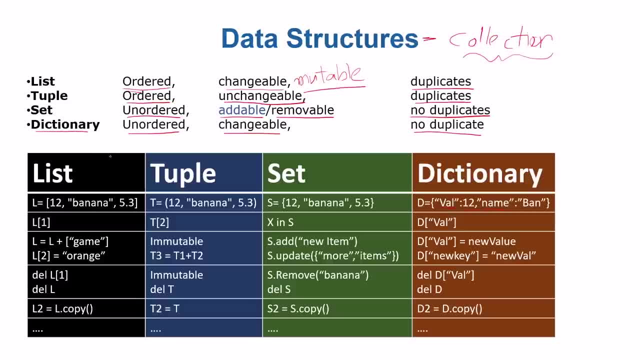 So in the next video we will actually try to get a good grip on list, tuple, set and dictionary and we will actually define them, code them, access different methods of those, and we will be trying to become comfortable with these data structures by coding them. 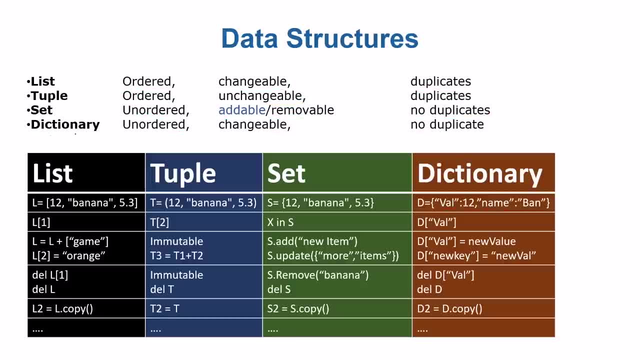 in Python, So hope to see you in the next video. Okay, Continuing previous video, We were talking about data structures, So let's get started. So let's get started, Okay. So let's go to the Jupyter Notebook and see how a list can be defined or declared, how. 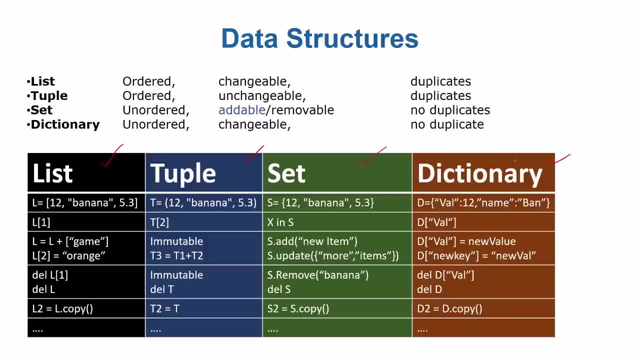 a tuple can be defined or declared, set and dictionary. Let's see how can we make these data structures in Python. So then, one by one, we will compare. how can we access elements of the list, how can we insert more elements in list, tuple, set and dictionary and see the comparisons of all? 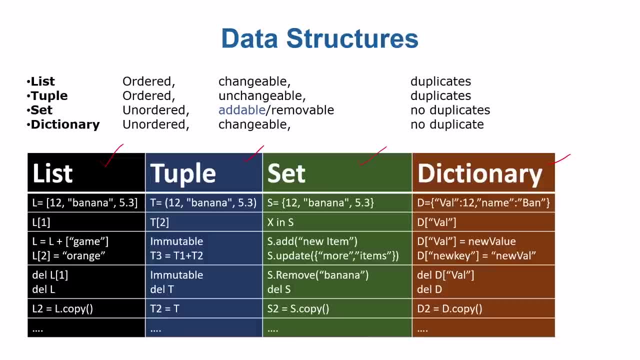 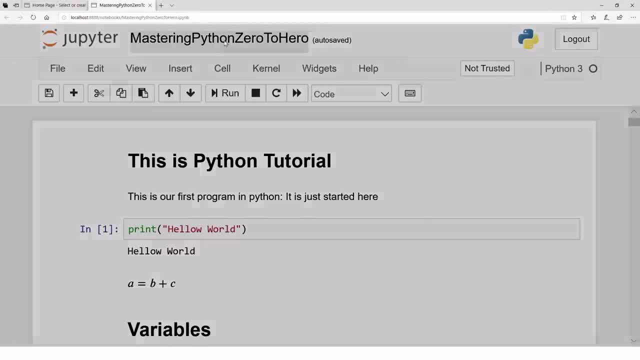 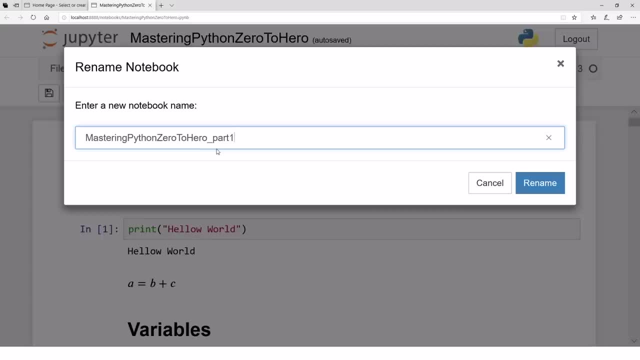 these one by one, operation by operation. So let's see. So let's go to Jupyter Notebook, our friend. This file is getting lengthier and lengthier. Let's make multiple files. Let's say this is part one. 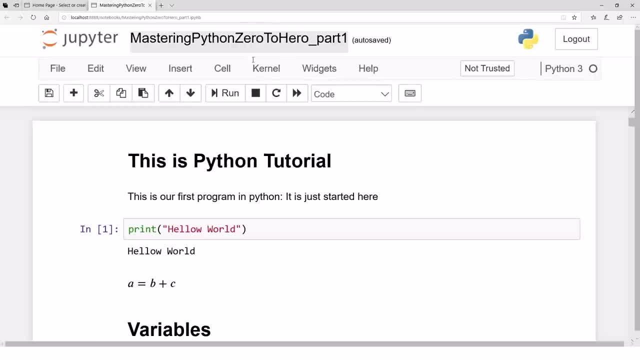 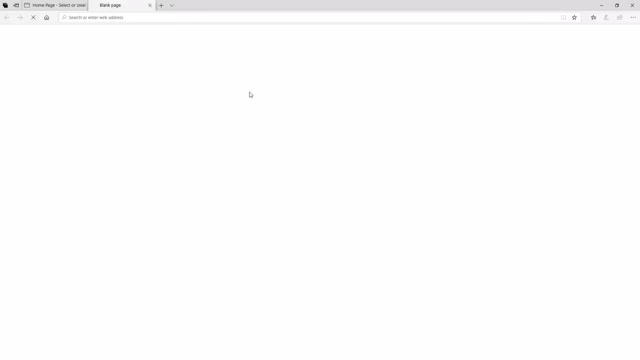 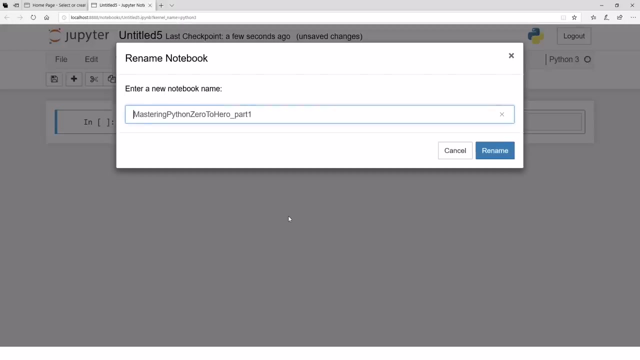 Just save it and let's make another file. For example, let's just close this file or maybe state opened, Let's close this file and make another file. Okay, Python 3.. Yeah, So let's name that file as this: part two. 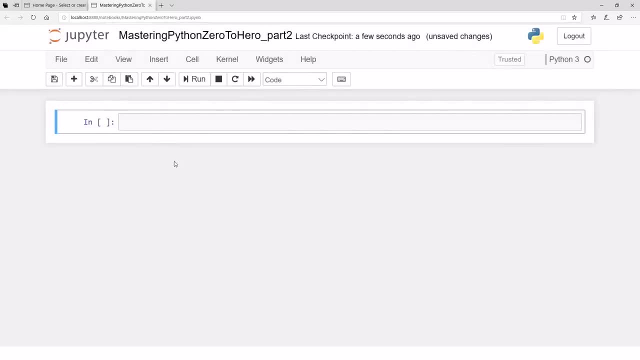 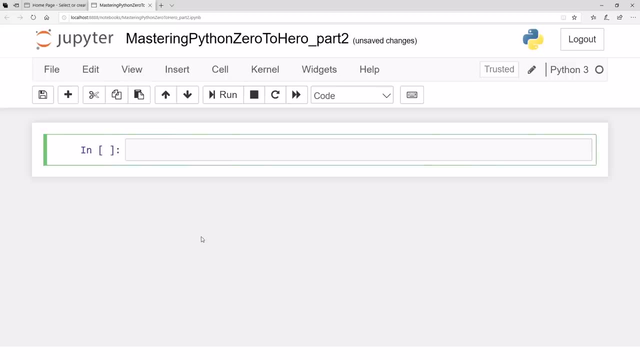 Let's start a new file. That file was. I mean that was okay to stay with that file as well. but just let's make another file, Okay. So let's just have a markdown cell And let's have a heading. 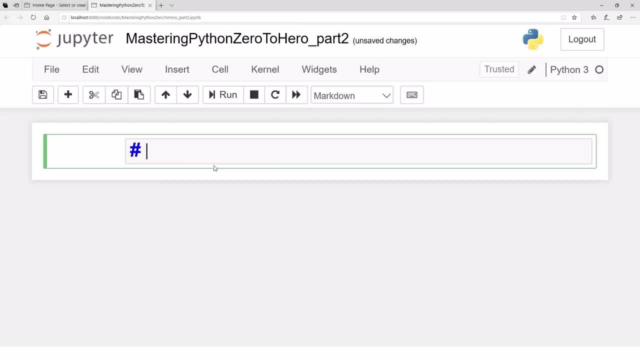 Okay, Let's try the datastructures. Remember the markdown cells? I just introduced them, introduced those just in the very beginning, and then we just forget them, because writing these description again and again will make the video lengthier And the purpose is not to actually format the notebook. 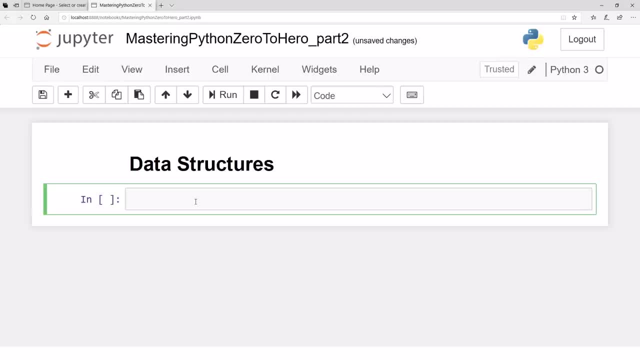 The purpose is just to show you the power of Python and more, But just write a few descriptions in the start and then we will forget again. Oh, that's it. That's amazing. Let's define a list. So list any variable name. that's a variable in. 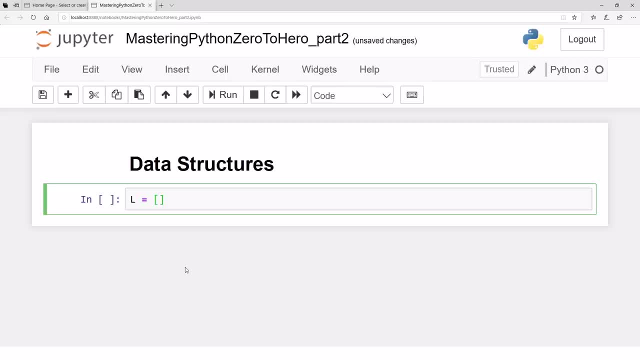 list is, let's say this: you define list by square brackets and different elements. they are separated by comma. Let's say 1,, 3,, 4.9, name anything I mean. or 5,, or maybe 3 again. 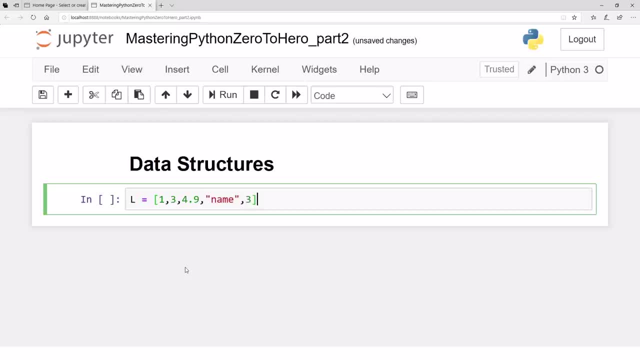 So that's a list, Okay. Doppel, on the other hand, is defined using parentheses. So let's say 1, 3, 4, 5.. 4.9, let's say name and let's say 3 again. That's okay. That's a doppel. A doppel is defined. 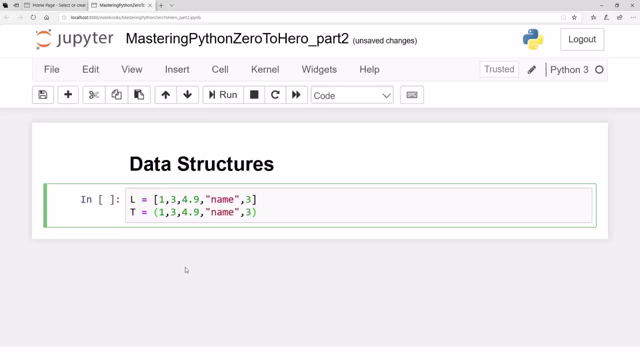 in. so when you write parentheses that means by default that's a doppel. The variable name has. I mean if you have written t, that has nothing to do that It's a doppel. That's because the Python is dynamically typed. 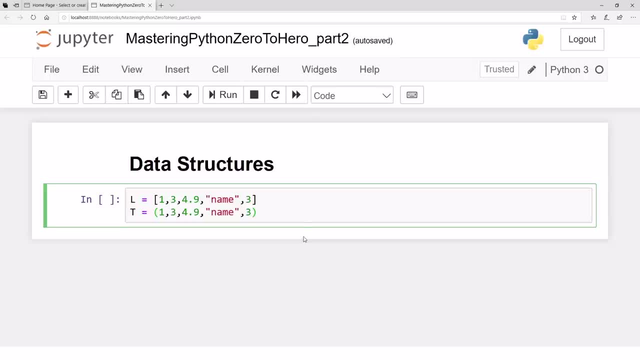 When you will write the parentheses. that means the doppel is being defined. Let's define a set. Let's call the variable as s. The set is defined with these curly brackets, So let's say 1,, 3,, 4.9.. I want to tell you that all these things they can contain, each element can. 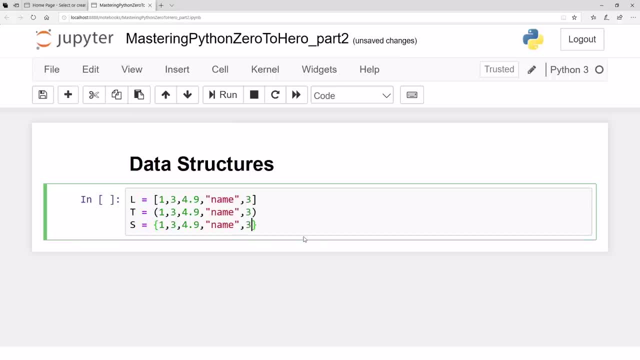 have a different type. But then even if we include this 3 again, because the set cannot contain the duplicates- later on we will see that only one copy of 3 will be there in the set. The other will. even if we want to include, it will not be included. Okay, Then let's say a: 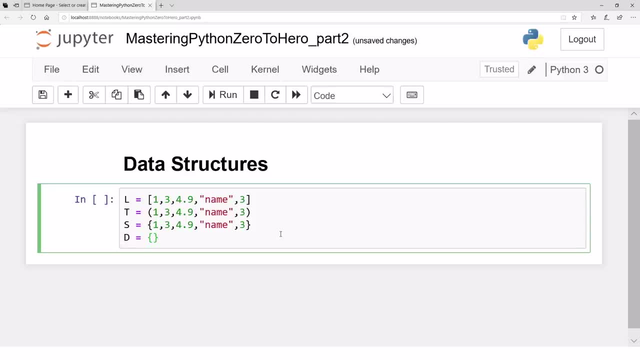 dictionary Dictionary is again defined like a set, but each element is a pair separated by a colon. Let's say the key value is 23.. That's a key value. That's a key And the value here is a string. Let's say: 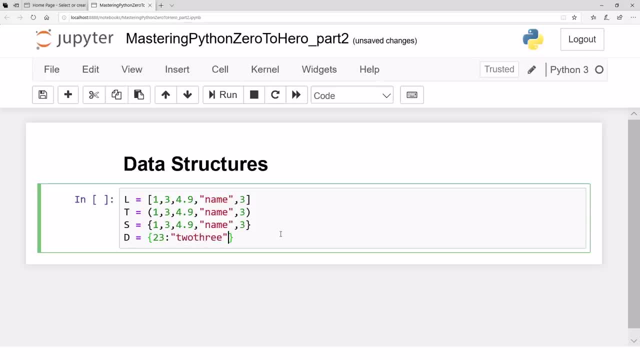 2, 3.. That's, let's say, the value, Now comma, Now one element is there, This one element that can, that consists of key and value pair. Another element, another element may have a key with string, So so the keys can be of different types, The the values can be of different. 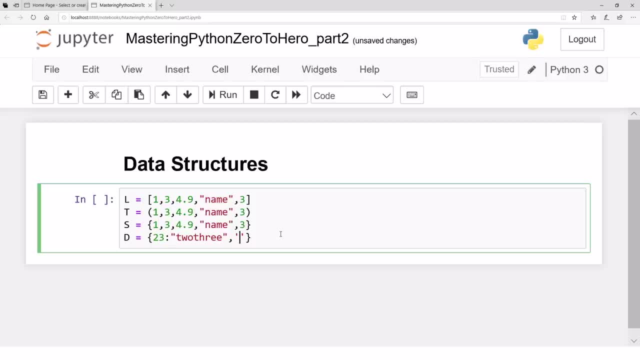 types and so abstract. So the key is, let's say, let's say B, and the value for this is, let's say, 43. Then maybe we can have another key value pair with key, as let's say C and the value is, let's say, CC, CCD, that's a charge coupled device. Okay. 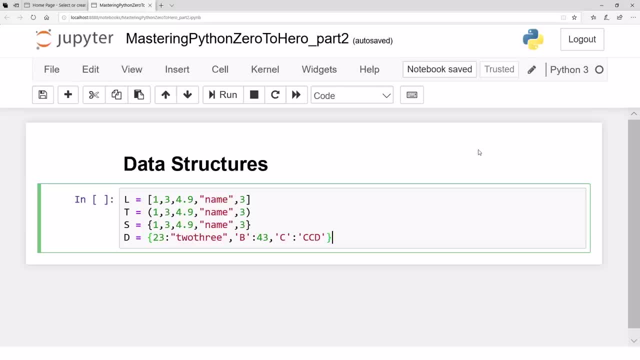 Anyways. so so you now you know how to define the list, how to define a tuple, how to define a set and how to define a dictionary, The, the, the difference is is the. the main difference here is in dictionary, because one element consists. 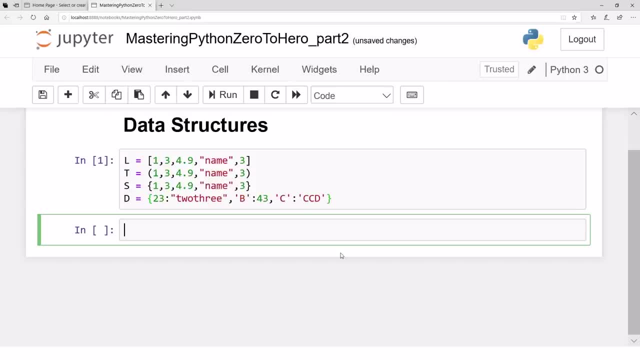 of two values rather than one. okay, let's print that. and see the types. let's print all the types. print type, so let's print them. the type of L is, so the type of L is just printed. that's L. let's print that. let's see the other types. let's print the rest as well. 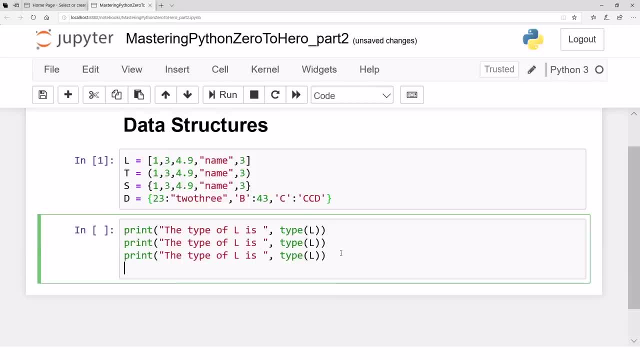 so just copy them and paste. the type of list L is that the type of tuple is T and let's say we have T, then we have s, and we can just replace this with s, and then we have, let's say, D, dictionary, and that's, that's D. okay, so let's print: so the type of L is list, the type of T is: 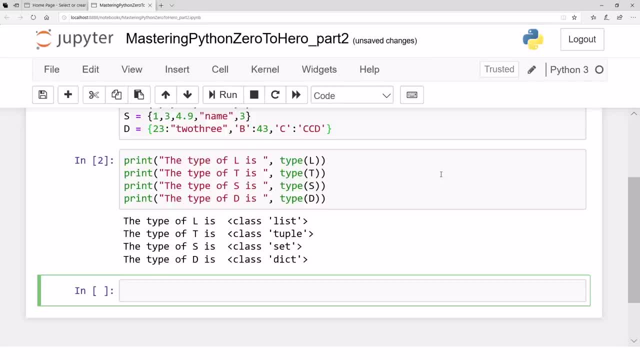 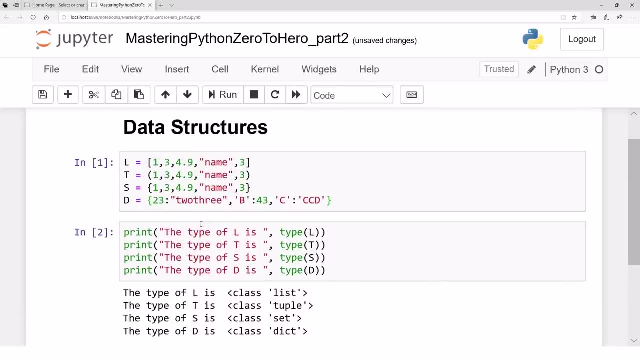 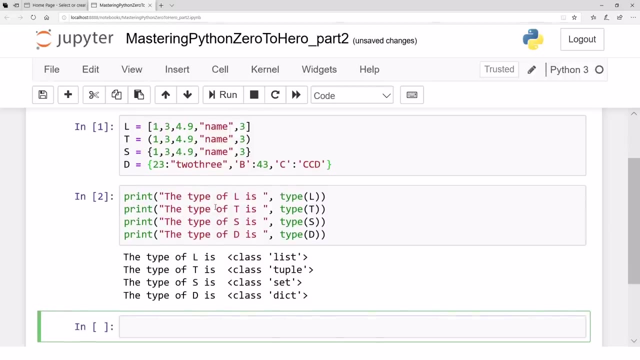 tuple, the type of S is set, the type of D is dictionary. oh great, so that's how you can define these lists. you can define list, you can find tuple, you can define set and you can define dictionary- no problem. next Let's see how to access different elements from these data structures. 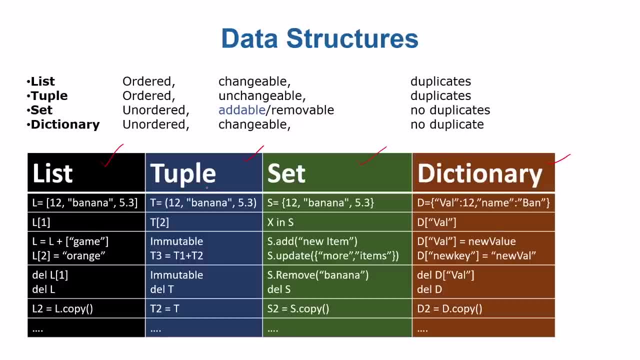 What are the ways, For example, to access an element from a list, let's say the element that indexed with one. Remember, the element that indexed with one is element number two, because indexing starts from zero. So you can access that using the square brackets. 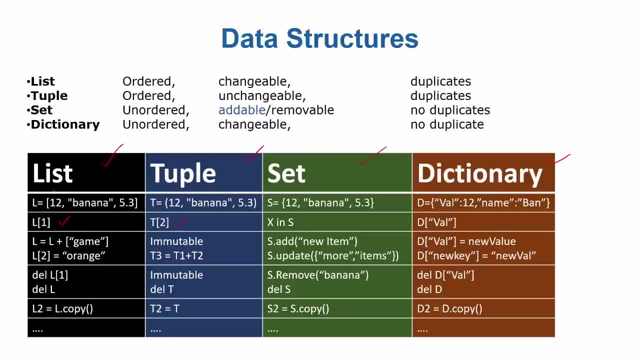 If you want to access from tuple again from the square brackets, exactly like the list In set, for example, you cannot index it because the set has no ordering. First, second, third element is no longer there. But you can check whether a particular element is there in the set or not using in keyword. 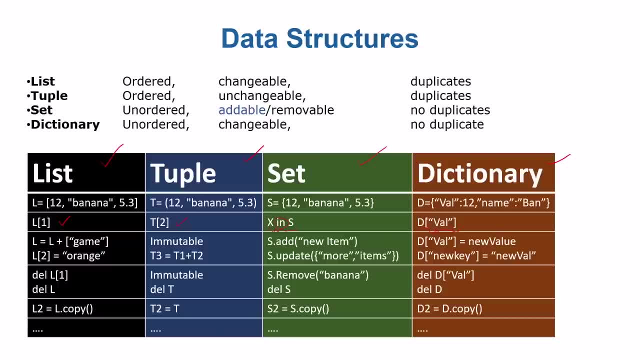 In dictionary, for example, if you want to check whether a particular element, if you want to access value for a particular key, you just write the dictionary variable name and then write the key and it will return the value. Okay, so let's practice this in Jupyter. 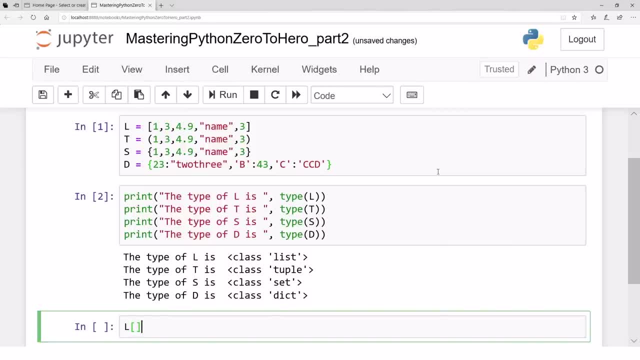 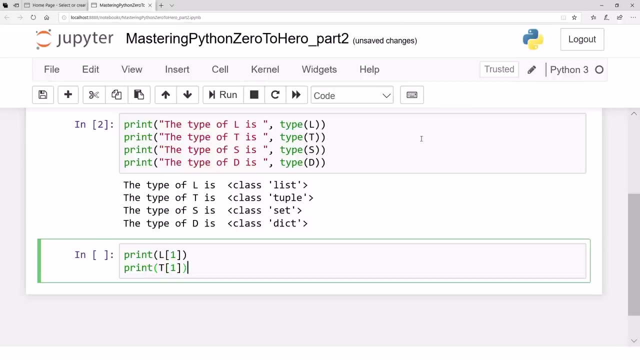 Let's just practice this in Jupyter. So let's say list value at index one. So let's print this list at index one. The value should be printed as three print tuple at index one. Again, the way of accessing is this: Accessing is the same. 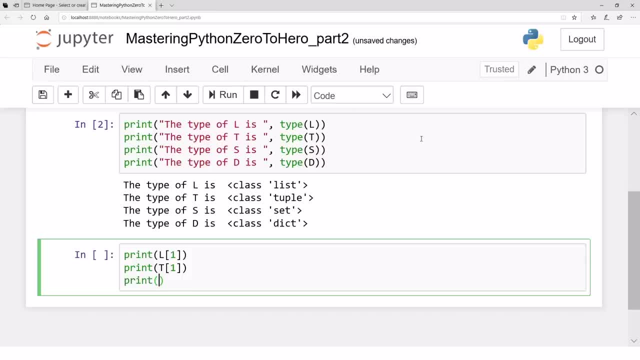 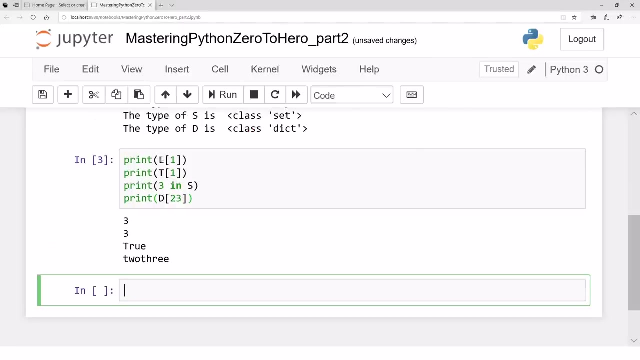 Print, print, whether three in s or not, The return value will be true or false. So print will be true or false. And then print d and just access the value with the key 23.. So let's see what happens. So l at index one is three. 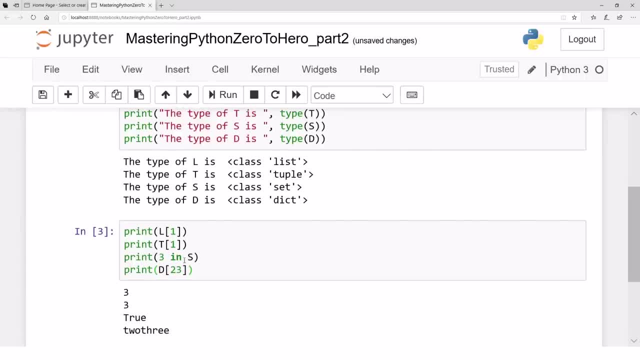 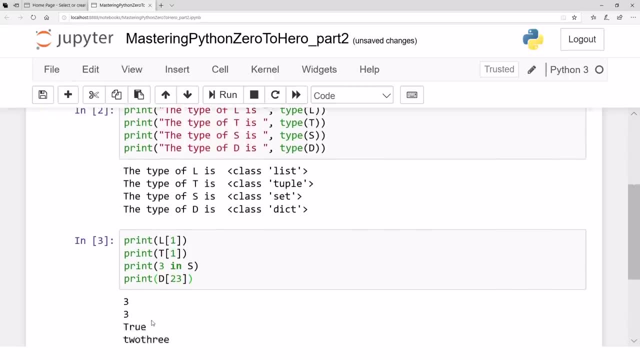 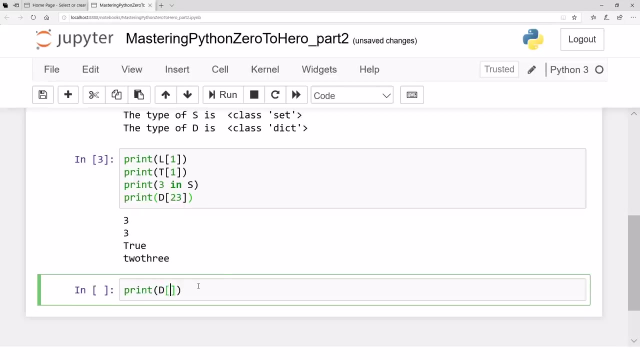 D at index one is three, Three is in s. yes, And what is the value with the key 23?? The value is two- three. Let me just describe more about this d. What is the value at index b, for example? 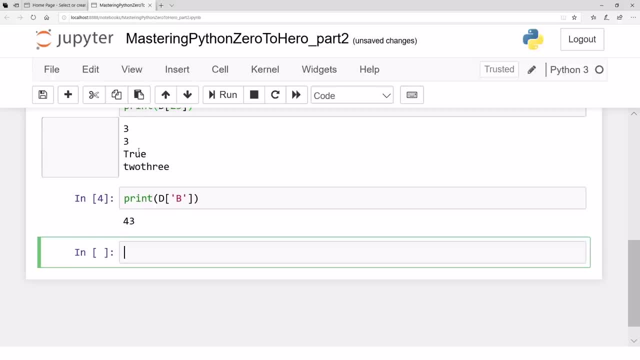 Now we have to give the index b in the string format, That's 43.. Yeah, So that's how we can access that. Let's print s also. Let's see s, because when we have defined s, we have defined this duplicate three. 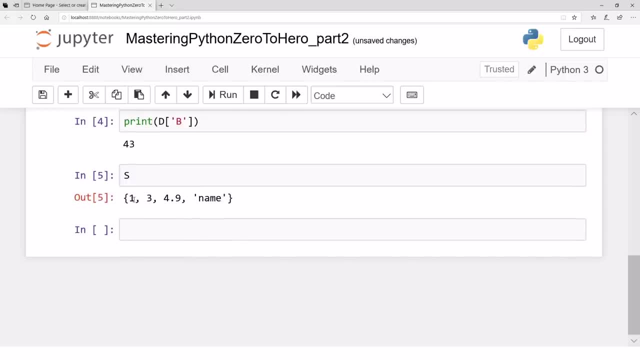 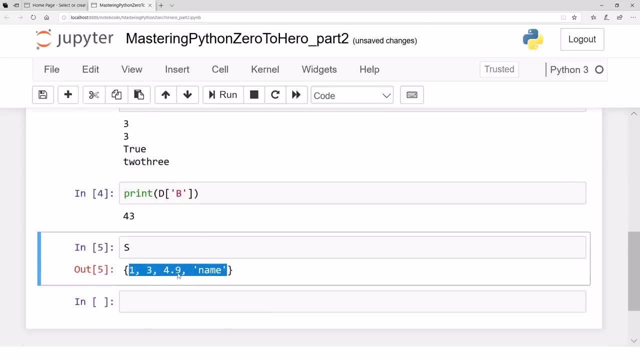 But if you see the elements of s, there are no duplicates and it does not maintain even any ordering. I mean, we have defined s in a different way. It is maintaining everything, maybe in a different way. one, three, yeah, oh, the ordering this. 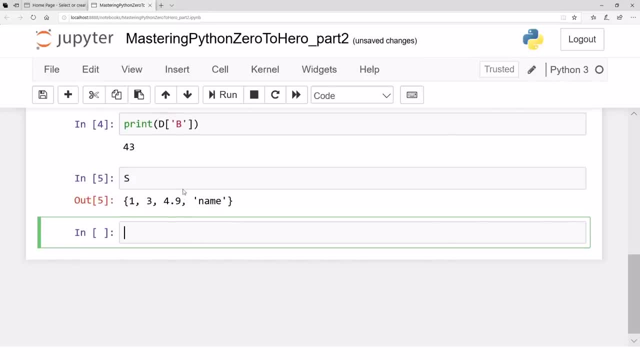 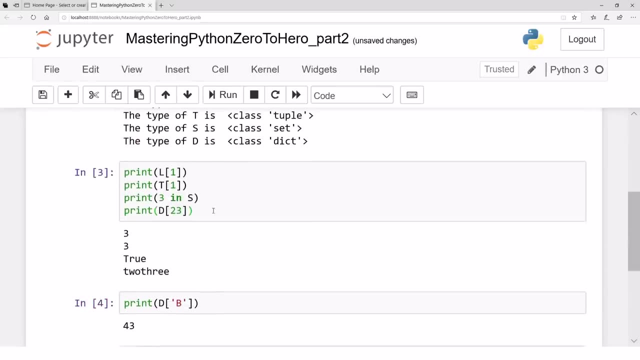 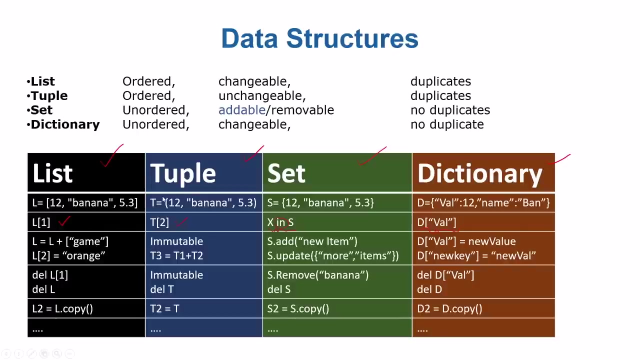 way is the same, but there is no index for the first or second or third element, and so on. Okay, So that's about the defining, declaring or accessing different elements. In the next video, we will see more about the data structures. 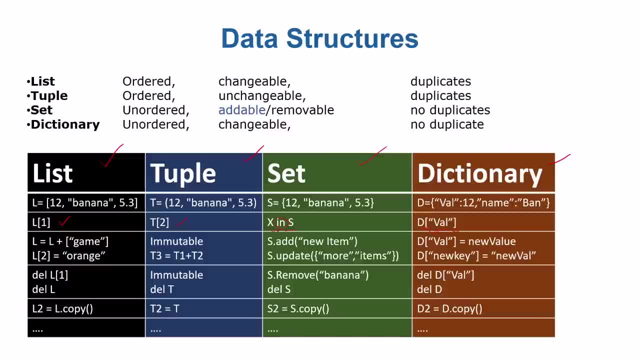 Actually, I want to spend some time on the data structure, because that will be a basic building block for the data science packages. If you know very well about these data structures, we will be very fluent in the data science packages and working with those. 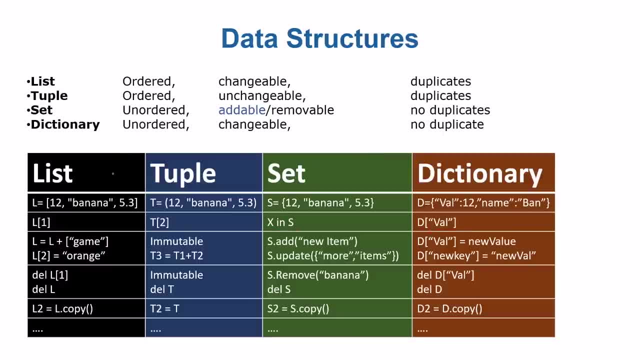 Okay, Hope to see you in the next video. Okay, In the last video we defined list, tuple, set and dictionary and we actually accessed different values. In this video I'm going to actually introduce more indexing: how to access list and tuple. 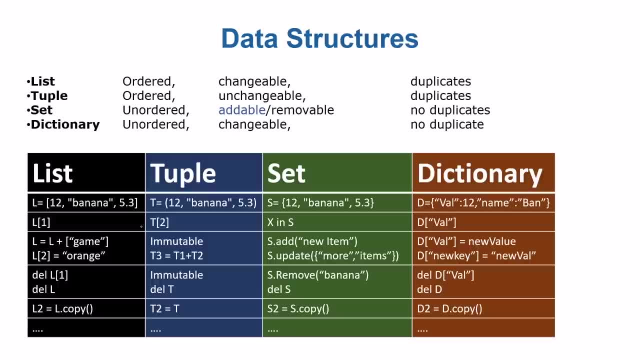 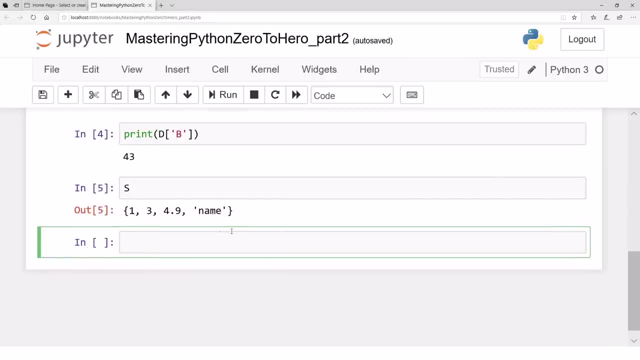 in particular because both are very easily indexable like strings, and I want to show you that all kind of indexing that you have seen- Okay, All indexing that you have seen in strings- exactly works in list as well as in tuple. So let's go to Jupyter and see what a list is. 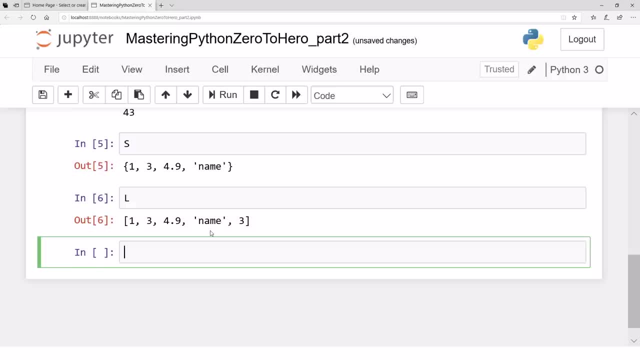 For example a list. if you print the list, that's a list. It has these kind of values. If you just see the list, for example starting from index one ending at index three, that means the same. pick a slice, for example: 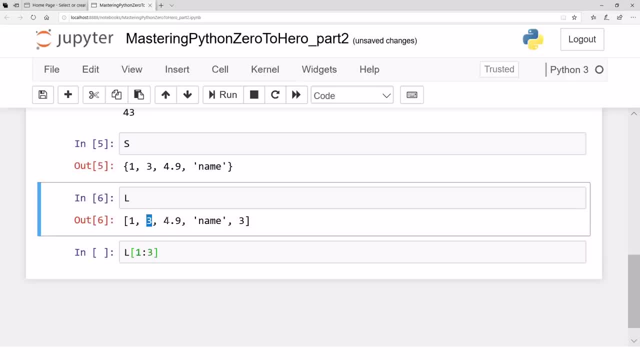 So index one value is three, index two value is 4.9, and the last element is not included. So if you get that, you get three and 4.9.. So exactly the same kind of indexing that you have seen in strings. exactly that is. 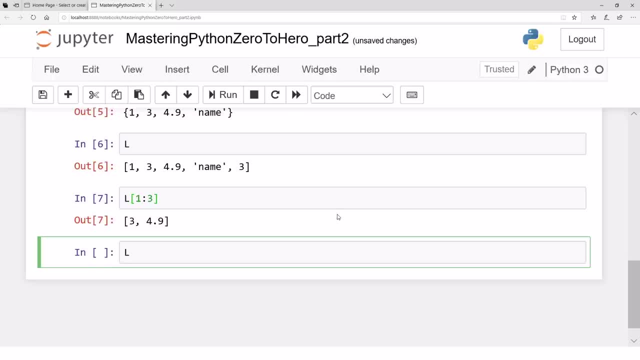 working here as well. So, for example, if I say list, start from the beginning, go to end, but then I just give minus one, it will reverse the whole list. I mean the whole list will be lost. Okay, It will be reversed. 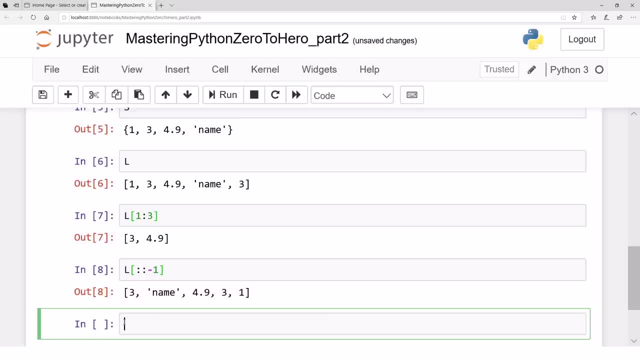 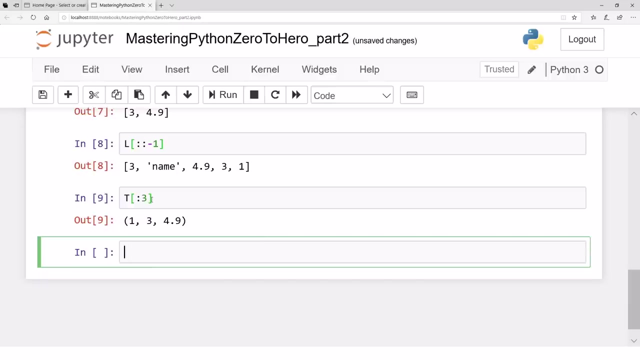 I mean all the things that we saw in string indexing stays exactly the same in list as well as in tuple. So tuple, for example, let's access element from, let's say from the very beginning, till the third element, not the third element till index three, which is actually the fourth. 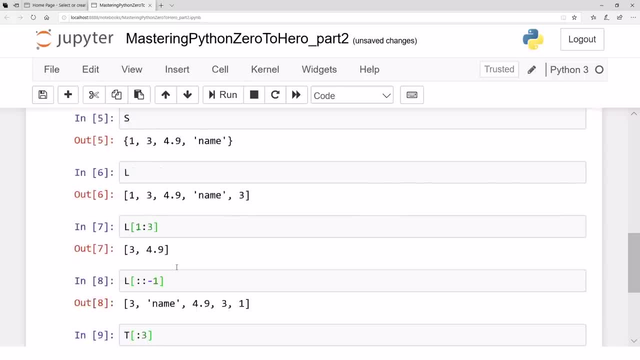 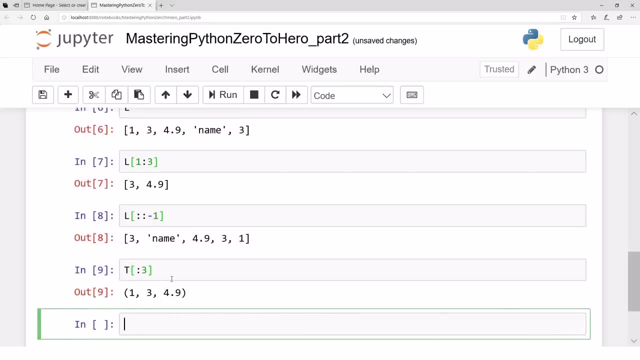 element. So tuple and list, they are exactly the same. They will be exactly indexed as it is. So all the slicing, all the indexing, all the sublistings, all the subtuples, they can be accessed exactly the same way as you've gone through the string. 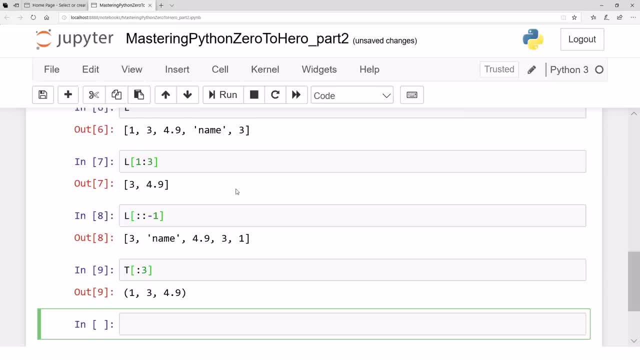 One difference here that I will explain later on. because list is mutable, it is changeable. I will discuss one thing: When you slice it, what happens? What happens When you get a sublist? then actually it refers to the same memory, and if you change, 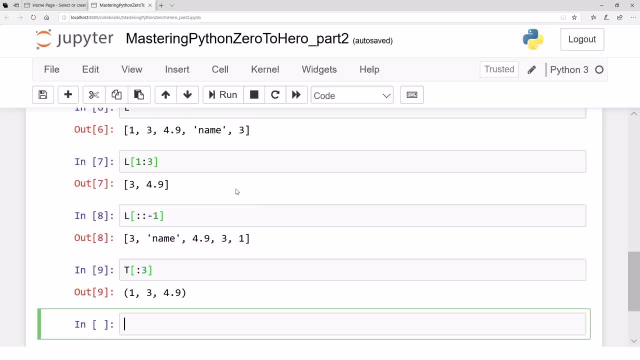 the sublist contents. the actual list got changes. That is true for list in slicing and that is true for sets and dictionaries in the copying, the references and so on. So I will discuss that later on. but rest of the things are roughly the same as they're. 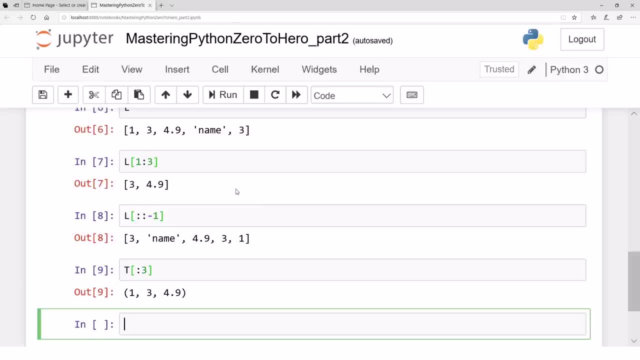 in string indexing. Actually, indexing is almost the same everywhere in Python. It has this kind of slicing. it's almost the same. If you know the index, how to index strings, you know how to index lists. If you know how to index lists, you know how to index tuples and strings and everything. 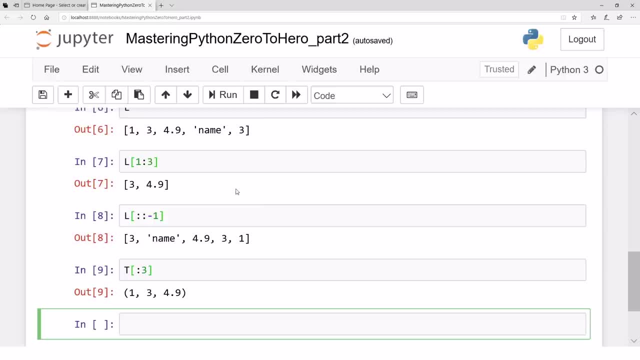 And, by the way, if you know how to index lists, you'll be very fluent in NumPy. That's the very powerful data structure. That's the very powerful kind of array processing. That's the very powerful kind of array processing. You'll be able to get a very detailed package, with some differences that we will see. but 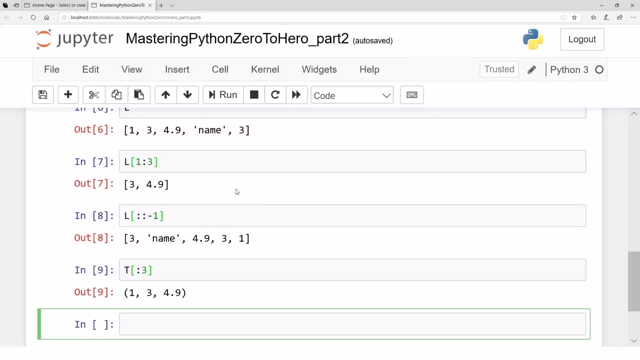 even the indexing is same in Pandas when you are working with a large amount of data, data files and stuff like so. The indexing is more or less the same that you've seen in strings. We will cover indexing, masking and fancy kind of indexing in much more detail in NumPy. 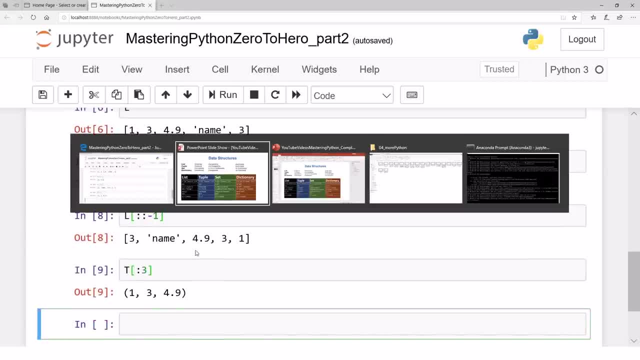 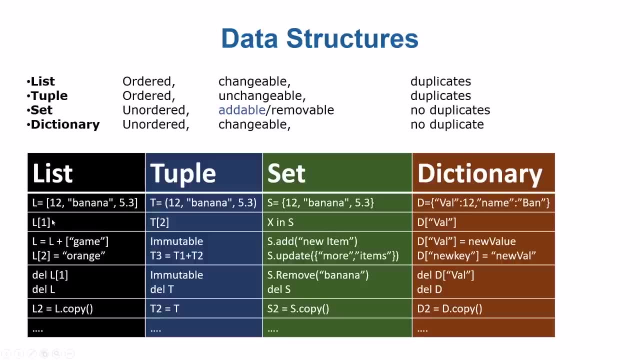 but this stays the same, as you've seen in strings. Okay, So now can we expand the list? can we add more elements? can we insert more elements to the list? The answer is yes, because list is changeable, mutable. you can insert more elements. 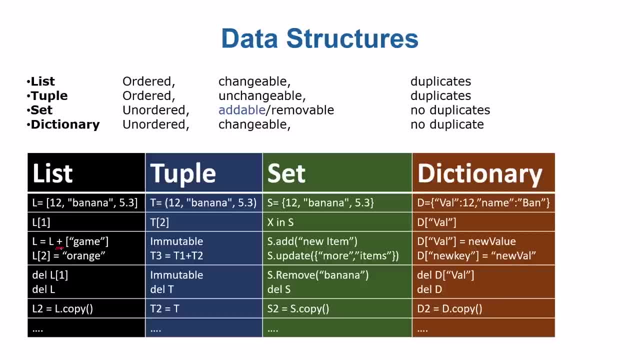 One way of inserting that is just to call an add operator. You just add plus and you just insert another list. So like two strings are concatenated by plus, two lists can be concatenated or combined together again by plus. But there is a faster function called append lappend. that is sometimes faster than using 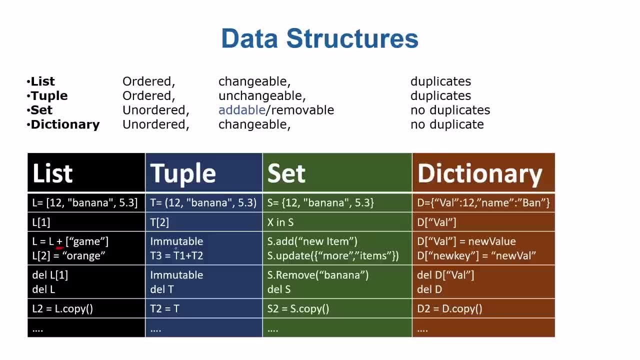 this operator, We will see that Tuple because it is immutable. you cannot touch any content of the tuple. You cannot actually insert any element to a tuple. you cannot delete any element to a tuple. There are workarounds, for example, convert a tuple to a list, change it, then convert. 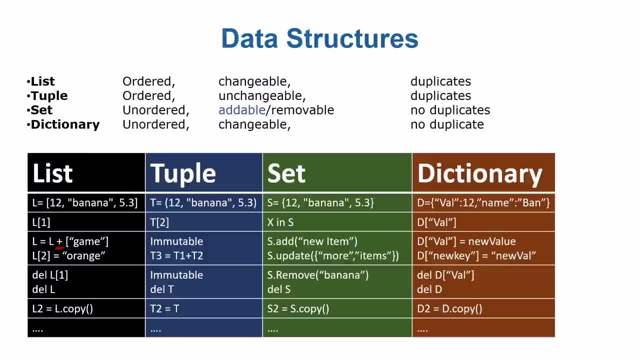 the list to a tuple. There are ways to do that, But tuple in its true form is immutable. In its true sense, in the literal sense, it is immutable. You cannot insert any element, you cannot delete any element, you cannot change any. 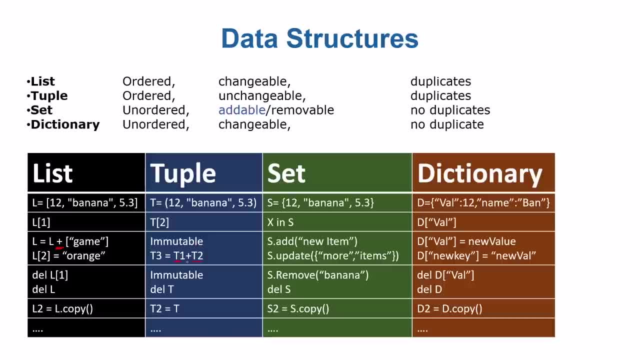 element. However, you can combine two tuples together. you can concatenate two tuples together again by plus operator and save the result into a new tuple. that's possible. You can insert elements using an add function. Add function allows you to just insert one element. 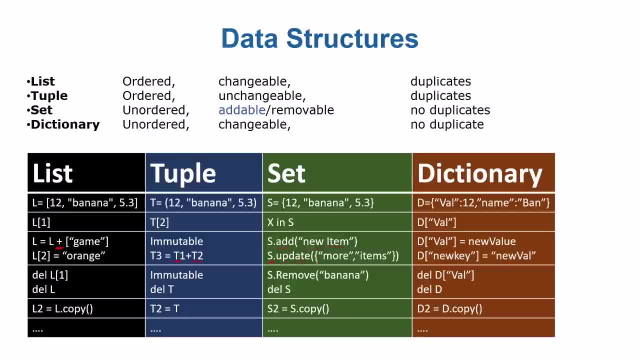 If you want to insert more than one element, then you can call an update function that actually accepts more than one element, That accepts another set that needs to be inserted. That's possible. Dictionary: you can insert a new key by just d. 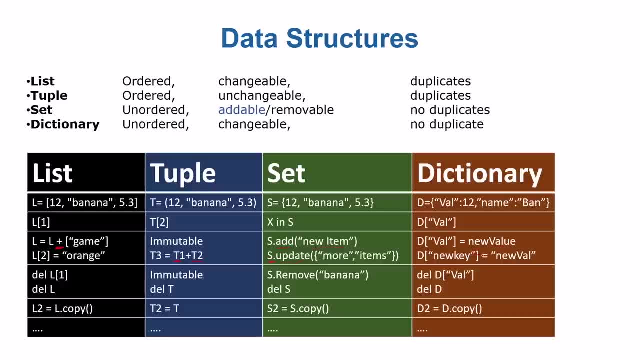 New key equals to that. You just assign a new value to a new key and the key value pair is just inserted there. Great, You can delete or remove any element from the list using del command, Del l1.. That means this particular element. 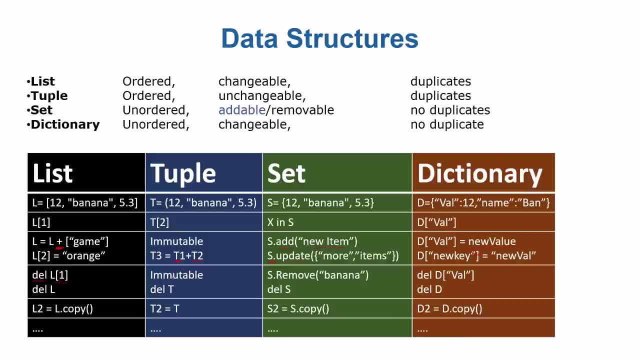 This particular element is deleted from the list. that is possible. Deleting particular element from the tuple is not possible. however, you can delete the whole variable, whole tuple. that is possible. You can remove elements from the set using remove function, sremove, and then you just. 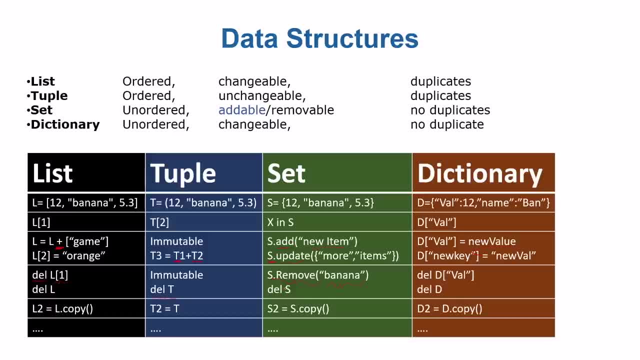 give the element that you want to remove. that is possible, it will be removed And you can delete the whole variable. that is always available. Similarly, you can delete a particular item from the dictionary By just deleting, by just calling the d of the value, for example, whatever the key. 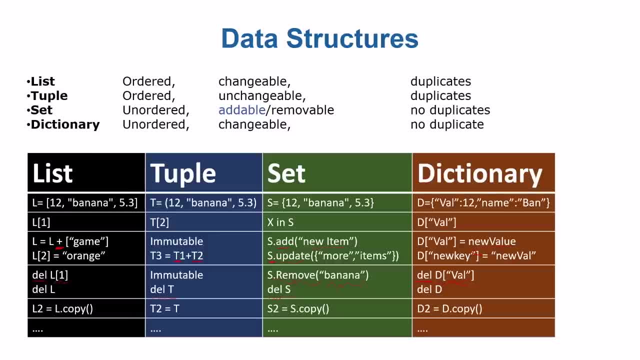 is So you call with the key and call the delete and it will delete everything I want to mention here to remove items from the list. there are other methods and functions that are also available. that I mean there is a remove function, there is a pop function. 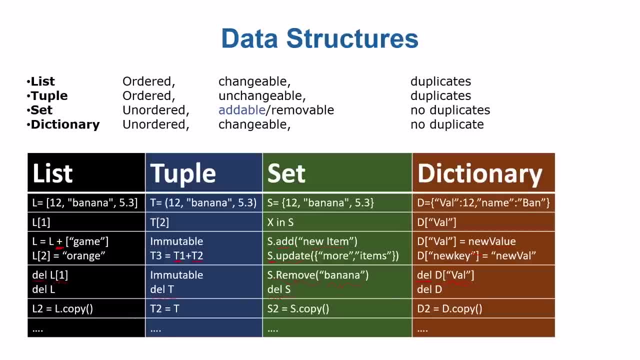 These are available. Similarly, from removing elements from the dictionary, there are other functions that are available. To compare them together, I'm using this del command, although there are other ways of doing the same stuff as well. So let's end this video here, and in the next video I will show you all these operations. 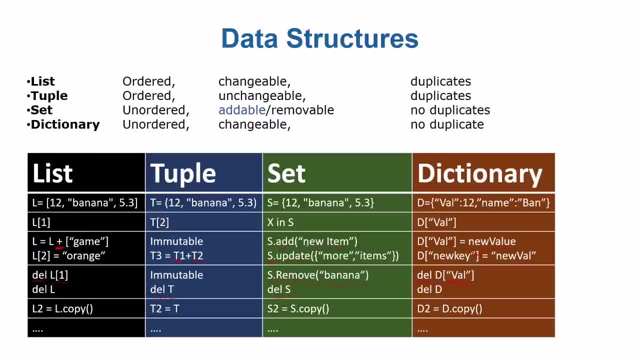 that, concatenating together, inserting more elements, deleting different elements. I will show you all these things in Python, So hope to see you Bye In the next video. Okay, in the last video we saw how to insert different elements to different data structures. 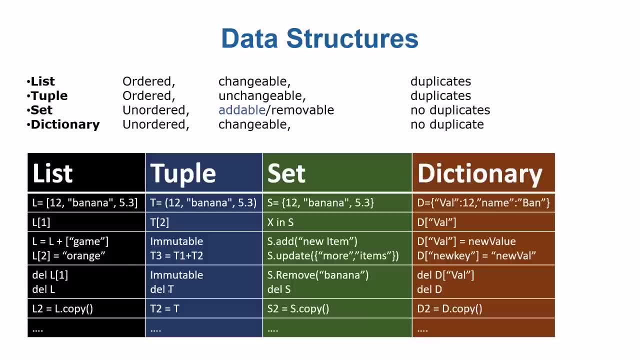 And, for example, in the case of tuples, it is not possible, and we also saw how to actually delete different elements wherever possible. So let's go to our friend Jupyter Notebook and see all these concepts in a running form. 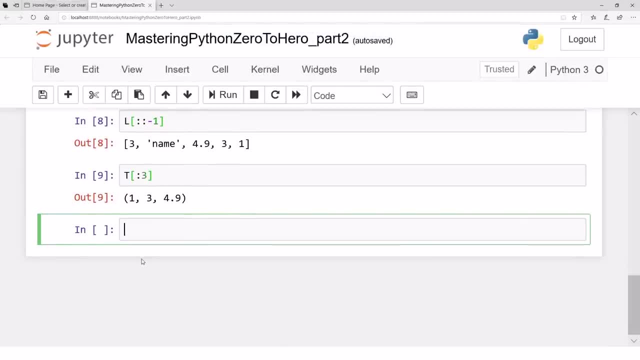 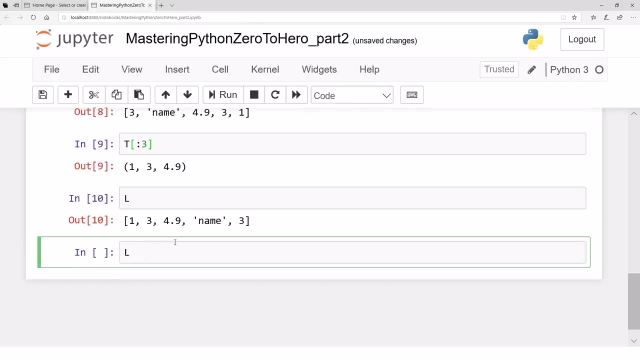 So let's go Okay. So let's: for example, we have list, that's our list, We have our list list. Let's append an element to the list, or maybe more elements. That is L plus. let's say we can have another list, For example how R, that's six, and then U. 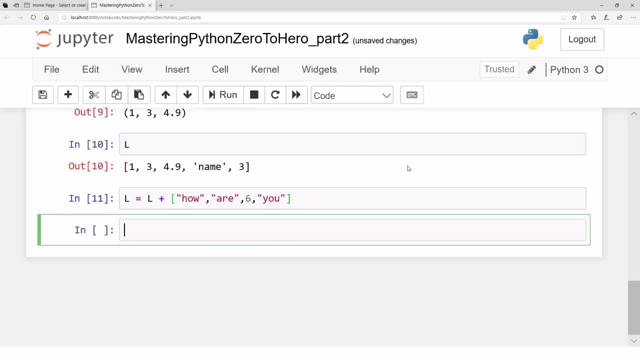 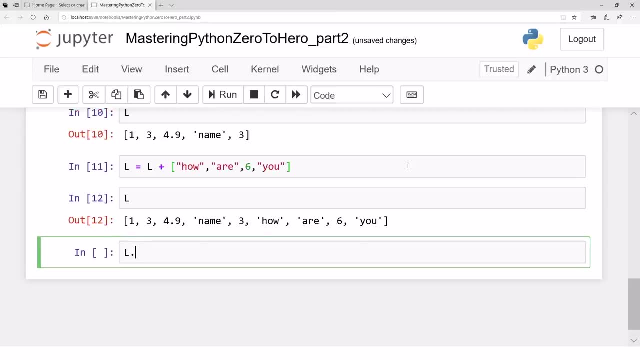 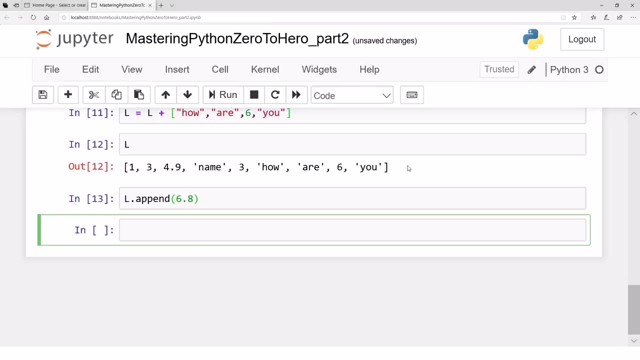 That's it, And these two lists will be appended And the new list will be, as you can see this. Similarly, we can append an item using append function, For example, 6.8.. That will also be appended and the list will contain these kind of values. So yeah, 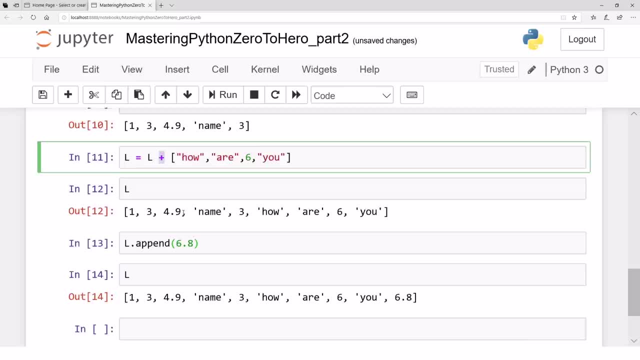 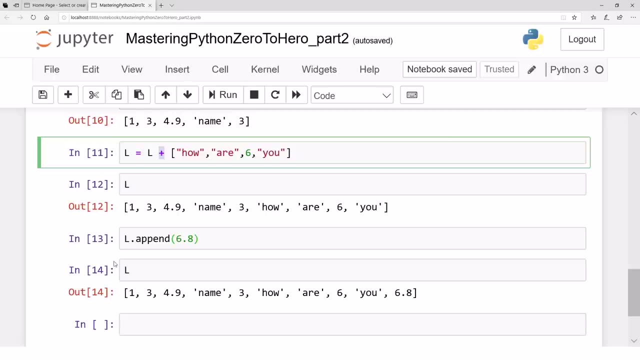 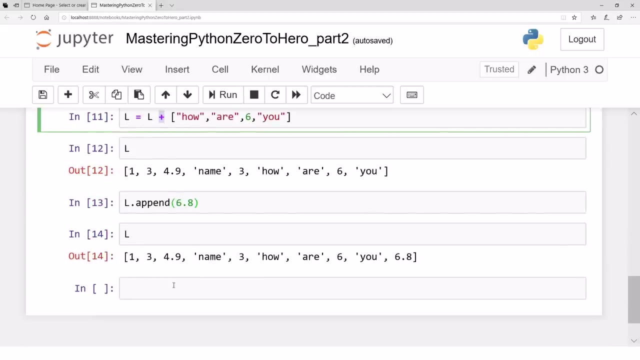 so both ways are fine. This plus is: this plus can be used to append to lists and this append function can be used to simply append a list with a list. So that's it, Thank you, With an element, Okay, great Tuples. you cannot change a tuple. You cannot change a. 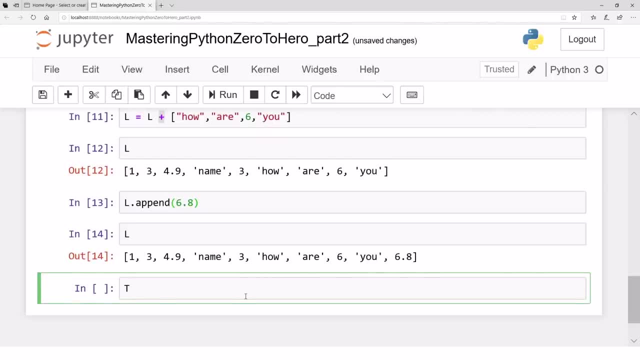 tuple. But what you can do is you can have two tuples. For example, T2 is a different tuple. Let's say A and B, And let's say you have 45. Let's say that's tuple 2.. Then you 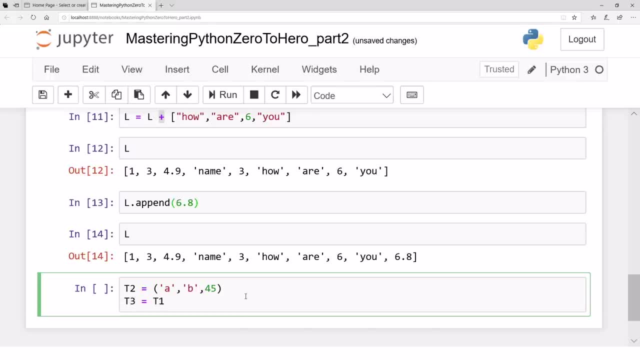 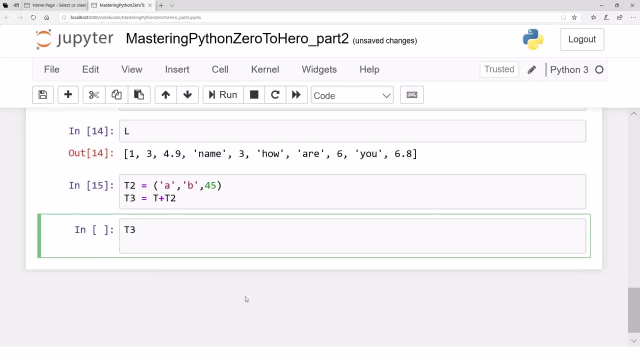 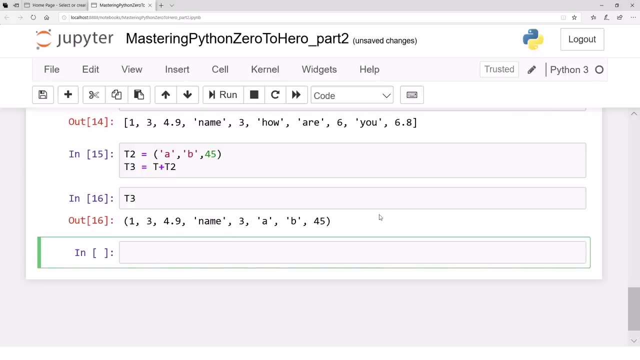 can have a third tuple, that is just the combination of tuple 1 and tuple 2.. And in this case you have tuple 3, which is this: Yeah, So tuple 1 and tuple 2 are combined together, but you can not actually insert into the tuple. The tuple is immutable. 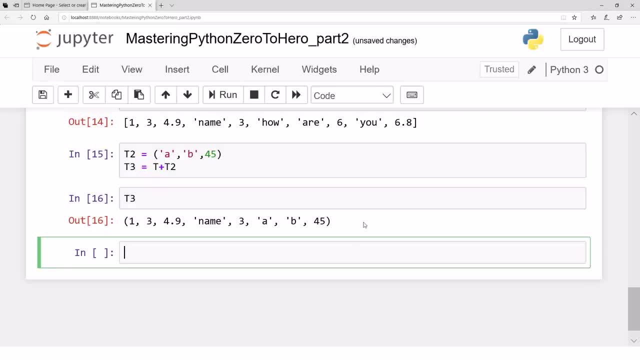 You cannot insert another element, You cannot delete the existing elements, You cannot update any elements, and so on. Similarly, S the set. Let's see the state of the set. That's the setsetadd function. You can add anything, Let's say 56.. That is added there And the 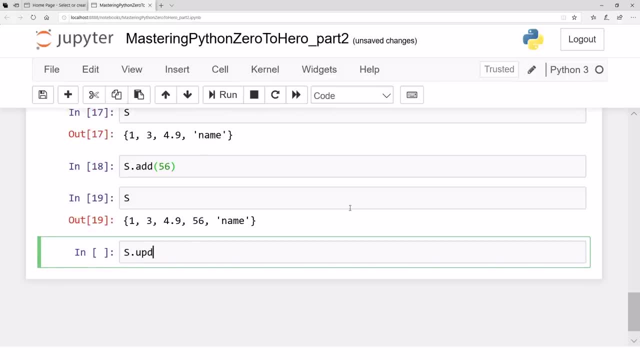 new state of this is this: or you can call the update function. if you update method, if you want to insert more elements, for example, if you have multiple elements to be inserted- 23 game- and let's say you wanted to insert an element that is already there, so, for example, one- then 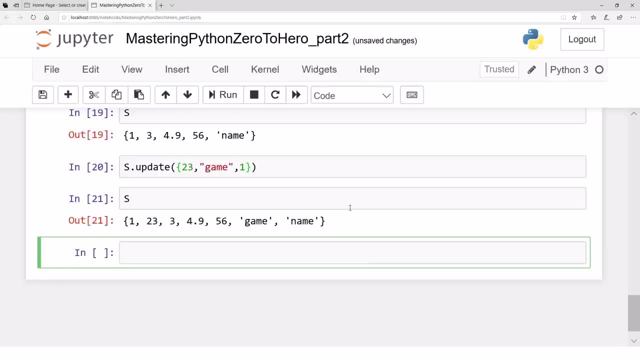 the duplicates will no longer be there, but the new elements will be inserted. now let's see the state of d. the state of d is this: if you want to add another key value pair, you can add a key here. for example, a key might be a new key, for example, new key and the value might: 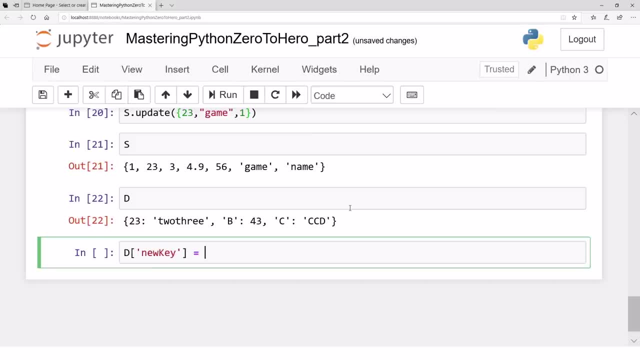 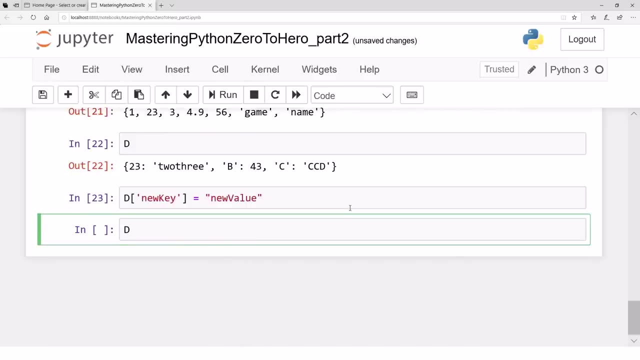 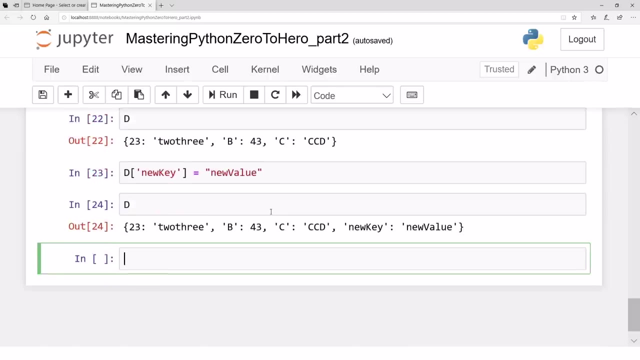 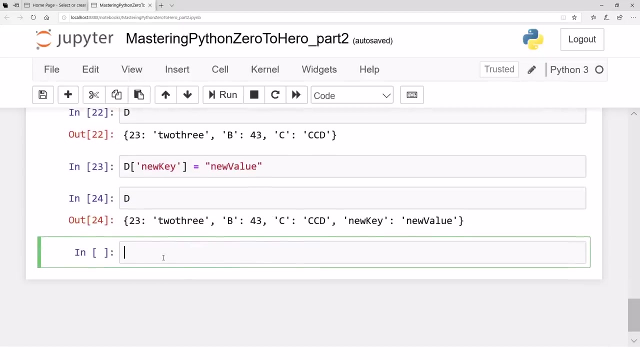 be the value might be, for example, a new value. well, and now, if you see d, the, the d, the contents of the d has changed, changed. wow, that simple. um, yeah, great, uh, can you concatenate two dictionaries together using a plus operator? is it possible? um, is it possible to concatenate two dictionaries together? 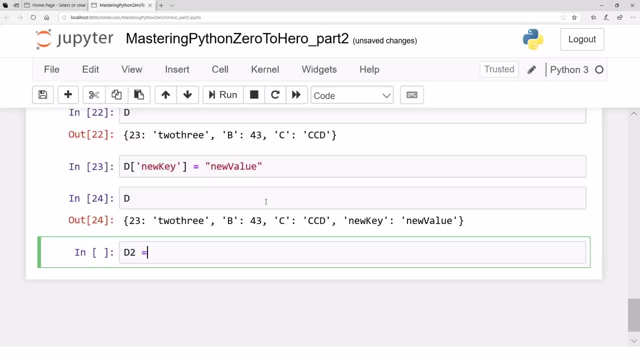 let's say i have another. i have another dictionaries, dictionary t2. um, that is, let's say the key is y and the value is yy. and then we have another key, let's say z, and the value is: let's attend. can i concatenate d and d2 together? can i? can i just update my d? 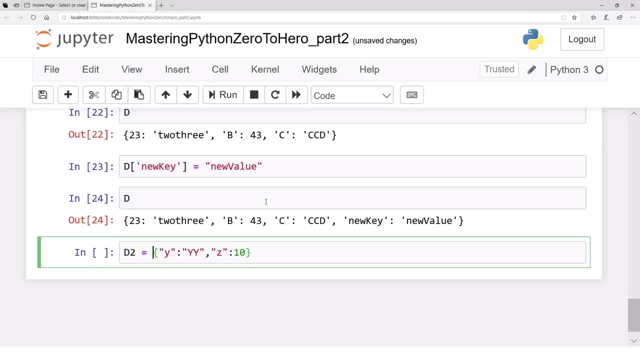 and add these values. insert these values also there. okay, i left you with this question. you try to answer this and in the next video i will answer this question, but try to answer this question yourself, and one way to try that is just to go in jupiter and just type and check whether plus is working or not, or maybe. 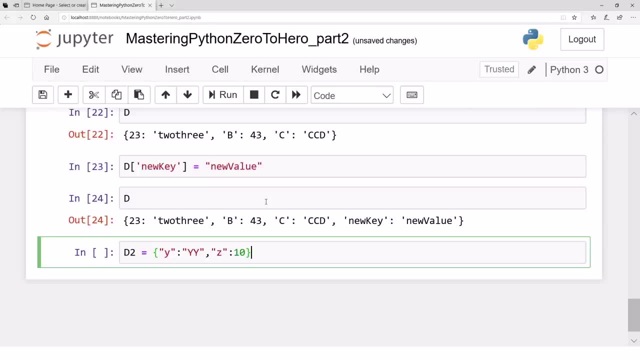 there is another method and stuff like: so okay, great hope to see you. oh, i have not used the del delete and all that stuff and so on. so this question is there. let me use the removing the elements. so let's say l is this list. if i want to remove any element, let's say element. 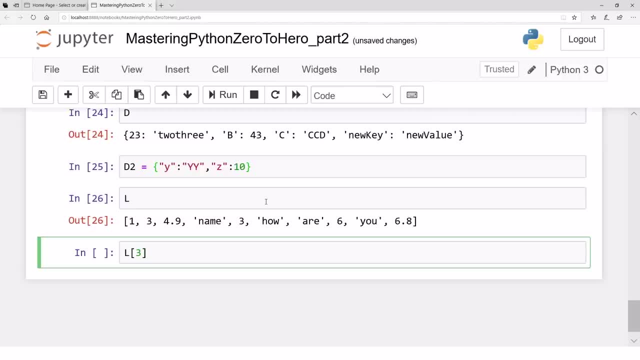 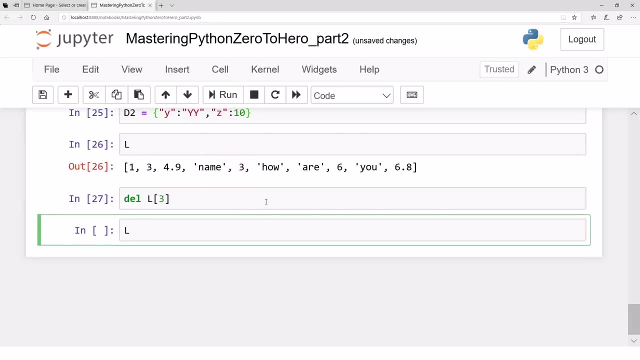 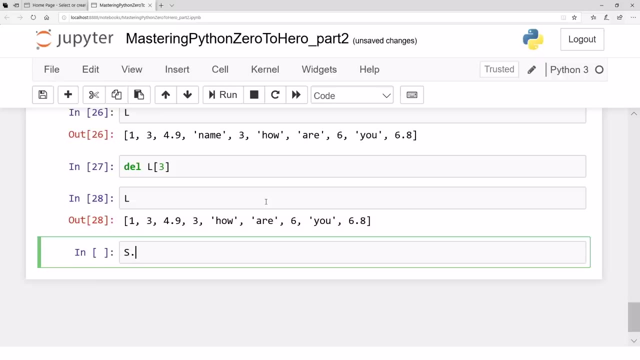 number three. if i want to remove element at index 3, which is this string name, i can use simply this delete and the l is everything, but without that element similarly i can remove. if i want to remove any element from s, i can call the function remove and whatever i want to remove, let's say i want to- 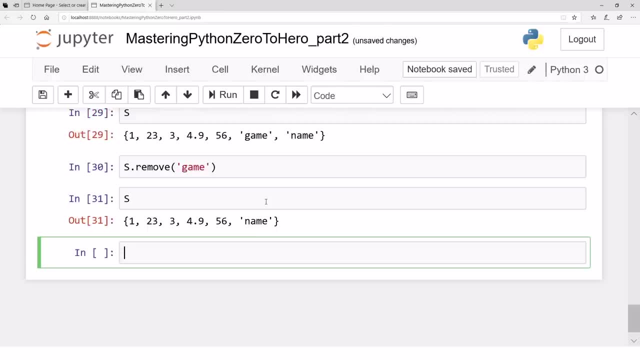 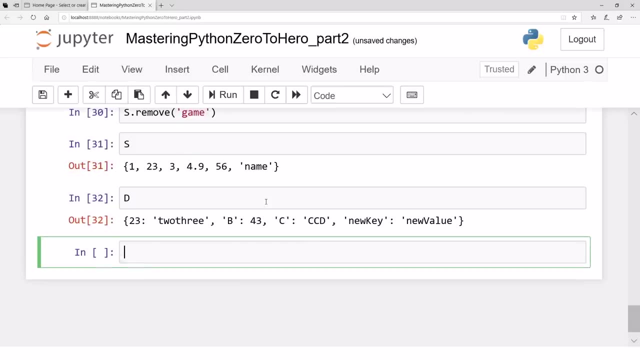 remove game and the game will no longer be there. great, if i want to remove some element from dictionary again, let's say that's the. that's a view of dictionary. i can call d and i can. i can remove the element with key. let's say c, whatever the element is, with key c, delete that element. 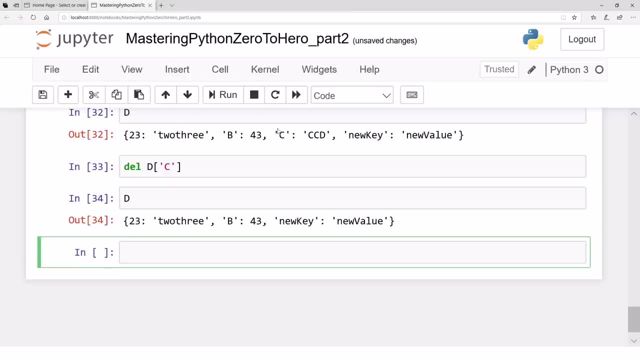 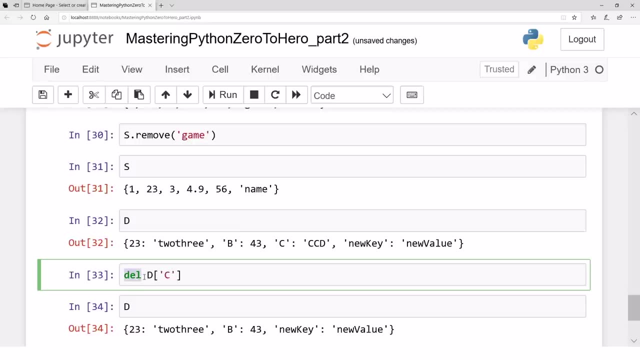 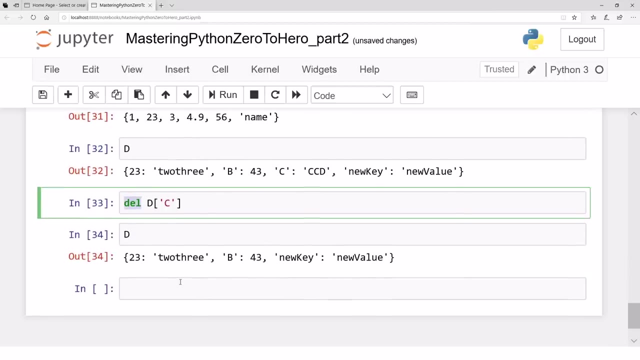 and the dictionary has this particular state with this item. this particular item is gone. okay, great, i can do that, but but del is not the only way of doing that. there are so many methods- i mean a lot of methods- to do that. but just to just to compare all these, i am just giving you the most similarities and 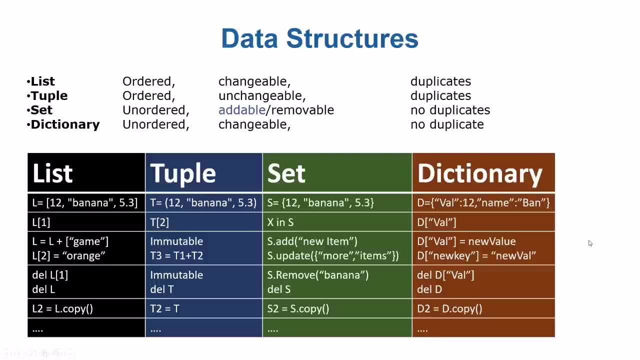 differences wherever available. okay, great. so i have asked you a question in this particular video: can we concatenate two dictionaries together, particularly with a plus operator? if yes, then we are done. if not, then are there other ways and stuff like that? so i'm going to do that. 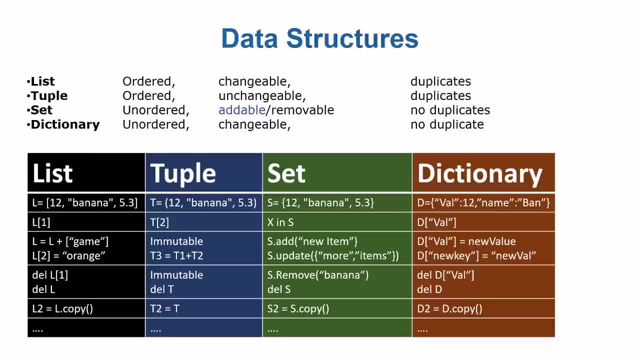 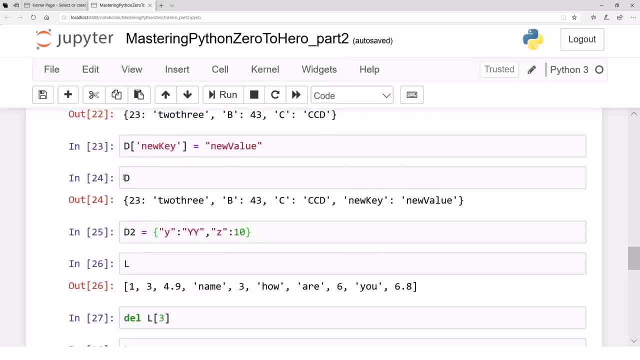 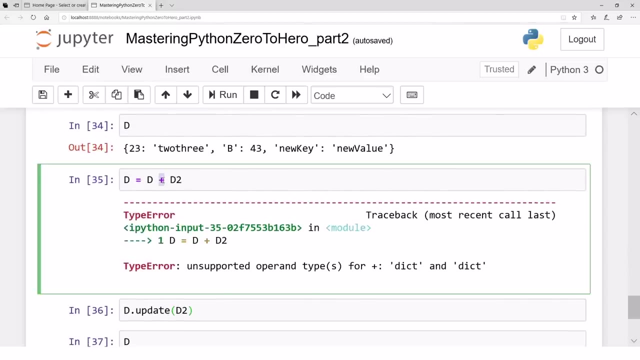 so that's the question. so hope to see you in the next video with more on these data structures. okay, uh, i asked you a question last time: can we concatenate this two dictionaries together with a plus operator? so what's your answer? um, yes or no? the answer is no. yeah, so we cannot concatenate them together. we cannot insert another dictionary. 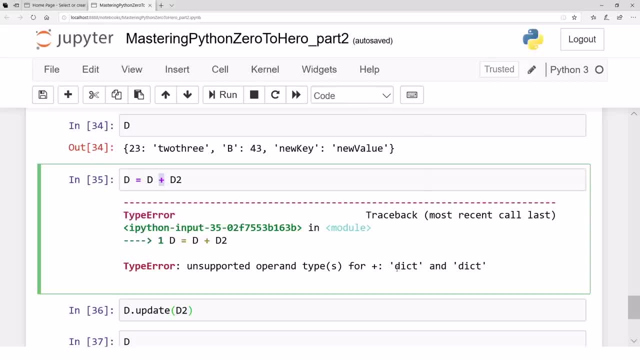 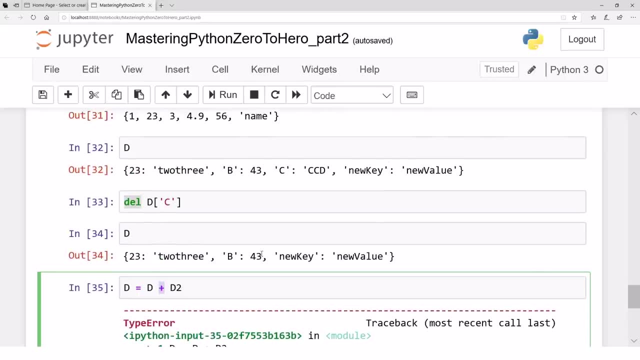 to this dictionary using a plus operator, because this plus operator is not defined for dictionary. what we can do is we can call an update function, because dictionary is also a set, i mean a set of key value pairs- but at the end of the day it's a set with specialized function, of course. but we can. 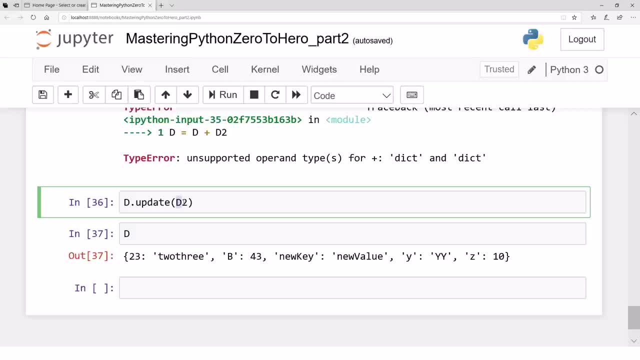 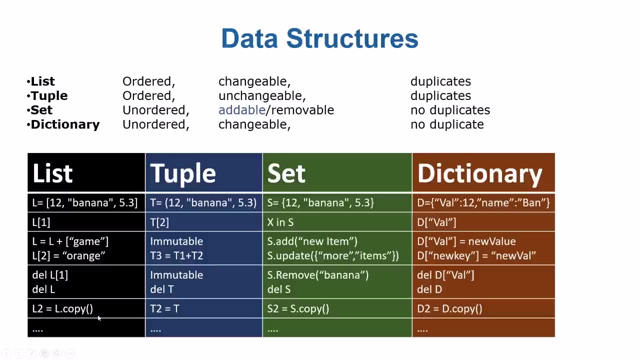 call update functions and insert the whole new dictionary inside dictionary as as as follows: yeah, so the answer is using plus operator. no, but there is a way using update method. great, so next we we focus on the copy function. the copy function is available for list. the copy function is available for set. 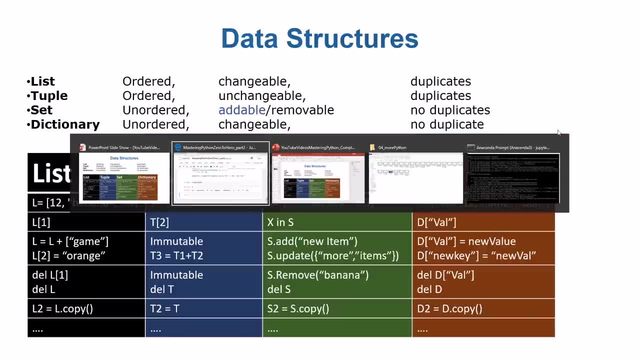 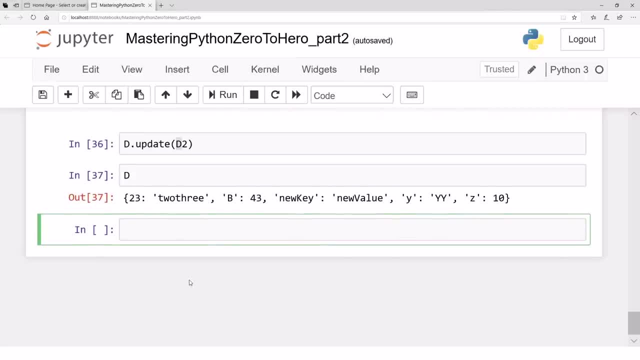 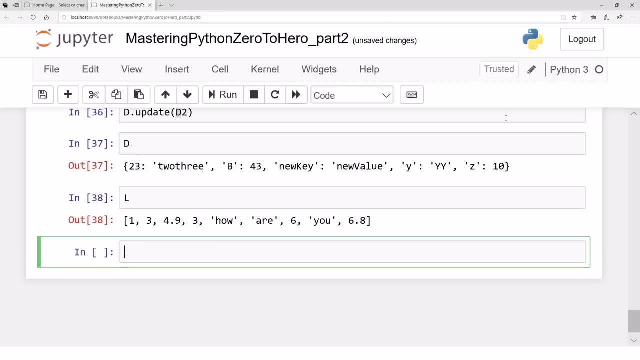 the copy function is available for dictionary, so let's see the need of this copy function here. i want you to be very careful, uh, because, uh, that that's really important. uh, let's say we have a list, let's say that's list. and, by the way, the same goes with set and dictionary as well, whatever. 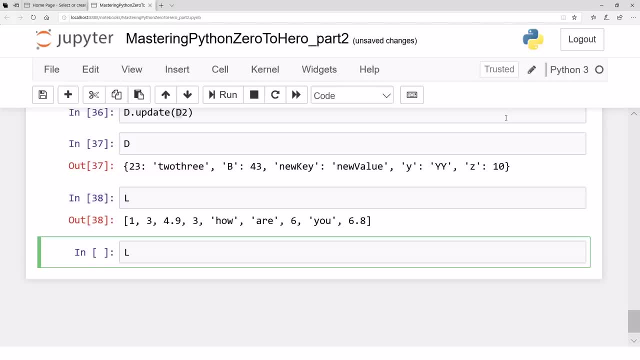 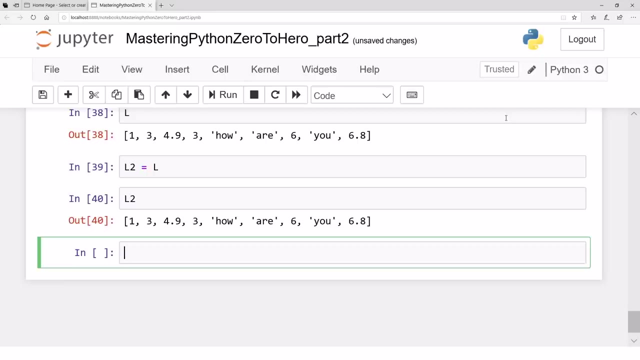 i'm going to do with list. let's see a list now. what you do is you copy the list or you just make another variable. like you can assign the value of l to another variable, l2. what you do is that now l2 is also is this: now these are two. 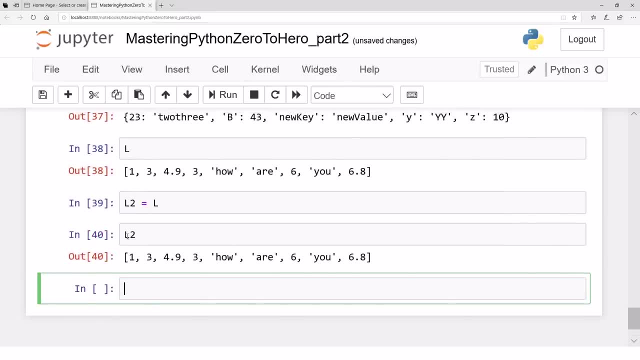 different variables. l is this variable, l2 is this variable. so you might be thinking l2 is separately, completely a new thing, and l is a new thing- you might be thinking that both are independent. right, but you also have three new variables. if you use a new variable- l2, l2, which is it's 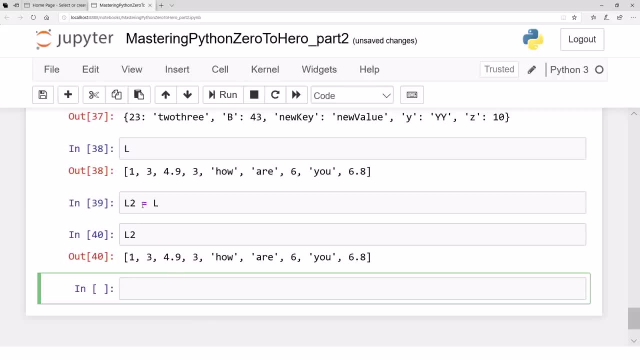 different and you add a new variable: l2, l2, l2- that's actually a new variable, l1, which is a new variable, so you can't use it in this way. but the data structure is a collection of a lot of data it has. it is consuming a lot of memory. what it does is when you assign a variable or data. 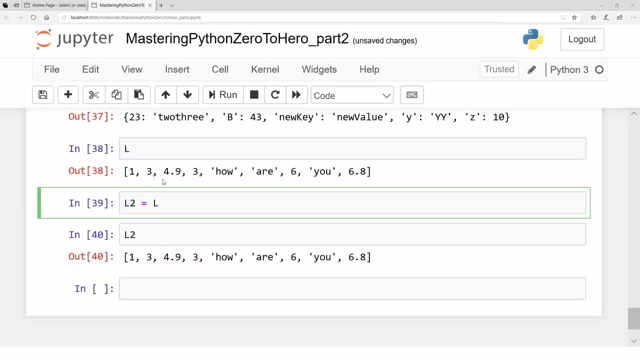 structure to to another variable. it does not actually copy all the contents, it does not actually make a new memory, points to the same memory as this. And the consequence of that: if you change any value, for example in L2, let's say you change the index to value form, the index to value is: 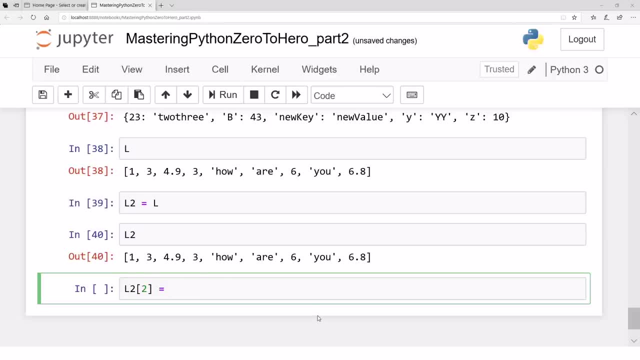 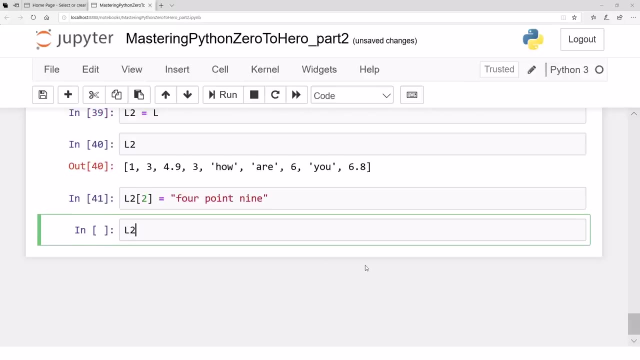 4.9,. now you're working in L2.. Let's say, you change this L2 value from 4.9 to, let's, 4.9.. So you do that. So you might be thinking that this happens in L2.. Well, in L2, that has happened. 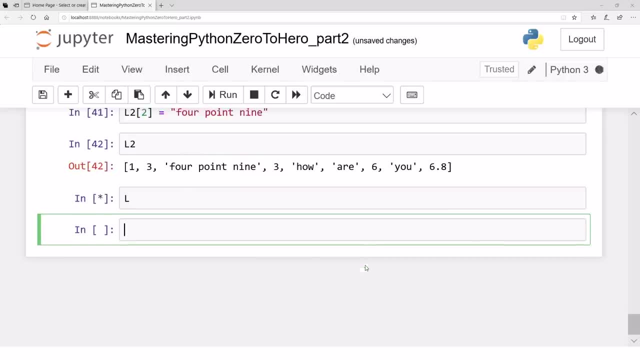 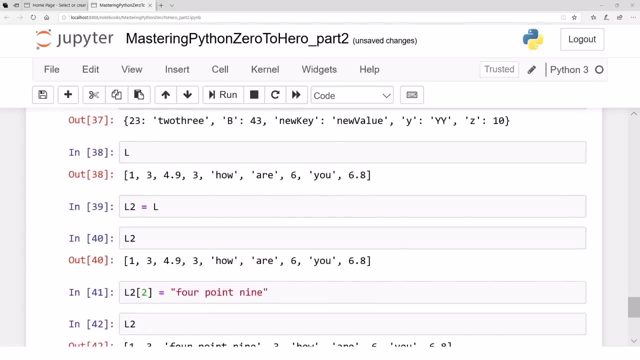 But what it also does is it does the same thing in L as well, So L also changes. The reason is L and L2, they both are pointing to this structure in the memory, And whether you approach that structure through L or you approach that structure to L2, you're approaching the same. 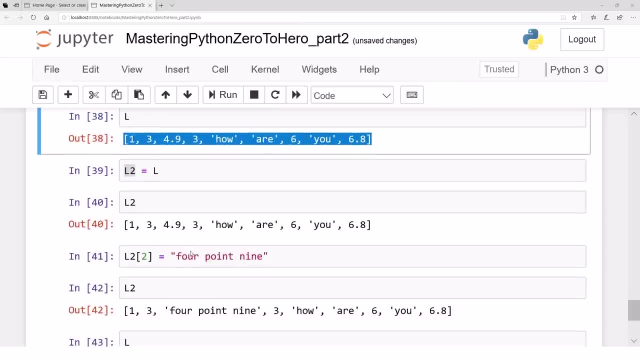 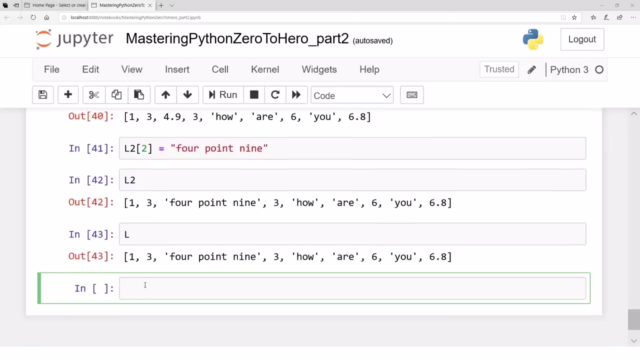 memory Anyway, and that is called referencing. I mean it does not create the data, it actually create a reference in the memory to actually create a new name for the same memory And both are pointing to or accessing to the same memory And, if you really want the behavior so that L2 becomes different, 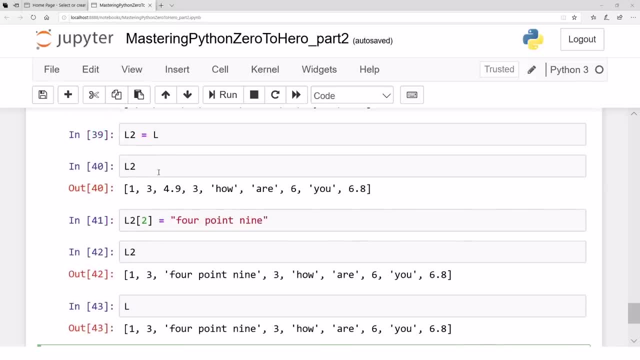 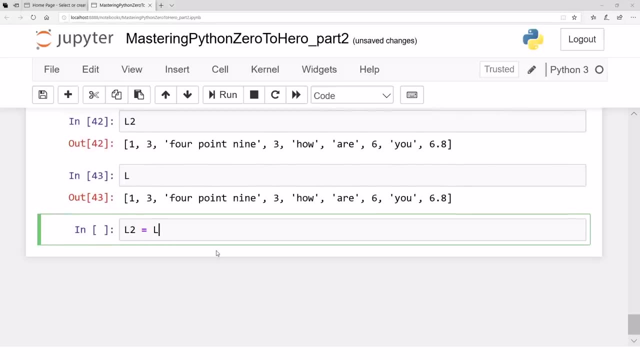 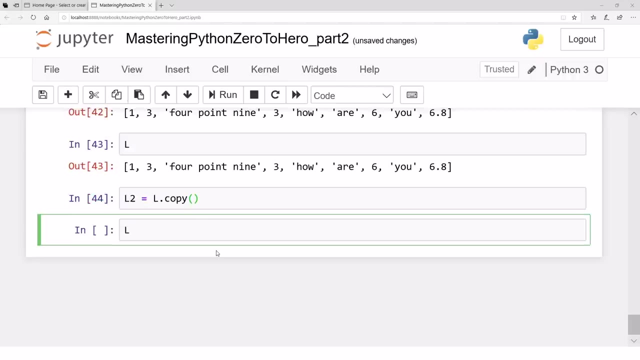 than L, and whatever I do with L2, that should not affect L. then you should call copy function. L2 is L dot copy. Yeah, So that's the function L dot copy. Now you have L2.. Now you do whatever. 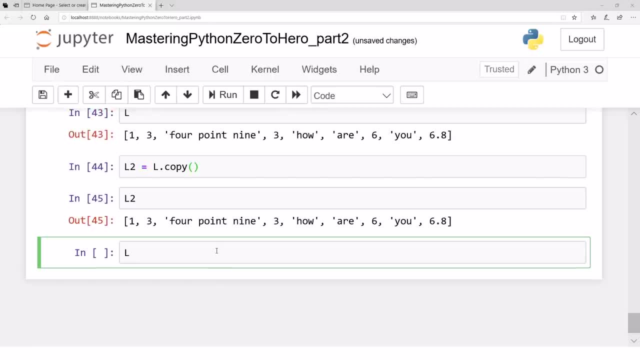 with L2, it will not affect L. So L2,, for example, index at index two, you again say, okay, this is 4.9.. So L2 changes Now, L2 changes, but L doesn't change. 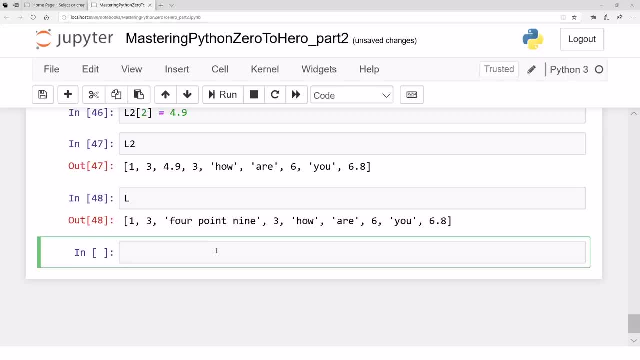 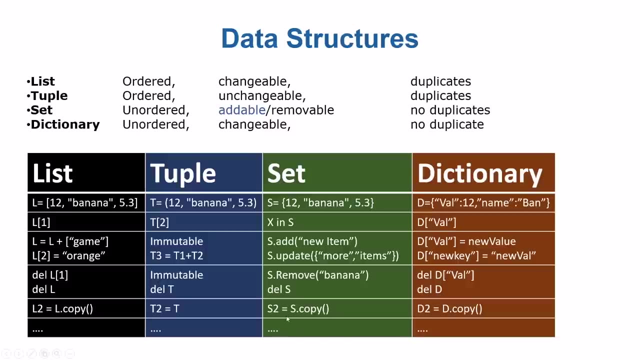 L doesn't change, L stays the same. Now this has different copy. Same concept: go with the set and same concept go with the dictionary. If you just make another variable, S2, and equals to S, then if you change the contents of S2, S will change. If you don't want that, then copy it Similarly. copy. 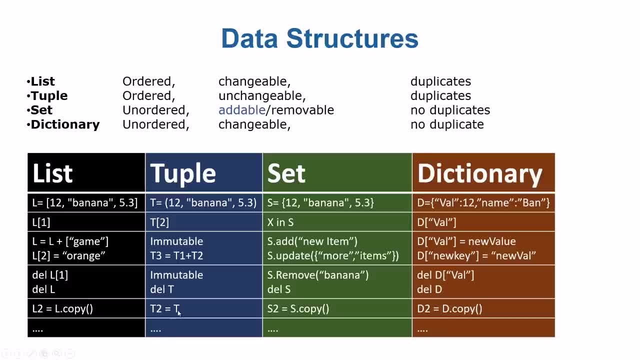 the dictionary Because the contents of the tuple, they are not changeable. the copy function is not available for tuple Because even if you assign this T to T, you can now not change T2 because it is immutable. So having a copy function doesn't make sense in. 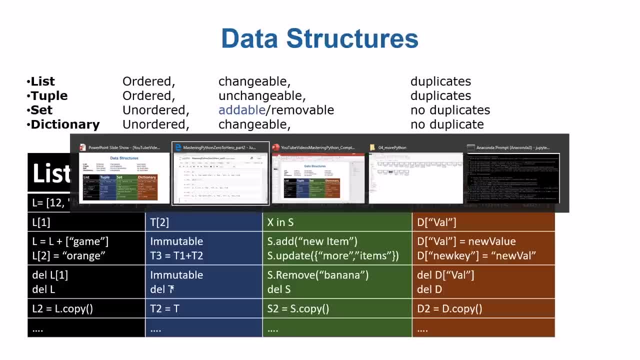 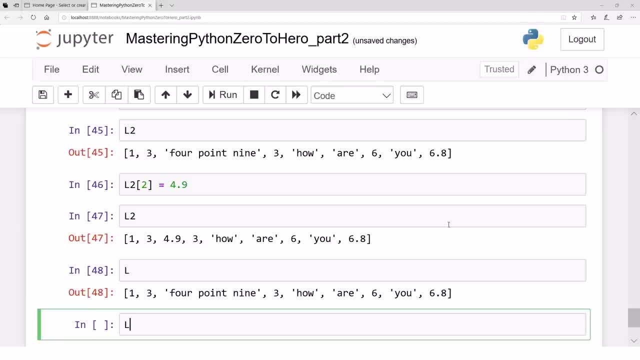 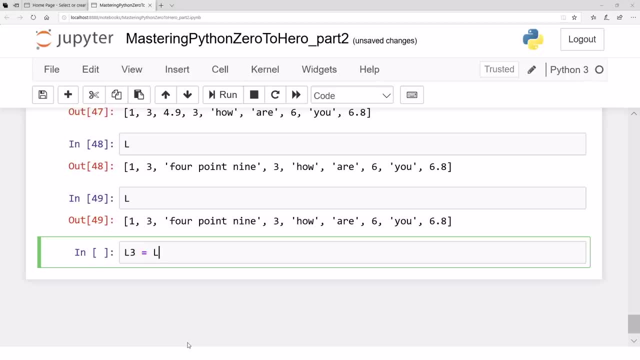 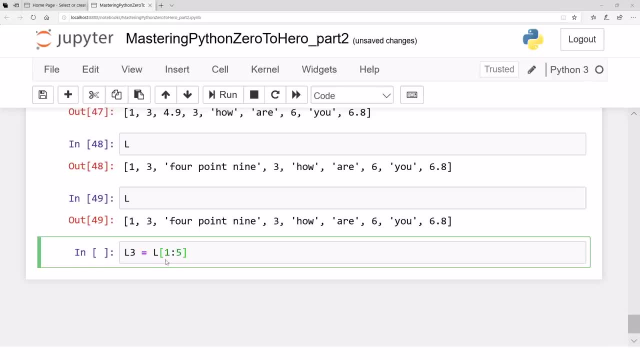 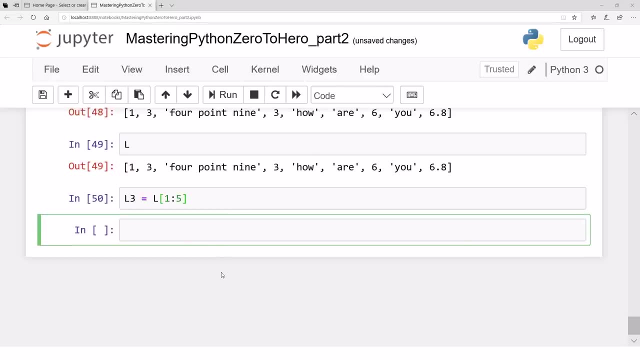 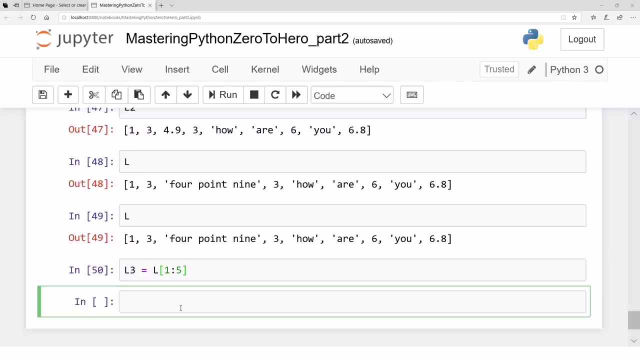 one, two, five, Let's say. So you start from index one, which is three, and you go to five by not including five. This way, the L3 is automatically a copy. It is not a sub list which is referencing. So L3 is a different. L3 is a completely new list, a new memory view. if you change the contents, 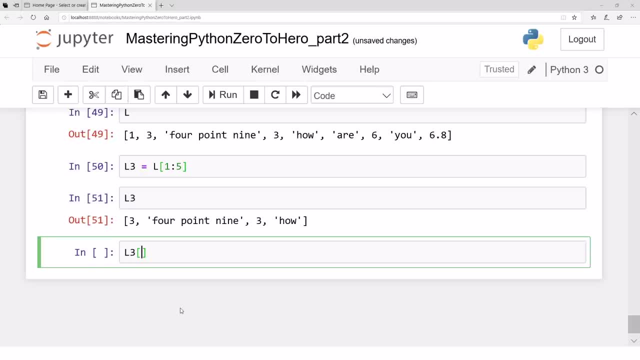 in L3, if you change the contents in L3.. For example, if you change the contents in L2, for example l3 at index 0, it should go from 3 to, let's say, 3 if you change the contents. 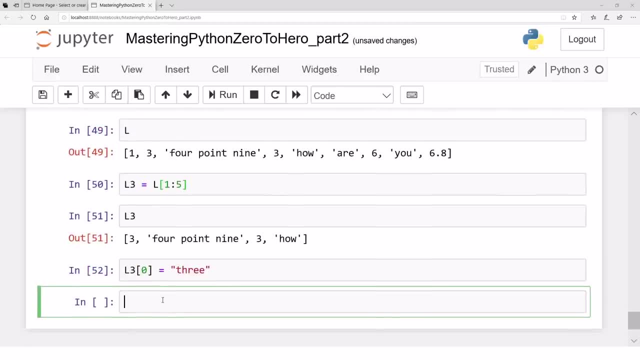 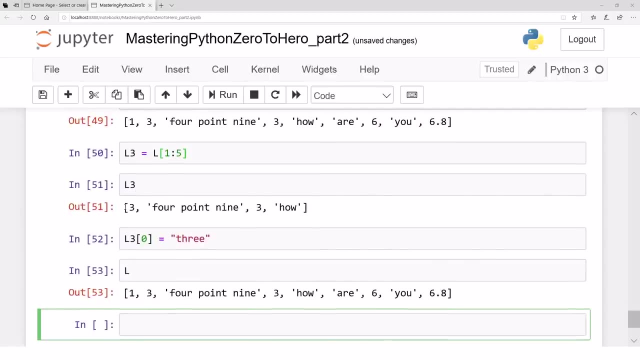 in l3. these contents, these change will not reflect in L. so if you do the slicing, slicing picks a copy by default. it does not fix a reference and that's a huge difference between this list and a numpy array. when you and we will see that, when we will see a numpy array, the slicing actually also again refers to: 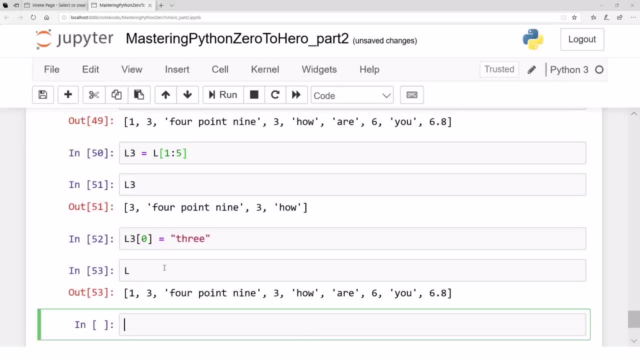 the same memory location and that might be one difference in indexing, indexing in the whole Python. whenever you do slicing you get a copy. but in numpy- when we'll see numpy in detail? in numpy when you do slicing you get again a view, not a copy. and if you change in the sliced for Ian, anything the actual, the actual. 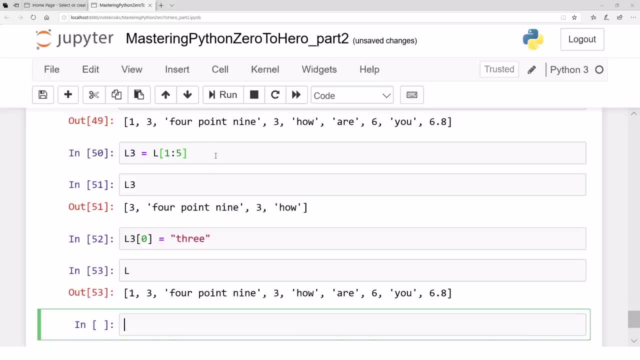 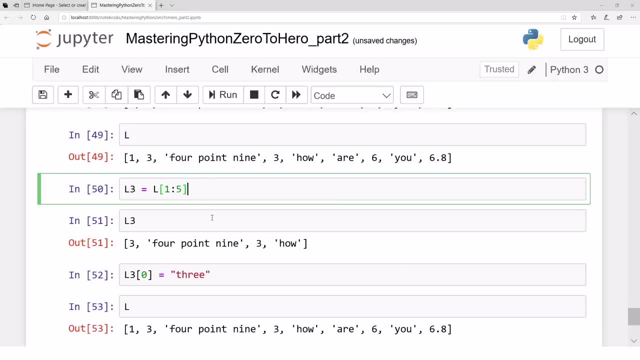 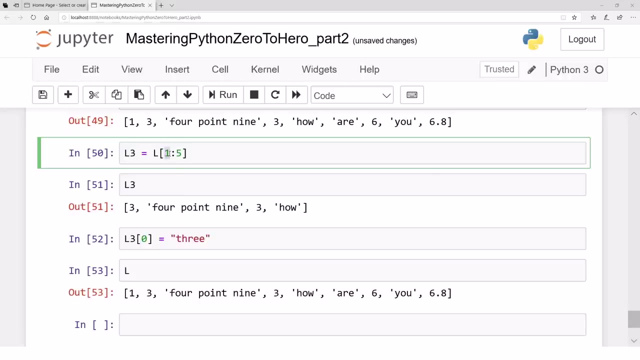 contents also change, change and there is a reason to do that, there is a there are efficiency reasons to do that and stuff like so again, the dot copy function becomes the copy function become more more applicable there as well. so so so you need to know that even if you do, if you do, slicing in general in Python, in any collection in 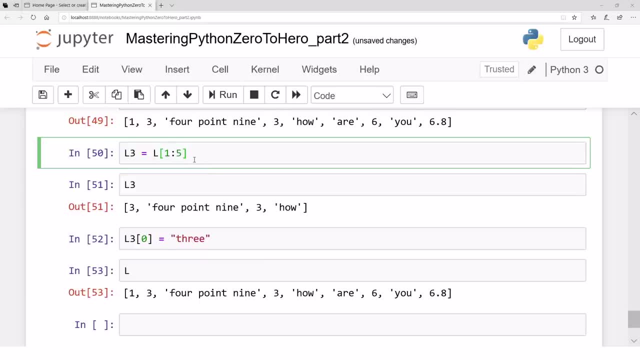 any array in any. if you do select a collection for, even for mutable objects like list, you get a copy. but in numpy array, the, the things, these things, this particular thing with with a lot of other things, this. but this indexing scheme actually changing changes with, with this kind of? 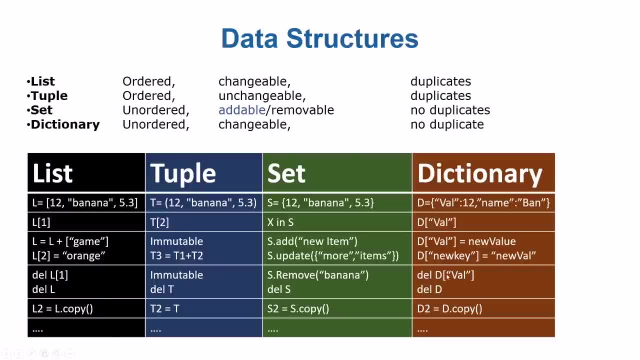 slicing. okay, so I am this video here. I mean, you can explore much more functions of list, tuple, set and dictionary and what you can do with each of them and what you I mean in which scenario, what kind of thing is more suitable for the other. that completely depends upon the problem, and 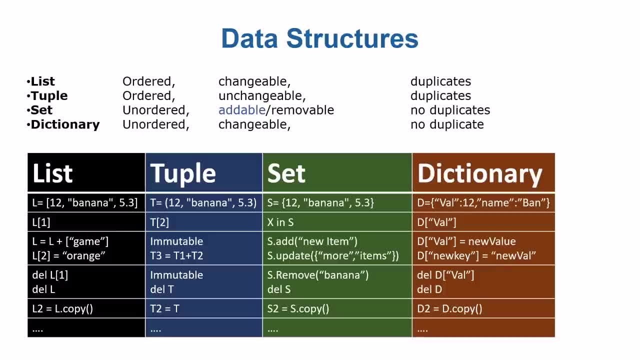 hand, but what we can do in what, what we will do, what we'll be doing in the last next video we will be seeing some really seeing some functions of just list, and then I will be just just letting you to explore the, the tuple set and dictionary. 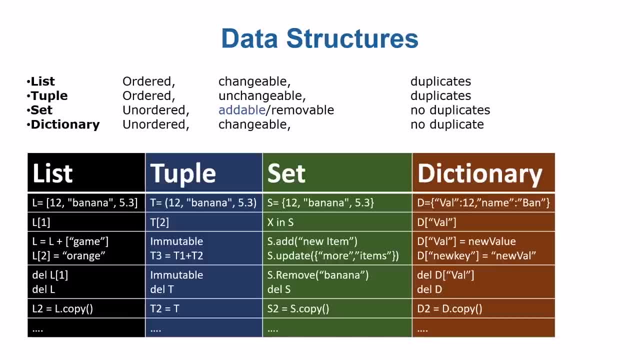 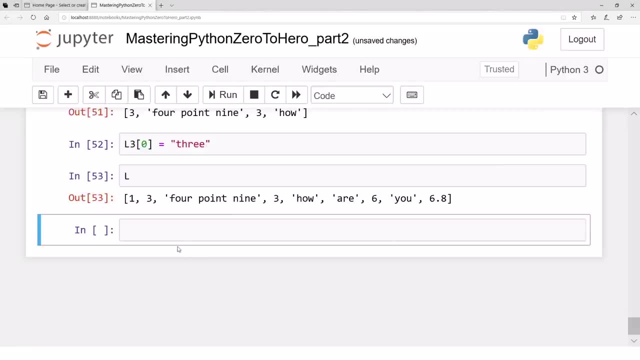 and all their functions on your own and to see what function or what method is doing what for what, which kind of data structure. so in the next video we will be seeing some methods just for this data structure. hope to see you in the next video, like in strings, let's- let's explore a lot of. 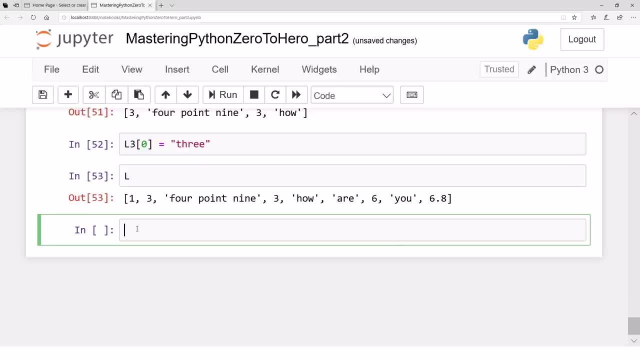 functions in list, although in, in, in sets and dictionaries and tuples, tuples as well. but many more functions are available in list and, by the way, let's see how how many things are there in this list. and let's say l dot tab and tab will open up a lot of things with me, for me, append, we know already. clear copy. 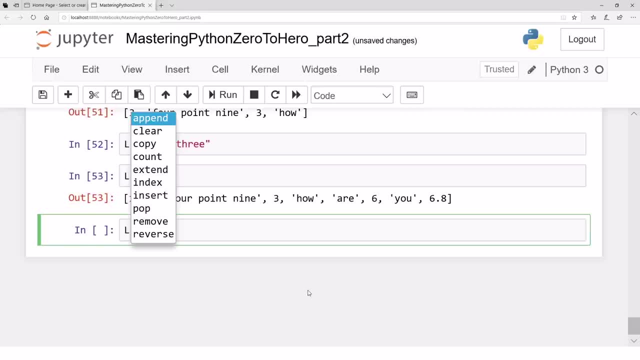 copy. we know already count. we don't know count. extend, index, insert, pop, remove, reverse- some of these functions. they make sense by the just their name. but let's see one by one. let's see some of those, what they do. one way to do that is go to internet and see. 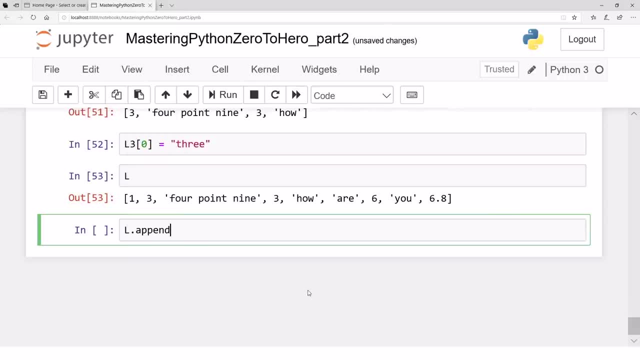 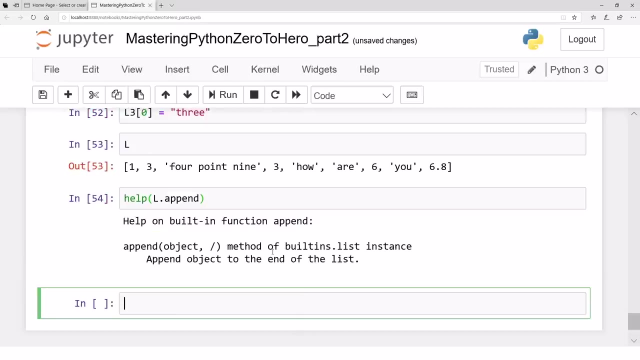 some book or tutorial or something like. so another way is just write this: apply maybe maybe help function. maybe apply a help function. it may help you how to use that great, this help function is great. so append an object. method of built-in list instance. append object to end of the list. oh, it appends an object. 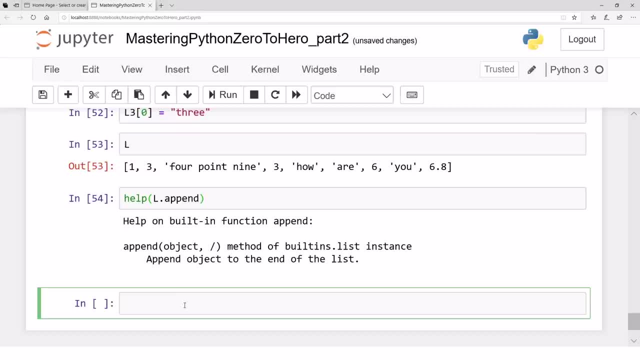 to the end of the list, which means we may be able to append another list to to do a list. maybe have you thought about that. the append method just takes one, a one, one object. maybe it takes a whole lot of list, but then it may be possible. 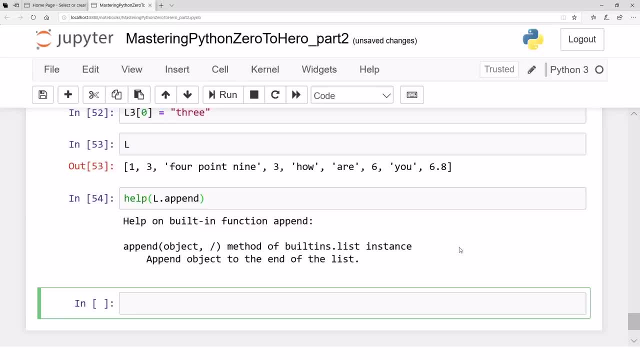 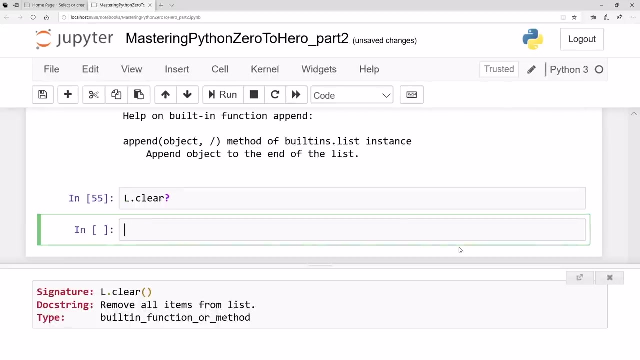 that a list is appended inside another list and that whole list becomes, becomes one element, because let's can contain other lists as as elements. now that's a problem. yeah, so let's see more functions. yeah, so let's see clear what this clear. what is this clear? what it does. sometimes i use help, sometimes i use that: remove all items from the. 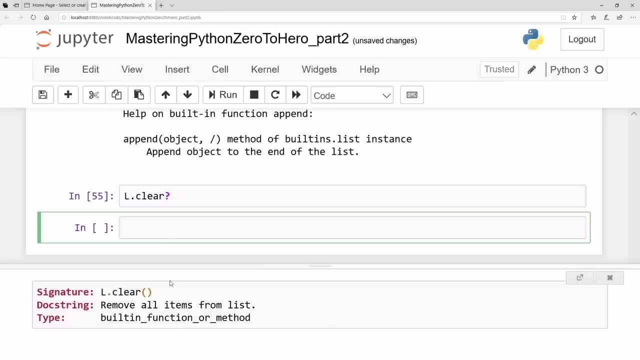 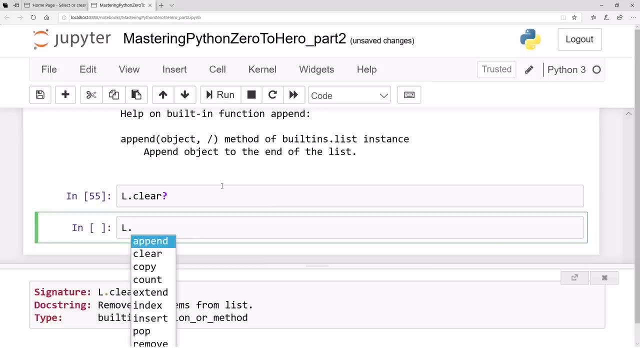 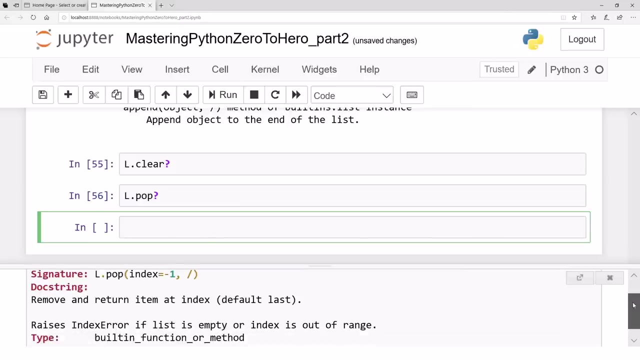 list. oh my god, if you call the clear that the list is empty. okay, uh, if you, if you, if you just call clear function on a list, list will become empty. be careful. okay, great, what else? so let's see, i have this function, maybe pop what it does, pop does what. so let's see, uh, so pop. 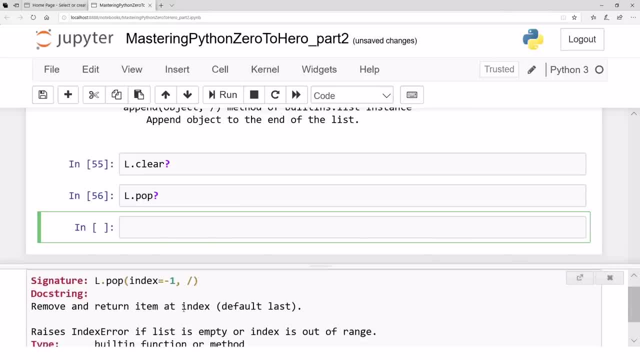 um. removes and returns. item. add index: default is the last, which means if you also that's a default value, remember the default value. so if you call a pop function without an index, it will return, it will remove the index, it will delete the last item and it will give you that it will. 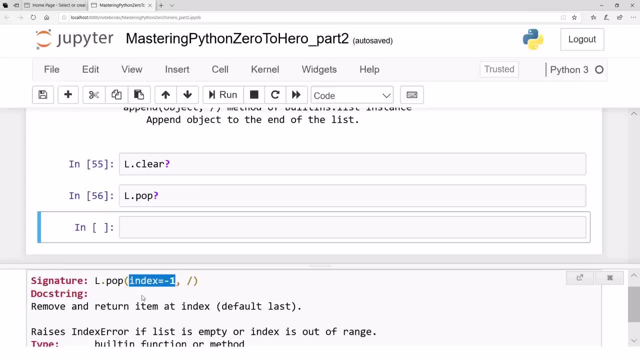 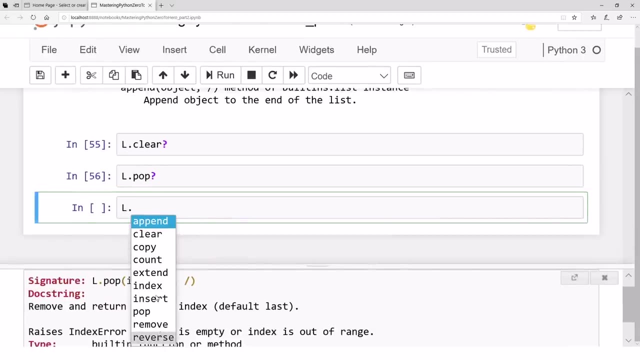 return that. or if you give an index, it will remove that value at that index and it will, after removing it will, return you that, so you can use it wherever you want. so, um, there are many more functions. for example, you can see all of them one by one. remove function, for example, reverse, reverse, like. 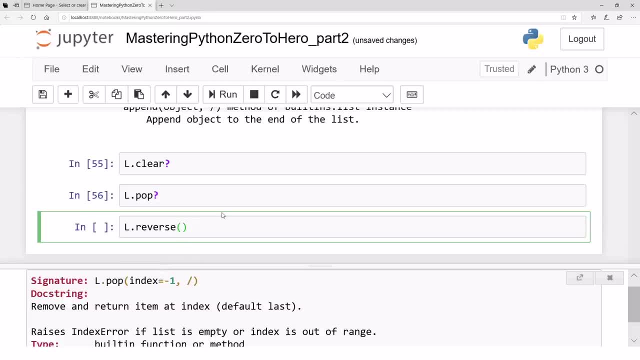 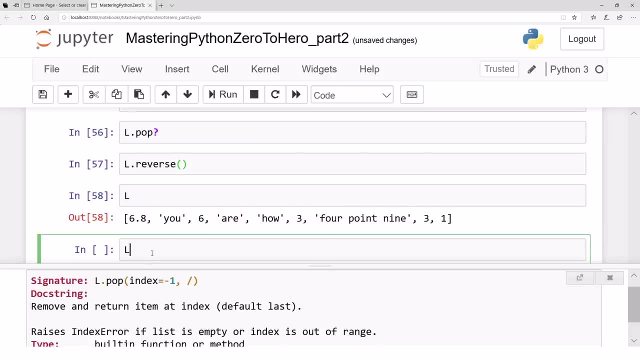 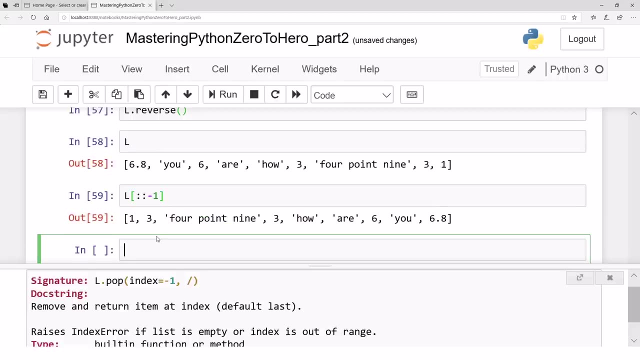 like, like the name suggests, if you call the reverse function, the list will be reversed. yeah, and remember, we have reversed the list in the following way as well: we have a way of reversing any way this way. so now, if you see, the list is again reversed, so i guess both of them are working like so same. similarly, you can explore several functions from: 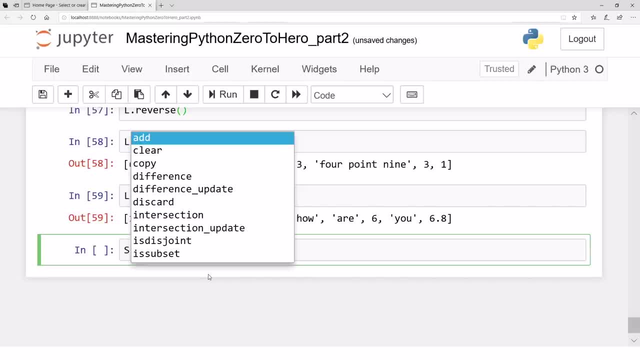 a set. you go and say add clear. clear might be working as same as intersection. intersection and update is disjoint, is a subset of the other. um, yeah, add by default or update by default. actually take a union. so i'm not seeing update function here. where is update? oh, union, is there. 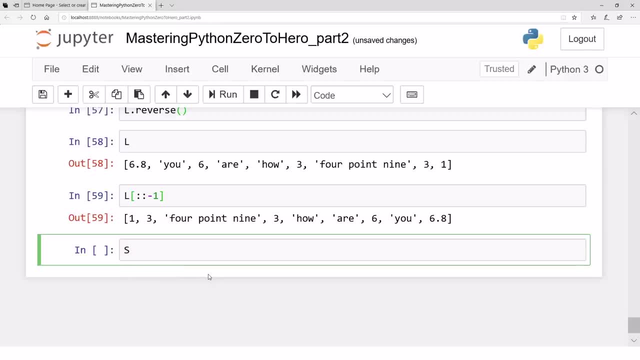 update is there, which means: uh, the list you are seeing is here is not a complete list. you may be writing what are the functions that start from you. so here are they, and and several others. similarly, you can go to dictionary and call for several functions. clear copy from keys, get items. uh oh, 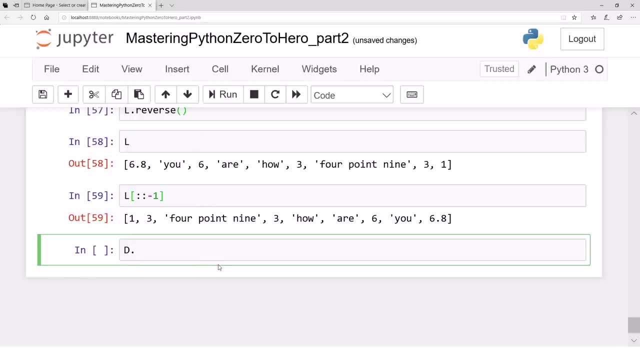 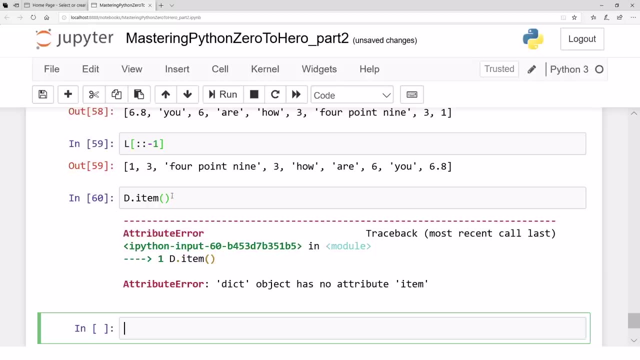 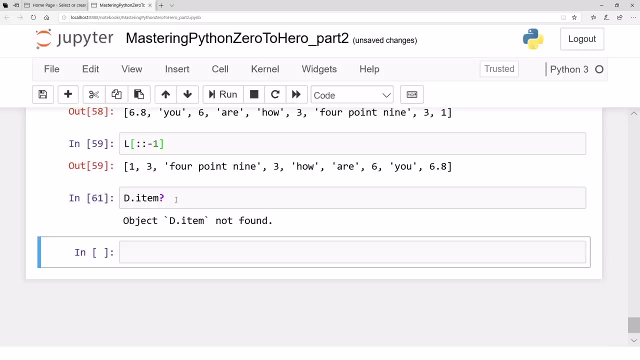 that item might be, might be interesting. oh, it has an error. what so? how can i use this? how can i use this function? let's see. oh, this is just an object, it is not a function. uh, i don't know. let's see again. or? or it is not listed anywhere. 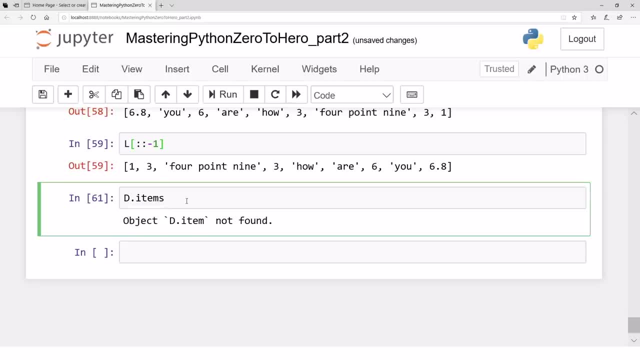 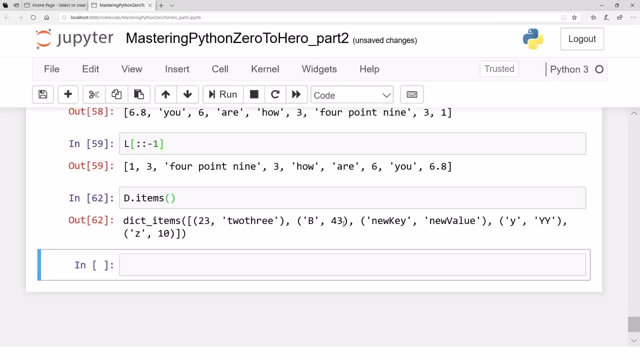 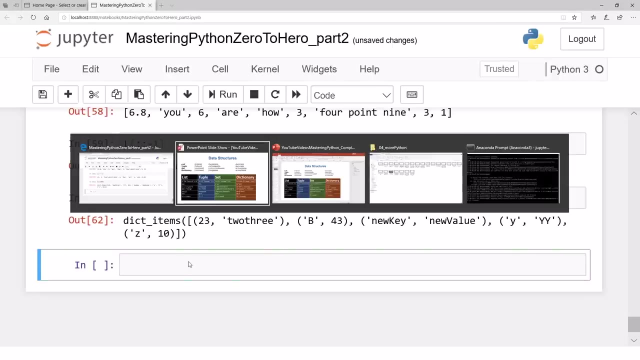 oh, it is items, not item. okay, items, that's a function, maybe. so these are all the items 23, with this b, with that new key, with that and so on, Great. so actually the purpose here is not to tell you each and every function and what it does. It will. 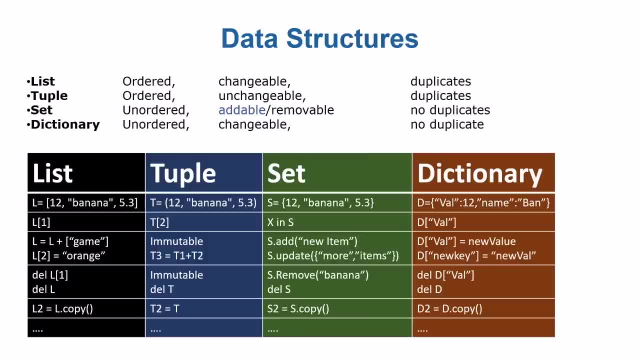 take a whole lot of time. You can go and explore all these functions. The purpose here is to tell you what kind of data structure has what kind of properties and what are the similarities and differences in between. So if you remember this, one slide for list, tuple set and dictionary and some text. 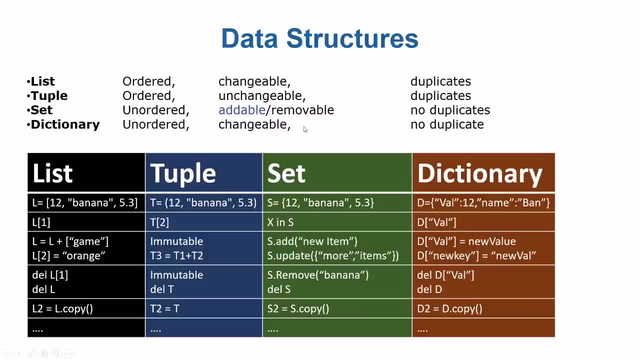 that is written out above, you'll be having very good knowledge of where to pick what kind of data structure in practice. So in the next video I'll be actually going to Jupyter Notebook as our style, and I will be coding or solving some problem for you. 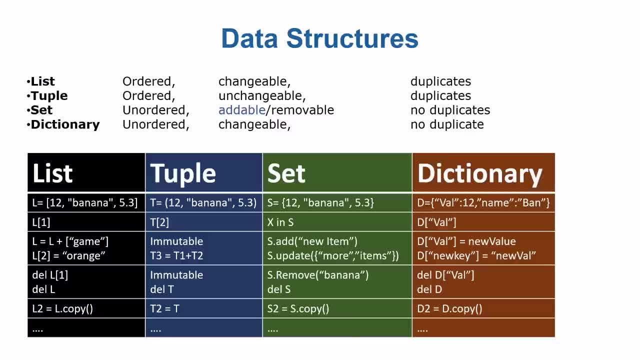 that will involve list, tuple set or dictionary, or one of them, or we will be choosing based on problem: what kind of data structure is well and what? So we'll be doing that, but before that I just want to mention that. 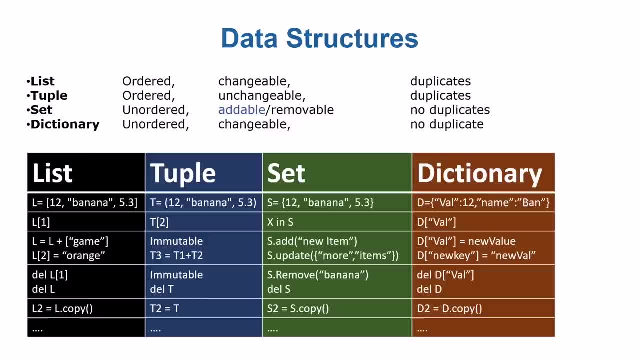 list, tuple, set or dictionary. they can contain any items inside any kind of type, which means a list can contain another list. A list can contain a set. a list can contain and dictionary. A dictionary can contain a list which itself contains a dictionary. I mean, this is all abstract. This is all abstract One. 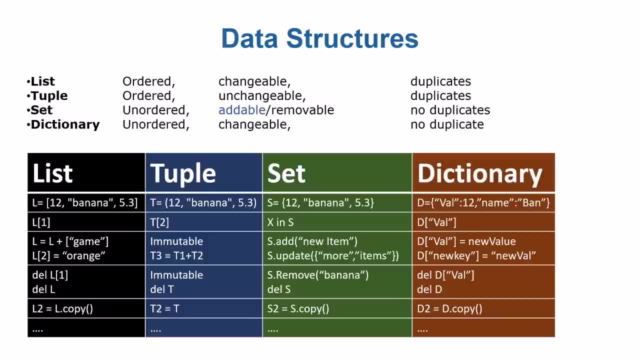 thing can contain the other. One thing can contain an instance of. I mean, a list can contain multiple lists and those lists can contain more lists, and so on. So before actually going to problem solving, let me give you a flavour of that. how abstract those lists are. 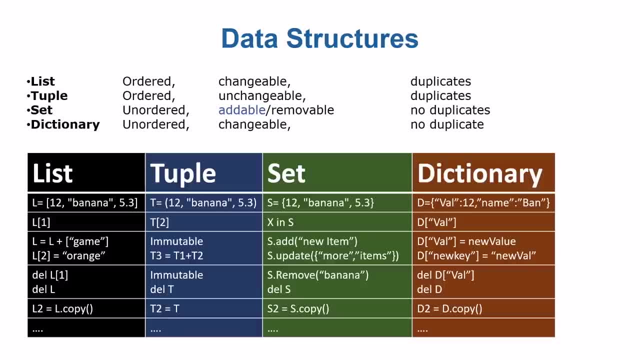 these things are. Let me give you a flavor of that in just in a couple of examples. So in the next video I'll be giving you a couple of examples based on the abstractness of these data structures, And from the next video we will be doing some problem solving based on that. 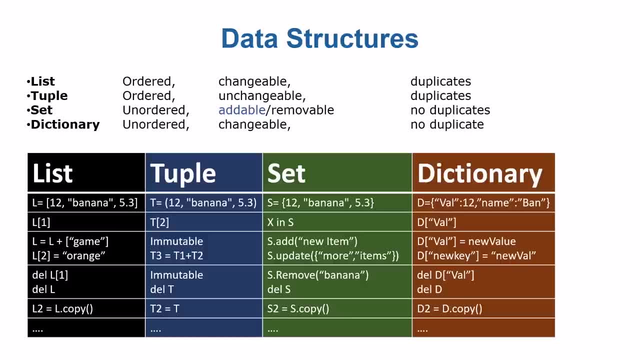 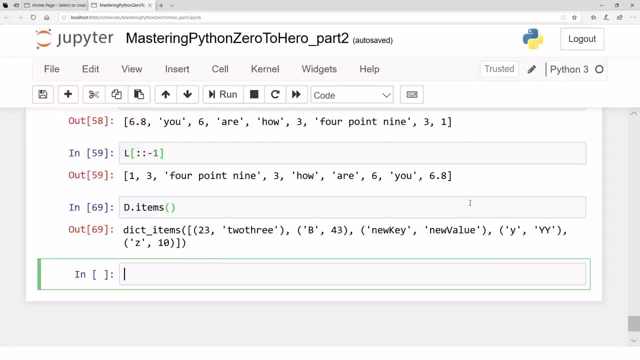 So next two videos are completely on Jupyter Notebooks. So get ready, Hope to see you in the next video. Okay, let's see the abstractness of all these data structures. Let's see just one example. Let's say we have L, that's the list. We have all the rich tuple, that's tuple. Let's say: 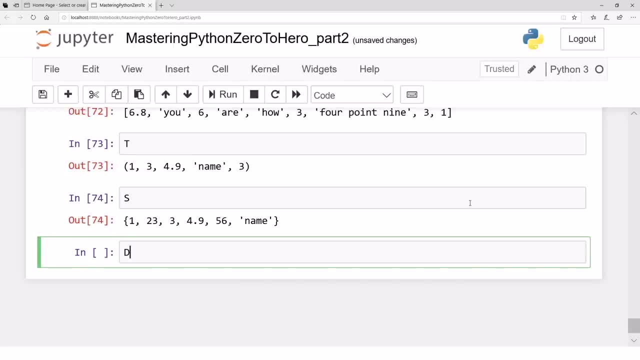 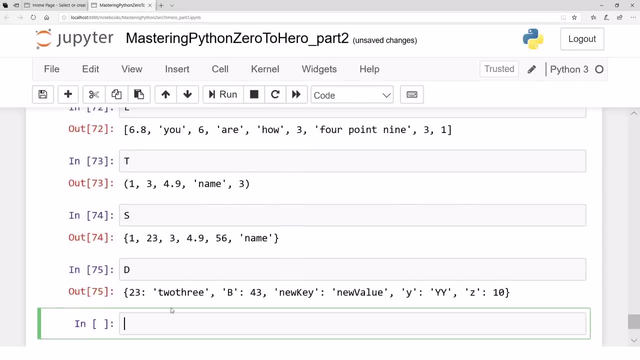 we have set, that's set. Let's say: and we have dictionary, that's the dictionary. Okay. so let's say: we have all these things, let's say available somewhere, So let's make another dictionary. For example, let's say: 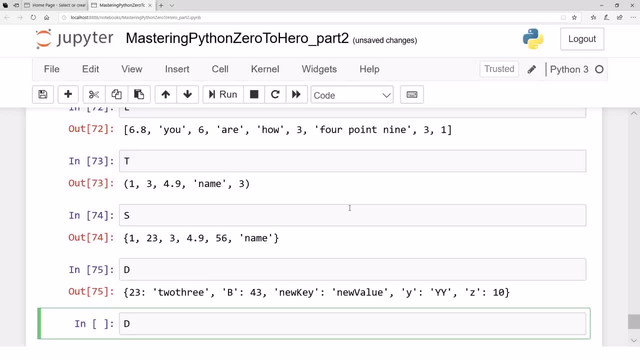 D2 and that dictionary has key value pairs less. the key is A and the value is the whole list L, that's the value, is possible. let's say the key is B and the value is just a tuple, the whole tuple, that's a value. let's say the key. 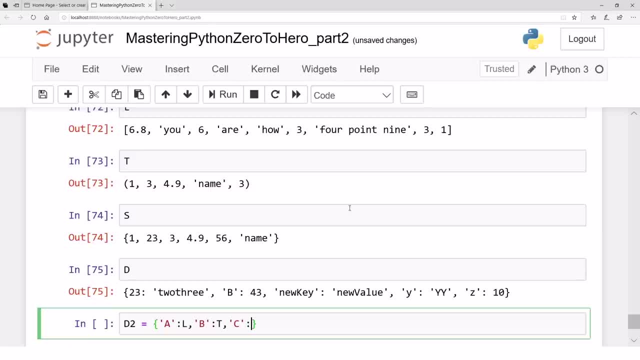 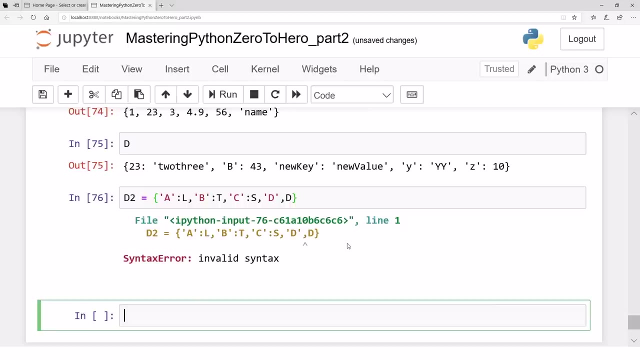 is C and the value is the set. and let's say the key is D and the value is the dictionary, the whole dictionary D. it is possible, I mean, you can just do that, that that is just one example. oh what's? oh sorry, I should have, I should have. 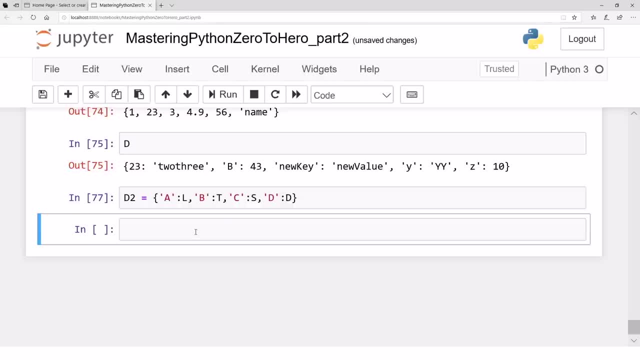 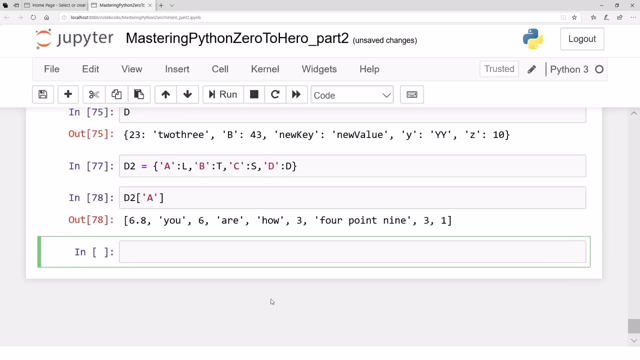 incorporated this way. okay, so this is possible now. for example, if I access you, if I access the element with, let's say, a, I will, I will get the whole list. and not only that, I can, I can access the whole element. and then after that, for that element, I can access, for example, the third element, the element at index. 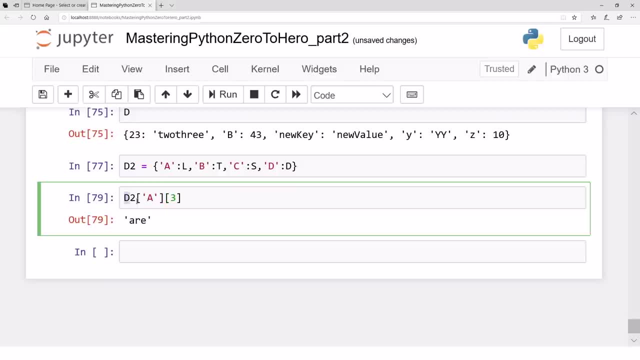 3. so this particular, this particular first first level will extract the list and that will in. that is just the indexing. or for that list, see, for example, if I access d2 and inside d2, if I access the dictionary that is inside and let's say I save that dictionary in K, then if I 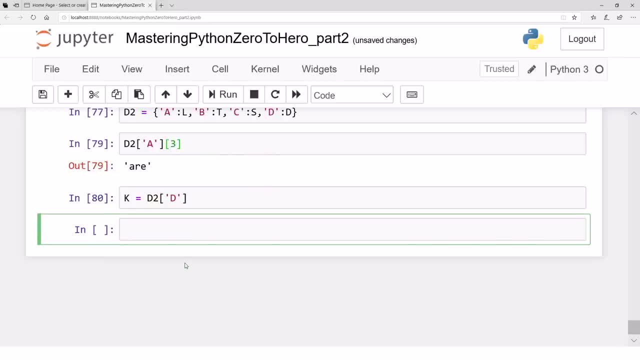 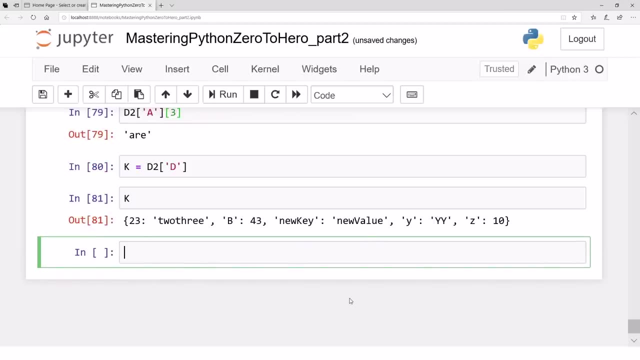 can see the contents of K, but I can just, for example, this: or I can just access all the elements of this dictionary or K by just having for X in K print for example, X and K of X, just do that I can. I can just do that. we have done that in. 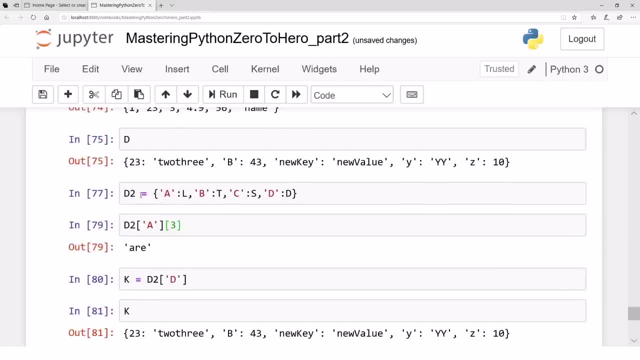 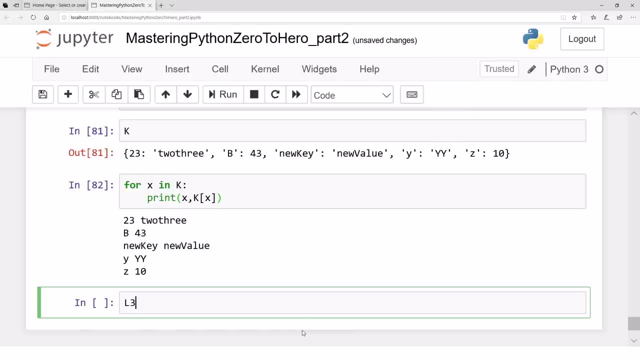 loops as well. so I want to tell you that these, even if, for example, if you want to create a list L, let's say L3, let's say you want to create a list that can contain the whole list, that can contain what will get- oh, I mean one element is the list, another. 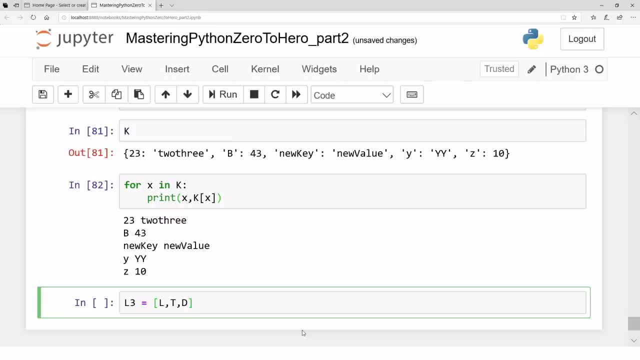 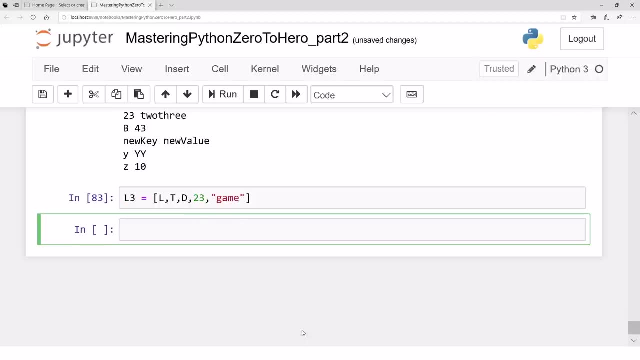 element is a tuple, another element is the whole dictionary inside, and then you have some other elements, let's say these game, and that's perfectly fine, I get. I mean, you can do that. these data structures are much more abstract. I mean now, if you, for example, excess element at index 2. 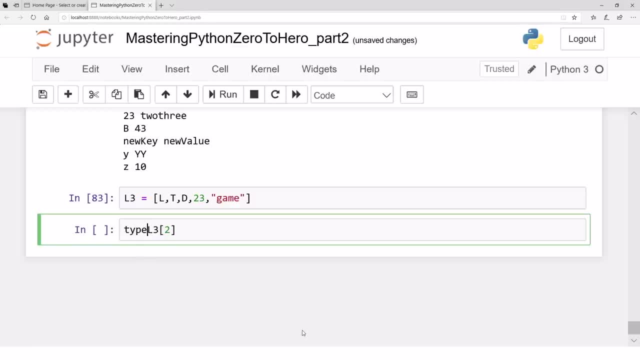 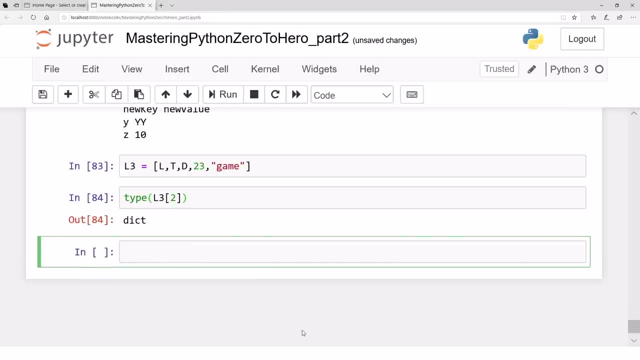 which is dictionary, that is completely a dictionary if you, if you check the type of that element, that that will be a dictionary object and you can extract that element and play the way you want to play and whatever. one more thing we can, for example, lists. we can, let's say, we want to make a list, list very quickly. 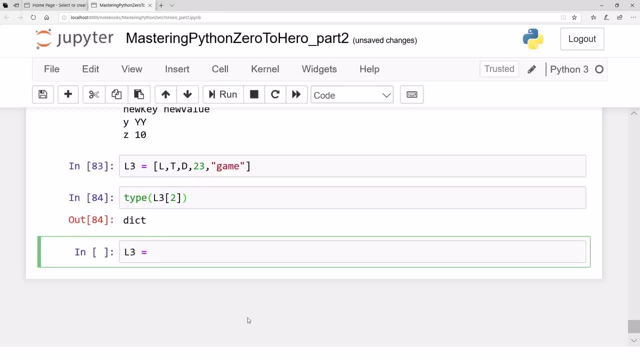 for example, list of all the squares till till, starting from 0. list of all the squares till till 10. for example, 0 square, 1 square, 2 square. let's say we want a list of that. so one way of doing that is a quick shortcut- is to just use 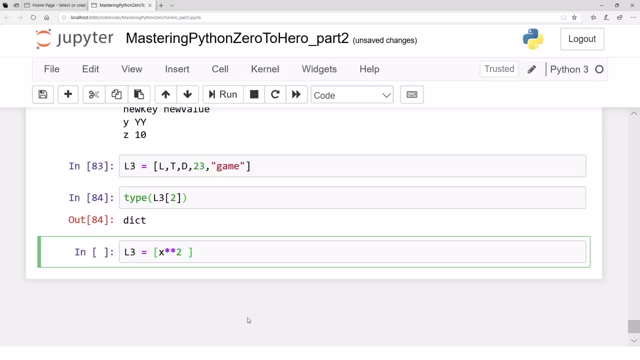 loops. so in loops, for example, we write: okay, X square for X in range 10, for example. so it will start from 0, go till 9, including 9, and you will get X 1 by 1, and all this syntax is for making a list of X squares where X starts from 0 and 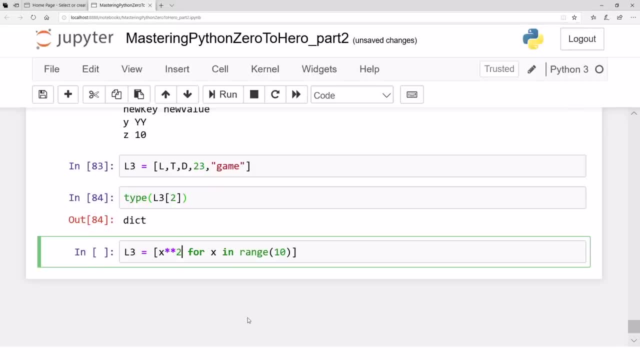 go till and go till, including 9, go to 9, 1 by 1, and that's how you can make a list. and I mean these kind of these are kind of shortcuts. again, you can make a set, for example, let's say you want to. 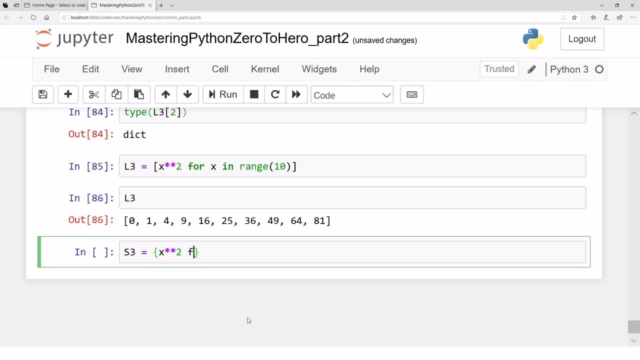 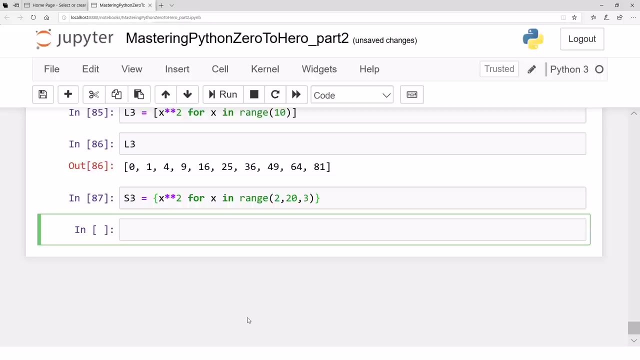 make a set of all the squares for X in range, let's say, starting from, starting from 2, ending at 20, and you want to take a step of, let's say, 3, so start from index to go till 20 and do not include 20, but take the step of 3 and you can. 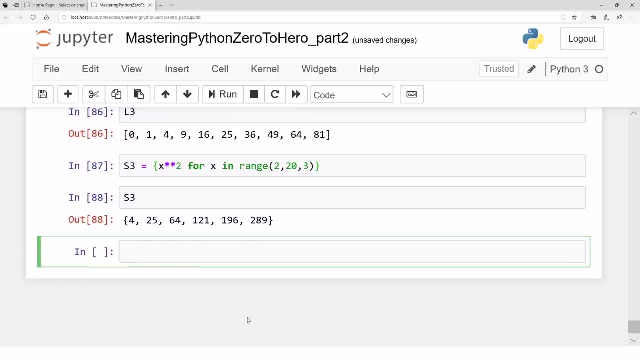 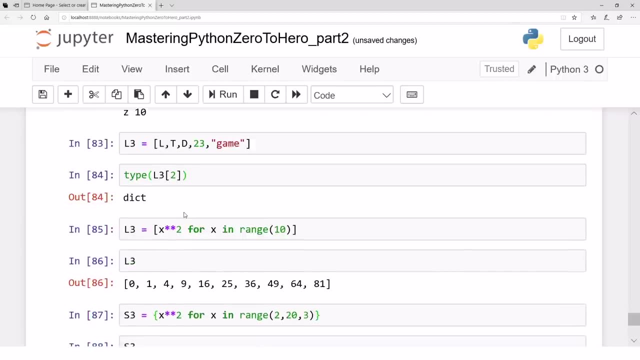 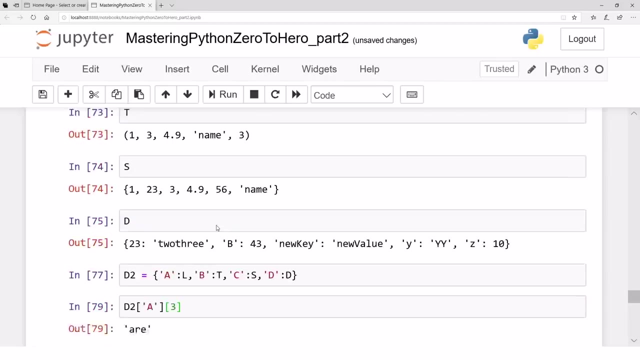 now have a set, which is, which is this? I mean, there are, there are a lot of ways of working these, working with these one. one can explore more and more about these things. but but what? what? the basic thing about these data structures are? they are very, very abstract. they can, I mean a 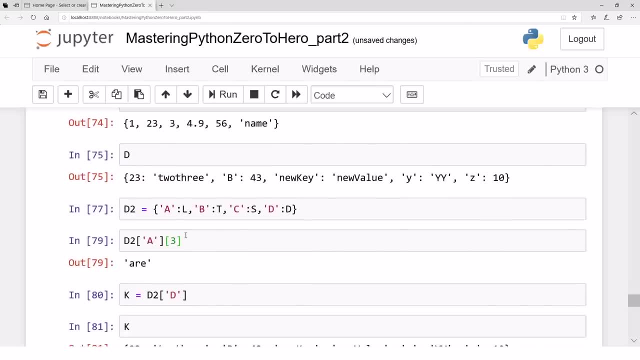 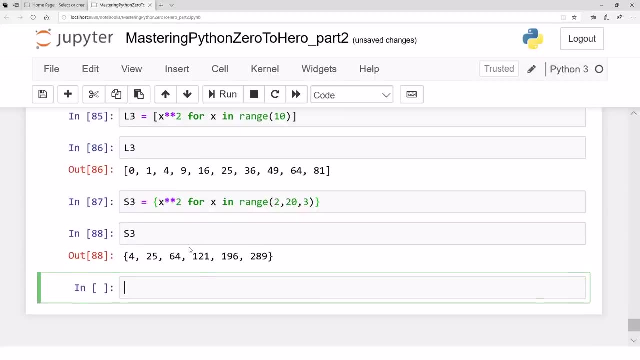 list can contain a dictionary, and that dictionary can contain a tuple, and that tuple have an element which is another list, and so on. it is. it is that abstract. it allows you to do each and everything in that way. okay, so I end this video here. in the next video, we will actually solve a problem using these, one of these. 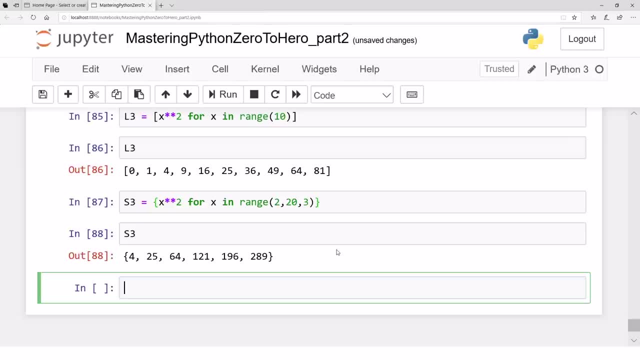 data structures or we will try to choose one of those, and that video may be lengthy, may be small, because we may have bugs inside and we will. we will play around with these data structures in the next video. so do attend the next video, because it's really the practice and you will get your hands. you will get a very 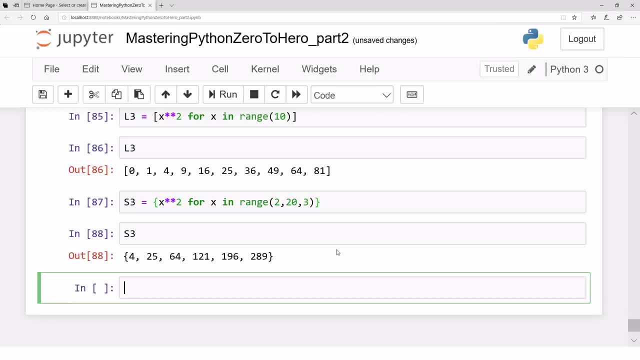 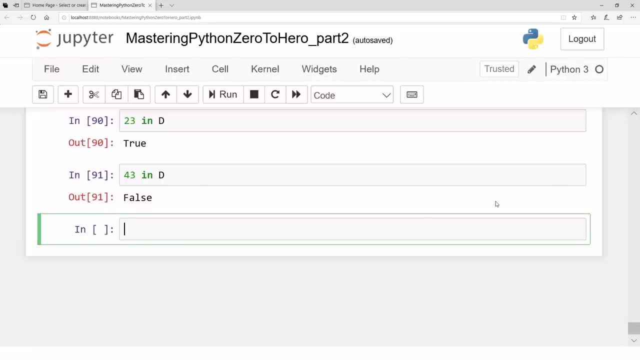 good grip on the data structures in in the solving the next problem that we are, that we are launching for you. okay, hope to see you in the next video. okay, let's see a problem, just to get comfortable with these data structures. so, let's, let's design some problem and 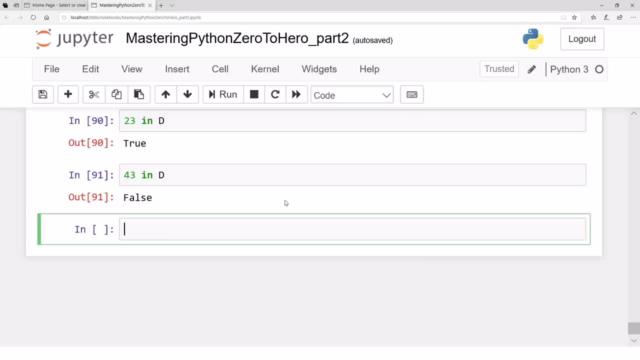 solve that problem here using using these data structures. so the problem that I'm thinking is, let's say the following: let's say: let's say you are a teacher, should I type all these things? okay, yeah, let's say you are a teacher, you are a teacher and you have different student. 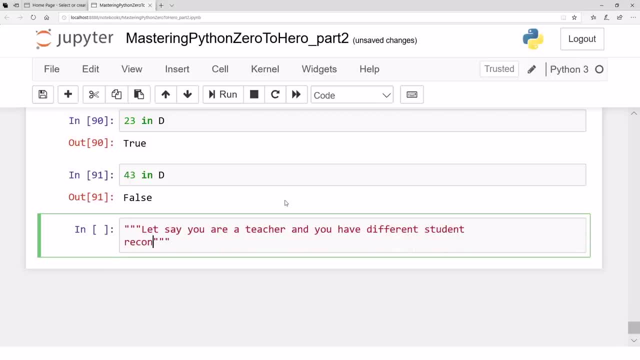 records, student records containing containing ID of a student and the mark marks list in each subject where different students have taken different number of subjects too. and all these records, all these records are in hardcopy. you won't, or coffee, you want to enter all the data in computer. 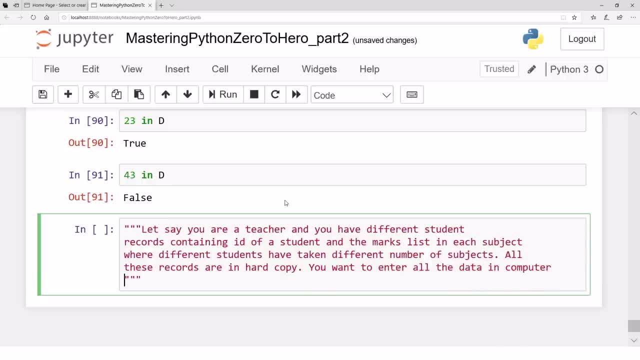 and, and, and, and, and and one to compute the average marks of each student and display. that's the problem. so the problem, let's say, is: you have, for example, you have a hard copy, you have a, you have some papers upon which you have different students. each student have a. 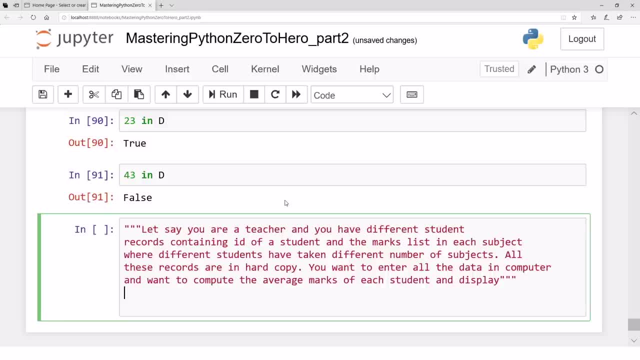 different ID. some students may have taken seven subjects, some student may have taken three subjects, some student may have taken eight subjects, and so on. different students may have taken different subjects, and records is there. you want to first enter for each student. you want to first enter the. 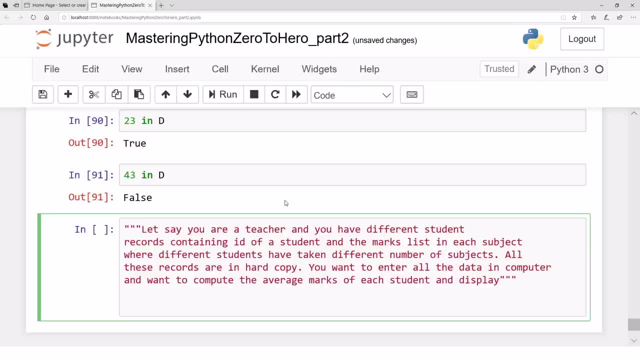 records, I mean all the data that is in, and then you want to compute from that data. you want to compute the average marks of each student. for example, if a student have taken five subjects, then the marks for all the five subjects are available. you just add all the marks and divide by five and that's, let's say, the average marks. so 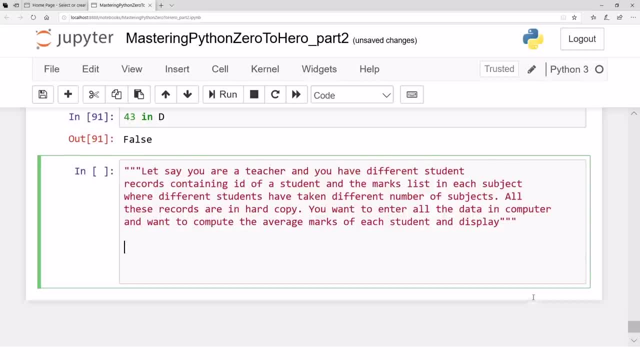 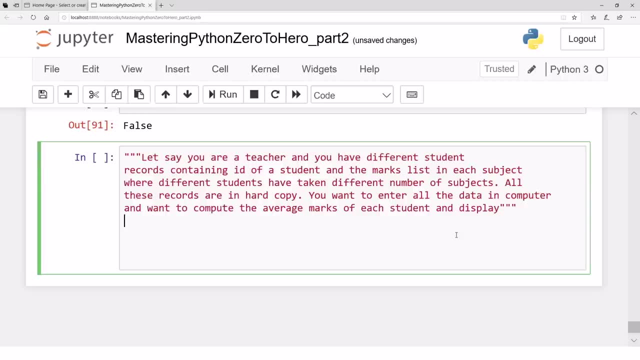 first of all, let's write a way to way to compute, for example, the to just collect the data, how to collect the data. so let's write a function for that. so let's say: define a function. let's say, get data from user or teacher. let's say: and let's say: that's a function and it. 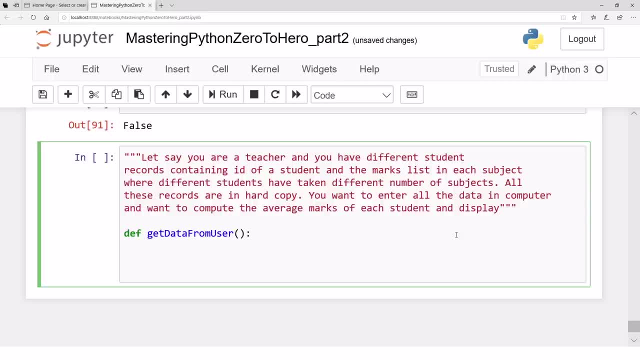 returns data. okay. so what I do really is: I say okay, while true, I made a loop, while true, just take the data from the, from the user, and the data is in the form of. you first say okay, ID, student ID. let's say that is inter or actually input inter student ID. so he: 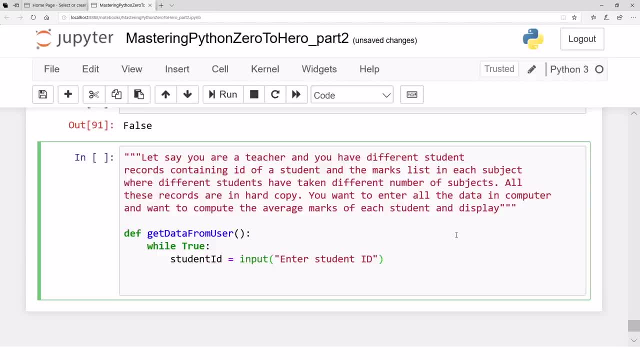 enters the, the person enters the student ID. yeah, so drop. you might have defined a dictionary, maybe a dictionary D that is empty right now, but you may. you may add and remove different values. so what you do is you add a student ID, you get a student ID, and in the string form, and then you get the. you get, for example: 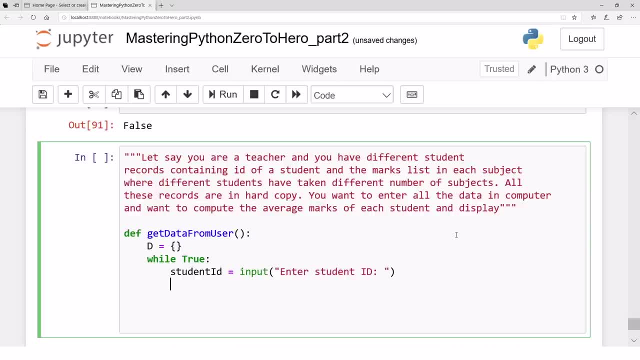 the input as the marks list, so marks list as input. enter the marks by comma separated values. so in through the marks, using, for example, if you have five subjects, just Just write the five subject marks by separating each with the comma. Okay, then let's say more students is equal to, let's say input. enter yes or no for. 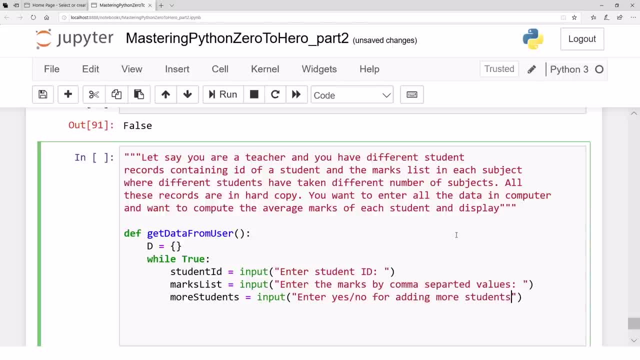 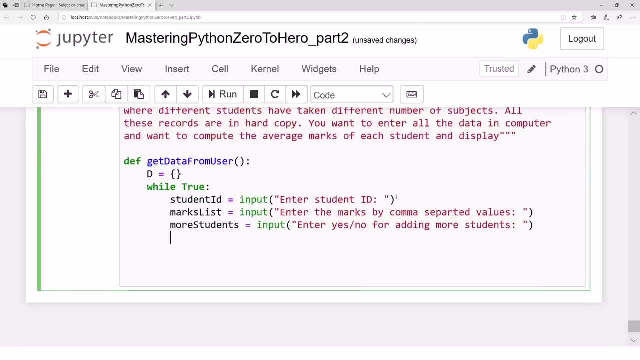 more students. So if, for example, you have more data to insert, then press yes, otherwise press no. So that's, for example, our setup. So we will keep on getting more and more. we will keep on getting more and more data. 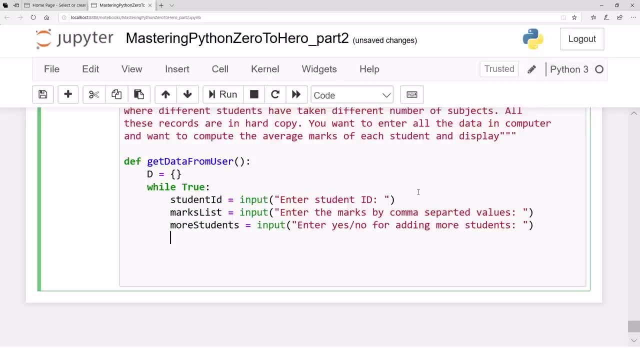 from the user. User will keep on entering the data. But one thing that we must know is that if, for example, a student ID, student ID is already in D, if that is already in D, then we should give a message print, print that. 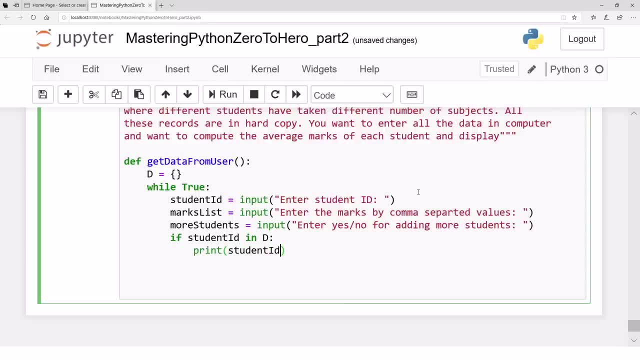 student ID is already inserted, So that might be a message Else else. we want to do something Else what we want to do. What we want to do is the following: What we want to do else is we will make a dictionary. 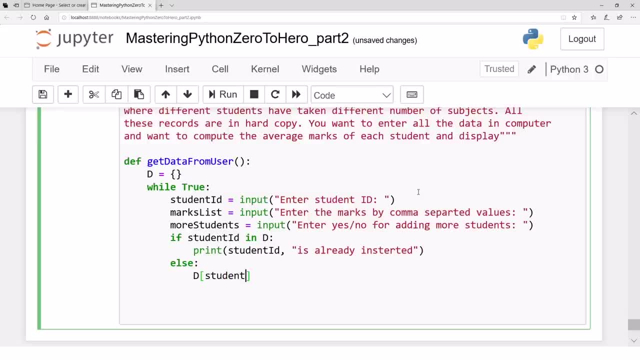 We already have a dictionary with the student ID as our key. That's our key And at that key, what we do is we pick the marks list and just split it using comma because we are expecting And all the marks, they will be saved as a list. 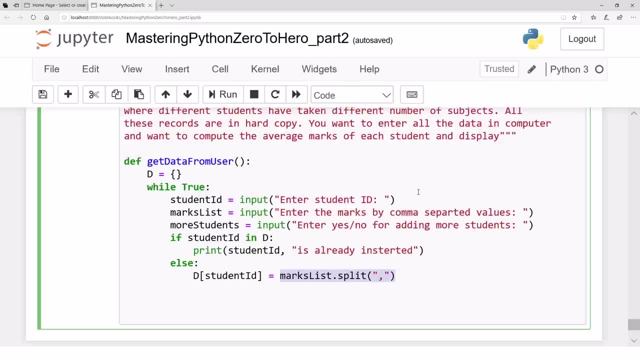 So that will return a list, a list of string values. These are not integer values, These are string values. But all these lists, they are tagged by this ID So that, as a dictionary, that will be getting populated on and on and on. 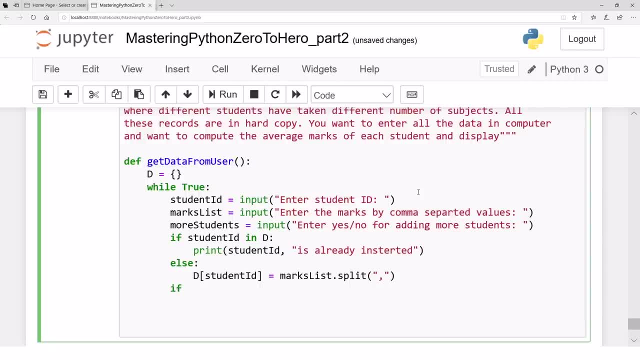 Further, if we check, if, for example, more students dot lower, for example, Let's call the lower function because the user may interest it in a lower form. or if that is equal to, let's say no If that is equal to no. 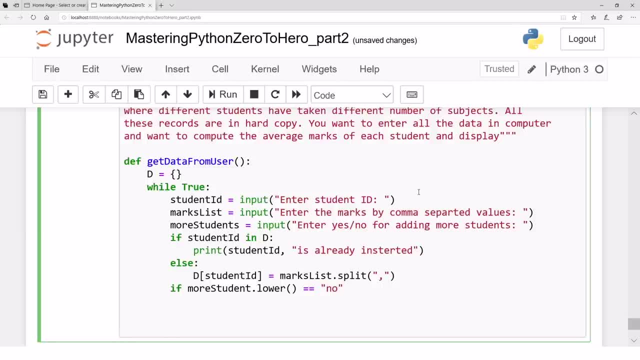 If this is the case, or if that is no Enter, for example: no Enter, no Enter, Enter, Enter, Enter, no Enter, no To quit Quit insertion. Insertion: Enter no to quit insertion. 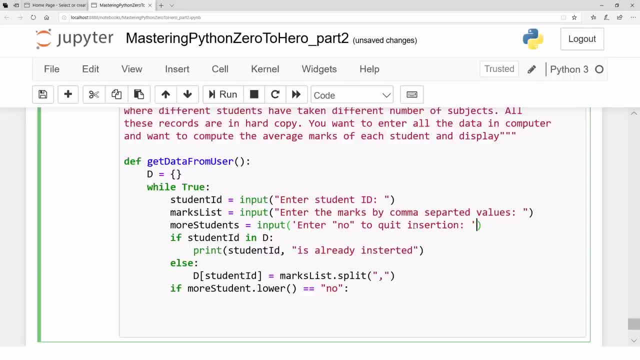 So let's say that's your message. So, wherever the user inserted, if that's a, no, then you return D and that's it. Otherwise you keep on moving. So that's the answer, That's the whole code. 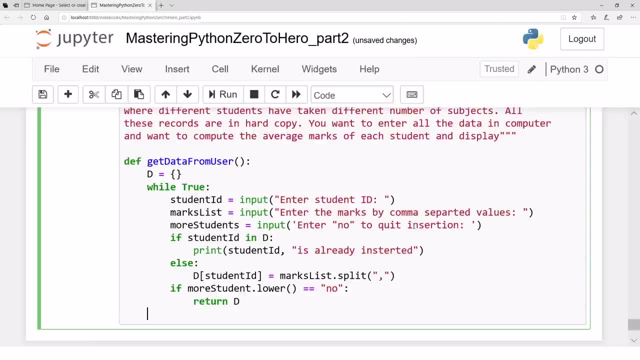 So you keep on asking more and more values. If, whenever the teacher enters a no, then you just return, Otherwise you make another iteration, you make another iteration and keep on moving. That's how you get the data. So the data will be available to you once you are done with that. 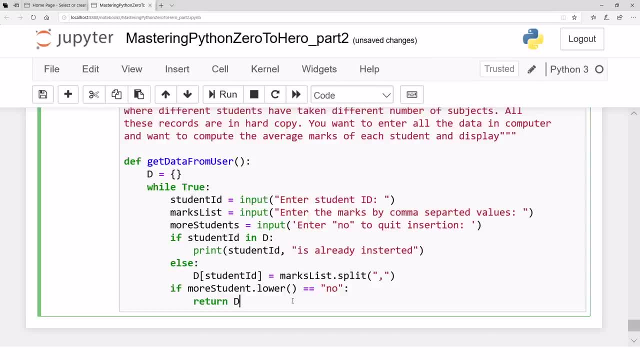 Then, after that, we will see how to. Once we have this data collected from the user, then we will see how to. Once we have this data collected from the user, then we will see how to. Once we have this data collected from the user, then we will see how to. 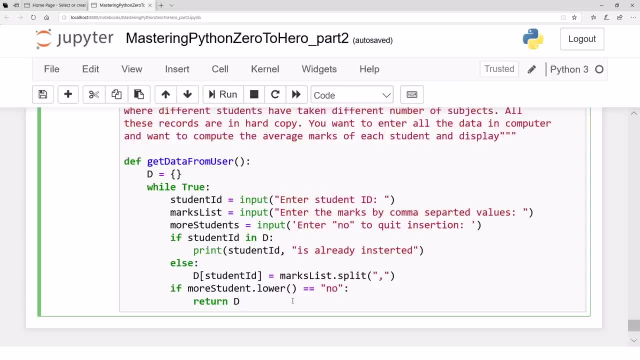 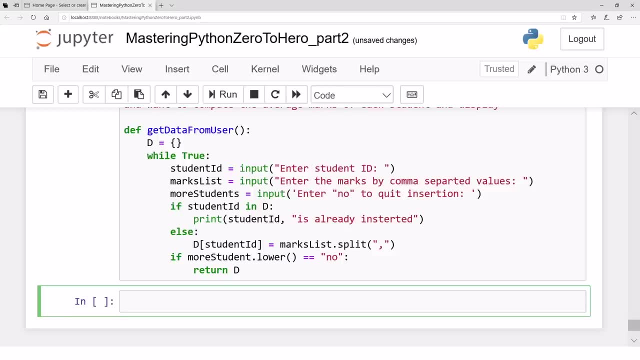 Compute marks for each student individually, average marks and so on. So let's just check whether this function works or not. So let's say we have our dictionary. Let's say student data is equal to get data from user. Let's just call that function. 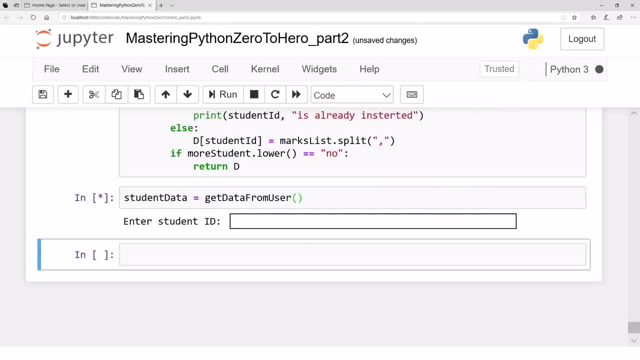 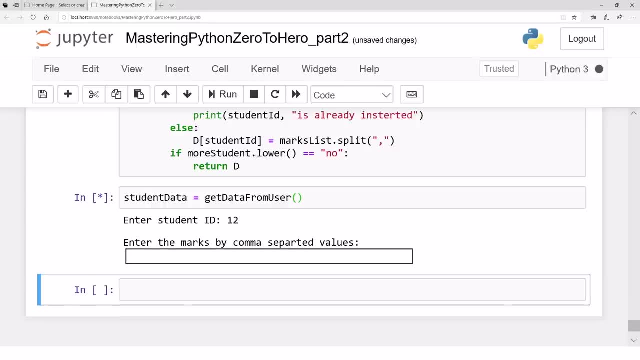 Let's see what happens. Okay, Interstudent ID. Let's say ID is 12.. Okay, Intermarks by comma separated values: Let's say 12.. Let's say 24,, 65,, 87.. Let's say the first student. just have these three subjects. 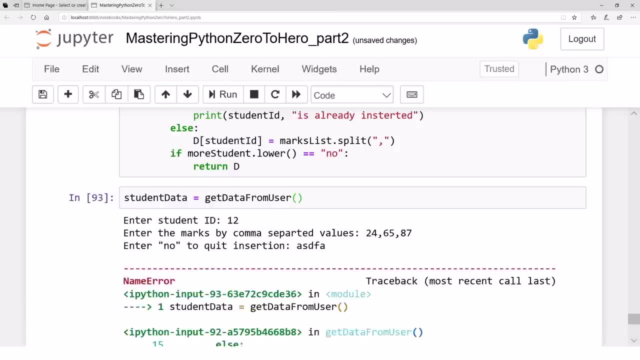 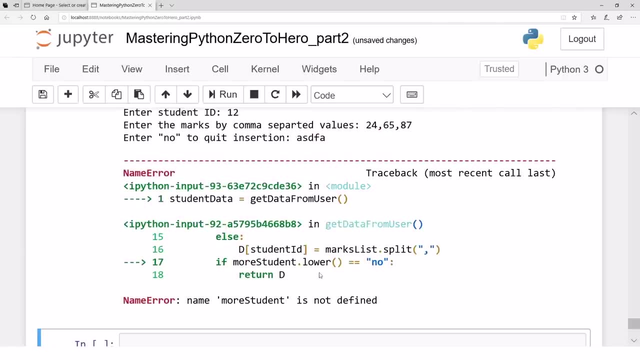 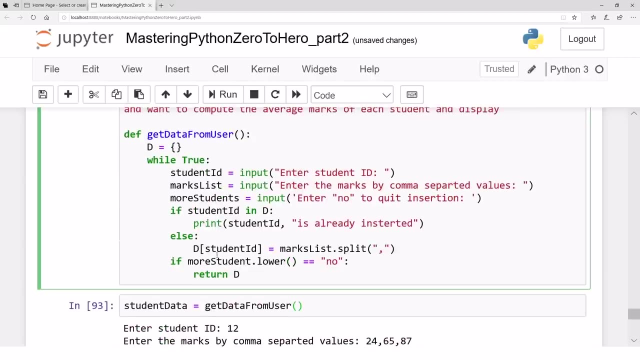 Then enter no to quit, So I will Something else. And Oh, what's the problem? There is a problem. If more students dot lower, is more students not defined more student that's, I guess. more students, more student here. 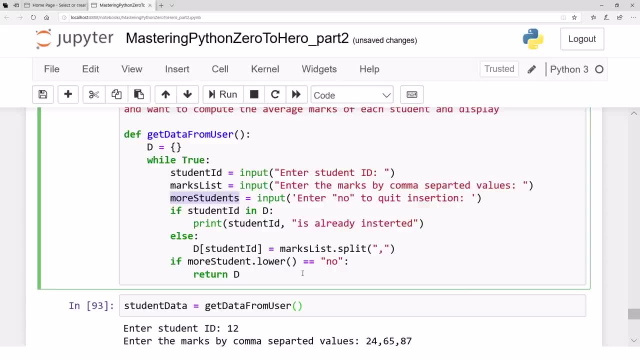 Oh, the spelling mistakes. That's a huge mistake. So I just copy there. These bugs are there. That's part of life, Part of programming life actually. So I guess now it will work. So let's do the process again. 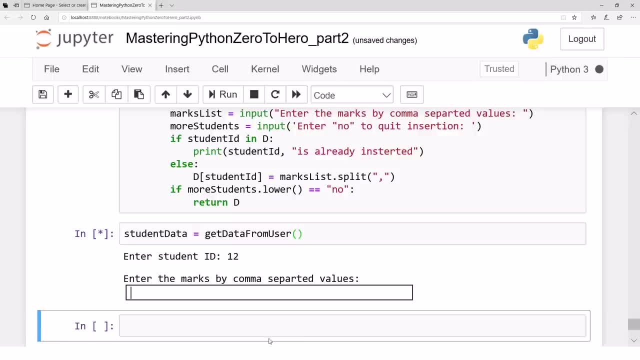 So 12,, let's say, And the marks are 56, comma, 45, comma, let's say a bad subject with, let's say, 13.. Enter no to quit No, I will enter something else. 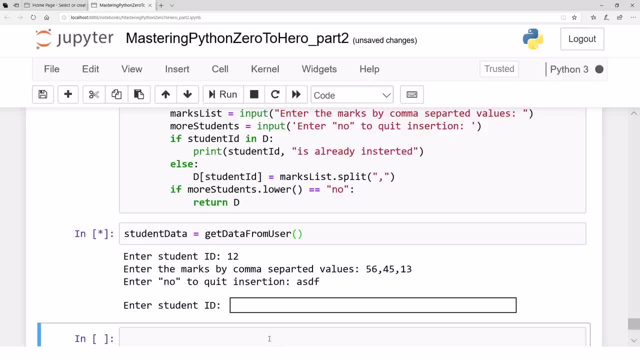 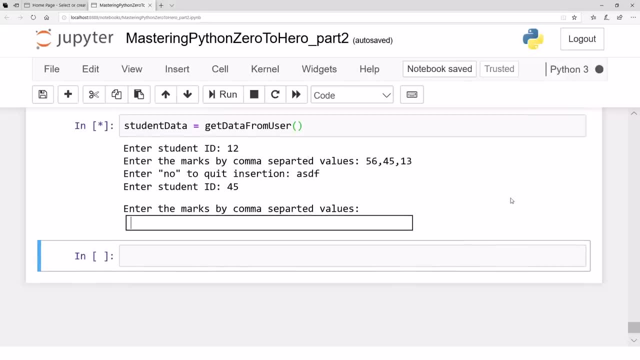 And I will keep on moving. The other student is: The student ID is 45,, let's say, And the marks that This student has gained. Actually, let's say, this student has already registered seven subjects, or let's say five subjects. 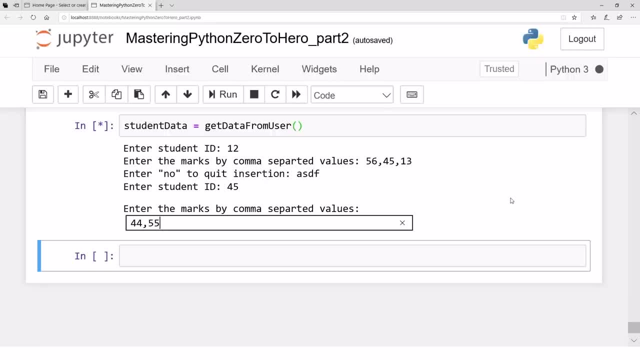 And the marks are, let's say 44,, 55,, 66,, 77, and let's say a bad subject, let's say four. Okay, Then enter no. to quit: No, I want to insert one more. 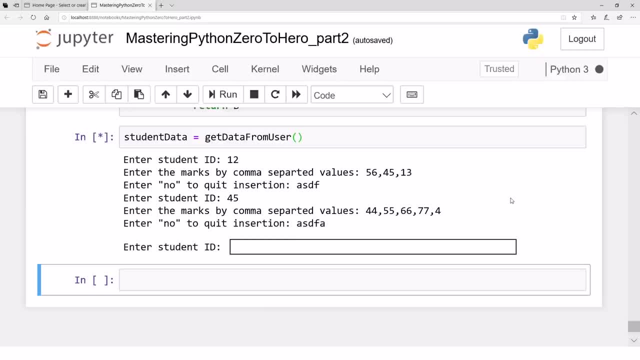 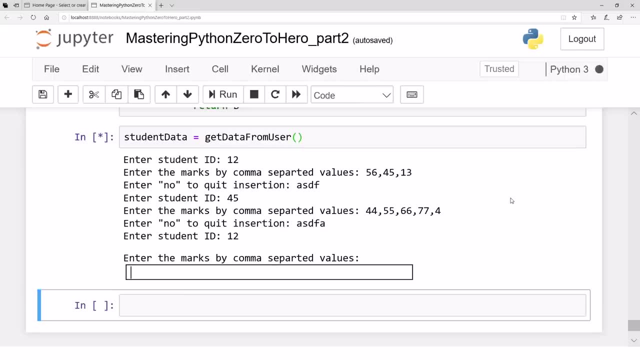 So do anything else other than no. So student ID. let's say Now the student ID is 12 again. let's say: Let's say I want to insert another ID again And whatever the marks. let's say 45 and 45 again. let's say: 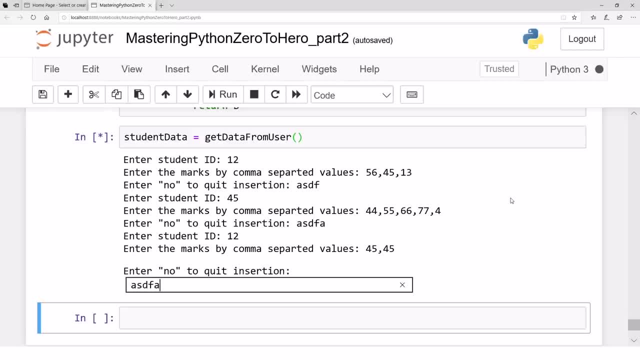 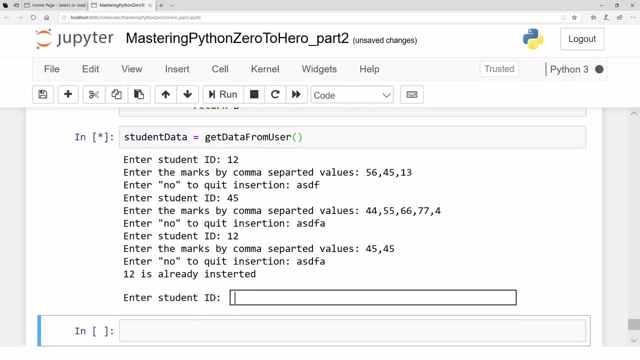 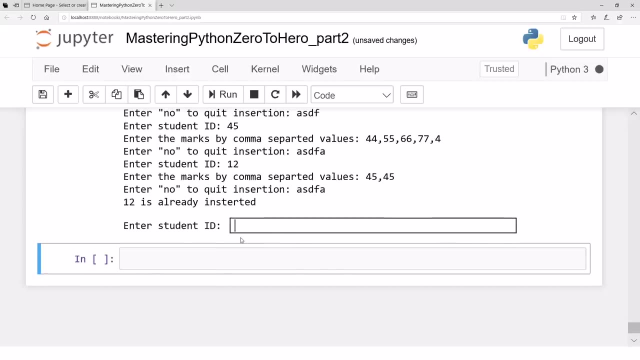 Now enter no to quit, No, something else. But now the message is there. The 12 is already inserted because the ID, The key, The key value in dictionary cannot repeat, and so is the student value. So it does not insert it, because this may be my mistake. 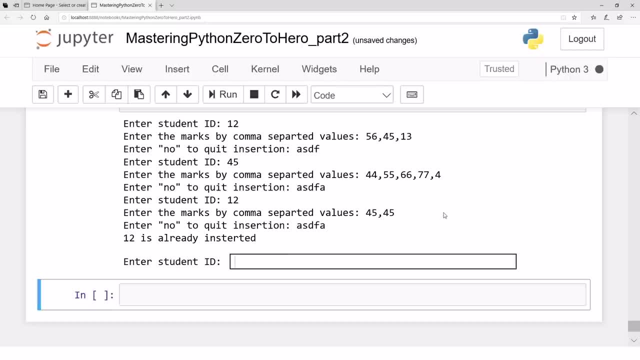 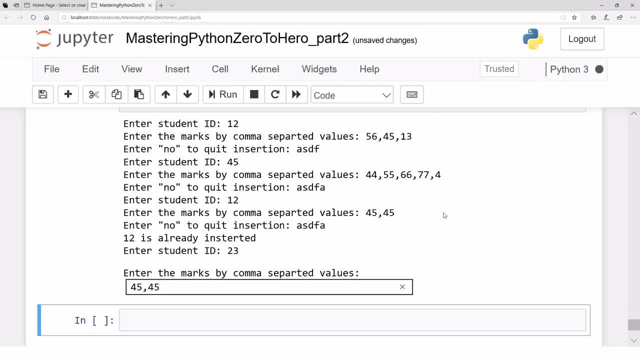 So it asks again. So now let's say I enter ID, let's say 23.. That's the ID, or maybe a different ID? That's the ID And the marks are: let's say 45,, 45,. let's say: 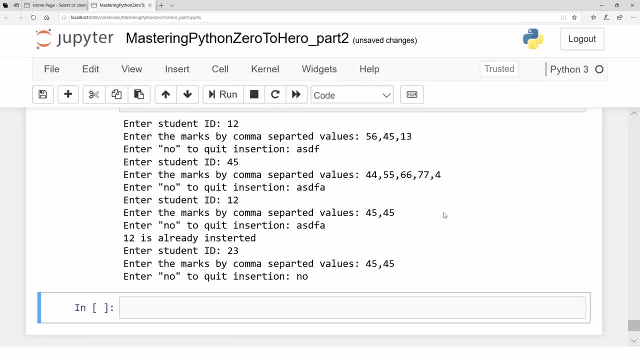 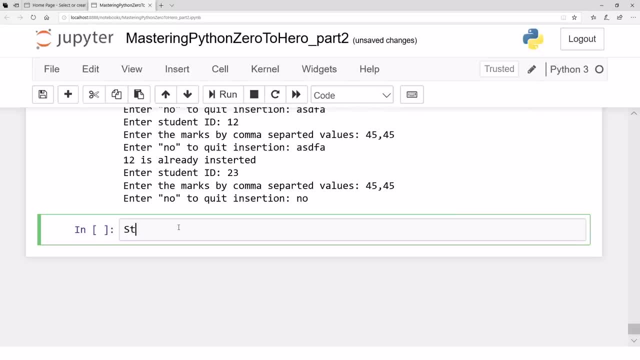 And enter no to quit. So let's say I enter no And that's it. So now I have received the student data, If I show you the student data, that student data is student data. That's a dictionary. 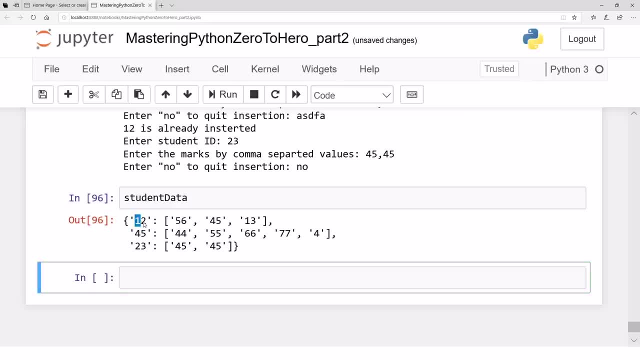 That's a dictionary with a key 12, and that's a list. But this list contains all the values that are string type. You will see how to handle that. That's a 45 as a key value, That's ID and that's the marks list. 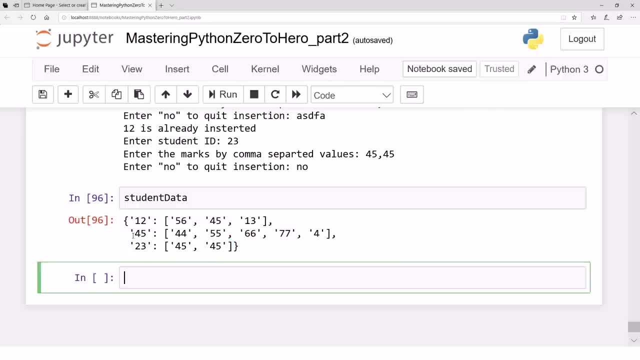 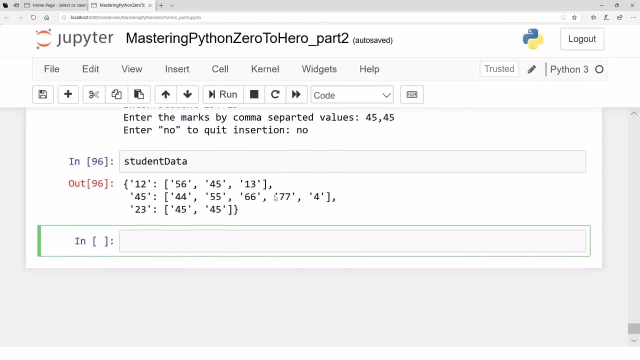 And that's the ID And that's the marks list. Okay, great, Now we have student data. Let's write another function that helps us working on the student data. Basically, we want to find out the average marks of each student and then we want to print those. 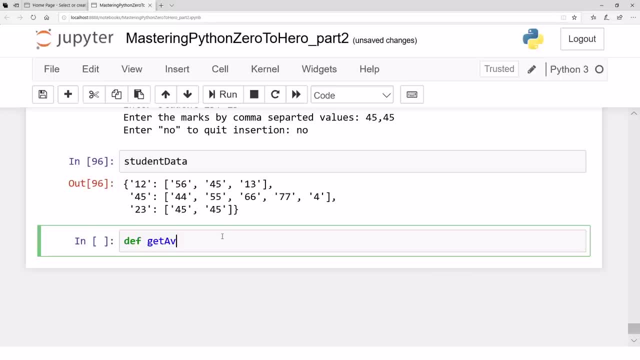 So let's define another function, get average marks of each student, And that function actually receives this dictionary. Let me call it as D Any anywhere, That's a local variable. Okay, So what we want to do with that is the following: 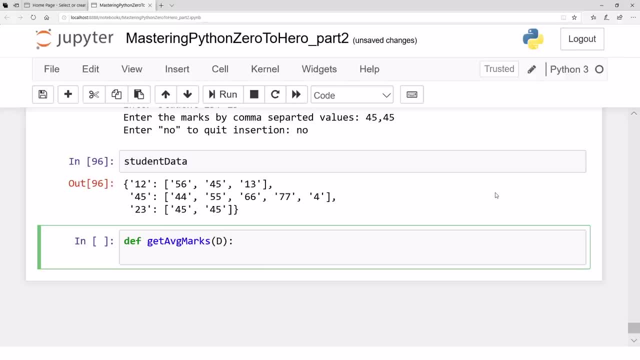 Average marks for each student. So we will define another dictionary. Let's say average marks dictionary. Let's say that is empty, in the beginning Maybe. And then what we do for X and D. Let's say I create over X and D. 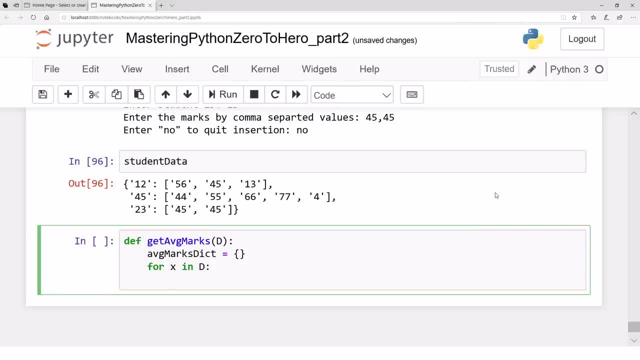 What we really do is We go to We find out the list of located at X. So L is basically D sub X. So let's say: that's our list, That's our list that is located there. So then what we do, for I in L. 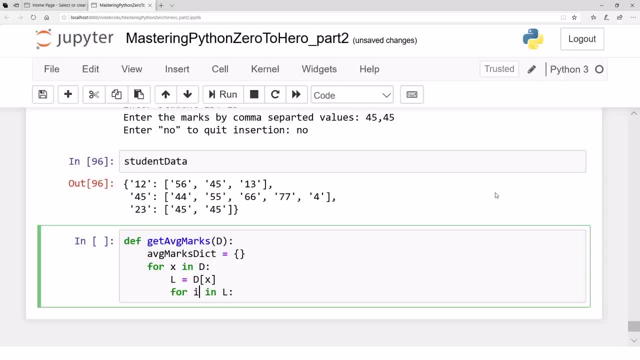 So for all I that is in L, Or let me call it for marks, Marks in L In this particular list, What you do is You actually have this sum, Oh, sum is equal to zero. Right now, there is no marks. 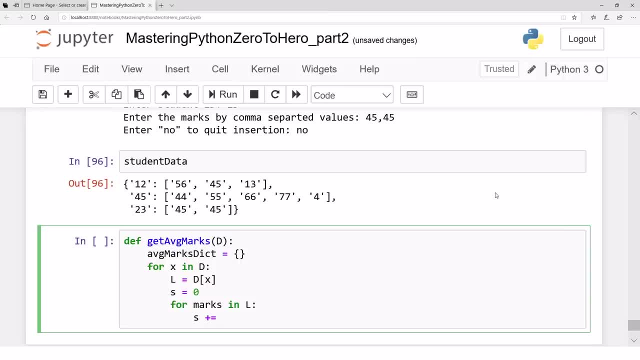 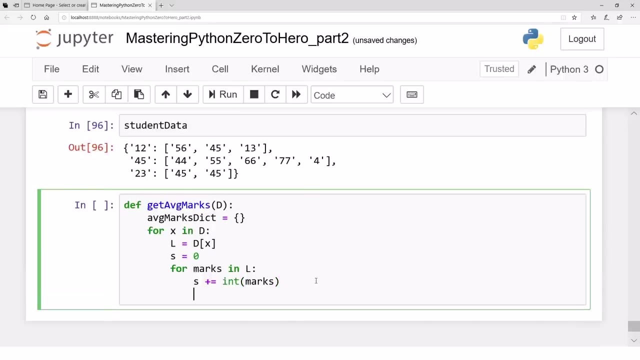 So what you do is S plus equals to marks, But convert the marks to integer because they are already in string format. We have saved everything in string format, So you populate all the list. Once you are done with this loop, the S will contain the sum of all the marks. 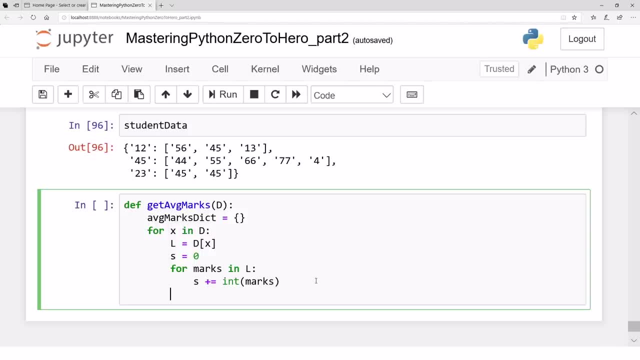 Then what you do is you compute the average and just save that average in AVG marks, dict, dictionary, let's say, Or average marks, Just don't use the word dict, for example: You can, but let's stay casual. And at X, you just write the average marks. 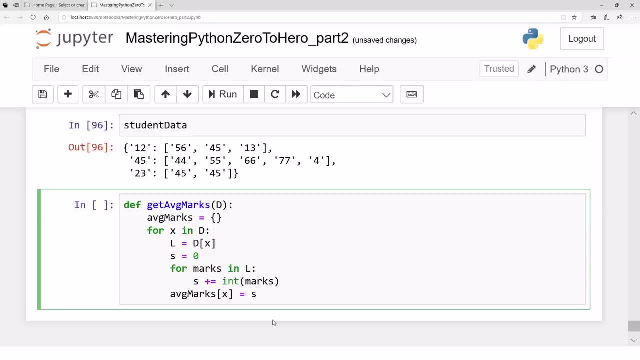 And the average marks can, Can be computed by S divided by the length of the list, whatever the list is. So that's what the list is. Yeah, So that's the average marks, And once you have, And one by one, all the average marks will be populated. 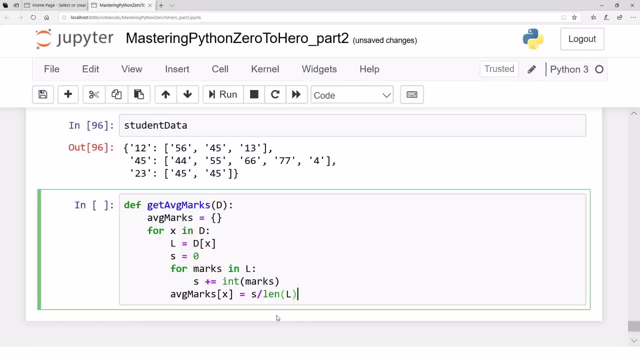 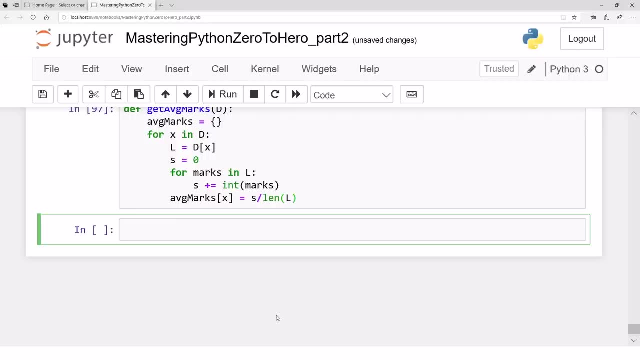 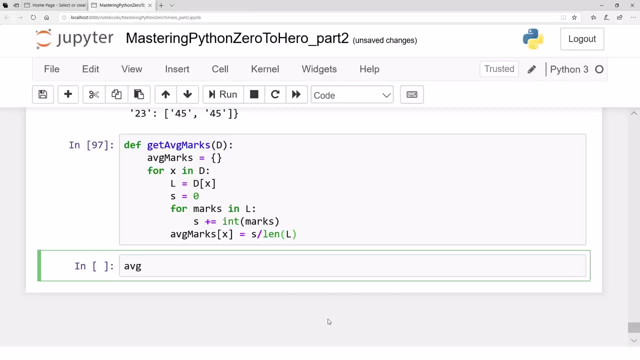 And once we receive all these, we will, then We can, then We can then just display by populating the average marks. So let's see, Let's call that function, So, let's call that function. So AVG marks, for example, equals to get AVG marks. 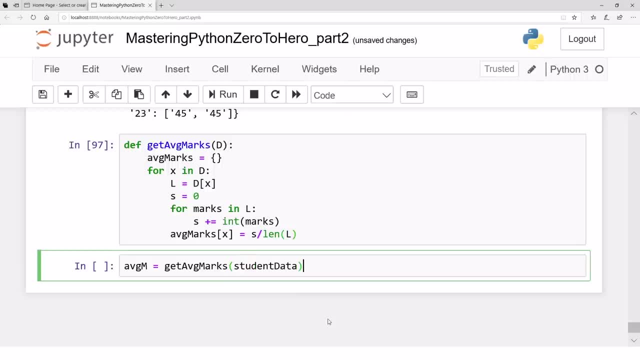 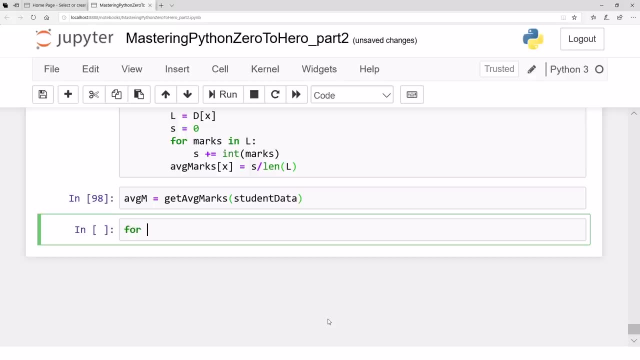 And let's put the student data inside And if there is no error then it will return everything. Then just print the average marks for each student for X in AVGM And print, let's say, Student, And then print X. 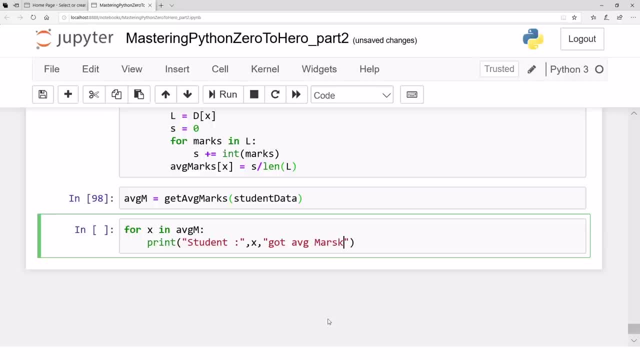 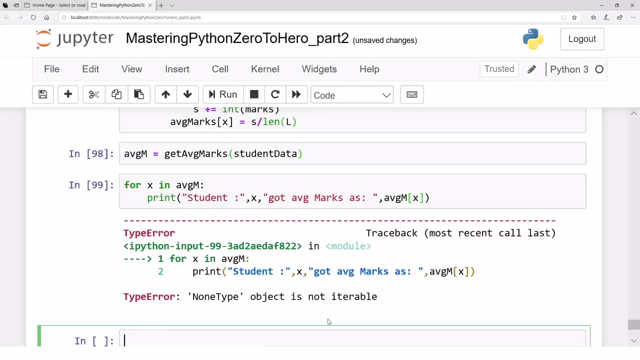 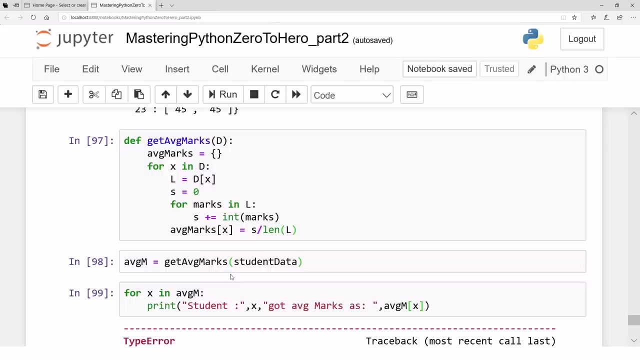 Got average marks as, Then you just print OK, AVGM of X, X And that will display everything. Oh, if there is an error, None type object is not iterable. Iterable None type object. Why none type object? We have done some mistake. 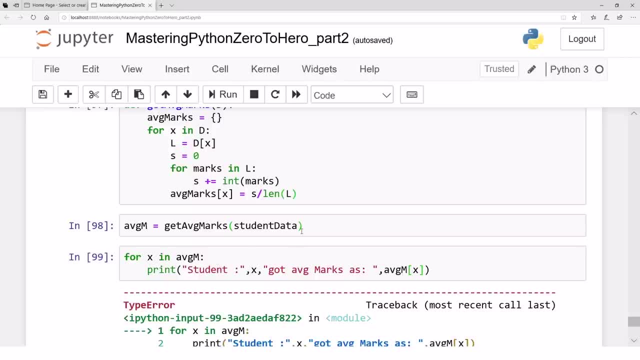 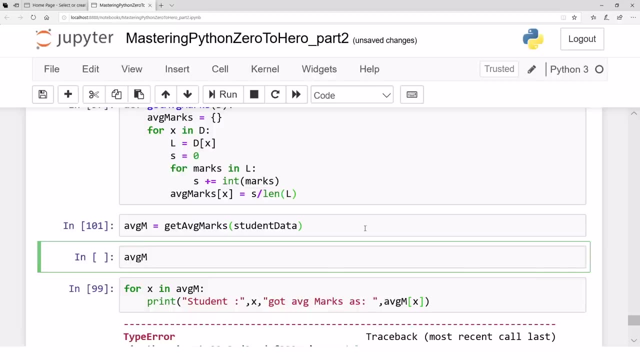 Yes, Maybe Let's see. Let's see, for example, when we have run this. So let's run this and create a cell. Let's run using Alt-Enter, It will create a cell. AVGM- What is that thing? 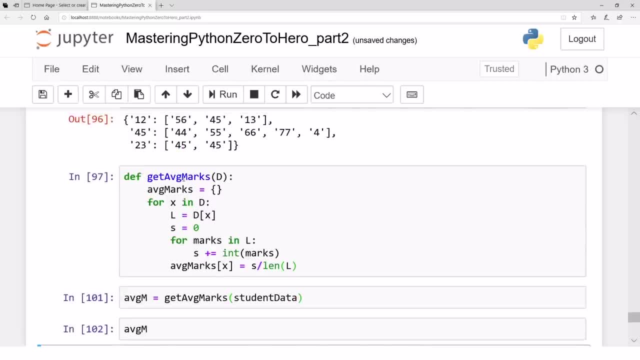 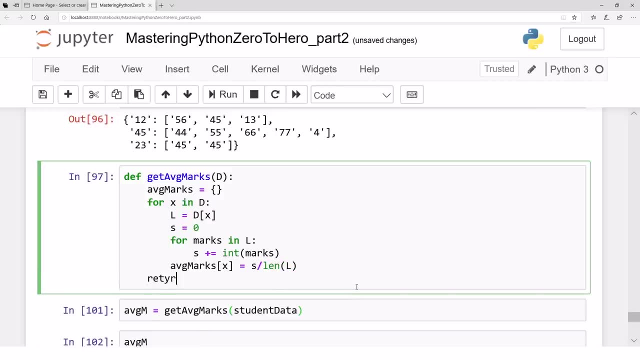 Oh, that is nothing. Why? Oh, we haven't returned anything. That's a. That's a bad programming, Really bad programming. We have not returned actually the value that we need, So the default value is none. 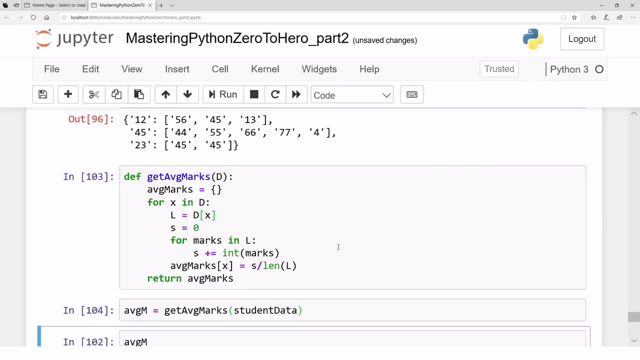 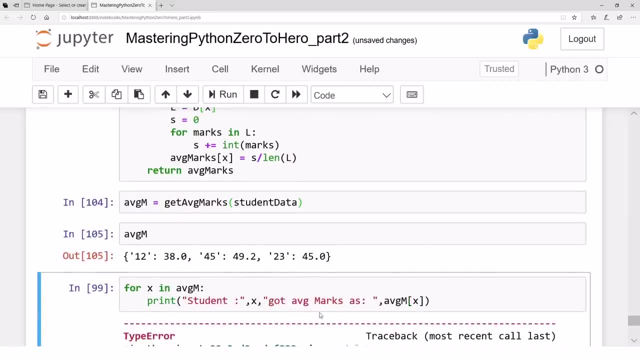 Great, Actually not so great. Okay, great, Yes, this, And now we have something in average marks. Yes, this is, And now we can just populate that And we have the student 12.. Got average marks 38.. 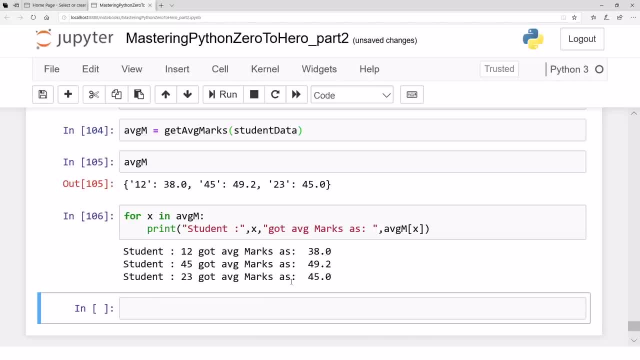 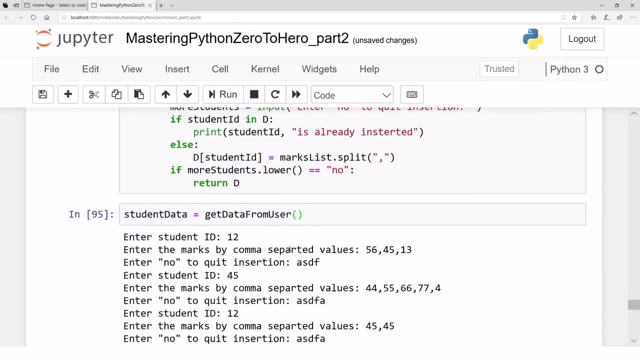 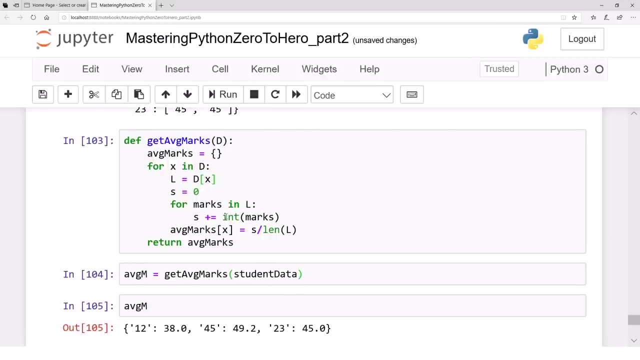 Student 45 got average marks 49.2. And student 23 got average marks as 45.0.. Okay, great. So that was just a review of split function of string type conversion through int and functions in general, input function and dictionary and list and all that stuff. 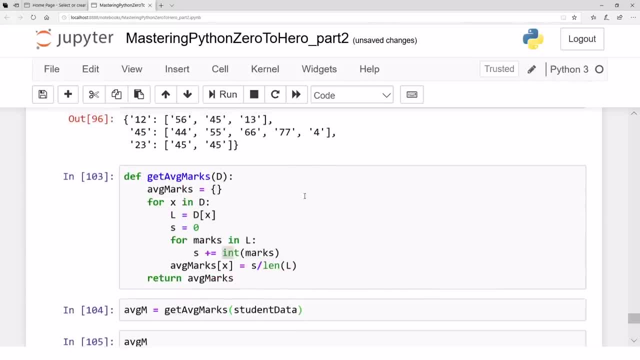 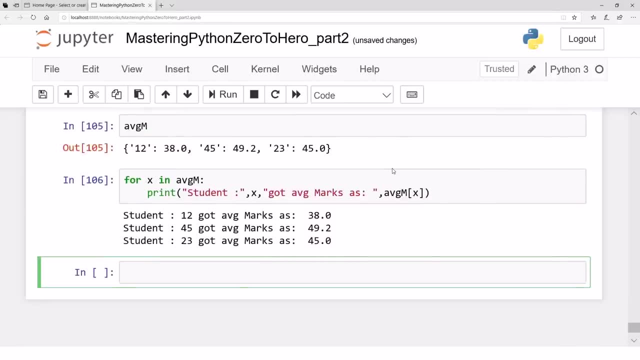 So, although It wasn't just a tiny problem, but it gives a good flavor of the data structures and strings and all that stuff. Okay, that's about the data structures. From the next video we are actually diving into the data science packages. 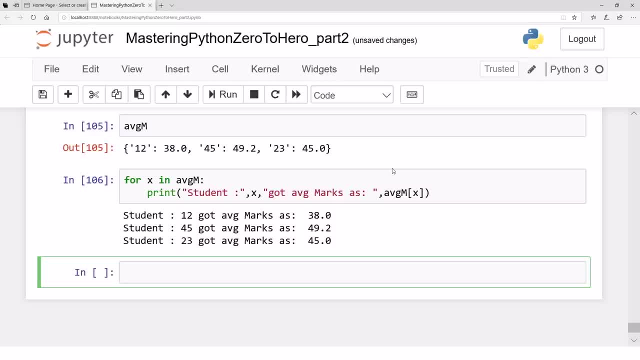 And we will start from NumPy and we will spend some time on NumPy and then we will be moving towards Pandas, Which is very, very powerful, built on top of NumPy, And after that we will be moving towards Matplotlib. 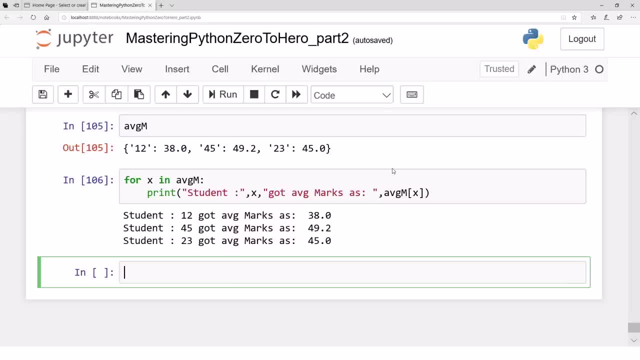 And we will also try to give you some snapshots of gets Pscykit Learn as well. So hope to see you in the next video. Okay, adding to that which was a little moonshy for some of the others subjects, that 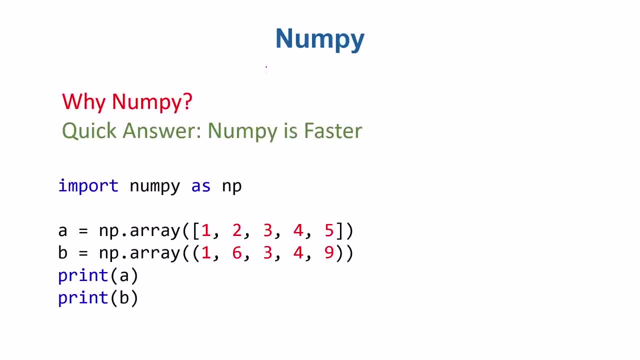 a little events would be. or the very, very, very popular package, numerical Python. actually, numpy is like list, but it is much, much faster than list. one one restriction: if we restrict the list- remember a list actually is a collection of a lot of data objects. that was so abstract, as we saw in previous. 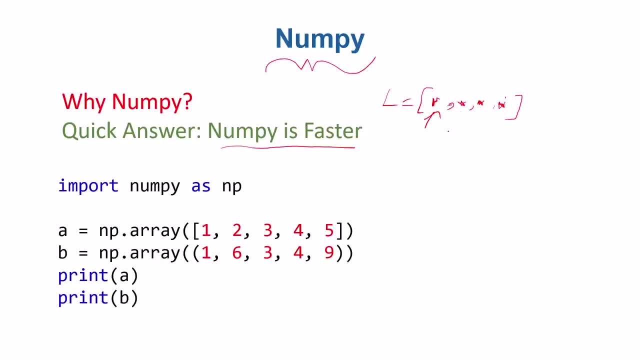 videos. if, for example, we restrict a list that all the objects they must have same type, all the elements in the list, for example, they have same type, then that list with all the same type, there is what the numpy looks like. but numpy is very, very more faster. and the reason is, even if you define a list with all the 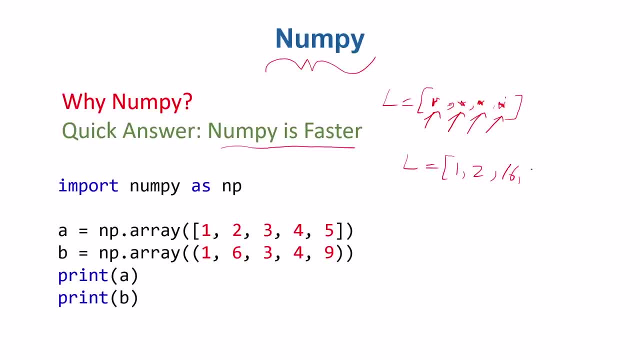 elements that are, let's say, of same type. you, yeah, but because list in abstract way can handle heterogeneous kind of objects, the functions that we will apply on these items, they will no longer be faster further to store each element. we have to store that information or metadata for that element in numpy. it is both. I mean it is efficient, with respect. 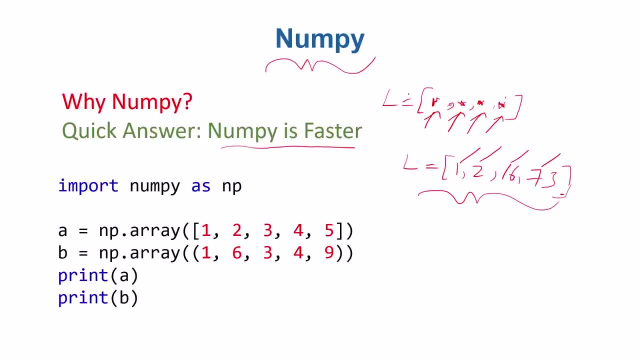 to memory, because if the type is same, we need not to save information about each element, because we need just to save the information about the type, because it's all elements, for when the type is same we can write function that are much more faster than then last. so numpy is very, very popular. it has very, very fast. 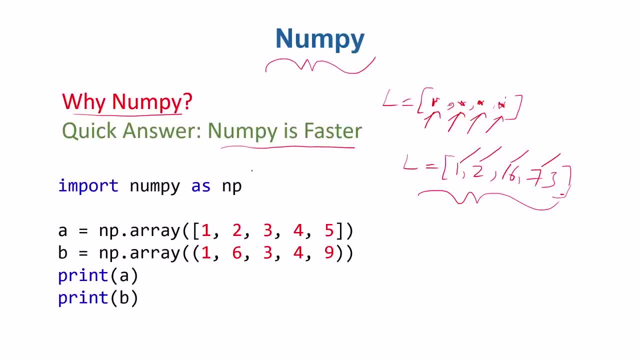 universal functions available, the methods that are all of them. by lets the package, I mean it. so it's a whole director Defenceเรา. loads of packages inside a lot of these, and so much uh. at the end of the day, it's uh, it's, it's uh. simply, or in layman terms, it is like a list with 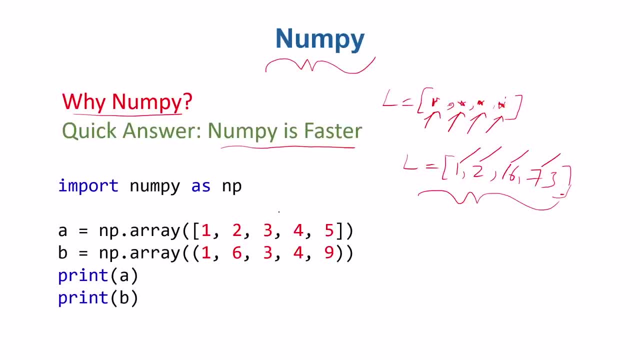 all the same type objects and it is much more useful when all these objects are numeric type, although you can have a numpy array with, uh, with string data types. i mean, all the strings are all, uh, general objects as well- but the the most the the power will the power of numpy array will be. 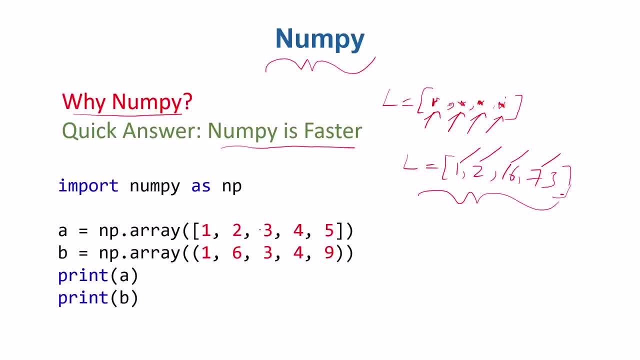 will become much more evident when we will be working on numeric type data. so in this particular um, in in this particular uh course, we will focus more on numeric data uh than other kind of data. so, um, that's how you you write, import numpy is installed, or if you, if you have installed python. 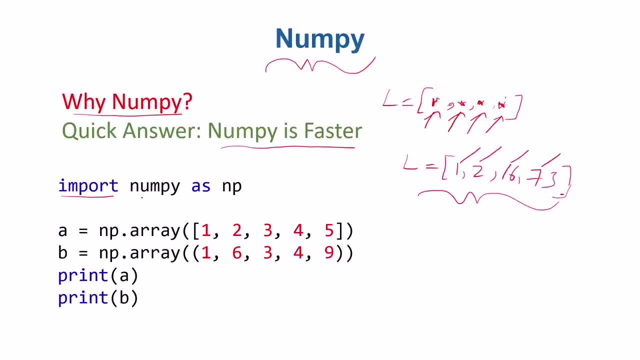 using anaconda. numpy is already installed there. uh, it is in the site packages, kind of a built-in package. so, um, that's how you you can write import numpy. we can stay as it is, but we can rename this numpy just np. that's most popular name. we can write any other name, but if you see the books or internet or 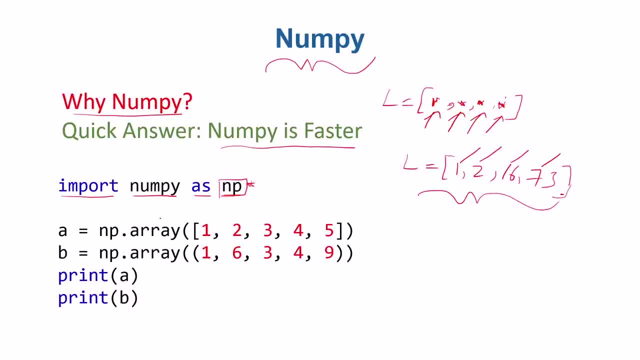 somewhere this np somehow becomes much more popular. okay, now we can define an array, for example np, dot array. that's arrays, just a method of np kind of function, and we can define, uh, an array using list- this is the list of several numbers- or we can define array as, as a tuple. 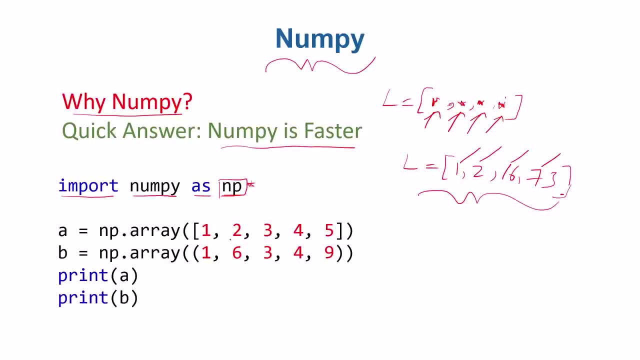 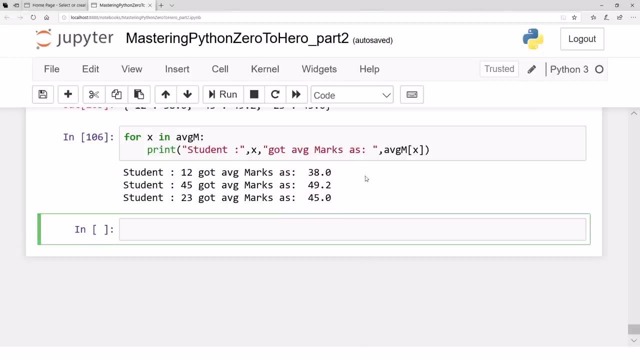 as well. so, whether we give a tuple, whether we give a list, and array is defined and then we can see the contents of this array, uh, this np array. so, uh, let's, let's just go to our friend jupyter notebook and gets our hand, uh well, gripped on on this numpy. so first of all, we need to import numpy package. 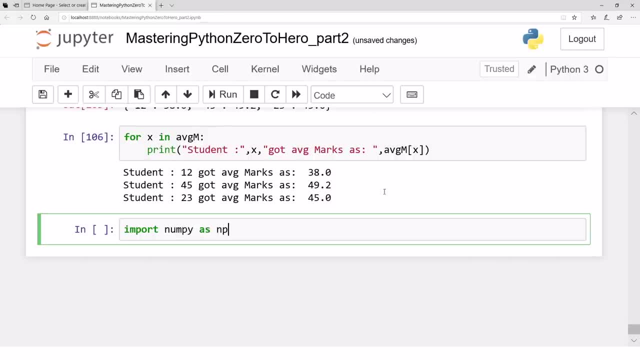 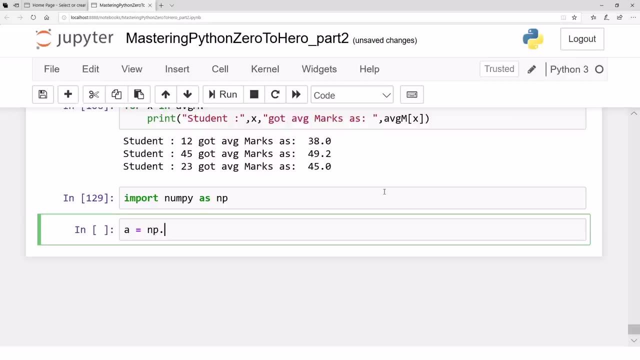 and we may rename, as for future use, as uh, np. so let's say that is important, right. so now let's say a is an array, let's say nparray, that's a function, and we may have a list inside. let's say one, two, three, five, seven. let's say that's a, that's array. we can also. 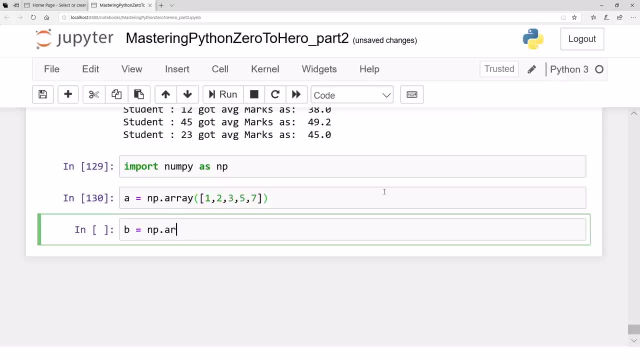 define the array using a tuple rather than a list. it's our choice. uh, which way we define the array either way. um, two, three, five, let's say that's, that's another array, for example. so if we print, for example, a, it will give us a, but if we just 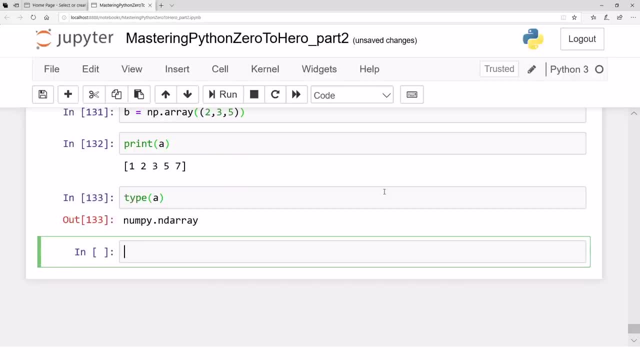 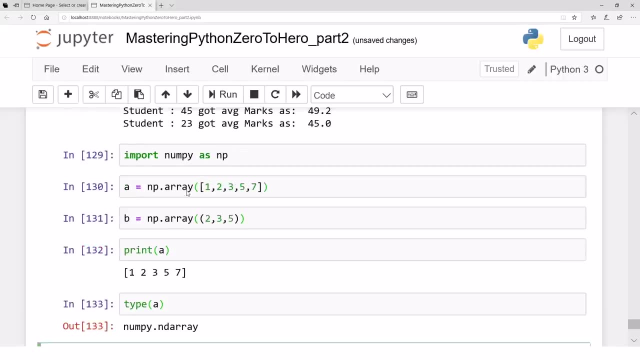 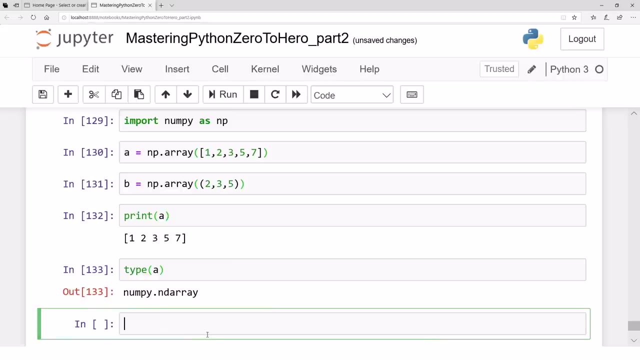 see the type of a. it will no longer be a list, it will be an nd array. numpy dot nd array, that's an dimensional array. okay, great, so there are so many attributes of this a and this b same. similarly, if we see the type of b, although we have defined this b, 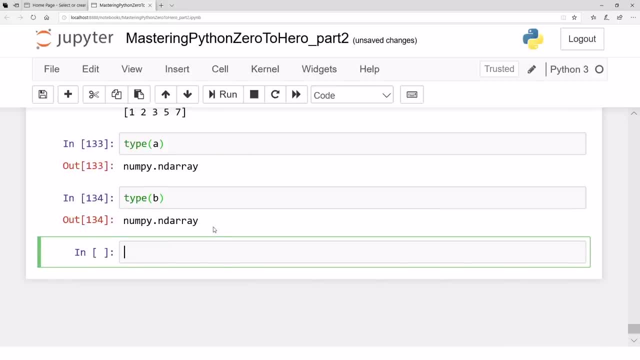 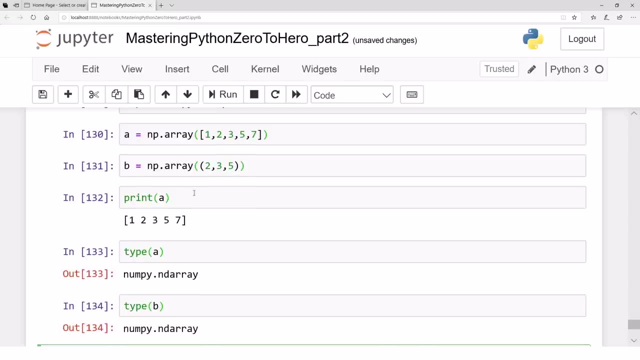 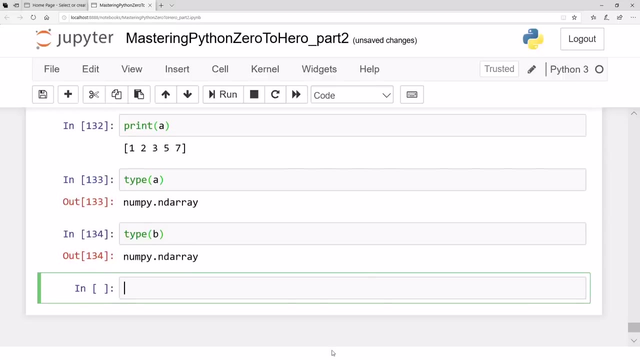 using a tuple, but the type is the same. it's a numpy object rather than a list or a tuple. so that's how you can create the, the array one one. one more thing that is that is important is to to check the attributes of a, for example, a dot d type. that will tell us the data type. 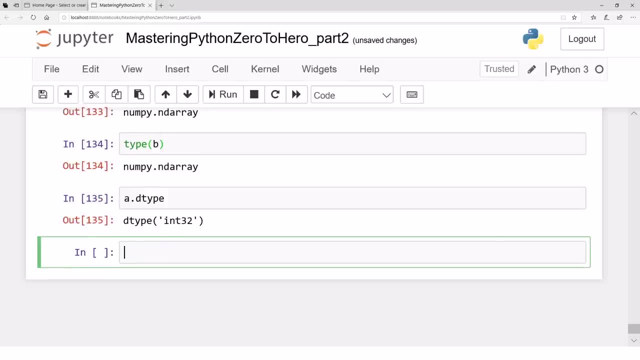 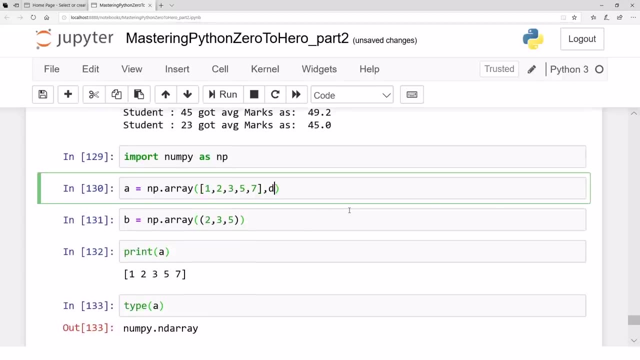 in a. so, for example, a stores all the data, that is integer 32 at defined time, for example. we can, we can specify the data type if we want. we can specify d type if we want. for example, integer, that means a is integer. here we can, here we can define, for example, d type. 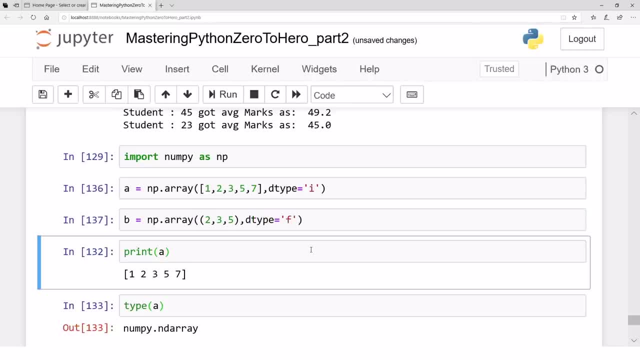 as float, for example, so data type becomes float. there are several other other options that are available to define the data type. but but even if we don't define, the data type can be defined automatically based on contents. that's what the dynamic typing means. so if we now define type, that's this. if we, if we now check the 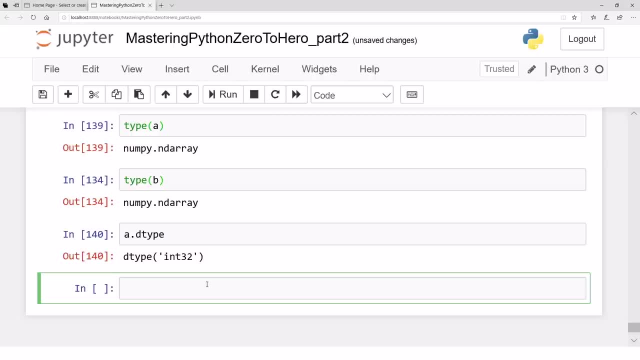 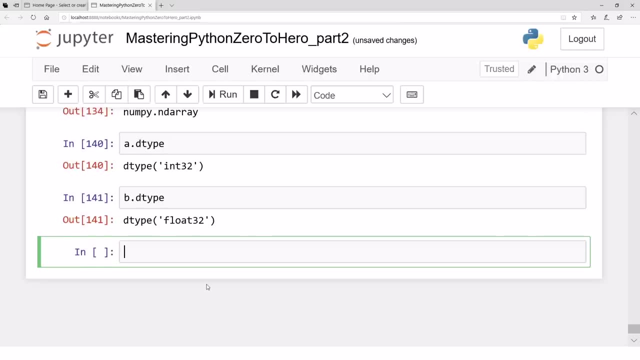 type of a, that is again integer 32. but if we check the type of b, d type that a, that might be a float number. yes, that's float 32. again, there are 64-bit support as well. i mean, we can define here. there are multiple options available. so that's the. that's how we can define the numpy array. that's just. 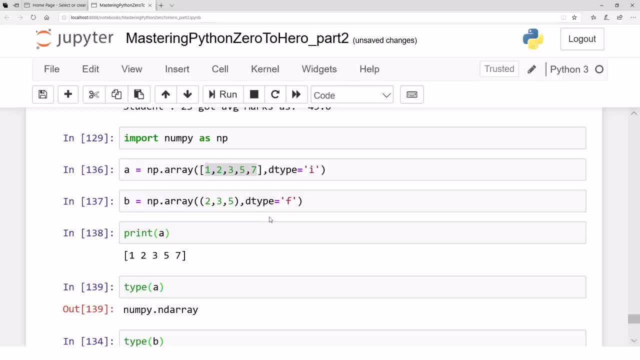 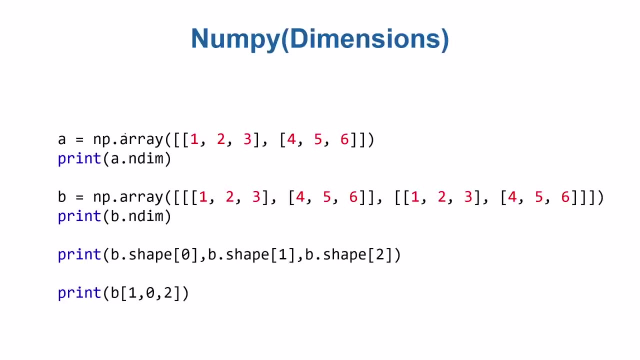 getting started with numpy array. in the next video we will play with these arrays a bit more, so hope to see you in the next video. okay, in the last video i introduced numpy and we actually declared a numpy array using a list as well as a tuple. in this particular video, we will be seeing some of the properties of 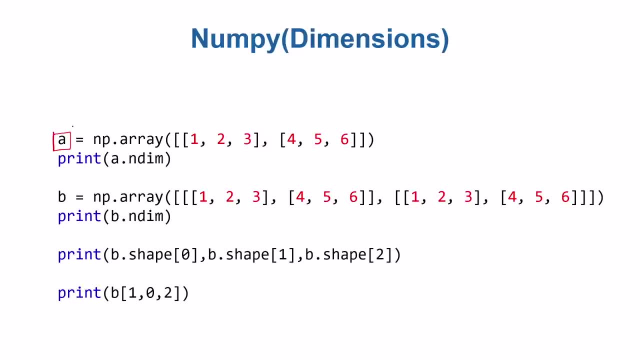 pri array variable, or sometimes called the object that variable. so there are several properties, but i will discuss. for example, last time i discussed one property which is d type, a dot d type, and that store actually the in that actually stores the information of the data type of the elements. 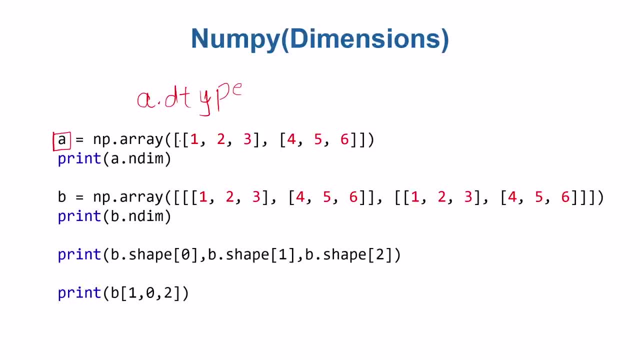 of the array, of np array. remember np array, all the elements of np array. they must have same data type. it cannot store heterogeneous arrays. as it is okay, now there is another property, sometimes called the dimensions, or n dim, that tells actually what are the dimensions of, of, of the array. 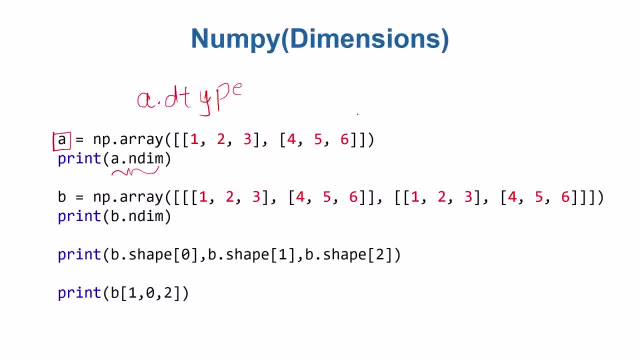 i need to explain this term dimensions with the following example. let's say, for example, that's that's, that's an array. just consider that's a list. for example, one, two, three. that's one list. and if it is, if it is an array, for example, if np dot, if this is np dot array. 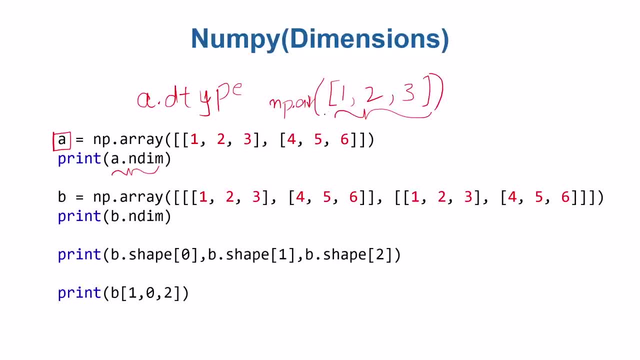 with that list. we will say that array as a one dimensional array, because we only need one index to access that. for example, if you need to access any element in this array, you only need one index, either zero, one or two. only one index, that's okay. so in this case we have just one dimensional array. 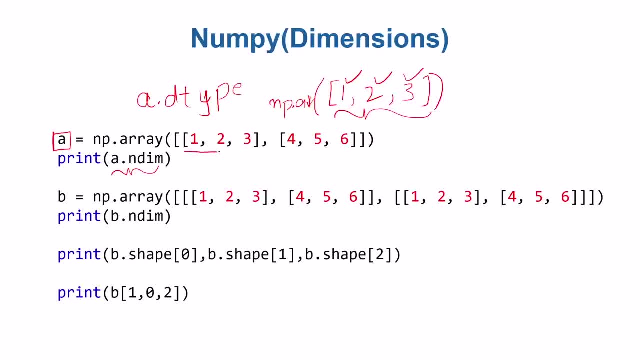 so we will say one now. if we need to access any element in this particular array, we need two indices. first of all, we have to locate whether we are going to talk about a1 or a2. we need one index for that. for example, if we want to locate a1, that means we are going to access with element zero. let's say: 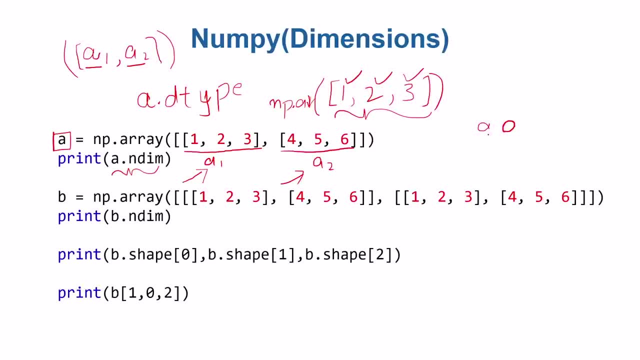 this, this whole array is a. so first of all we say, okay, zero means we are going to access from from a1 and a2, one of those. so zero means the first one. okay, now a1. now inside a1, which element? this is the zeroth element, this is the first element, this is second element. let's say: 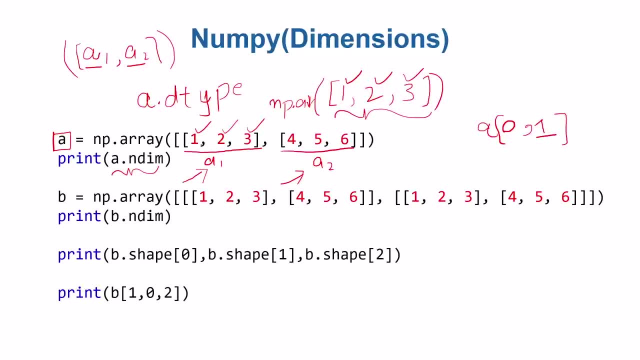 we want to access the first element, so that means we are going to talk about we are talking about this. so, very loosely speaking, the total number of indices that are required to access an element inside the array is called dimension of the array, an end dim that actually. 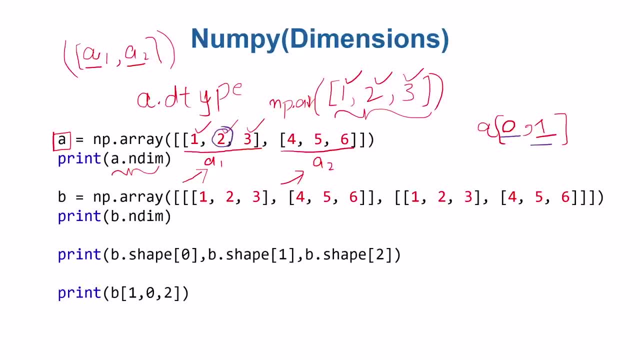 that actually defines that. that actually describes the, this property, the total number of dimensions. consider, for example, this is a 2d array or two-dimensional array. let's say that's a two-dimensional array, a1 and less, that's another two dimensional array. a2, that's another two. 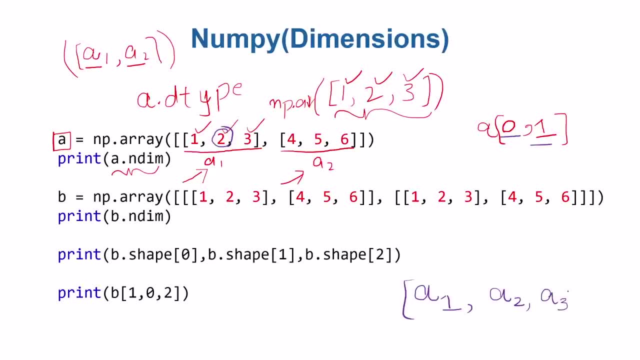 dimensional array a3, for example, and let's say this is an array of two dimensional arrays. let's say: and p dot array. now that that's that whole array, whatever that array is a three-dimensional play and the reason is to access any element. we need three indices. first index will define which one of these we are selecting. 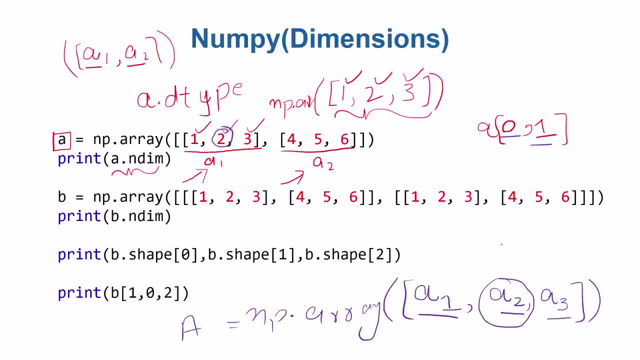 for example, let's say we are selecting that, so one index is needed. that index is one. for example, then inside this structure, like so we need two more indices to locate a particular particular index, for example, because it a2 is a two-dimensional array, it has two one-dimensional 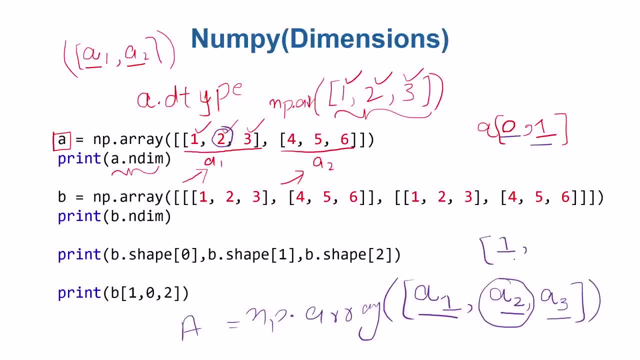 arrays. so which one-dimensional array you are? it has more. it has many one-dimensional arrays. so which one-dimensional array you want to pick? let's say the sixth one with index, with index five. now you have located the fifth, a sixth array. now in that array, what element? let's say the eighth. 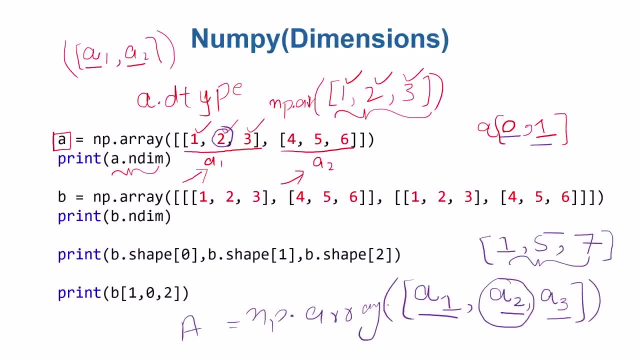 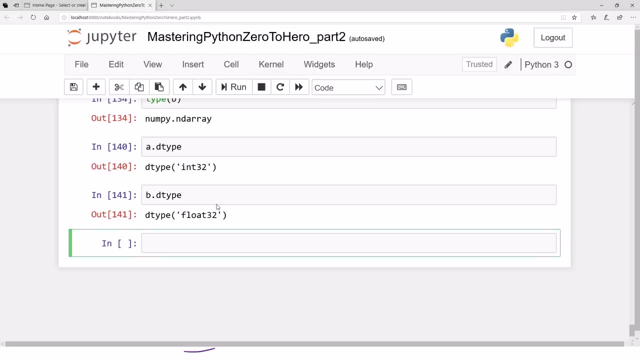 element. so we need three indices to access a particular element. so the dimensions of this array is three. so let's play with that in Jupiter notebook, just to get more comfortable with with the term dimensions. so let's say, for example, we have an array, let's say a is np, dot. 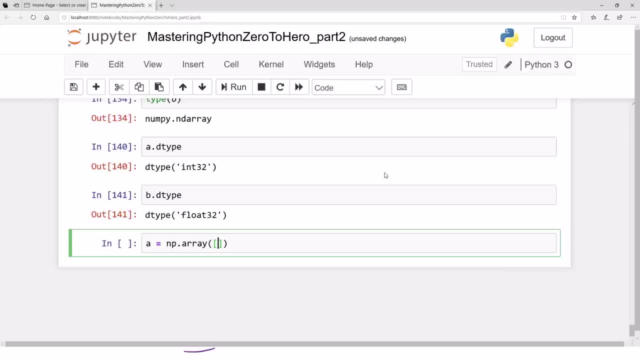 array and let's say it contains a list. let's say one, two, three, and then we have another array, one dimension array. let's say 4, 5 and 6. that's another array and that is an array of these two arrays. so that is basically a two-dimensional array. it is array of arrays, a list of. 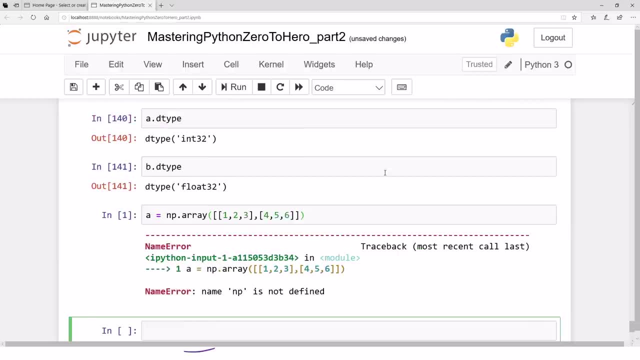 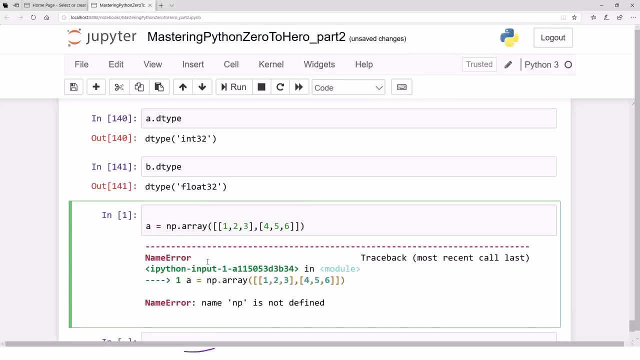 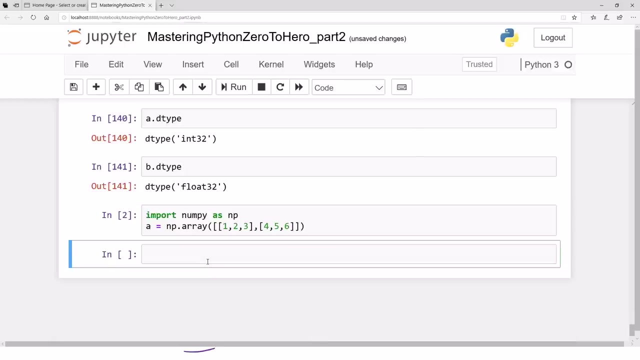 lists equivalently. so that's a for example. oh, what's the problem? oh, we have an imported numpy we should have, so import import numpy as NP. okay, we need not to import that every time. actually, I'm recording this video after a few, after a few hours, and I'm reason, I have restarted all these things, so I have to. 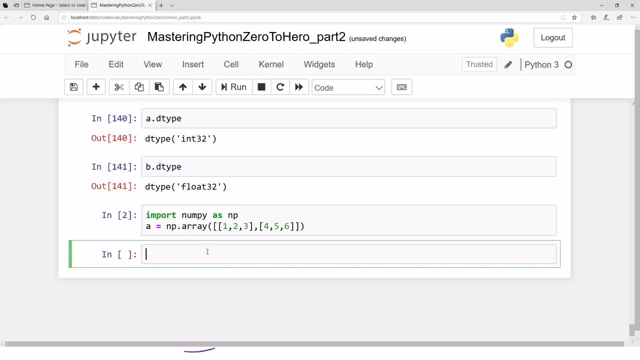 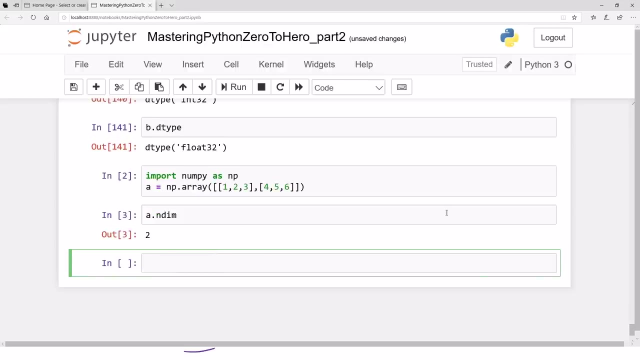 import now for the first time. but once imported, imported in the notebook, as long as a notebook is running, you need not re-import anything. okay, so a dot, for example, and them. a dot and them. so that is two here, because there are two dimensions. for example, if I want to, 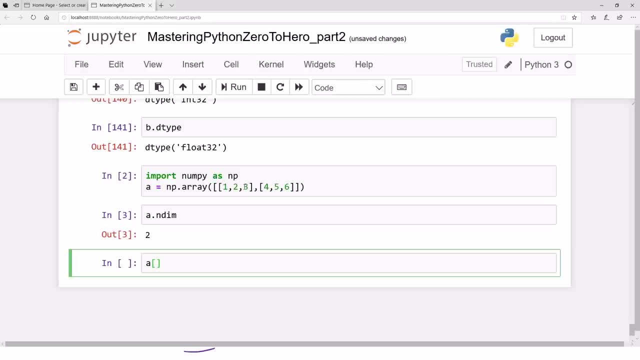 access element number three: this element. so this element is located in the first array of the two arrays which has. so the first array. there are two arrays, it with index 0 or 1, so I am going to look into the first array, which is 1, 2, 3 and 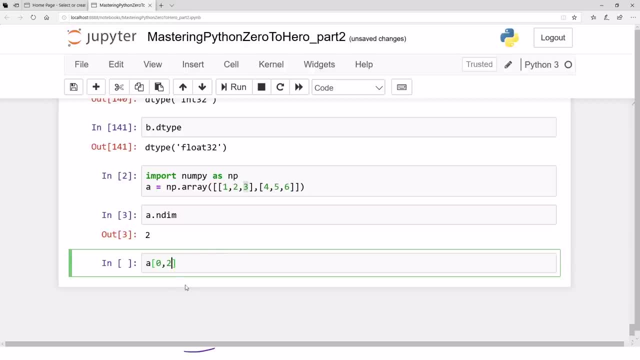 in that array I'm going to look for the element number two, element with index 2. so that's how you can access the elements of multi-dimensional arrays or arrays with more, more kind of dimensions. let's say, we have another array just to, just to get more familiar with NP array. let's say, and we have a list and that's. 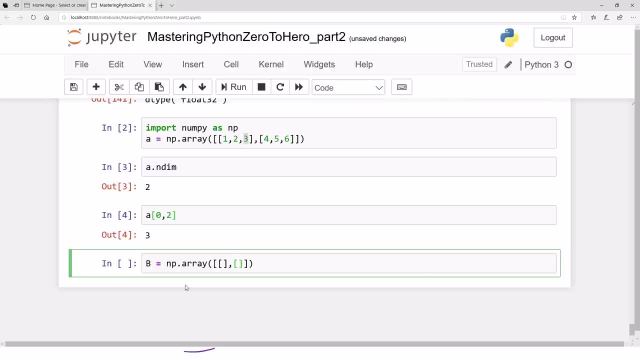 that list actually contains. that list actually contains three one-dimensional arrays. not only that, actually. oh, I'm confusing you a lot. let me. let me just. let's say we have one, two, three. let's say we have three one-dimensional arrays. let's say we have another two, four, five, nine, the, the sizes of arrays. 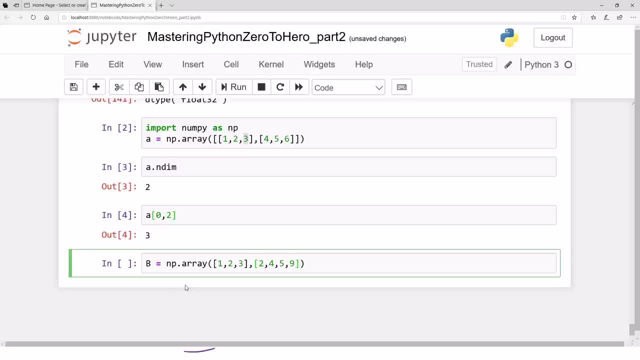 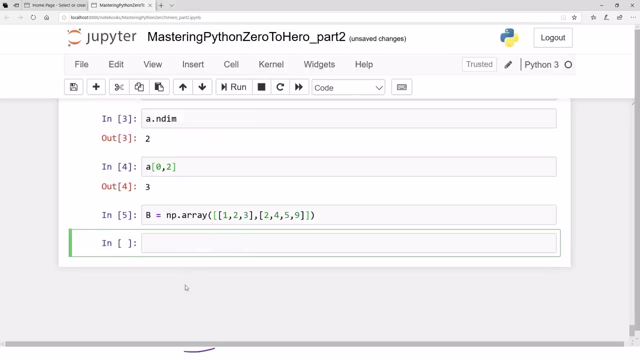 maybe, maybe, maybe, I mean maybe different, yeah, is that true? maybe different, yes or no? let's see, for example, the first array has size 3 and the second array has total size. is that okay? I guess yes. and now, if you want to access, for example, an, 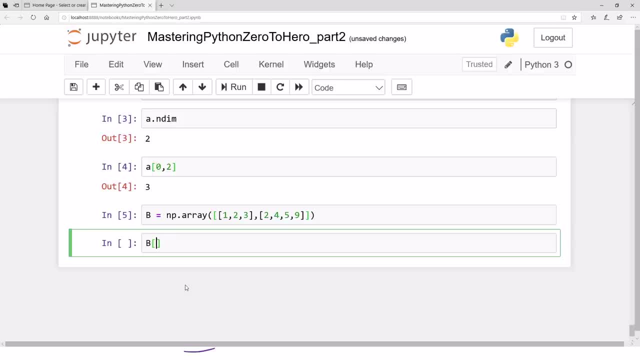 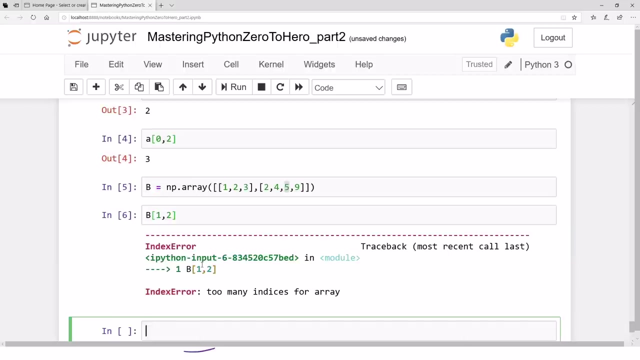 element of an element with. let's say, I want to access this element five, so that is in the second array indexed with one, and then in that array it has indexed two, so I've accessed this element. oh, why not too many indices for an array? why, um, why is that? why too many indices uh for for an array, uh, B. so let's say B, dot, n, dims. 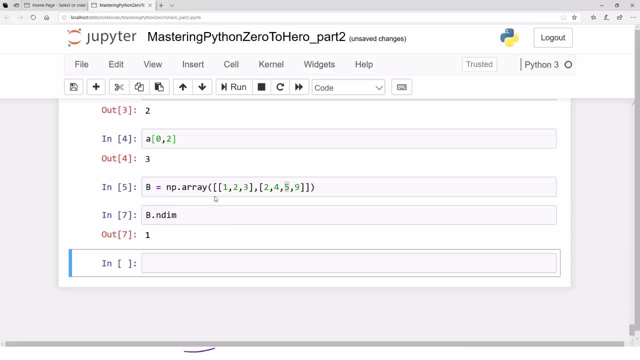 and then that is one, why one-dimensional? I have two. uh, I have this one-dimensional array and this is another one-dimensional array and I have made a list out of it. I mean, this is one D array and another one D array. I've concatenated them together, so I should have accessed this element. the problem is when you are 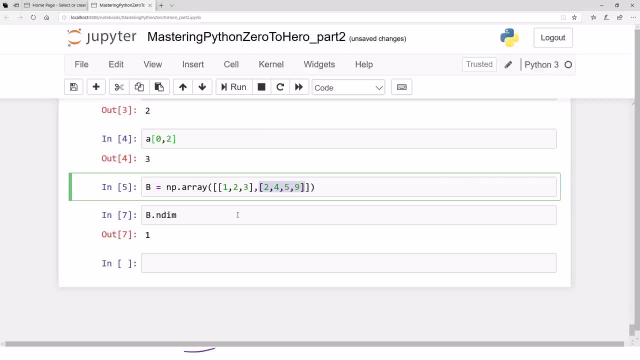 going to define multi-dimensional arrays the the number of elements for each dimension. they should stay consistent. for example, if the first array has three elements, the second array must have three elements. or if the second array has four elements, then the first must have four elements. if that is not the case, uh, the array will not. 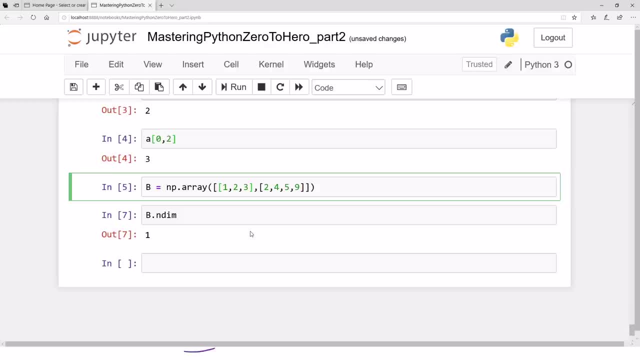 be defined like a multi-dimensional array. for example, if we, for example, extend our first array with, let's say, minus one, now B will be having two dimensions, no problem. and now we will be able to access, for example, this element five. uh like so. so we will go. 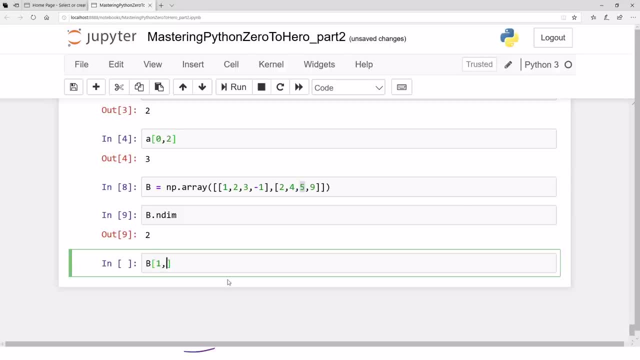 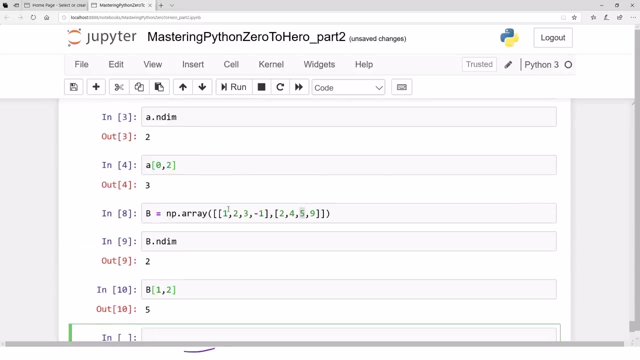 to go to b again, we will say, okay, select array number two and in that array, uh select, uh Index, Select the value indexed by two, which is five. so accessed, no problem, and that stays true. if you're going to define, for example, a three-dimensional array, let me 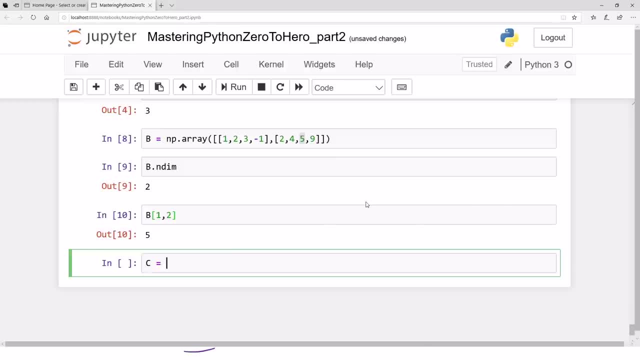 just give you an example of three-dimensional array. that's a, c equals np, dot array and let's say we have one, two, three arched array elements and we need to write down the fighters of the array. we also need lowercase andермands, the Val function, for this example. another three-dimensional array will not appear if we don't define it normally. each sentence will appear at напupack null, Install values andricht. 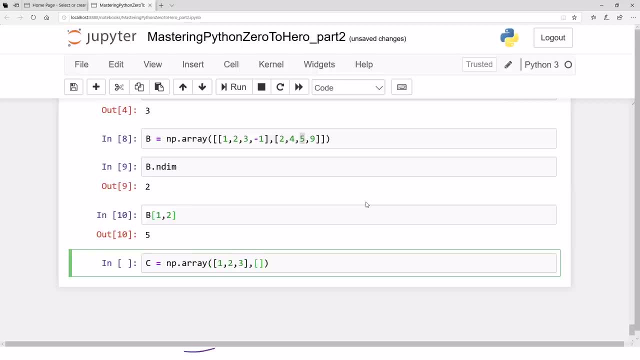 and 3, and then we have another array, for example: um, four, five, six, remember all. so let's say: that's uh, that's uh, we can have one more. for example, we can have one more list, why not? so let's say, we have a zero, zero minus one. let's say: and that is, that is, that is a two-dimensional array, yeah. 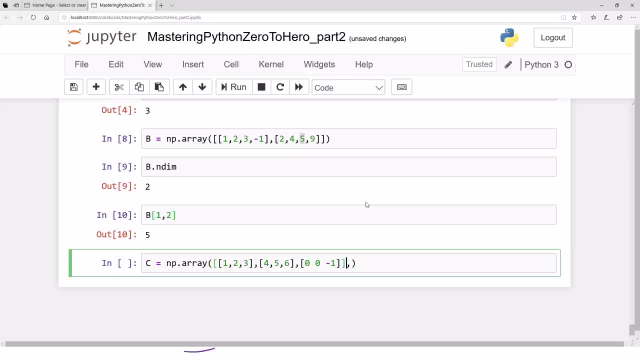 that's a two-dimensional array, great. let's say: we have another two-dimensional array. let's say, we have another two-dimensional array with same kind of consistency, the number of elements and stuff. let's say, these elements are all minus of the the other ones. let's say this: 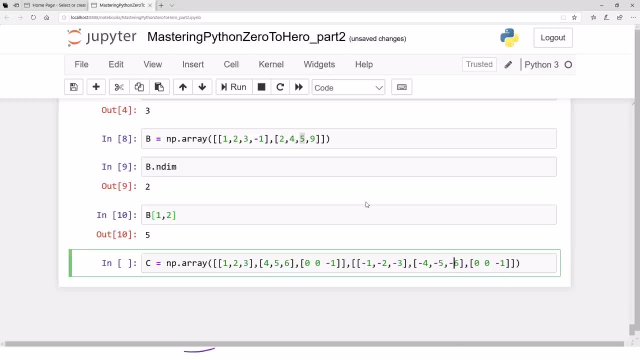 minus, minus, minus, and this is plus one, and now we have this. if, if you see this thing, that's a 2d array, that's a two-dimensional array, that is also a two-dimensional array. an array of two-dimensional arrays is basically a three-dimensional array. now, that's a three-dimensional array, this one. 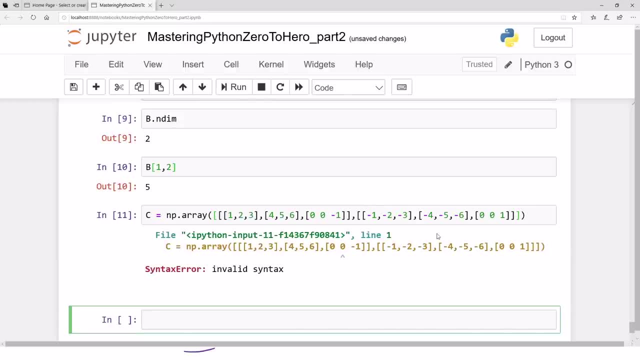 c. so if you uh, oh, we have some. oh, uh, i i should have defined this with commas rather than rather than spaces. actually, yeah, the reason i did that is matlab i i worked in matlab also, so matlab allows this, uh, space separated list, but i just confused the things with with python as well, but python. 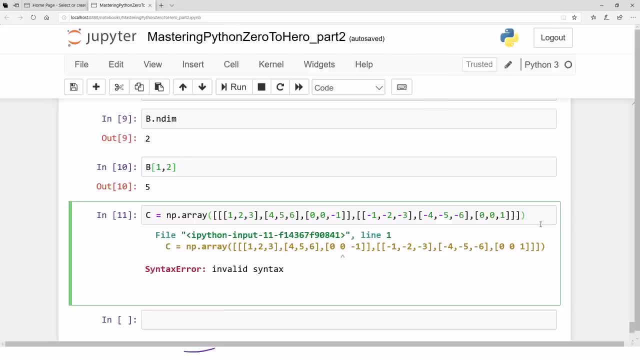 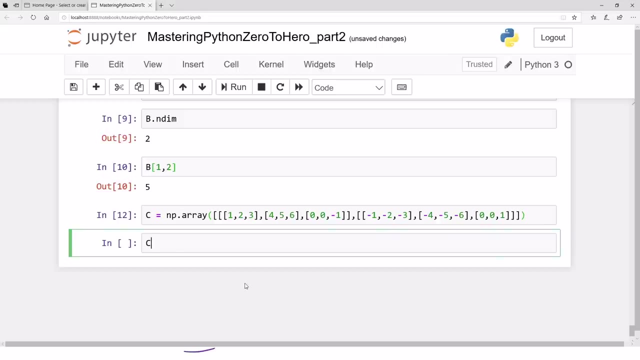 requires comma there. okay with matlab, by the way, just as a side note, matlab allows you to have commas as well as spaces. but this python is just restricts everything to comma. that's great. okay, that is c. so now, if you check c, dot, and then that is three. if you, for example, want to access 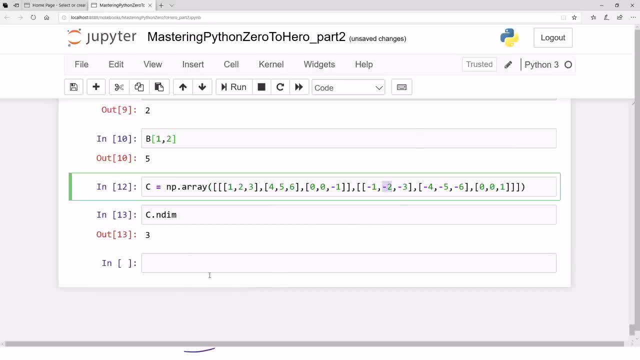 this particular element. what should you do? first of all, you select the the one of the 2d arrays. there are two 2d arrays, so this is the first 2d array and that's the second 2d array. and if you, for example, want to access this particular element, this particular element which is minus three, if 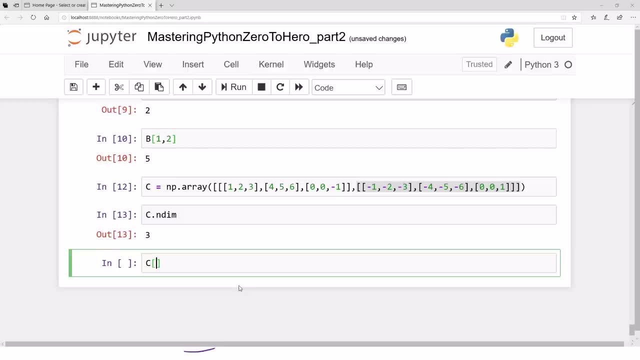 you want to access that, you first have to access one of the two, two, two dimensional arrays. so let's say, i access the second one with index one. now you are in this particular 2d array. in that array, which list, which 1d array you? 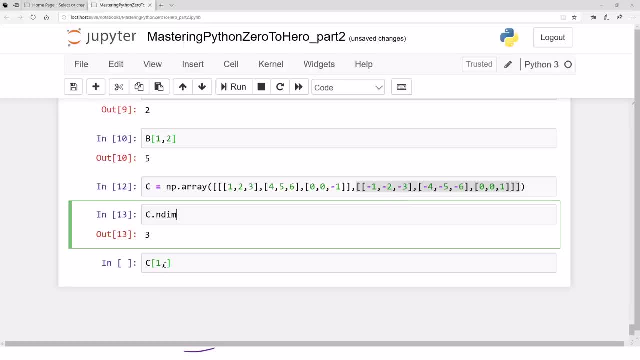 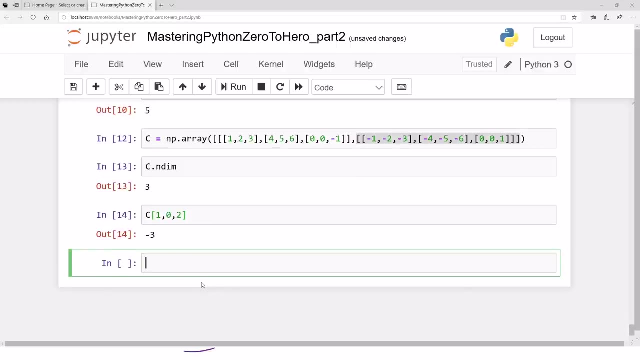 are talking about. so i'm talking about the very first 1d array. so the very first 1d array is indexed by 0 and in that 1d array, which element you are talking about? so i'm talking about this element that has index 2 in this particular array. so now if you press enter, you will get minus 3.. 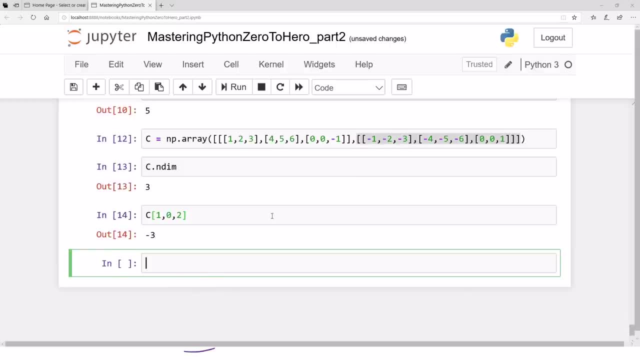 wow, so that is basically uh, how, and, by the way, you can make a four dimensional array. a four dimensional array will be an array of three dimensional arrays, and so on. you can make, uh, you can make, for example, n dimensional arrays, and that's one reason why we call this as nd array. uh, n dimensional array, the the type of 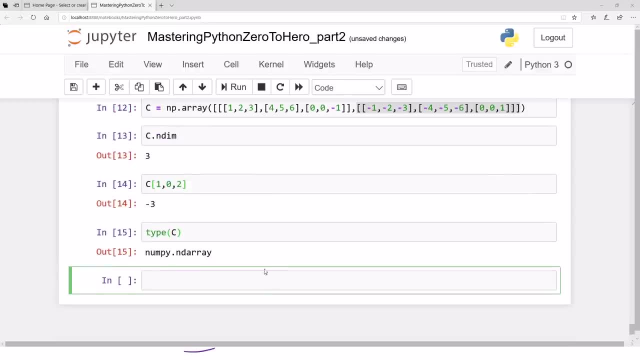 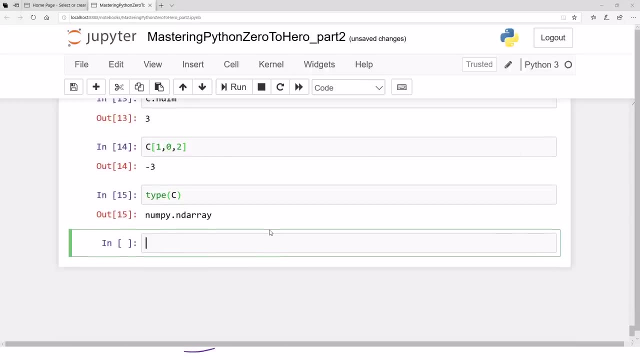 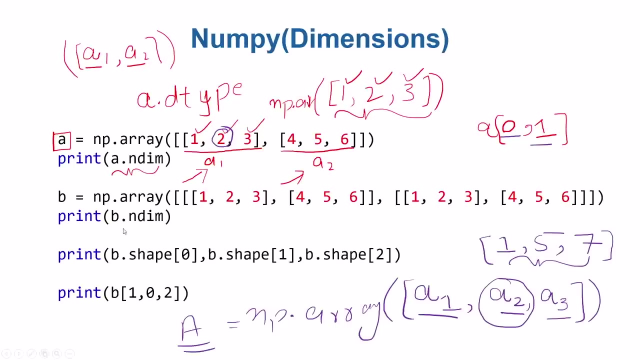 c is n? dere. and dimensionally, uh, you can add as many dimensions as you want. great, uh. we will continue exploring this numpy more and more uh in in the upcoming videos. in particular, I will talk about this shape property of this numpy. we have already discussed D type. we have discussed and in in the 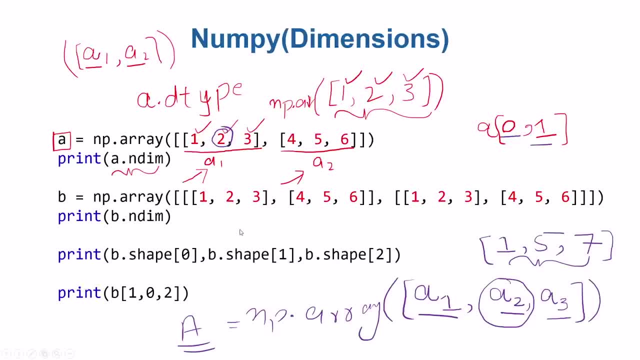 next video we'll talk about shape and we will discuss more about about the numpy. so hope to see you in the next video. okay, in the last video we discussed this number of dimensions or and in property of any, any numpy array, and we also saw an example of defining a three-dimensional array in Jupyter. 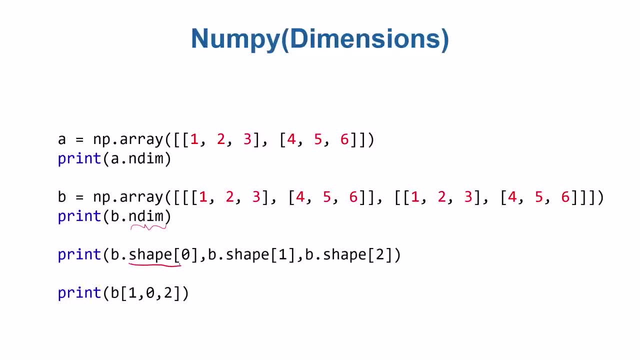 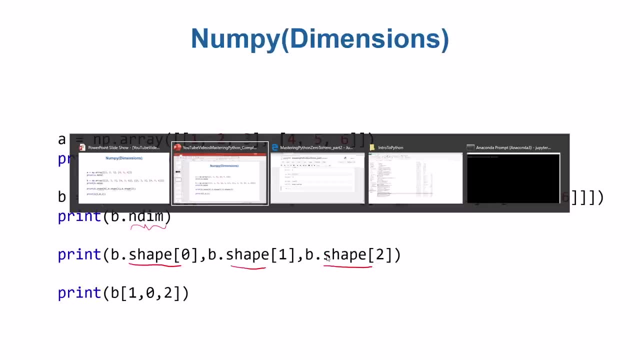 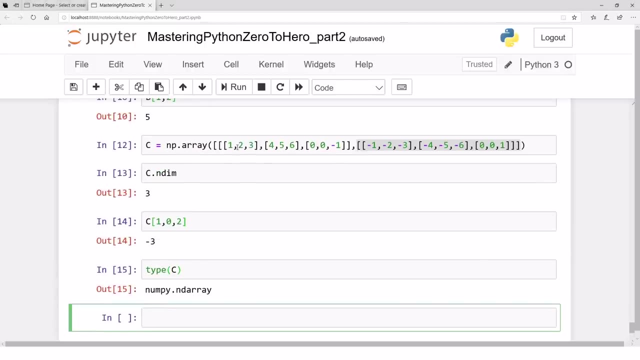 notebook. let's discuss another property, which is which is the shape property. let's see what what this shape actually represents. so let's go to Jupyter notebook and see what actually this shape represents. for example, you have seen this C, as in the last video we defined this C. 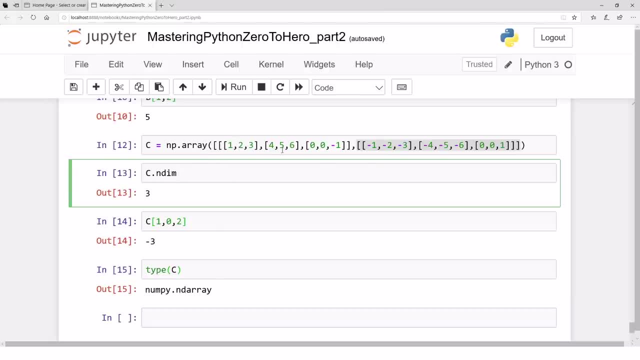 as a three-dimensional array that contains two arrays of 2d, and each 2d array contains three 1d arrays and each 1d array contains three elements. so what do we mean by shape? so if we just say shape, what is that thing? so shape is 2. 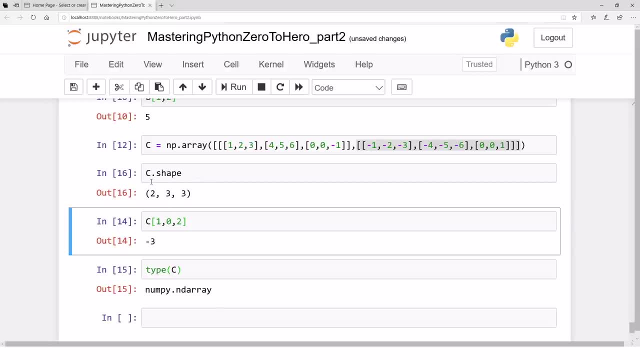 3, 3, and let me tell you what that means: the, the return is tuple, so that's a tuple that is returned to 3 & 3. this 2 means how many 2-dimensional arrays are there? here we have two. so in each two-dimensional array how many 1d. 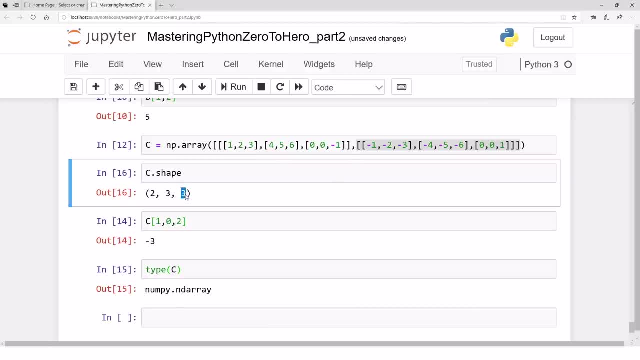 arrays are there? well, 3. in each one the array. how many elements are there? well, 3. so basically this: see dot shape 0 tells you the total number of two dimensional arrays, that is, two. and this shape, for example, one, tells you in each 2d array how many 1d arrays are there. these many, and this shape, for example. 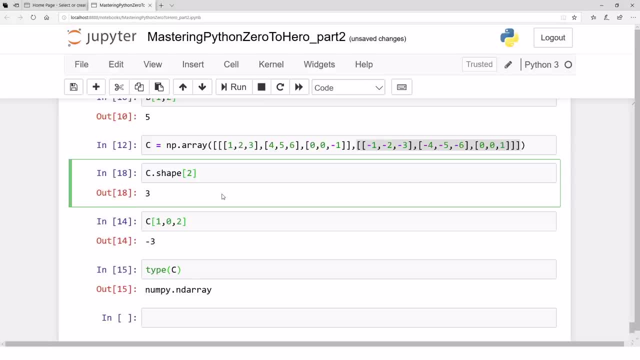 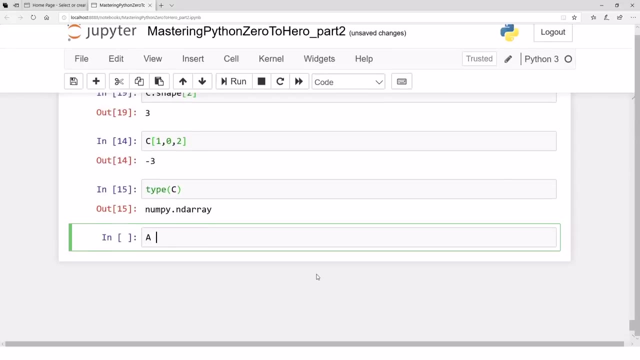 two tells you in each 1d array how many elements are there. well, three, great, that's awesome. um yeah, uh, can i tell you one, one, one strange kind of thing you can. you can define a numpy array, for example a as np dot array, with just one element. let's say two, that's an array, great. 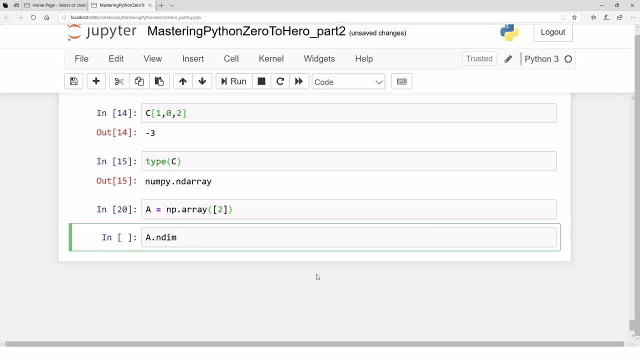 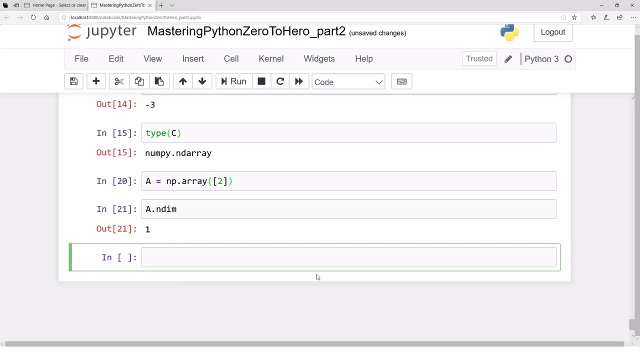 what's the number of dimensions here? what do you think? what is that? is that a 1d array? what are the number of dimensions? strange, it's a 1d array. yeah, it is um. see another thing. for example, b is equal to, to nparray, and you define it with, let's say, 3.. And what are the dimensions of b? 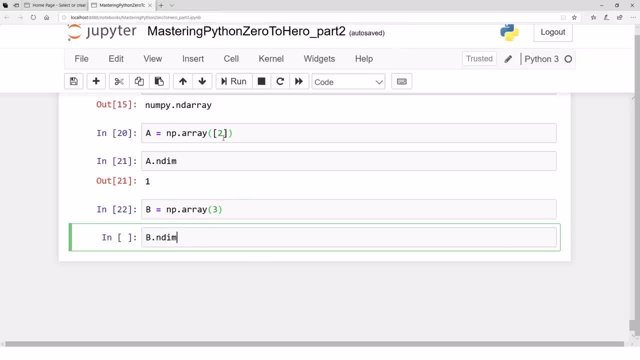 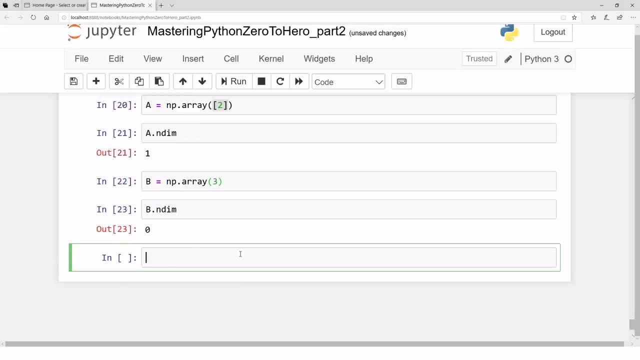 It looks like the same. the dimension of b should be 1,, as there the dimension of a is 1,, it looks like the dimension of b is also 1.. No, it's 0,, because that's an array. 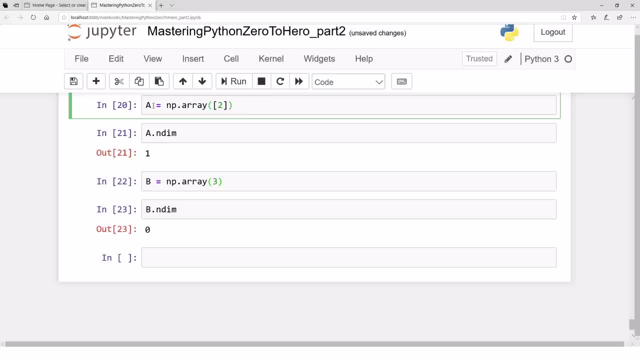 If you pass it as a list, it's an array of 1d. If you just define just one number that can be defined as an array, numpy allows you that, but that one number is just a 0d array. Now, if you concatenate a lot of 0d's, you get 1d. If you concatenate a lot of 1d's, 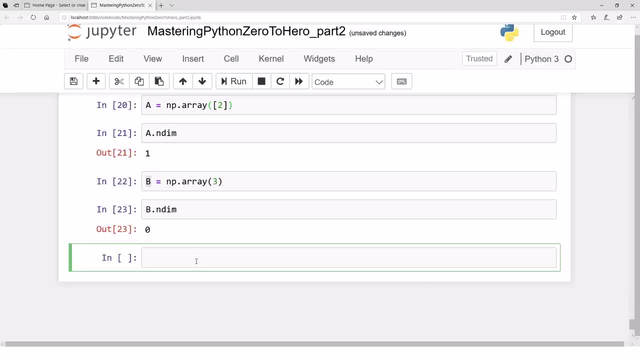 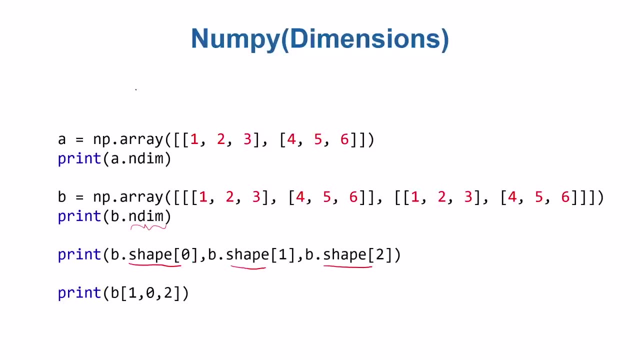 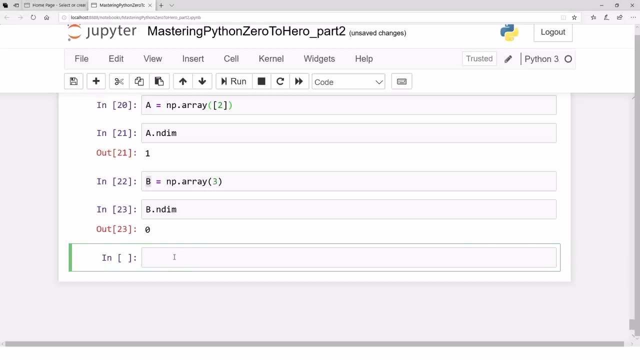 you get a 2d. If you concatenate a lot of 2d's, you get a 3d, and so on. Get a look and feel: Yeah, So that's what it is. So, yes, Okay. In this video I discussed the shape. There is another, there is there are so many properties. 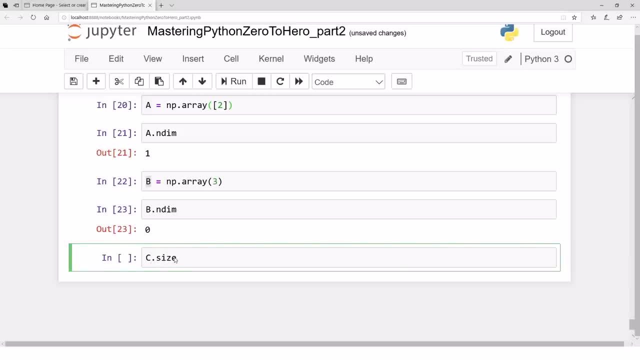 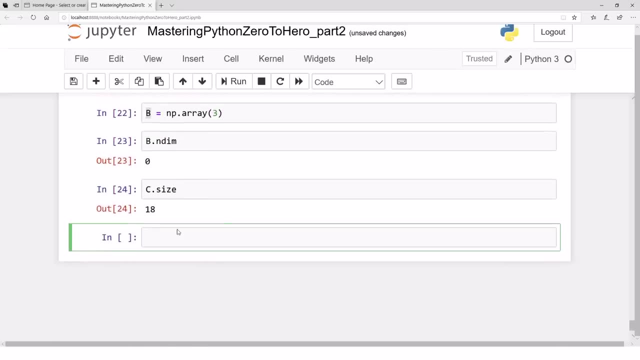 Let me, let me discuss some properties, Let's say size. That actually tells the total number of elements, complete total number of elements in the array. So how many elements are there? That is size. There is also, I guess, n bytes property that tells the how many total number. 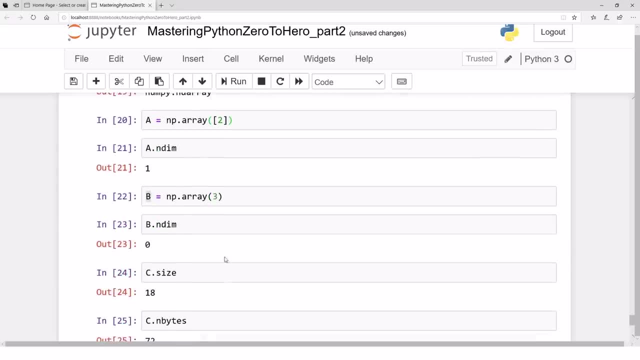 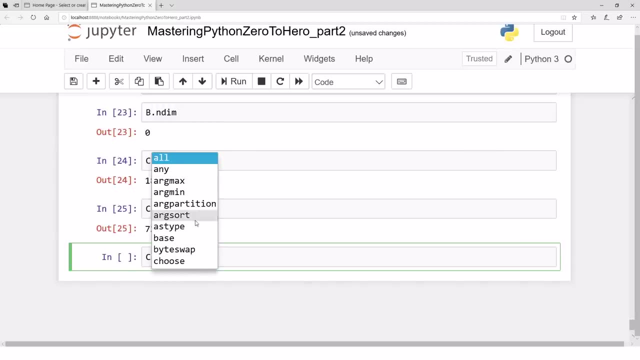 of bytes, that that this structure is taking inside the memory, And there are several other- I mean properties. If you just apply a tab and get certain things, you will see a lot of functions and you can- you can- check a lot of properties that some 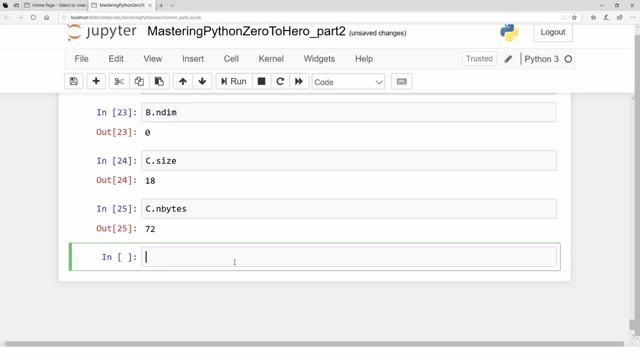 of these functions we will explore later on. Sometimes they are called the universal functions. We will see them because they are very, very fast. And these functions, the vectorized implementations of these functions. that is the reason why numpy is so, so fast. 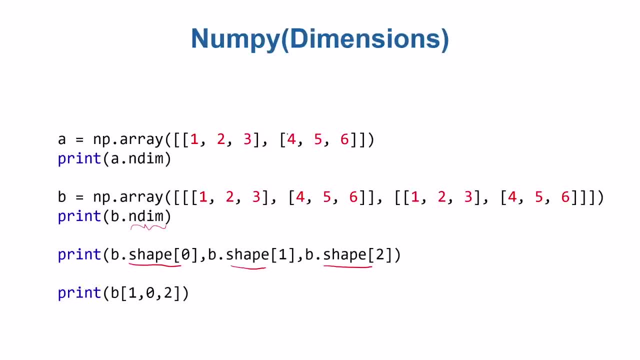 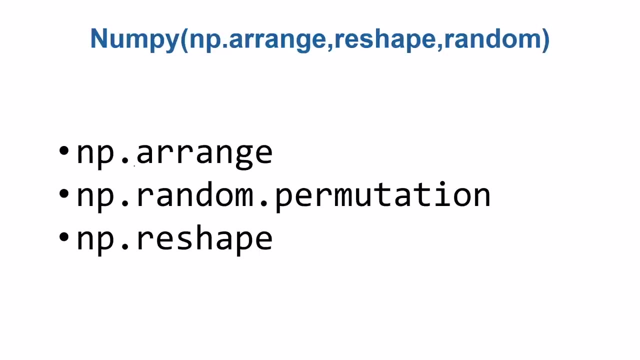 and why it is so popular, Anyways. Okay, So in the next video we will go to explore the numpy a bit more And we'll show you more fun stuff with numpy. So hope to see you in the next video. Numpy actually provides a lot of functions to create arrays, special kind of arrays. 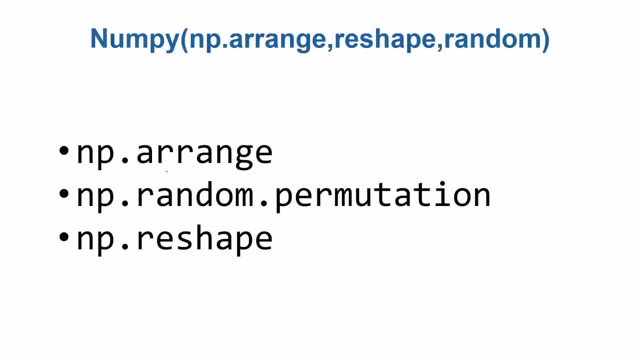 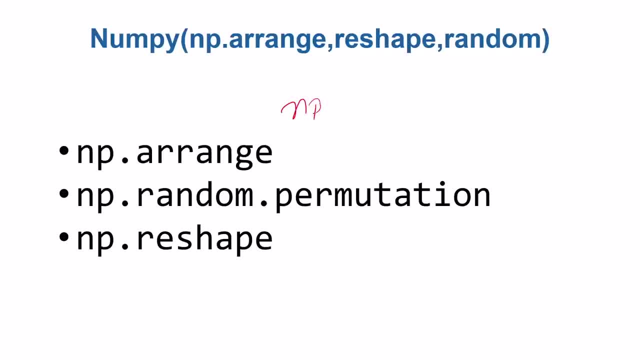 know, But you create blank, empty or, in the name of Lau, you will create an array containing all zeros. So there is a function in numpy, np dot zeros- that tells you how to do that. Similarly, if you want to generate a lot of, generate an array containing a lot of ones or all. 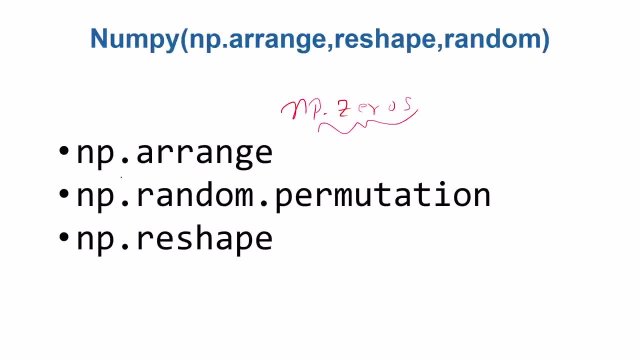 once there is a function to do that and and stuff like so. There are some functions that are actually used a lot and I want to discuss those. One function is np dot arrange. Actually this is a single R. This is noted to ours, This. 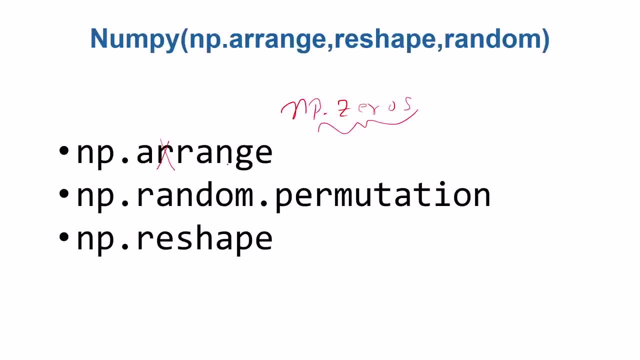 is singular: N P dot Arrange with one R and NP dot arrange function. what it does is it creates an array, for example, if you say NP dot arrange. it creates an array, for example, if you say, okay, hundred, so it creates an array that. it creates a 1d array that starts from: 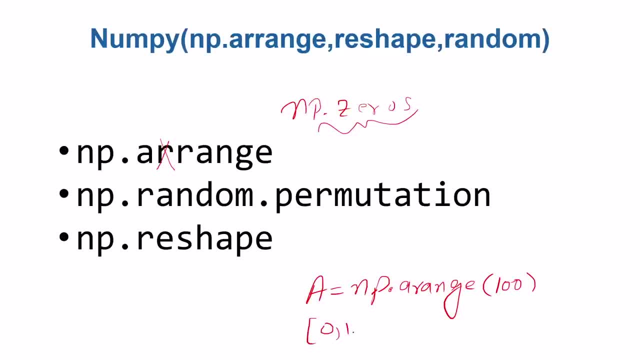 the. the values in that area starts from 0, 1, 2, all up to 99. so that's an array. that's a quick way to create an array with all the numbers till hundred. yeah, so let's see. let's see running example of this NP arrange method in Jupyter. 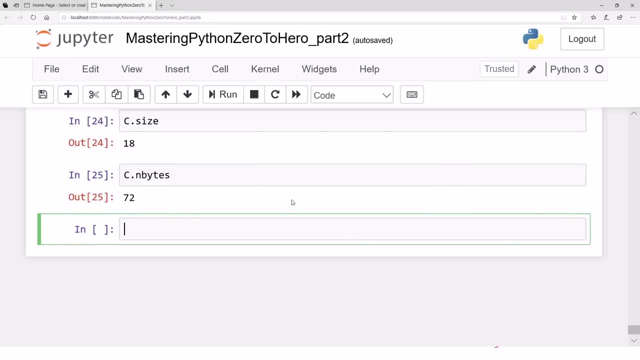 notebook, just to get a better look and feel of how it works. so let's see. so let's say we have a equals NP dot arrange and let's say hundred. so that's it. if you want to see what is inside a, you can see. this is an array with all the values, starting from. 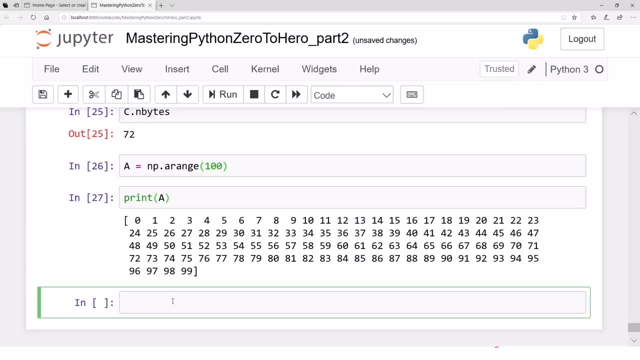 0 up to 99. maybe you want to, to create an array that starts from a particular number, ends at a particular number. maybe those two numbers are different and maybe this arrange function actually allows that. and let's say, I want to start with 20 and I want to end at hundred and I want to create all 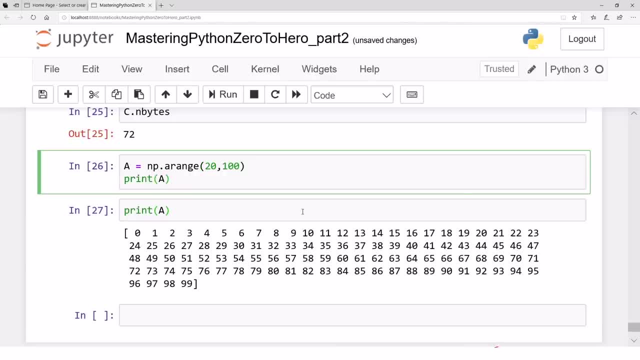 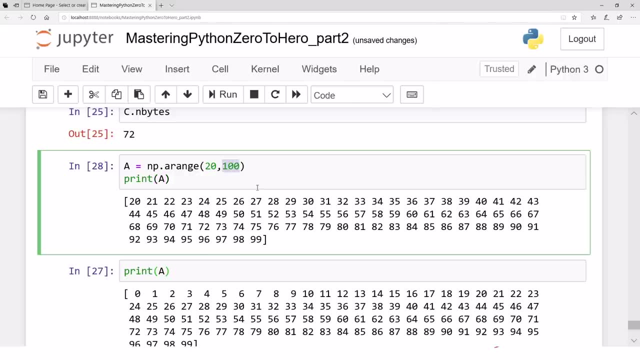 the array that does that. so let's say this: so that's okay, start from 20 and at hundred, but the last element, last index, is not included. that's possible. last but not the least, if you want, for example, to start from 20 and at hundred, and let's 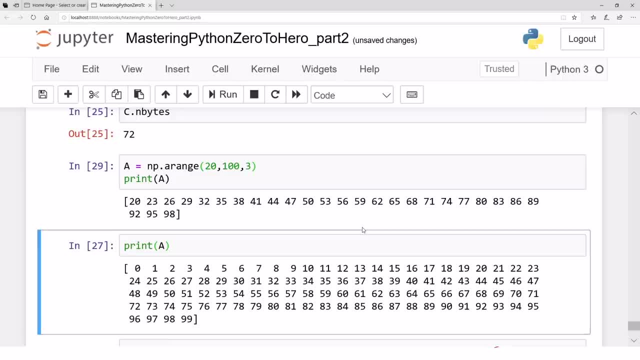 say you want to take a jump of three, that's possible, remember? does this? does this resemble with something that you know already? remember that. yeah, let me pause for a minute, not for a minute, just for some seconds. let me pause. do you remember this? arrange NP dot. arrange function. it looks like. 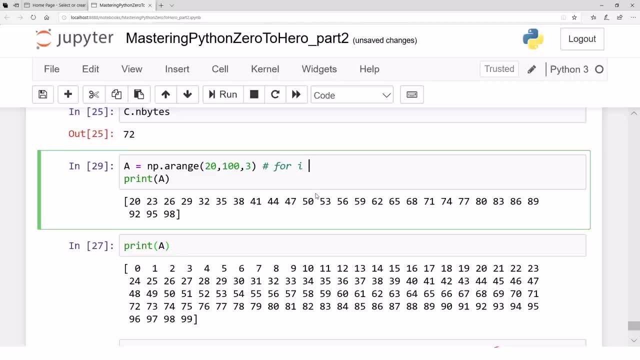 something like what? remember that, for I in range. yes, for I in range, for example, start from 20, go to hundred, take a jump of three. remember that. so it has some resemblance with the range function. yeah, although. So range is an iterator. What's an iterator? 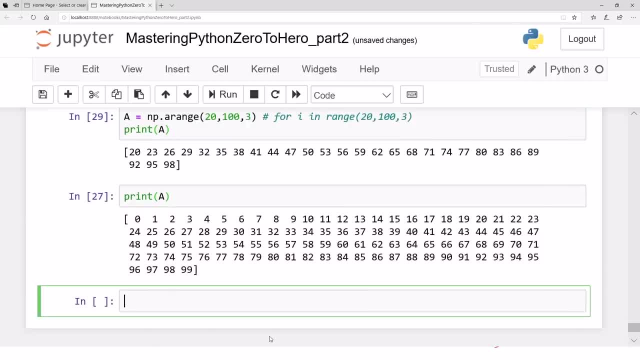 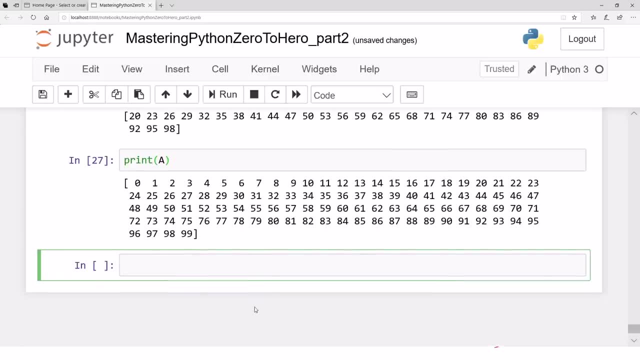 Why am I telling you that? Okay, let me tell you an iterator as well here. Just spend a few seconds on this range function. You might be thinking when we call this range- let's say range 10,, you might be thinking that it returns a list of numbers starting from 0 to 9, but that doesn't happen. 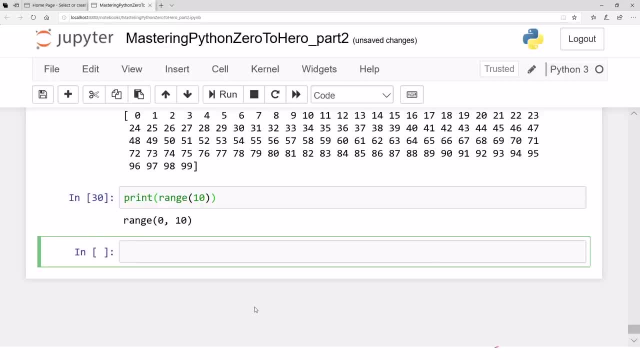 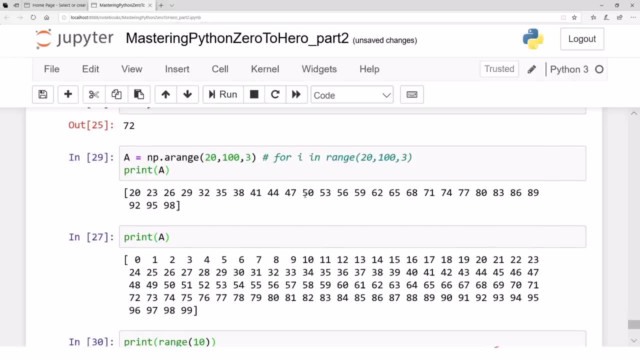 It returns nothing actually. When you actually call it, it returns just an object. When you call it in a for loop or somewhere, it progressively returns one by one element, one by one. So it returns an element, then it iterates and returns another element. 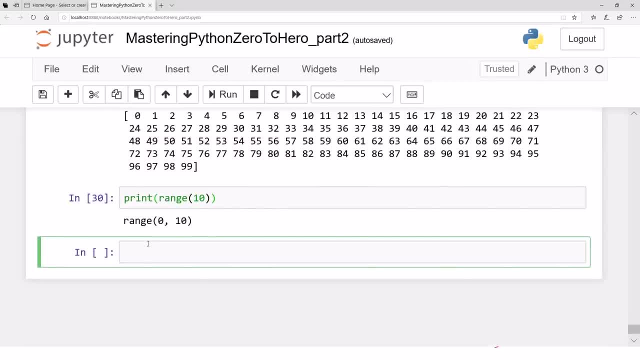 It never creates a list of elements. It never creates a list for you. That's awesome. Actually, it generates numbers. it generates the next number and the next number as you move on, So it saves a lot of memory. And these kind of objects- they are called iterators that iterate- they never create. 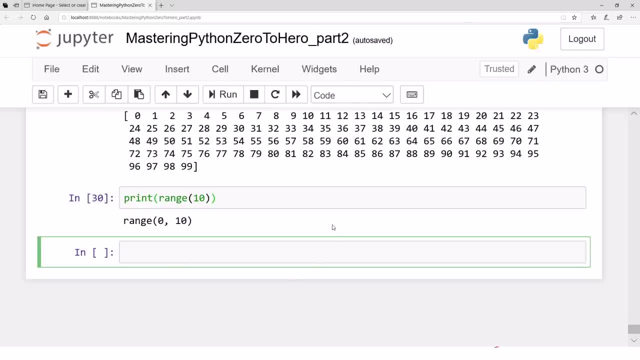 But if you want, for example, to get a list, if you really want to get a list, then what you can do is you can call it a range, let's say the same way- and you can just write a list. So provide me a list, don't just provide me an iterator and that will give you a list. 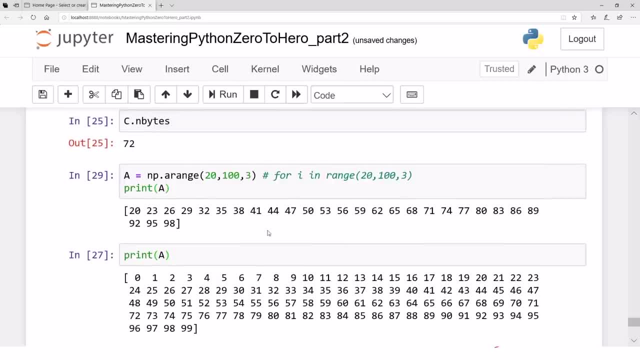 How cool is that? Great. Anyways, that was just a side note. It has nothing to do with this arrange function Anyways. so nparrange, it actually returns an array. It is not like an iterator. It returns an array, complete array, the way you want. 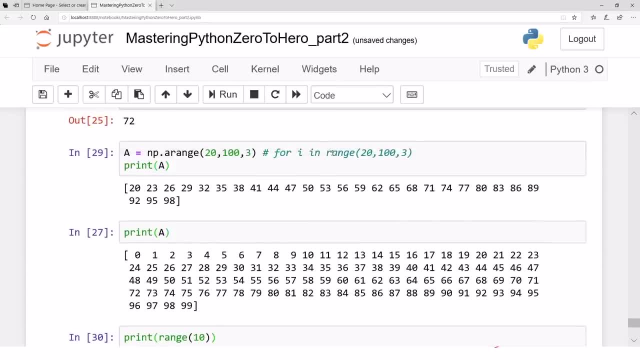 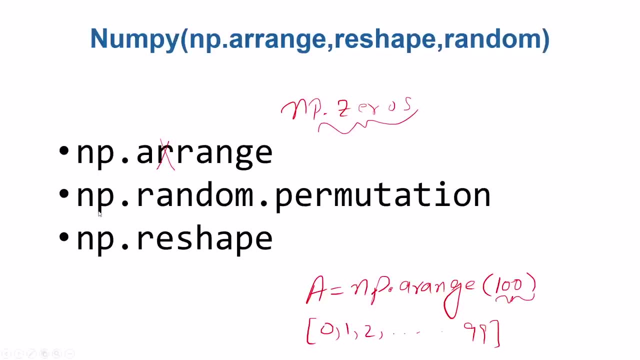 So that's what this arrange is. It has resemblance with this built-in range function that's mostly used in for loops. Okay, Next let's discuss this: nprandompermittation. nprandom is a package. np is a package. It has a lot of sub-packages. 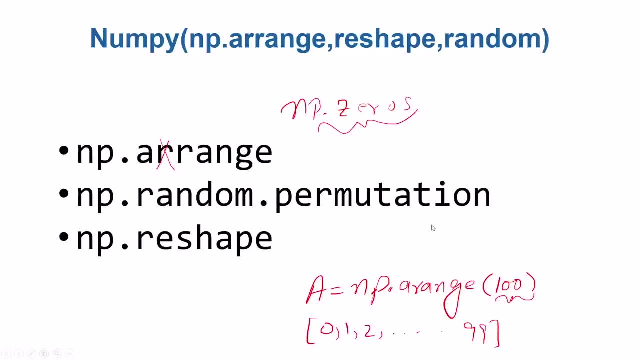 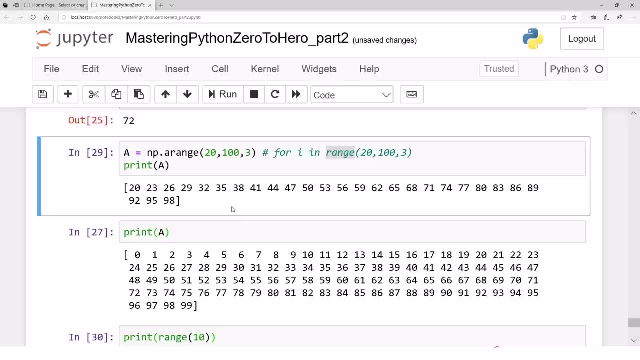 It has a lot of sub-packages. It has a lot of packages inside. Random is a package. Random has a lot of modules. One module is permutation. There are a lot of other modules. So let's see this random, Let's see what it does. 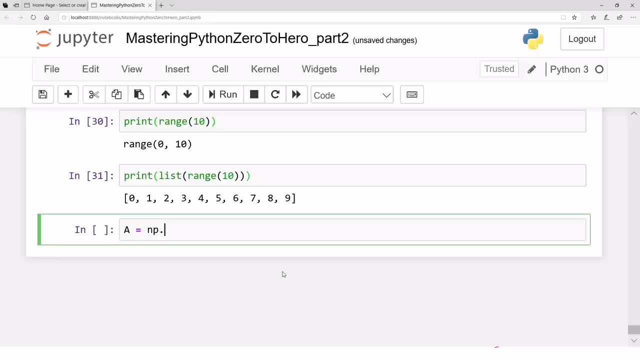 So, for example, let's say a equals nprandompermutation, let's say permutation, And what I do is I say, okay, nparrangepermittation. Okay, Let's see, Let's say 10.. What it does is this: nparrange will return an array containing all the values 0 to 9.. 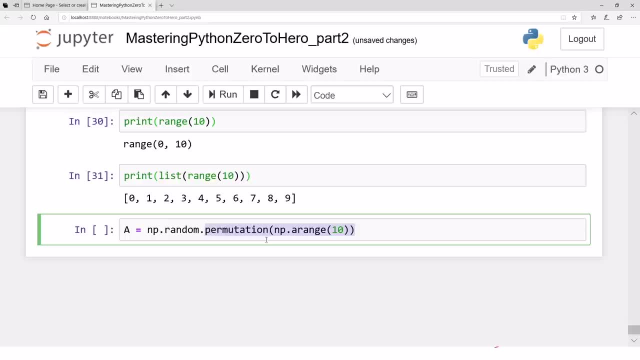 These are 10 values. And then this permutation function that resides in the package nprandom, that is, in the random package of np. it actually shuffles all the values and rearranges all the values in random fashion, And it will now be an array containing the same elements but in a different order. 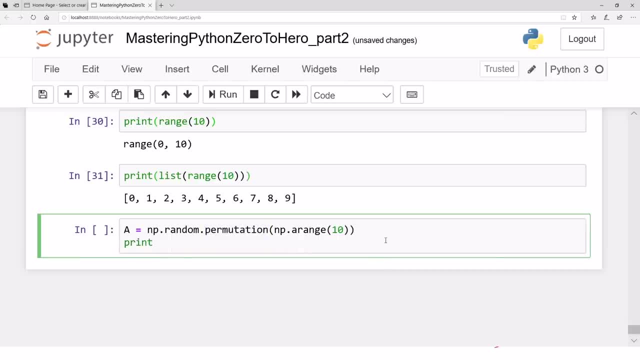 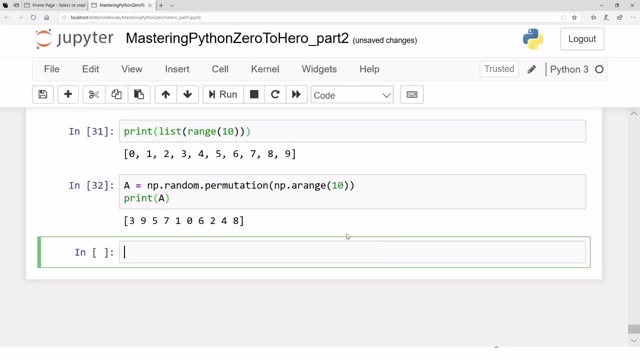 In a different random order. So let me now print this a. It will be having all the elements from 0 to 9, but in a really shuffled way, And that shuffling is completely random. Yeah, You see that Sometimes you may call some function. 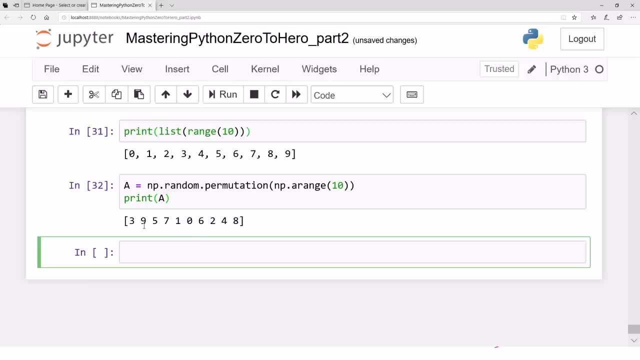 You may want to write some function on arrays And you may want arrays that do not have a particular ordering, that are just random arrays. Just to test your code, Just to test how it works on any kind of arrays. Okay, In that case, one way of getting a shuffled kind of array, one quick way, is to just use: 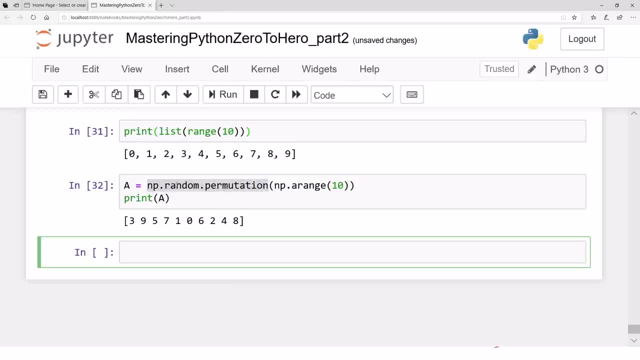 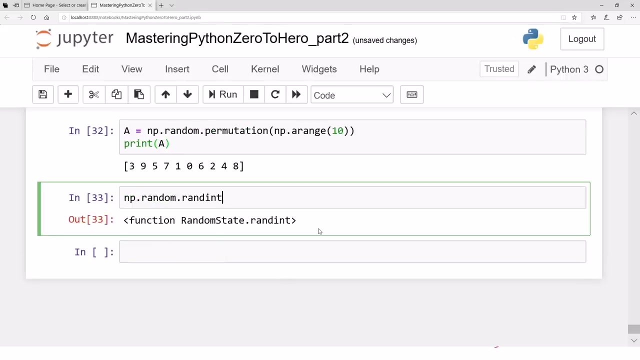 nprandompermutation function. The nprandom package does not only have this permutation. There are a lot of other functions- nprandom, For example, nprandomrandint, for example- that creates a random integer. That's, for example: If I that's, let me call this, and we have, how can it be used? 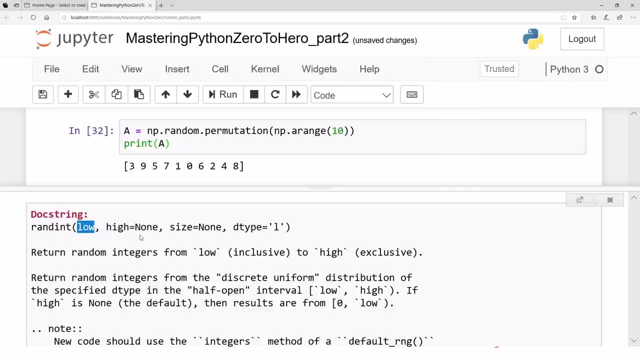 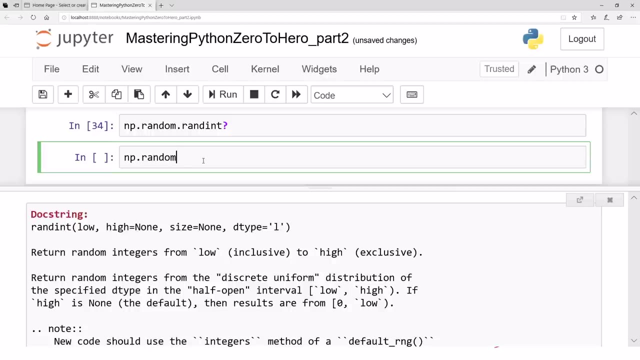 Okay, We can give a low value from where we start. We can give a high value, I mean, and it creates actually random integers starting from low, ending at high. So that's how it can be used. For example, let me call it as nprandomrandint. 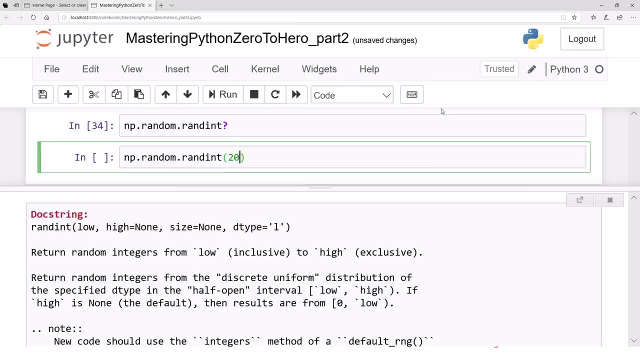 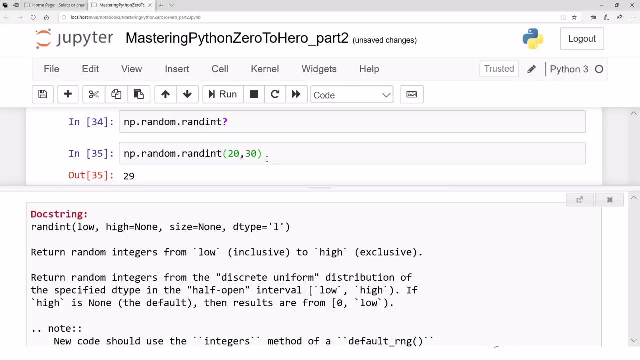 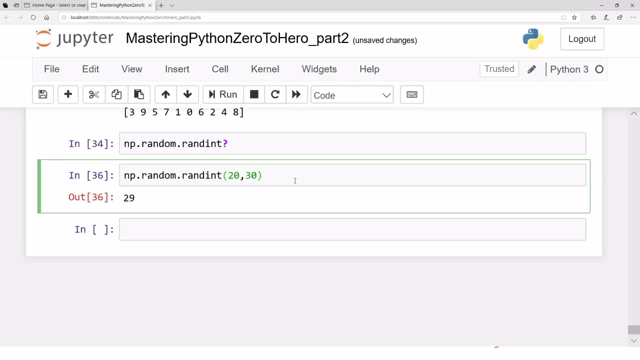 Create a random number Between 20 and 30. Create some random integer and it will return some random integer between 20 and 30. If you call it again, it may return some other. oh, it is, it is returning 30 again, 29 again. 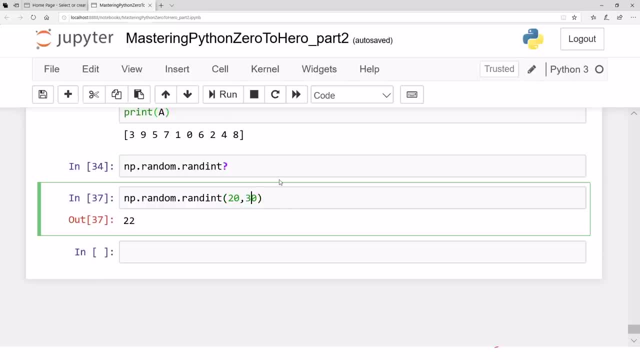 and again. Now it returns 29,, 22.. Maybe we want to, maybe we want to generate random integer between 20 and 30. So it creates a random integer, Okay, Okay, So we will be noticing what is the, what is the return value? 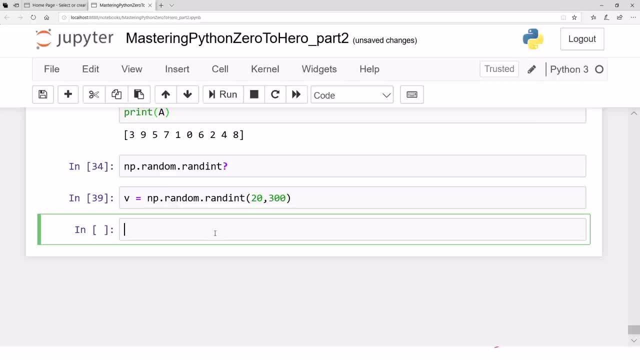 The return value is v, for example. What should be the type of v? What do you think Is this? v is an array. No, it is a number. It's an integer. The type of v should be an integer because it is returning a random integer. 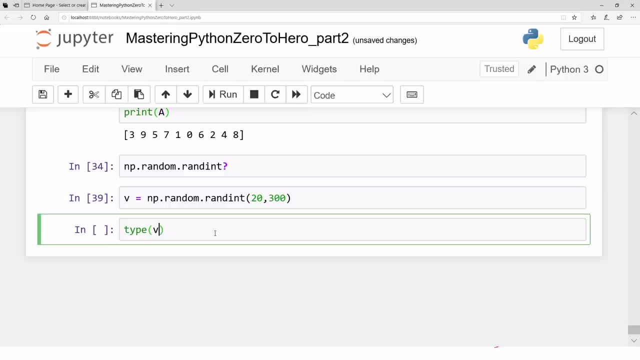 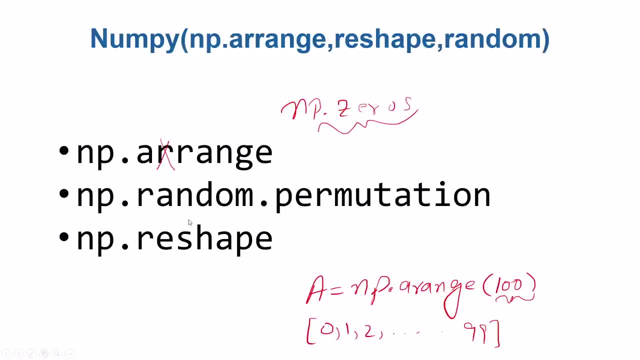 It is returning an integer, but it is selecting that integer randomly from 20 to 300.. So it should be integer And it is Yes, Wow, Yeah. So So we will be moving some more functions in the random package of NP. 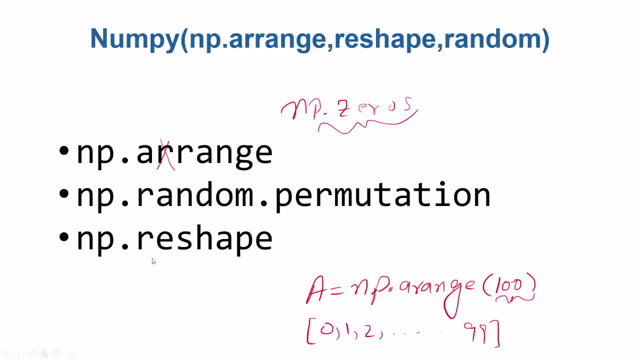 And then we will be moving towards this fascinating functions called function, called reshape. So there is more to come for NumPy. So hope to see you in the next video. Okay, In the last video we saw a range function. That's a very useful function to just create a test, testing array and just see, see output. 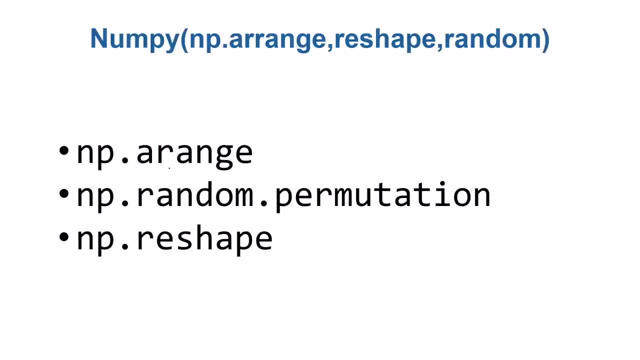 of a particular operation or algorithm. Just It's based on different kind of arrays. Further we saw permutation functions. permutation function in NP dot random package and we saw that this permutation function actually it reshuffles, It shuffles different kind of odd. 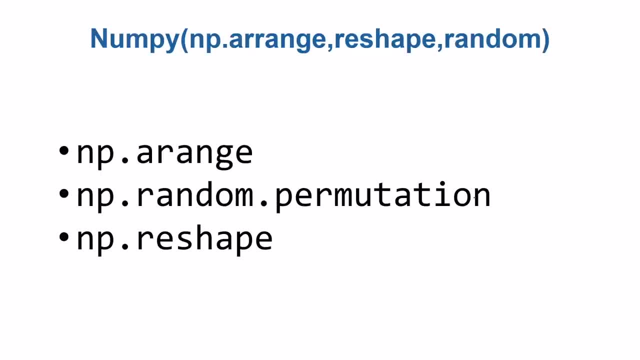 If array is applied to this permutation function, it actually shuffles all the all the elements of that array in a random way, In a completely random way, random way. today we will explore this random package a bit more and then we will see a reshape function. but that reshape does basically this reshape for. 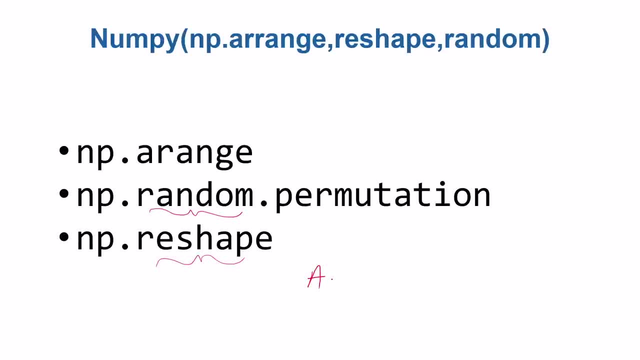 example, if you have an array, let's say array is, let's say we have an array with, let's say, 10 elements, and if we call a dot reshape and we give, let's say, 2 by 5, so it will make a two-dimensional array out of a, which is B, and that will be a. 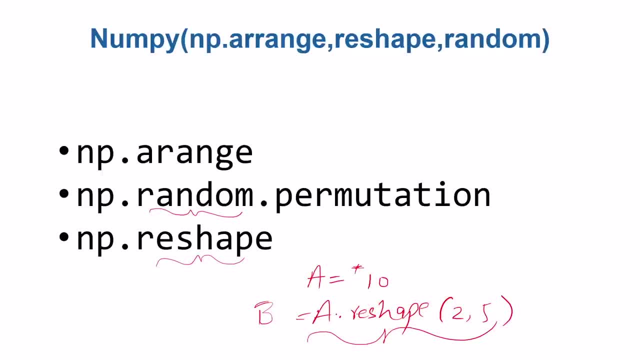 2 by 5 matrix, or that will be an array or a matrix with two rows and five columns. and- and now we can, we can just work with this B just like it's a two-dimensional array and we can just, we can just treat this B as a. 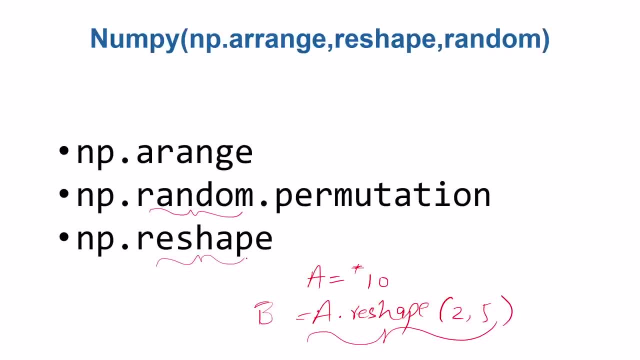 two-dimensional array and work with that it is. it becomes handy sometimes if, for example, we want to, we want to test certain operations on on matrices. a quick way to make a matrix is just to call it a range function and then, whatever the result is, just reshape. 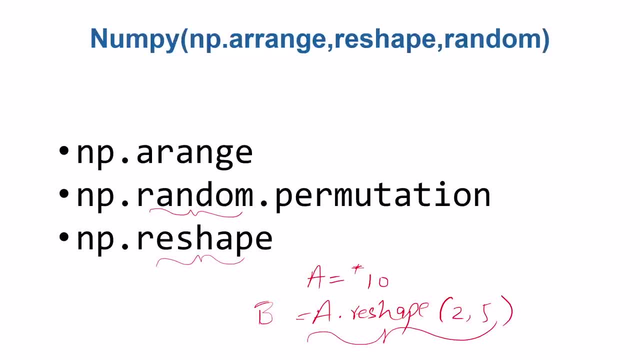 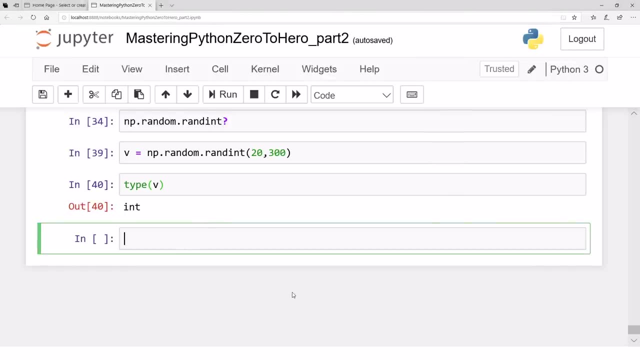 into the desired order matrix and test the algorithm. so let's go to the. let's go to Jupyter notebook and check this random package a bit more and then see the reshape function. so let's go to Jupyter notebook. yes, so there are a lot of ways to generate these random numbers. 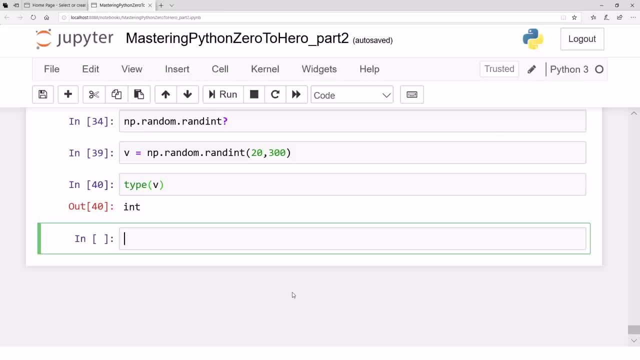 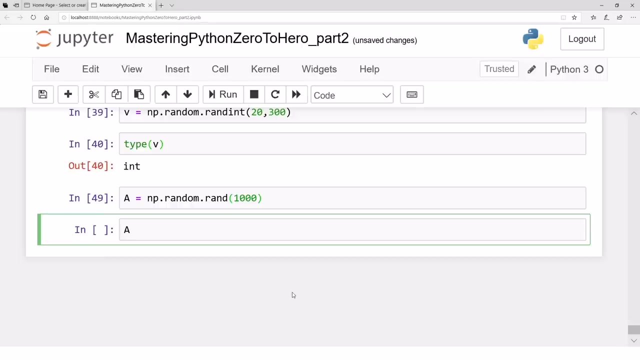 1, for example. we already have seen randint another way. for example, array and array a can be generated like NP, doc, random dot, rand function. so now, if we create this, if you create let's, if you pass, let's say, a thousand, a random value array will be generated, an A, and each value of A will be a random number. 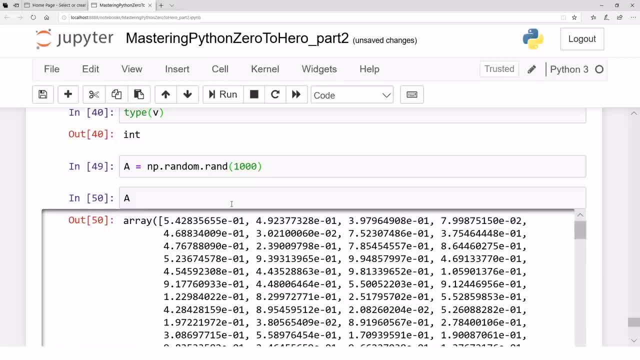 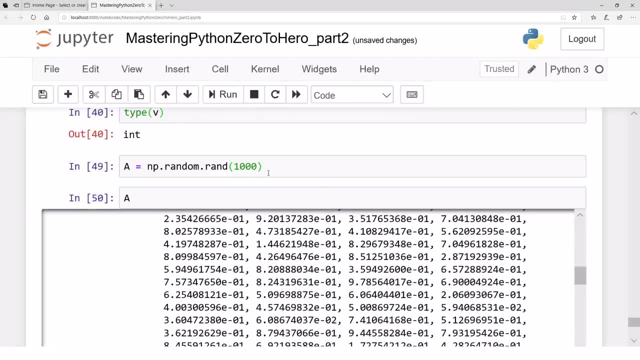 between between 0 & 1, so all these numbers are just random, between 0 and 1. each number is 0 and 1 random number and and this distribution basically is the distribution of this random number, is all the distribution is uniform. if, for example, we want to: 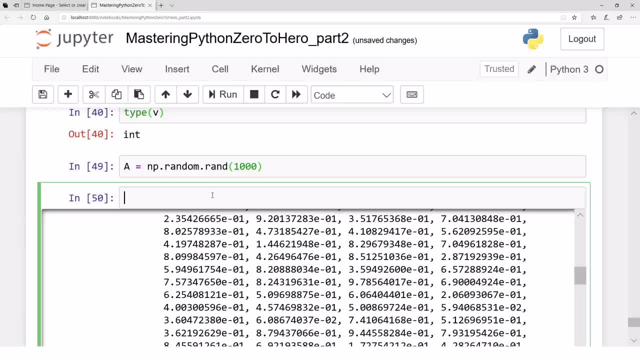 plot the histogram, the histogram or the, the distribution of a. it will look like uniform. let let me just give you give you one or two plots using matplotlib package- although we will see matplotlib package later on- but let's assume that this is just a plotting package. this is just 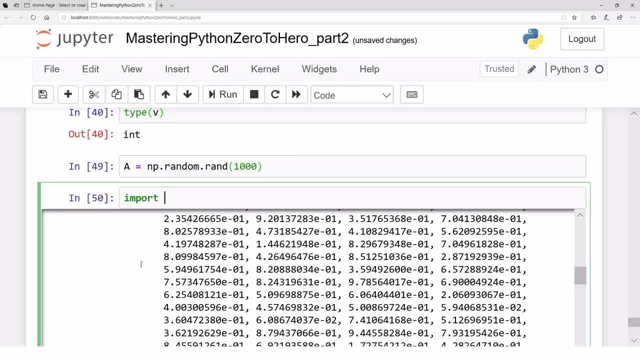 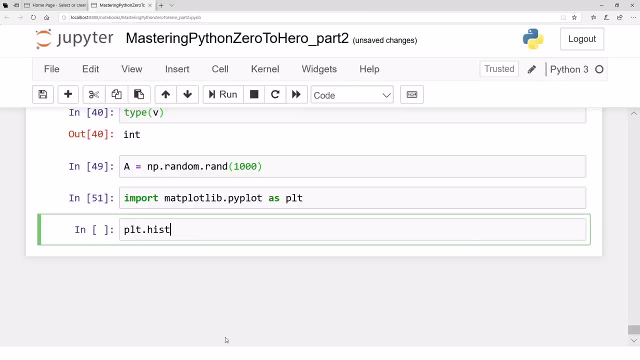 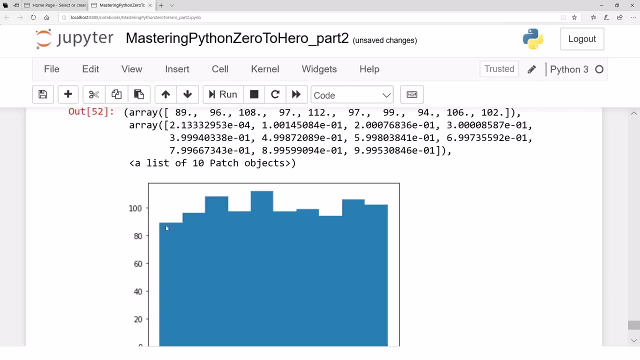 a package that helps us plotting. just import that, import matplotlibpyplot as plt, import that, and after importing that you just plot a histogram, plthist for example, and pass a and you can see the histogram is roughly uniform. i mean, everything is equally likely. we can make more bins, for example. we can 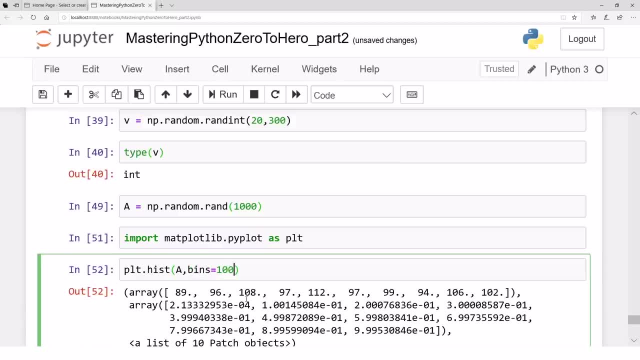 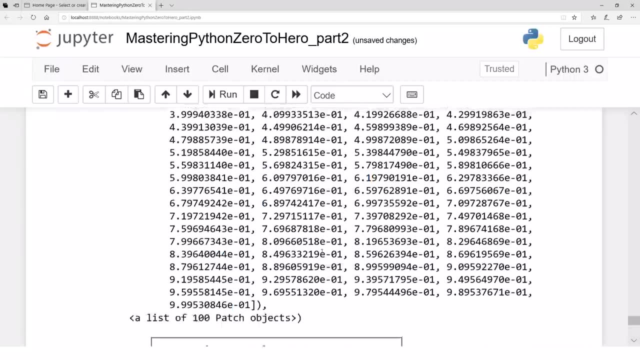 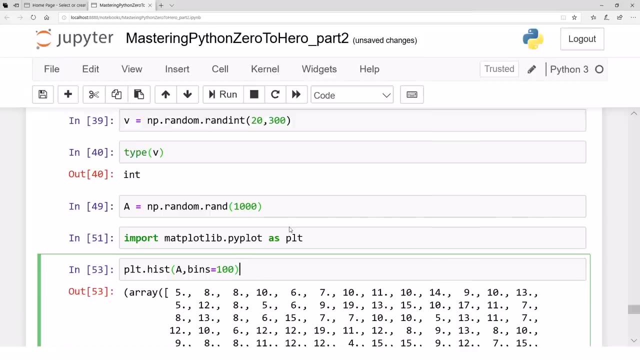 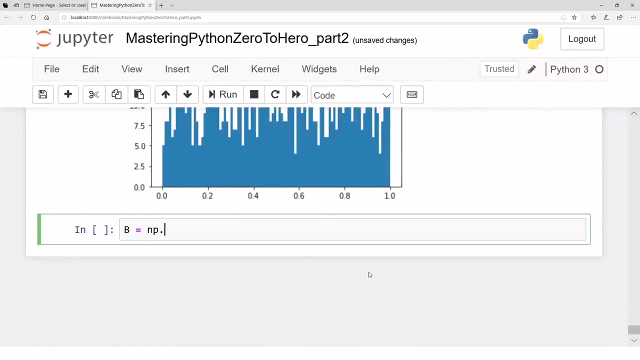 have bins equals, let's say 100, and we can see almost all the bins they are, i mean, just look like uniform. if we make more and more data set, then they will all look uniform. one more thing we can: we can have, for example, this: and let's say b equals np, dot, random dot, rand n, and that generates normal random numbers or gaussian. 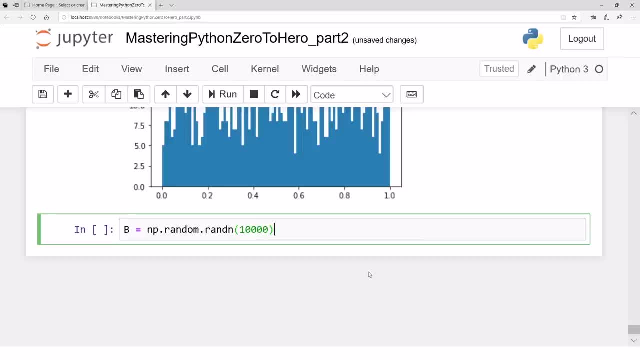 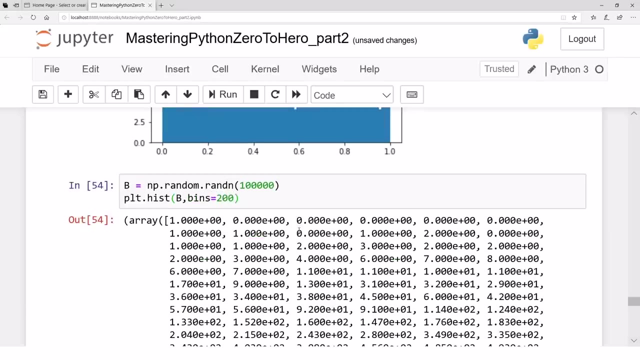 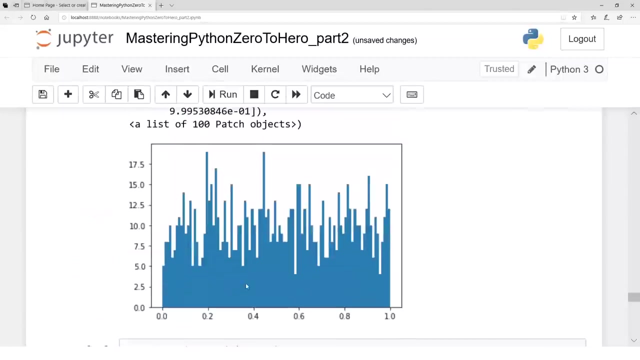 random numbers. let's say which which the distribution of the numbers are. is the bell shaped curve, for example. so let's just plt, dot, hist b and bins, let's say, equals to 200, and we can see a bell shaped curve, because the distribution of this data is: is gaussian distribution, looks like so. so, um, this, this random package is, uh, this np dot. 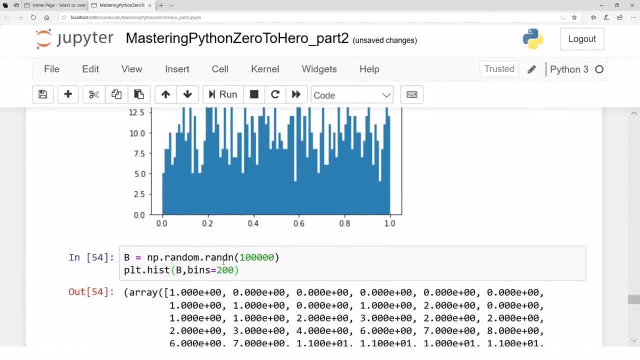 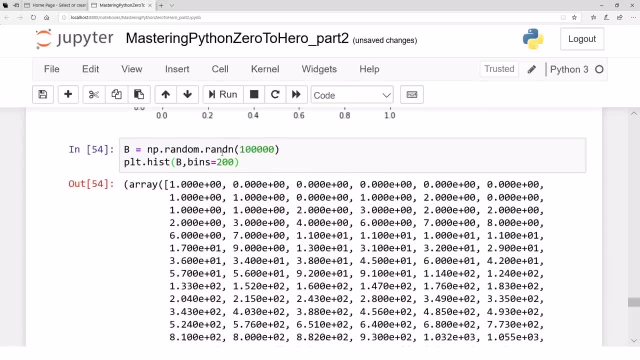 random is really important package. it has a different. it can create different kind of random numbers from following, from different distributions and doing in machine learning or in statistics. sometimes we need to generate these kind of random numbers, uh, for sometimes for testing purposes, sometimes for adding noise of a particular type, to test our model and stuff like so. 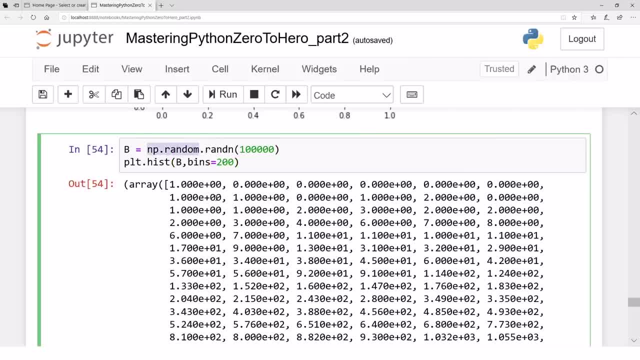 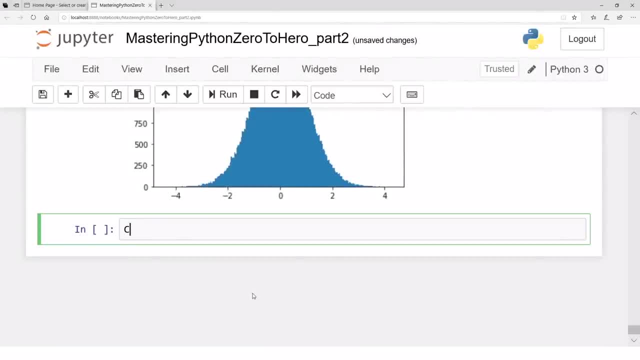 so it's good to have a good grip on np dot random package. okay, um, next we see reshape function. one more thing, for example, if you want to create, for example, a two-dimensional array of just random numbers, let's say you can call np, np dot, random dot, rand, and you can just call, you can just pass. 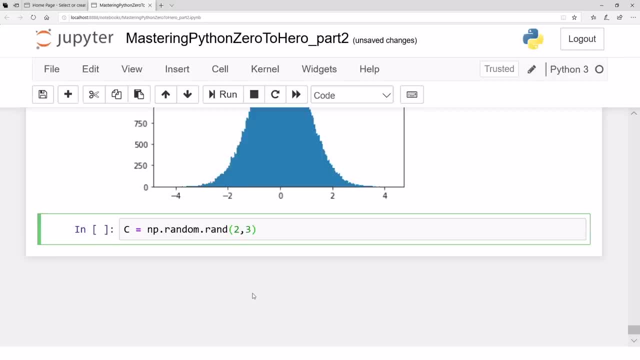 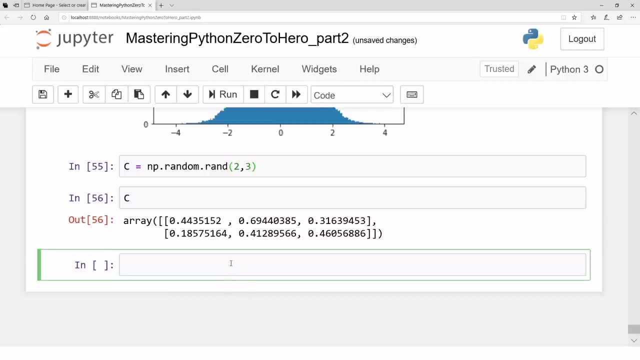 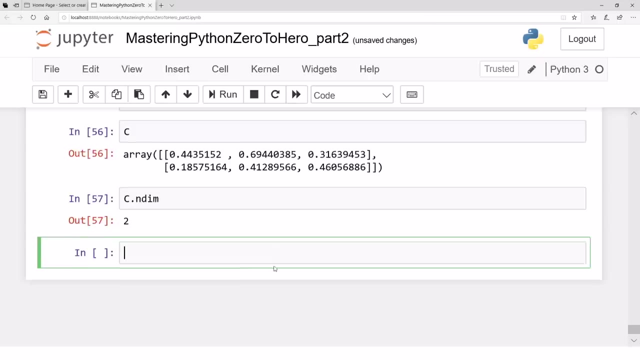 two arguments, for example, two by three, and this c will be a two by three matrix. uh, if you see the c, it will be a two by three matrix of all random values. if you see c, dot, n, dim, it will be having the dimensions of two and it's a two-dimensional array. further we can create for: 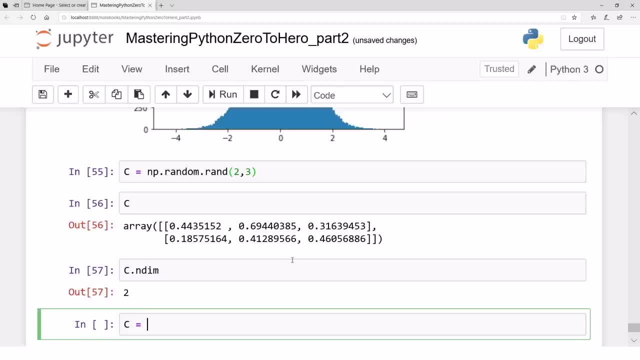 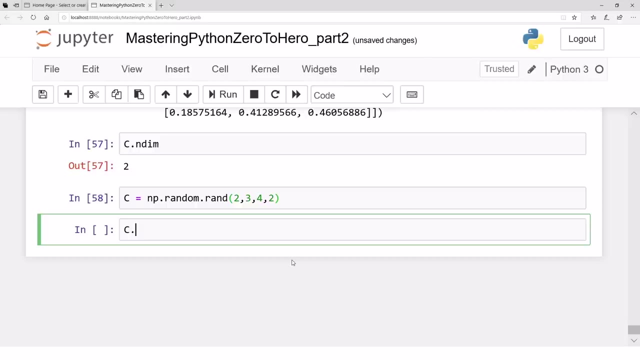 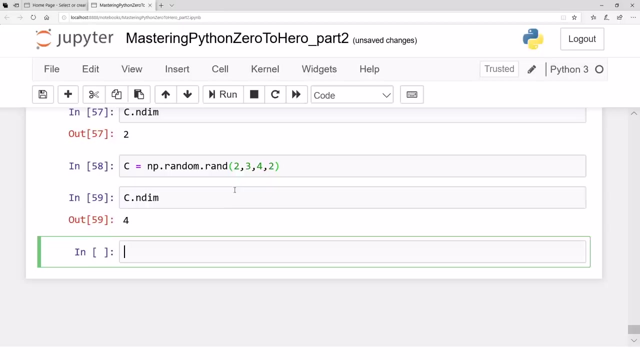 example, a four-dimensional array. c equals np, dot, random dot, rand, maybe two by three, by four by two, and that's a four-dimensional array with this particular order. if you see this, c, dot, n, dim, that will be um, that will be this um. yeah, so let me, let me just uh give. 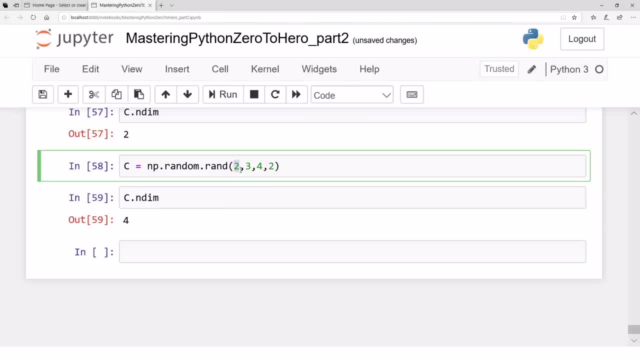 you an interpretation of what that thing is. there are two arrays that are three-dimensional and there are two of those. okay, now, each three-dimensional array has three two-dimensional arrays. wow, so each uh- two-dimensional array has four one-dimensional arrays, and each one-dimensional array has two elements in it. so that's what the structure is. um, yeah, get a good look and feel uh. 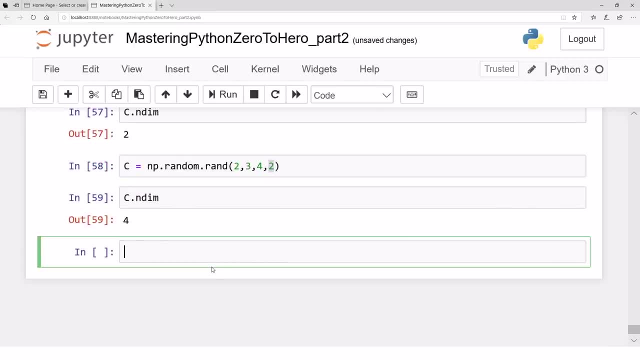 so let's see the reshape function, for example. let's say we have d equals np, dot, arrange. let's say we have a hundred values and then we say: reshape these hundred values to, let's say um, um, let's say four by twenty five, so this d will be a four by twenty. 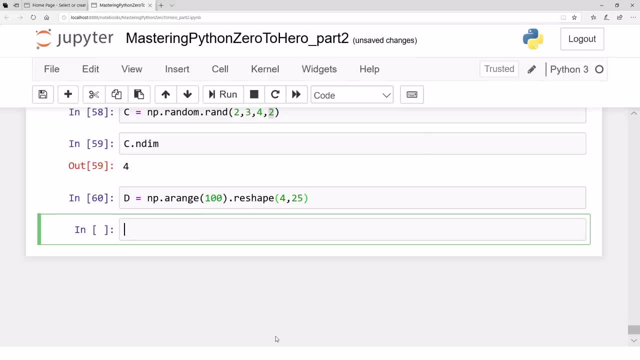 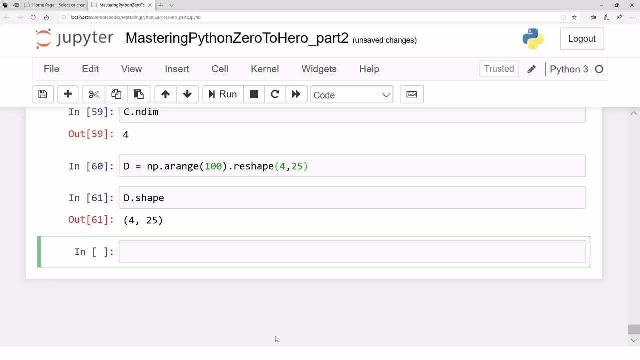 five Matrix. so if we just uh get the shape of d, so that will be a 4 by 25 Matrix, or a two-dimensional array with four rows and 25 columns. um yeah, so sometimes we want to work on matrices and we just we can just uh plug in these, arrange, function to generate a bunch of numbers, and then we can reshape. 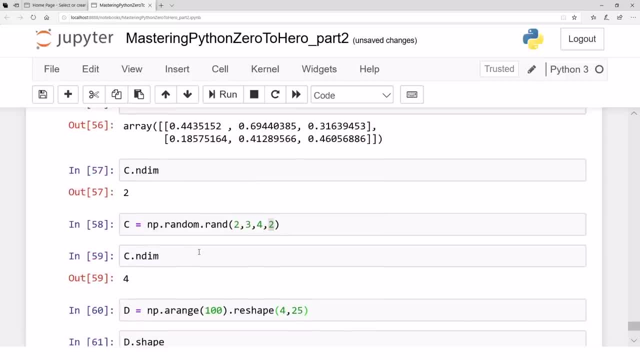 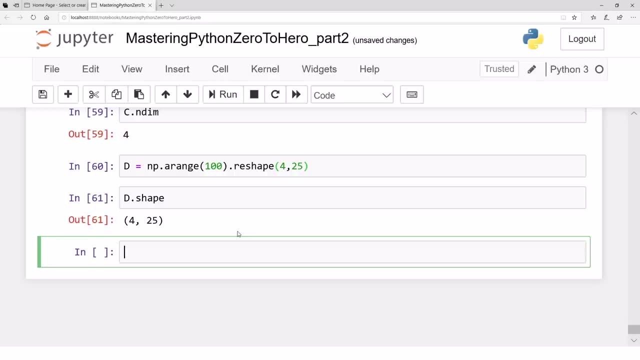 those and build a Matrix quickly and then just test the performance of our algorithm or or stuff like so, uh. so not only the reshape, not only returns the uh, uh, the. I mean you can. you can reshape a Matrix and you can reshape an array into more than two-dimensional array if you want to. for, 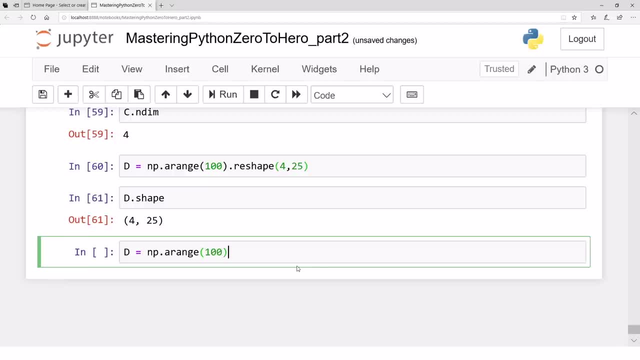 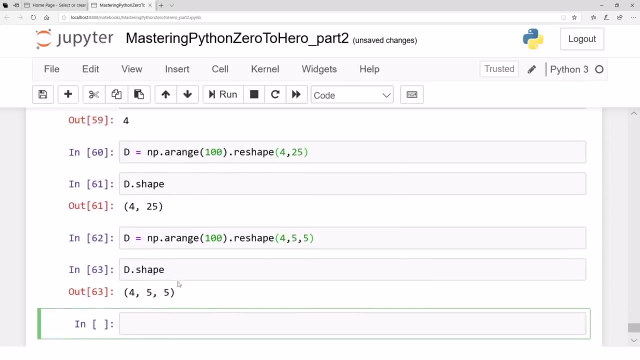 example, arrange hundred, let's say dot. reshape maybe, oh, as four by five, by five, it's a three-dimensional array. now this, uh, D will be a three-dimensional array containing different values. um, yeah, so now you can access it and and do whatever you want to do, so not only the reshape, arrange and permit a. 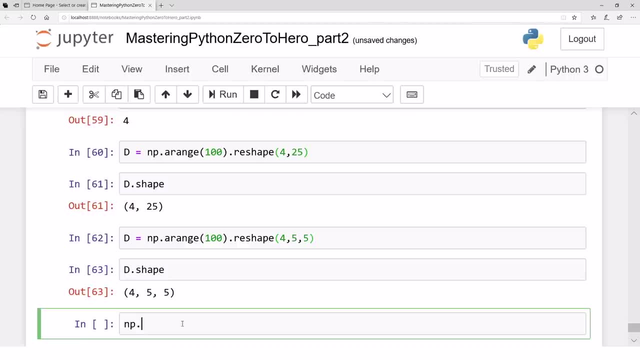 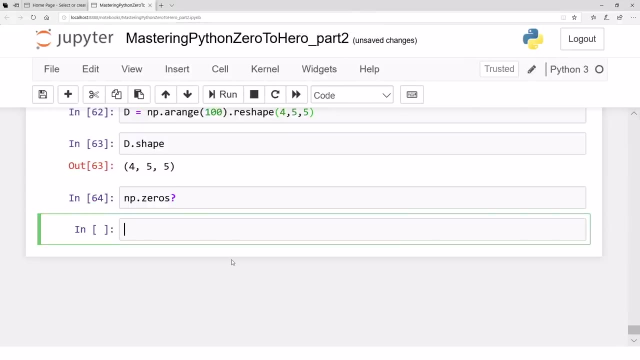 random. there are other functions as well: np, dot, zeros, for example. if you press Z and you just see the zeros and then you just press a question mark, you will know what that function is, how can we use it, and so on. similarly, you can have several other function. there is an important function once, for example. 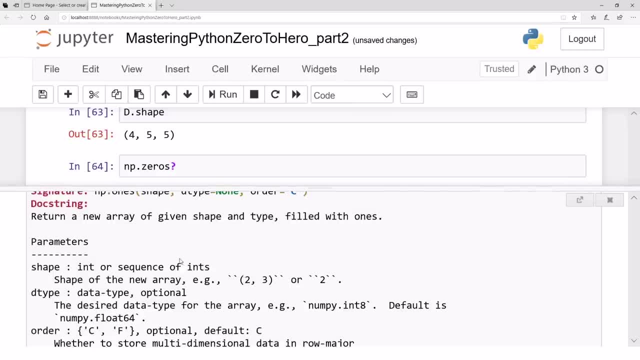 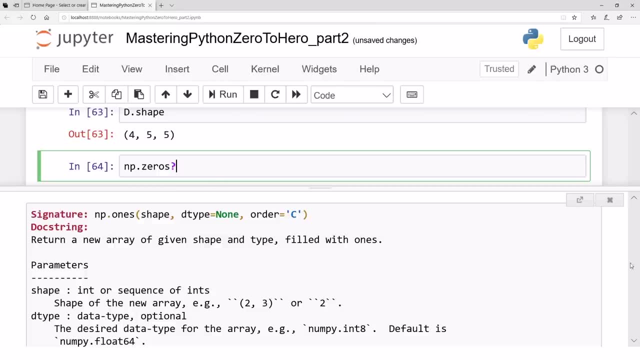 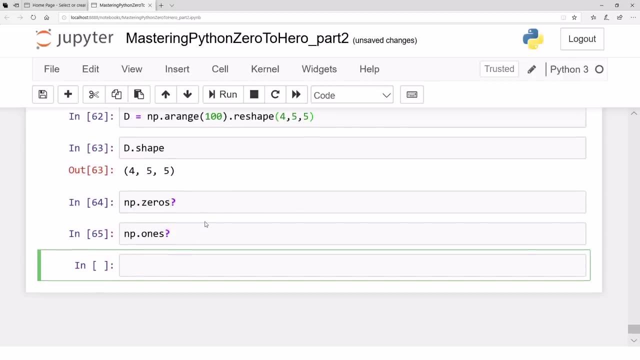 you can call that function and that will generate an array of all ones. you can see how to call that function here. uh, there is np dot empty. there is m np dot empty, like there are so many functions, just to create some matrices very quickly. uh, and you want to test your code or algorithms based on 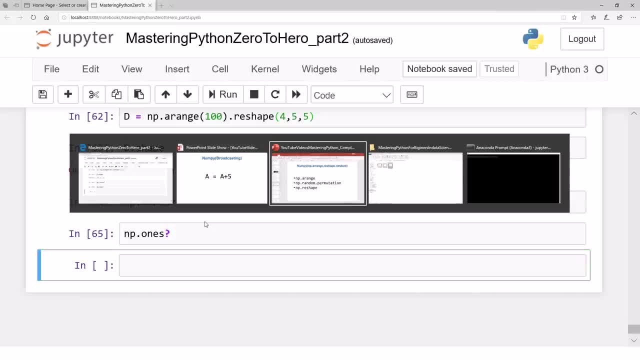 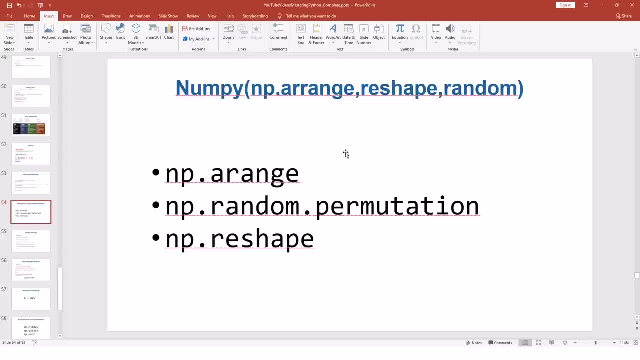 those. so, um, yeah, so there are a lot of functions that we want to that we can work on, so, um next. so so there are a lot of functions, uh, that can quickly create a NP array and an n dimensional array. um, we can quickly create an array. test our 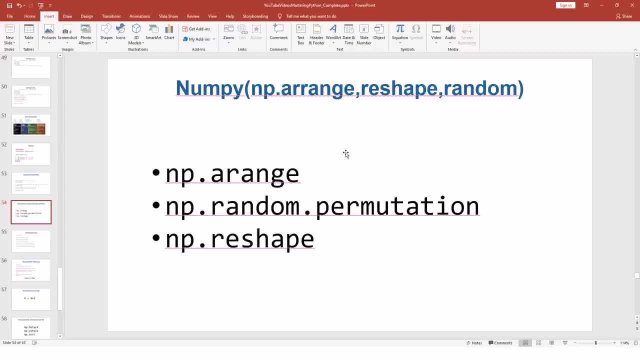 algorithm or use that array wherever we want to like, wherever we want to use, and we can move on um just a few functions like arrange ones zeros- they are there- or a random dot rand, random dot rand n and other functions. they are available. In the next video we will be seeing. we will be seeing. 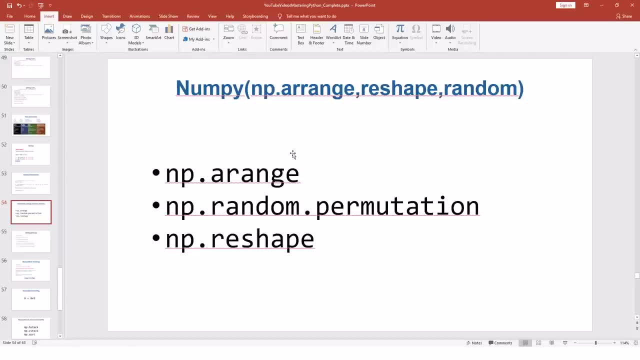 the indexing or slicing inside numpy array, and we will also be seeing the difference of that indexing with or slicing from the ordinary list or or or the ordinary data structures. what is the difference in? what is the difference of slicing in numpy with the, for example, with the? 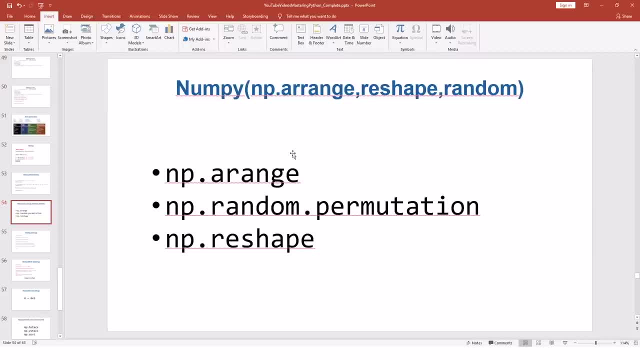 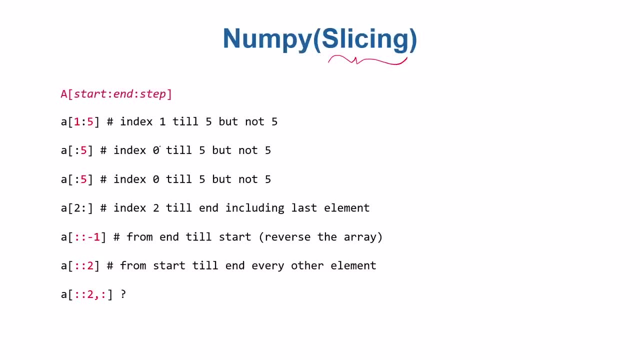 list. We will see that in the in the next video. Hope to see you in the next video. Okay, here is my favorite topic in numpy: slicing. Actually, indexing or slicing in numpy is the way you access sub arrays is just the same as the way you access sub strings or sub lists, and you already 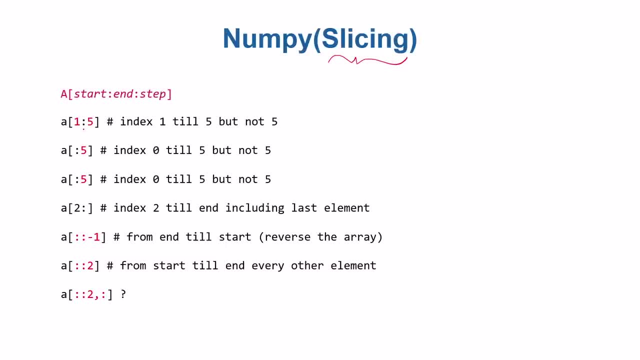 have seen how can we, how can we use this slicing or indexing. So let's see what we can do here. So let's see what we can do here. So let's see indexing in lists and in strings. The difference here in NumPy is in list, for example, if you 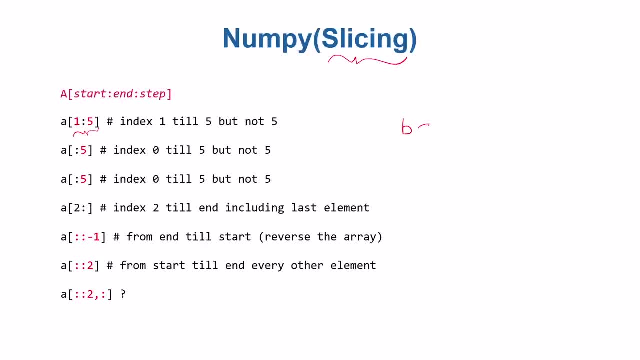 slice, you get, for example, let's say b equals a, 1 colon 5.. If you slice that thing from NumPy, then b is not a copy. It is actually accessing the same memory view as in a. Now, if you change, 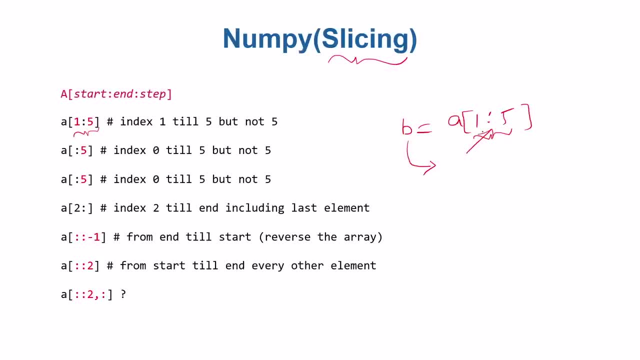 any element in b, the corresponding element in a will change as long as a is a NumPy array. However, if a is a list or any other data structure, ordinary data structure, then the slicing- this kind of slice- gives a copy rather than a view. So that's an important 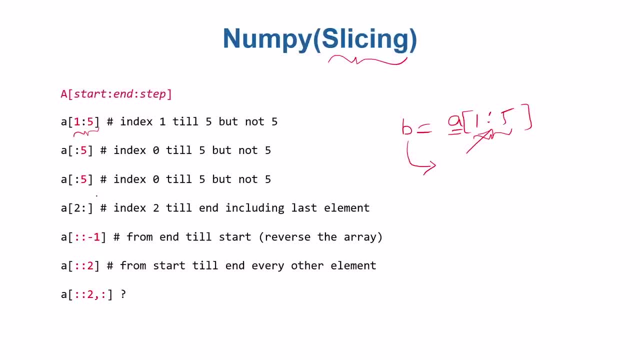 difference. We need to know that The rest of the indexing technique is almost the same. You do this kind of indexing. That is how you can reverse. This is start, end, start and end. So if you do this kind of indexing, that is how you can reverse. 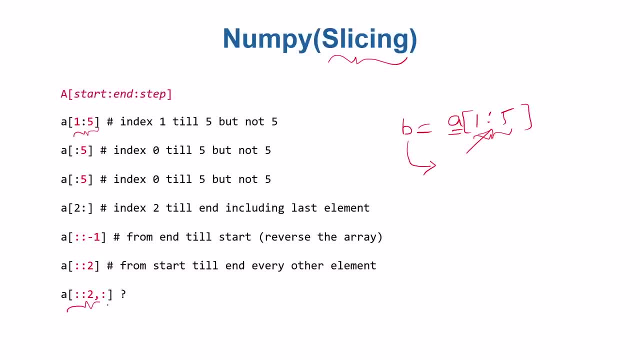 All the things are same, except how can we play with the two-dimensional arrays? Let's see some examples of indexing one by one in Jupyter Notebook and see how the slicing actually creates a view rather than a copy. So let's go to our Jupyter Notebook and see. 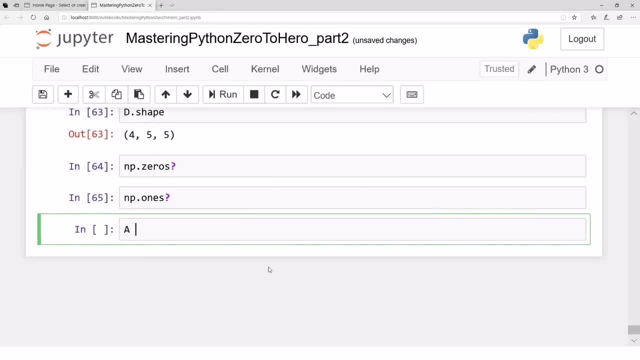 how can we play with different indices? Let's say a is nparrange, nparrange. Let's say 100.. And let's shuffle them. Let's stay as it is. Let's say: that's a, Now a. let's say: let's print some certain things. Let's say b equals a. Pick all the. 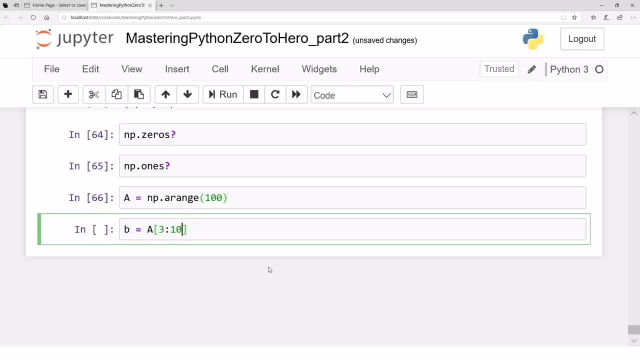 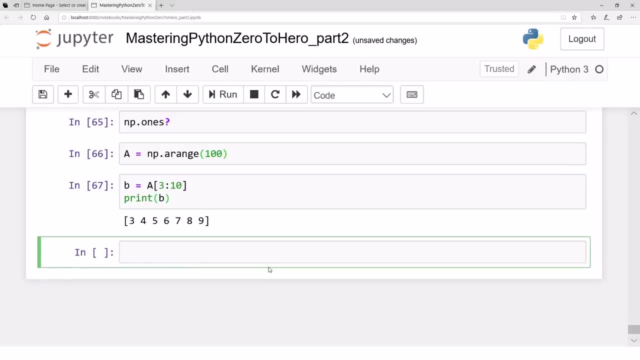 elements, starting from index 3, ending at index 9.. So 10 is not included. That's b. Let's print b. Let's see what's b. So b is 10 is going to be 10.. So 10 is not included. That's b. Let's print b. 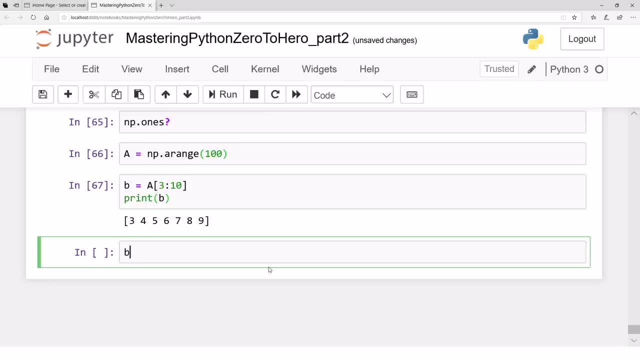 this array. okay, now what I'm going to do is I'm changing the contents of b. this numpy array is mutable. you can change the elements inside, no problem. so I'm going to change the elements. let's say one element in b. let's say I'm going to change element number zero in b, which is three. 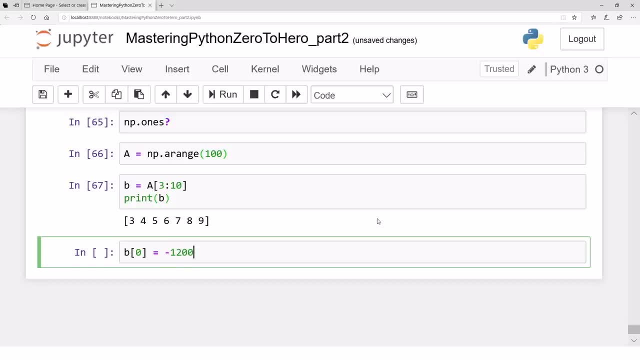 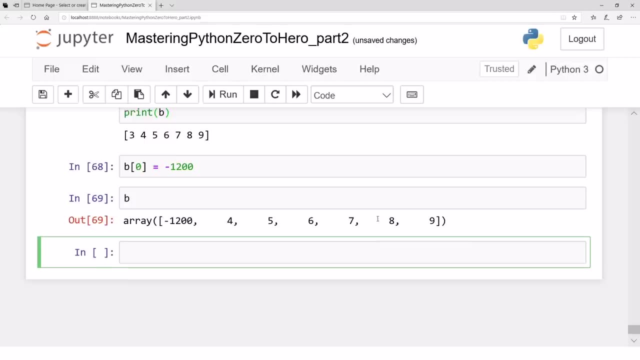 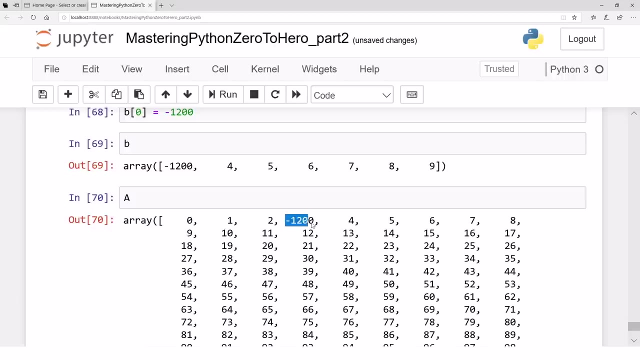 and I'm just placing that element as minus hundred minus twelve hundred. let's say that's the case. okay, now the contents of p has been changed. yeah, but now let's see the contents of a. the contents of a also has changed. that's a big difference between slicing an ordinary list on ordinary data. 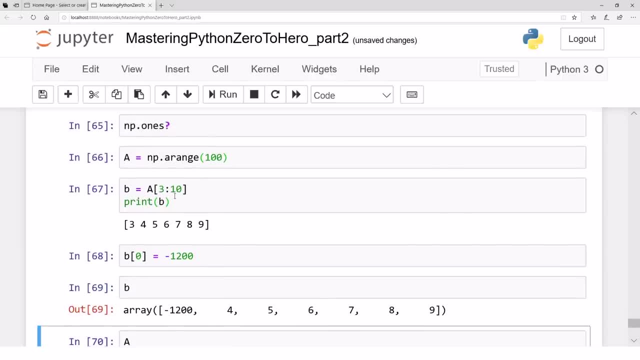 structure or slicing a list. when you slice a list, you get us, you get another label, but that label or that variable is accessing the same memory. the memory is accessing the same memory. the memory is accessing the same memory. the memory actually is not copied. There is one memory view and these two different names. whether you 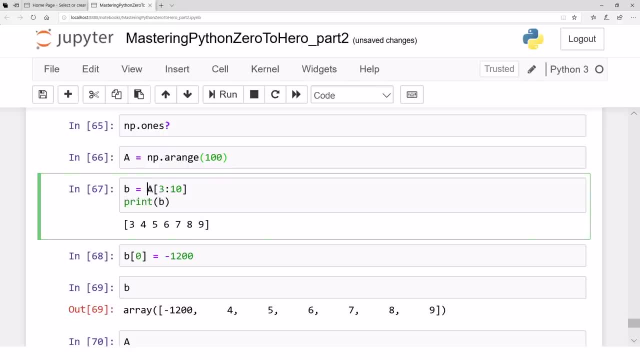 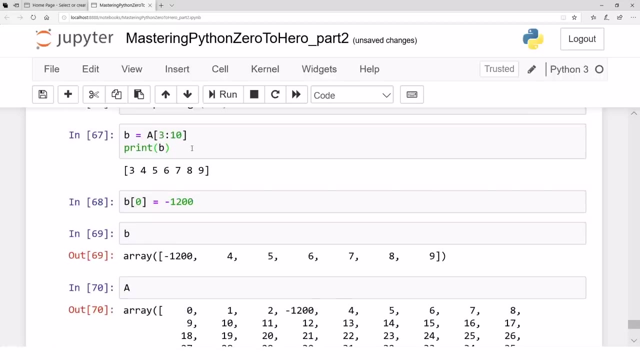 access those elements using b or you access those elements using a, the same memory is being accessed. if you change the memory using b or a, you will see the effect in both of the variables. So that's one difference. Now, after having knowledge of this difference, if you really want this behavior to not, 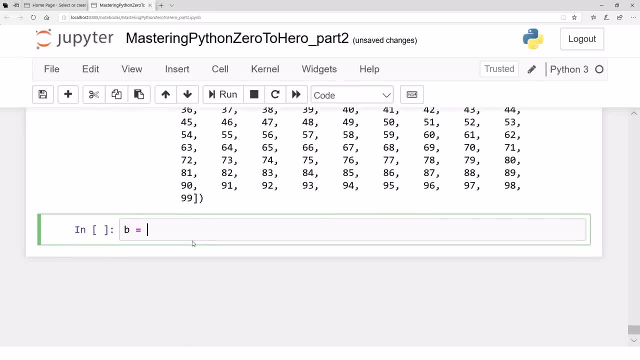 happen. one thing that we can call is: we can say: okay, a, for example a, let's say three, two, ten, and then we can call our famous function, remember that: copy. you can copy that. and now b is completely a different array, it's has, it's a different memory view. if you change b now the, the effect will not. 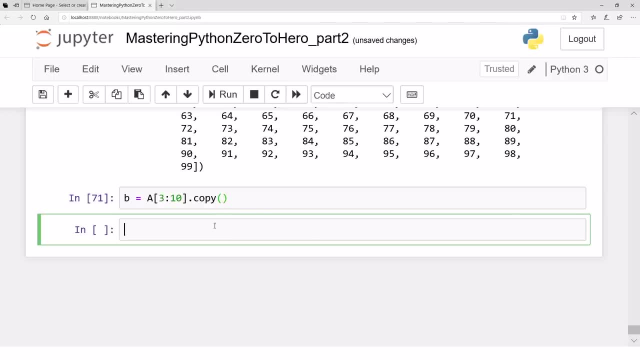 be seen in a So copy function is there whenever you need copy. One thing: if you are not going to change elements, the numpy is applies. So, if you are not going to change elements, the numpy will give you very fast implementation of slicing by not changing the memory view if, if you are aware, your algorithm is not going to change. 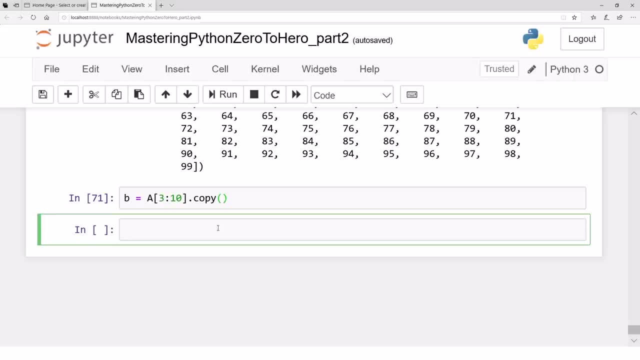 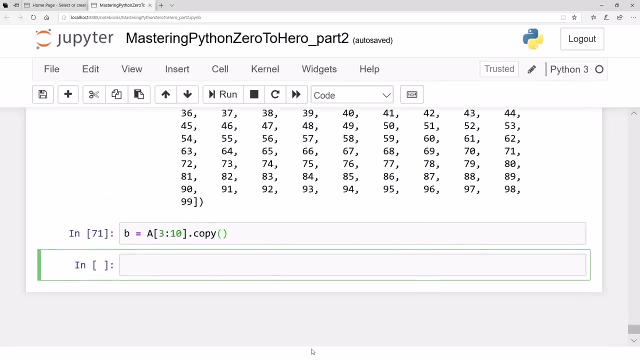 the elements. slicing will give you much, much efficient access to the elements or the or the sub blocks or sub arrays, without actually making the copies inside the memory, which can take time and space both. So this is one plus of numpy over the, over the other data structure that we have seen. so 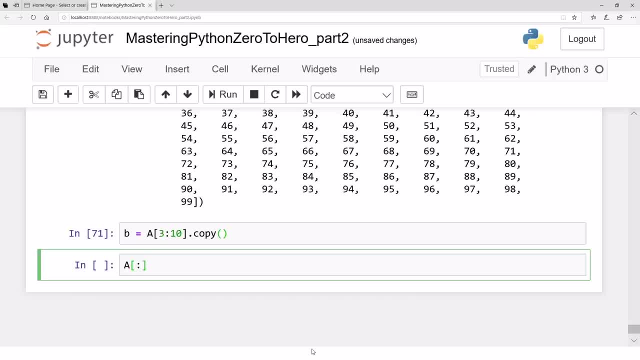 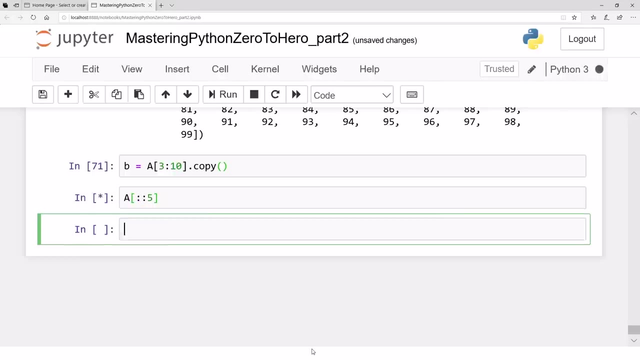 let's say, let's say what do you think? what is that thing? colon colon, two, what? or colon colon? let's say five. what it will do, it will start from the very first index, which is zero. it will go to the last index, but it will pick every fifth element. so let's see. so it picks 0, then 5, then 10, then 15. 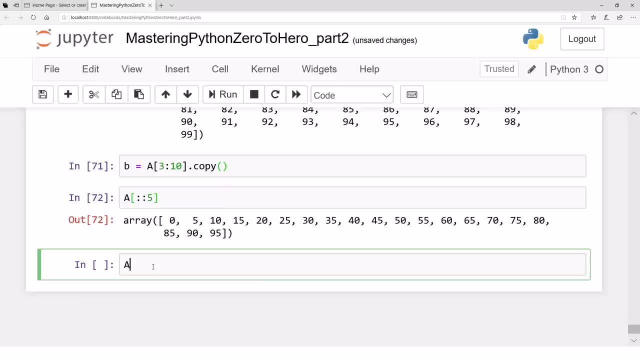 because the jump is 5. great, what do you think what this will do? let me just, let me just teach you by example what this will do. Yeah, what it will do. remember, if you apply a minus here, the end and the start and end, they just get. 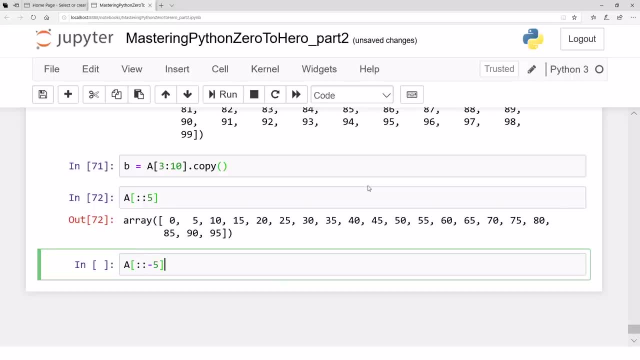 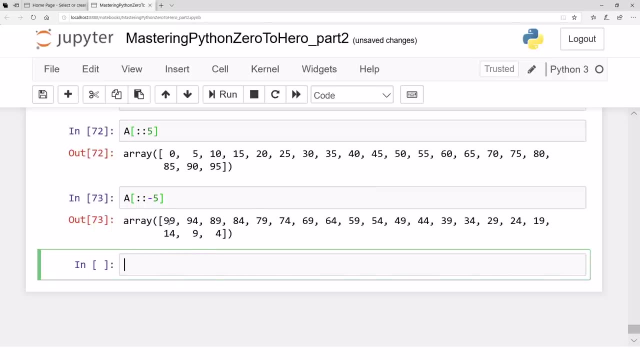 swept and this becomes a step from from the end. so what will happen is the same kind of impact. you start from the very end, then you take the step of minus one from the end and you just paste every element. so this is kind of reversing the array with one element. 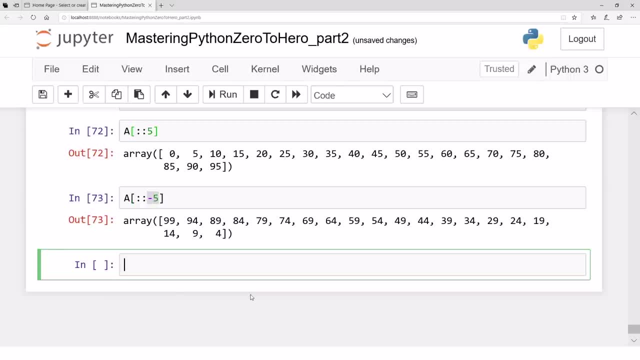 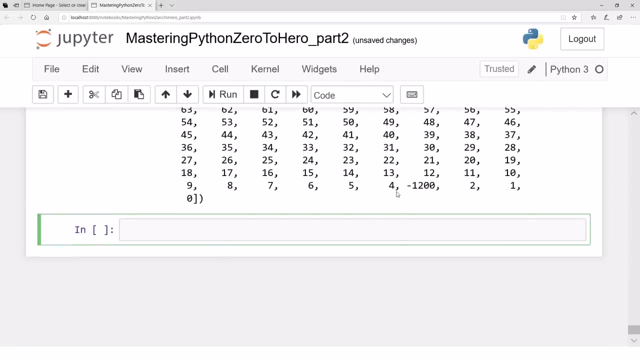 With kind of steps starting at the end rate. so another way of reversing the array is, if you want to reverse the array as a whole, just supply minus one, which means start from the end and pick every element from the end till the beginning, and the, and the array will be reversed. 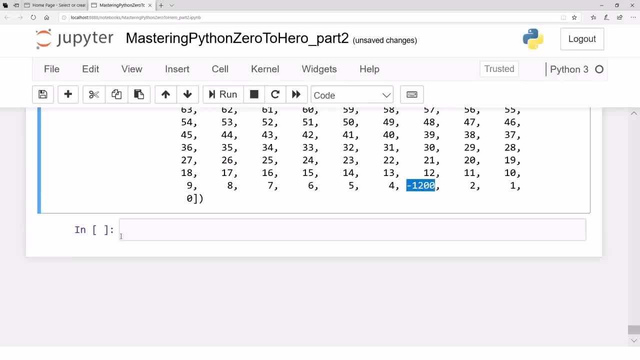 This element is there. remember that. this is there. Let's change that element. Let's change that element. So So a At position. So I want to find out the index where this minus 1200 is located. so IDX is equal to a dot index. I guess there is a function index, yes, yes or no index? oh, there is no index. there is there an MP dot index? MP dot index. I want to find out the index where. 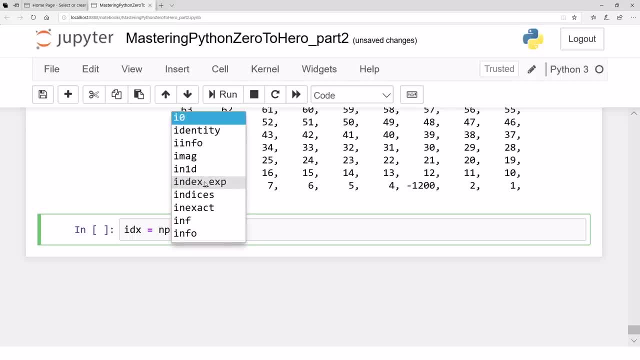 So index: There is no index function, indices or something. I want an index function. is there any index function? I want to find out the index where minus 200 is located. there are several ways, but I want to find one. so, for example, For example, let me see whether there is an index function or not, available in NumPy or not. 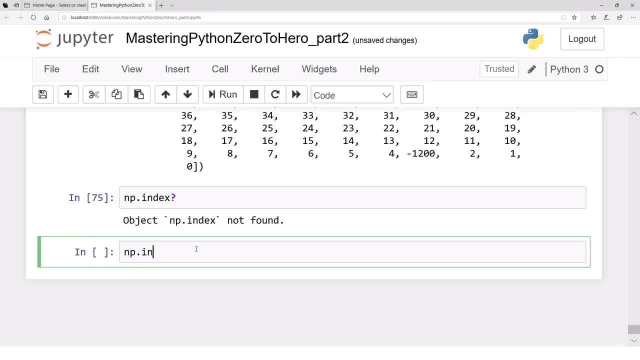 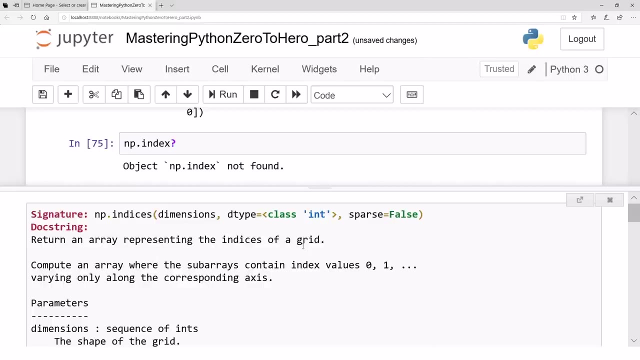 No, it is no longer there, But there is In this Function, I guess. So In this What that does. I guess that does the same job. Let me see: MP dot indices returns an array representing the indices of a grid. OK, 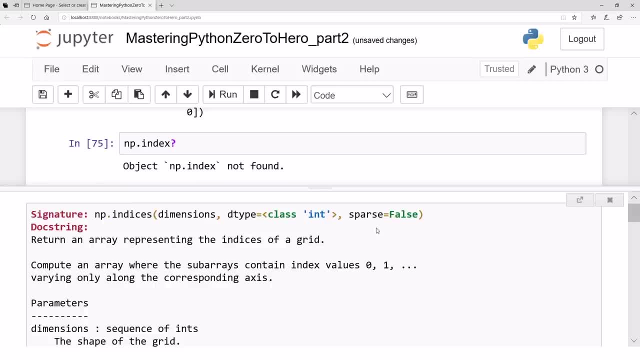 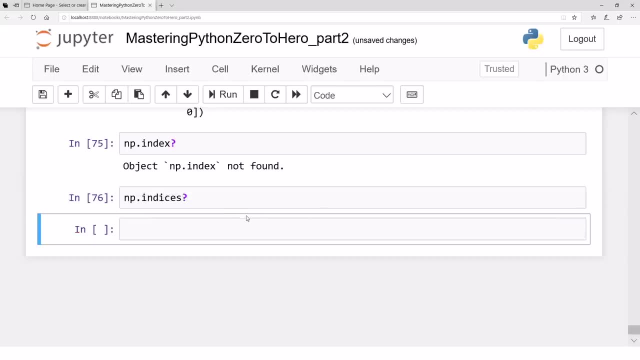 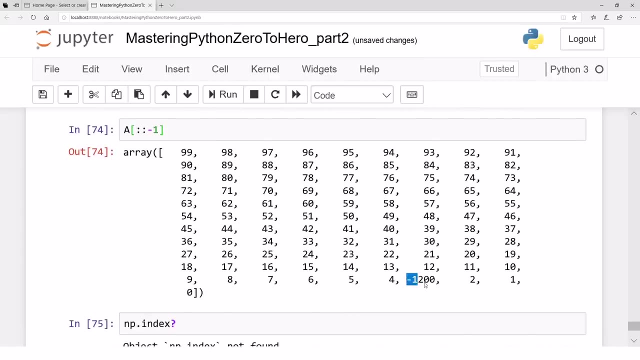 So I have to give a grade and then it returns, for example, the indices of all that grid. How can I use that? Well, It becomes. It becomes difficult. There may be a find function, or how can you locate the index where the minus 200 is is located? 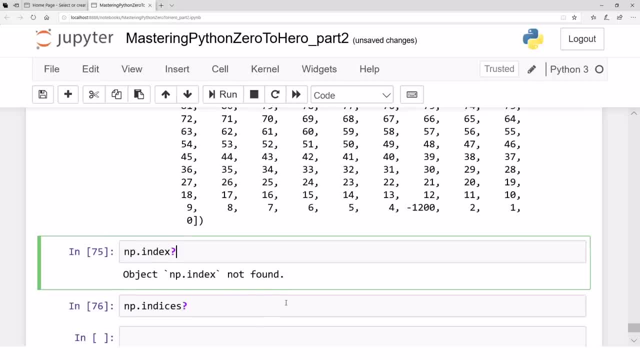 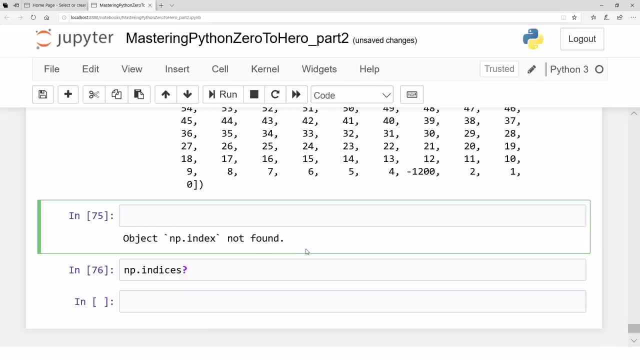 How can I? How can I do that? Hmm, Yeah, Very difficult. Seems like very difficult. Oh, why don't I, rather than finding out a function, Why don't I just play with Play with NumPy? Why not? 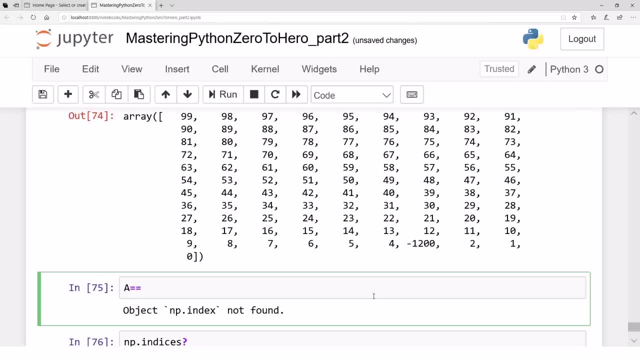 So let's say: A Equal equals Minus Twelve hundred. That gives me a Boolean array Comparing each and every Element with minus twelve hundred. So the array, the returning array, let me call the index array or the Boolean array. let's 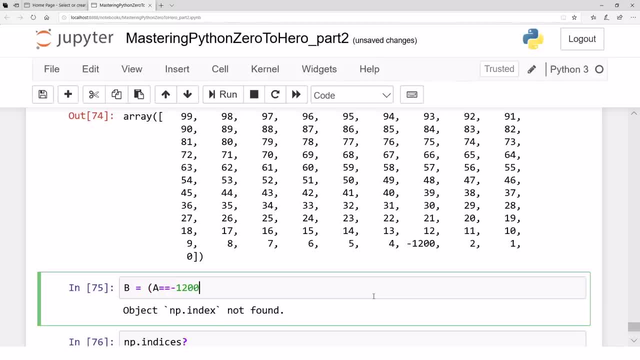 it be That array is true or false array, or zero or one array, Wherever there is minus twelve hundred, that index is one, that value is one, otherwise it is zero, completely zero. And then what I do is I just Multiply that. 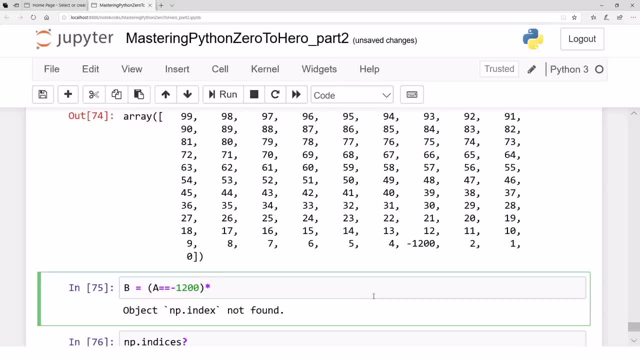 With With The N P Dot Arrange, N P Dot Arrange With, With Saying that A Dot A Dot Size. So whatever the size of a is, So Because these are the indices. 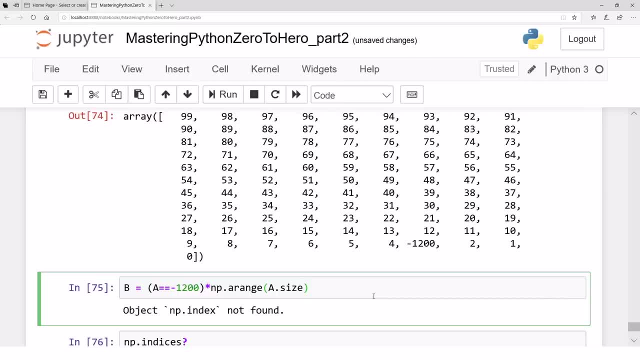 Okay, Then what? That's the pointwise multiplication grade. So When I will multiply them together, What I will get is Is What I will get After multiplication. I will get: How can I? How can I find out? 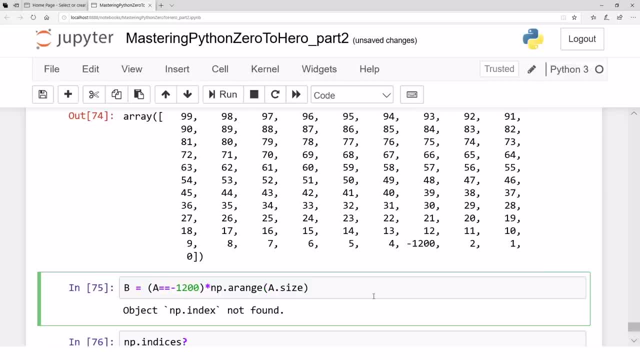 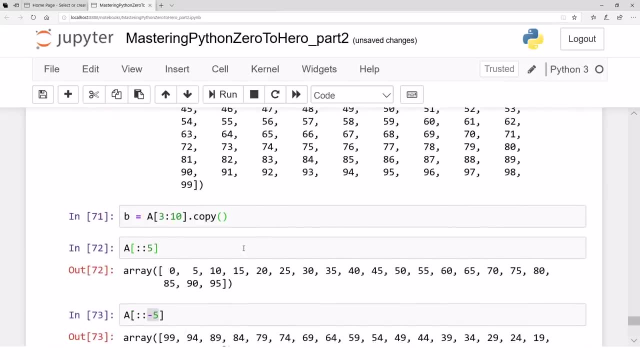 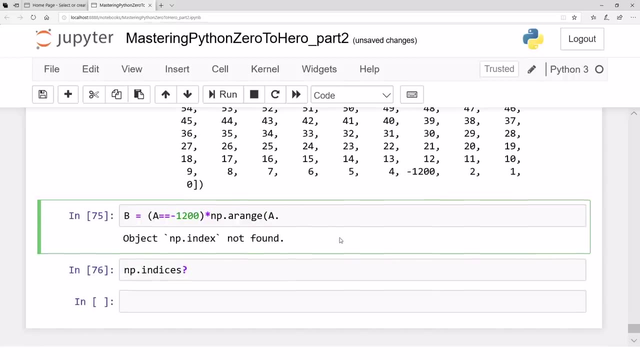 Actually, Actually, I'm lost here literally. How can I find out, How can I find out The Index Where? Where Am I So So that That That Is The Index Where, Where? 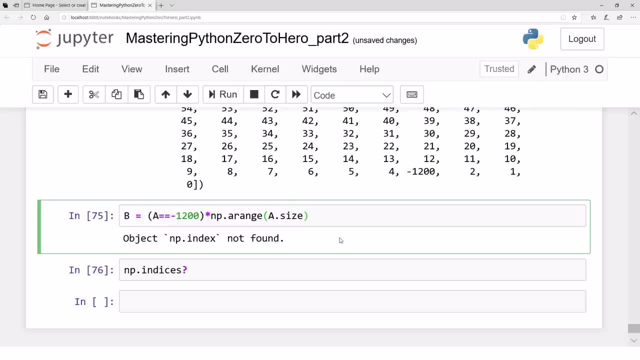 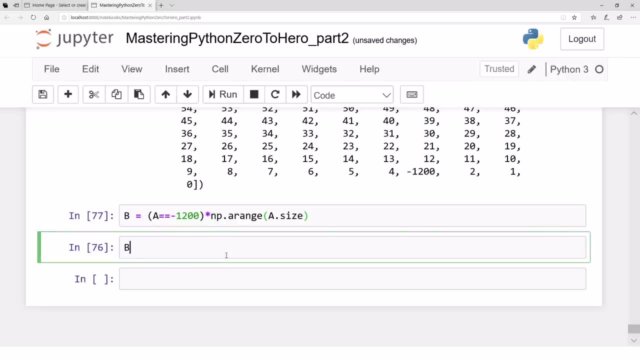 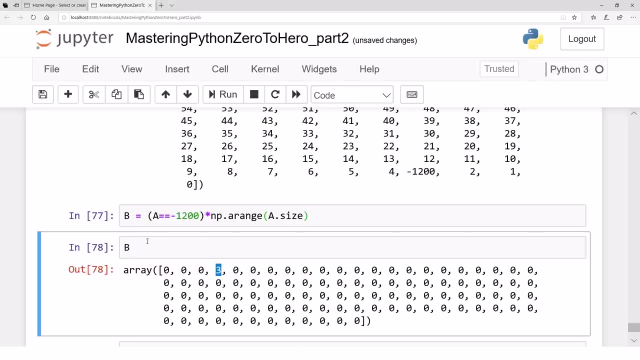 Am I So? So that will give me what. Let's see, What is B Now? The B Is B Is Just An Array. B Is Just An Array, And There. 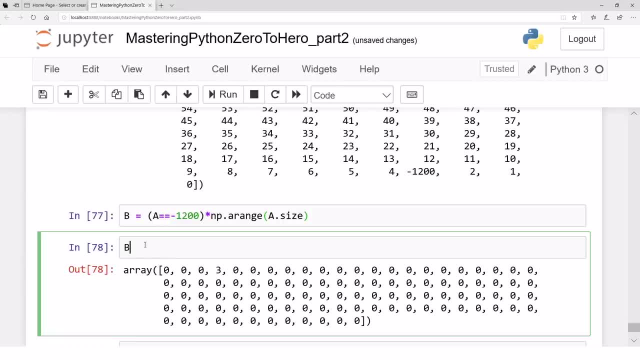 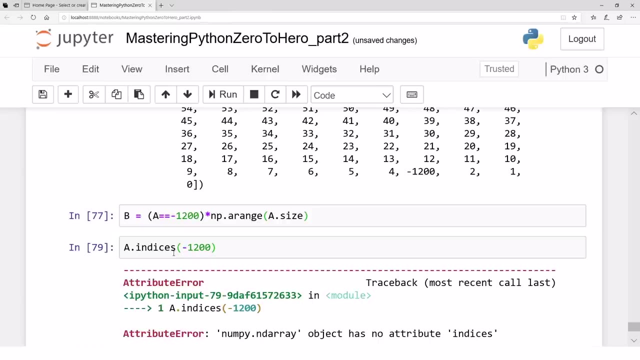 Is This Three That Is Located. So How can I find out? Where Is This Indices? And Just Give A Minus Twelve Hundred And Everything Just Worked. 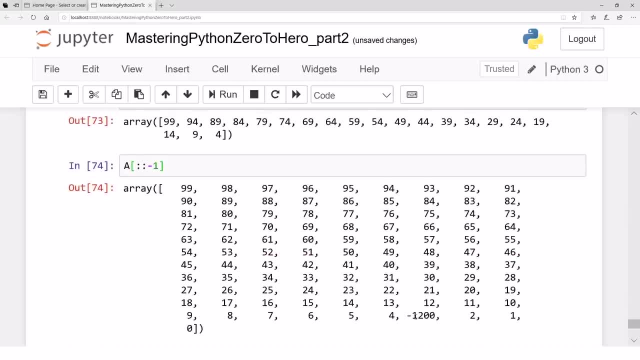 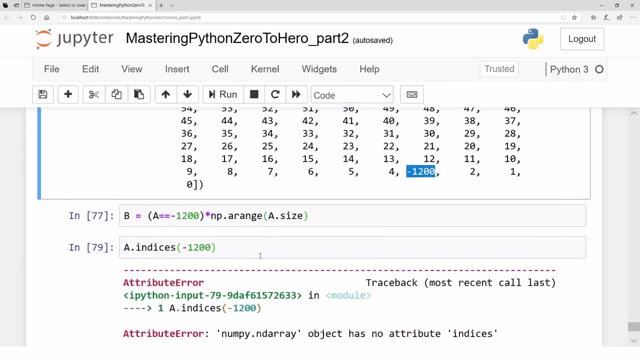 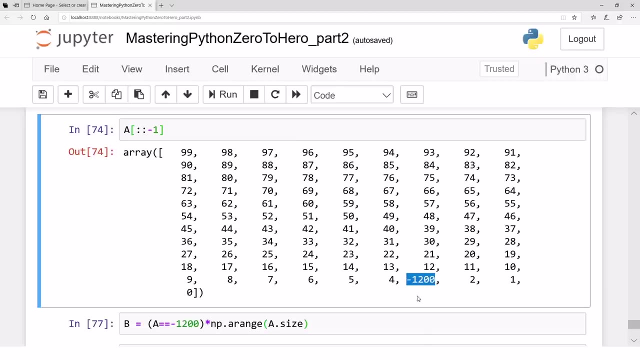 Out. No, There Is An Error. There Is An Error. Oh, I'm Lost Here, Literally I'm Lost, Attempted To Find All This Problem To. 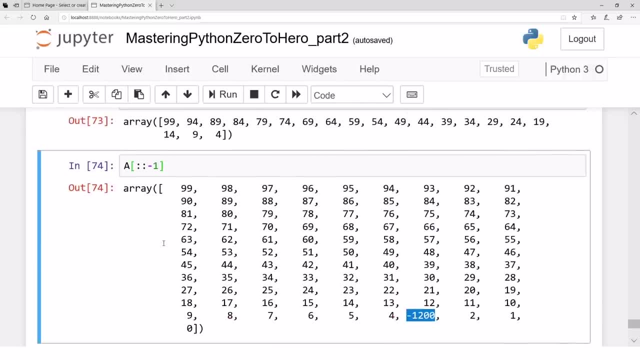 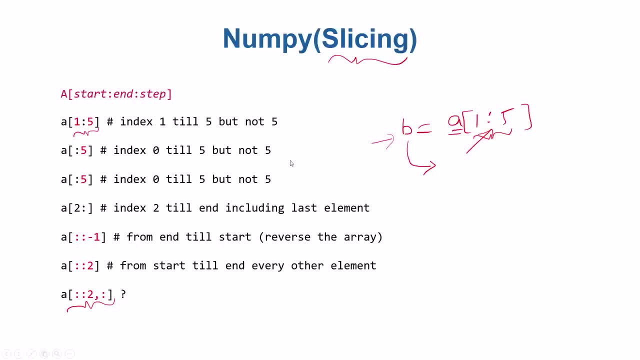 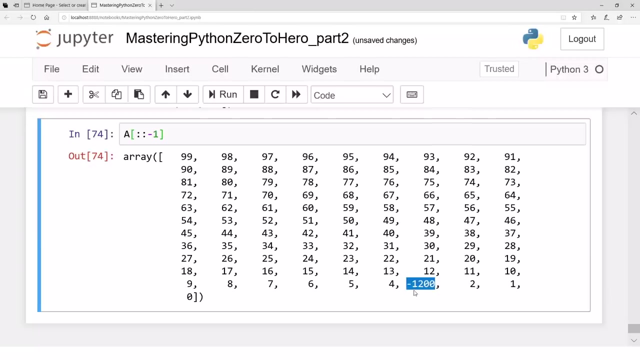 Find Out The Index Of A Particular Element, Or Maybe A Lot Of Elements, And Then We Will Continue From There. Okay, Hope to see you in the next video. Okay, Let's say this element is there and let's say: 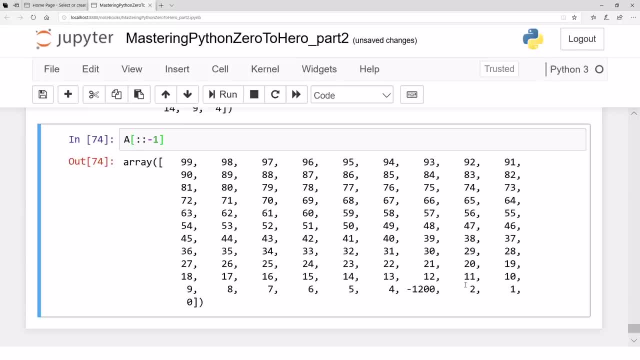 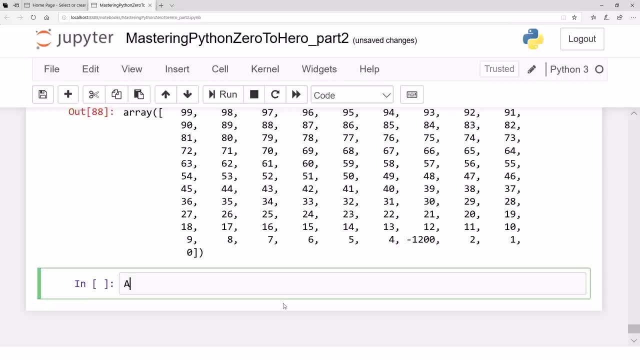 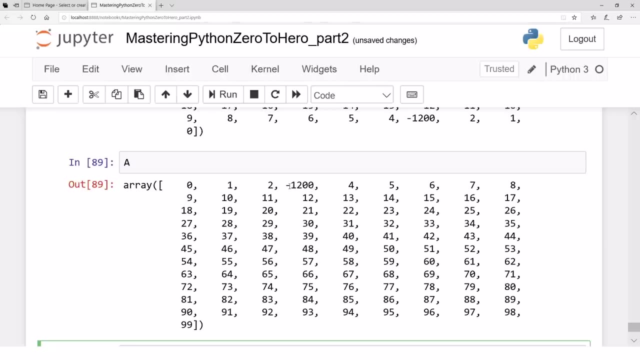 we want to locate that element in the array. We want to just know where this element is in the array. So array A has this element. Let me print array A as it is. This array A has this particular element and we want to know what is the index of this element inside the array. There are several. 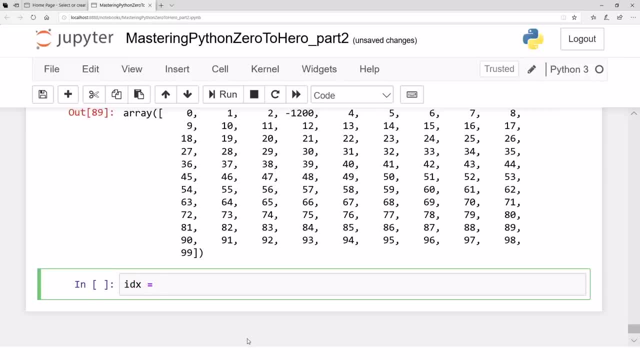 ways of doing this. One way is to find out that index is simply: you call the function arg, where, for example, arg where A is equal to minus 1200. And that will return a 2D array. And if you just want any one index, then you return that kind of thing. So if you write this thing, you will get. 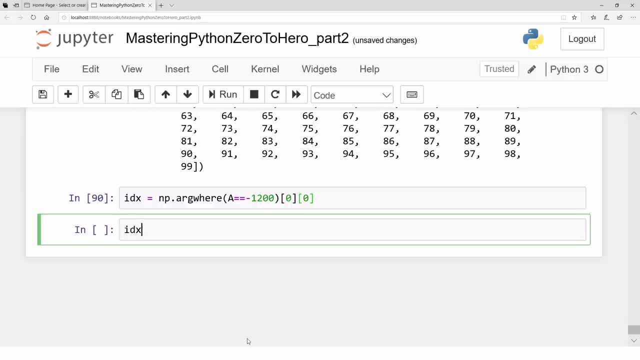 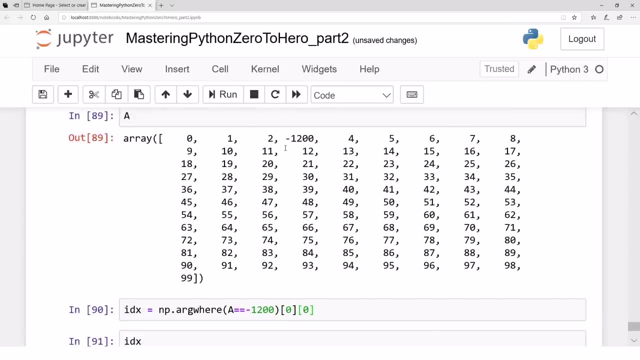 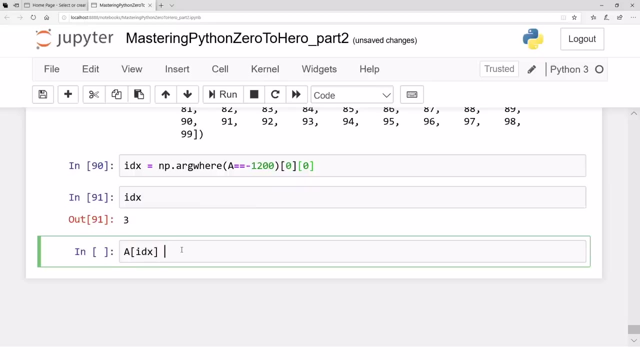 the index exactly of the element That is there. So the index is 3.. If you want to change that value- for example, the value should be 3 here- If you want to change that value- what you can do is you can write: okay, A IDX is equal. 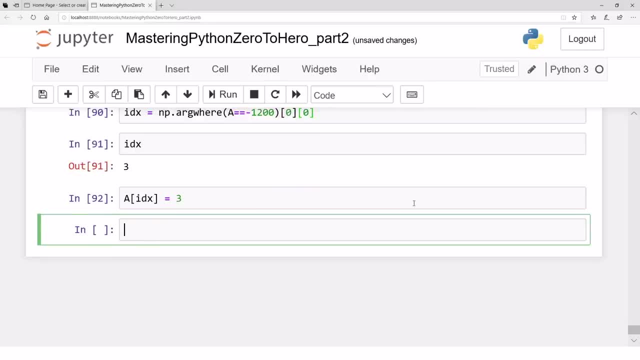 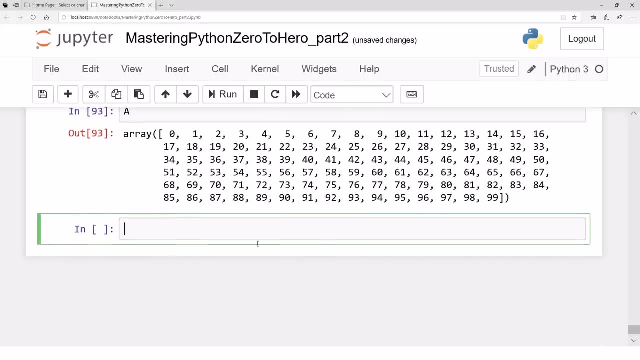 to 3 and A is reversed to its position wherever it was created. Okay, Great. Now let's play with the two-dimensional indices, Let's say two-dimensional arrays. Let's say we have A equals nprandomrand, let's say. Let's say we have a 5 by 4 matrix, Let's say a. 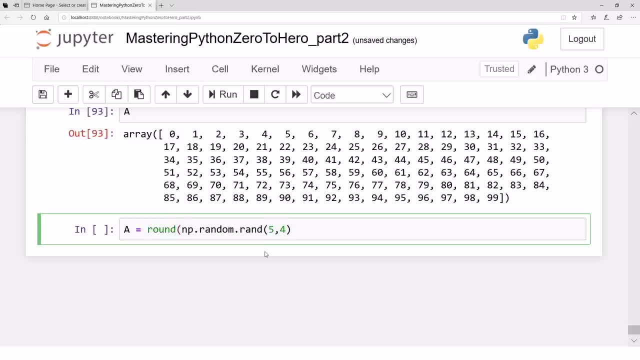 two-dimensional array. Let's round all the values by multiplying them to 10.. What it does is because all the values this rand function, all the values it generates are the values between 0 and 1.. What this multiplied by 10, what it does is it actually scales up all the values to 10 and then 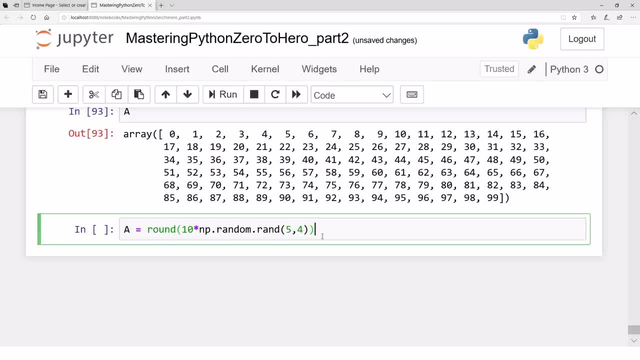 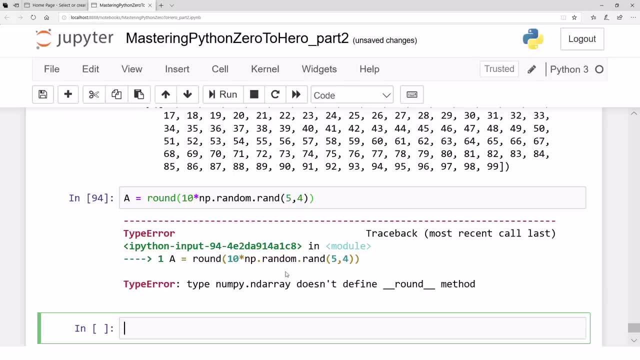 rand function actually rounds the values to the integers. Now A will be: what's the problem? rand method? rand method is no longer there. Okay, Maybe there is nprand, Maybe that nprand, Maybe nprand is there, Yes, nprand. So rand function. 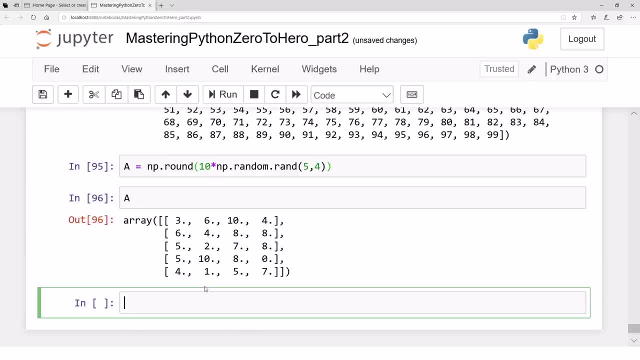 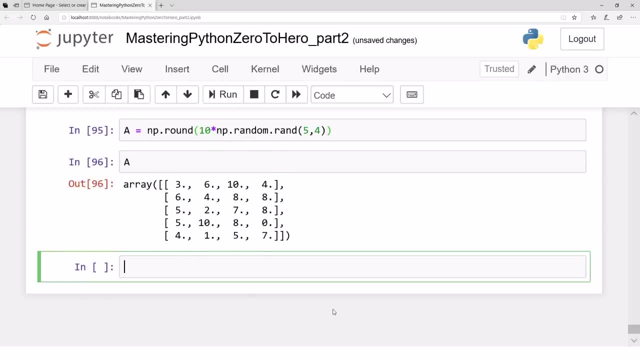 nprand. So this A is A, is this array, for example, That's a 5 by 4 array, four, five rows and four columns. So let's say I want to access the second row First of all. let's say I want to access this particular entry. This particular entry is second row and third. 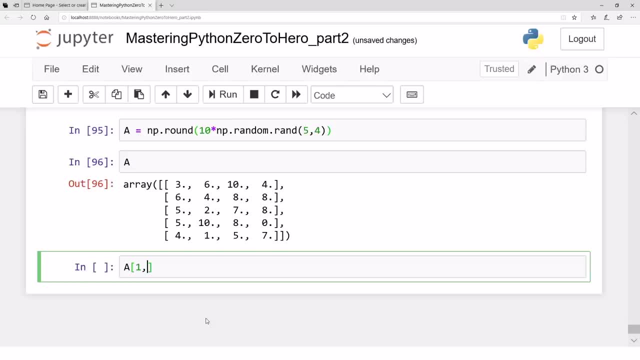 column, which means the index is 1 comma 2, because a second row means the row. row first has index 0, row 2 has index 1.. Similarly, column 1 has index 0, column 2 has index 2,. 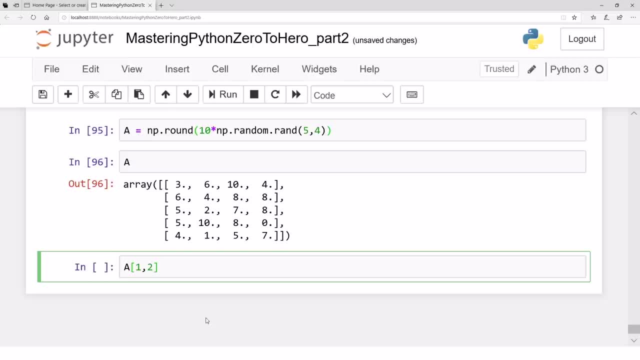 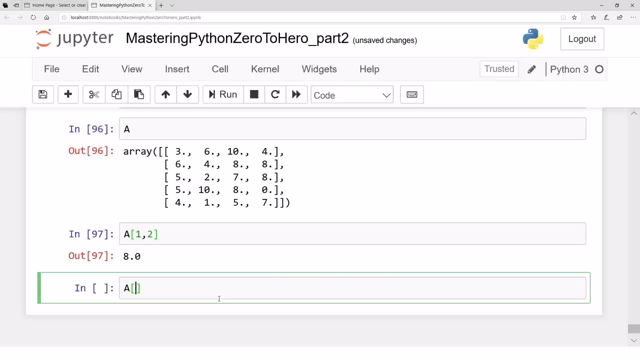 1 and column 3 has index 2.. So that is what this particular entry is. What if we want to access the whole second row, for example? We want the second row. So that's how you call, that's how you slice. 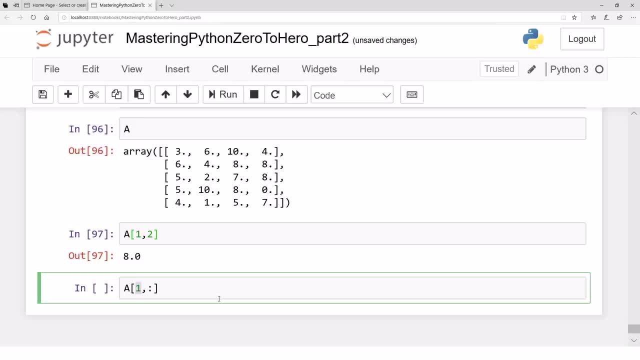 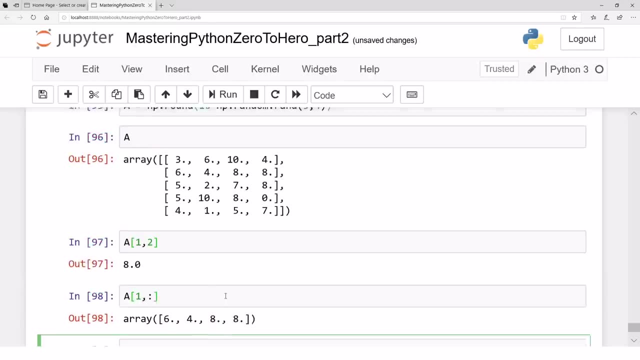 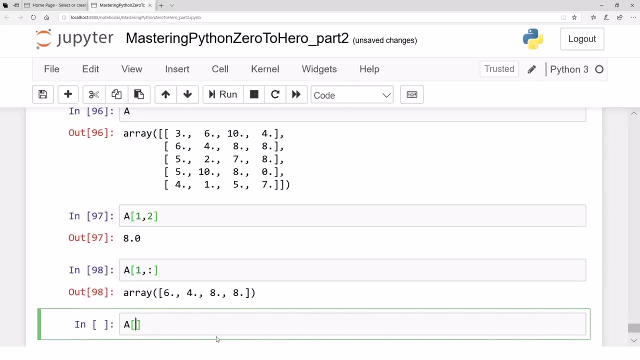 A normal meaning of this is you, the the row should be 1 and the columns all the columns. So that's how you access the whole second row. If you want to, for example, access the whole third row, for example, or whole second column, let's say, That means you say this. 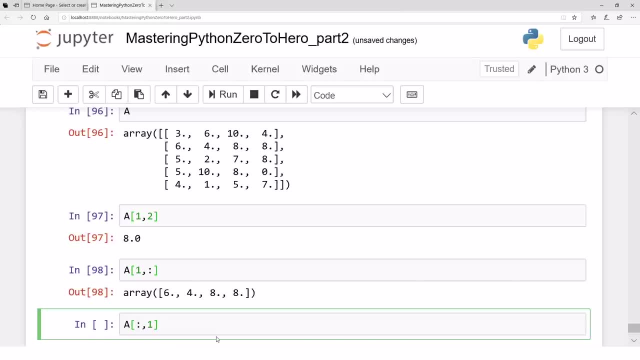 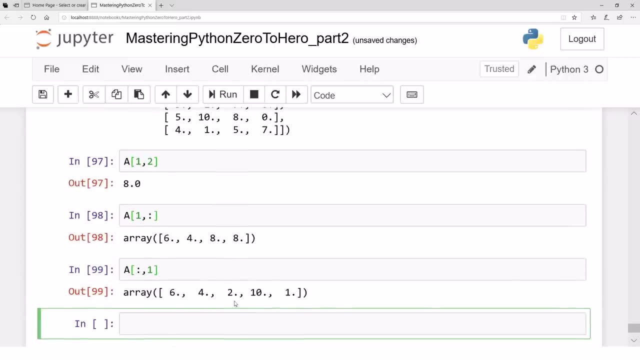 okay, the column number second and all the rows, which means the whole second column that is accessed And that, if you see, that's the whole second column: 6,, 4,, 2,, 10, and 1.. That's what. 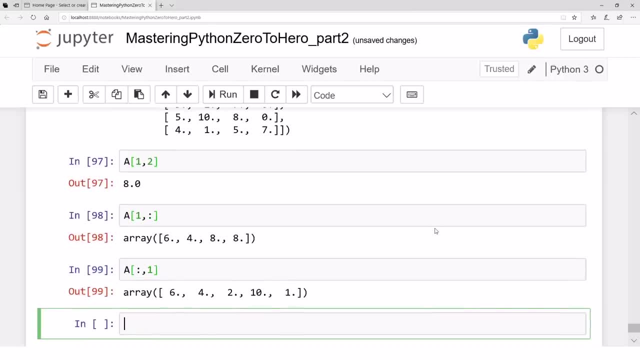 the second column is Further. once you have, you can. you can, for example, access a sub-matrix. Let's say you want, you want row number 1 to row number 3, not including 3.. And then, of these rows, 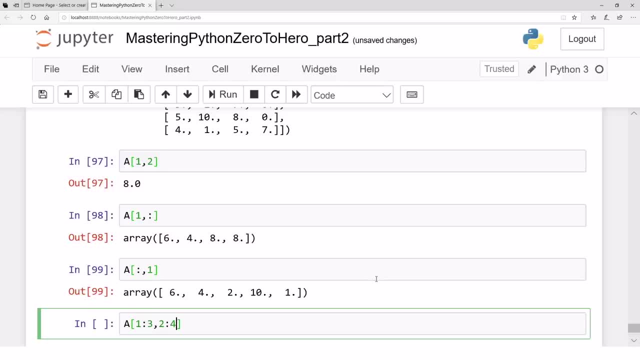 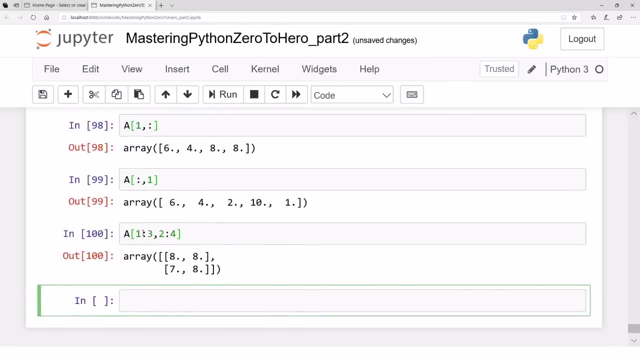 you want column number 2 to column number 4, let's say, And if you do that you access the whole sub-matrix. First it it actually picks row number 2 and row number 3, because row number 2 starts from 1. And then of those rows it picks these columns And you can. 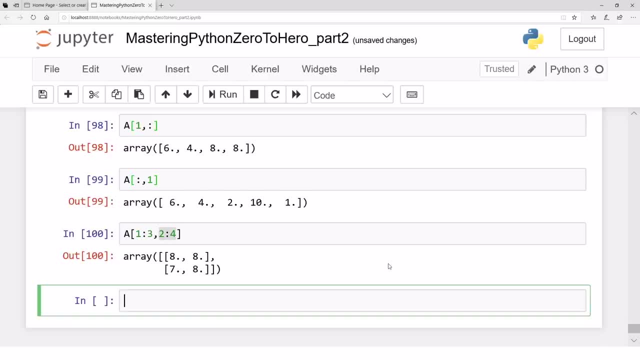 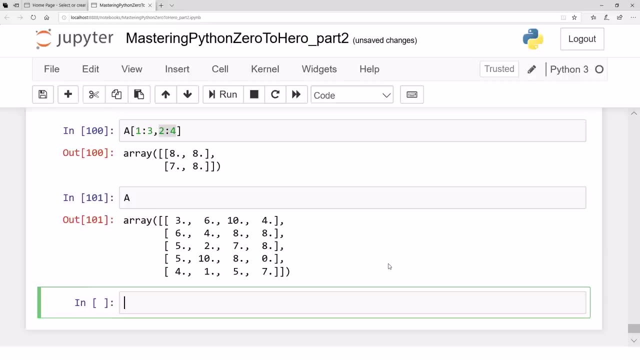 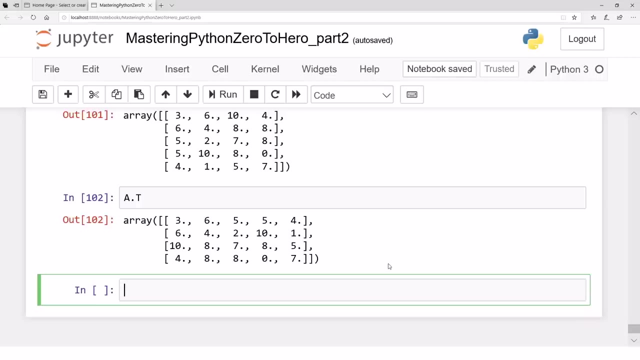 just pick the, pick the sub-matrix inside, More you can. you can do a lot of processing on these matrices. For example, this is matrix A. If you just type A dot transpose, that T is for transpose, the matrix just is taken, transpose of it. Further there is a complete library: linear algebra. 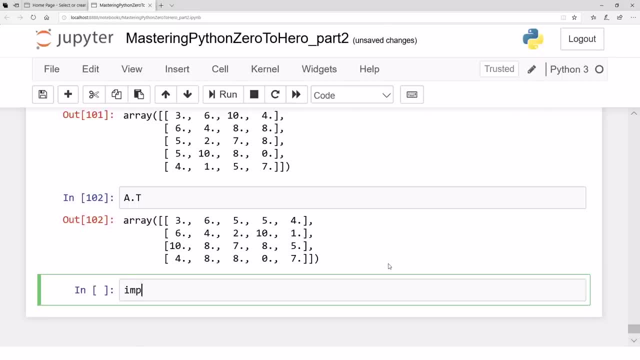 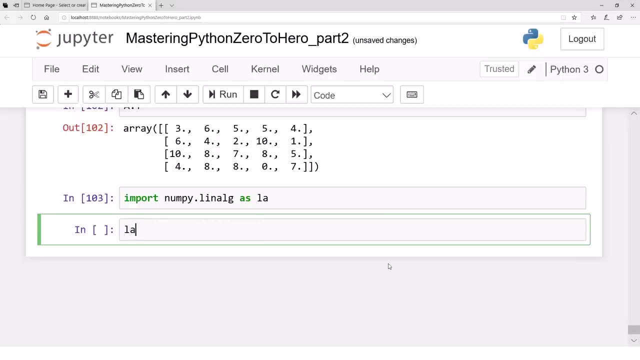 library in NumPy. For example, if you just import NumPy, NumPy dot linear algebra as L A, for example, then this linear algebra library in NumPy has a lot of functions: eigenvalues, Cholsky, decomposition, computing, determinant of a matrix, finding out the inverse of a matrix, and and whatnot. 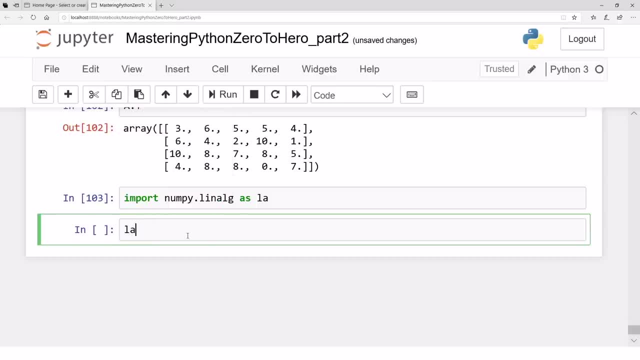 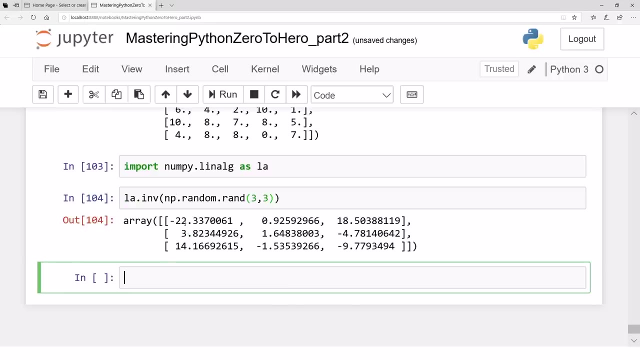 For example, let's say we have L A dot inverse and here is N P dot random dot rand, Let's say some 3 by 3 matrix. So what it returns is it returns the inverse of this matrix And this linear algebra library. and there are other. 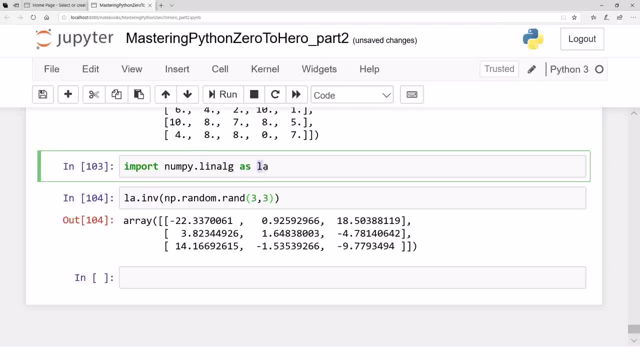 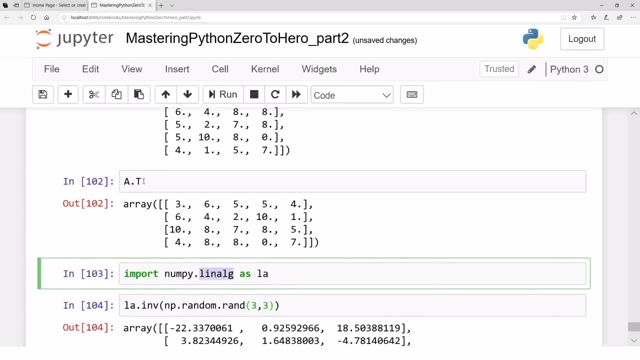 libraries as well, but this is one scientific library that maybe most of data science experts who actually want to do research they might be thinking. this linear algebra library, that that's, that specifies a lot of functions related to related to these matrices or two-dimensional arrays. 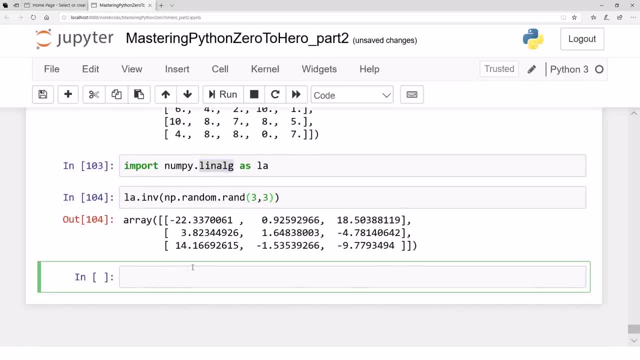 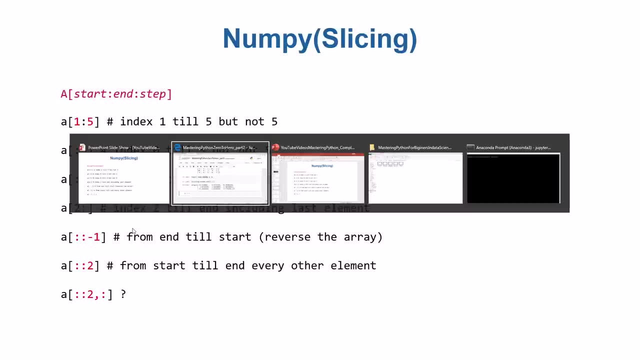 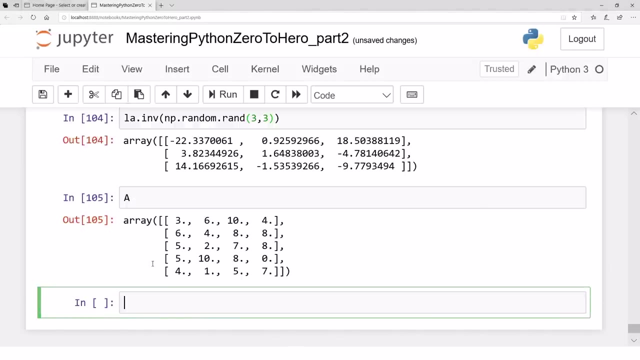 So that is there. Okay. So that's about indexing. We can play with these indices a lot if we want One more thing, just just one. one last thing. Let's say this is our A, and what we want to do is let's say we 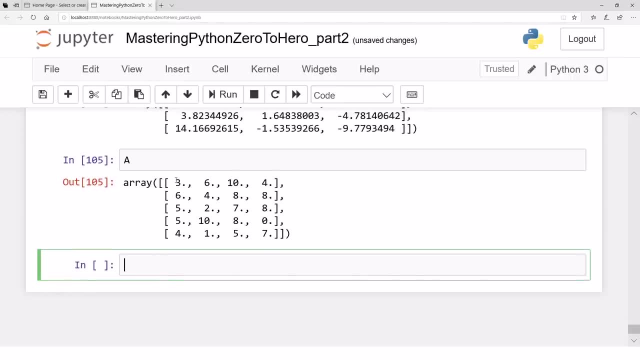 want to sort this A with respect to the columns. We want each column to be sorted individually. What we can do is we can call sort function and we can pause. x is equals zero. X is equals zero. That means sort all the columns individually. 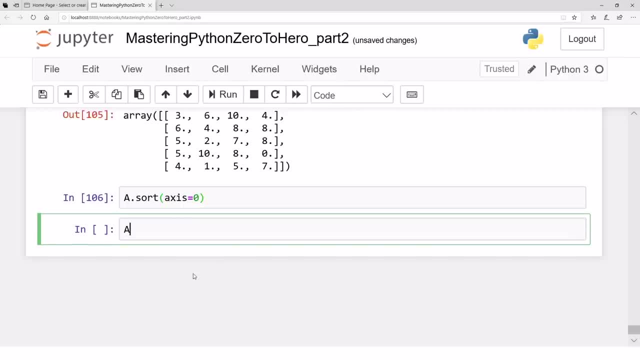 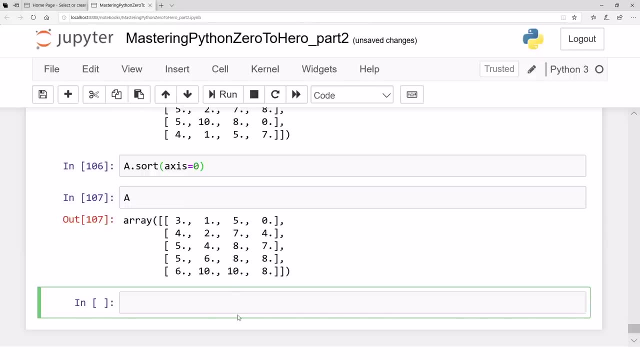 and the result will be. if you see the result, the result will be: every column is sorted individually. If we want to sort, for example, every row individually, we will say, okay, sort x is equals one and every row will be sorted individually. 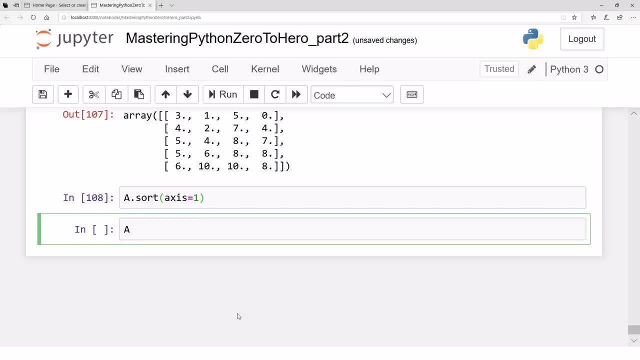 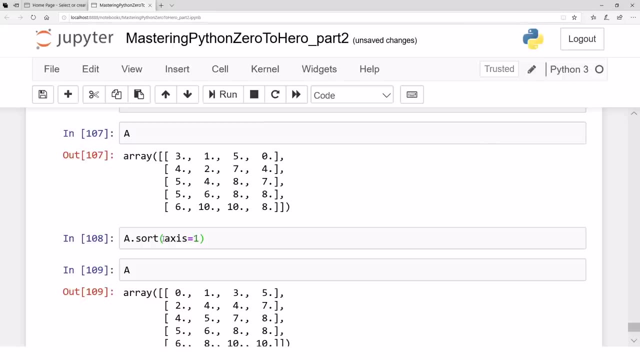 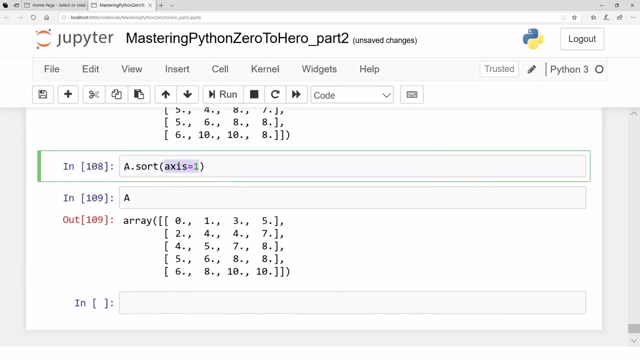 And if this is a multi-dimensional array, more than three, more than two dimensions, then x's can be two, x's can be three, So which, with respect to whatever x's you want, your sorting can happen. It can do that If A is one-dimensional array. 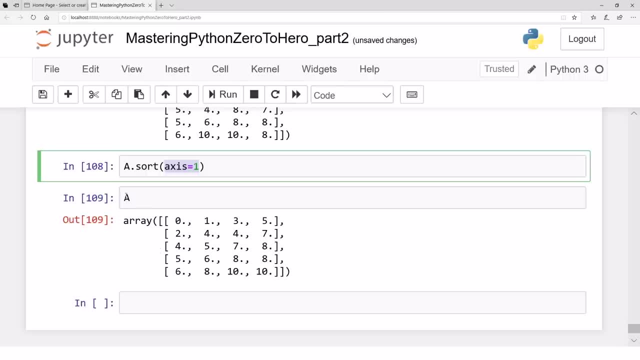 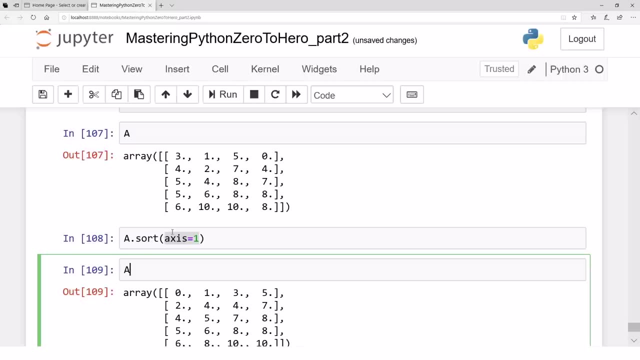 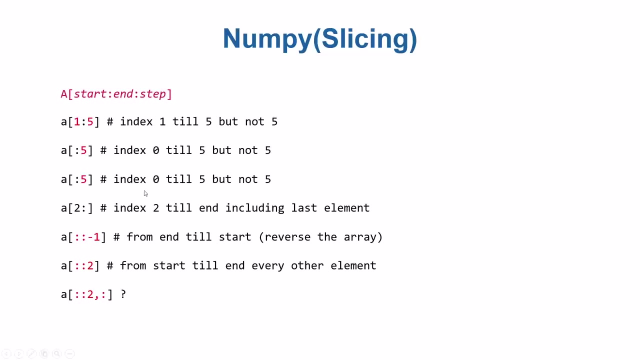 then dot sort function without an x's, just sorts. just sorts the one-dimensional array from beginning to the end, And if you want a descending order sort, just sort them. sort it first and then reverse it using indexing. Great, I mean, there is a lot to discuss. There is a lot to discuss. 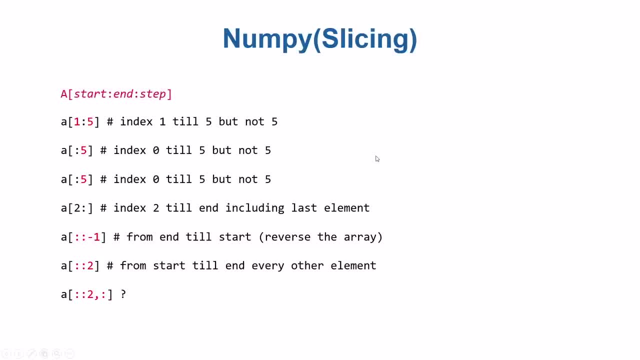 I'm ending this slicing here. In the next video I'm going to show you a kind of masking, or sometimes called the fancy indexing that is much more powerful and useful in a lot of different contexts. So hope to see you in the next video with more NumPy indexing. 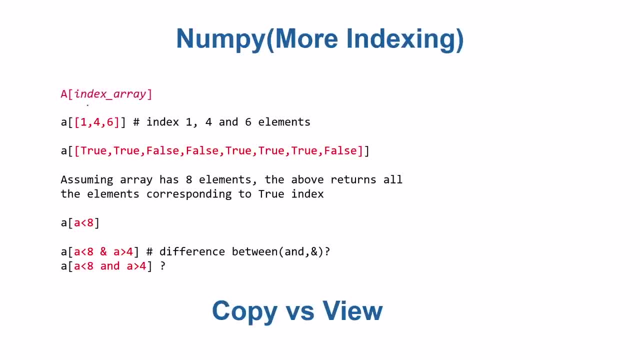 Okay, There is another way of indexing a NumPy array. In the last video we saw we can do slicing notation, For example, start from here, end at here and stuff like so. There is another way of accessing a NumPy array as we have an array A and we can just give the 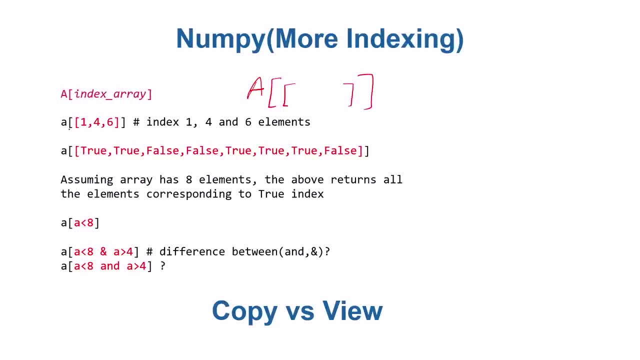 give an index array inside. For example, let's say A is one-dimensional array, and then we just give one four, six. That means pick the element at index one, pick the element at index four, pick the element at index six. So this kind of 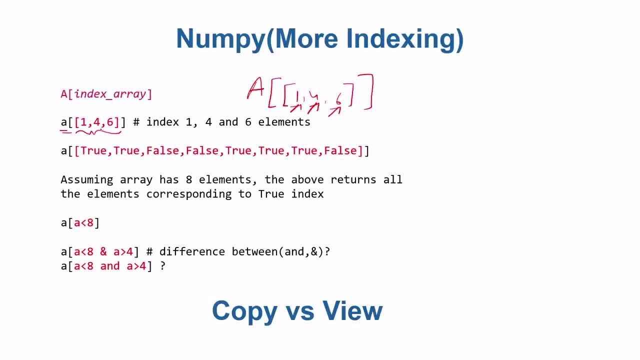 array. inside can be a list or an array. that is called an index array And you can just pick the elements that you want to pick. For example, you want to pick all odd elements. You want to pick first element, fifth element and 17th element. You can just create an index array and pass it. 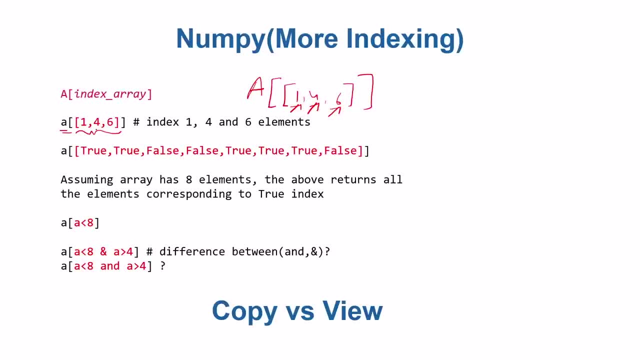 and index your and access your elements using that index array. That's possible in NumPy array. Further, you can access different elements using a Boolean mask as well. So Boolean array, for example. So it's true, true, false, false. Wherever there is a true, pick that element Wherever there is a 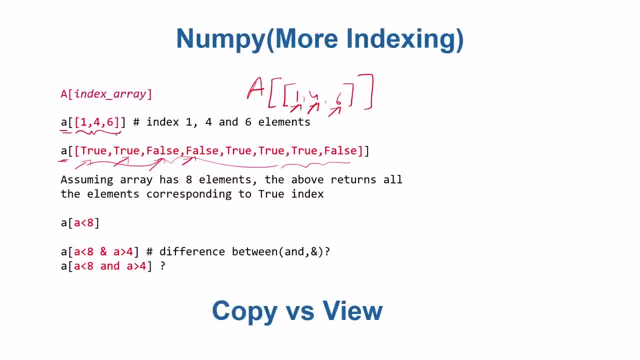 false. don't pick that element and return the elements that are picked. For example, assuming here that you have an array A which is one-dimensional array, let's say Assume that has eight elements- One, two, three, four, five, six, seven, eight elements. Now you pass a Boolean. 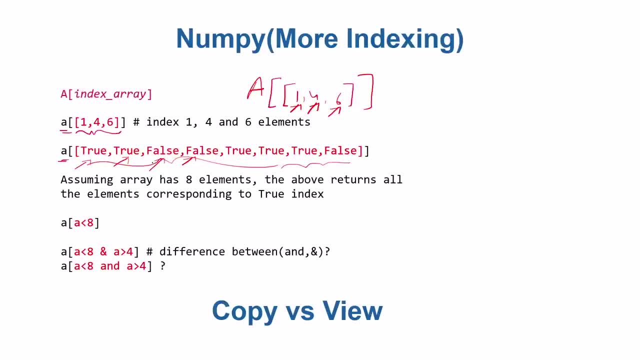 mask inside with obviously eight elements, eight true or false values, wherever that is true. So pick the very first value, Pick the second value, Don't pick the third value, Don't pick the fourth value, Pick the fifth value, Pick the sixth value, Pick the seventh value And don't pick the last value. So that is also possible. 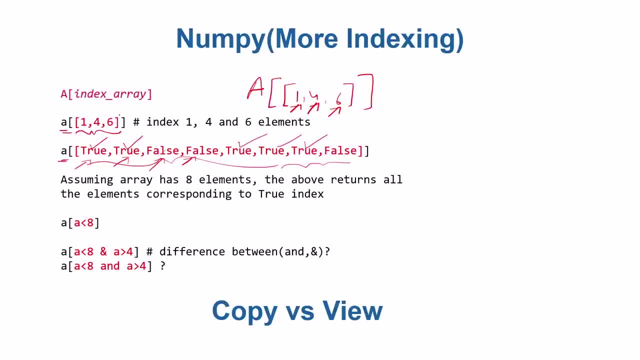 in NumPy. One thing that is important is if you do this kind of indexing, which is sometimes called masking. if you do that, if you supply an array, index or index in a Boolean form, you by default get a copy as compared to slicing. In slicing you get a view. that's a separate copy. You need not to call a. 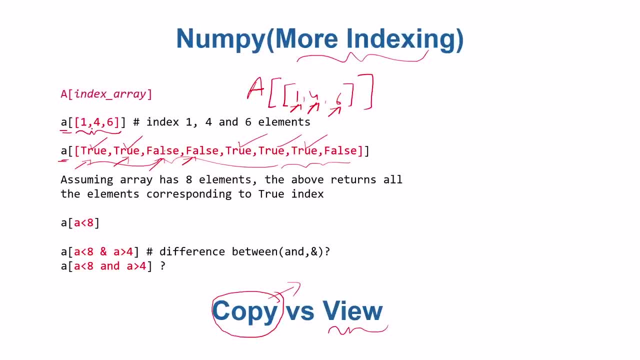 copy function. It is by default a different copy And this is a difference between the ordinary slicing that you do. For example, start from one, go till 50, take a jump off, let's say two. If that is your indexing style, that is called a slicing. the return value is a different view. 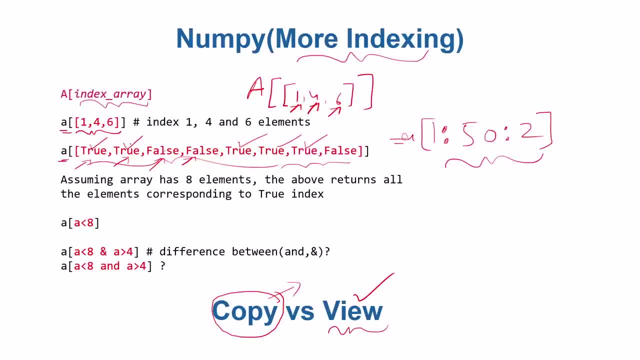 having the same memory. However, if you do the, if you use the array index or the Boolean array called masks, then you get a copy rather than so, which means if you get a new array, you change the elements in the new array using the array indices. you're not getting that change. 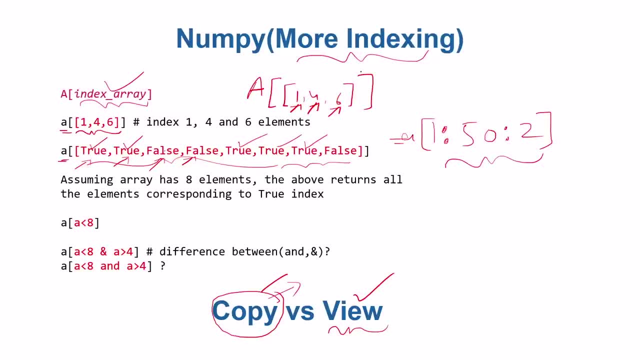 happen to the original array. So that's the difference between slicing and masking. Okay, This kind of Boolean indexing becomes really handy. For example, what if you want to get all the elements that are smaller than eight? One way to do that is just write. 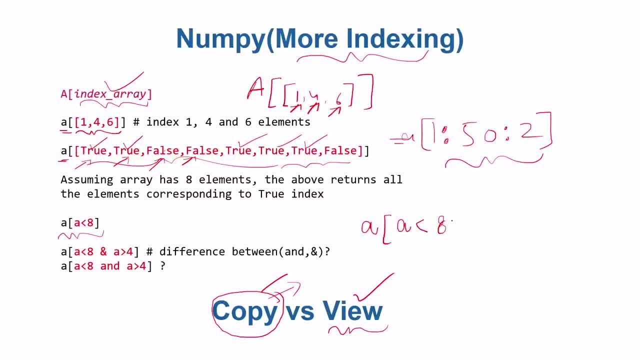 a and then apply a condition: a is less than eight. Well, a is less than eight will create a Boolean array and everywhere where the element is smaller than eight there will be a true. otherwise it will be a false. Now the inside array is a Boolean array and you access all. 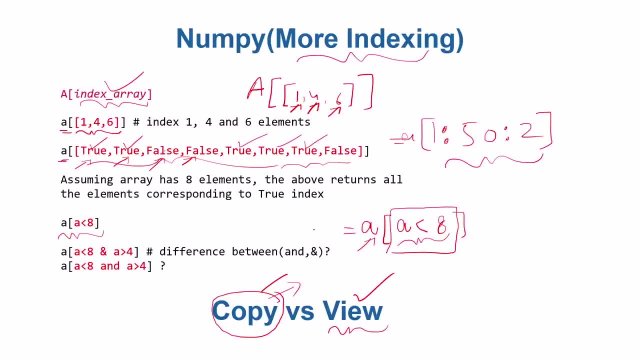 the elements with respect to that condition. So it will return all the elements that are smaller than eight. How fancy is that? Further, you can have these conditions in a combined way. There is one difference: There is an and operator, a and the and. 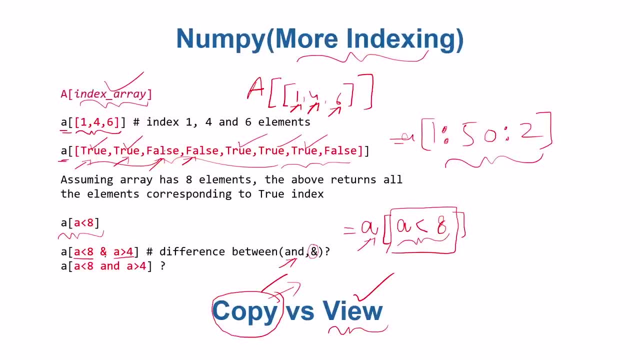 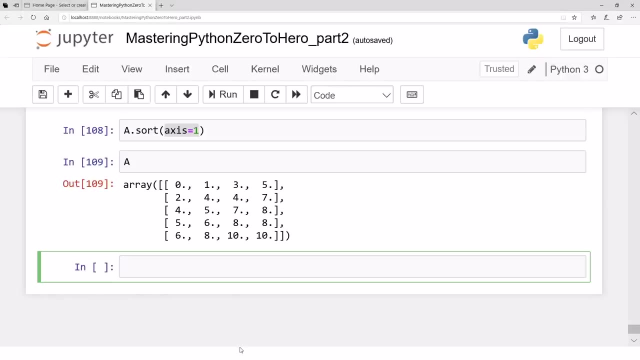 and there is an and operating in a different way. So I'm going to discuss the difference of this and and this and as well in this video. So let's go to Jupyter Notebook, our friend, and see how can we play with this masks. So let's say a is again nparrange. 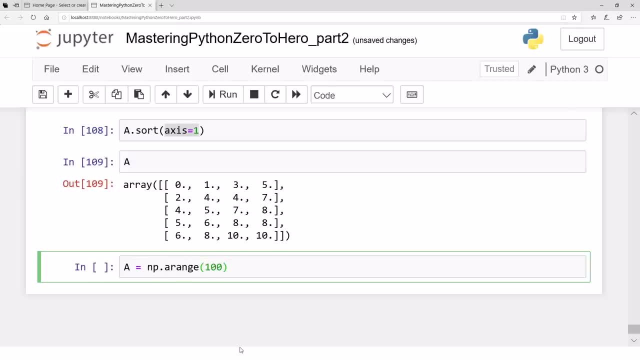 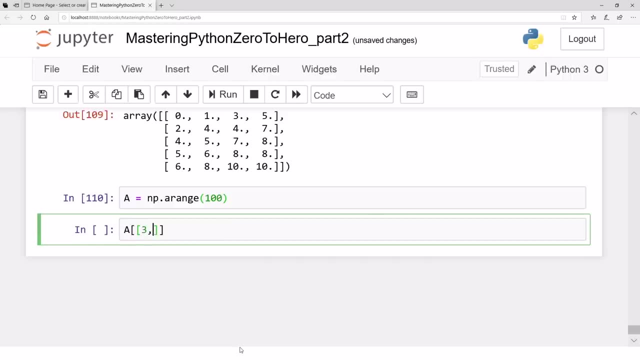 change. let's say 100.. Let's say that's our A And what we now do is we access the elements of A. we access, for example, the third element and the fifth element and the sixth element. Let's say we want to do that And that's our B. So that happens. let's say So what B is. 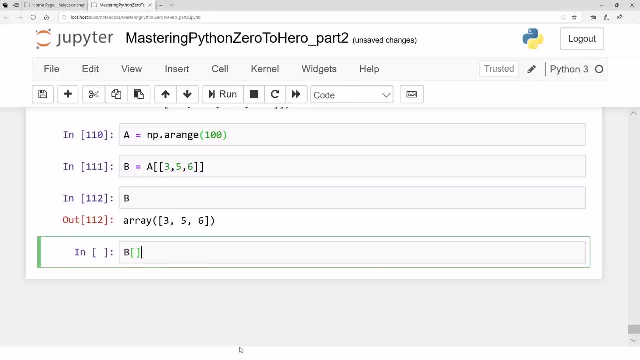 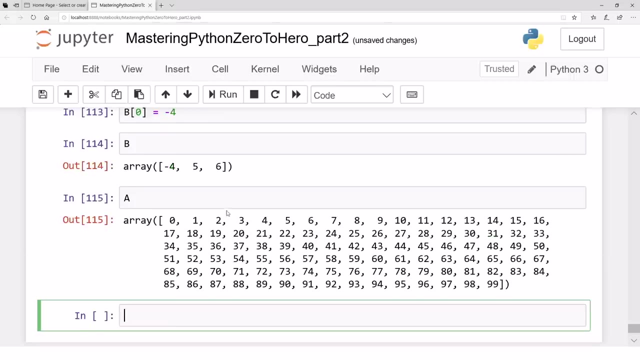 B is this? Something that you need to know is, if you change the elements of B now, because that's a copy, let's say minus four, that change does not happen in A. That happens in B for sure, but that doesn't happen in A. A does not contain any value. that is minus. 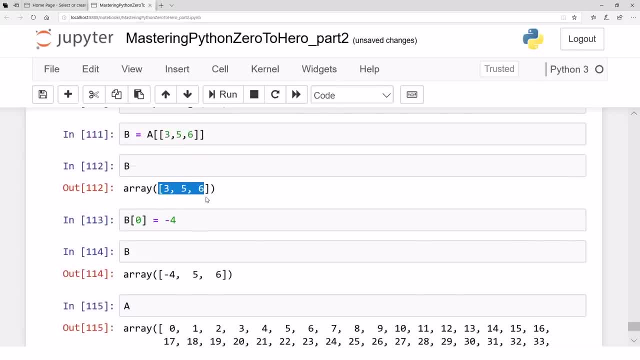 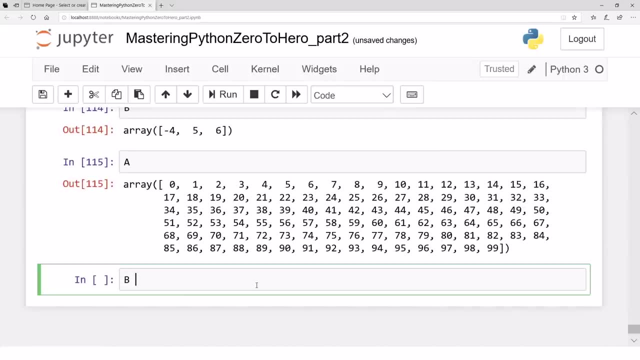 four, because using these kind of indices- the array index- by default the result is a copy rather than a view. Further, let's say you have this A and you want to access all the elements that are smaller than, let's say, 40.. Access all the elements that. 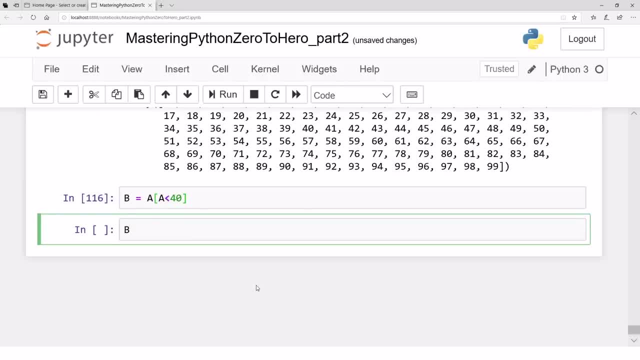 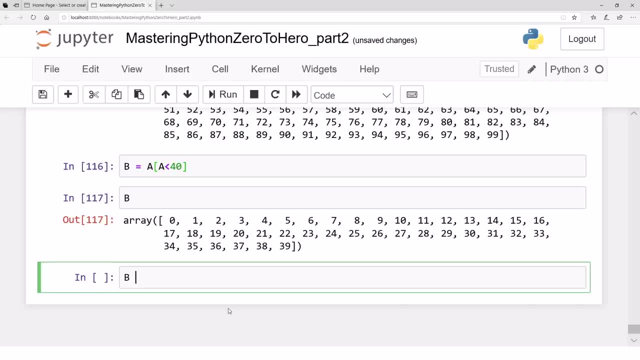 are smaller than 40.. smaller than 40. So that is possible. Now we will contain only the elements that are smaller than 40, all the elements. Wow Further, if you want to access all elements that are smaller than 40 and they are bigger than. they are smaller than 40 and they are bigger. 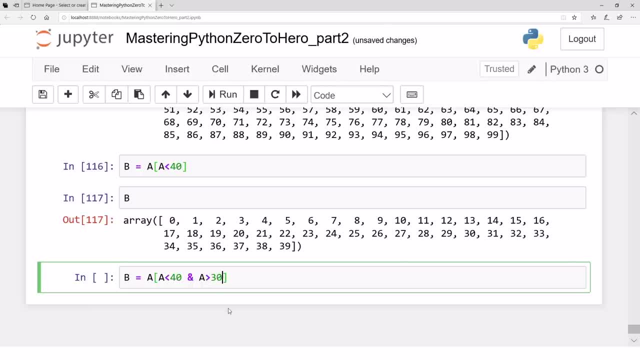 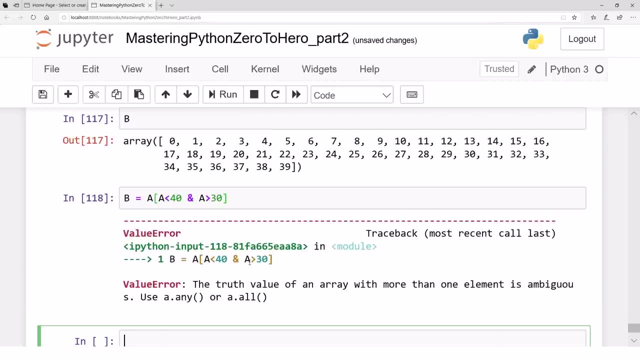 than 30. Let's say you want to access all the elements that are between 30 and 40. You can just access those elements like. so There is a problem, aany aall. What's the problem here? The truth value of an array with more than one element is ambiguous. Use aany or. 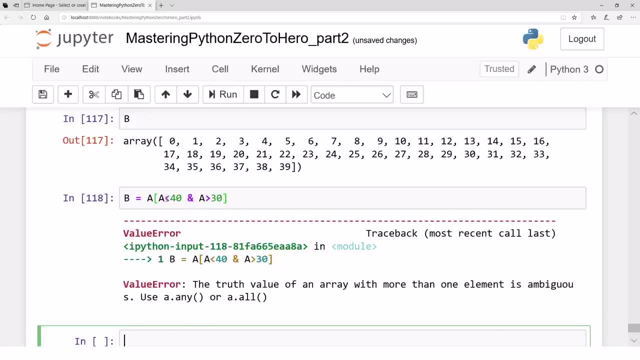 aall. Okay, this a is less than 40. It is a Boolean array. a is greater than 40. That's a Boolean array. So what's the problem? Why can't we not use a Boolean array? Why can't we not use a Boolean array? Why can't? 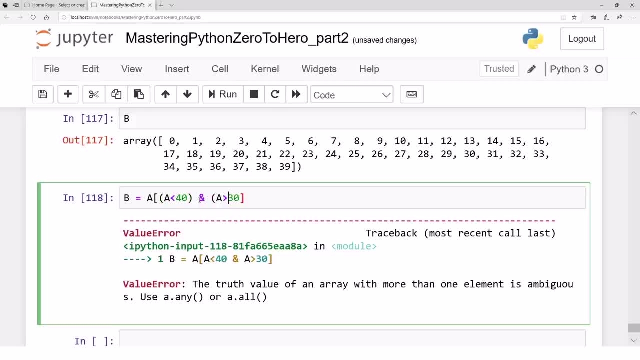 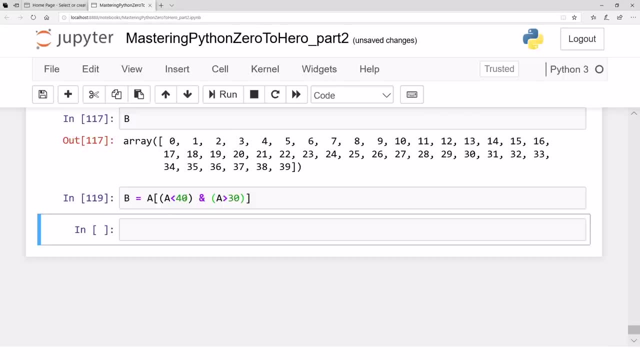 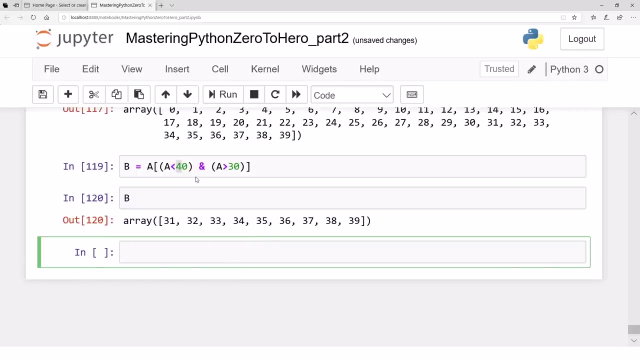 we not use a Boolean array for, say, a fast � Now, b contains only the elements that are between 30 and 40. Now, one thing, what's the difference between this particular and, and this Woah! This is great!!! 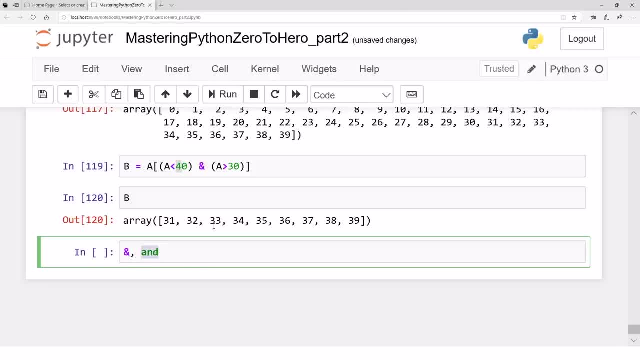 symbol AND The difference is this: AND AND operator. it is used when both of the sides of this AND is one object and it has one true value, either true or false. And this particular symbol is used when the left side and the right side can be arrays and each element 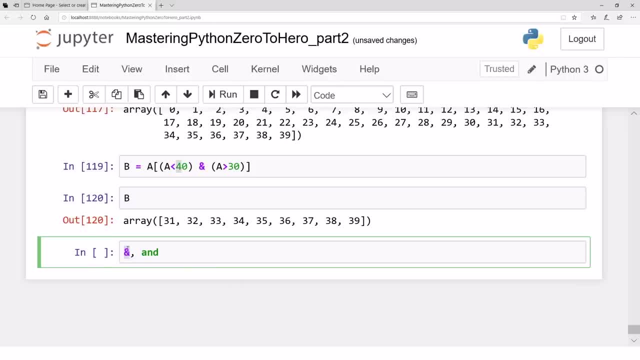 of that array can be true or false, and so, So you can think of this: AND is used in arrays. however, this is used when both the sides are single objects, So that's the difference. Other variants of AND- I mean the AND- is like this: these are the same things, But remember. 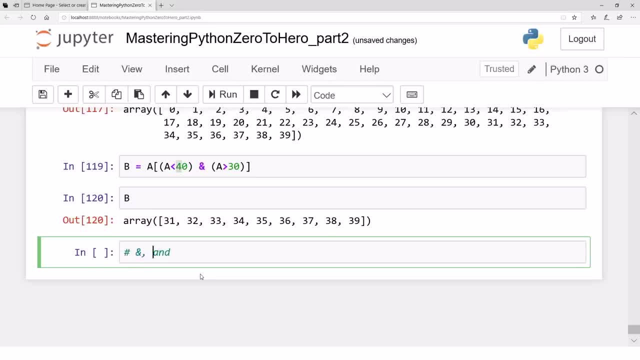 the USE. this is used for arrays. this is used for single objects. Similarly, there are other symbols like OR that is used this way, OR that is used that way. Similarly, there is a NOT for arrays is used like this way and not for otherwise is used like that way. so 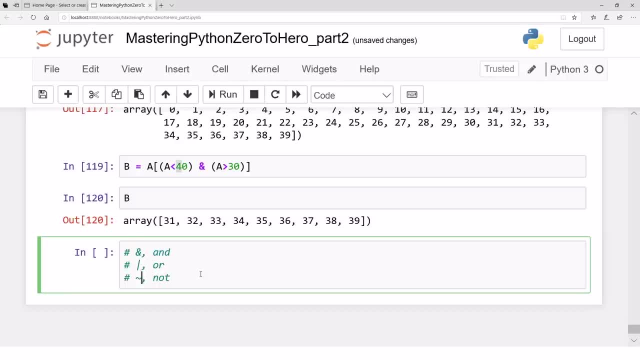 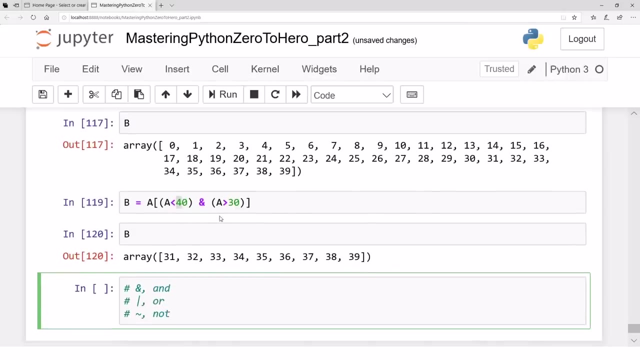 remember these: the left side kind of symbols: they are used for arrays. the right kind of symbols: they are used for single objects that has true or false values. so these, this kind of masking, is really, really powerful. later we will see in pandas accessing different kind of data with particular kind of 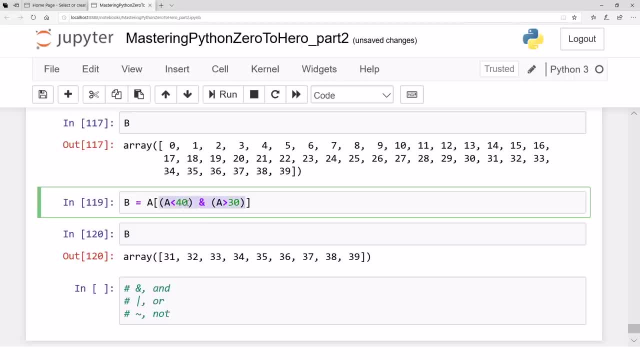 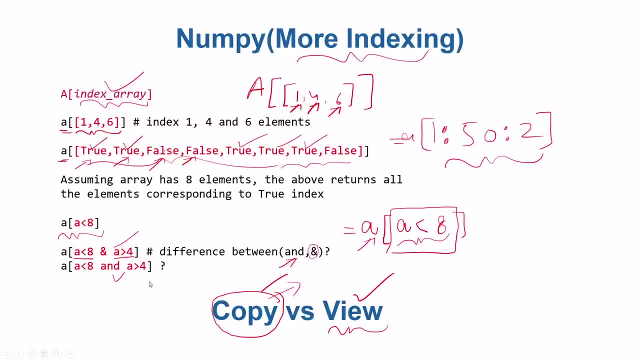 conditioning. that becomes really handy if we, if we- are comfortable with these kind of indexing, and that's really powerful indexing, okay, so I've told you the difference here between an and and I've told you that this is copy rather than a few. so just bear with me some more time on numpy and I will tell you. 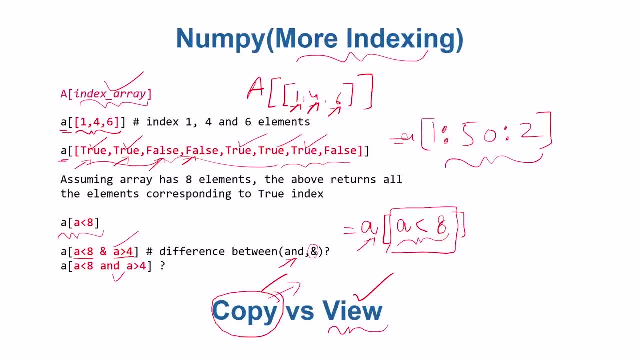 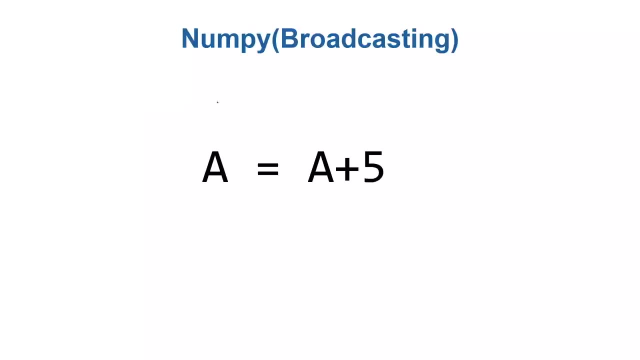 some more truths about numpy and then we will move towards another package called pandas. so, before pandas, more numpy is coming. hope to see you in the next video. okay, in the last video we talked about how to use pandas and how to use numpy. in the last video we saw masking, which is sometimes called the fancy indexing, as 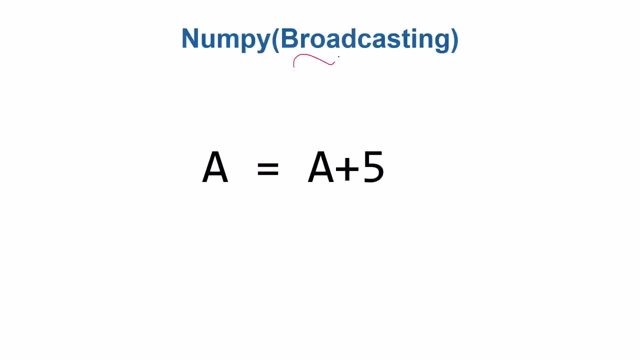 well, and- and here we are going to discuss one more feature of numpy which is very powerful, feature called broadcasting. I think, for example, you have an array, let's say two, three, a matrix, that's a two-dimensional array- two, three, five and nine- and you want to add in every element, you want to add a. 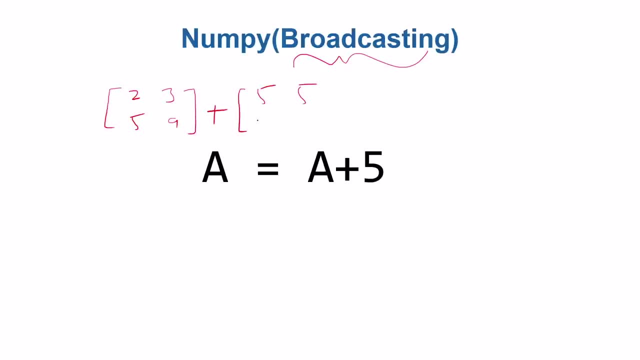 number, let's say five. so one way to do that is create another array with five, five, five, five and just apply this add operator and you are done. great. but this numpy allows you to just write. let's say: this is aana numpy allows you to just do this particular thing and this five is 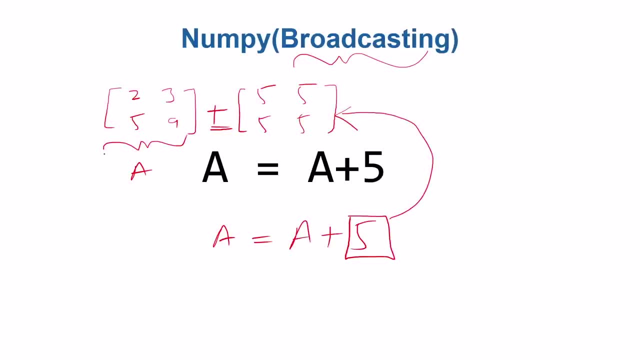 automatically broadcasted to match with the dimensions of its other operand and addition happens. you need not to do this explicitly. and this broadcasting is not just one scalar value. for example, if you have one variable, let's say a, is this and you want to add, for example, this particular column, let's say 1, 3.. You want to add this? 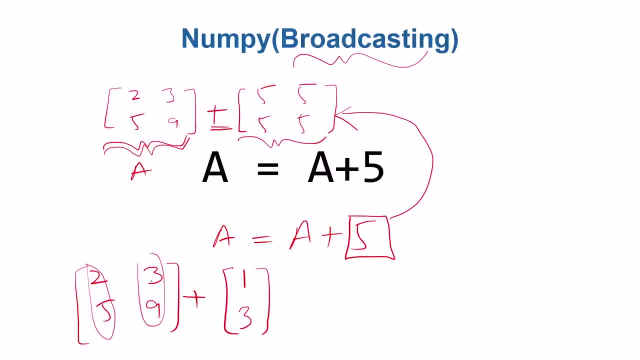 particular column, in the first column as well as in the second column. But then you need this 1, 3 to be copied again and make a bigger array, and then you do that. Well, broadcasting allows you. if you just write this as A plus 1, 3, it will be automatically broadcasted. 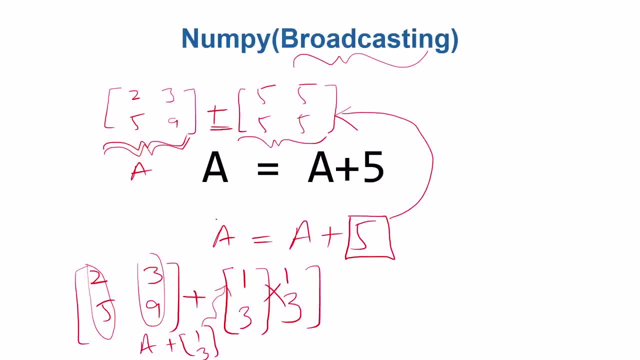 to match the size of the other operand Wherever the broadcasting is possible. there are certain rules to know when broadcasting is possible. It is not possible each and every time. For example, if you have this matrix- 2,, 3,, 9, and you have 4,, 2,, 1, let's say this matrix. 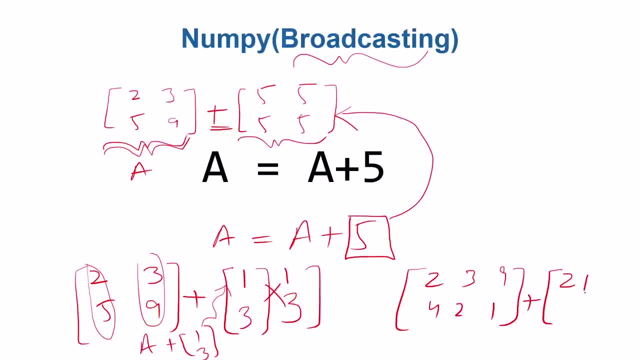 and you want, for example, 2, 1, and 6, 2,, for example. if you want to do that, the broadcasting may not happen, Because in this way, if I want to broadcast this structure, this structure should be. 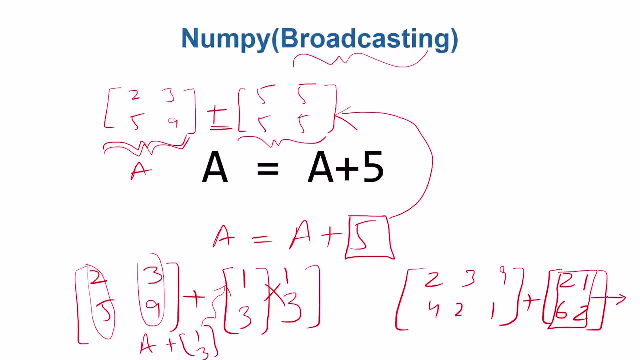 if this structure is broadcasted to in a horizontal way, the two columns will be added and the addition cannot happen. If it expands to a vertical way, still the addition cannot happen. So this here you will get an error because broadcasting cannot happen, But in 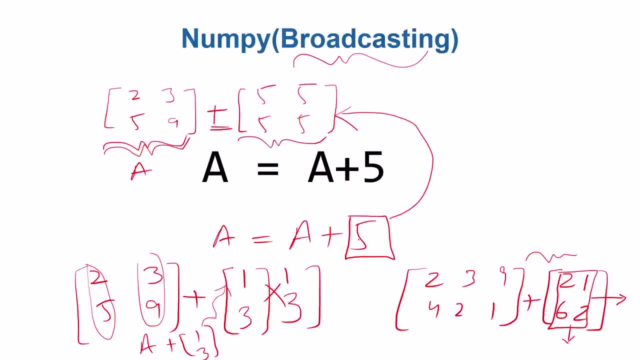 several cases when you want to add, for example, a scalar multiplier with a particular thing. wherever possible, this broadcasting is possible And broadcasting is just. I mean, it's just a feature of NumPy that allows you to not repeat to match the dimension of the other. 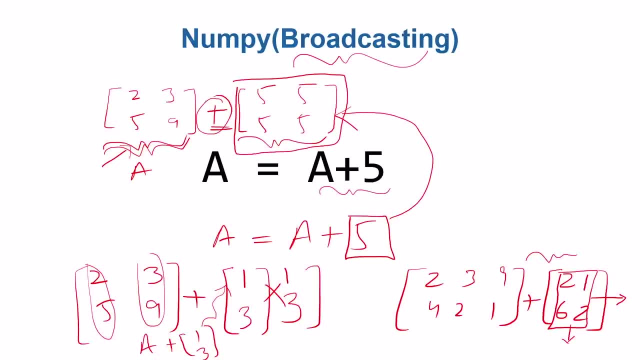 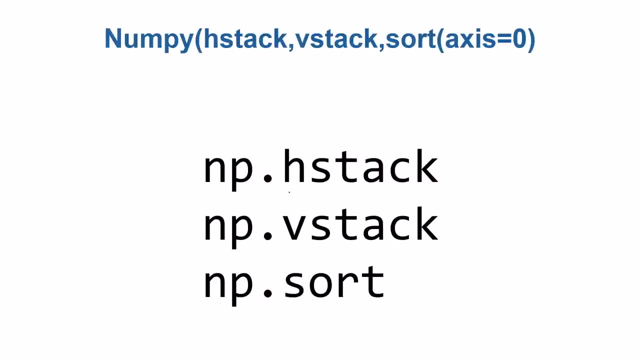 operand to apply a particular operator, It does it by itself, Great. Next, we see some more important functions to know. One is horizontal stack. That means if you want to concatenate two different array, two arrays that are that can be concatenated. 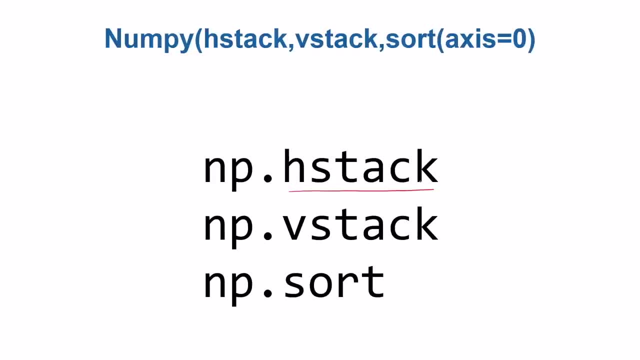 together horizontally you can call, you can call at stack function and that will concatenate the two arrays together and returns another array. Similarly, V stack is if you want to concatenate two arrays vertically, if they can be concatenated vertically, vertically. Similarly, there is another powerful function sort and there are a lot of other functions. 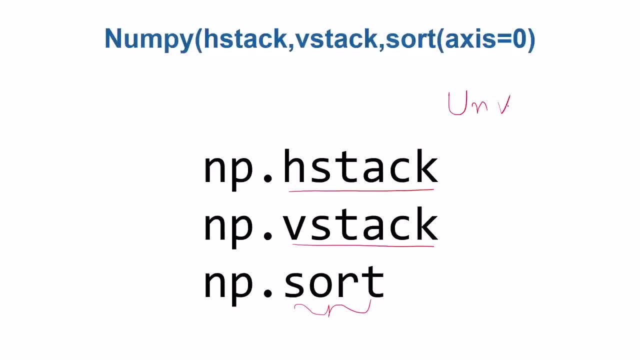 These kinds of functions. they are called universal functions and they are very, very, very powerful, Very, very, very powerful. It's a more vectorized code and the artificial one can do all these things really fast. Their implementation is vectorized. Vectorized means the implementation, the all loop kind of layer. 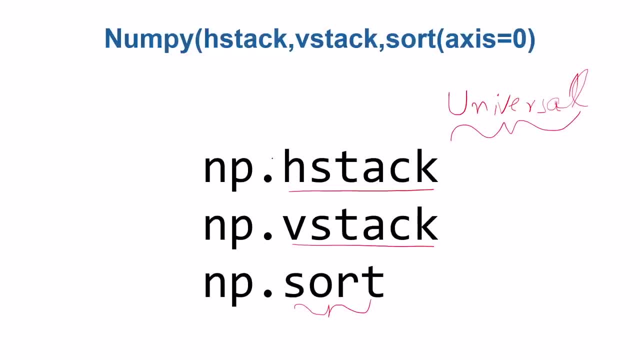 is the defer to at the compile-time, and the things are really faster when you do a vectorized code. So, having said that, it is always recommended to not use explicitly four-loops to achieve these kind of to achieve these kind of results whenever a universal function is available. 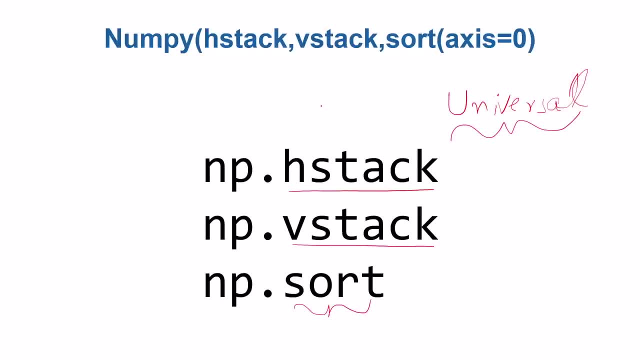 Use that, because the efficiency of that universal function will be very, very, very, very close way, way more than than whatever loop, loop or whatever function you will be writing other than the universal function. so, and, by the way, there is another function, concatenate as well, in which you 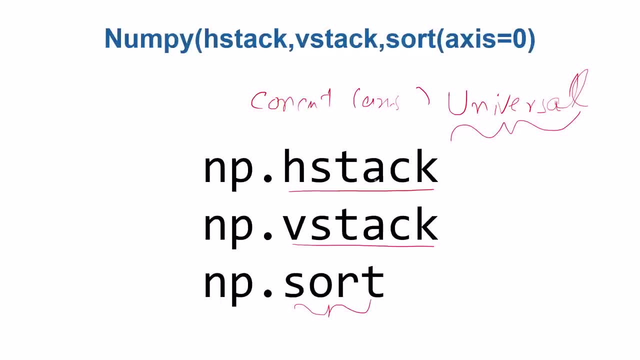 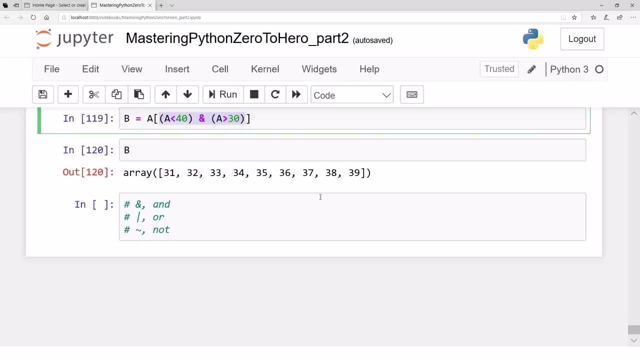 can specify, x says, and it will either act as horizontal stack or either act as vertical stack, depending upon whether the x's value is zero or one, whatever. so let's just get comfortable with these. these three functions just quickly in jupyter notebook and see an example of, let's say: 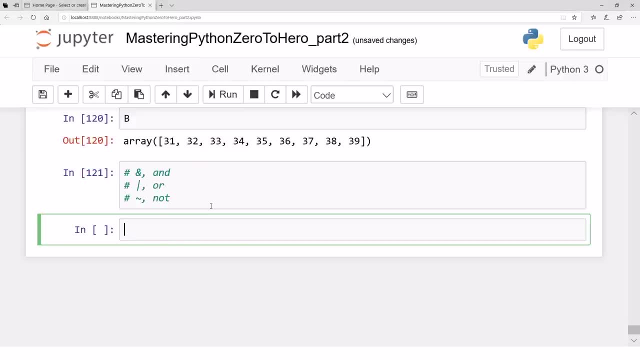 broadcasting as well. so let's say we have a function, let's say we have an array: a, a is, let's say, nprandomrand. let's say that is two by three, and then i just multiply this with ten- remember the this thing. and then we just nprand. 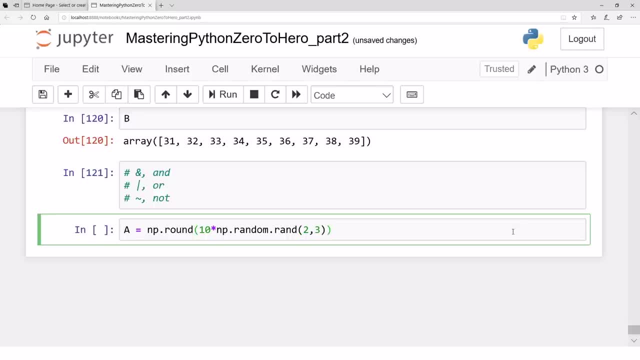 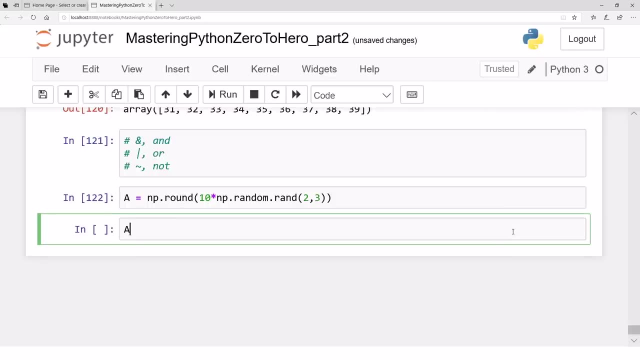 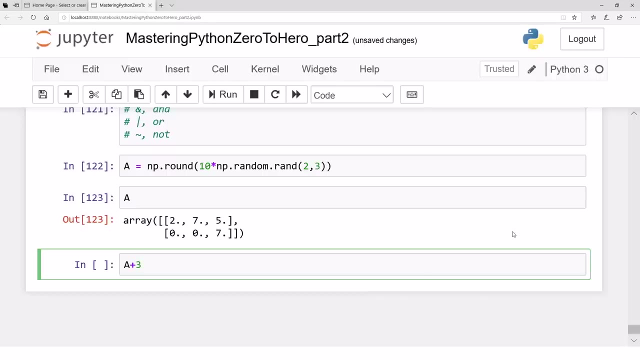 we just round everything so that it becomes, it becomes whole in this particular way. okay, that's a, let's say so, that's our a, that's the. now, if we say a plus three, three will be added everywhere in a, and that happens through broadcasting. well, if we, if we do, for example, a plus, for example np. 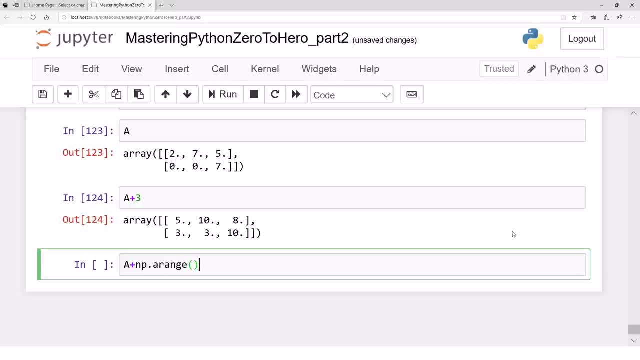 dot a plus, for example, np dot and and u just 17, seven a, then we have two x, say ip b matrix. if you do that, then still what will happen is just apply the phrastic just to show that this should happen first. which, what happening is there really? there will be a column that 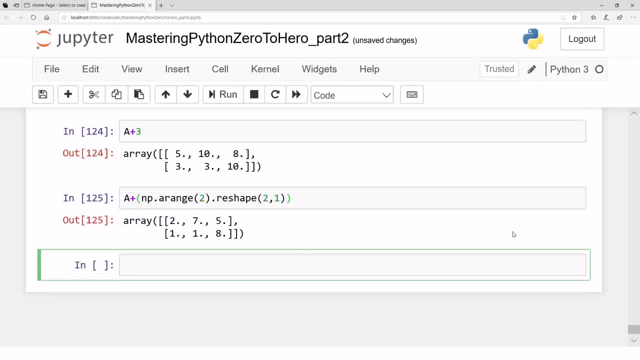 will be added to every column a and that have auzkeed真的 and zit will be happened through through the broadcasting. so broadcasting, is that powerful. next, let's see the stack. so let's say this is a. let's say we have B, that's another array. let's say NP, dot, random, dot, Rand. let's say that new array. 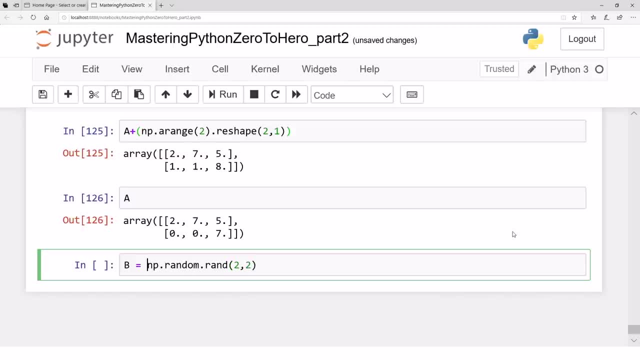 is 2 by 2 and again let's say it is multiplied by 10 and NP dot round just to avoid the decimal points, that's, this is B. now a is a 2 by 3 array. B is a 2 by 2 array. if I just concatenate them horizontally, I will get another ray. 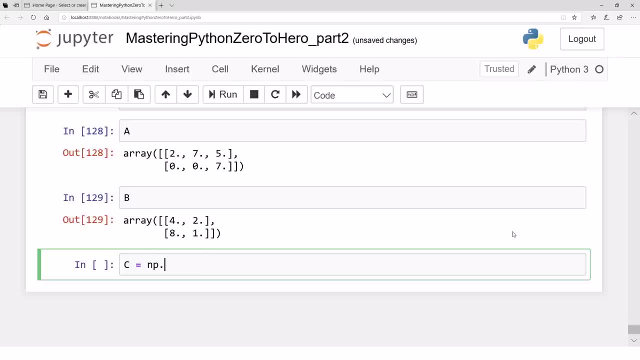 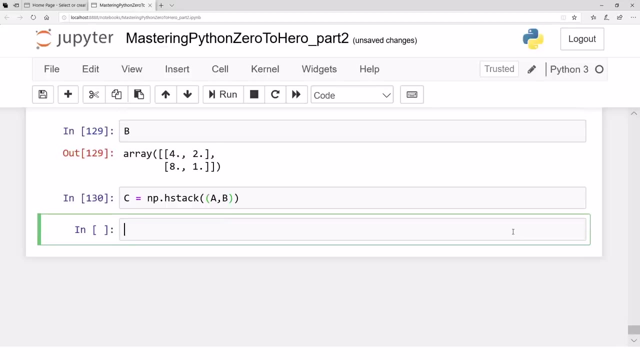 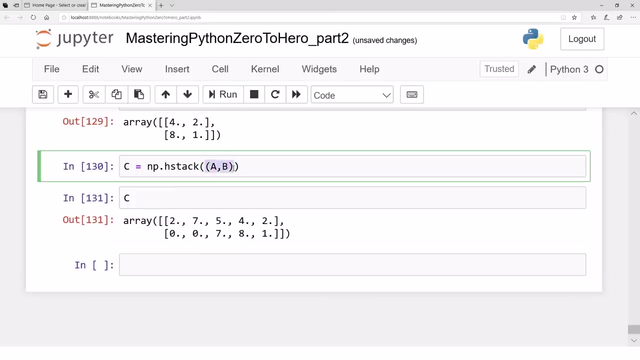 which will be 2 by 5. so C equals NP, dot at stack, horizontal stack at stack, and I will call these a and B. one thing that you need to know is if you, if you want to call this X stack, horizontal stack or vertical stack, these arguments a and B that you want to concatenate you. 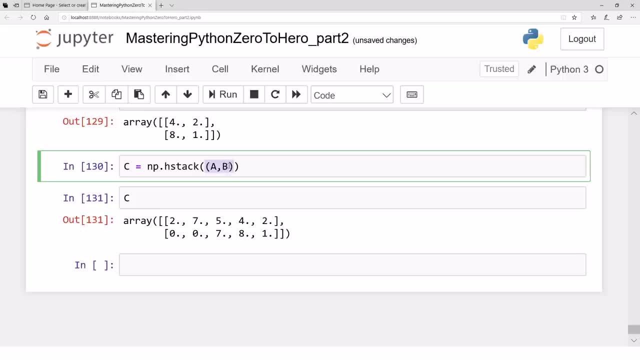 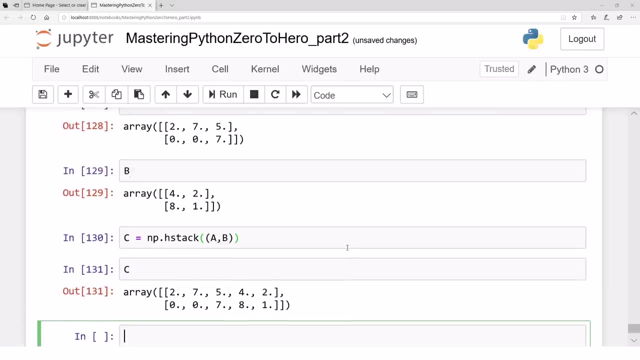 have to give them in a tuple, or you may, you may want to give several values to concatenate together. maybe you have, maybe you have- 10 matrices to concatenate together horizontally. you have to give all these as a tuple inside. okay, right now. similarly, we can do a vertical stack if we want. I mean one. 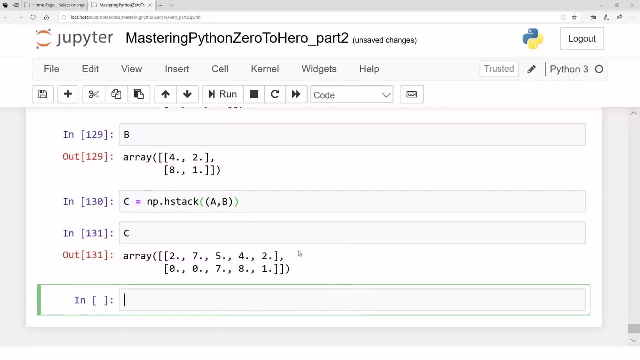 i mean one on top of the other and we can call again carrying it function as well, if we want. third is a sort function. uh, for example, if we want um, if you want to use np dot, let's say a. is np dot random dot permutation? let's say np dot arrange, let's say the 10 values. 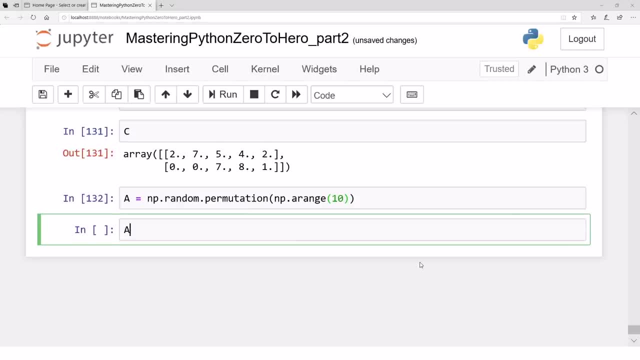 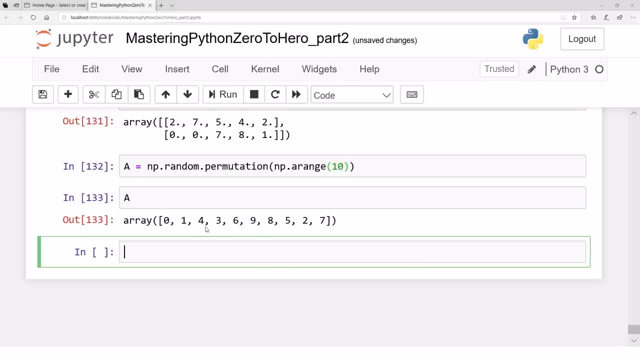 let's say that's our a. let's say this is a and we want to sort this array. um, oh, this is already sorted. why, um, is it sorted? no, it is not sorted. uh, one, fourth, it is not sorted. yeah, let's say we want to sort it, a dot sort. one way of doing that is just call a dot sort and you are done. 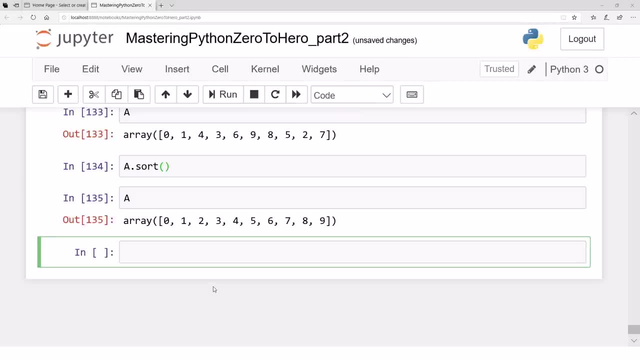 that's the value of a another way, which is, uh, sometimes more readable, although exactly the same, is to use a universal function using NP dot, that thing. that also is the same thing. now, sort by default. sorts in ascending order. if you want to sort in descending order, then 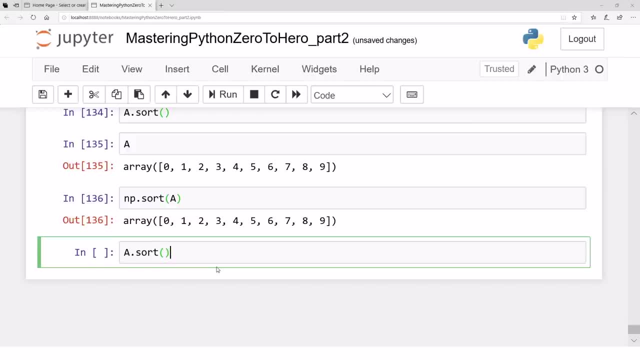 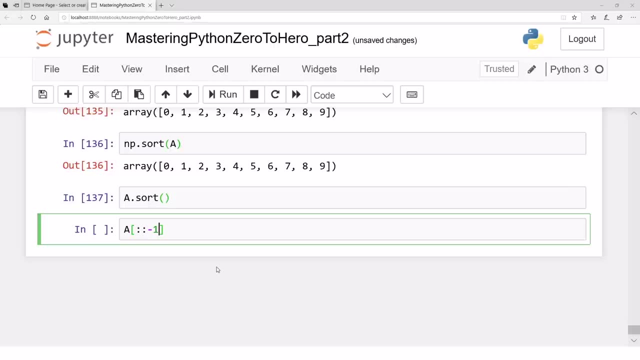 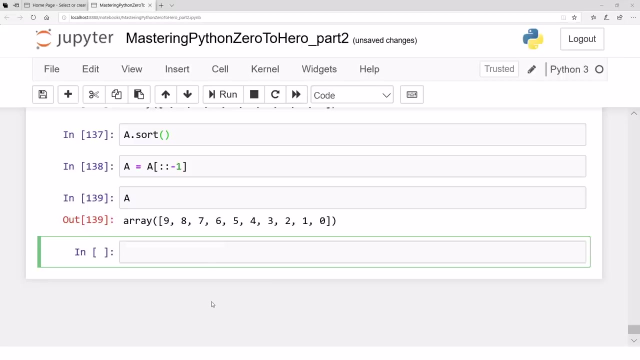 what you can do is you can sort a dot sort, for example, you do that in ascending order. then what you do is you just reverse it minus one and just copy that in a again. now a will be sorted. Wow, sorted in descending order. yeah, great, one more. just just just just to give you one more flavor if you create an array. 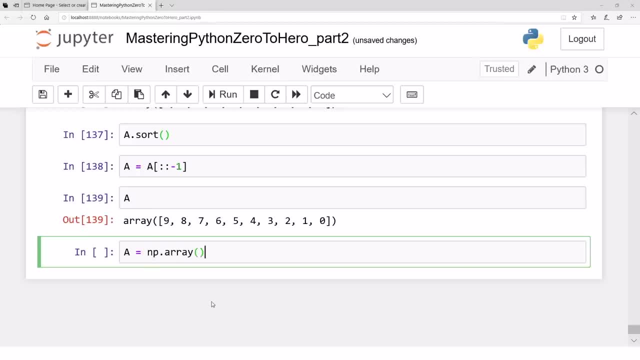 for example NP, dot, array of strings, for example ABC, and another string is: how are you and and and and maybe we have another string, you seven, eight, five and maybe we have another string, 13, er. let's say that's a string that is possible as long as all. 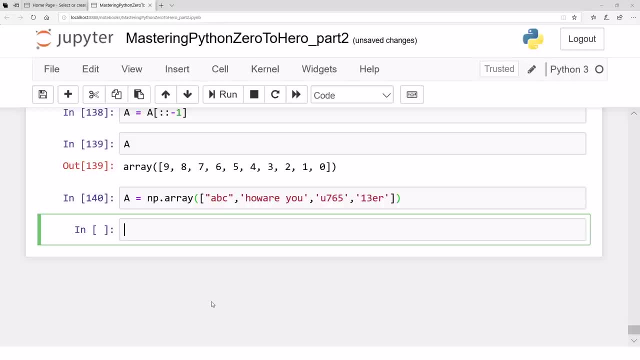 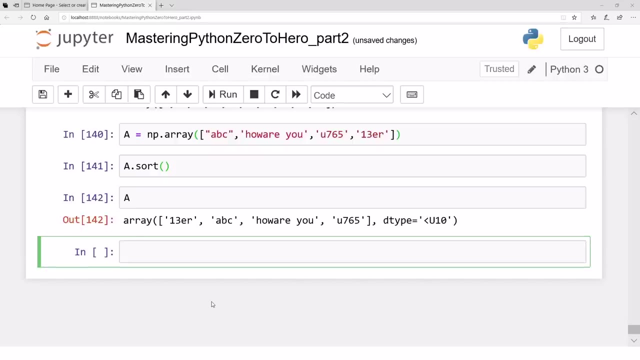 the objects have same type, you can create an NP array. now you might be wondering what will do this sort function on a, because these are all strings. well, the answer is: it will sort the strings according to the alphabetic order. whatever the alphabetic order is, whatever string according to the alphabetic order should become first. 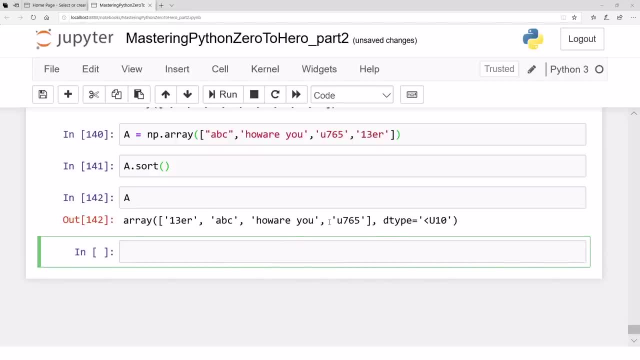 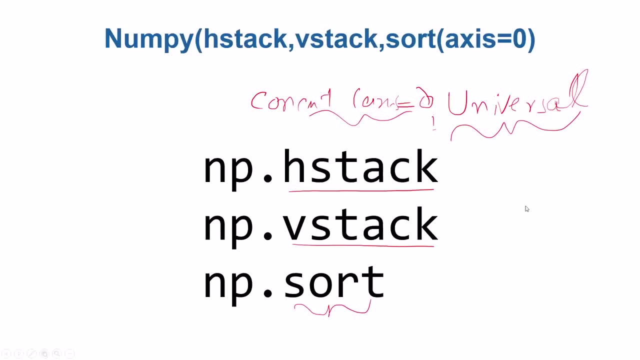 that will become first and the other strings they will. they will just join. yeah so, yeah. so that's about something that is not. that is not the nummatic value. ok, great, there is a few more things to come about. number year a, and then we will be moving towards bandas library that is built on top of number. 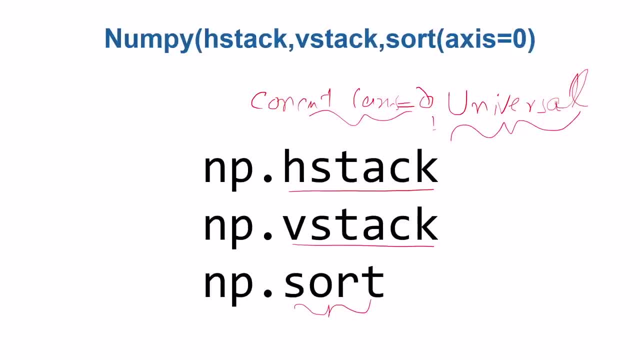 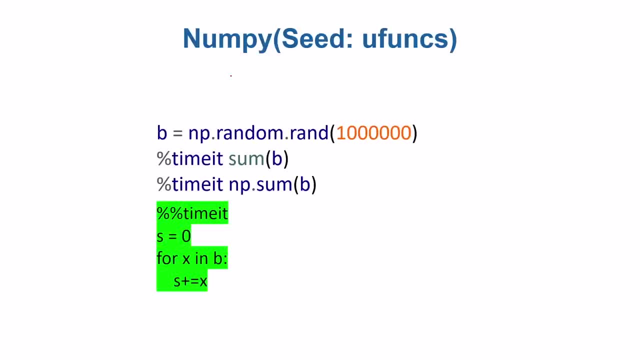 a for better processing of theta. hope to see you in the next class. thank you for watching you video. okay, in the last video, um, we saw horizontal concatenation, vertical concatenation, sort function. we also saw some broadcasting and stuff like so, um, universal functions, it should be speed here. 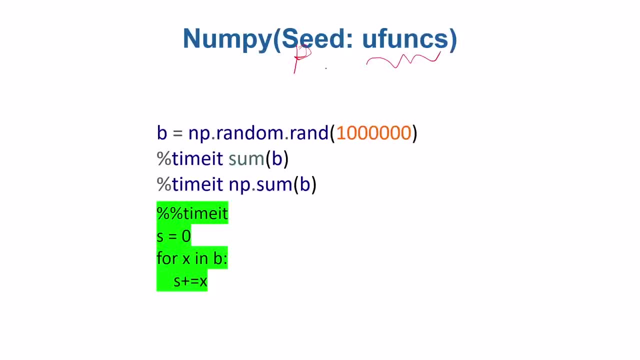 sorry, it should be speed. speed. universal functions are really, really speedy. i i always i'm talking about numpy. whenever i start numpy, i said it is fast, it is fast, it is fast. i never show you how fast that is, so let me give you an example. let me, let me just create a numpy array with a lot. 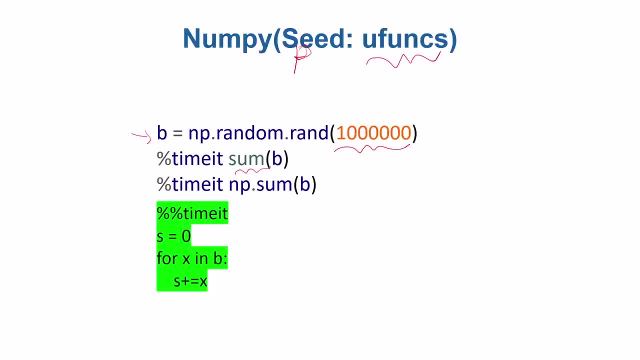 of numbers and then just apply an ordinary function. let's say i want to add all the numbers in this array b. let's apply an ordinary function that is not in numpy. and then let's use a universal function- dot, sum- and see how speed difference is there if, for example, we apply a. apply a universal. 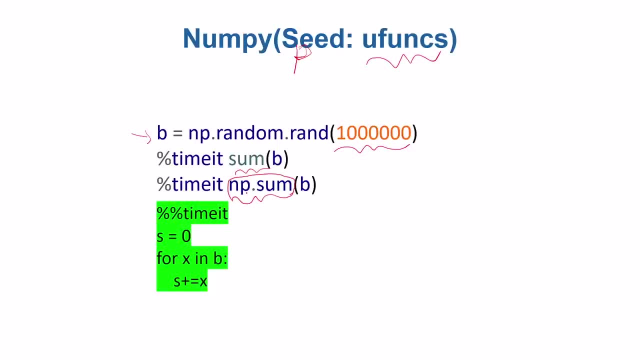 function to achieve a particular task. how speedy that is universal function is because the back price implementation, as i told you, is much faster. how faster? let's check that out in new jupiter notebook. that's a magic command time it. that will tell us how much time this particular task has has taken. and if you run this command, it will. it will. 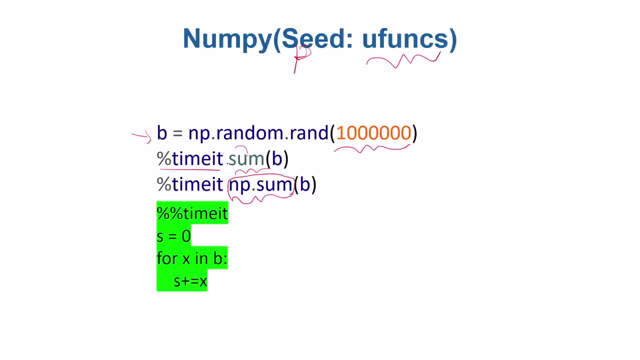 call this function again and again, several times, and then we'll report an average value. that will be much more stable than just calling once. um, after that we will also. we will also write our own sum function using loop, and we will see whether that is even closer to a universal function- speed or not. 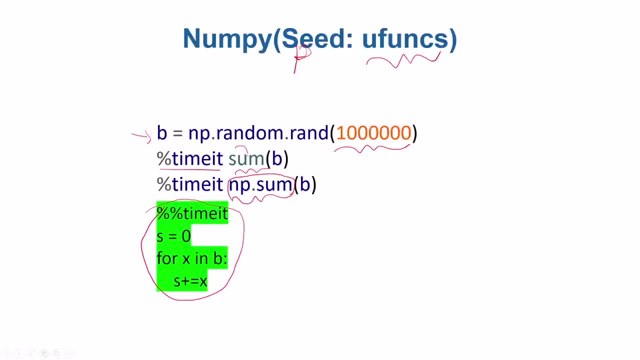 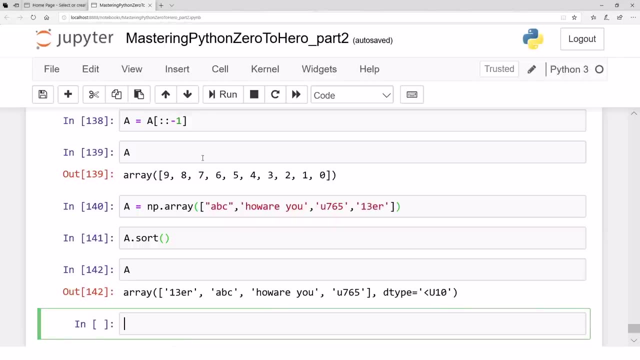 let us just check the speed of universal functions. that will give you a look and feel of how much numpy implementation is faster. so let's say we have an array, let's say b, np, dot, random, dot, rand, and let's say that array is huge, really huge. that's it. that's the case. now what we do is 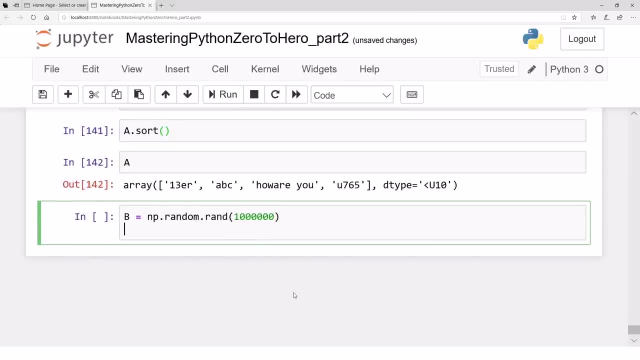 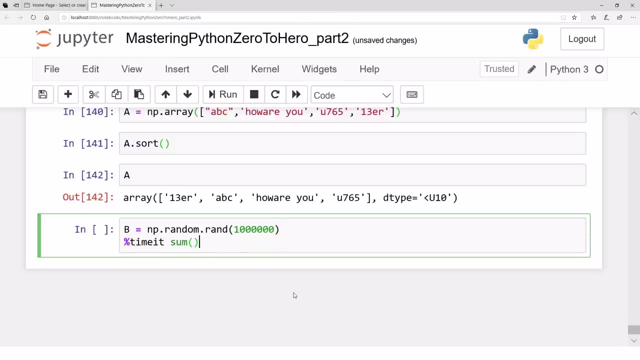 we. let's say we, we call a function sum. so let's say we call a function sum, that's a built-in function in numpy. that's a built-in function. that's a built-in function in python, not a numpy function. and then let's say we do the same task using numpy universal function, np, dot sum. 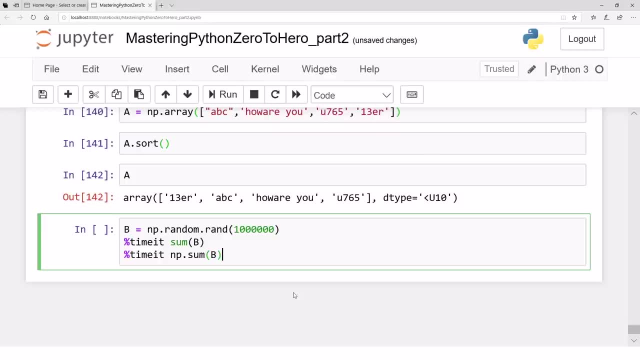 that's the same as np dot sum is the same as: uh, if we, if we write, for example, b dot sum. so whether you write b dot sum or you use np dot sum and be passed and passed as an argument, both these things are roughly the same. so let's run it. it will take a while, it will take a time. 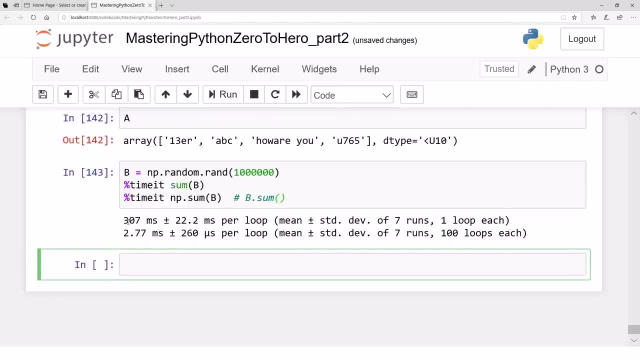 because, uh, okay, the sum function takes 307 milliseconds. that is not a universal function in numpy, that's python function. uh, that is not written in numpy, that is not a web price code, nothing. it takes three zero seven milliseconds to perform, to take the sum of the sum function. 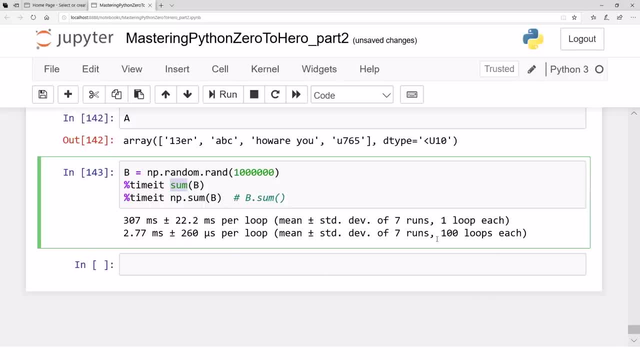 the elements of this array, and it does that by applying seven runs and then seven loops. however, the universal function takes just around three milliseconds. I mean two minutes two point seven milliseconds. how will? how are you going to compare this three zero seven with three? how much faster you are. 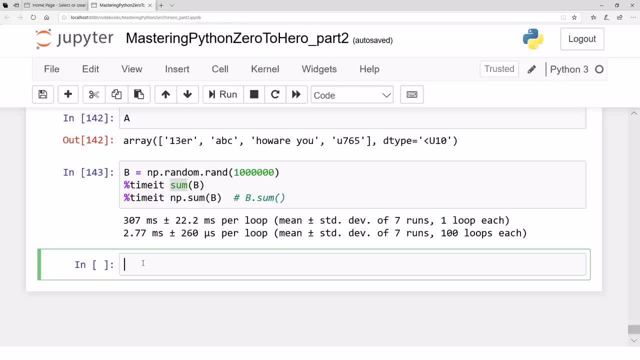 around around a hundred times you're faster. I mean, yeah, I mean this numpy is literally faster, numpy, the universal function, that are faster. maybe you attempt to know that. okay, there's some function might be too slow. let me write my own function to do that. let me define my sum and my sum just take an argument. 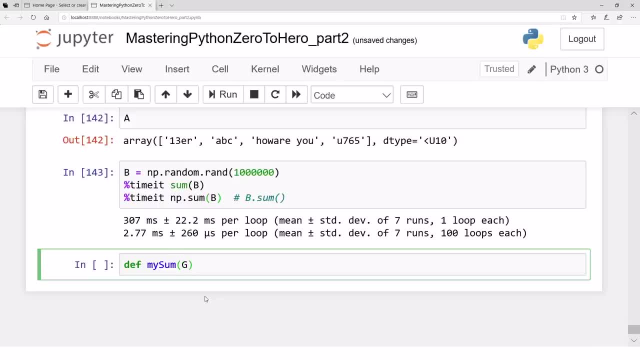 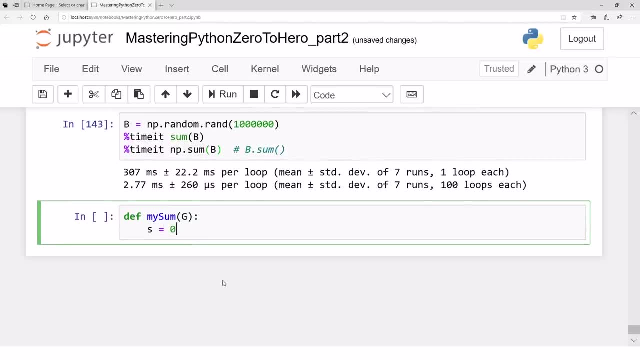 let's say something. let's say G, and what it does is for. let's say, s equals 0. what it does is for X in G, s plus equals to X, X plus equals to X, and then just return s. let's say that's your function. let's say you think that this is really a great function. 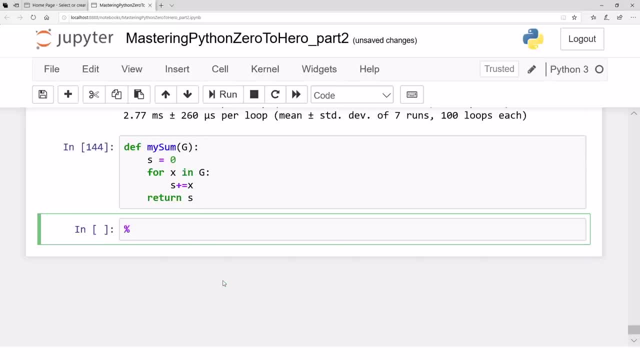 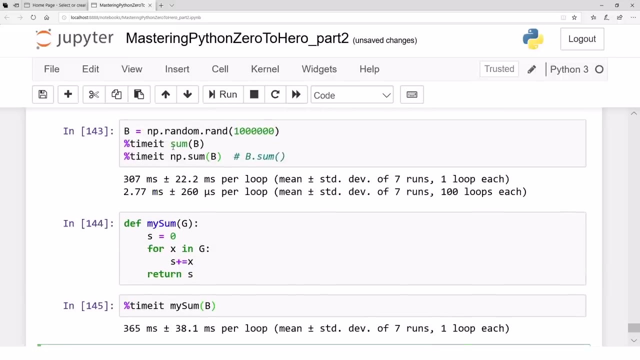 let's do that. okay, let's compute the time for this time it my son, and let's pass the ray B and see how faster this is. this is roughly the same as you're calling the sum function, but this NP, dot sum or the universal function is very. 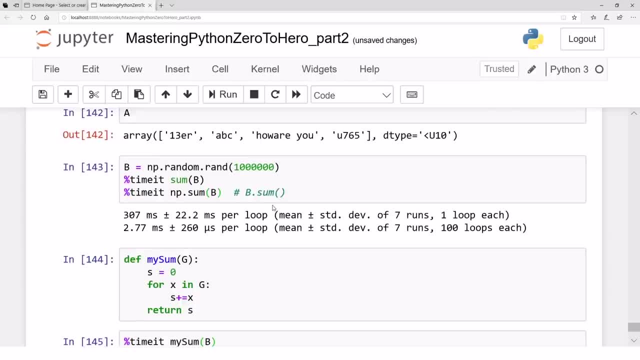 very faster, very faster. so use universal functions, avoid for loops, avoid your own functions. if the same task has been a, can be achieved through universal functions, whenever possible, avoid loops. so, for example, let's say you have a large array of functions and you're going to multiply them with a large number, but those functions will be. 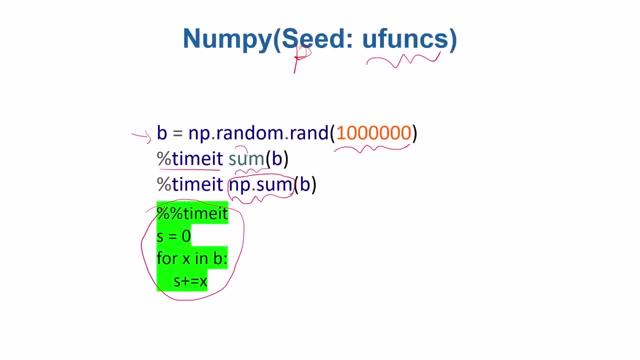 harder to comply with, then you're gonna multiply them with a few more properties, more than you would like to do, and so that's where that's the recommendation, and this is a useful one. when you are working with numpy. that's a serious suggestion. follow that, because the the universal function. 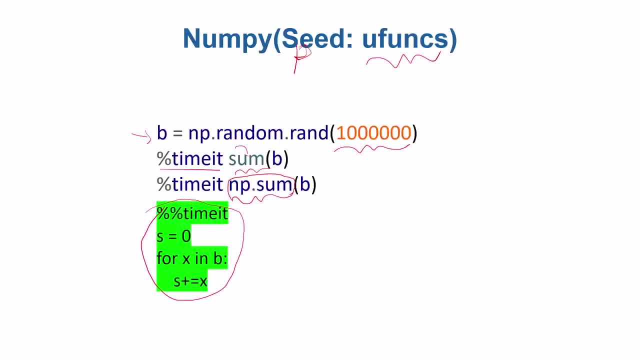 written in numpy. they follow the vectorized code. all the interpreted a NumPy. but I have told you some basics of NumPy and we end the NumPy here and from the next video we will be moving towards a very, very fancy and beautiful kind of package called pandas to handle. 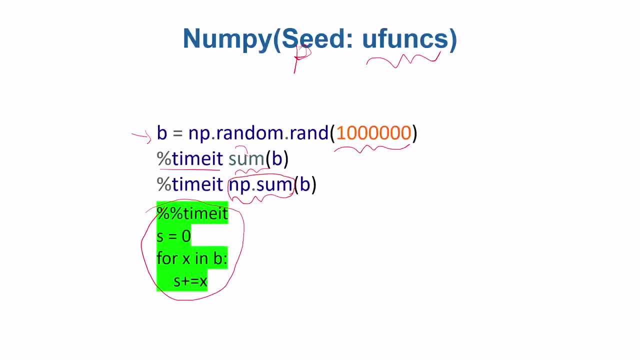 data and, by the way, the pandas library, the pandas package completely, is built on top of NumPy. everything that is there in pandas is built inside is built on top of NumPy. so all the indexing and all kind of stuff, slicing and speed, all is there in pandas. that is due to the NumPy. so we will see. 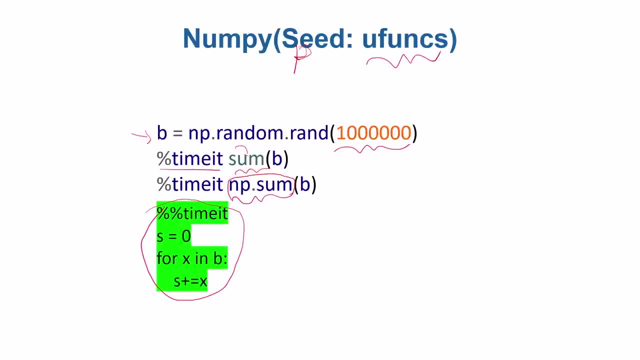 one more package after pandas, which is matplotlib for for plotting afterwards, and we'll do a project at the end using scikit-learn as well, just to wrap up all these things together. but for now I'm ending NumPy here, and in the next video we will start pandas. hope to see you in the next video. 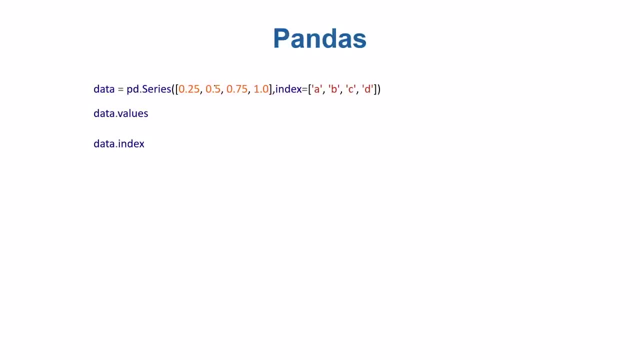 okay, welcome to pandas, a data science package that is very, very powerful of handling data, manipulating data and used a lot in data munging and data cleaning and data pre-processing and whatnot. this pandas, basically, is built on top of NumPy, so most of the features of NumPy is also available. 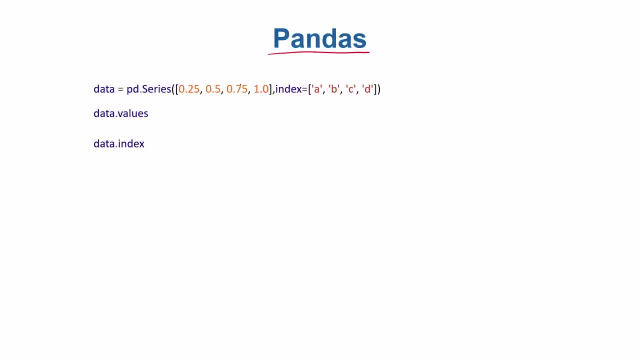 in pandas. let's let's dive in. I mean this, pandas is a very, very fancy library, very, very fancy package that you can handle very large amounts of data in csv files or in excel files. wherever the data is located, the missing entries are there. you can handle all the data. you can manipulate all the data. you can. 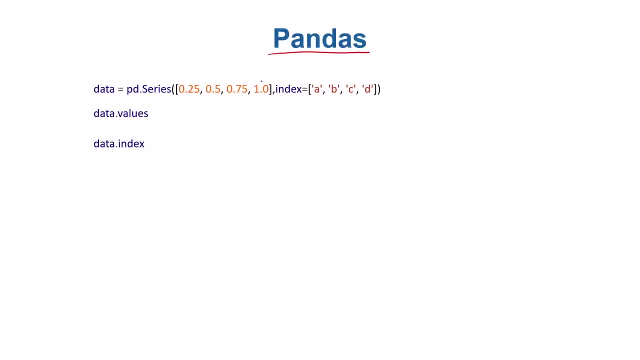 prepare all the data in just a few lines of codes using this pandas package. so let's just start pandas package. there are two most important objects of pandas. one is series, another is data frame. that we will see later on. there is one more index, but the most important. 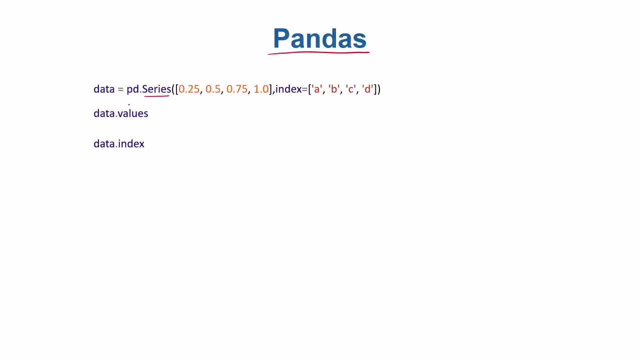 one is, or the useful one is, the series and data frame. so let's just define. first of all, you need to import pandas package, import pandas and you can rename this as pd, that's a. that's the most popular renaming, although you can rename it any, and then you just say, okay, pd dot series, and then 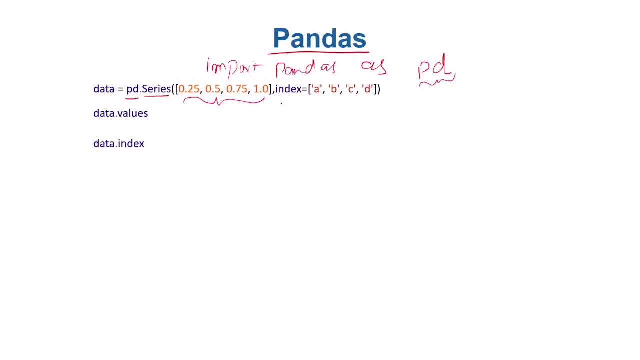 just like a NumPy array, you pass the data that you want and you can create your own indices. for example like: just like dictionary: this a is a key value, this a is a key or index for this 0.25, this b is index for 0.5, c is index for 0.75 and d is index for 1. so you can, you can, you can supply. 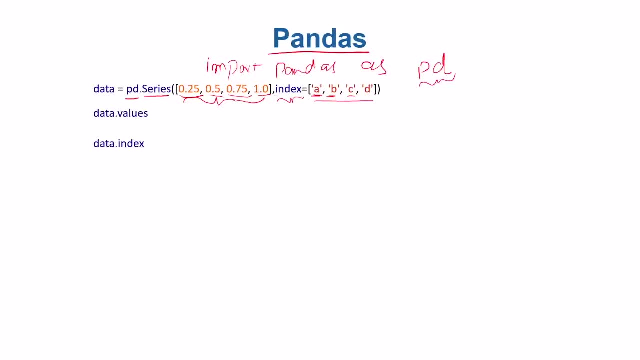 your explicit indices as well, if you do not supply the indices. the default indices are 0, 1, 2 and 3, but you can define your own own indices in the way you want to do it. so let's just start with that first. let's just find the index information and, as you can see, I have d value over here now. 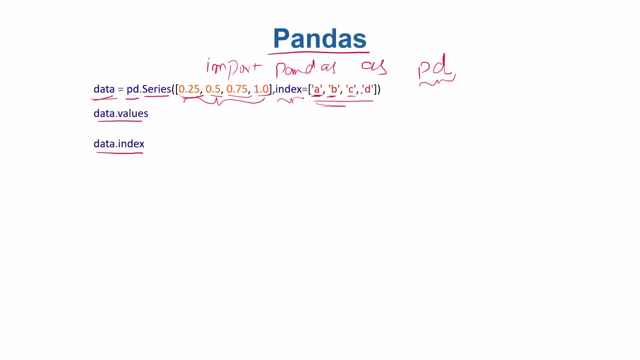 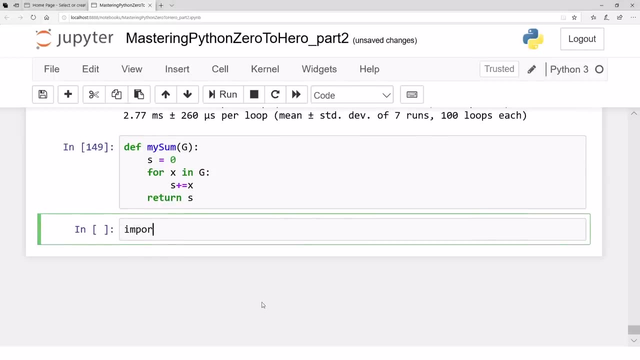 we will call the index the index also to show that what is the index that you want? now, once this data object is created, you can call the data values and you will find out the values. you can call data dot index and you will find out the indices. let's see in the jupyter notebook: just 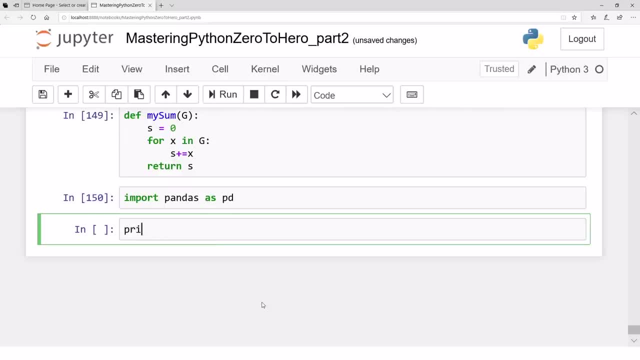 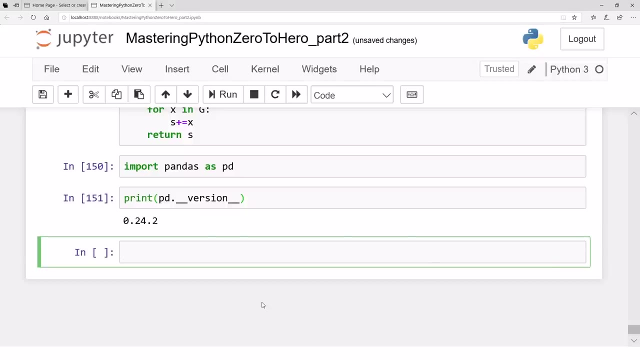 to get comfortable with pandas. first of all, import pandas as pd maybe or something else pdvarian. the varian of pandas we are working in right now is 0.2, 4.2, fine, great. So let's create a data or whatever variable. let's say a as pdseries, pzseries and 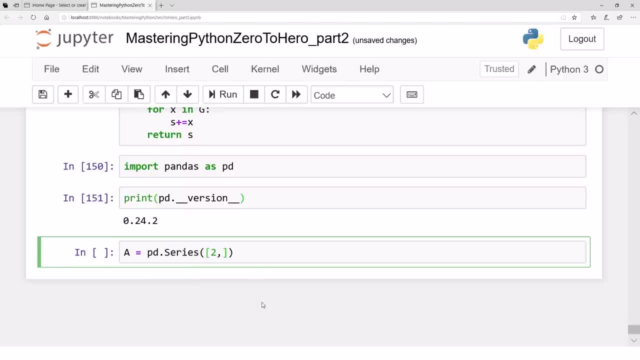 there we just give a list of some values: 2,, 3,, 4,, 5, let's say these are the values And then we can give index as another list. let's say the indices are a. maybe the indices. 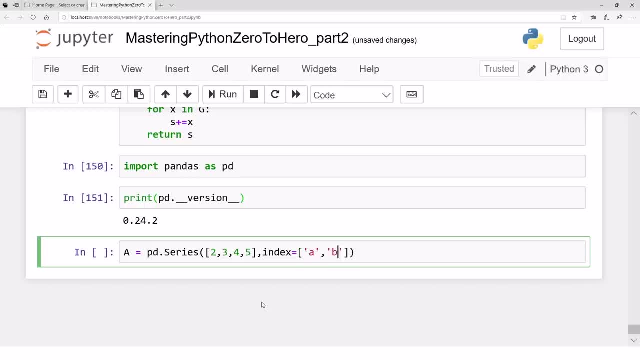 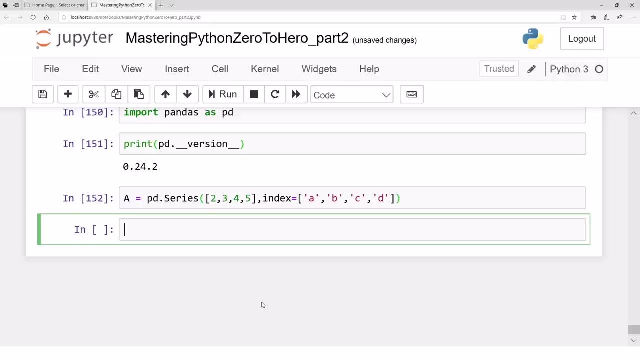 need not to be strings anything: a, b, c and let's say, the index of 5 is, let's say, d. So now the series object or the pandas object, series, is created. Series basically handles one dimensional arrays. Later on we will see data frame handles multidimensional. 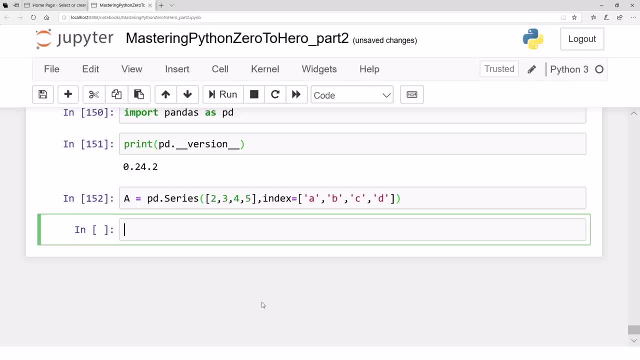 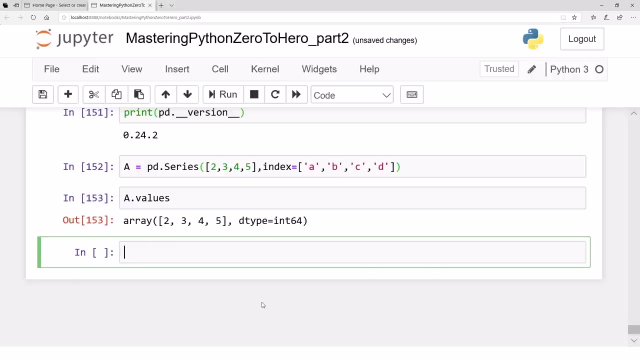 I mean more than one dimensions, normally, typically two dimensional arrays, but okay, avalues. So let's call the values values, and you will get all the values inside the series And, by the way, this values array that you get, let's check what's the type of that array. 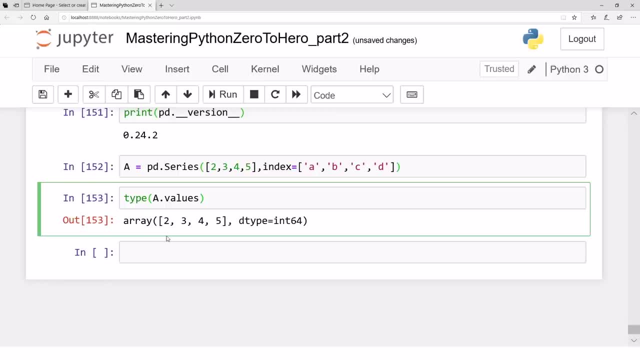 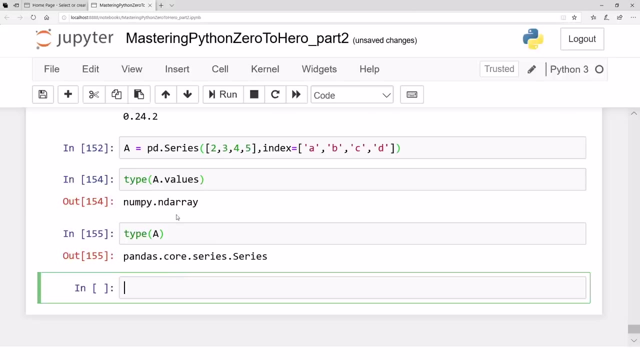 What's type of that array: avalues. What is that thing? That's a NumPy array, wow. And what's the type of a itself? That will be a pandas object, great. So everything inside pandas, the NumPy is playing all the role inside pandas- great. 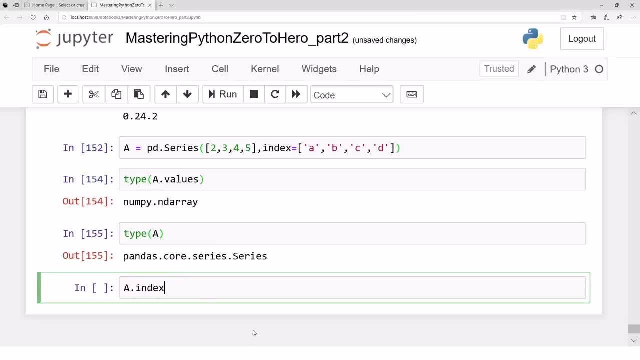 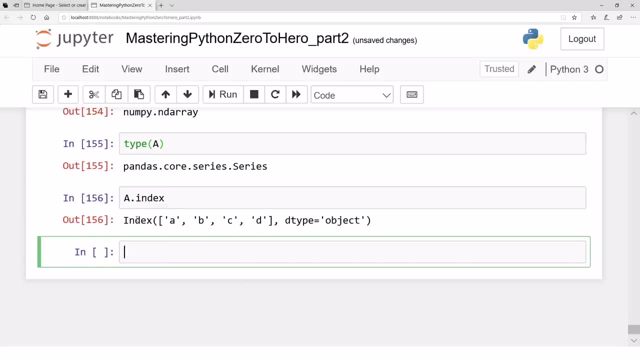 So now let's check the index. aindex, that's also a NumPy. that's also an array of index type. That's a different. Actually, index is also an object in pandas. That's an index type object with these kind of indices. 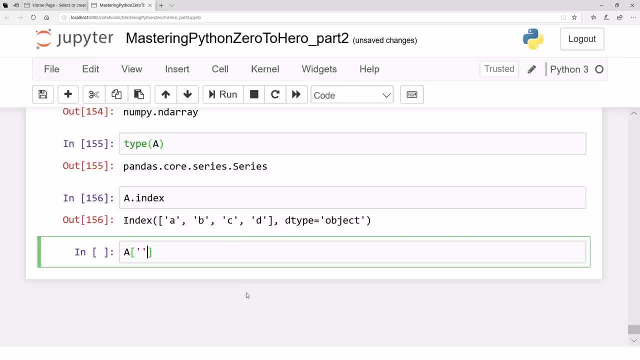 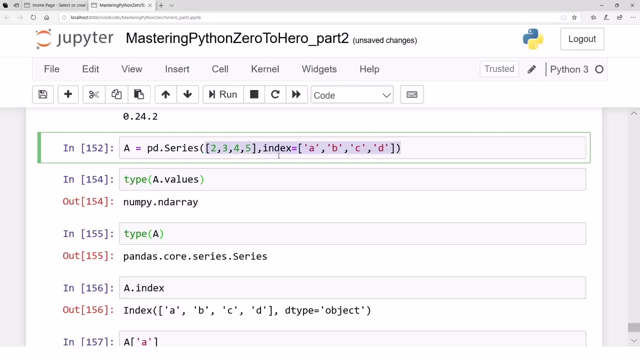 We can access, for example, this, a, just like we are working with dictionary, For example, a of a that returns a value. We can change the values, we can add different, we can add more key value pairs. So just think like these, just think this data, just like the dictionary object. that. 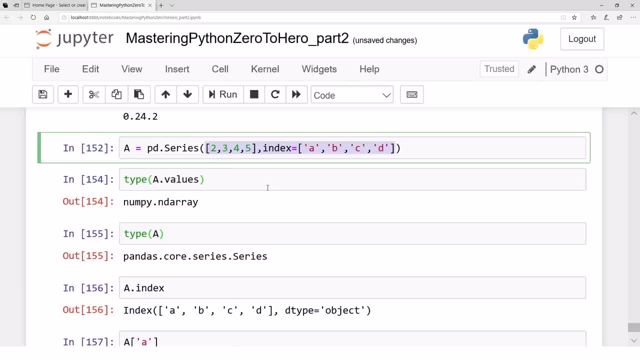 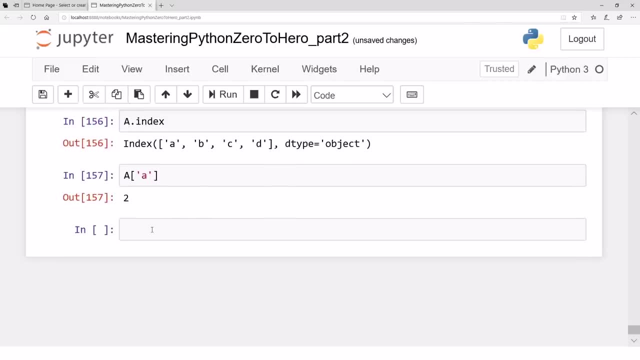 we saw. These are the keys and these are the values, And this is what we're looking for. Okay, So this is one very good way of remembering what the series does and manipulating series the way we want. Okay, One we can access a like this: 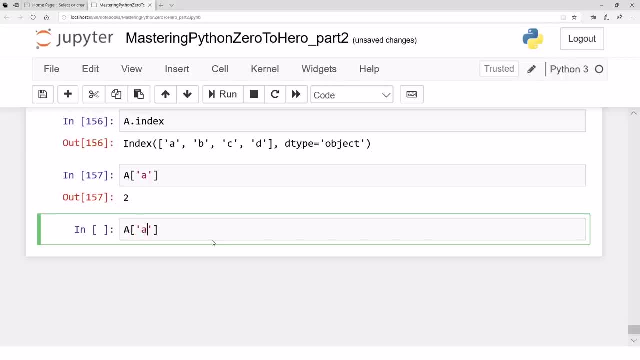 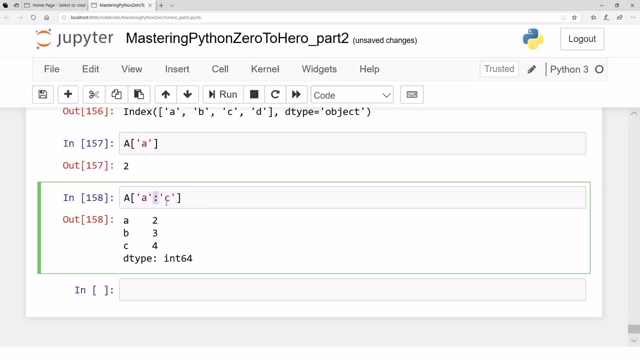 We also can do slicing. Let's say we want to access from a to. let's say c. Let's say we want to access all these. One difference is when you access like this in the normal slicing using implicit indices, for example One, two, three or zero, the final index is not included. 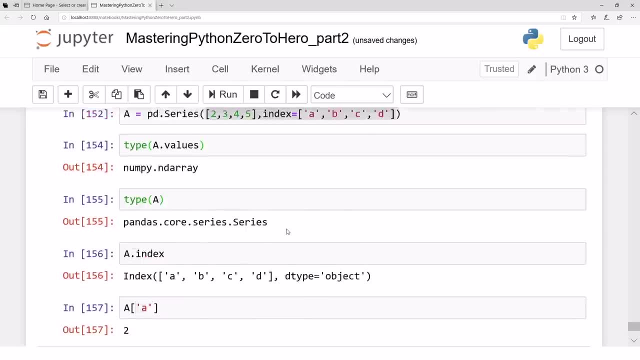 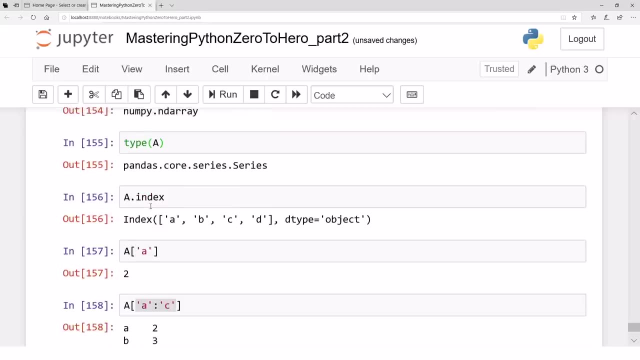 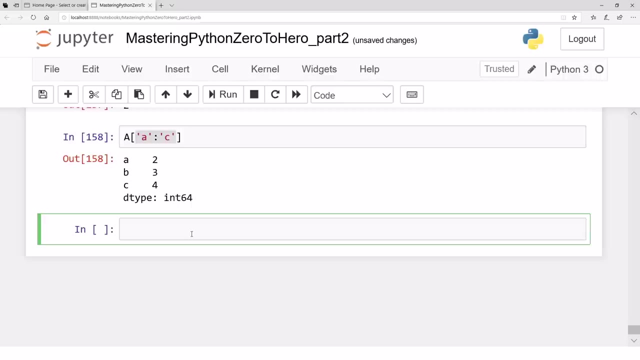 But if you access like so, using explicit indices that are there, the final index is also included. So that is one more fancy way of indexing, using, in this, Pandas. Okay, great, That's a series object. By the way, we can create a series object by first creating a dictionary. 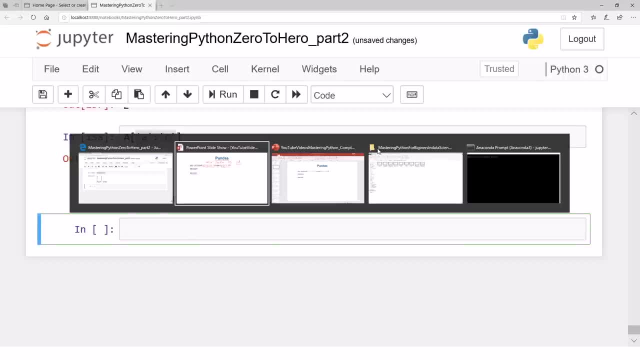 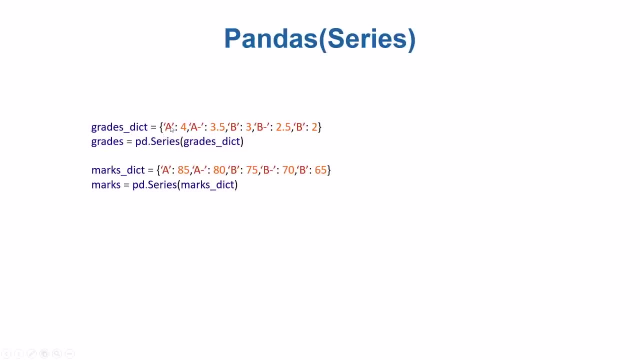 For example, let's go back to our slides and see this example. Let's create a dictionary, for example, of grades. Let's say we have a lot of students with grade A, grade A-, grade B, grade B- and let's 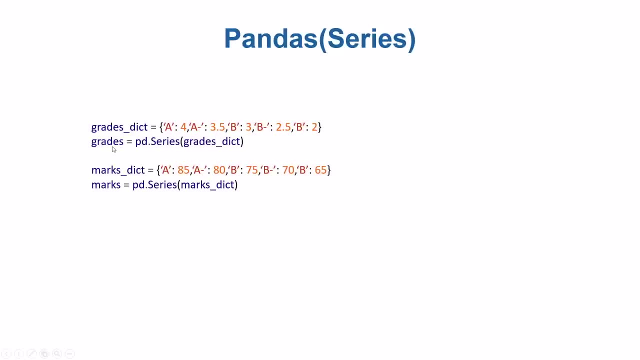 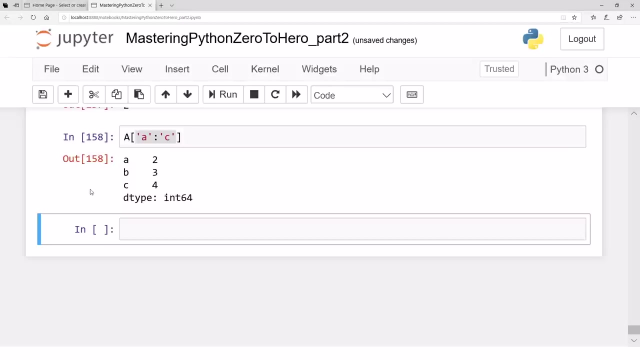 create that dictionary, Then we can just create a series object or Pandas object. by just passing this dictionary inside We can make another dictionary, for example, and we can make another series object. So one way of defining the series object is just to pass the data. 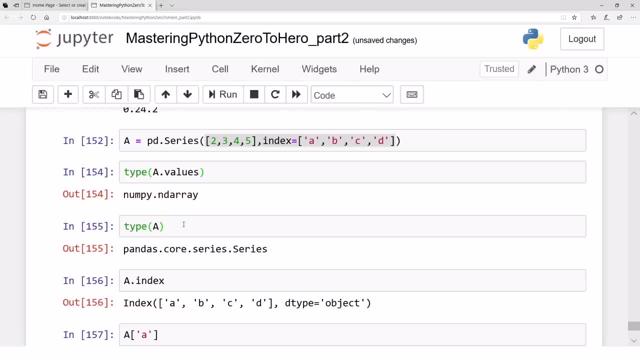 Okay, So that's one way of defining the series object. Another way is to just pass the data as well as index. Another way is to just first create the dictionary and just pass the dictionary variable inside and the series object will be created. 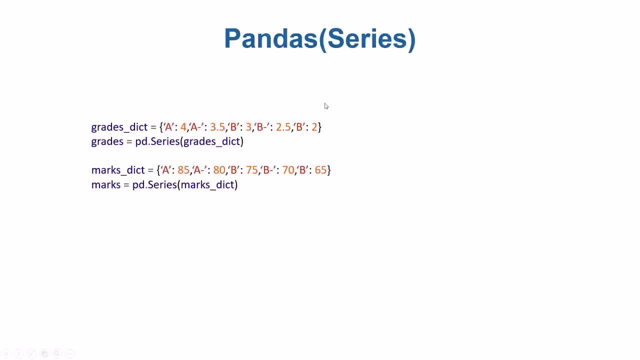 Okay, That was just the introduction to series. We will move on and see more features of Pandas as we explore it more and more in the upcoming videos. Hope to see you in the next video. Okay, Let's say we have two different dictionaries. 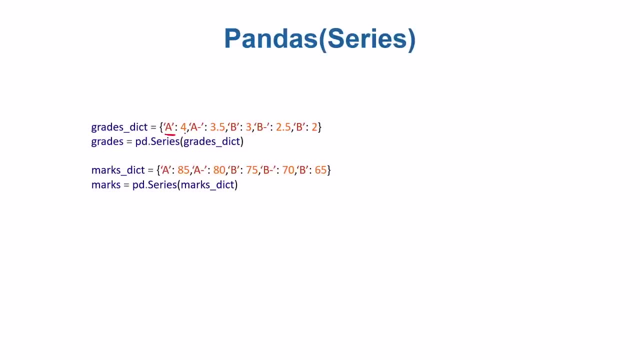 Let's say we have a lot of students and the A grade is defined to be four And the A- grade defined to be 3.5.. The B grade has a number three. The B- grade has a number of a numeric value that is 2.5. 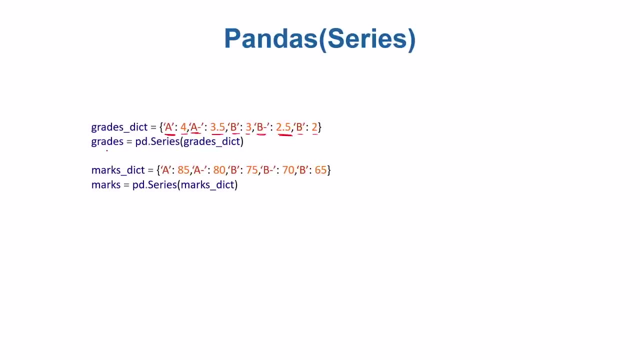 And similarly B grade has a numeric value, that's a two, And then we create just a series object using this dictionary, Let's say, rather than just the numeric values, as GPS or something like so. let's say, A grade also is defined at 85 marks in total. 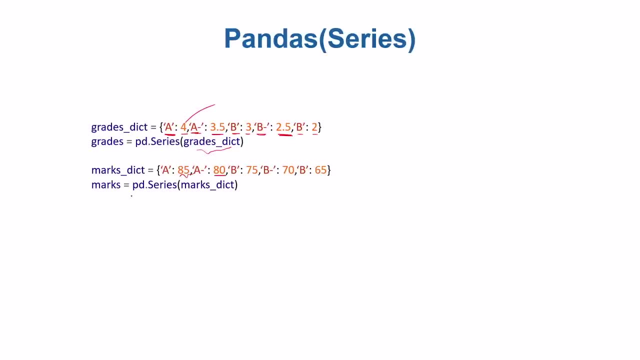 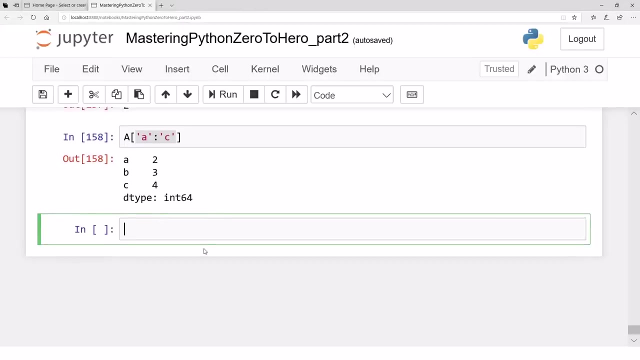 A- grade is defined at 80 marks in total. And then we create another series object, let's say named with marks, using these pdseries. So let's go to Jupyter Notebook and just play a little with these dictionaries and build the series object. 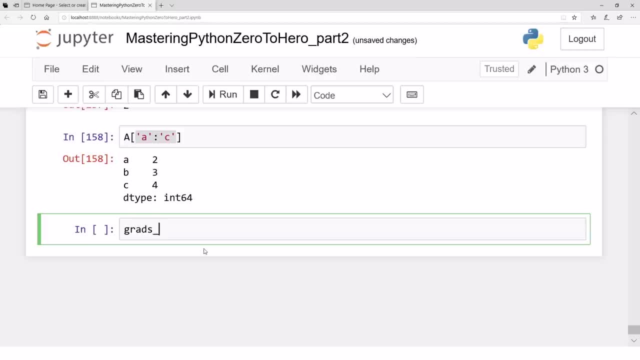 Let's say marks or let's say grades, dictionary equals. let's say A grade has number value four or GPA value four. Let's say, let's say we have a B grade with GPA value. let's say B is, let's say, 3.5.. 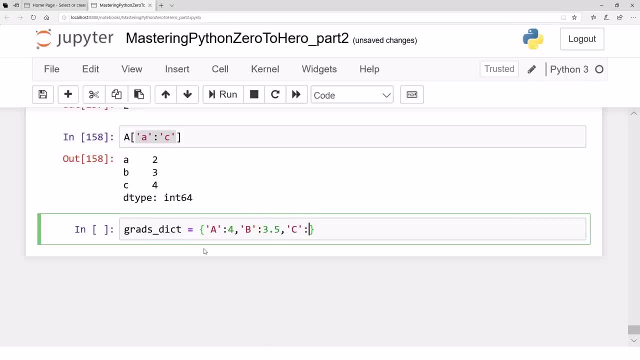 Let's say we have C grade with GPA value, let's say three. And let's say, finally, we have D grade with GPA value, let's say 2.5.. Let's say: that's dictionary, Okay. What we do now is we create grades series. 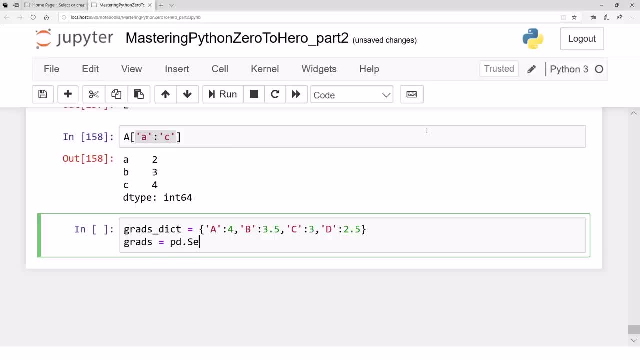 Let's say using pdseries, and just pass this grades underscore. dict Now this capital A, capital B, capital C and capital D: they will act as indices, and this four, 3.5, three and 2.5, they will act like values. 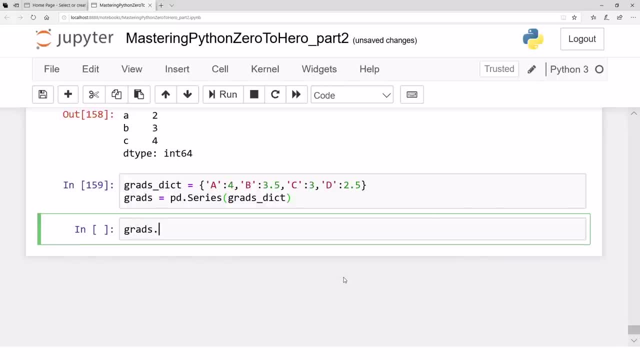 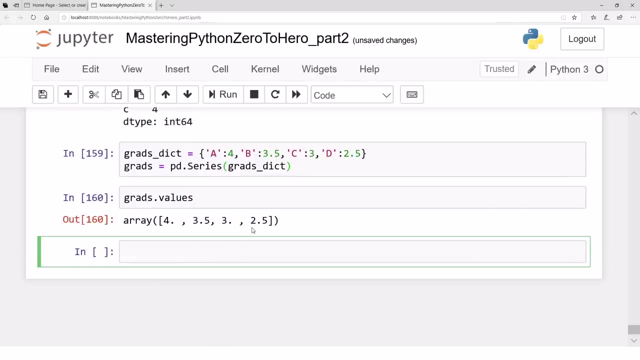 So, for example, if we call that and just now call grades dot, grade dot values, So we will get, for example: well, what is that that? just values. let's say, we get this grades dot values and we get all the values that are available. 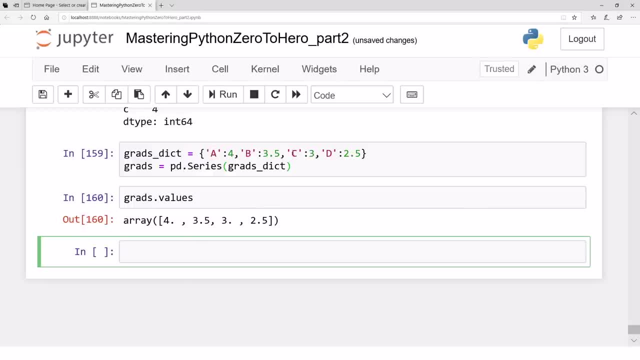 Similarly, if we find grades dot index, we will find out A, B, C and D. Let's define another dictionary, for example marks dictionary dict, and that is, let's say again, A. the total marks are 85.4.. 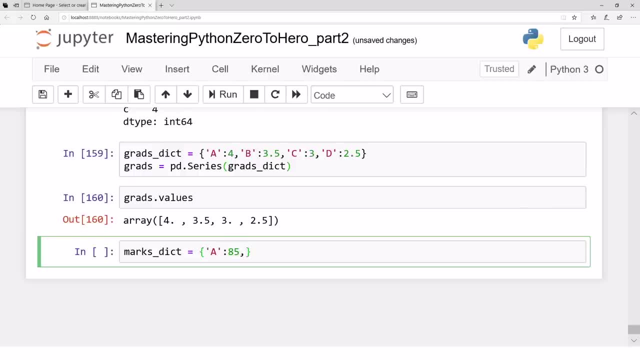 Okay, Let's define another dictionary, for example marks, dictionary, dict, And that is, let's say again, A, the total marks are 85.4.. Okay, For the A grade, let's say for B grade, the total marks are, let's say, 75.. 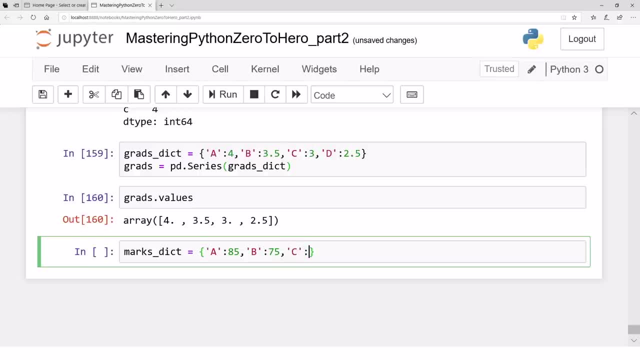 Let's say: for C grade the total marks are, let's say, 65. And for D grade, let's say the total marks are 55. Let's say So. let's say: that's another dictionary. Now let's create a series objects, a series object- pd, dot, series series. let's say: 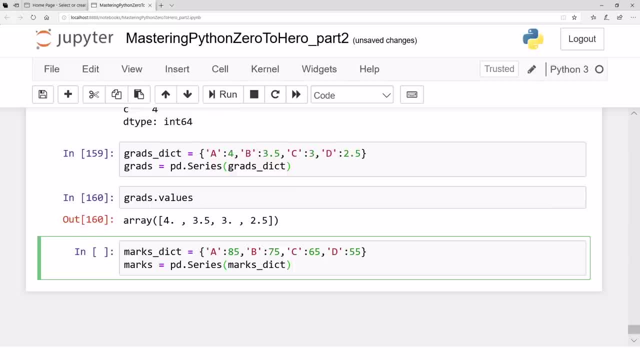 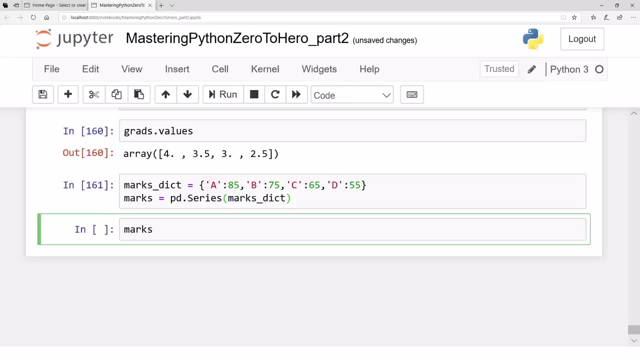 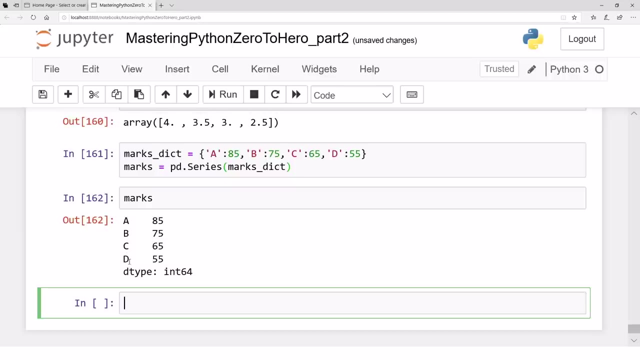 marks dictionary, dict Yeah. So now again we have. if you just write this marks, just like so, you will see the marks A is 85,, B is 75,, C is 65,, D is 55, and all the values there are integer 64 kind. 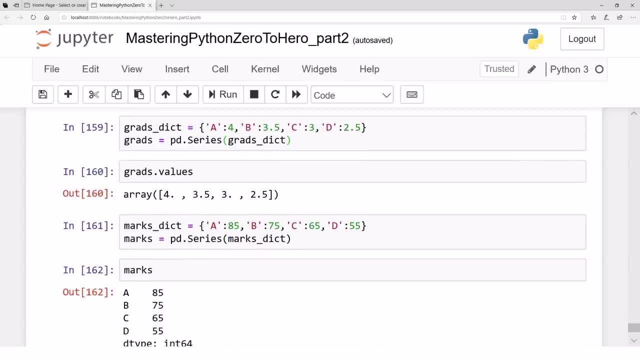 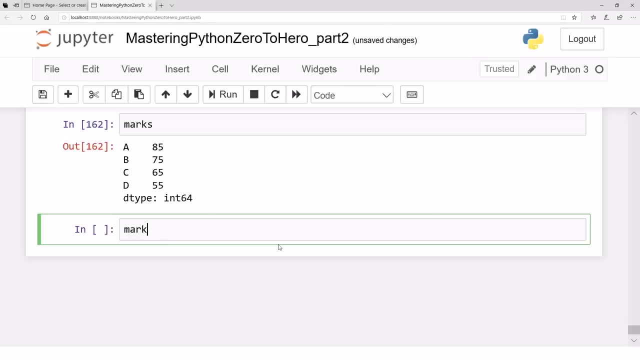 of values. Now we can access, now we can play with this- marks, for example. if we just want to access, for example, what are the marks, what are the marks between? let's say, for example, what are the marks given at A? We can access that, we can change that, we can just play. 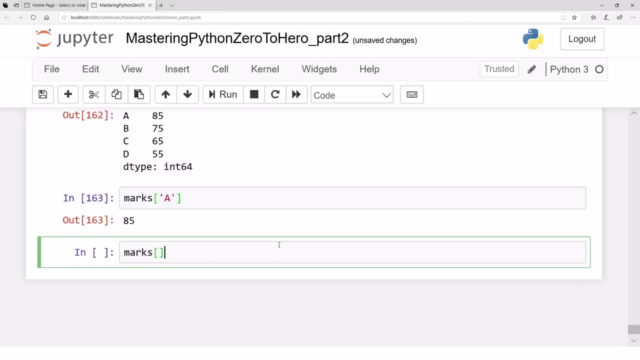 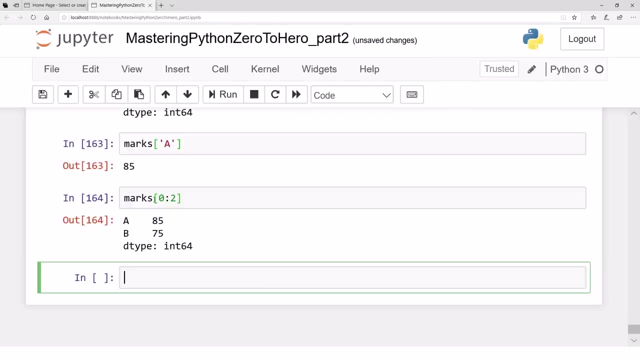 like a dictionary. What if we, rather than using the index A, we use, for example, slicing? We want to start from the very beginning and let's say we want to go to two. What will happen? Let's see, yeah, so the slicing is there, for example, if you want, these are explicit. 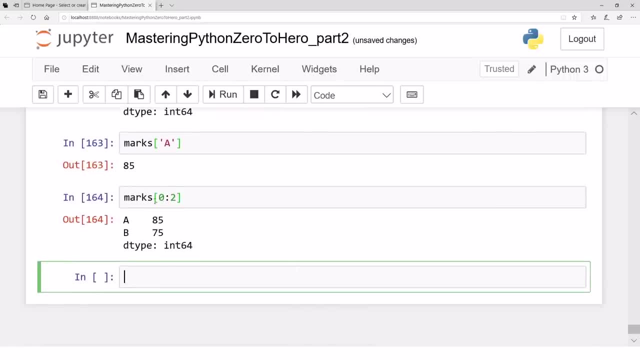 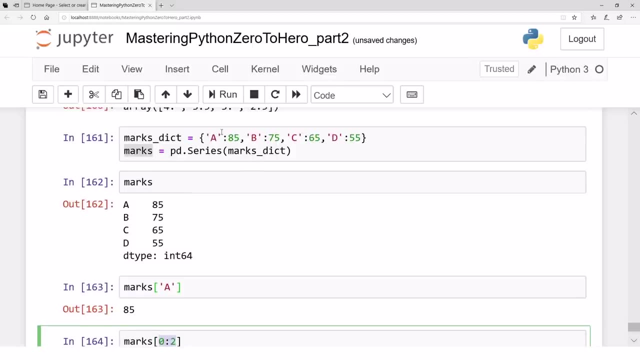 indices A, B, C, D. these are explicit indices and they are there. For example, if you can slice the data using explicit indices that you are given or implicit indices, that are the default indices. the first value, indexed at zero. the second value: 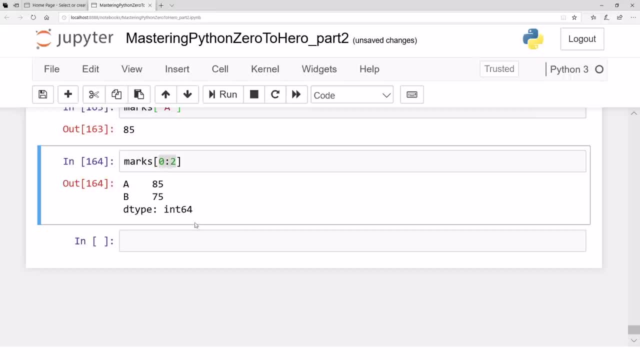 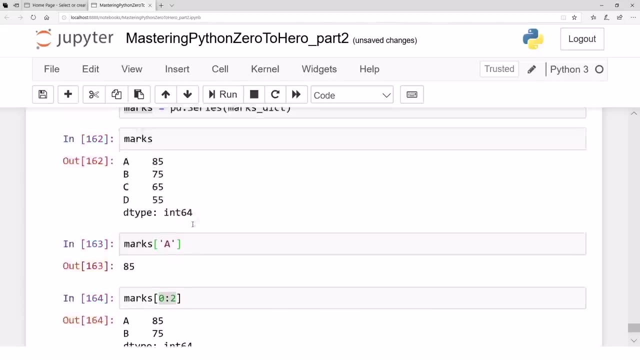 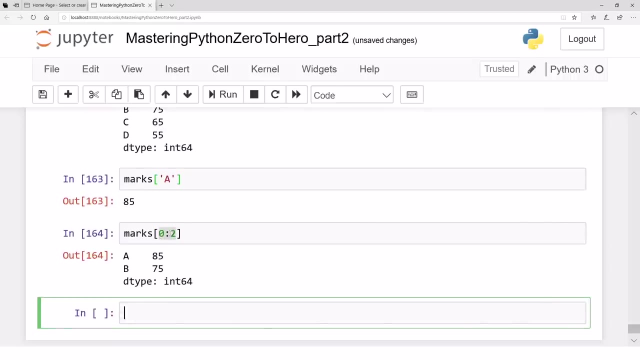 is indexed at two, one and so on. So you can do that as well. One catch here, for example, that we will see later on, there may be a problem that your explicit indices- they are also numeric, and then you do the slicing like. so then 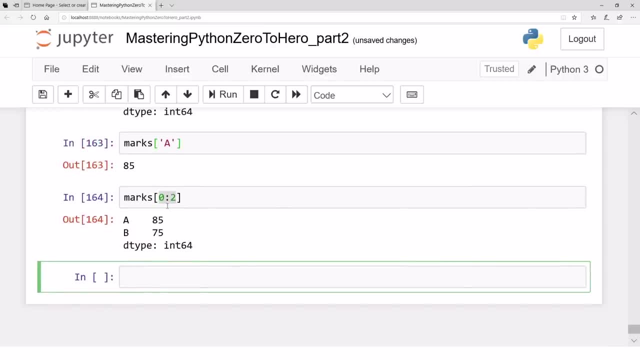 the series object may be confused whether I have to use the explicit indices or implicit indices inside. We will see how to resolve that issue, but this panda is allowed to use explicit indices as well as the Implicit indices. Okay, we were here. 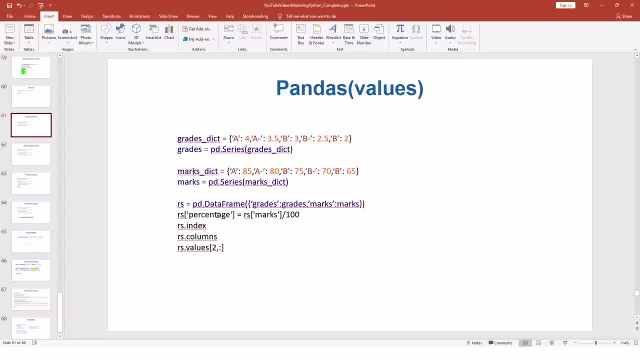 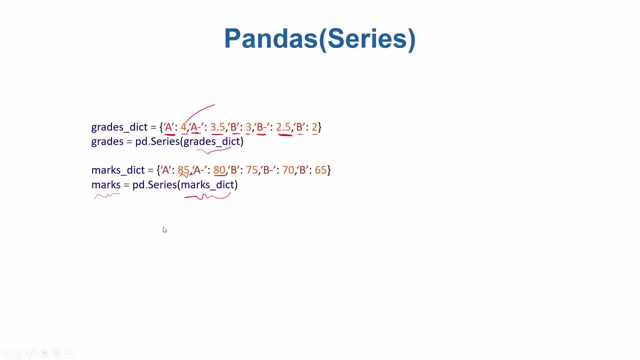 Sorry, I just So. yeah, so we were here, so we have created these grades. a series object- this marks as a series object. The series object is good for one-dimensional arrays or data with just one-dimensional list or dictionary kind of. 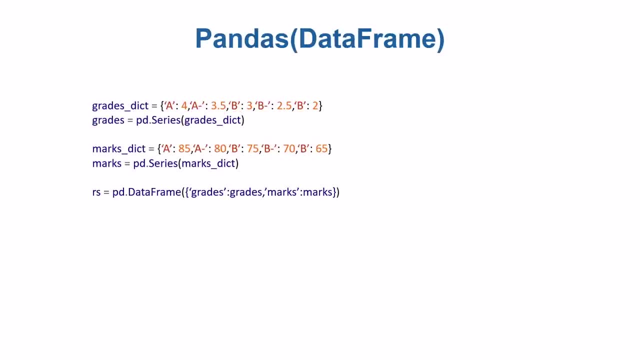 With just one dimension, With just one dimension. Later we will see a data frame that actually is the extension of Can be looked like as an extension of series towards more than one dimension. We may have, for example, two-dimensional arrays or two-dimensional data structures. 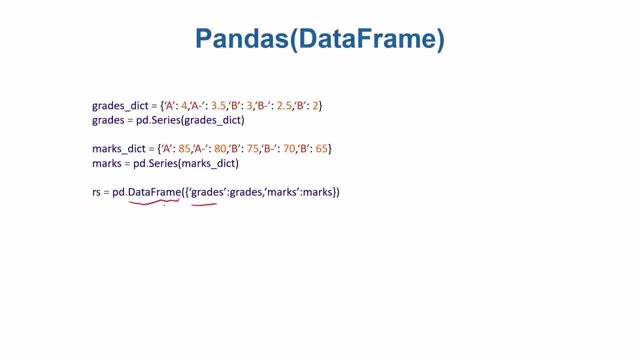 something like so, and we will be seeing this data frame, which is much more powerful, particularly for reading data from files and manipulating it. So we will see that in the next video- data frame, that running form of data frame, in the next video. 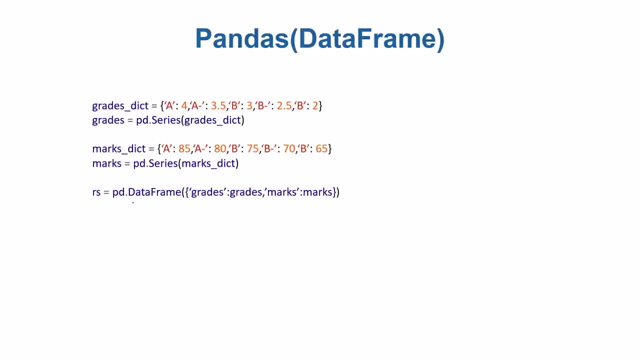 Hope to see you in the next video. Okay, in the last video we were discussing series and I told you that data frame is basically: if the data has, If the data is in the form of different columns, for example, a record as an array, then you 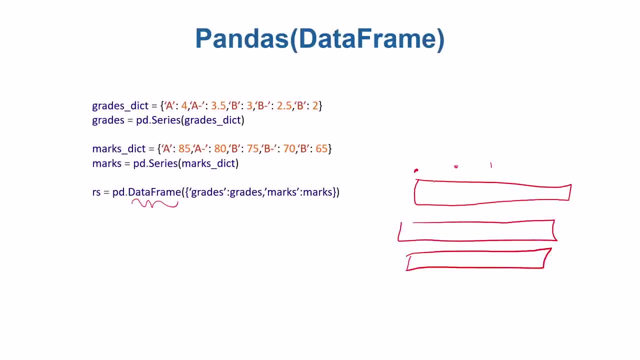 have another record, then you have another record And each element in that record is a different attribute. so this particular way of two-dimensional data is very well handled using data frame inside pandas rather than series. But you can make these data frame object using different series objects, for example. 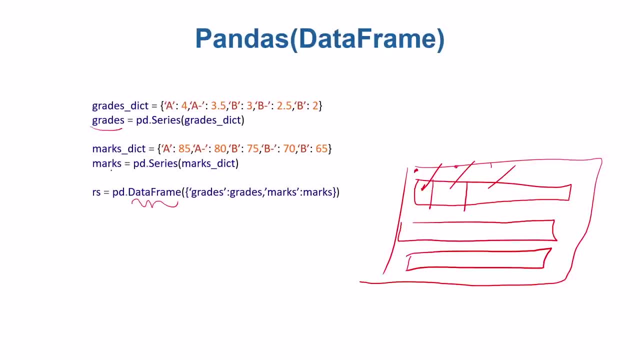 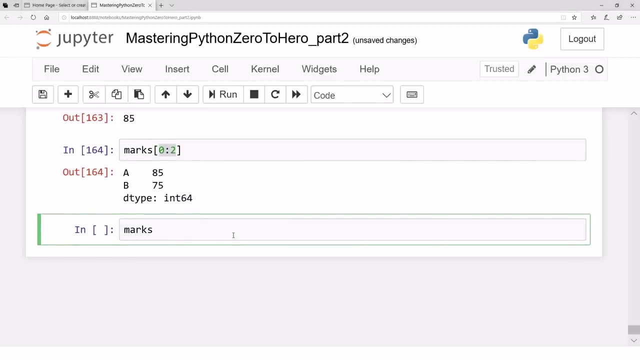 You have a grade object, that grades object that we created last time. marks object that we created last time. Let's build a data frame using these two And see what it looks like in Jupyter Notebook. Let's see that. So remember, we have a marks series object and we have a grades series object. 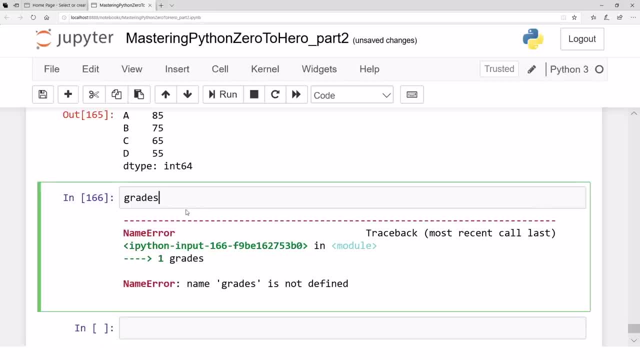 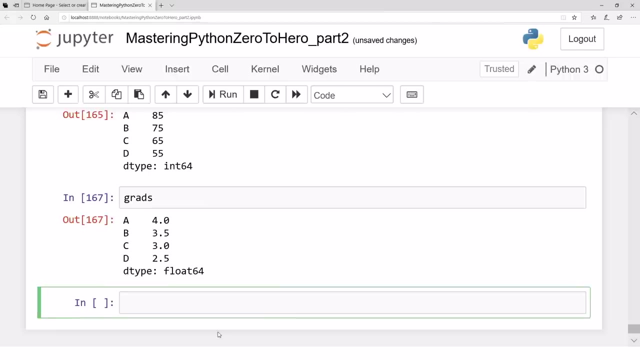 Let's now make grades. maybe the name is grades okay, The name is like grades okay. So grades, object this one. Let's make a data frame. Let's say d or maybe whatever name you want to do data frame with. again that: 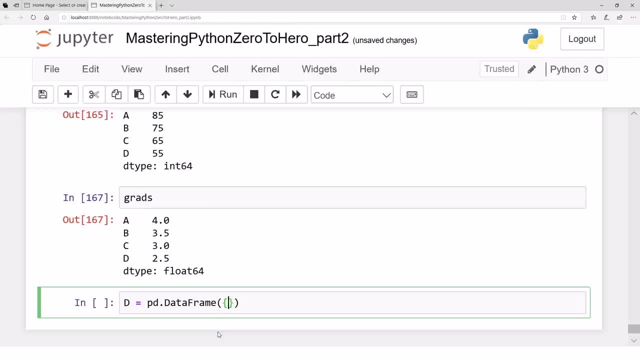 data frame can also be defined using a dictionary. Again, now we have, let's say, marks is the key for data marks and grades is the key for data grades, let's say. Let's say, we define a data frame like so: 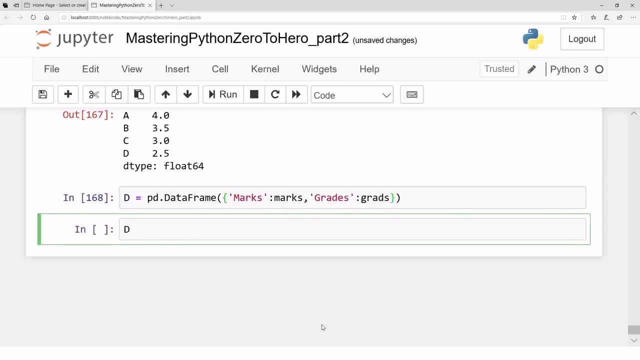 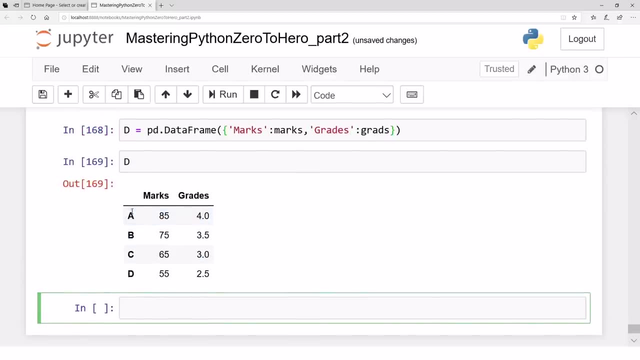 And now, if you see, if you just display this d, we get a very beautiful look and feel of. I mean this: a is the index. a is the explicit index. at index a, The marks is 85,, the grades are 4.. 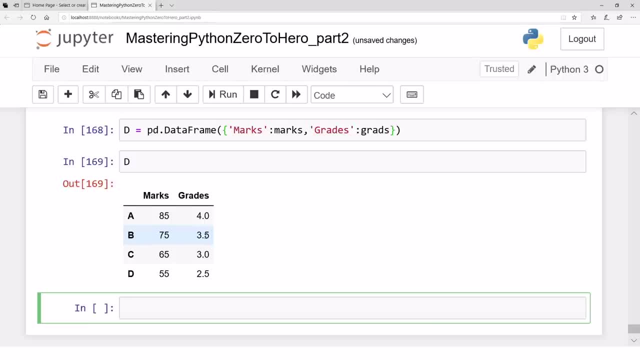 At index b the marks are 75,, the grades are 3.5, and so on. That looks like. so. Not only that, you can just transpose it like you have transposed the numpy array and you will get the numbers. 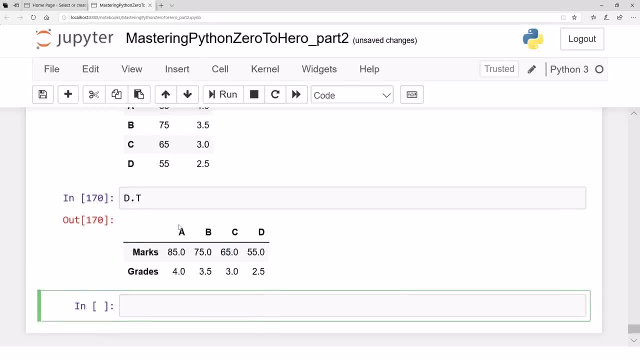 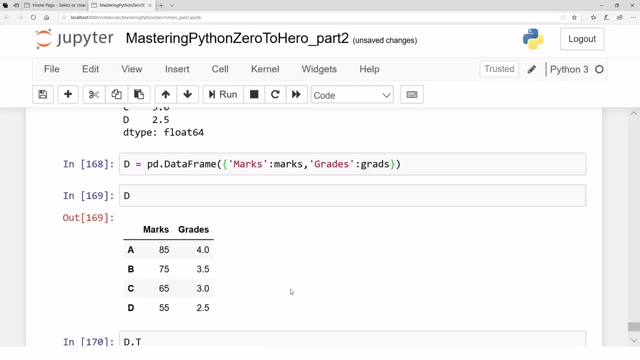 You will get the flipped variant or the transposed variant if you want. Great. So that's how, and you can have, for example, more dictionaries to concatenate together and more columns will be added here. And that's what the real data looks like. 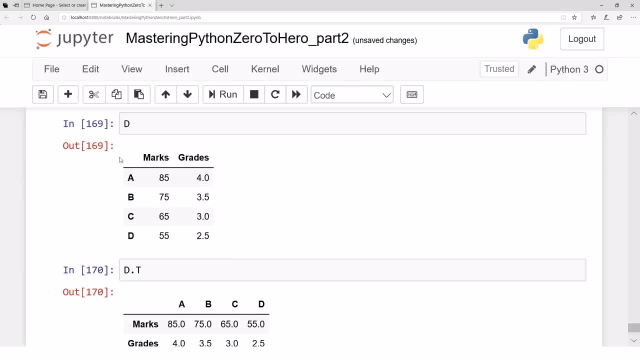 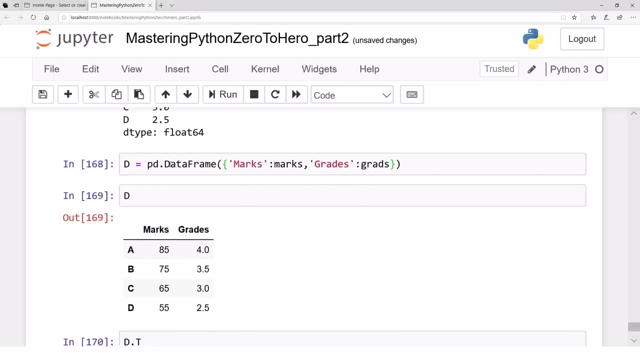 I mean, it has a lot of columns, which normally are attributes, And each row is basically one record or one sample of the data that you want to work on. So this data frame is really, really ideal data structure for working with files having 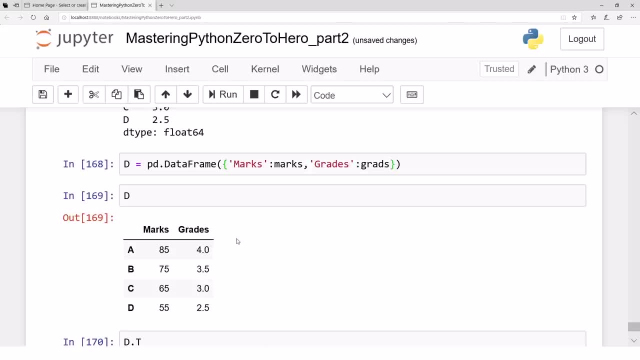 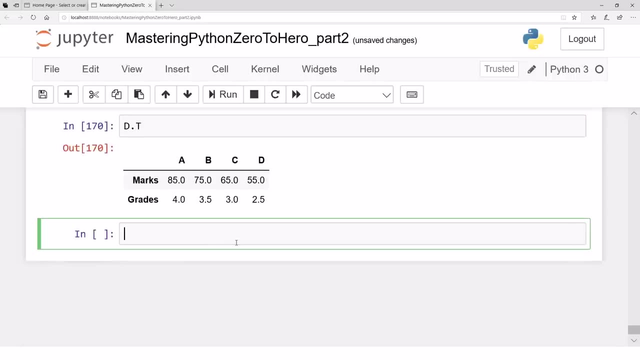 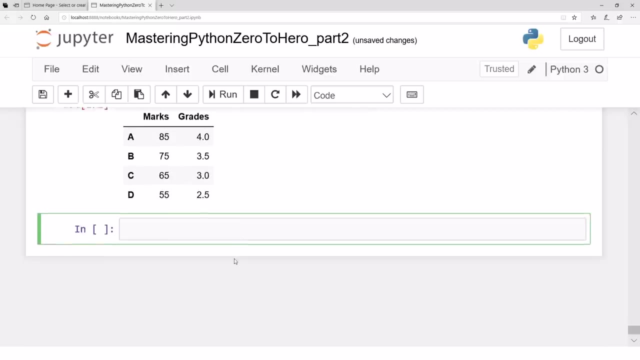 a lot of records And you want to manipulate that data and stuff like so. So yeah, So one more thing. Let's access the d. for example, Let's print d. That's the d. Let's access the values inside d other than no. 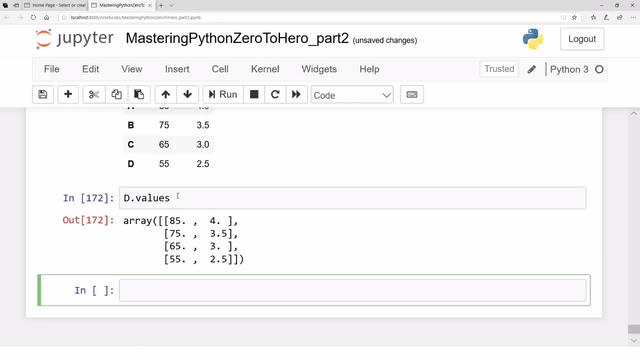 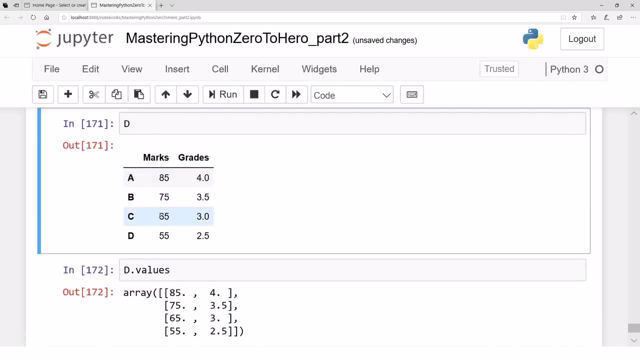 So what are the values? So the values inside d is completely again a two-dimensional array. that is completely like so. So, for example, So if we want to access this particular element 65, that is, row number three and column number, 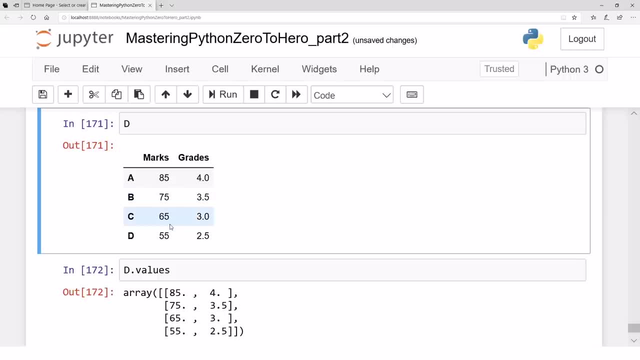 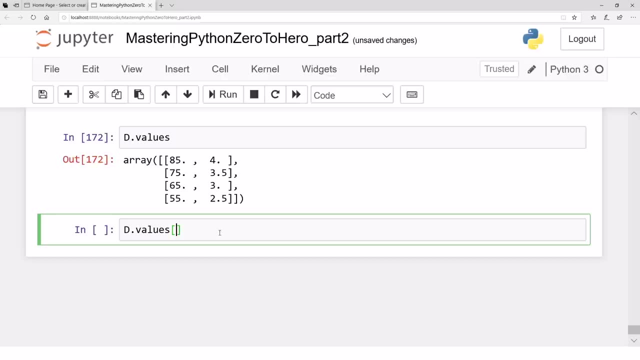 one, excluding the indices. that's row number three and column number one. So we can access that particular value dvalues. just assuming that's a two-dimensional NumPy array, Row number three is two, index with two and column number one is indexed with that. 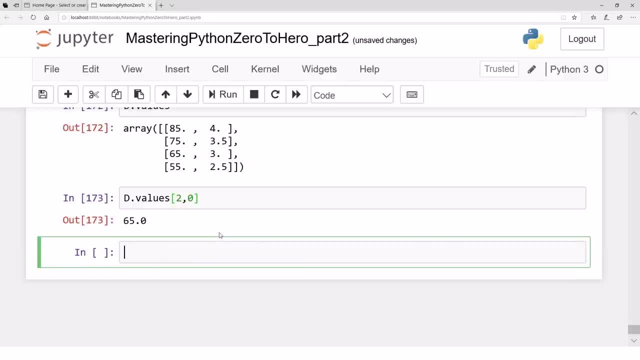 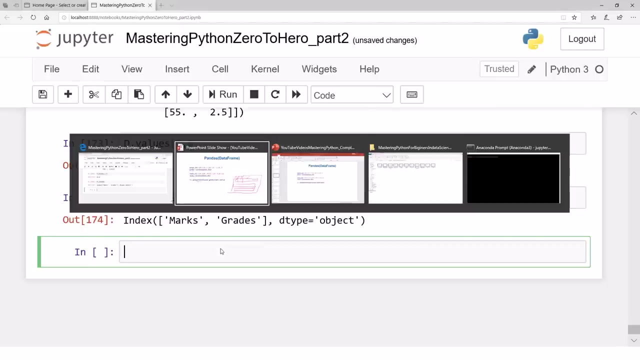 And we will be able to access 65.. Wow, Great. So that is there. There are more things that are available: D dot, for example, columns, d dot, columns, columns. it will give us what are the columns. The columns are marks and grades. 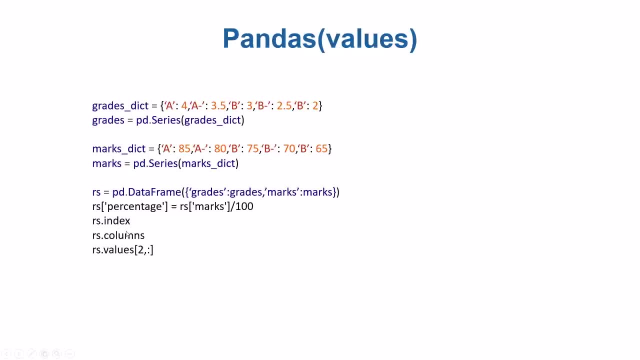 And there are other properties, and there are other several properties that we need to know: Rst, for example, This There, And that is what we need to know. So we need to know the columns, But we want to know the value. so it says that's the d. 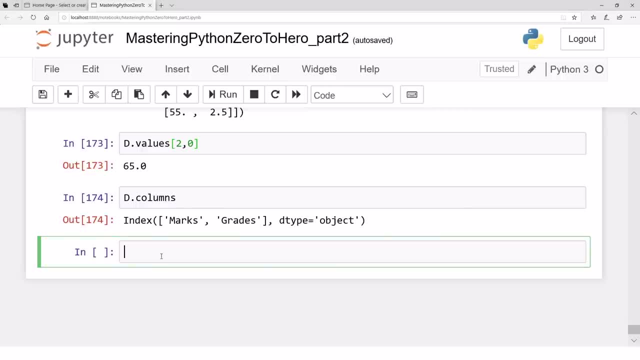 We do not want to add another column here, And so d stands for d dot index, And so that's kind of the way we want it to work, And we'll talk about that later, but you just need to know, okay, one more thing that. 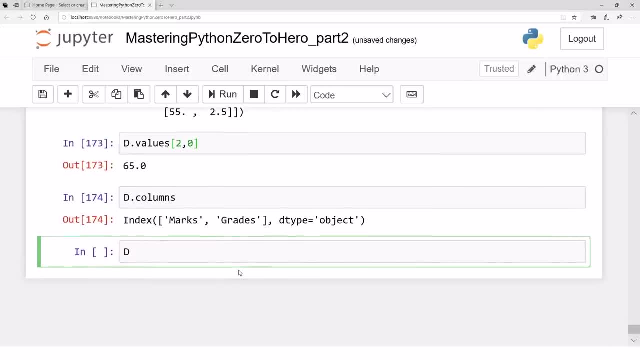 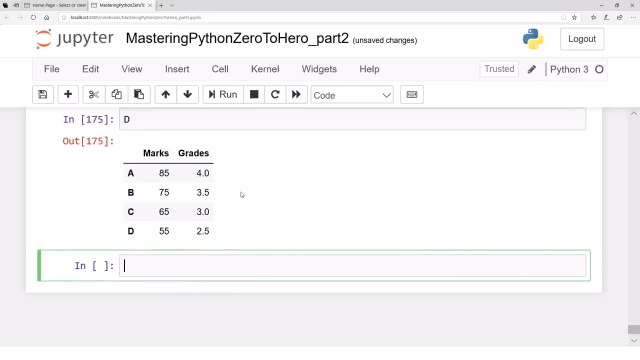 you need to know is we can. right now we have that's a, d, that is this one, That's d. Let's say, we want to add another column here. Just, we want to add another column here, And that is the name of that column is scaled marks. 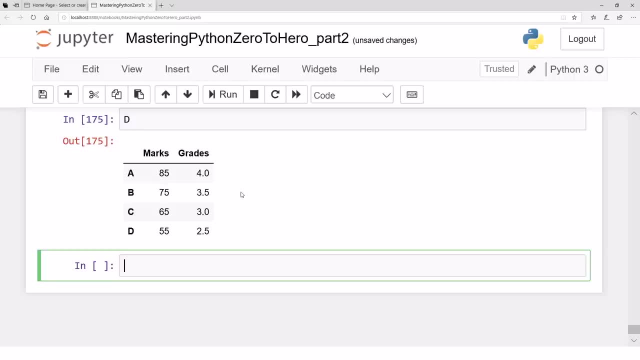 And the scale marks are. what if we have computed marks rather than from hundred? what if we have computed marks out of 90? what are the scaled marks out of 90.. so one way to do that, and very quick way to do that, is just like a dictionary. again like a dictionary, you just add a new key. 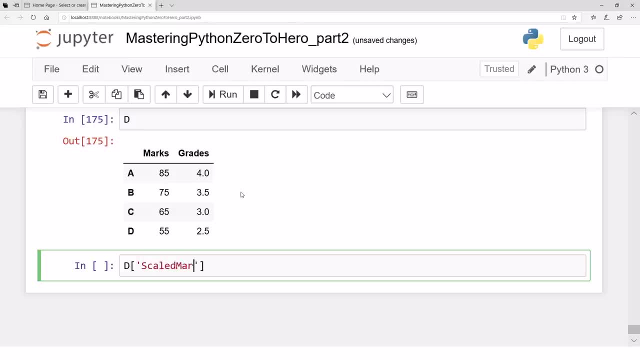 let's say scaled marks. that's a new key- and the value is simply all the marks column divided by 90. so is that true? no, um, divided by 90? uh, if, if we have just computed all the marks by 90, and then how can we? how can we compute the marks from 90? it is rather than 100, it is from 90. I, I guess, um. 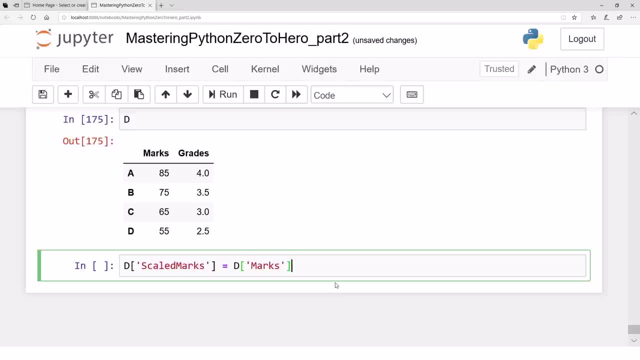 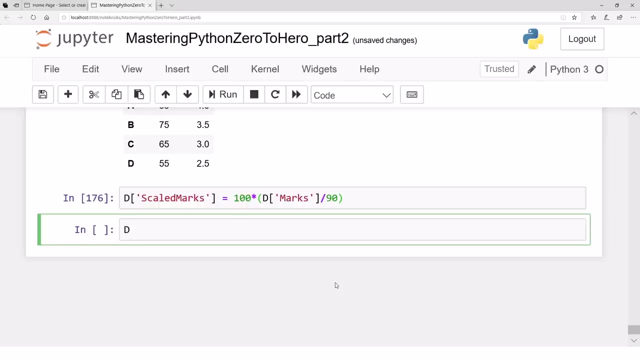 how can we compute the marks from 90? uh, if you want to compute the marks from 90, from 90, I guess they will look like divided by 90 and maybe 100 is multiplied here. I guess, maybe the formula. I guess that that that's what it is, I guess. let's see. so now, if you see D, there will 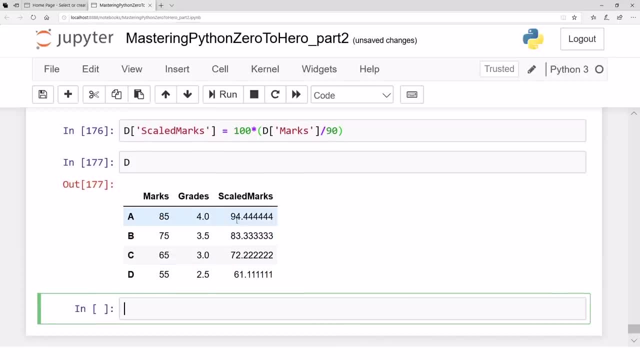 be another column that is there and oh, it does something else anyways. I mean it does something that, yeah, so something anyways. so we have see, we have just. I mean, you've just computed this, we, we just, we just found, we just inserted that column inside that. I mean, that is a processed for you. 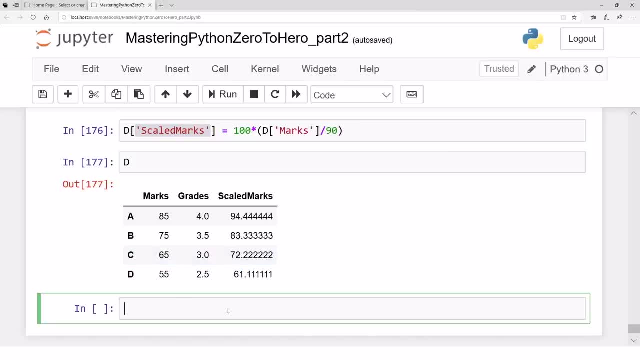 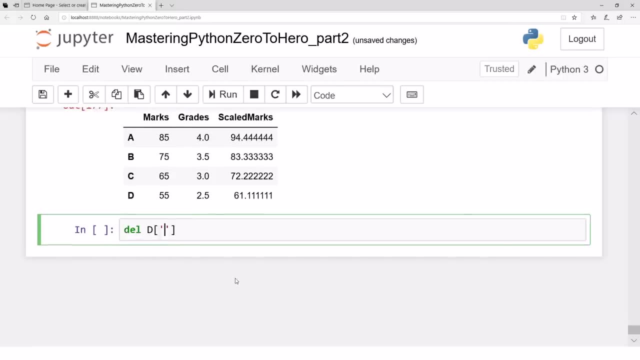 know these kind of values. maybe we have added this column in a very wrong way and later on we suggest that, okay, we should delete that column. well, that's very simple. again using the, the concepts, again just like the dictionaries. delete this and this column is deleted from data. 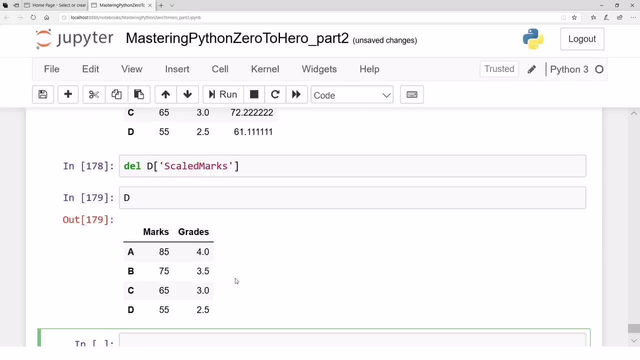 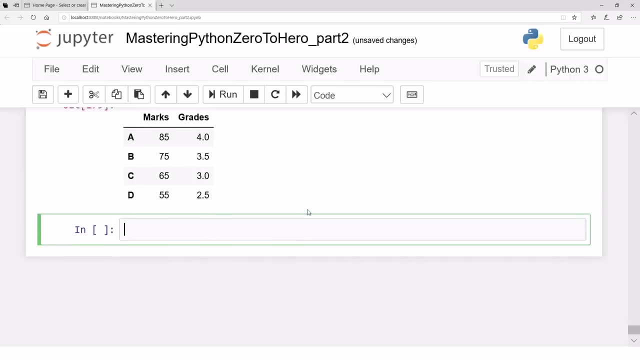 and you are again with the data that you had. so you can add columns, you can delete columns and indexing is really fine. I mean indexing like, like masking. let's say you want to pick, for example, all you want to pick the data frame, such that you want to pick all the records, such that the marks. 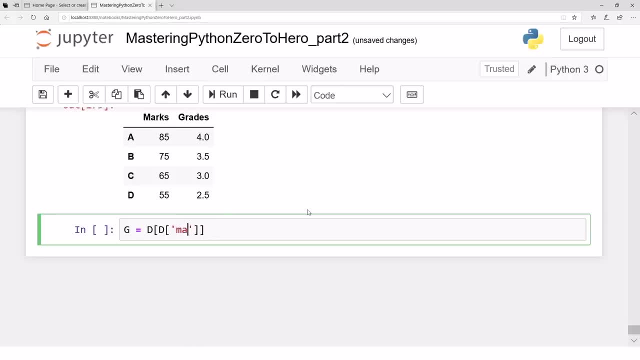 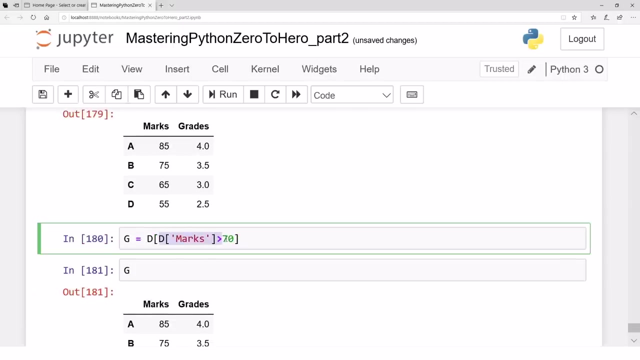 are the marks are the marks are greater than, let's say, greater than, let's say, 70. you want to pick all the records where the where the marks are greater than 70. this is that simple. all the data will be will be copied into G with this condition, and this condition can be arbitrarily. 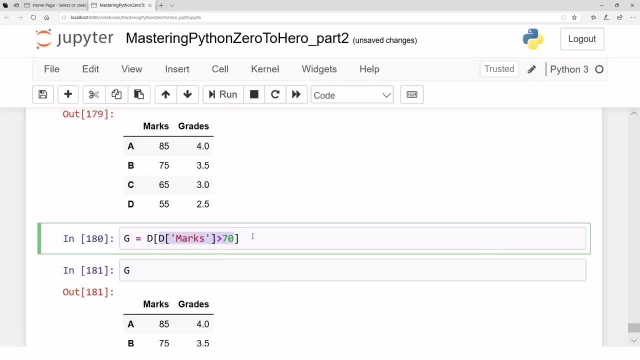 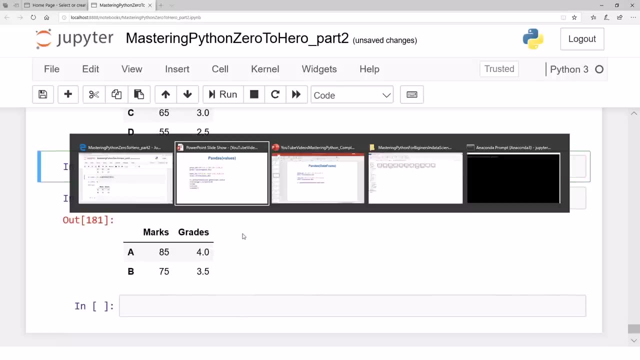 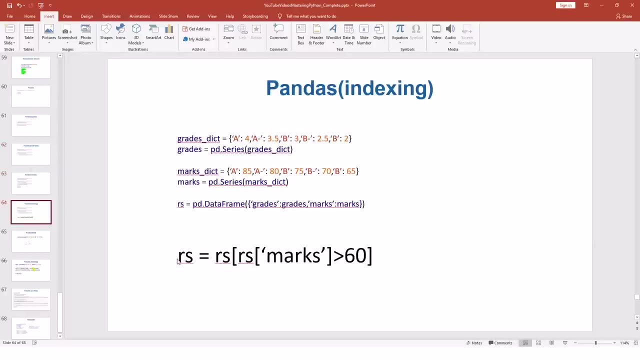 complex using ands and ors and combinations and all that stuff. we have seen this kind of stuff in numpy as well. I mean, this is called masking great, so that's available in pandas as well. okay, so, um, that's how you can index um in in the next. uh, in the 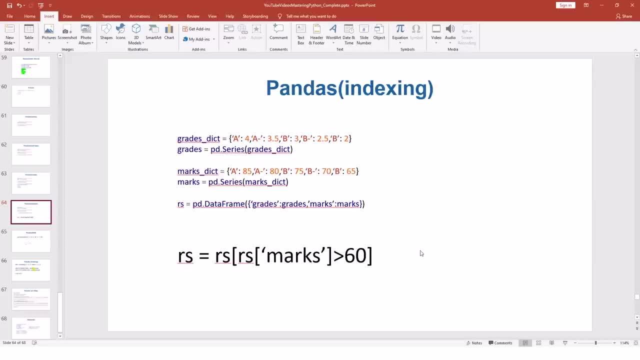 next video I'm going to basically uh show you, uh one type of problem that normally happens in real data, that is, the missing value problem. sometimes, uh, you, you read a data and some of the attributes or some of the row, column, pair values, they, they are just missing. I mean, they are not. 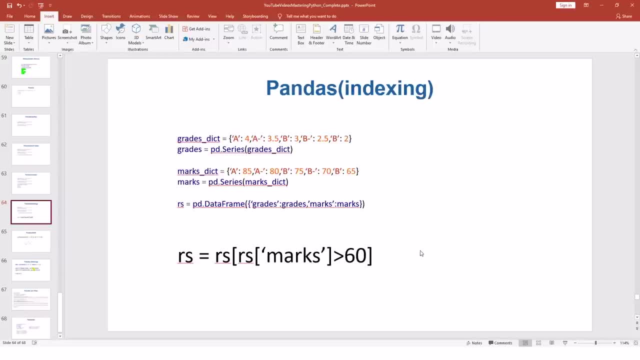 available due to certain reasons. how can you, how can you handle those values and how actually pandas suggest you to handle those kind of um missing values, which is sometimes called nan values or none type values. also they they mostly used interchangeably in pandas. so in the next video, 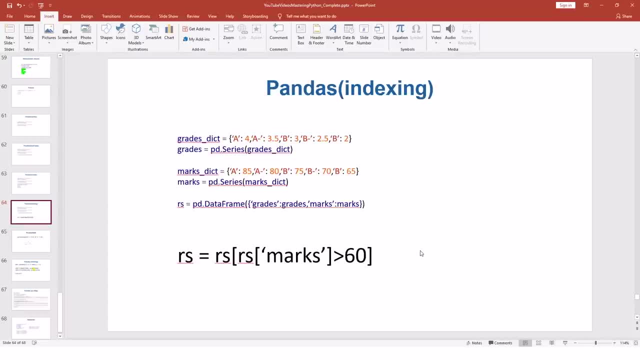 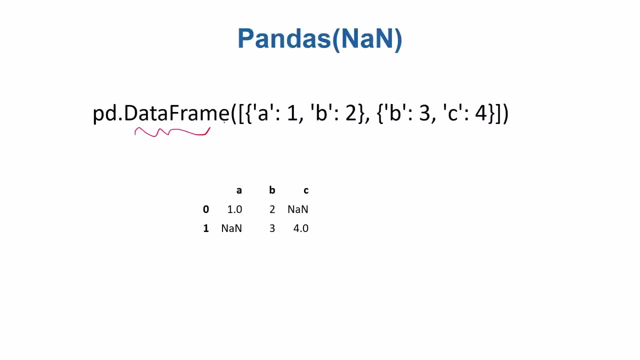 we are going to handle, or see how to handle missing data in pandas. hope to see you in the next video. okay, in the last video we saw data frame object and, uh, we, we saw actually how to add and remove columns, how to process data, how to index. 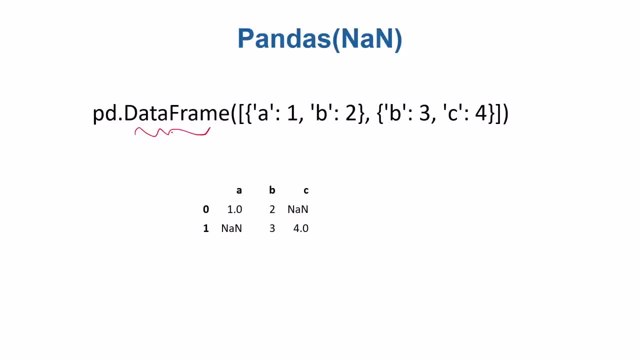 um, how to actually mask or how to apply conditions and selections in in pandas. we we saw that very briefly, but in this particular video we are going to see one kind of missing value, sometimes called nan, or not a number, or or maybe not anything, or sometimes this none type, none which is the default return type of any. 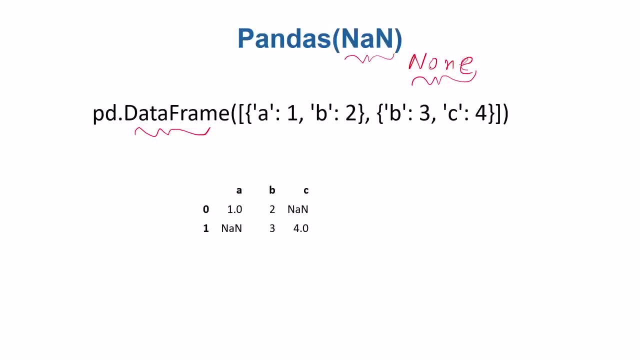 function in in python. this none type is also sometimes in pandas- is treated as nan, or nan is treated as none or interchangeably any anything. let me give you what do we mean by that. let's say we. we have two dictionaries. let's say, one dictionary is a with key value a and the. 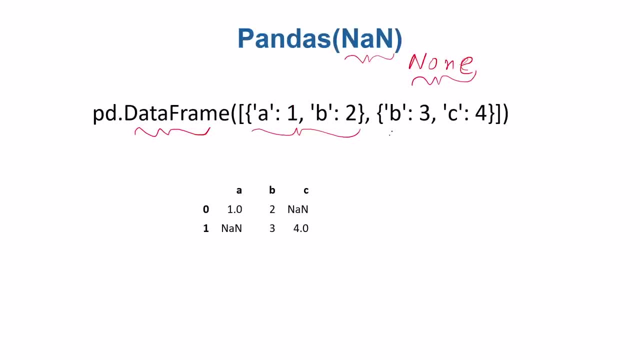 value is ones, then b and the value is two. okay, the other dictionary is b and c. so for example, that is one record with columns a and b. so a and b are the columns on the first record. the value of a is one and the value of b is two. now let's say we want to insert another record in the same data frame. 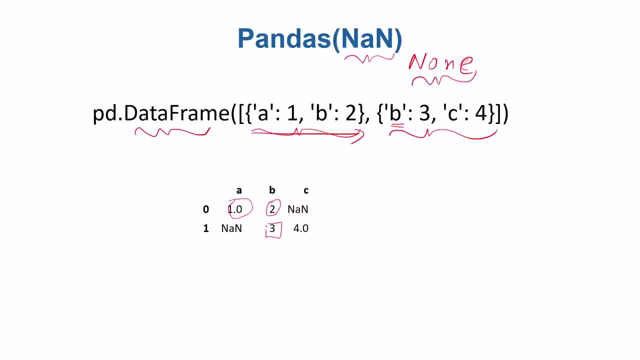 now the value of b is available. in the second time the value of b is available, which is three, and the value of c is available, which means a c column is added now. but for the value c, the first row value is not available. so we will say this value is missing. 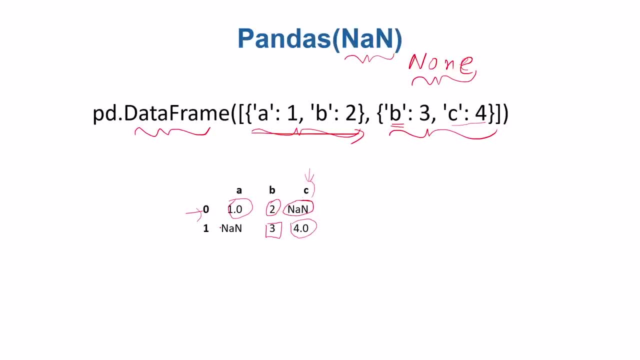 here, but in the second row we have four. similarly, the value of a is missing for for the second row, and that is a missing value which is sometimes called nan. so these are missing values and they are typical when you are working with data and you're reading data and you're getting data from. 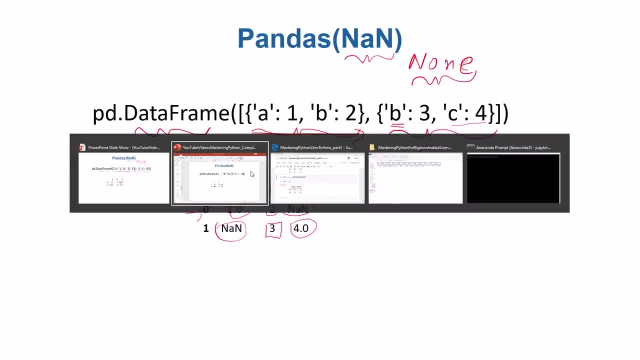 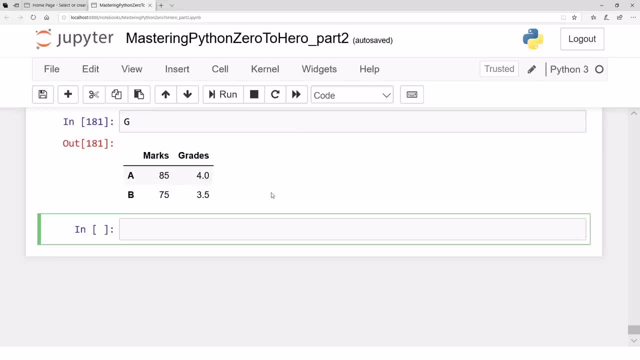 from out from somewhere, or large files and stuff like so. so pandas, give some methods to handle these kind of, these kind of- i mean this kind of situation. let's say, let's say a equals pd dot dataframe, dataframe- again a dictionary. let's say: we have a. one and b, let's say four. that's the first family you probably already know of зап, slow data. that's an example, hi, it's an example of overcoming non- API cases. welcome, i get my пожetti movie back in省thsi num nursing examDERmäß họBu去了. 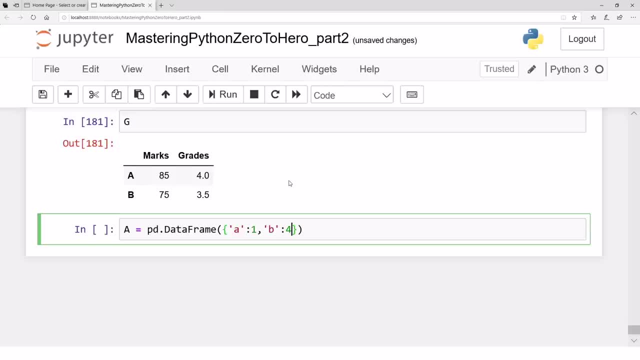 And B, let's say 4,. that's the first row or record. The second record, let's say, is another dictionary. Let's say B is minus 3.. And C is, let's say, 9.. Let's say that's our data frame A. 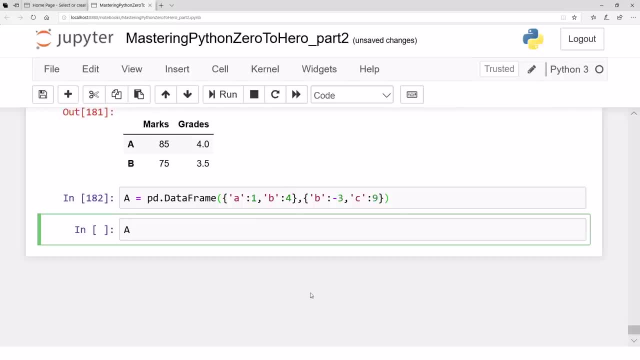 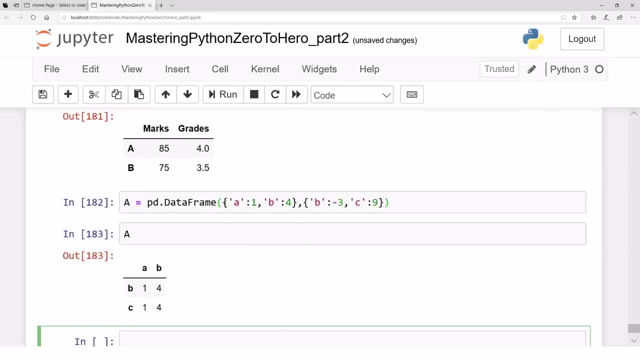 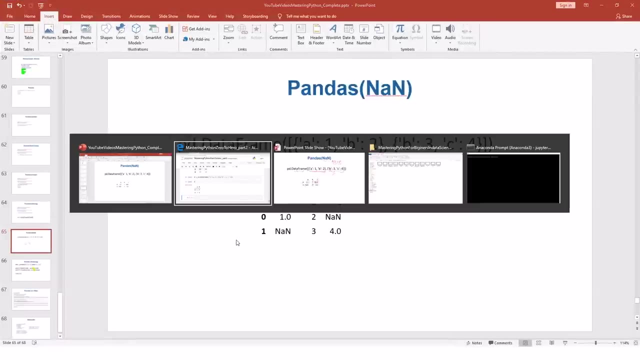 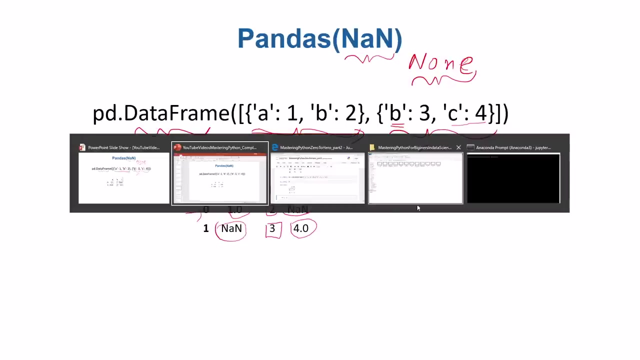 So now, if you print this A, if you see the data inside A, you will see: oh, what's the problem? A is this and B: have we applied something in a wrong way? Let's see: Oh, we have to create a list, That's the okay. we have to create a list of it. You have to create a list of dictionaries. That's the proper way of calling it. 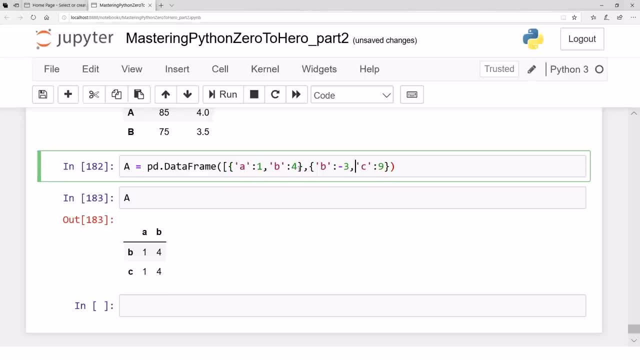 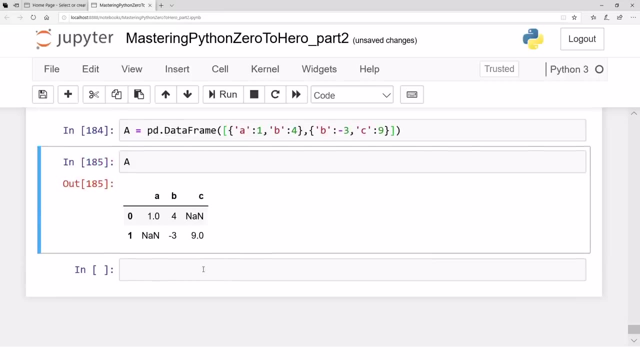 So we missed just the syntax list of that. Okay, right, So now we have this A, we just call that A and this value is missing. and that value is missing, And in large data files this is typical. I mean, there are a lot of values that can be missing. One way that Panda supplies to handle these missing values is to just fill these missing values with some fixed number, for example. 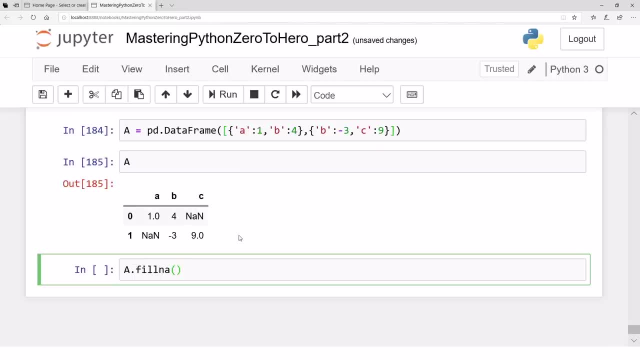 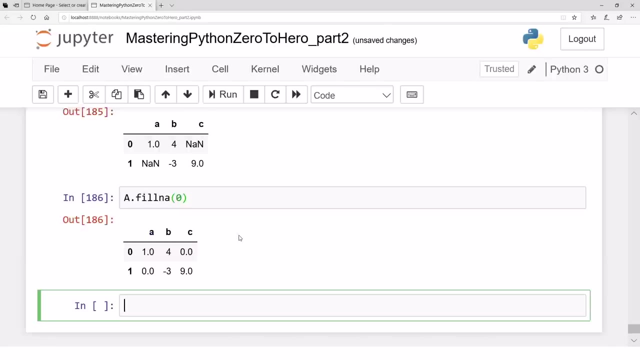 There's a fill na function. Fill na function and let's say you supply a zero. That means wherever there is a not available or not a number value, fill that with zero Or maybe any value you want to fill that with. So that is one way to do that. And now, if you see, the value of A is all the non-values are filled with that. 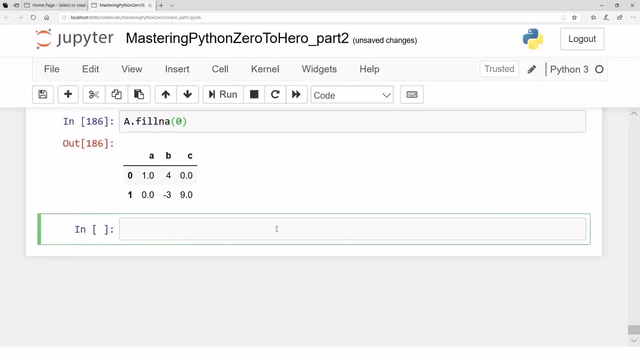 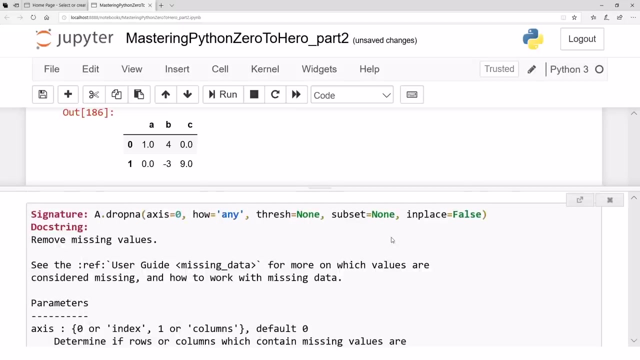 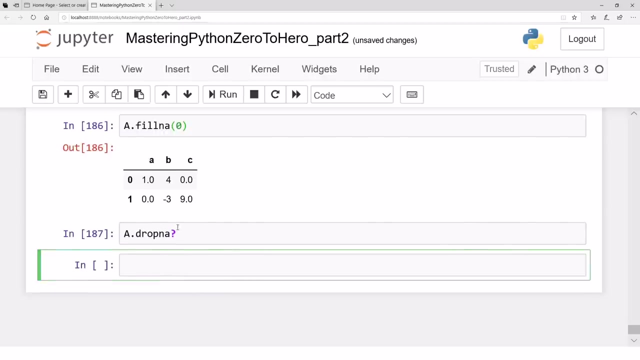 Another kind of function that is available in Pandas that is sometimes used, A that is drop na. that function, drop na. What that does is it drops all the records that contain a missing value. Sometimes, if that is feasible, I mean dropping all the records that contain missing values. if that is feasible, then go for that. 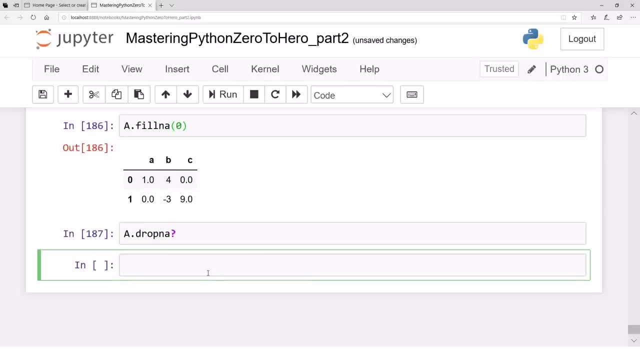 But if the missing values are a lot and they are spread over a lot of rows, then dropping all those kind of records they will create a lot of- I mean- data loss, and then it becomes really, really important how to handle these missing values. 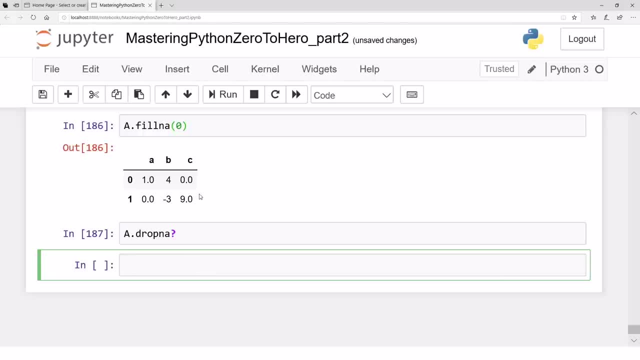 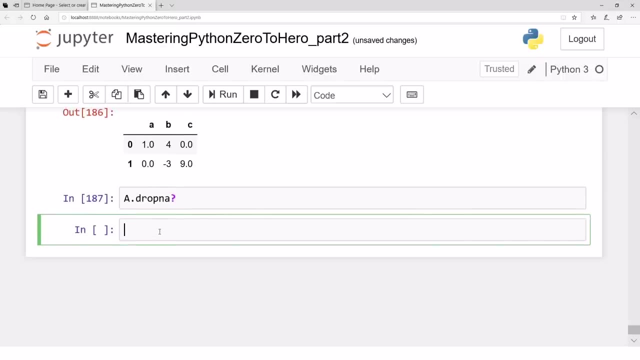 However, you can fill the missing values using fixed value or you can drop them, And later on we will see in Scikit-learn that there are other ways of handling the missing values as well. You can fill each column missing values in each column using: 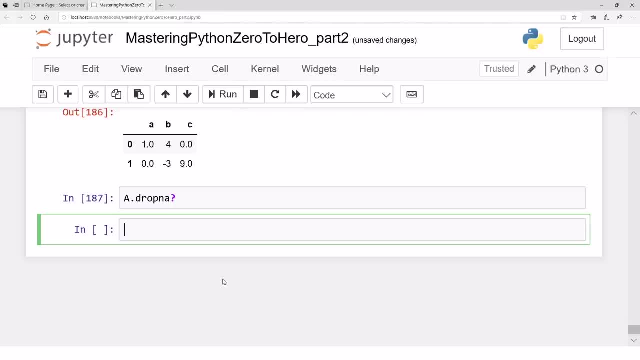 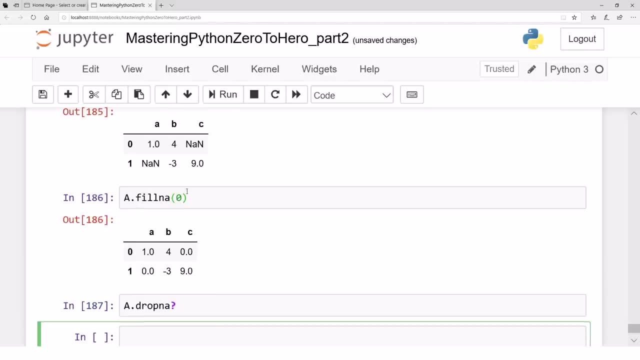 an average or using, for example, a regression. There are ways to to handle these missing values, but in Pandas, these two functions are right away there. You can fill all them with a fixed value, for example, or you can drop them and you are ready to go. 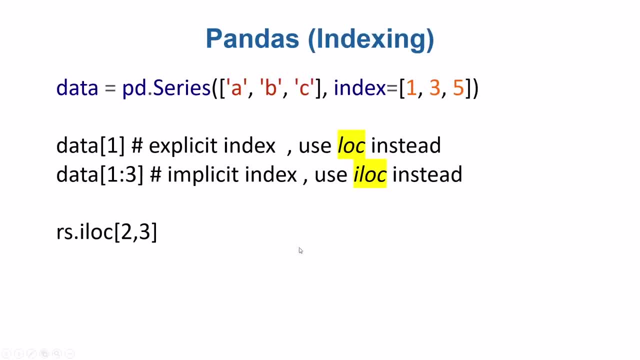 OK, great. Next we are going to see, as, as I mentioned earlier, what is a what is a confusion between what if there is a confusion between implicit and explicit intact, OK, great. Next we are going to see, as I mentioned earlier, what is a what is a confusion between, what if there is a confusion between. 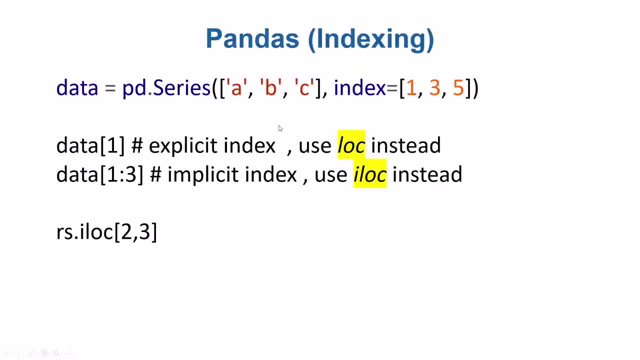 indices and that I will discuss in the next video. basically just to give you a look and feel. what if the explicit indices you supply? they are 1, 3 & 5? and what if you call this, this particular command 1, colon 3, will it call the? 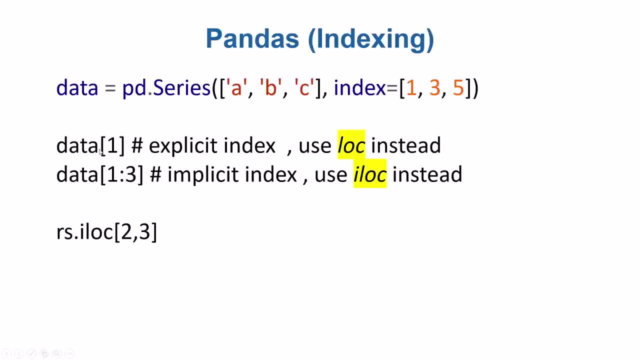 implicit index or the explicit index. that's a problem. so we will see, because 1, 1, colon 3, 1 & 3, they are also explicit indices and whether this 1, colon 3 is referring to the implicit indices that are default indices or they are. 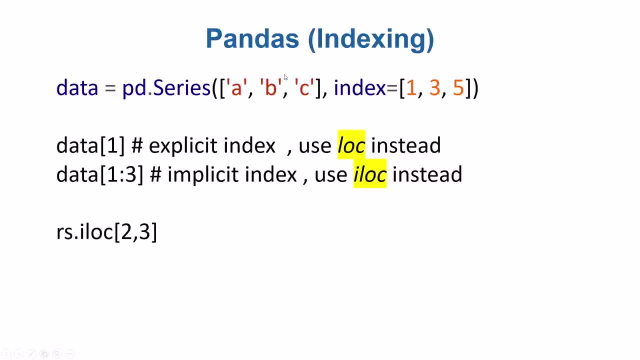 referring to these indices. so this confusion is there and we will see how to handle that confusion using this log LLC function and index log ILC function. we will see that in the next video. hope to see you in the next video. okay, in the previous video I mentioned a confusion that can be there if you have. 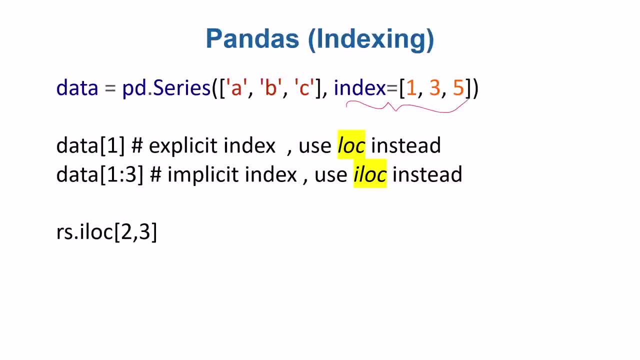 supplied the explicit indices that can conflict with implicit indices in particular. for example, if this is the series object, or maybe a data frame object, if you want to. if for indices, let's just think about the series object. it has these values: ABC with index 1, 3 & 5. if we, for example, access a particular 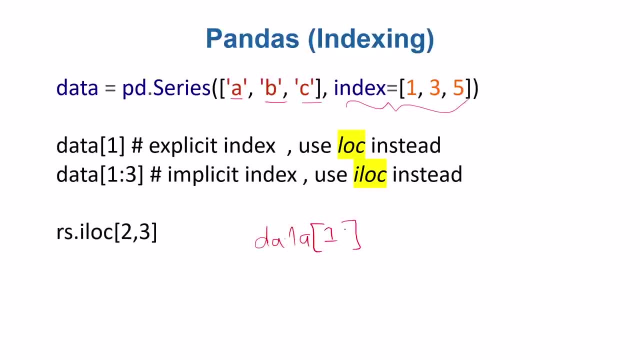 element, let's say data, with index 1. that means the explicit index, for sure. but if, for example, we slice the values, for example one, colon three, the default behavior of slicing, if you give the numeric indices, that is to use implicit indices. and by implicit indices we mean by we mean that what is add index one at 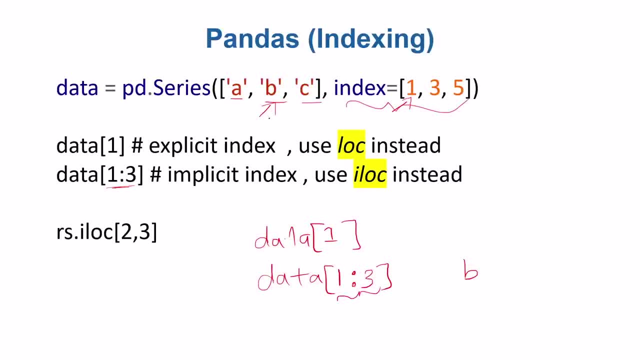 index one. this is B, so B will be printed, for example, or B will be fetched, and then you move to 2, which is C, then C will be fetched and these are the will be printed, but the behavior might be different. you might be expecting to use explicit indices, which means XS, 1, colon 3, and when the explicit indices 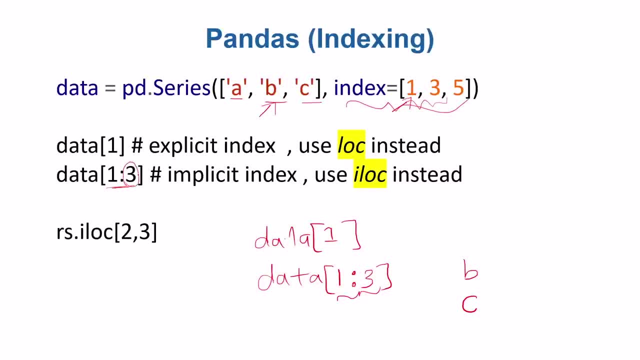 are used, the last index is also included, and in that case you might be expecting: the index 1 is of a, so a should be printed, and index 3 is of B and B should be printed, and this confusion might be there if. if this is there so to handle. 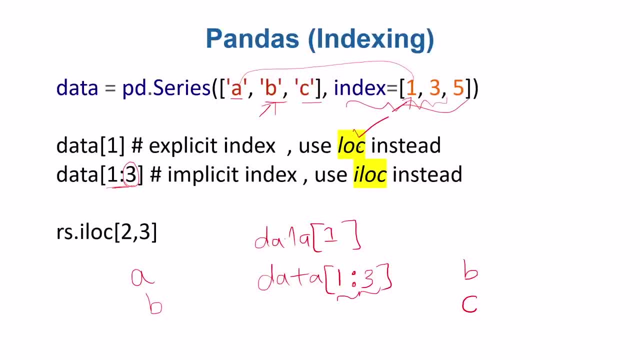 that there is. there are two functions. one is called LOC and another method is called ILOC. whenever you call LOC, that means you are using explicit indices- I mean you're forcing to use explicit index- and whenever you call ILOC, that means you're accessing elements using the implicit index- what whatsoever. so 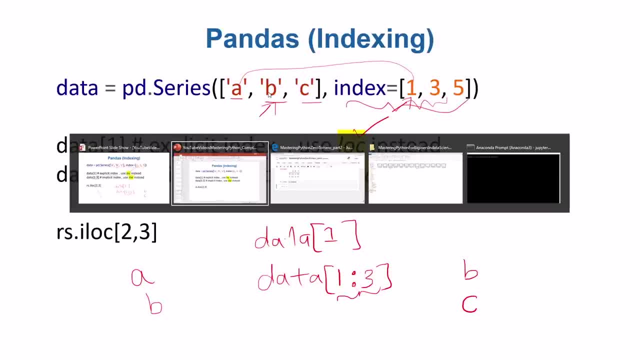 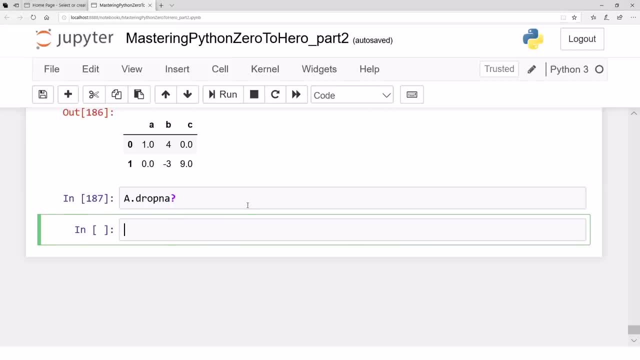 let's let's practice this and see the confusion, see the detail of this kind of confusions in in here. so let's say we have a series object, let's say a equals PD dot series, and let's say it has values as a, B and C. that's the value. these are the values. 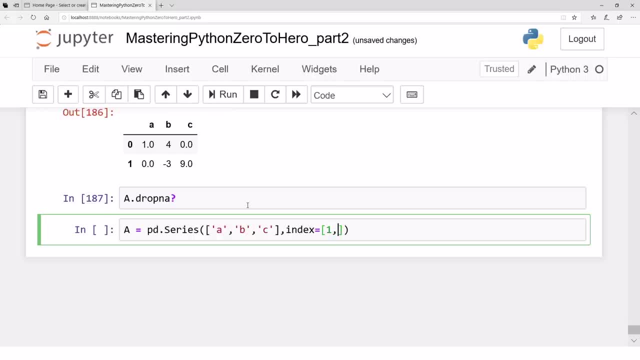 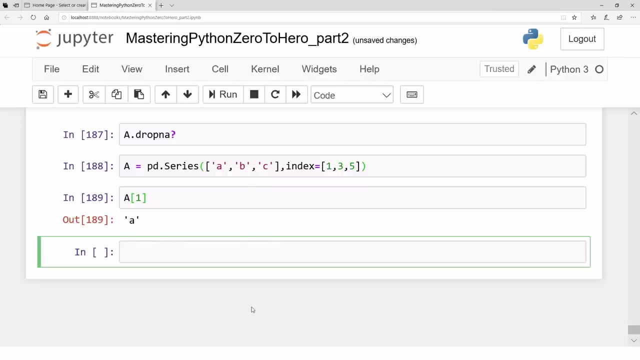 and index, as, let's say, one, three and five. let's say these are the indices. so let's say this is a. okay. let's say we access a using one. that means that means the explicit index and that is this. let's say we access using a slicing. 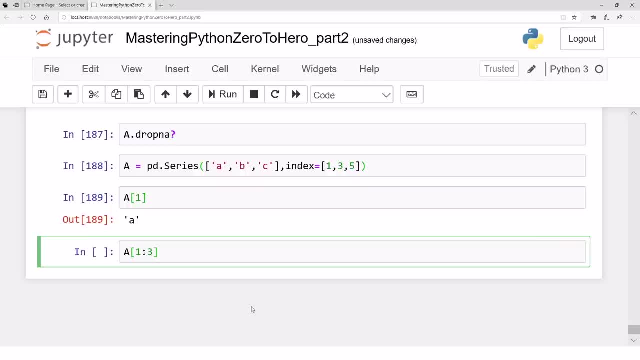 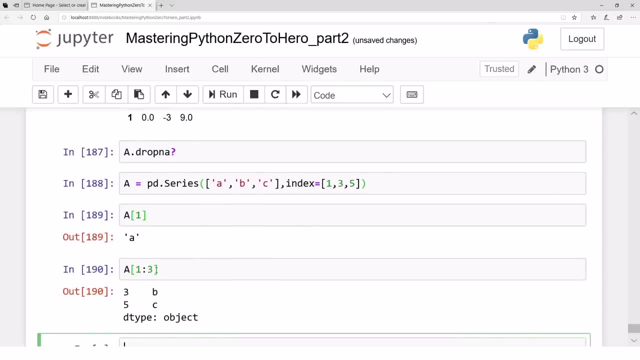 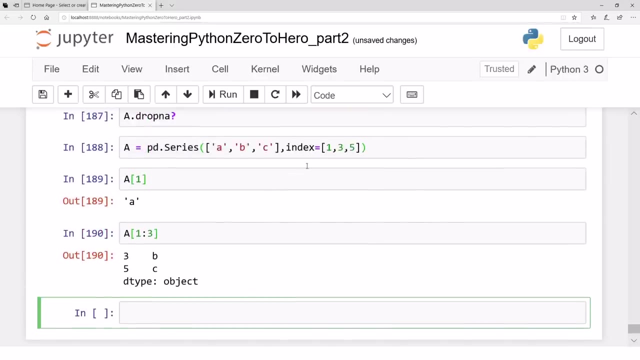 operator. now this will use implicit indices and it will access- I mean it will access these B and C, because 1, colon 3, using indices, implicit indices, results that and we might- we might be expecting that- use this kind of stuff. so if we are really interested, 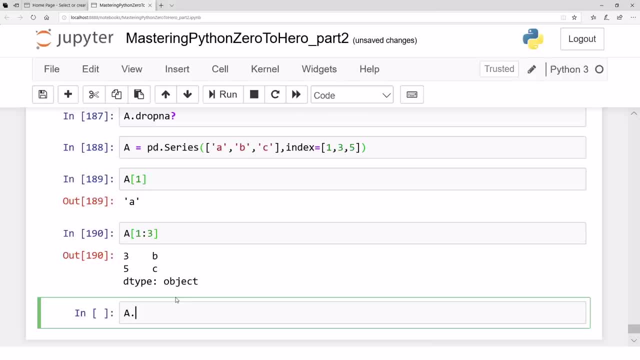 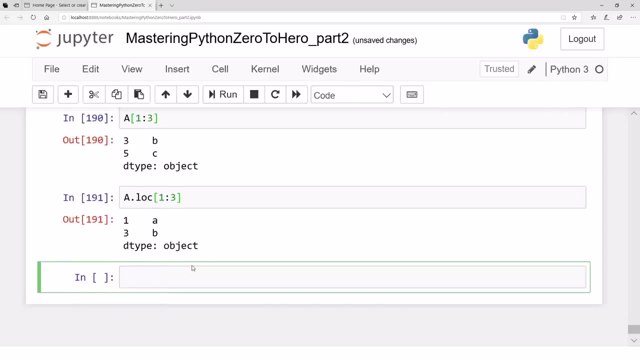 in using explicit indices. what should we do is we should call the LOC function a lock, and then 1, colon 3. that means use explicit indices. that is to remove the confusions. now it will use the explicit index 1 and 3 and if, for example, we are: 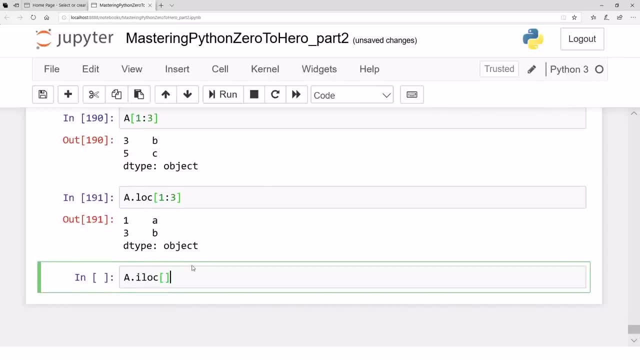 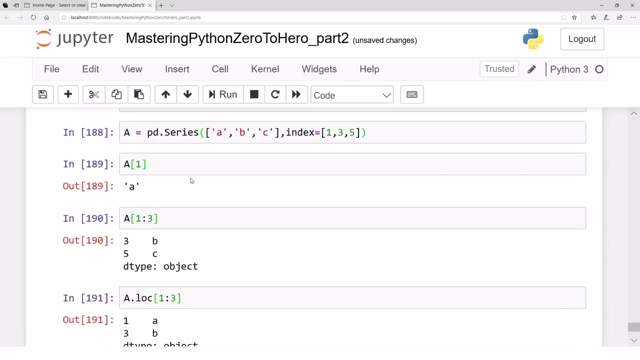 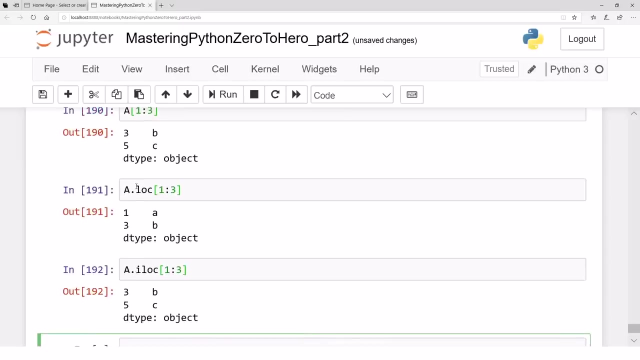 interested in using implicit indices, then it is good to use ILOC function. and now 1, colon 3, is to use implicit indices and the implicit indices are like these. so and like in series objects, you can, you can, you can do the same in data frame objects. once you are using LOC and ILOC, then the further indexing inside. 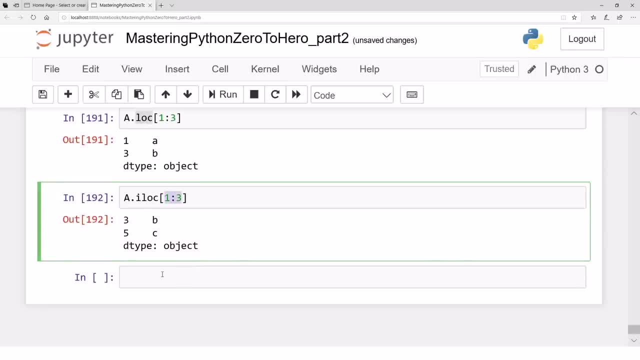 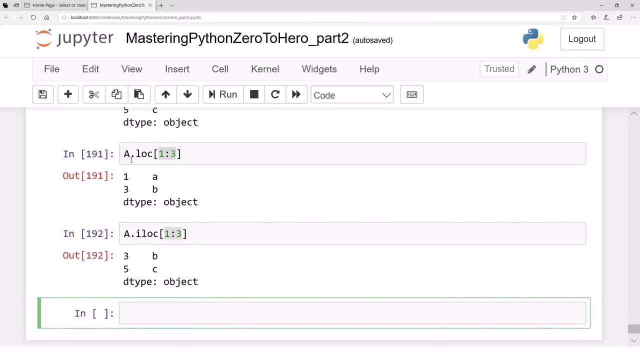 these square brackets is exactly the same like numpy. so whether you use LOC or ILOC, the, the indexing mechanism is exactly does. the slicing mechanism is exactly the same, like like you. you you have used in in numpy I mean all indexing that stays the same. lock means you're using explicit index. I log means you are. 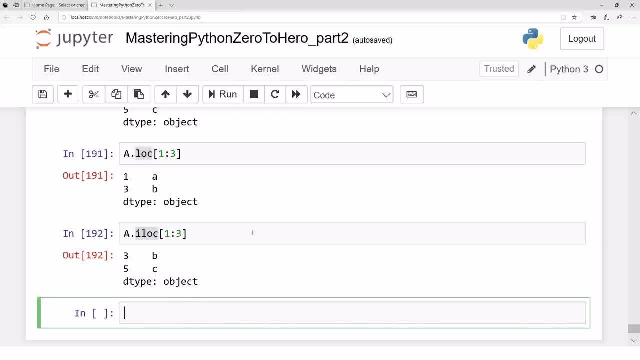 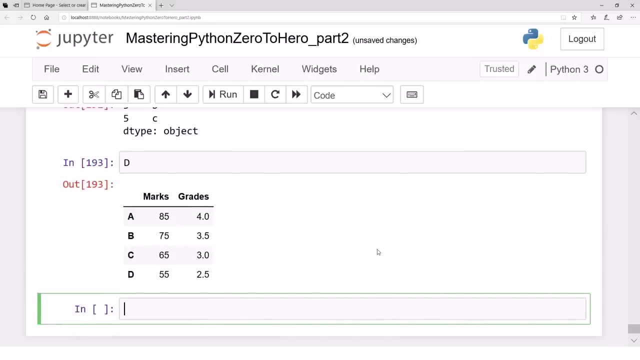 using explicit, implicit index. let's say, for example, we have our data frame, I guess D. that's our data frame available to us. let's say I want to access D dot I log. say I want to access the second row completely, the second record come oh the. 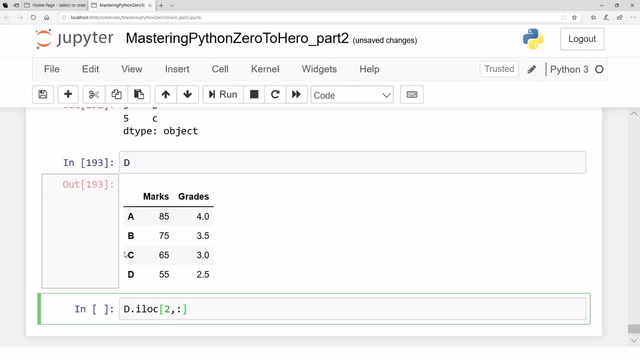 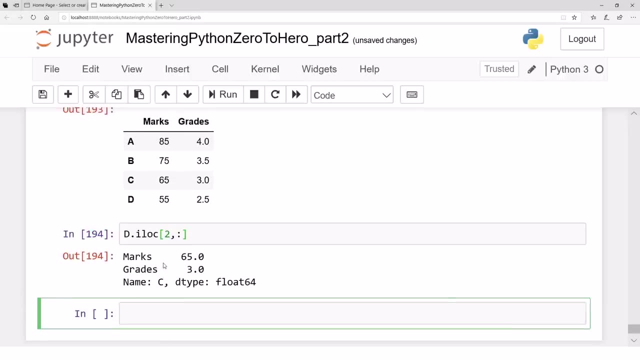 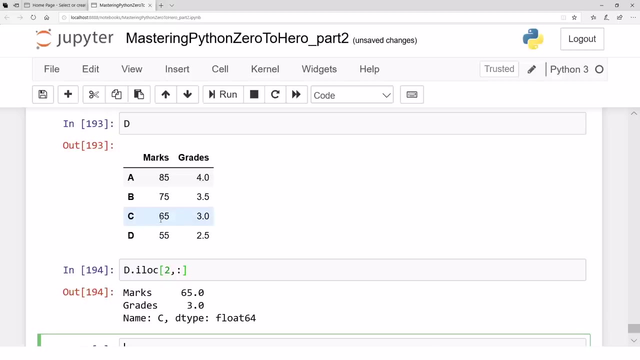 record that is indexed at. look at index at 2, which is a third row completely. let's say, I want to access that now this 2 is acting as. this 2 is acting as, for example, if you see the, the second row, or the, or the row at the second index, which 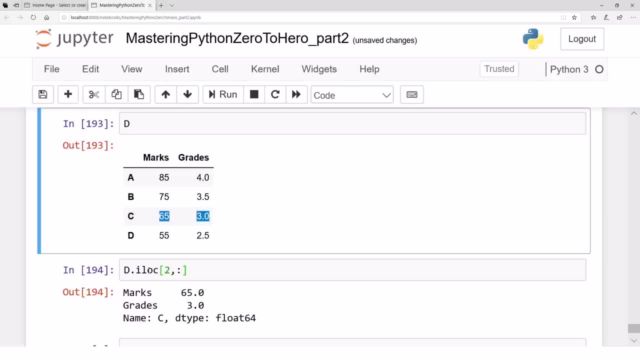 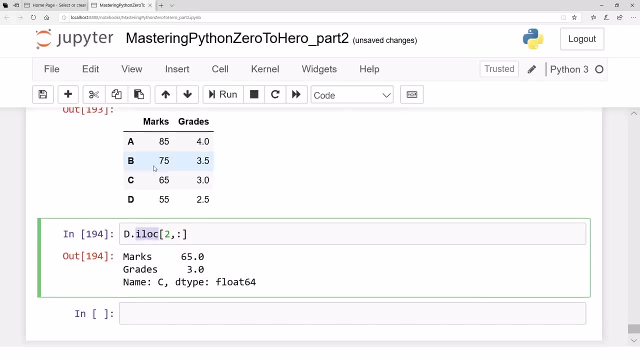 is a third row. that is completely this and it returns that once you have used I lock, for example, and mostly people use I lock, sometimes lock is also required, but I lock is just to explicitly mentioning that I'm using. I'm going to use the implicit indexing scheme again. you can consider hold that thing as a. 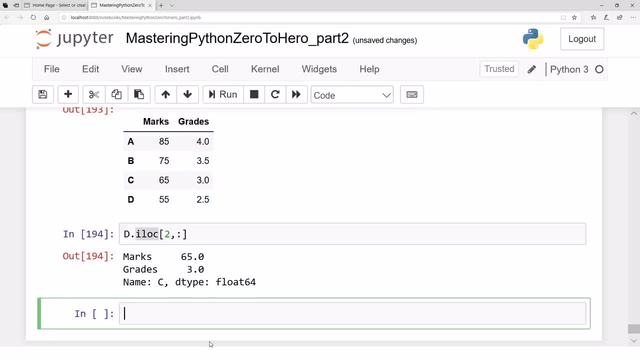 matrix. and once you have applied this, I lock. then you are free to play with the indices like you play with two-dimensional arrays, for example. I want to, for example, to reverse, for example, all the rows and I want to reverse all, the all, the all, the structure, for example. let's say, I want to do that, and and you can see. 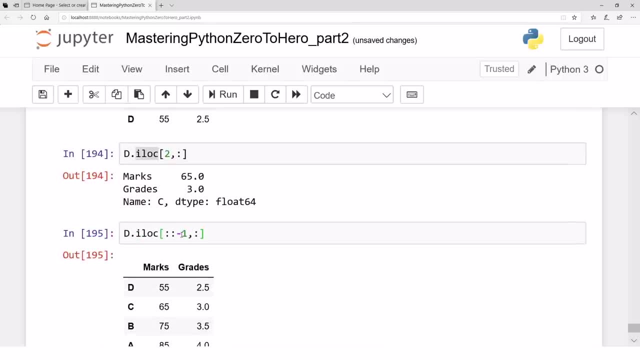 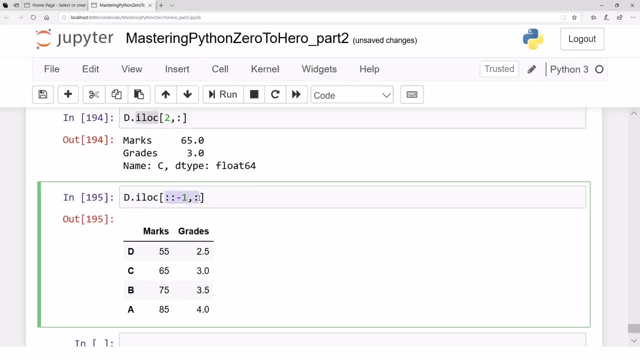 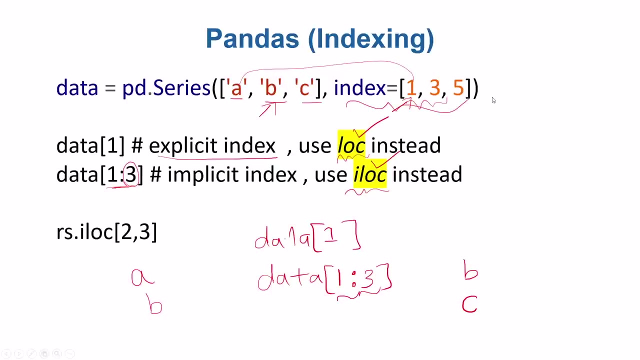 everything is reversed. I mean all the indexing, like like nine by all the indexing is there in, in, in pandas. I mean, once you have used I lock, inside is just just remember the numpy indexing and everything like so. okay, so that's the lock and I lock function. in the next video we are actually going to going to just 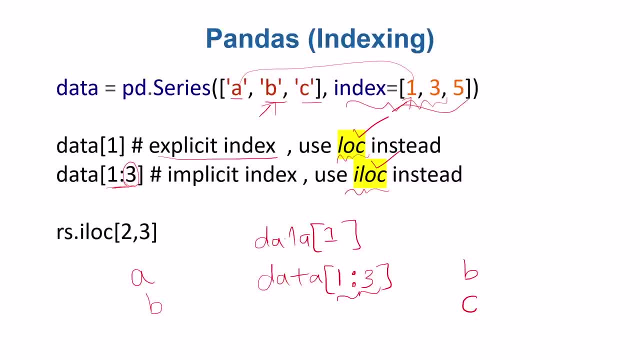 practice the pandas to, to actually to actually work on a data file that is saved as a CSV file. so we will. we will show you how to, how to actually at how to actually manipulate, read and write the data and play with the data that- the real data that is there in in some of the other things that we are going to do. 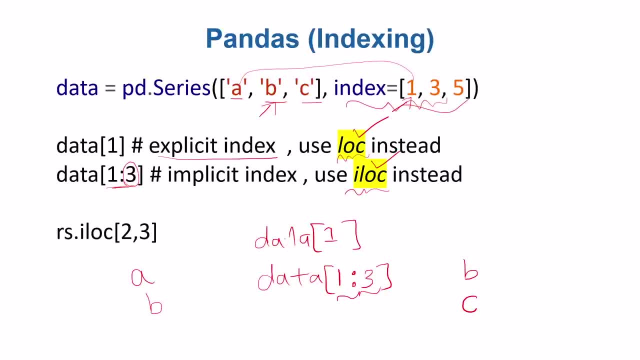 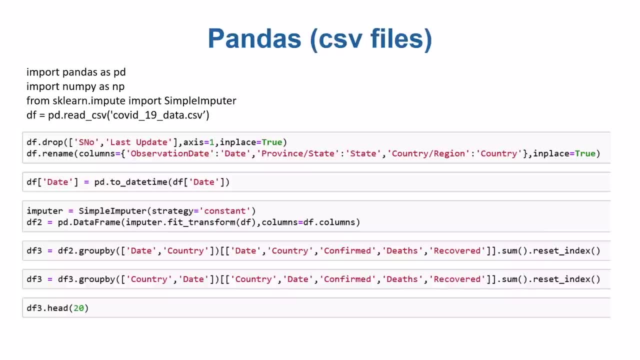 in some CSV file and how pandas will help you to to manipulate the data very efficiently and very quickly. so hope to see you in the next video. okay, in this particular video I will be talking about a real data set, the data set I have chosen just to show you some, some functions that are available in pandas. 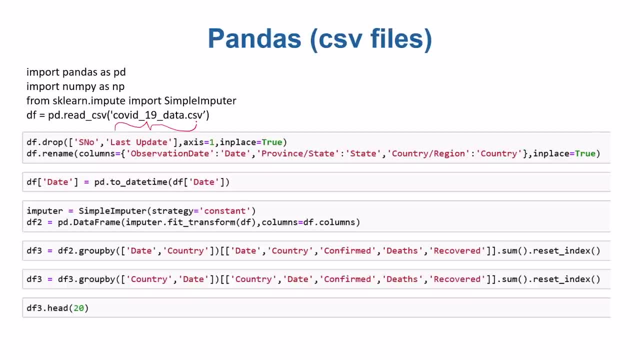 to work on real data set, the, the data set I have chosen as kovat 19 data set. I will just show you in this particular video: I have chosen it as the actual data set. now, please, for those of you who are not familiar with that data set, I am: 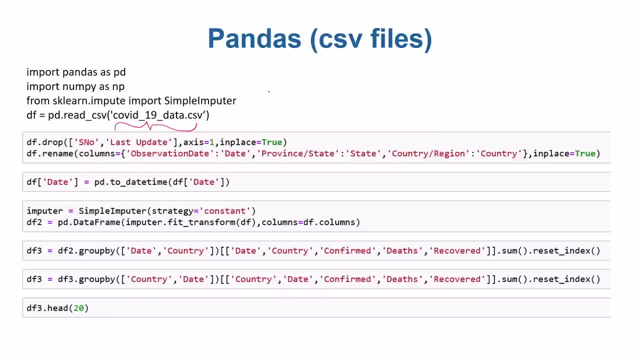 the data set that was first used as a AES data set, which is a set of data sets that were already used in the previous model. the data is a set of data that was available in Kaggle and it's a real data set that contains information of: 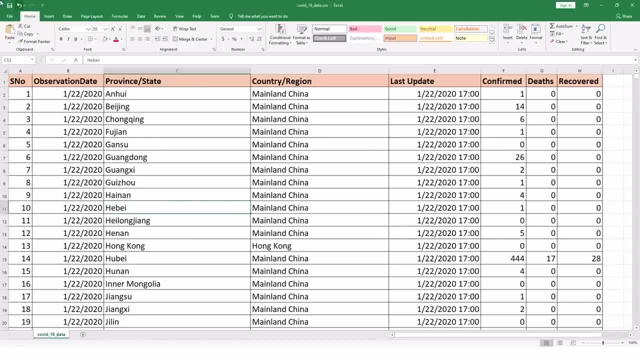 victims recovered, the total number of recovered people in per country, per province, the total number of died people and the total number of reported people. number column that contains the, just the record number, that's. that's a column called observation date. that's a date that's a province or state. that's 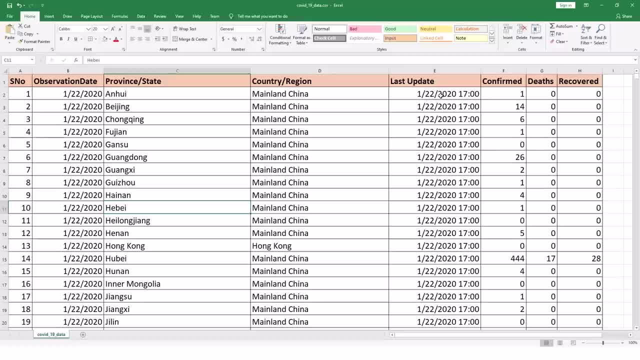 country or region. that's a last updated. when the record is updated, what's the time and how many confirmed cases were there at that date and how many deaths at that date and how many recovered at that date. as the date is moving on and on, you will be seeing that the number of confirmed cases and the number of 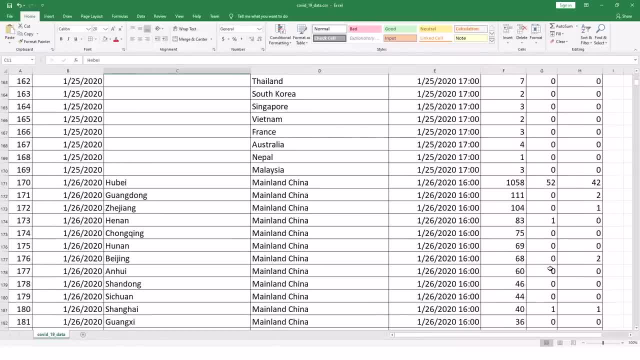 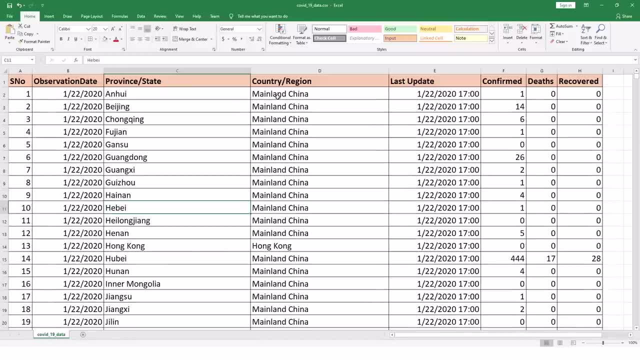 recovered cases, they will be increasing. maybe the number of deaths they also increase. so let's see this data, let's read that data using pandas and do some manipulation of this data and see the look and feel of that data in in Jupiter notebook. let's go to. 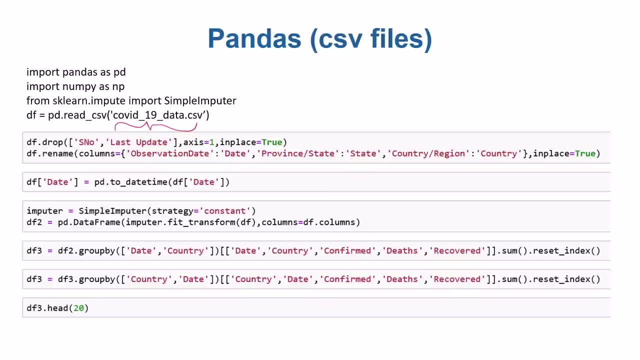 you get a notebook and see. so first of all I need this pandas library and put it that maybe somewhere I need this numpy library as well. I'm also loading a scikit-learn sklearn library because I want to. I want to use impute function just to handle the missing values. it is just more powerful to use the. I mean the. 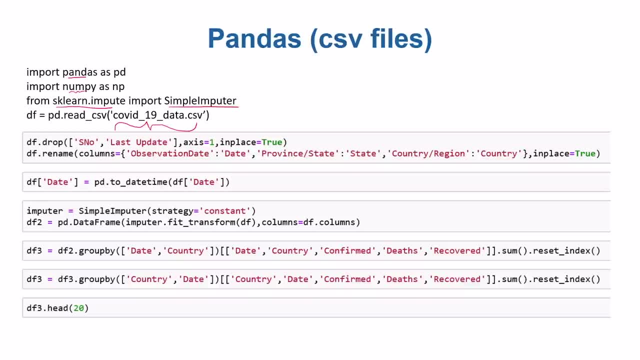 sklearn library that is also a data science library, a package that is particularly a machine learning library or package that actually gives a better sport or a larger support of handling missing data, although here I have used this sklearn function just for an example and but but I could have used this data frame, fill any function or 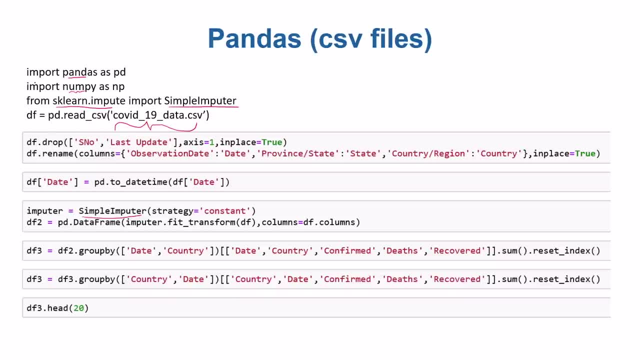 something like so, but I'm just using that one. okay, after importing all these, what I did is I just call pd dot, read CSV function and I load that data and then I did this stuff one by one. let's, let's, let's spend some time on all these. 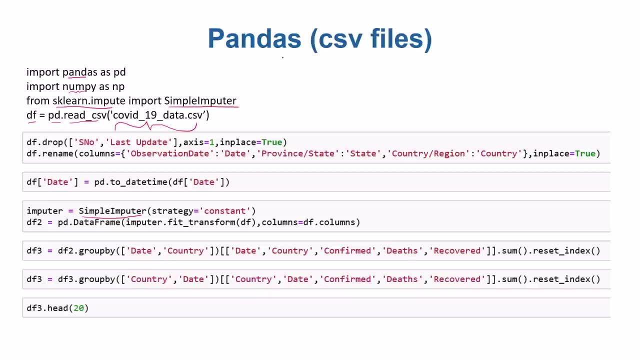 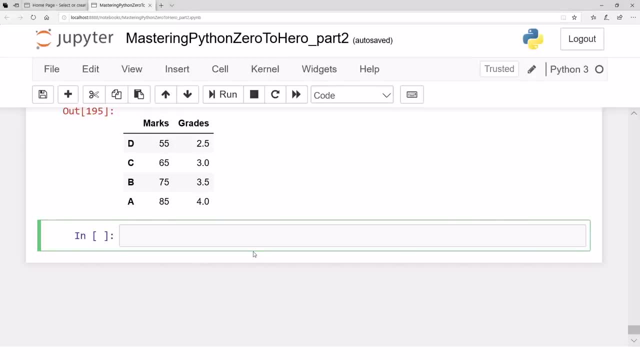 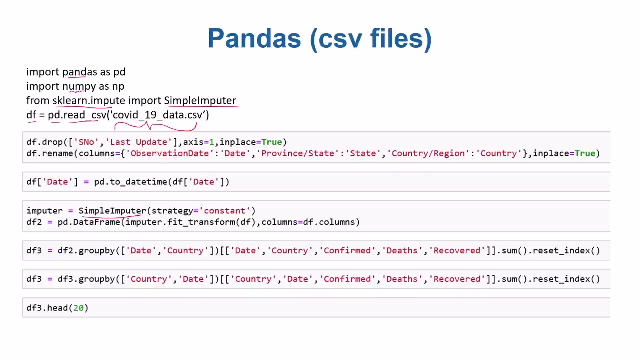 commands one by one in and let's see in Jupyter notebook what is happening. let's go to Jupyter notebook and actually read that file and do whatever we are doing here. so first of all, import numpy that is already imported. import, for example, pandas, that is also already imported. then from SK learn daughter, impute. 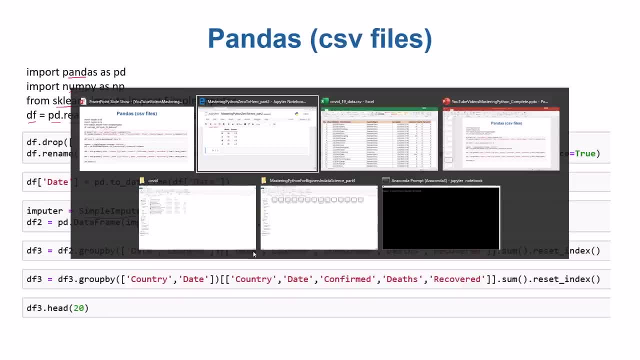 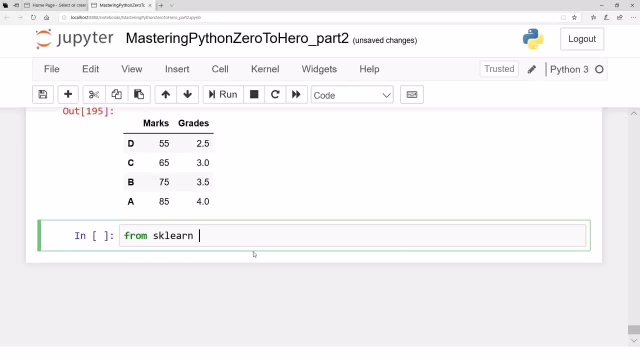 import, simple impute er. so let's, let's use that, all let's. ok, let's do that from SK. learn dot impute. sk, learn dot impute. import, simple impute er. OK, Meteor, okay. so what we're actually doing here is: we're she Kleoc q-spell. p o a T. 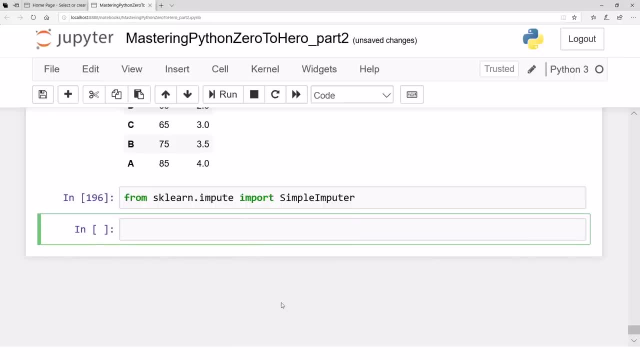 import that because that's a new thing. we need to import that now. read the data. for example, data frame in df. so df equals pd dot. read csv. there is a csv file, read csv and it contains the path of the file. the path is located in my directory. it is located at this particular. 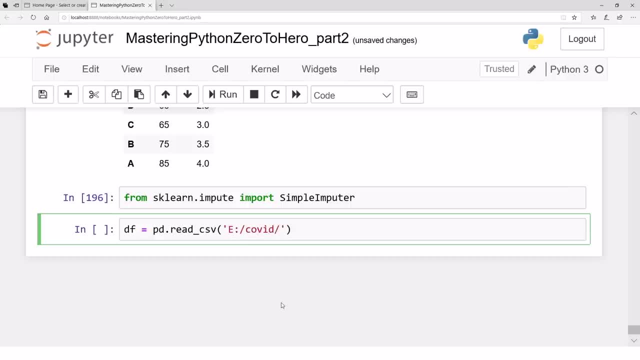 location: covid, and the name of that is covid underscore 19 underscore data. so covid underscore 19 underscore data dot csv. so let's read that file. uh, the file will be read, if you just see that some of there is a function, let's say head, that gives the top records or the records that appear just 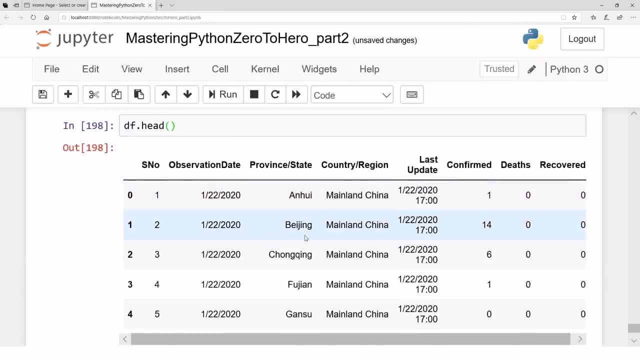 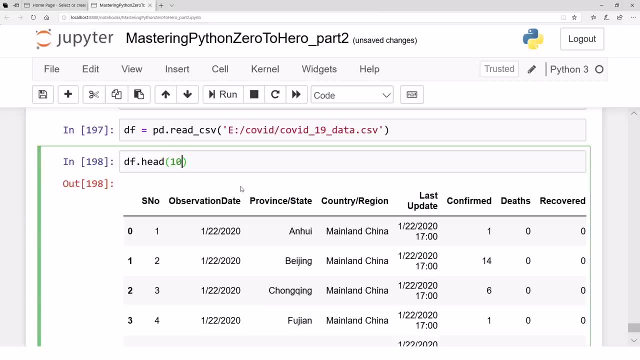 in a very top. that's. that's what the data file that i was showing you in excel. uh, it is showing just the first five records. uh, i can show the first 10 records, for example, just by calling the head function in this particular way. okay, great, um, let's say i, i just want to remove this serial. 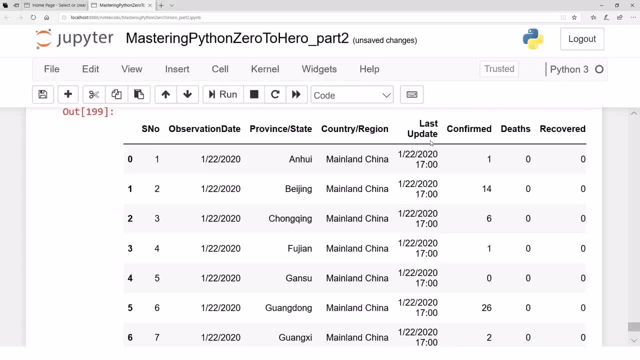 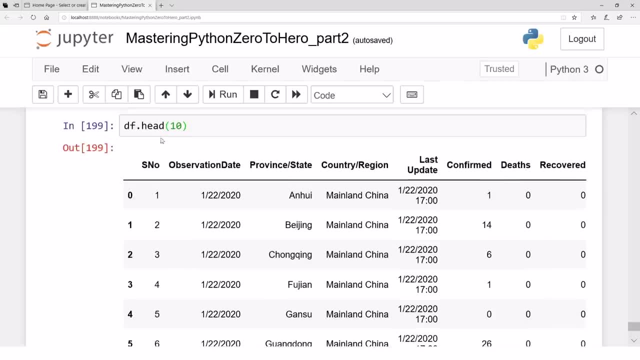 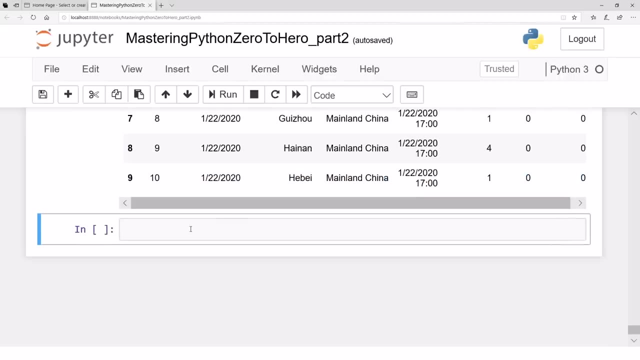 number, because i think that is not required. and let's say, i want to remove this particular column because that is also not required. there are multiple ways of doing that. i can call a del function on this and i can call del function on that, but there is another, uh. 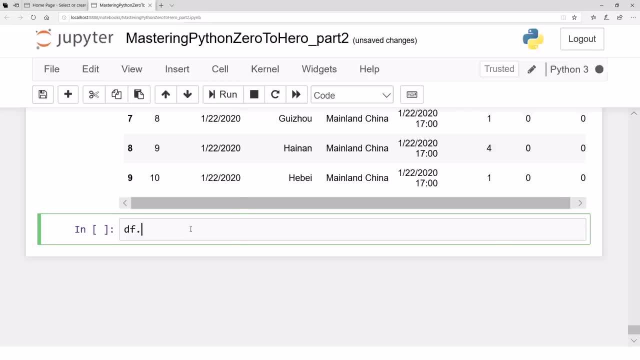 way of doing that by df dot drop, df dot drop, and in that you just give the columns that you want to drop. one column is serial number, i guess. what's the column name? that's s and no. so you want to, you want to drop that column, and then you want. 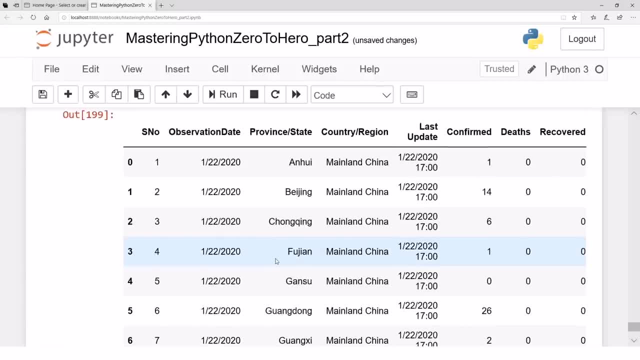 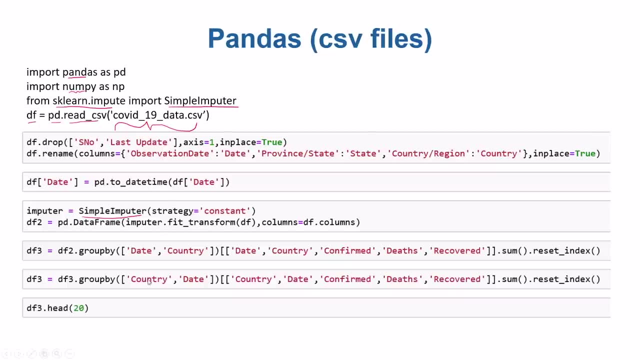 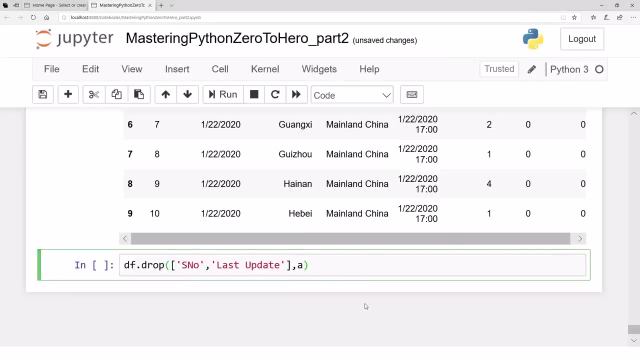 to drop this particular column with having last update. so that is, uh, last update. so that is, i guess what is there? x is 1 in place, true, so access one is just meant mentioning: do do that stuff with columns in place equals, true, that actually is. uh is telling that, whatever this operation is. 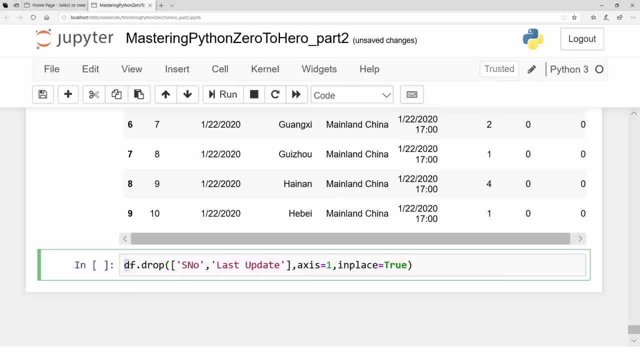 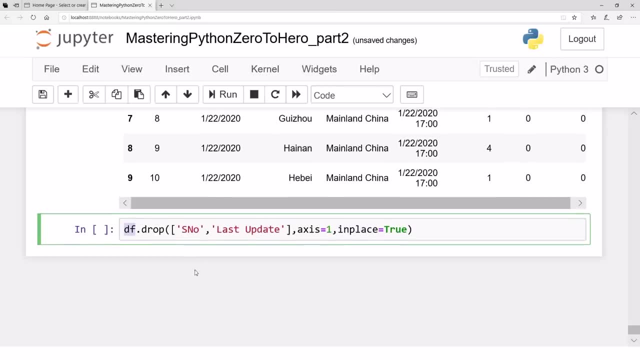 you are going to do reflect the changes in this df frame. if we do not write in place true, it will do everything and return onto a temporary variable or underscore variable or whatever we are saying, but the df, the data frame, will stay unchanged. so in place true means do that changing in df. 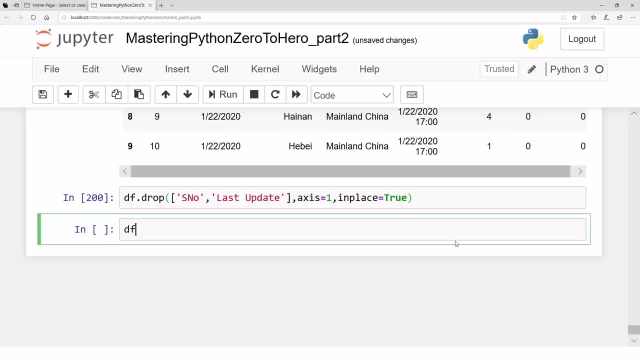 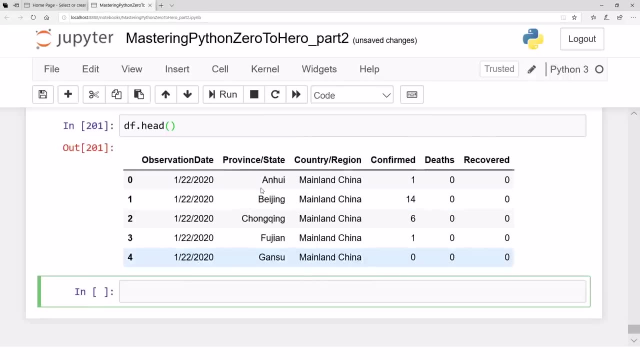 variable itself. so now, if we see df dot head, let's say it will no longer be showing us the serial number column and the last updated column. what next we can do? we may, we may want to rename this, this name to just date, for example, this to maybe another. let's rename all these. 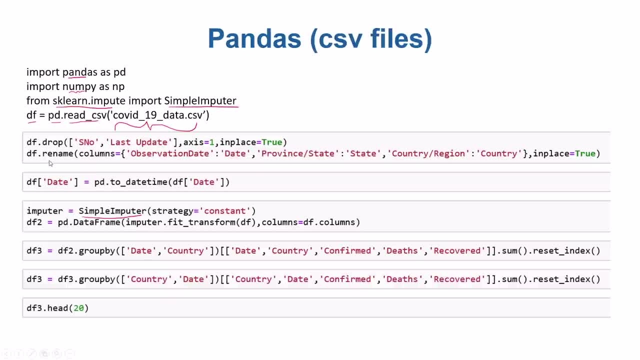 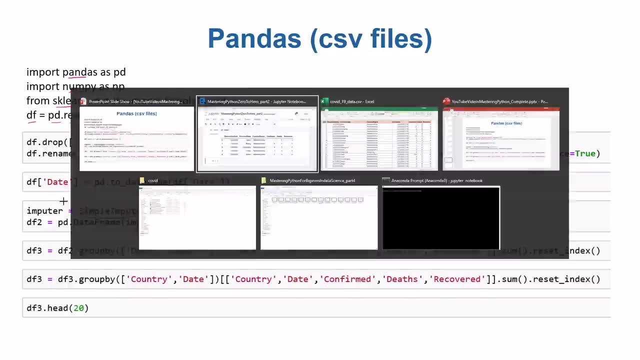 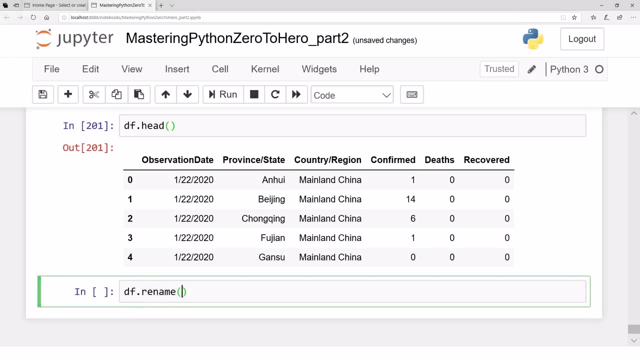 columns using using a rename function: df, dot, rename. columns equals to- and then we have that dictionary again in place: equals, true. so let's use, uh, let's, let's use a, let's use this rename function: df, dot, rename, let's say that. and here we have columns. 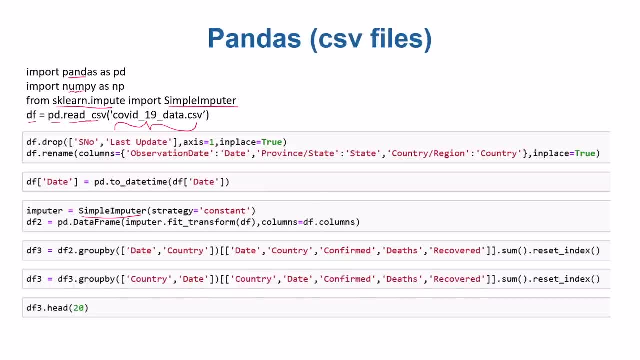 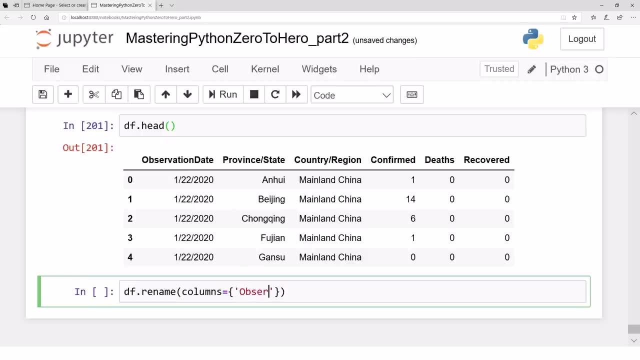 columns, if i spell right, columns, and then that is dictionary. what columns you want to change? i want to change observation date. i want to change that to simply date, let's say. and i also want to change province, province, province, province, state to simply state, to simply state. 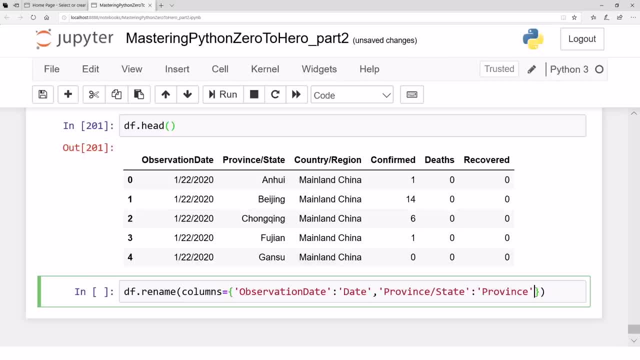 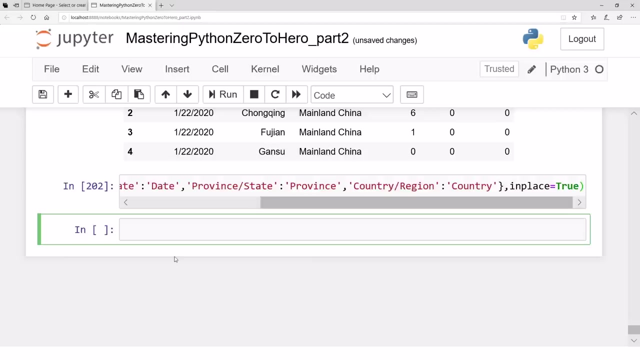 or province, province. let's say simply that. and i also want to change this country slash region to simply country. so maybe i want to change this country slash region simply to two country cu and try country, and i want all that should be happen in place. so in place equals true. so after that, if you run that on this particular step and now if you see, 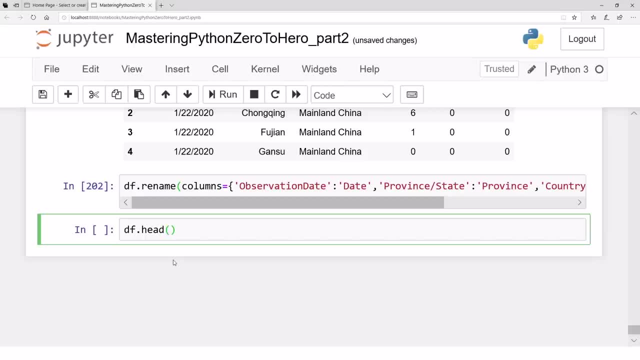 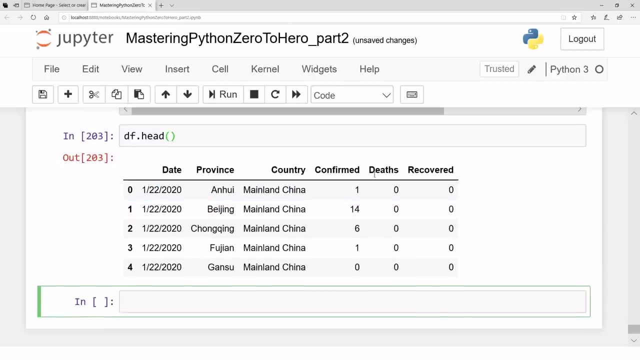 the state of df. you will get like: so okay, these many, uh, so date, province, country, confirmed deaths, and so on. so this is much nicer form than earlier. um, moreover, we may have a lot of missing values. oh, one way, this date format, the date format, is not in a format that. 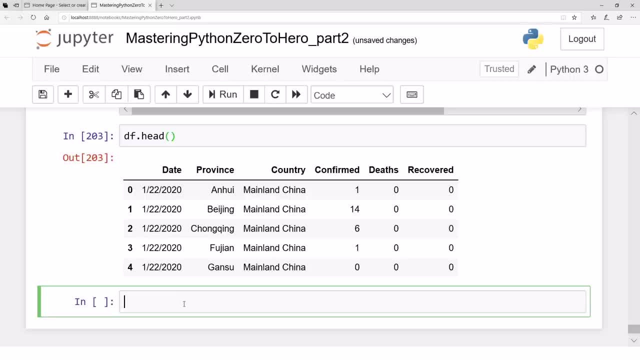 panda's uh internal date format. so let's convert the date format into into into the internal uh panda's date format using two, two pd2 date time function. so let's say df date equals to pd to date time and convert this df date in that particular format. and now, if you 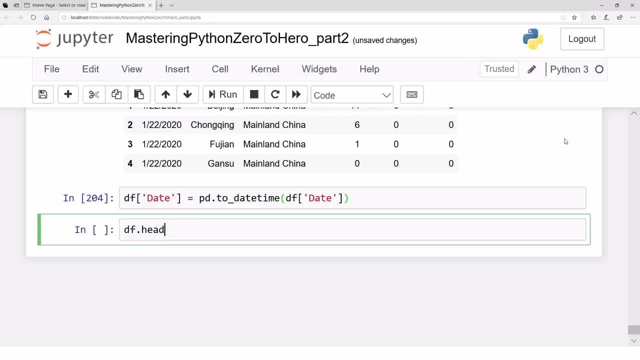 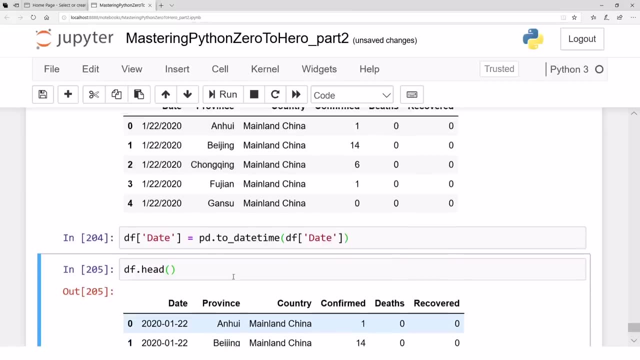 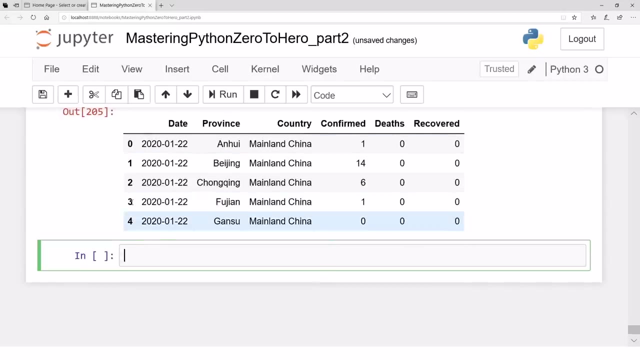 run this df dot head, you might be seeing the date format in a different way. see that that's the. that's a. that's the date format that the uh pandas is expecting now, uh, we, we. that. that is just showing, showing some records. if you want to see more, 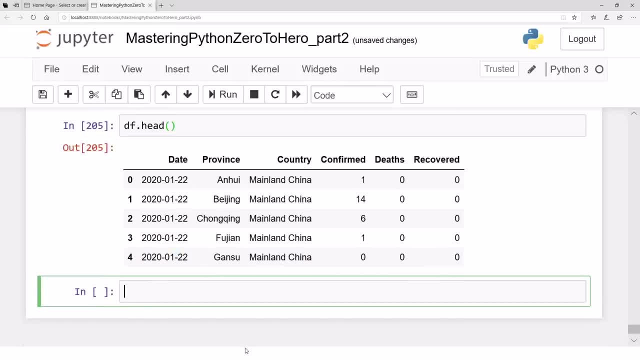 records. we can see those. um. let's say i want to uh, just um, i want to just uh count. or let's say let's just describe all the data in that bit- textbook history data. but i actually want to just to see. um. let's say i want to just um, i want to just count. or or let's say: 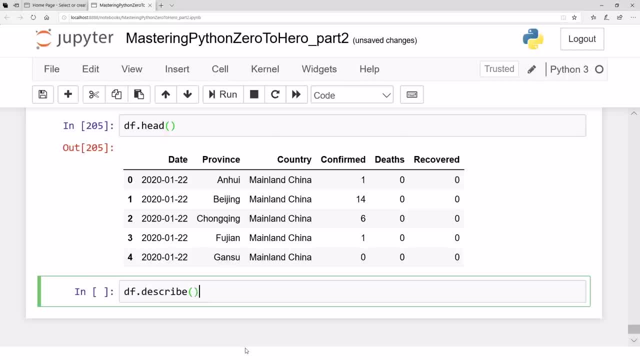 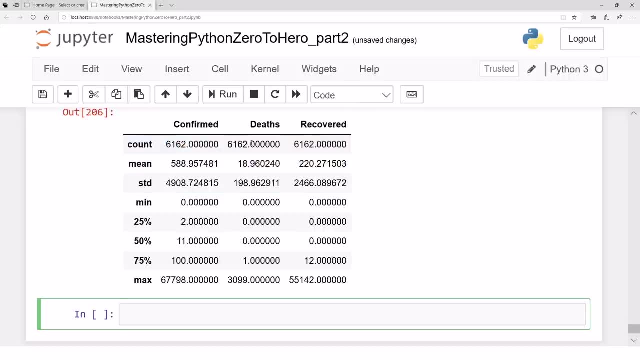 tfdescribe, there is a describe function that describes most of the statistics, of the data. I mean the total count of confirmed cases are these? the deaths, are these? recovered of these? these many columns are there, these many values are there. The mean is that: and standard deviation. 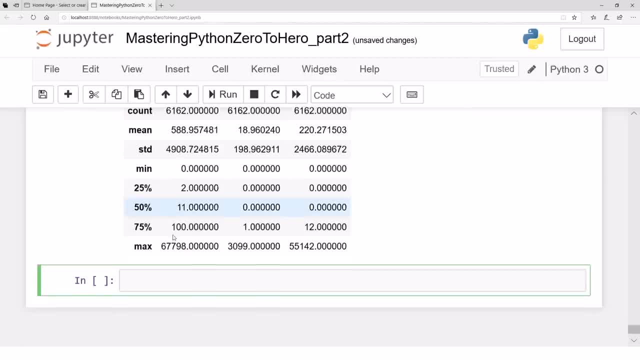 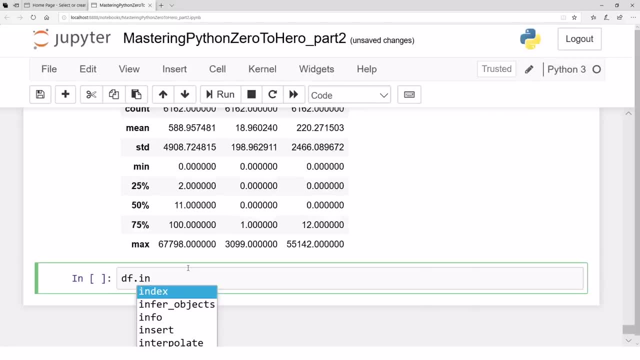 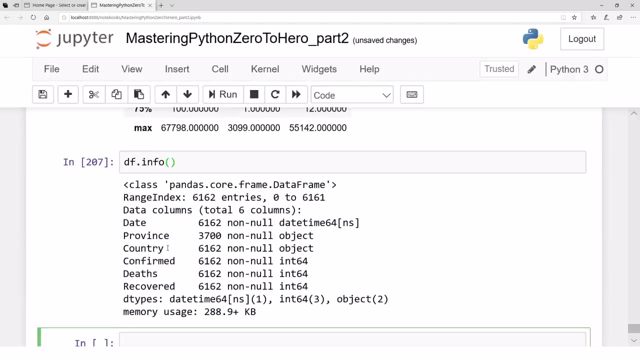 is that the minimum 25, and these are the statistics. Let's say there is another function info, dfinfo. If you call that function info, it will give us the more information about the null entries and the non-null entries and so on. For example, if you see the total number, 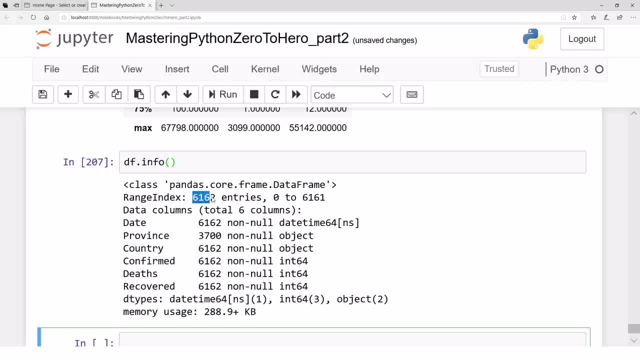 of data columns are six. the total number of records are six one six two. the data entries is always available. The province entries are only 37. The rest entries are null entries. So province entries, most of the entries are null entries. 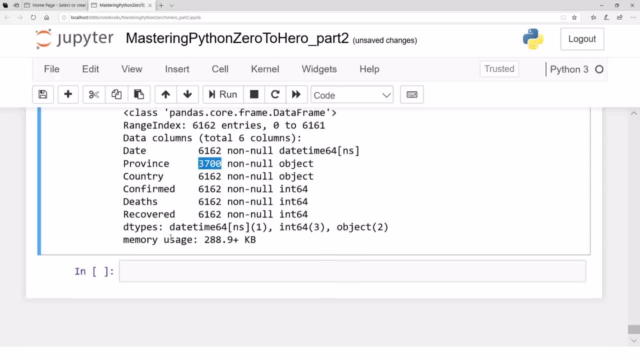 and they are there. Maybe we want to drop those or maybe we want to impute those entries and stuff like so. But there are null entries that are available in the province column. Some of the province values are no longer available. Let's see that here, For example. 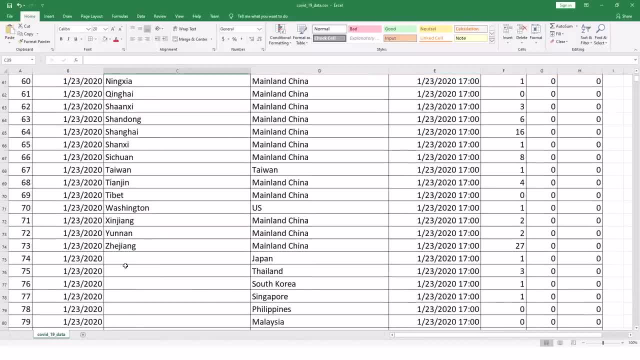 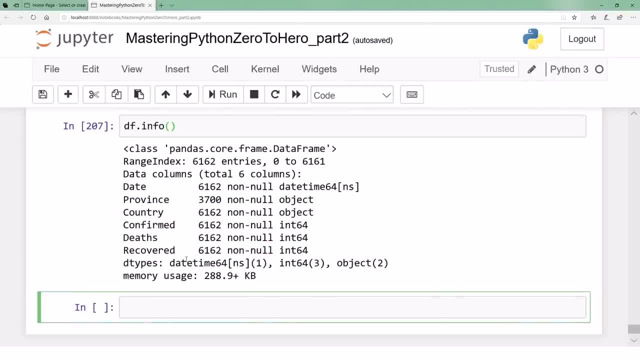 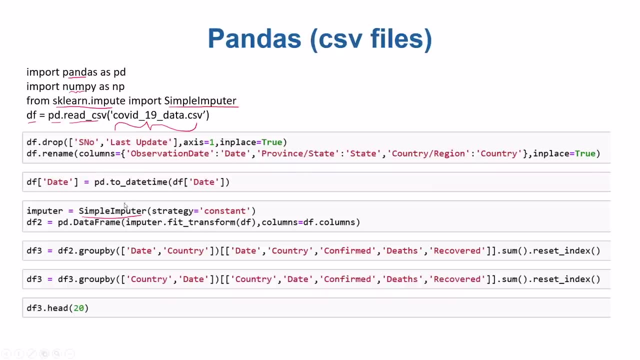 this is not available, this is not available, this is not available, And that's what the real state of the data is. This is not available, this is not available, and so on. So this can happen, Okay. next, what we do is we actually use this simple imputer just to impute the missing. 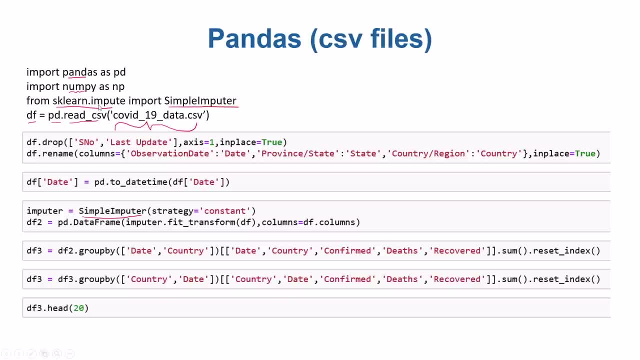 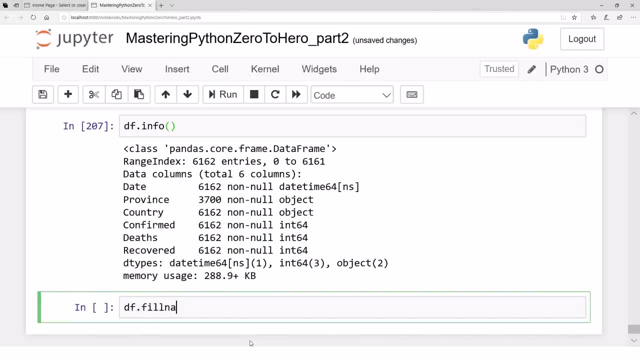 values. One way is to do that using simple imputer from sklearn. Another way is, as we already know, just dffillna, fillna with. let's say with. let's say not available, Let's say string. some string not available, Let's say that string, And with that, if you. 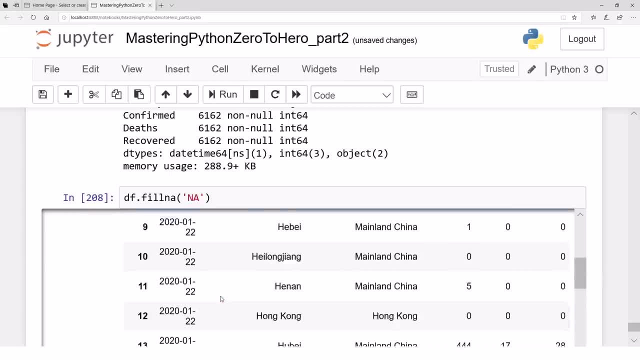 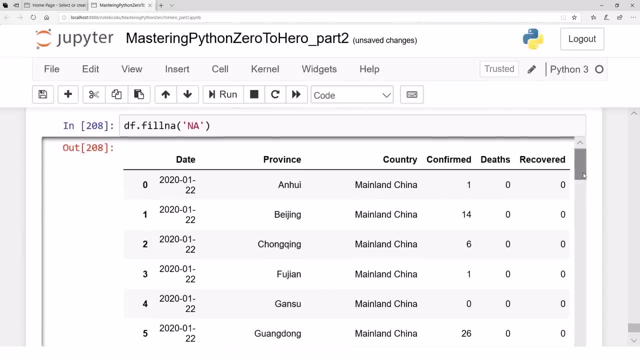 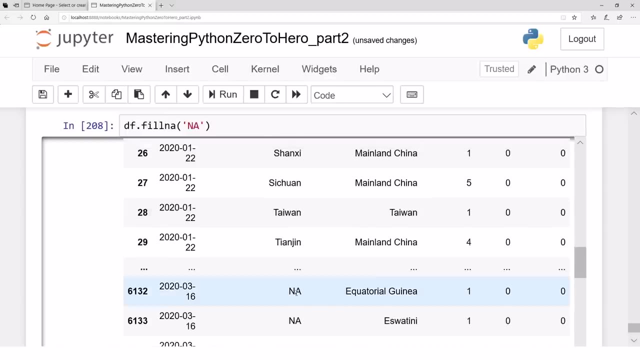 fill that, fillna, using that Now. after that, we will be having all that data. the missing values will be filled according to: let's see some missing values, Because in the province there were some missing values. Now you can see, for example: let me go on. yeah, So not. 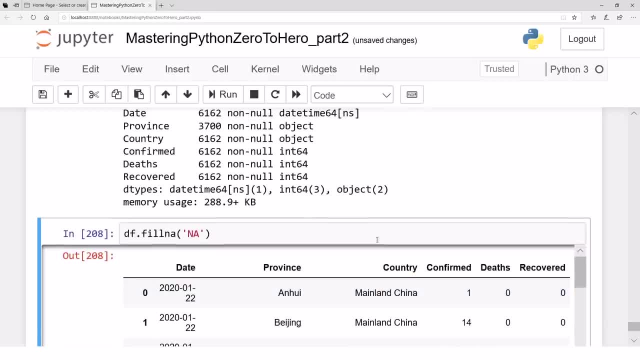 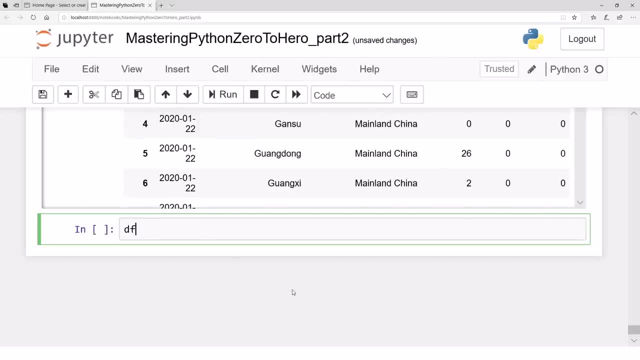 available, not available. We can, we can use that, or we can use a fancy kind of you know rough thing that is available by scikit-learn and so on. Okay, after that, if you now see the information, info now- you will not be seeing any null value. All the columns are: 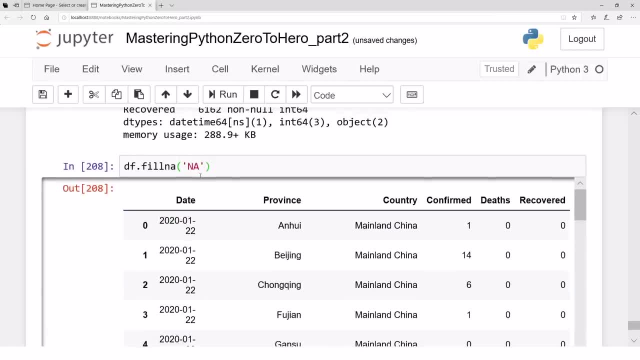 there. Oh, this was not in place. So fillna, that is. and let's change the df with it. So this doesn't happen in place. So, df, just change the df. Okay, df changes Now, let's. 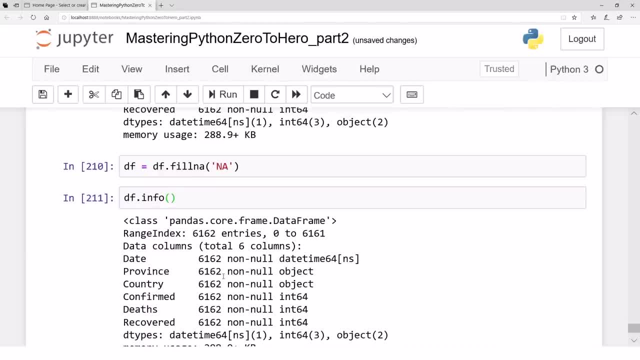 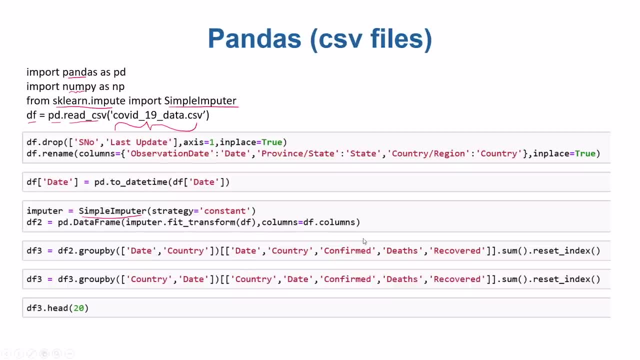 see if we now, if we now call info, there is no null value anymore. Yeah, So I end this video here. In the next video I will show you this group by command to just see these kind of stuff in a more detailed way, because this, this particular video, is getting lengthier. 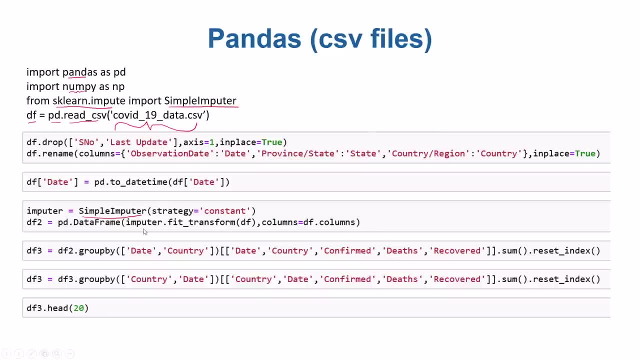 and lengthier. We I'm stopping here in this particular location. Next time I will show you the group by command in the in the Pandas data frame And I will show you what that does. So we will explore all that code that is written. 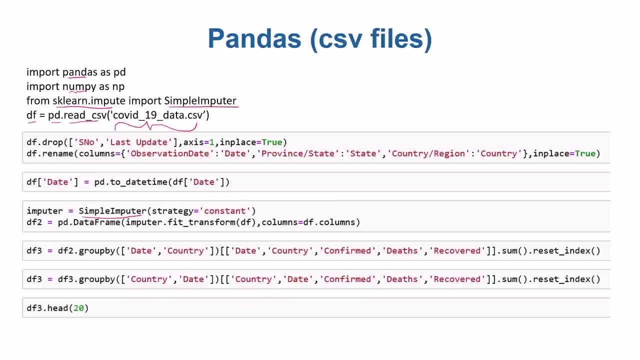 here And we will in in in the upcoming videos when we'll see the plotting and matplotlib. we will be using the same data file to to work more and to get more insight how the how this Pandas and matplotlib and NumPy in combination, how they can actually, how they. 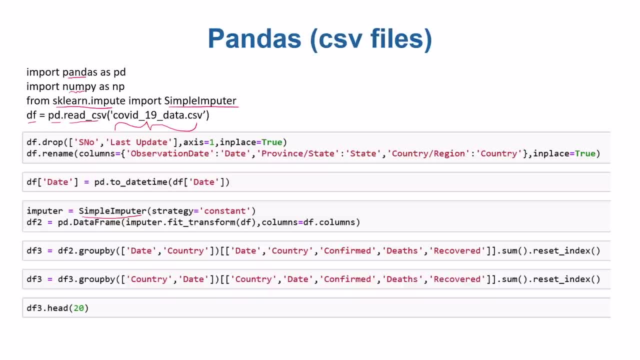 can actually play a very important role in analyzing data. Okay, So I end this video here. I will start the next video right from this command and we'll tell you what is happening. what is this group by command? So hope to see you. 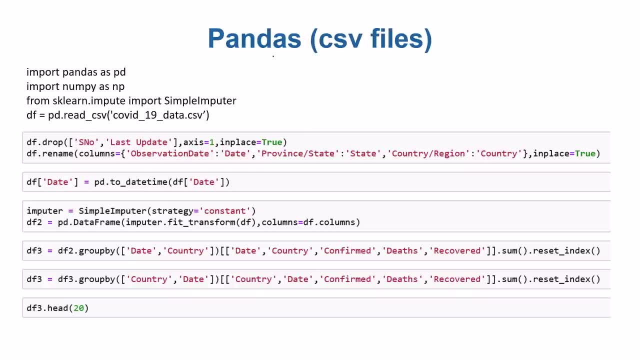 in the next video. Okay, In the last video we were discussing this COVID-19 file and we reached here, but we didn't use this sklearn imputer, We just use the fill, any function of data frame. Now let's discuss this. 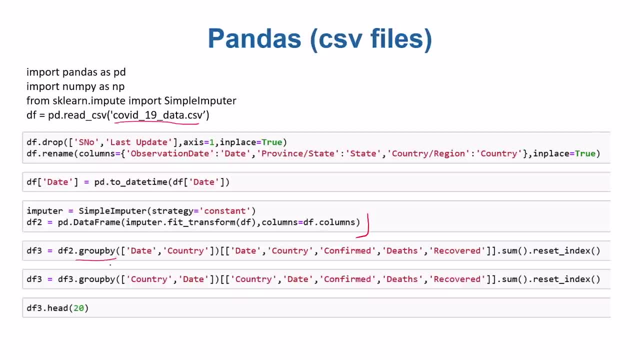 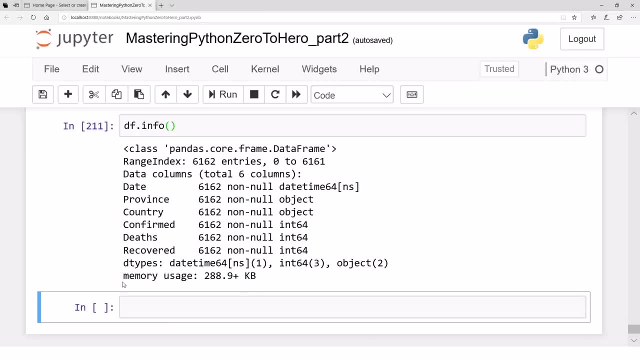 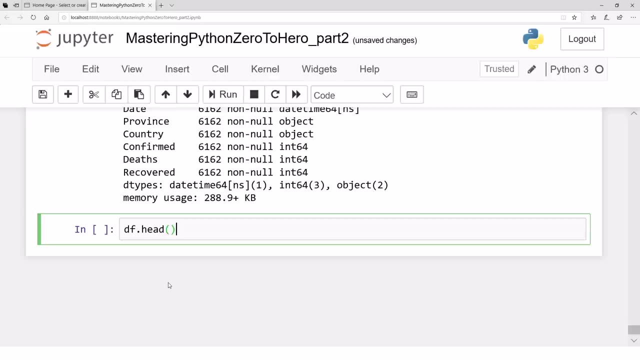 This group by command or a query in in Pandas, that is much more visible. Let's say: our goal is now, for example, if you go to go back to Jupiter, if you see your data dfhead or all that's a dfhead, let's say 10 records, If you want to see that there are so many. 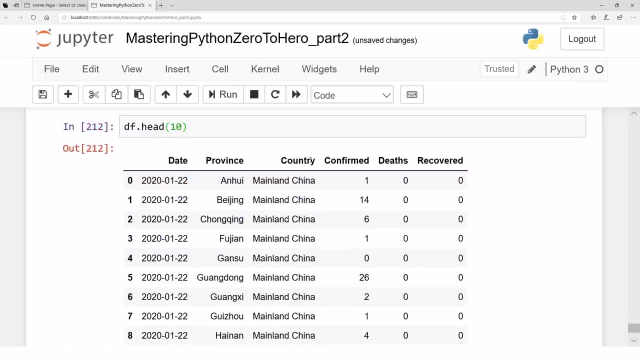 records. let's just see 10.. Let's say what you want to do is you want to just see how many, how many total confirmed cases? Okay, How many cases are there in each country, regardless of their date? And for example, 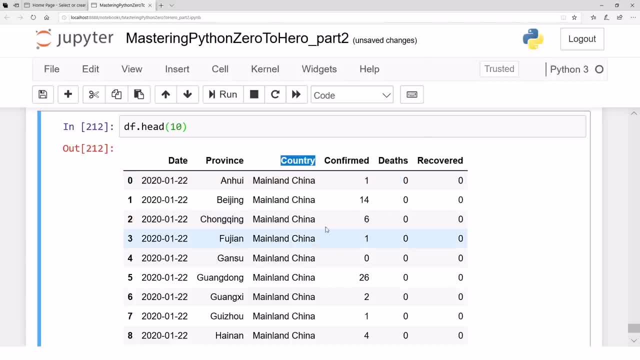 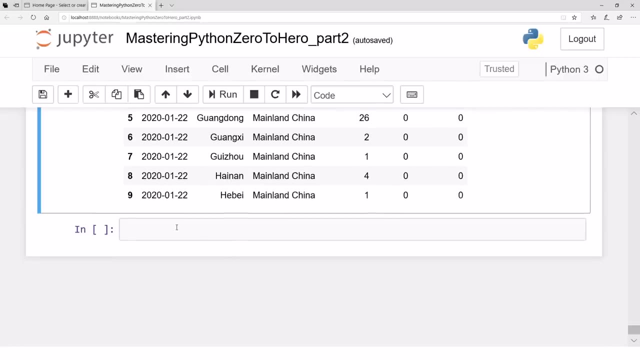 you want to just see all the all the con, all the confirmed cases, all the deaths and all the recovered cases in each country, for all the dates and for all the provinces combined together. One way to do that is to write a group by command. For example, let's say df2. 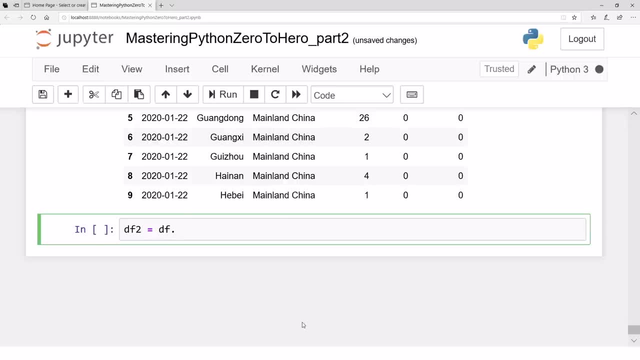 equals dfgroup. Okay, So let's say df2 equals dfgroup. Okay, So df2 equals dfgroup. Okay, This is what you see. Okay, So df2 equals dfgroup. Now you can see what different types of data here. 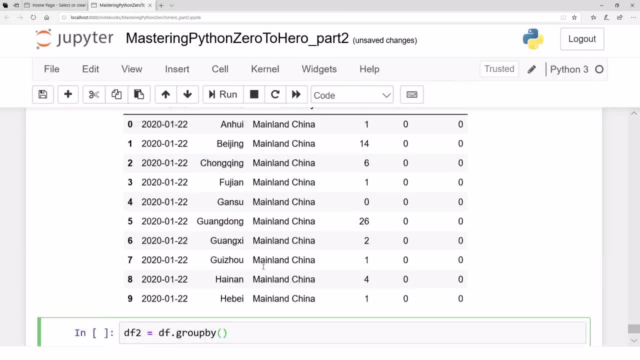 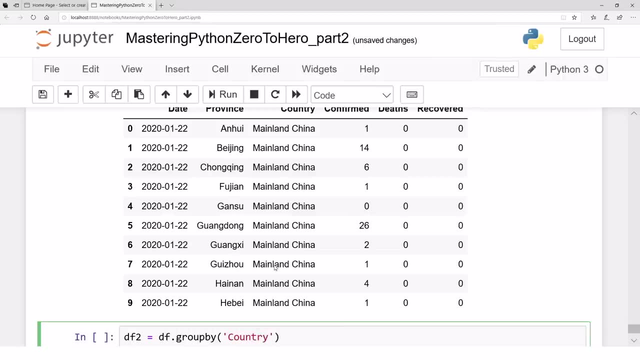 So df2 equals dfgroup. This means that the data is grouped by and in grouped by. what you see is for what kind of columns you want to. you want to group all these, all this data. So, for example, you want to group by country, country, so that's your grouping. 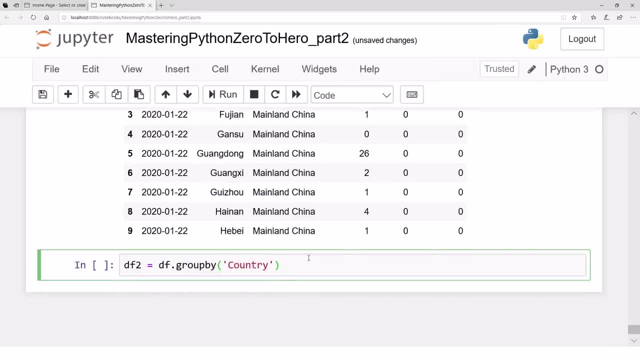 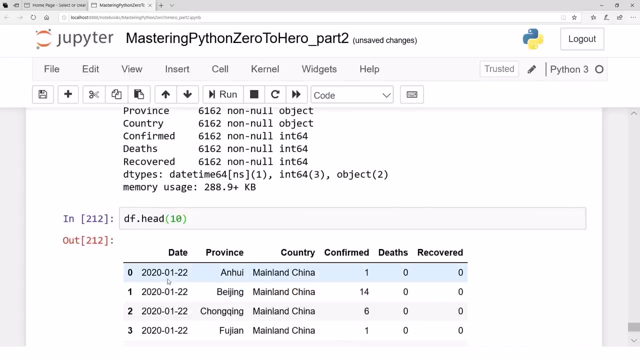 Now, after grouping, what do you want to see? what kind of? what kind of? what kind of, for example, the values you want to see, because now you're grouping. Well, after grouping, I wrote: really want to see, because date is gone. once i group all the dates, they are grouped together. 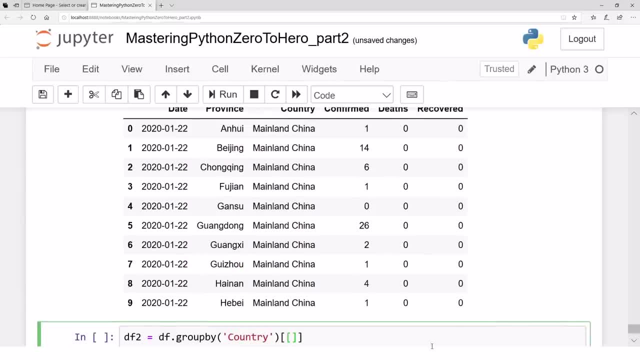 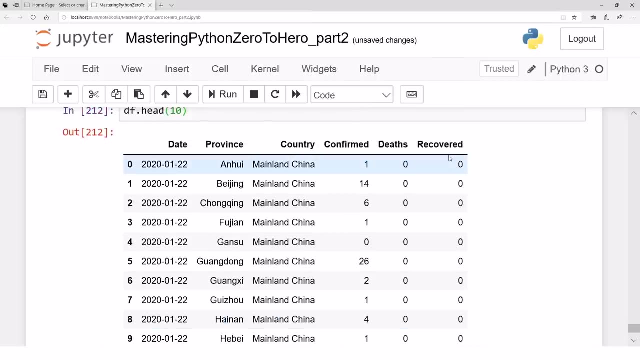 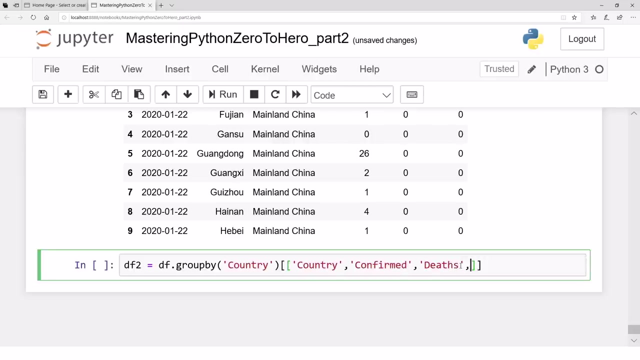 all the provinces that are grouped together. so what i really want to see is just the country and i want to see the confirmed cases. so pick all these records confirmed and then i want to see deaths and recovers, for example. if i want to, that's uh and let's say, then i want to see the recovered cases. are e? 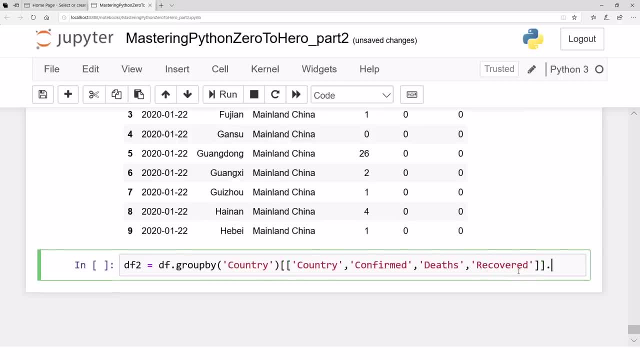 and just, i want a pick group, all the countries together, group all these things together and add all the records under each country. so some, all of them. and maybe we want to reset any index if it is not available there. so, for example, reset, reset index, so that thing. so after this query, for example, is grouped, 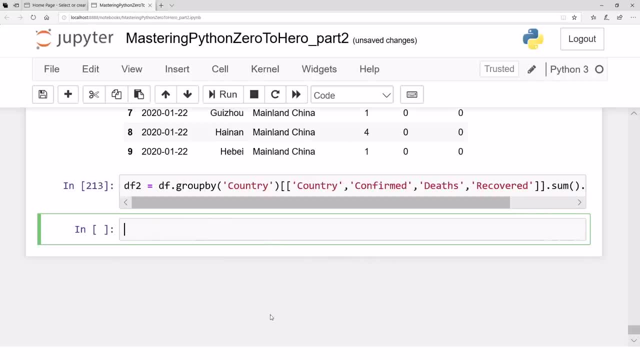 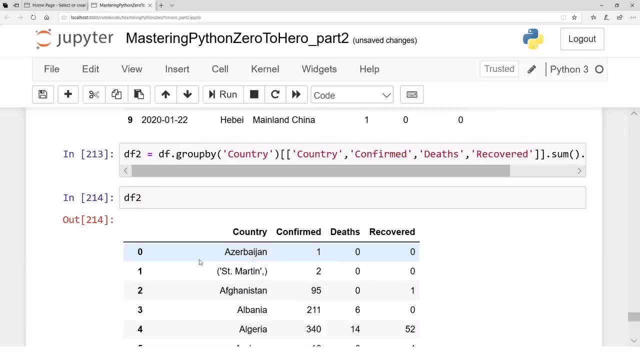 by query. what will happen is this: df2 will contain a summary of the data with respect to each country and the total, for example, in this particular country, the total confirmed cases. are these all the confirmed cases till now and the deaths of these and recovered as these for this country? 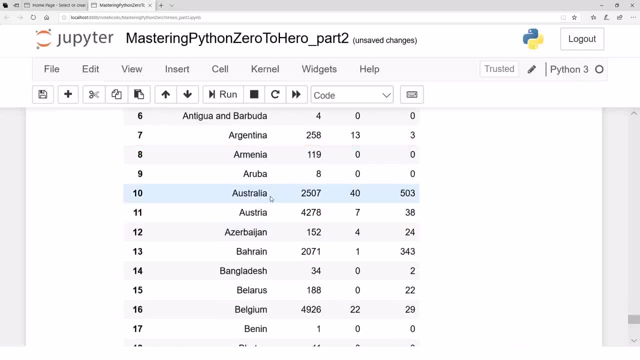 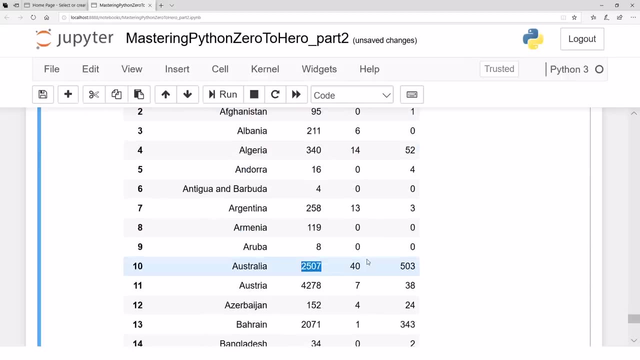 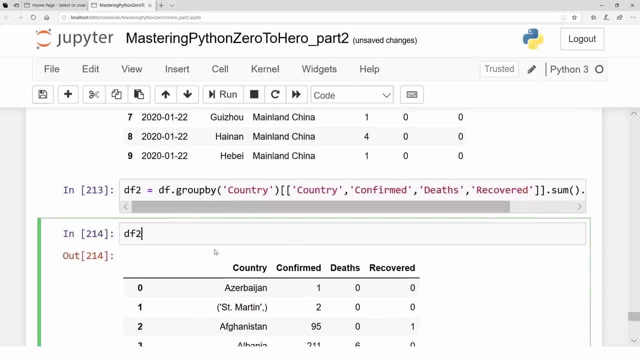 for each country. now each country is describing australia, for example, uh in all till till now australia has total, these confirmed cases, these total uh deaths, and these are recovered cases and so on. so that is, if we want to group all these with respect to country, what if we want to group? 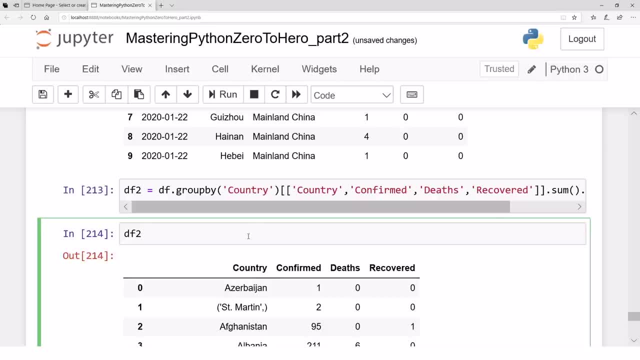 all these with respect to country and then date, for example. so first we want to group them by country, so country, and then for each country display all the dates and then do the, the same stuff. um, the, the query will stay almost the same. a group by command will say almost the same, with one kind 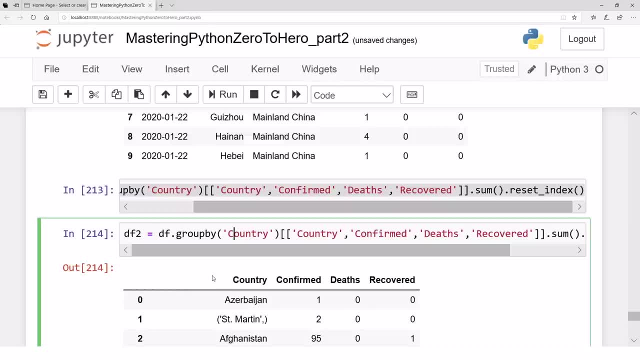 of uh, with one kind of. let's say, we want to first group by country. once the it is grouped by the country, then i want to group them by date, and now i want to see all the results in the form of. i want to see the date as well, and what will happen now is for each country. 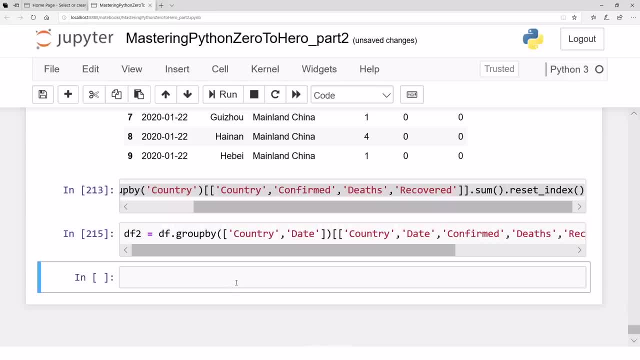 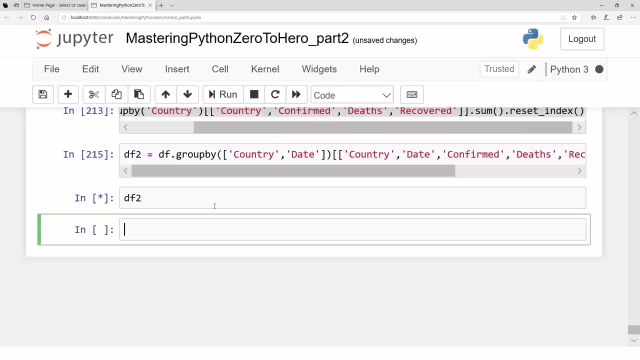 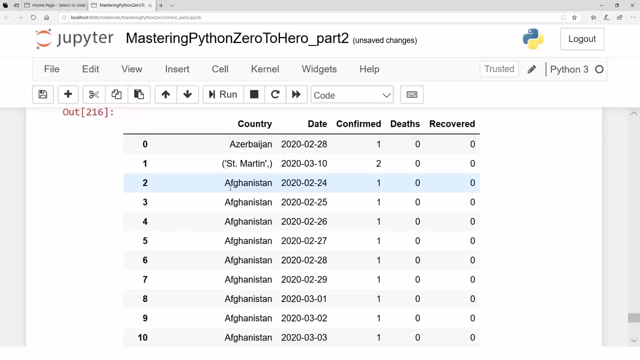 it's trend with respect to all the dates that will be displayed here. so let's see df2 now df2. so if you see df2 now, you can see, for example, this particular country, it has just one record. then this country has one record. then this country for this date has this record for the same country. 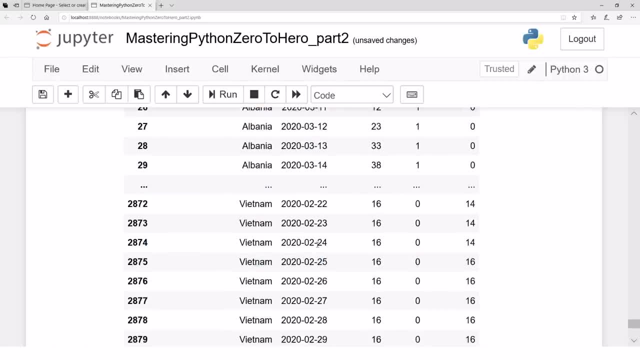 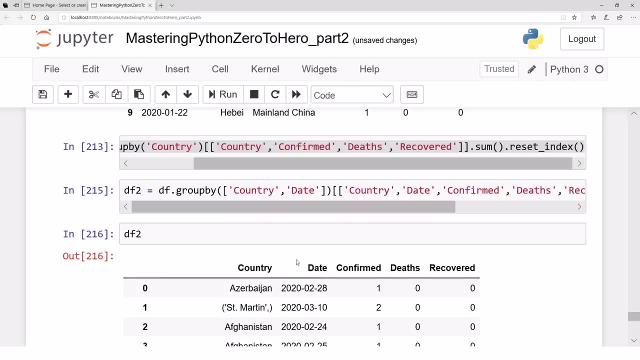 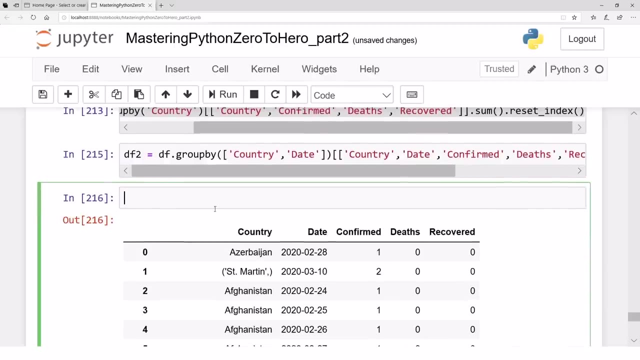 so if you see df2 now, you can see all the records in a very incremental way, so that may give you a very good look and feel of what is happening. or or, for example, another thing: what if you want to- uh, what if you want to, for example, find out all the records, all the records? 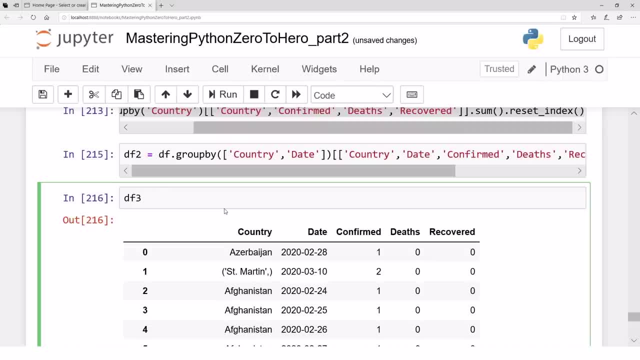 you just want to find out all the records- that's df3- for which the the confirmed cases. for example, the confirmed cases are um, are more than a hundred. let's find out all the records. let's, let's, let's, let's get just, let's just pick all the records for which the confirmed cases are larger. 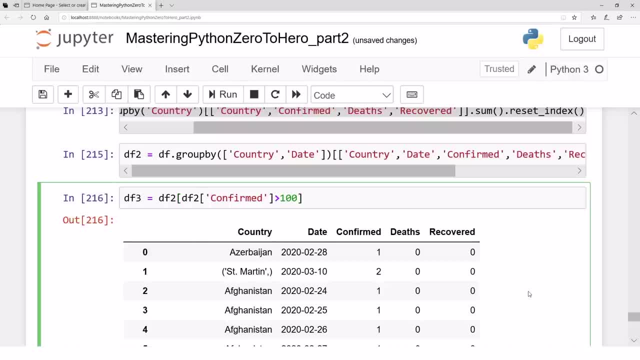 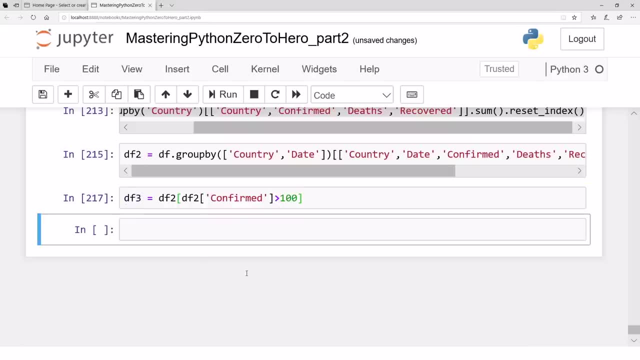 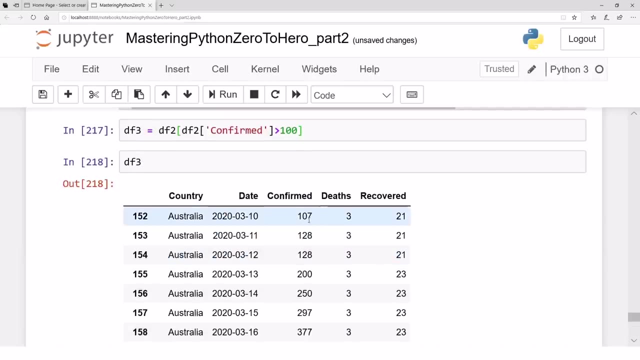 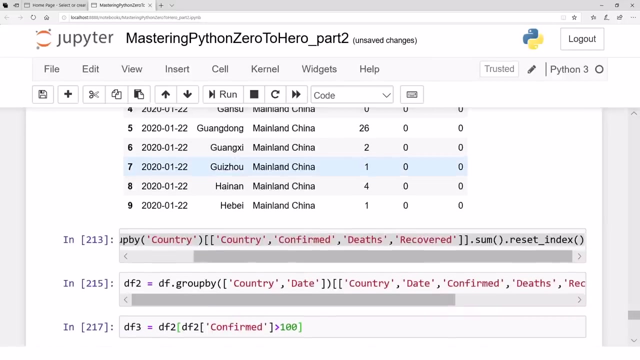 than hundred, and let's copy all these records, just those records in this. so if you do that, we have df3 available and we have df3 this. these are just the records in which the confirmed cases are for sure larger than 100. just those, um, yeah, so we can do, i mean, a lot of, a lot of data analysis, the real data analysis, a lot of. 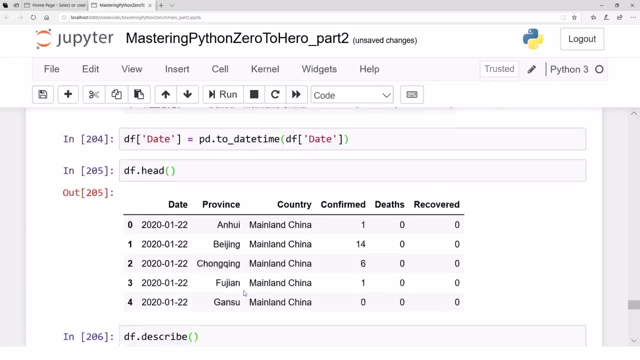 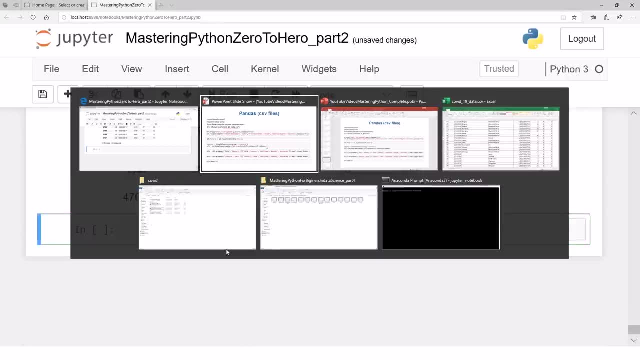 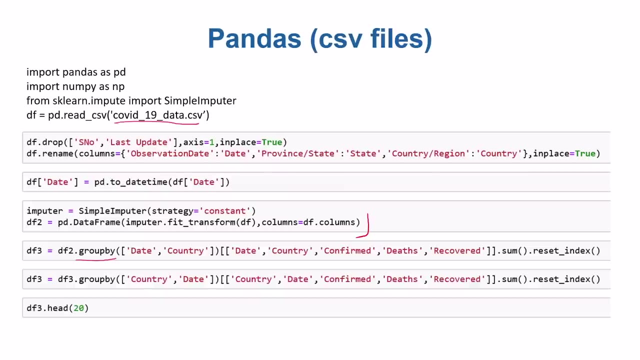 a lot more. i've just shown you a very small snapshot of what we can do with pandas. on on the real data set. i mean, there is a lot more that we can do with this pandas library. um on on real data sets, on multiple data files, combining them together, joining them together or seeing their 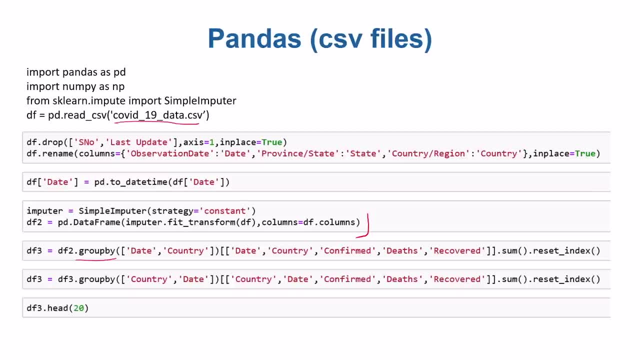 correlation, a lot of stuff, and this pandas really is a very, very fancy and very high level library, very high level package to work with data. so, um, due to time limitations, i'm just ending this pandas here, although there is much more to explain in that. but in in the next video we will be 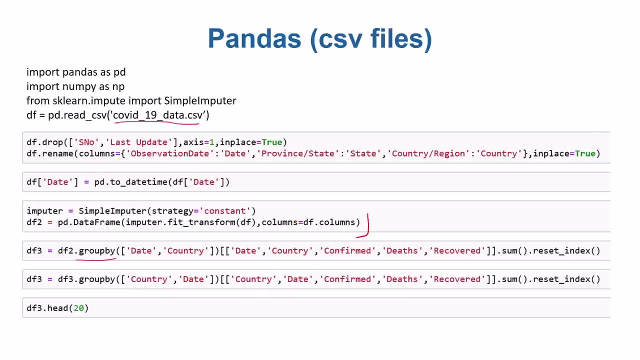 jumping towards matplotlib, just. we will see how to do that in the next video. so thank you very much and thank you for joining us today. we will be moving right to our next topic, which is matplotlib, and we will see some, some functions of matplotlib and we will see very briefly how. 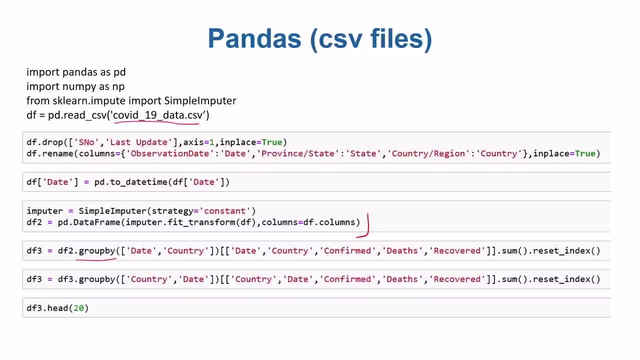 can we plot, how can we analyze data using visual graphs or stuff like so, so that that sometimes this visualization of different attributes of the data give very good insight to the data wherever possible, wherever possible or the visualization techniques are in a way that you can visualize the trends in the data. 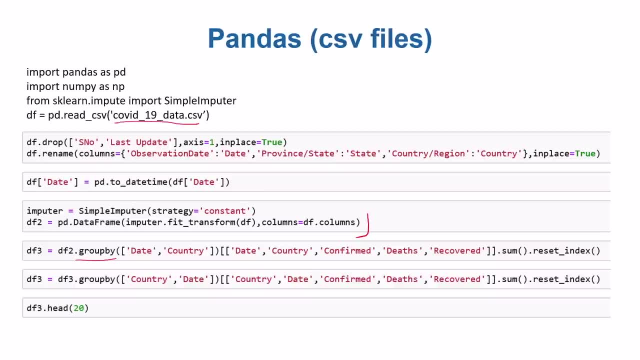 that gives you much more, much better insight than the numbers or statistical results. but it completely depends in what situation you can visualize the data. there are situations- high dimensional data, for example, is not always visualizable, so in in those cases the statistical results or the numbers may play a more important role, but in more in many cases, visualization. 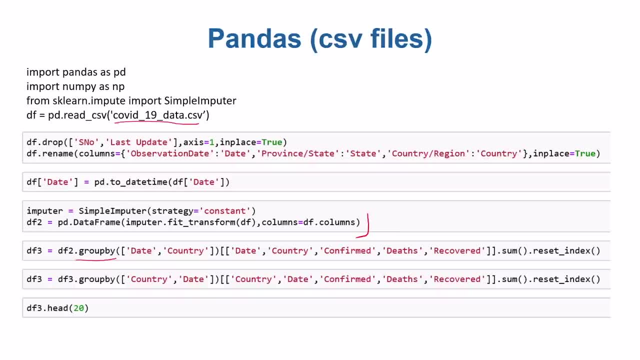 give a very good initial insight into the data, and the design process can become very, very fast if you know something about the data, whether you get that information by visualization or by other statistics or whatever. so in the next video i will be just explaining some very few functions. 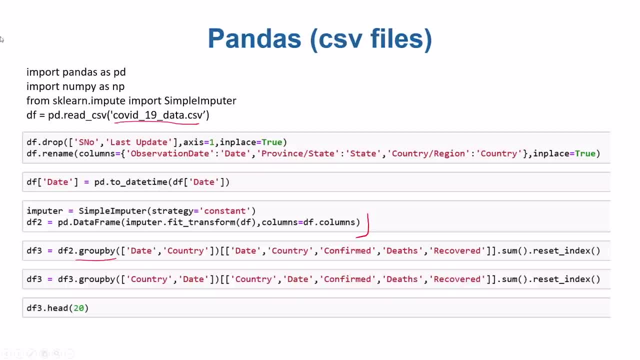 of matplotlib, and then we will be. then we will be exploring the same file and we will be doing something else in the next video. stuff, um, doing some stuff using the plots and matplotlib and doing seeing the trends of death rates, seeing the trends of. i mean we will be playing with this file a bit more, using. 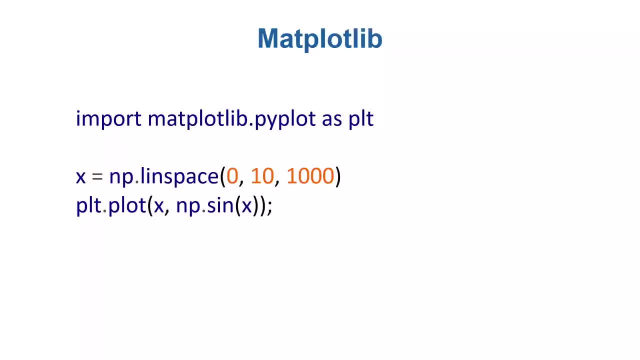 matplotlib as well, so hope to see you in the next video. okay, in this video i'm going to discuss matplotlib, a very powerful package for plotting graphs and scattered plots, line plots and 3d plots and plots on the globe and whatnot. i mean very, very powerful tool. uh, the most important uh module in this matplotlib, or the most. 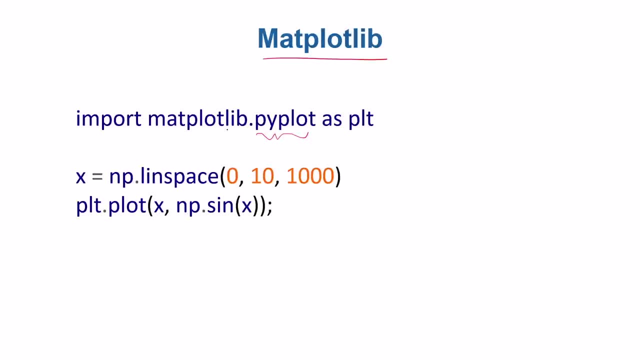 popular module, or the most uh used module, is by plot. so we can import matplotlib dot by plot as plt. another way of writing the same kind of stuff is we can. we can write like: from matplotlib, from matplotlib, import by plot as PLT. so either way is fine. whether we write this as a dot notation or that one, that is fine. 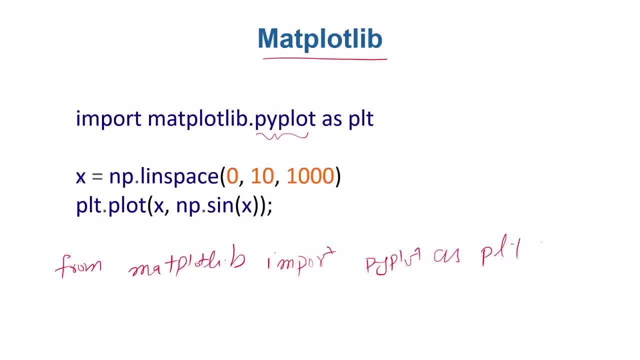 NP is for NumPy, so let's create some points. just just just make our first plot. let's let's make some points starting from zero. let's say all the points starting from zero till 10, and let's create a thousand points in between. one way to do that is to use built-in function or a method in NumPy. 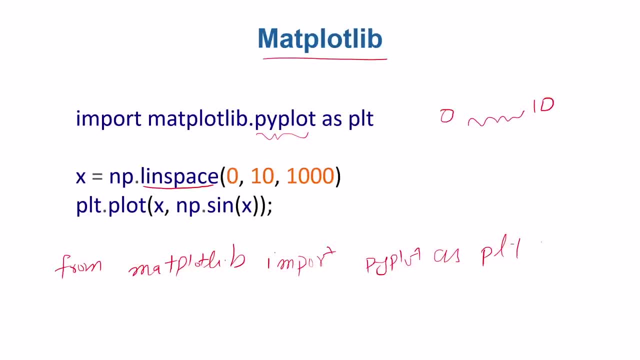 which is linspace, or linearly spaced points starting from zero, ending at 10, and there are a thousand of those points. let's say, this is our x and this is our, let's say, y, which is npsign. this sign function is actually will apply element by element on this NumPy array and then this PLT. 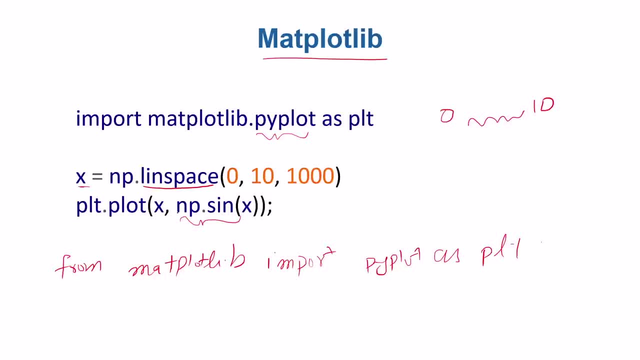 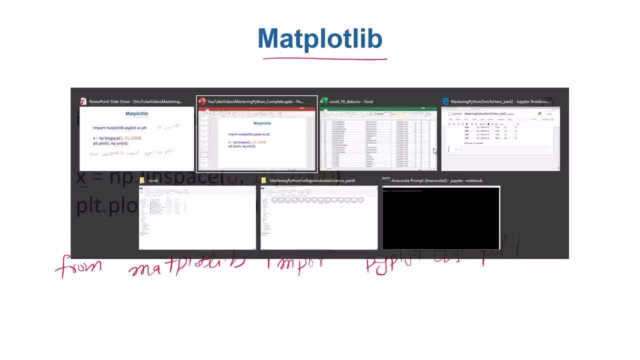 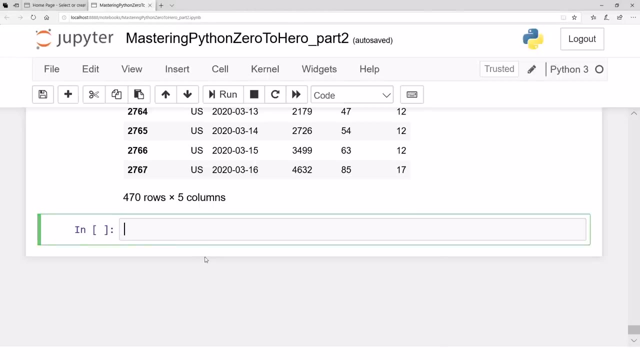 will plot, will actually plot x, comma y, all the points in front of you. so let's go to Jupyter notebook and actually see this matplotl in running form for the very first time. oh, we have seen this matplotlib. when we saw nprandom we, we plotted a histogram, wow. so this is not the first time. we actually have seen this, once, once. 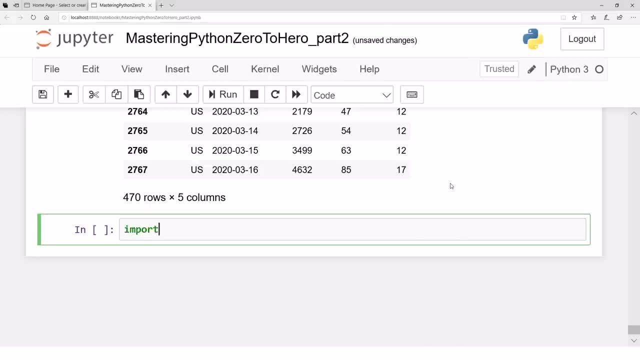 once before. so import matplotlibpyplot as plt. that's your import command. for example, now plt is available, let's say: we want to import this matplotlib. and we want to import this matplotlib. let's say x is nplin space. let's say: start from zero, go to 10 and generate. let's say a thousand. 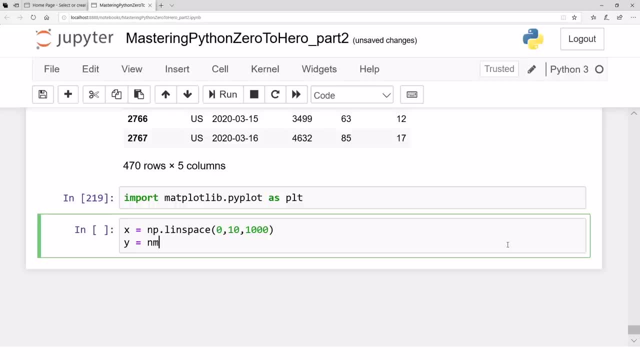 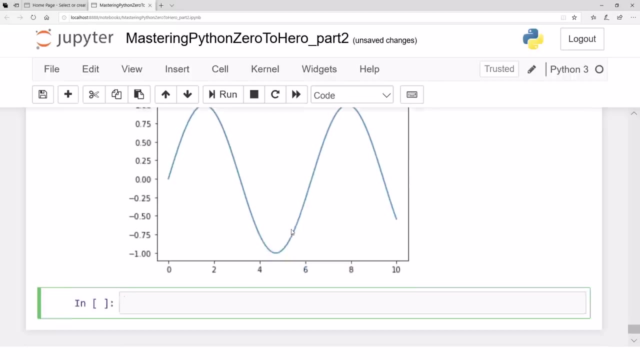 points. let's say that's your x, y might be your npsign x, let's say that's your y. and then what you do is you say, okay, pltplot x, comma, y, point by point, and then you press shift, enter, that's it. oh, this plot is there in front of you. that simple, i mean that's. 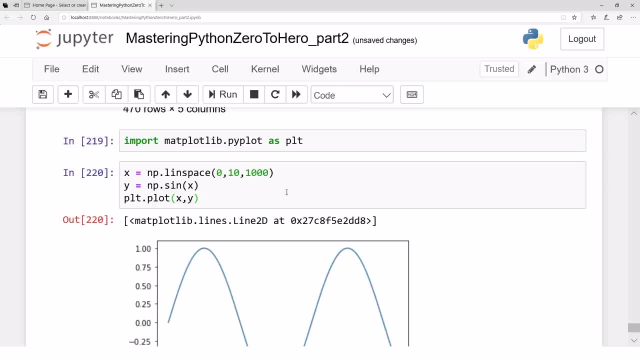 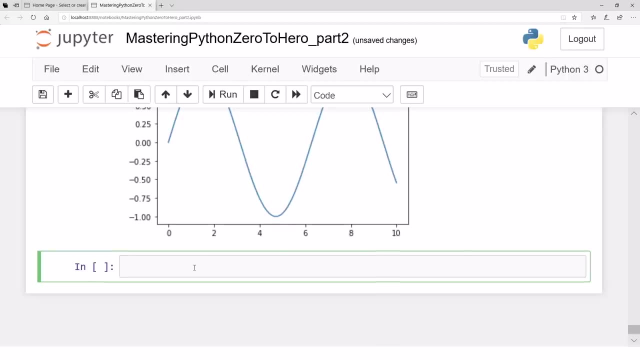 simple. can you imagine this? is that simple, um, yeah, this is that simple, um. so i mean plotting. this is a line plot. for example, if we want a scatter plot, we can say, okay, pltscatter, there is a scatter function, uh, that allows us to uh plot all these in points form rather than rather. 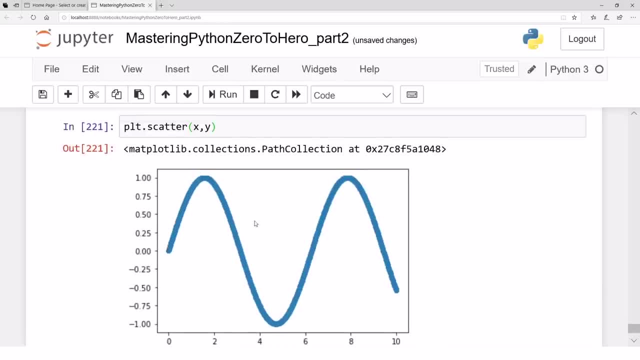 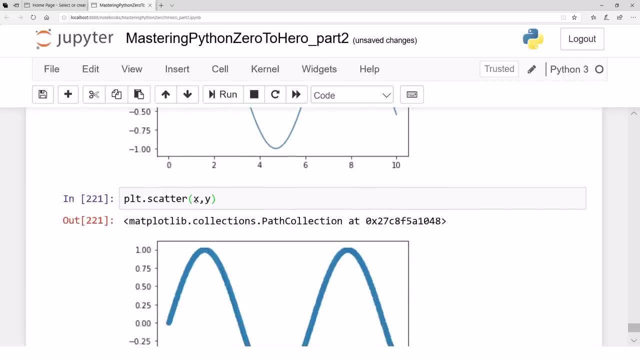 than these line form these are: oh, these are a lot of points. that's why you you're not seeing these scatters. so let me, let me, let me take this: n uh, x as fewer. let's say: let's take x as uh, let's just take a few points. let's say just um, just just 30 points, and let's 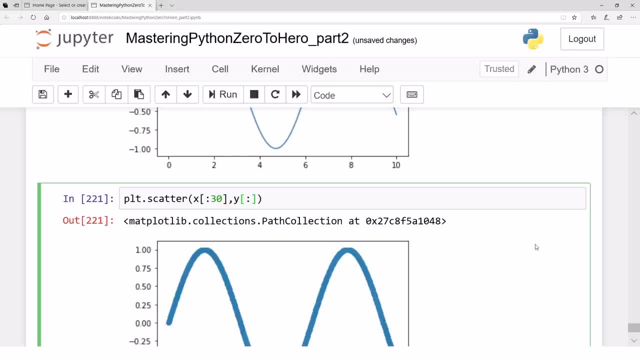 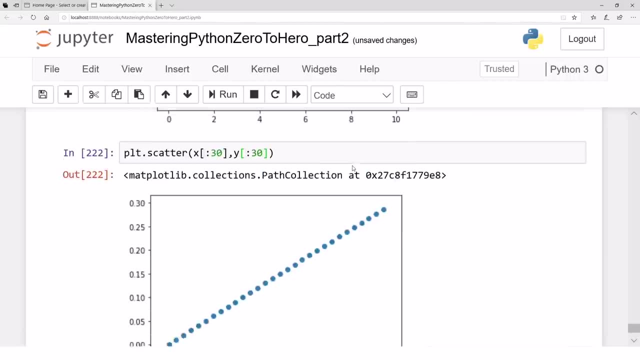 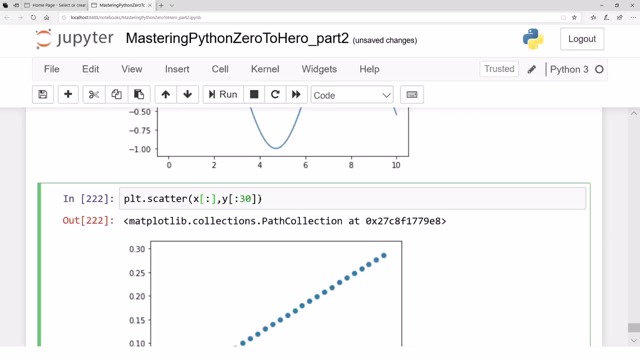 see the corresponding 30 points. see that. remember the indexing of numpy arrays. i'm just using that. so now use the scatter plots and you have this. oh, that's a, that's scatter. maybe we want to use, let's say a: uh, start from, uh, the very beginning, go to the end and pick every, let's say, 10th. 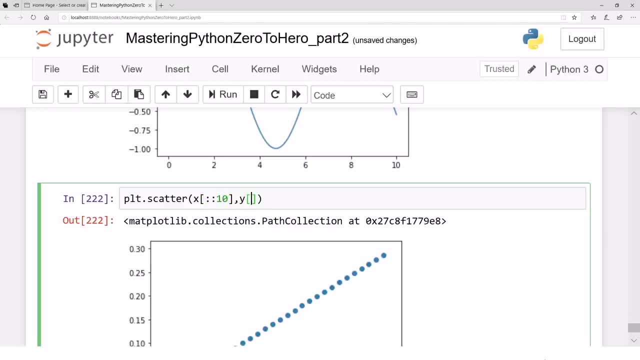 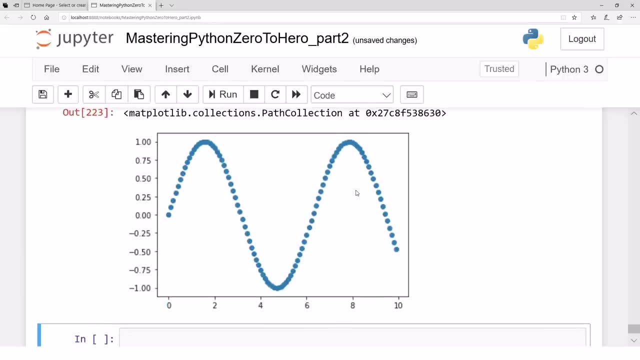 point and do the same with why. just to just to see a plot in a better way, just sample some points. so that's the scattered plot. it is just like. i mean the points and so on. uh, it is not a. it is not a continuous plot like the line plot, it's a scattered plot. 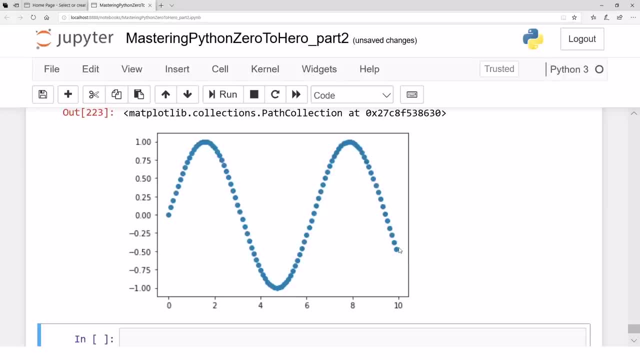 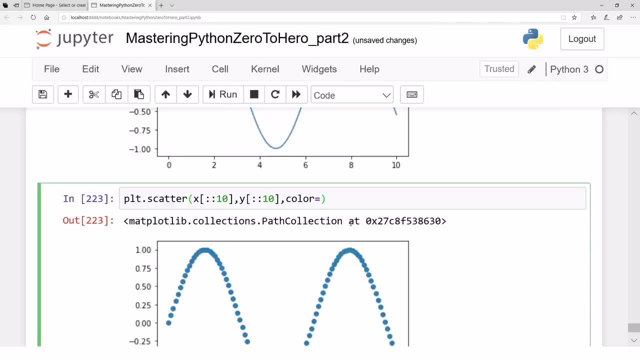 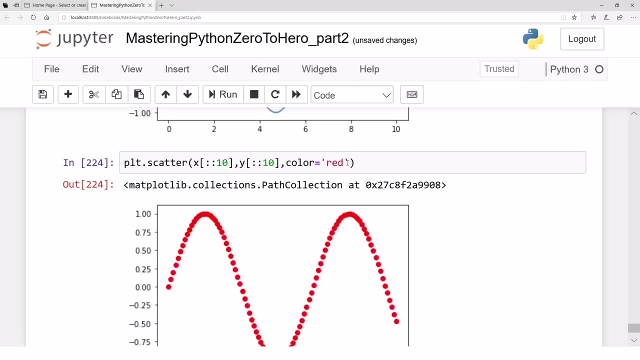 We can annotate the scatterplot, We can change these colors to any color we want. For example, we can have a property. for example, color is equal to, let's say, red and everything will become red. Yeah, so that's red We can have. I mean, we can label it, we can X label it, we can Y label it. 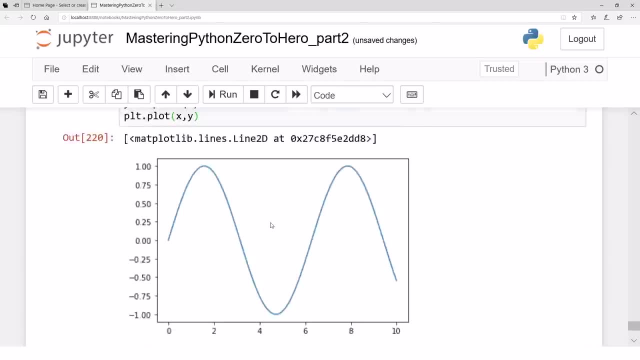 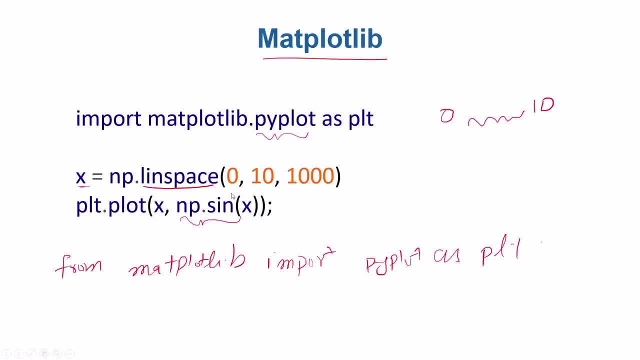 There are a lot of properties, But the main point is plotting. is that simple? Plotting is that quick using matplotlib. So yeah, this matplotlib is really, really powerful. We have just seen a snapshot, just a plot function and a scatter function. 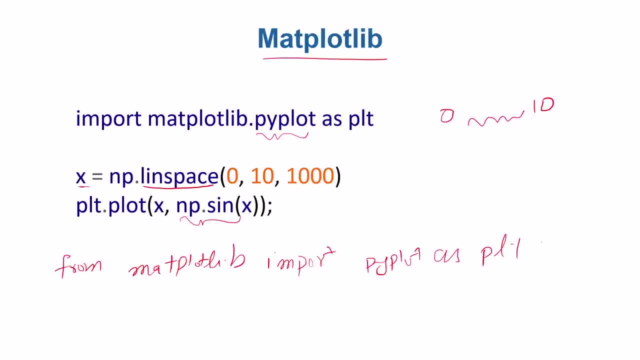 There are a lot of properties to be set, There are a lot of things to be considered And we will see. we will see actually one lengthier code on this COVID-19 file And we will actually analyze the death trends and the confirmed trends. 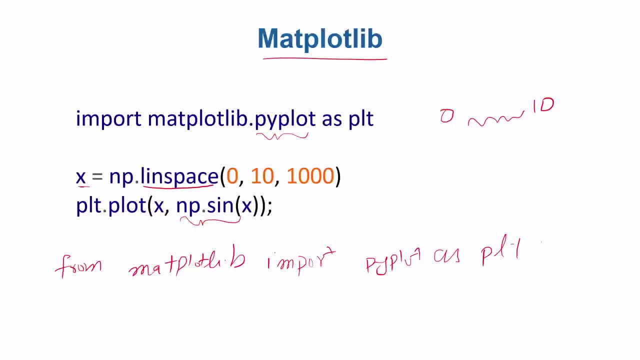 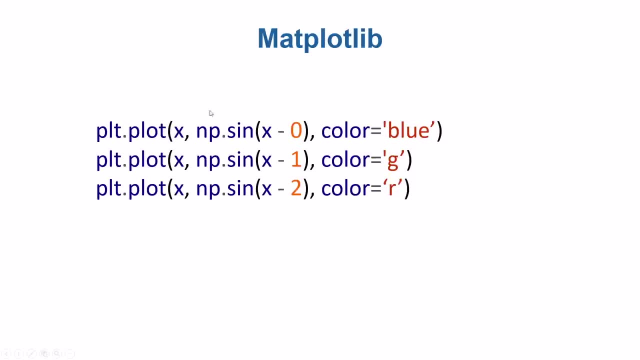 And some trends that, and we will plot them and see the trends really using matplotlib. So, but before that, let me show you that if you call this plot multiple times, for example maybe with different colors, then you will be having a lot of curves on the same plot. for example, 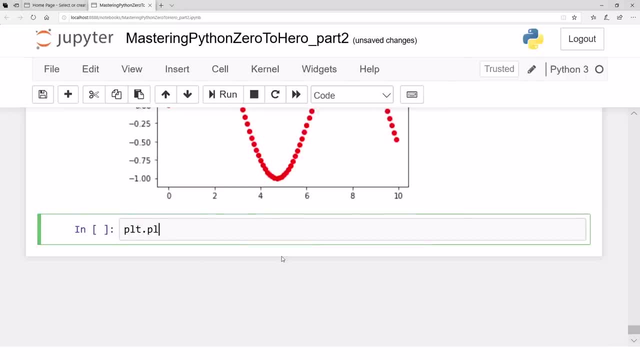 So, for example, let's see pltplot x, y, Let's say With color. let's say color equals to blue. You can write blue the whole, or you can like write just p, That's fine. pltplot x and let's say npcause x. 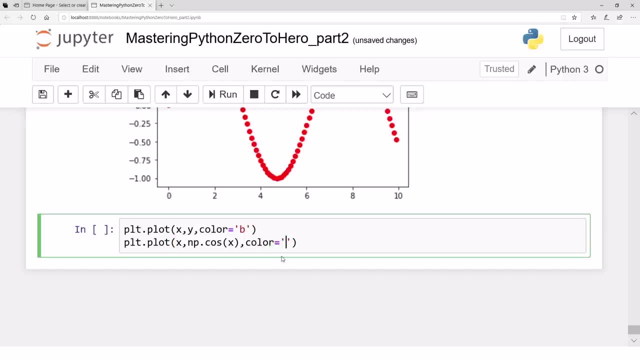 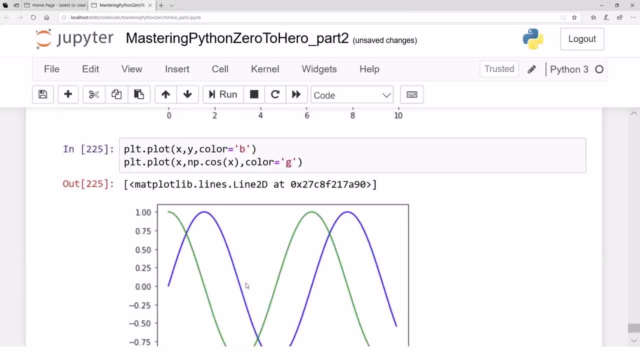 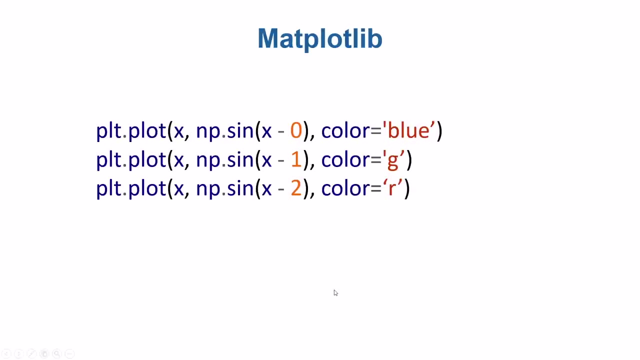 And the color you are interested in. let's say the color is, let's say, green, And that's perfectly okay, And that will give you two plots in the same Figure, sort of, and you can just get to go. well, yeah, so that more you can. for example, you can plot with a green green color and you want the solid line, or you want, for example, cyan color in a dashed line, or you want a dash and dot black line, or or maybe you want a completely dotted line in red color. 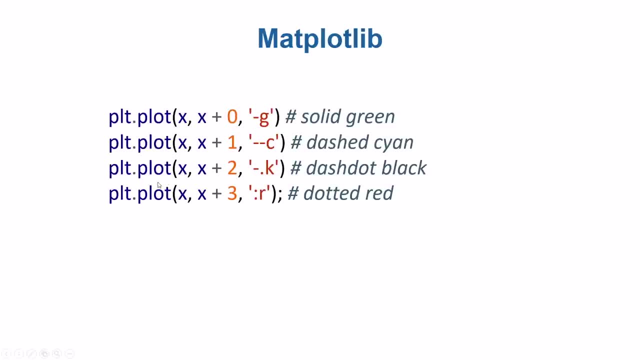 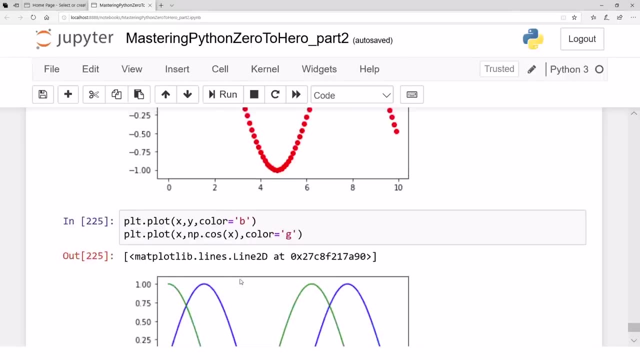 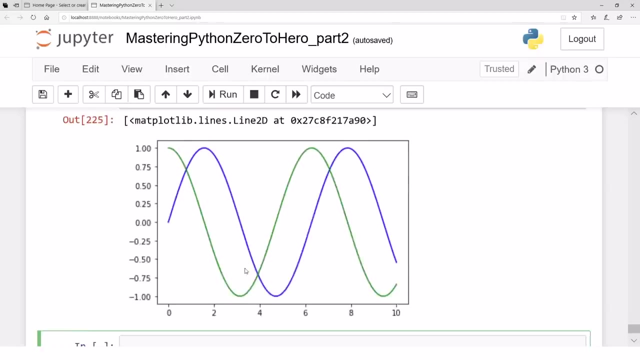 So there are several things that are available in matplotlib. This is just a very few, very simple snapshot and I have given you a very quick start, And actually actually the whole point is using matlab, is that quick? I mean you can, you have your data, you just plug in their data, you just call the plot function and you're good to go for analysis. 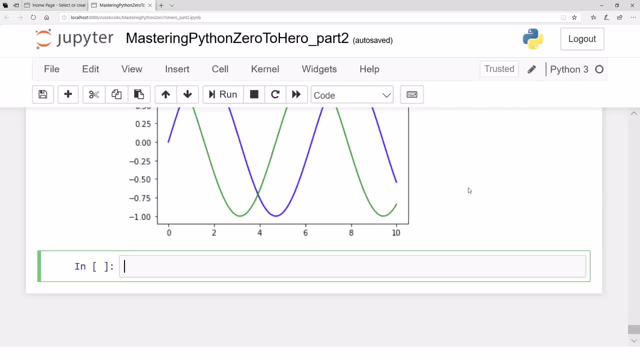 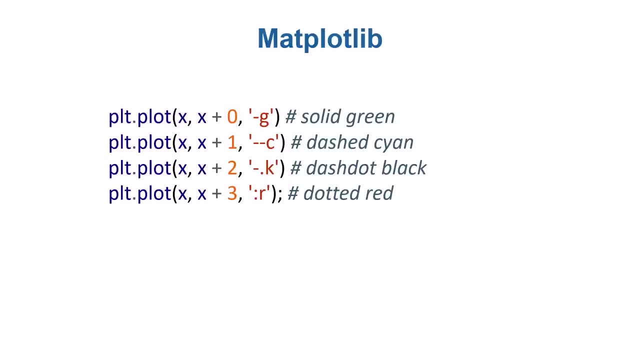 Okay, In the next video we will actually walk through the, we will actually walk through the COVID-19 data set and we'll actually analyze the trends And The death rate trends for each country individually and then we will see the death confirmed and the recovery trend of the overall world till the 16th of March, till the day till the date the data is available. 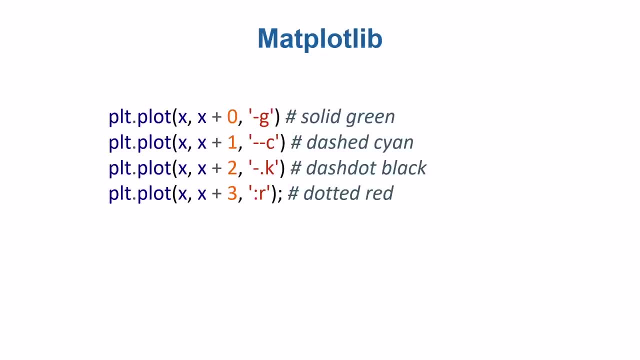 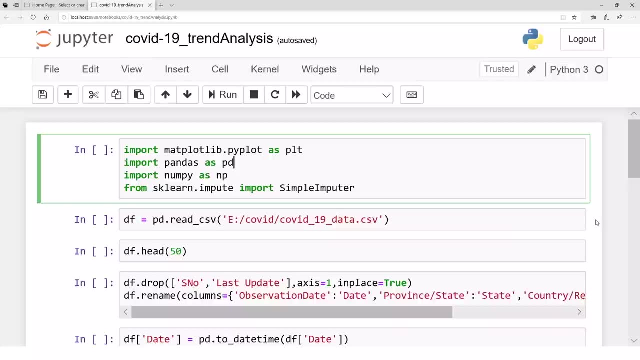 So next video will be actually the. you will see the running form of pandas and matplotlib together. So hope to see you in the next video. Okay, I already have shown you the COVID-19. File and here I have a notebook on that- that uses matplotlib and pandas to to find out the deaths, confirmations and recovery trends using using different plots. 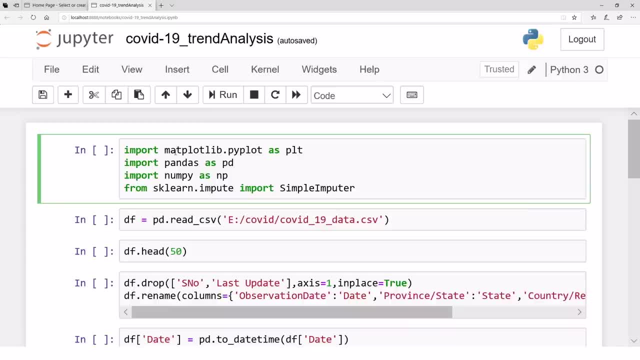 So let me import all the packages that I need. I need a plot pi plot function from matplotlib, I need pandas somewhere, I need numpy, And I'm using a simple computer here for missing values. So let's run this, let's run this command and, yes, everything is imported. 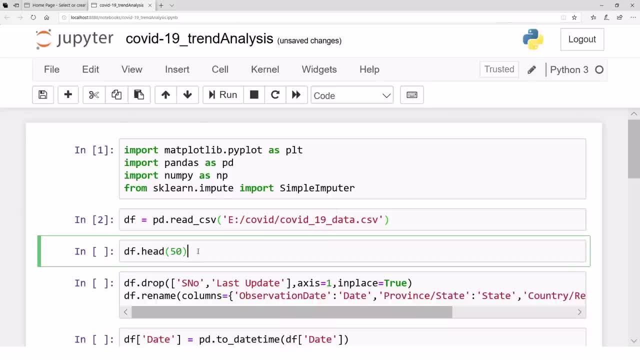 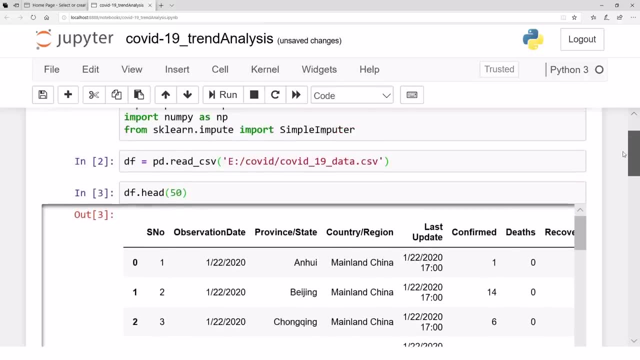 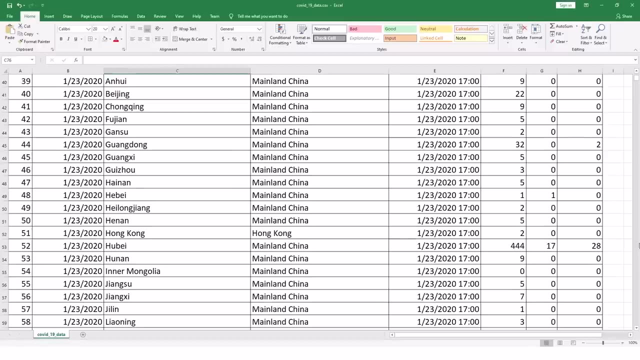 Now let's load the data that I've shown you earlier. The data is available now- and let's run this thing. that is the first 50 records. Yeah, Remember that. Um, yeah, so that's the data that is available. If, if you just want uh another view, uh, another view of the data, that's the data file, which is COVID-19 file, and it has observation date: province. 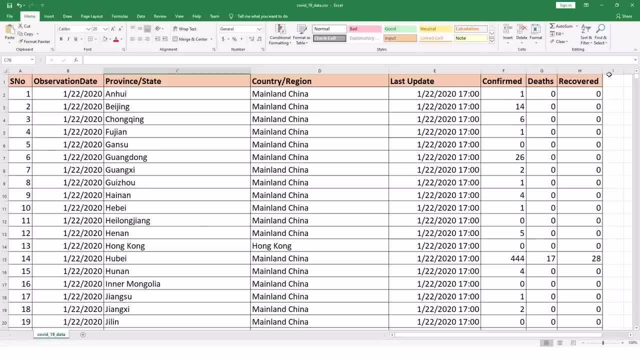 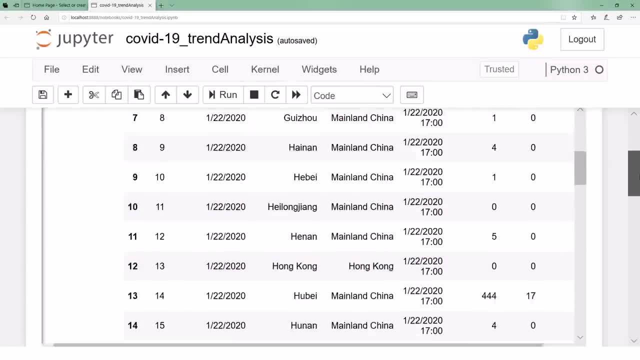 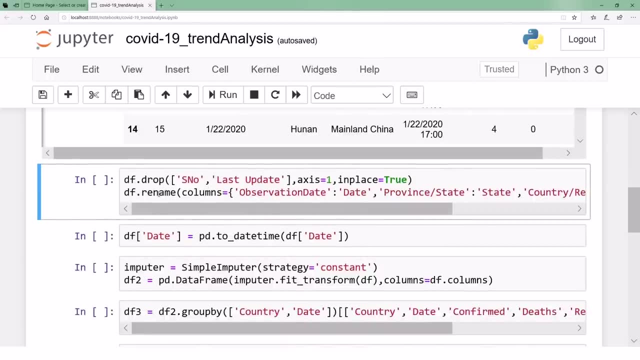 Country: last update, confirmed to date, death to date and recovered to date for each country and for each province individually. Okay, great, So that's what, uh, we have now. what we can do is now let's drop the serial numbers and last update- uh, using in place that we- and rename the columns. that we did already in a previous video as well. 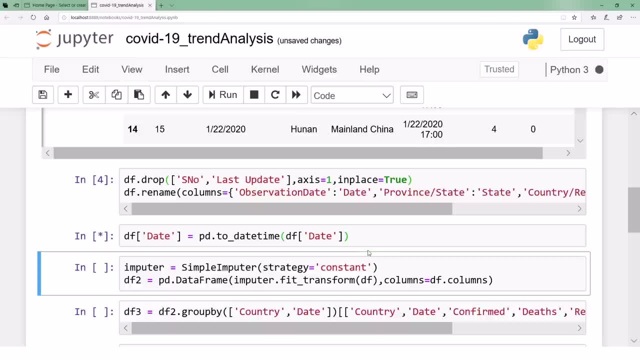 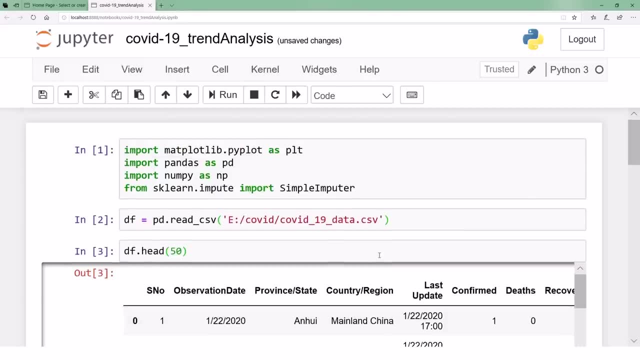 Uh, let's convert the date into the pandas built-in date uh frame. Okay, Let's uh use the Uh scikit-learn imputer, uh SK learn imputer. uh, using the constant strategy. 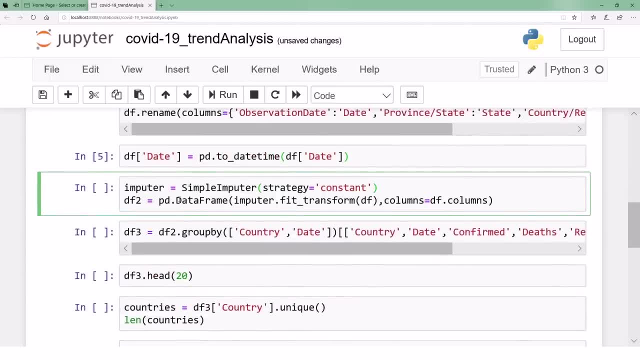 There are a lot of strategies there. Let's use the constant strategy and this PD dot data frame. uh impute dot fit transform. that will help. uh imputing all the missing values with a constant strategy imputer. So that's there. 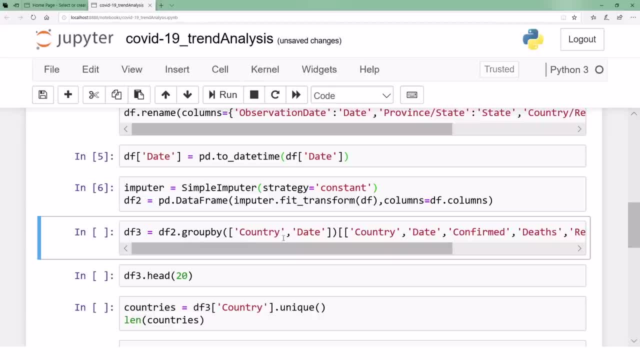 Okay, Next let's apply this group by command and group all of all the records using country, for each country And for all the days. Let's sum all the records that some, all the values of recovered stats and confirms um using this, but now let's first country, and then all its state, then the second country, then all its dates and so on. 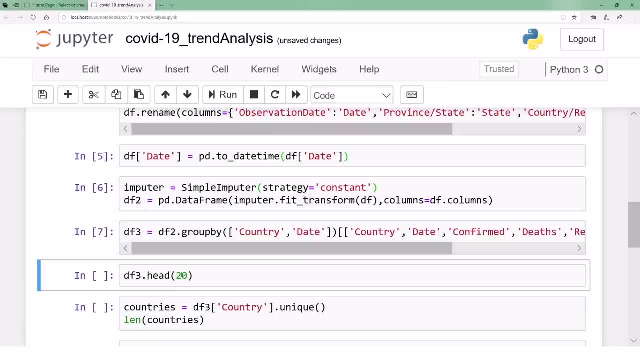 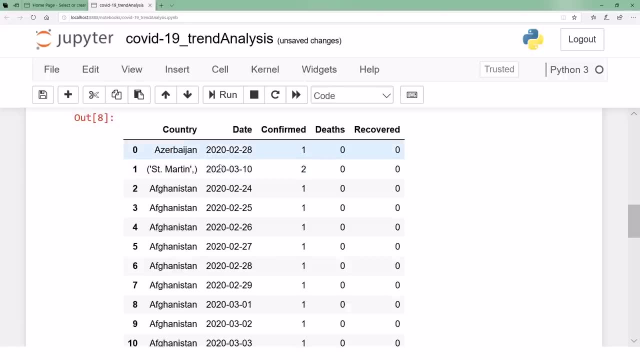 Uh, we have seen that in one of our previous videos. just running that again just for a double check. So that's what the data state is. So country one, all its states, country to wallet states, So this country has a lot of dates, then another country, and so on. 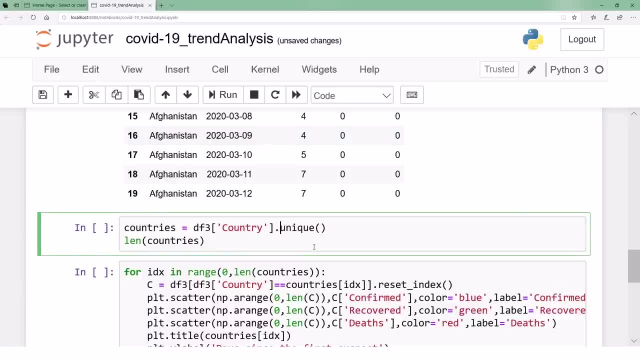 Next, let's see how many countries are there. uh, in total, how many unique countries are there? So what I? what I do is I find the column. I actually picked the column with country and call it unique function on that. 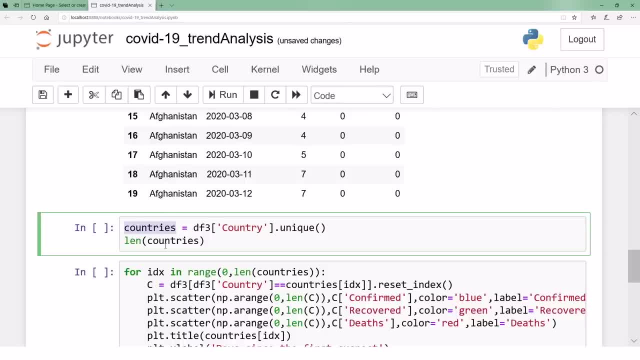 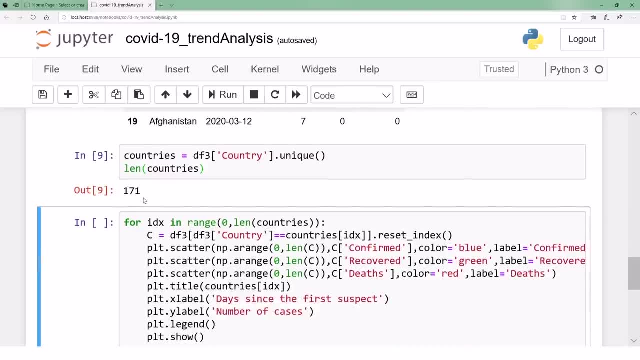 And that gives me all the countries without repetition, And I just compute the length, length of countries. Tell me how many unique countries are there. in this uh data file There are 171 countries. So, um now, my goal is for each country. 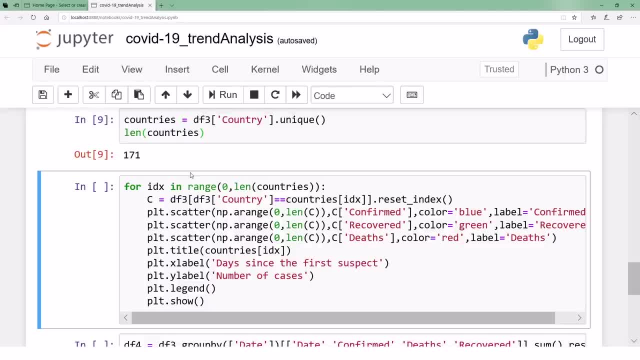 I want. I want to see what is the trend of uh with respect to the date, as the data is moving from the first day till 16th of March. what is the trend of uh death, uh patients, what is the trend of recovered patients and what is the trend of confirmed patients as the date moves on? 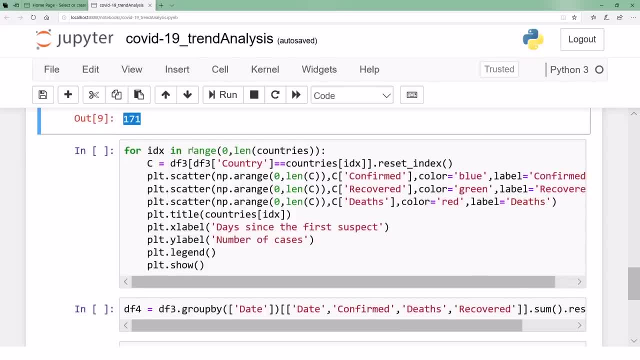 So, because we have 171 countries, so let's loop over each country again, again and again, let's loop over what we do is for IDX In the range of: uh, this, that's a loop, You remember that. 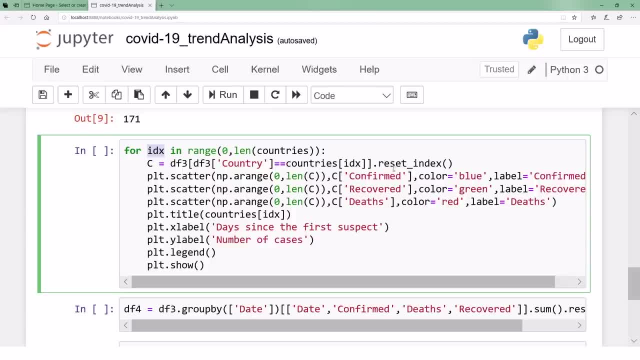 And what I do is: let's find out the indices where the country is like this, Let's find out the index, all the indices where the country is like that. Then what I do? I make a scattered plot that uh, with starting from this and that I just pick the confirmed cases and all the confirmed cases for this one country. 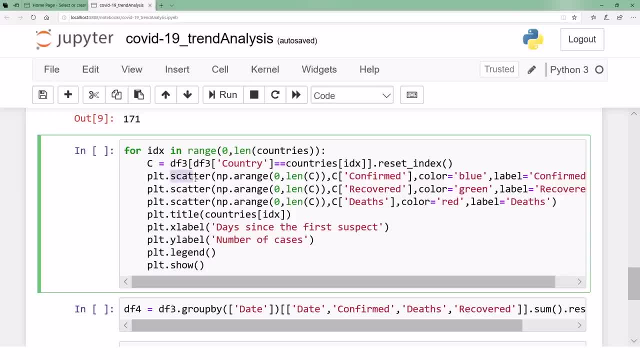 I just picked those and and I I do that using this scattered plot. Then I Use another scattered plot just to get all the recovered cases. Then I do another scattered plot to get all the death um uh cases, And then the title of the uh, title of my um figure becomes the country name. 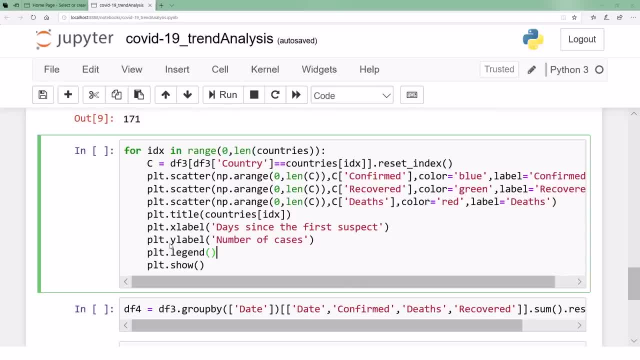 The X labels the date. uh days, since the first suspect, the Y label is the total number of cases, The legend command actually will be there. That will show what eat. That is it So these kind of labels that are rewriting here, they will appear in the figure. 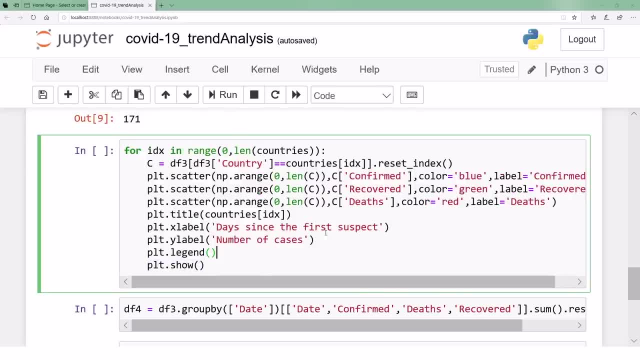 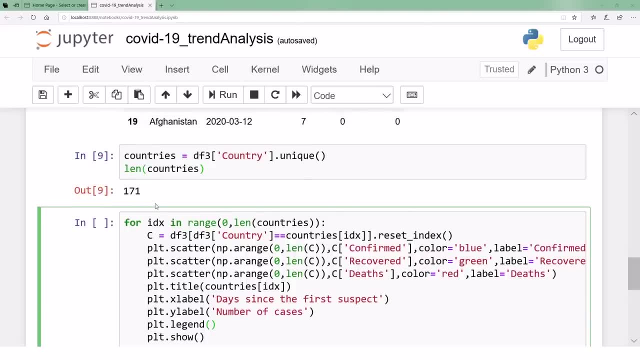 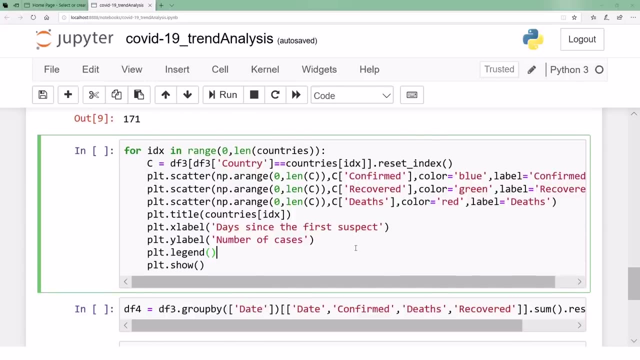 Then we force them to show that in each iteration and show the show the far. So this will show, uh, the trends of confirms, recovers and deaths for all uh one 71 countries, one by one. So if we run this command we'll be having one 71 plots in front of us. 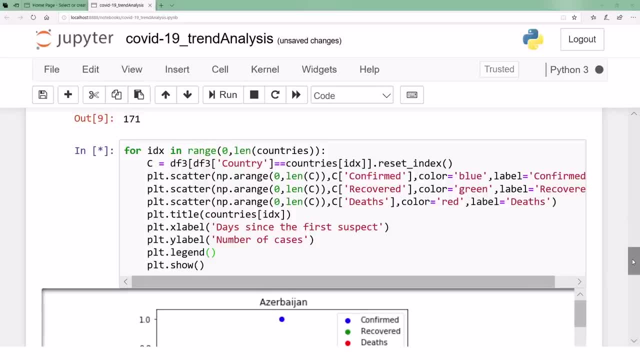 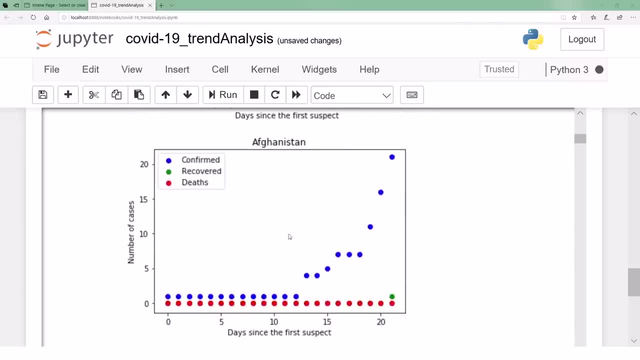 Let's see all of those one by one. So, um, yeah, so this is for the country. It has Just one such thing. This is for that. This is for Afghanistan. as days moves on, the confirmed cases that are written blue: 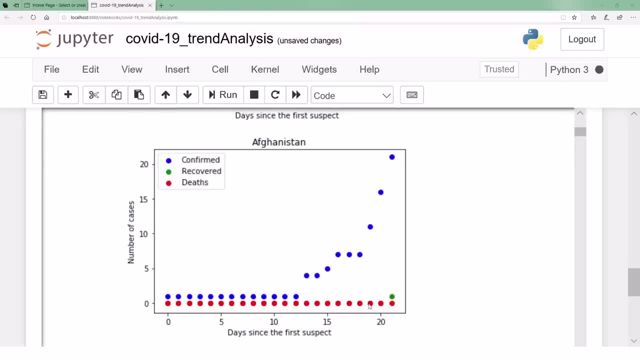 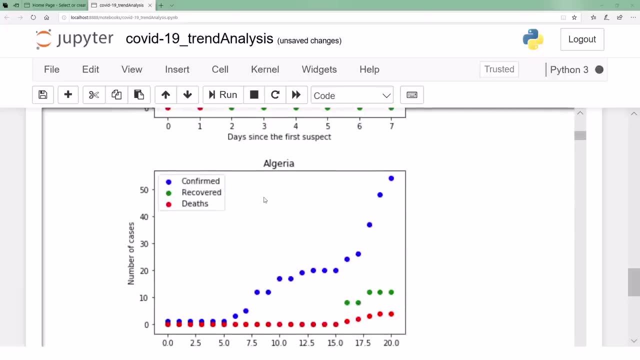 They are moving up. These are the number of cases, These are the number of days since the first day, and the green is the number of recovered cases. for Albania, That's the trend. for Algeria, That's the trend. I mean. these are each and everything is a separate. that is for Argentina. 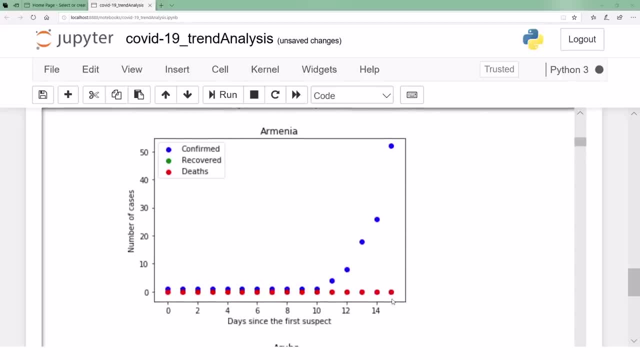 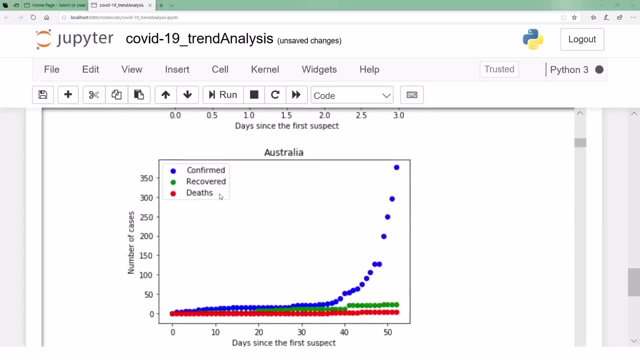 That is for America. This is for America till the 16th March. by the way. Uh, today, um, the news says that America is really in a dangerous position. Anyways, that's for Australia till till the date we have the data. that is for Austria. 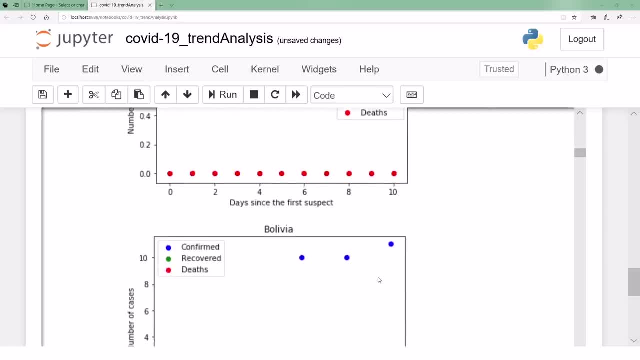 Um, yeah, so these are all the trends for all the countries. you see, I mean the matplotlib. how powerful that is. Um, although I walked through this code very quickly, but um you, you can see this video again and again and check how that happens. 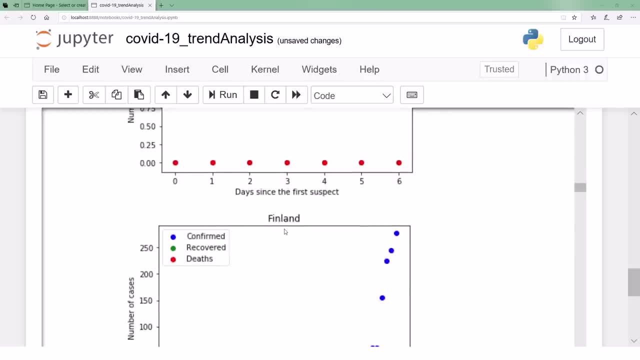 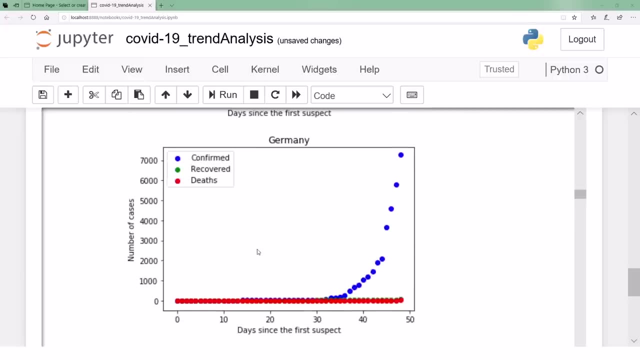 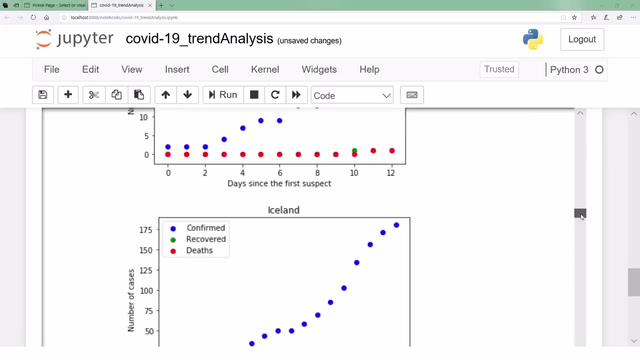 Uh, yeah, So So that's what. uh, this is for Finland. Oh, Finland is also in trouble. So, France, Okay, So that is for Germany, And, yeah, so all the countries that are available in data set. they have these kinds of plots. 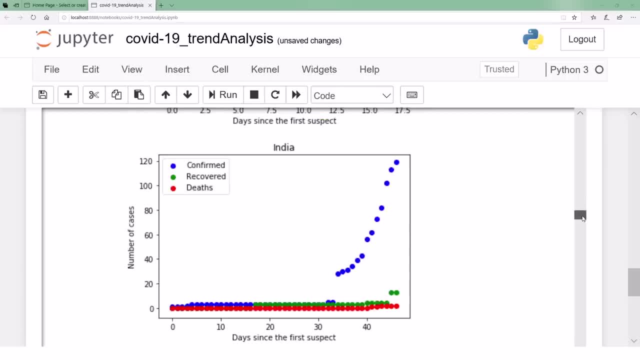 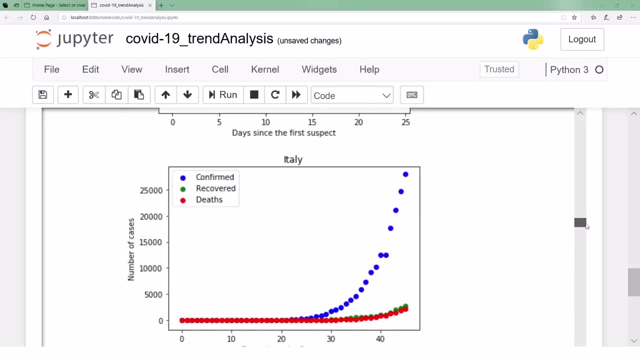 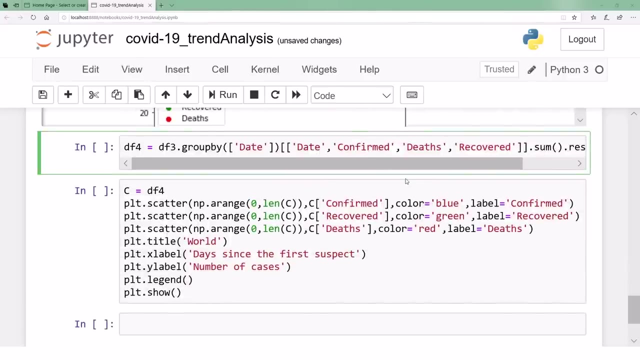 Uh, this is for Hong Kong and this is for India and this is for Italy. So Italy is uh, yeah, so that's it. So that is for, uh, each country individually. What if we want, um, the overall trend, or the overall confirm and the deaths and the recover trend for all the world together? 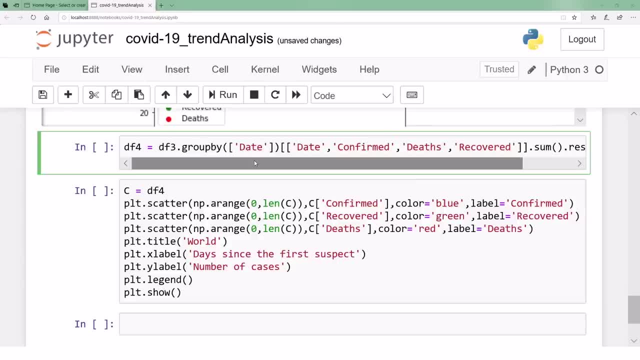 So what I do is I pick, I group all the data with date, So I pick the first date and add all the records, then the second date for all the records, for all the countries, and so on, and then I plot the trend using the scattered plot: again confirmed, recovered, and that's for all over the world and seasonally. 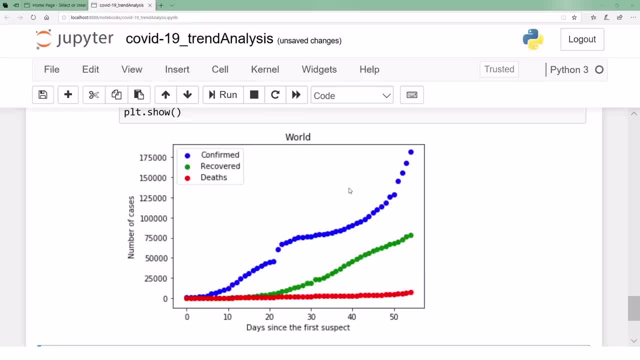 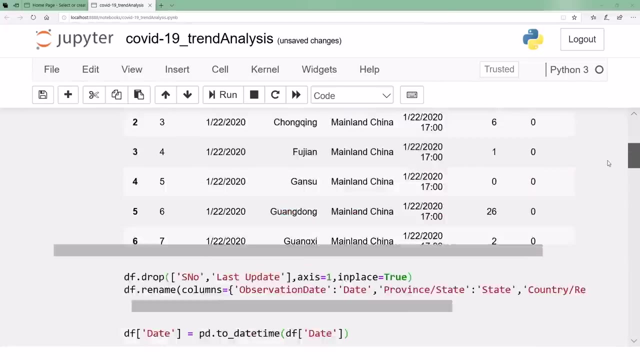 See the trend where the world is moving. So that's the trend of the world. um, as the days are going on, These are the death trend, That's a recovery trend And that's a confirmation trend that is moving on. Um, although I I walked through, or this notebook. the notebook will be available to you. 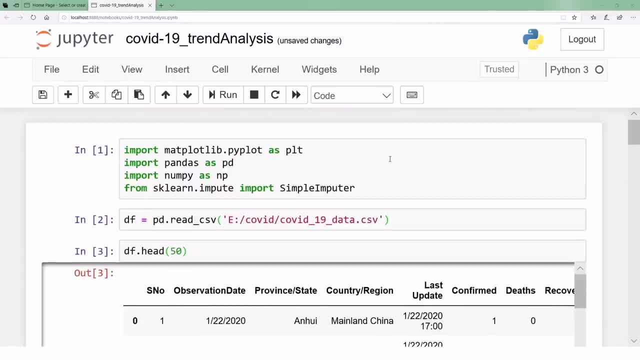 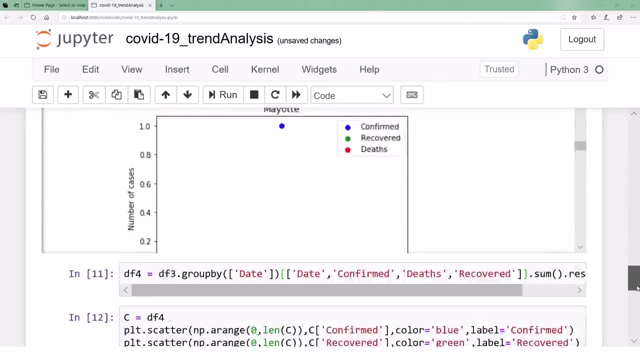 Um, I've walked over this notebook very quickly, but um, the goal was really to show you the the. I mean, that was a file. Um may not be that informative if you see that in Excel, but now it makes much more sense. when you see these plots, you know what is happening and you have an insight in the data. 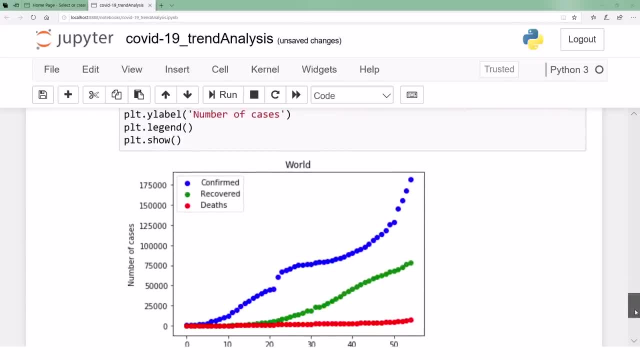 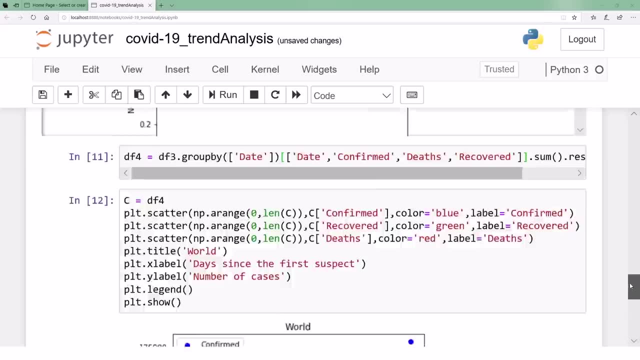 And later on, we may, we may want to predict, we may want to make predictions and the next date, what is going to happen? We, we, we may want to predict using this plot or using some machine learning library like scikit-learn or or TensorFlow or something like that. 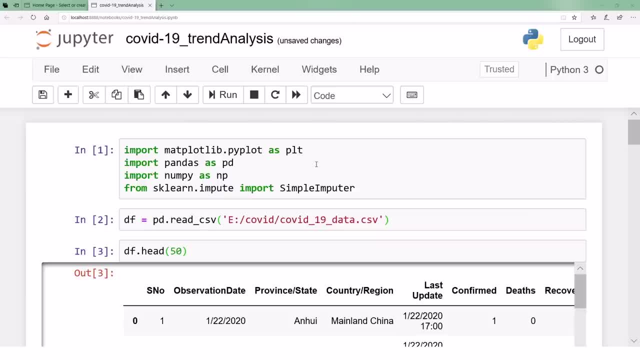 Okay, So, um, that's it. Um I I can talk much more about Pandas, NumPy, uh, Matplotlib, Uh, there are so many other data science packages, very important packages. One of those is sklearn. 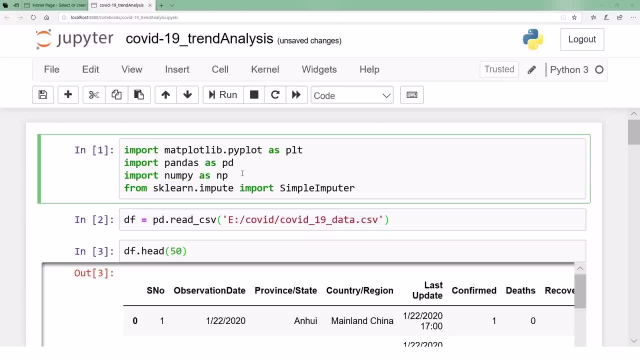 Uh, we, we can. that is for machine learning, basic machine learning. Then there are other packages like TensorFlow for deep learning, PyTorch for deep learning. There are a lot of packages with a lot of specialities in data science and stuff. 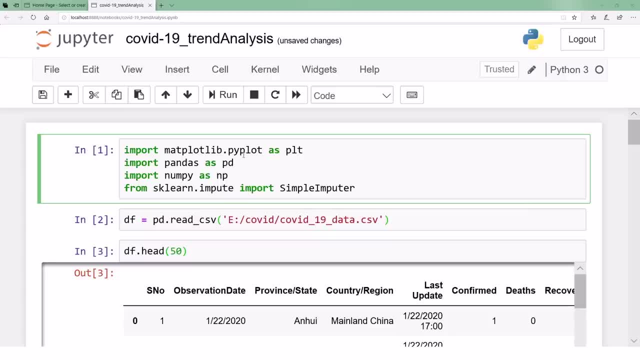 I just discussed a few of those, the most important of those, to to manipulate The data, to make predictions, to make classification or regressions, uh for uh one. one way is to go to sklearn or scikit-learn. 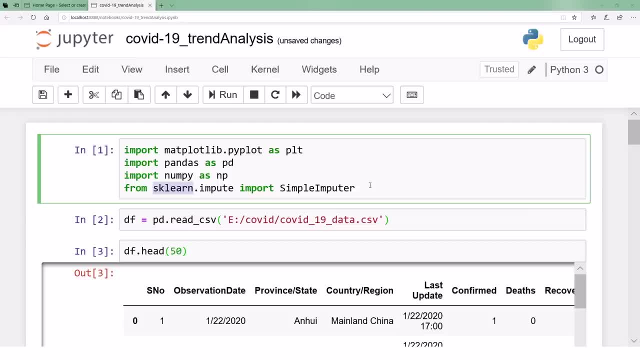 And if the data is huge and you have a lot, of, lot amount of data and you have good expertise over deep learning, then you should go to either TensorFlow or PyTorch. These are the Python packages that are available for predictions, classification, regression and a lot more. but either way, whether you are going to use scikit-learn, whether you're going to use um, 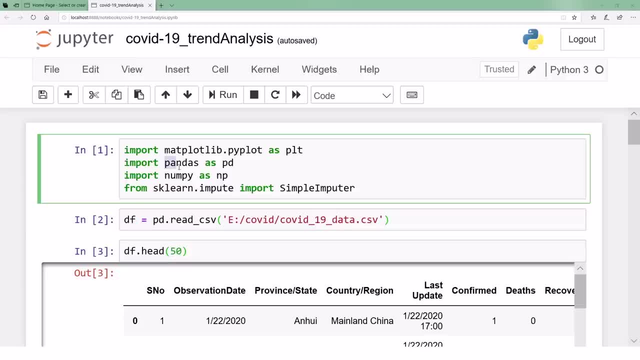 TensorFlow or PyTorch. uh, either way, you have to use pandas, numpy and sometimes matplotlib to pre-process the data and to make the data ready for for these kinds of libraries to to perform predictions, Um, either either in the form of classification or in the form of regression. 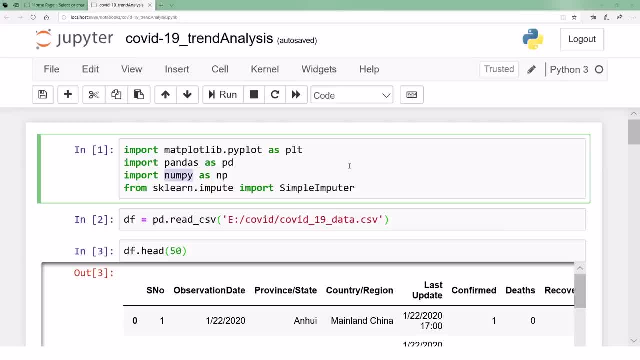 So, um, so, so this whole course was about for, for beginners, um, who want to, who want to learn Python. Um, specifically, uh, I, I discussed a lot about, uh, the, a lot about Python in general, then, uh, then then I spent some time- uh, not a lot amount of time sometimes- on exploring the, the data science packages as well. 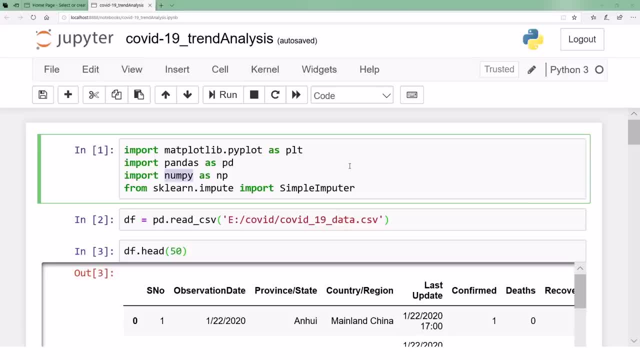 Um, but I mean there is no end. We can explore more. We can talk about, uh, the packages, more We can talk about other features of Python, more, a lot of uh. I mean input formatting, output formatting. 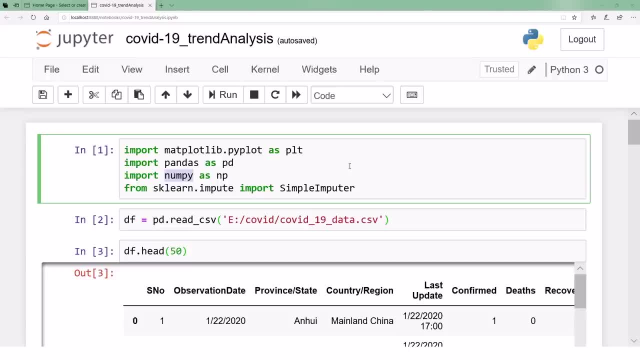 Modules, packages, uh, standard template library, um, um, file handling, internet access database, uh. I mean, this is a whole universe. I have discussed a few things for beginners, uh, but but these few things were very carefully selected for data scientists. 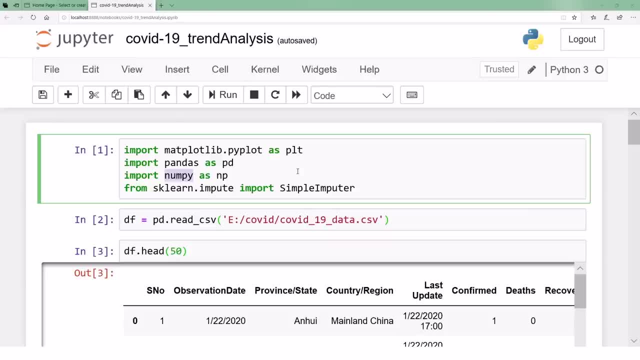 Um, the if. if you have this course available to you, as you have gone through all the course, you now have a very, very good understanding And now you can. you can move towards further advanced uh courses, towards data science, and you will be ready to implement the concepts in Python using using the packages I have discussed so far. 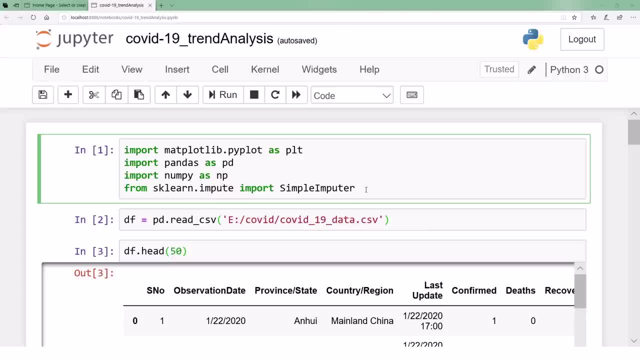 So um I thank you all and good luck.